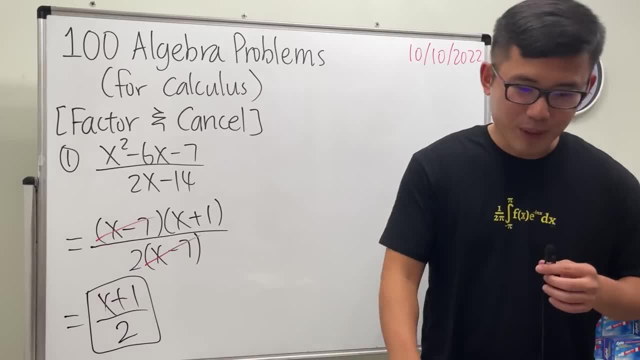 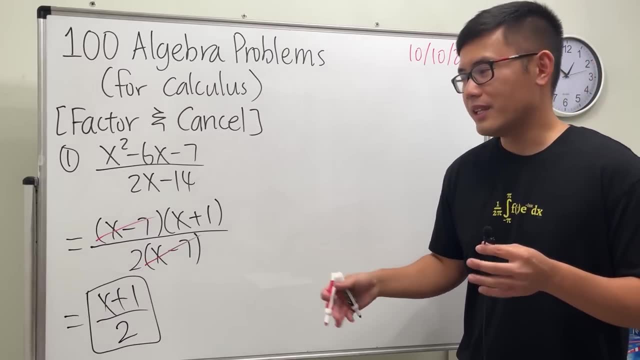 over 2, and then we are done. Yep, the first question. nice and easy, huh? Oh, by the way, this right here: sometimes, if we cannot factor, maybe we'll have to do long division, And again this is just like. 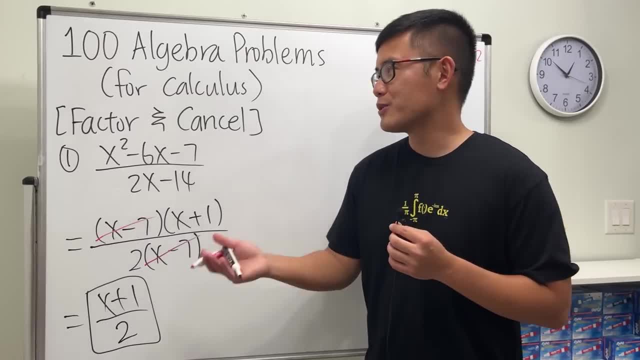 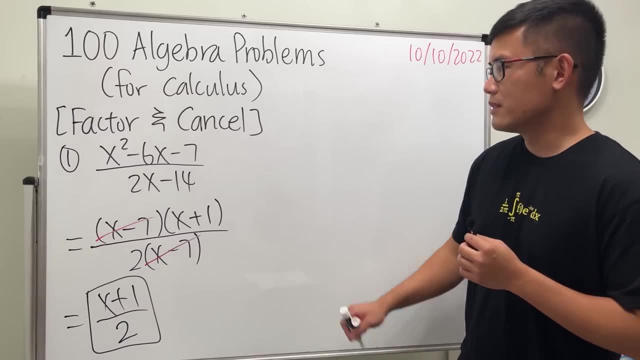 an overall review like an ultimate study guide, algebra review before you are taking calculus or before you are taking calculus all that stuff. So hopefully you guys will find all these things helpful. Either you are about to take calculus or you're in calculus. 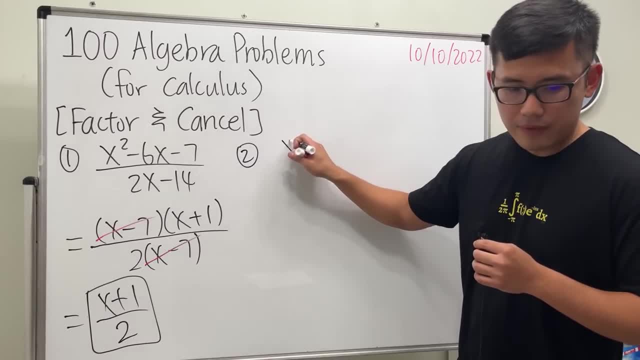 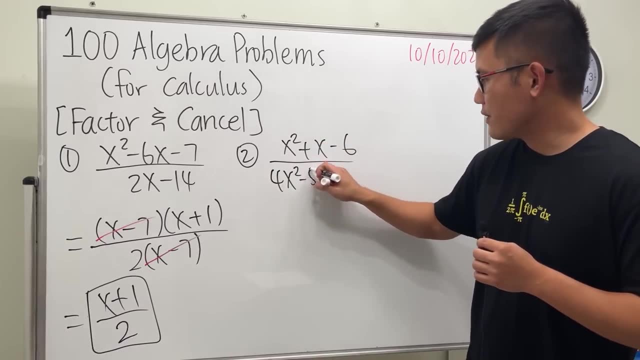 and you just want more review. Anyway, number two: we have x squared minus 6x minus 7 over 4x squared, plus x minus 6 over 4x squared minus 5x minus 6.. All right on the top, this. 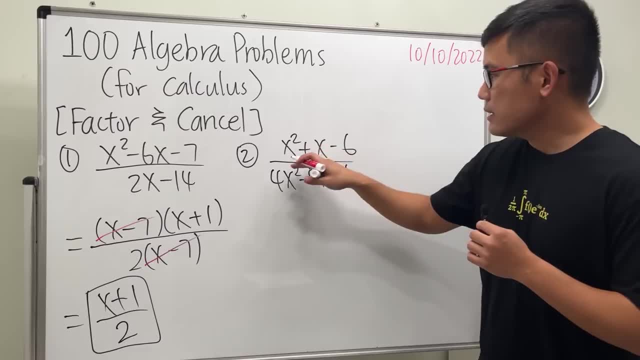 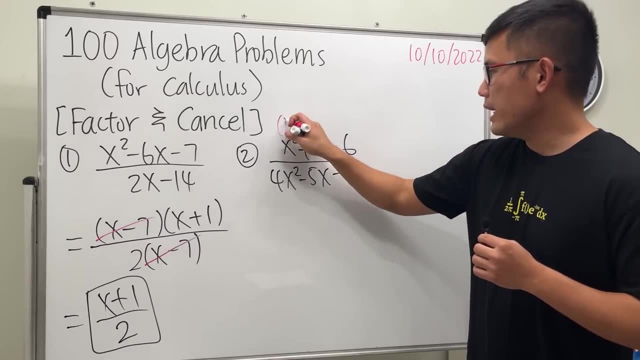 is not factor to factor and it makes you get this little thing. Sometimes, when we want to factor things out, let's just put the result above it. It's easier that way. So if we do that well, we get x, and x One times 4 gives us negative 6.. Together they add up to be: 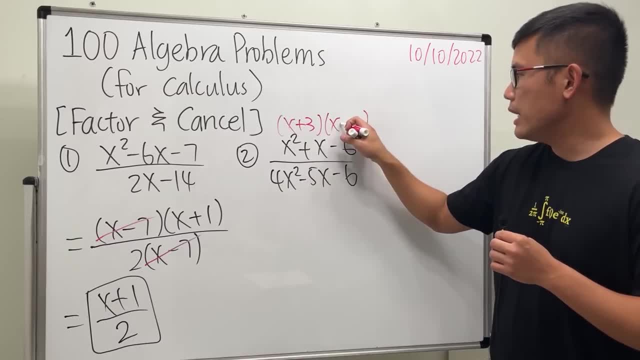 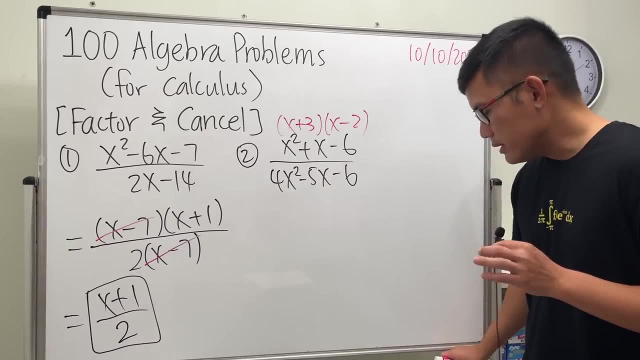 positive 1.. Well, the combination will be plus 3 and minus 2.. And now to figure out the equation, you can just add up to the negative 6, and then you can find x squared minus 7 over 4x squared, plus 6 over 4x squared, minus 7 over 4x squared, minus 7 over 4x squared. 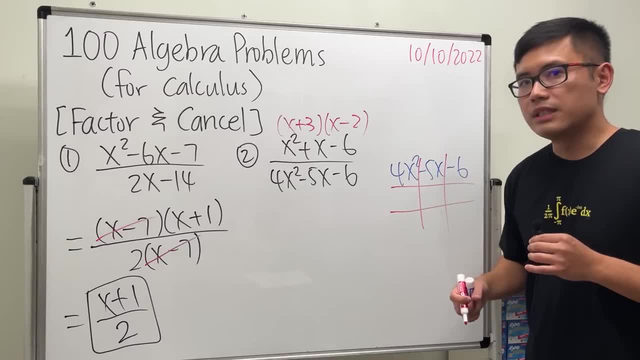 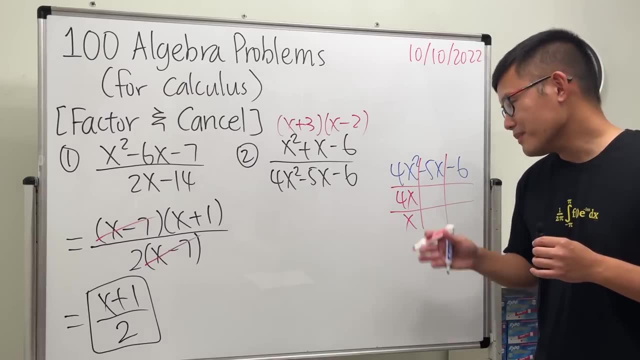 minus 7 over 4x squared. Now let's go back to the bottom. This is not so nice because we have a 4 in front of the x squared. but don't worry, I will show you guys. with the tic-tac-toe method on the side, 4x squared minus 5x minus 6, tic-tac-toe in action. What 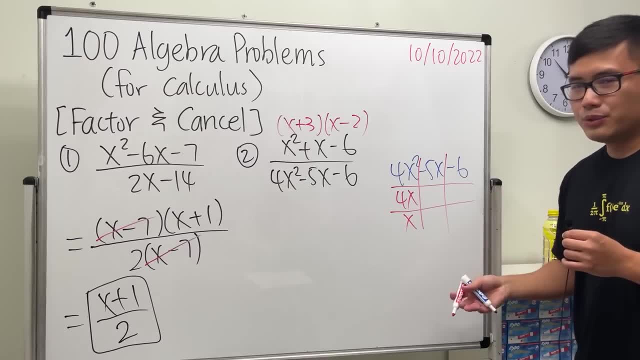 times 4 give us 4x squared. Yes, we can use 2x and 2x, but let me tell you, let's try 4x and x. All right, Why This is going to work. Let me show you We are going to break. 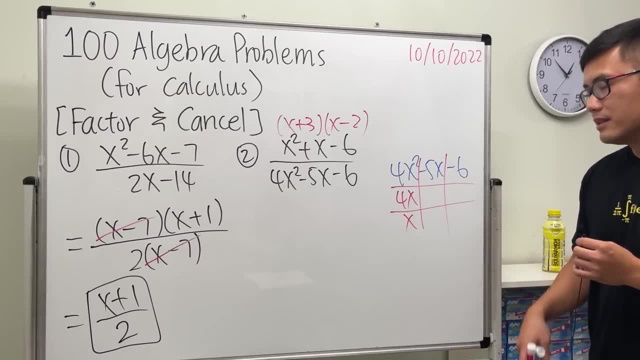 or negative 6,, 1, or maybe more right. The correct combination is that we are going to put, let's say, negative 2 here and 3 right here. Let's see if it works. Well, it does work, because this times this 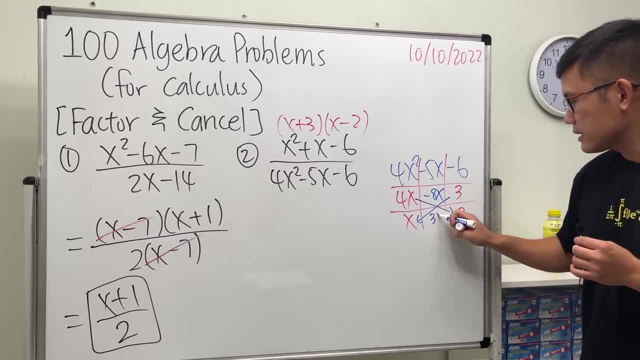 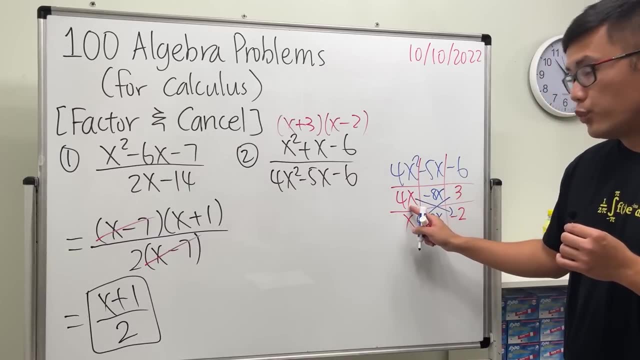 is negative 8x, and this times that is 3x Together, we do end up with the negative 5x. So that means this right here can be factored here really across. okay, So 4x plus 3, and then 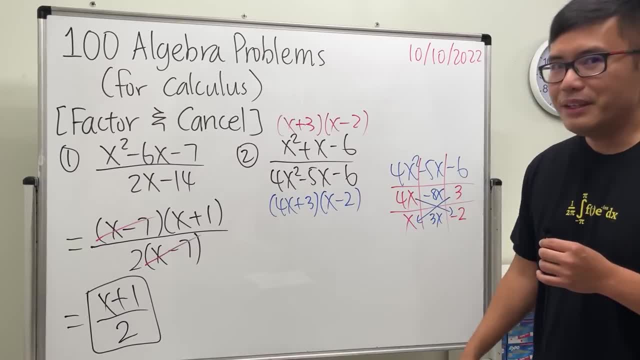 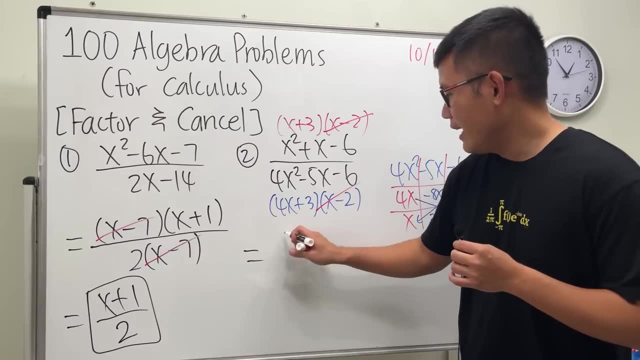 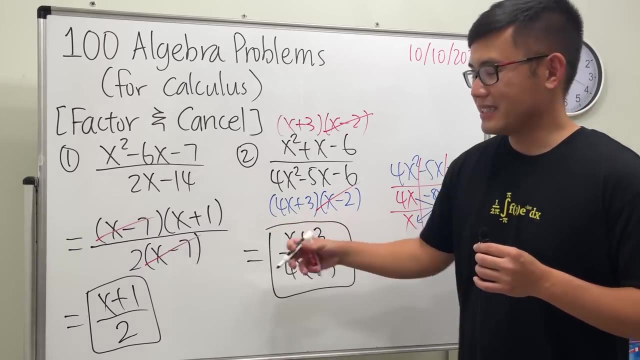 x minus 2.. And you see it, This and that cancel out very nicely, of course, And we will just get x plus 3 over 4x plus 3. And, of course, do not cancel out the 3.. Just leave it like this, alright. So that will be for the first. 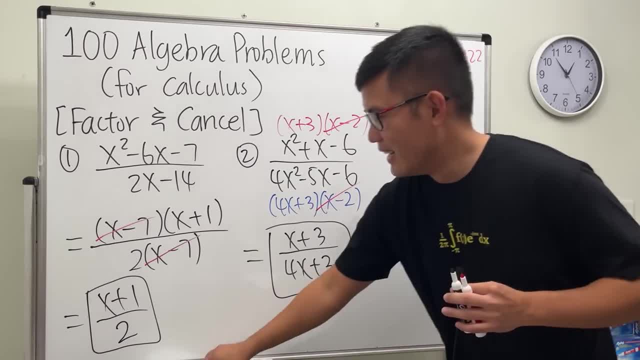 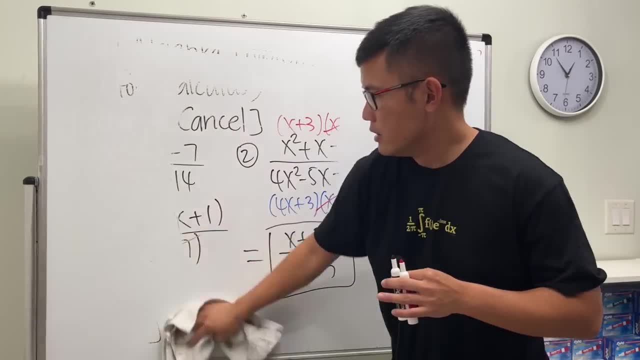 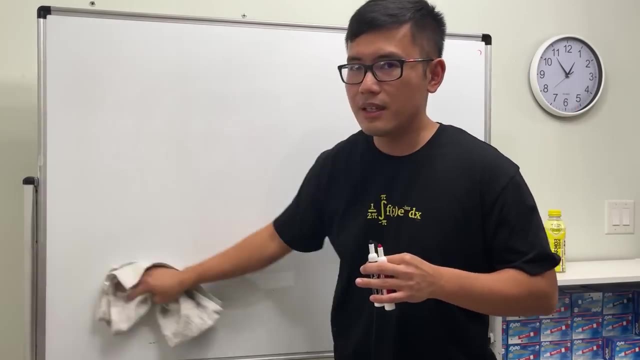 two. Alright, so you have a lot of algebra problems, Okay. So again, all these are just pretty much algebra drills that you should know, so that's why we can go a little bit faster than usual. But again, if you need any help with any specific 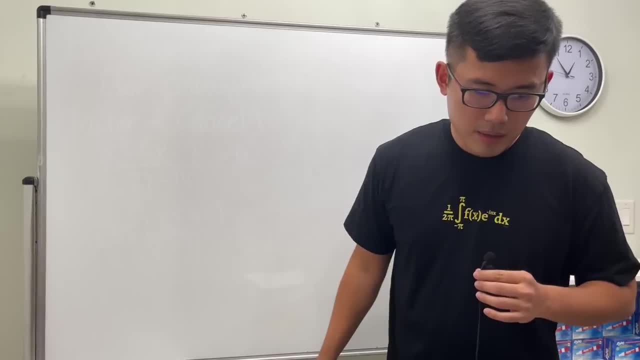 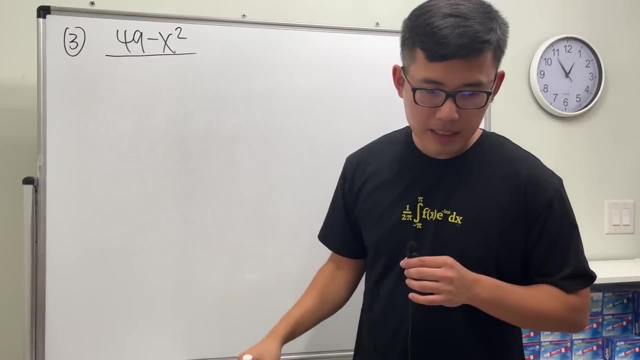 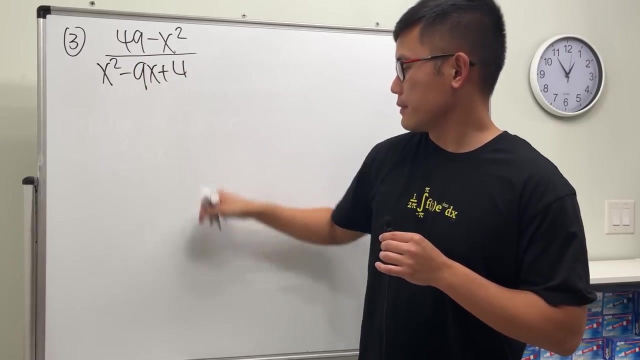 topic. feel free to comment down below and let me know. Let's see number 3.. I have 49 minus x squared over. on the bottom, I have x squared minus 9x plus 14.. Alright, on the top we have. 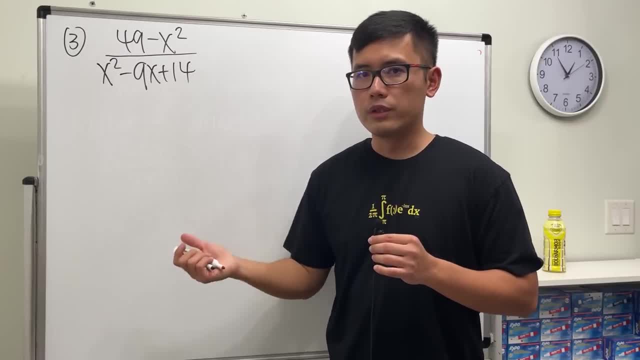 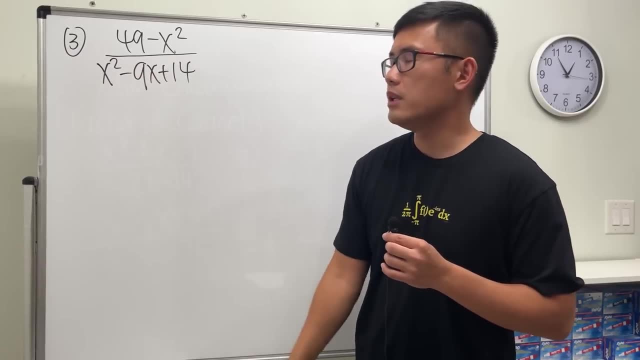 49 minus x squared. I like to call this out of order because we usually like to have the x squared part goes first, Especially on the bottom. we have the x squared part goes first already, So I'm going to just switch the order of the subtraction and make sure that we take 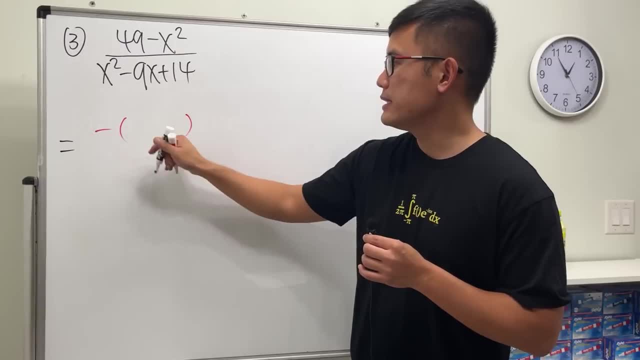 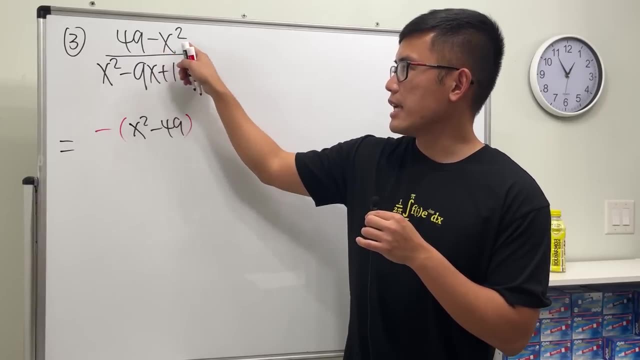 our negative like so, And then for the inside we can put this down as x squared minus 49. This is true because if you distribute, you see this times that it's negative x squared and this times that is positive 49.. 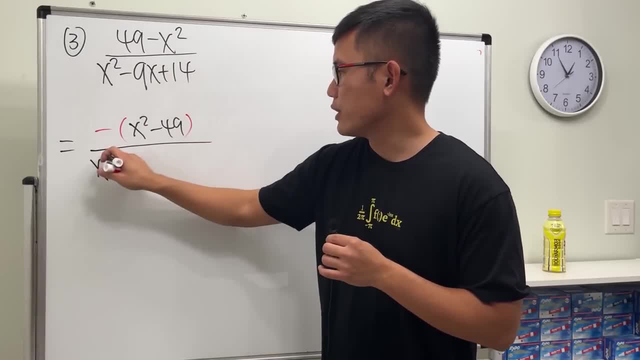 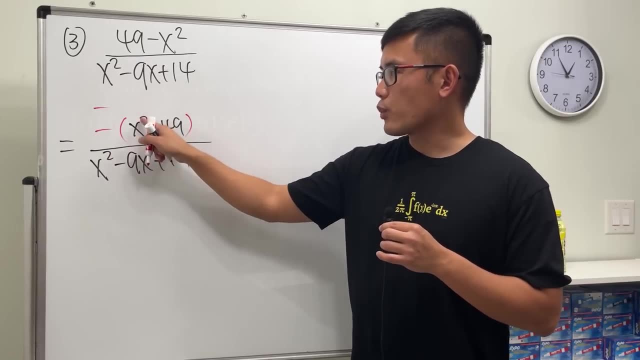 So let's take this part and then, right here, let's just write it down again. Okay, now let's factor it On the top. we still have the negative. This is x squared minus 7 squared, so we can use the difference of two squared formula. Factor this as x minus. 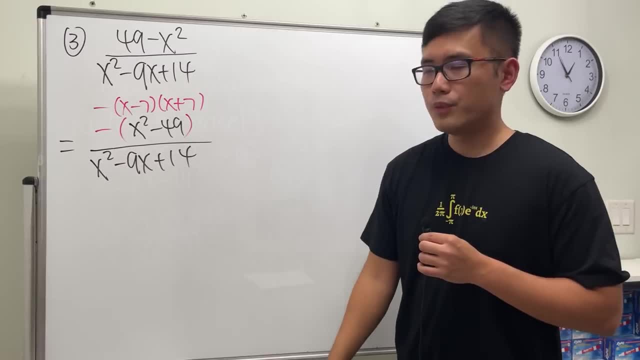 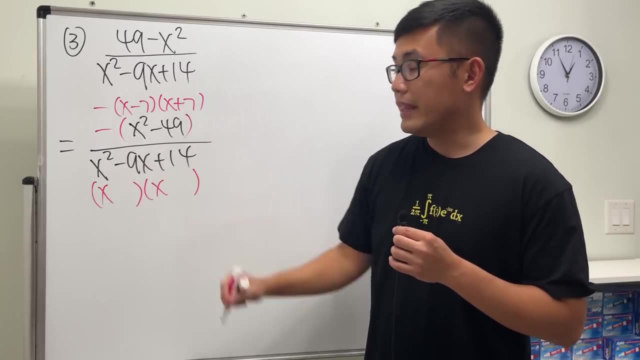 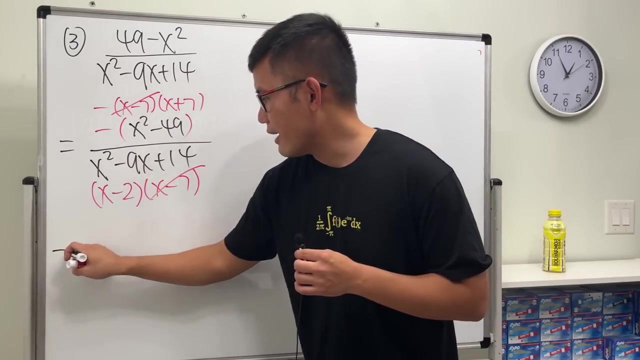 7 times x plus 7.. And on the bottom we'll see x and x. okay to give 14, and together we need to add up to negative 9.. Let's use negative 2 and negative 7.. Yes, this and that cancel and we have the. 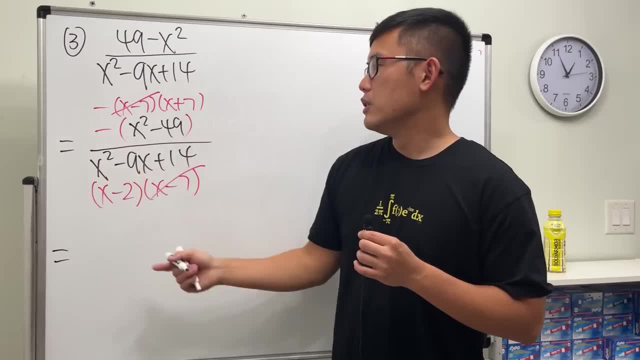 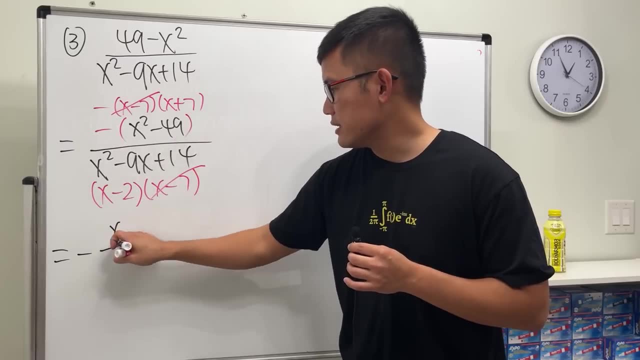 following. Notice that the answer is negative. It depends on how you want to write it. You can put a negative at the front like this: If that's the case on the top, you can just leave it as x plus 7 over x minus 2.. You don't need the parentheses. 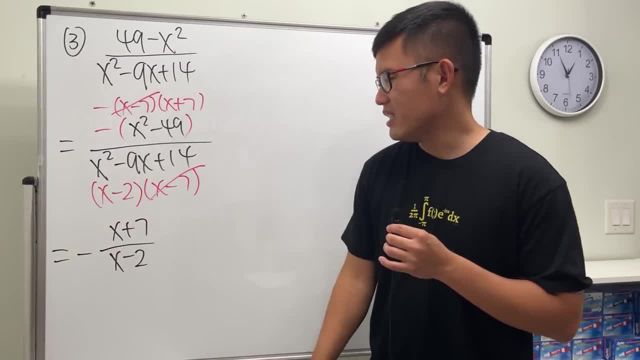 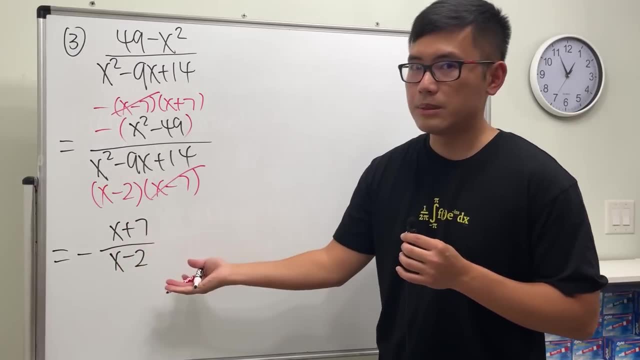 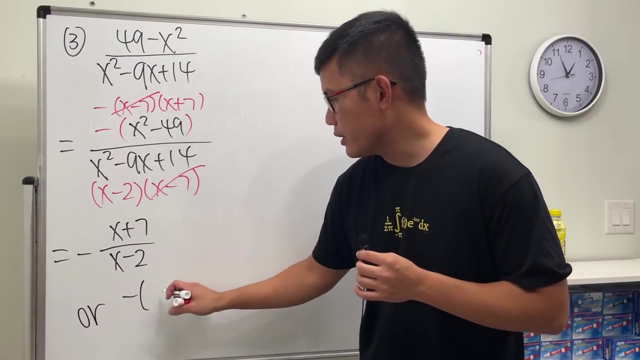 if you put a negative at the front right here in the middle of the fraction. So just technically, there's invisible parentheses. you have to know. Likewise, the button is also invisible parentheses. If you want to write the negative on the top, then make sure you write it like negative parentheses. 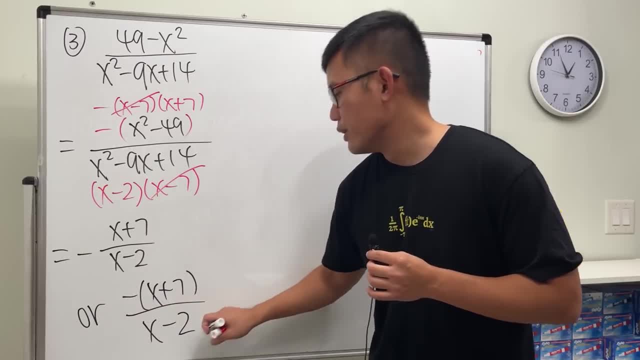 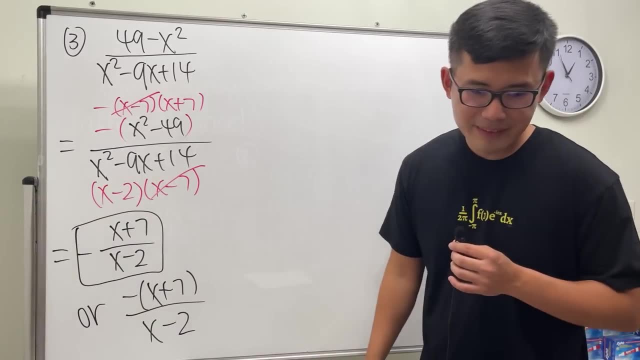 x plus 7 over x minus 2.. Of course, if you want to distribute, be my guest as well, but I'm going to leave it like this, Right. So that's number 3.. Okay, number 4.. 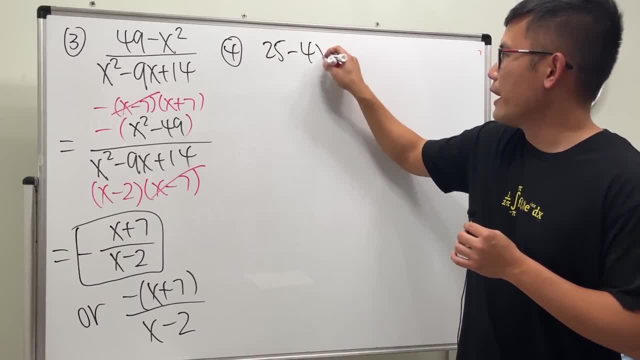 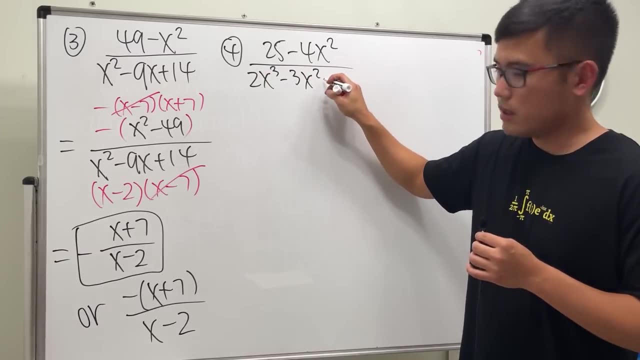 We have 25 minus 4x squared, and then over, alright, 2x to the third power, minus 3x squared, minus 20x. Alright, on the top again. this is out of order. We'd like to have the x. 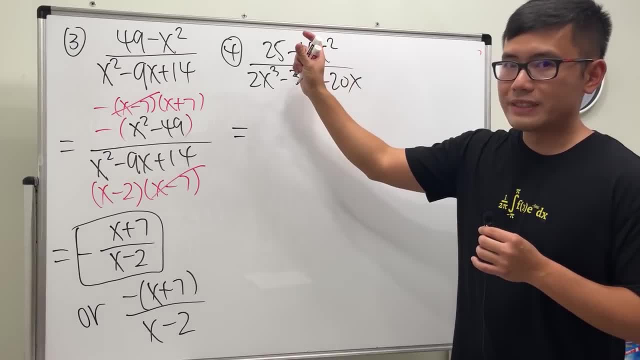 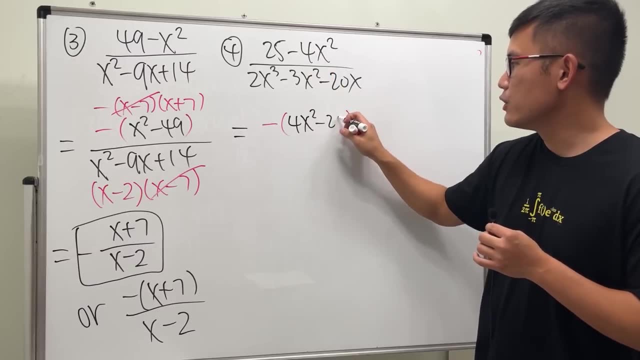 squared term goes first. So let me just switch the order of subtraction. I will put down negative parentheses and then inside this is 4x squared, and then minus 25, similar to this one, And then, on the bottom, let me just keep it as how it is. 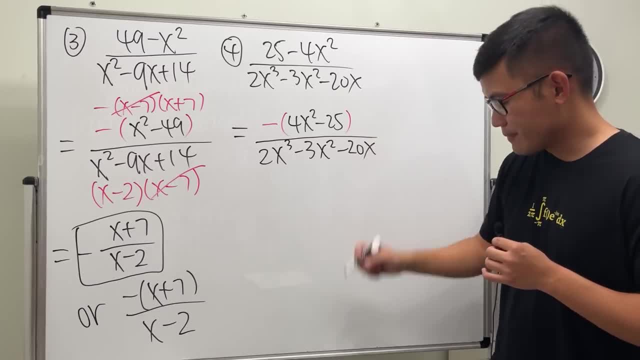 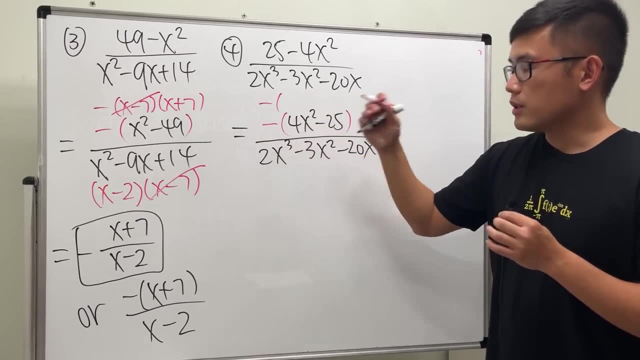 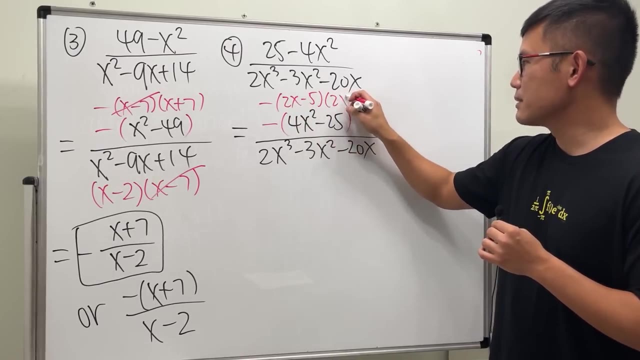 and then I'm going to factor the top and on the bottom as well. Alright, so on the top it's a difference of 2 squares, so let's write down the negative. This is 2x squared minus 5 squared, so we get 2x minus 5 times 2x. 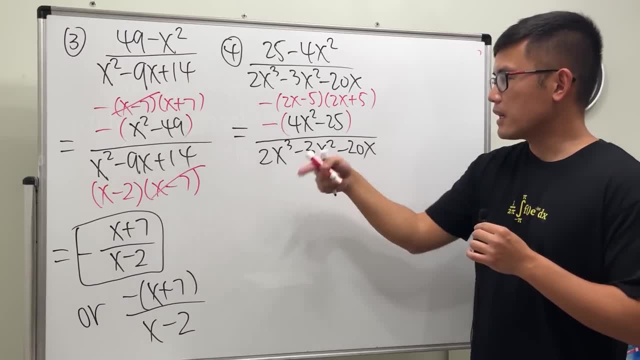 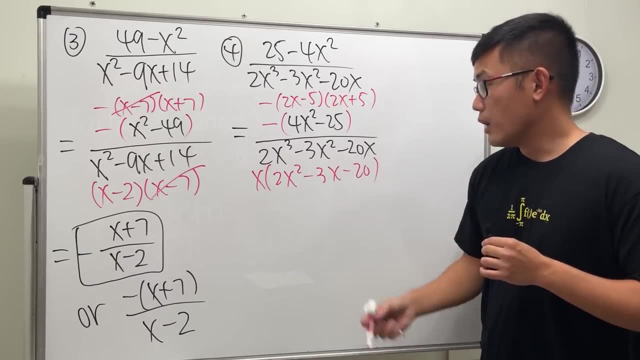 plus 5.. On the bottom, let's factor on x first, so we get x, and then here we have 2x squared minus 3x minus 20.. Okay, this right here is a trinomial. Again, the coefficient right here is the 2, so maybe we will need to do some. 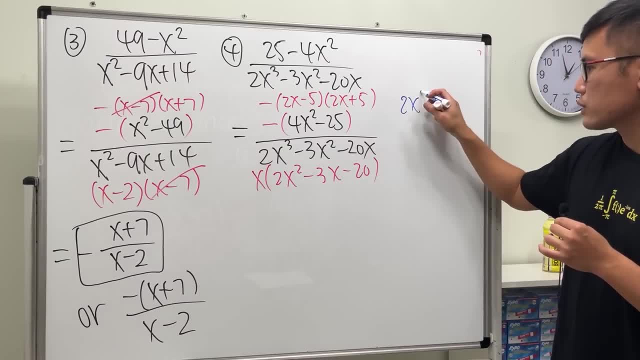 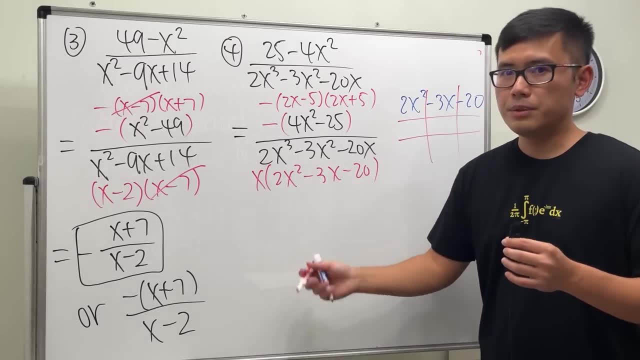 scratch work. on the side, Let's see Tic-tac-toe in action: 2x squared minus 3x minus 20.. And, of course, if you can just look at it and write down the correct answer, be my guest as well. 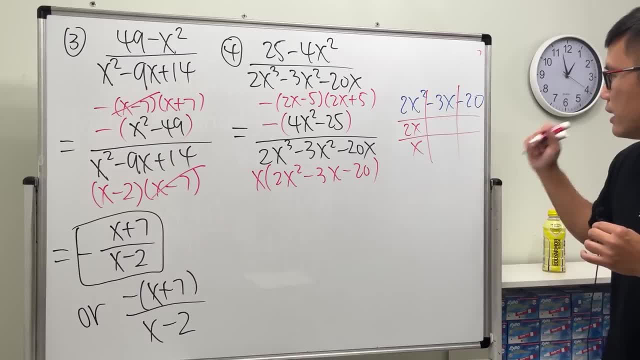 But anyway, already let's see 2x and x. that's the only choice. And then to get negative 20, let's see, shall we do 5 and 4? 4 times 2 will be 8,. 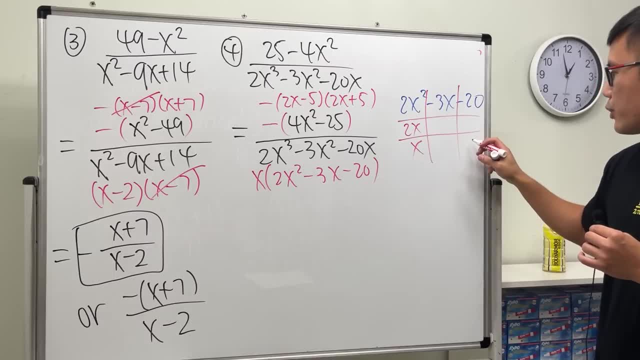 and then 5.. So I'm going to put down 4 here and then divide it here, and then I need to get negative. I need this to be negative 3, so this should be bigger, Because together we get a negative 8x, and then this right here is 5x Together. 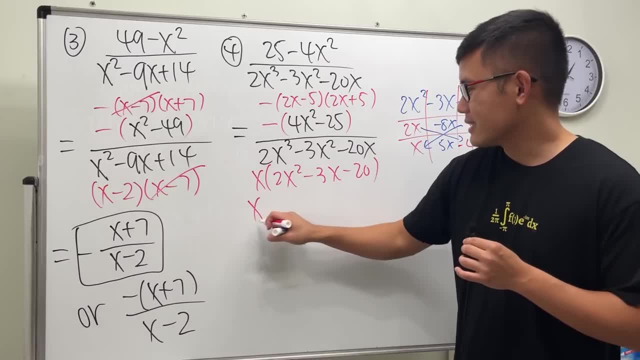 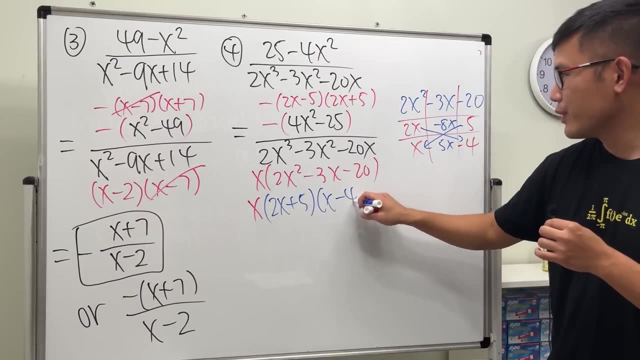 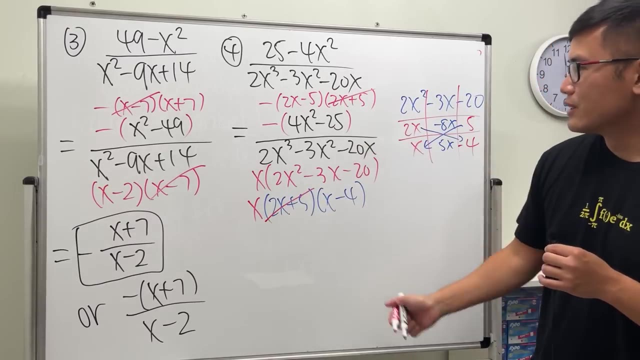 we do end up with negative 3x, Alright. so here we have x times, read it across. we have 2x plus 5 times x minus 4.. Good, And then let's see What can we cancel? This and that? 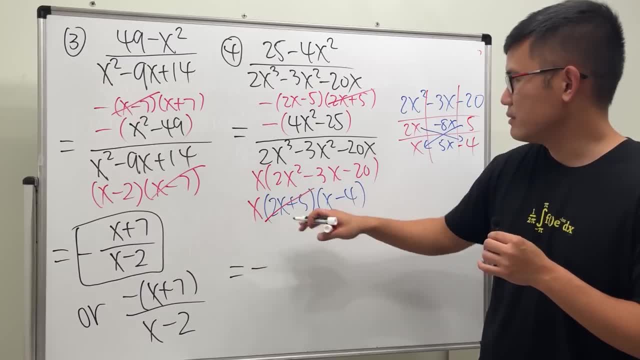 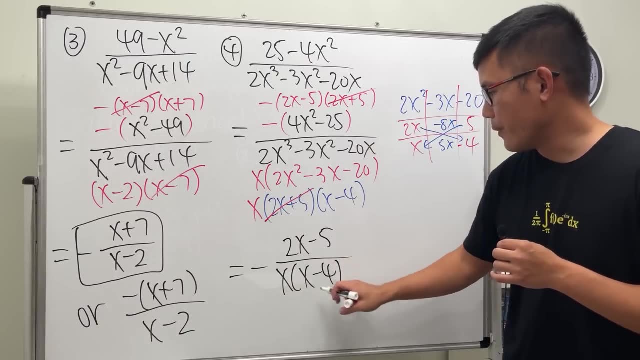 So let's just put the negative at the front right here and then like that, and then 2x minus 5 over x right here, times x minus 4.. Usually you want to keep the top like distributed or factored. 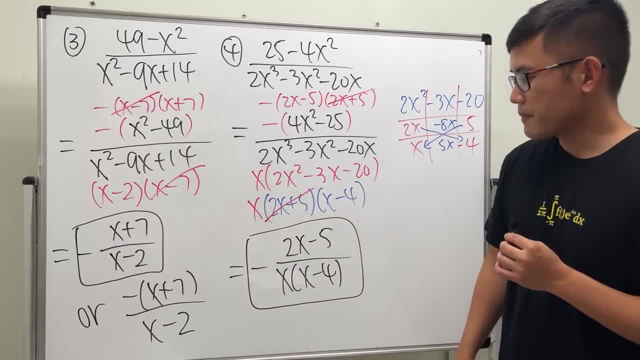 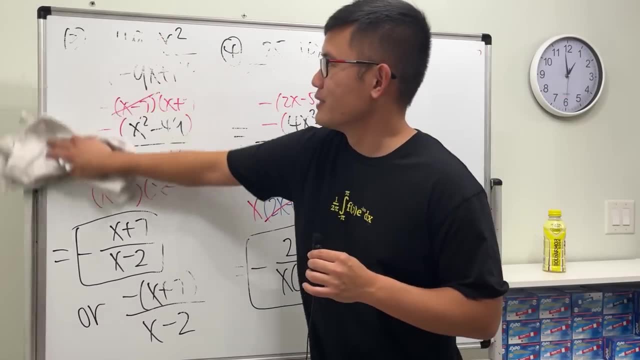 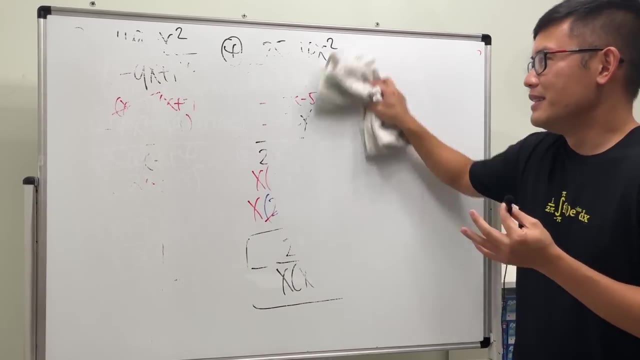 or just leave it like that On the bottom, leave it factored in like this: Alright, so that's usually the case. So do you guys miss the algebra today? All this stuff, Yeah, And in calculus you know all these algebra things- is just going to be like a little thing, little. 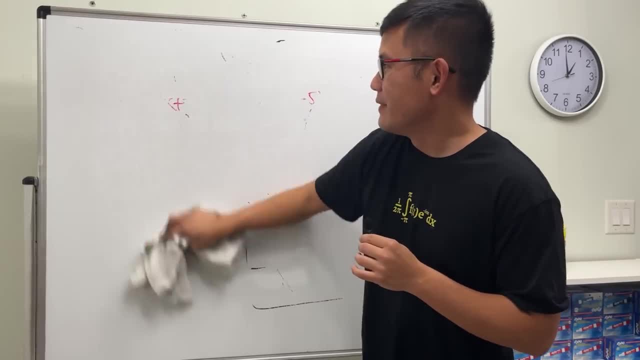 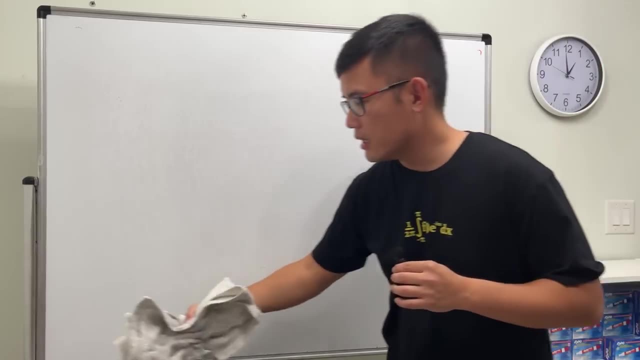 steps of your big calculus questions, right And later I'll also tell you guys these simple applications that you guys will have to do because you guys will encounter that when you do derivatives. So I'll tell you guys once we get there And 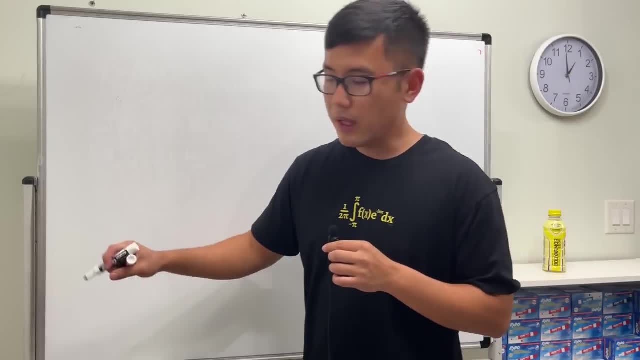 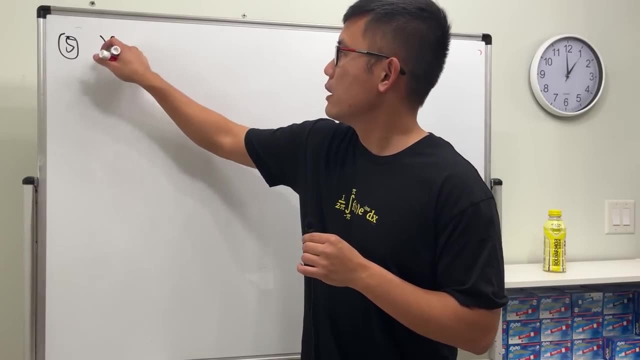 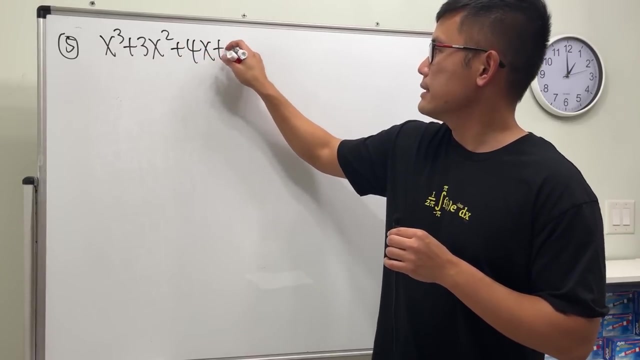 let's see number 5.. We have the following On the top, we have a four-term polynomial: x to the third power plus 3x squared, plus 4x plus 12 over 4x plus 12.. So on the top, 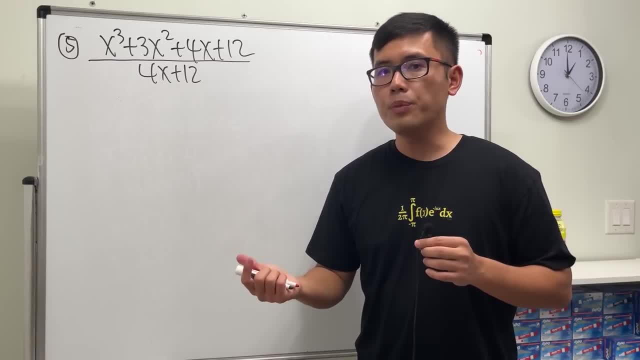 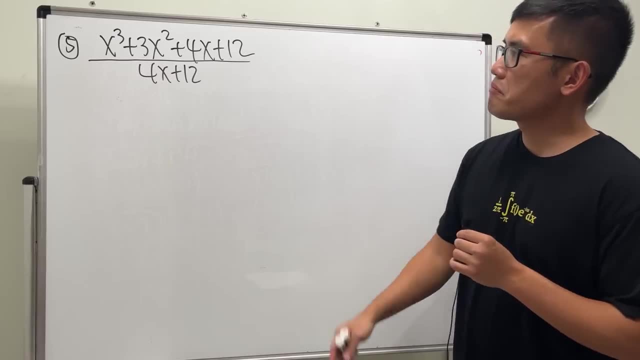 we have four terms. Let's go ahead and use factored by grouping. That's usually a strategy for that And, in fact, if you want to do this right here by long division, yeah maybe, But you'll end up with 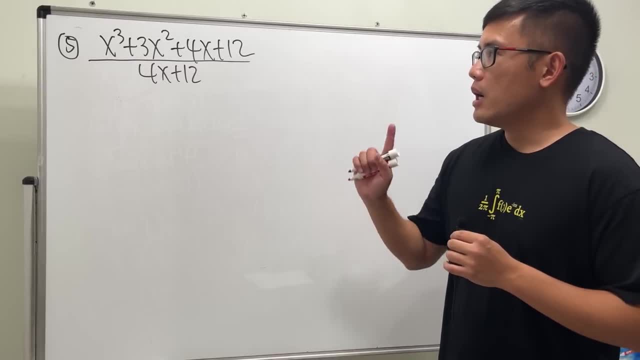 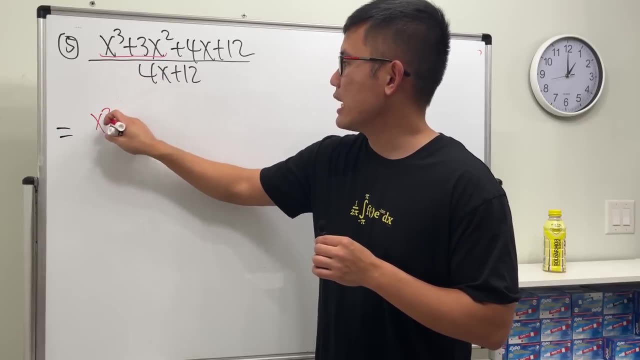 fractions. so up to you, Let's go ahead and factor by grouping, because we notice that these two terms, we can factor it with the x squared on the outside and then we get x plus 3.. And then these two terms. 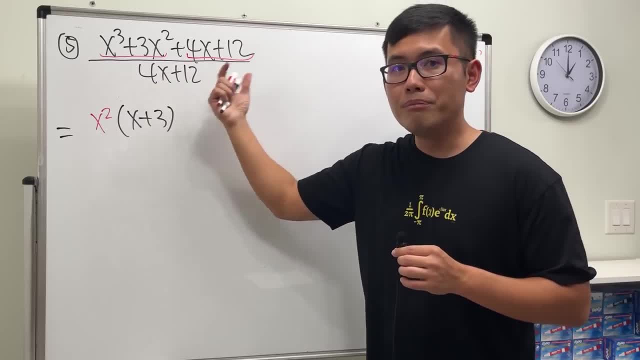 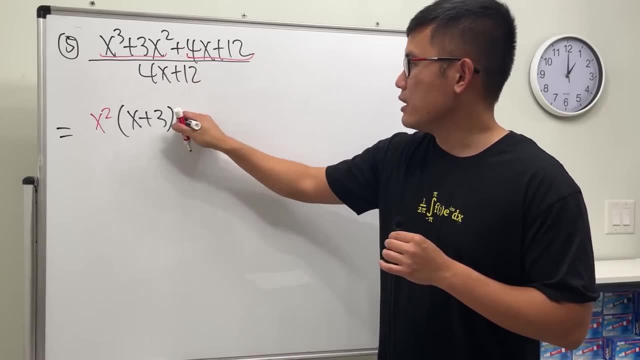 notice this and that are the same, but do not cancel this and that We must factor the top and then cancel things out after that. So this and that let's put down the plus right here first, and 4 and 12. 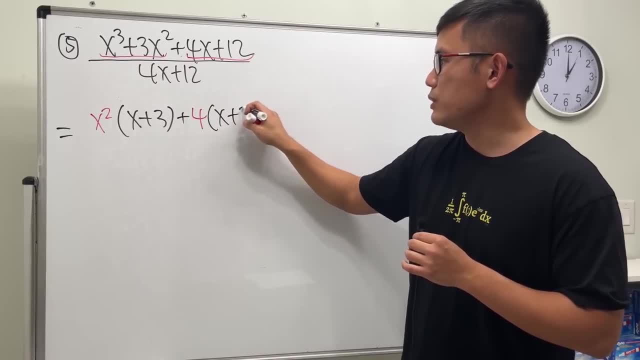 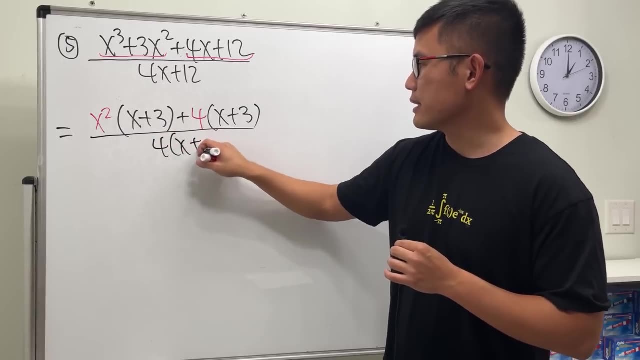 we can factor out 4, and then we have x plus 3 left like this On the bottom. hmm, we can factor out 4,. might as well, right? So let's put down 4, and then x plus 3.. And notice: 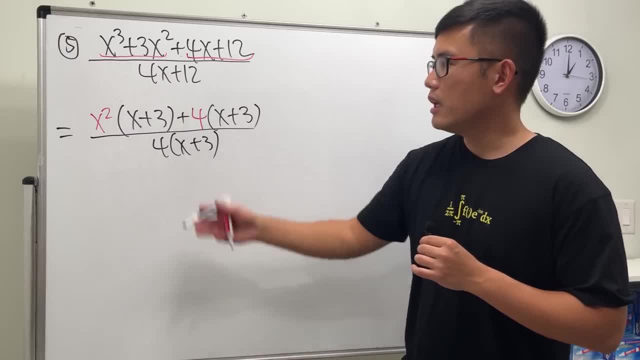 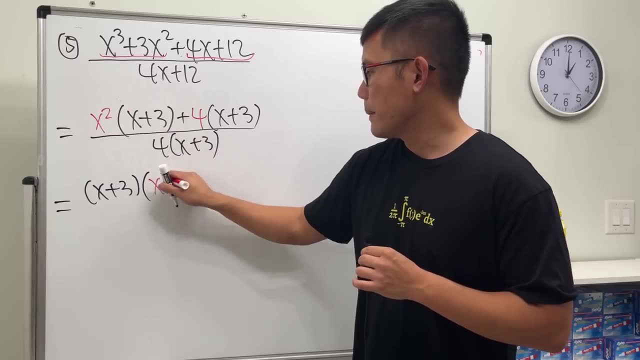 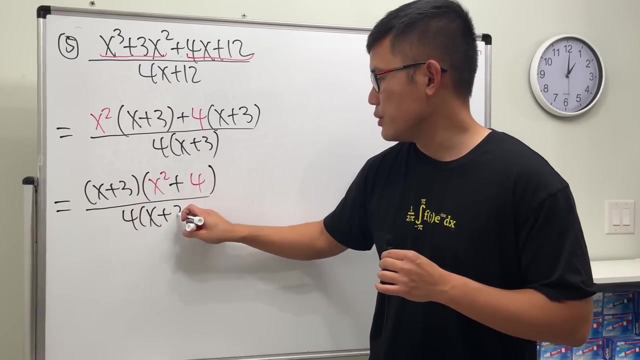 everybody has the x plus 3.. But let me do this properly. Let me factor out the x plus 3 right here, and then we have the x squared plus 4, and then over this and that which is 4x plus 3.. And we see this and that cancel. 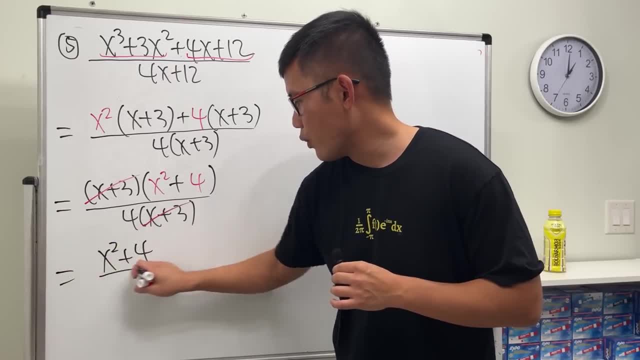 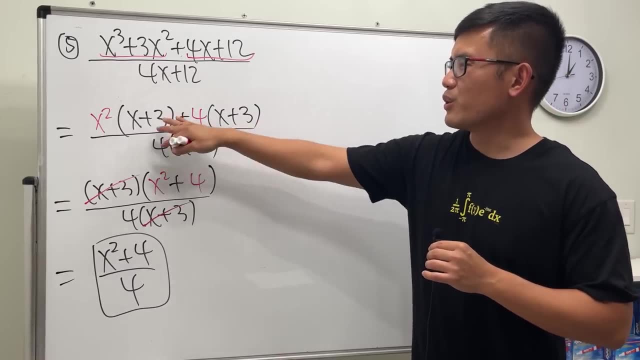 and we get x squared plus 4 over 4.. And then we are done So just like that And notice that, yes, you can just cancel this out, but usually I prefer to show my students factor everything completely on the top and then 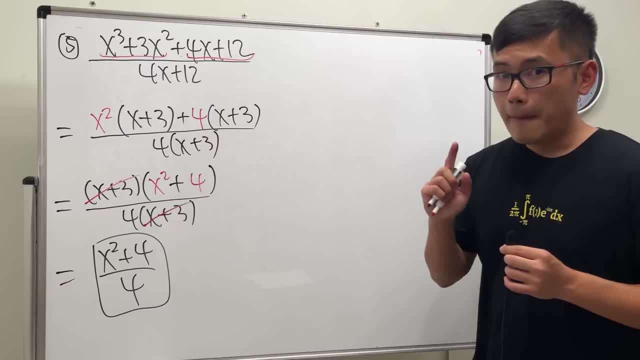 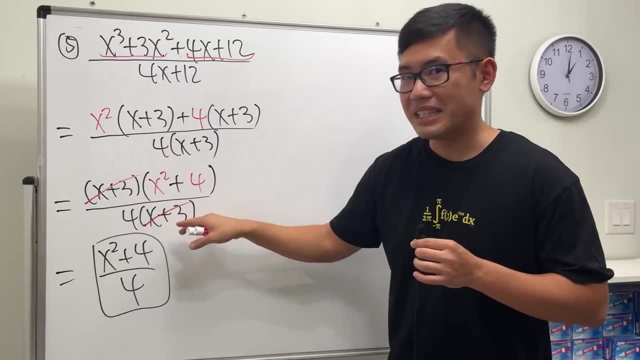 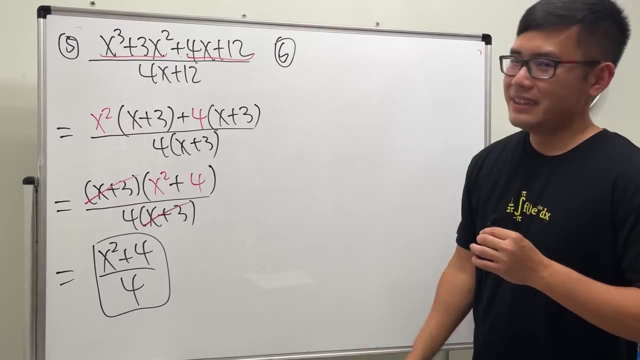 cancel out the factors And pay attention, attention to the top right here. notice that everything is multiplying, or two things are multiplying. that's how we can cancel this and that later on we'll encounter some trickier questions. right? so these are just a phone like warm up the Google algebra days, the days that you didn't. 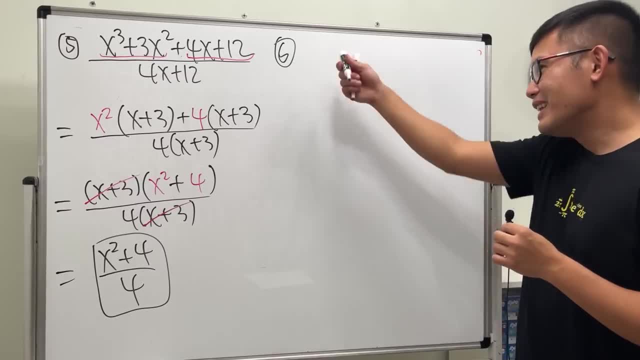 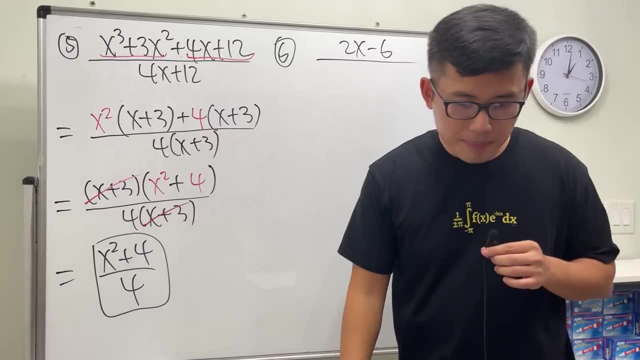 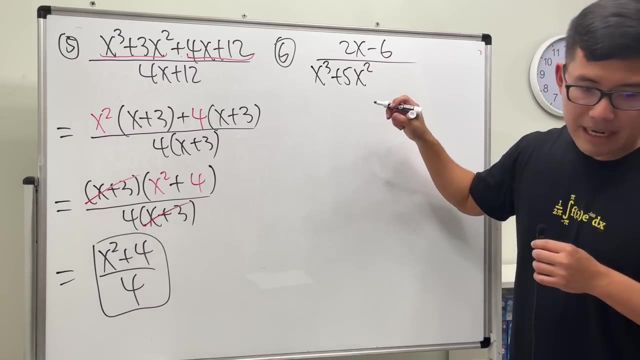 really need to study and can still get the a on the test, right? yeah anyway, number six, right, kind of refers to a little bit. we have 2x minus 6 on the top over on the bottom we have x to the third power plus 5x squared, minus 5 minus 9x and then minus 45. all right, so let's see, on the top I'm. 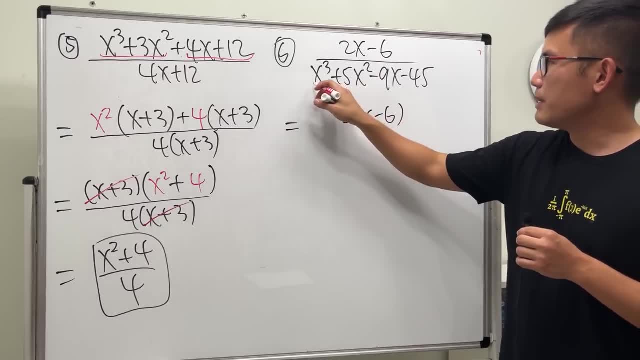 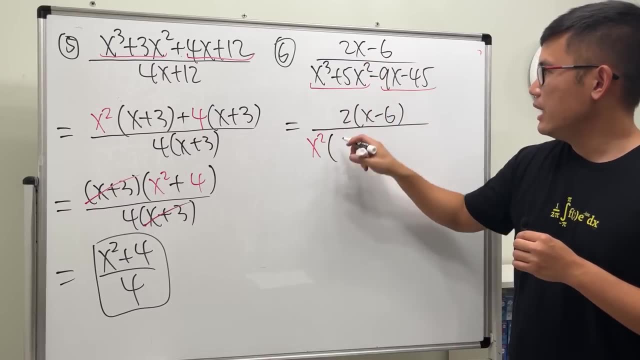 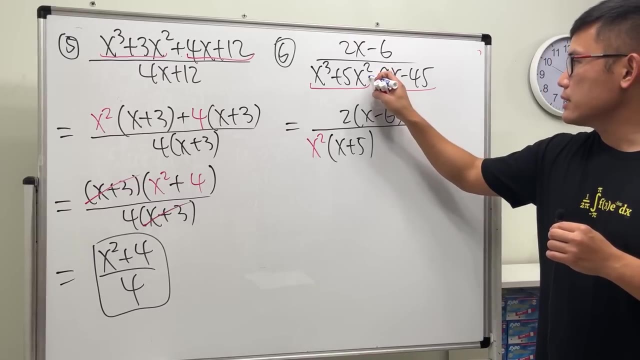 just going to factor out 2, 6, like this on the bottom. again, factor by grouping. right here I'm going to take out x squared and then we get x plus 5. all right now. right here, we have the minus. so let's go ahead and write that down right away, just like what we did earlier. it was a plus, we write it. 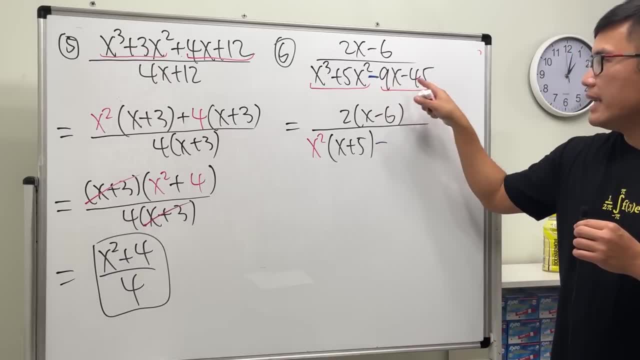 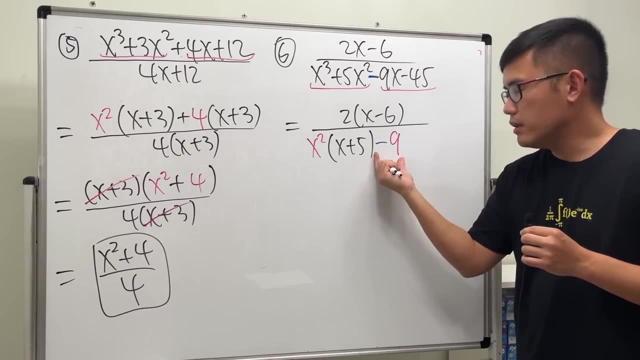 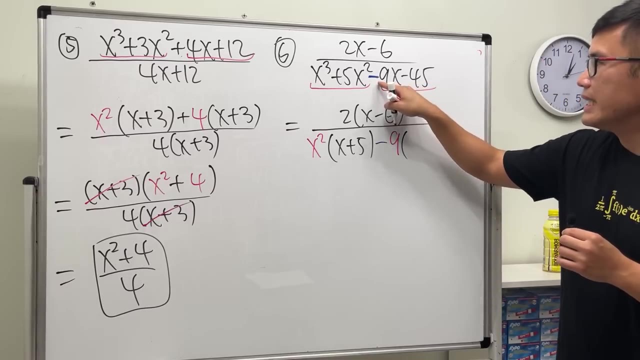 down right away, right, okay. and then let's look at the 9 and also the 45. we can factor out 9, so let's put that down right here. but you see this way, right here we are technically factoring out a negative 9, so be really careful. originally this term is negative 9x, but we took out the 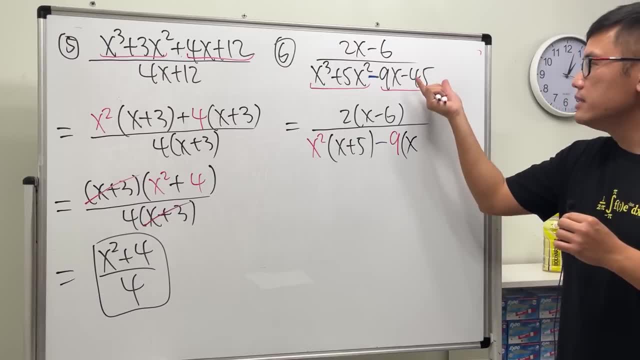 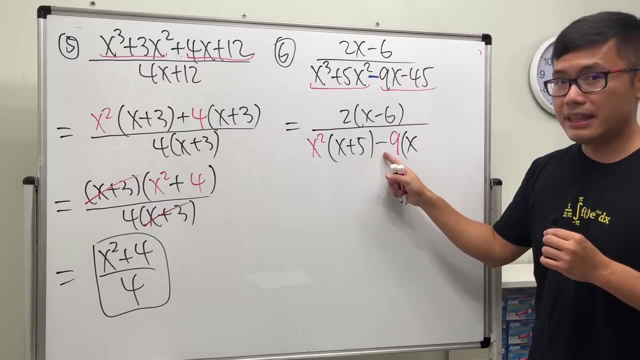 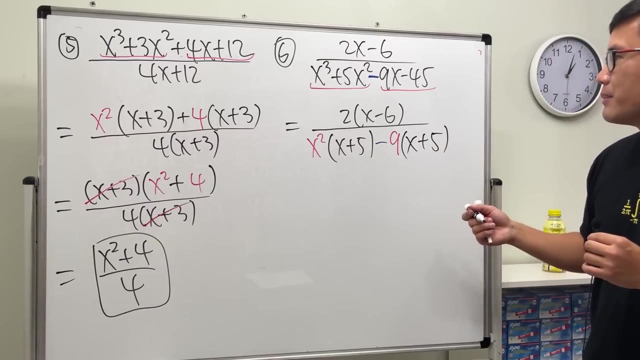 negative 9. so, right here, we just have x, and then this is negative 45, but we took out negative 9. so just do this: negative 45 divided by negative 9, we get positive 5. yes, this and that will have to be the same right. 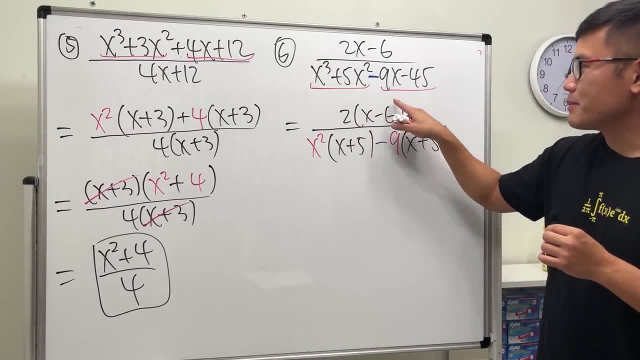 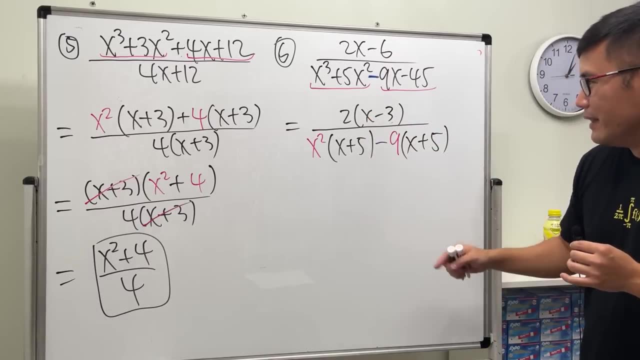 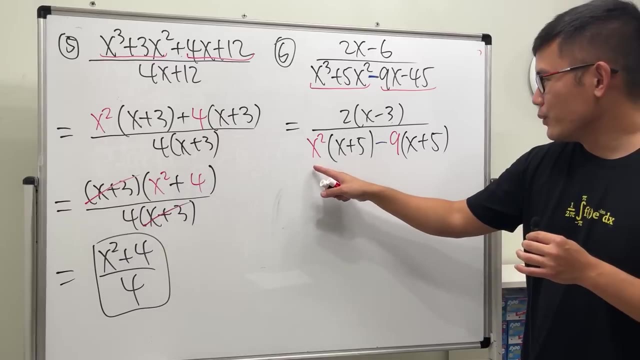 yeah, hold on one sec, my bad sorry. X minus 3.. just kidding. okay, now let's see right here. okay now let's do this, because I know on the factoring right. so let's just go and put this and add like this: x plus 5, and then times x square. 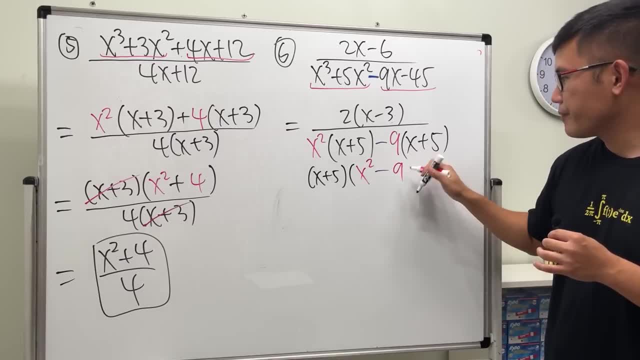 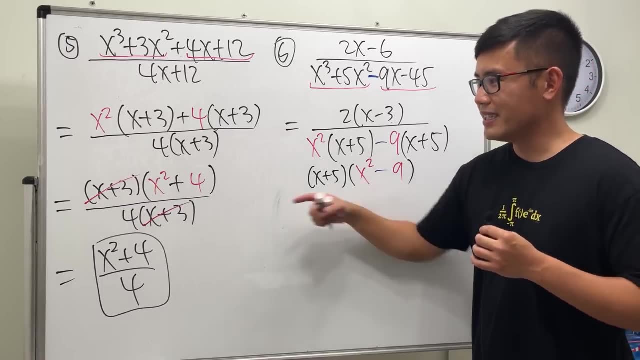 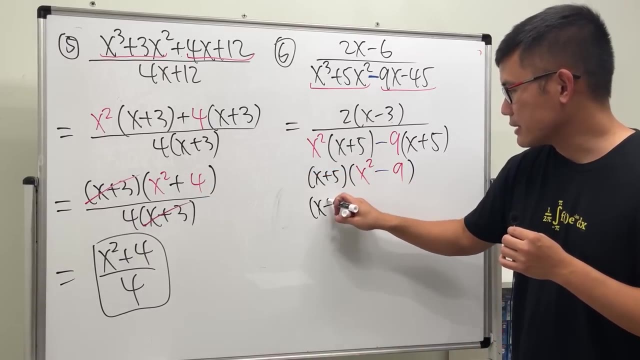 minus 9, like that good. but the thing is that- notice, x square minus 9 is actually factorable, because this is the difference of two squares. earlier we stopped it right there because that was not factorable. all right, so let's go ahead and just factor this: x plus 5. factor this, we get. 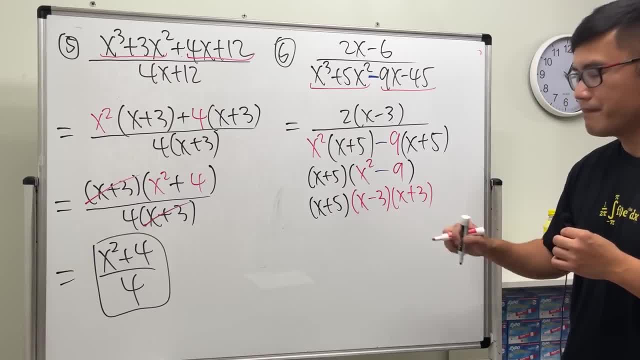 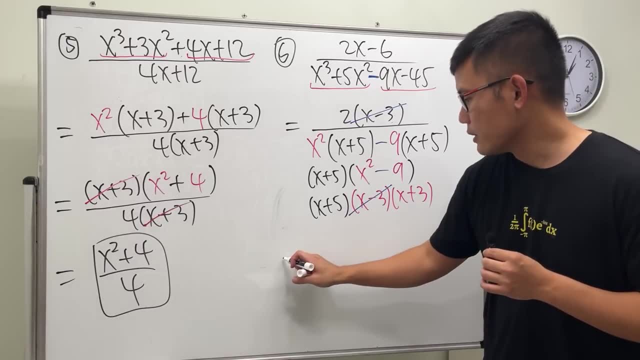 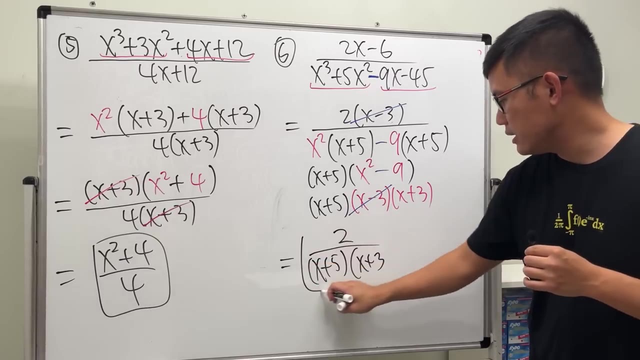 x minus 3 times x plus 3.. yep, x minus 3 and x minus 3 can be cancelled. and finally we have 2 on the top over x plus 5 times x plus 3, and then we are done. okay, so for this one, you might. 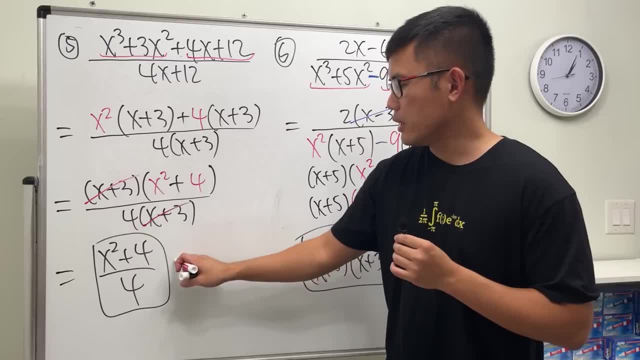 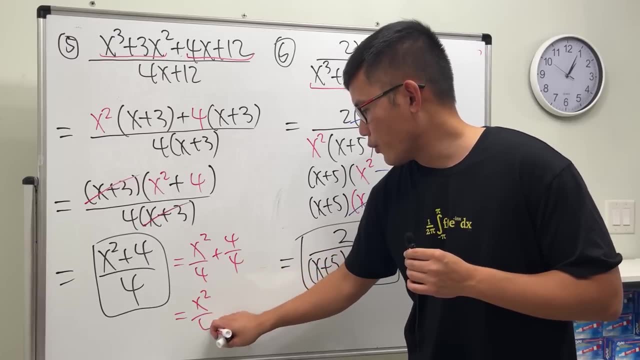 have been wondering: hmm, don't we want to just split the fraction and write it down like this: x to the second power over 4 plus 4.. over 4, and then you can also write this as x square over 4 plus 1.. you could, but this is also. 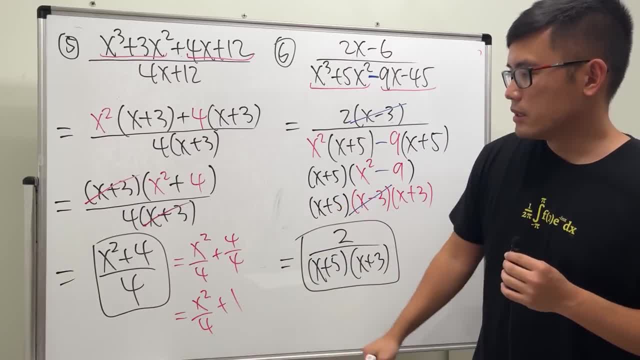 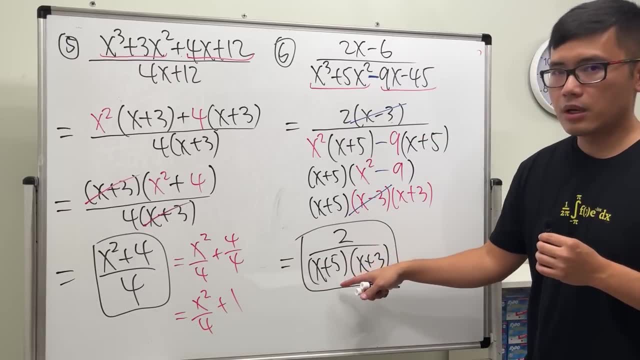 okay, so depends how you like it. sometimes you actually have to write it down this way. it's actually easier. but we'll talk about the situation later and then, as you can see right here, i just leave the answer in the factory form, especially for the denominator, and on the top we actually 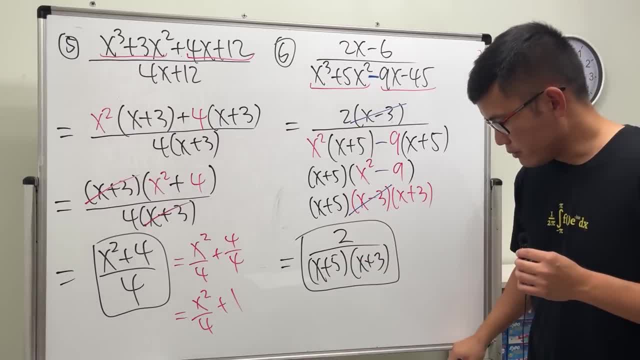 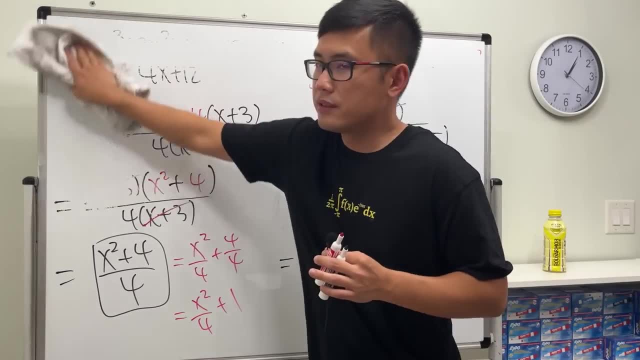 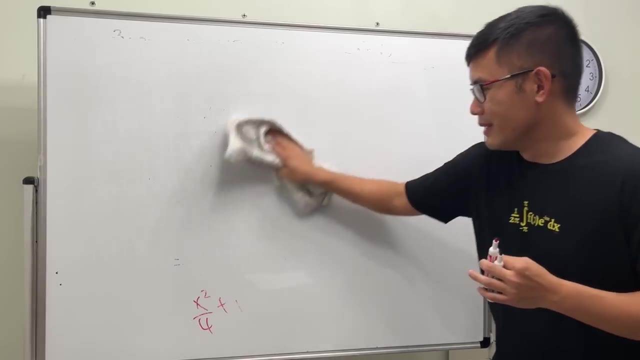 just have two, so that's what we have. so so far, so good. yeah, for a lot of this, seriously, just go ahead and do the work and know the usual things that we have to do, that's all. so remember your algebra and that, seriously, we'll do like 100 algebra equations that you guys should know. 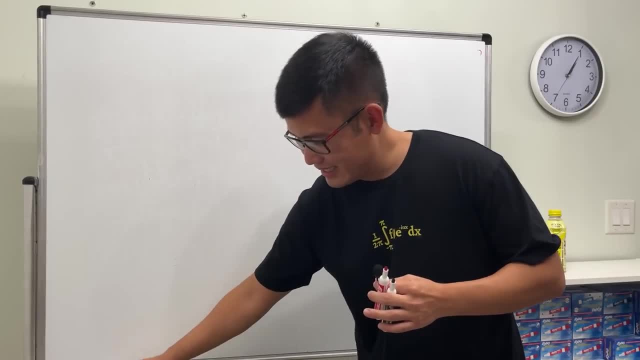 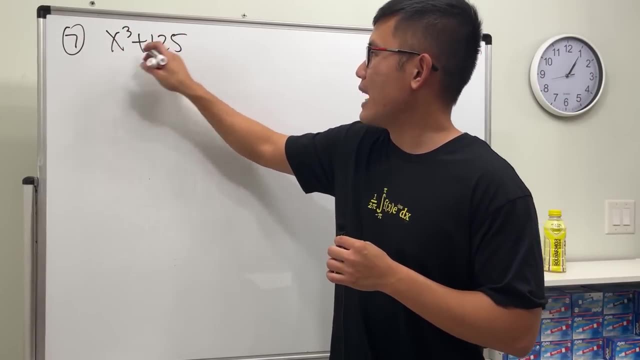 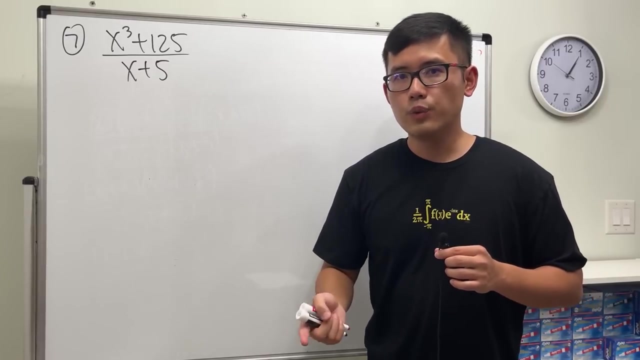 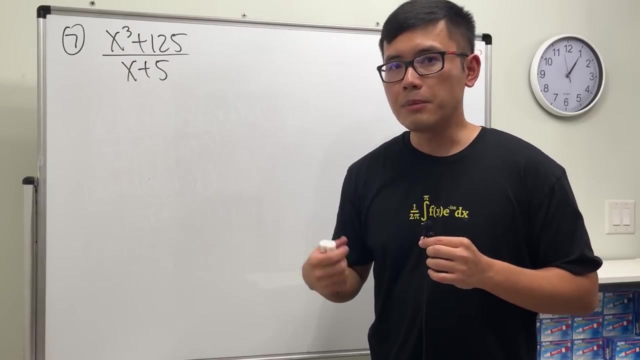 like quadratic equations, especially all right number seven, x to the third power plus 125 over x plus five. so i'm going to show you guys two ways to do this. the first way is by factoring. so here we have: x to the third power plus 125.. this is the sum of two cubes. it's actually. 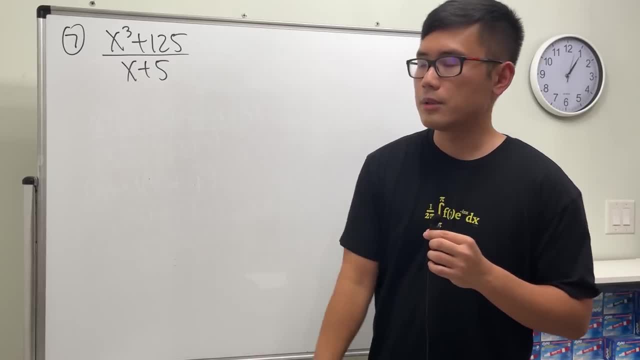 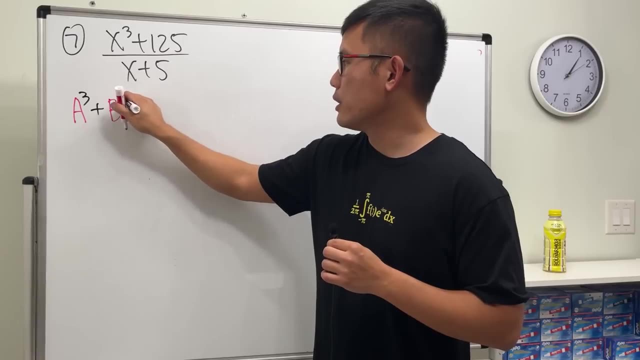 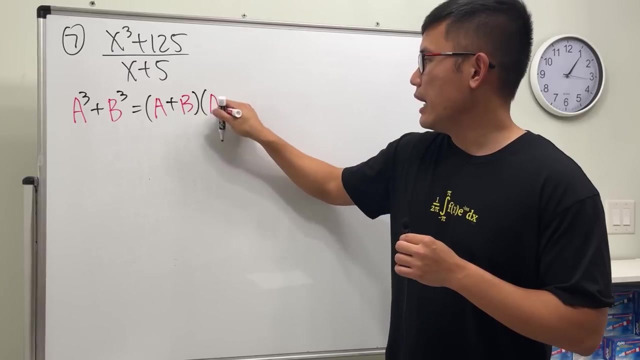 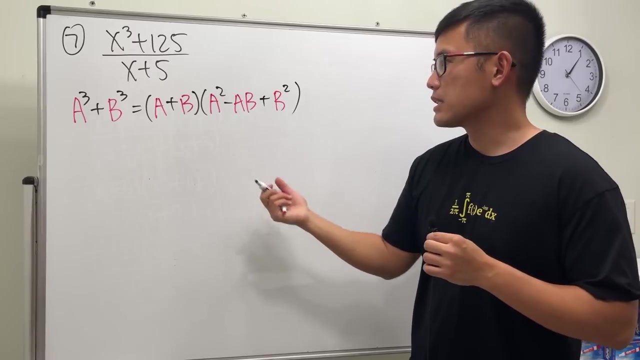 factorable earlier. the sum of two squares is not factorable. this right here, when we have a to the third power plus b to the third power. to factor this we get a plus b times a squared, minus a, b and then plus b squared. so this is the sum of two cubes. factoring formula. 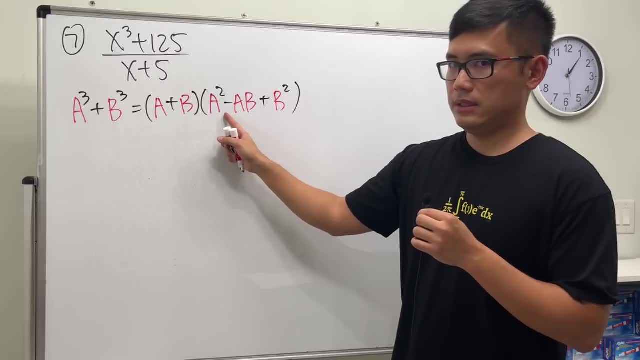 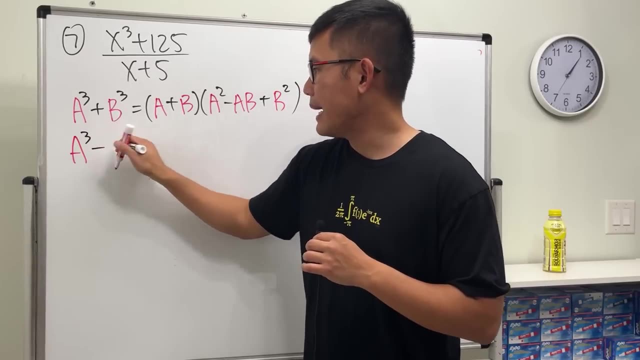 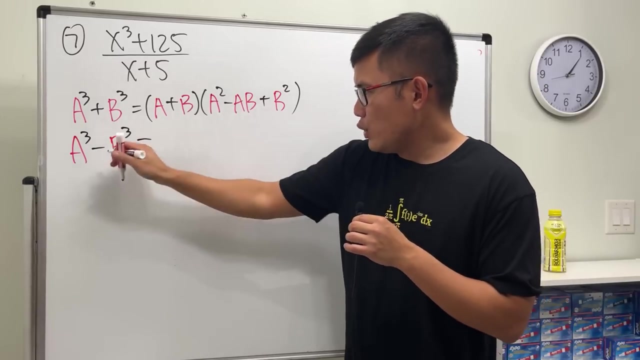 and the way i like to remember is plus, plus, minus. the last one is always plus. why do i say always? because if we have a to the third power, minus b to the third power- i might as well also put this down for you guys, because later on you might use it. if we have this, then we get a. 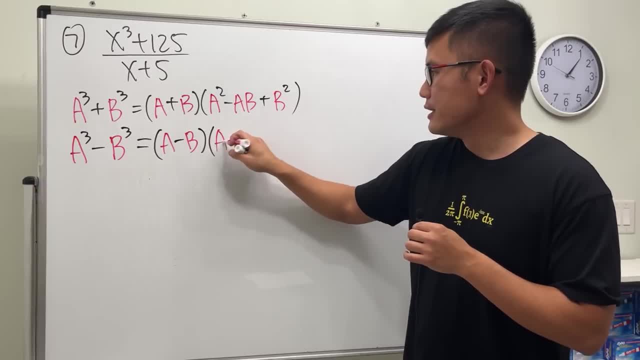 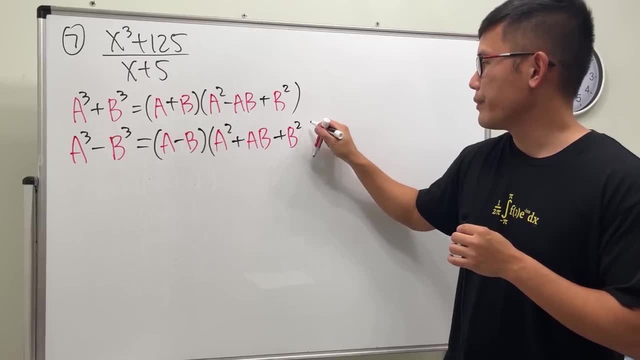 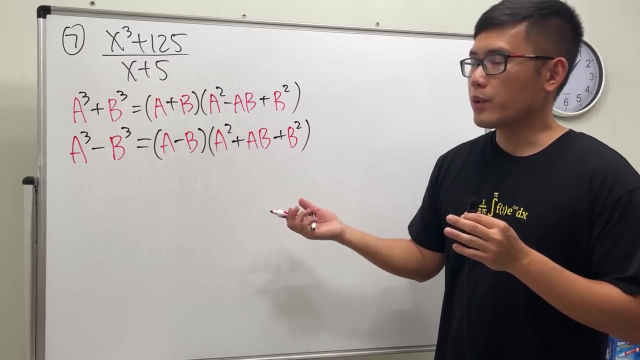 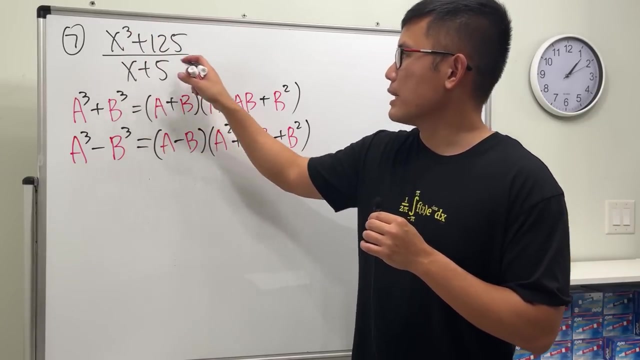 to the third power plus b. to the third power minus b. times of Course, a nations a minus b, times a square plus a, b and then plus b squared. you see last term, right here, is always plus and for the minus version is minus, minus, plus. cool. so that's what we have and of course we are going to use the first one for this. 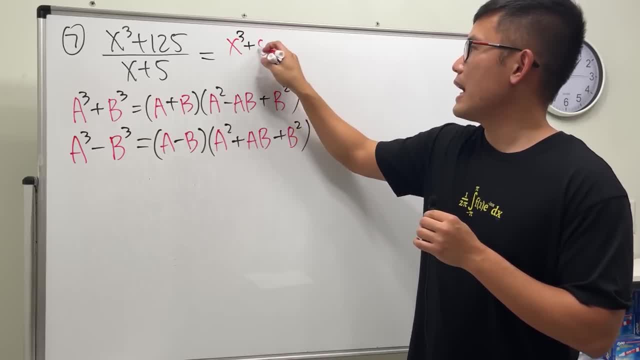 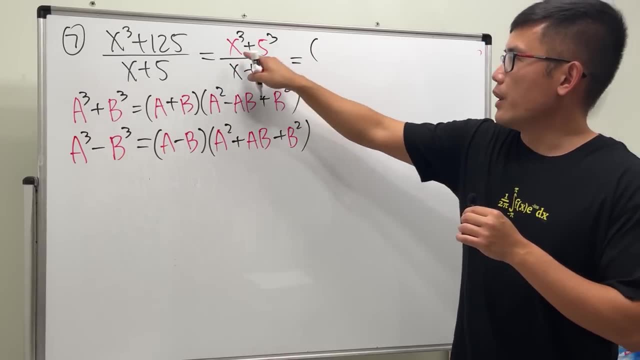 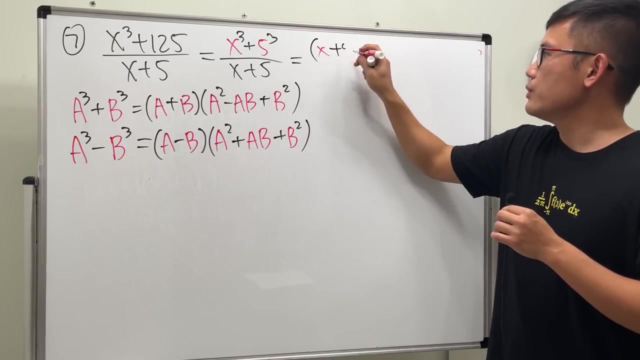 so notice: x to the third power plus 125- we can write that as third power and over x plus 5. when we factor this, where x is the a, 5 is the b, so we get x plus 5, oops times a squared, which is x squared. let's go and write that down. and then next we have the. 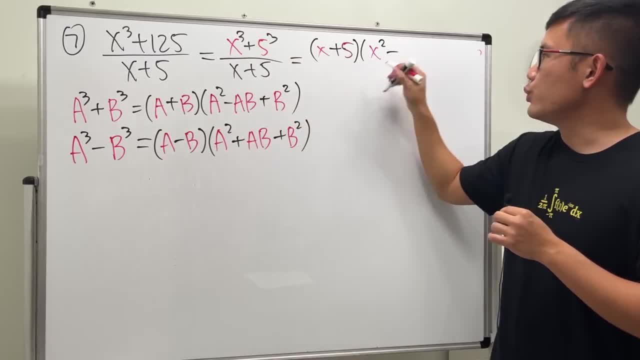 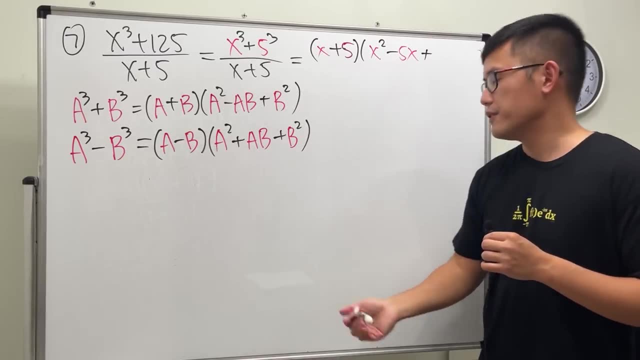 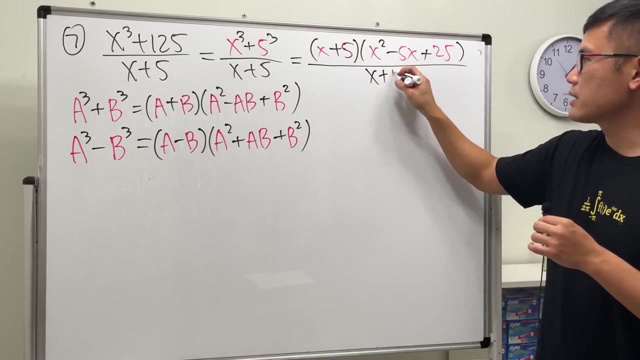 minus, and then a. b means this times that which we have, 5x, and then, lastly, we have the plus b squared 5. squared is 25. so, right here, let's put on 25, and then, all over the denominator, which is just very nice, it's just x plus 5.. better yet, this x plus 5, that x plus 5, cancel and finally. 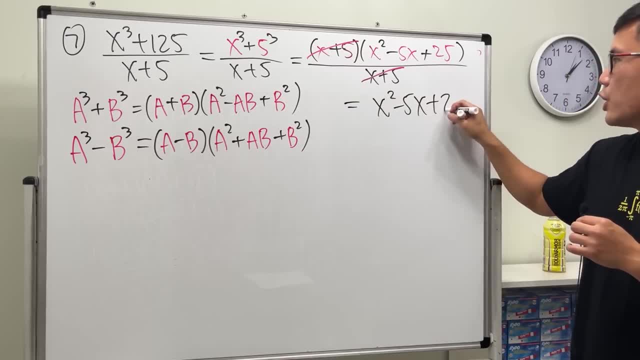 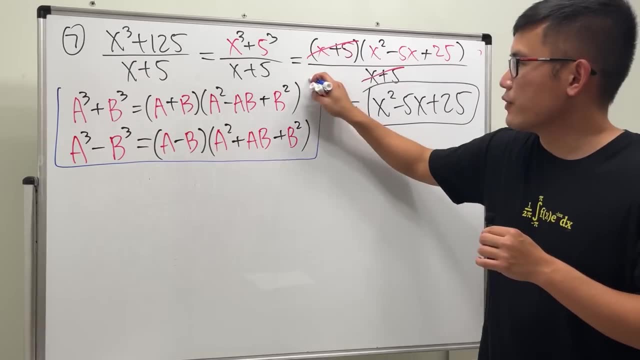 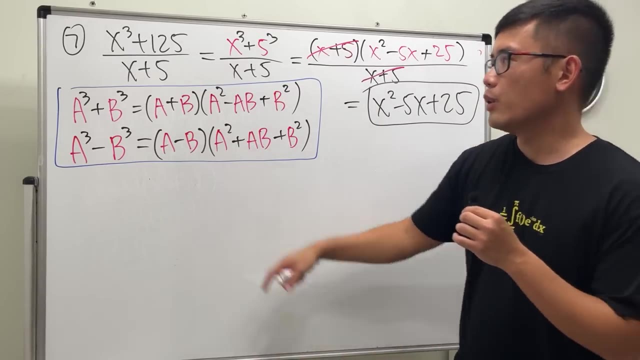 this is the answer: x squared minus 5x plus 25. so that will be it. and, of course, definitely remember these two factoring formulas for the sum and also the difference of two cubes. so this is the first way. now, the second way is that: notice that on the bottom we 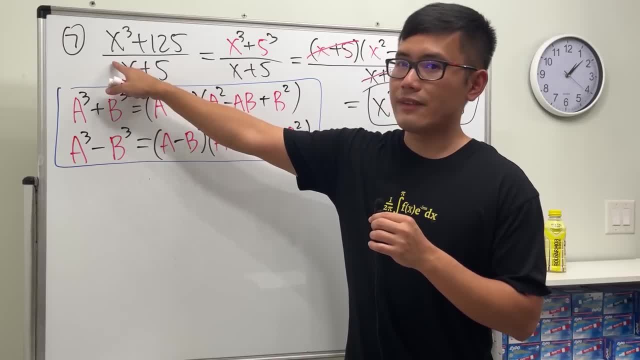 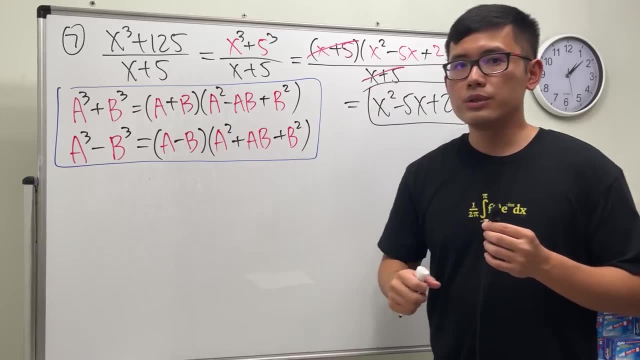 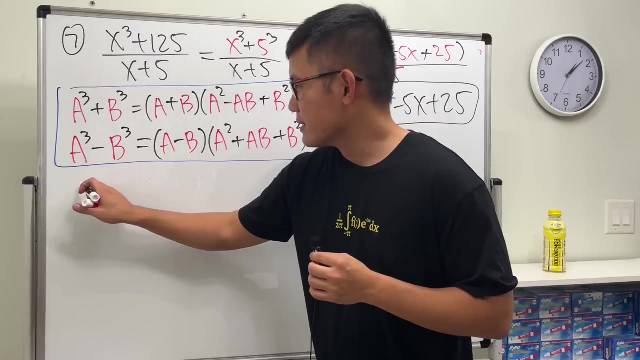 have a binomial and this is very good because we just have a 1 in front of the x, and this is super good because it's just in the form of x plus the number, so we can use long division or tensetic division. so i'm actually going to show you guys both all right. so that's the x to the power plus. 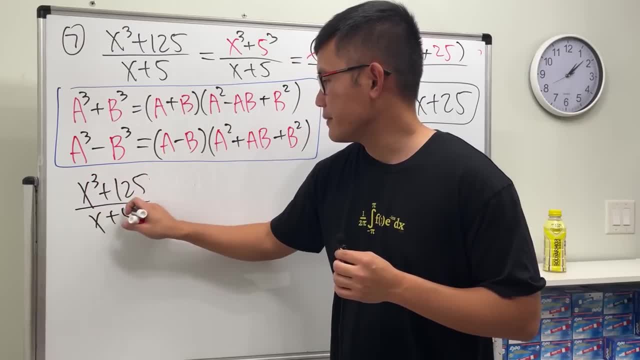 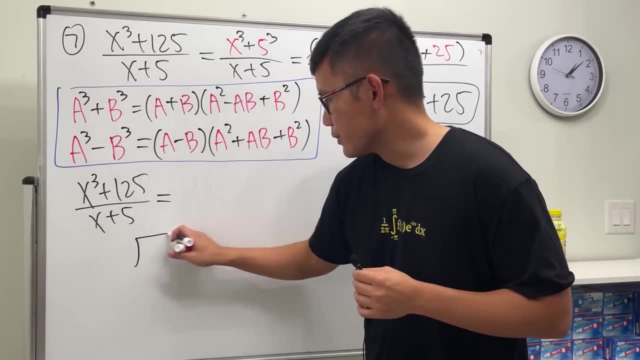 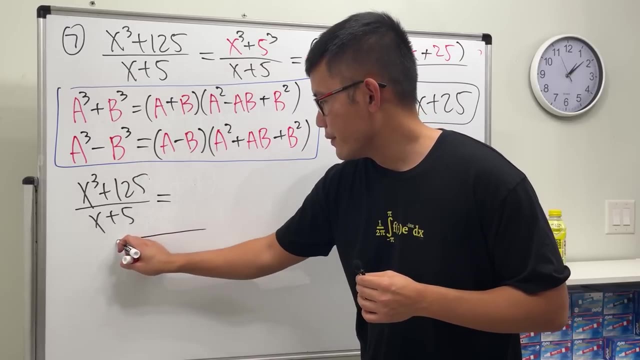 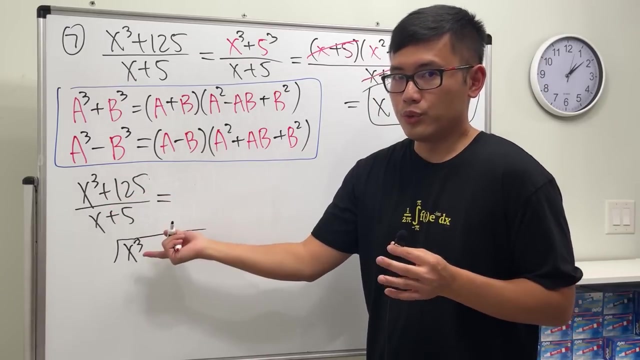 125 over x plus 5.. synthetic diffusion later. let's do the long division first. all right, so that's how you do it. this is how you do it. we are going to put x to the third power, plus 125 inside. but notice, we do not have the x squared term and we do not 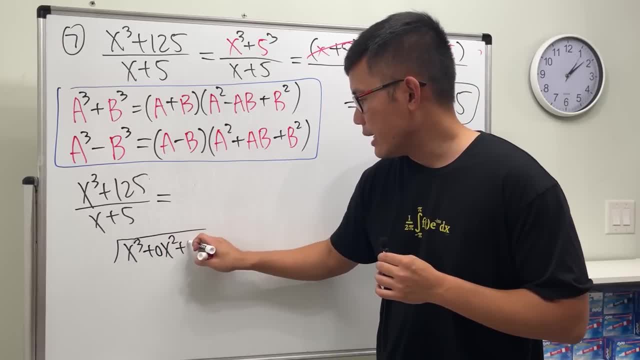 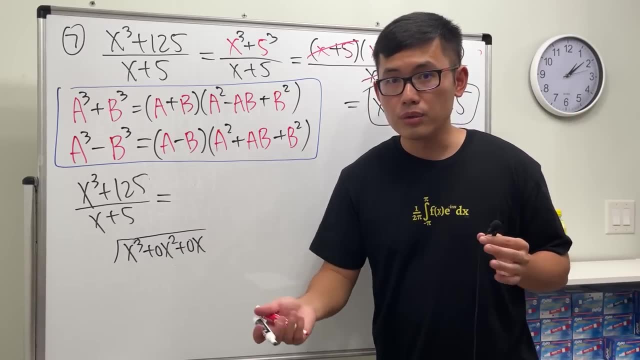 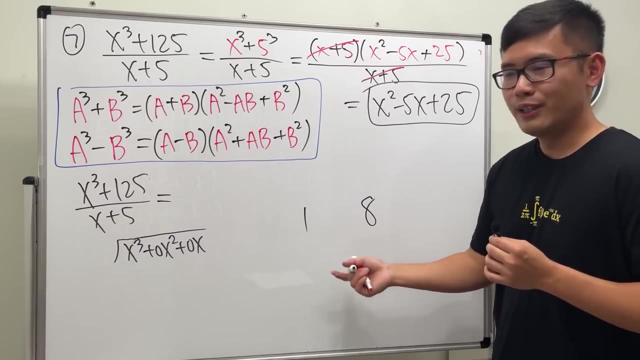 have the x term, so let's go ahead and add 0x squared and also 0x. they are just like the place value. it's just that if you want to write a check for one thousand eight dollars, what do you do? 1 at the thousandth place and 8 at the unit place, right, but what's in the middle? you cannot just put. 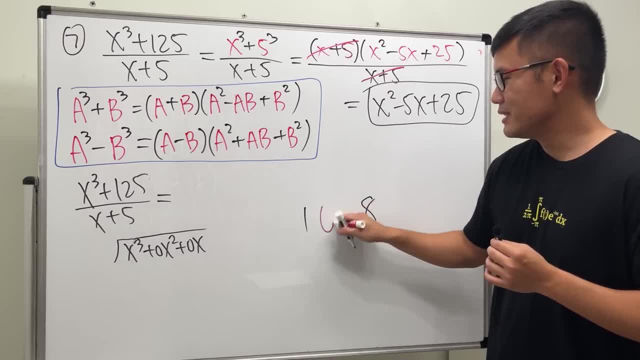 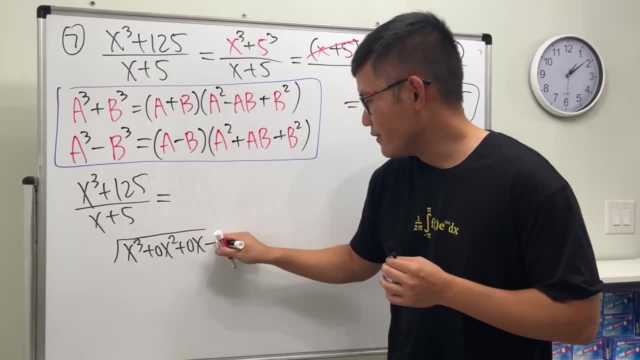 1, 8, that's 18. you will have to put 0, 0 right. so it's like, it's like that idea. and then right here we have that 125 at the end. okay, and then on the outside here we have x plus 5, and here we go. 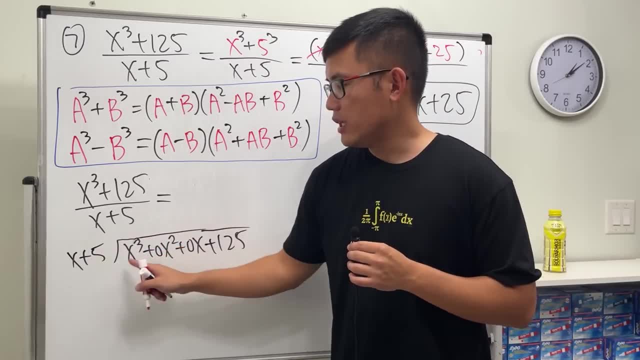 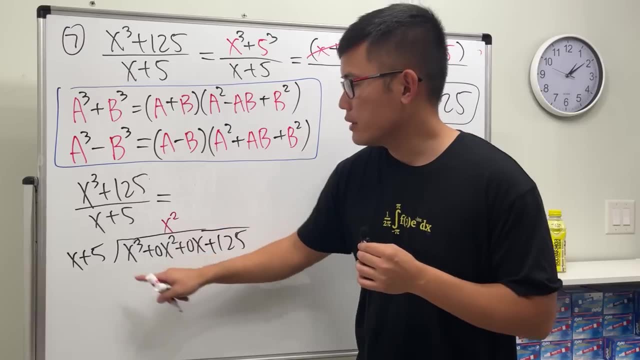 we ask ourselves what times x will give us x plus third power. well, the answer for that is x squared. so let's line up with the x squared right here, and we take the x squared times this, which is x to the third power, and then we take this times that, which is five x squared. 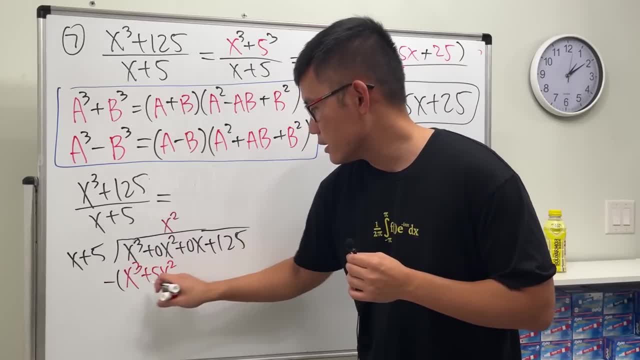 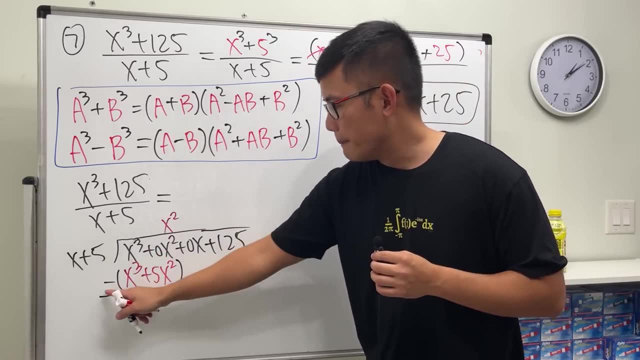 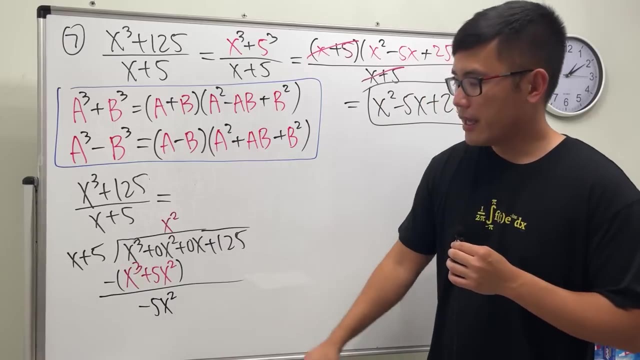 all right. and then when we do long divisions, we are going to subtract like so: and now x to the third power minus x to the power cancel, 0 minus 5 x squared right, and there are the x squared terms. so we get five x squared, and then we bring down the zero x, and now we ask ourselves what times x will give. 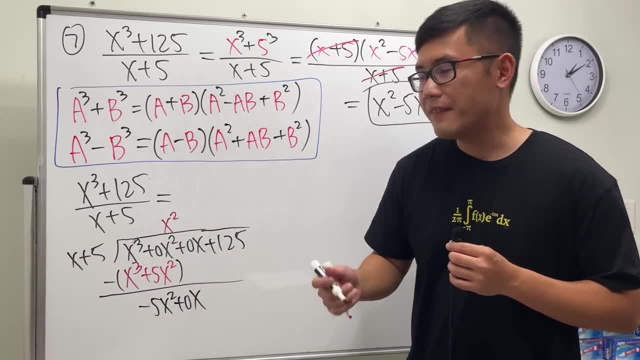 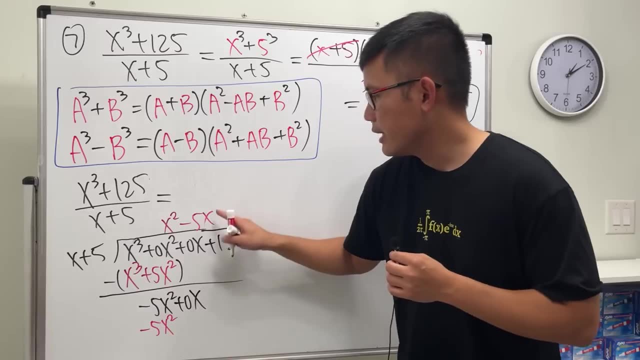 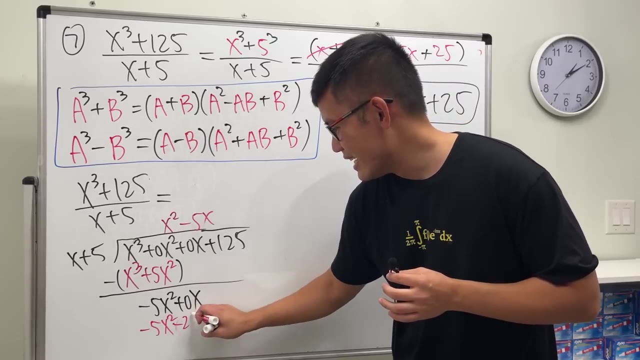 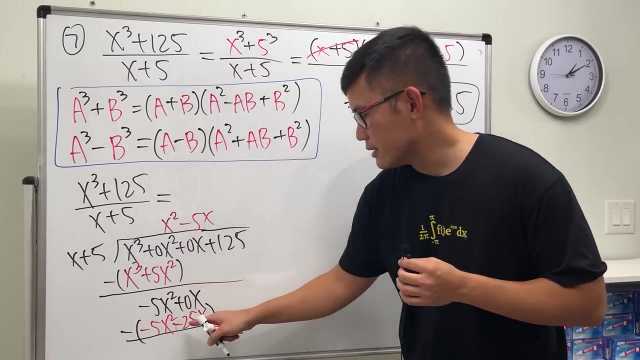 us negative five x squared. well, we need negative five x. so let's put on my negative five x right here. this times that gives us negative five x squared. this times that gives us plus no, minus 25 x. again subtract and we see this and that: cancel zero minus minus, become plus 25 x and bring down. 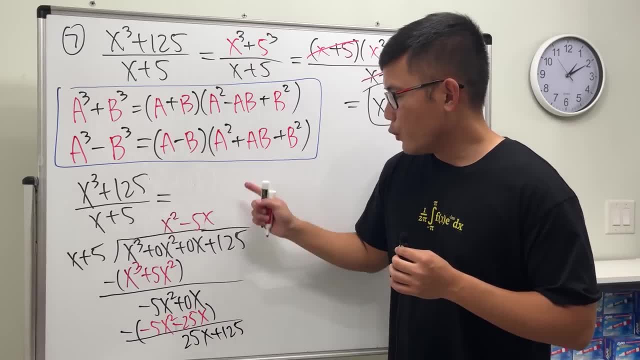 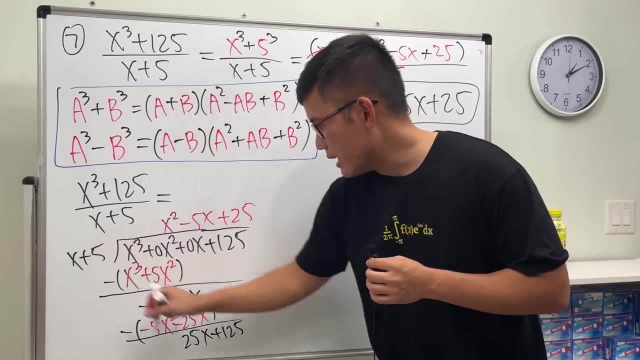 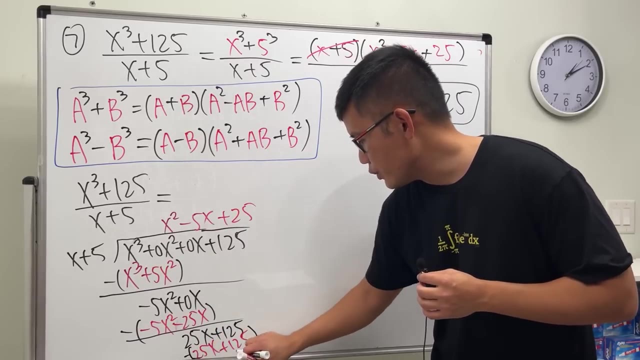 this 125. finally, what times x will give us 25 x? the answer is 25. so we add 25. so 25 times x is 25 x, and then 25 times 5 is 125, and you can see that when you subtract, the remainder is zero. this, right here, is the answer. so this is: 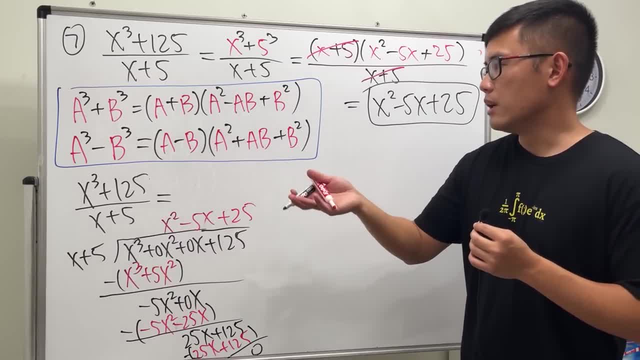 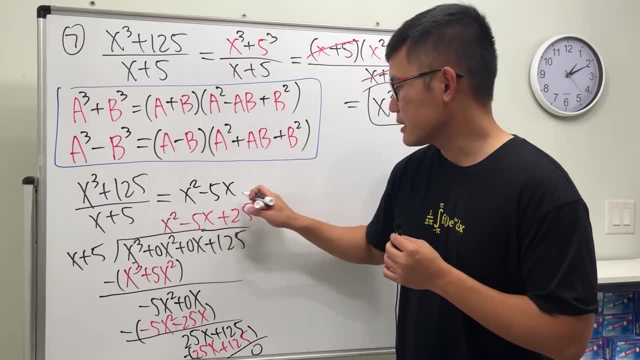 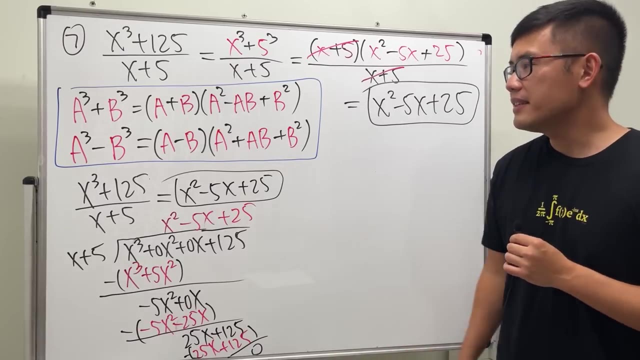 also another way to prove that- why the formula has to be like this. so the answer, of course: x squared minus 5x plus 25 long division. now let's take a look at synthetic division. I'll do this. one blue. when we have x plus 3, power plus 125. 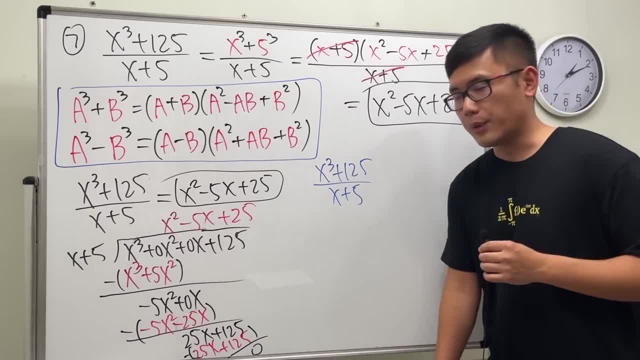 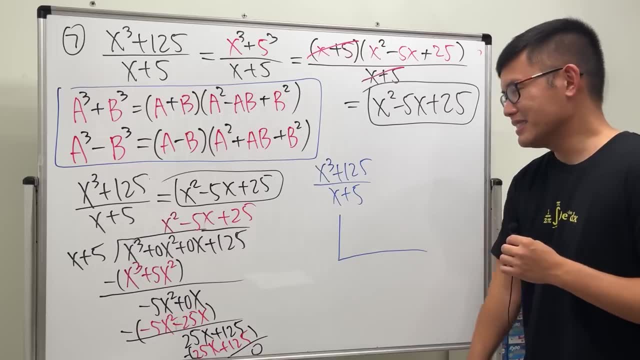 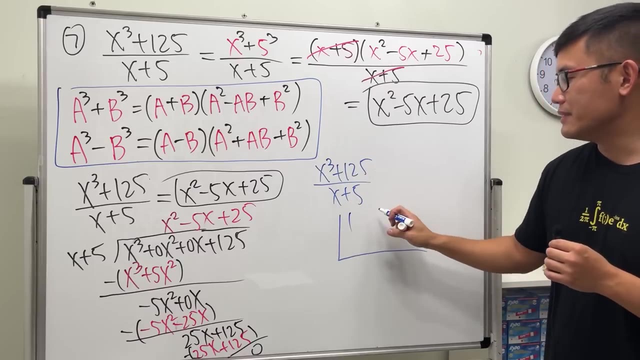 over x plus five. this is how we do. it depends on how you have seen it before, but usually I draw like a left corner, like this, and then you write down the coefficients of the numerator. so we have one, and then again we have zero x squared and we have zero x, and then, lastly, we have 125. 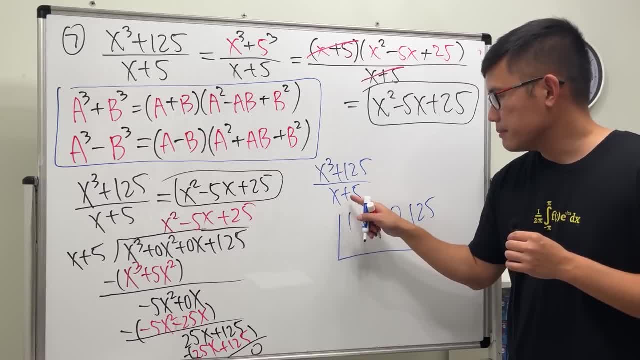 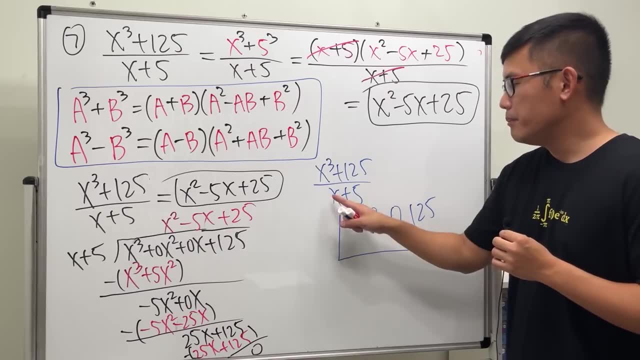 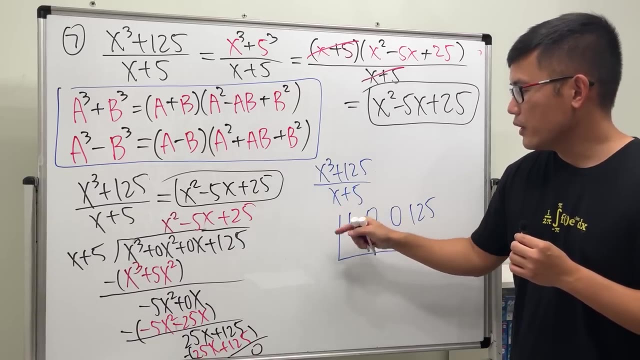 now, on the bottom, we have x plus five. in order for us to use long, in order for us to use synthetic division. this way, we have to make sure that we have a one, and this has to be x to the first power, which they are. so that's good, and if this is plus five, we are going to put on minus five here, the opposite and this: 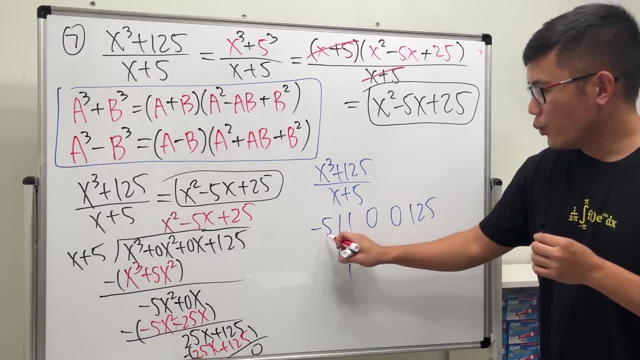 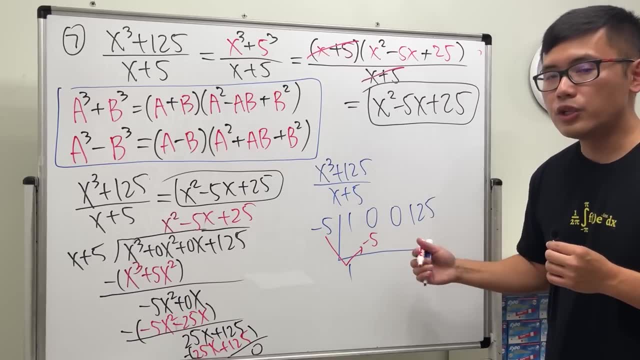 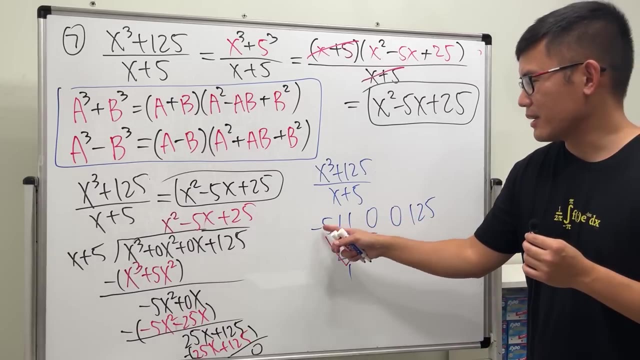 is how it works: first we bring down the one, and then we take negative five times one, which is negative five, and then we put it here and then for synthetic division we are going to add so, and you might be wondering why the? the reason is kind of like because we did the opposite, so 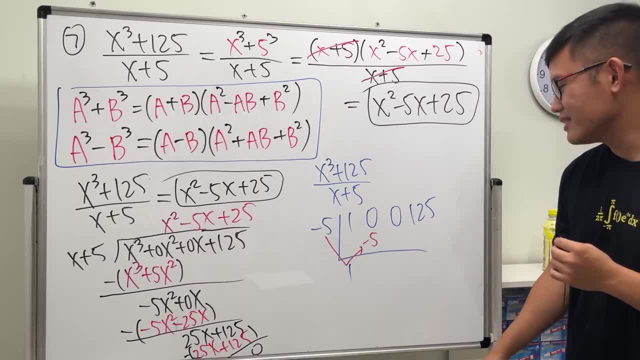 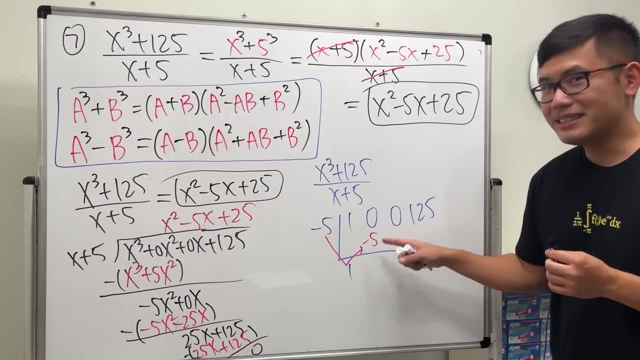 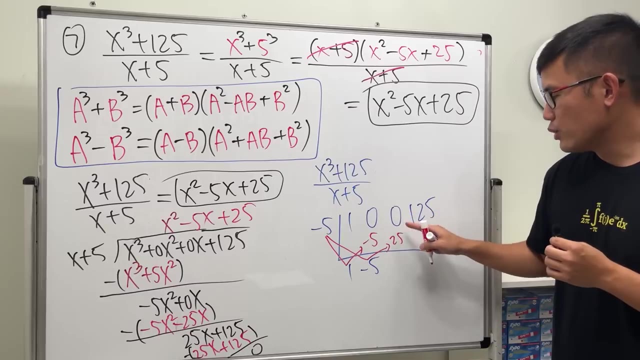 that's why you add okay. so that's one of the reasons. yeah, okay, anyway. this is just how how people do it anyway: zero plus negative five, we get negative five, and then just go and do it: negative five times negative five, we get 25, and then zero plus 25 is 25 and lastly, this times this: 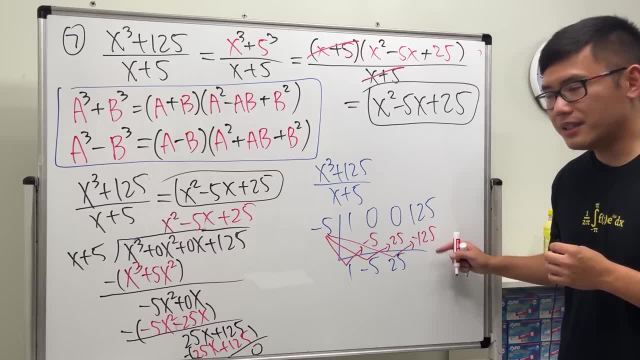 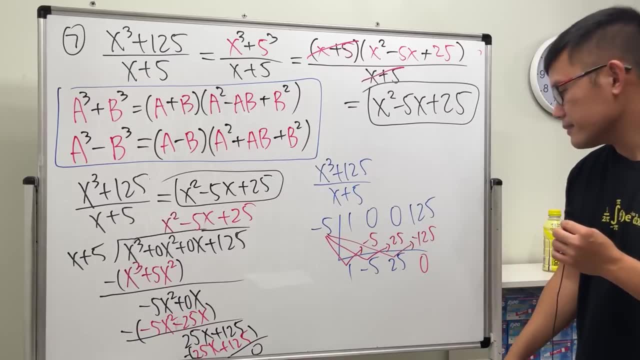 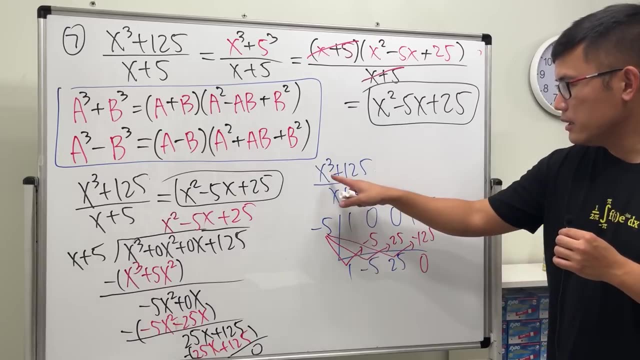 is negative, 125, together, we get zero. this is the remainder is zero. that means it goes into that evenly and this is how we are going to read the answer. these are the coefficients of the result, the quotient, and earlier we started with x plus third power. that means this right here: 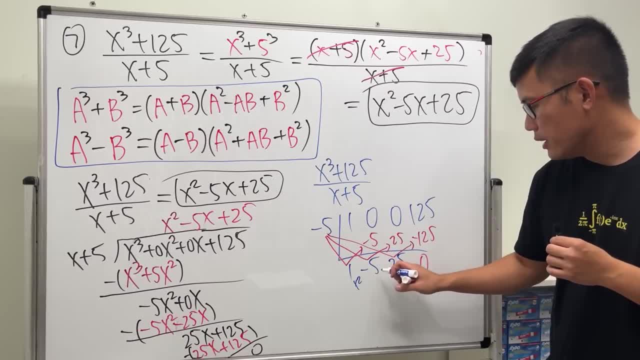 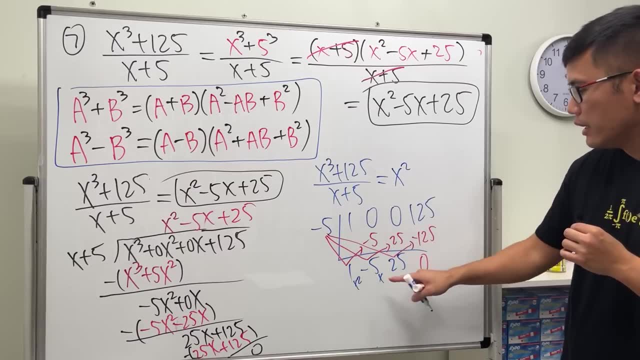 we go down by one power, so that will be x square x to the first and then no x. so this right here will give us 1x squared, which is just x squared, and then minus 5x and then, lastly, plus the constant 25. 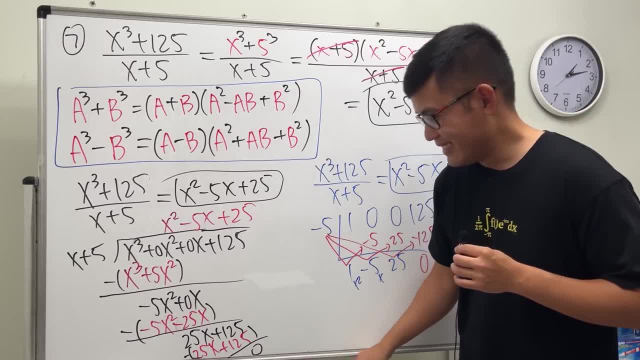 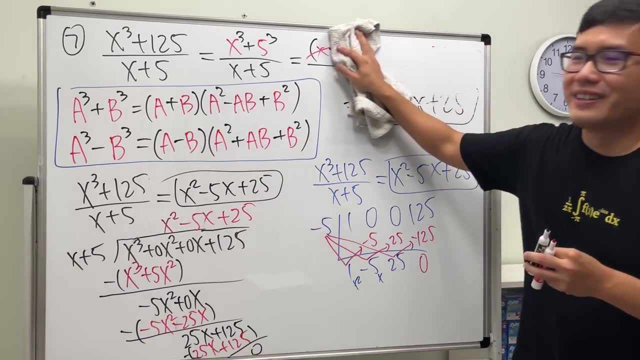 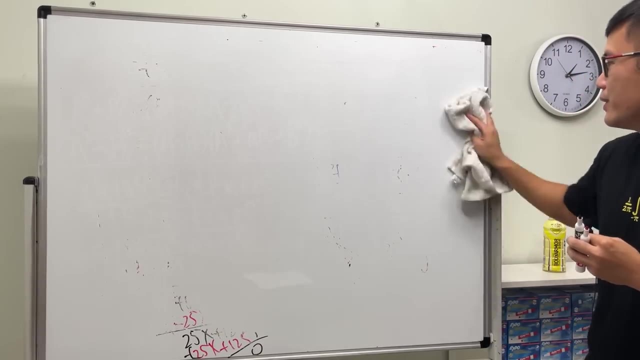 right. so three ways to do this question. so let me know which way you guys like the most. later on, whenever we can factor refactor, I will say: and then, for the long division with synthetic division, I just practice. maybe you'll use it here and there. that's excited. 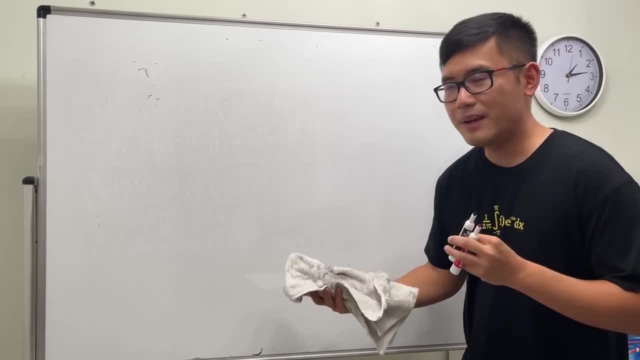 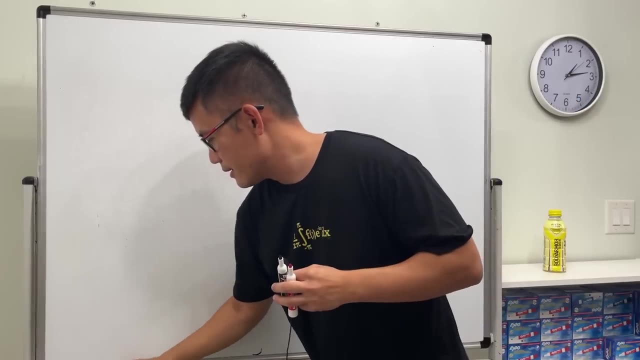 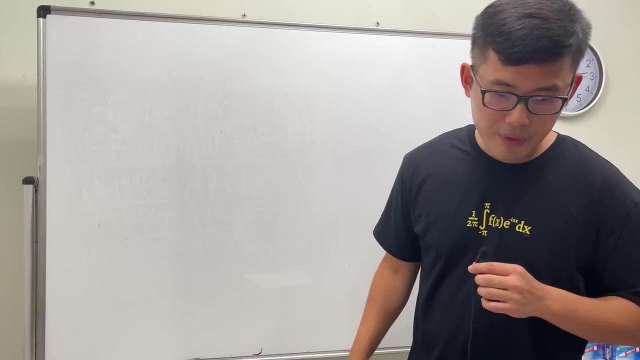 you guys want to take a guess right now if it's the 1: 15 am or 1: 15 pm, 14, actually 113, I don't care. all right, number eight: we are looking at x to the third power minus 27. 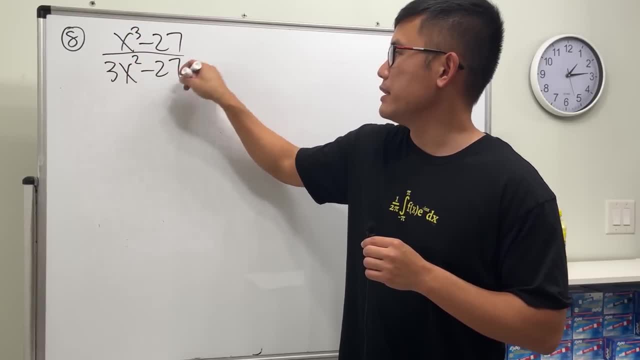 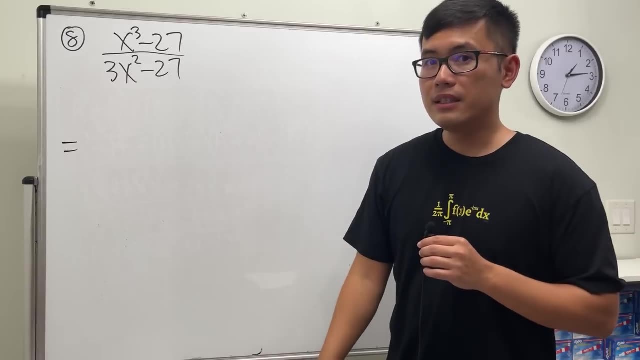 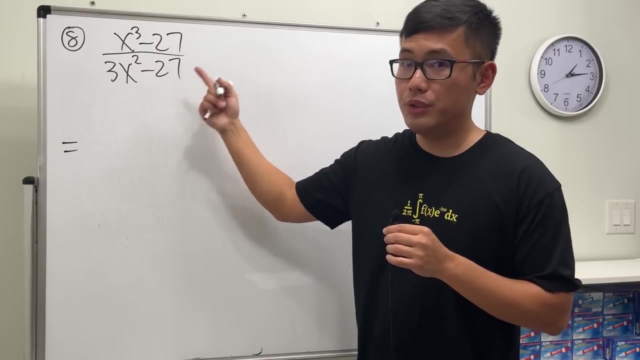 over 3x squared minus 27.. okay, let's go ahead and get started on the top right here it's a difference of two cubes. So let's recall the formula. This is x to the third power minus 3 to the third power. 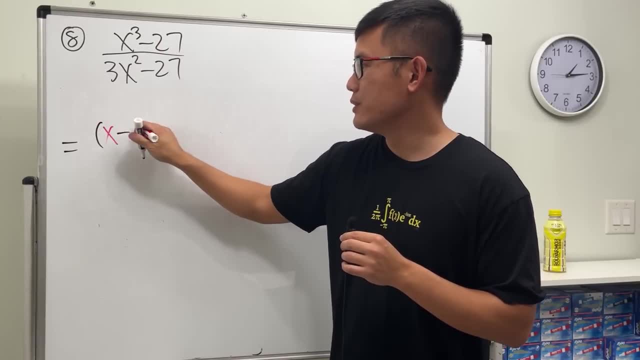 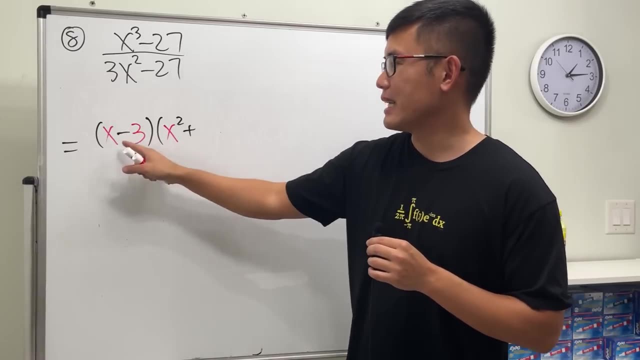 So we are going to get x minus 3.. And then multiply by x squared plus ab right, Just this times- that, which is 3x, And then, lastly, we add this squared, which is 9.. 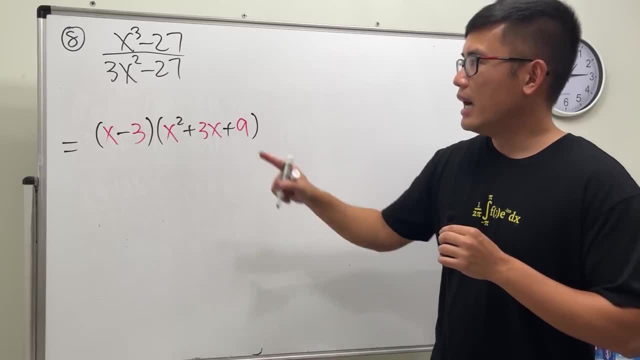 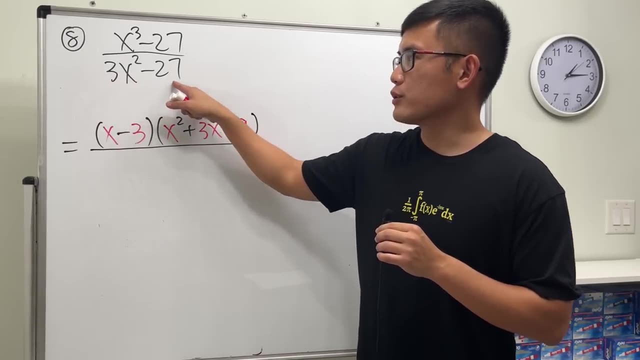 So this right here is the factoring for that On the bottom. this is not difference of 2 squared yet Because, notice, we have 3 here and also 27 here. We can actually factor out a 3 first. 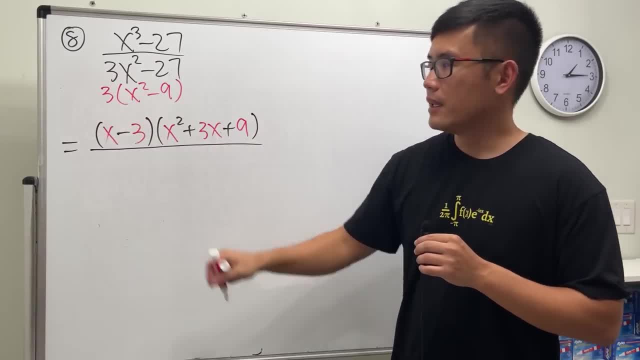 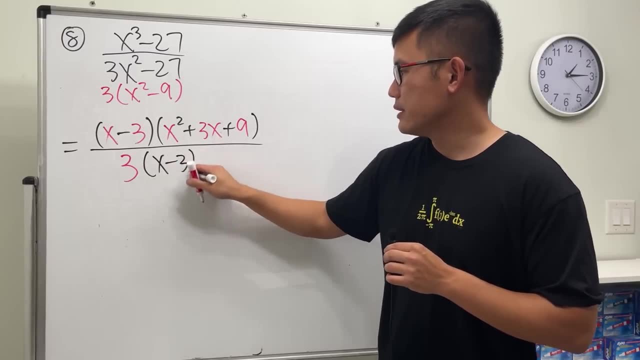 And then we get x squared minus 9.. So let's put down this 3.. And then x squared minus 9.. Well, that's going to be x minus 3 times x plus 3.. So that's the factoring. 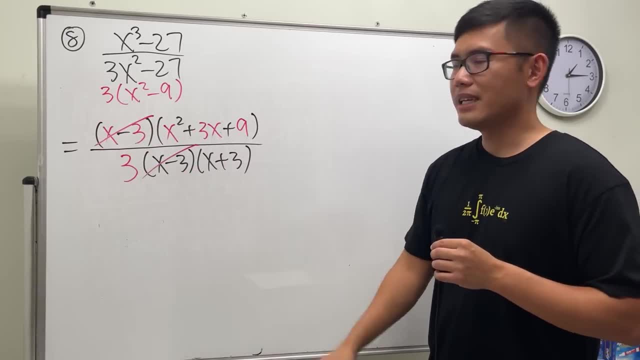 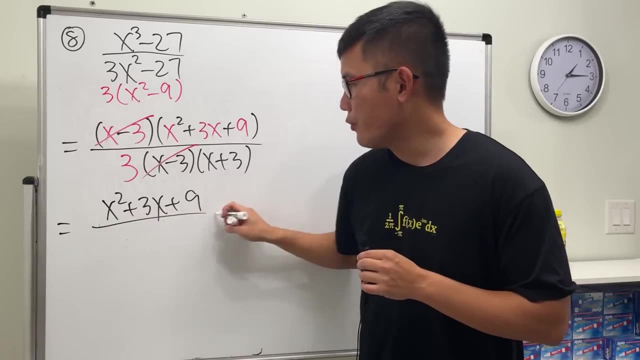 And then we see this and that can cancel. That's it. So finally, we just write down the answer. We have x squared plus 3x plus 9 over 3 times x plus 3. And then we are done. 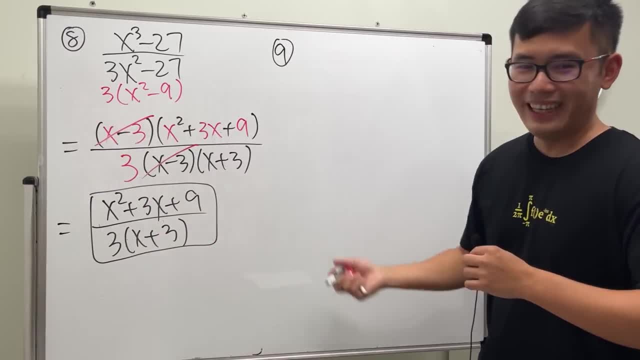 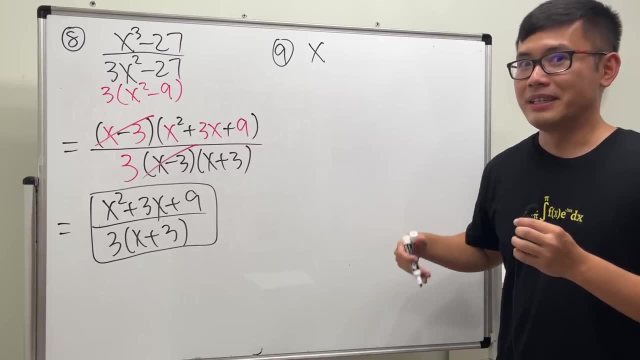 Yeah, Don't you guys just love algebra? Yeah, Okay, Number 9.. And, by the way, a lot of these questions are actually based on calculus questions. I just took away all the calculus languages and then focused on algebra. All right. 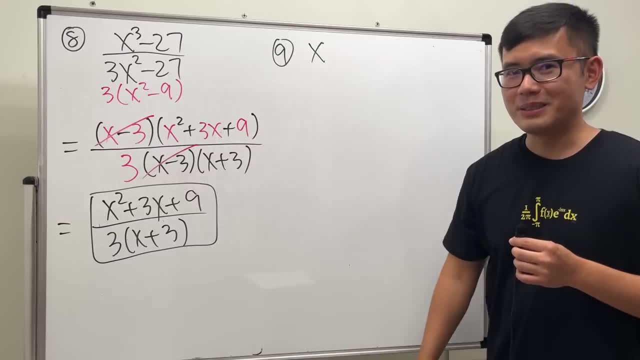 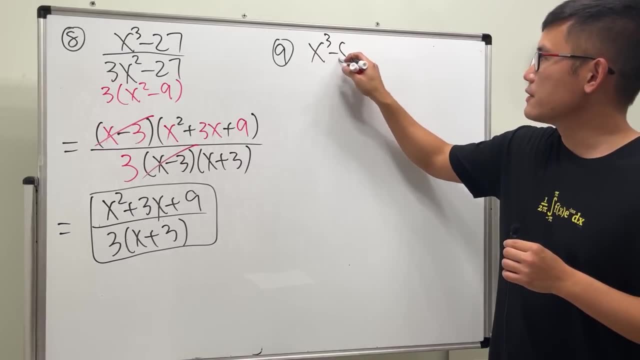 So they tell: when you study like limits, you will see things like this. So I'm going to show you how to factor and cancel: Yeah, Number 9.. Let's look at x to the third power minus 5x plus 2 over x minus 2.. 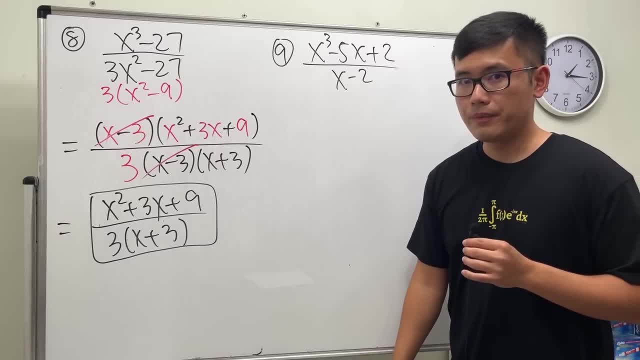 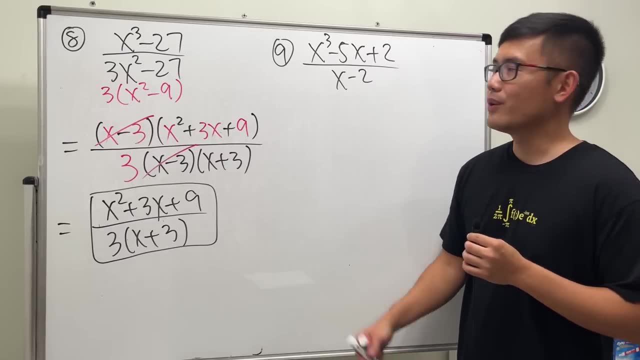 Unfortunately, the top right here. it's not easily factorable. It's not easy to factor. It's factorable, of course, but it's not easy to do that. So what do we do? Well, notice that on the bottom we just have 1x to the first power, minus 2.. 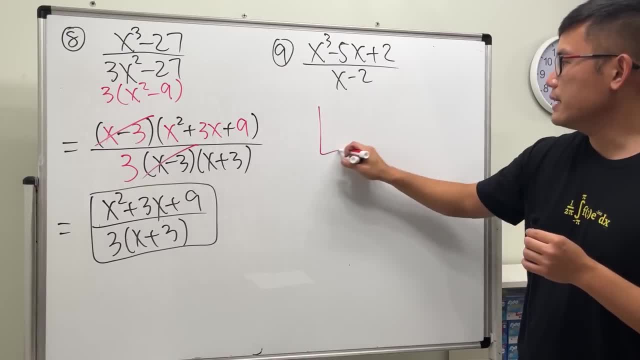 So we can use the synthetic division. So let's go ahead. Let's go ahead and do that. Write down the coefficients. We have 1, 0x squared, so we put down 0, and then this is negative 5, and then we have. 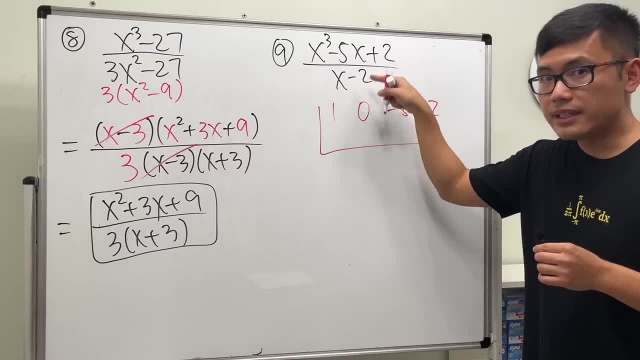 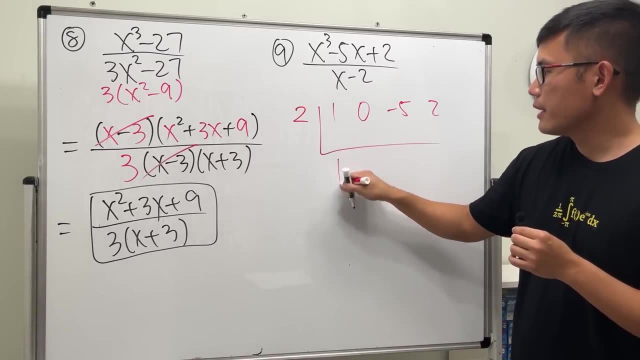 2, and then this is x minus 2.. Look at the negative 2. We do the opposite, which is positive, 2.. Now synthetic division action: Put down the 1, and then we do this times that which is 2, and then we add 0 plus 2. 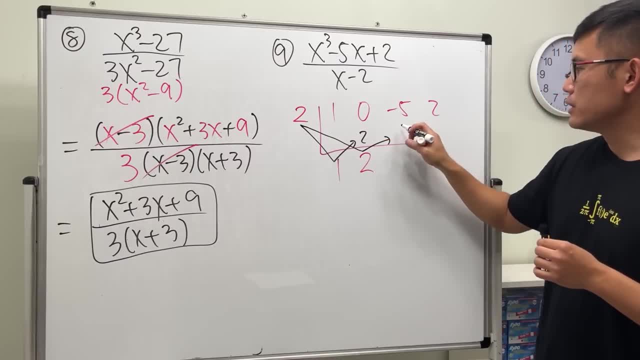 is 2, and then we do it again: 2 times 2 is 4.. So this times that this plus that is negative 1, and then this times that is negative 2.. Put it here Together we get 0.. 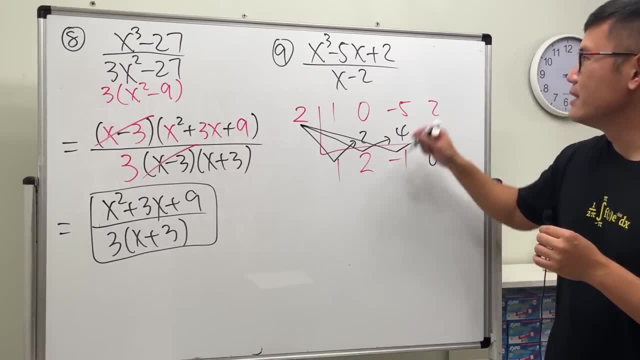 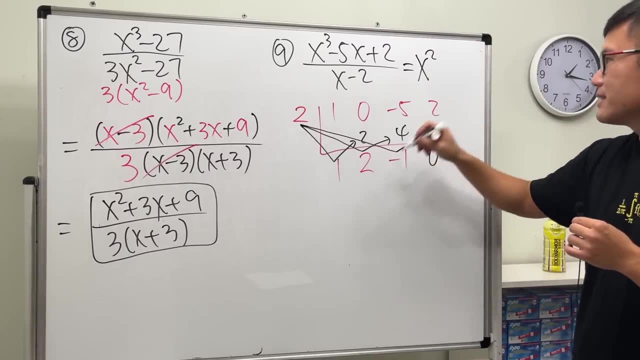 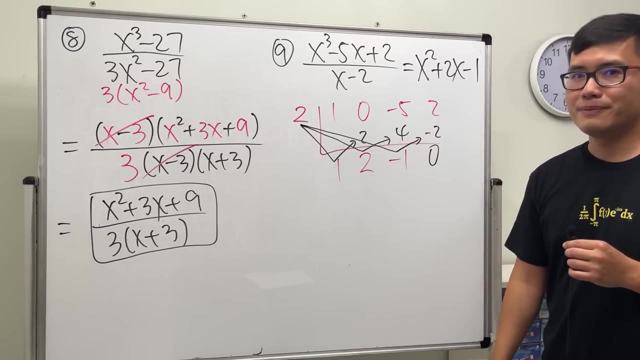 Ladies and gentlemen, this right here is x squared, because earlier it was x plus third power. So x squared minus, sorry, plus x plus 2x and then minus 1.. Take a look, right here Can we factor it? 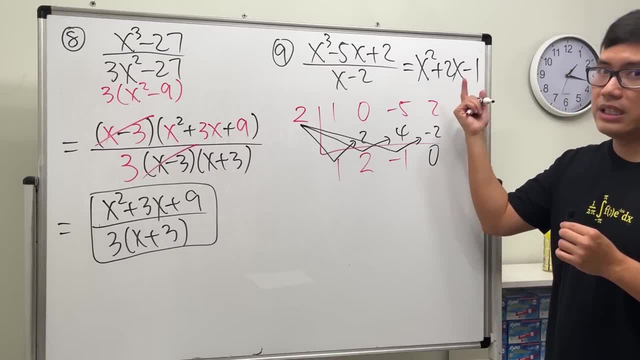 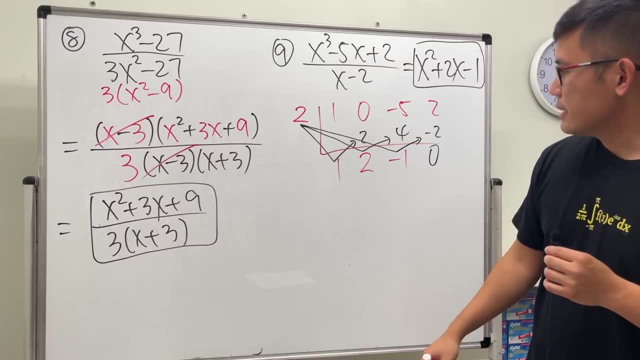 No, This is a minus 1.. If it was a plus 1, then, yes, You can factor it, but right here, no, This is it Okay, Leave it like that. Cool, All right, Number 10.. 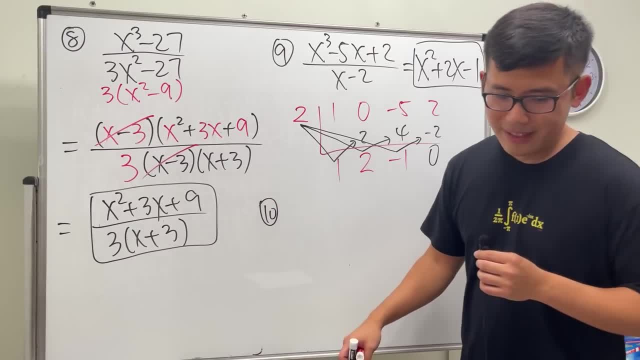 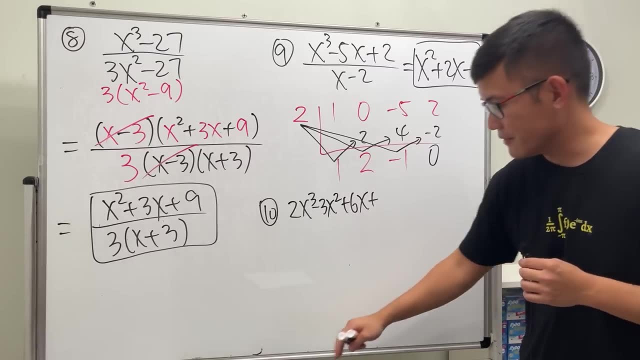 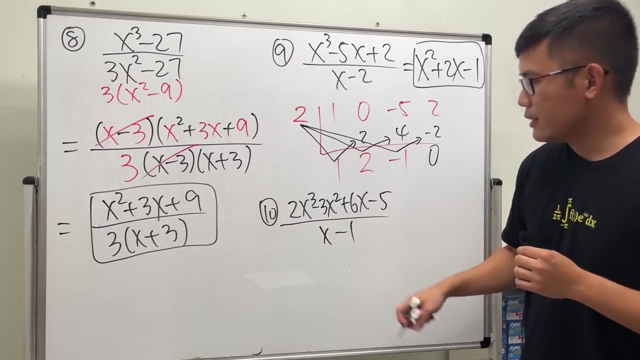 I'm going to fit in number 10 right here as well. Here we have 2x to the third power minus 3x, squared plus 6x minus 5, and then over x minus 1.. So similar thing. Just use the synthetic division. 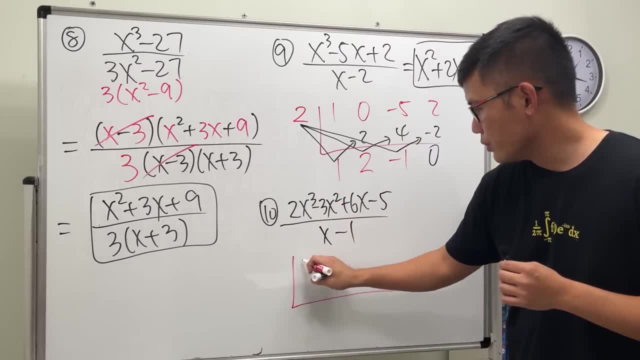 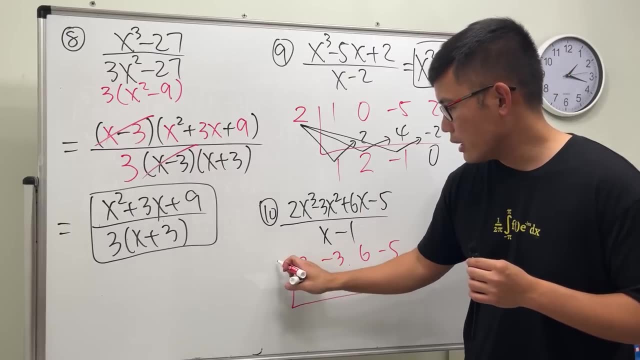 Here we go. We have 2, negative 3,, 6, and negative 5.. This is x minus 1, so we do positive 1 on the outside here. Okay, Put down the 2.. This times, this is 2.. 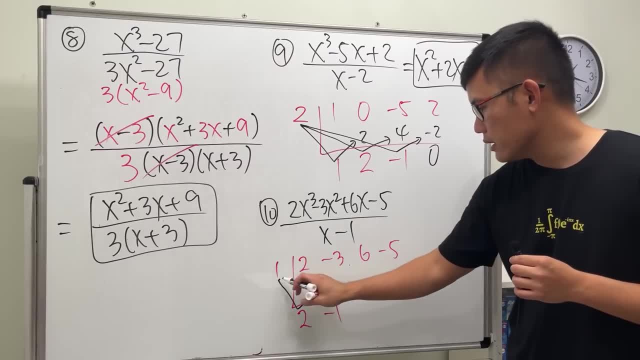 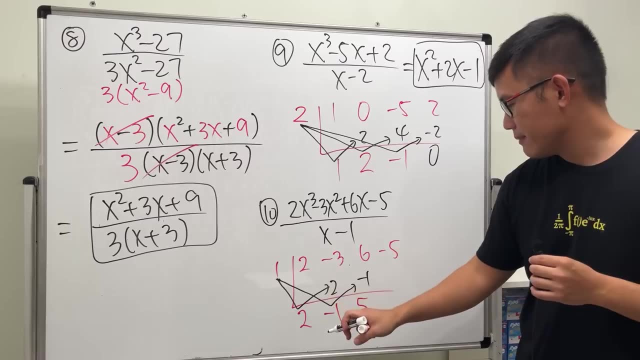 Put it here: This plus that is negative: 1.. Okay, This times this is negative: 1.. This and that together is positive 5.. Yes, And then this times, this is positive: 5.. Together negative: 1. Together we get remainder 0.. 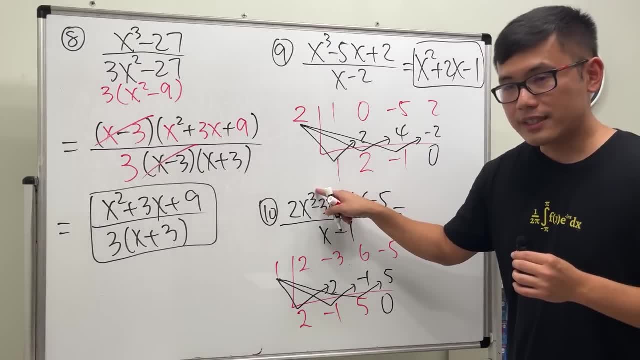 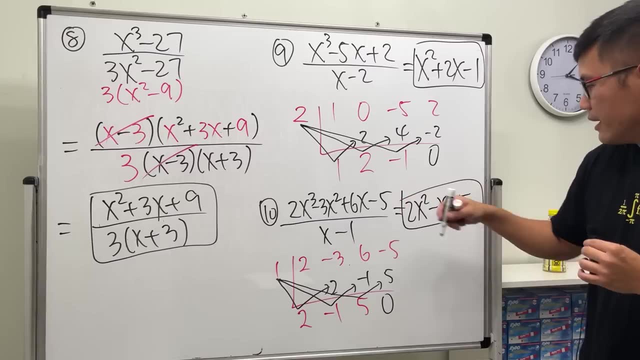 So this right here started with x cubed. That means this: right here is x squared term right, So 2x squared minus x plus 5.. Can we factor this? No, because I boxed the answer already. No, I'm just kidding. 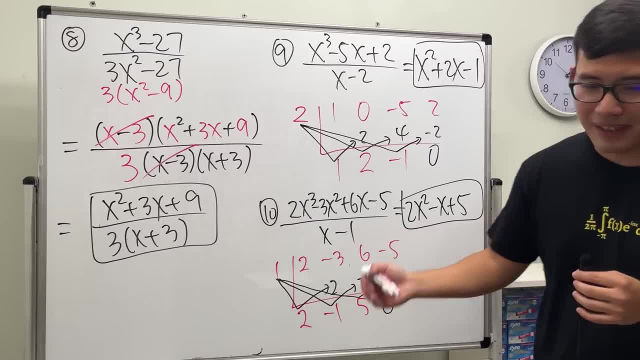 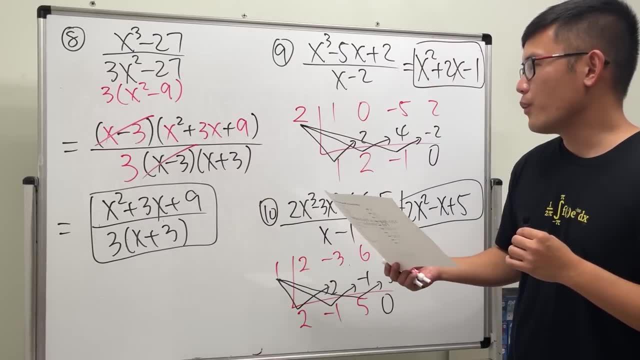 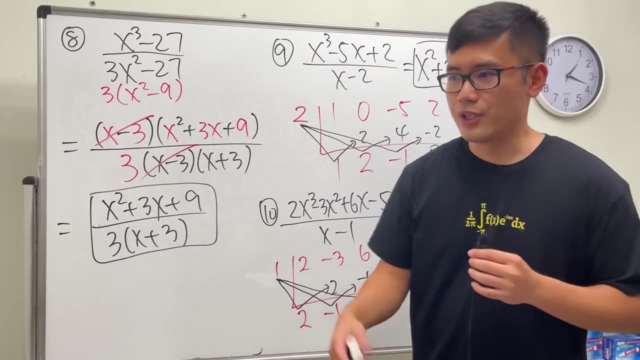 Of course, But it's really not factorable. That's why I just boxed this. Okay, Cool. So definitely you know how to factor and do long division or synthetic division. And, of course, if you guys need more help with factoring, you guys can check out my other. 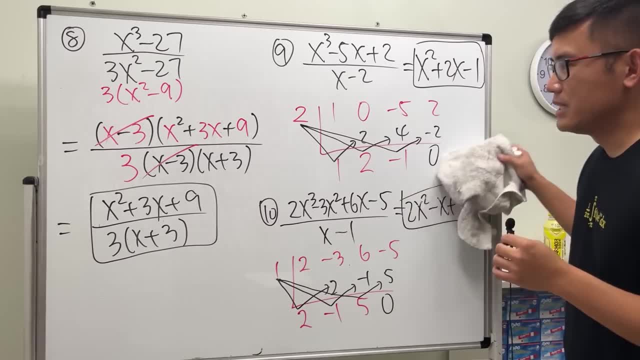 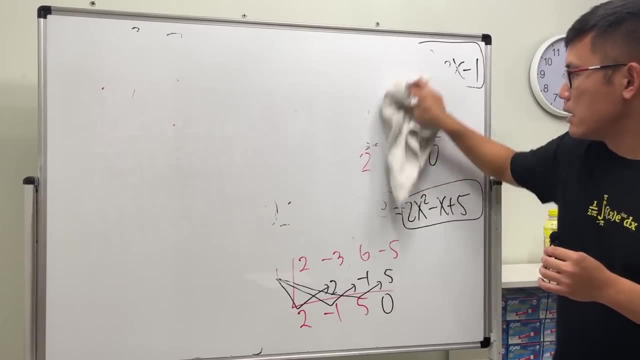 videos, or just leave a comment down below and let me know if there's any specific type of algebra problems that you guys would like to see. All right, I know How about the trick. I told you guys I will also work out the 100 trick. 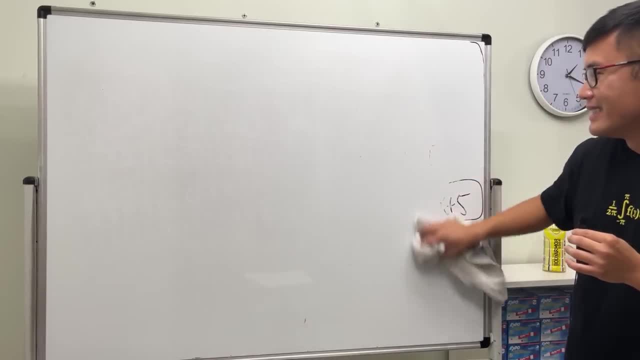 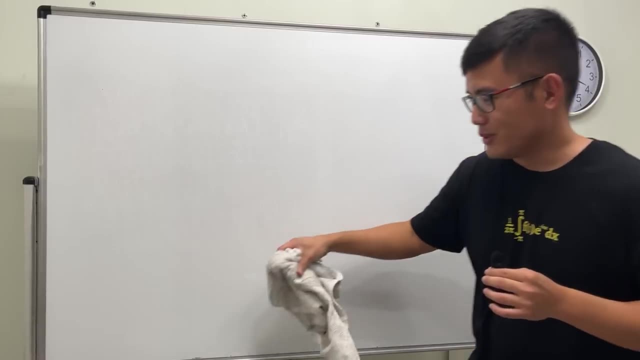 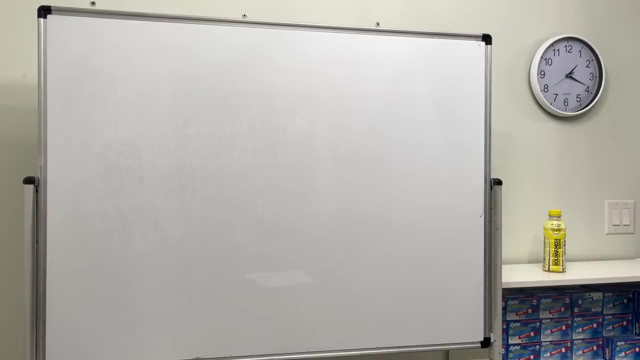 I don't know if I can actually come up with the 100 trick problems though, So it may take me a while. I will try my best to actually come up with them as soon as possible for you guys. Okay, So let me just take a look. 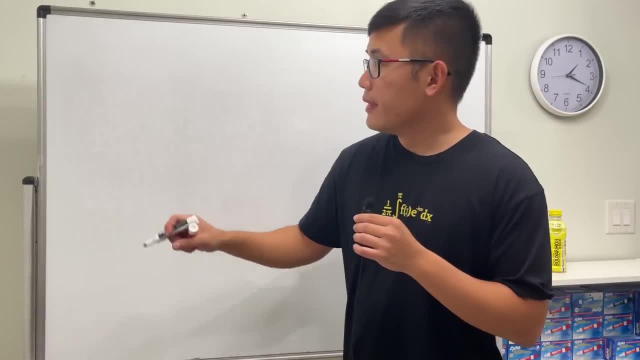 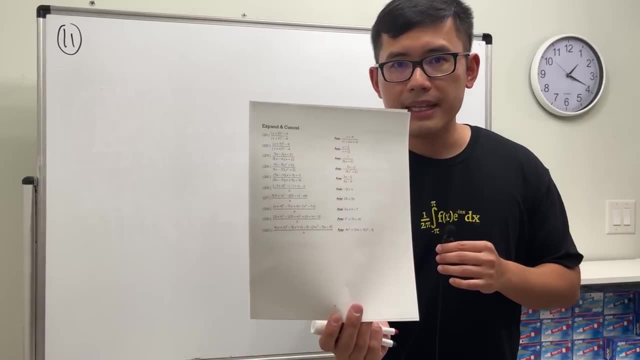 Good, Okay, Number 11.. Okay, From number 11 to number 20, we are going to talk about expand and cancel. So instead of factoring, we will actually focus on multiply things out, And then I'll tell you, guys, what are the things that we should keep in mind. 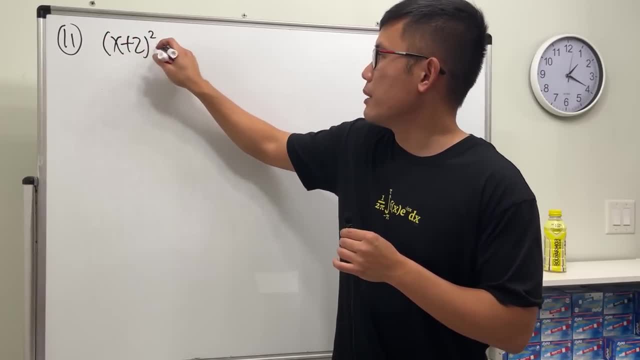 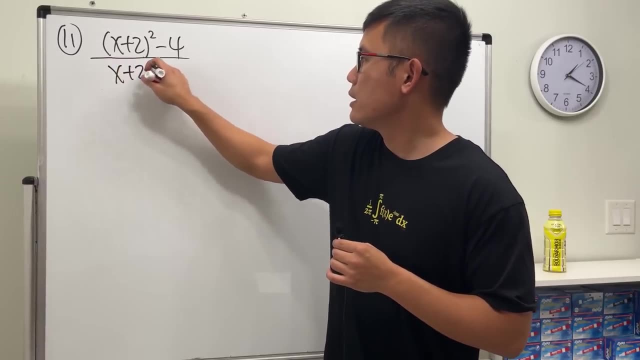 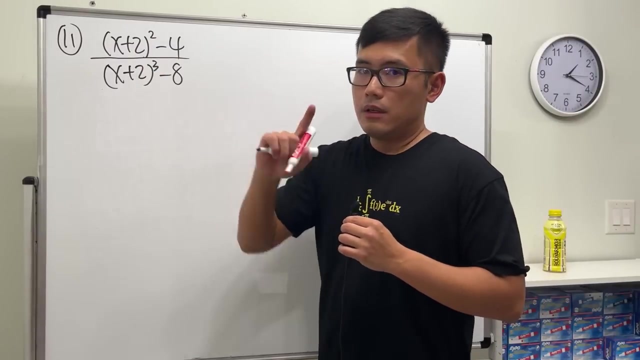 Okay, First one x plus 2, square minus 4 over x plus 2 to the third, power minus 8.. All right, So again expand and cancel. Here is a common mistake A lot of students when they see the x plus 2 in the parentheses right here on the top. 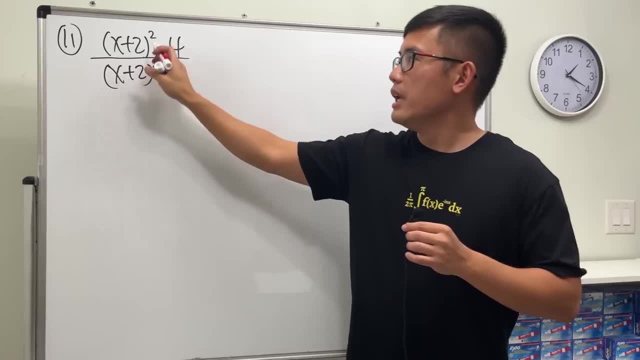 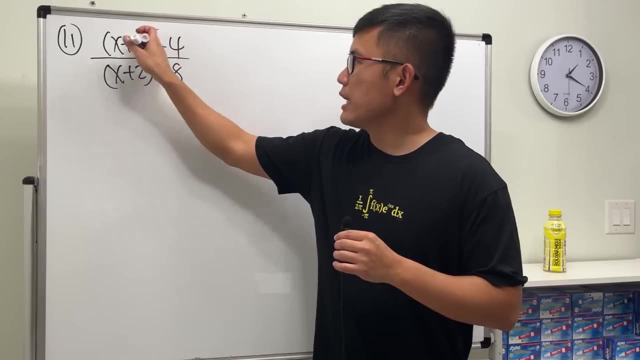 and then on the bottom we also have the x plus 2 in the parentheses. right, They will just cancel this and that That's not correct. All right, So let me show you what I mean If you just cancel this and that this is wrong. 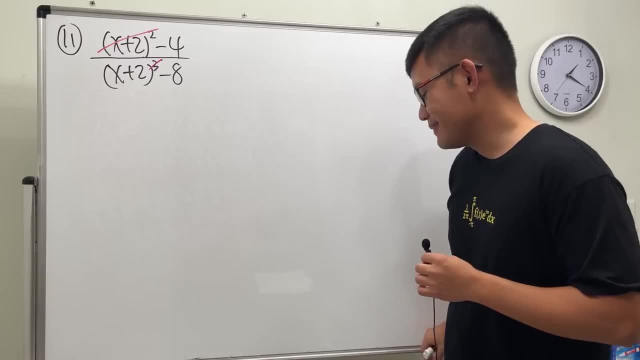 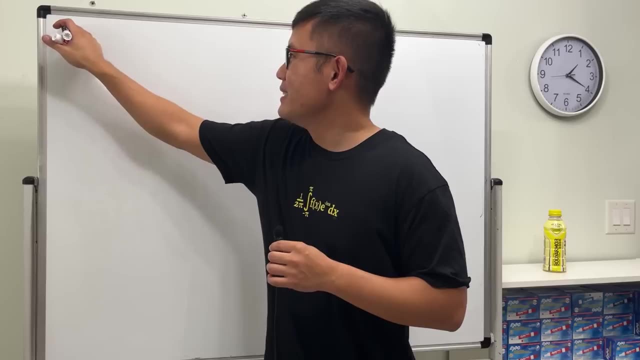 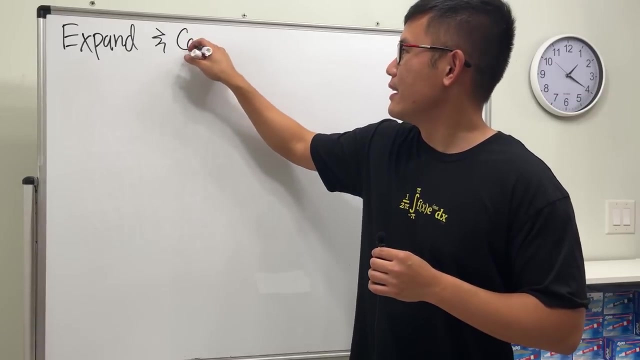 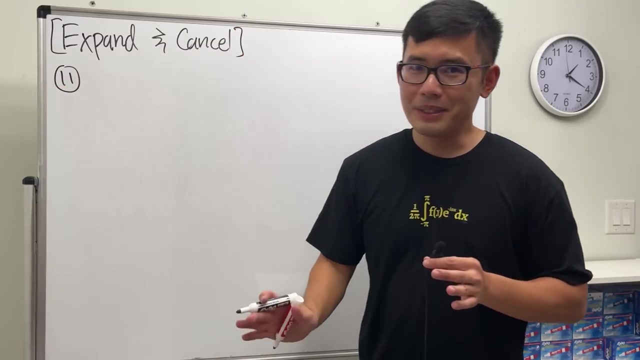 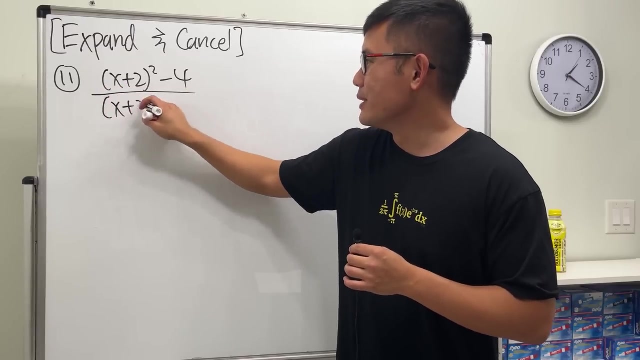 This is wrong. This is I. Yeah, Just don't do that, No, Okay. So for number 11,, this is: expand and cancel. All right, Now number 11,: x plus 2 square minus 4 over x plus 2 to the third power minus 8.. 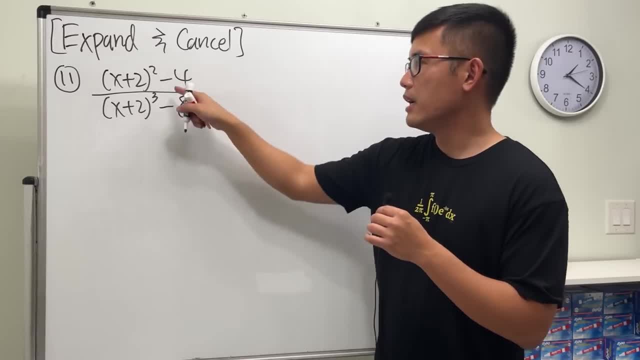 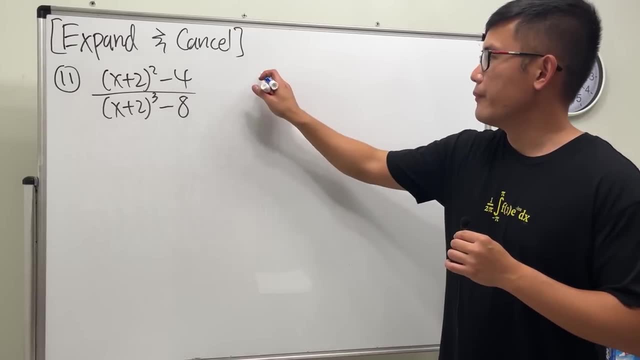 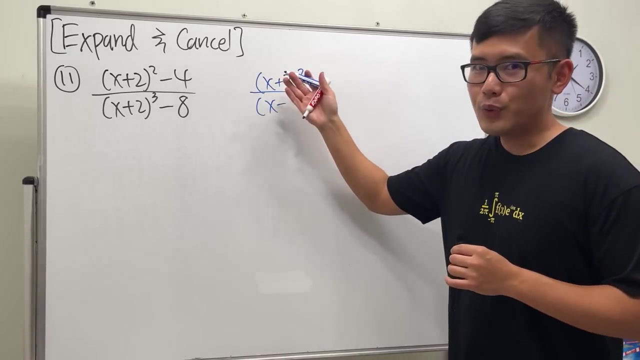 Do not cancel this and that. The reason is because at the end here we still have the minus 4 and also the minus 8.. If the question was this: x minus 2 square over x plus, Sorry. If the question was x minus 2 square over x plus 2 to the third power, you see there's. 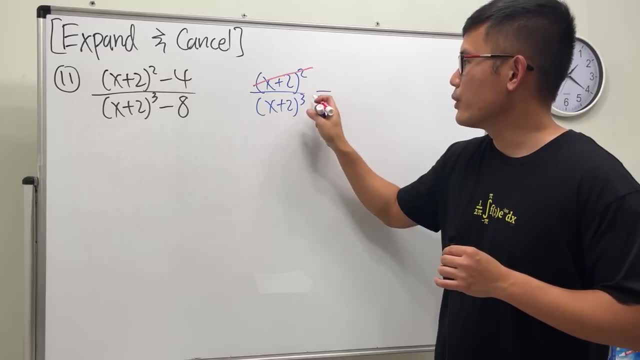 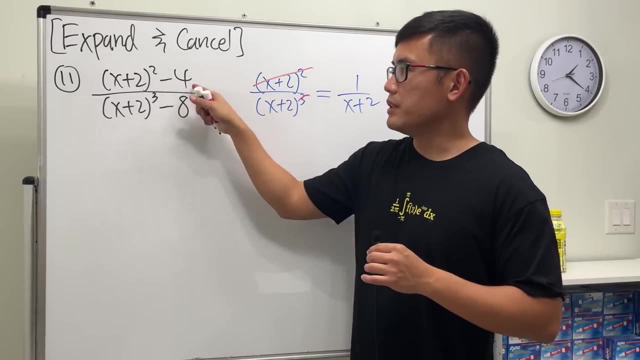 nothing else. Nothing else In this case. yes, we can cancel. cancel and say it's 1 over x plus 2. This is okay, But because of this and that we actually have to multiply things out and then combine, 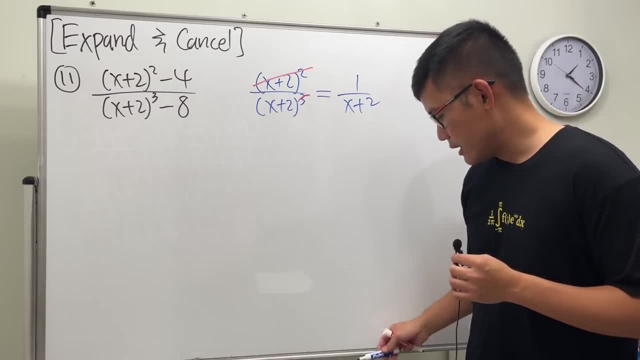 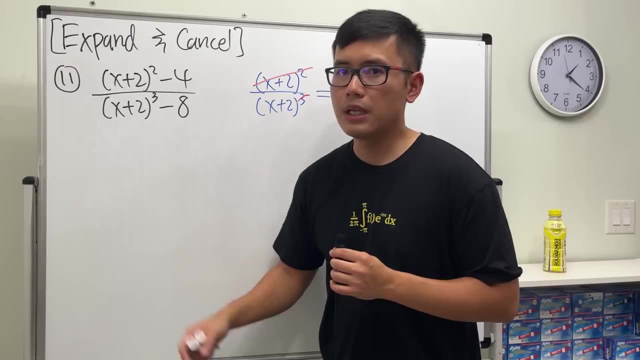 terms and then see if there's anything we can factor and then cancel. Notice This: right here is actually a difference of two squares and the bottom here is actually the difference of two cubes. but I find it's more straightforward if you just multiply things. 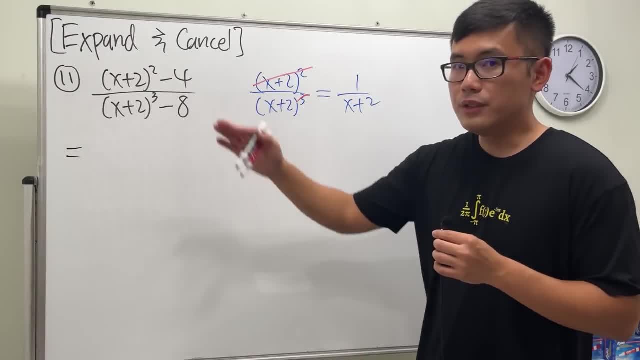 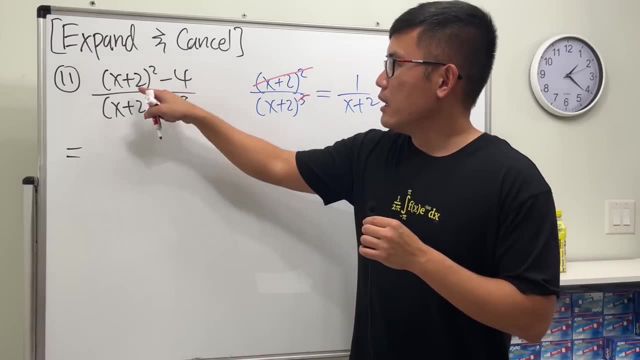 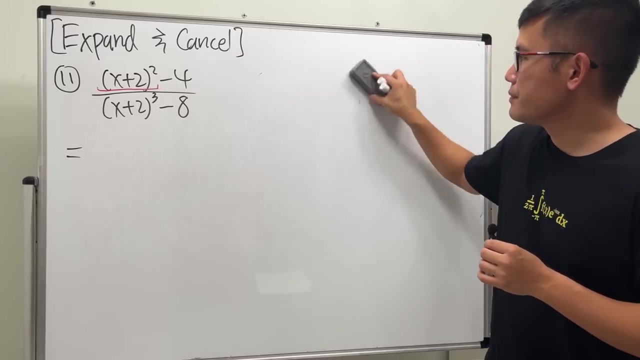 out and then combine and all that. So, even though you can actually factor them and then cancel, but let's just multiply things out and combine terms and then factor. Anyway, right here we have x plus 2 square, First formula that you should know. 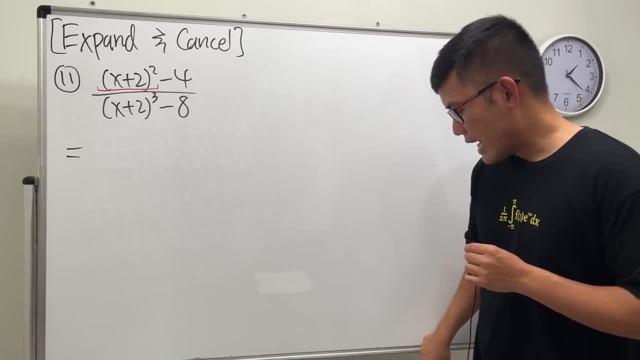 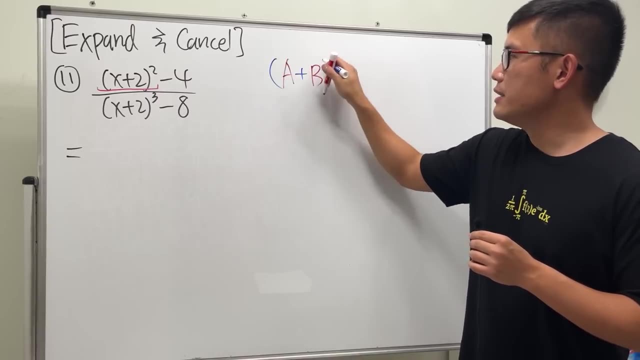 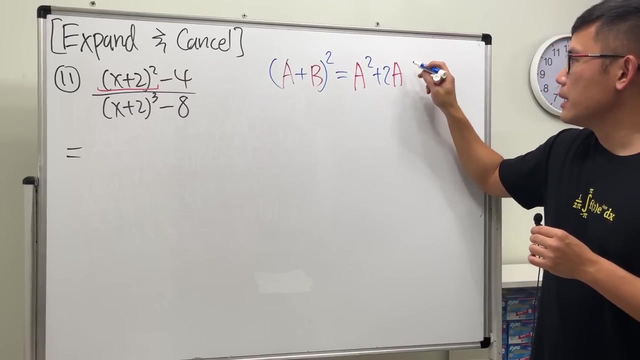 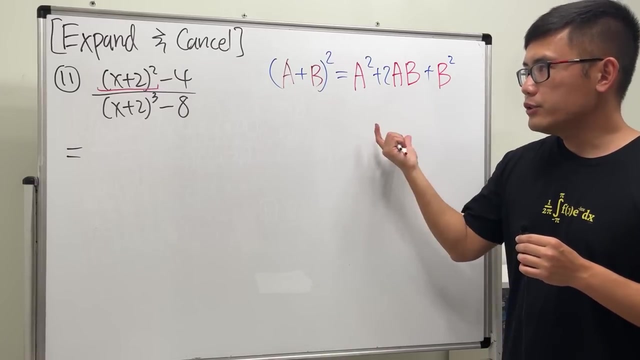 Definitely Okay. So whenever we have a binomial square, namely a plus b, if we have this square, this right here, we get a square plus 2ab plus b square, All right. So we are just going to be using this kind of formulas in our head to multiply things. 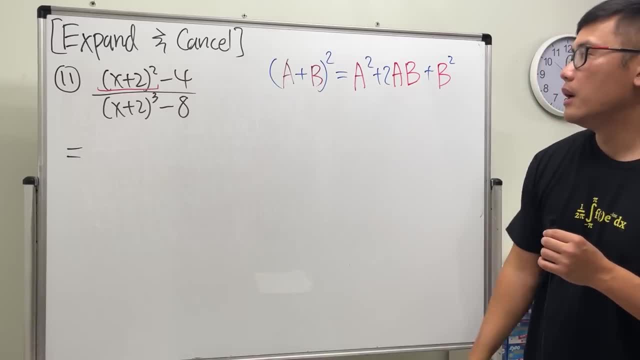 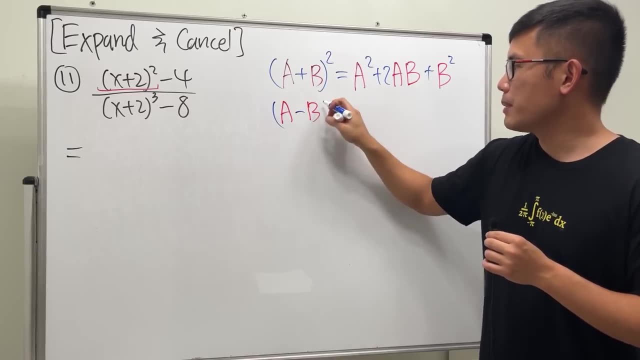 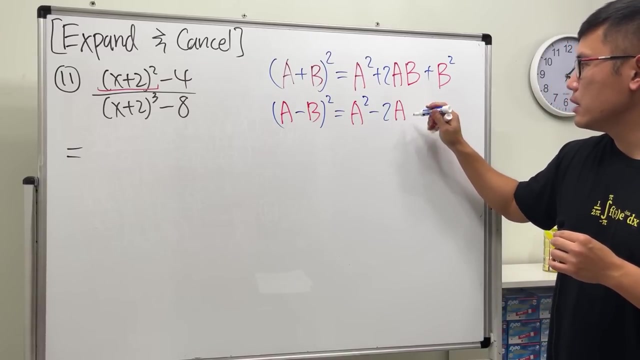 out. Just make sure that you have that middle term. And also let me write down the minus version. If we have a minus b to the second power, this right here is equal to a square minus 2ab and then plus b square. 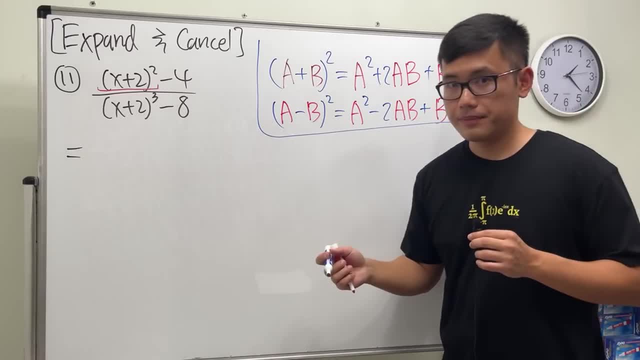 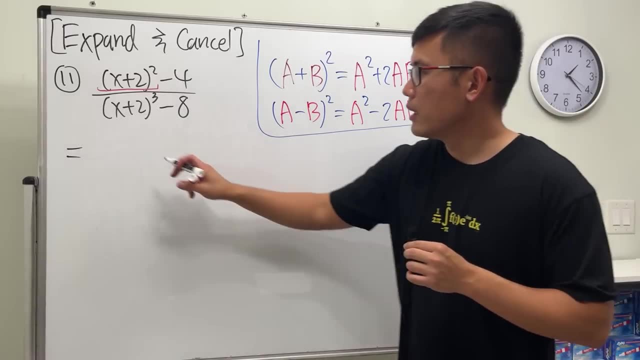 So this is how we multiply out these two things. So, with that being said, let's just work that out of the first part here. So notice: x plus 2 square. So we first square the x, So we have x square. 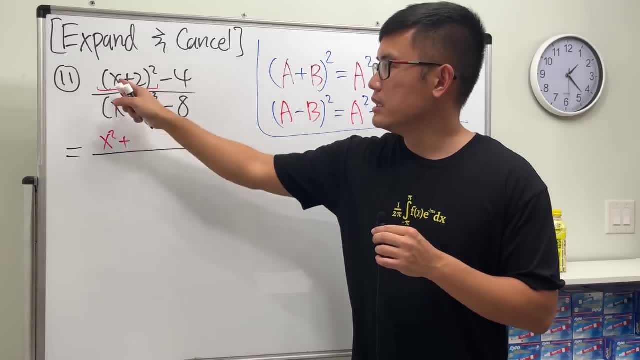 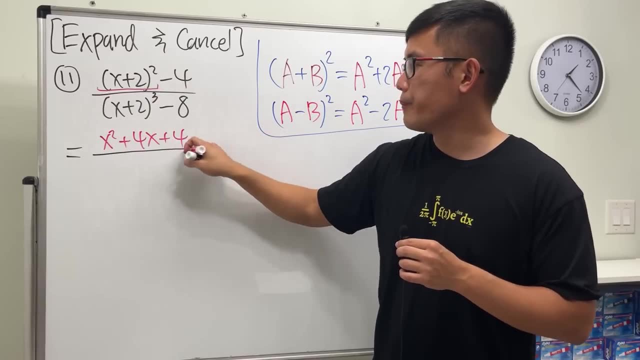 And then we add two times this and that which is going to be 4x, And lastly, we have the 2 square, which is 4.. And then, right here, we still have the minus 4.. So that's the top. 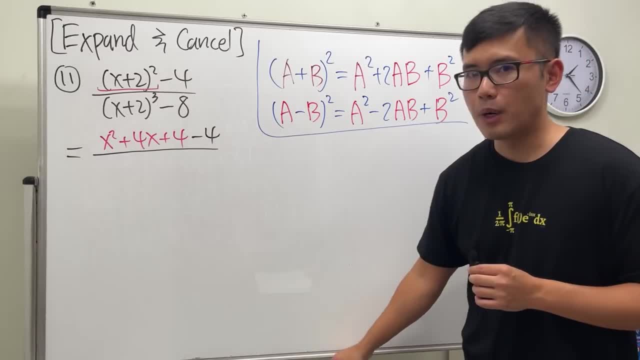 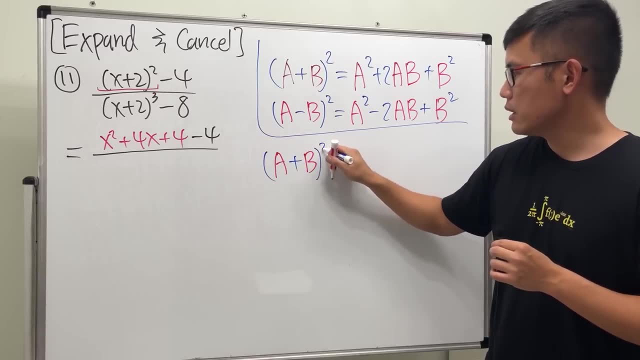 On the bottom we have the third power. I will also give you guys a third power version. The third power version says: if we have a plus b, If we have a plus b to the third power, the coefficients are 1,, 3,, 3, 1, because that's. 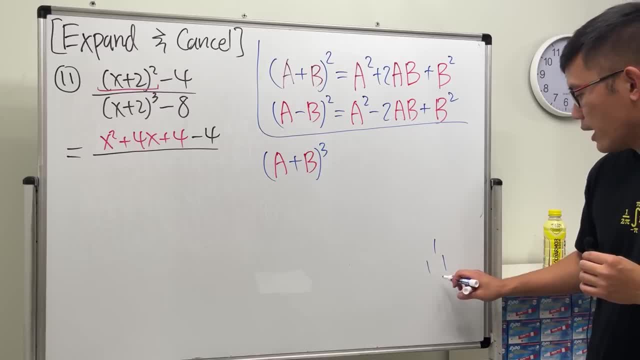 from the Pascal's triangle: 1, 1, 1, 1, 2, 1, 1, 3, 3, 1, 1, 4, 6, 4, 1, etc. 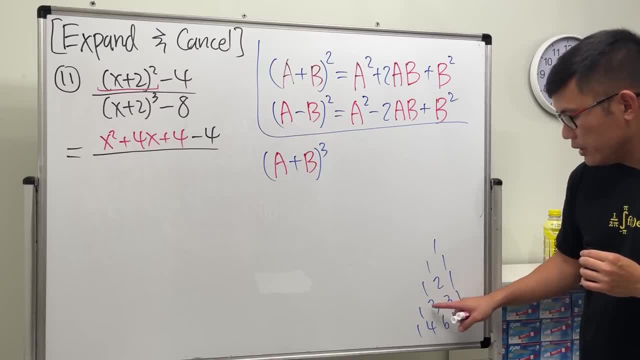 How did we get these numbers? Well, if you look at the 3,, it's because 1 plus 2 is equal to 3.. How did we get the 6?? It's because you look up to the previous row and you just do this plus that and you get. 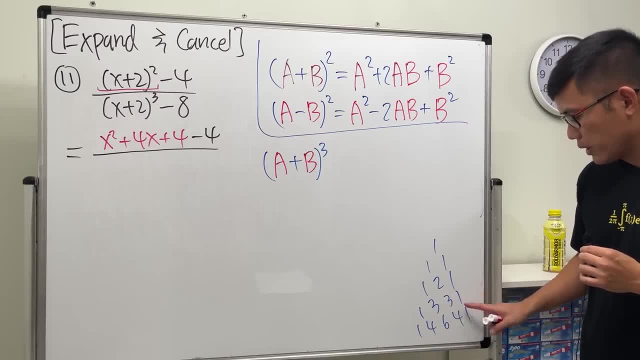 6. How did we get the 4?? 3 plus 1 is equal to 4,, etc. etc. So when we have a plus b to the third power, we look at this row. This is technically the 0th row. 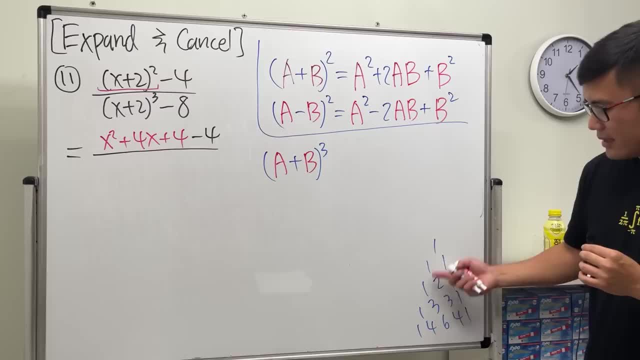 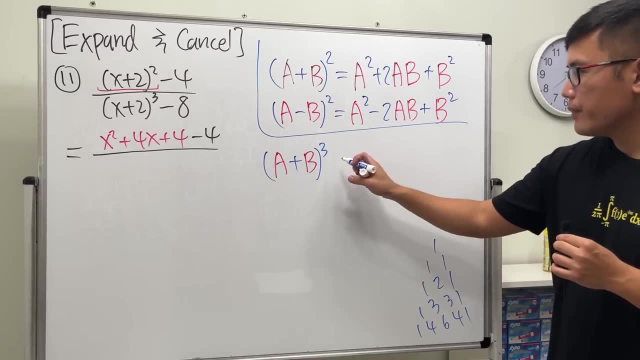 So this is the third row. Sorry, yeah, the third row: 0, 1,, 2,, 3, because this is actually corresponding to the third power. So, right here, all we can do is just remember 1 times a to the third power. 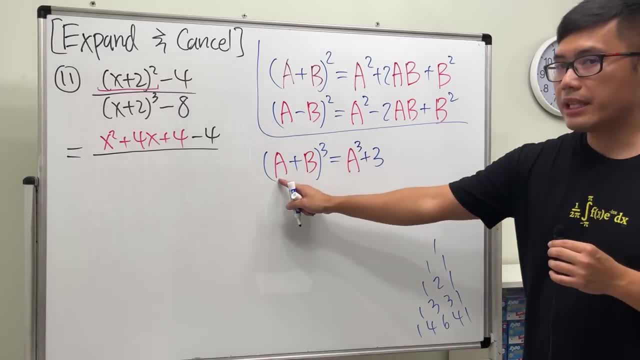 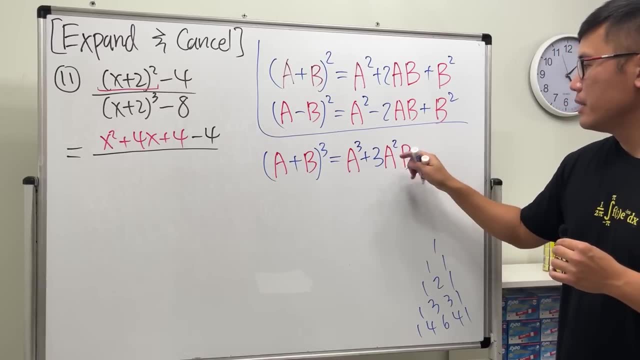 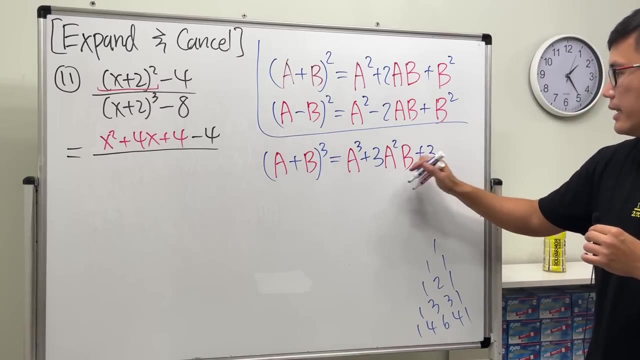 And then we add 3, and then right here we have a- the power goes down by 1, but introduce the b, because the powers together they have to add up to 3.. Next 3, and then a- the power goes down by 1, but introduce another b, so b squared. 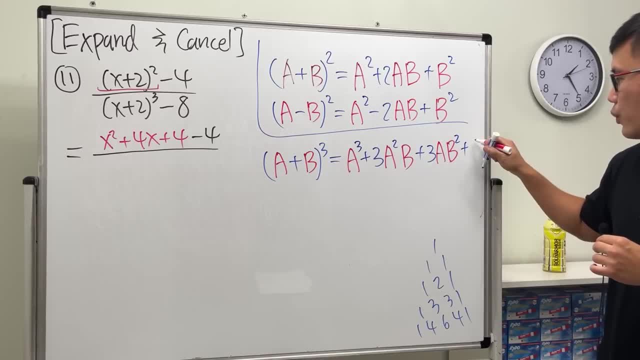 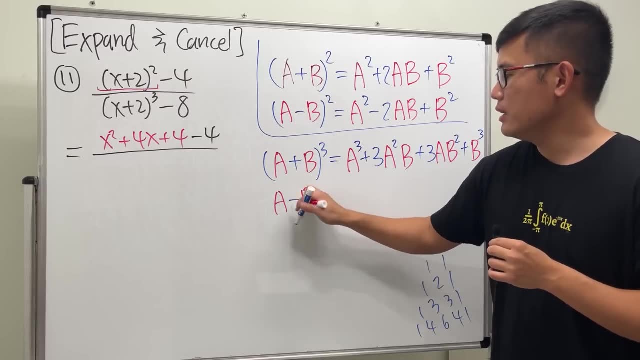 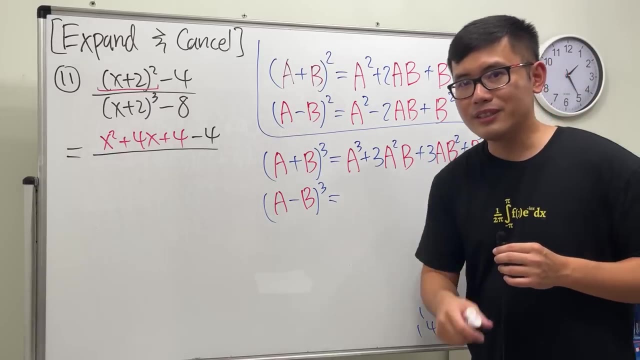 and lastly, b to the third power with a coefficient 1. Like that, Okay. And then if we have the minus version, let's say a minus b to the third power. this right here, it's pretty much the same thing. but then the sign in between alternates. 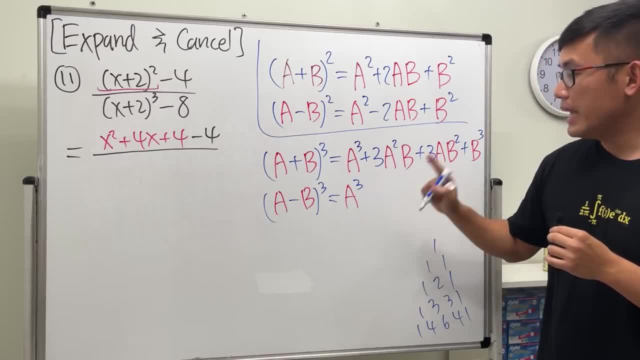 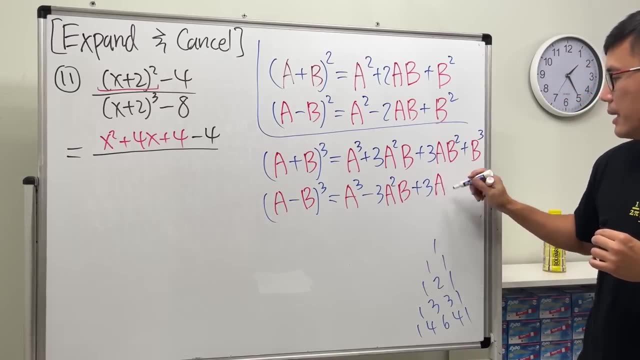 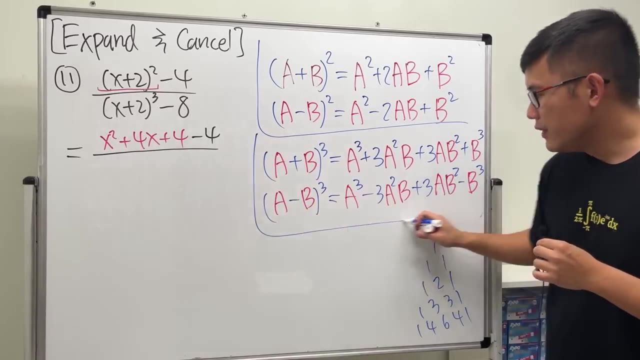 We start with the positive version: first a to the third power, and then minus 3a squared times b, and then plus 3ab squared and lastly minus b to the third power. So If you use this right here, yeah, it will also work out pretty well. 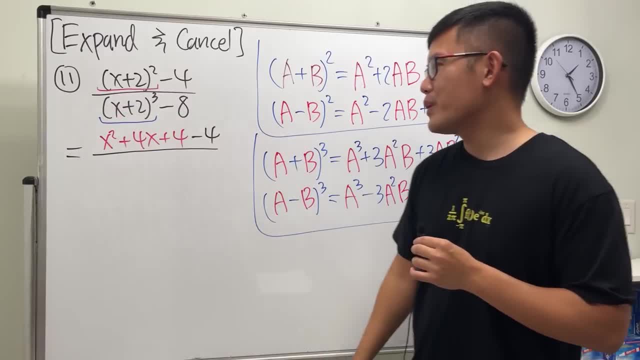 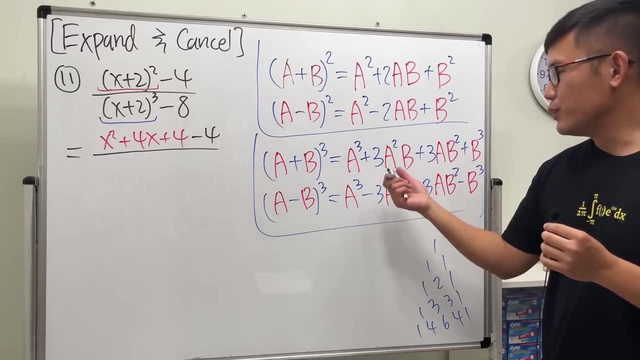 Usually for the third power. maybe I would recommend you guys to actually write it down and just multiply things out, because if you do this in your head it might be easy for you to make a mistake. so it takes practice, I would say. 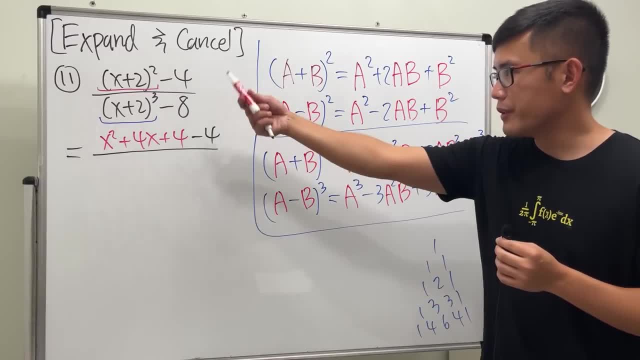 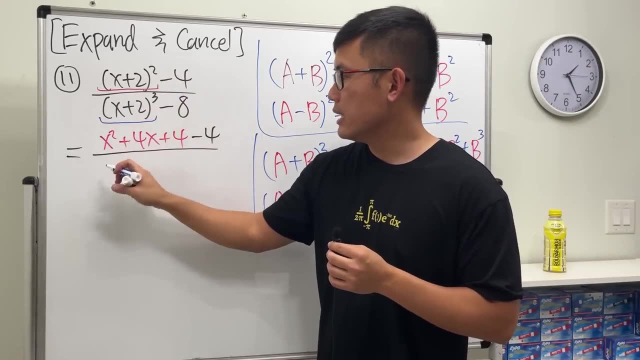 So let's see- though, This is just forwarding that out right, Right here- Okay, So we have x plus 2 to the third power. We start with x and we raise that to the third power, so we have x to the third power. 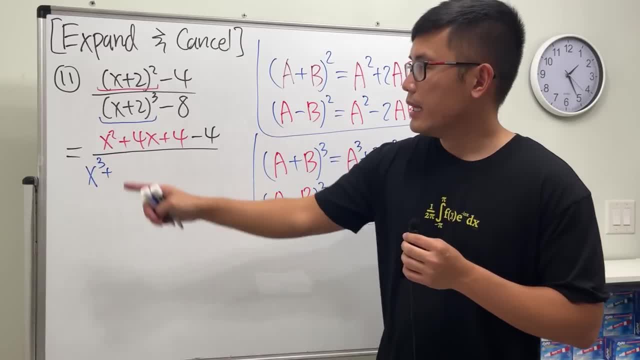 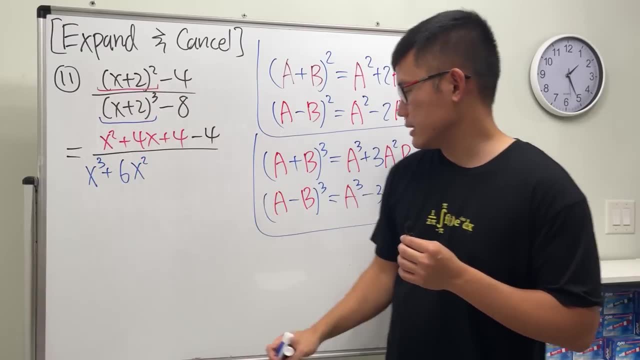 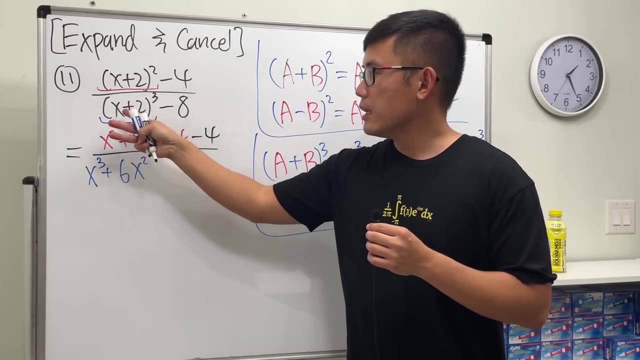 Next, we do plus 3 times x squared. so we have the x squared, but we do 3 times 2 to the first power, which is going to be 6,. right, Because we are following this formula. Next we have plus 3, and then we have x to the first power. so let's put down x, but 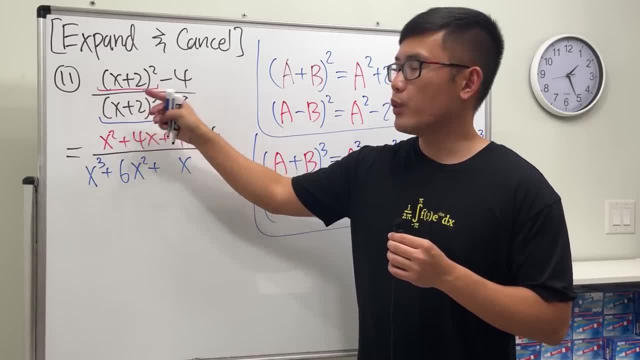 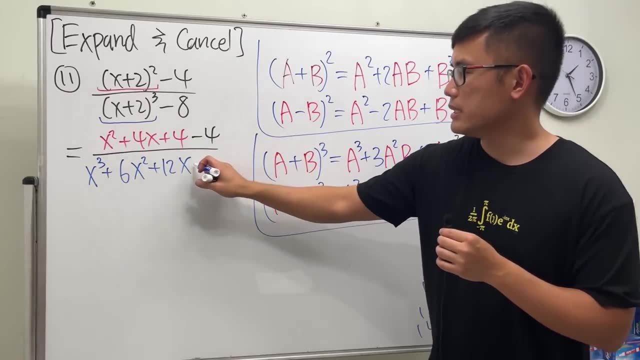 then we have to multiply by 2.. 2 squared 2 squared is 4.. 3 times 4 is 12.. Okay, And then, lastly, 2 to the third power is 8, so the blue part corresponds to that. 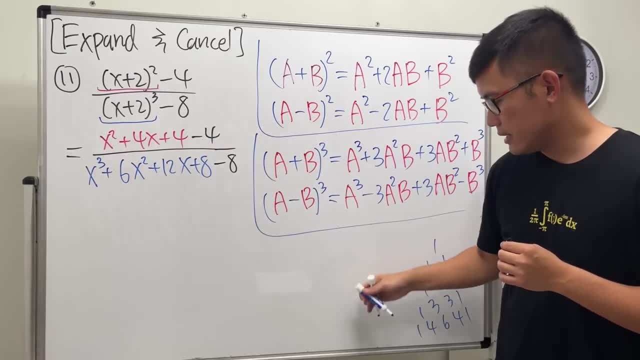 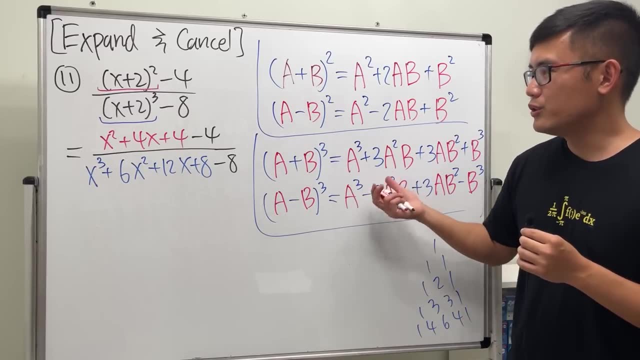 And then at the end here we have that minus 8.. So that's how you multiply out the third power. I would maybe recommend you guys to really just practice this a few times, because it would be much faster. Yeah, because if you can save your time for doing the algebra here, then you're going. 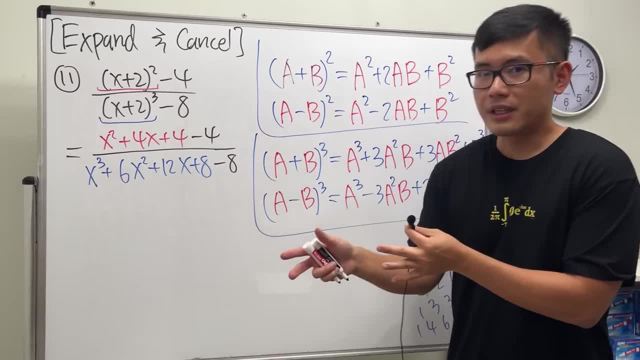 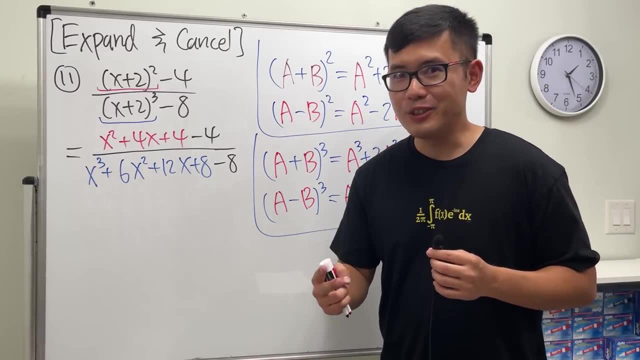 to actually focus on actually learning the calculus or like thinking about the calculus part. Yeah, I would say algebra should be your second nature when you're in your calculus class, because that's like the reality You have to. Okay. 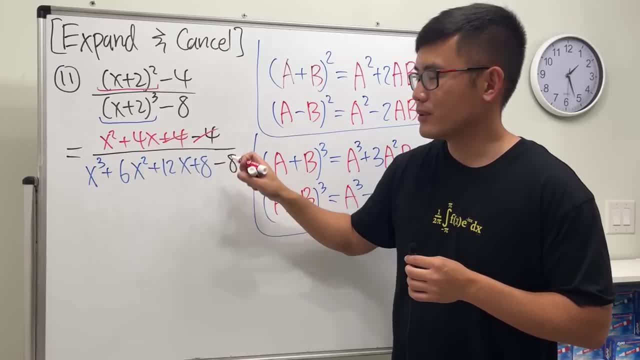 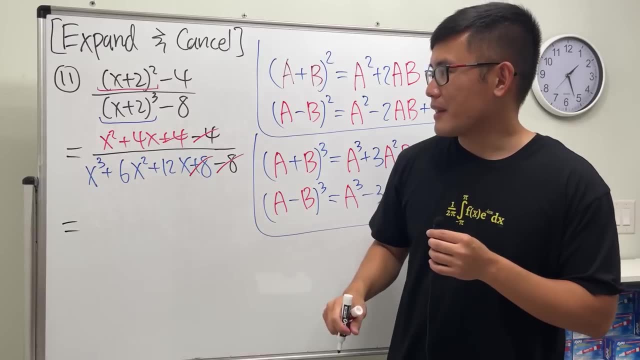 Here let's do the cute things first. This and that, cancel This and that. cancel Cute huh. Okay, anyway, On the top, here we can actually factor things out. Let's factor on x And then we get what. 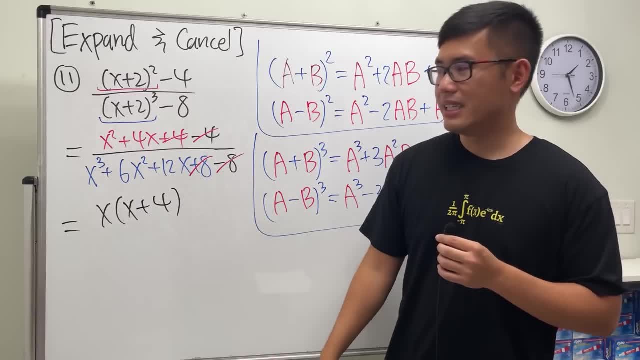 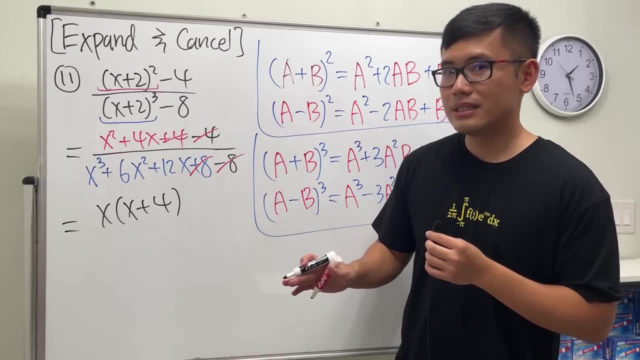 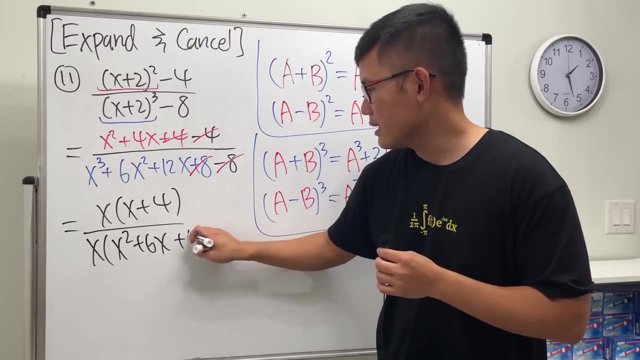 x plus 4.. That's it On the bottom. can we factor anything out? x? Yes, we can factor on x, And then we get x squared plus 6x plus 12.. Can we factor this though? Well, we can try. 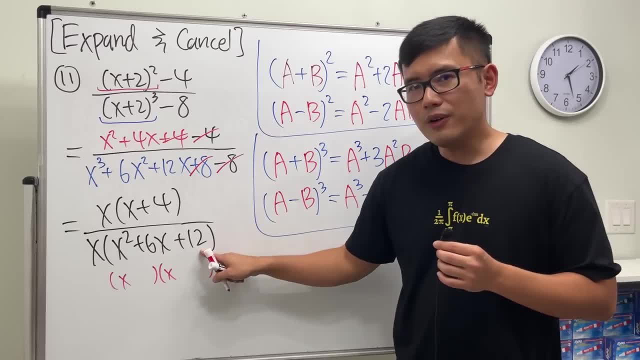 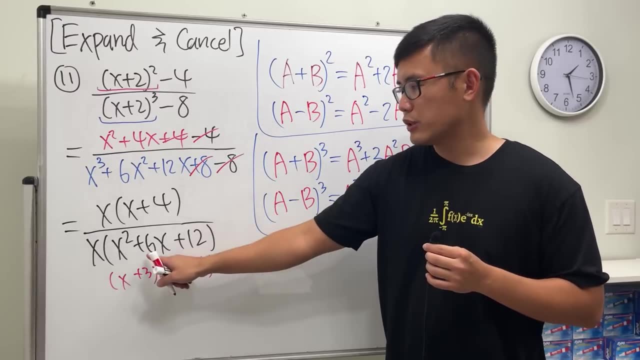 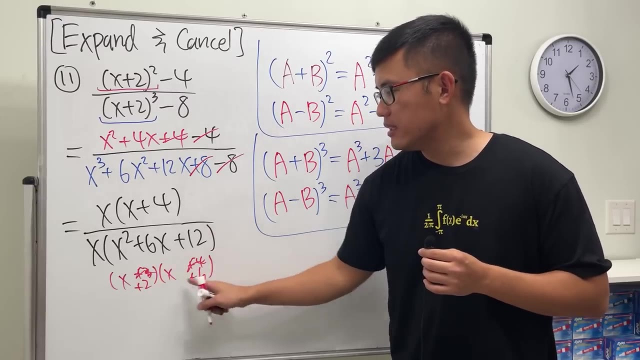 Let's say x and x To get 12? Well, we can try 3 and 4, but together they add up to 7.. We are trying to get 6, so this is no. Let's try 2 and 6, but together they add up to 8,, not 6.. 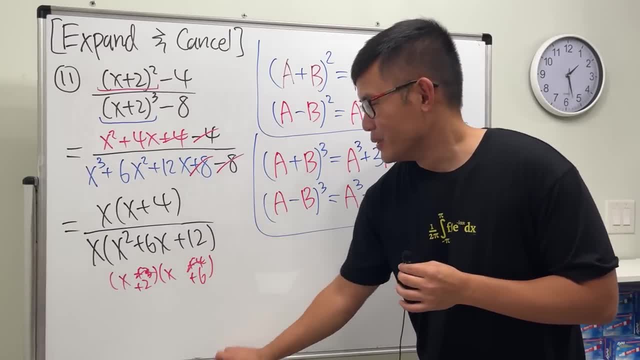 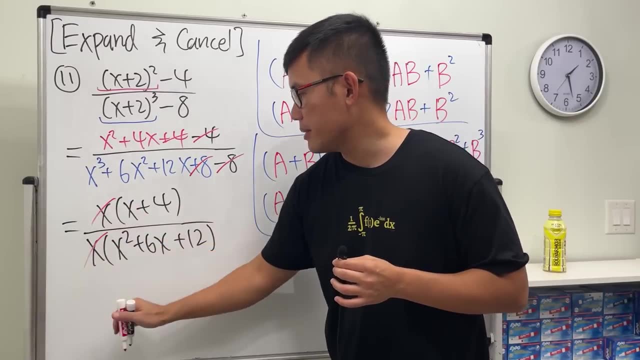 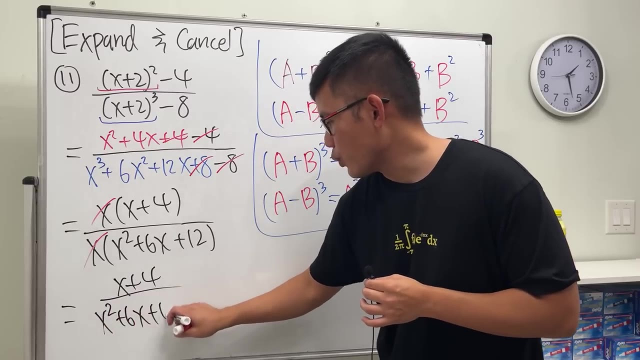 So in fact, this right here is actually not factorable. We'll just leave it like this: And then this is x times that and this is x times that, so this x and that x can be canceled, And the answer is just x plus 4 over x squared plus 6x plus 12.. 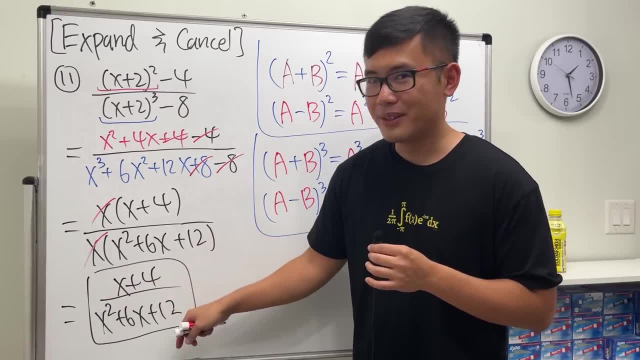 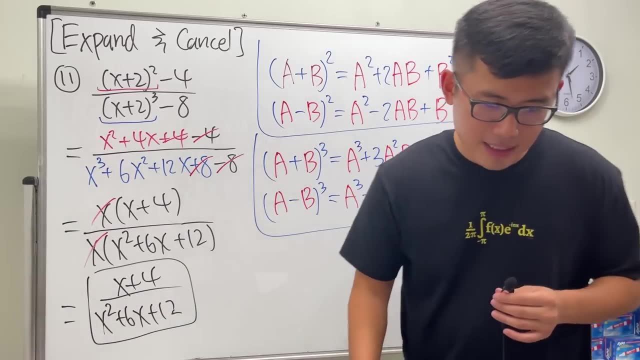 And, of course, do not reduce the 4 and the total 12.. Just leave them as how they are, because you see that x plus 4 is one term, one factor. Yeah, So that's that, Okay. Hmm. 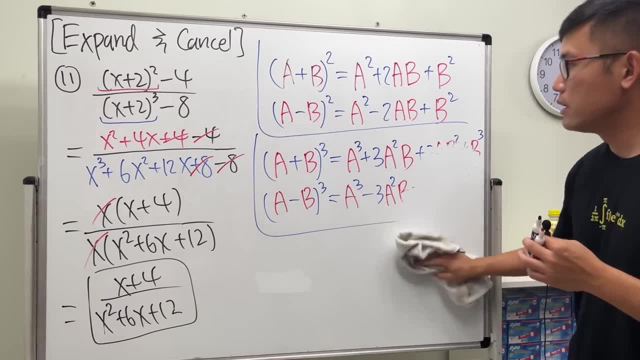 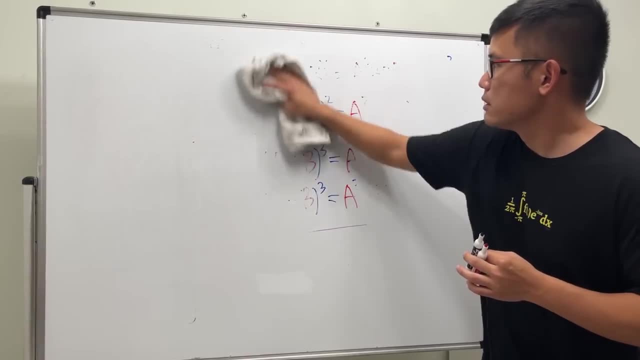 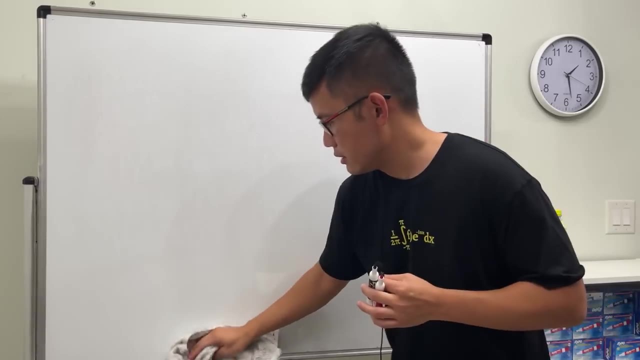 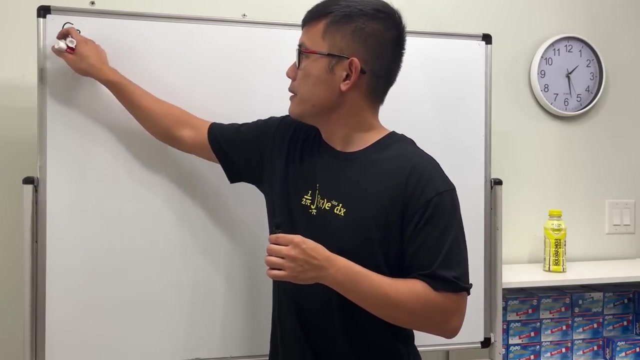 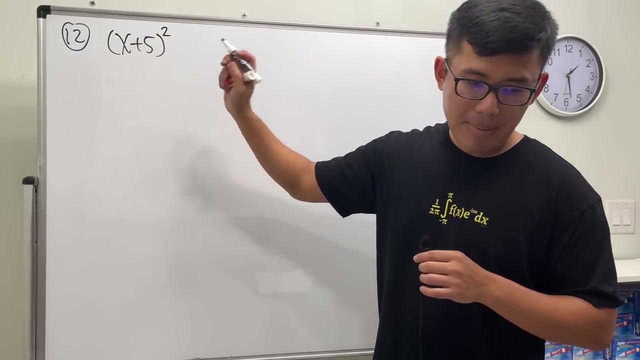 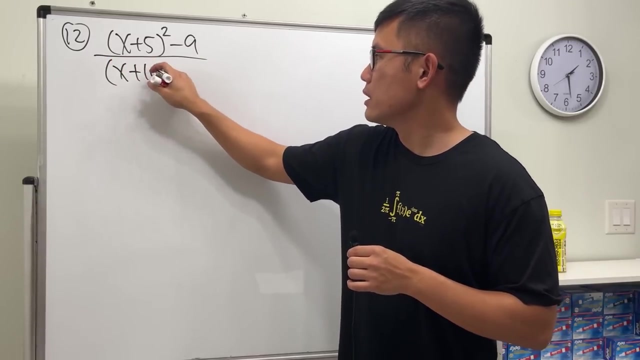 All right, Let me just erase this. Let's take a look, Number 12. Here we have x plus 5 squared minus 9.. over parentheses: x plus 10 squared minus 4.. Alright, so these are not so bad. 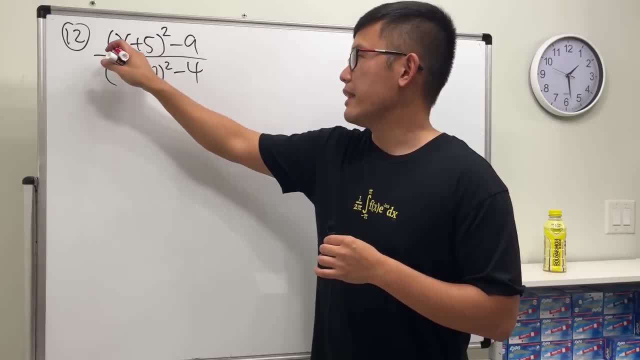 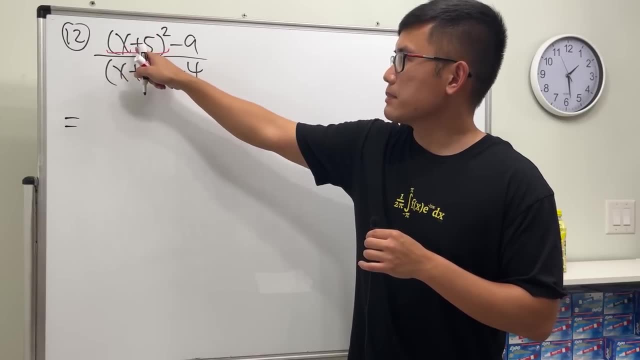 Of course you can again try to factor the difference of two squares, but I think it's just more natural to just multiply things out and then factor it. So when we multiply out x plus 5 squared, we get x squared plus 2 times this and that, which is 10x. 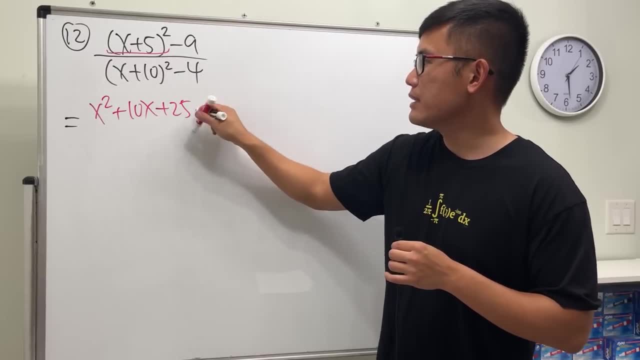 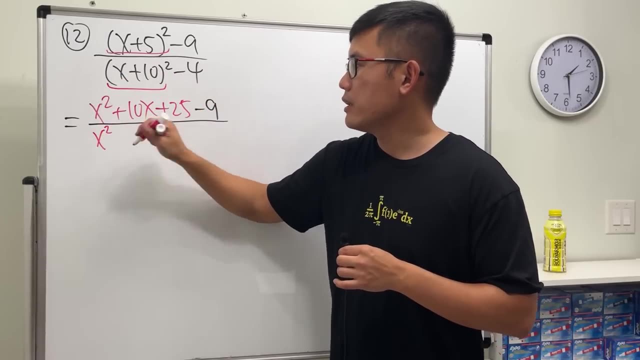 And then we add a 5 squared, which is 25.. After that we have the minus 9.. Over right here, multiply this out. we get x squared plus 2 times this and that, which is 20x. 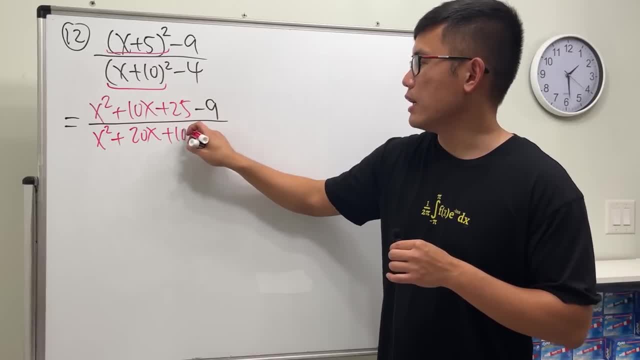 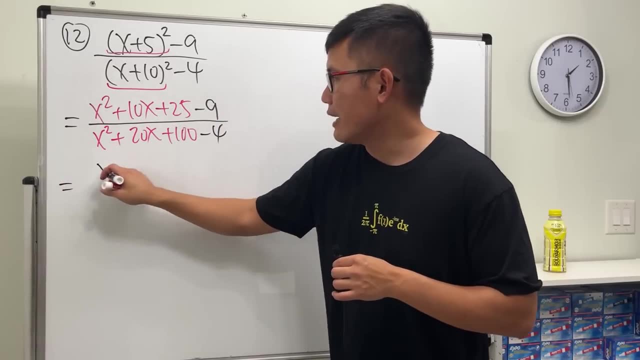 And then we do 10 squared, which is 100, and then minus 4.. Okay, cool, Now this and that can be combined, So we have x squared plus 10x, and then 25 minus 9 is plus 16.. 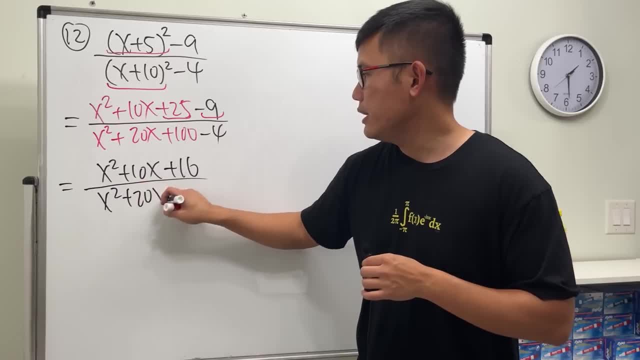 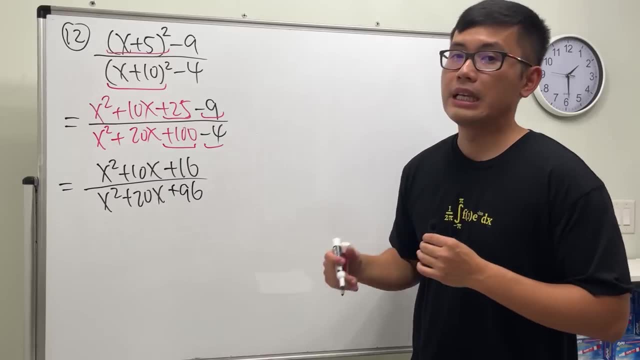 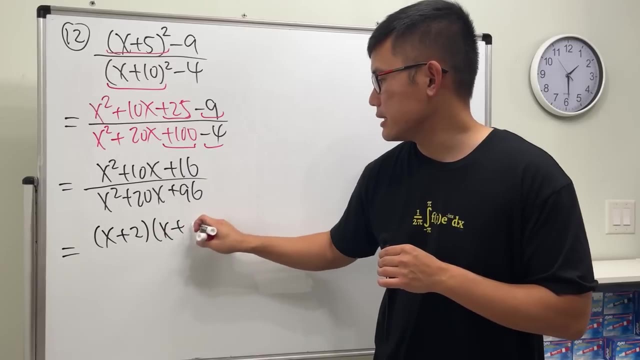 Over this. right here is x squared plus 20x. This and that together is plus 96.. Can we factor this? Yes, On the top here we can break it apart as x plus 2 times x plus 8.. On the bottom here, hmm, what times will give us 96 and together the other to be 20?? 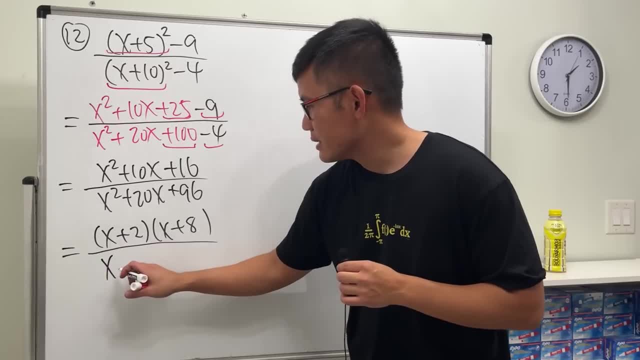 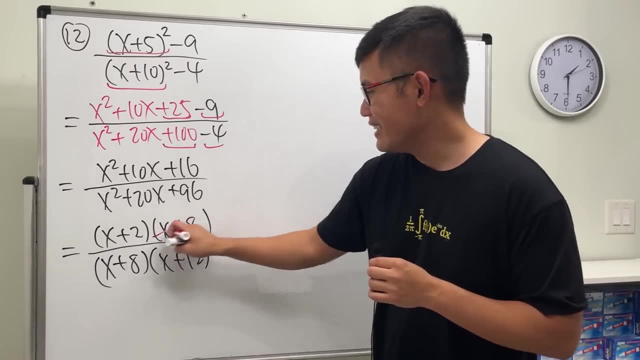 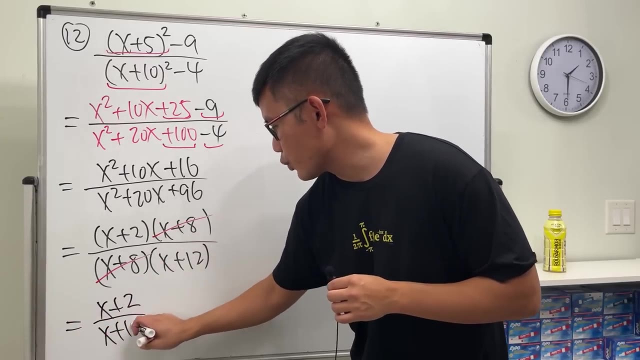 8 and 12.. It works. So here let's put on x plus 8 times x plus 12.. Aha, We see that the x plus 8 in common, so cancel them out. And finally, the answer is x plus 2 over x plus 12.. 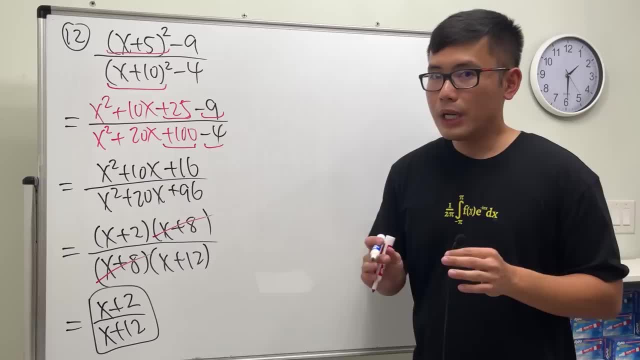 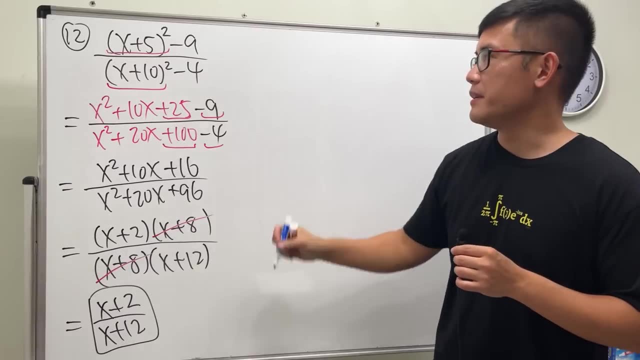 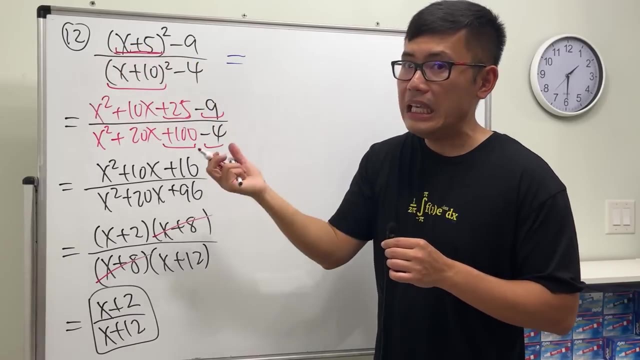 Yeah, Okay. I would like to take some time to show you, guys, what if we really did factor by the difference of two squares at the beginning. Let me show you. Firstly, we will look at This right here as our a and then the 3 right here as our b. 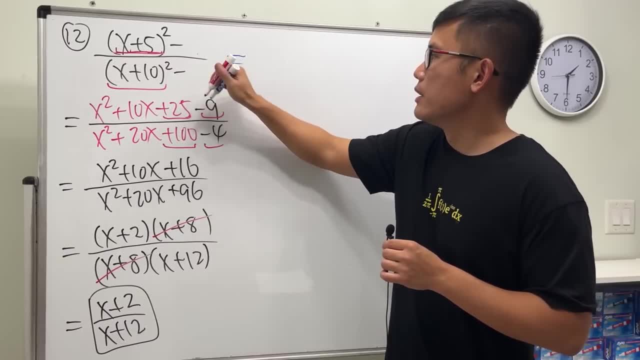 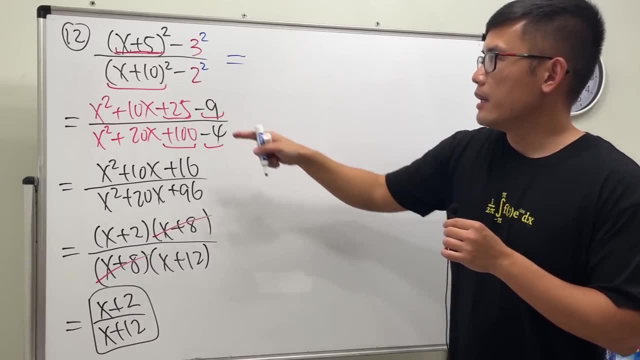 So I'm just going to erase the 9. And I'm just going to write it as 3 squared, And likewise the 4,. I will look at that as 2 squared. Okay, So a minus b times a plus b. 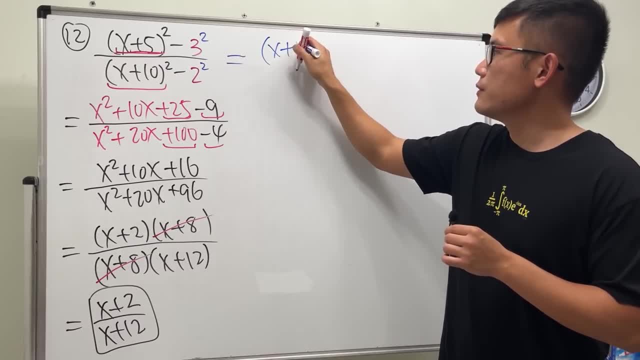 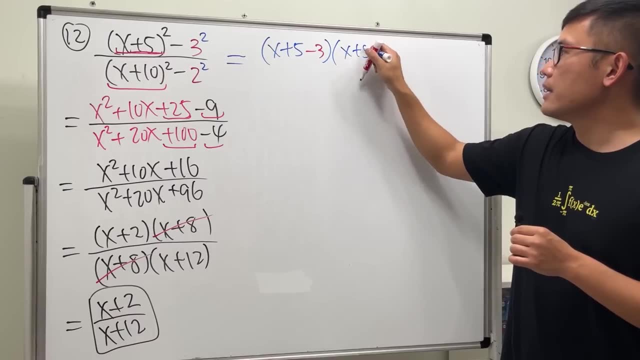 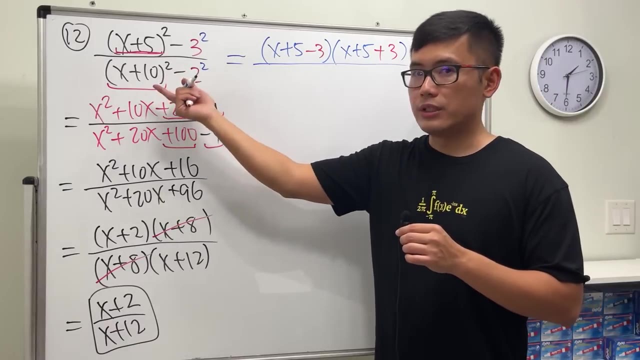 We will have. the first part is x plus 5, and then minus 3 times x plus 5.. And then plus 3.. Over Right here do the same thing. The inside here is x plus 10.. So that's our a. 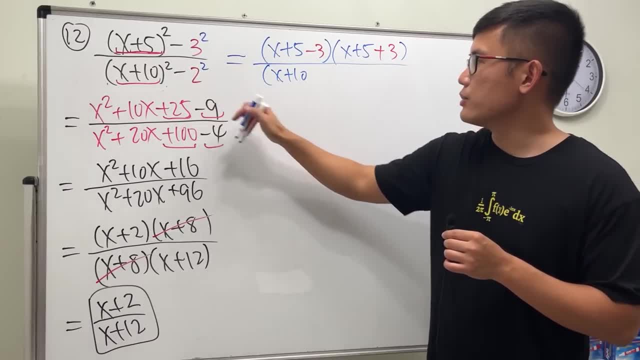 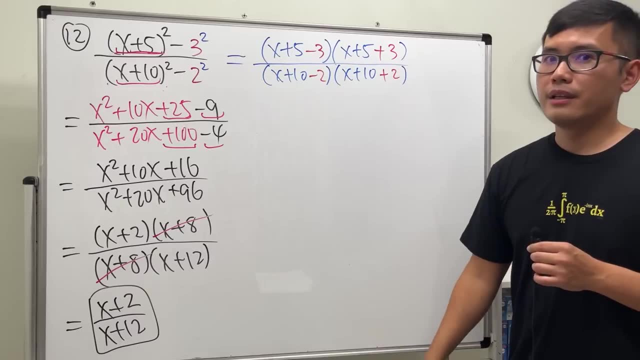 So I'm just going to write it as x plus 10. And then minus 2 times x plus 10. And then plus 2.. You see, if you use the difference of two squares formula to factor the top and bottom, 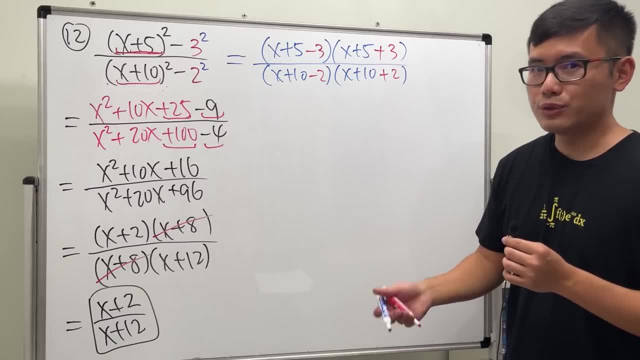 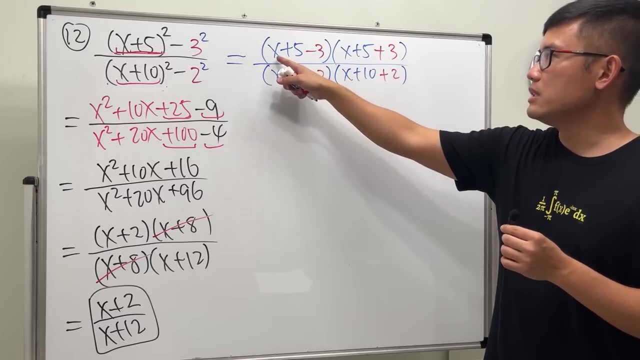 it may take you some practice to get used to this kind of things, right, But the difference of two squares is not so bad And it's actually much quicker, because now we see this is just x plus 2. And then this, and that is x plus 8.. 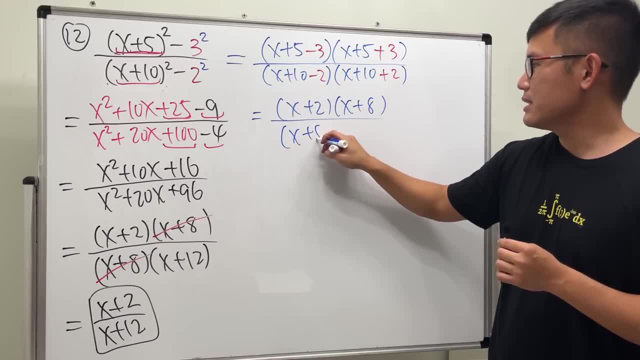 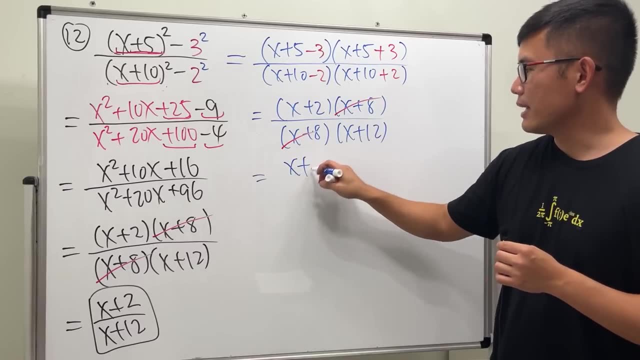 And 10 minus 2 is 8.. So this right here is x plus 8.. And then this right here is x plus 12.. Aha, This and that cancel x plus 2 over x Plus 12.. 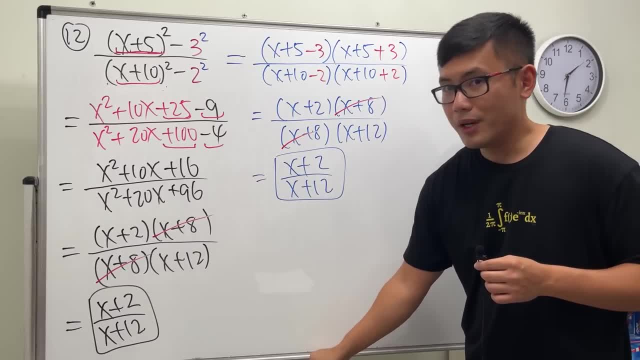 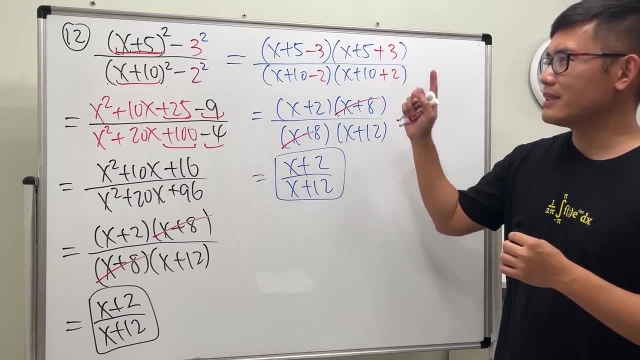 Yeah, Yeah, Earlier, it was the difference of two cubes for number 11.. That's why multiply out, I think might be easier to follow along, But difference of two squares. you may also want to try this. Okay, So far, so good. 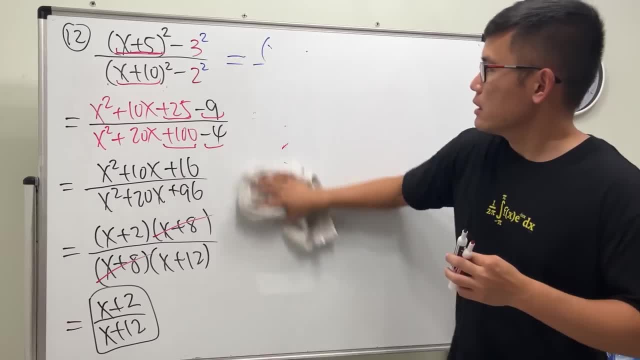 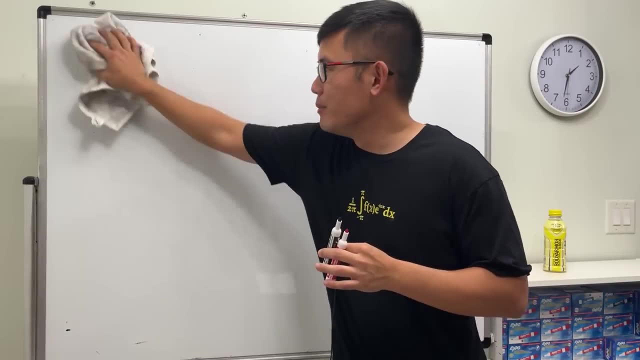 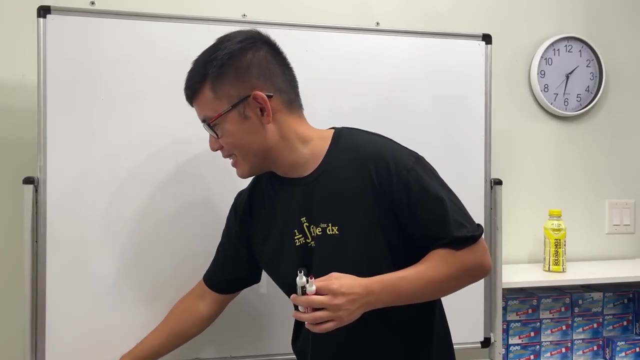 Yeah. So let me know what classes are you guys taking? Maybe you're just taking Algebra right now, but you just want to look at how the algebra will be in calculus and things like that And again all these questions. they're just like parts of the calculus questions. 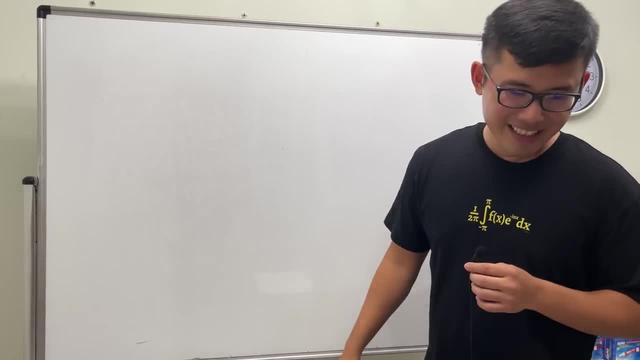 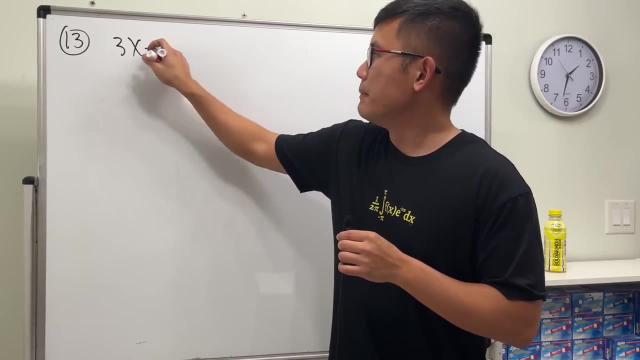 Oh, by the way, do you guys recognize what this is? If you guys know, let me know. Number 13,, one of my favorite ones, Number 13,. we have 3x minus 2 times the parentheses, And then we have x plus 2 over. 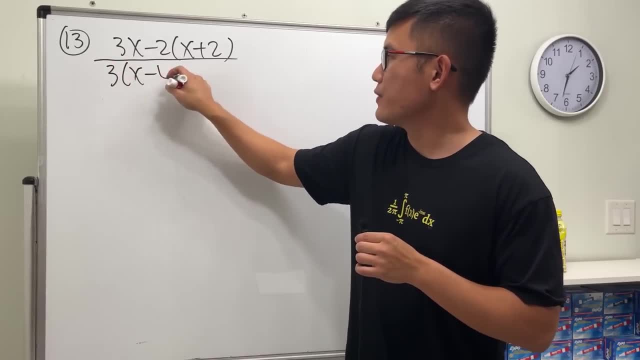 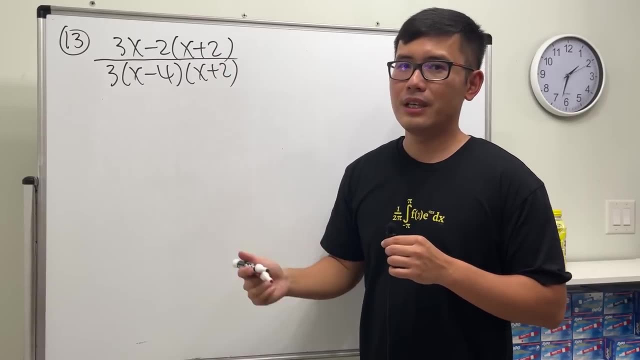 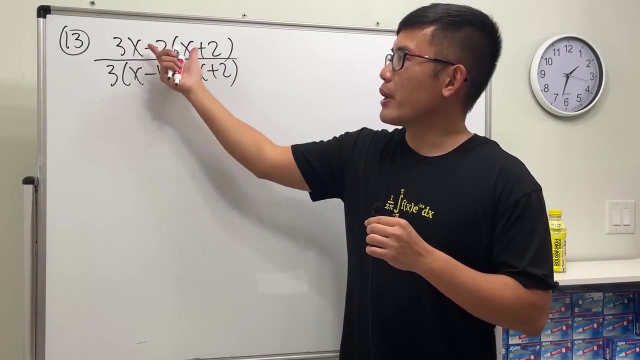 On the bottom we have 3. Times x minus 4 times x plus 2. Hey x plus 2 in the parentheses here and here. can we cancel them? No, If we cancel them, that's wrong. And the reason is because on the top right here we have not cleaned things up yet. 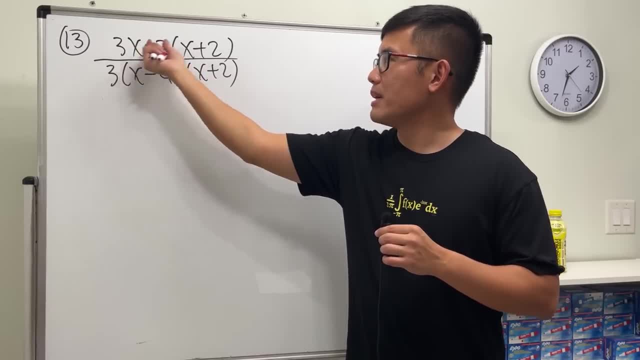 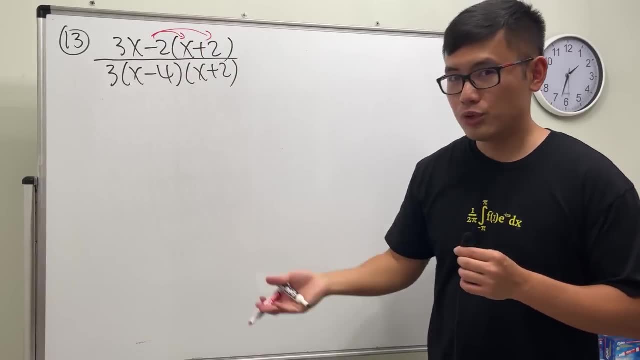 Because we have the 3x that's waiting to be combined with this. So we must- Okay, we must, We must- multiply this in, distribute and then Combine like this on the top Again, do not cancel this and that. 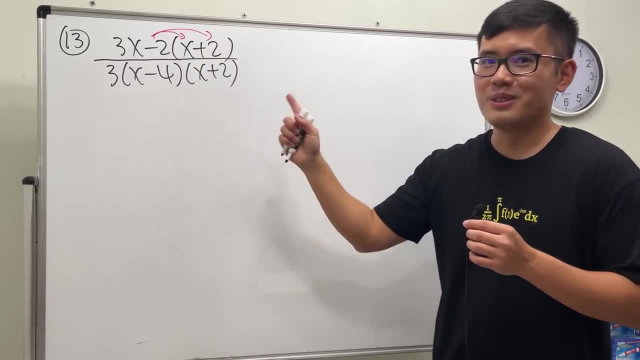 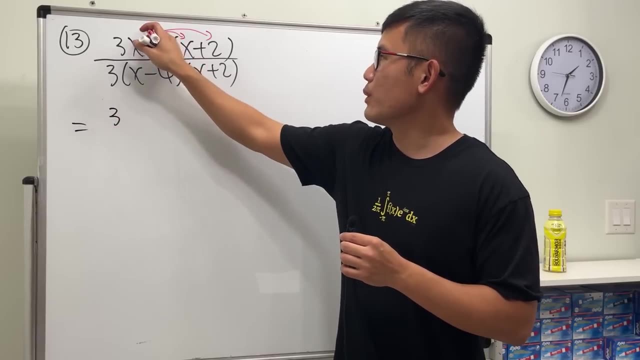 It's a super common mistake that I see a lot of calculus students still make too Okay on the top. we actually just have: Let's see, if I multiply this out, we'll just have negative 2x Sometimes. if you want to just do some scratch work, just put down the result on the top. 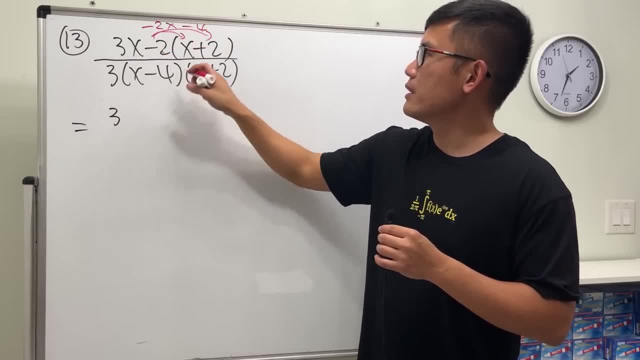 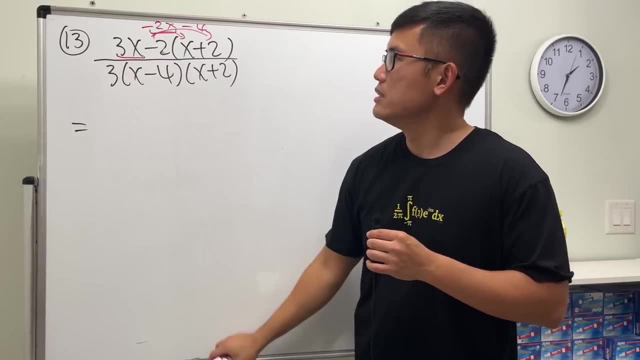 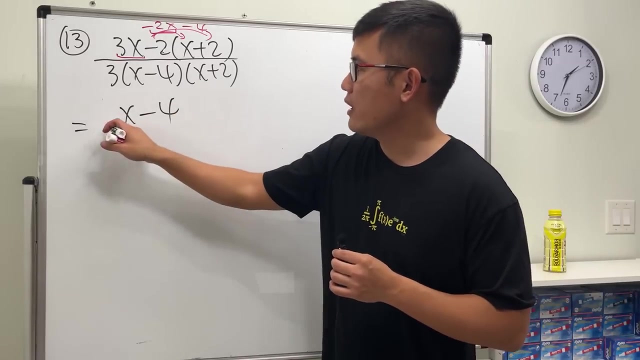 Negative 2 times x And then negative 4.. So we see this is 3x minus 2, which is just An x. Yeah, So on the top we actually have x minus 4.. Yeah, Over 3 times x minus 4, and then x plus 2.. 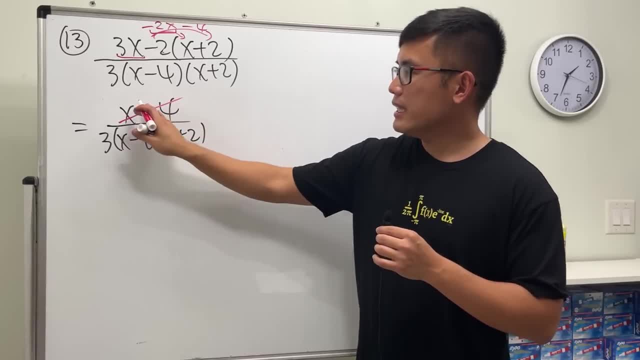 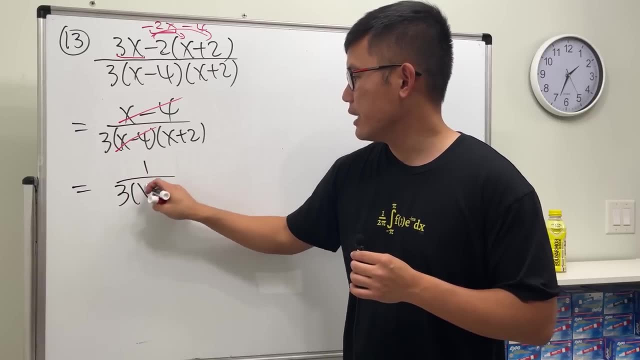 And we see that this time x minus 4 can be cancelled out with that x minus 4.. So the answer is 1 over 3x plus 2.. Okay, Again, do not look at the parentheses. Say: 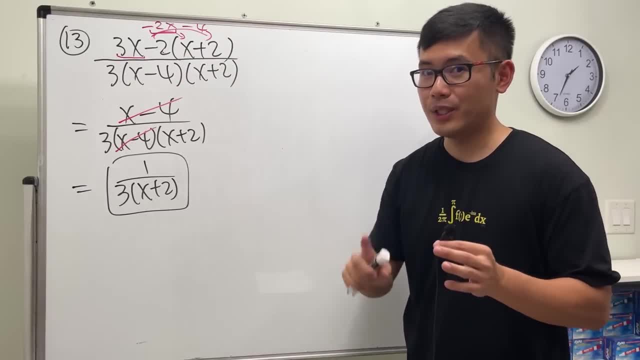 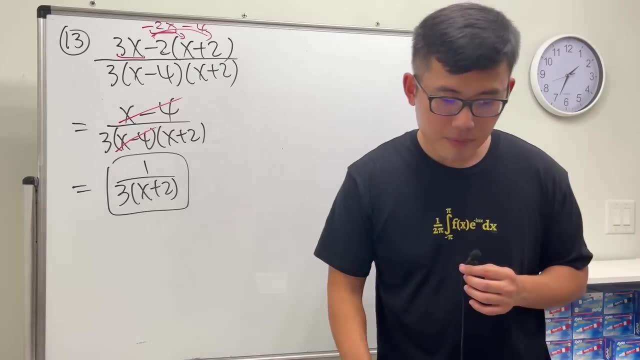 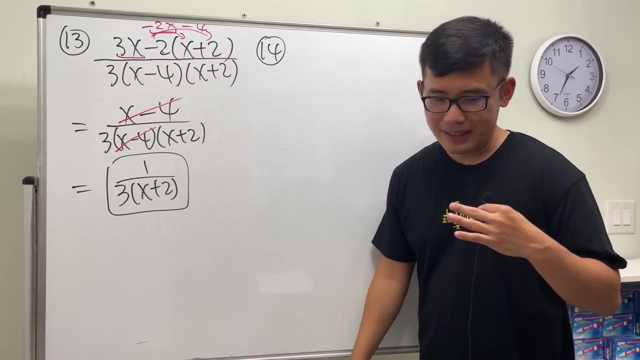 Be too happy and just cancel them out. It happens a lot and I'll tell you guys when it will happen once you end up with this kind of expression. But that's it for number 13.. Number 14 is perhaps my favorite for this worksheet here, because not only I came up with it, but it's so beautiful. 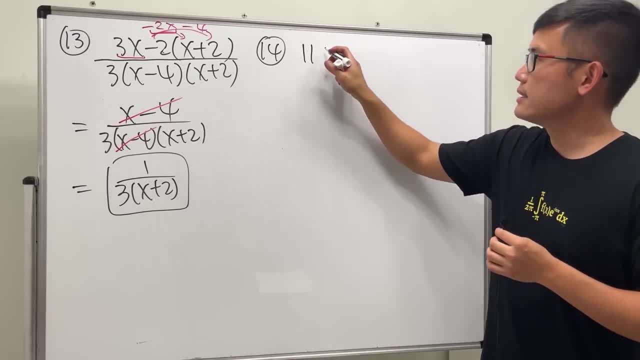 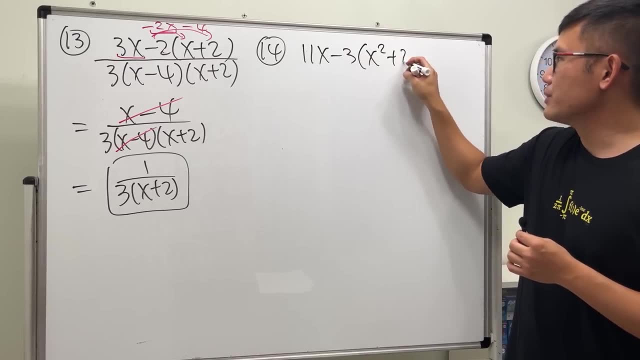 Let me show you. We have 11x minus 3.. So far no parentheses, but you know the parentheses will be coming here. And then we have x plus 2.. Well, x squared plus 2 here Over on the bottom, guess what? 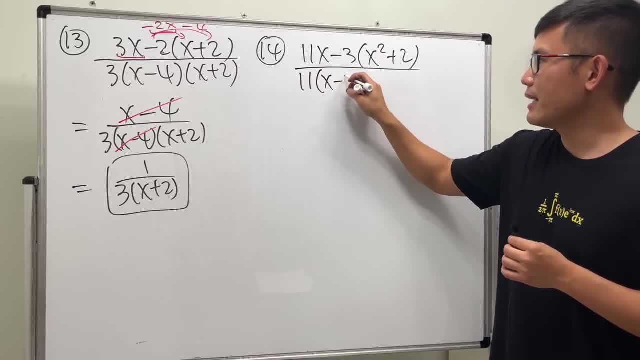 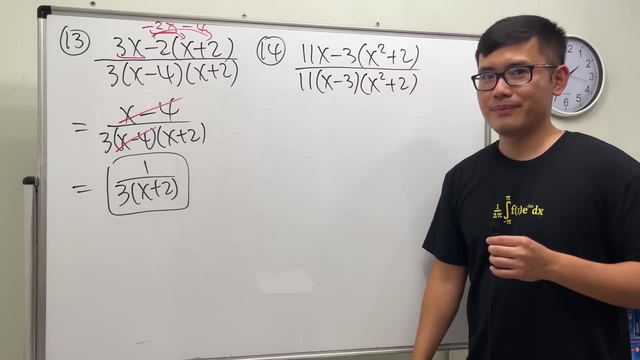 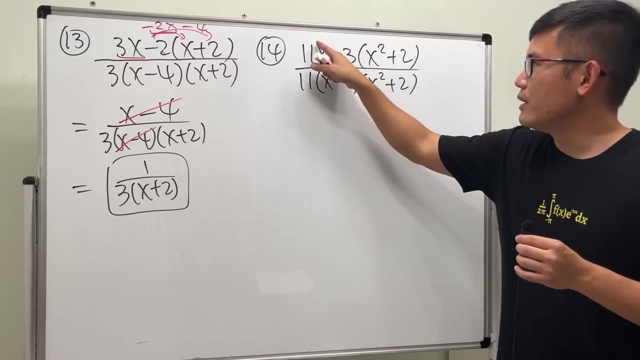 We have 11, parentheses, and then x minus 3.. And then parentheses x squared plus 2.. Wow, You see the top and the bottom. they're actually pretty much the same, huh, Except for this part right here does not have the parentheses, but this part does. 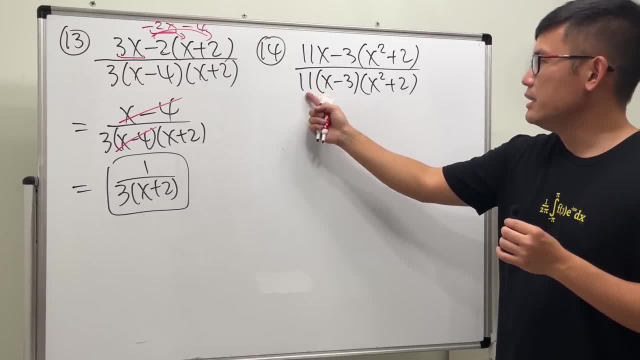 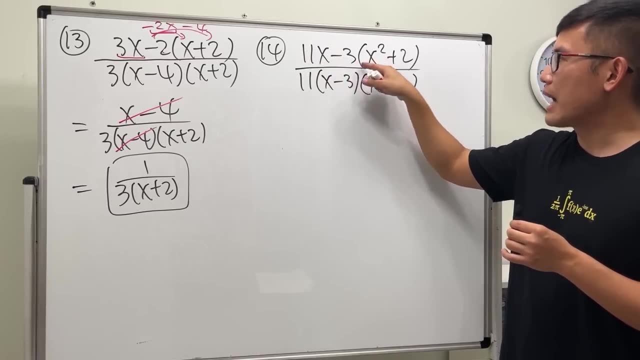 Be super careful with this. On the bottom, On the bottom, On the bottom This times, this times that. so it's already factored in for us. But on the top you see that we have 11x minus 3 times the parentheses, x squared plus 2.. 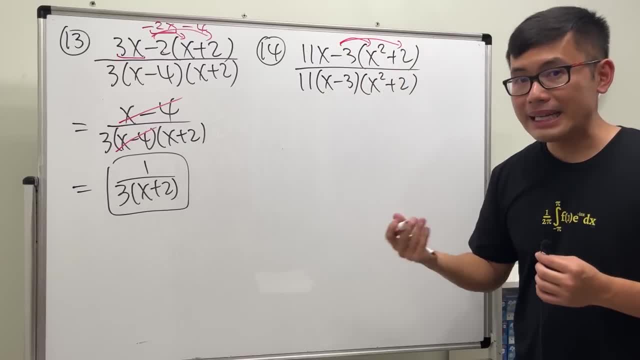 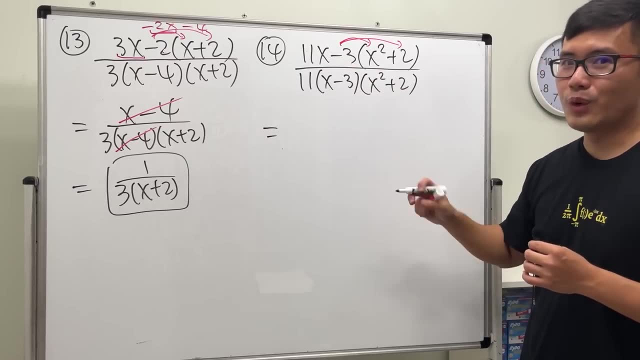 We will have to take this and distribute it inside, combine like terms before we can do a thing. alright. So do not just cancel everything and say the answer is 1 or 1, not. Don't do that, Check this out. 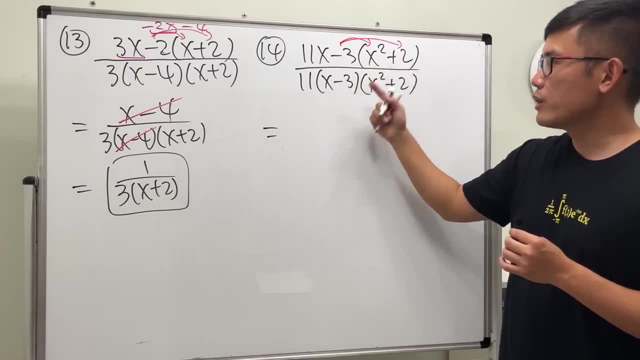 Negative 3 times x squared. Well, that's the x squared term, so I'm going to write that down first: Negative 3. Negative 3x squared, And then I'm going to put down the plus 11x. 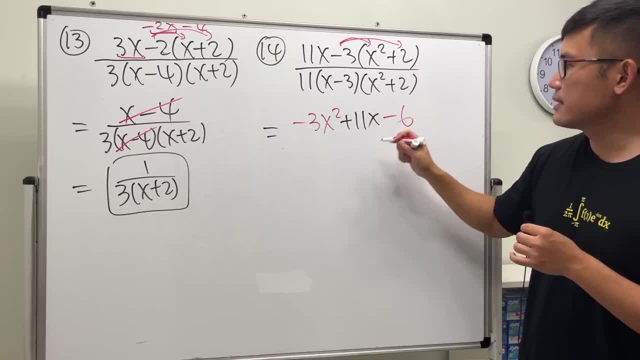 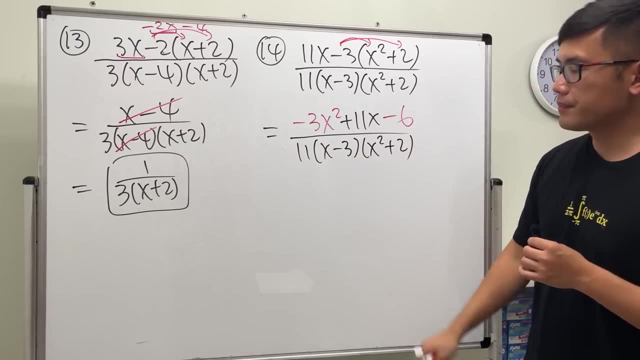 Then we have negative 3 times 2,, which is negative 6. And over the denominator, 11 times x minus 3, and then x squared plus 2.. Can we simplify this? You bet? I set this up, so of course we can do more and cancel things out. 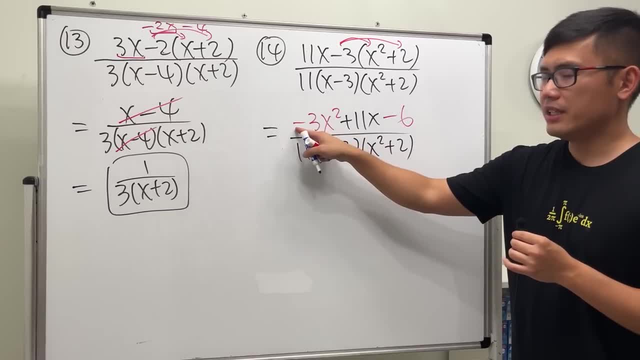 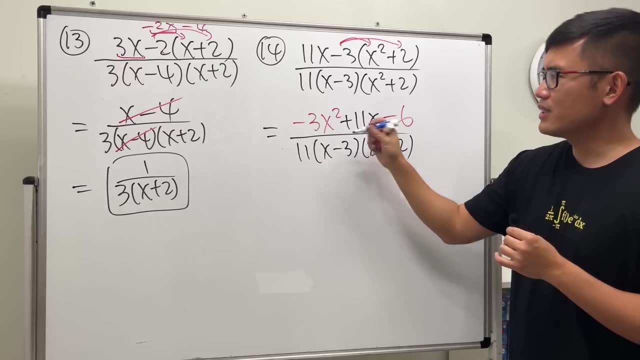 So right here I will tell you, though We see that we have a negative 3 in front of the x squared. Usually we like to keep the x squared term positive, so let's go ahead and just factor out a negative. 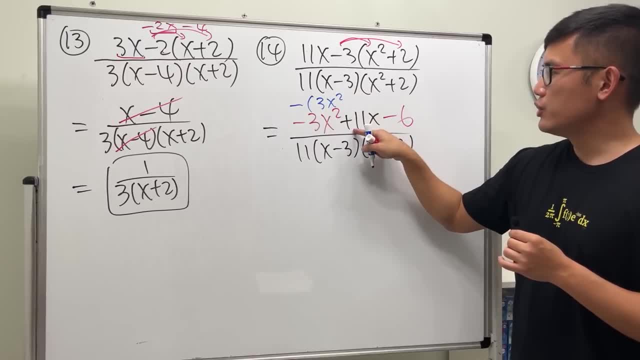 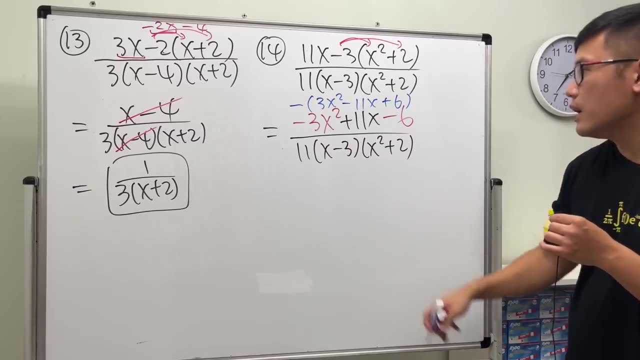 So negative and then we get 3x squared, Change this to a minus and then change this to a plus because we took out the negative at the front, And then, if we look at this, let's see we can do the tic-tac-toe right here. 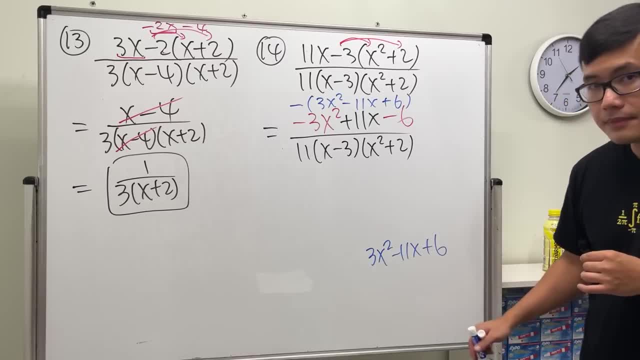 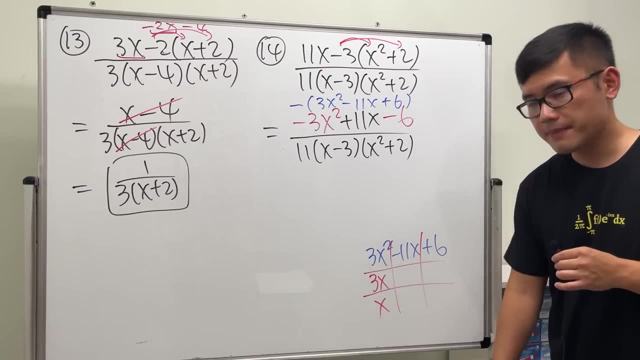 3x squared minus 11x plus 6.. Just go ahead and do it Tic-tac-toe in action: 3x times 6, that's the only way. yeah, And then, right here, negative 2,, negative 3.. 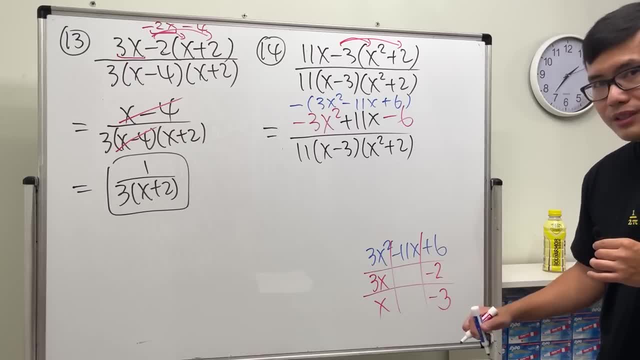 Let's put a negative 2 here and negative 3 here. It works. This times this is negative 9x and this times this is negative 2x. Together we do end up with negative 11x. So here the top right here will be negative. 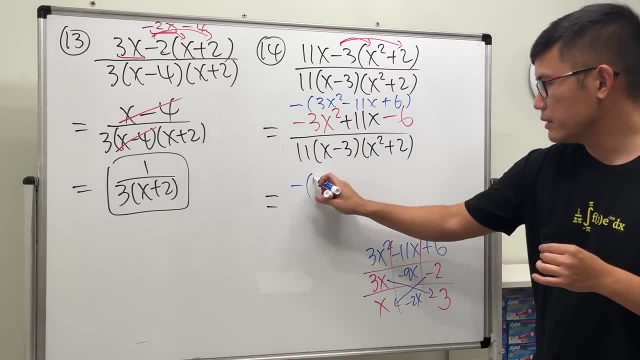 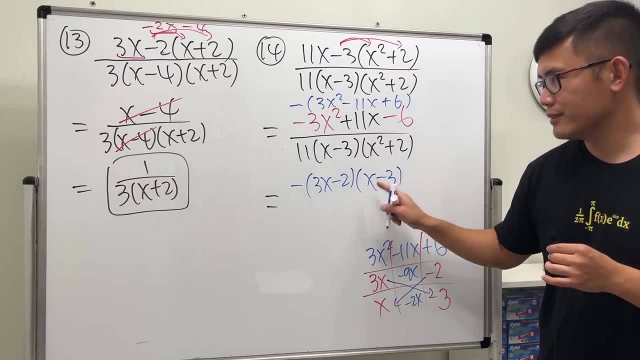 The factoring is 3x, So 3x minus 2,, yeah, 3x minus 2 times x minus 3, see Okay, over 11 times x minus 3, and then x squared plus 2.. 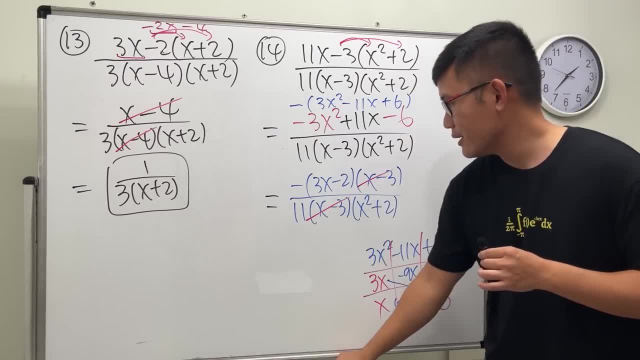 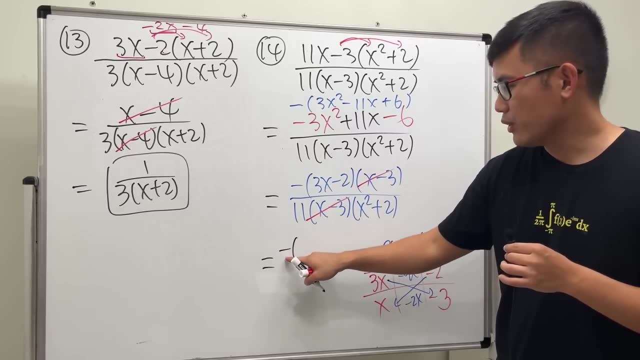 And we see that this and that cancel. so of course that will be the final answer And we can just leave it like that. You don't have to distribute the negative, Just leave it like this and if you want to put that at the front, 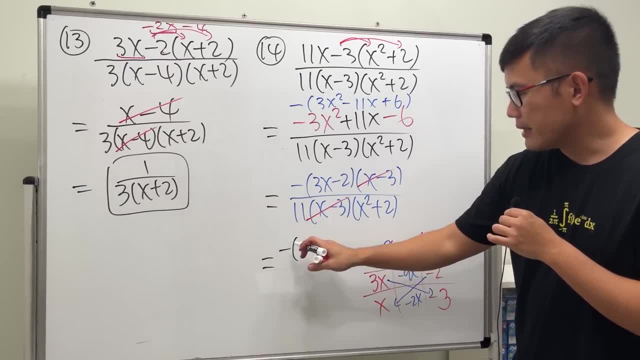 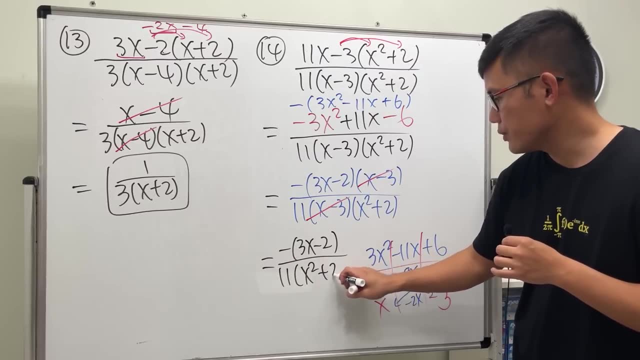 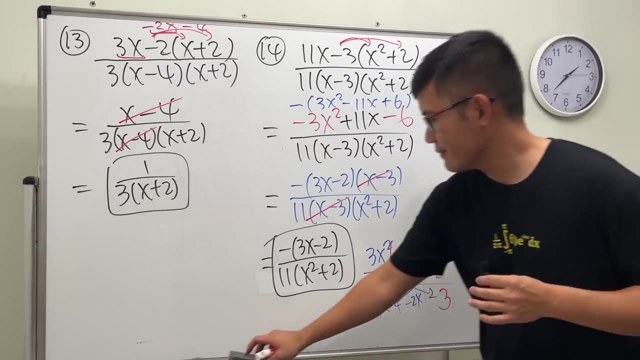 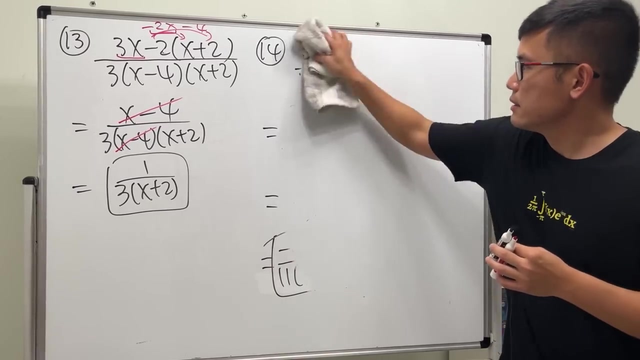 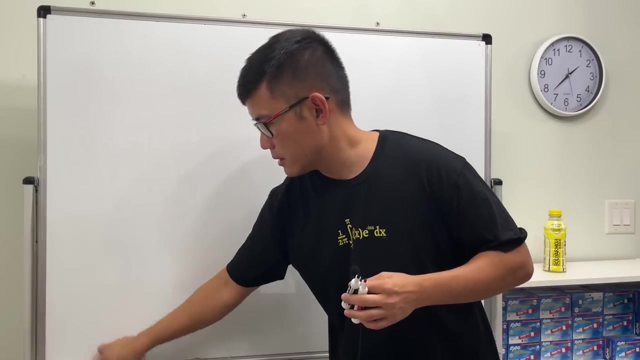 in the middle of the fraction part. that's okay too, But negative parentheses: 3x minus 2 over 11 times x squared plus 2.. So this is it. Yeah, All right. number 15 is also one of my favorites. 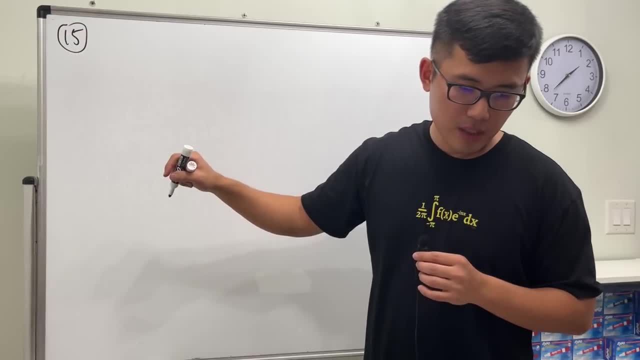 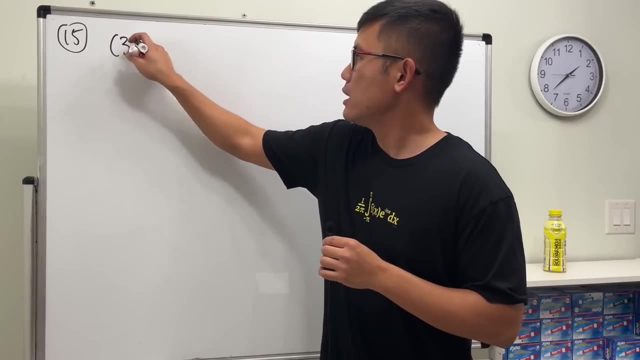 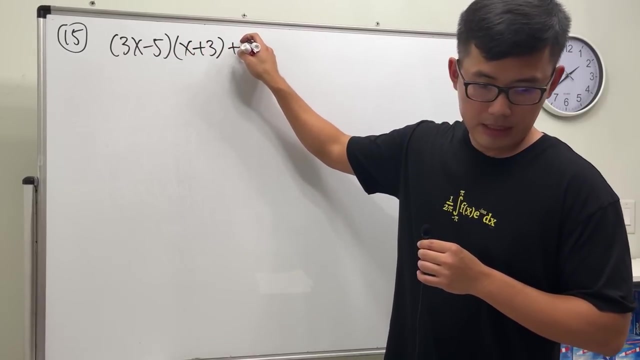 Let's see Number 15, we have 3x minus 5 times x plus 3, and then plus 11 over. Here we have 3x minus 5 times x, squared plus 2, and then plus 11 over. 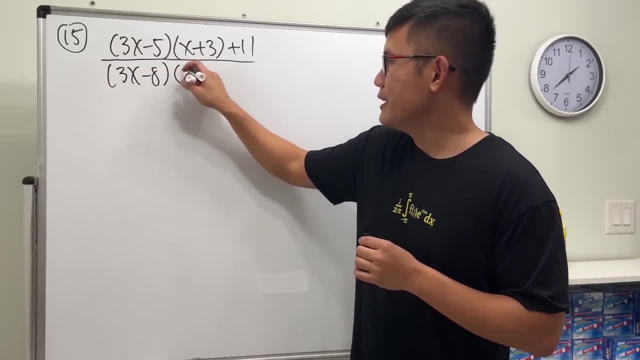 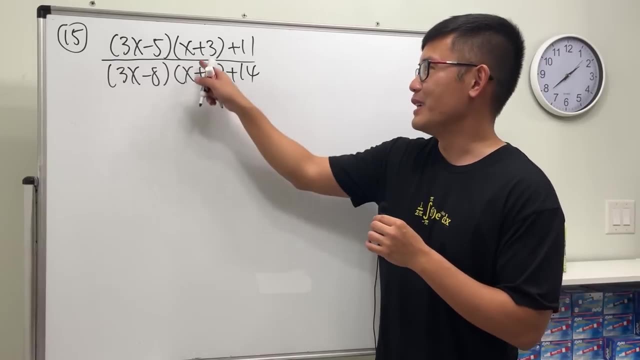 Here we have 3x minus 5 times x, squared plus 2, and then plus 11 over, And we get 3x minus 8 times x plus 3, and then plus 14.. Hey, hey, you see that at x plus 3, x plus 3?. 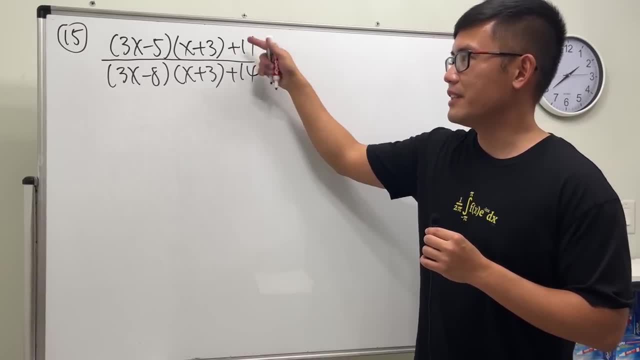 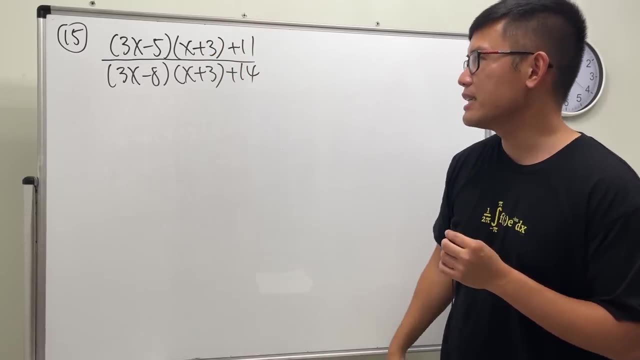 Cancel them. No, don't do that, Because again the plus 11 here, likewise the plus 14 here, all right. So in this case we really just had to multiple things down and then combine item and all that. 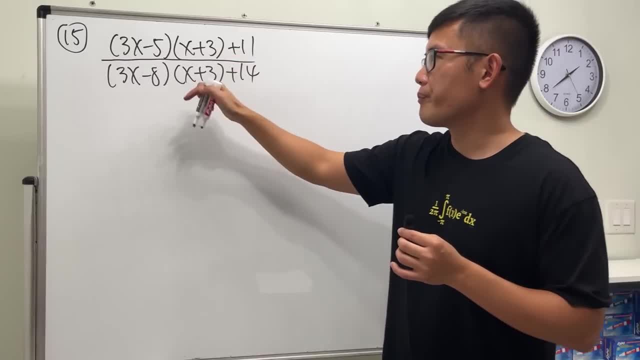 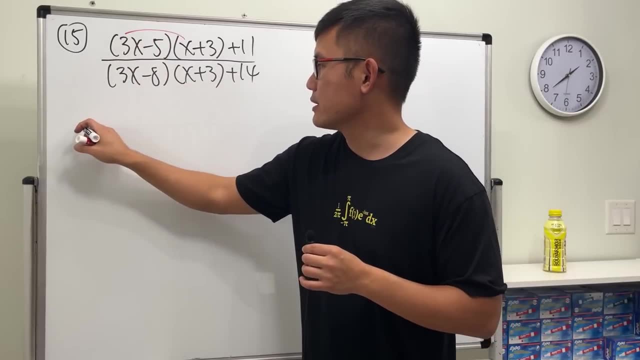 and, yeah, it's not like a nice factoring, So we cannot do the difference of 2 squared left over here, unlike question number 12, so let's just go ahead and multiply things out. so this times this and all that stuff, right? so let's see, i'm just going to work it out along the way for you guys. 3x times. 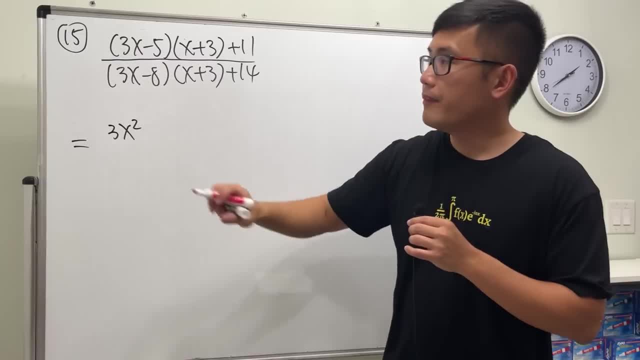 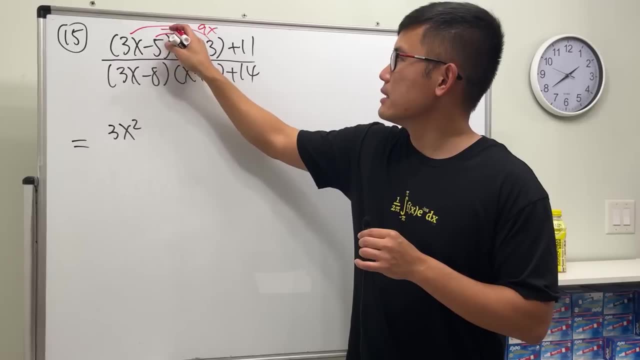 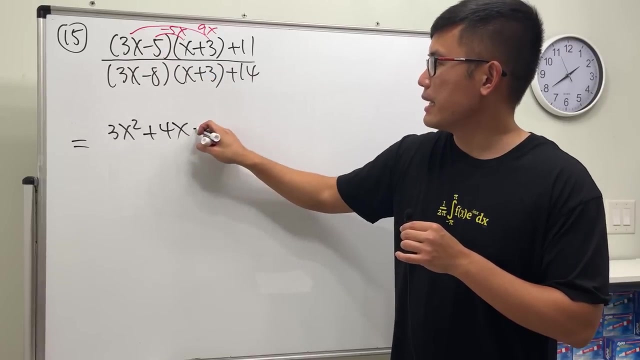 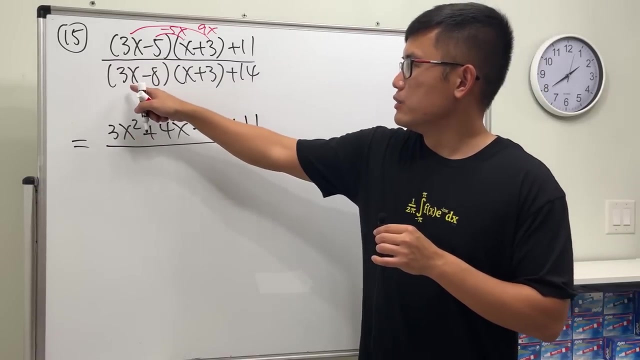 x is 3x squared, and then this times this: the outer term is 9x and the inner term, right here, negative 5 times x. together, we end up with plus 4 x. and then this times that is minus 15, okay, and then we have the plus 11. over, do the same thing. this times that is 3x squared, and then this times, this: 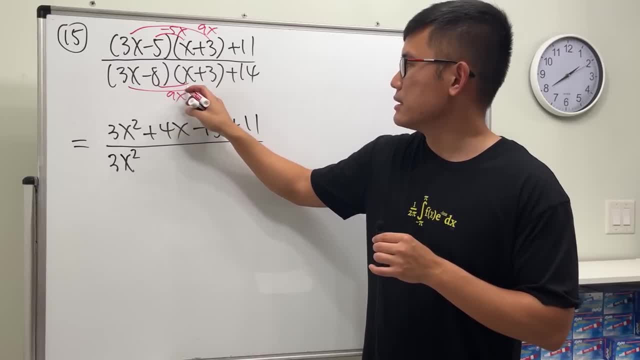 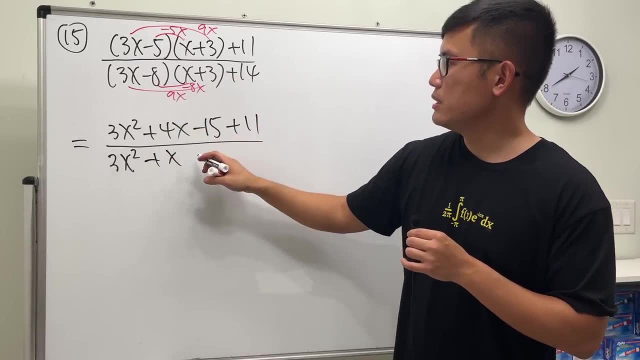 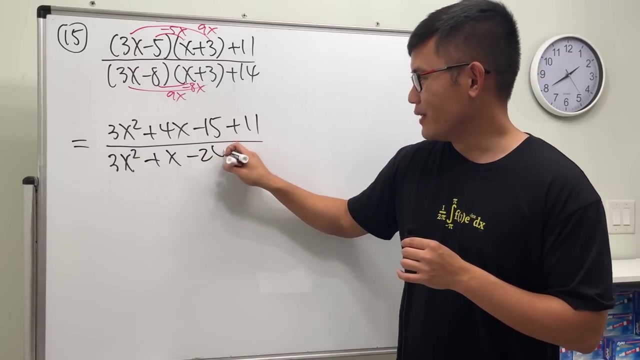 is 9x and then this times this is negative 8x. so together we have plus x and then negative 8 plus 3 is negative 8 times negative. negative 8 times 3 is minus 24 and then plus 14. yeah, all right, and. 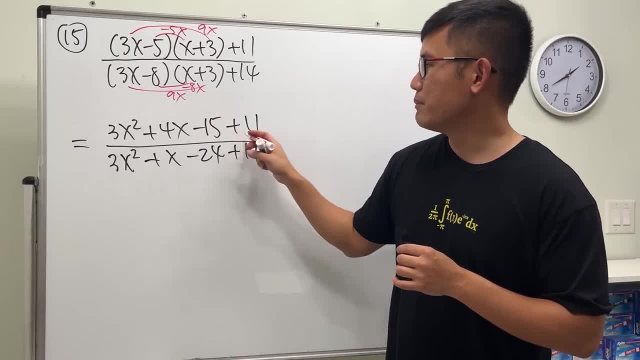 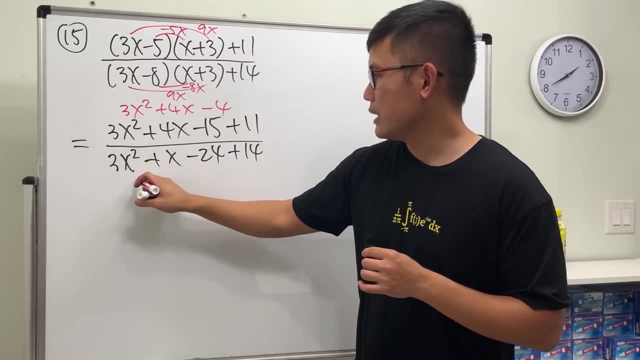 then just continue and notice that this is just pretty much minus 4, right? so on the top it's just 3x squared plus 4x and then minus 4, and on the bottom we have 3x squared plus x minus 10. okay. 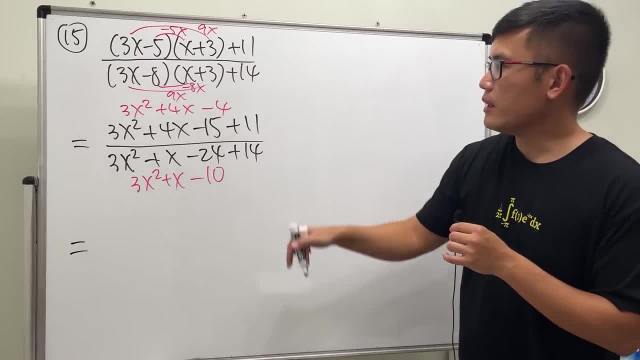 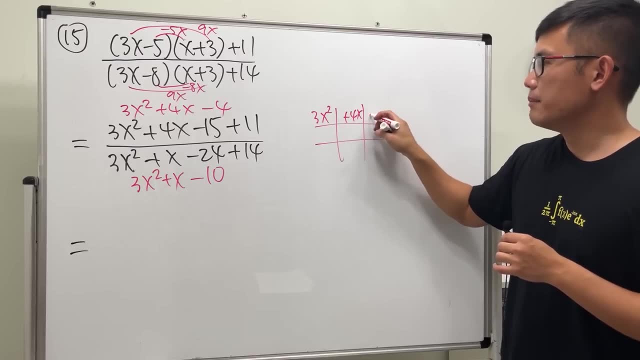 let's just go ahead and factor it. so let's see on the top here we have 3x squared plus 4x minus 4. so let's put down 3x and x and then let's try 2 and negative 2, and we want to pass the 4 right here, so this should be negative. 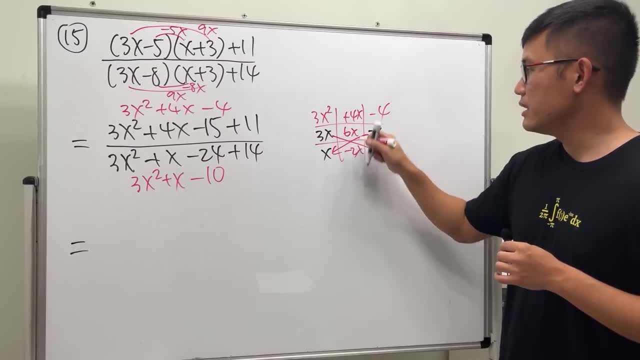 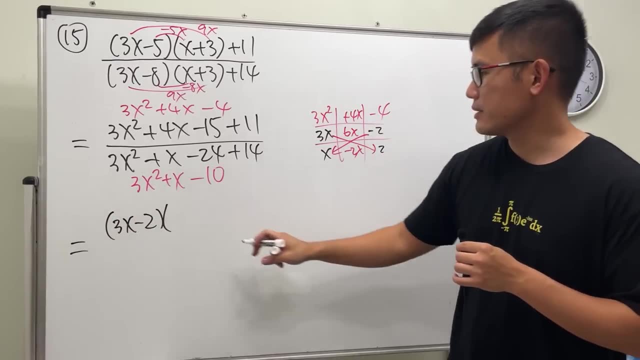 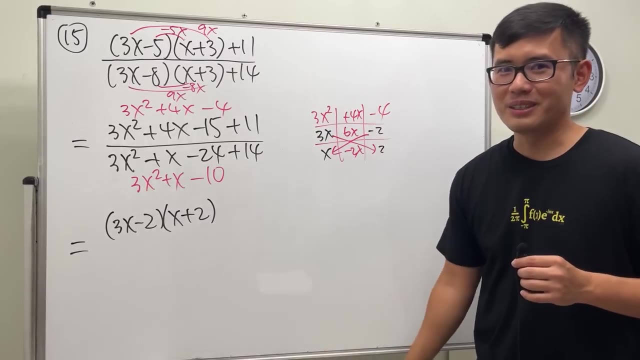 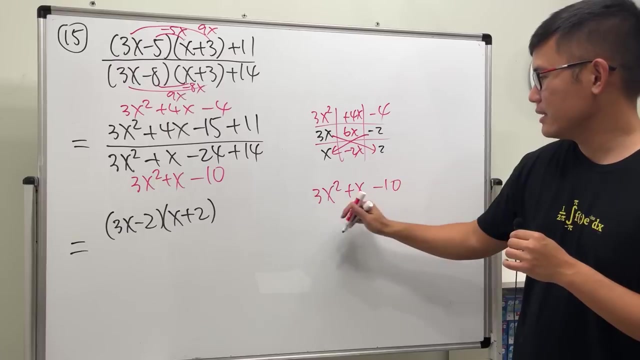 this times this is 6x. this times this is negative. 2x: yes, works. so the top is 3x minus 2.. times x plus 2.. yeah, so the original first is the simplified version. they look kind of different, huh okay. and then the bottom. let's just go ahead and do this: 3x squared plus x and then minus 10.. 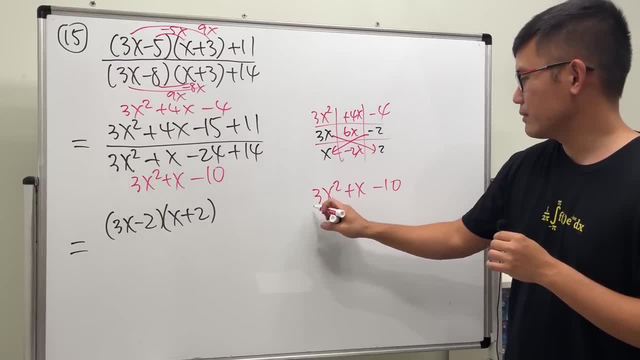 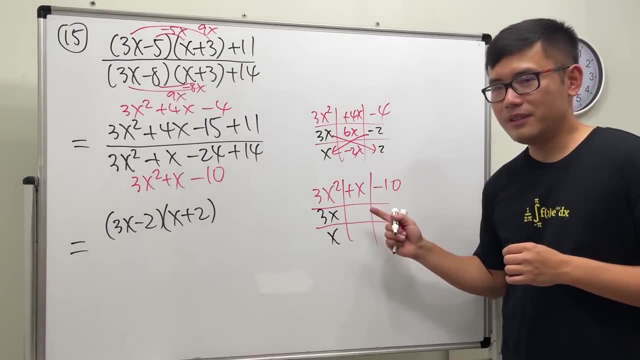 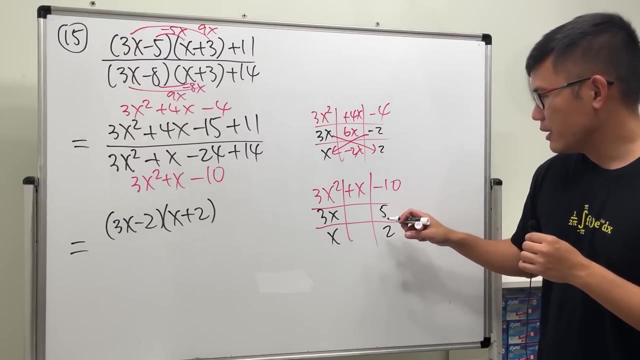 again. factor this now. let's just keep the same color way. let's see this is 3x and x. to get negative 10, we need 5 and 2, and 1 of them should be negative. let's put down 5 here and 2 here. we need a 5 to be negative because 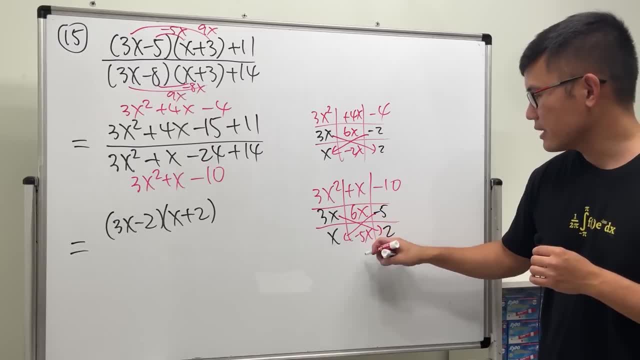 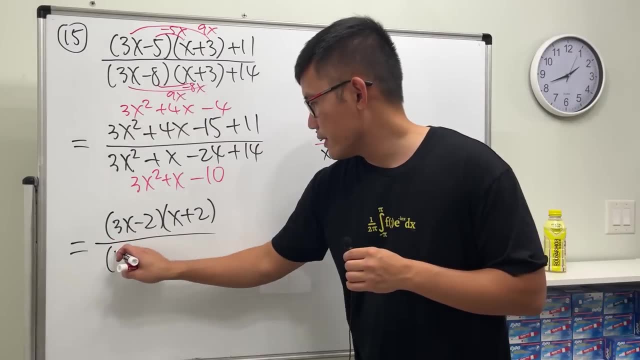 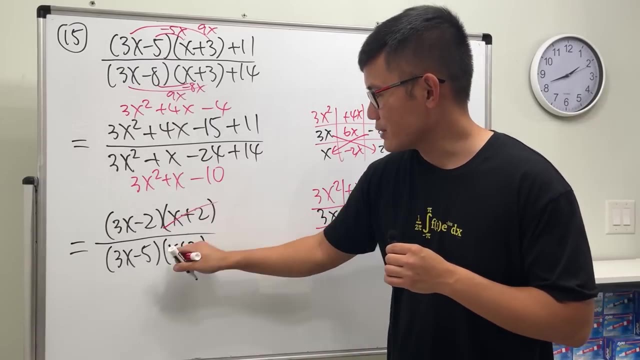 this times this is 6x. this times this is negative 5x together. we do n double x, so the bottom is 3x minus 5 times x plus 2.. and you know it: x plus 2 cancel. so the answer is 3x minus 2 over 3x minus 1.. 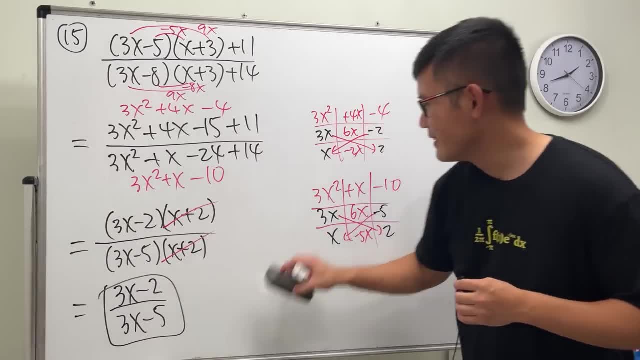 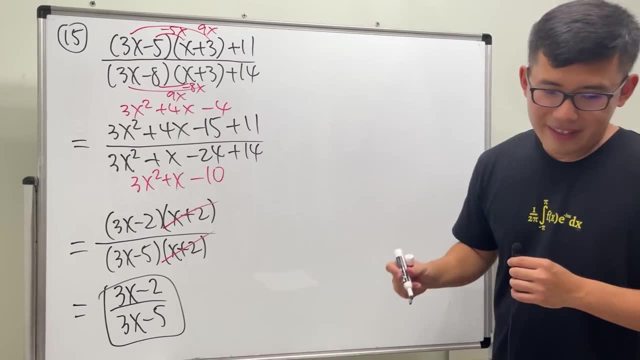 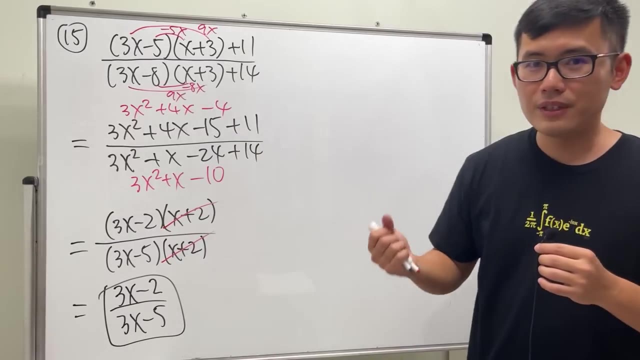 5. Done Cool, I came up with this just to let you guys know. Yeah, Okay, number 16.. And once you guys look at these right here, from number 16 to number 20, yeah, they are from the so-called definition of derivative. 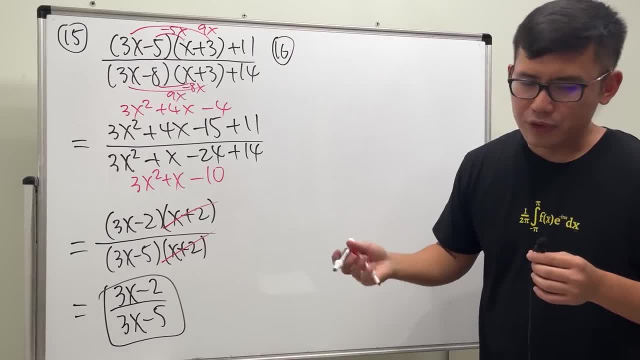 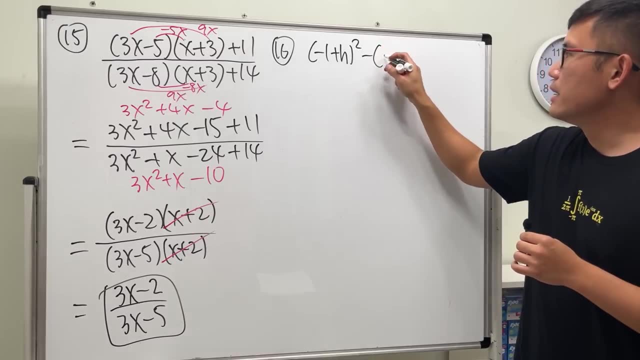 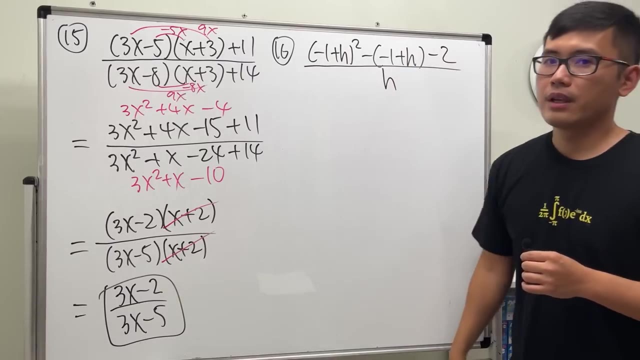 And it looks like this: The ones with h: First we have negative 1 plus h squared here, and then minus negative 1 plus h and then minus 2, all over h. For this kind of equations, our goal is just to multiply out. 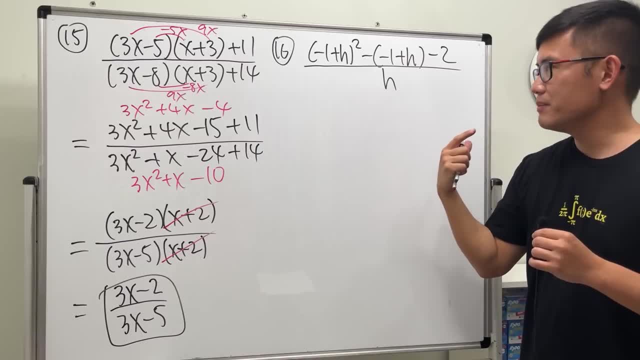 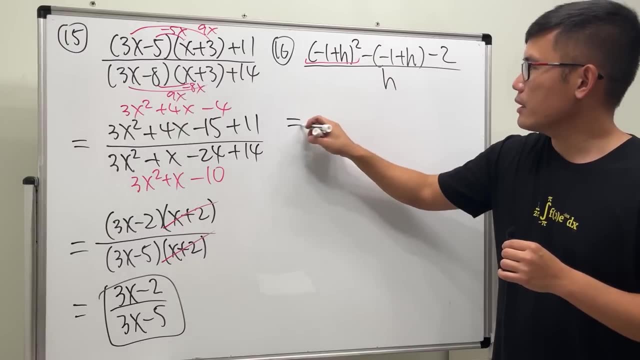 open the powers and all that, and then combine the terms and then somehow we are going to factor and cancel out the h. You'll see. First let's do this right here. Okay, this right here is negative 1 squared at, we get 1.. 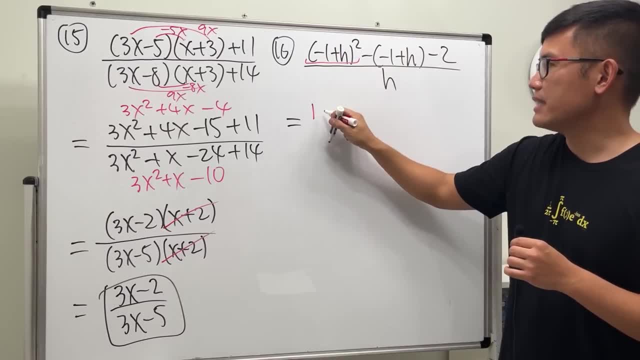 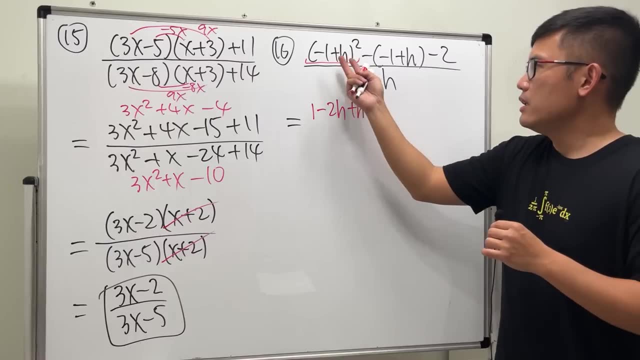 And then 2 times this and that that's negative, so it's minus, And then we have 2h, And then, lastly, h squared, Yeah, And if you would like, you can also reverse the water: h minus 1,. but 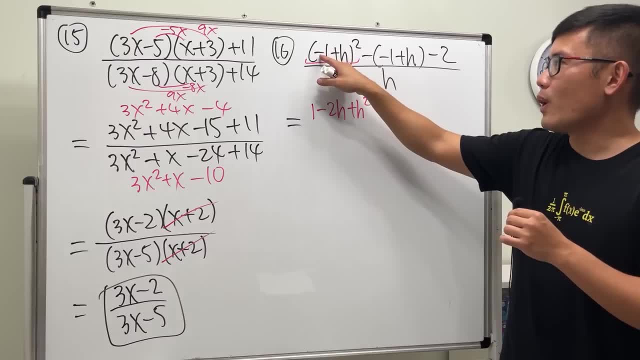 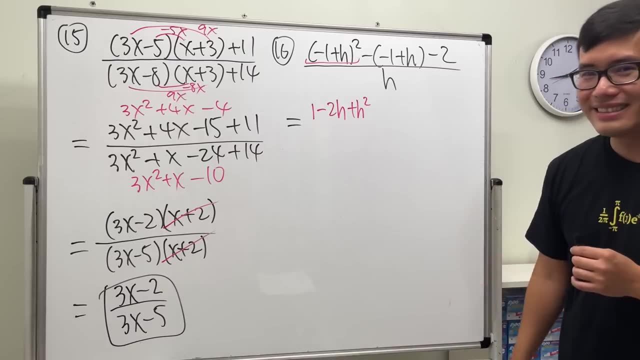 later on in calculus. well, if you're in calculus already, you'll know exactly why this is in this water, Because the definition of derivative is a plus h. You know stuff like that, Anyway. Okay, so that's done. 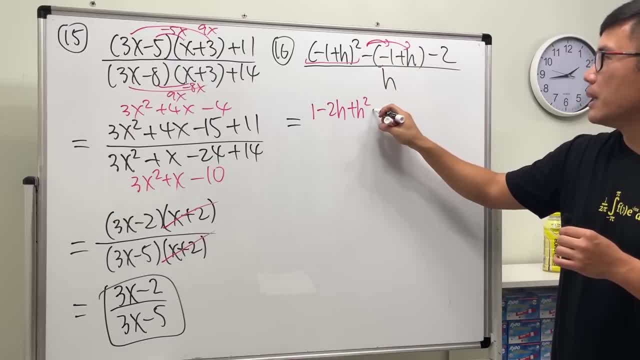 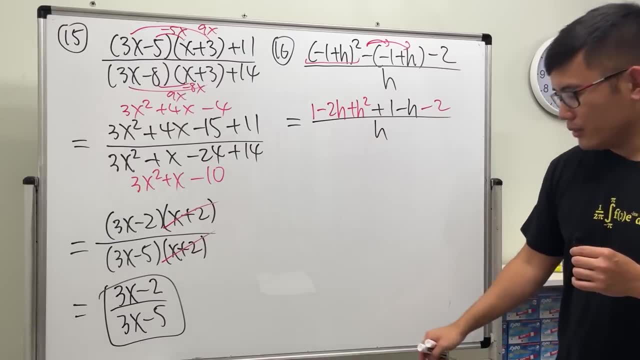 And then for this right here, just distribute it, Distribute the goal away, so we get plus 1 minus h And lastly we have the minus 2, or over h. Now we see that 1 plus 1 is 2, minus 2 is 0. 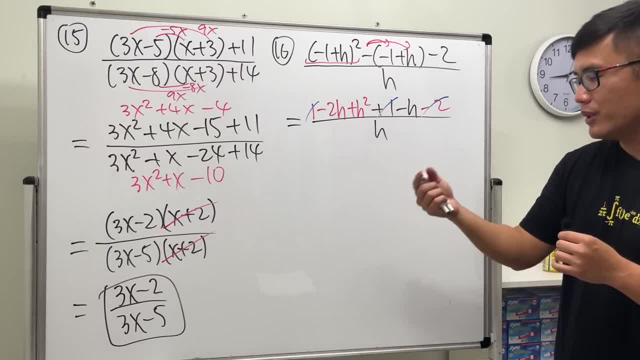 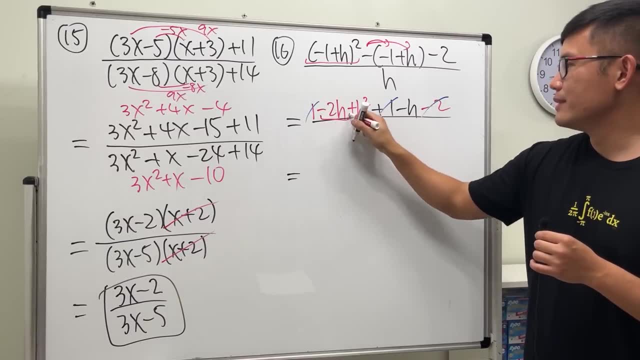 And, as you can see, this, this, and that they all have an h, So we can factor it out And notice that we can actually. Let's combine it first. Yeah, So in fact we have negative 3h plus h squared. 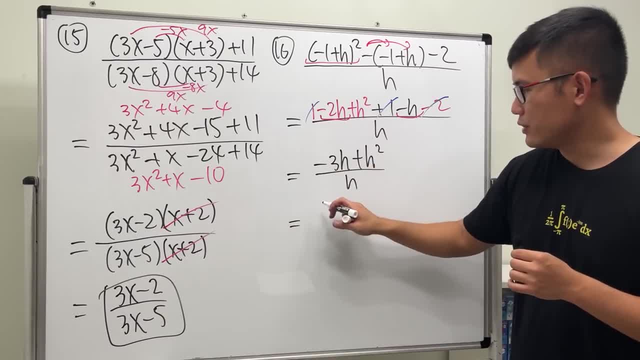 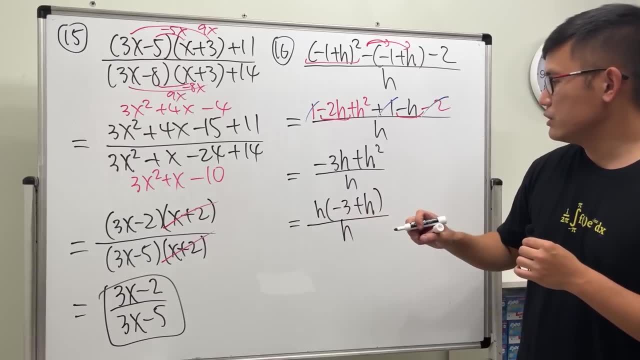 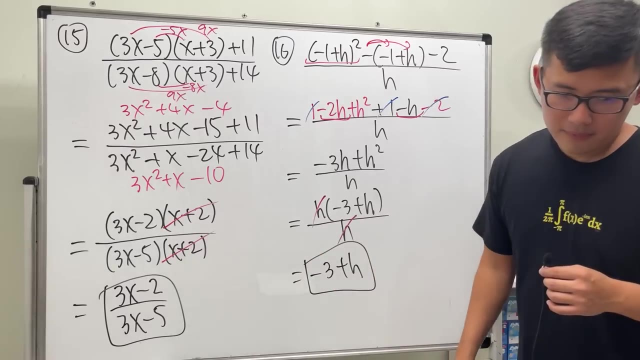 h squared over h, And then we can factor out the h And then this is negative: 3 plus h only over h. Yeah, And then cancel. cancel. Final answer: Negative: 3 plus h. Done, Yeah, just like that. 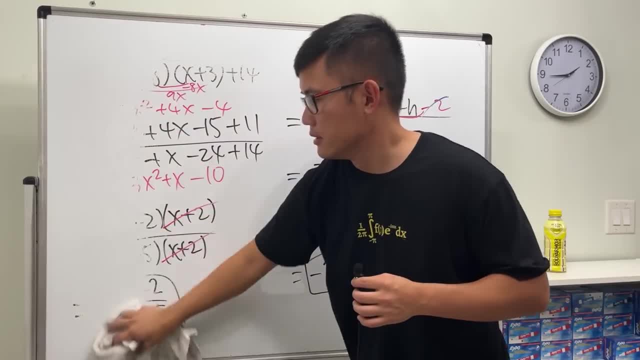 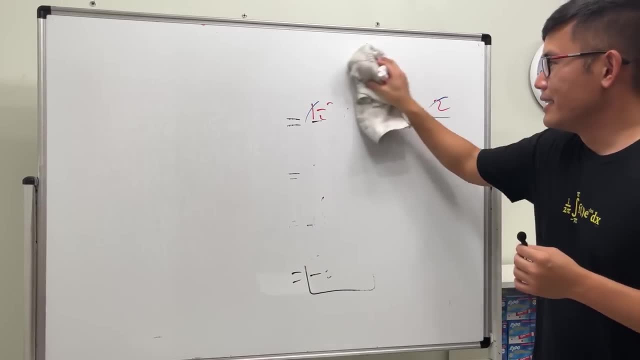 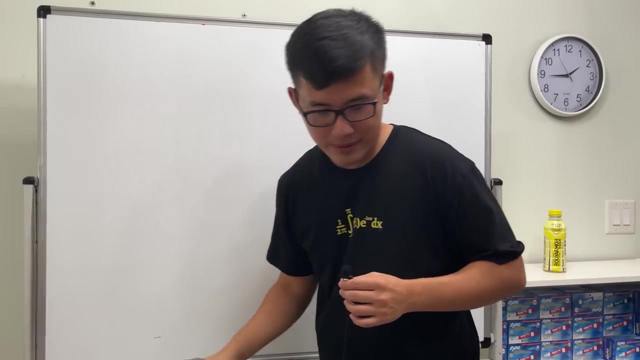 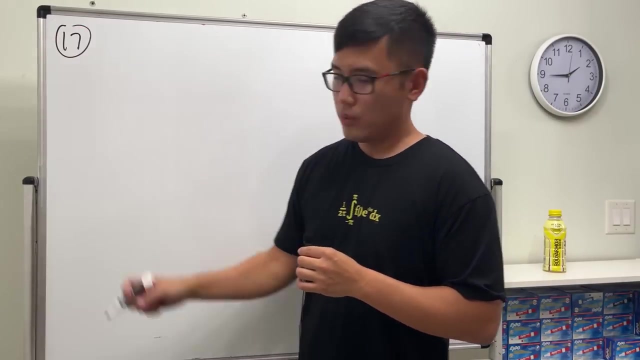 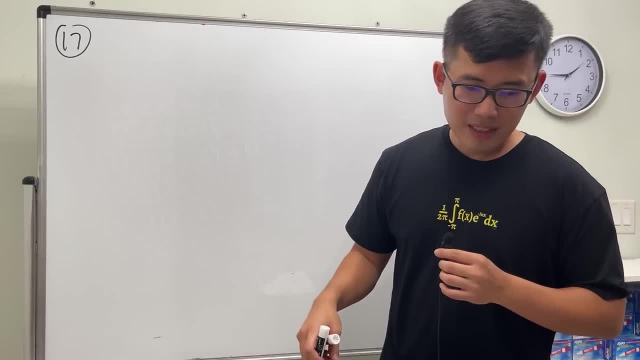 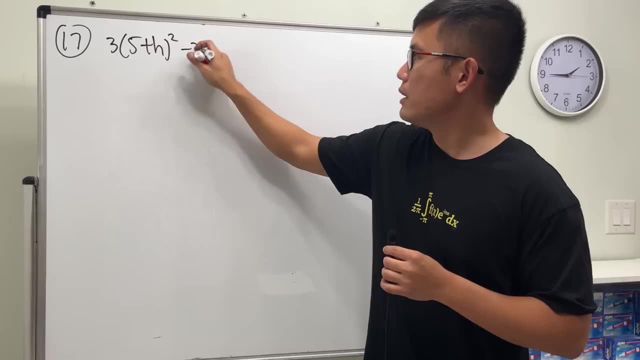 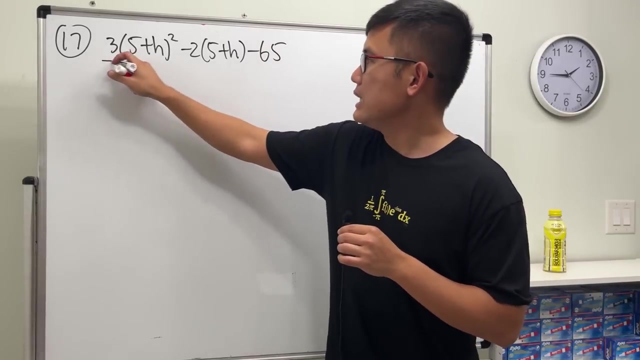 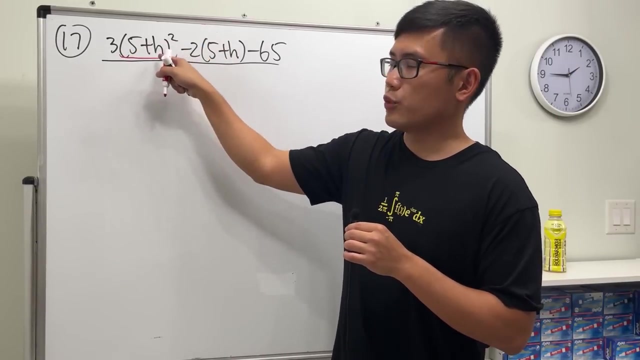 what a placing cell workout workout. workout, okay, 3 times 5 plus H square, and then minus 2 times 5 plus H and then minus 65. everybody over H just go ahead and get to work. so multiply this out. let me just put on a resort right here. 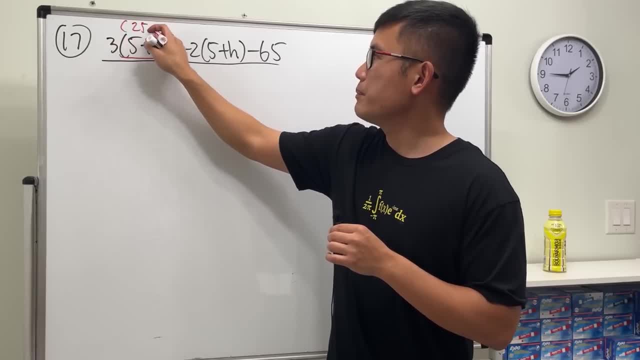 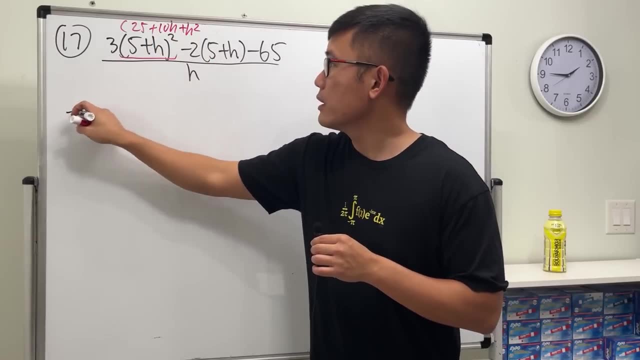 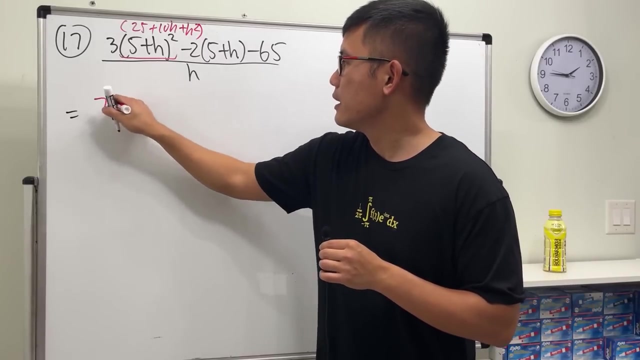 because we'll have to street at the front right. so 5 square is 25 plus 2 times this, then this now, which is 10 H, and then we have plus H square. so we take the street, distribute 3 times 25 is 75 and then 3 times 10 H is 30 H and then 3 times H. 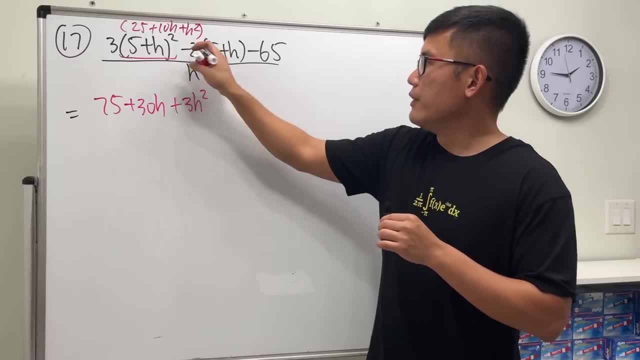 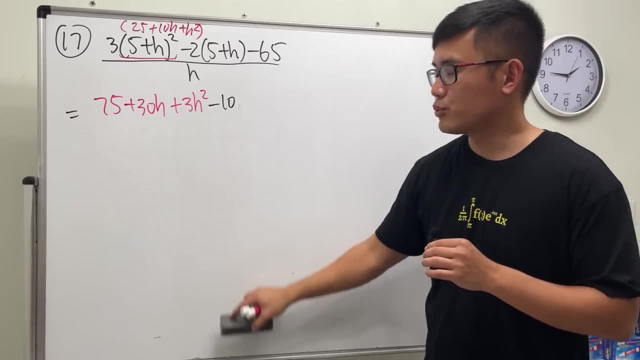 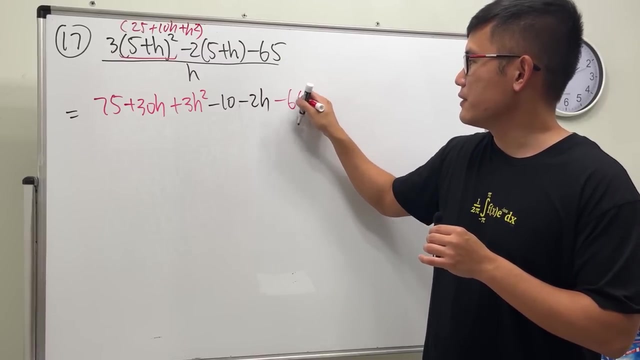 square is 3 H square and for this, right here, just multiply the L, we get negative 10 and then minus 2 H. so just be super careful. okay, number 17, each effort is not making careless mistakes, right. minus 2 H and then last you have the minus 65. 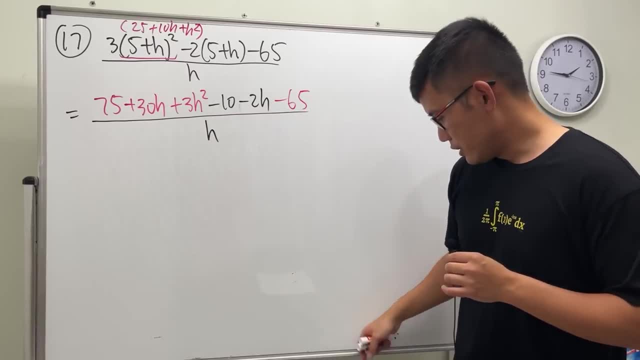 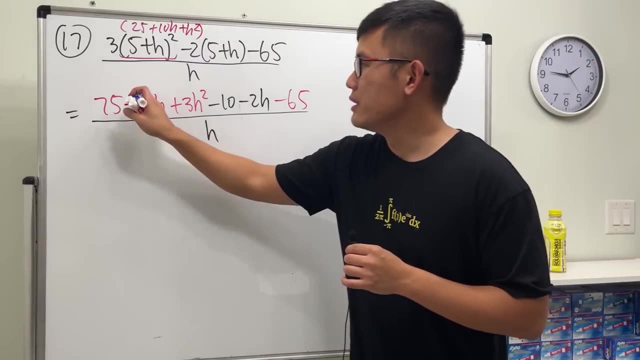 over a sheet. all right, now check this out: 55 minus 10 is 65, and then minus 65 is shareable. so this, this and that they all cancel each other out. and then we see that this and that is 30 H minus 2 H is 28 H by area through 0 and the 0 and 2 are: 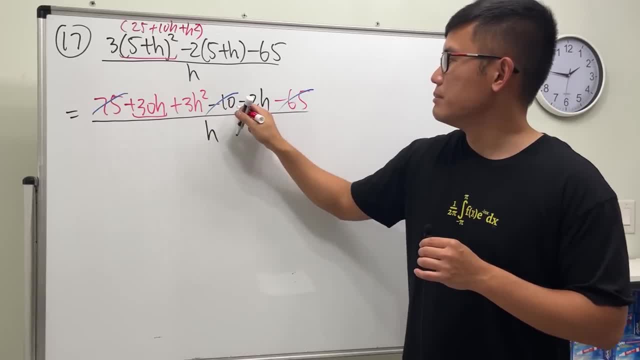 zero was equal to 7, 10 per sign number point digit, and then we got a 0 in the year los, and then we want to get over, to get over, to get over to throughout. what what I can do is try these outowie. which we talk about is that, if we talk about 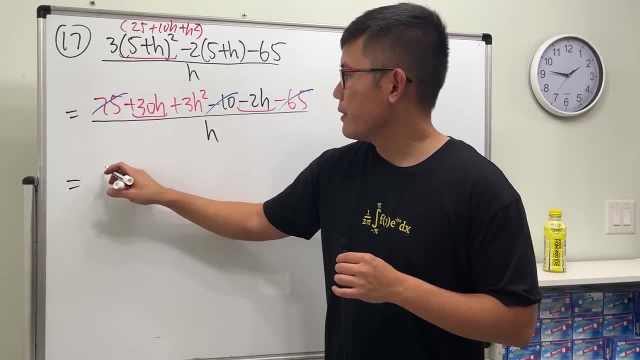 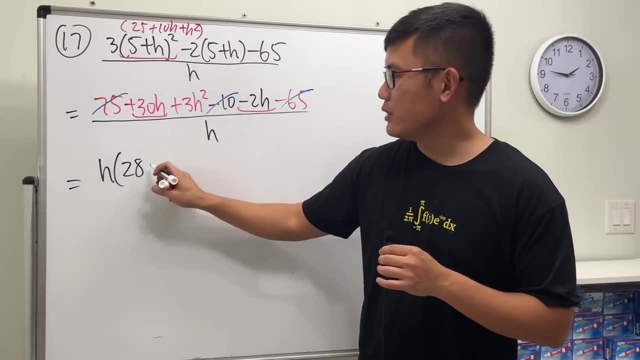 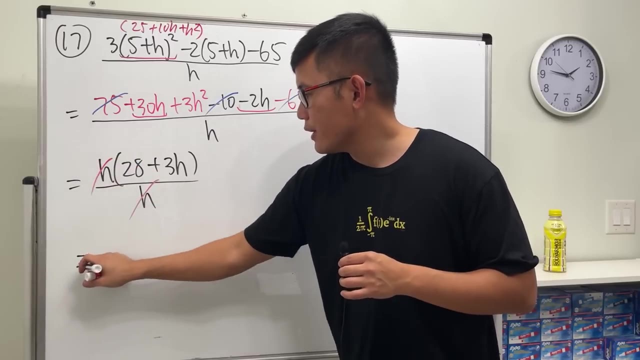 noise and говорю we kind of focused on those two presentation and get some, so we can write this: well, 28h, that's factor on h, so just be 28, so save a step right here. and then we took out the h, so this right here is 3h all over h, h cancel. so we just have 28 plus 3h. 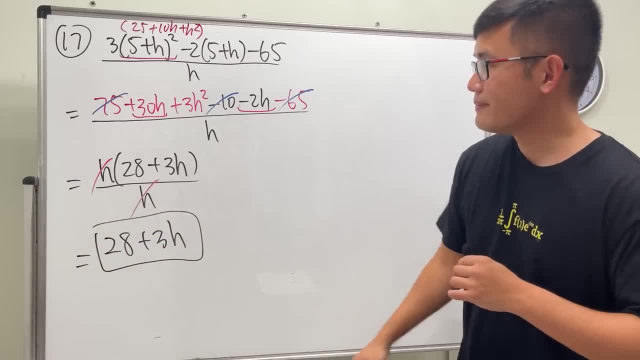 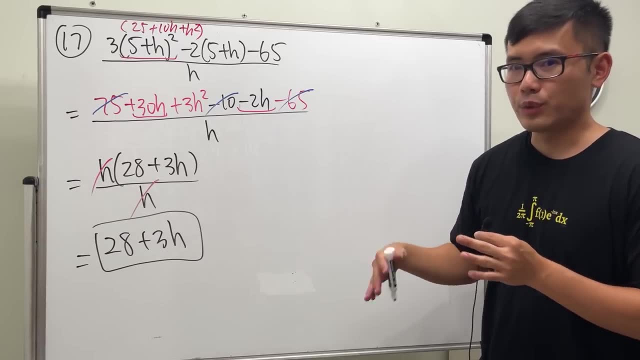 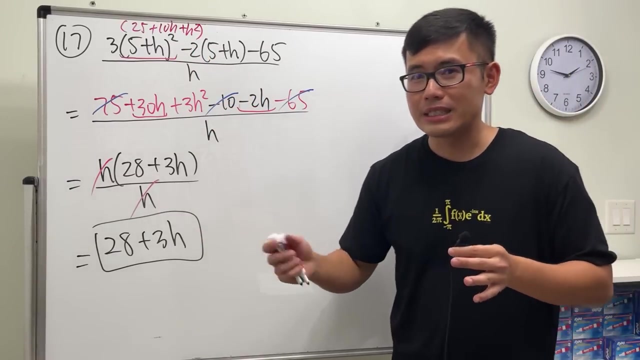 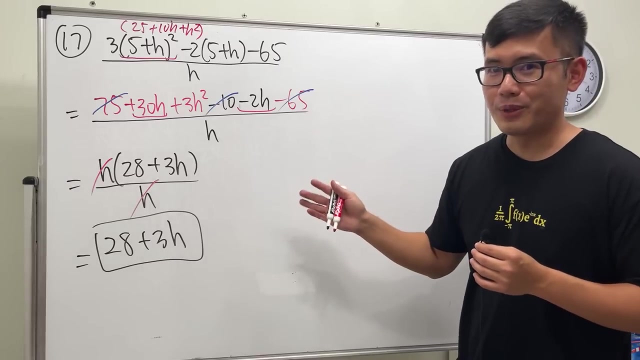 just like this, yeah. so let me just tell you guys this real quick. sometimes we may make like small mistakes or careless mix, like why about what? what i was doing earlier, right, forgot a number. or like add it wrong, subtract it wrong in the learning process it's okay as long as you know what to do. that's the most important part. and then 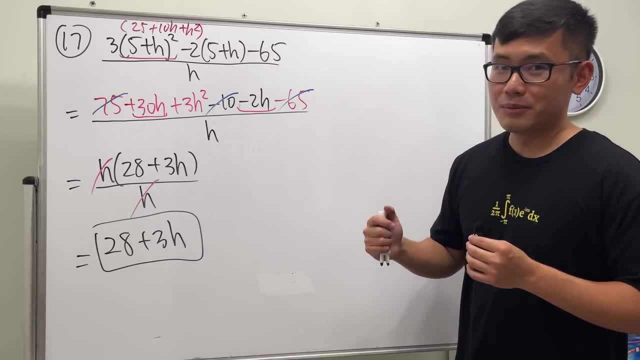 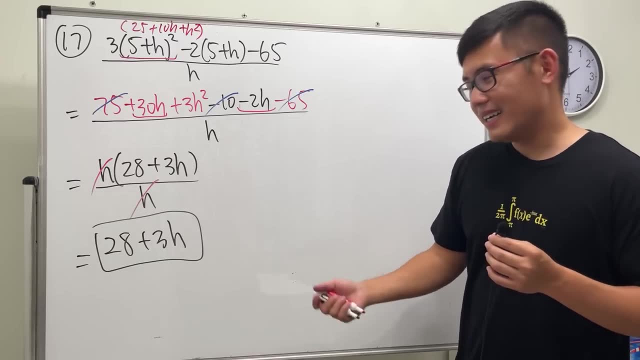 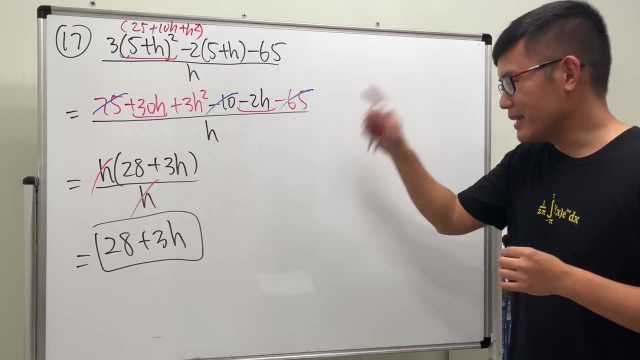 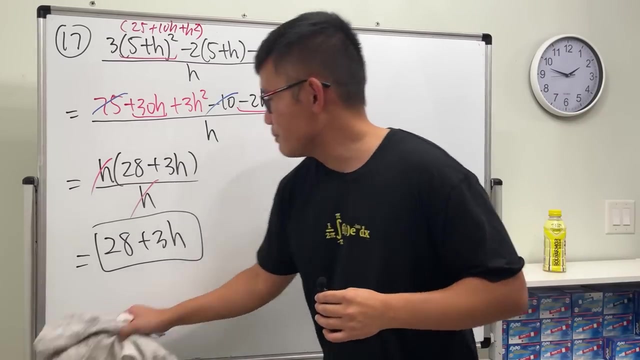 i might make a lot of mistakes here. the reason is because why am i doing this in the midnight? i don't know. no, i know the answer: because i don't really have time in the mornings and all that stuff, and yeah, anyway, let's just continue. all right for number 18. let's just have more space, so i'll be happier. so let me just erase this. 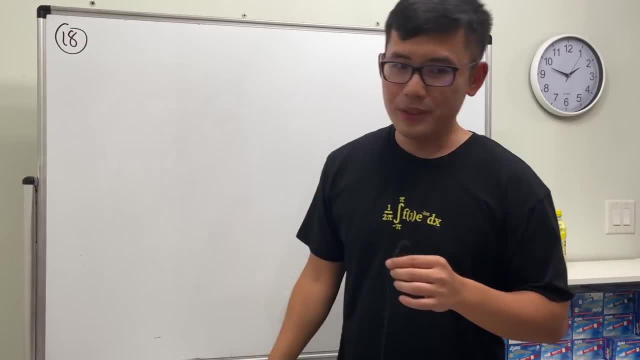 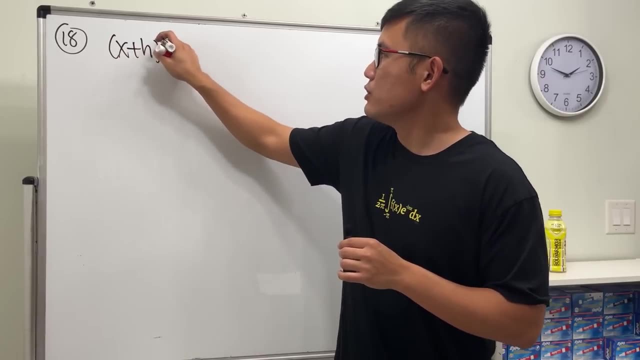 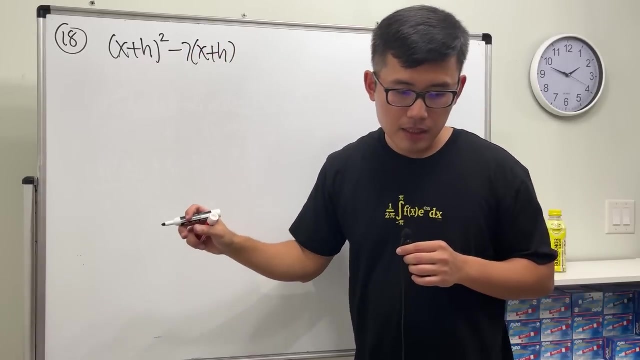 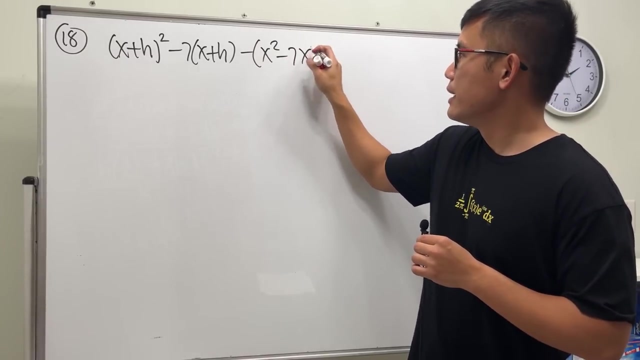 all right, number 18: crazy equations. it's not just with h but also x, so x and h together, first x plus h, square, and then minus seven, x plus h, like this, and then minus parentheses, x square, minus seven x, and you know it all over h. 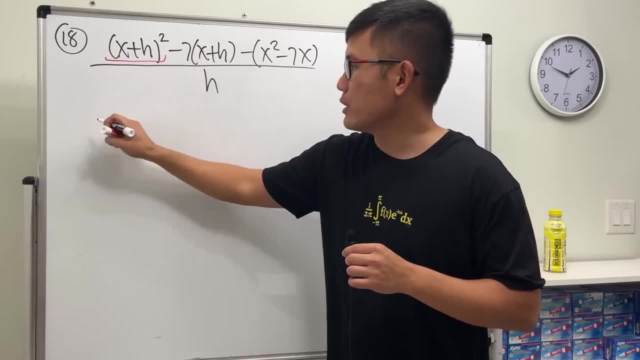 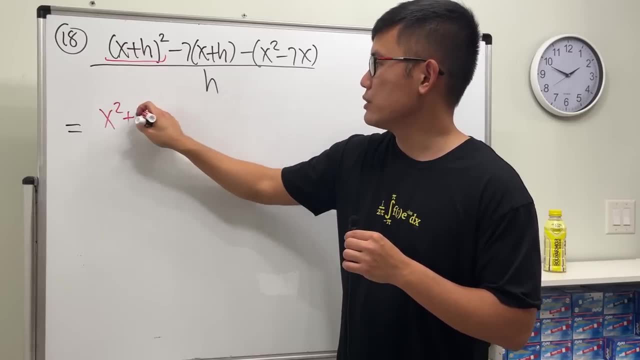 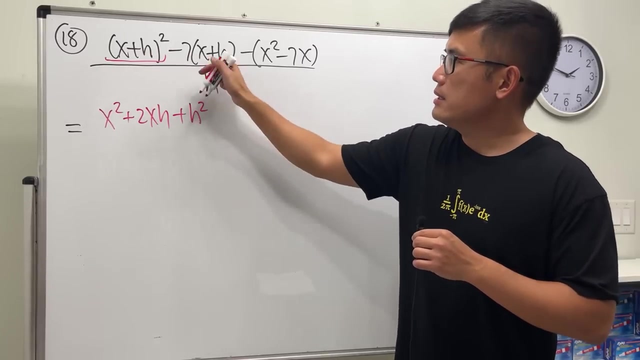 all right, that's just go ahead and get to work. so for this part it's not bad. we can just multiply the out like how i showed you guys earlier. so x square plus two times this and that which is two x h, and then plus this thing squared, so plus h squared for this, distribute so we get negative. 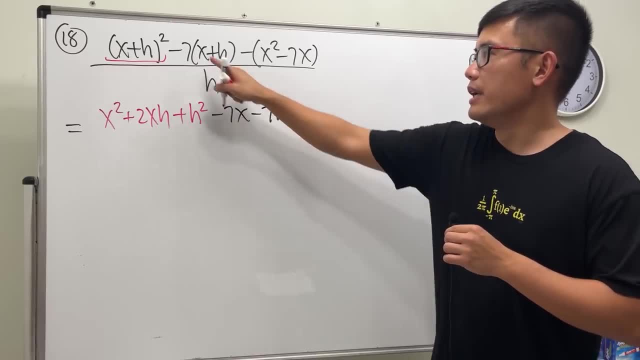 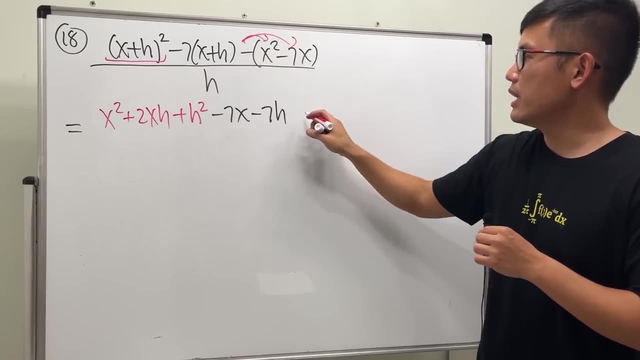 seven h and then minus seven, sorry, negative seven x and then minus seven h. and then, for this right here, just distribute, right. distribute, so we get negative seven x and then minus seven h. and then, for this right here, just distribute, right. distribute, so we get negative x squared plus seven x everybody over h. 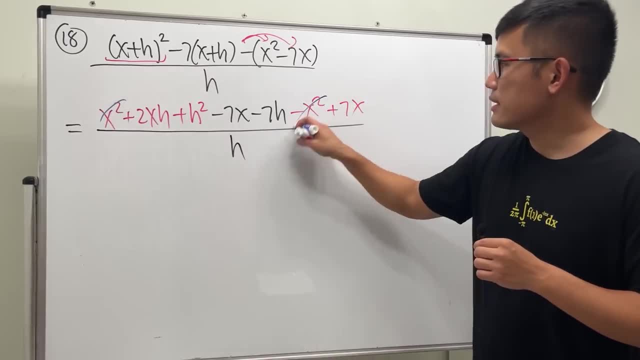 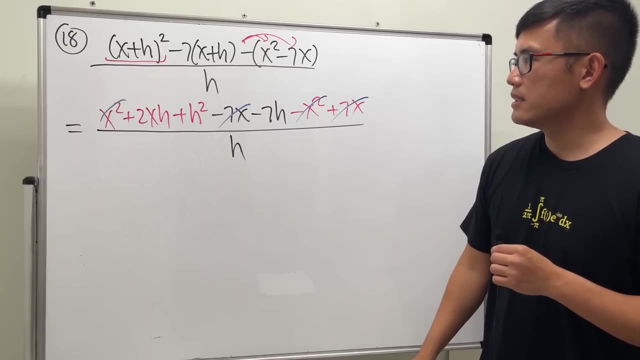 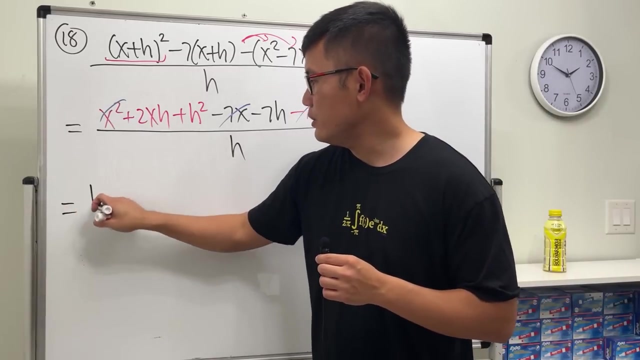 now happy cancelling: x square, x squared. cancel negative 7x plus 7x. cancel. very, very nice, that's about all. and for the remaining things, everybody has an h, so let's factor it out. so we have the h and then 2x from here. 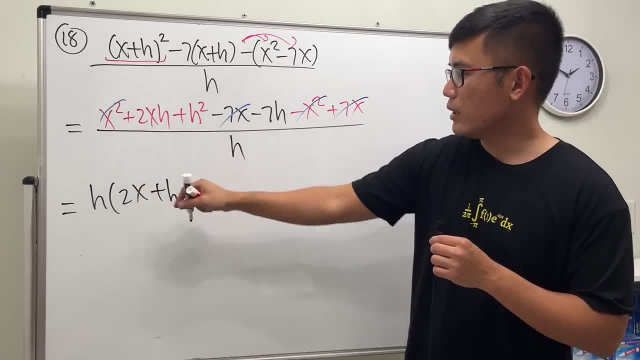 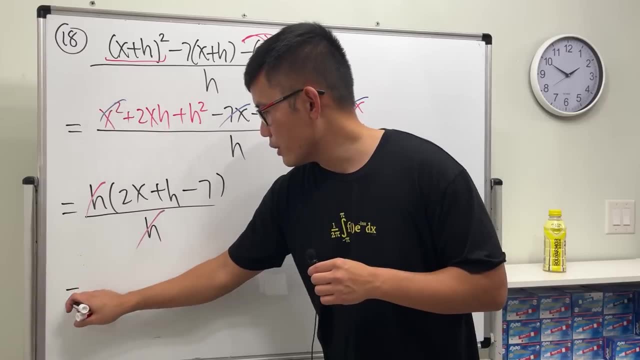 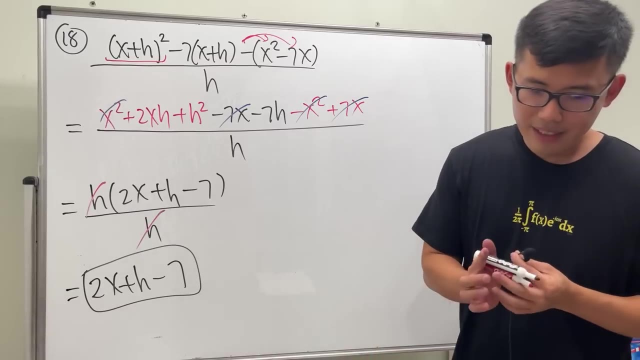 is h, square took on h, so it's just h, and then the h is out, so we have the minus 7 all over this h and the h cancel. cancel. so 2x plus h minus 7, done. okay. the question is actually getting bigger and bigger, because when i was coming with these, 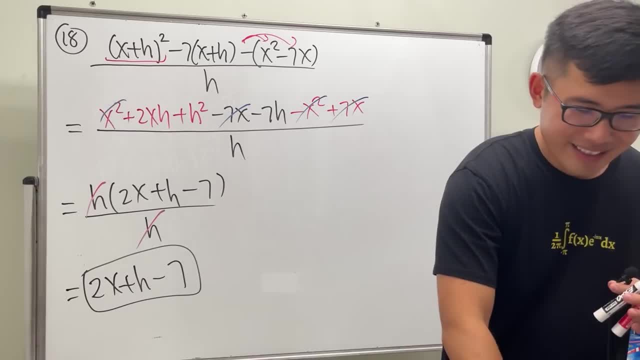 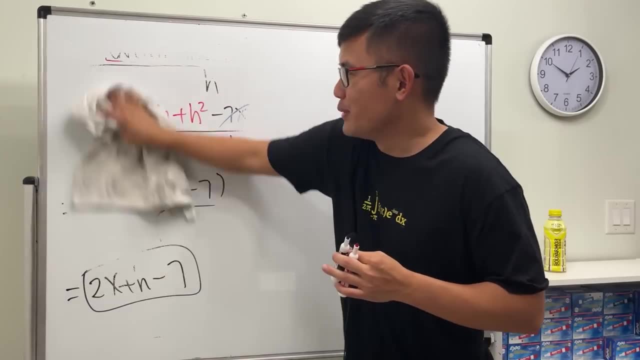 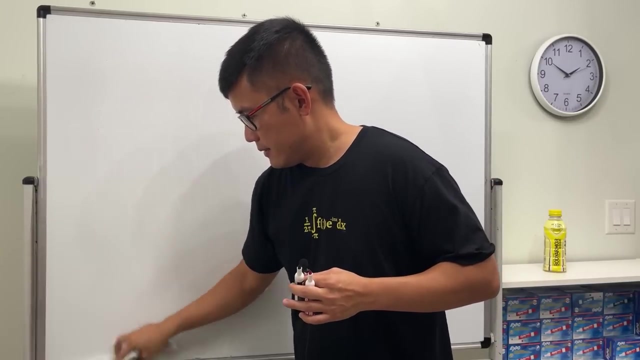 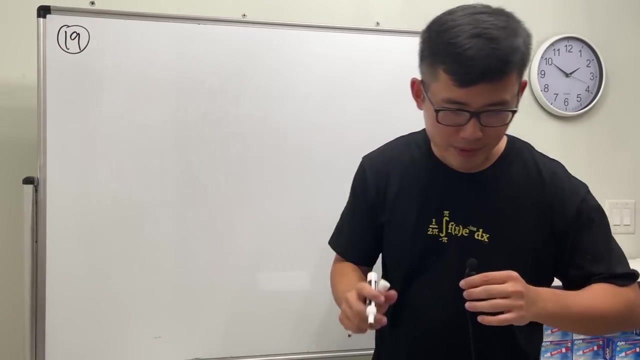 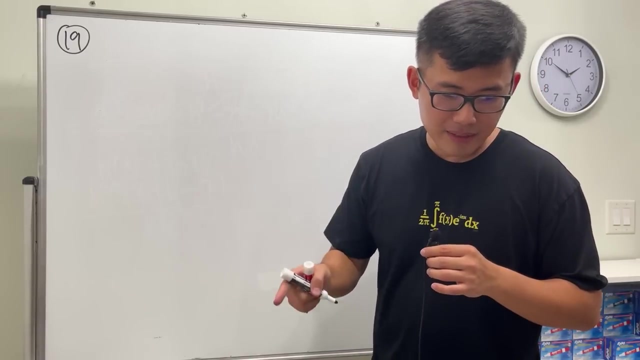 questions. yeah, i still want to increase the difficulty. yeah, to entertain, not only for myself, but also try to entertain you guys. so i need to erase this again. all right, number 19: crazy questions. it's october, so halloween's coming anyway. number 19. first we have 3 plus h to the third power and then minus. 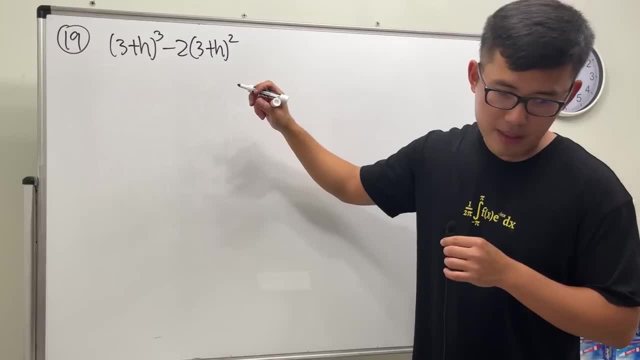 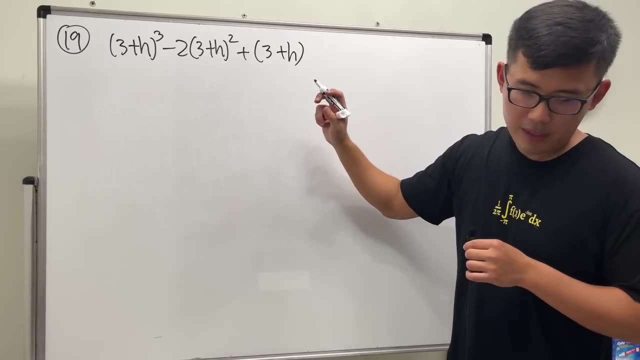 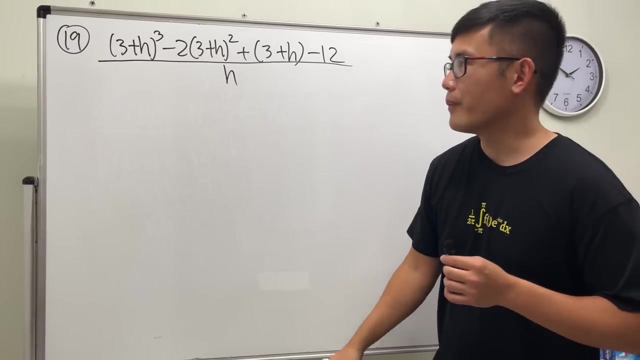 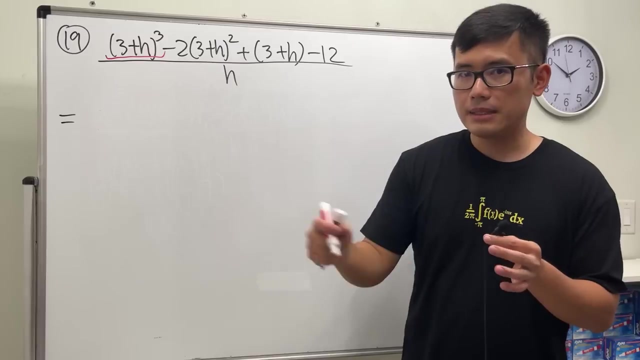 2 times 3 plus h square, and then plus 3 plus h and then finally minus 12, like this all over h. here we go. this right here has the third power. So it's your call If you want to write it down three times and multiply things out. 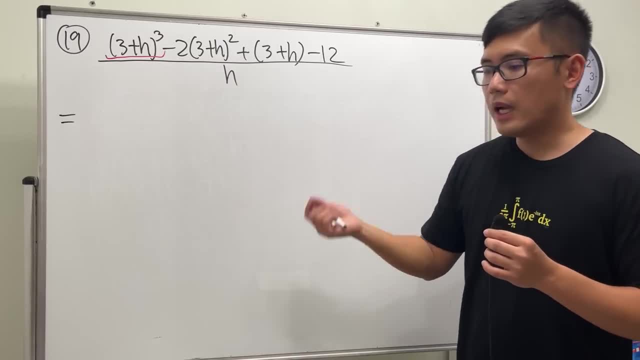 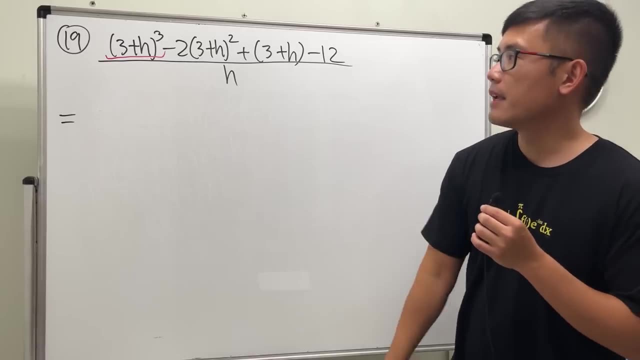 or use the formula I showed you guys earlier. I will use the formula I showed you earlier. If you want to multiply it out, just do it on your own and then try to see. your answer is the same as mine. Firstly, I'm going to take the 3 and then cube it, which is going to be 27.. 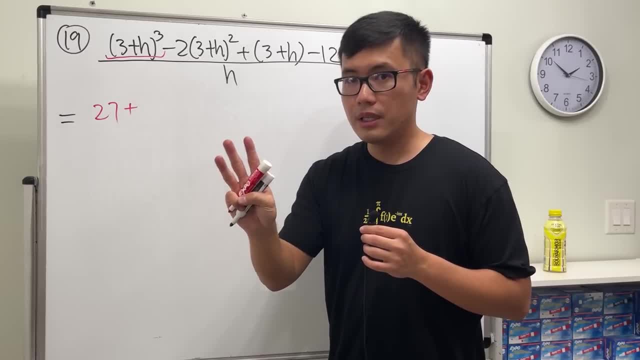 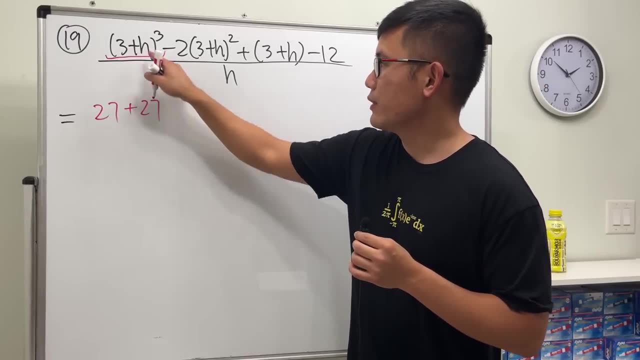 Next we are going to add the coefficient 3 times 3 squared, which is 9.. So 3 times 9 is 27.. And then we have to introduce the h, Then the coefficient is 3, times 3 to the first power, which will give us 9.. 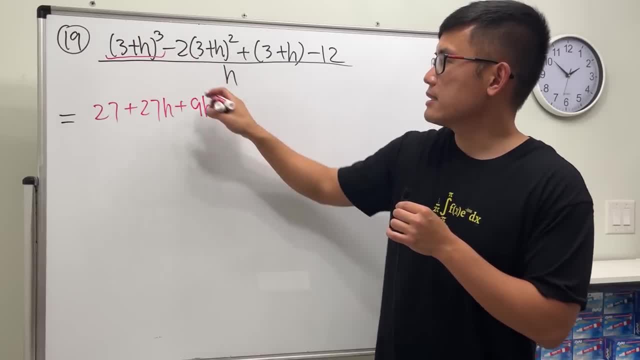 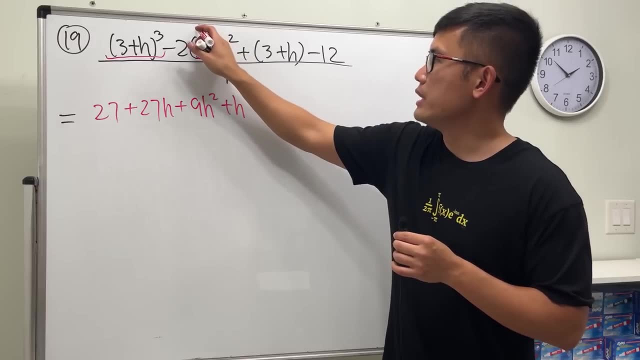 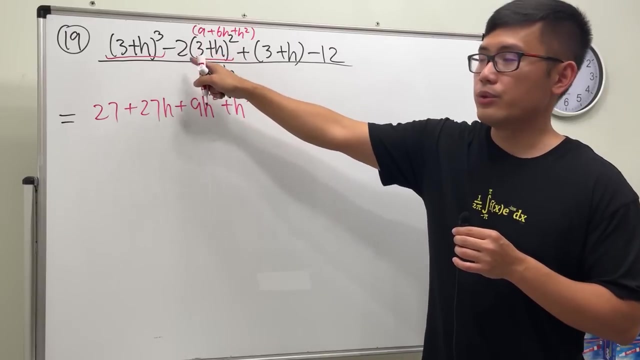 And then introduce the h again, so h squared. Last the h to the third power, And then, for this right here, when we multiply this out, we get 9 plus 6h plus h squared. and then multiply out the negative 2, right. 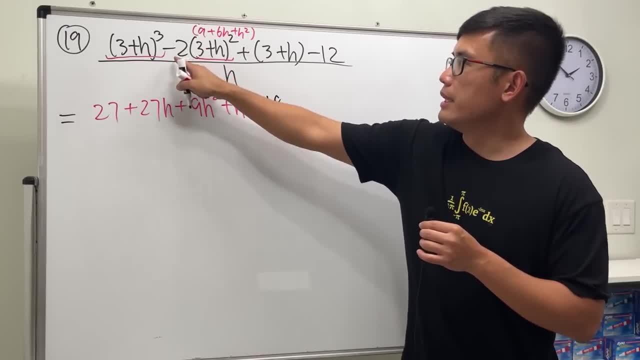 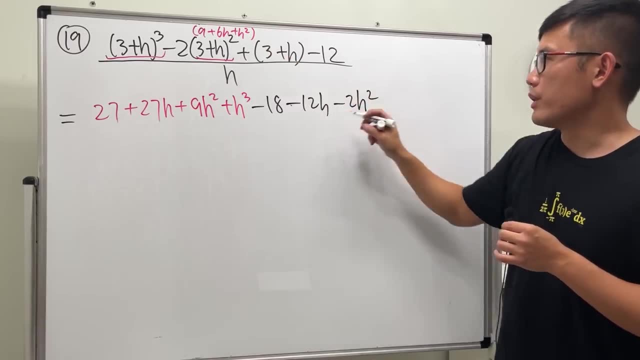 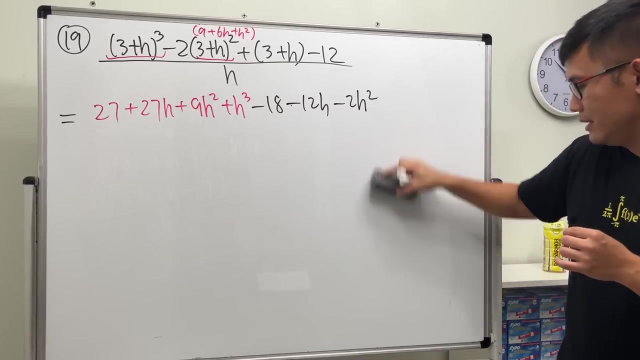 So we get negative 18. And then minus, Minus 12h, And then minus 2h squared, And this right here with parentheses doesn't matter. So plus 3 plus h. I will change this to red so that it's easier to see. 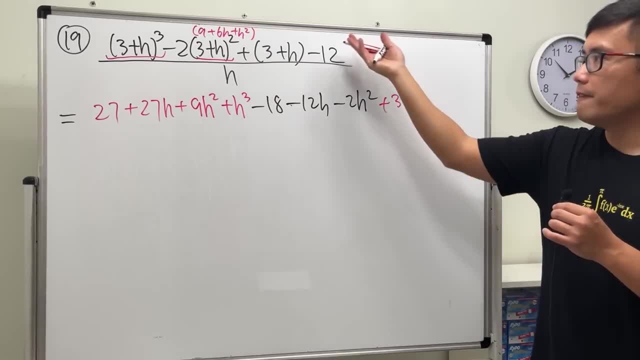 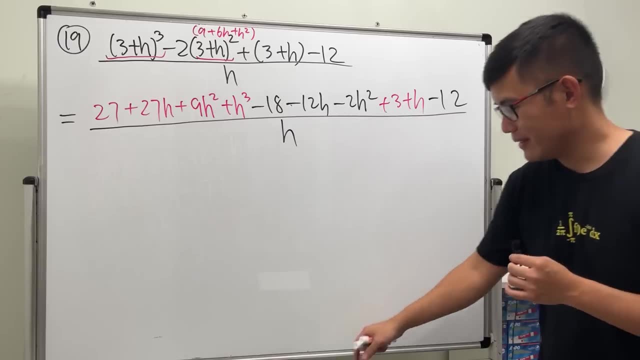 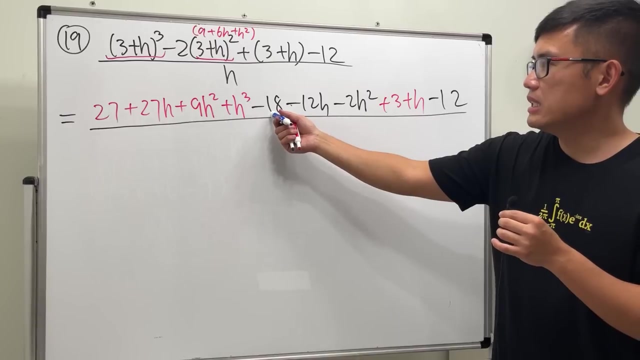 This right here is just plus 3 plus h. Finally we have that minus 12.. All over h. Okay, you know the blue pen. Let's see: 27 minus 18 is 9.. 9 plus 3 is 12.. 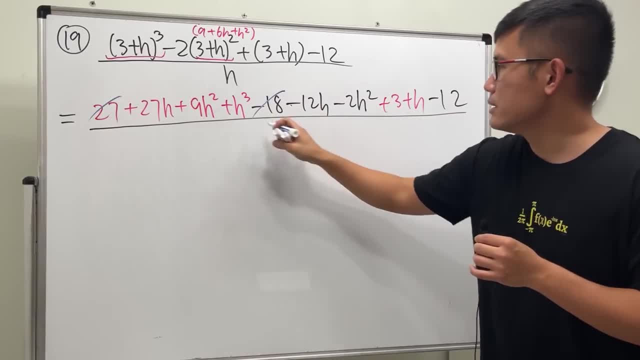 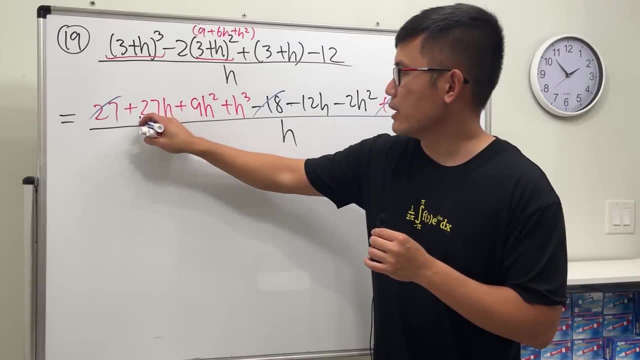 Minus 12 is 0.. So in fact, this cancels out with this, this, that Perfect. And then we can combine all the h's terms as well, right? So this is 27h minus 12h, and then plus one more h. 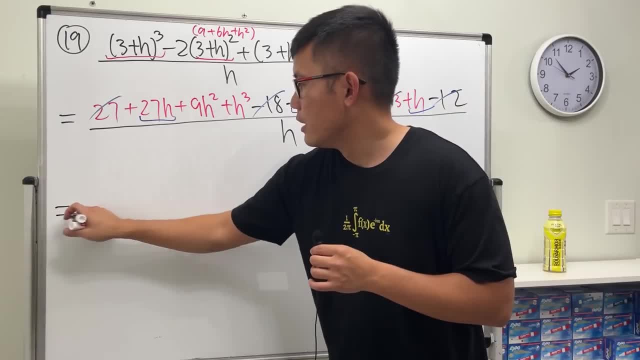 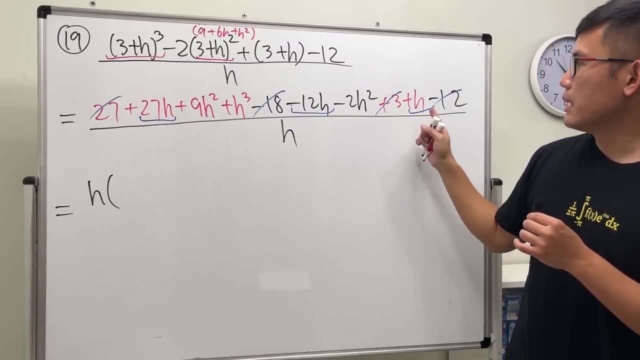 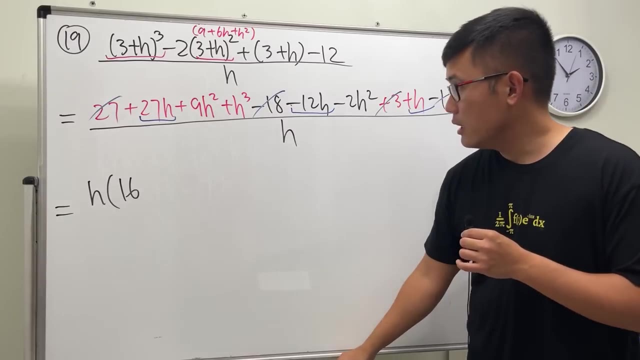 So let's see, Let's factor out the h and let's see how many is that? 27 minus 12 is 15 plus 1. So 16. And then the h is out already. And then next we have the 9h squared minus 2h squared. 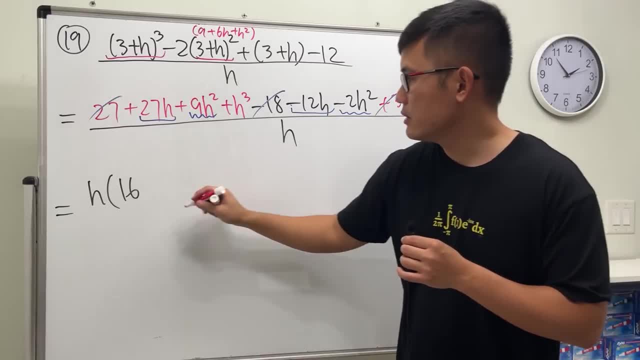 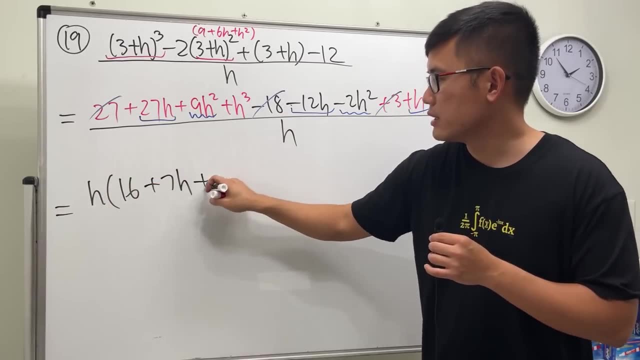 But we took on h already. 9 minus 2 is 7.. So this right here is plus 7h. And lastly, we have the h to a third power. We took out one of them already, So this is plus h squared. 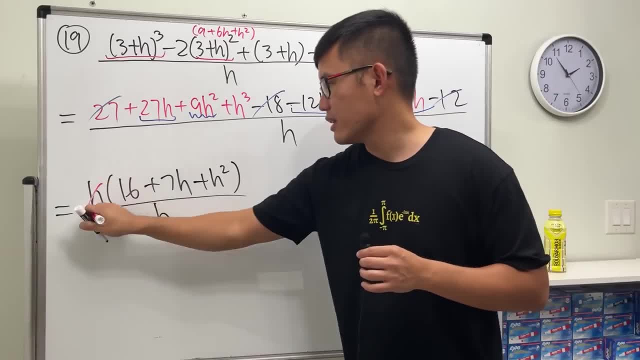 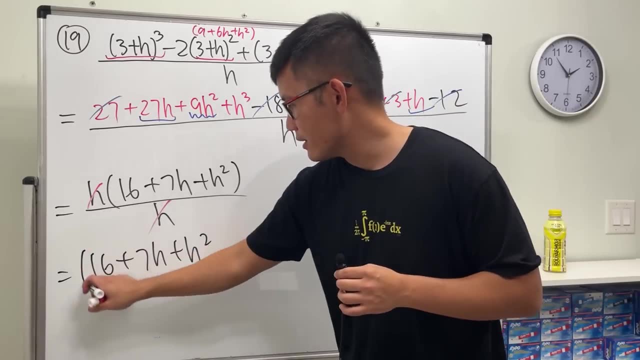 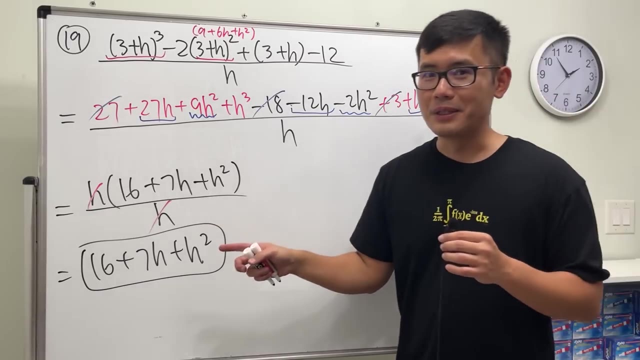 All over This little h, Cancel, cancel, 16 plus 7h plus h squared, And we are done. And of course, if you write it down the other way, it's okay too. Yeah, And in fact, in calculus, once you have all this right here, 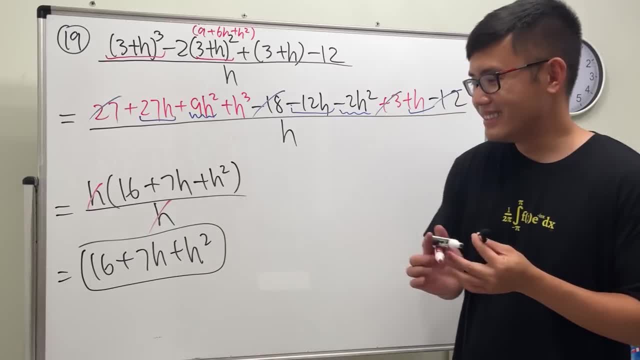 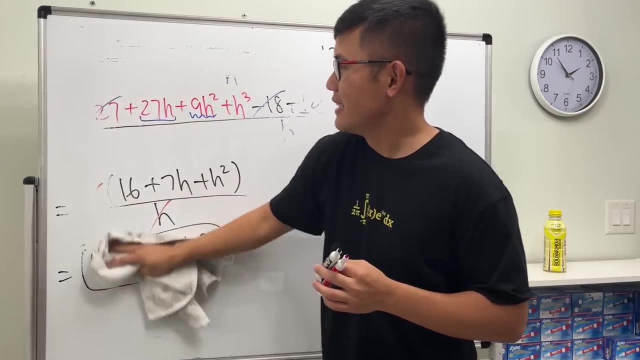 you are going to plug in h equal to 0.. Yeah, So if you have seen that part already. yeah, you know you are doing the derivative. Yeah, especially with the definition. Yeah, Like you are going to plug in h equal to 0.. 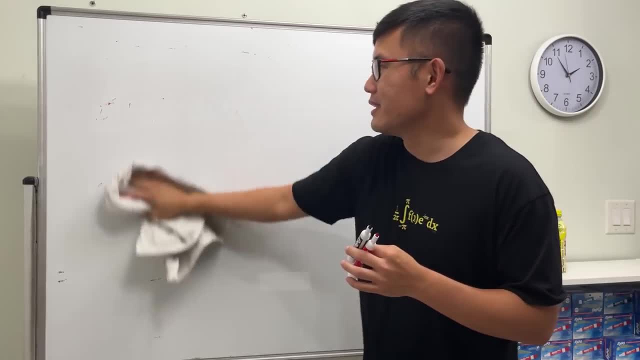 And so that's the first thing that you are going to do, And then, if you have any other questions, I'll leave it here, just in case you have any other questions. But I think we are going to talk about algebra in the next part. 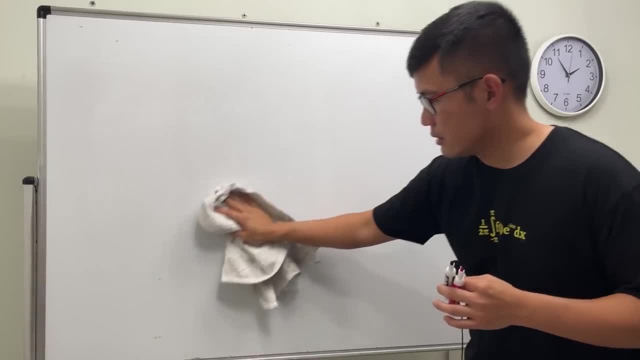 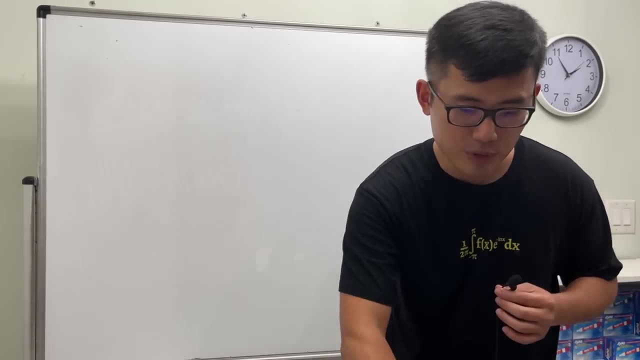 So I'll leave it here, just from here, And then that's one of the first few things that you guys will do in calculus. And, yeah, a lot of algebra. I'll tell you Number 20, perhaps the longest, definitely the longest one right here. 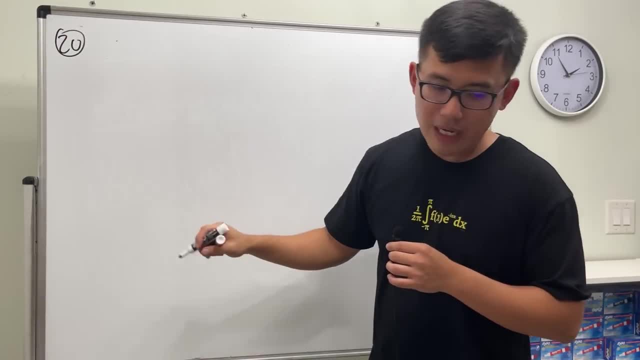 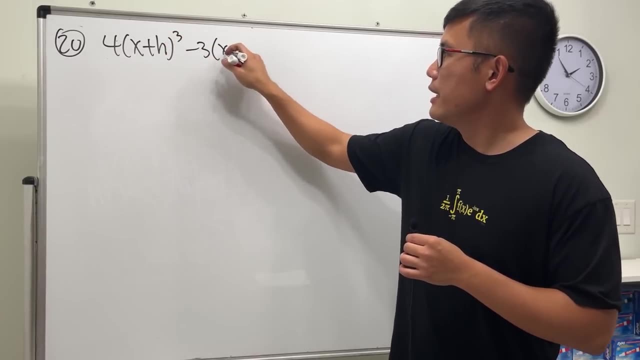 Okay, Number 20.. Here we have 4 times x plus h to the third power minus 3x plus h. And then you have 4 times x plus h to the third power minus 3x plus h. And then you have 4 times x plus h to the third power minus 3x plus h. 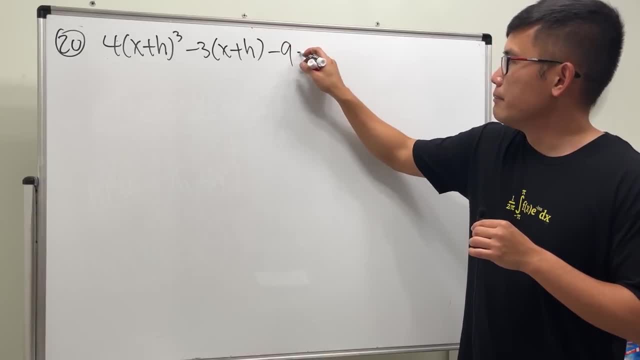 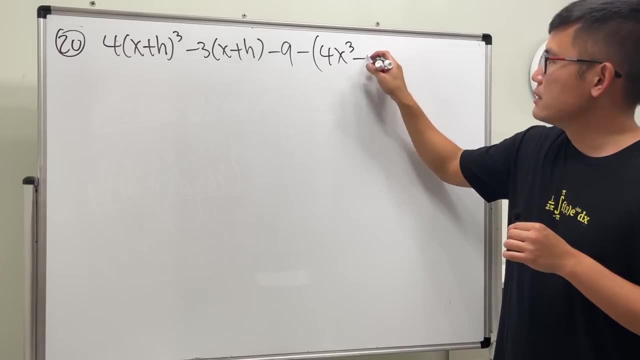 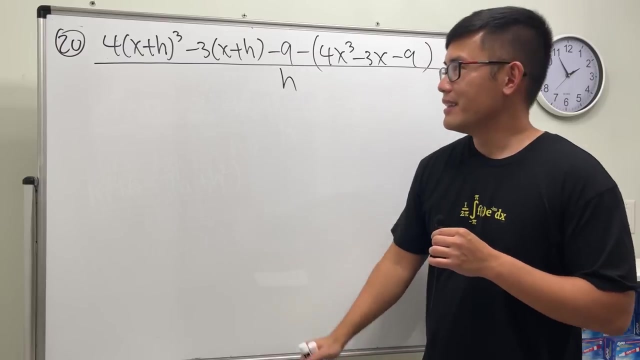 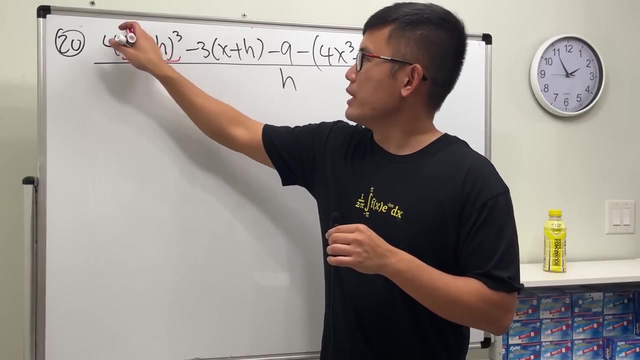 and then minus 9, and then minus a big parentheses, and then here we have 4 x to the third power minus 3x, and then minus 9 all over. you know it? h? okay, let's multiply this out, wow. and then we have a 4 at the front. so i'm going to put on the result on the top. so we get x to the third power plus 3x. 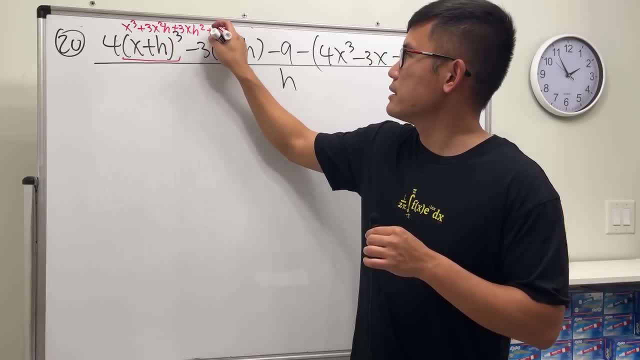 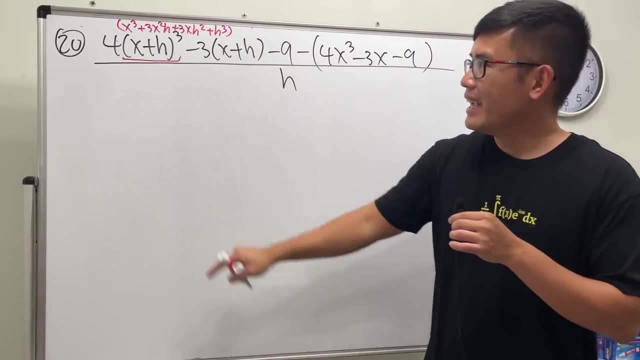 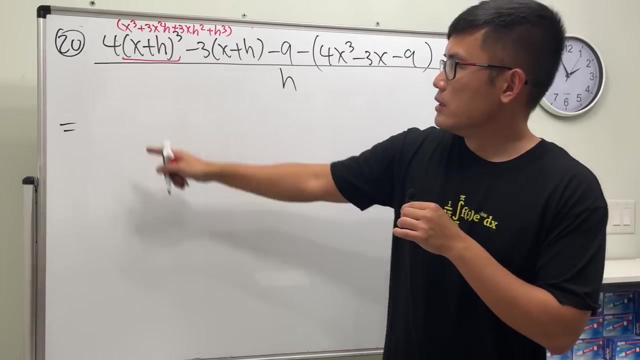 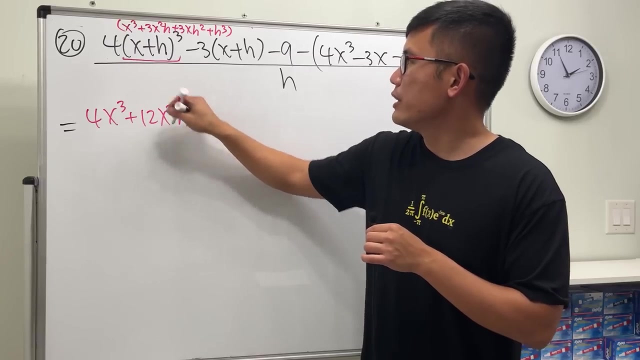 square h plus 3x h square plus h to the third power. it's just a formula, i told you earlier, with x and h instead of a and b. all right, then put the two and distribute the four into all the terms inside, so we have 4 x to the third power plus 12 x square h and then plus 12 x h square. 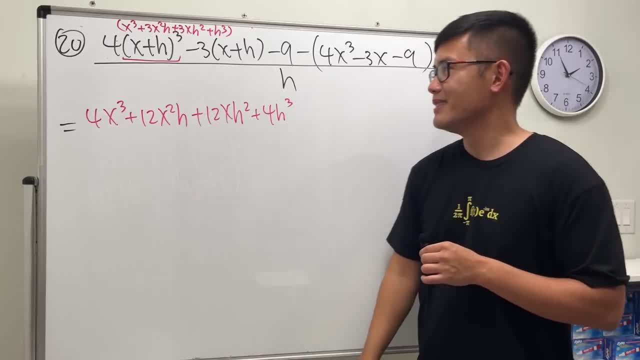 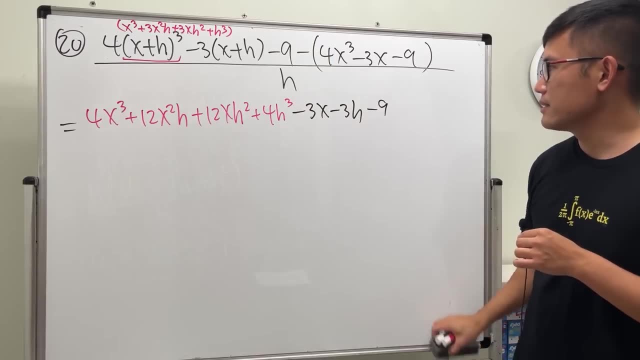 and then plus 4 h to the third power you, and then for this, right here we have minus 3x, minus 3h, and then minus 9, minus 9. let's just alternate the colors, so minus 9, and then distribute the negative, so we have negative. 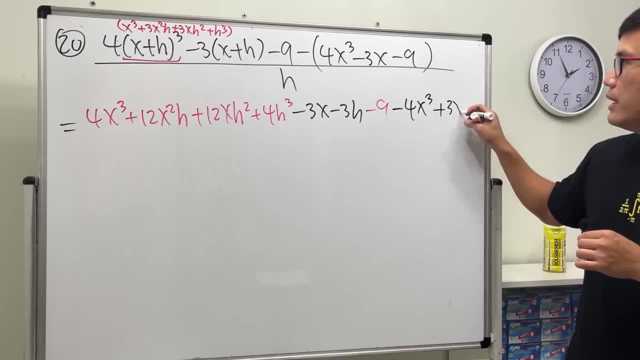 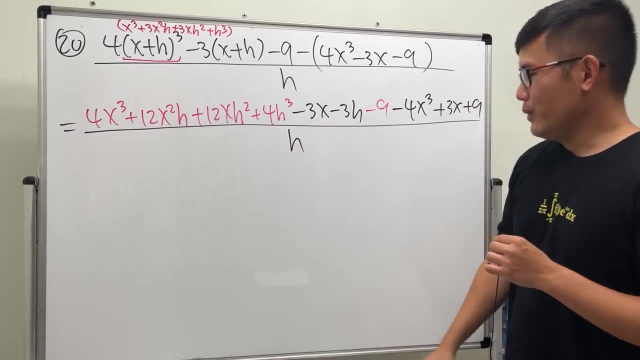 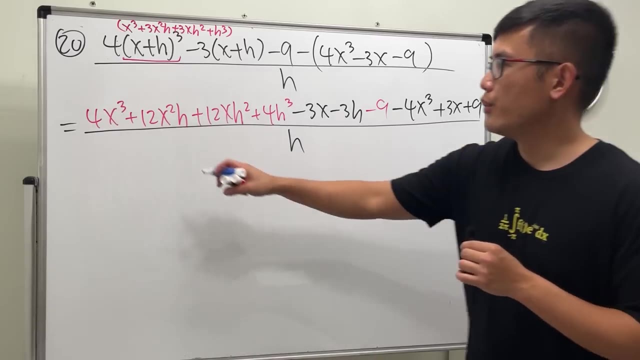 4 x to the third power, plus 3x and then plus 9. all right, all over h. okay, blue pen time. let's see, let's see, let's see. ah. 4x to the third power. cancel starts with this negative. 4x to the third power. 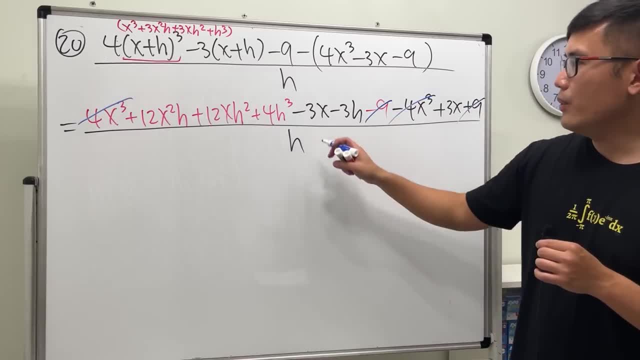 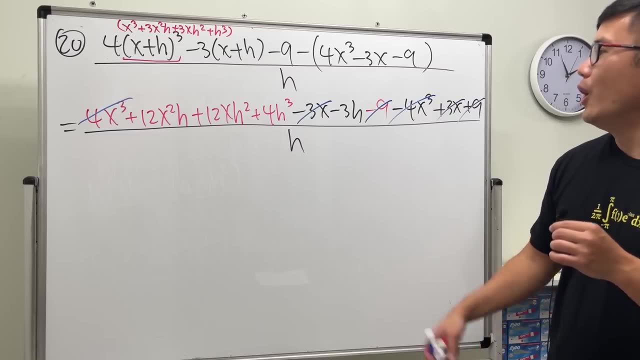 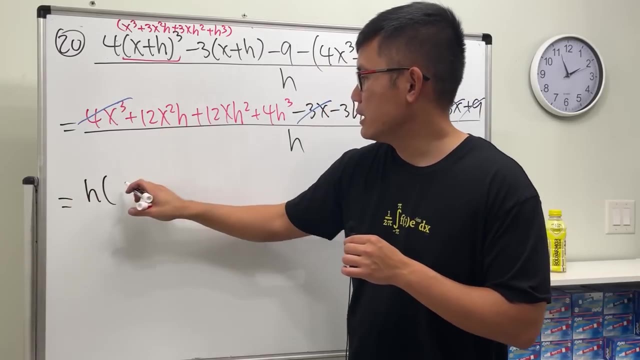 minus 9 plus 9. also cancel. oh, negative 3x. what are you doing here? right, cancel them out. good, okay, that's about that's factor of the h. then huh, so we have h, and then, right here, this is 12 x square plus 12 x, and then one more h, and 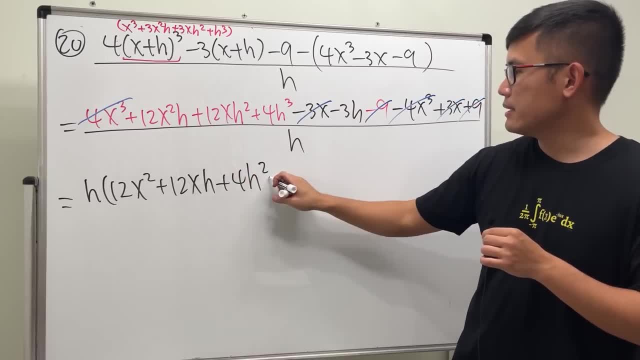 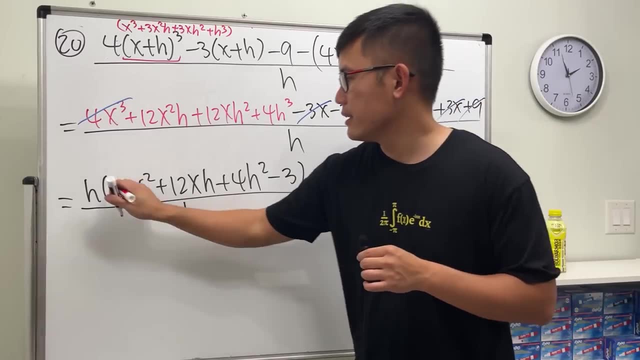 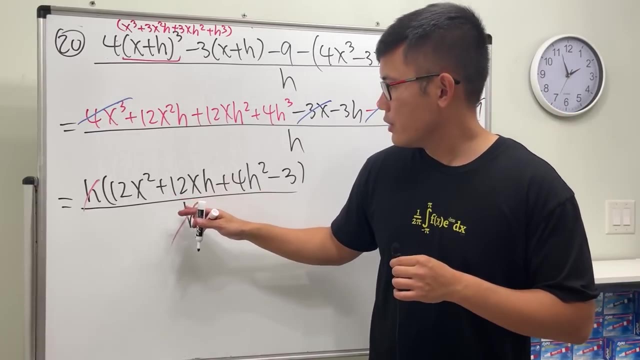 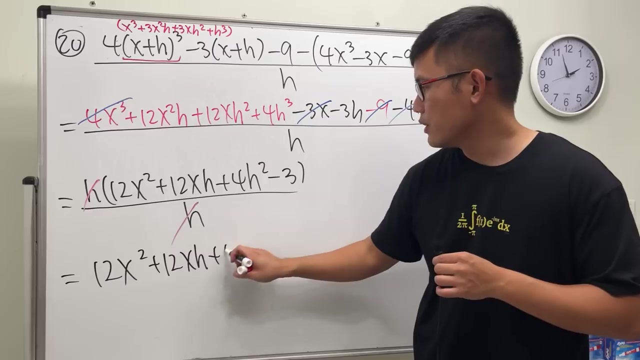 then plus 4h square and then minus 3, right, yeah, and then all over h, and then cancel this out. yeah, so 4h square 12x h. yes, yeah. so i'm just going to leave it like this: 12x squared plus 12 xh plus 4 h squared minus 3.. right, yeah. 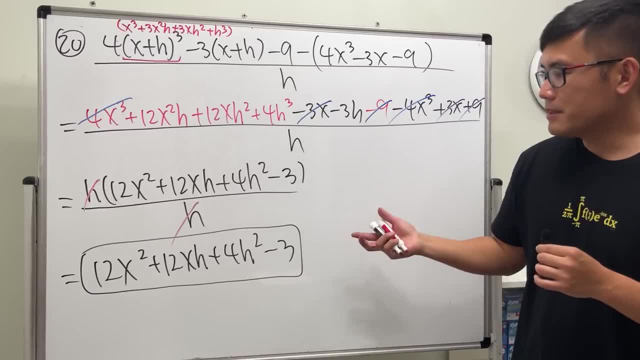 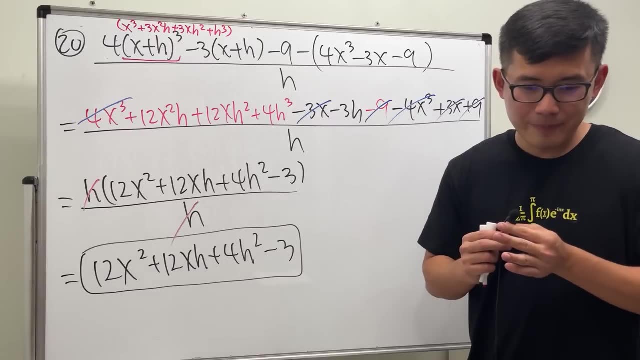 and the reason i have the answer is because sometimes, especially later on, you don't know when and you don't know which phone that you want to stop. and um, i'm going to. if i want to give this as like a quiz for test to my students, i will make this into like multiple choice. 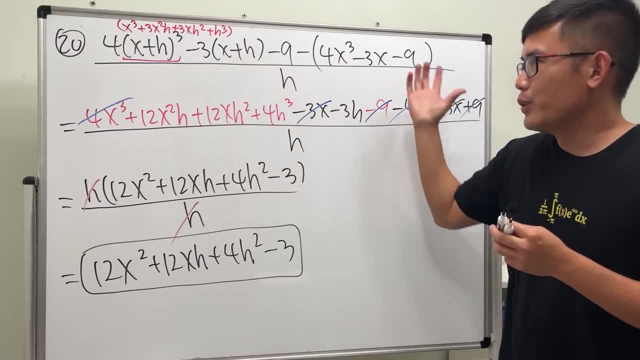 if i want to give this as like a quiz for test to my students, i will make this into like multiple format, like I give you a huge algebraic expression and I'll give you three or four answer choices. you just have to do enough algebra work and make sure your 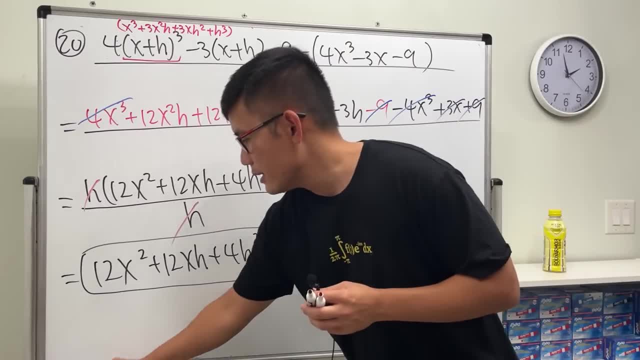 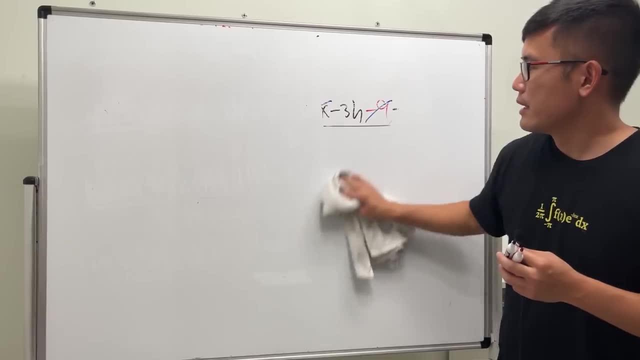 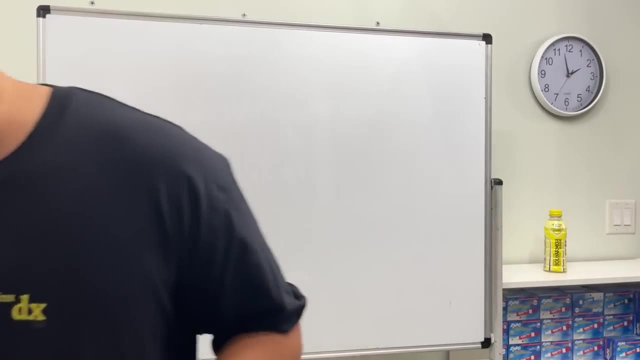 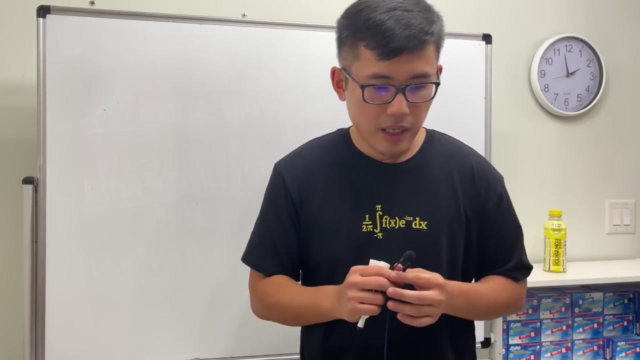 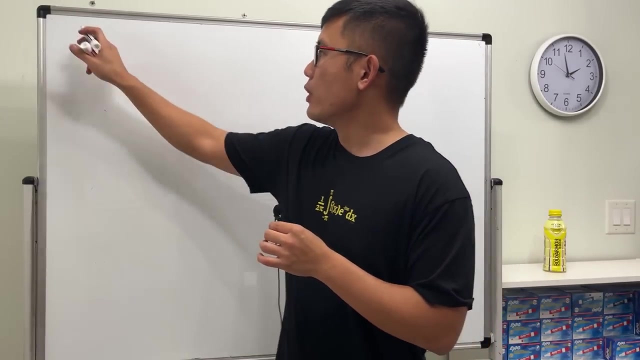 answer matches with one of the answer choices. all right, so 20 questions, not so bad. I will say good. number 21 to numbers 30. we are talking about expressions with square roots, so this is the time that we are going to use the so-called conjugate. 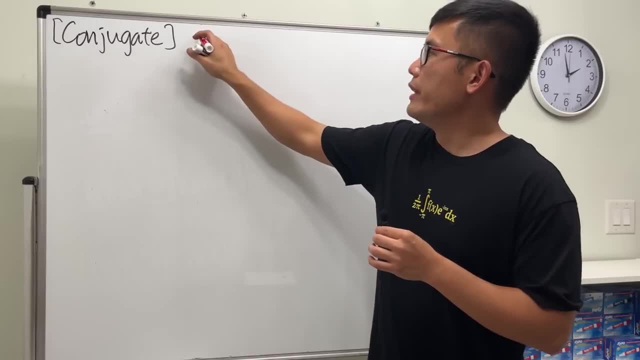 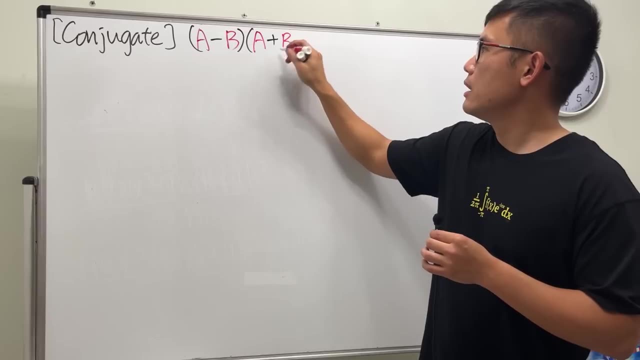 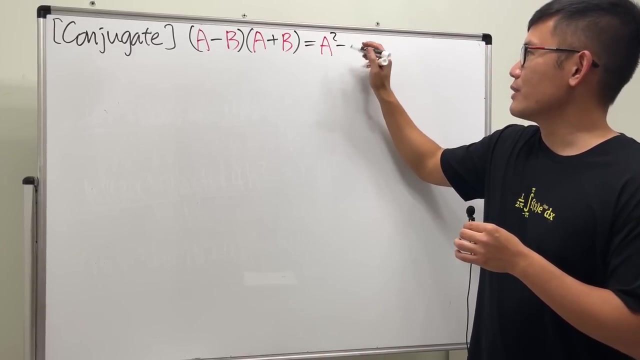 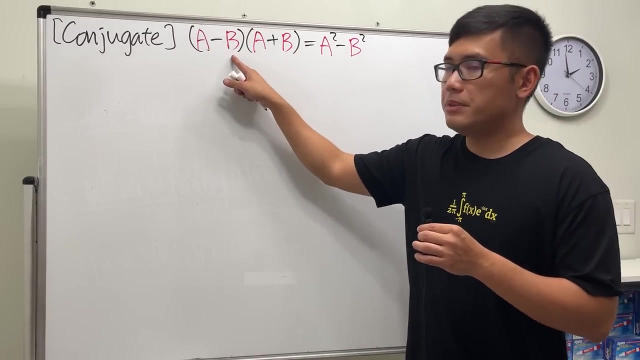 and the idea is that whenever we have a minus B times a plus B- this right here we actually have seen earlier- it's just pretty much the difference of two square formula, but you look at it backwards it's a multiplication version. if you go from here to here, the idea is that if you have a minus B this term and if you 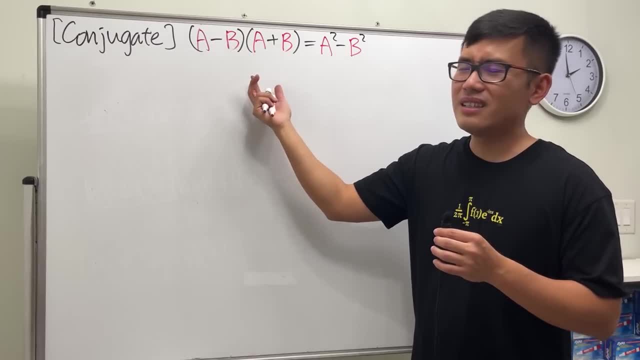 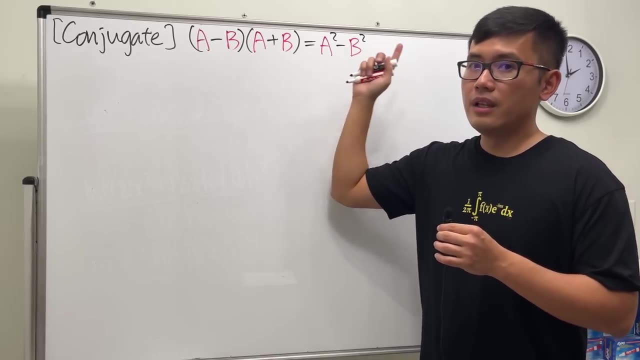 multiply this by this kind of opposite: huh, right, right, right. this is the so-called conjugate of that. you just change the negative to a positive and you keep the a and B. the good thing about this is that you get to just square the first term and then minus the square of the second term, and 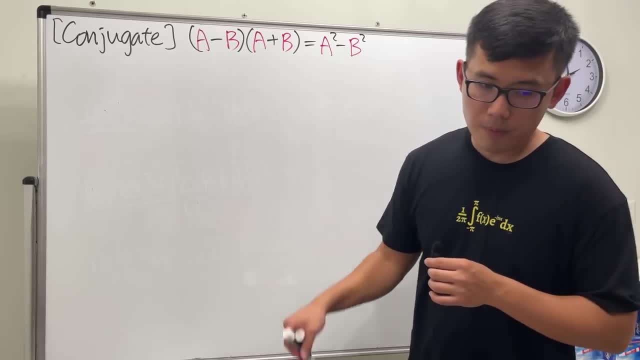 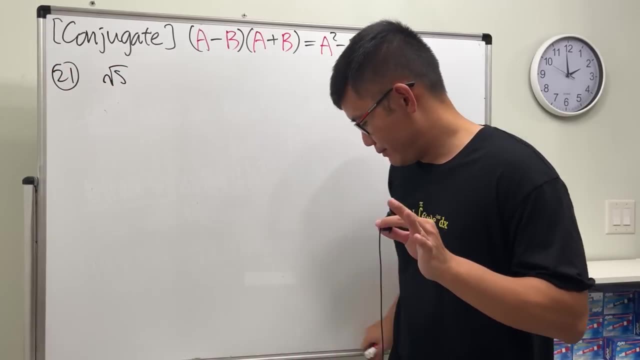 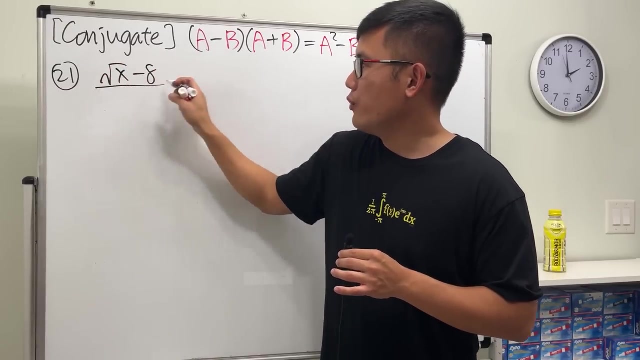 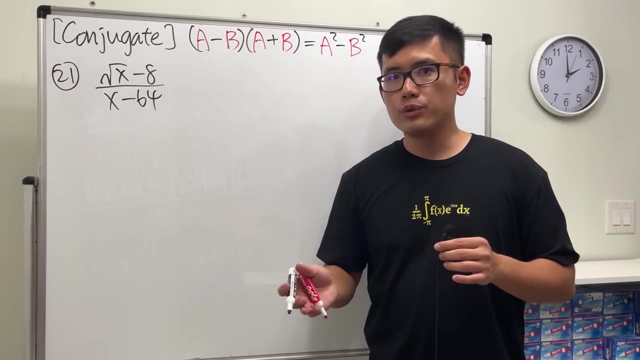 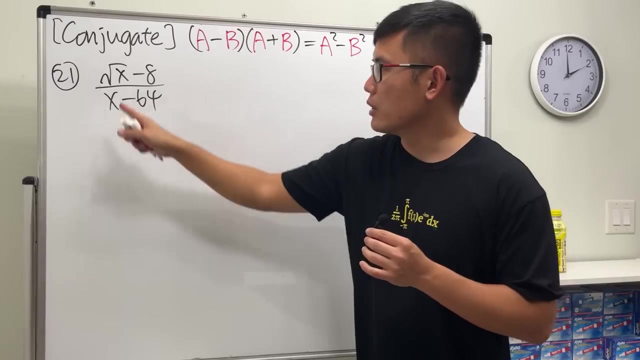 this is how you can solve the square roots. so let me show you number 21. we have square root of just kidding, square root of X minus 8 over right X minus 64. so whenever you have square roots, especially two terms: right, because this is one term and then we use the plus or minus to separate terms. so one: 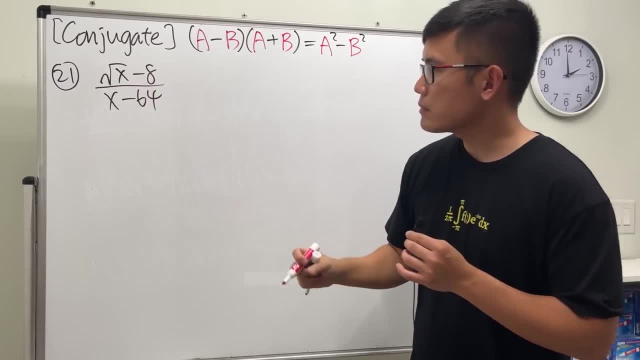 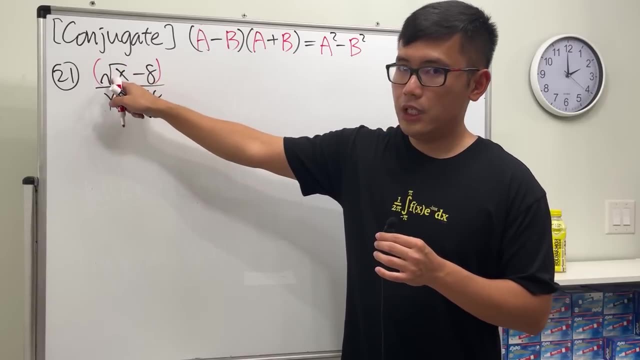 term, two terms. and then one term, two terms. so we have a square root. we will use the count you get. well, we will keep this. so we have square root of X. and then you change the minus to a plus, so we have square root minus plus 12 times. 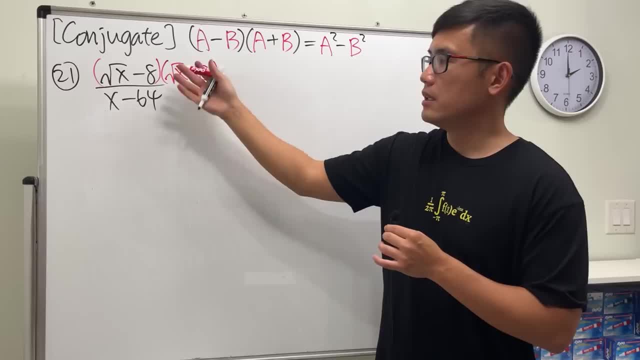 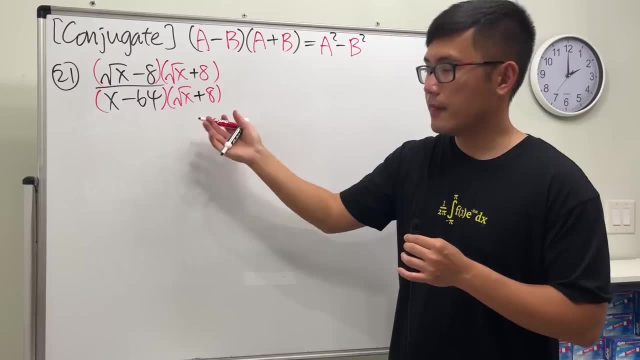 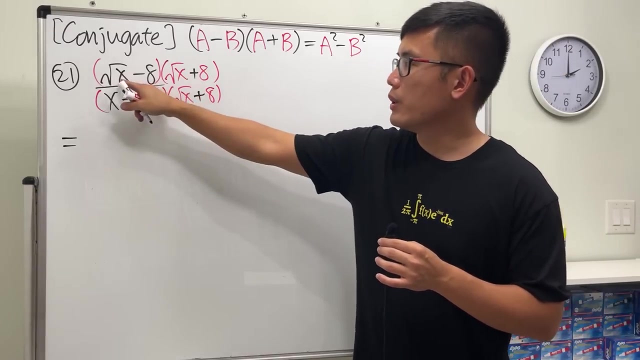 add, and then the 8 stays. so that's what we do. likewise, we do the same thing on the bottom. so square root of X plus 8, okay, and then for the top, to multiply this out, just use the formula. namely: we go ahead and look at this square, that. 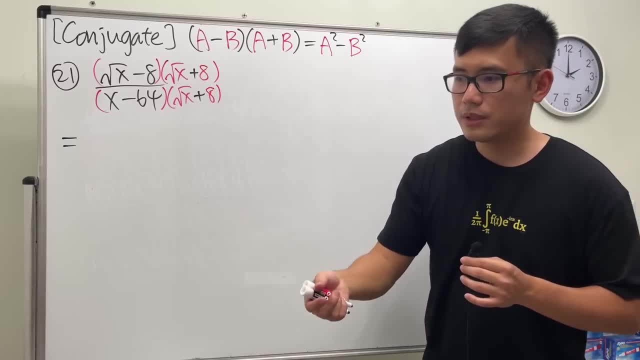 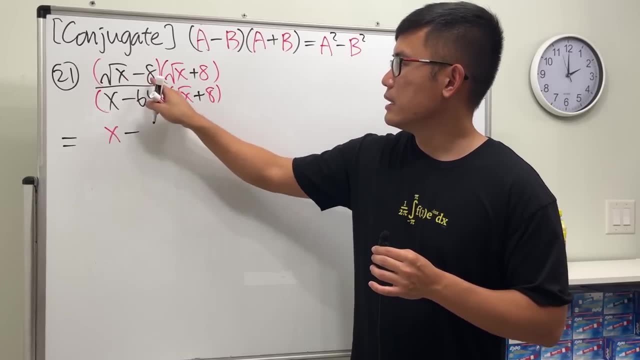 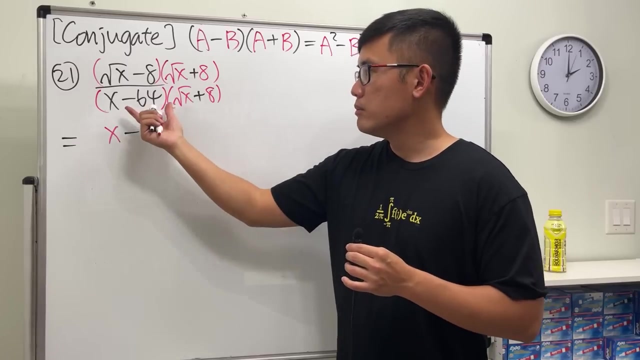 square root of x squared. square root of x squared is just X, so we have X right here, and then minus 8, and you square that, which is going to give us 64, just like that, and on the bottom, don't multiply it out. wait for good things to. 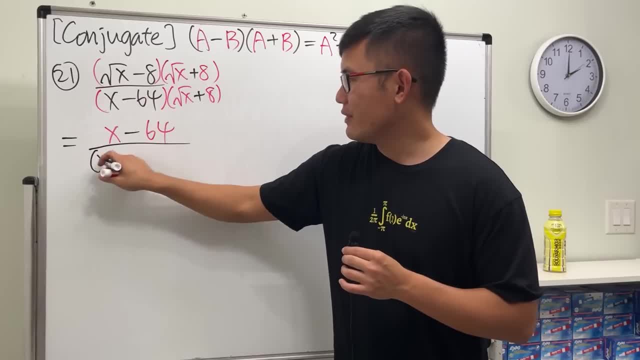 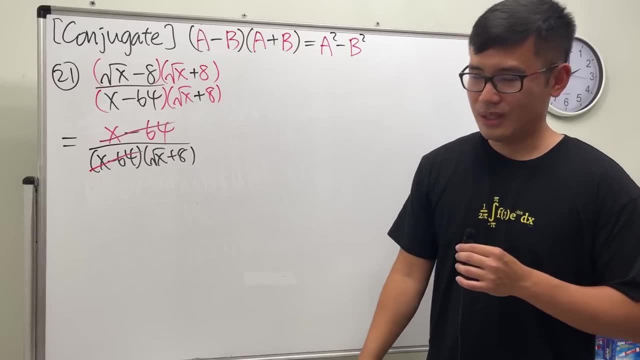 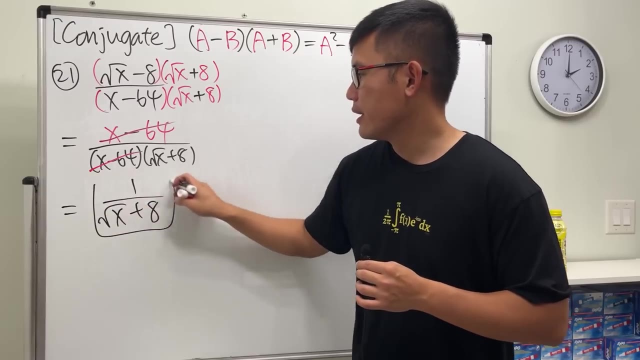 happen the cancellation. you see, here we have X minus 64 times square root of X plus 8. yes, this and that. cancel out. how cool is that right? and then we get 1 over square root of X plus 8, so the original can be kind of reduced to this. yeah, and in calculus, when you 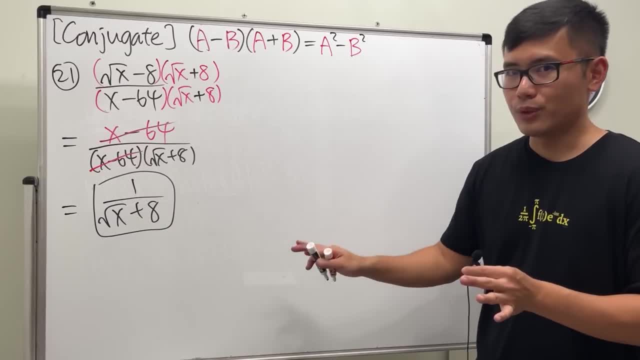 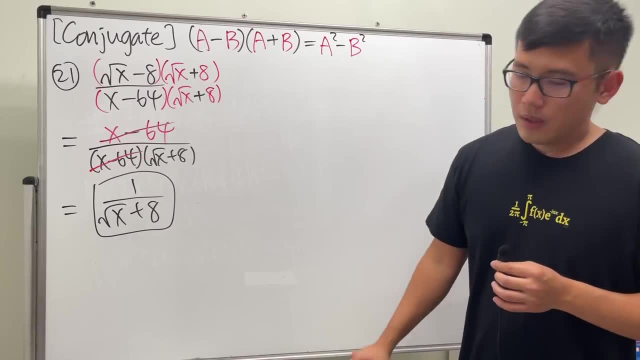 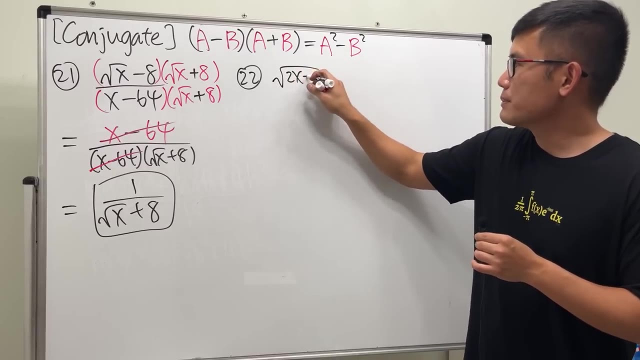 have square root in the denominator. it's totally okay, and we all adults. now, once we get to calculus, yeah, so that's that okay. number 22. so the expression gets a little bit longer, but same thing. square root of 2x plus 9 minus 5 over, we have 2x minus. 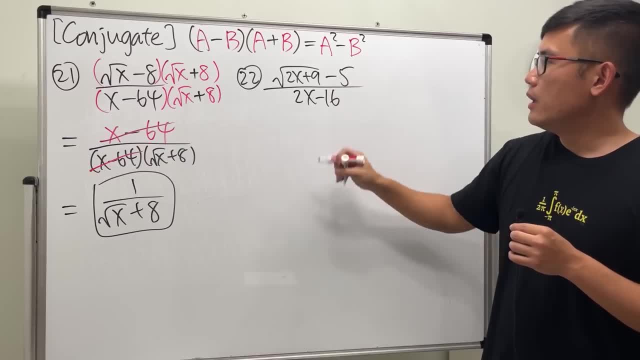 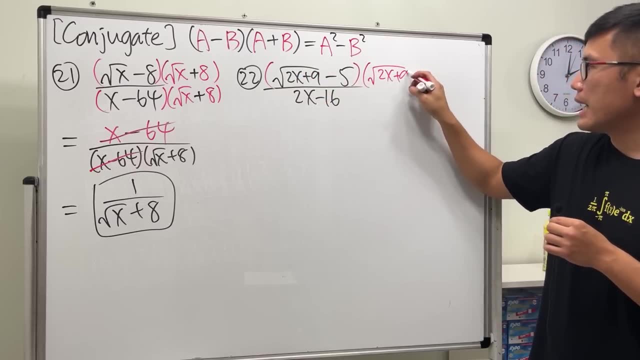 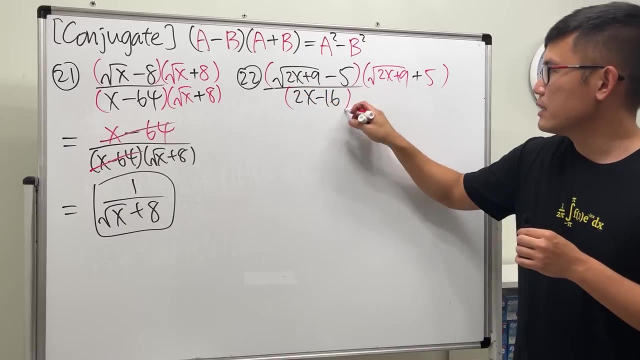 16. all right, so fix the square root by using the count you get. so let's multiply this by square root of 2x plus 9, change the minus to a plus and then keep the 5, like so, and then for the bottom, just leave it square root of 2x. 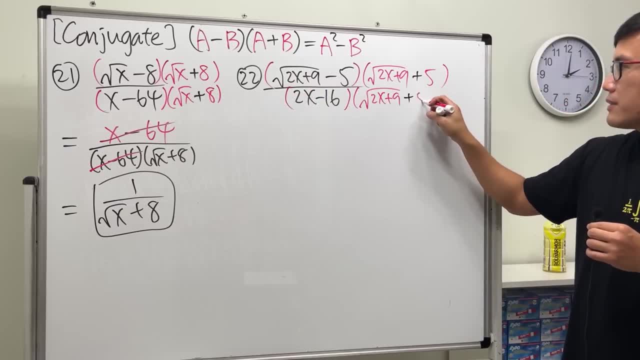 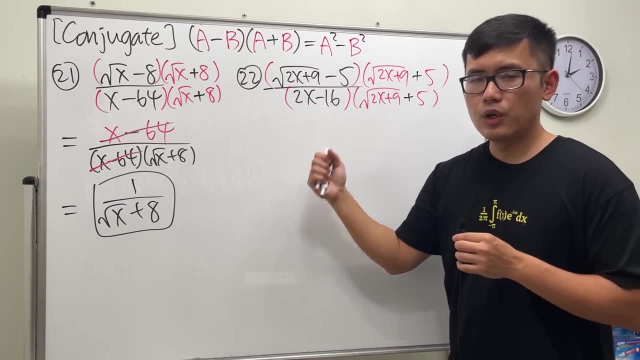 plus 9 and then do the same thing plus 5. yeah, now just multiply out and notice that this is 2x minus 16. we can find out that this is 2x minus 16 and then we can factor out 2, so don't multiply out now. if we can factor it, try to factor, okay. 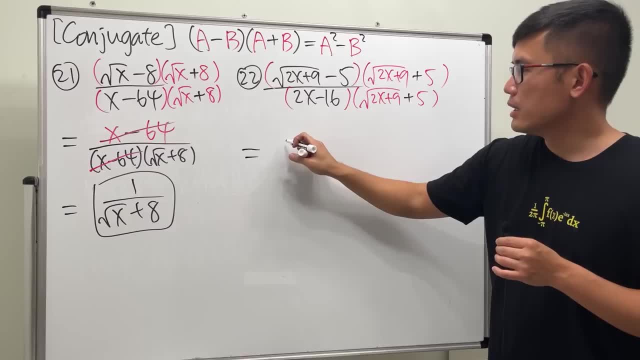 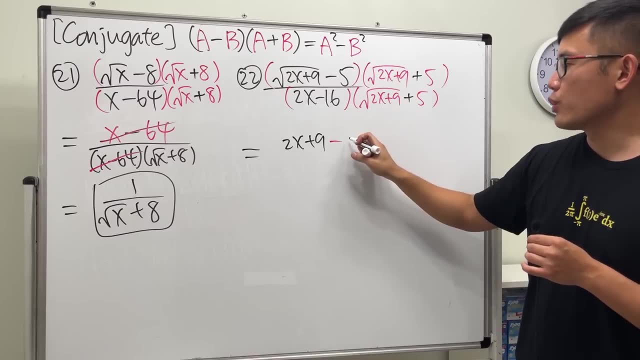 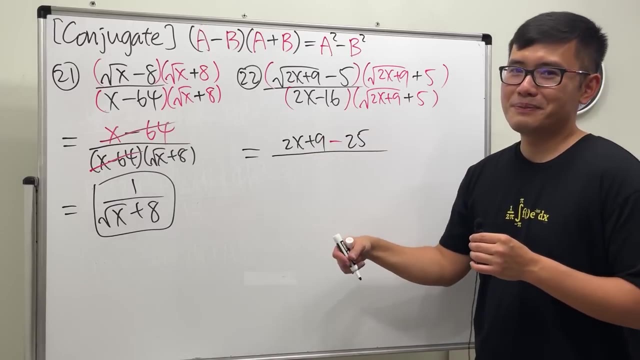 on the top square this, we just get 2x plus 9, and then we, minus the 5, we square that which is 25 over actually. no, you know, I take it back. yes, you can factor it, but you know, 9 minus 25 is minus 16. the. 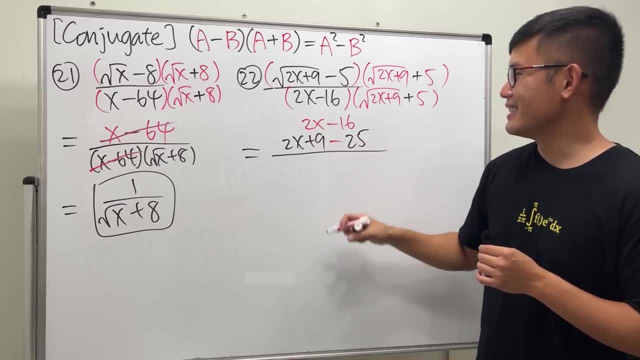 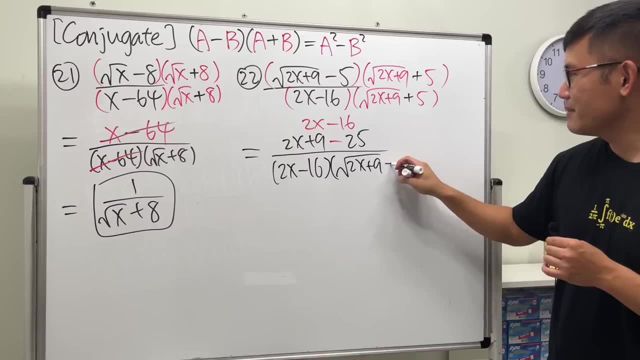 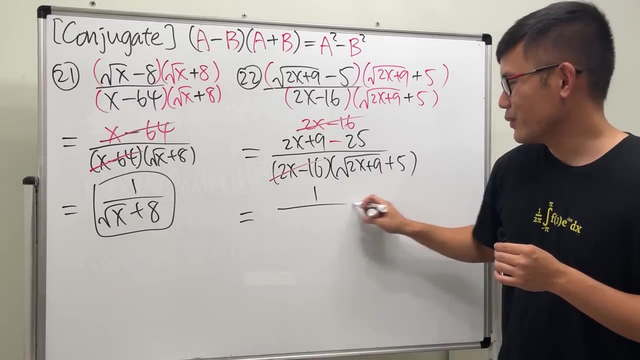 top is actually very nice: 2x minus 16, so let's just leave it like this: 2x minus 16, and then all this stuff, right? square root of 2x plus 9 plus 5, this and that cancel out. so the answer, the simplified version: 1 over square root of 2x plus 9. 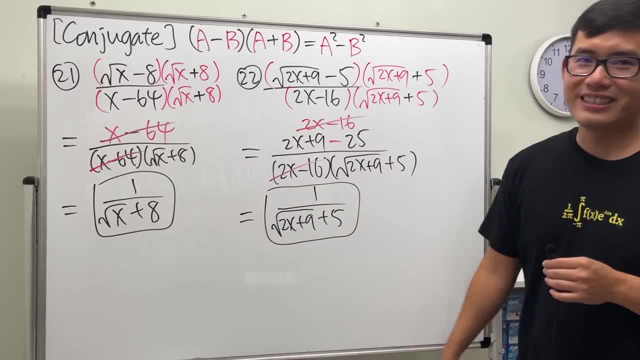 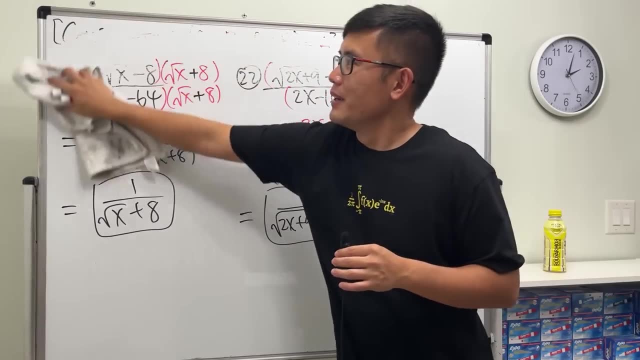 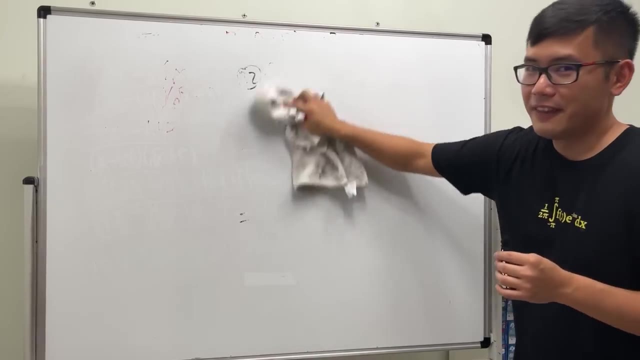 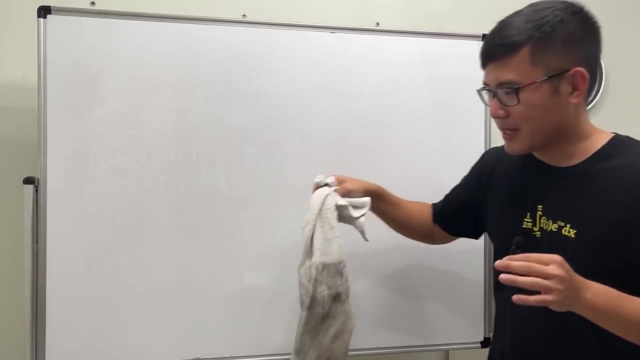 plus 5, just like that you guys can count how many times I erase the board I like from. let's just like have a blank board. yeah, this is like. perhaps this is definitely the most tiring thing when I do the marathon videos. okay, I'm not. 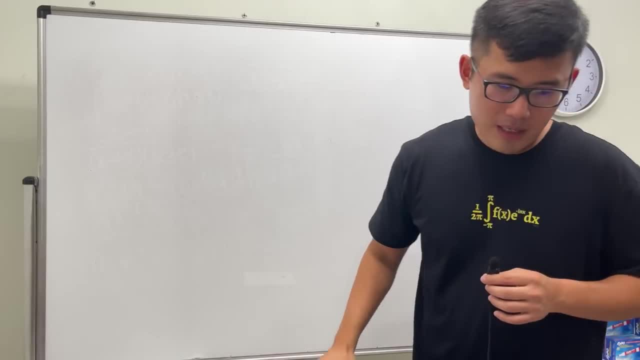 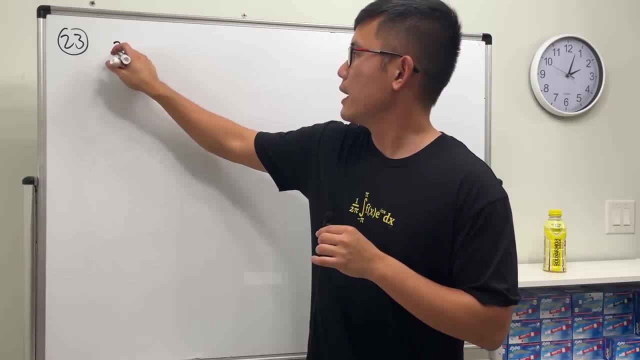 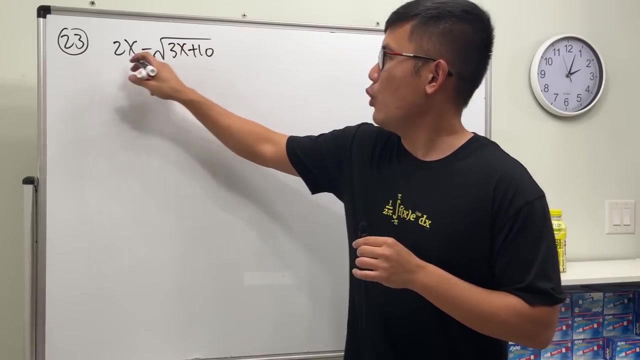 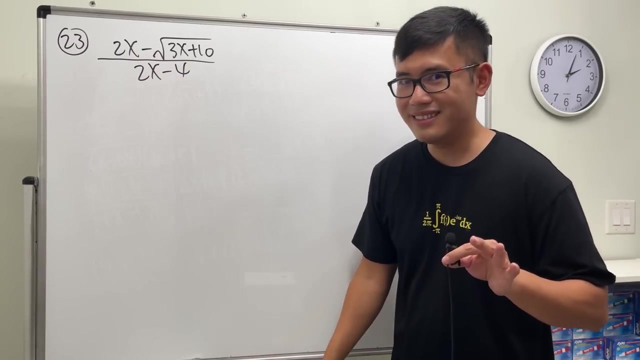 complaining. well, I am complaining, but I will try not to complain. okay, number 23: we are looking at 2x minus the square root, and then we have 3x plus 10 over 2x minus 4. whoo, 2x, 2x, but cannot do anything. okay, but we do. 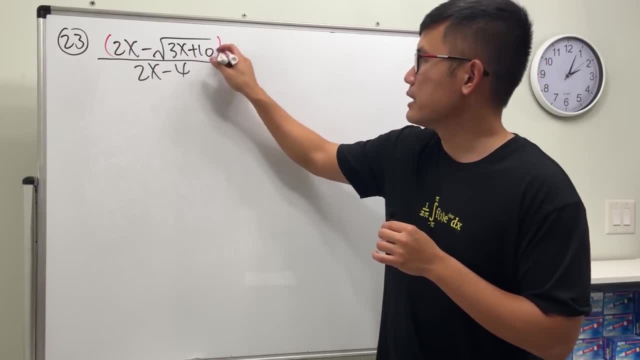 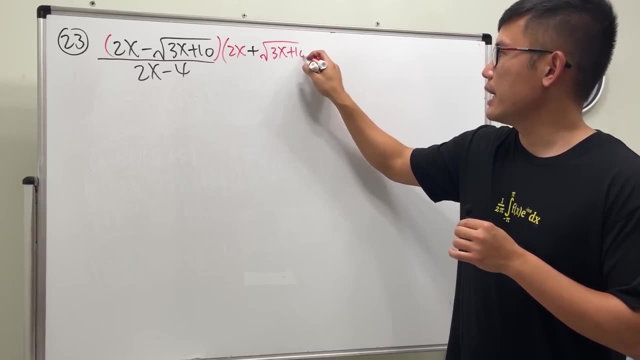 have the square root, so let's use the count you get. so here, let's multiply this by 2x plus the square root, so 3x plus 10, and then the bottom. let's go in and do the same thing: 2x plus square root of 3x plus 10. 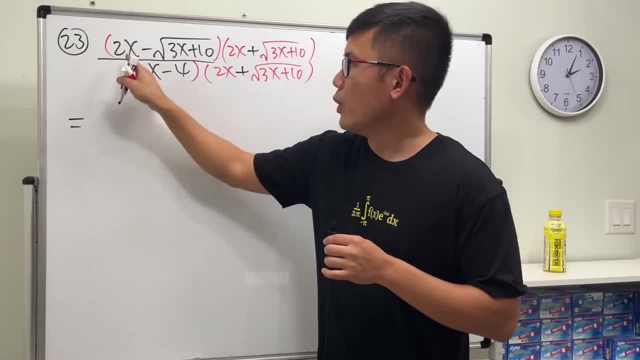 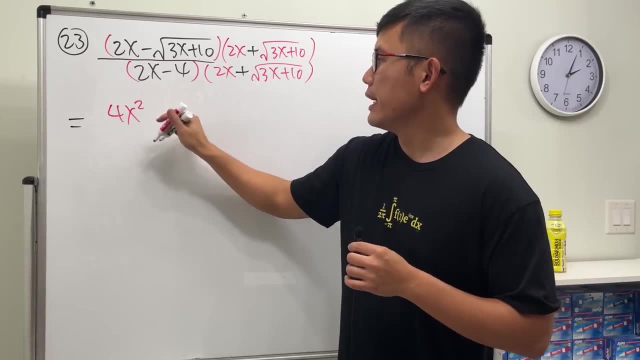 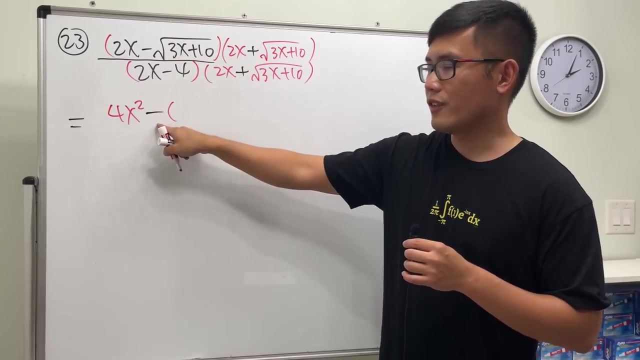 on the top. when we multiply this out, we just square the first term, so 2x square, that we get 4x square, and then minus square root square, they cancel, so we just have the inside. so put parentheses though, because we have a minus, we have to. 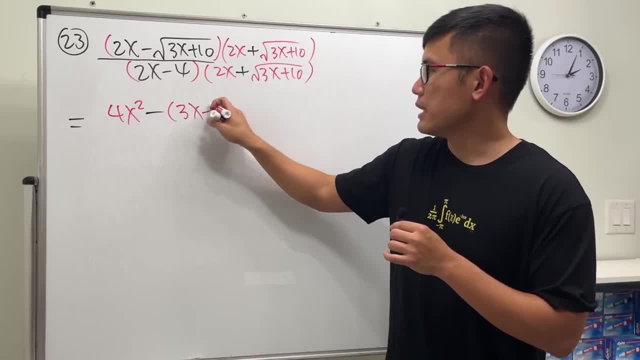 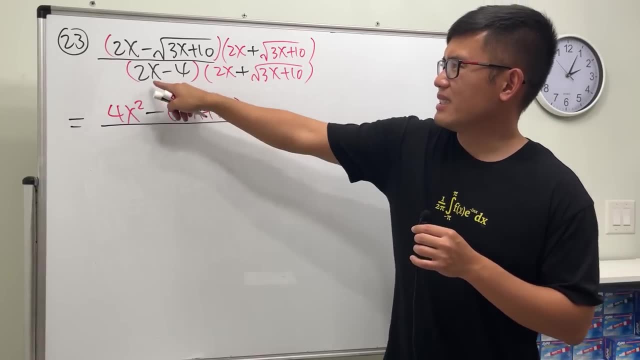 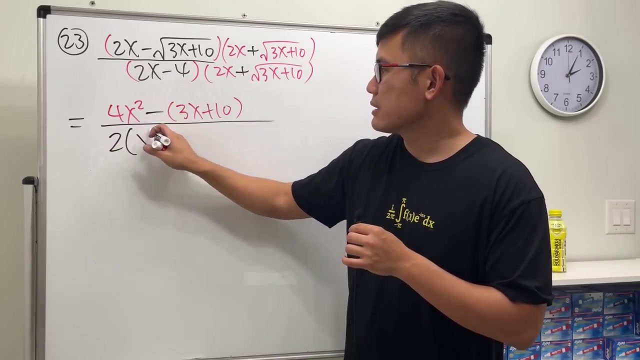 distribute that, so this is 3x plus 10. yeah, and then for the bottom here I'm going to leave this like, but we can actuallyrieben. so now we have 4x square root of 3x plus 10, it's participate 2, so it's 4x over 2. that to. 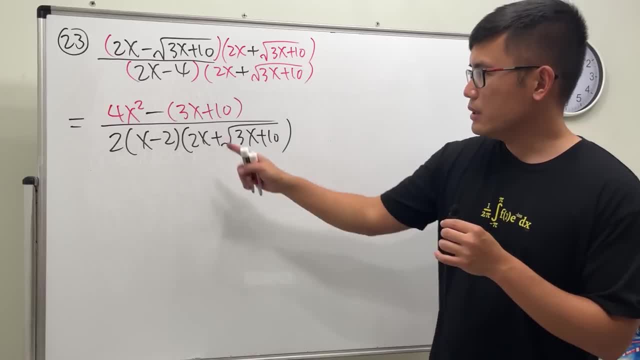 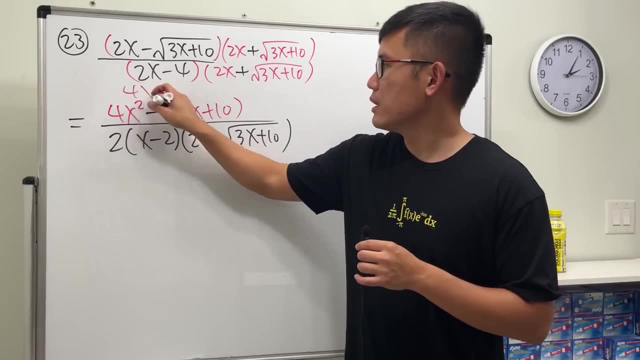 this. then we have- basically we got four titles in, but it's options- and and here we have 4 x plus 3, x plus a part of it. so that's extra all two, lots of factors, also 2, so right here I document 2, and then we have x minus 2 and in all 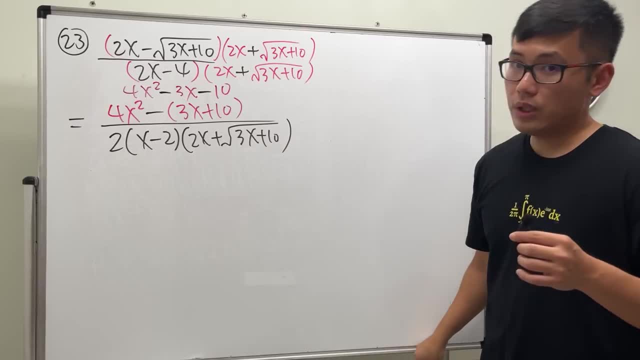 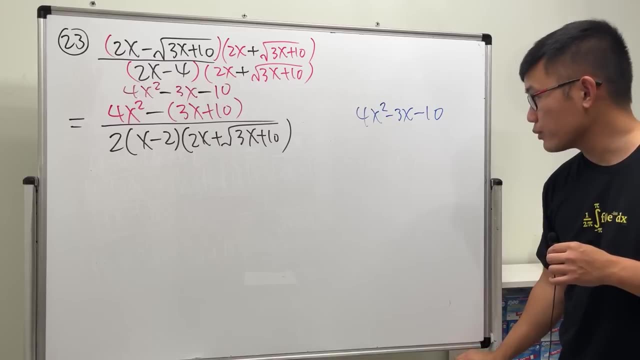 this stuffazon: 2 x plus square root of 3x plus 10, yeah, and then notice the top is right. so let's see 4x squared minus 3x minus 10. let's do the tic-tac-toe factoring right here. 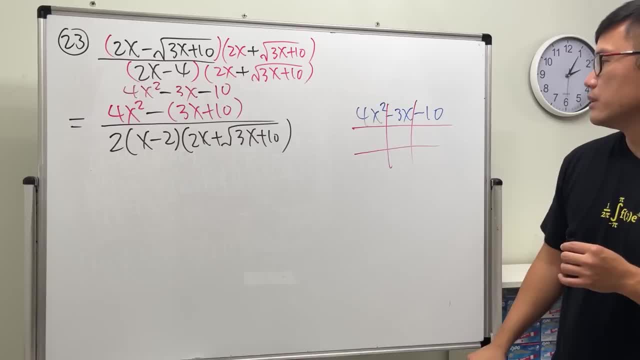 real quick, so let's try 2x and 2x. it's not going to work. 5 and 2: 2 times 2 is 4, 5 times that is 10. so it's not going to give us negative these three, so let's try this with 4. 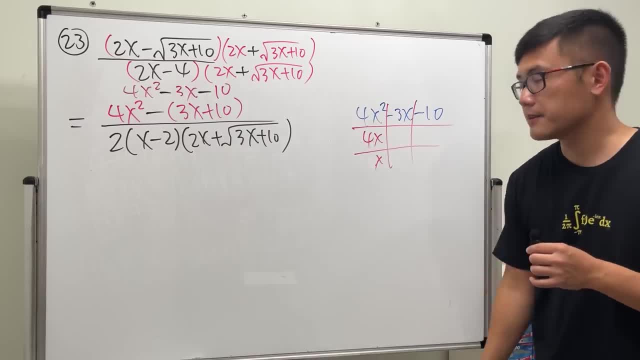 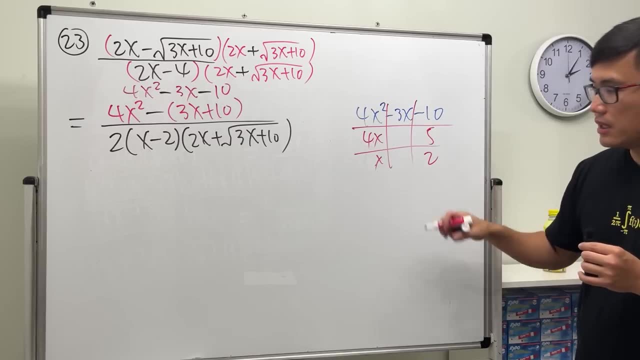 and x. yeah, 4x and x, and then 5 and 2. one of them should be negative. let's put on 2 here and 5 here, because make this negative this times. this is negative. 8x this times. this is 5x. aha, it works. 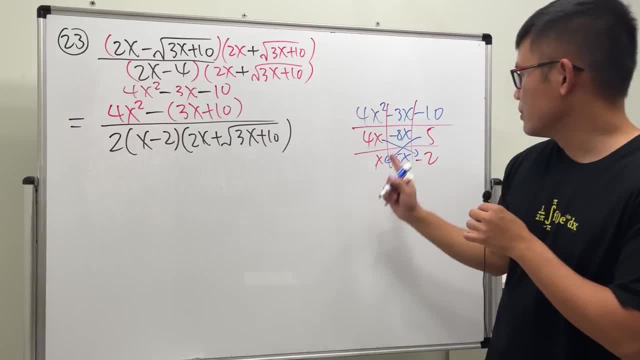 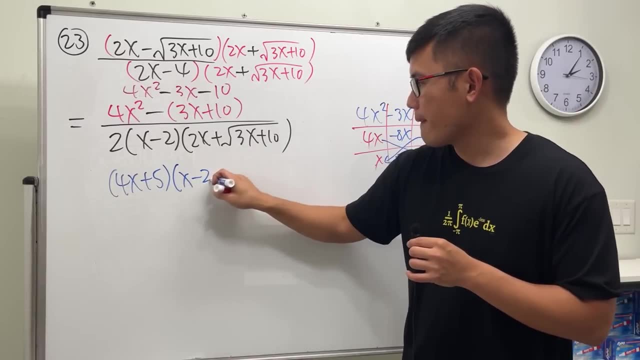 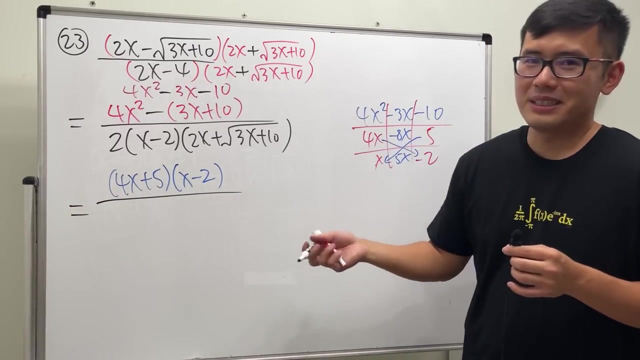 so the top right here factors to be 4x plus 5, and then x minus 2. aha, see 4x plus 5. yeah, of course, a lot of these questions are steady up so that they can have the next cancellations, but you have to keep in mind, though not all the time they have cancellations. 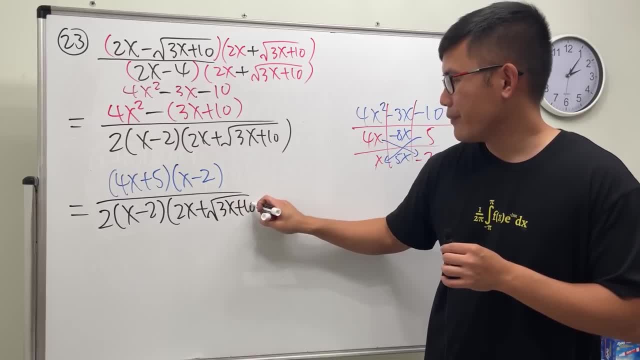 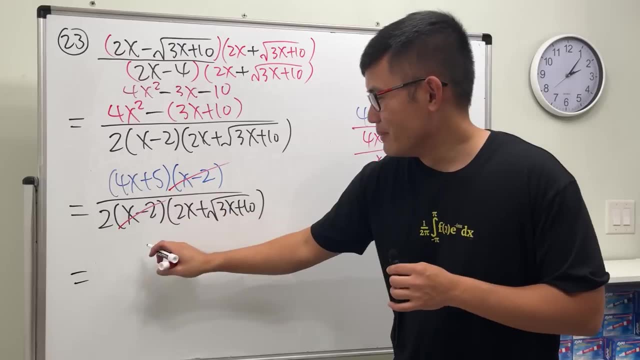 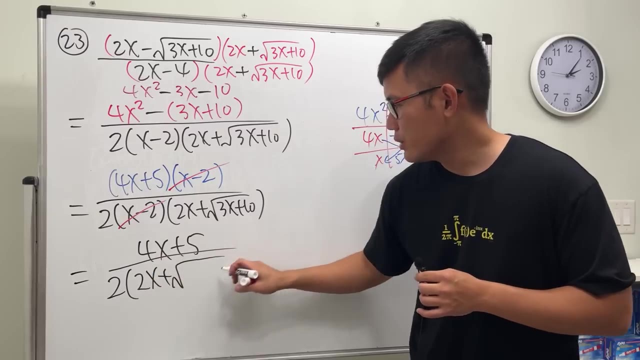 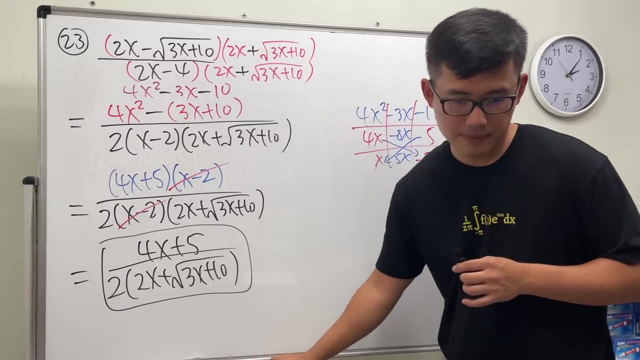 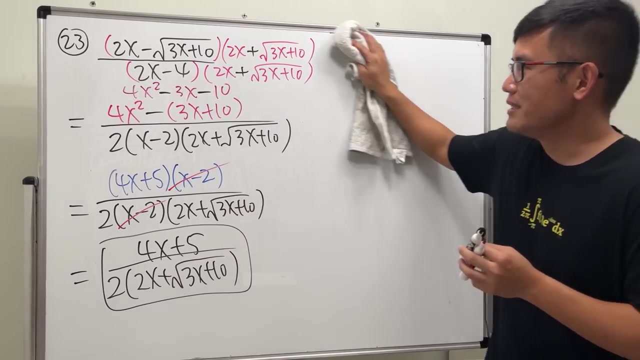 yeah, but of course, only the ones with, like beautiful cancellations are the fun ones. so anyway, though, 4x plus 5 over 2 at the front, and the parenthesis 2x plus square root of 3x plus right and 4x minus 4 must be 7 and 4, and so I think you, I think it's pretty predictable. 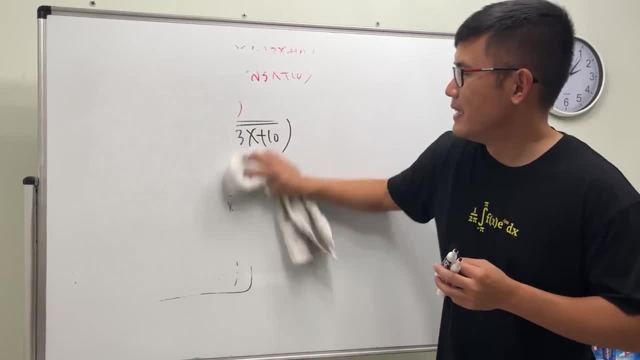 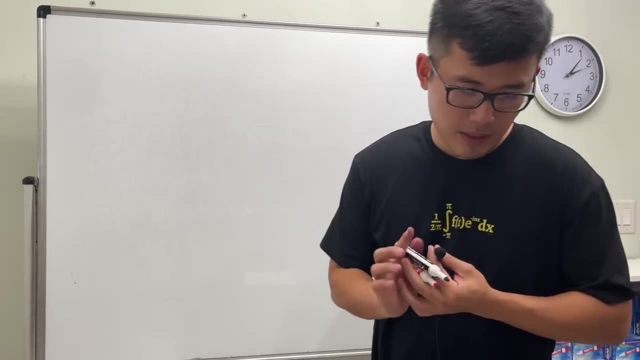 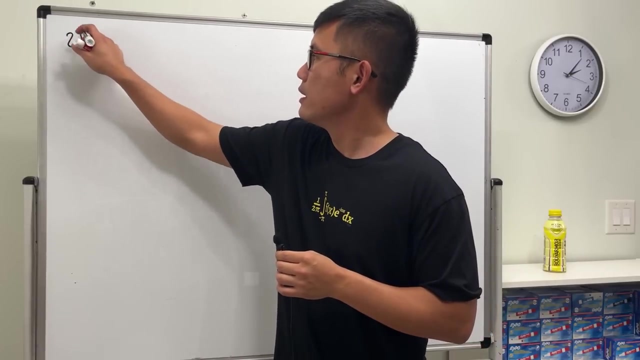 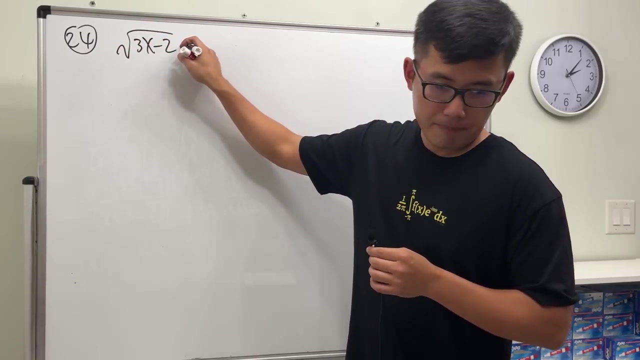 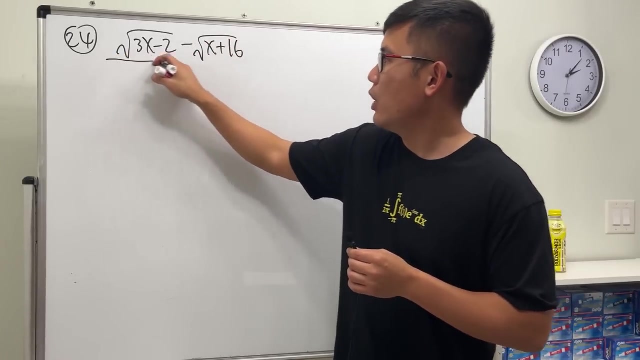 but I don't really know anymore. okay, we have 10, 10 or 10 done, just like that number, 24. so here we have square root of 3x minus 2 minus square root of x plus 16. over the bottom is 4x minus 36. 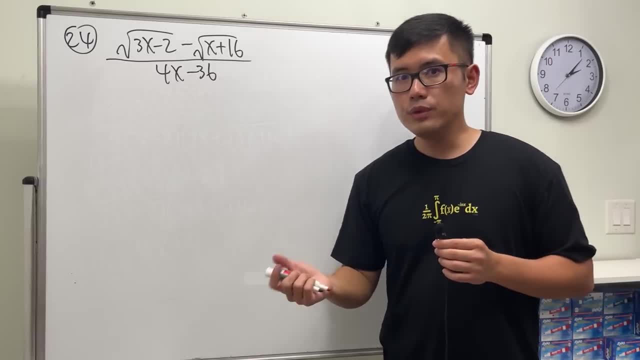 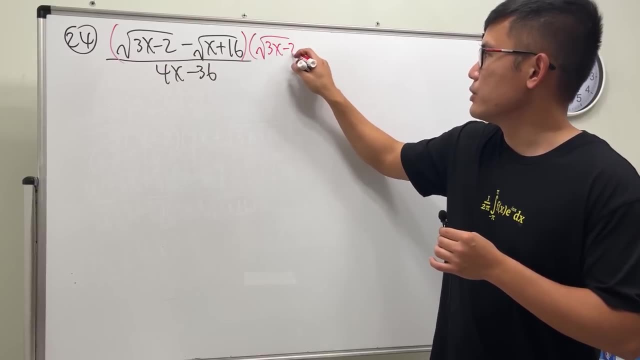 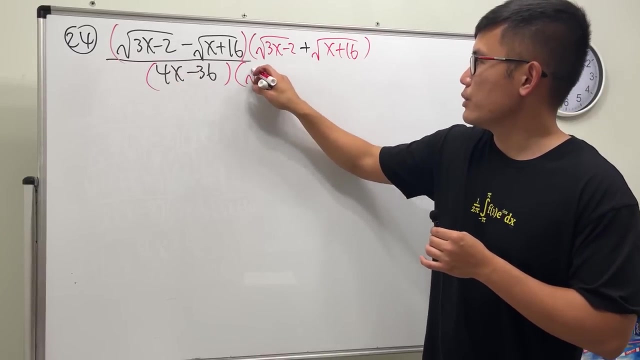 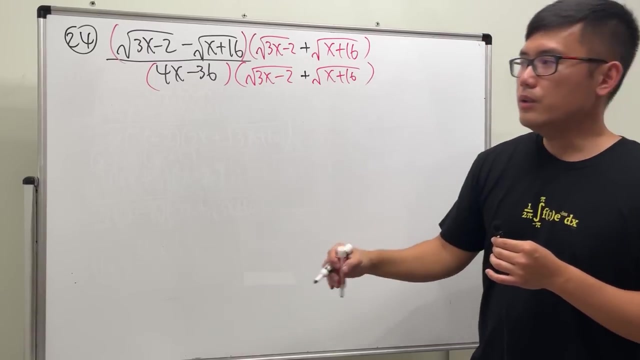 this time we have two square roots, but still same thing. let's do the conjugate. so right here, let's multiply this by square root of 3x minus 2 plus square root of x plus 16. so let's go ahead and do this: square root of 3x minus 2 plus square root of x plus 16. okay, 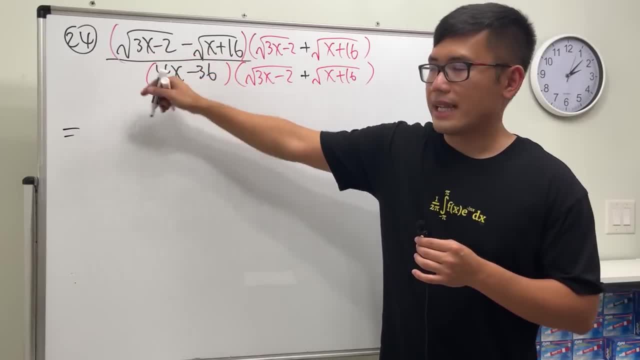 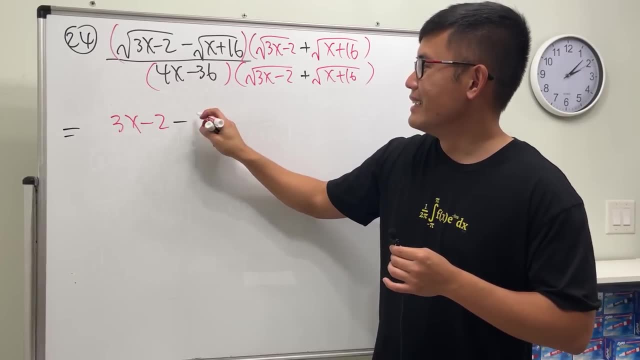 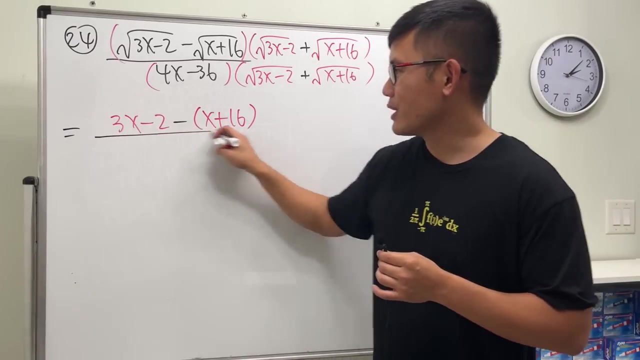 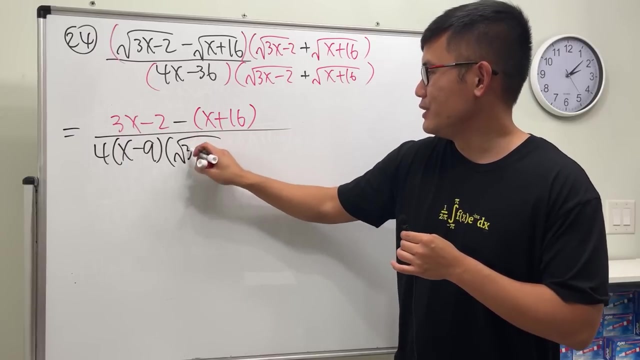 we are going to square that switch is 3x plus minus 2 and then minus, square that. so just parentheses, okay, x plus 16 and then the bottom. so keep it. so here let's factor out 4, 4, and then x minus 9, and then this right here is square root of 3x minus 2 plus square root of x. 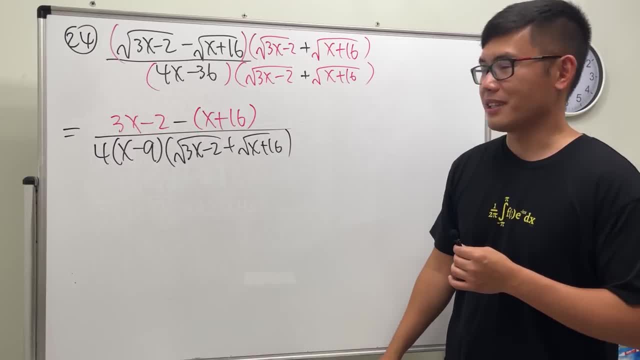 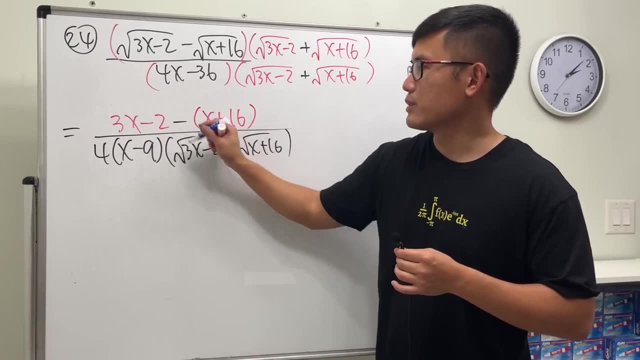 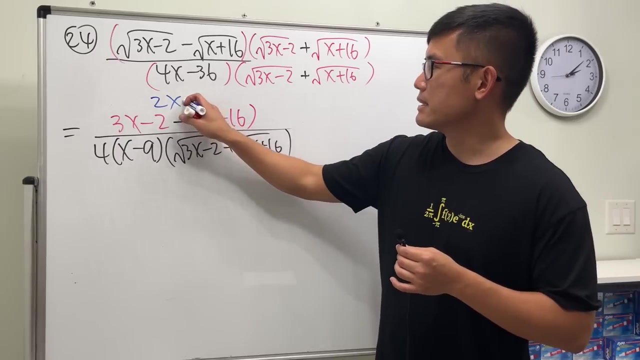 plus 16. on the top, it looks like we can do something. huh, yeah, definitely, let's go ahead and do that. so this is 3x minus x, which is 2x negative. 2 minus 16. 16 is minus 18. yeah, minus 2 minus 18, and then we see that 2x minus 18, we can factor out 2. 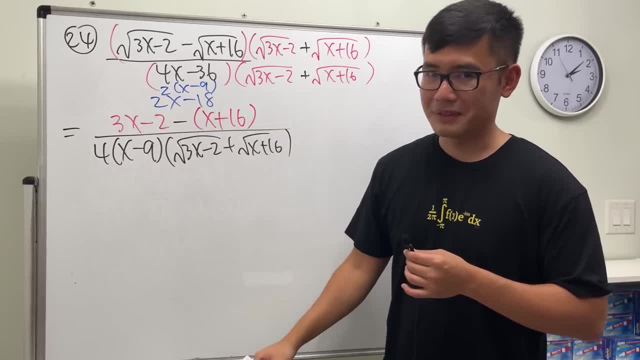 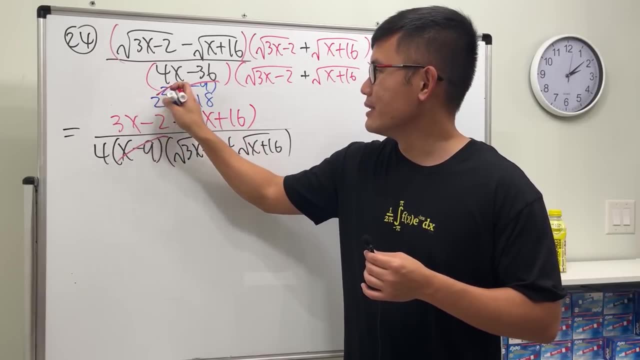 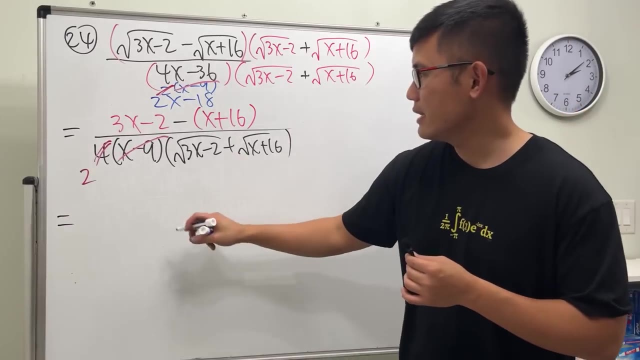 x minus 9. aha, this and that nice, this and that, cancel out very nicely. moreover, 2 and 4 can be reduced, so we have a 2 right now. yep, so, ladies and gentlemen, on the top we just have 1 over 2. 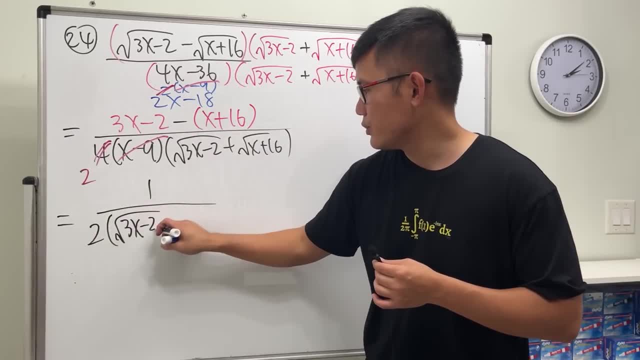 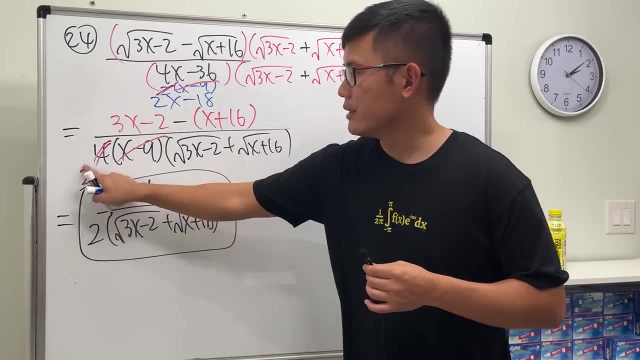 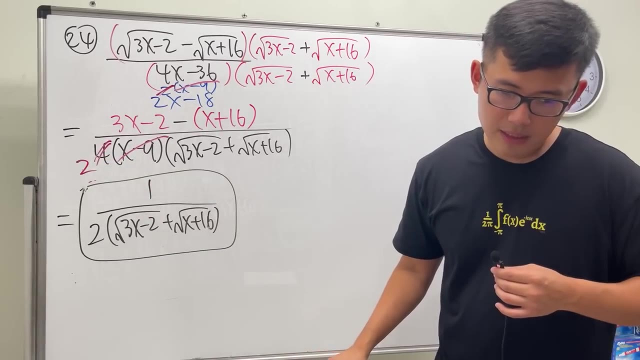 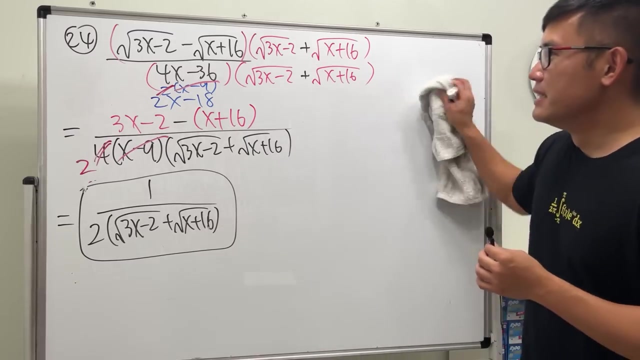 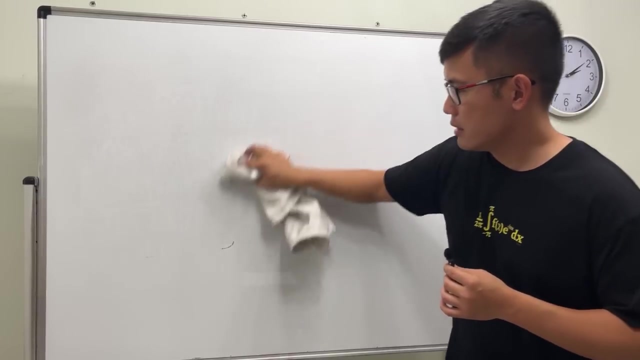 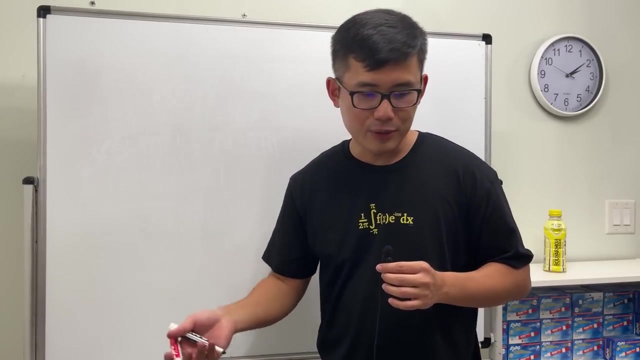 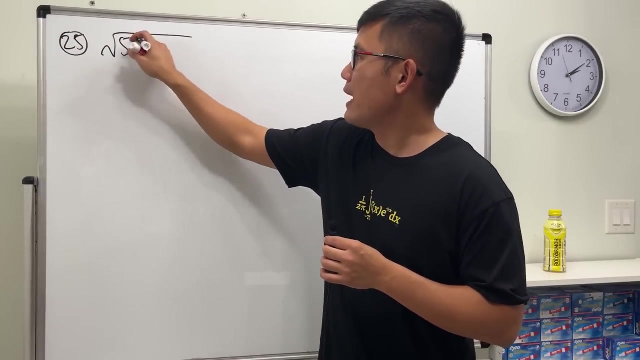 2 times square root of 3x minus 2 plus square root of x plus 16. done so? that was after the reduction. yeah, just like that. okay, i have to erase the board. okay, all right now. expressions with x and h: again number 25: here we have square root of five parentheses x plus h and then plus 2 minus square root of 5x plus 2 over our favorite lettering. 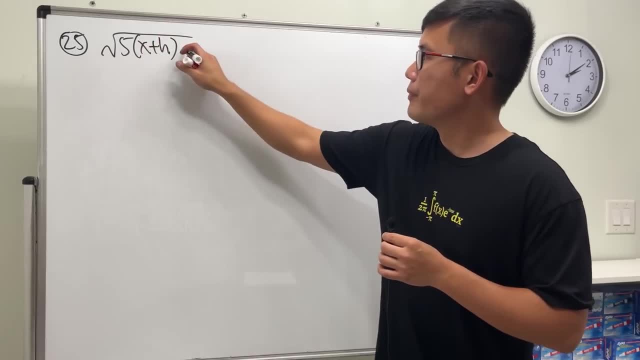 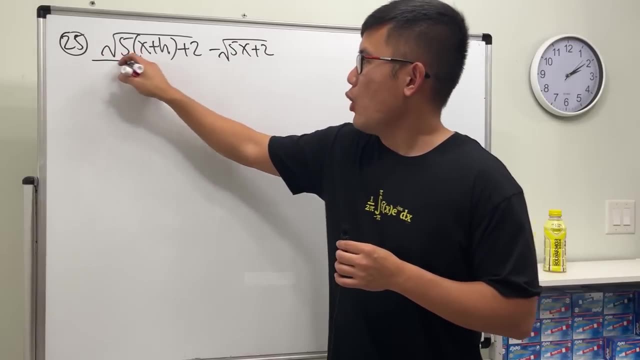 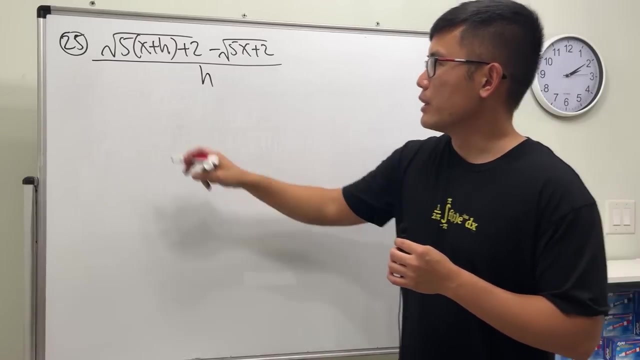 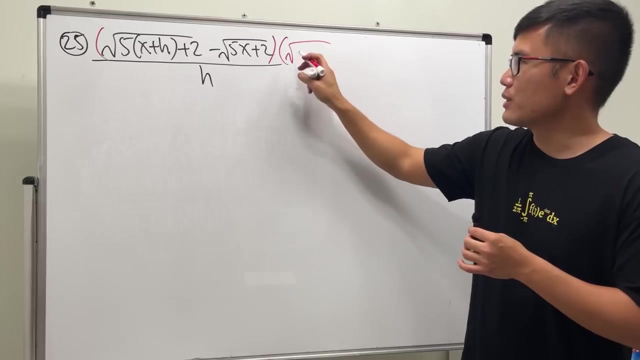 over our favorite lettering, over our favorite lettering. calculus, right, h, okay, so again same thing. let's multiply the top and bottom by the count you get, namely square root, and of course let's just multiply this out, right, so that's 5x plus 5h. 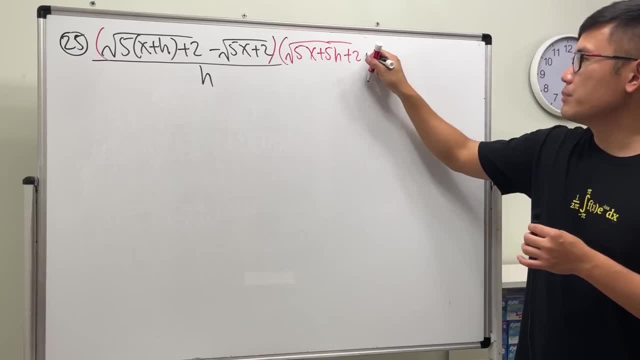 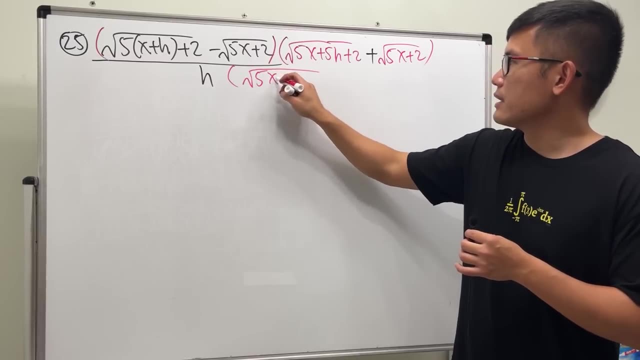 and then plus 2, and then this right here, just put it as plus and the square root of 5x plus 2, and then, of course, do the same thing on the bottom: 5x plus 5h plus 2, and then plus square root of 5x. 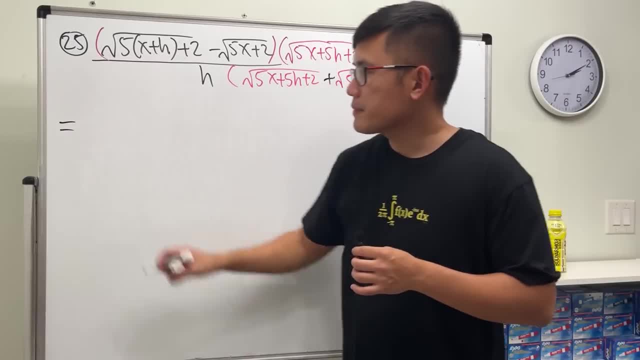 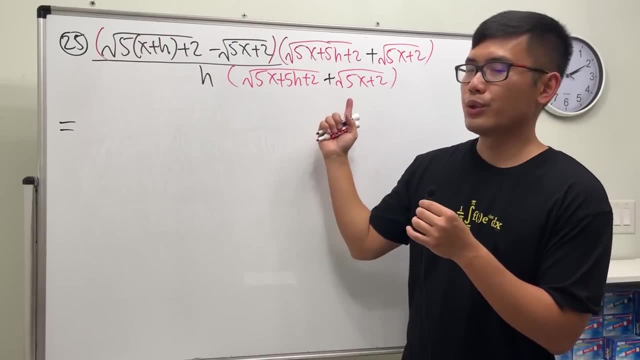 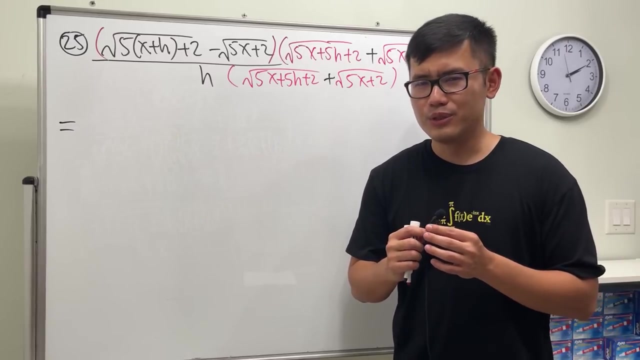 plus 2. okay, so multiply this and you might be wondering: do we really have to show the work right here? right? well, i will tell you. if this is like the first few times that you are doing this, then definitely you should just show work to keep keep track of everything. maybe we can try the next. 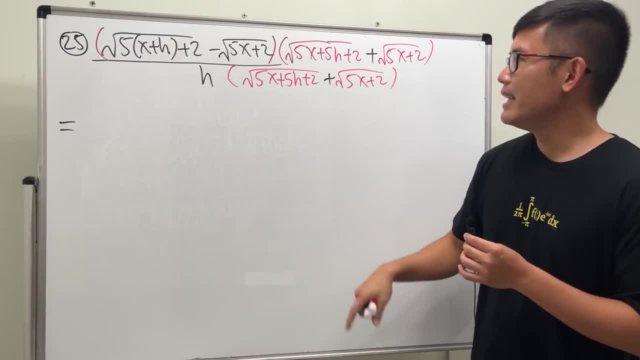 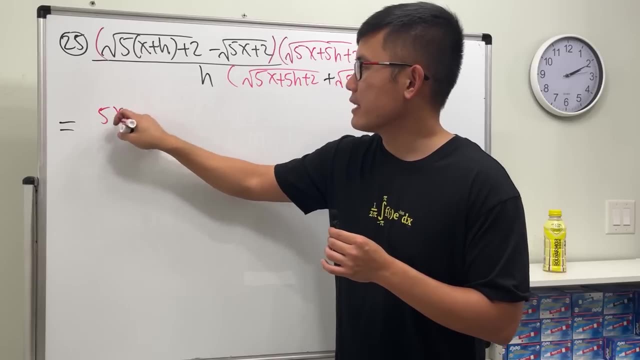 one that we don't show work. yeah, but let's see, we are going to just square this, which we'll just do it like this, and then we're going to do it like this, and then we're going to do it like this: have inside, and that will just be 5x plus 5h, and then plus 2 and then minus the second term, which. 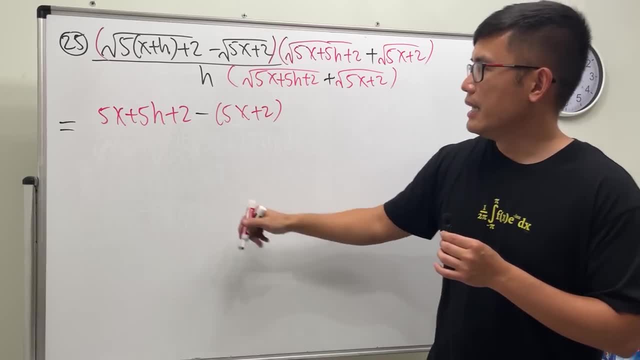 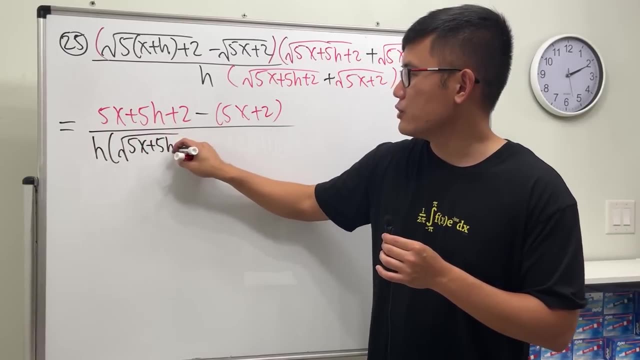 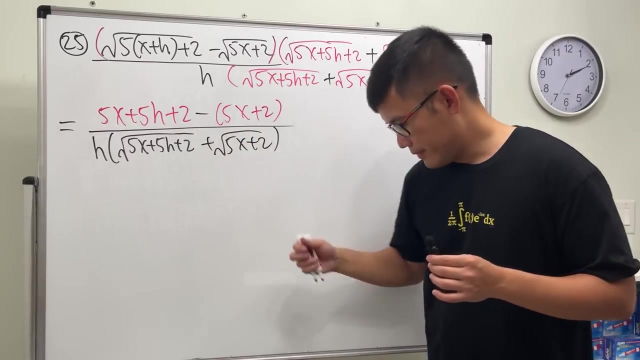 is 5x plus 2. yeah, all over all that stuff. so h times square root of 5x plus 5h plus 2 and then plus square root of 5x plus 2. now let's see we can distribute: this is negative 5x minus. 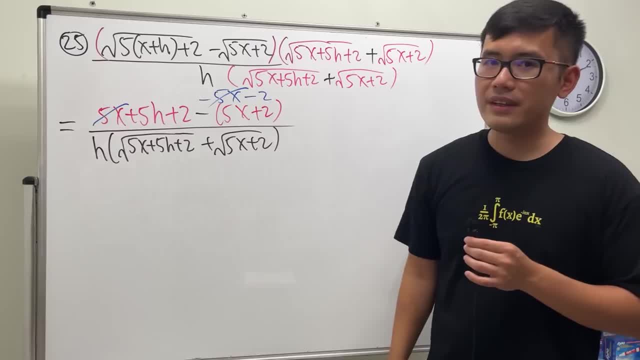 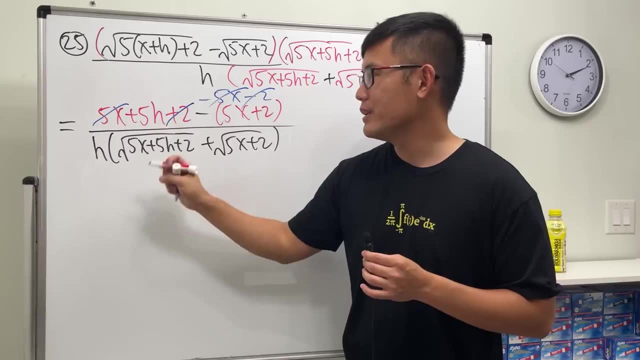 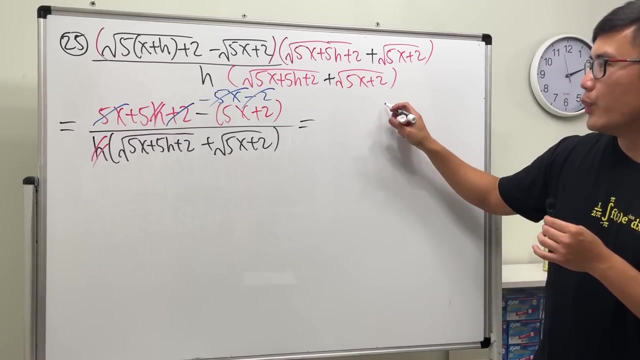 2, but the 5x minus 5x cancel, and this and that cancel on the top, we just have 5 times h. well, this h can be cancelled out with that h. so, ladies and gentlemen, the answer for this right here. i'll just write it down right here: we have just a 5 on the top over square root of 5x plus 5h plus 2 plus. 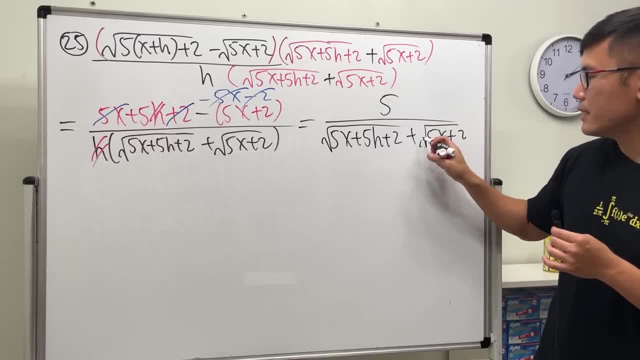 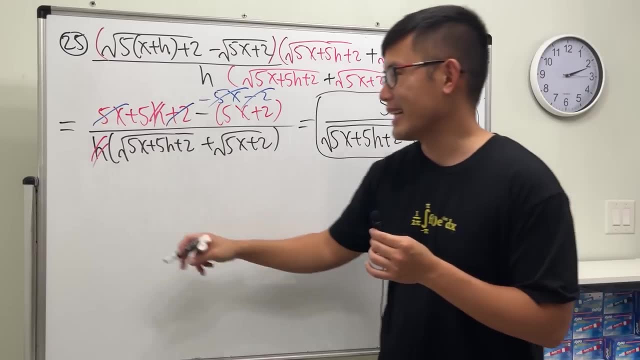 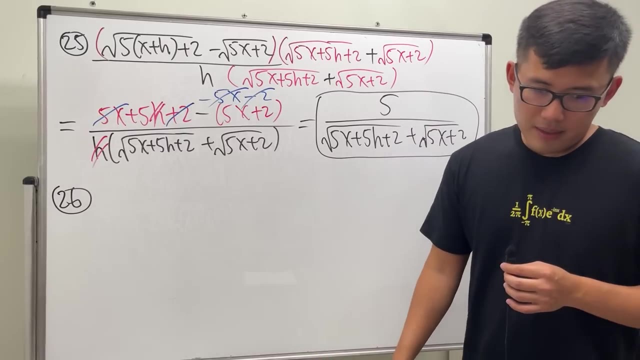 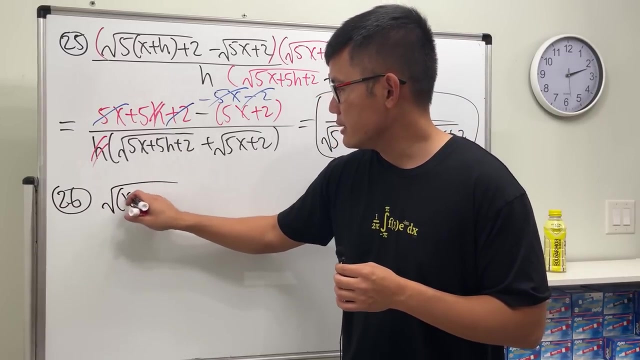 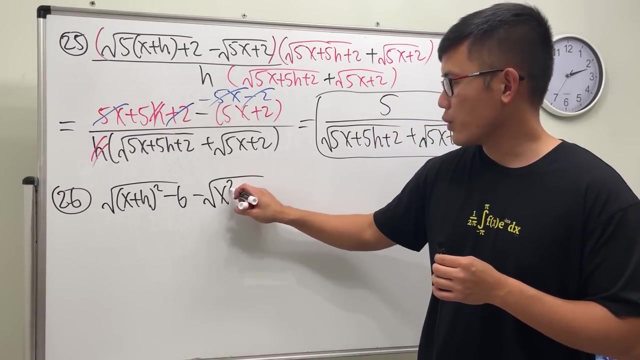 square root of 5x plus 2. yeah, who came up with all these kind of expressions? well, definition of derivative, and of course i did come words to them too. but anyway, though, number 26. so here we have square root of parentheses, x plus h square, and then minus six and then minus. square root of x square minus six. o of h. 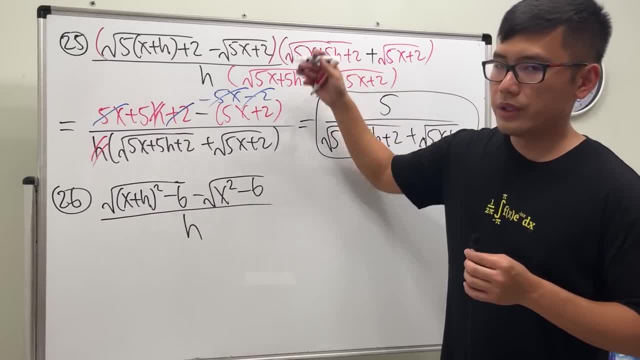 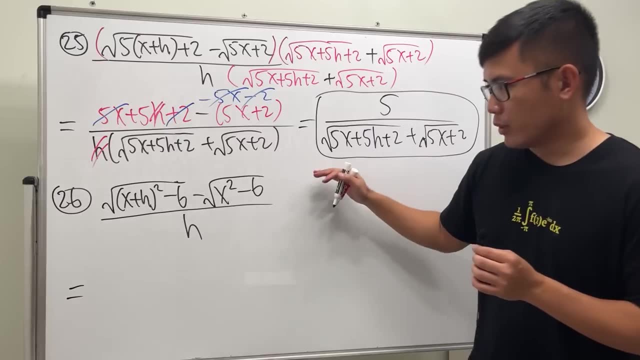 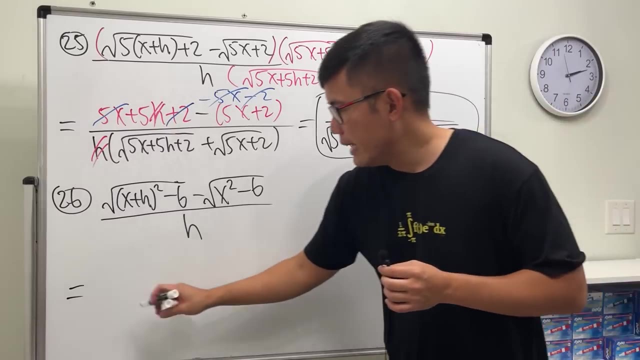 right. so we did the five count. you get earlier. already i showed you guys the work. so for this one, let's see. we know that we will have to multiply the top and bottom by this, but you just change the minus to a plus, right? so that's not sure working anymore and you know what's going to. 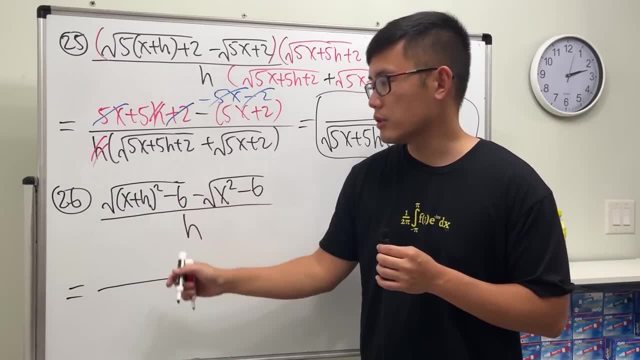 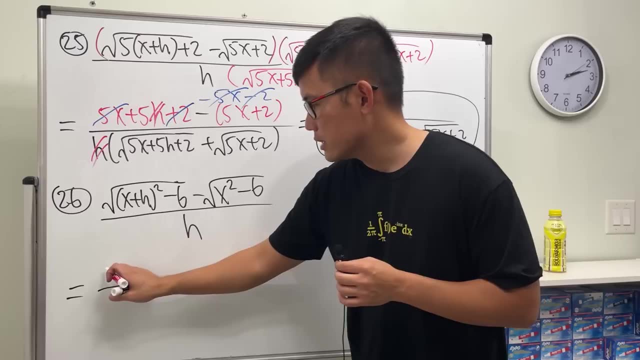 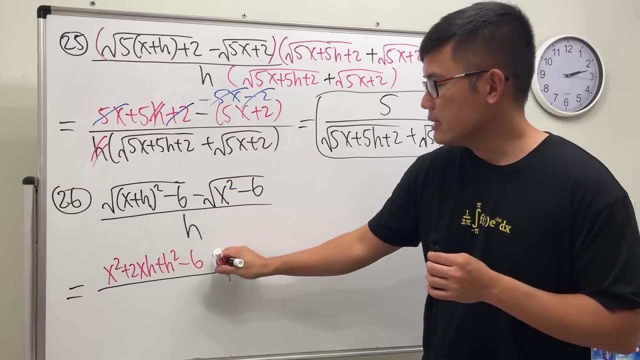 happen is that we square this, which is square, and that's what the square root cancel: square and the square root cancel. so we just have the inside and for this right here, let's just multiply the out, and that's x square plus 2x, h plus h square, and then minus 6.. and then we minus the square of this. 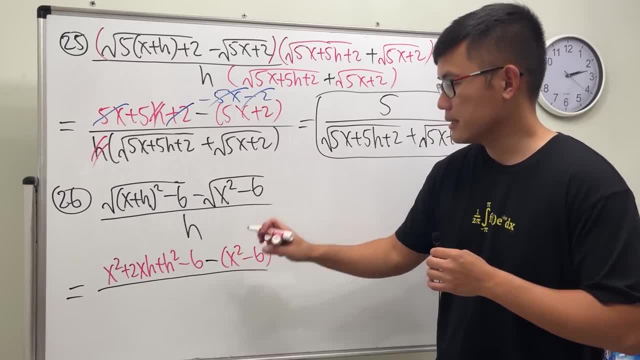 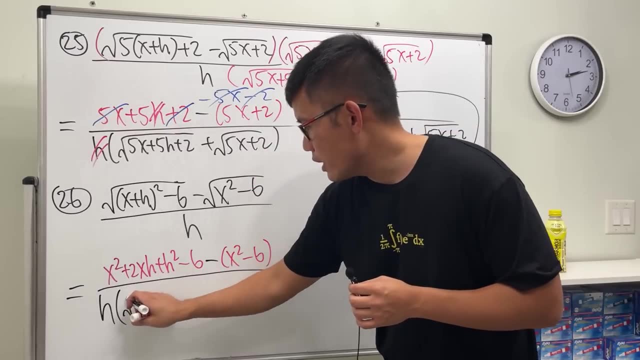 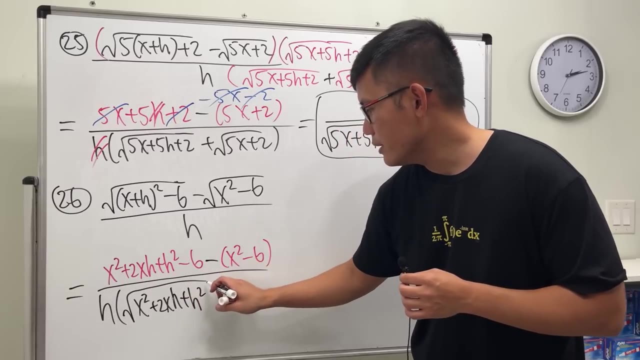 term, which is just going to be x square minus 6.. and then, for the bottom though, well, we will have h, and now let's write down the count you get, and that's square root of x square plus 2x, h plus h square, and then minus 6.. 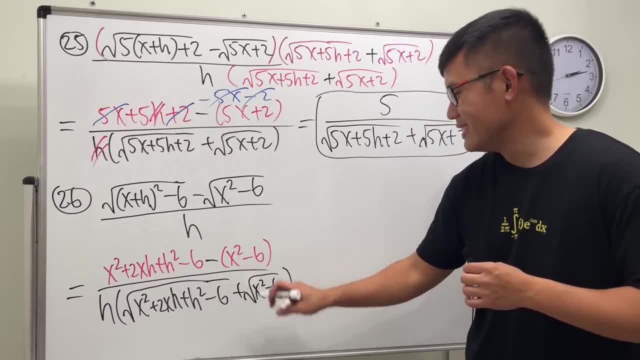 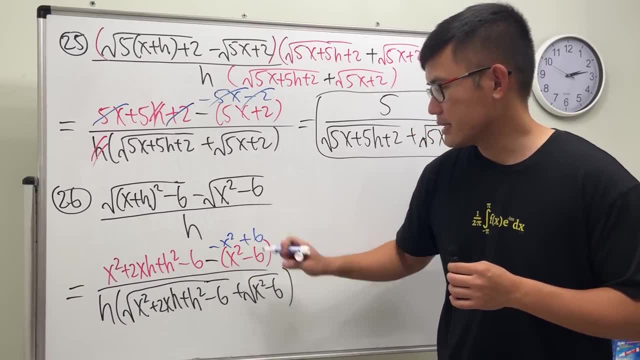 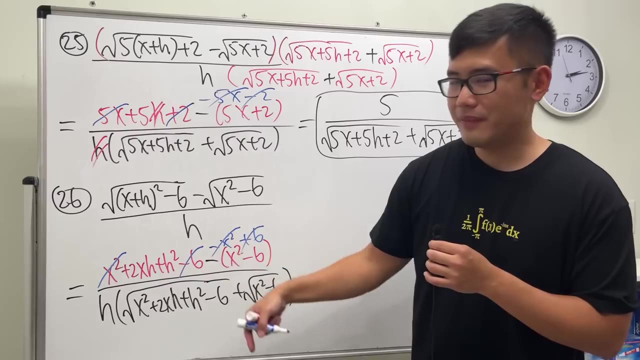 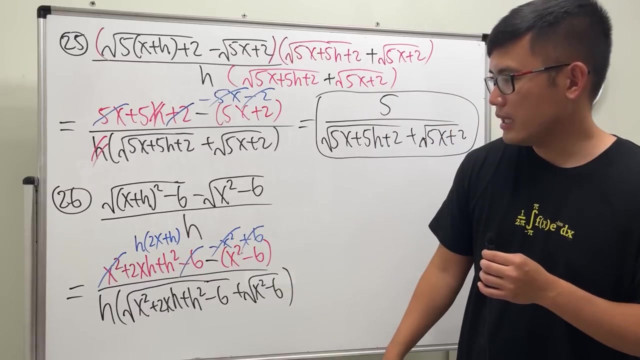 then plus square root of x, square minus 6.. okay, i don't know why i'm laughing, but like, yeah, anyway, this is negative x squared. and then plus six, cancel, cancel, cancel, cancel this. and that they both have h. let's factor it out. and then we get 2x plus h, yeah, and then this h and that h cancel. 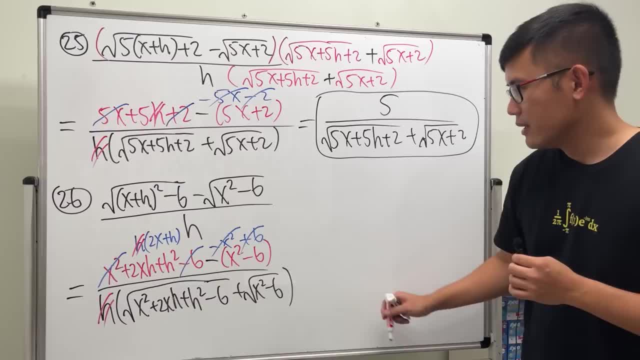 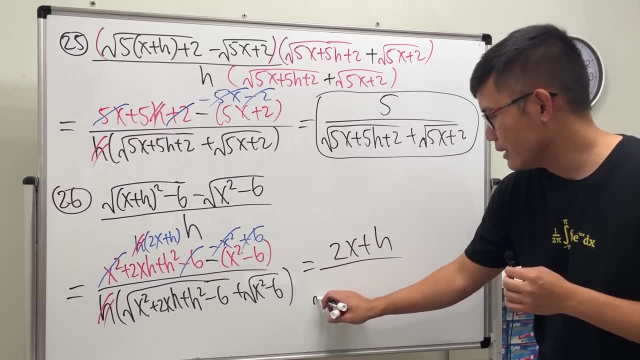 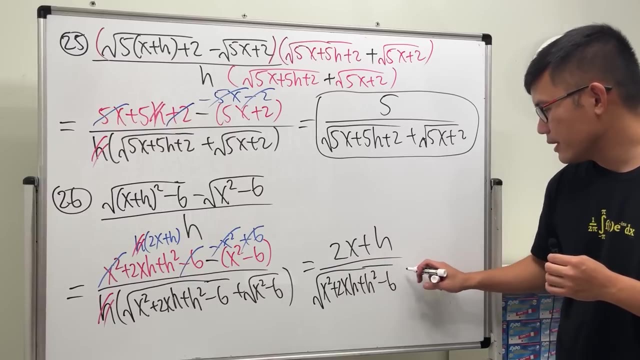 so finally, ladies and gentlemen, we get 2x plus h on the top over that big long conjugate. so x squared plus 2x h plus h squared minus 6, and then plus square root of x squared minus 6.. so let me just make it prettier for you. 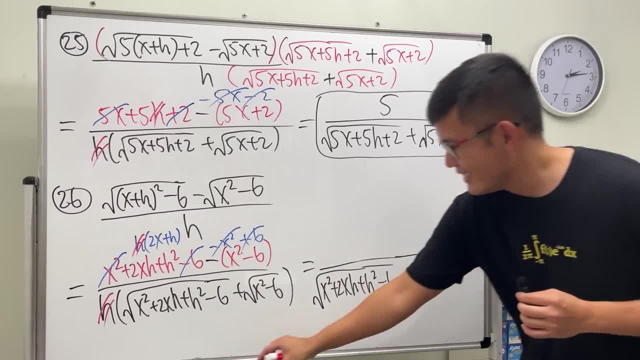 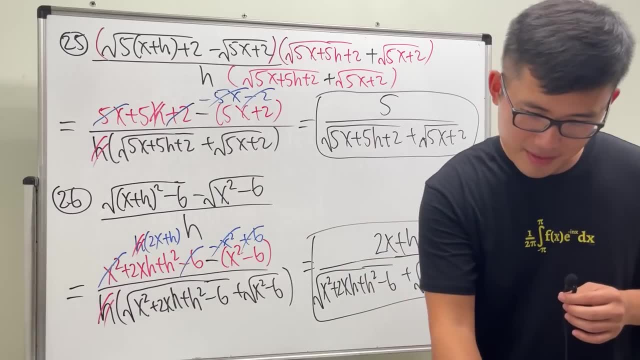 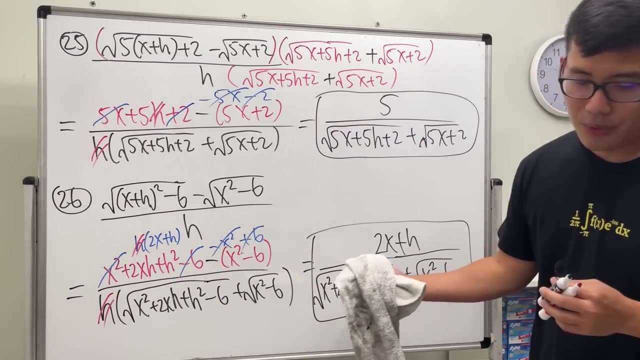 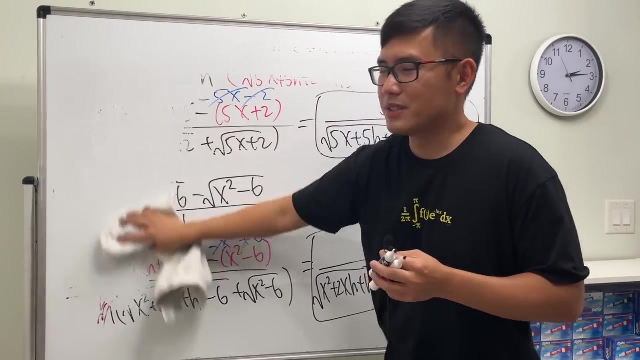 guys and then, uh, 2x plus h right here. yeah, okay. so for the remaining question, i'm just going to not do the count you get, just so that way we can save some time of writing. a lot of this is just really just because we have to write a lot. 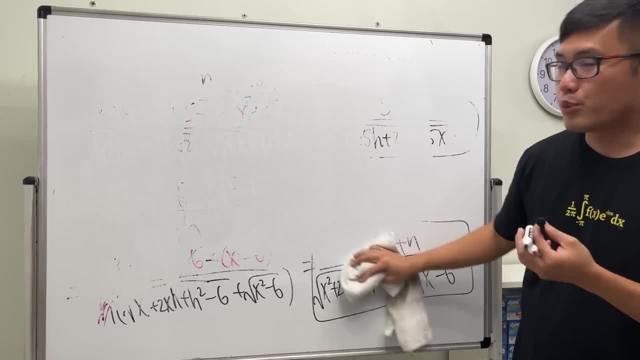 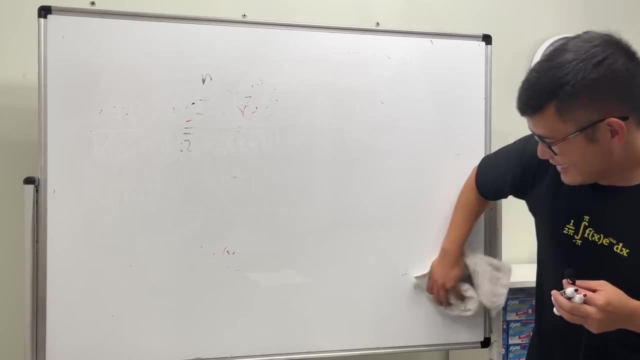 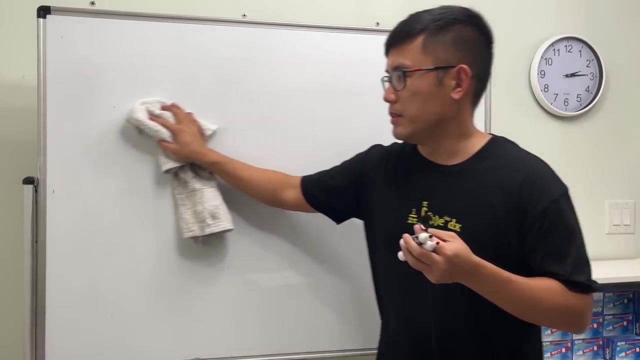 of stuff down and sometimes it's the same thing, the same expressions over and over, so that's why it seems really really long, especially if the question is pretty long already, then yeah, i really want to tell you guys, like this right here, it's actually not so bad right. calc 1. calc 2. 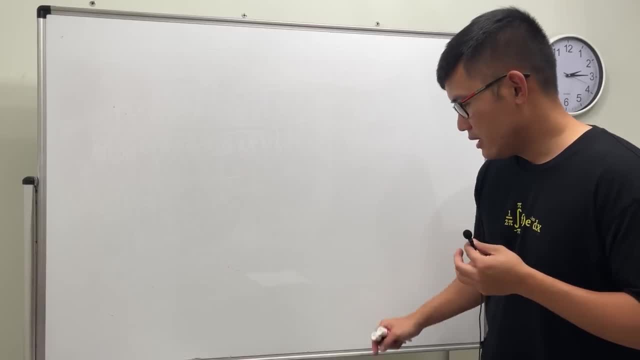 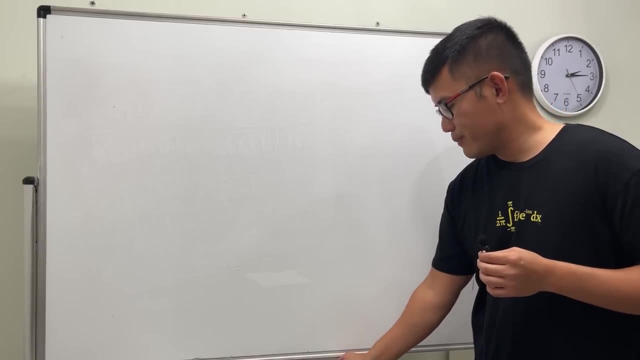 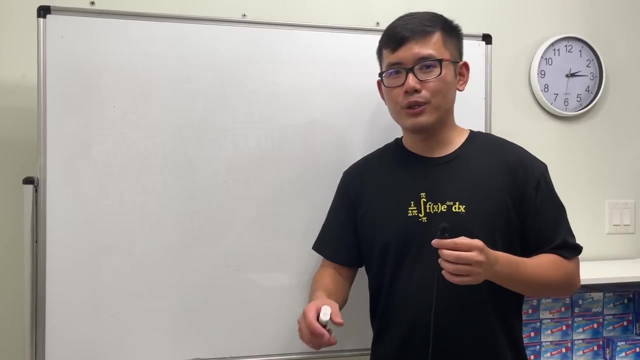 not so bad. wait for differential equation, yeah. and then, if you don't like computations, if you think computations are, uh, not that challenging, i would say: if you, yeah, if you think computations are not challenging, then try to take a proof. class analysis, yeah, that would really like work out your. 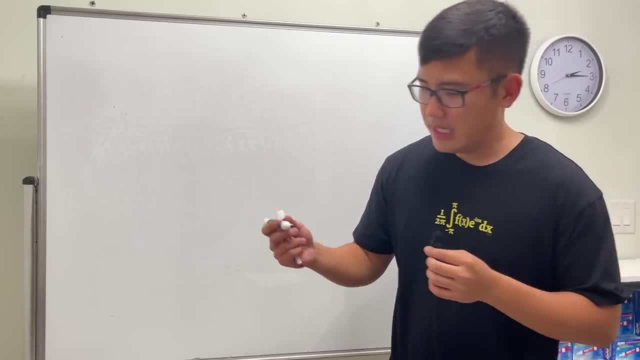 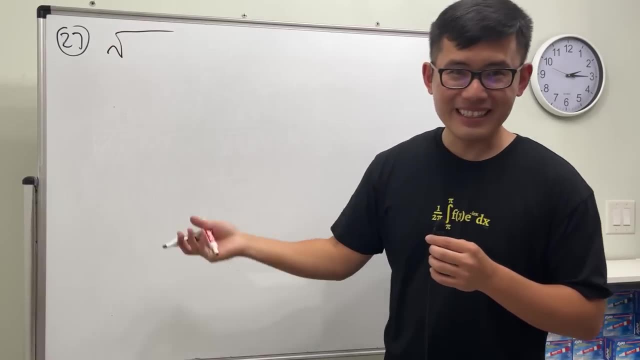 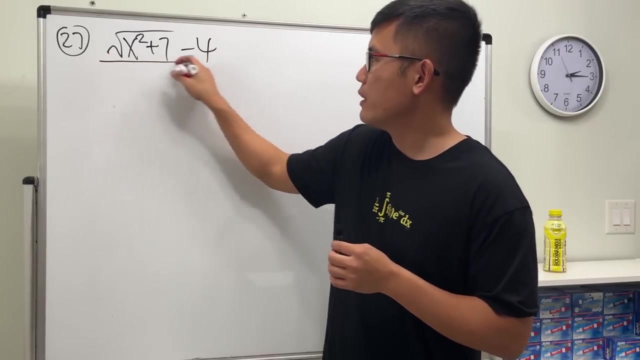 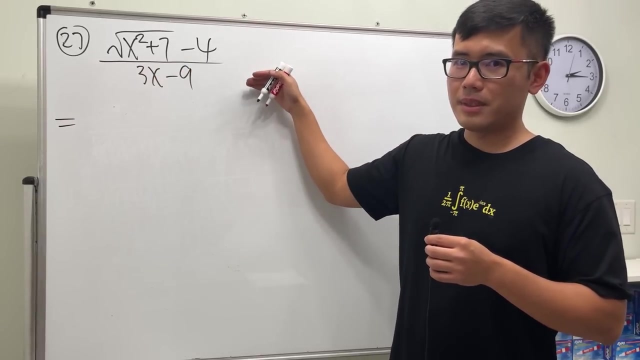 brain. okay, number 27: what's analysis? adult version of calculus. yeah, square root of x squared plus 7 minus 4, over on the bottom we have 3x minus 9.. you know the deal. multiply the count. you get on the top and also down the bottom first. we square this right. so we just get x squared plus 7 minus. 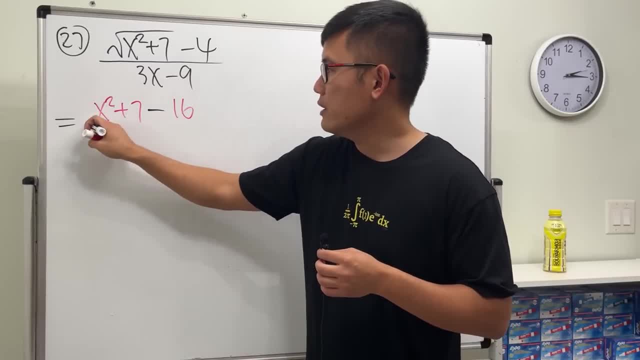 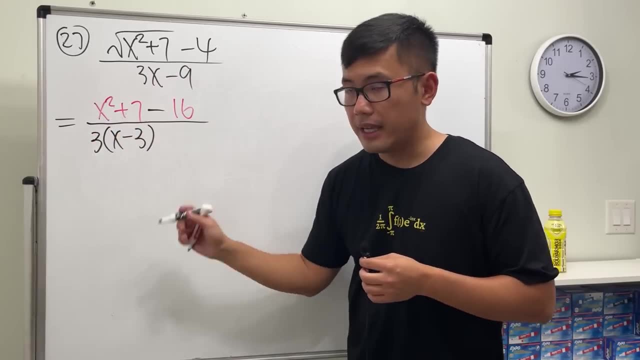 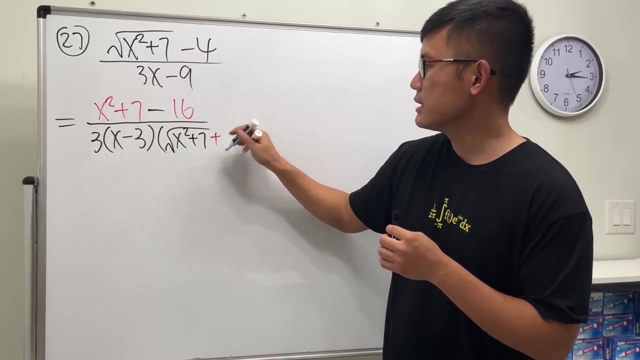 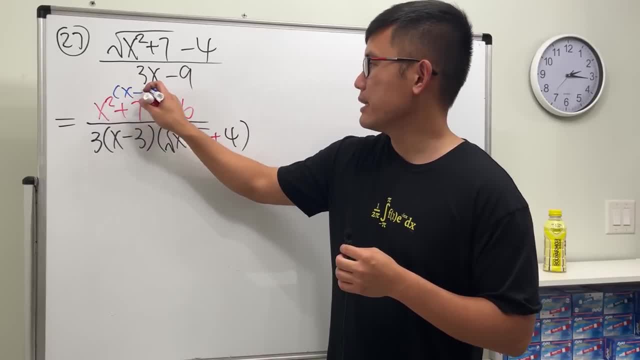 x square minus y, and then let's forget it in my goal you can try to practice doing twoặt QQ. and then let's ask: say x Escром, we can actually factor it as x Kmine. the second one is flush by N楽ans q2uration comma Claus passengers. xsen meets h to beöring in pasa Las STEVE, less significant two, honorary capital of the simple too blog. 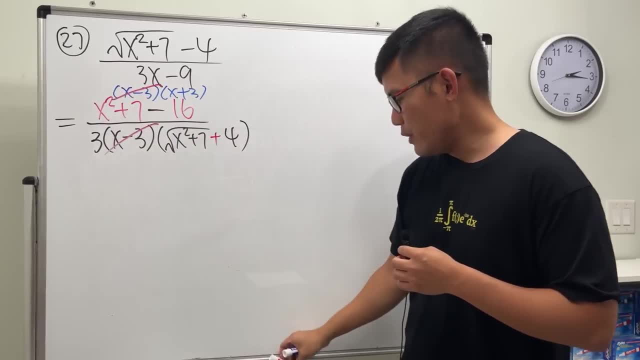 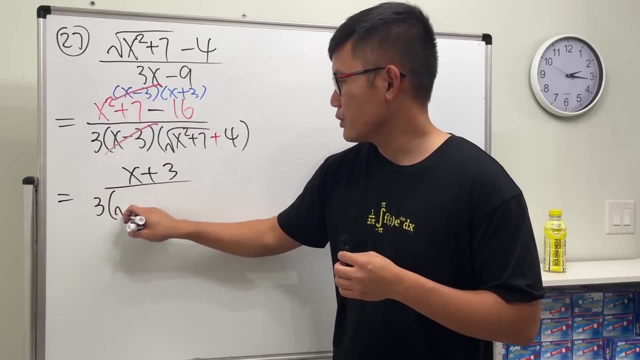 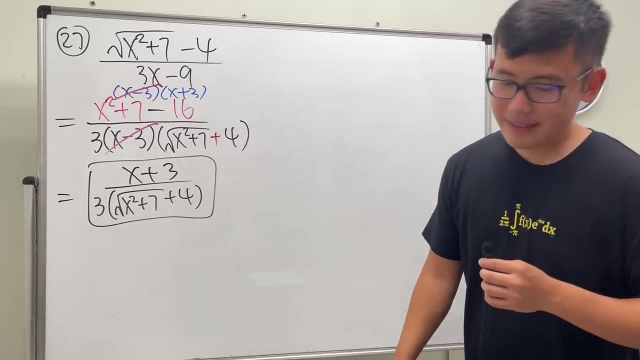 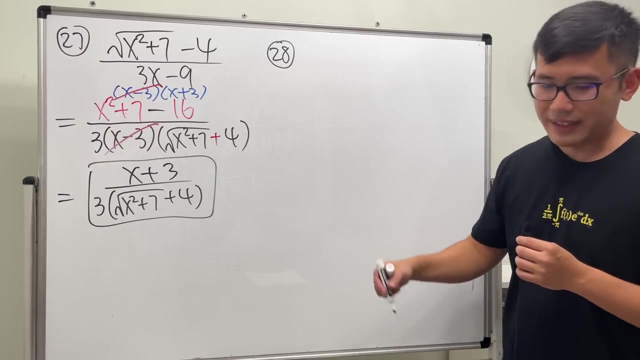 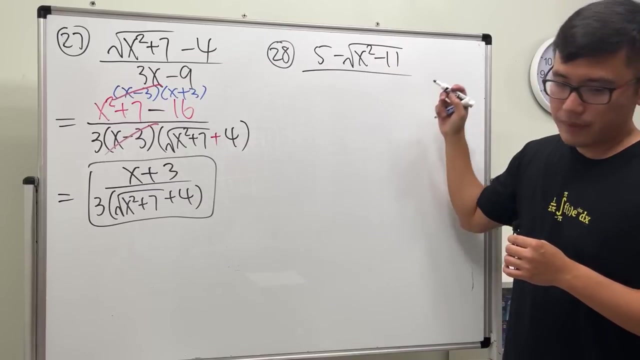 And we see this and that cancel out very nicely. so we just get x plus 3 over 3 times square root of x squared plus 7 and then plus 4.. Done, Yeah, Okay, number 28.. Alright, we have a square root on the top 5 minus square root of x squared minus 11 over 3, minus square root of x plus 3.. 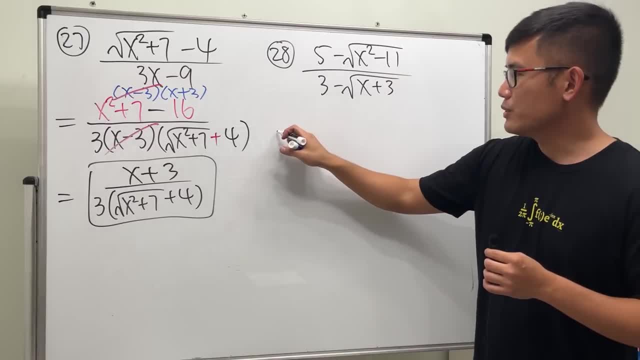 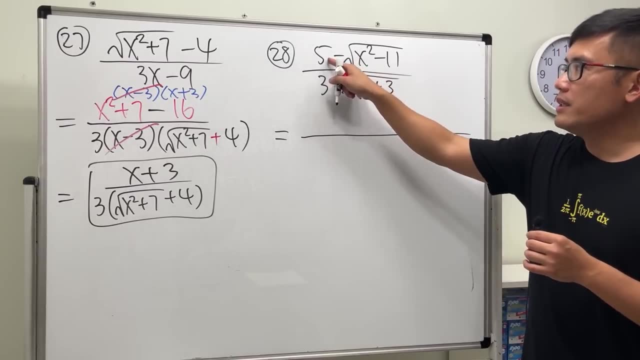 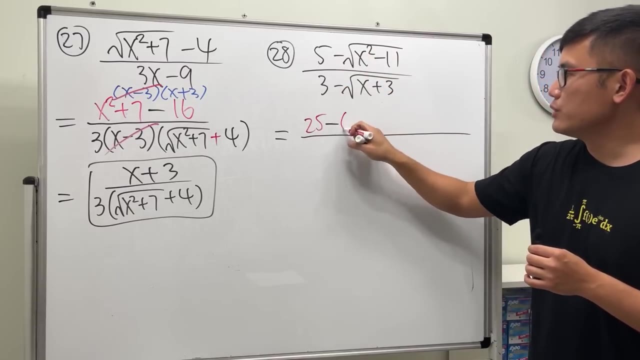 Yeah, square root on the top and also square root on the bottom, So just kind of keep track of what we are doing and all that stuff. So let's see: Square this minus the square of that, right? So we will first have 25 minus the square of this, which is just x squared minus 11.. 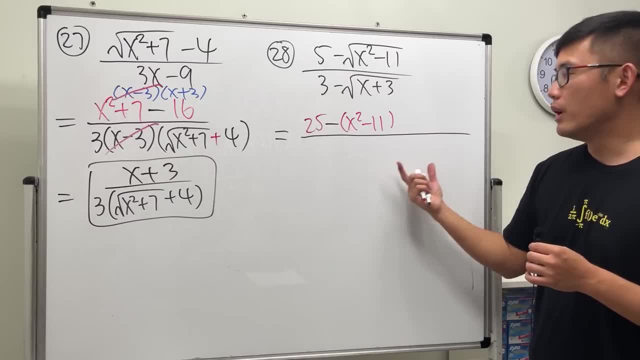 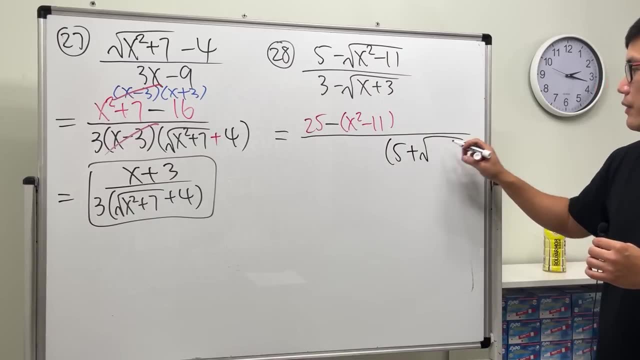 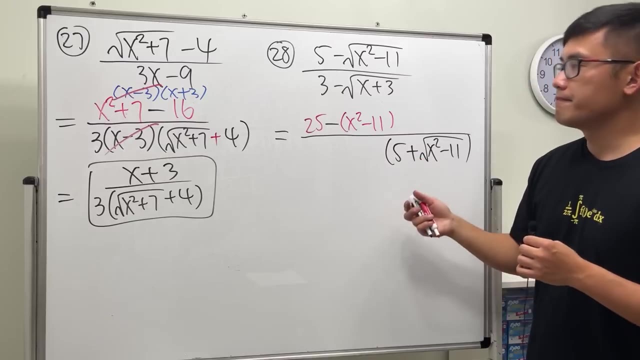 And we should have its conjugate on the bottom. So I'm going to put down its conjugate right here, and that is 5 plus square root of x, squared minus 11.. Because we technically multiply the conjugate on the bottom. But this right here also requires the conjugate huh. 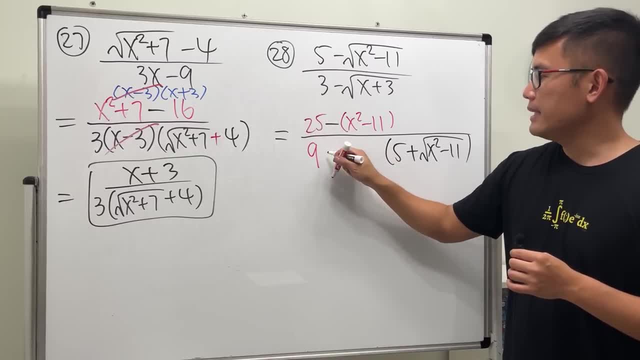 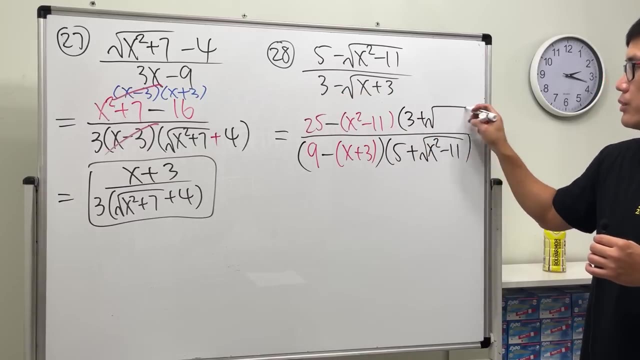 So I'm going to square this, which is 9, minus the square of that, which is x plus 3.. And this right here is a term, so I should put this in the parentheses And on the top right here we also need its conjugate, and that's 3 plus square root of x plus 3.. 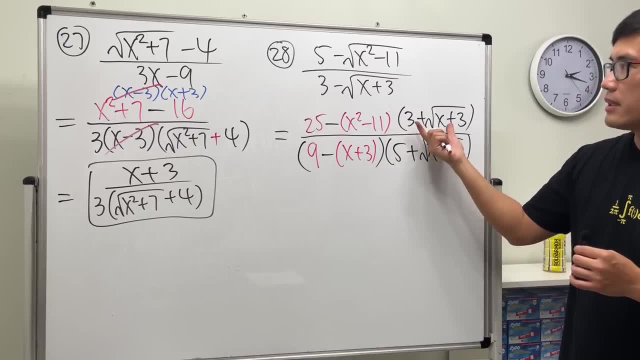 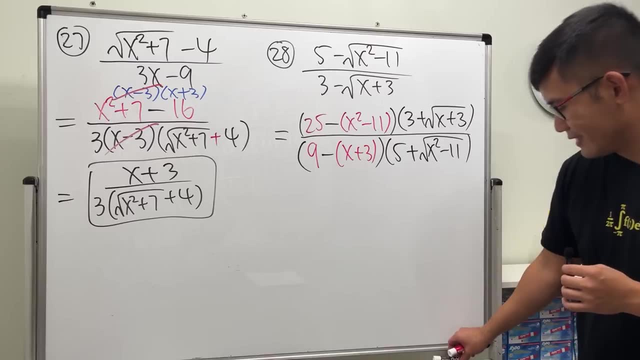 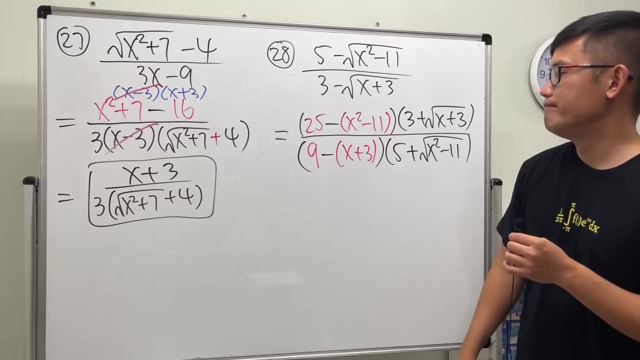 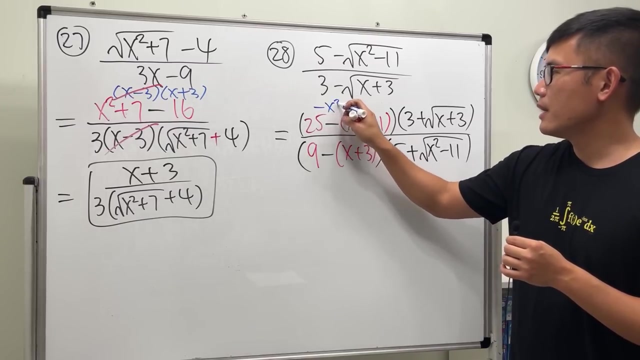 And this right here, because we multiply this on the top, so this right here also needs a parentheses, So it's like that. Yeah, pretty crazy stuff, I know. Okay, this right here, hmm, Okay, so this is negative x squared and then plus 11, so it's plus 36.. 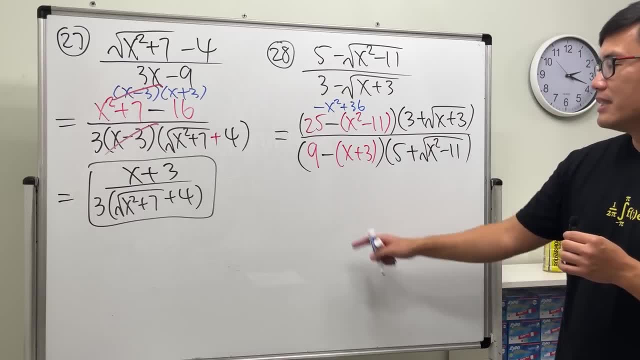 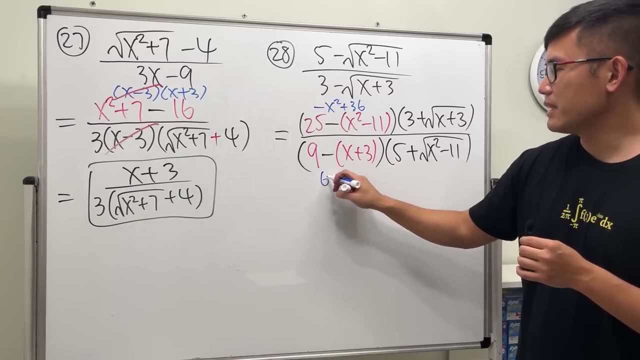 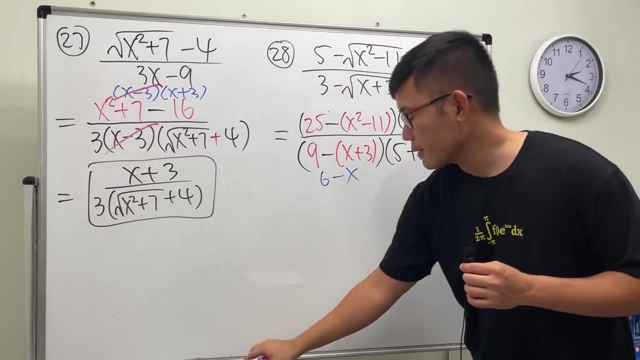 Okay, so yeah, and then this right here is Negative x, and then this is 9 minus 3, so it's 6 minus x. You know what? I'm just going to keep it like this. This is 36 minus x squared, which is the difference of two squares. 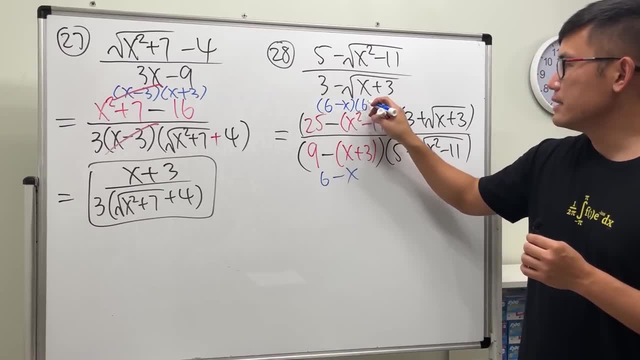 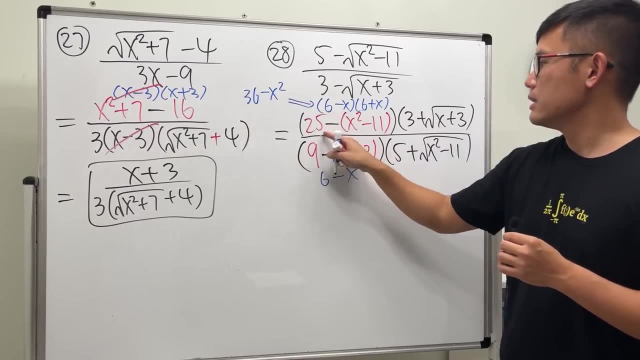 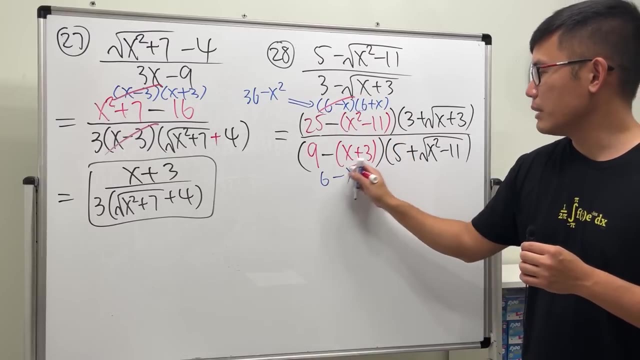 So we can factor it as 6 minus x times 6 plus x, Because earlier this was 36 minus x squared. so we factor it, Because now we see that they match exactly, so we can just go ahead and cancel them out. 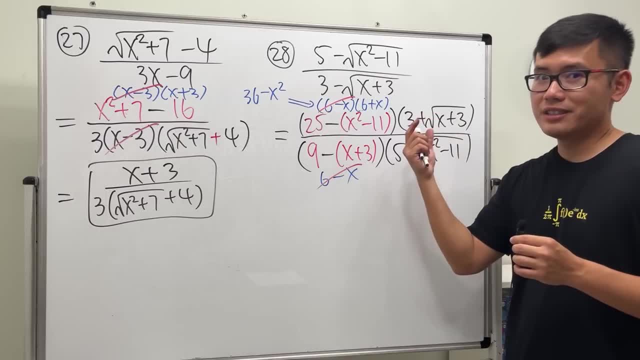 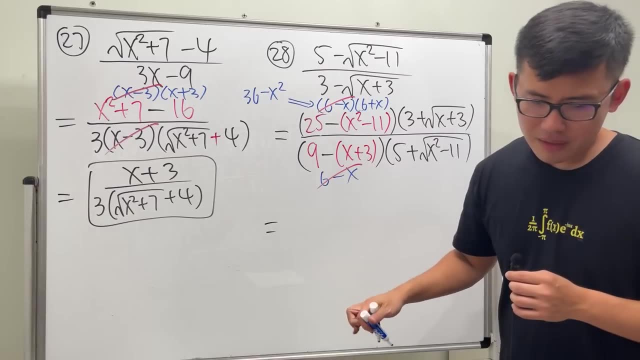 Yeah, And that's it. Do not multiply the conjugates anymore. We have some cancellations. we should be happy with it And we'll just write down the answer. And right here on my answer key, I wrote here: 6 plus x. 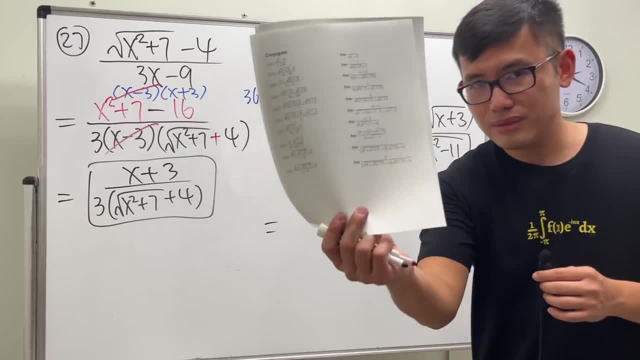 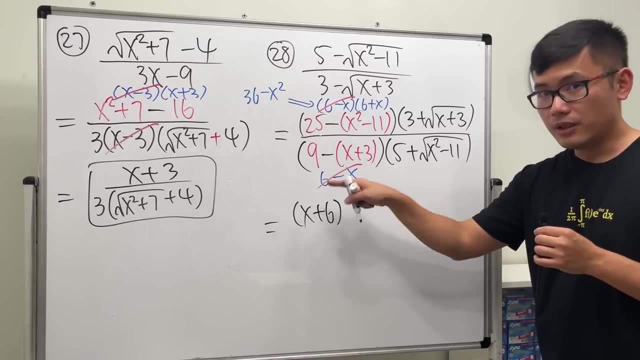 But let me write it as x plus 6.. Yeah Yeah, Usually we like to have the x go first, And if it's a plus, the word of addition doesn't matter. So x plus 6, and then all that stuff. 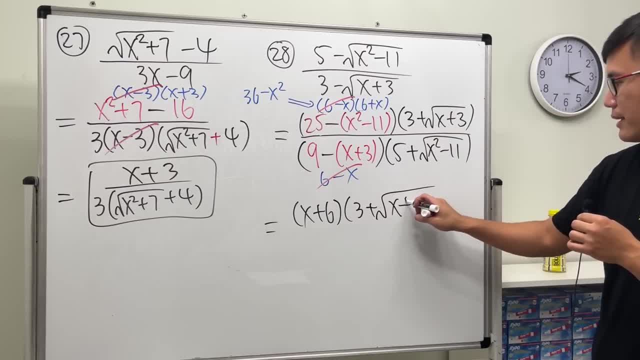 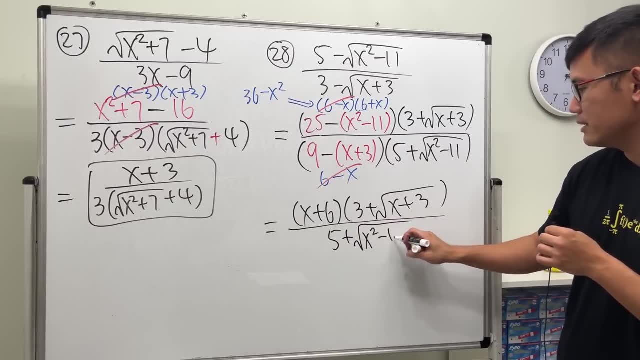 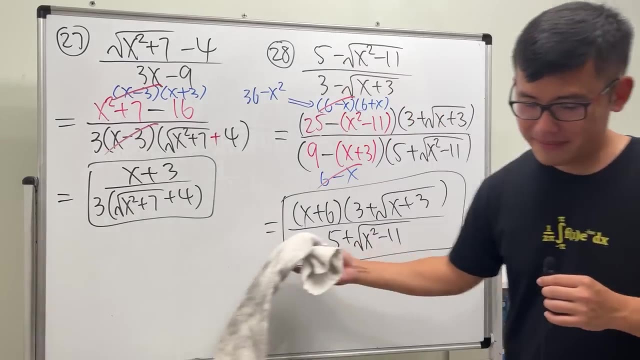 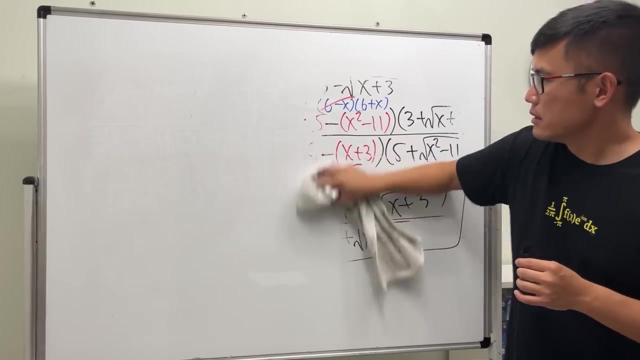 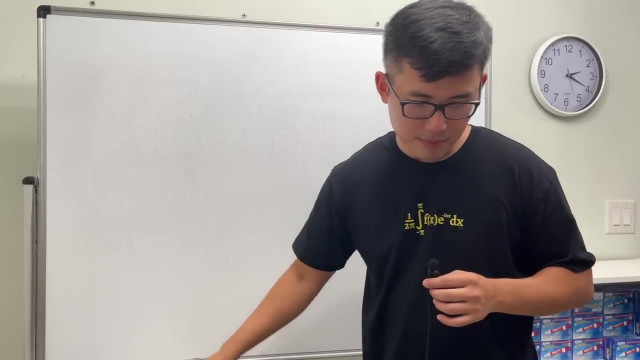 So 3 plus the square root of x, plus 3 over this guy, which is 5 plus square root of x, squared minus 11.. Oh my goodness, Yeah, just like that. Okay, Okay, number 29.. We have a square root instead of a square root. 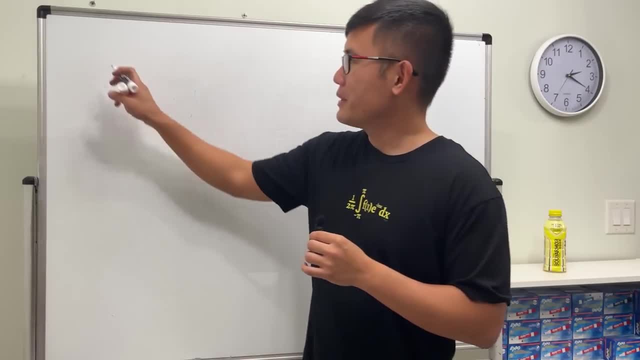 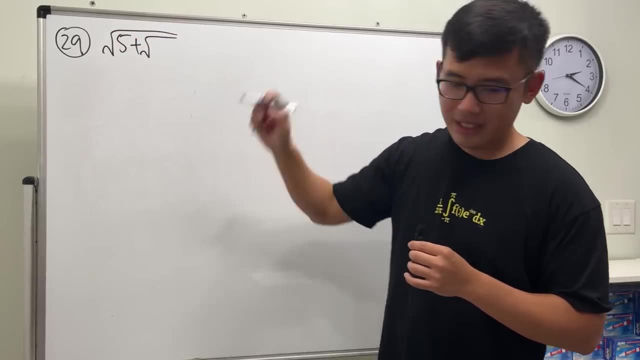 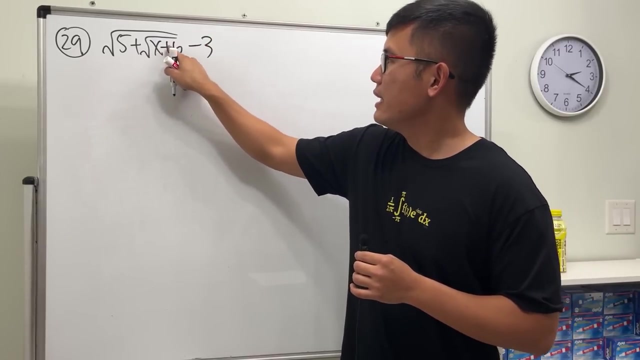 So we need some conjugates, of course. Alright, so it looks like this: Square root of 5 plus the square root of x plus 6. And then outside here we have the minus 3.. And then all over, x minus 3.. 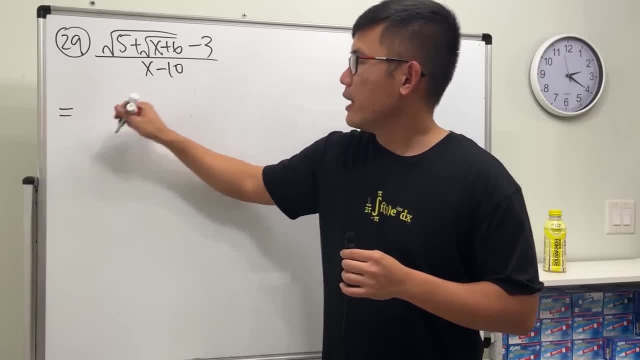 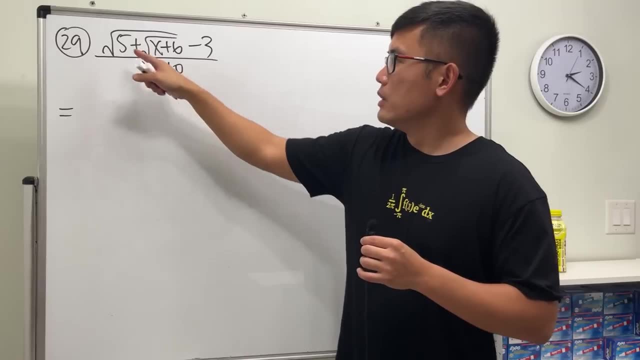 Okay, Okay, I'm going to multiply the time at the bottom by this conjugate, So it's this plus that. First I will square this, So I will just get 5, and then plus square root of x plus 6.. 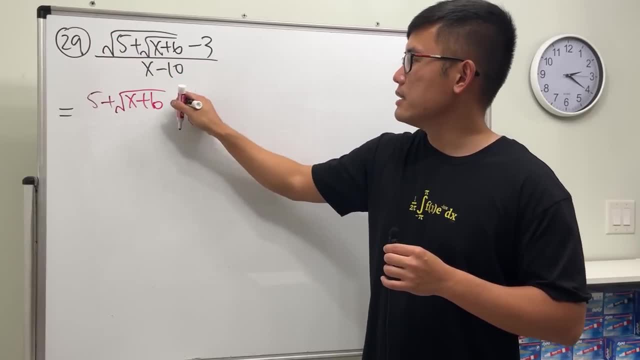 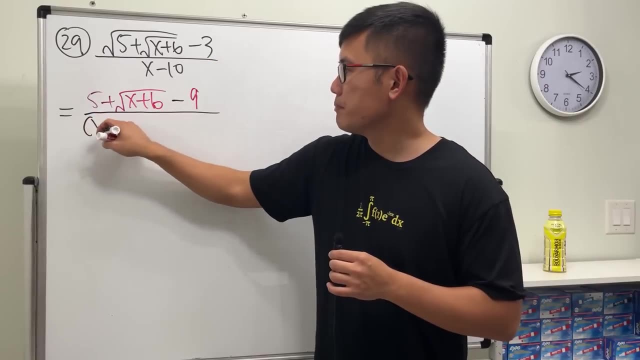 So pretty much the outer square root gets cancelled, And then minus the square of that, which is 9.. And then the bottom. here we have that x minus 10.. X minus 10.. And don't forget, we need a conjugate right. 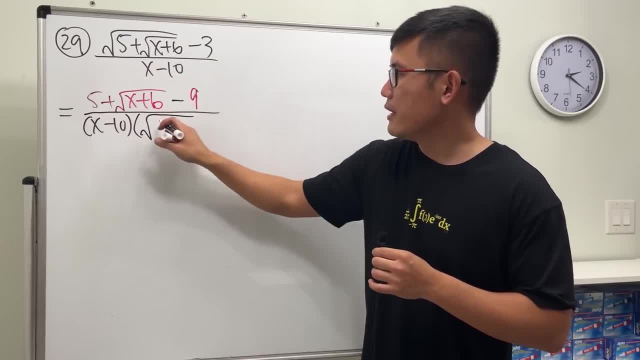 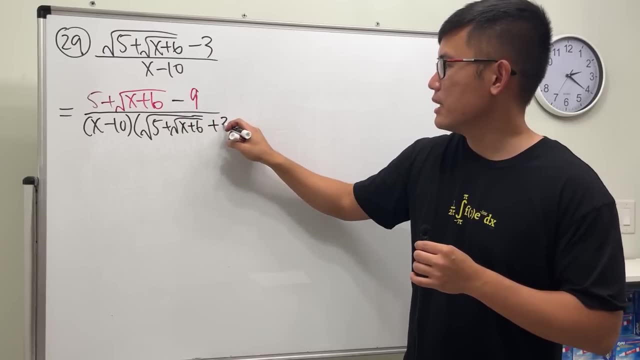 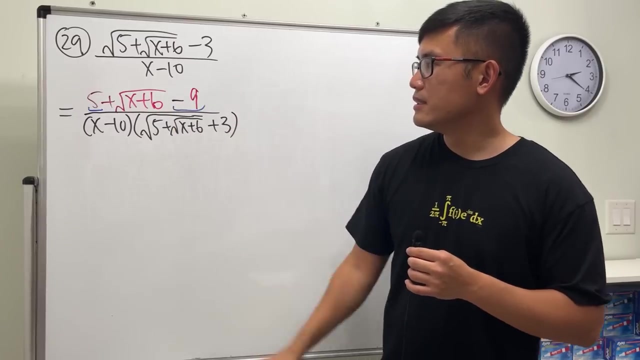 So that was the big square root, and then 5 plus the small square root, x plus 6. And then change the minus to a plus and we have that 3.. So it's like that. And notice though, 5 and minus 9 is minus 4, right. 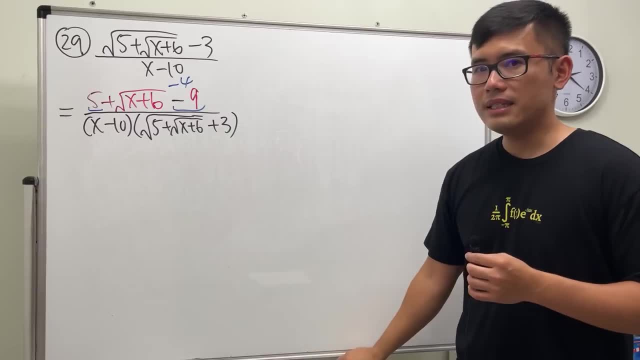 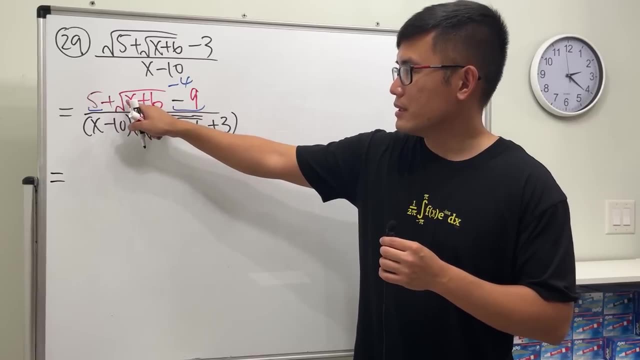 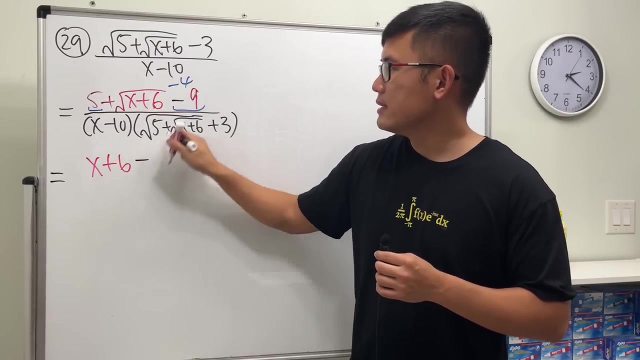 So we have this minus 4, and that's a square root expression, so we need a conjugate again. So I'm going to just square that which is x plus 6, and then minus 4 squared, which is 16,, like that. 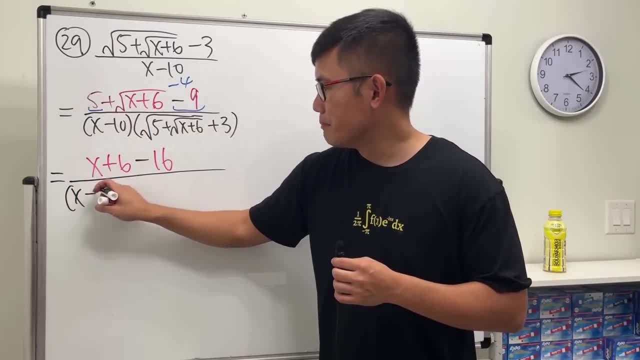 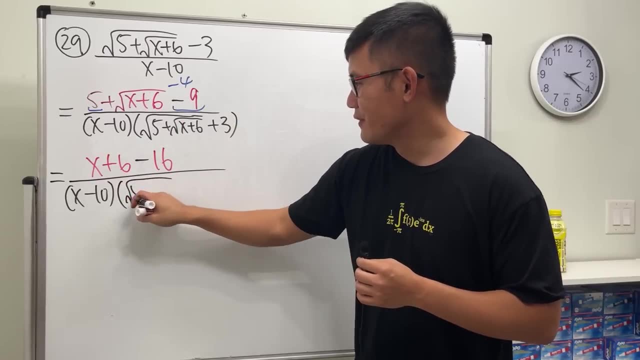 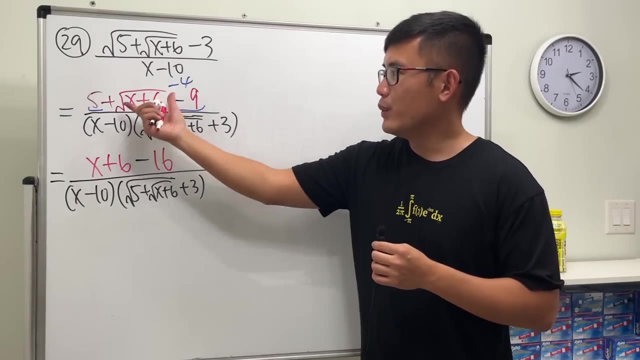 over. okay, we have that: x minus 10.. The first conjugate from the first expression, which is the square root 5, plus the square root of x plus 6, and then plus 4.. Plus 3.. And then earlier we also need that conjugate- 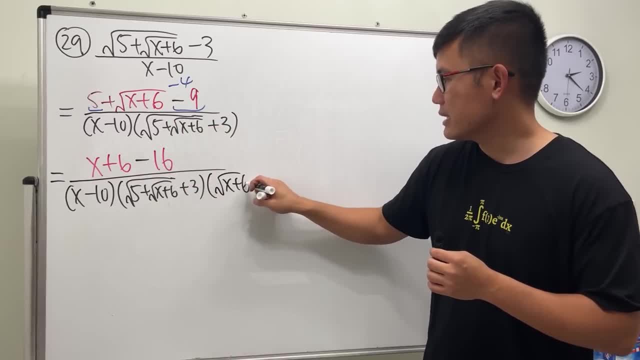 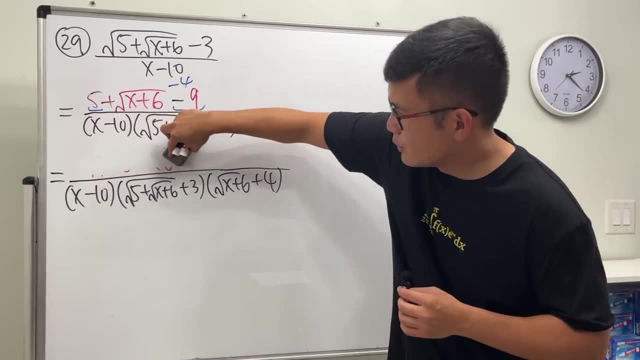 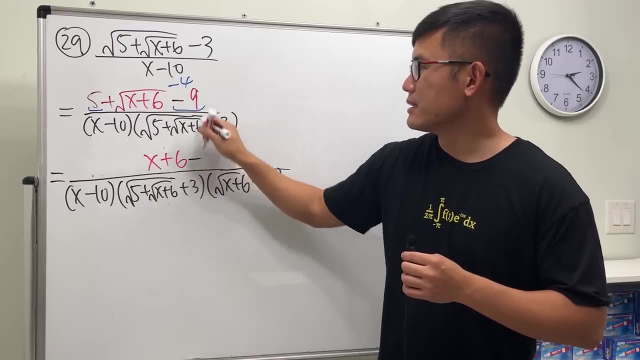 and that is going to be square root of x plus 6 and plus 4.. Yeah, Yeah, And you know, I would like to write it down better for you guys. Here it was x plus 6, and then minus the 4 squared, which is 16.. 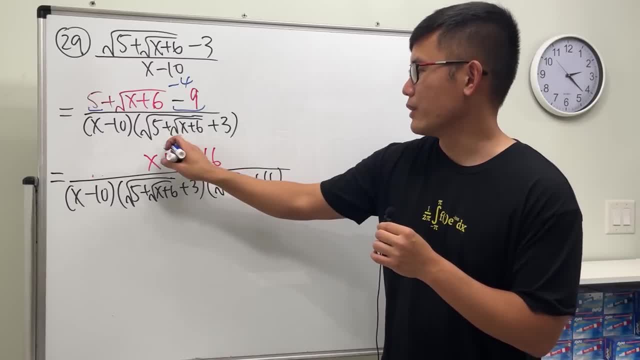 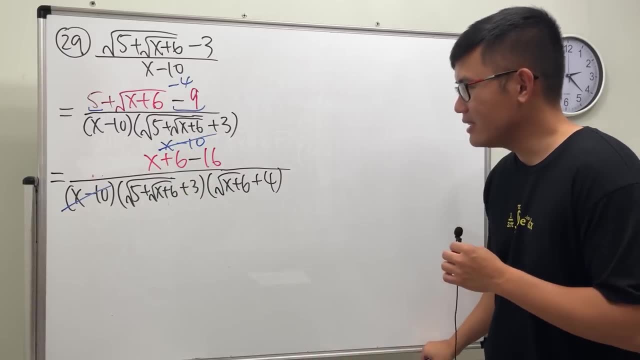 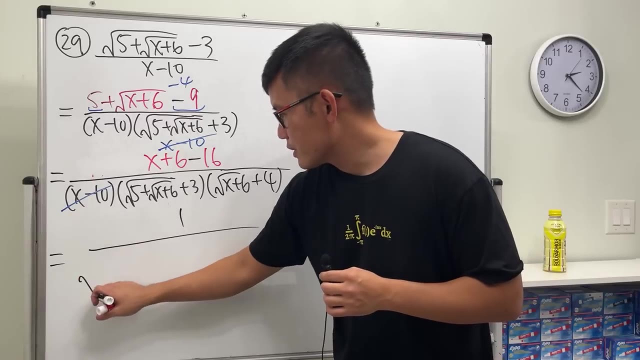 Now 6 minus 16 is minus 10, so this is just x minus 10.. But we see it, x minus 10, x minus 10 can solve very nicely, so we just have that. So finally we have 1 over big square root 5 plus small square root, x plus 6,. 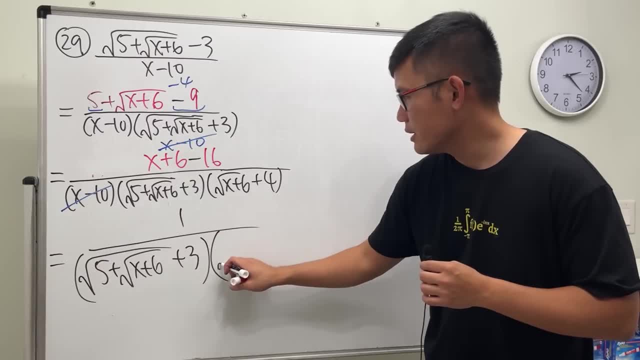 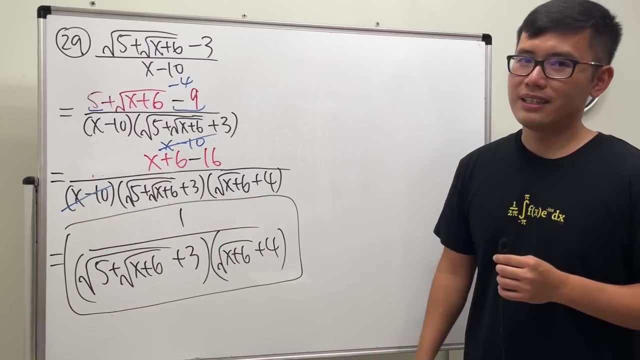 and then plus 3, parentheses, another parentheses, square root of x plus 6, and then plus 4.. Whew, Yeah, so just like that. Okay, number 30, it's similar, I'm going to fit it here. 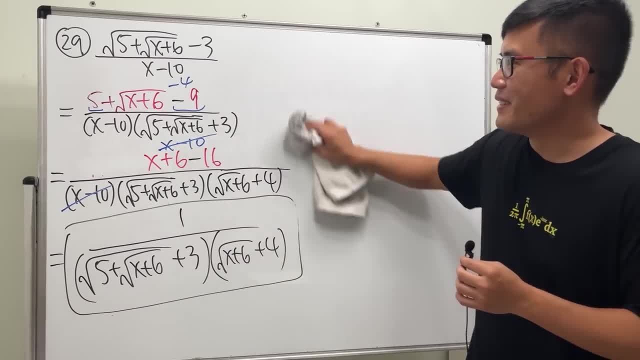 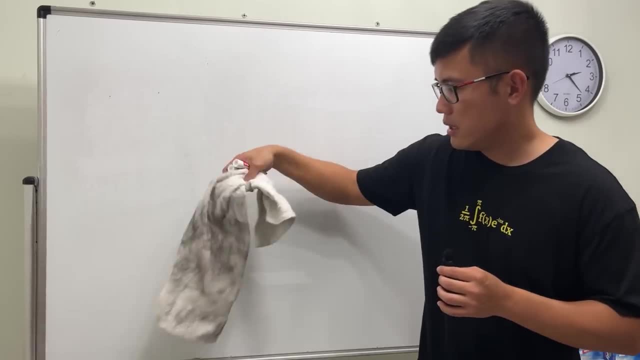 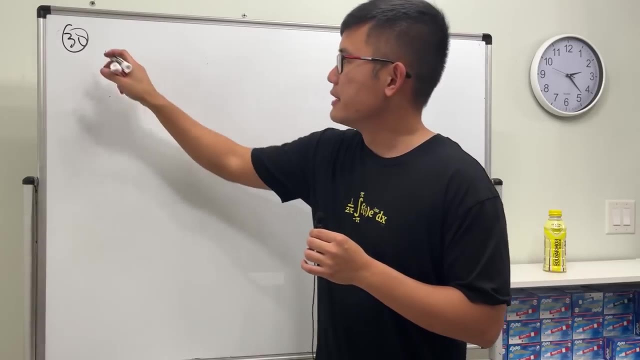 No, it's going to be too painful if I fit number 30 here too, So I'm going to just erase this. Okay, number 30.. Square root of 13. Plus Square root of 5x minus 11.. 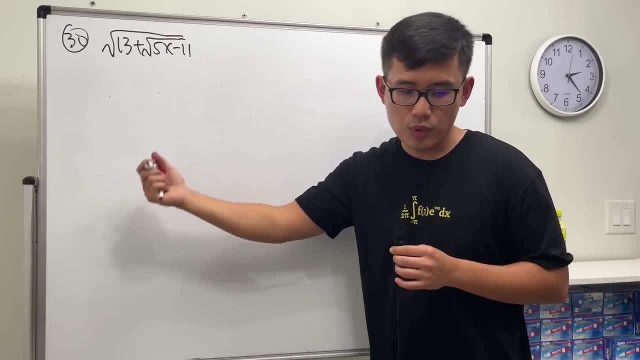 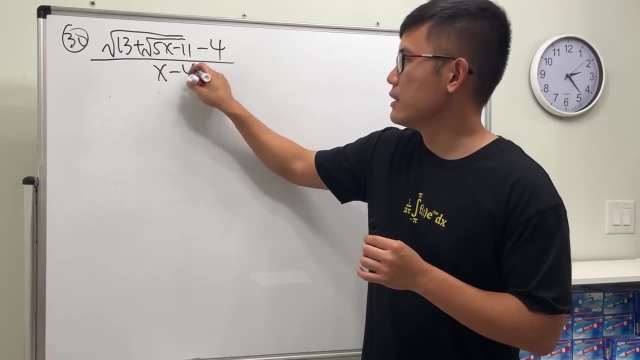 All right, so this is called the nested square root. So a square root instead of another. And then outside, here we have the minus 4 and the O over x minus 4.. All right, so similar equation, Let's do it again. 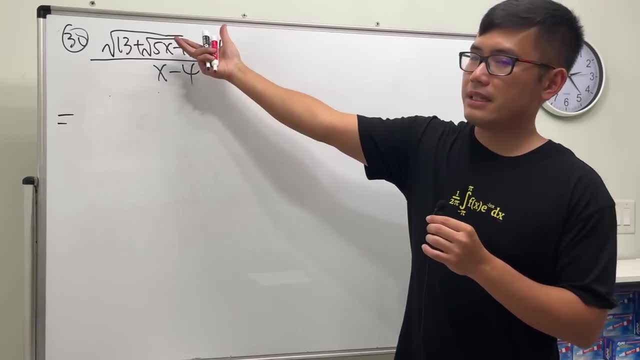 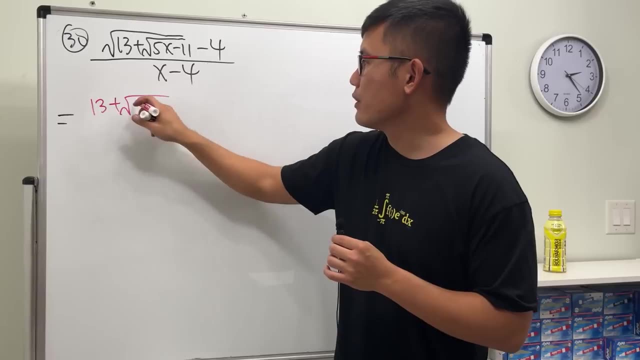 So first multiply the top and bottom by the conjugate. So I'm just going to square this, which is 13 plus square root of 5x, 5x minus 11.. And then minus this square, which is 16.. 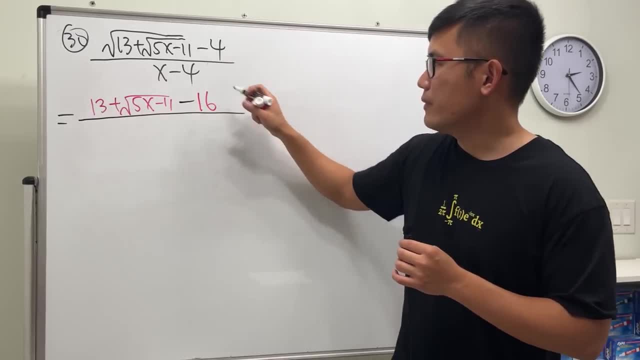 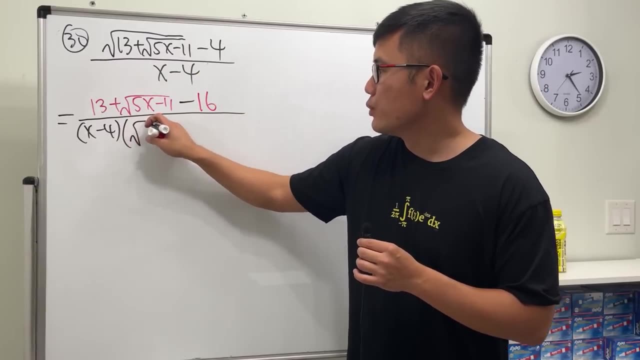 So that's what we have, And then over here we have that x minus 4.. And then we need that conjugate right here, And that's going to be square root of 13 plus square root of 5x minus 11.. 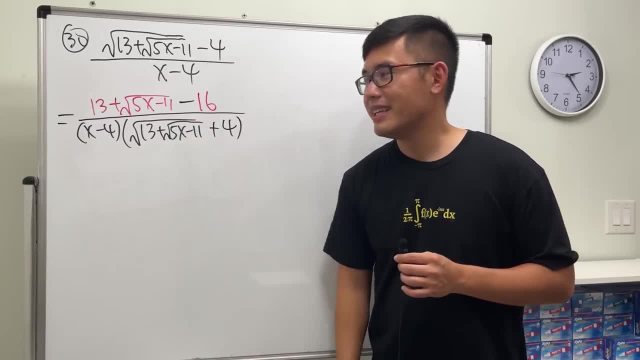 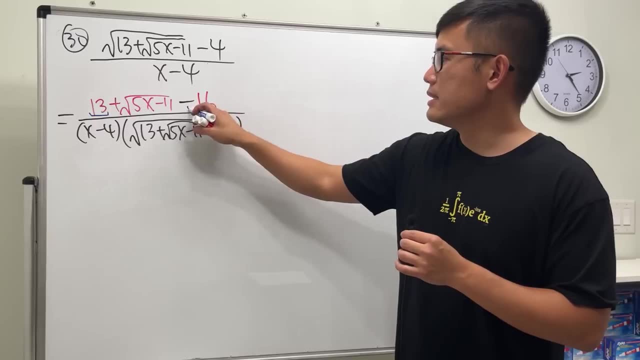 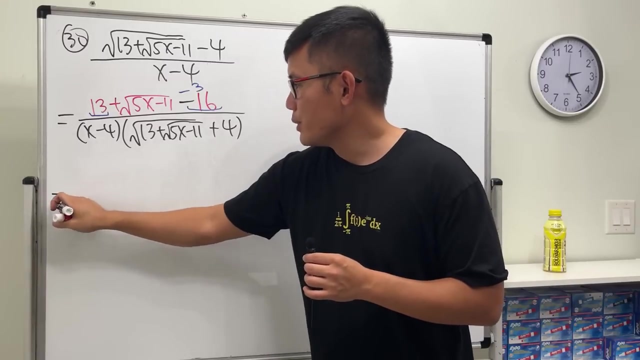 And then my plus 4.. Plus 4.. Okay, now we see that these two numbers can be combined. Okay, 13 minus 16 is minus 3.. So we need the conjugate for this right. So that's going to be what. 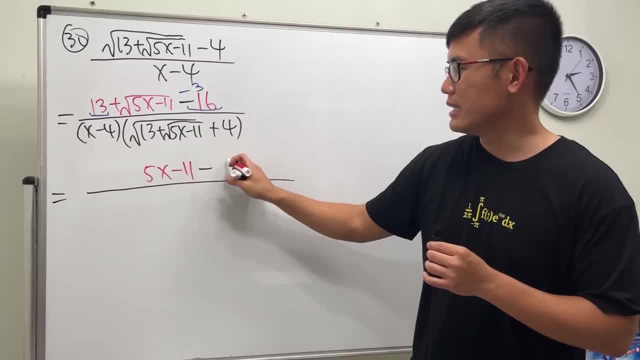 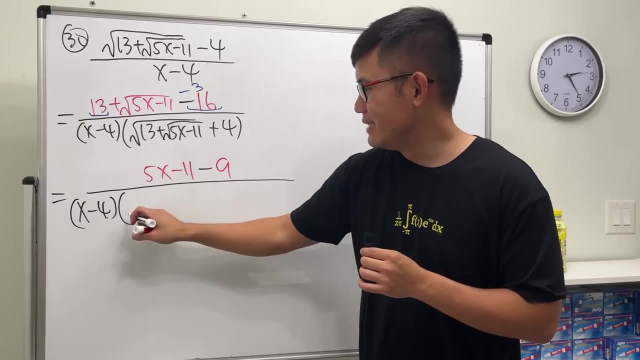 5x minus 11.. And then minus 3, squared, which is 9.. And then, on the bottom here we have x minus 4 times this thing, So square root of 13 plus square root of 5x minus 11.. 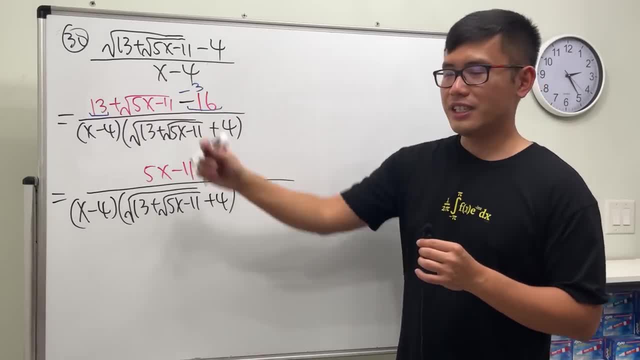 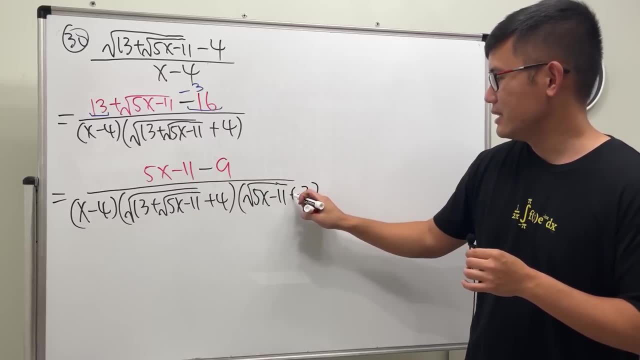 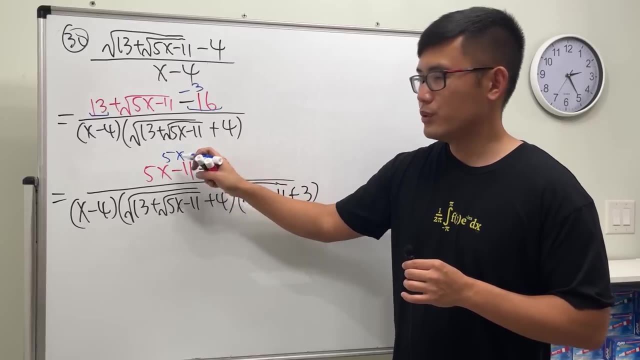 And then plus 4.. And then the conjugate which was square root of 5x minus 11 plus 3.. Okay, On the top this is 5x minus 20.. Which we can factor out a 5.. 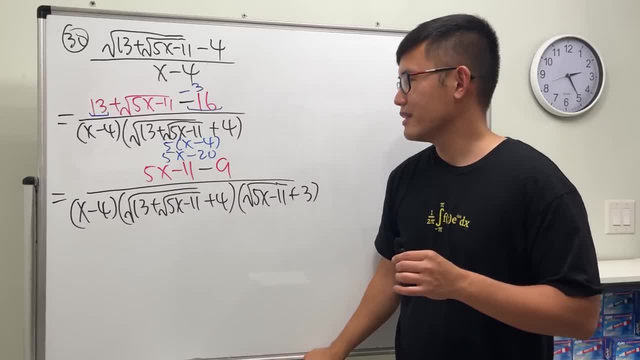 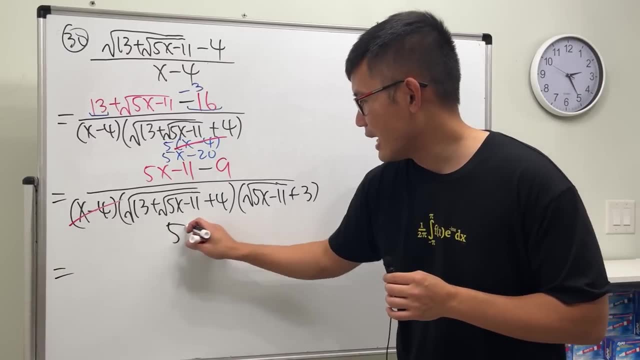 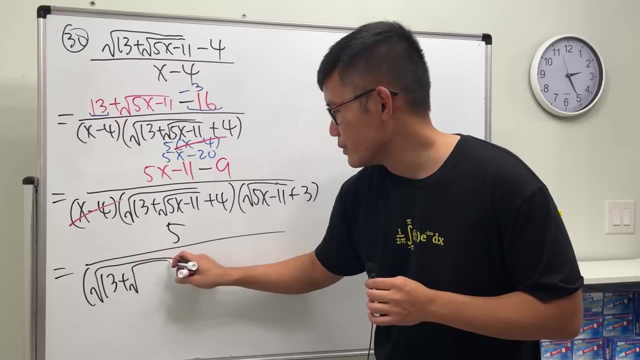 That's x minus 4.. Can anything cancel? Yes, x minus 4.. Cancel out: Very nice. So finally we have 5 over this thing. So big square root is 13, plus a small square root of 5x minus 11, and then plus 4.. 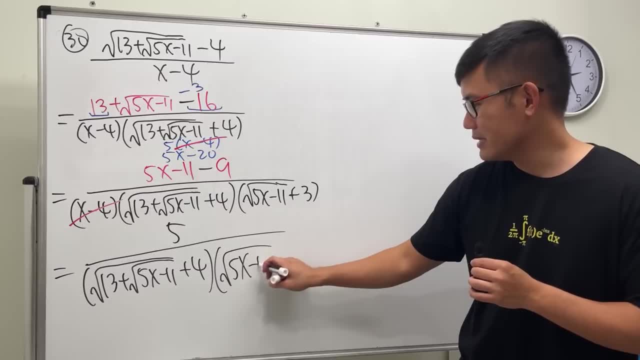 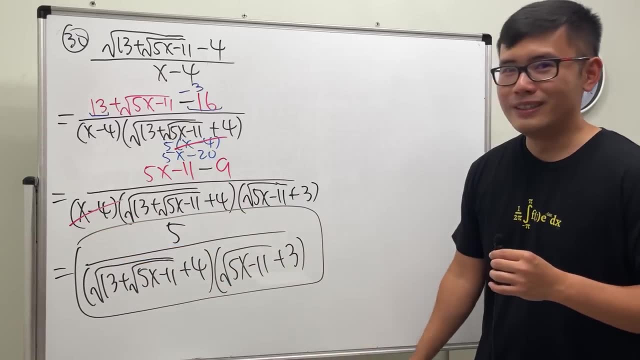 And then the square root of 5x minus 11, and then plus 3.. Whoo-hoo-hoo, Look at that And the box is the answer. And then hit the board. Okay, All right. 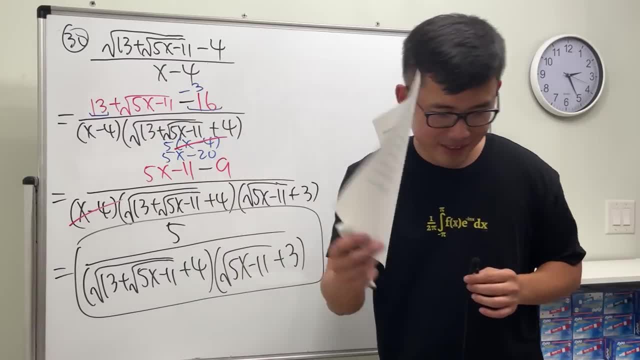 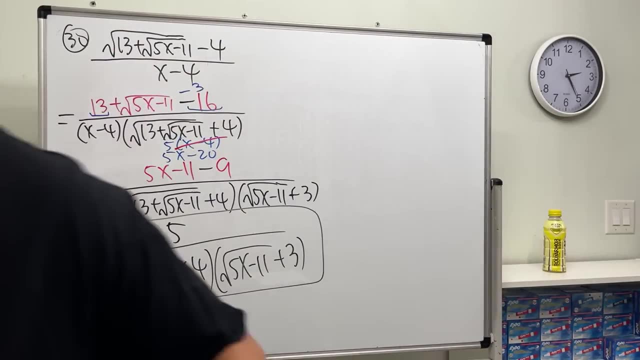 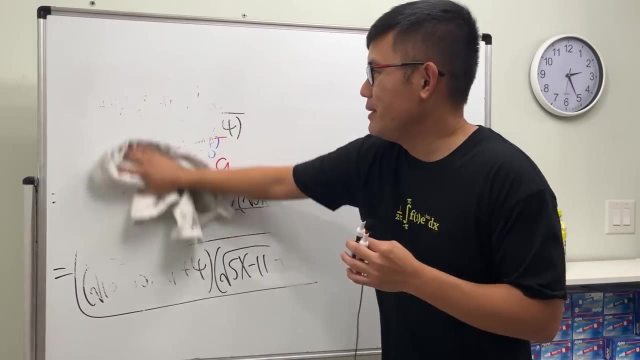 So that should be enough practice with the conjugate business. So the second sheet done, All right, Okay, All right, Let me take a look. Good, So it looks like so far each question takes about three minutes, while maybe the 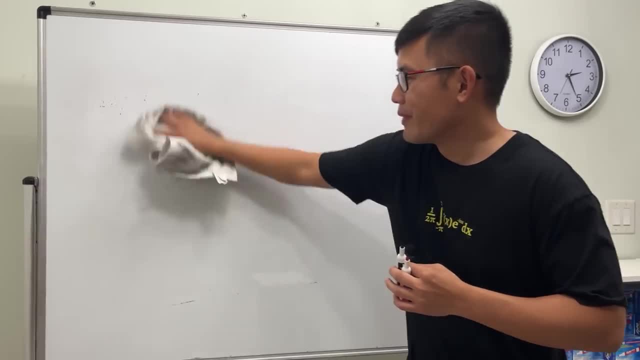 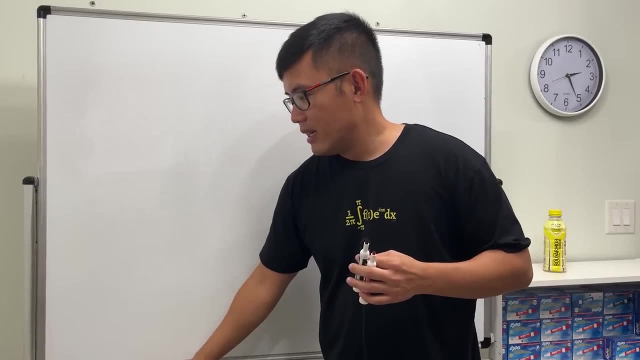 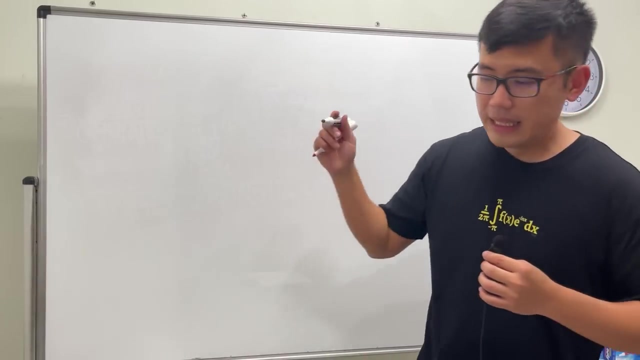 erasing the board takes about a minute or two. No, not really like 10,, 12,, 20 seconds. But let me tell you, the last 10 questions are the killer. Partial fractions- they are the killer, Anyway. 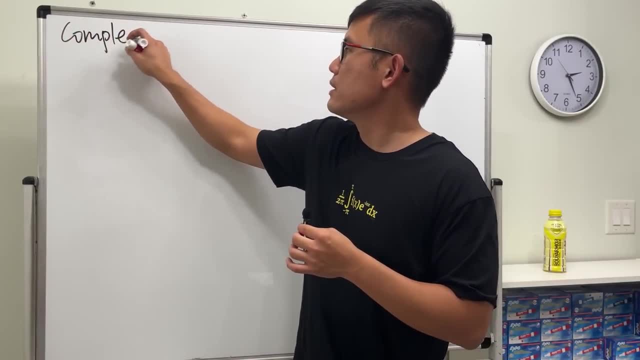 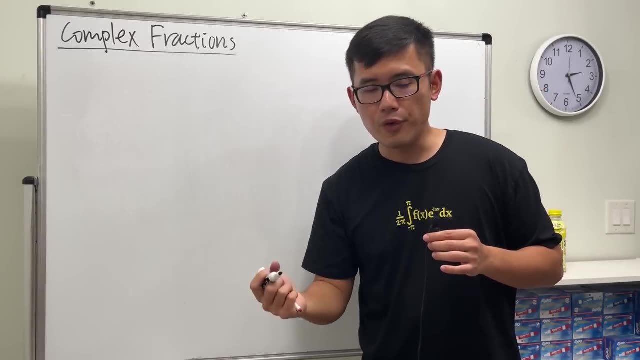 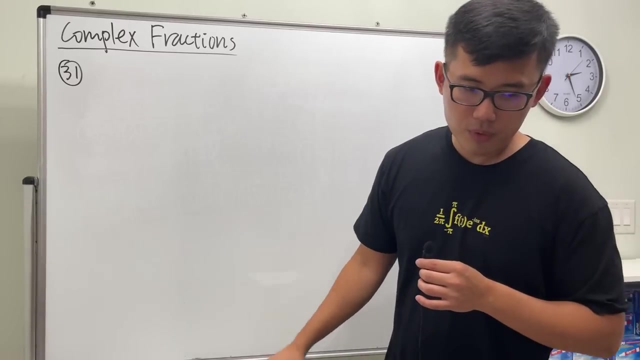 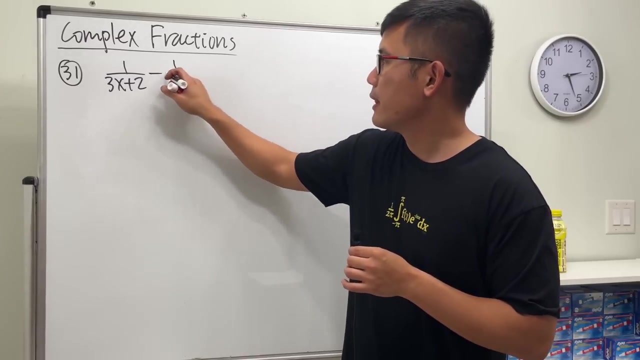 Next, We are going to do the so-called complex fractions. Complex fractions just means that we have small fractions instead of big fractions, And I'll show you, guys, the best way to simplify it. Number 31. I'm going to give you 1 over 3x plus 2 minus 1 over 5.. 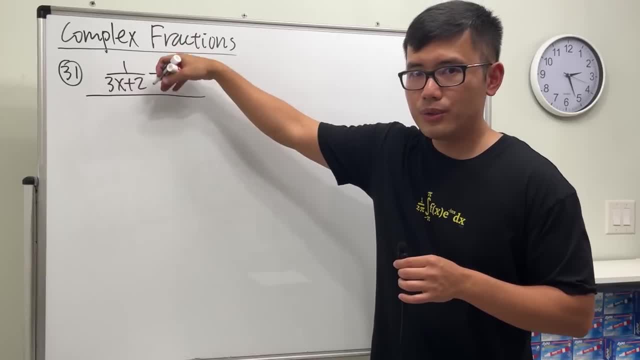 Oh see, One little fraction, two little fractions Instead of a big fraction. I'm going to give you 1 over 3x plus 2. Instead of a big one Like this: Yeah, So how do we take care of this? 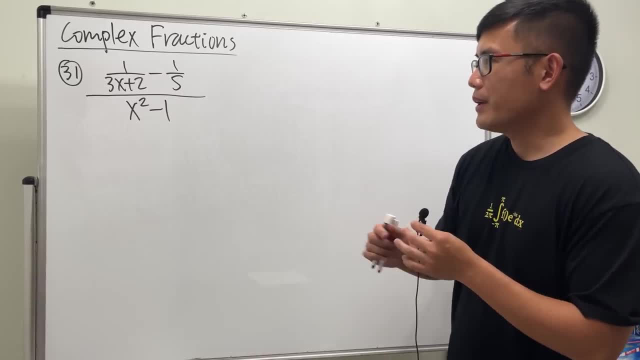 All right. Pay attention to the small fractions, especially the denominators. They don't have anything in common. right 5 and 3x plus 2.. Then in that case, just multiply the top and bottom by the lowest common denominator. 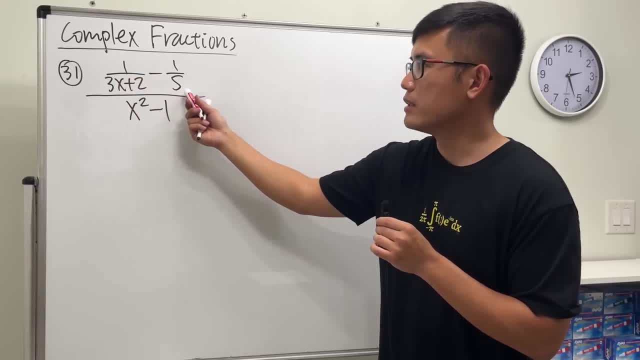 So that would just be 5. And then 3x plus 2. And then, of course, let's do the same on the bottom, So that's the same, And then 3x plus 2.. 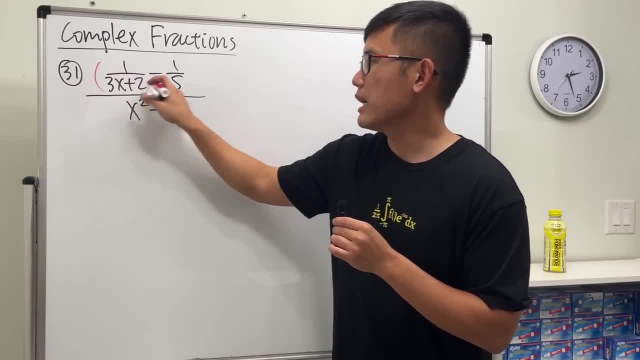 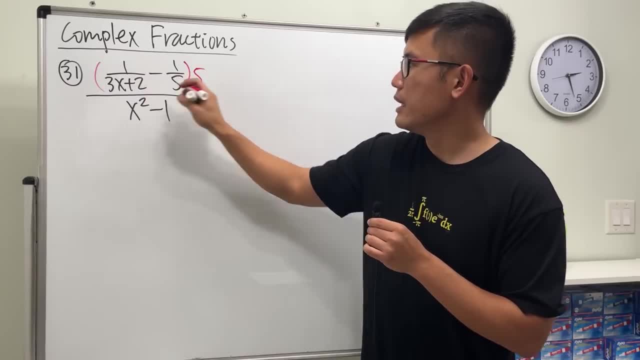 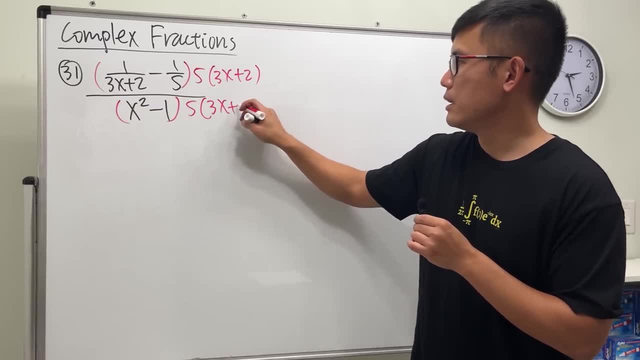 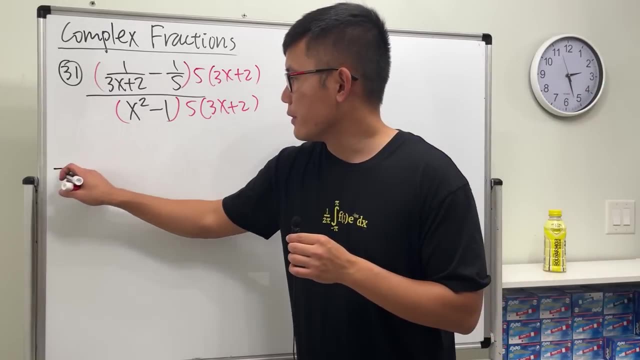 And then, of course, let's do the same on the bottom. So this is what we would have to multiply when we have a complex fraction, And then just be really careful, Take this times that The 3x plus 2 will cancel. 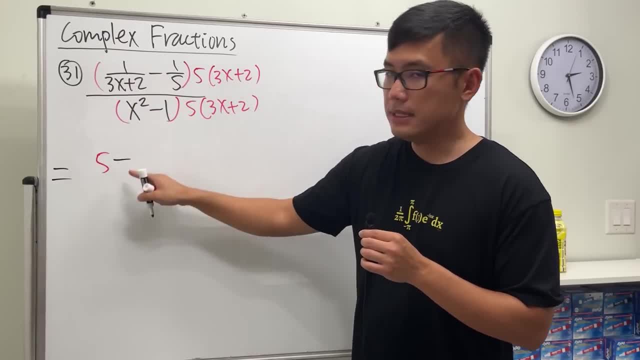 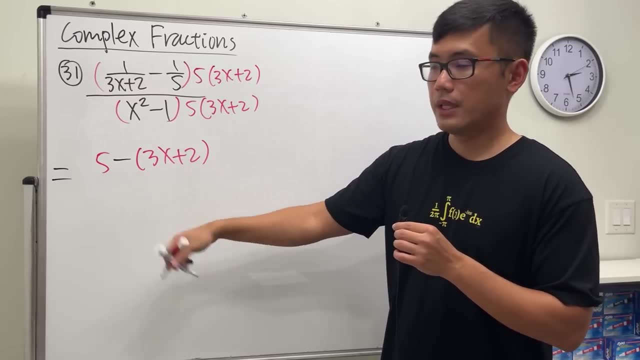 So we will have the 5 first And then minus 1 fifth and 5 cancel And we have that which is 3x plus 2.. Ok, on the bottom let's just rewrite everything again. so we have the five, but the x grade we. 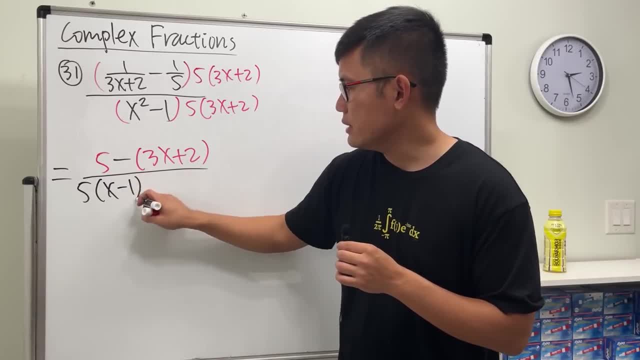 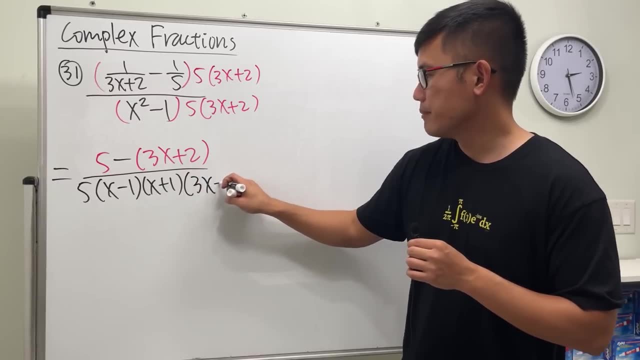 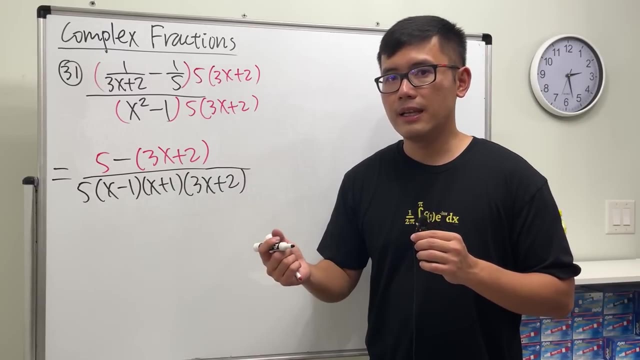 can factor it. so let's go and factor it. so x minus one, x plus one. so this is from here. and then we have that three x plus two, and you guys notice that this is very similar to when we were talking about expanded and cancel. you see the three x plus two. three x plus two. 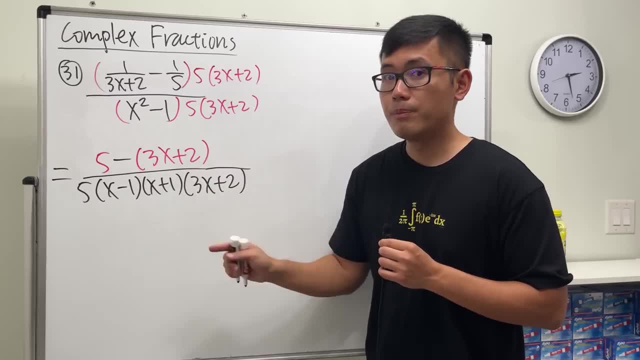 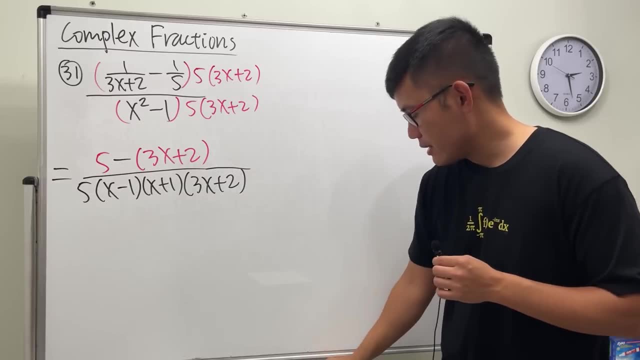 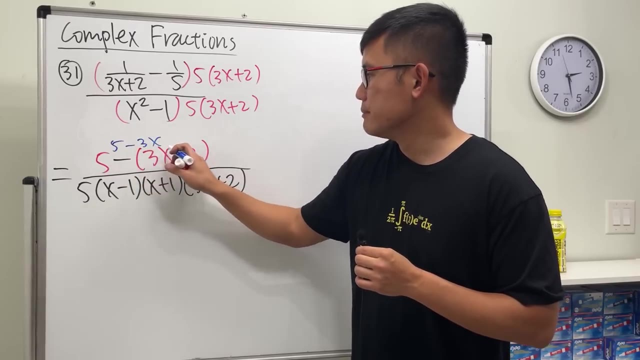 they are both in parentheses. can we cancel that? no, because right here we have the five minus that, so we have to work that out. we have to come by them, okay? so this is five minus three x minus two. so that's going to be five minus two is three, right? so this is. 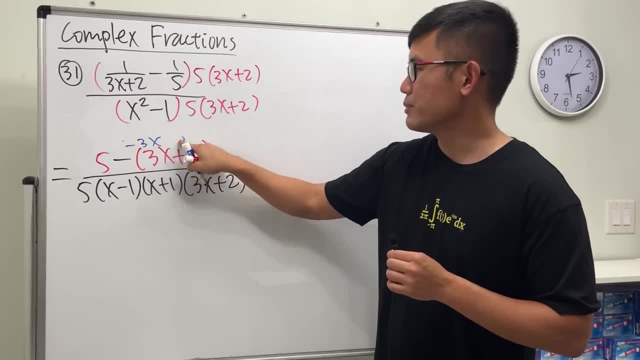 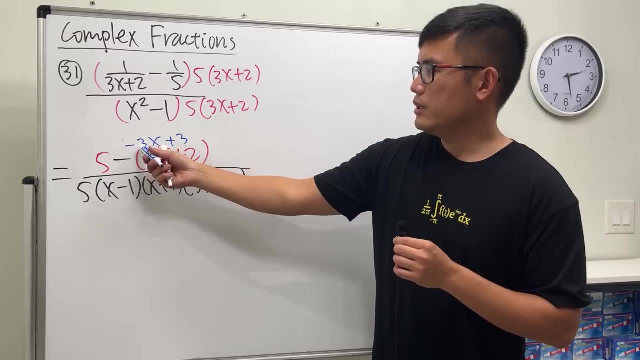 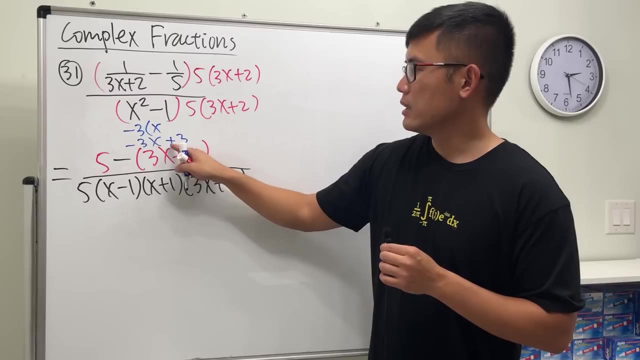 let's just write: yes, five minus two is three. so let me just put it down like this: yeah and notice: this is negative three, x plus three. we can factor our negative three and then that will give us x. but originally here was negative, wasn't positive three, we took our. 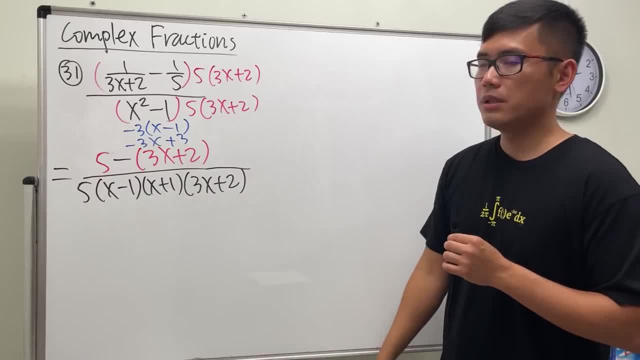 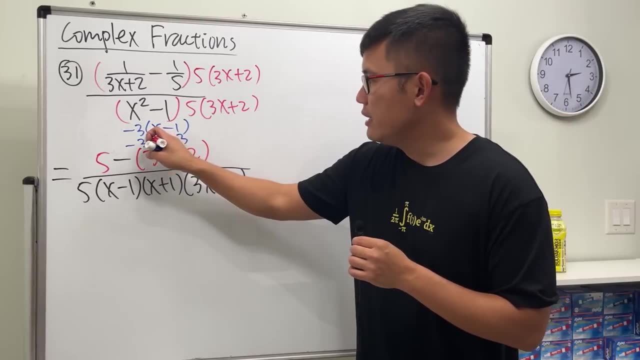 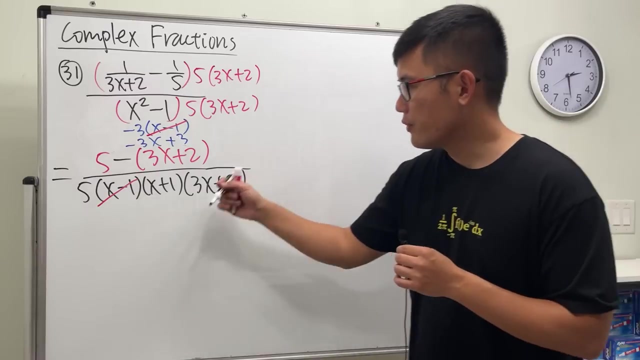 negative three. so this is minus one. so that will be the simplification on top. so just make sure that you really work out the top and then simplify it. then the x minus one can be cancelled. very cool, right? so finally, we just have the negative three on the top. 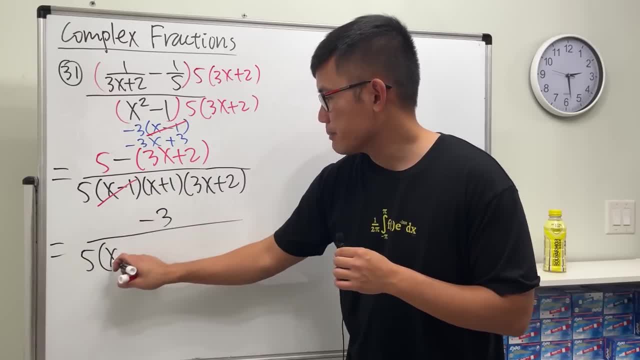 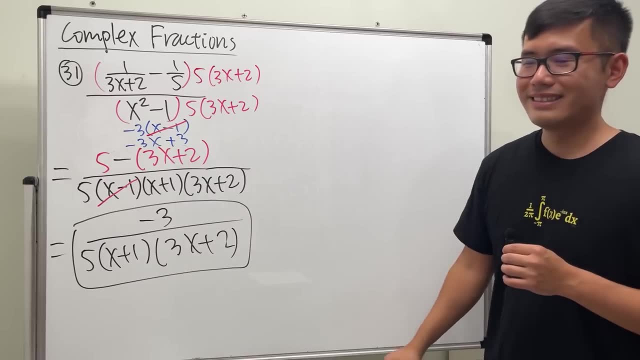 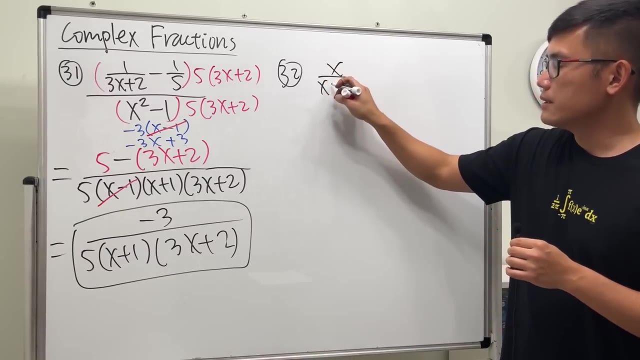 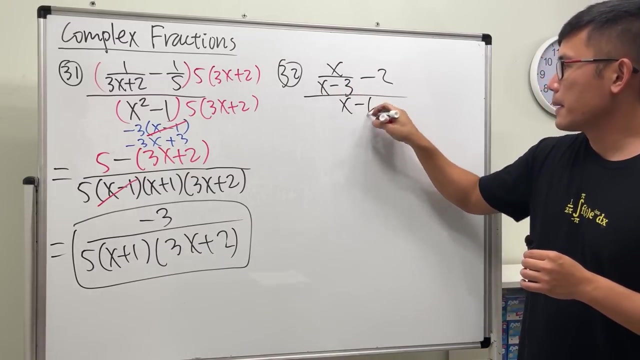 over. this is five times x plus one times three, x plus two. and then we are done and hit four, of course, number 32.. all right, x over x minus three, and then minus two over x minus six. so similar thing. let's go ahead and just multiply the top and bottom by. 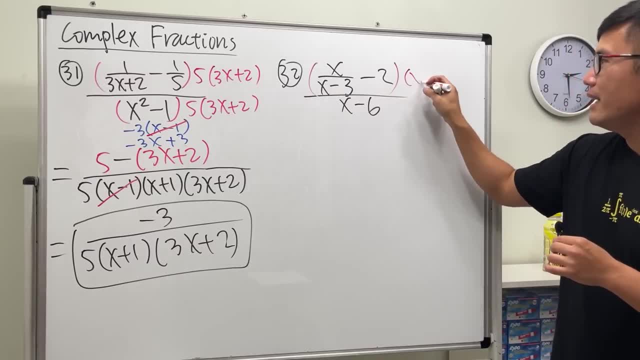 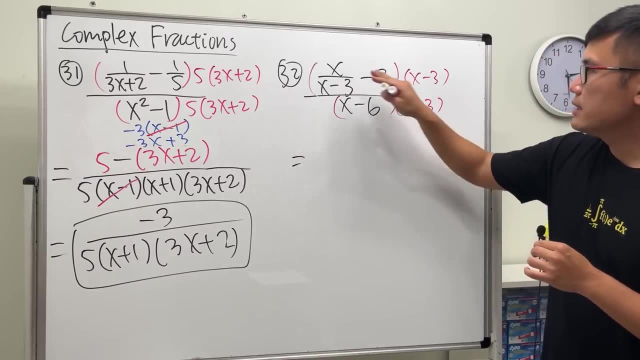 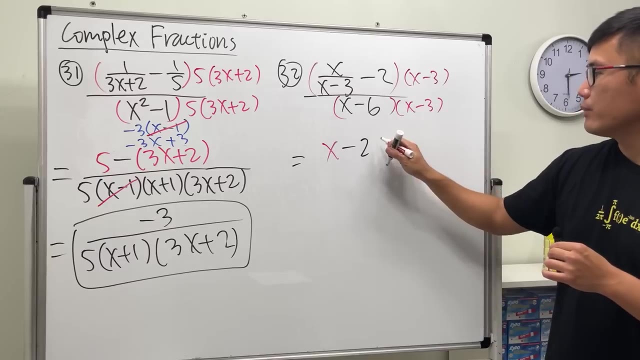 well, this is just a two, so we just need that, namely x minus three, x minus three. okay, when we take this times that they cancel, so we just have x first and then we have the minus. here we have the two. we will have to multiply by x minus three, right, this times that. 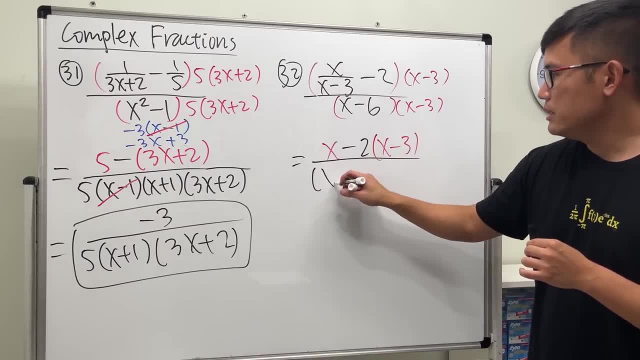 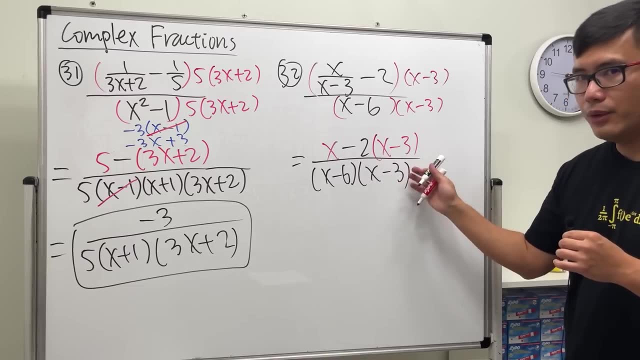 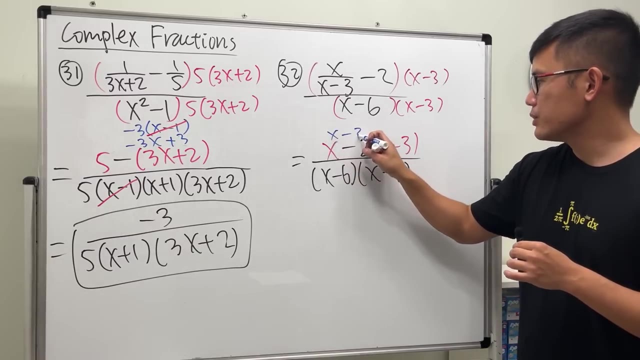 and then the bottom just leave it. so here we have parentheses, x minus six times x minus three again. do not cancel this and that. i know they are both in the parentheses, but we really have to work it out first. so this is x minus 2x plus 6, yeah, and then this is actually just negative x. 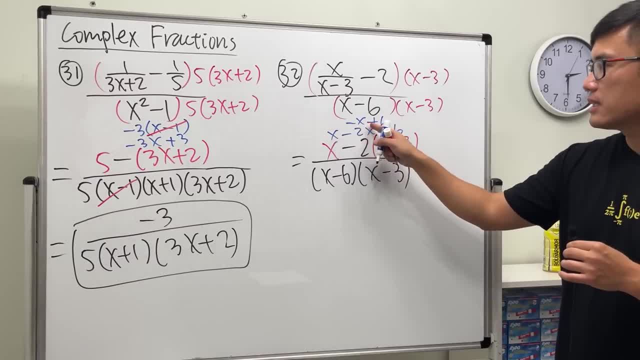 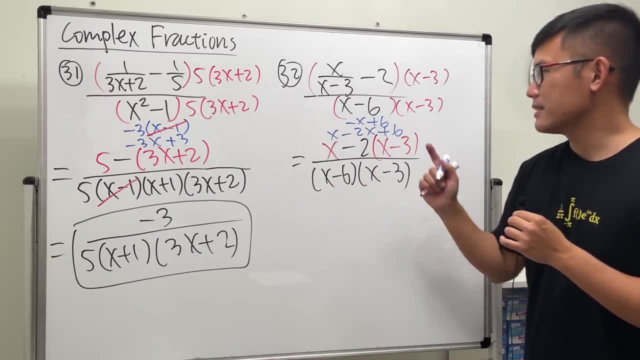 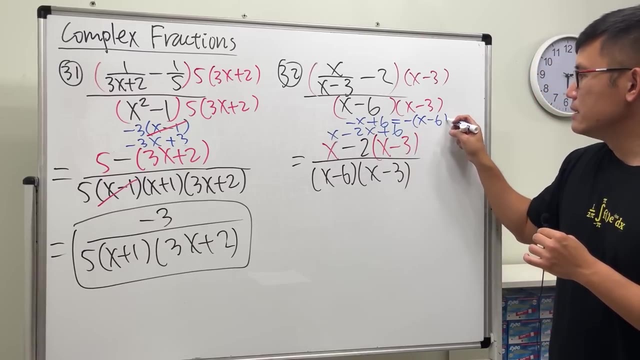 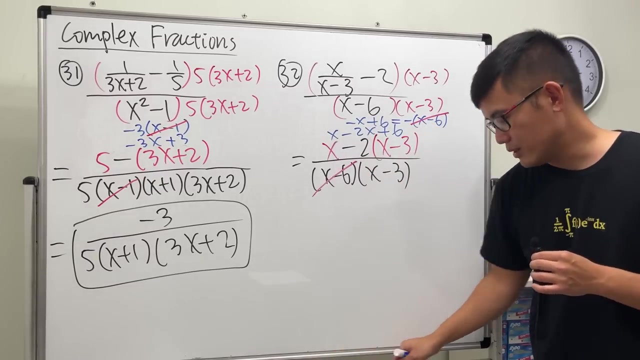 plus six. okay, so this is negative. x plus six. this is six minus eight. this is negative: x plus six six: this is x minus six. what can we do? well, this right here is equal to negative x minus six. we can factor our negative right and then this x minus six, and that x minus six can be cancelled. 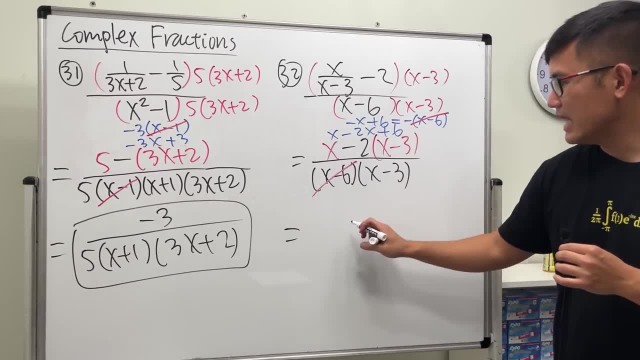 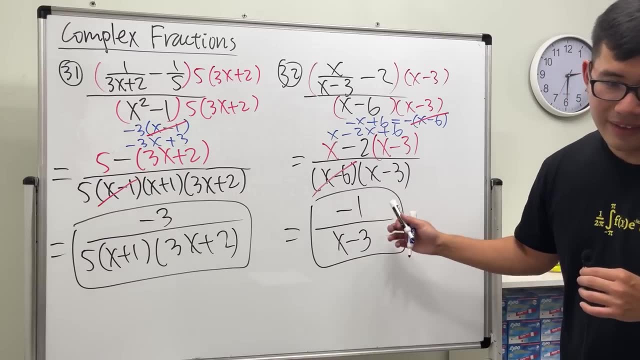 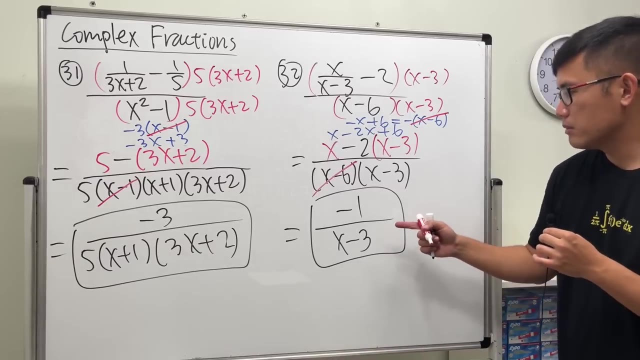 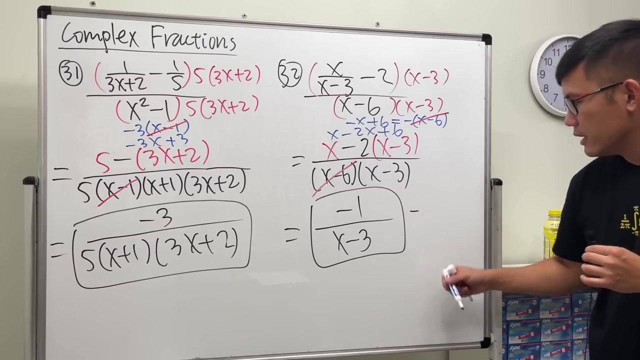 it very nicely. so we have a negative on the top over x minus three. so that will be the final answer: negative one over x minus three. and some people might notice sometimes, if you they want to put a negative on the bottom, they can do this and i'll put this down in blue. if you want, you can put a negative on the bottom. 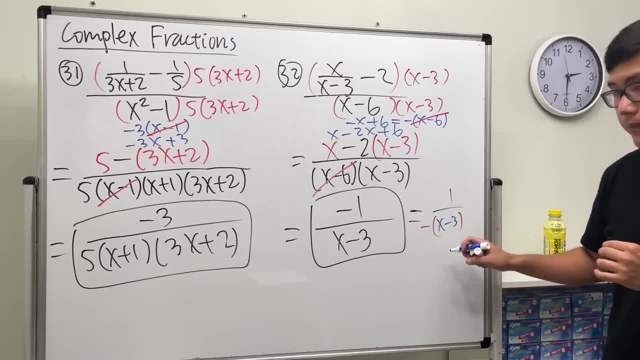 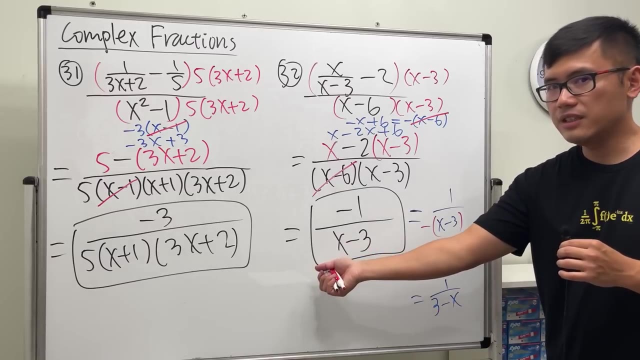 because negative parentheses. and then x minus three. you can distribute it. you can one over negative. x plus three. you can change the order as three minus x or another way to look at it refers this order: you get a negative, negative cancel. with next negative, you get one over three. 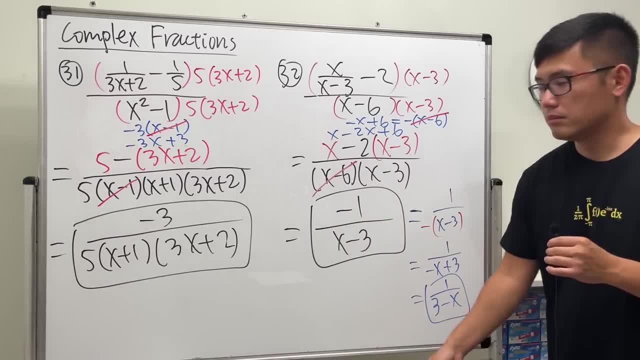 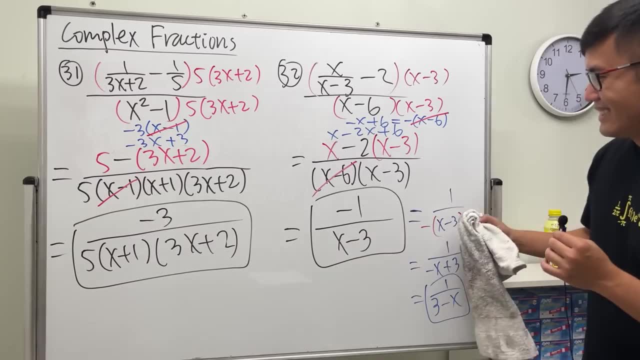 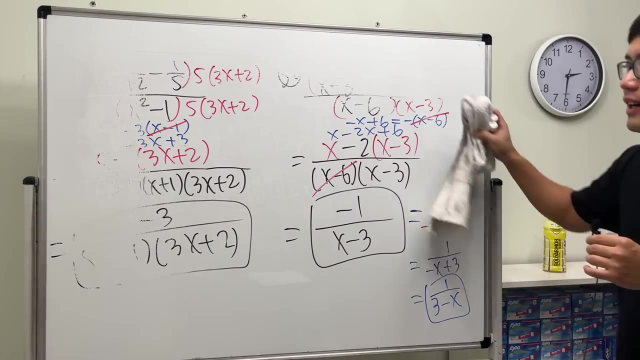 minus x. so this, what that? yeah, usually we like to have the x goes first. usually- like most of the time actually, not just usually- okay, so that's number 32.. you guys notice that to have a drink ready over here, i will take a drink, um, once we finish the complex fractions. 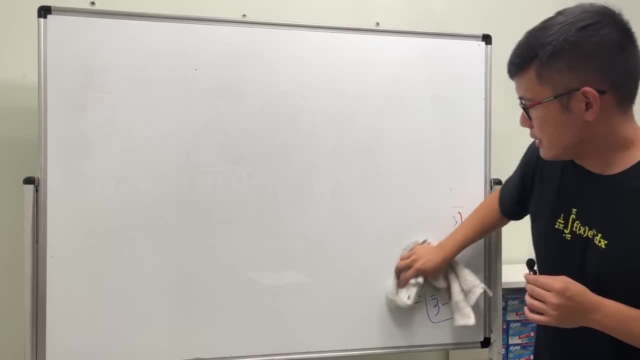 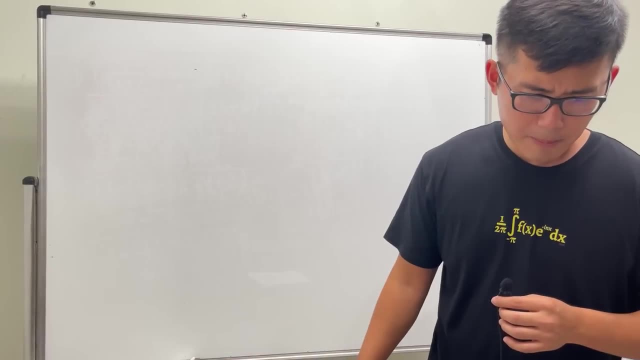 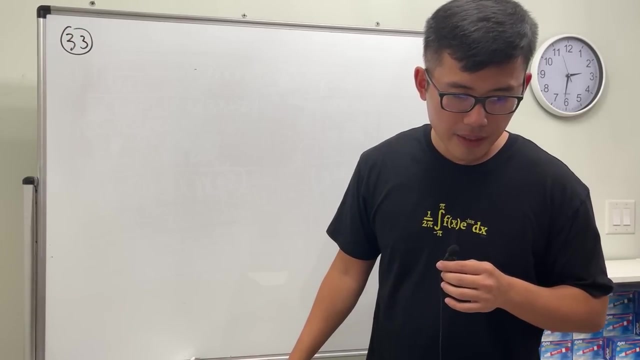 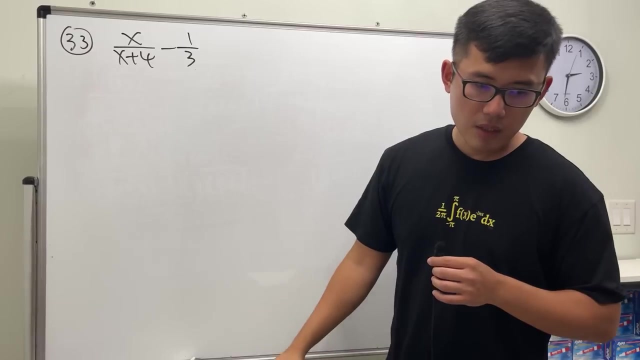 number 32, number 33, so number 33. we have x over x plus four minus one over x 3 and over x minus two. all right, now let's take a look at the quantum arithmetic. let's check out the common denominator. okay, let's take a look at the common denominator. 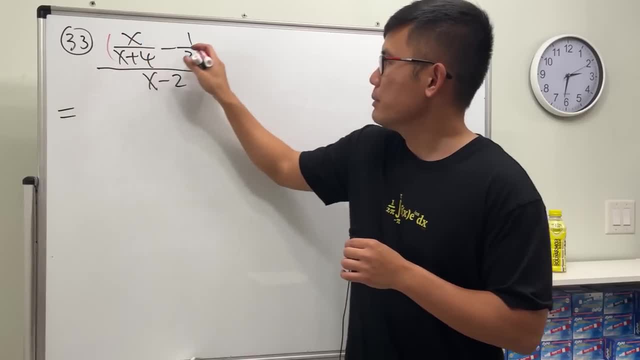 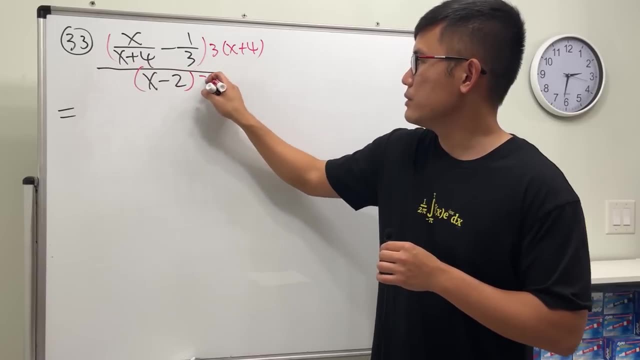 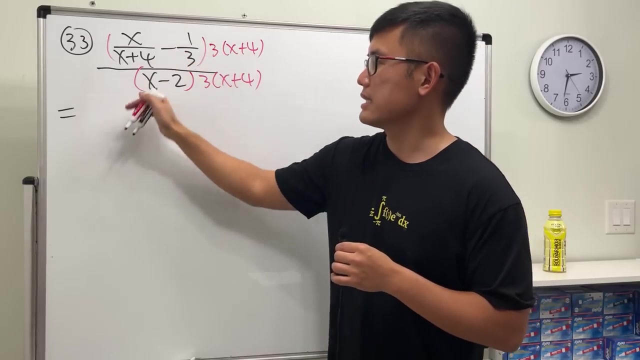 let's take a look at the common denominator. go ahead and get to work. multiply the top and bottom by this and that. so three times x plus four, all right. so multiply this by three times x plus four. take this times that the x plus four cancel. three x goes first and then hold on. let me just write it down right here, just right here. 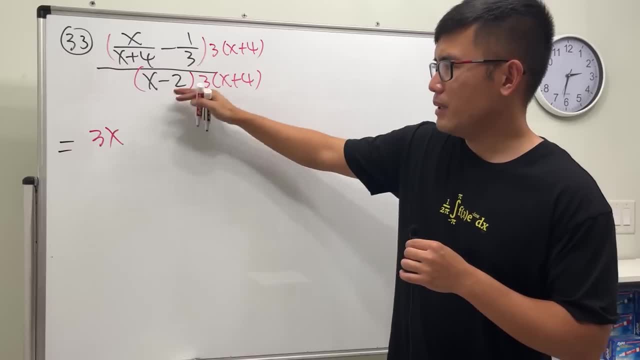 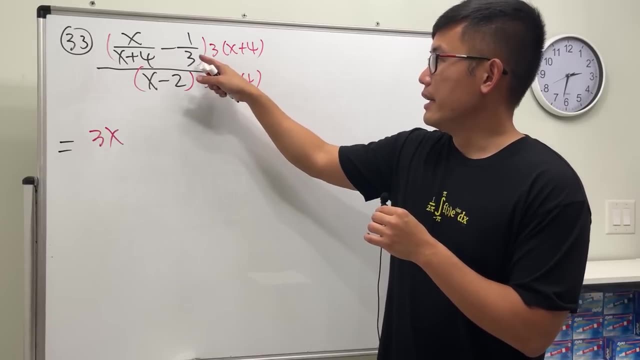 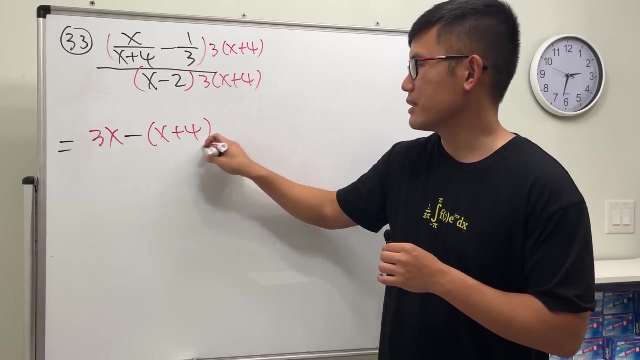 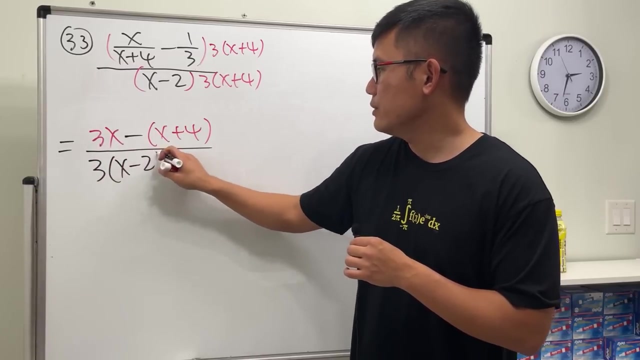 equals three, x. leave some space so that you can like do some computations above. it easier that way. and then minus three and three, cancel, right. and then we just have the x minus four. x plus four, sorry, yeah, all right. and then right here, let's just put a three first and then x minus two. 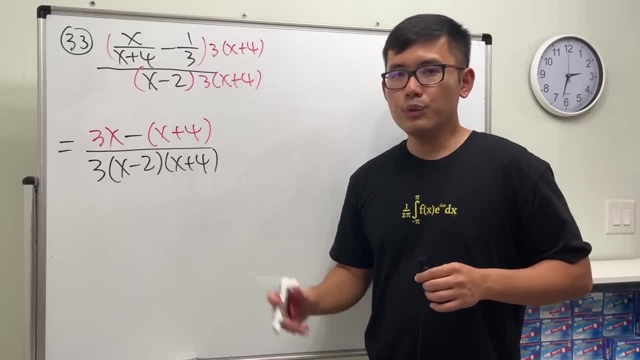 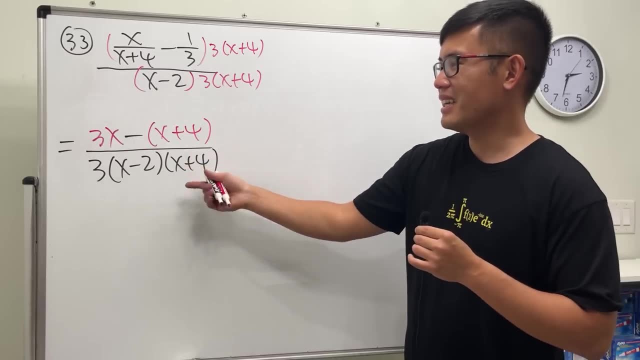 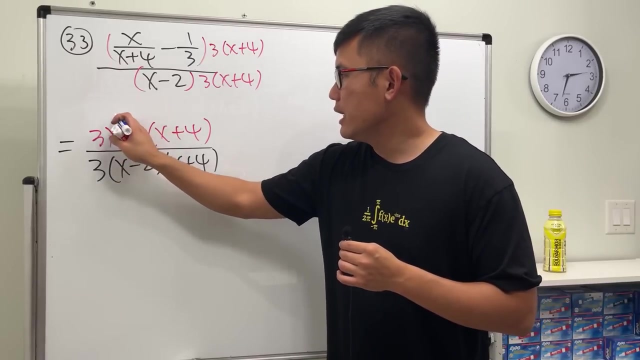 and then x plus four. so you see, once you simplify this complex fraction, this is just to make it easier for us to understand how to solve this problem. so we're going to do some expressions. these kind of expressions that we saw earlier just shows up naturally, like this and that, but don't cancel them out. work out the top first. 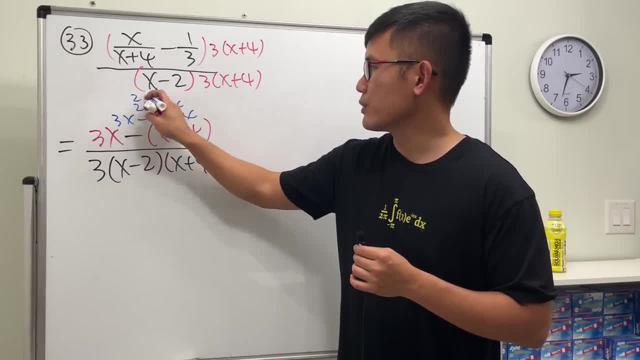 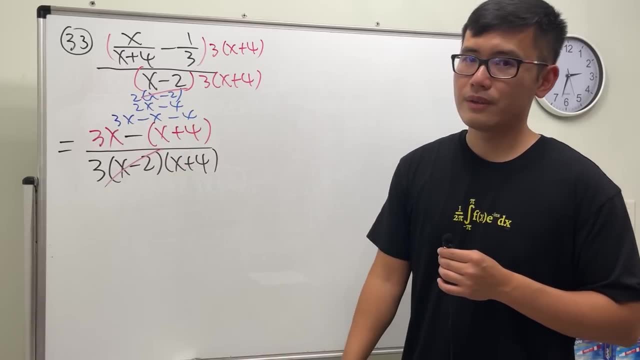 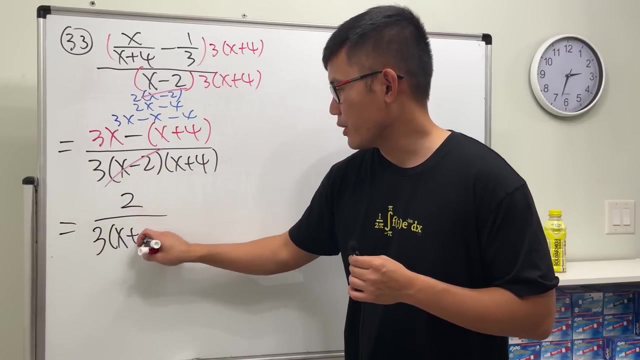 so this is three x minus x minus four, which is two x minus four, and can factor out two. so two x minus two, the x minus two x minus two, cancel over 3, and then x plus 4.. Done, Yay, I don't need to erase that number 34.. 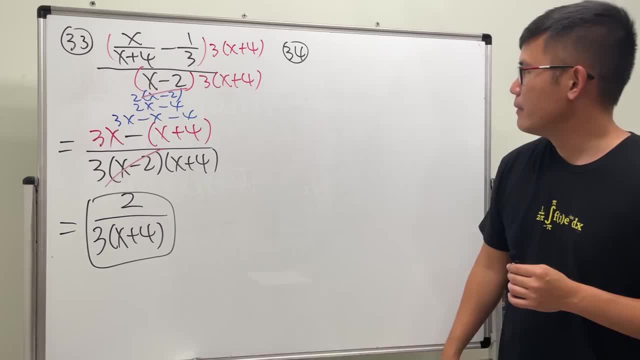 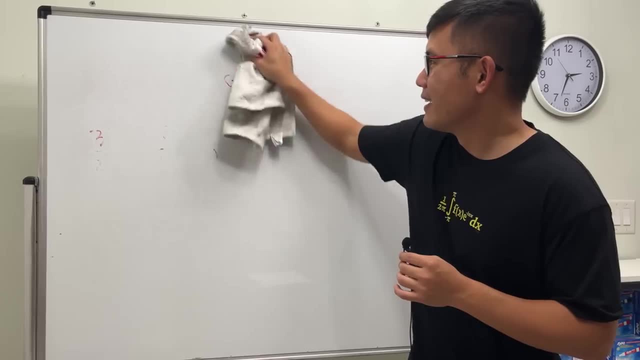 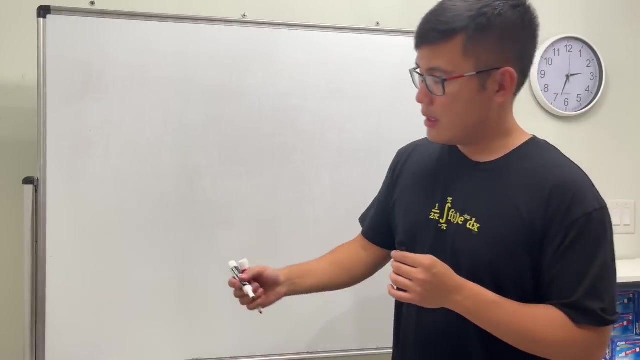 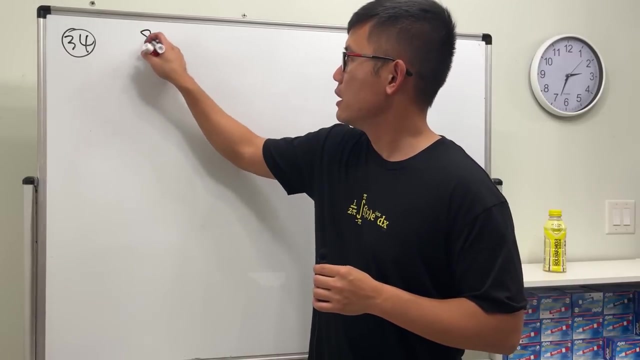 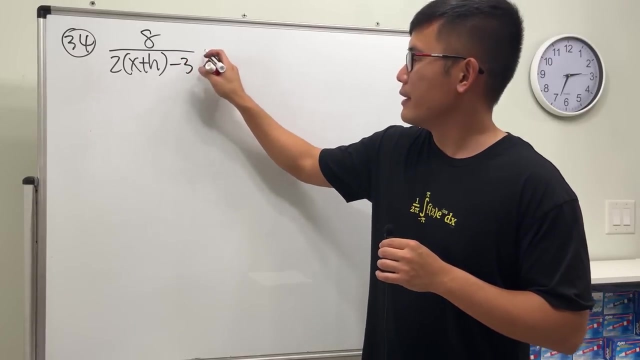 The one with h again. Okay, Me me. no, never mind, I am going to need some space. So 8 over 2 times x plus h, and then minus 3, and then minus 8.. See, this is why I need a space. 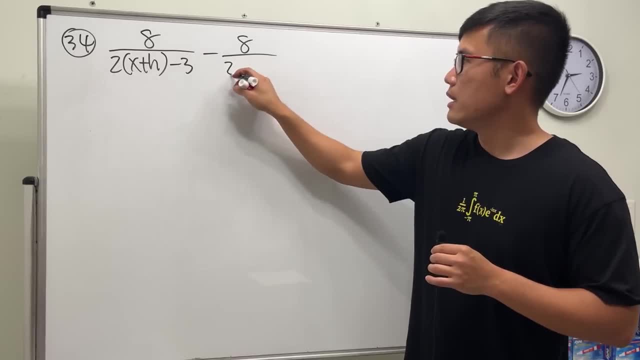 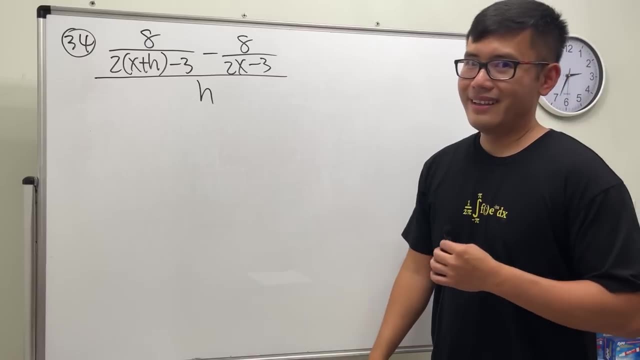 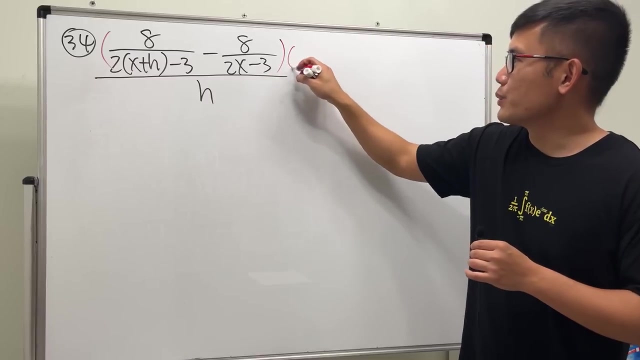 2x minus yeah, over h. Whew. Okay, Here we go. Multiply this by this and that, So I'll put this down first, which is 2x minus 3.. And then, for this guy, let's just multiply it out, right. 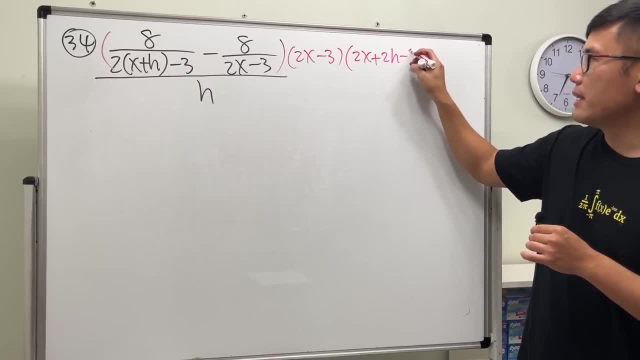 So that's going to be 2x plus 2h and then minus 3.. And then let's go ahead and do the same thing here: 2x minus 3, and then 2x plus 2h minus 3.. 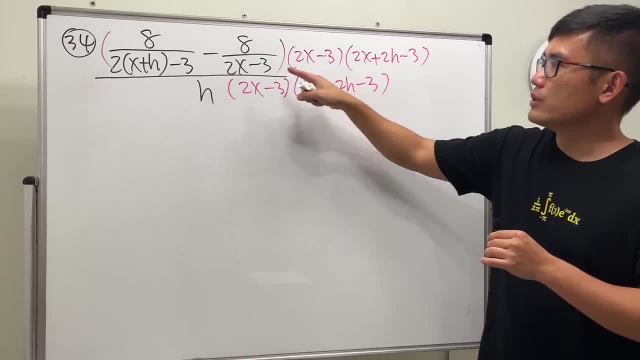 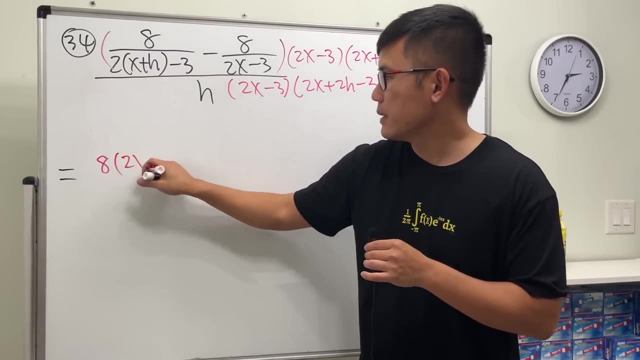 Take this times that this and that cancel. so we have 8 times that right. So perhaps I'll write it down right here: 8 times 2x minus 3, and then I'll distribute it later. Next we have the minus. 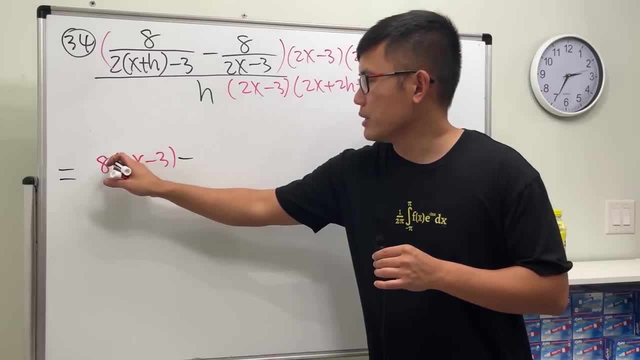 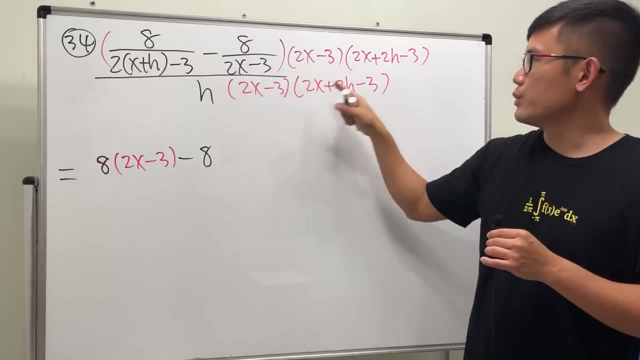 This is the 8. So perhaps I'll put the 8 in black from the original And then we also have this 8. This times that this and that cancel. so we have this, which is 2x plus 2h minus 3.. 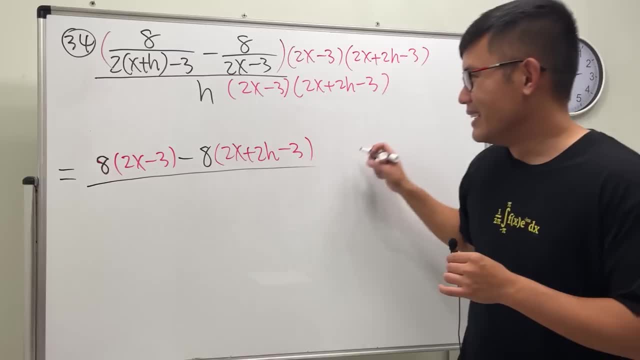 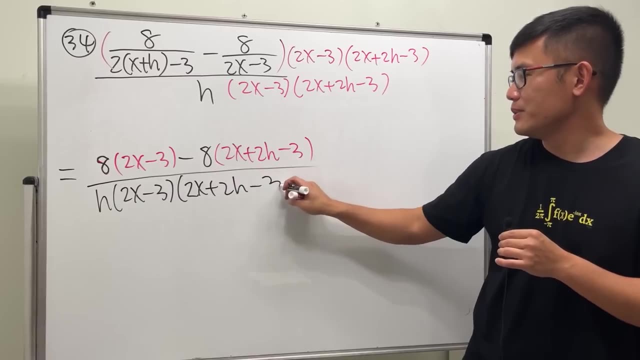 I feel like working out my art, Yeah. And then right here we have 8. h times 2x minus 3, and then 2x plus 2h minus 3.. Let's just go ahead and multiply this out. 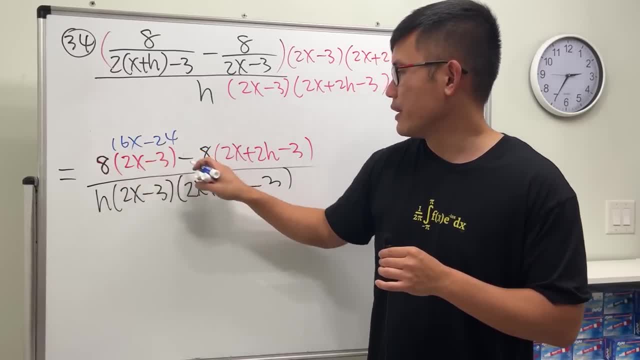 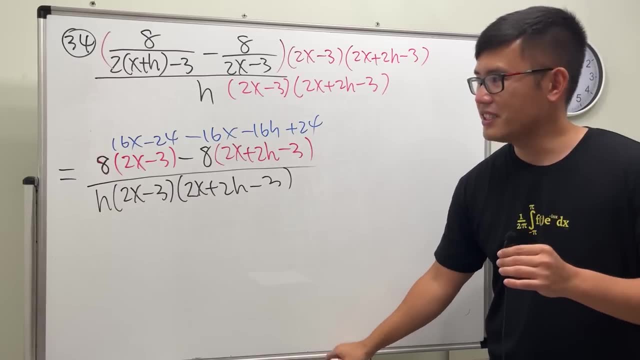 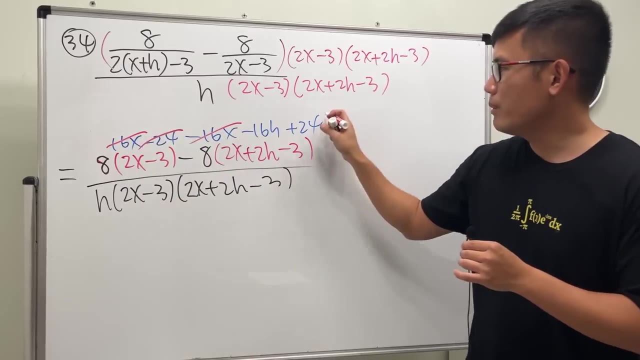 So this is 16x minus 24, and then minus 16x, minus 16h, and then plus 24.. And check this out: 16x minus 16x, Minus 24, plus 24.. This is negative 16x. 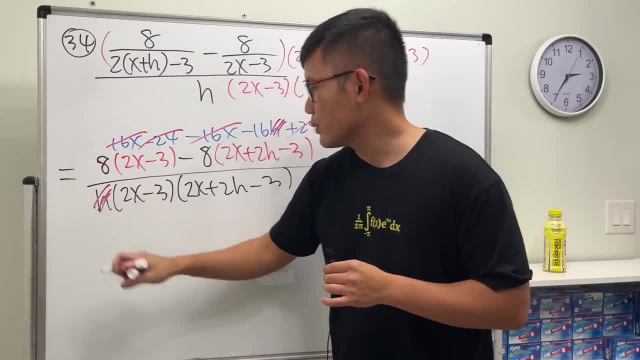 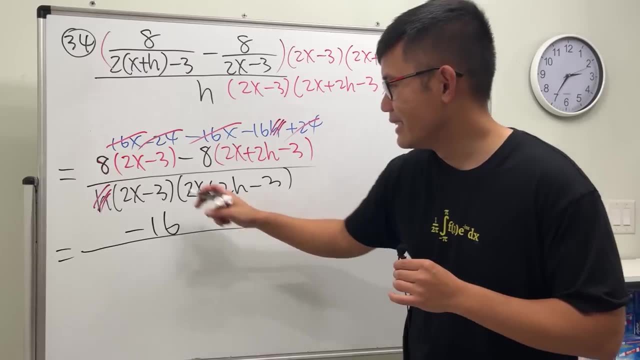 16h left. This h can be cancelled here with that. So on the top we have negative 16.. Wow, Over Here we have 2x minus 3 times 2x plus 2h and then minus 3.. 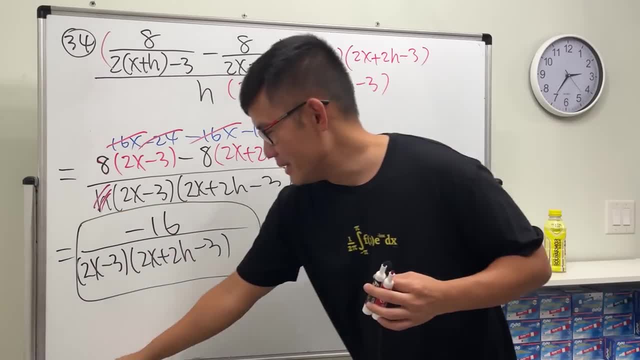 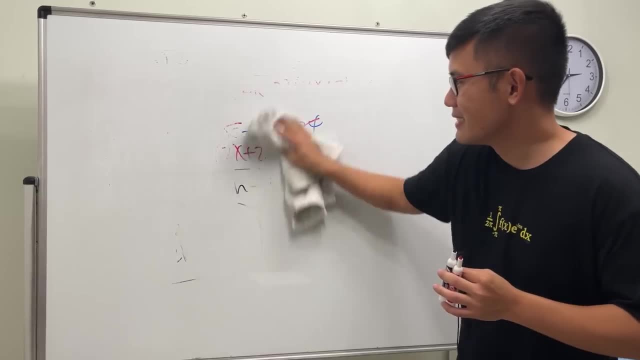 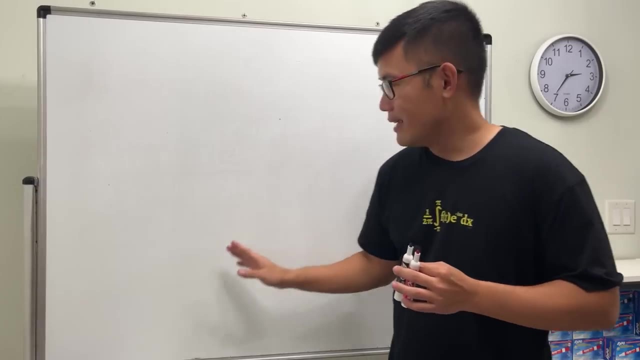 Done. Not bad, seriously, It's not so bad. It's just a lot of variables that you have to just keep writing them, writing them, writing them. And you see I'm doing this with you guys, okay, Yeah. 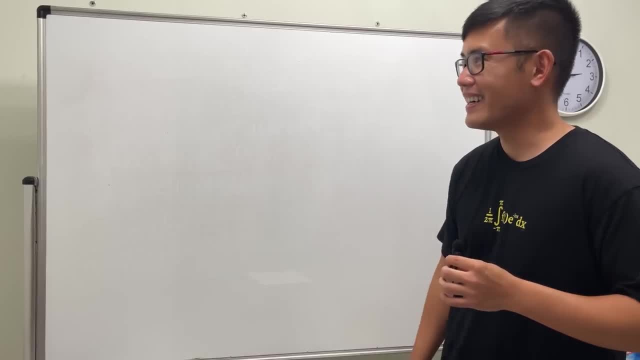 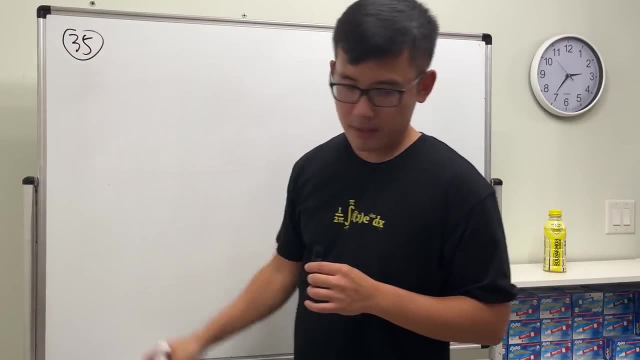 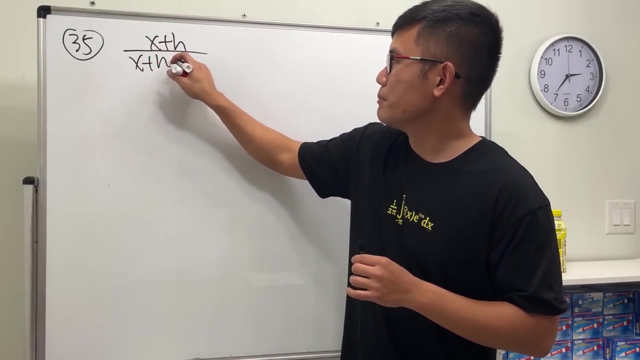 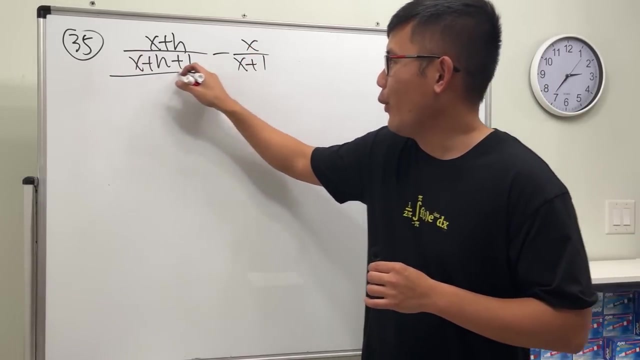 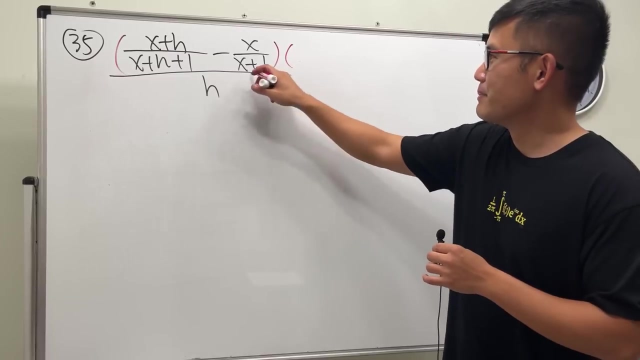 The main thing is: how much are you willing to do for your own good right Number 35.. x plus h over x plus h plus 1.. Minus x over x plus 1 over h. All right, Multiply the top and bottom by this and that. 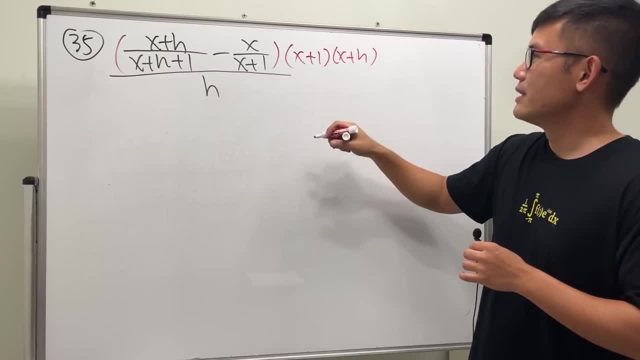 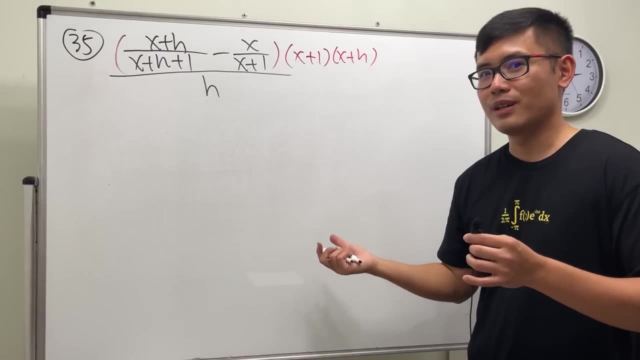 So x plus 1, x plus h, Okay, Okay, I will do one more of this and then later on I'm just going to show you guys like how to deal with the count you get. We will skip this step. 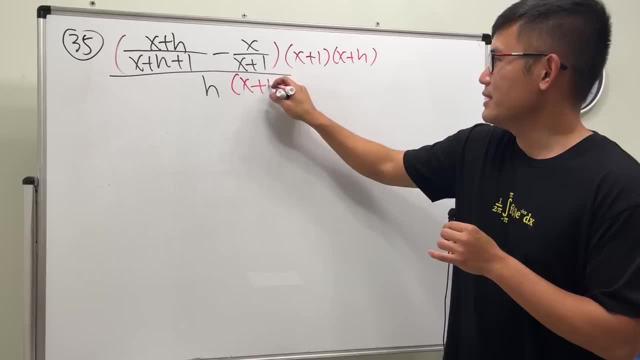 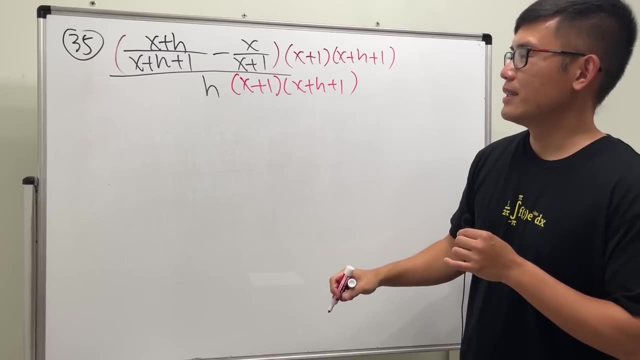 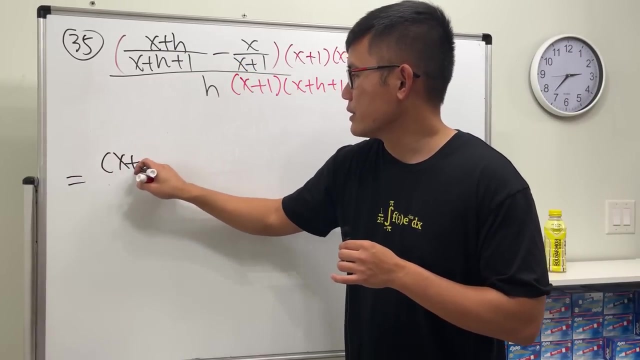 Just do the same ahead. All right, So this is x plus 1.. And then x, And then x plus h, And then plus 1.. All right, Cool, Take this times that This Cancel. So we actually have the original is x plus h times the x plus 1.. 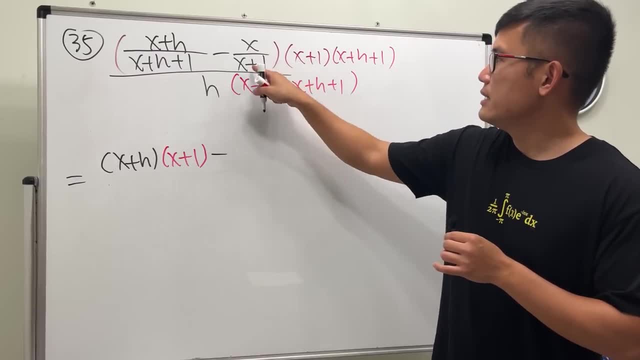 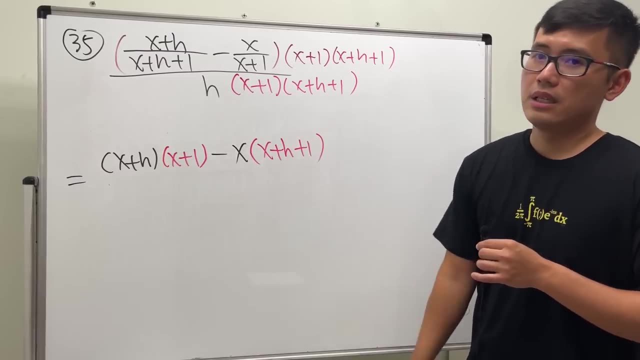 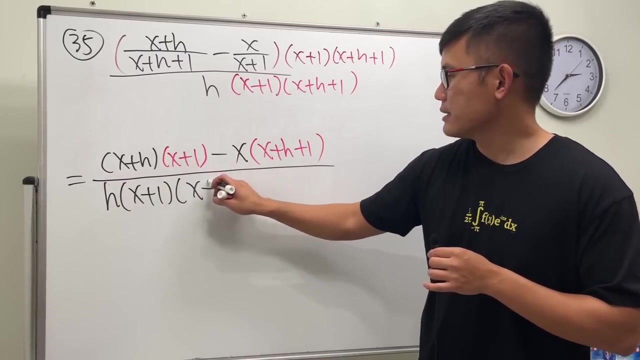 All right, And then we have a minus, And then this and that cancel. We have the x right here. times all that. So it's x plus h plus 1.. Over h x plus 1, x plus h plus 1.. 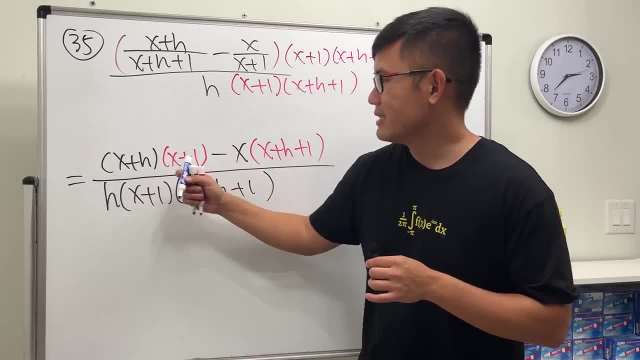 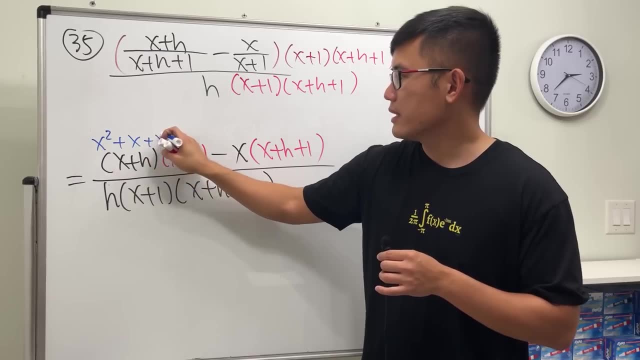 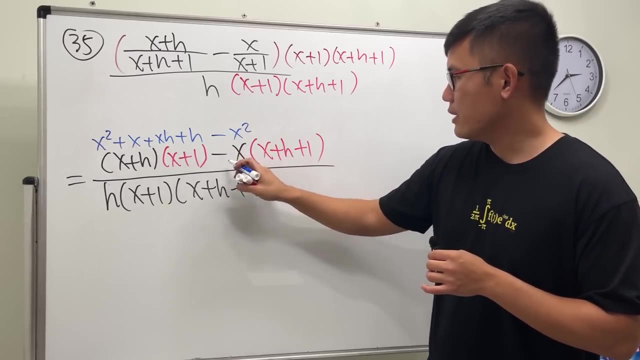 Okay, let's just do it This times: this is x square and then plus x Right. This times that And then this and that is plus x h and then plus h Distribute, We get negative h square and then negative x h. 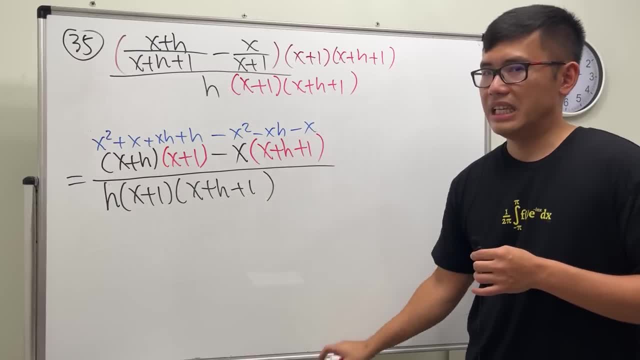 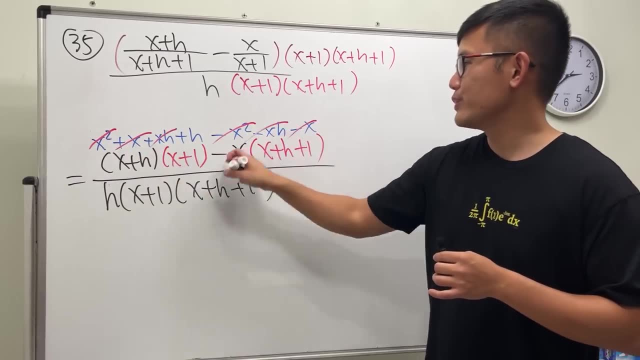 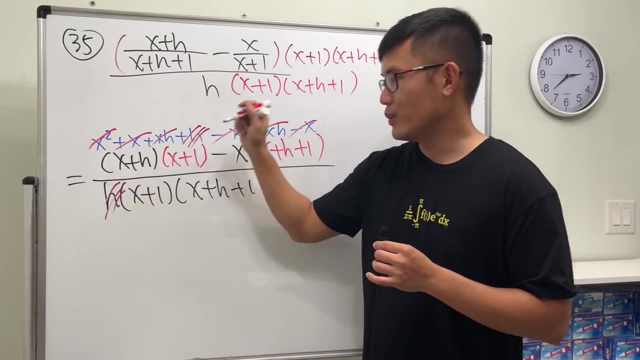 And then plus h And then negative x. Yay, Because this that cancel, x, x, cancel. on the top we just have an h. Cancel them, Cancel them. But don't forget we have a 1 on the top. 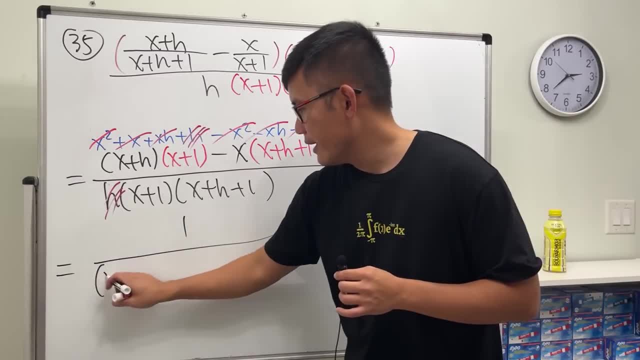 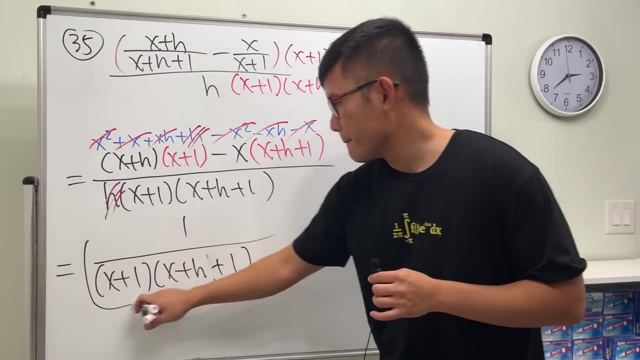 So, ladies and gentlemen, it's 1 over x plus 1 times x plus h plus 1.. Okay, All right, All right. Okay All right. One, two, three, four. Let's do it one more time. 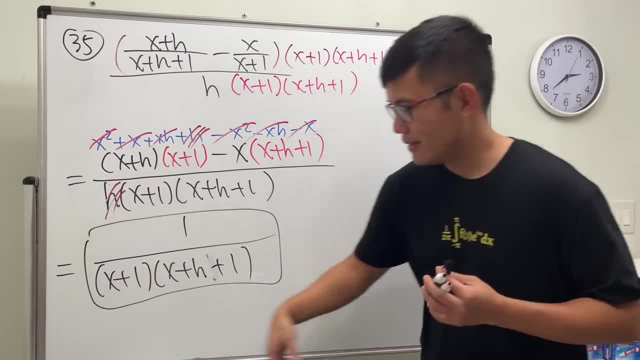 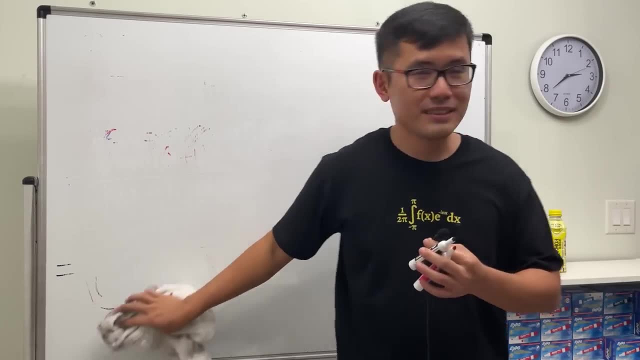 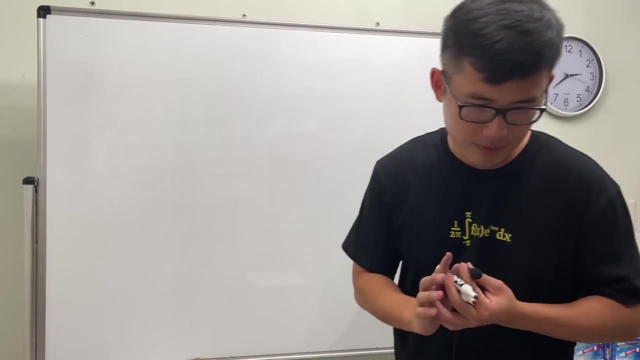 One, Two, Three, Four, Five, Six, Seven, Eight, Nine, 10., 11., 12., 13., 14., 15., 16., 17., 18., 19., 20.. 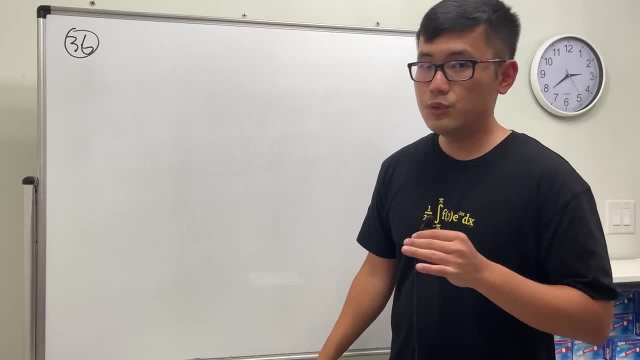 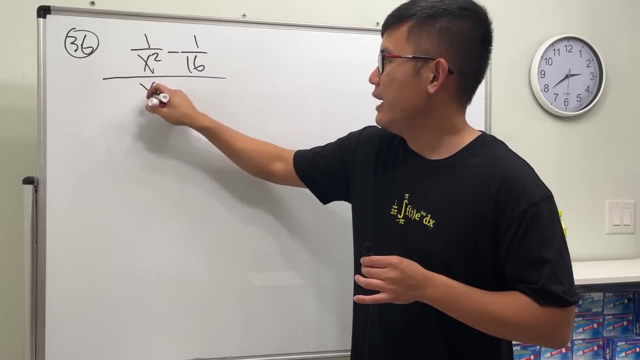 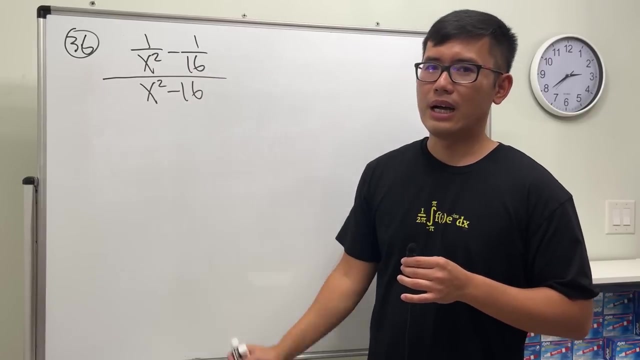 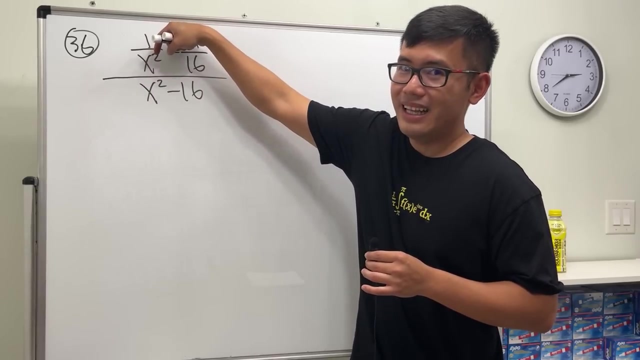 21. 22., 23., 24., 25., 26., 27. 28.. 16 over. x squared minus 16. x squared minus 16. wow, but remember that you see the x squared. it's on the bottom here for this little fraction. likewise, this is also on the bottom for this. 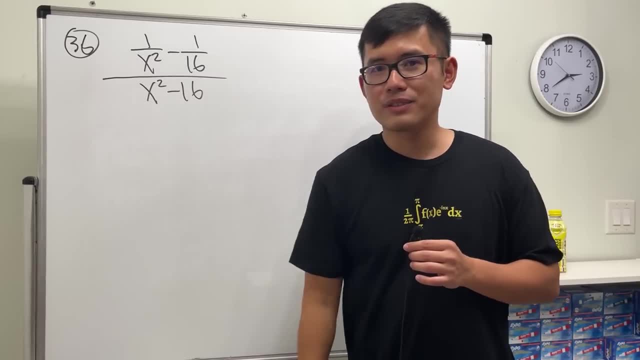 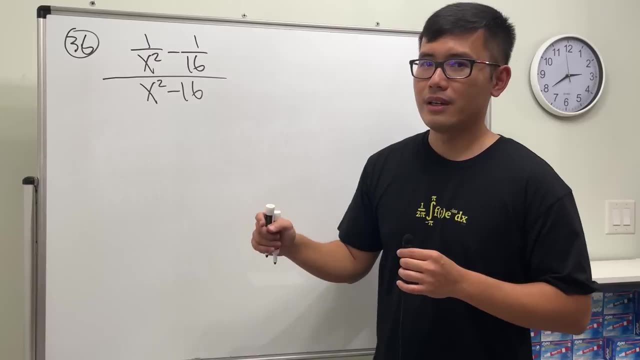 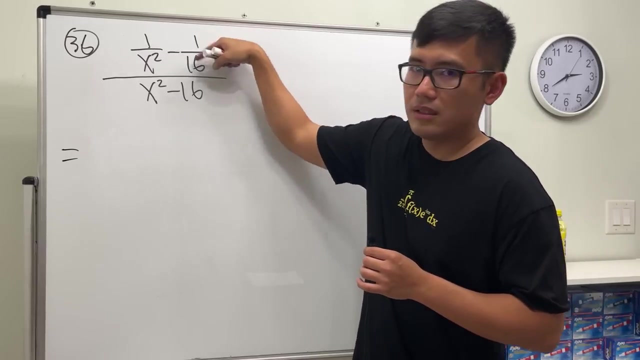 fraction. we have to clear the complex fraction first, and to do so we multiply the top and bottom by the lowest common denominator, which is 16 x squared. and now, this time this- let's do this, i'm not yet- so you pretty much multiply this and that together. that's the trick, right? so 1 times 16 of 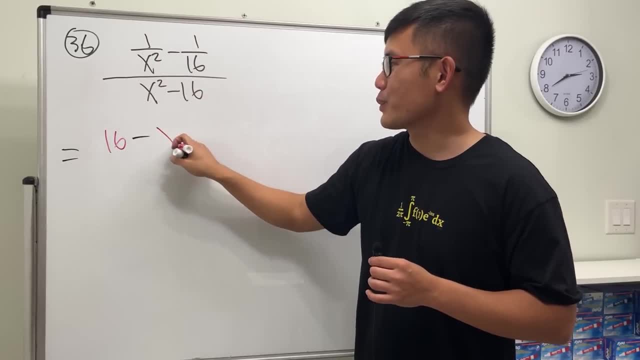 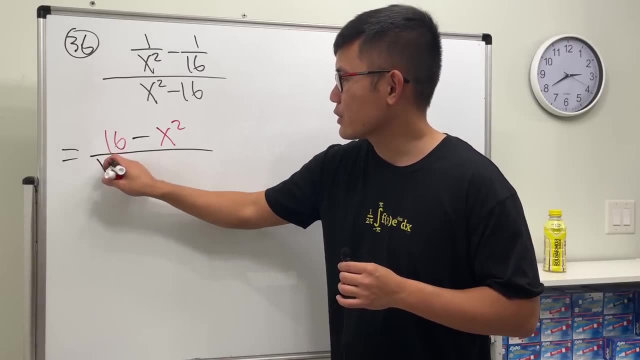 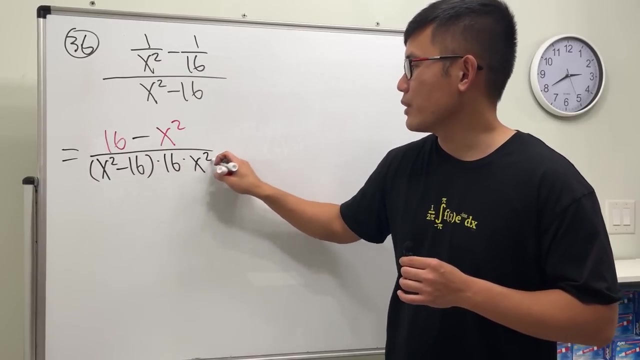 16 and then minus this times that, which is just x squared. yeah, over the bottom you keep it, so you have the x squared minus 16, but you multiply this and that together, which is 16, and also the x squared, like that, and then the dot means just that we are multiplying, okay. 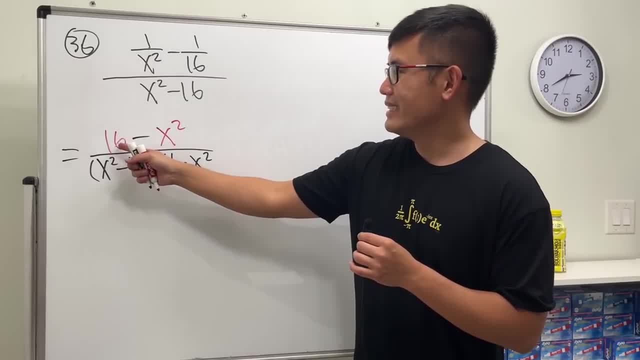 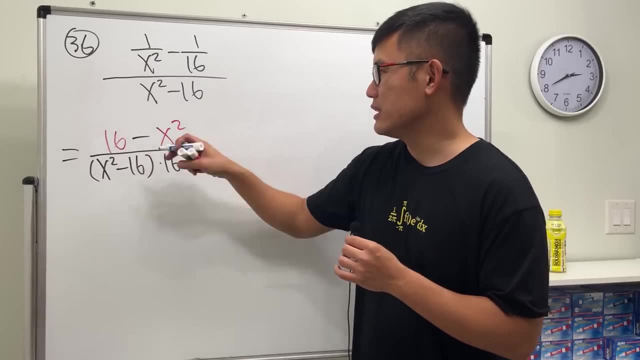 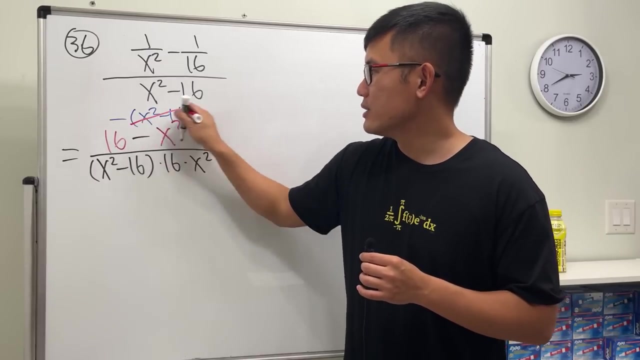 and you know what? you see it: 16 minus x squared, x squared minus 16. in fact, we can just change the water of the subtraction by just negating, so it's a minus, and then x squared minus 16, and we happen to be able to cancel this and that completely. so the final answer is negative: 1 on the top. 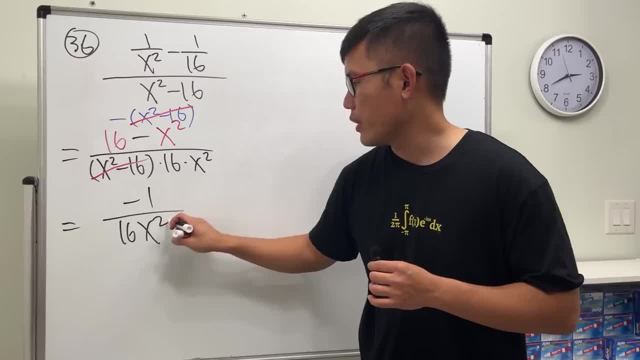 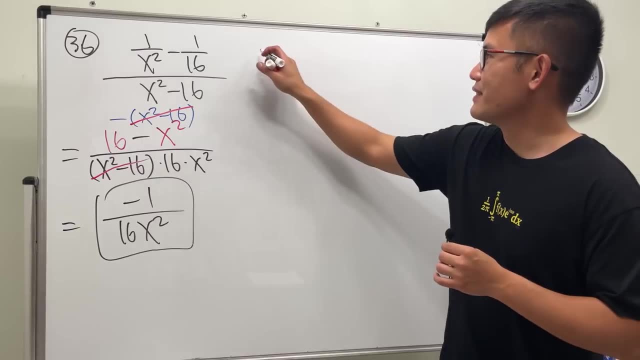 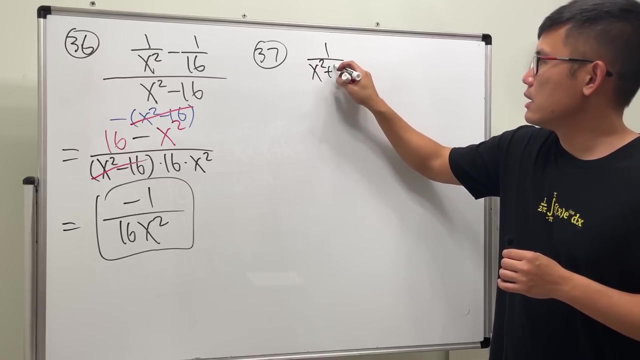 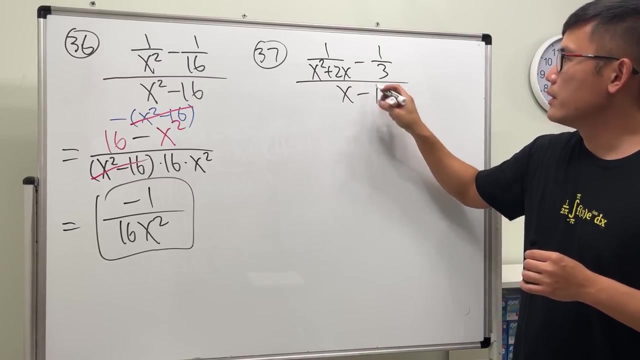 over this and now, which is 16 x squared done, next number 37: 1 over x squared, plus 2x minus 1 over 3 and then over x minus 1. all right, so i'm going to just multiply the top and bottom by the lowest common denominator. 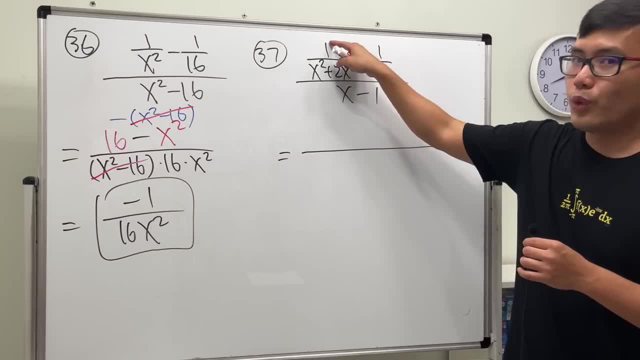 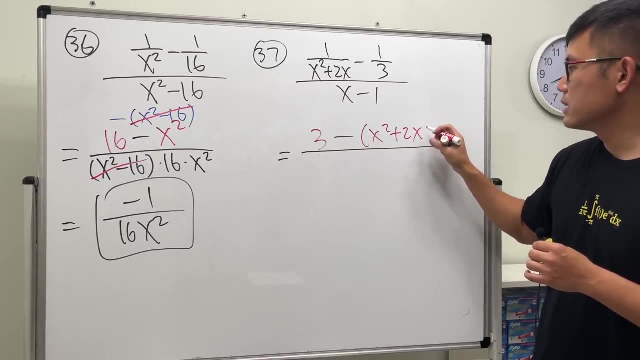 it's going to be like this, to put this right: 1 times 3 is 3 and then minus this times, that is just that, which is x squared plus 2x and then the bottom. here we have the x minus 1. actually, let's put it: 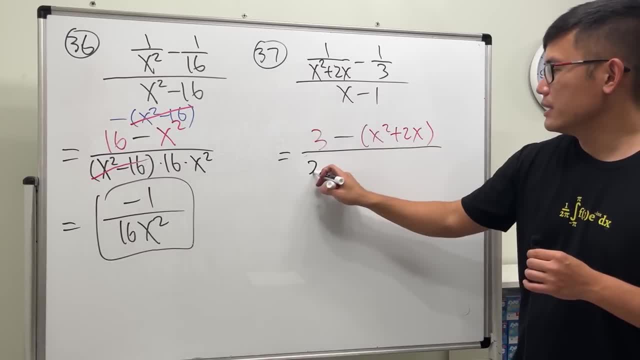 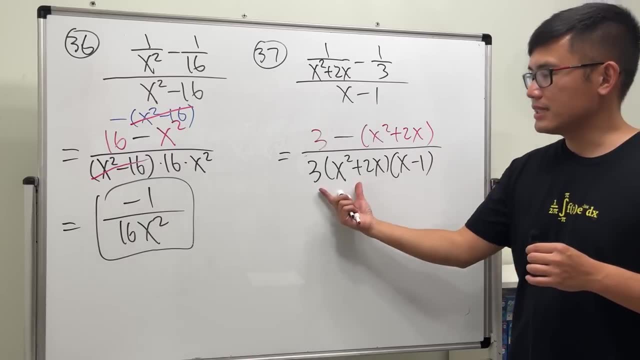 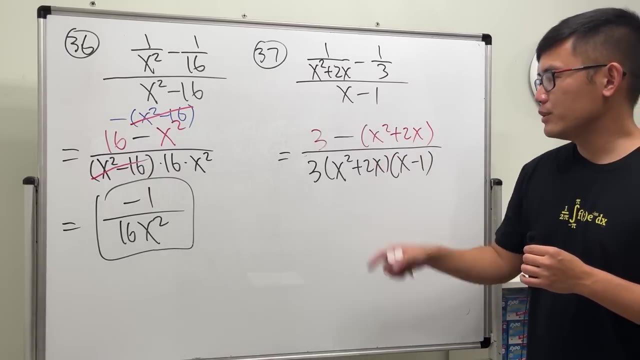 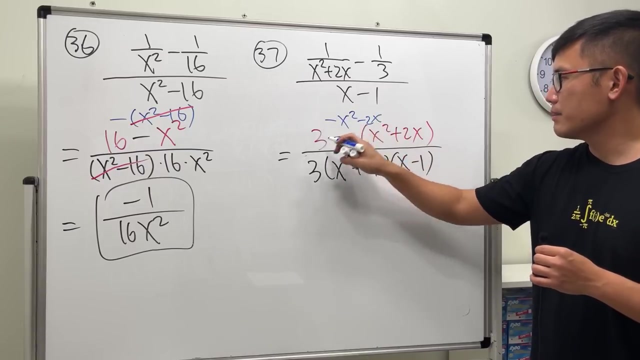 at the end, i'll put on the 3 first, and then that which is x squared plus 2x, and then the x minus 1, and so that's what's the lowest common denominator. okay, so how exactly do we do this? well, distribute this. we get negative x squared minus 2x, and then 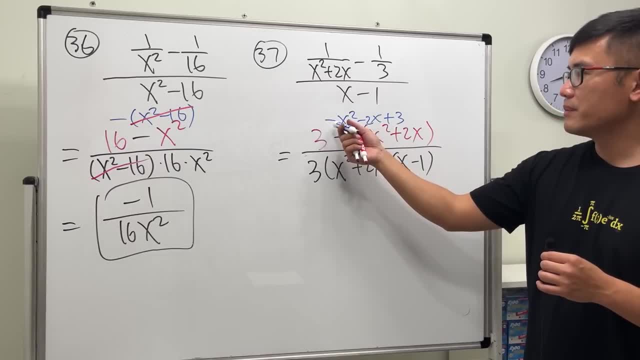 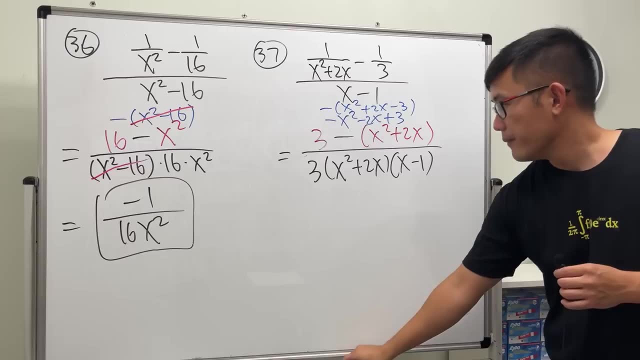 plus 3. we don't like to have this being negative. so let's factor our negative, so it's negative x squared plus 2x and then minus 3. so let's see on the top you have minus, and then we can factor this trinomial. 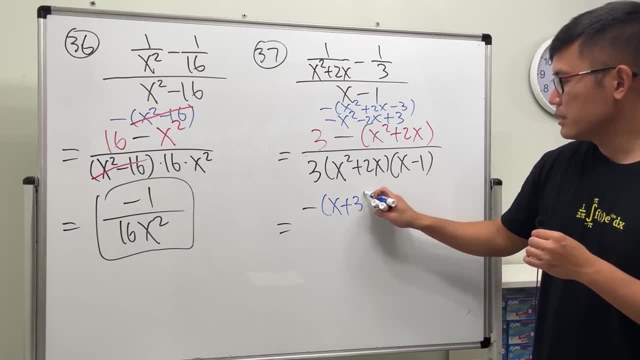 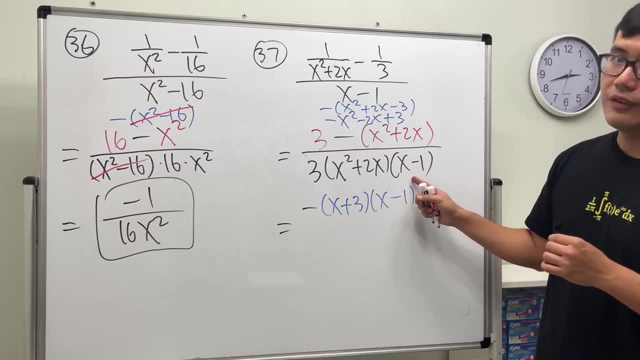 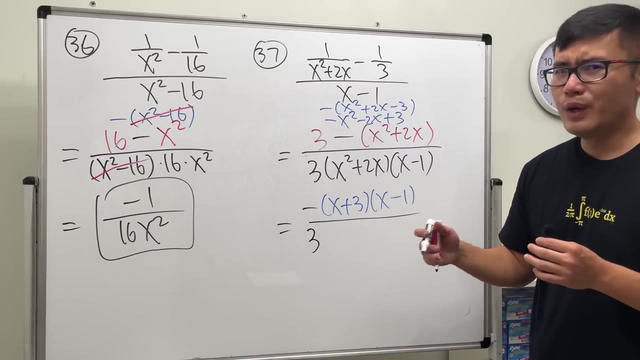 this right here is just x plus 3 times x minus 1. yeah for this. and we notice that here we have the x minus 1, so we can cancel things out and if you would like, you can also factor the denominator, because usually we just like to have the denominator being factored in. 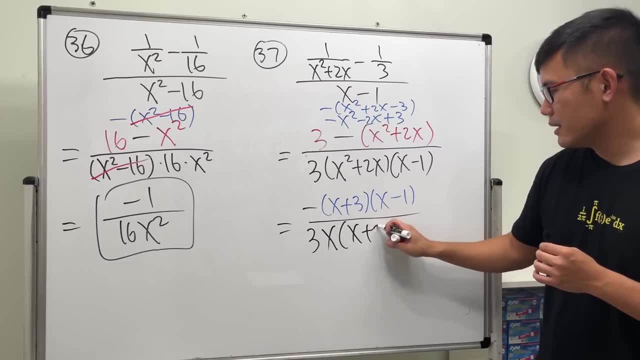 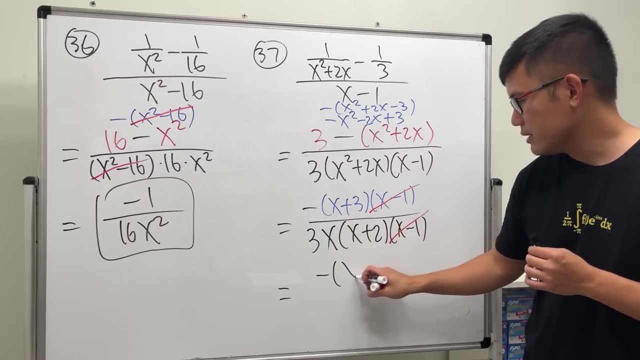 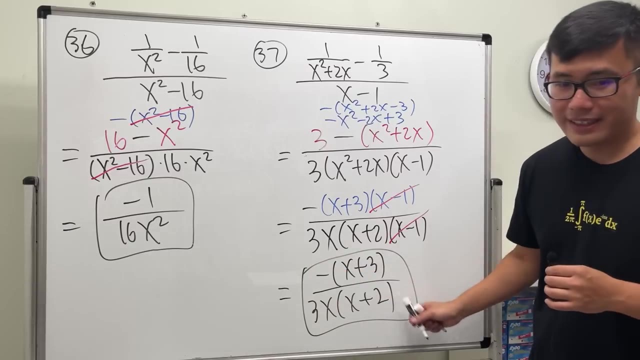 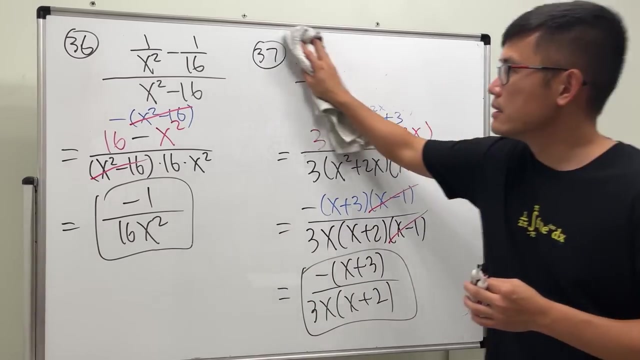 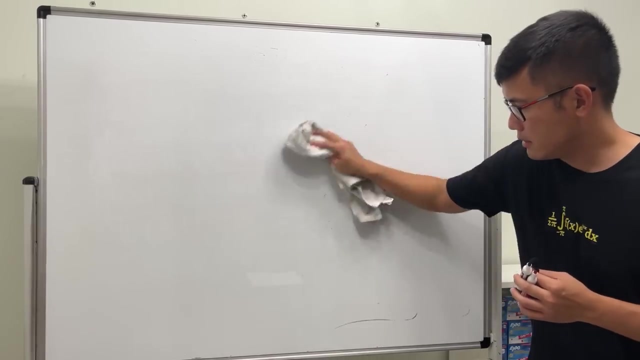 so i will do this, and then i will do this, and then we'll be done. so as negative parenthesis: x plus 3 over 3x times x plus 2.. yay, okay, so a lot of this seriously. just take practice, and i believe you have all seen. 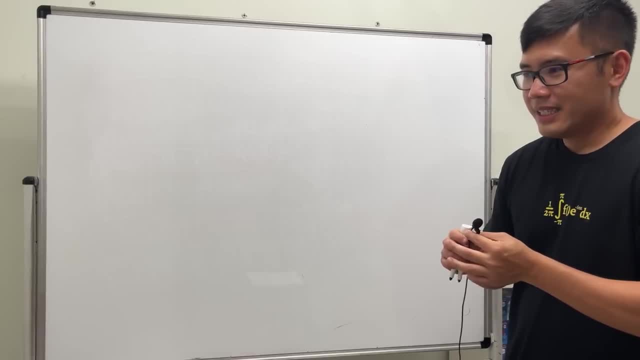 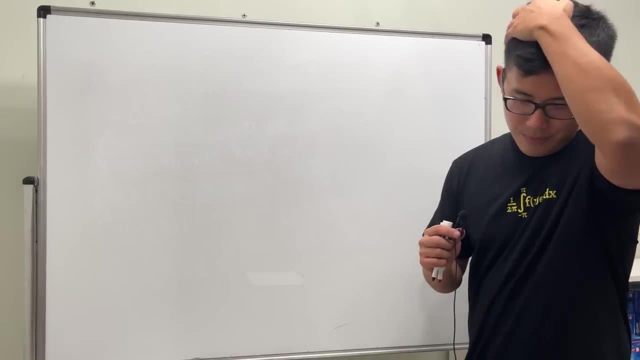 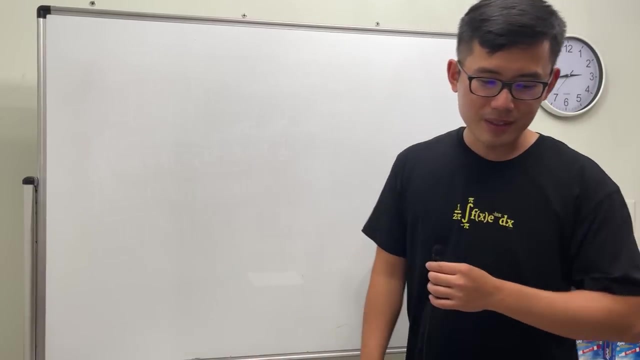 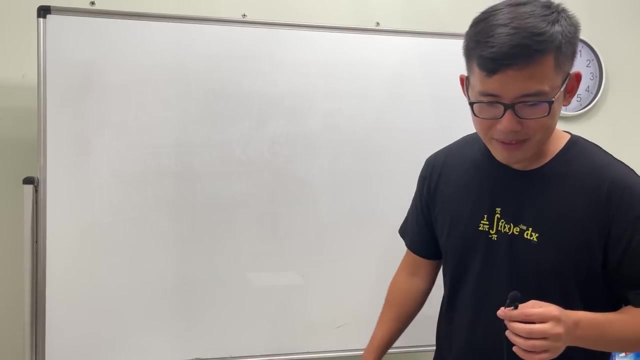 this kind of things before. so that's why i just want to tell you guys the things that you have to be really careful, because i know you know how to do the typical things. that's why we're going slightly faster than the integration video or the road video. oh yeah, number 38. okay, number 38 ready. 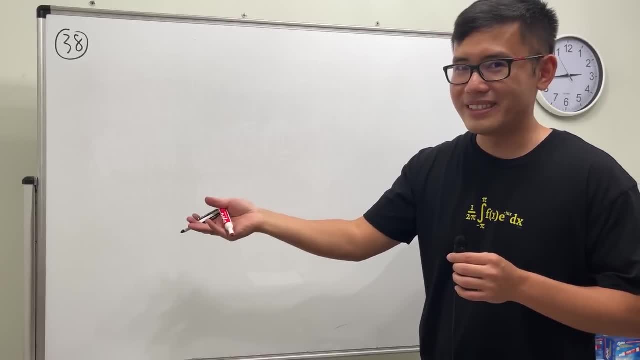 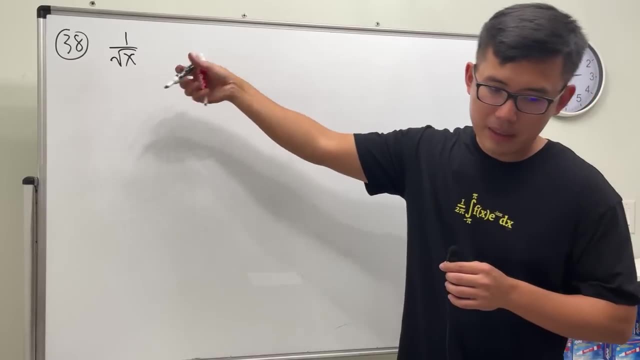 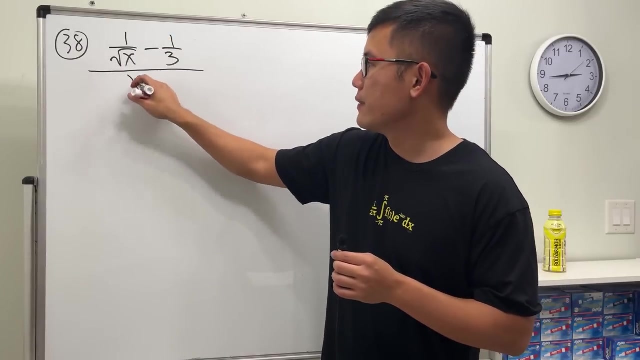 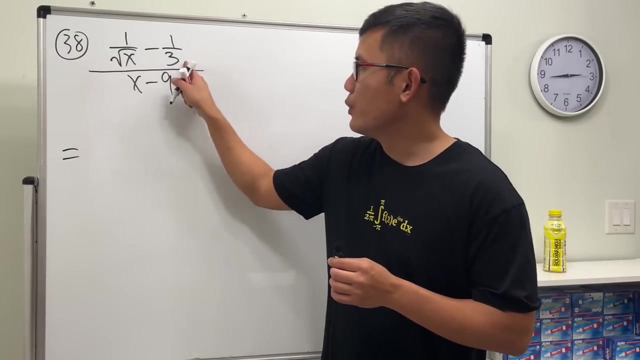 the previous category was the conjugate with the square root. this category is the complex fractions. we have them together right now: 1 over square root of x minus 3- sorry, minus 1 over 3 over x minus 9.. let's fix the complex fraction first. so here we will have 3 times 1, which is 3 minus. 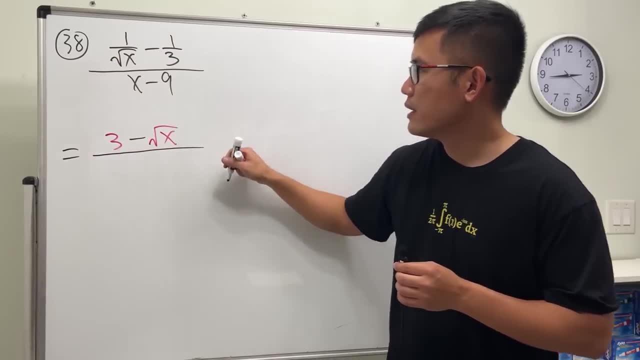 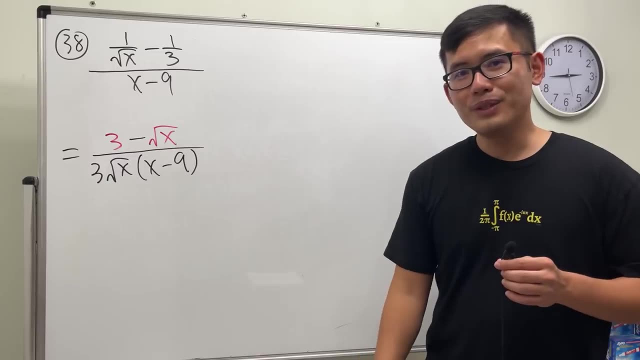 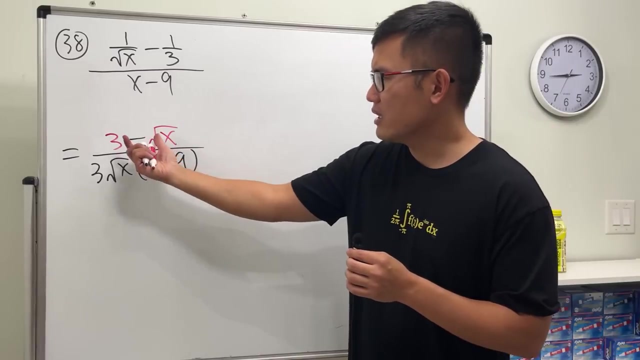 this times that, which is square root of x, over this, this, which is right here, 3 square root of x times that. and what do we do next? you know it, we are going to do the, the conjugate. but this right here again is kind of out of order. so let's fix the water first. so take. 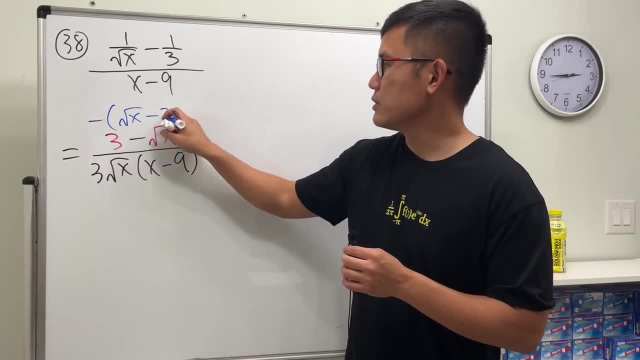 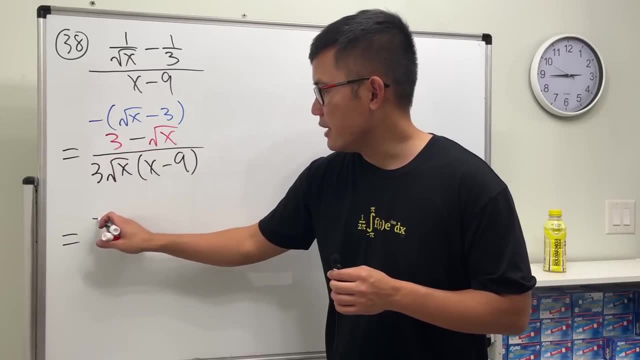 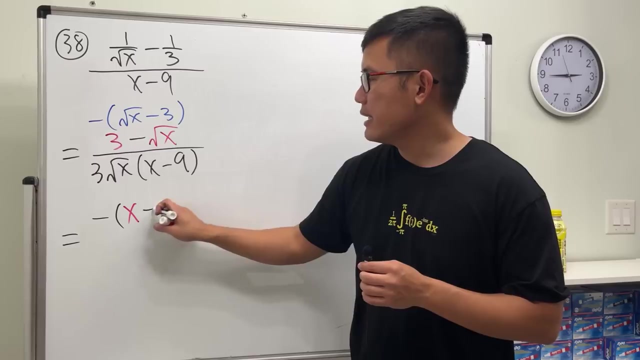 our negative, and then we look at this as square root of x minus 3 and then do this conjugate, so here the negative stays. so if you multiply this with the conjugate, you just square that which is going to give us x, and then minus the square of that which is 9, okay, and then the bottom. here just leave it. 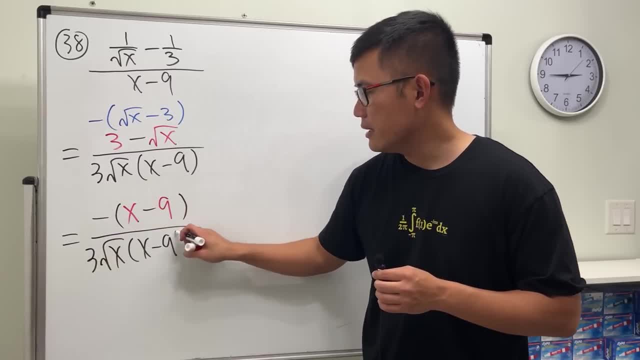 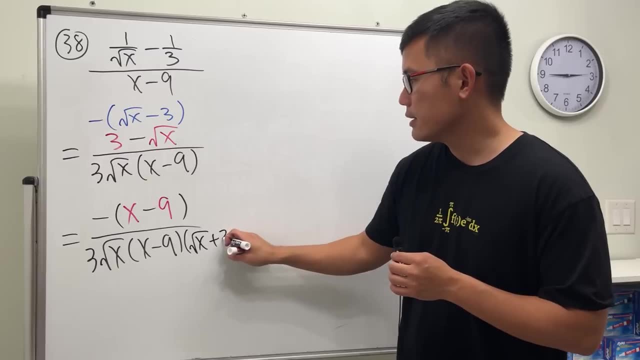 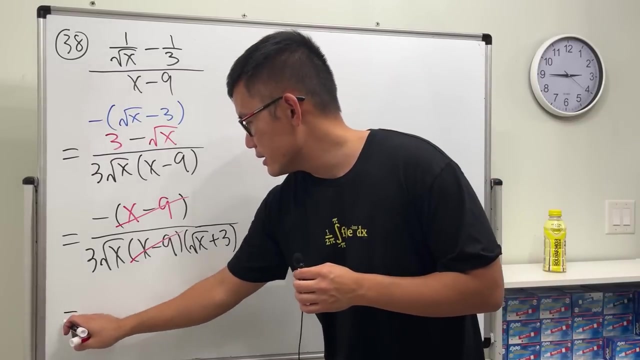 3 square root of x and then x minus 9, but we need the conjugate that we multiplied earlier, right? so the conjugate of that which is the square root of x plus 3, and we see it. this and that cancel. so we- the answer is negative: 1 over 3 square root of x times square root of x plus 3. 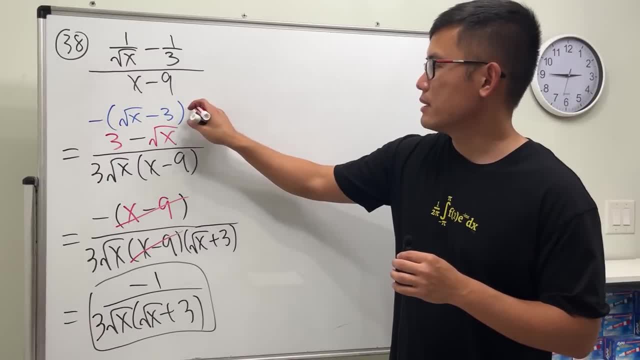 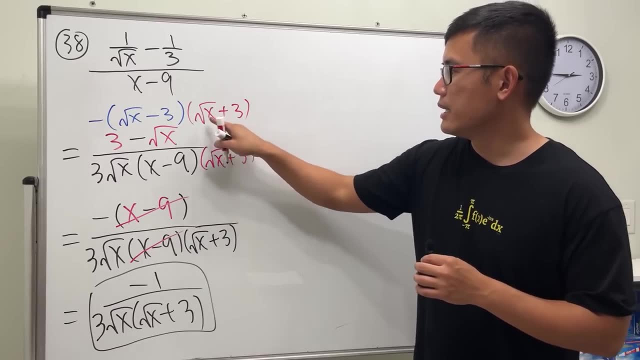 all right. so just like that, and again, just perhaps as a reminder, we multiply by the conjugate square root of x plus 3 here, and then the square root of x plus 3 here, and then this time that give us this. yeah, but sometimes it's okay to just go from here to here. now you see. 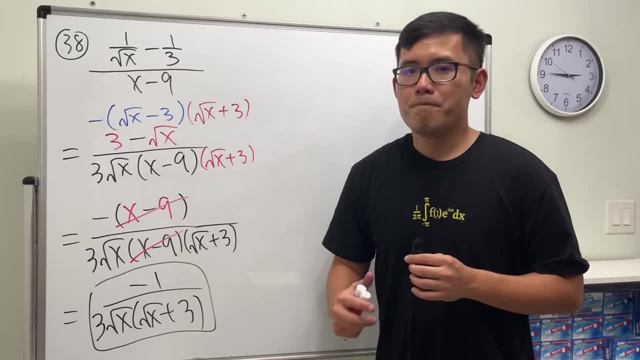 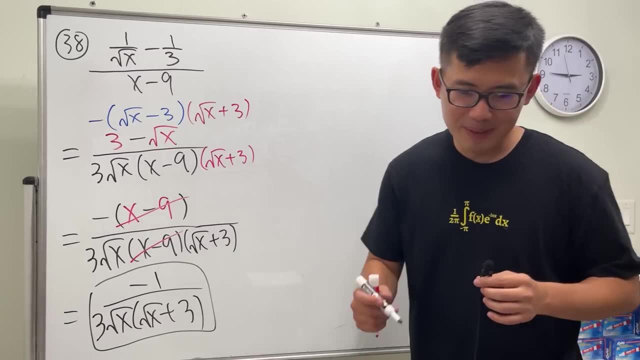 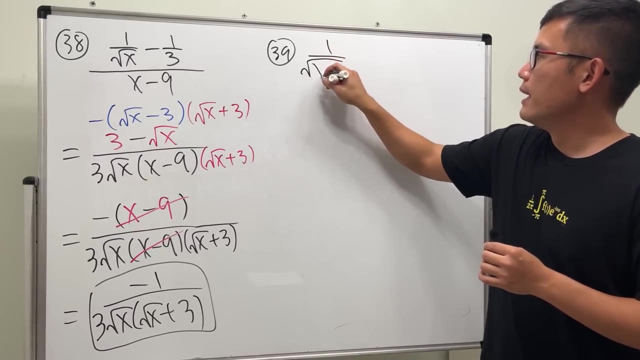 earlier. if you just go from here to here, to here to here, it's better than if you show all the other work every single time. yeah, number 39: 1 over square root of X plus H, and then minus 1 over square root of X over. 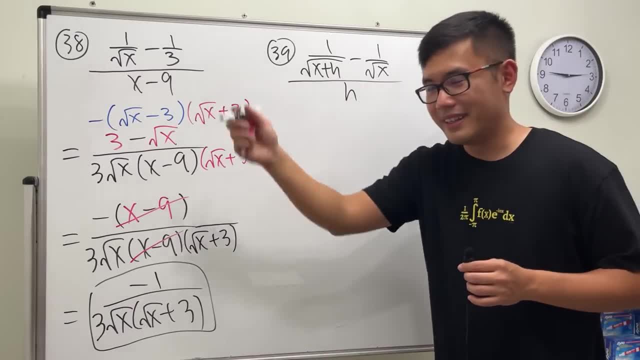 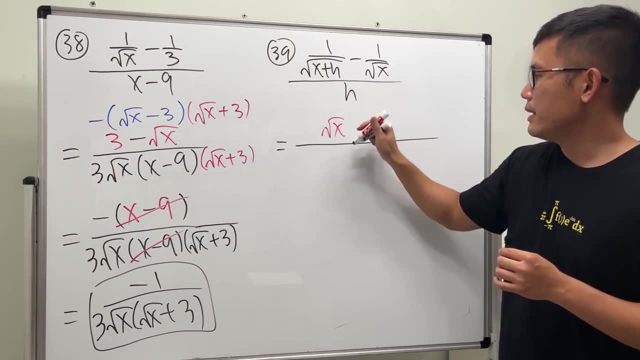 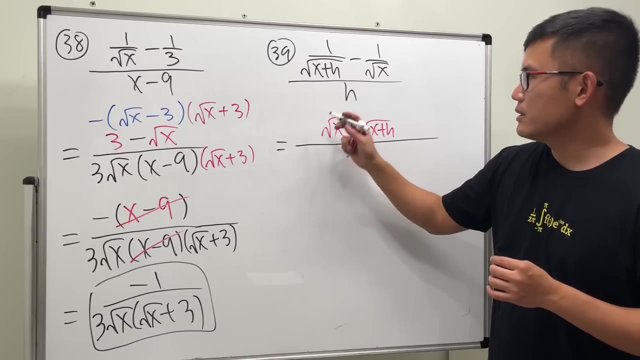 H, similar thing. that's just going to get work. okay, this and that which is square root of X minus square root of this analogous x plus H on the bottom star with X. so just just ask: what is just H, and then square root of x, and then the. 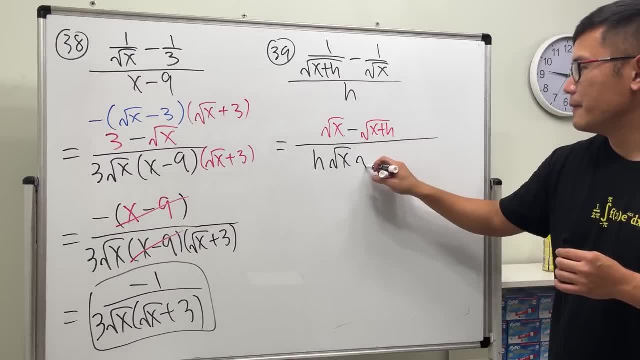 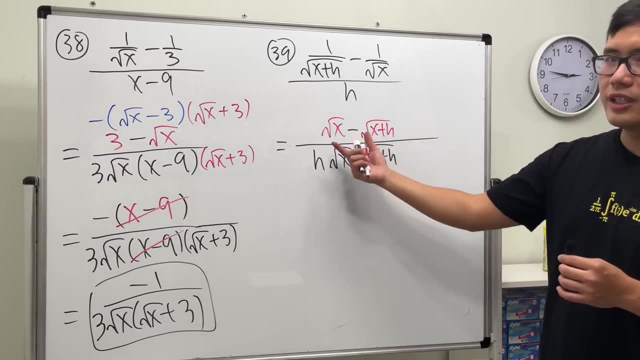 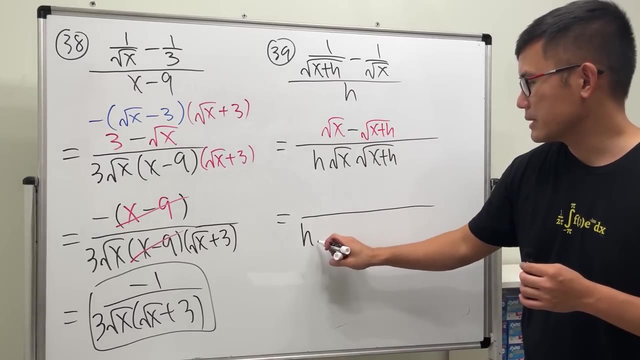 square root of x plus H like this, and also this: and not denominator. cool, now we need the count you get right. so the conjugate is going to be put a plus here. so let me justforme real out down, perhaps that would be easier. h times the square root of x and then square root of x plus. 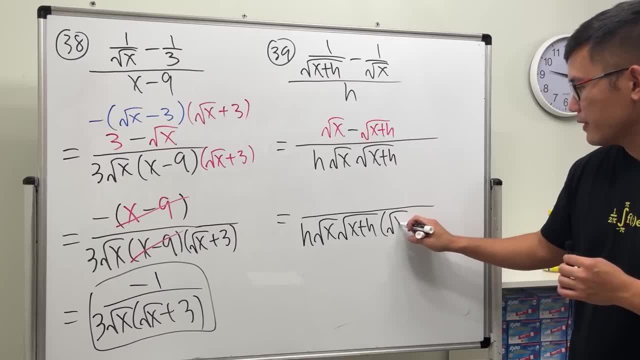 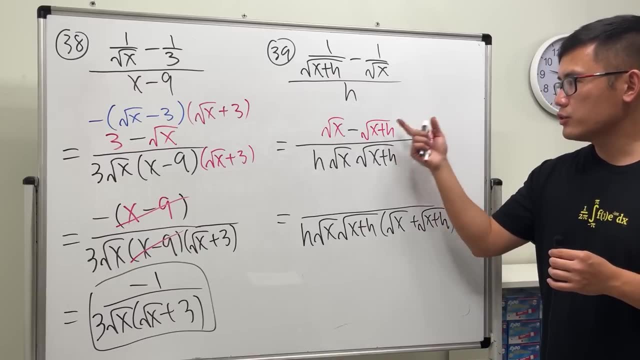 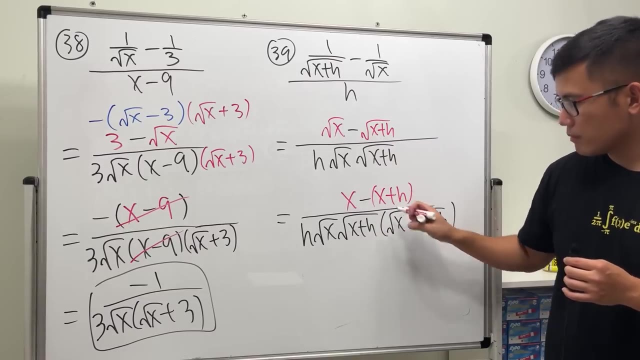 h, and then the conjugate also will go on the bottom: square root of x plus square root of x plus h. on the top, when we multiply by the conjugate, we'll just get the square of that which is x minus the square root of that which is x plus h. okay, so this right here is actually just x minus. 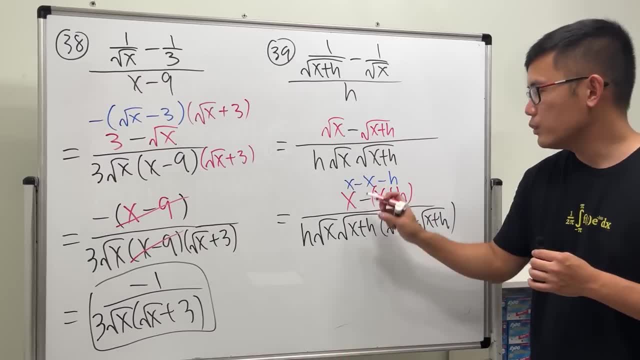 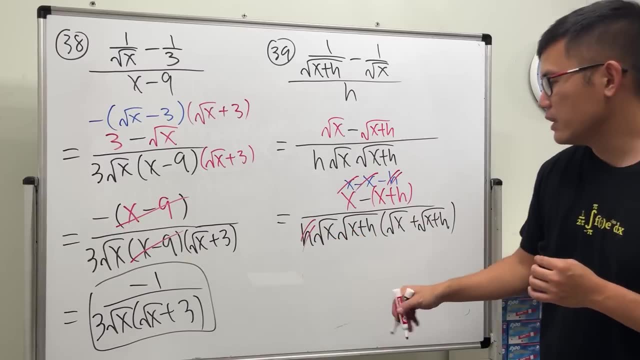 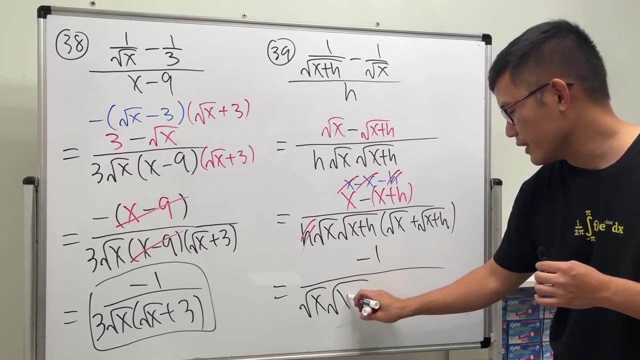 x minus h and we see that this and that cancel and this is negative h, this h and not reduced to one. yeah, but it's negative and that's it. so negative one over all the stuff. so square root of x times the square root of x plus h times square root of x plus the square root of x plus h. 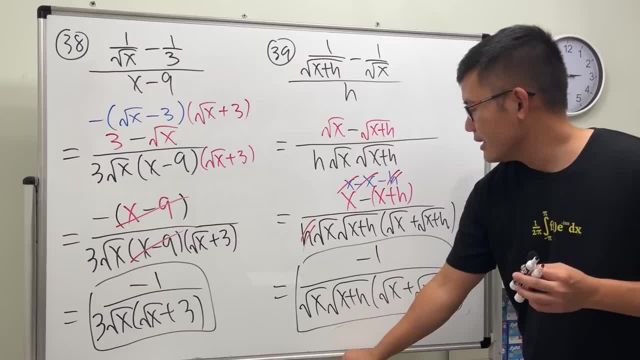 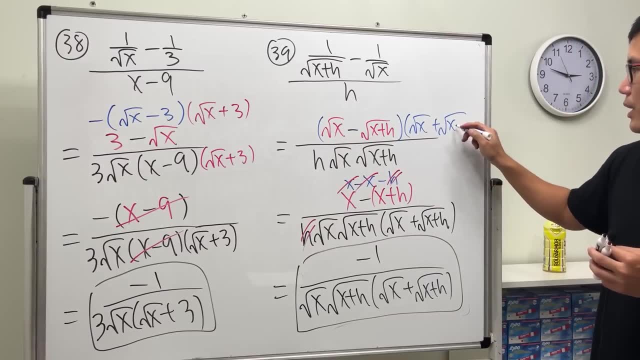 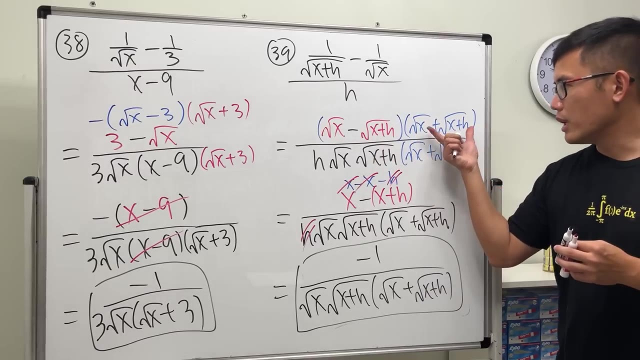 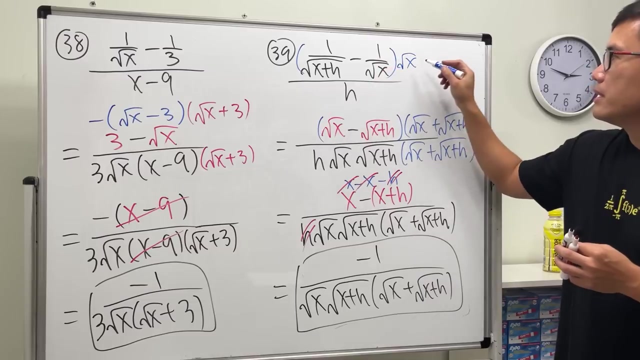 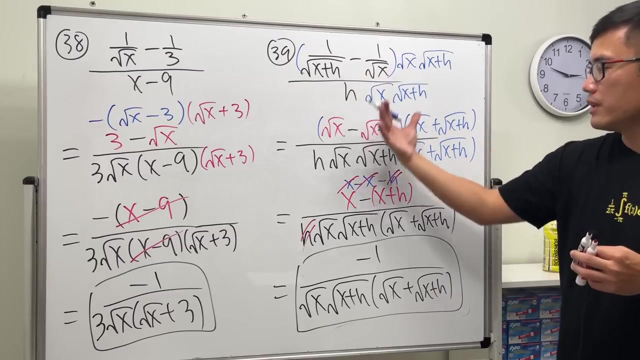 done. yeah, and let me just perhaps make this more clear: multiply the conjugate, right, that's what we did earlier, so that's how we were able to go from here to here. yeah, and then originally we multiply the lowest common denominator, so that's how we went from here to here, okay. 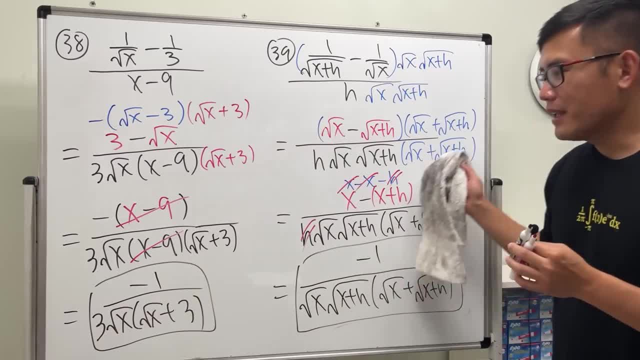 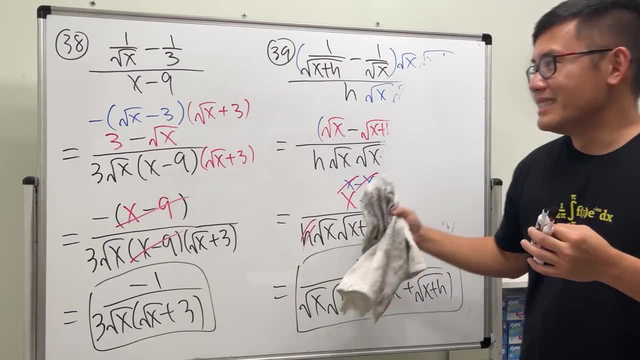 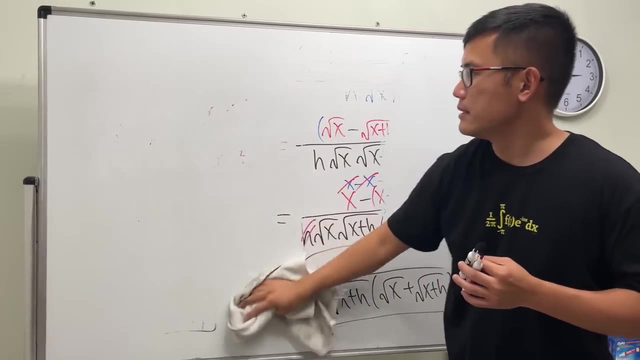 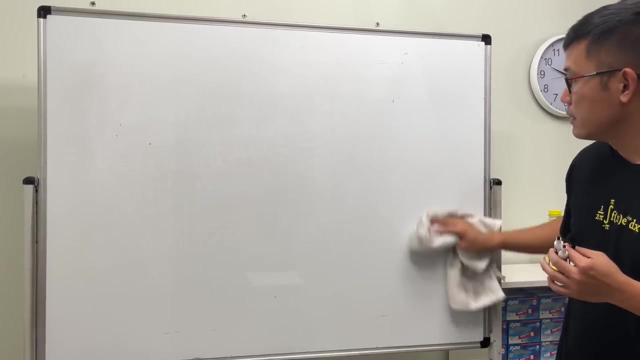 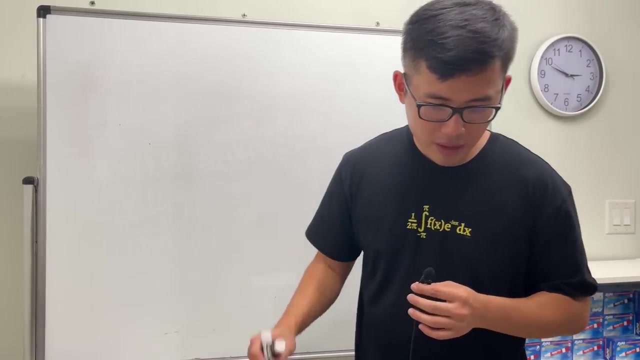 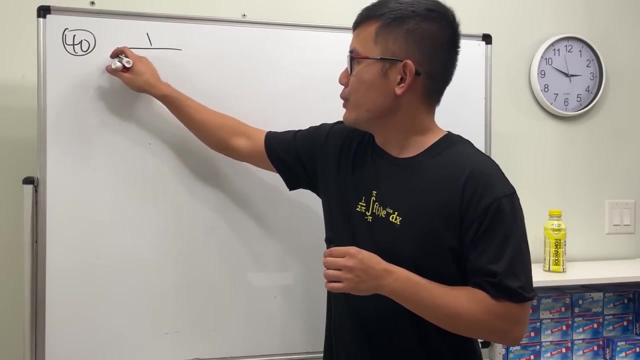 so, yeah, so if you kind of skip some steps like especially, like, uh, ultra steps, especially the steps that you have to write like very long, yeah, that would be much better, much better. number 40, wow, number 40, okay, 1 over 2 plus the parentheses x plus h. 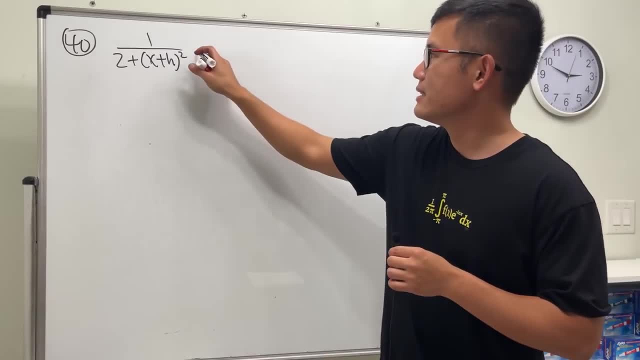 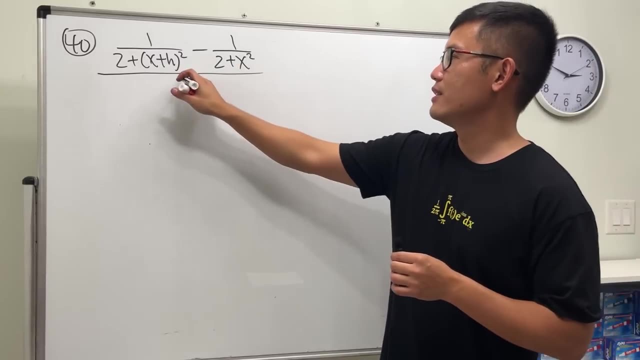 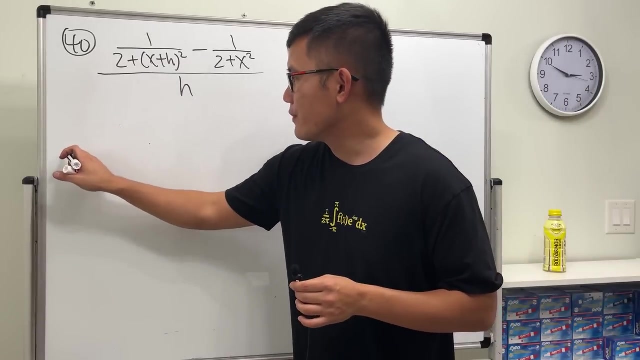 2 plus the parentheses x plus h square, and then minus 1 over 2 plus x squared over h. definition of derivative. that's why, all right anyway. so first thing, first multiply the top and bottom by this and that, right, so you know, this times one, yeah so. 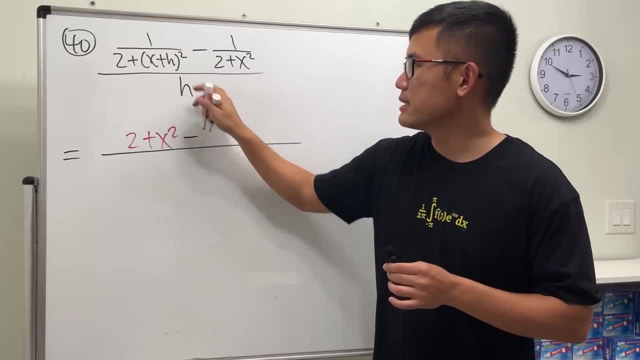 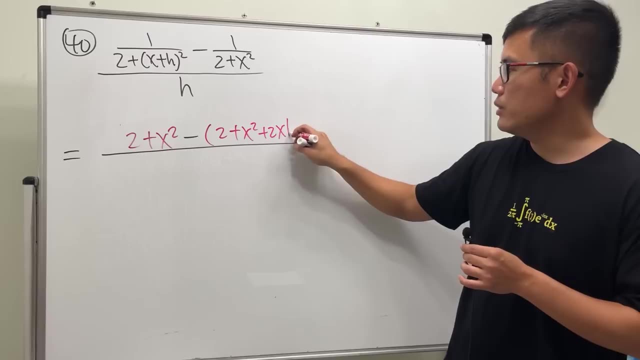 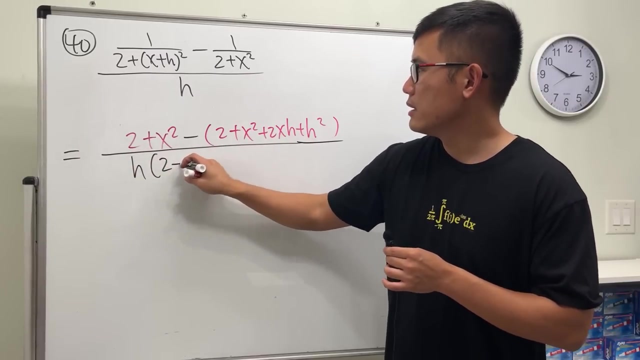 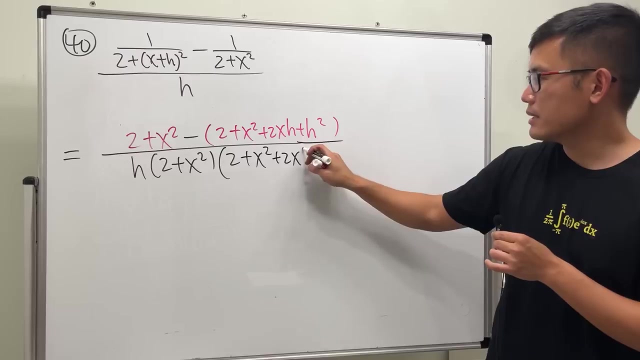 the first thing is two plus x squared, and then minus, this times that which is going to be two and open that. so we have x squared plus 2 x h plus h squared- wow over h. and then this denominator, and also that denominator, and now open that, which is 2 plus x squared, plus 2 x h plus h squared. okay, 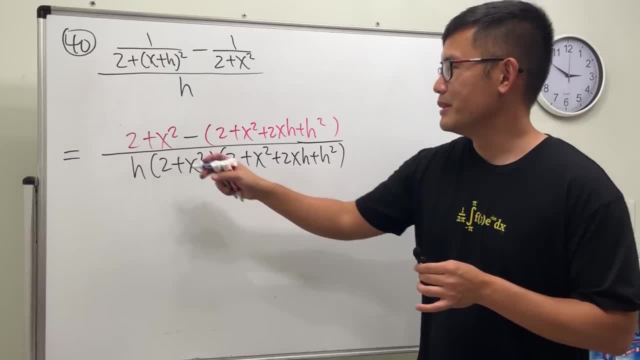 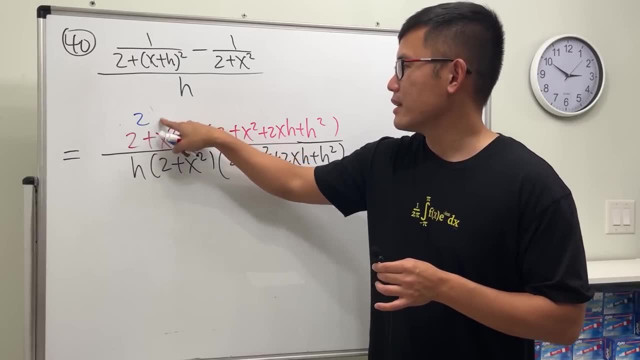 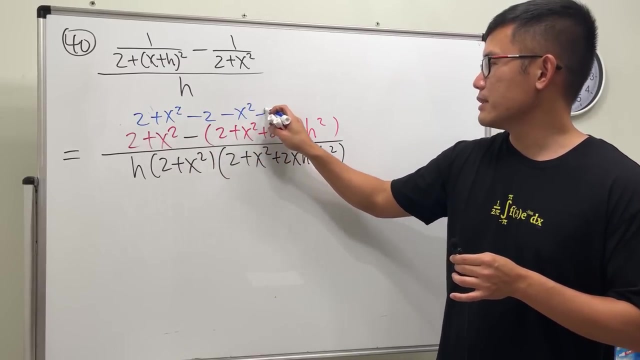 you can distribute and then cancel, or 2 minus 2. you can also cancel like that. i think i'm just going to distribute to make it more clear for you guys. so anyway, 2 plus x squared, and then this is minus 2 minus x squared, minus 2 x h minus. 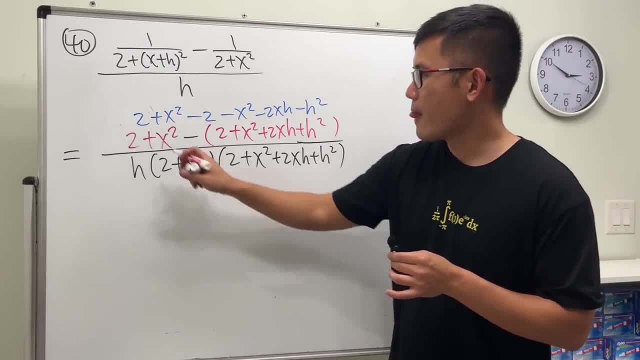 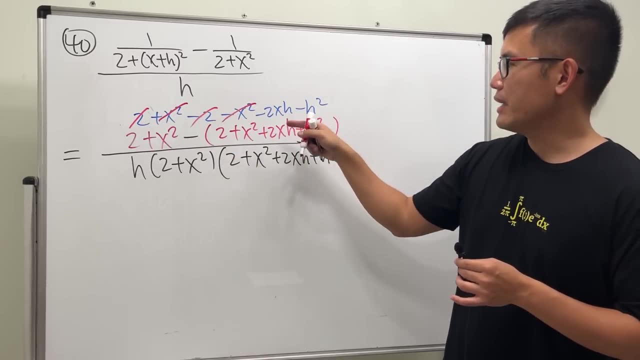 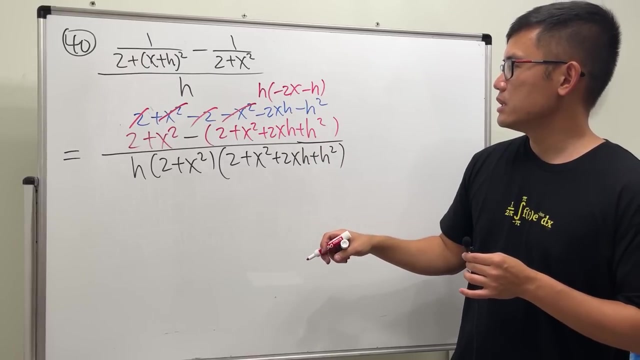 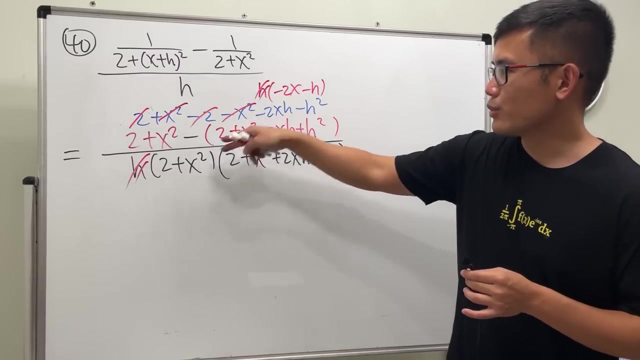 h squared, yeah, and then i'll cancel: 2 minus 2 gone. x minus x, squared gone. and then we have all this, but they have h, so we can factor that out, and then we have negative 2x and then minus h. yes, this h and that h cancel, yeah. i just want to match my cancellation with: 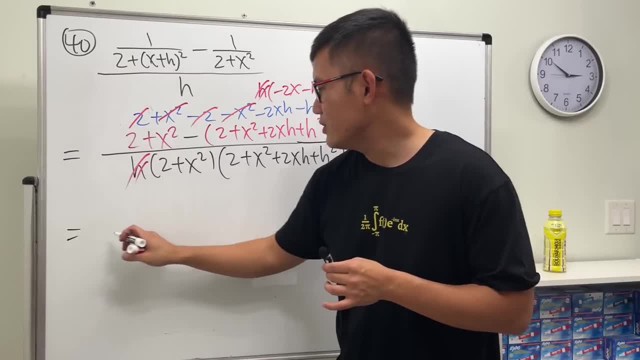 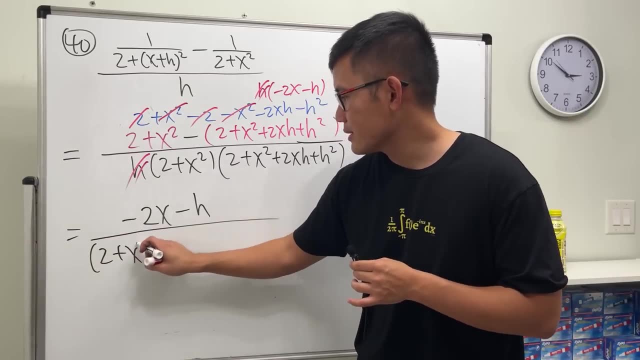 2 marks, and that's it. ladies and gentlemen, we have negative 2x minus h, over all that stuff. so 2 plus x squared times 2 plus x squared times 2x squared times 2x squared will be the answer. or over all that stuff. so 2 plus x squared times 2x squared will be the answer. 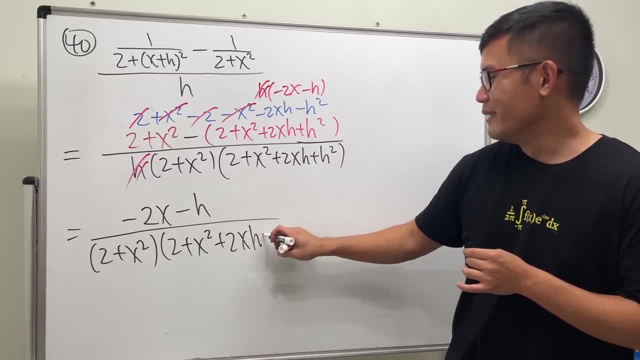 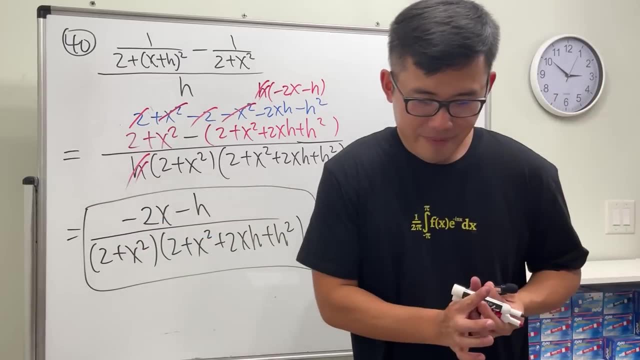 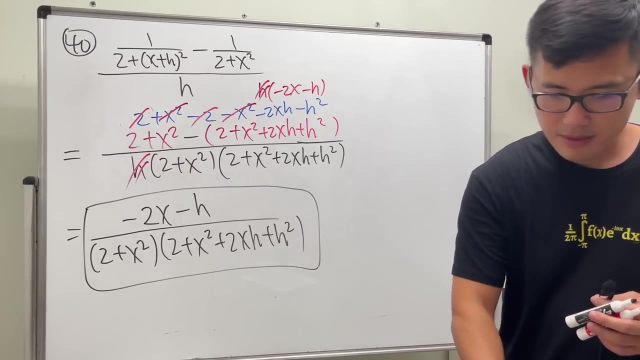 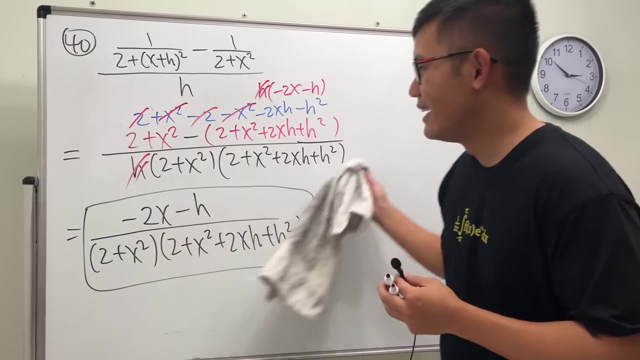 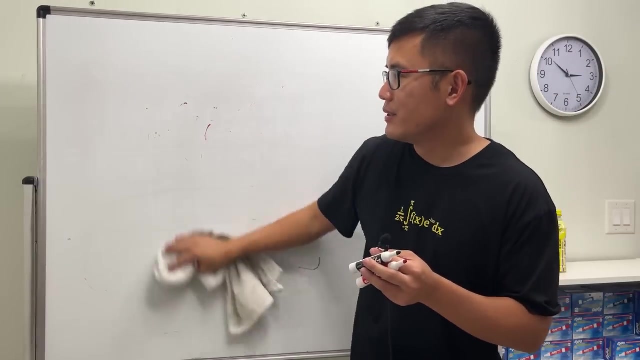 plus X square plus 2 X H plus H square. okay, it's only two hours, that's good. I'm actually not charging my phone yet and I'm going to wait for, like, my phone tells me that like 20% or temperate 10%. 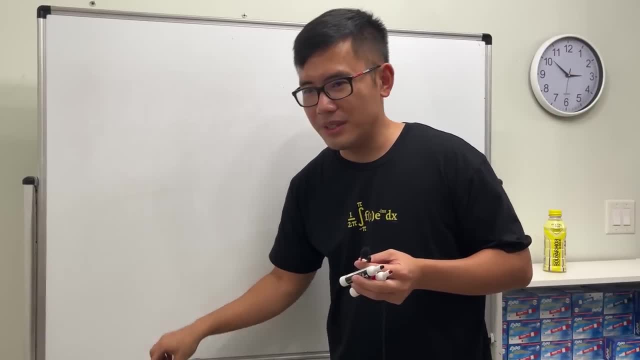 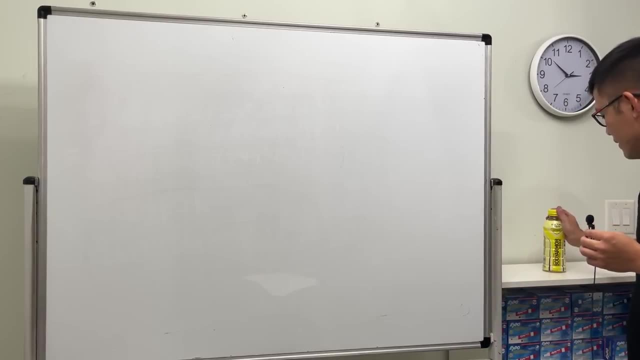 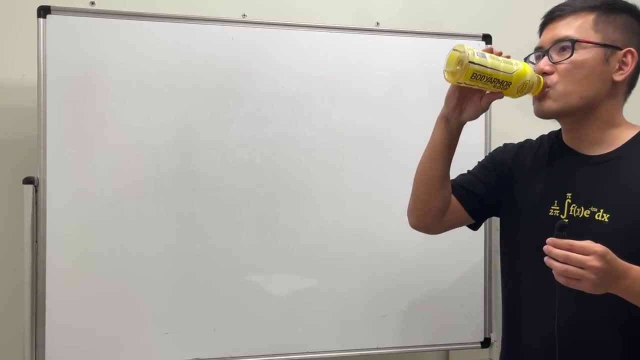 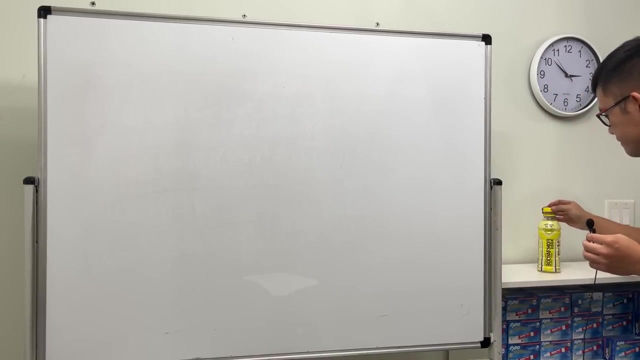 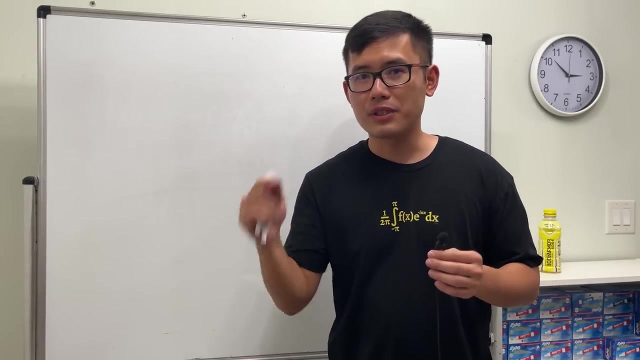 left and I will charge, because I'm afraid if I charge the phone to be like snow noises in the background and that's not good. anyway, not sponsored by this cream company, unfortunately, but it's pretty good. okay, early was complex fraction and we did a lowest common denominator right. 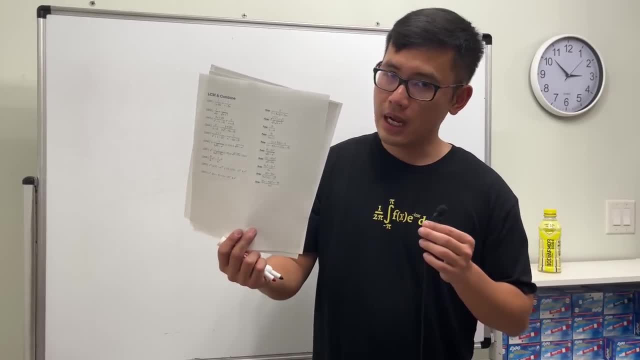 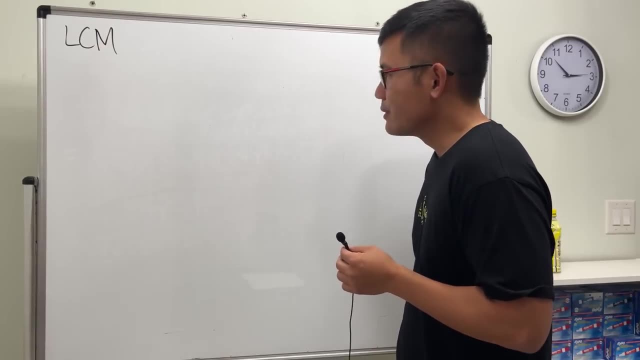 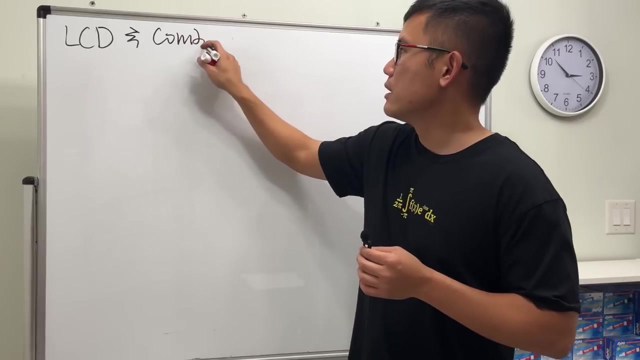 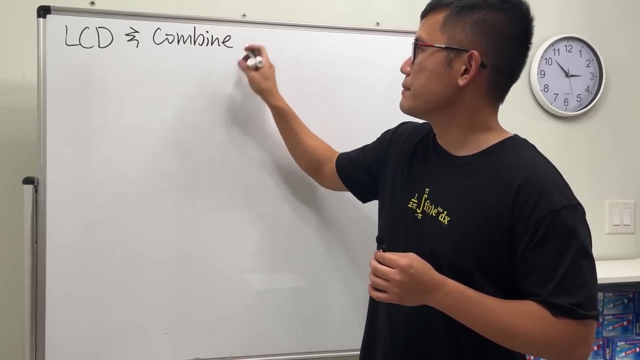 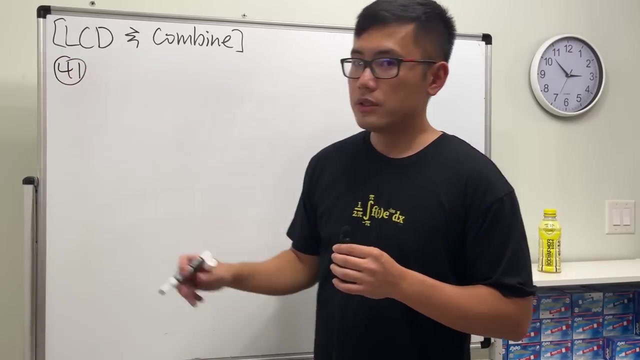 now we will do the lowest common denominator and combined fractions. so lowest common, the lowest common multiple for the denominator. so usually people just write yes, LCD, and then we will combine the fraction. that's the category for this part. combine, all right, number 44, number 41. so notice, now we are just going to have two fractions. so here we. 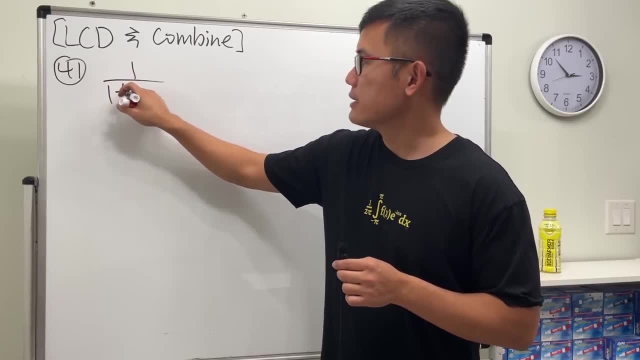 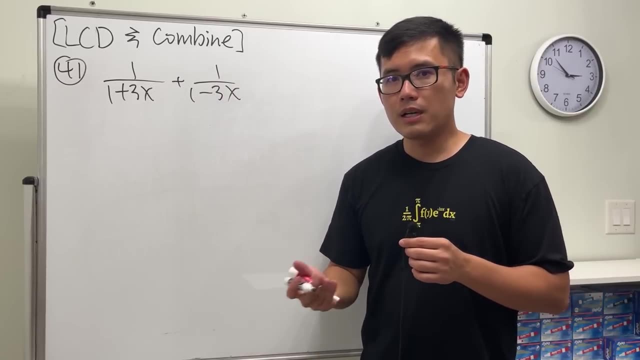 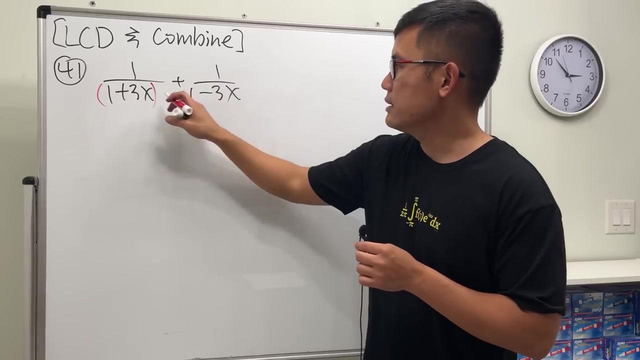 have 1 over 1 plus 3x, and the other one is 1 over 1 minus 3x. so what we are going to do is just combine them, and to do so, you see they have three different denominators. let's just go ahead and multiply this by this, which is: 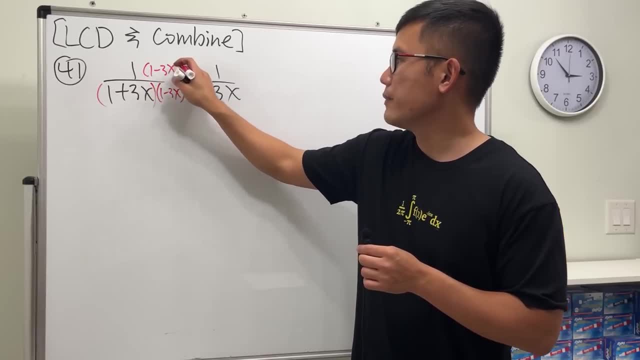 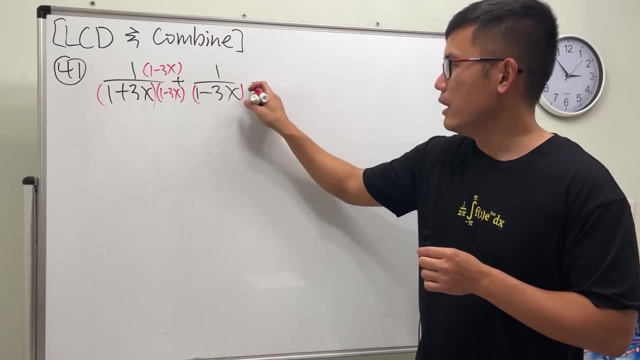 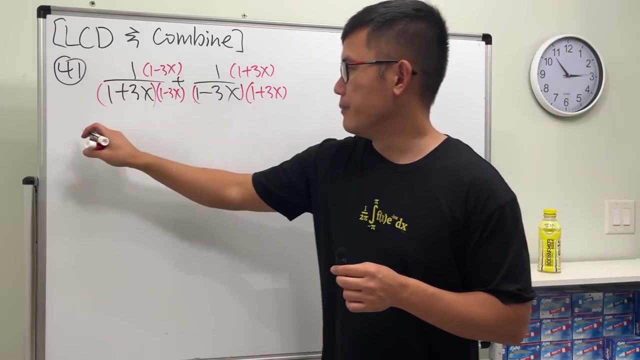 1 minus 3x, and likewise we do the same on the top. and then, right here, let's go ahead, multiply this by that 1 plus 3x, and of course do the same on the top, and then put them together, because now they have the same denominator. we can just 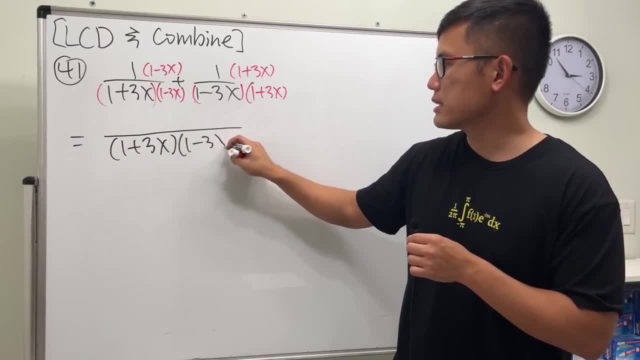 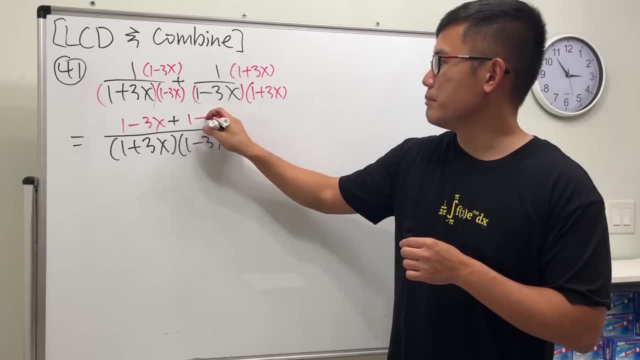 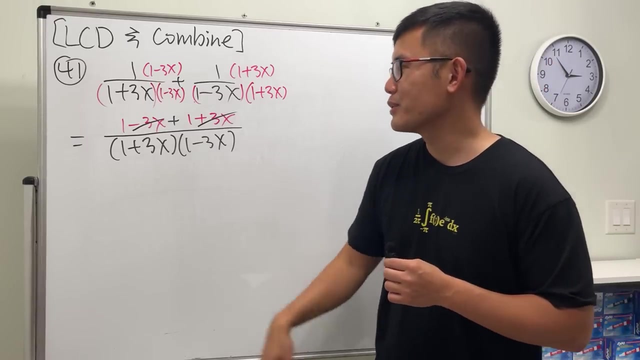 write it as 1 plus 3x times 1 minus 3x and then the top right here is just 1 minus 3x plus 1 times that is just 1 plus 3x, and we see this and that cancel and 1 plus 1 is 5, not just kidding, 2 on the bottom, just. 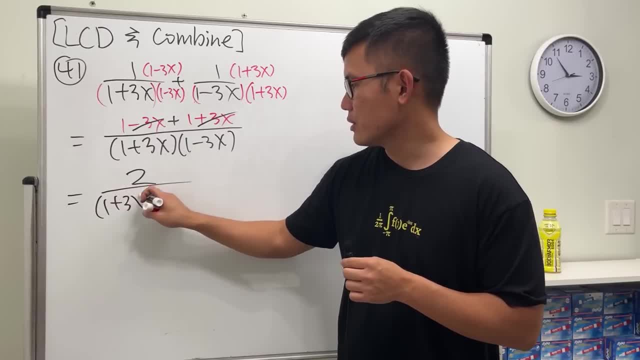 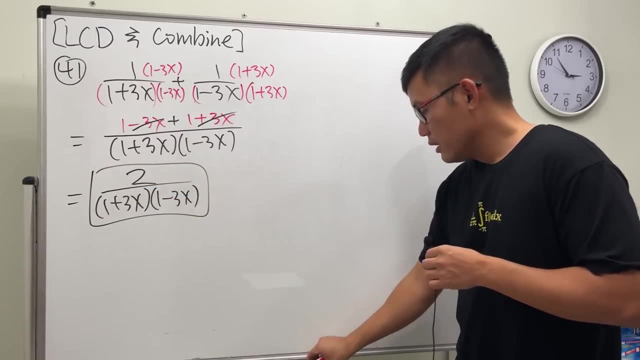 leave it. you don't have to multiply out the denominator. so leave it as 1 plus 3x times 1 minus 3x. yeah, if you multiply it out it will look like this, which is 1 plus 3x plus 1 plus 3x. so if you multiply it out, it will look like this: 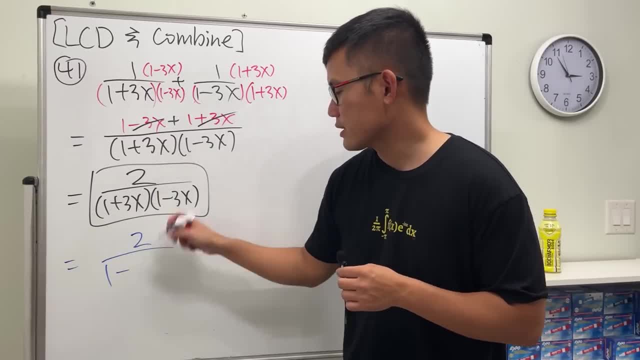 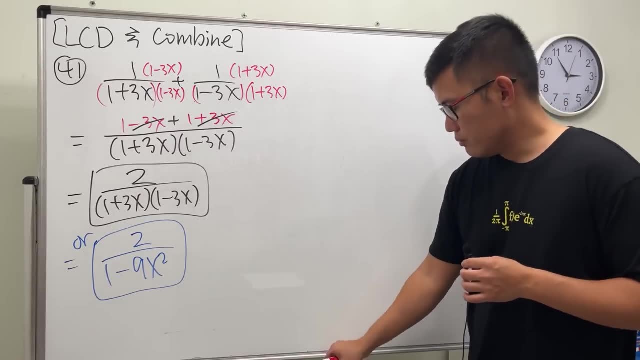 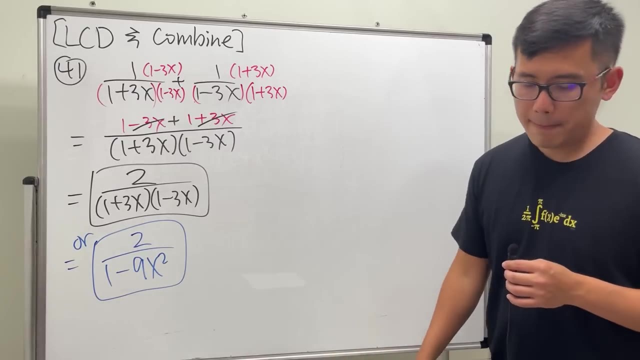 2 over 1 squared, minus 3x squared, which is 9x squared, That's 3x squared. So yeah, one way or the other. Okay, that's number 41.. Now 42.. 42.. 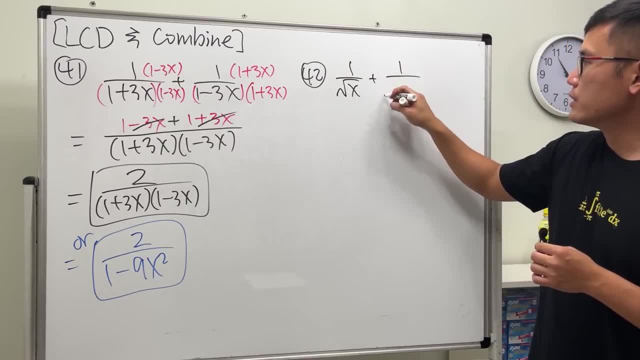 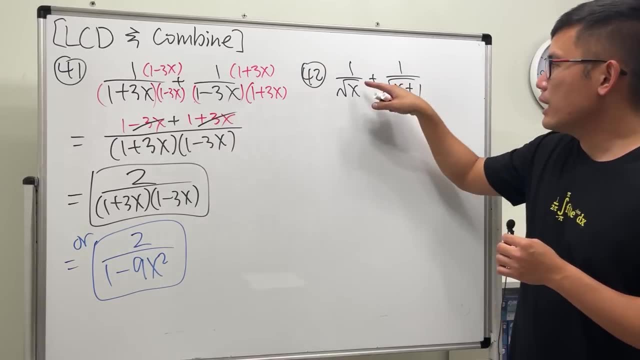 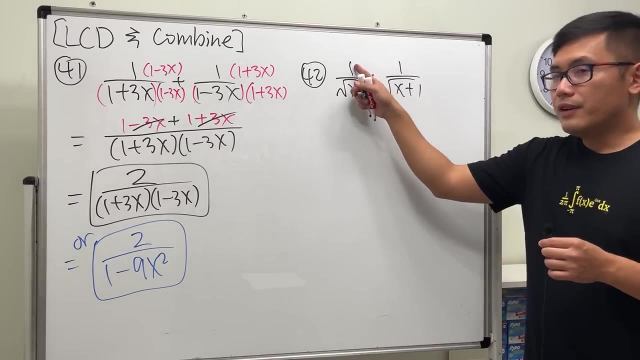 1 over square root of x plus 1 over square root of x plus 1.. All right, so for this let's go ahead and just practice that We know that this guy needs this and that And this, The first fraction needs the square root of x plus 1 on the bottom and also on the top. 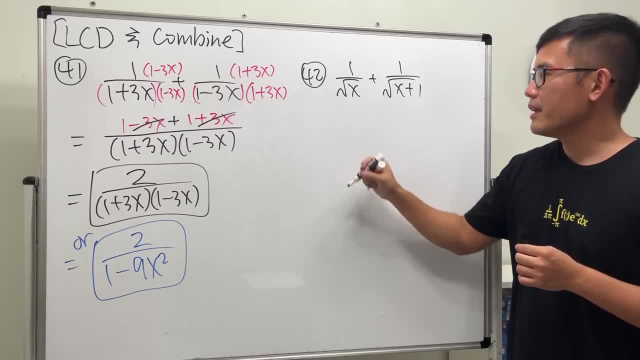 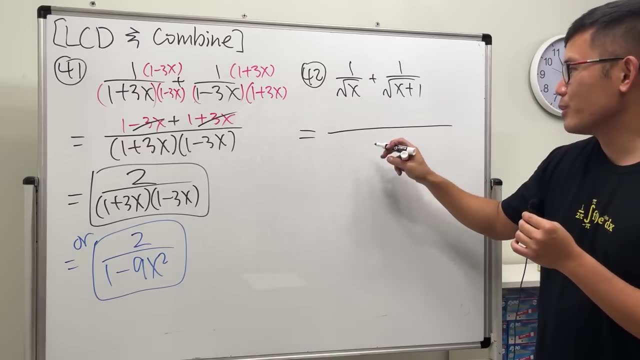 The second one needs the square root of x on the bottom and also on the top right, And let's just go ahead and kind of do this in our head, Save us some energy from writing. So right here I'm just going to do a multiplication together. 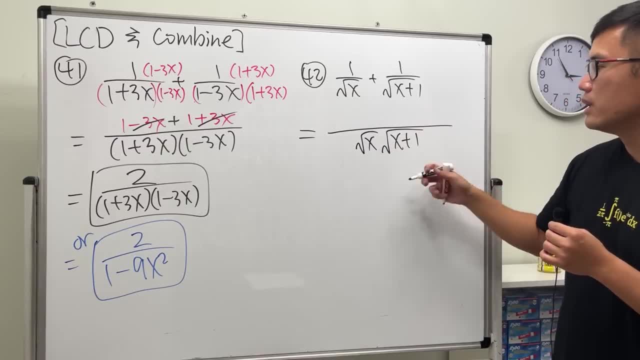 So square root of x times square root, Square root of x plus 1.. And you can just write it like this: And then you do 1 times that which is square root of x plus 1.. And then we add it with square root of x, like this: 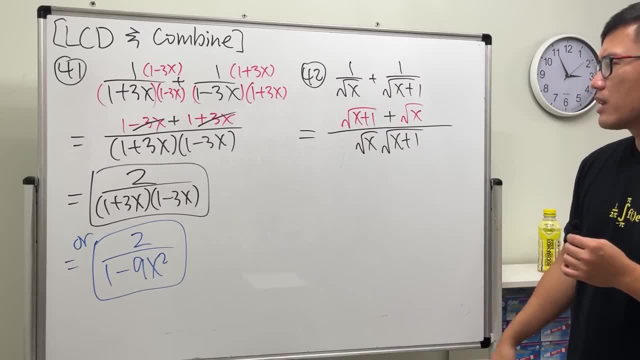 And that's it. And you might be wondering: do you want to do the conjugate? Well, right here, the main thing is just to combine them. If you leave it like that, that's okay. If you did the conjugate, this is the reason why I said that. 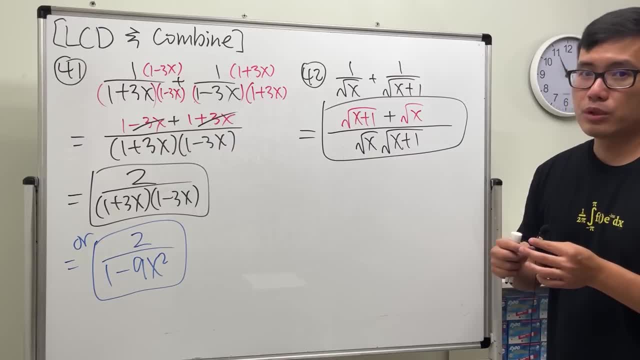 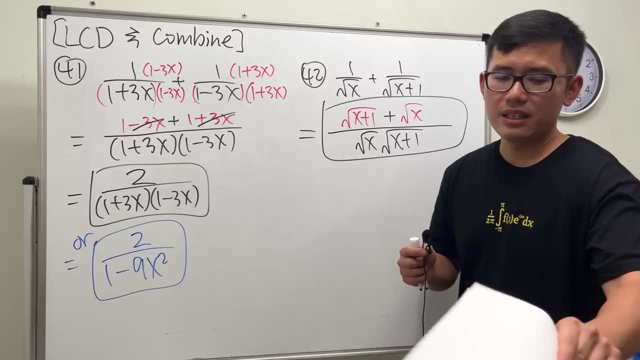 If I test my students, I will make sure that I give them multiple choice questions for this, And that's why make sure you follow the answer keys so that you know. okay, just stop right here and move on. Yeah, If you did the conjugate, it's not going to be so nice, I think. 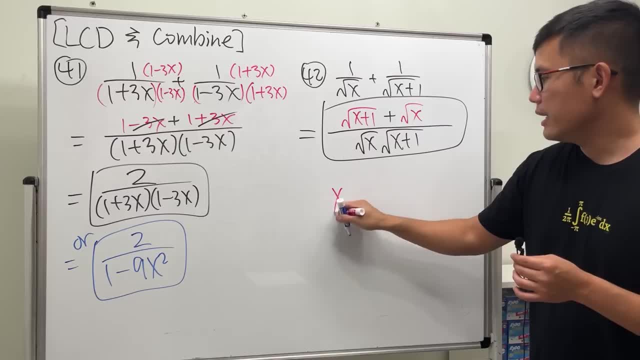 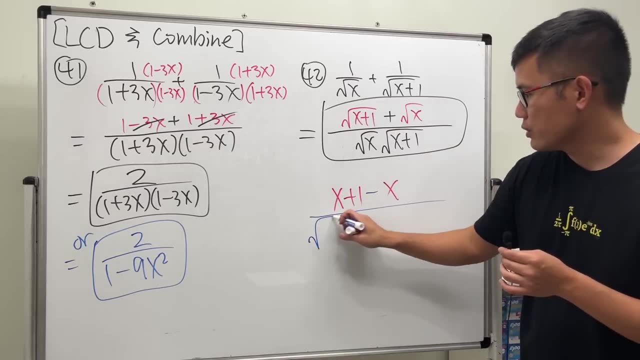 I don't think so, But let's try it. Square this, which is x plus 1 minus the square of that. Yeah And over, this thing is square root of x, Square root of x plus 1.. And then the conjugate earlier is the square root of x plus 1.. 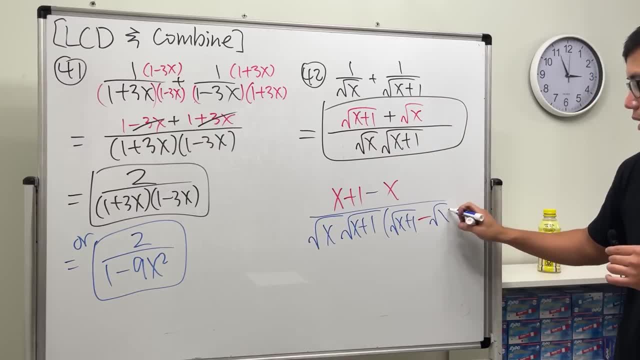 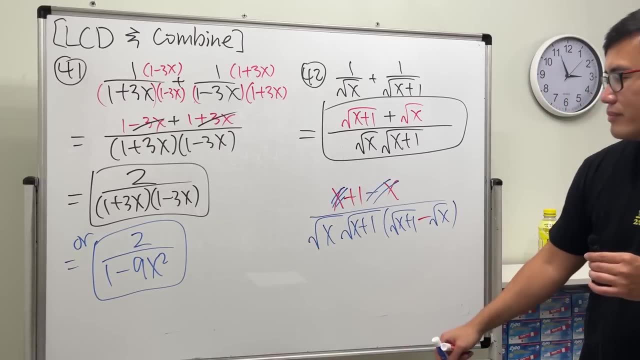 E was a plus, Right now it would be a minus And the square root of x And we see that. okay, this and that cancel. So we get this 1 over square root of x, square root of x plus 1.. 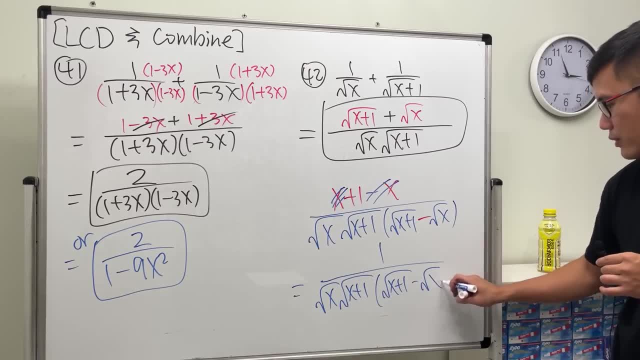 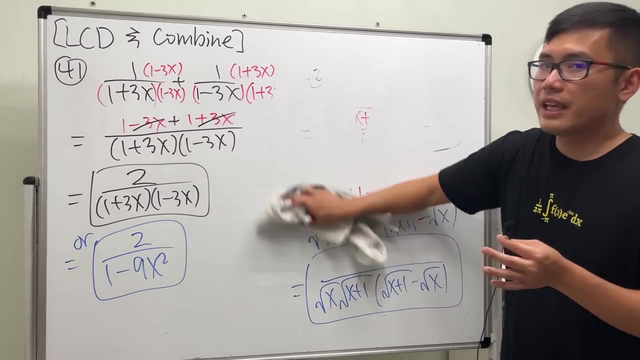 And then square root of x plus 1 minus square root of x. If you multiply the top and bottom by the constant, You get yeah. So just like that, Okay, But right here we'll focus on just getting the same denominator and then combine the fractions. 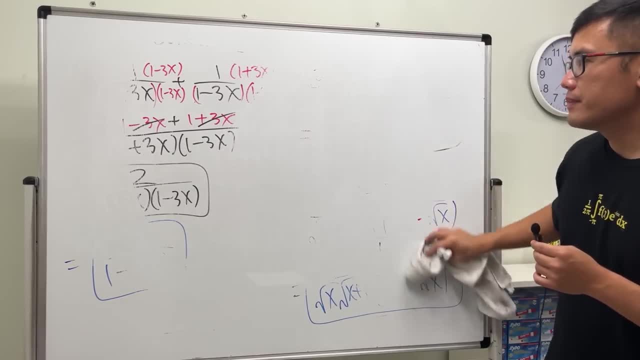 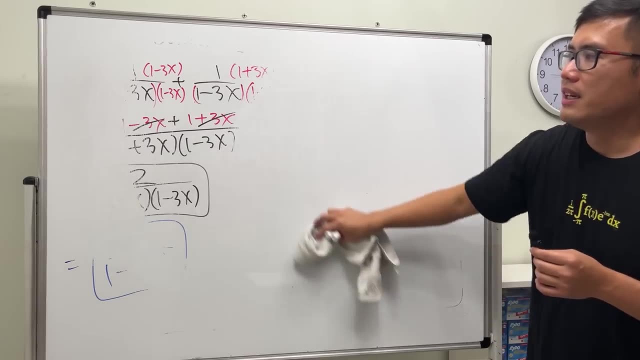 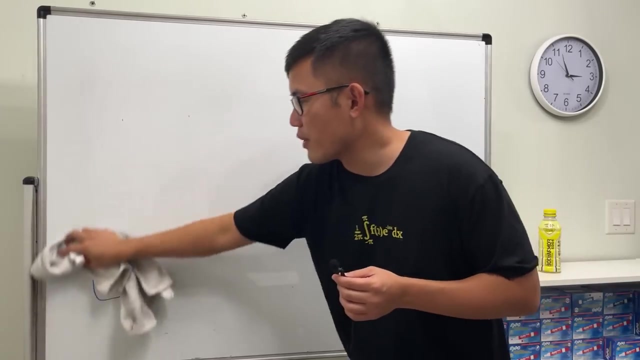 I put this after the complex fractions. I was debating to see which one I wanted to put first, But I think this right. here it's a little bit more difficult because you cannot cancel things out right away, So that's why I put it after the complex fractions. 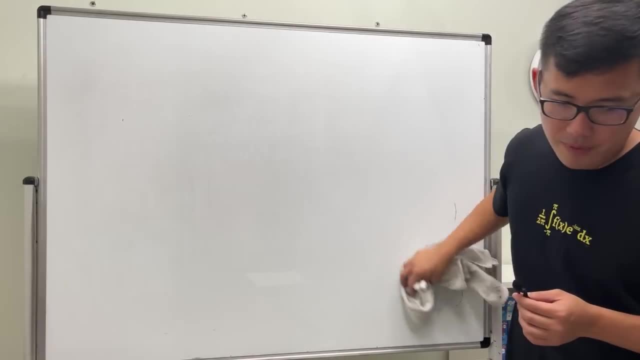 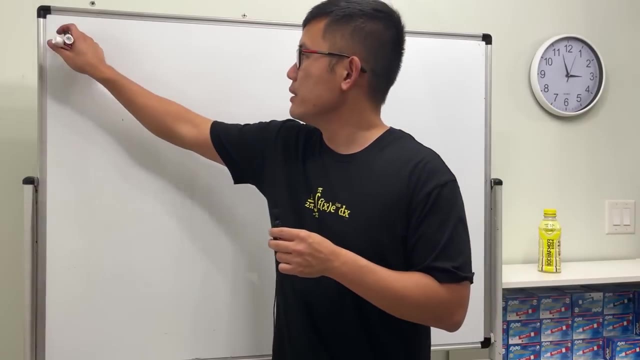 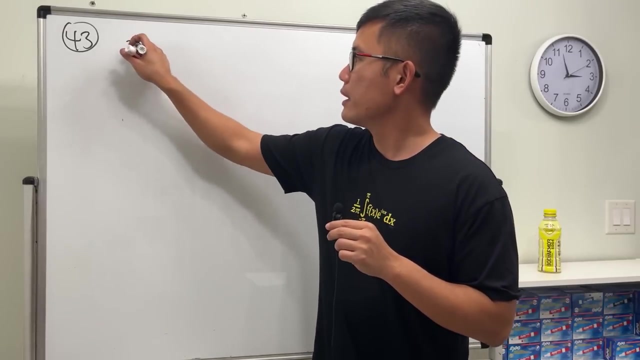 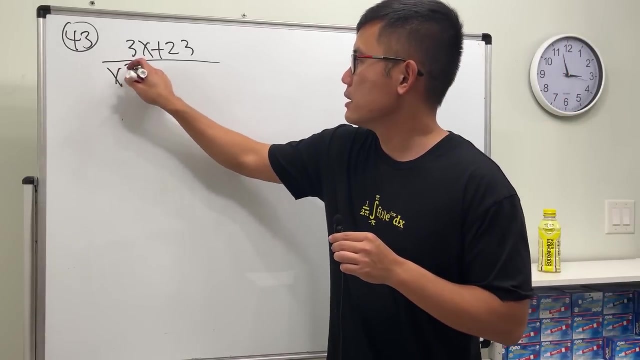 But you'll also see the later on cases why it becomes more trickier. Anyway, number 43. Here we have 3x plus 23. Over x minus x, squared minus x minus 12. And then the other one is plus. 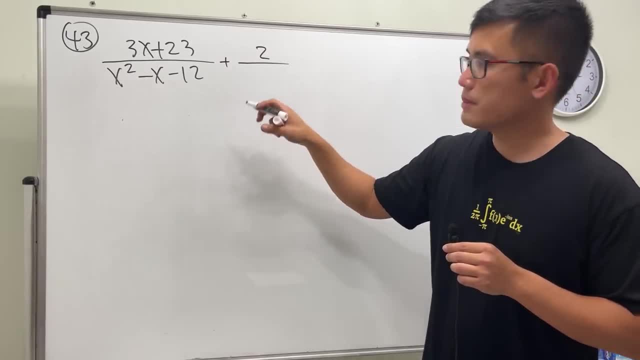 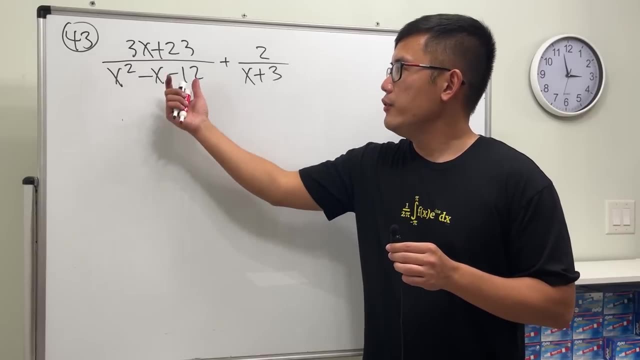 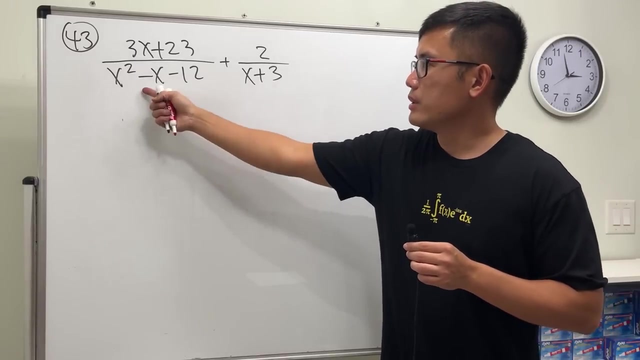 So that's 2 over x plus 3.. Alright, In this case, if you multiply this thing by x plus 3,, x plus 3.. And if you multiply this thing by this whole denominator, that's too bizarre, Because in fact we can factor this out. 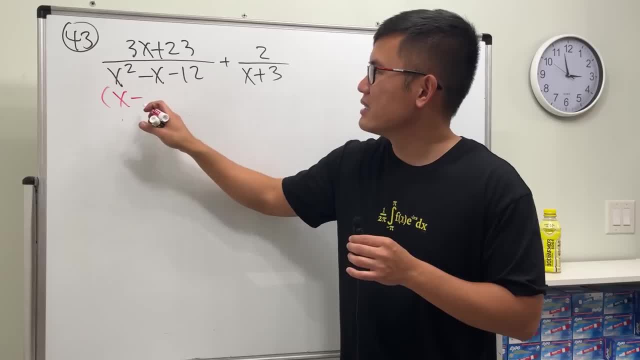 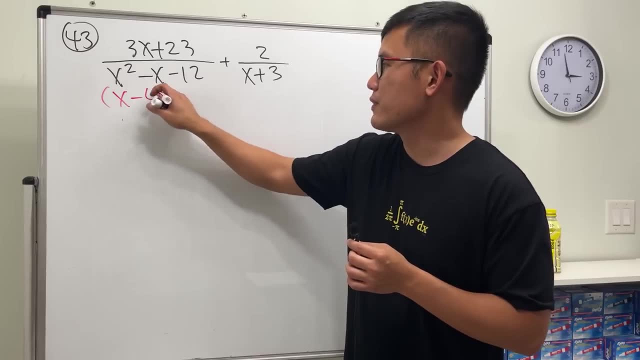 So let's go and factor it. We get what? x minus x minus x minus x plus 3.. x plus 3.. x plus 3.. x minus 3. x minus 3.. Oh yeah, x minus 4 times x plus 3.. 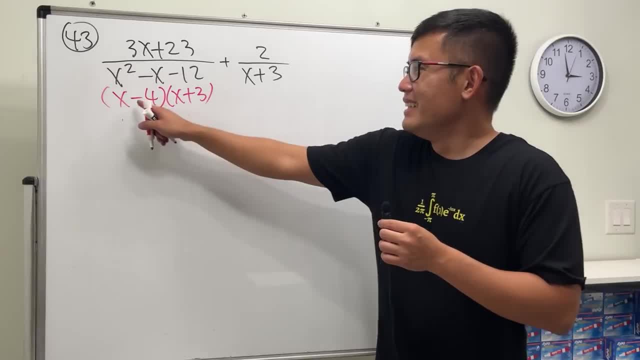 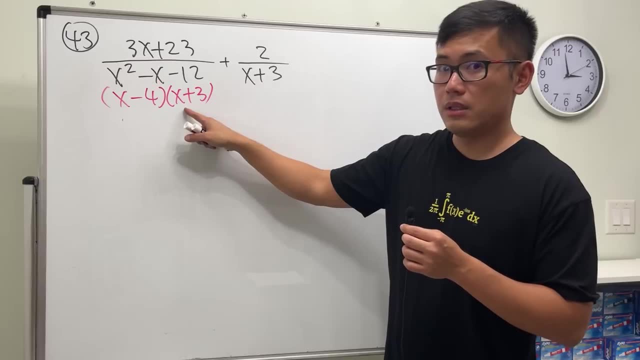 I don't remember what times. what is equal to negative 12.. Negative four times positive. three is negative 12, and together we get negative one. Yeah, So you see, we have the x plus 3 in common. So that means this first fraction is done. 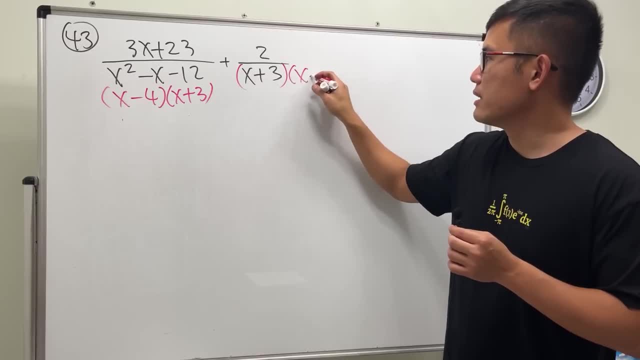 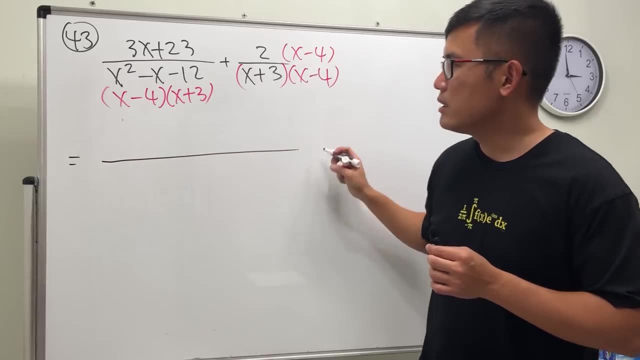 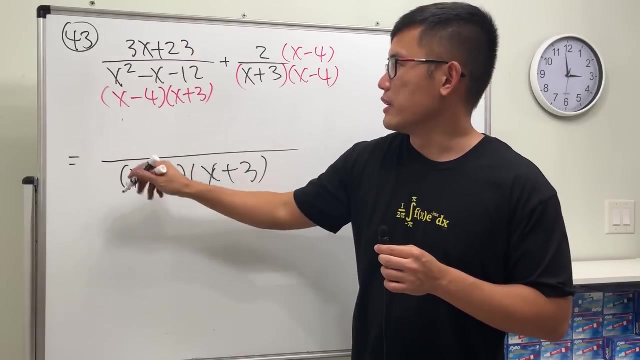 For the second fraction, we just need that x minus 4 on the bottom and also on the top, Okay, and then we see that we can put them together and we have x minus 4 times x plus 3. this thing stays the same, so let's keep it as 3x plus 23 and then multiply this out, of course. 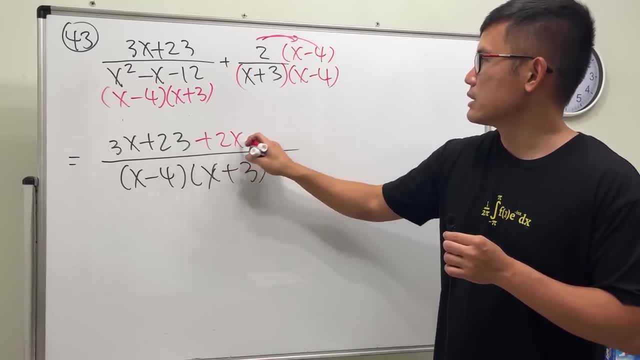 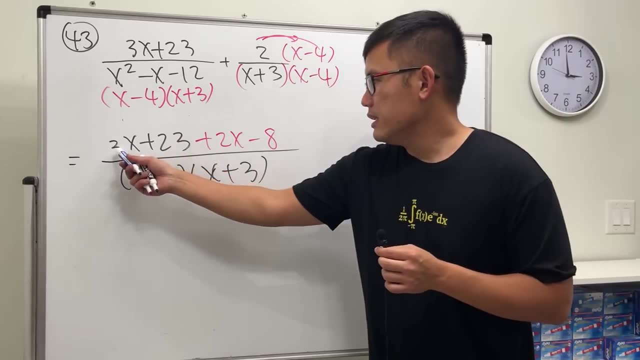 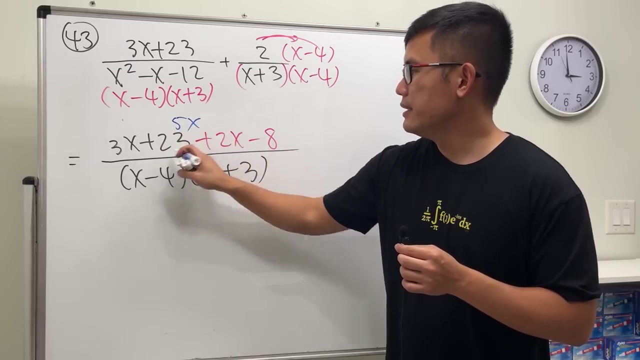 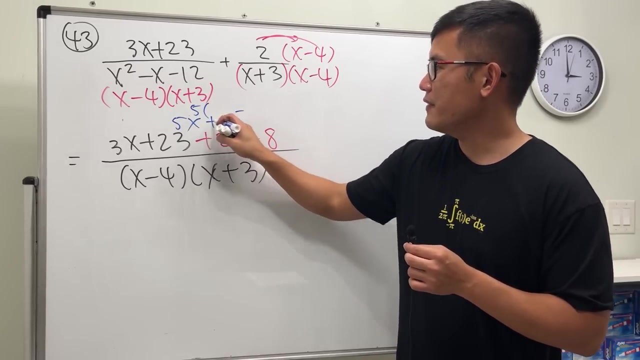 and that's a positive. so that's plus 2x, minus 8. can we cancel anything? well, let's combine things. first, this and that is 5x, this and that is plus 15, yeah, and then we can factor out a 5, so 5 and. 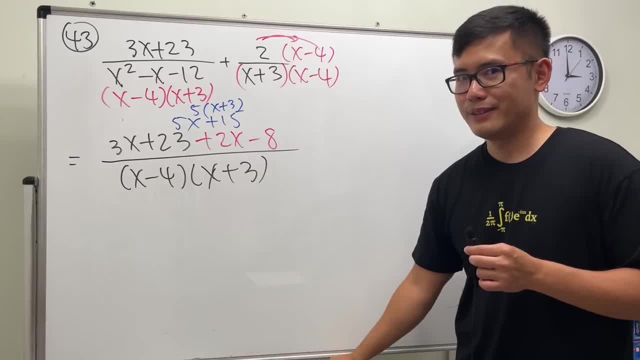 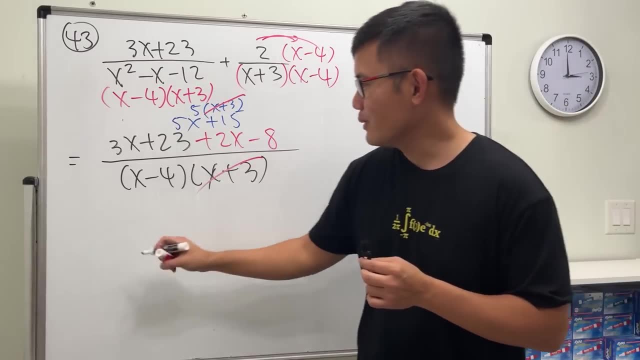 then this is x plus 3. aha, i told you i'd come with all these questions. set up nicely, huh. x plus 3, x plus 3, cancel. so the final answer is 5 over x minus 3 and that's 4 and we are done. 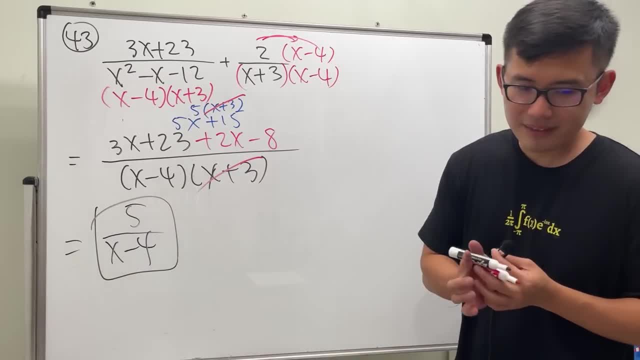 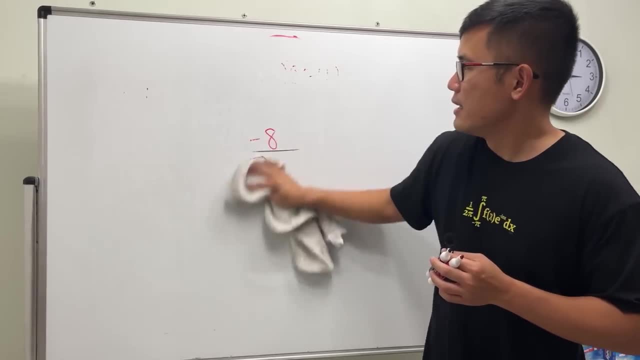 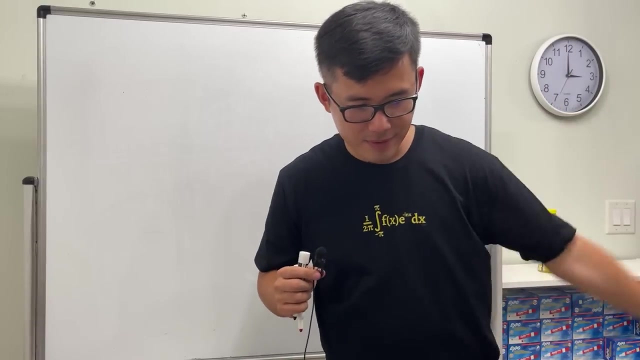 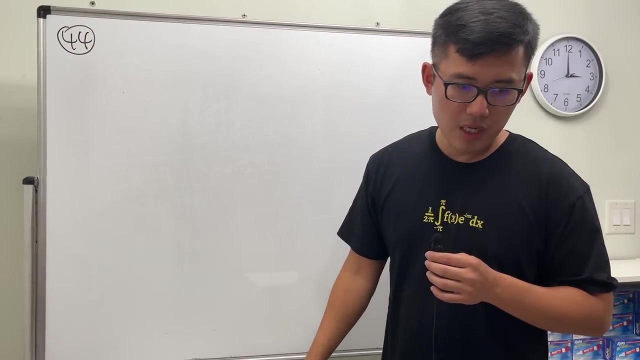 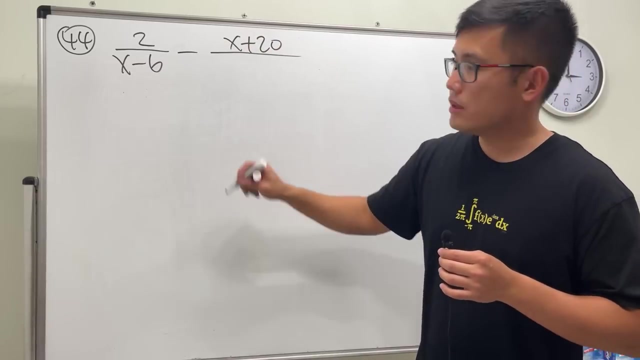 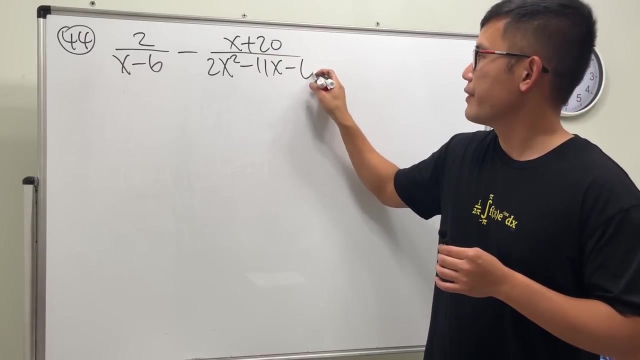 yep, just like that number 44. so here we have 2 over x minus 6, and then the other one is minus x plus 20 over 2x square minus 11x and then minus 6. this can be factored in this time. let's just go ahead. you can do the tic-tac-toe on the side, but 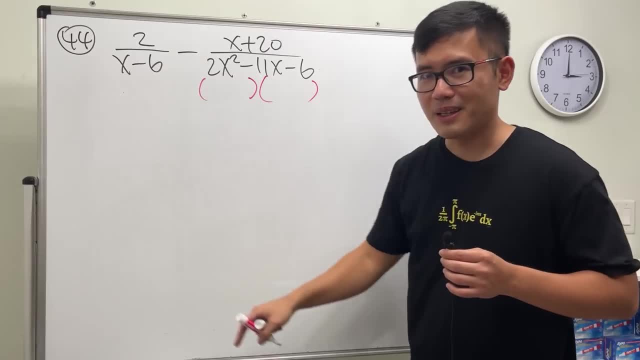 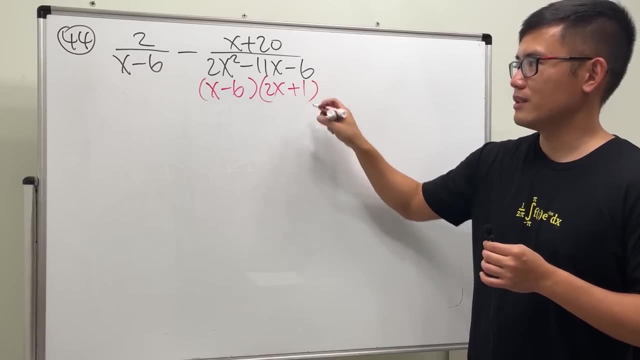 let's just try to see if we can do it. you know it's going to be that now. yeah, let's try x minus 6. so that means we have to have 2x. and then what else do i need plus 1? does it work? try it that. 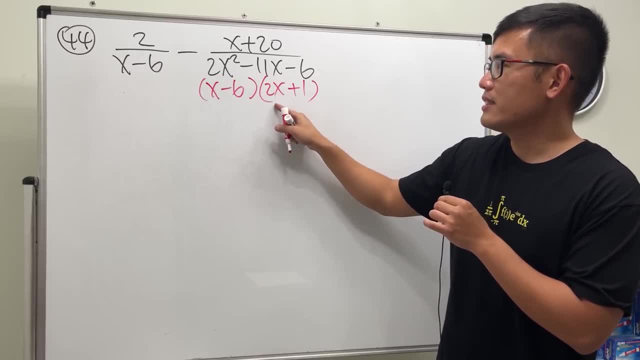 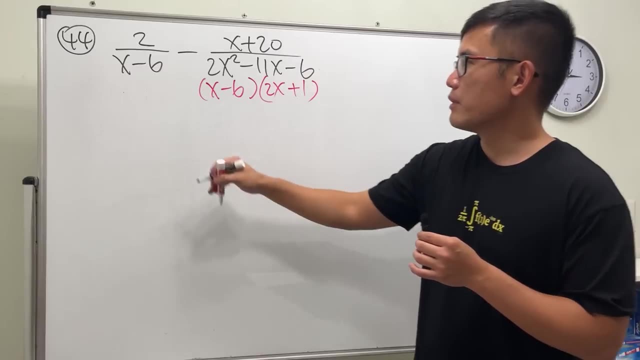 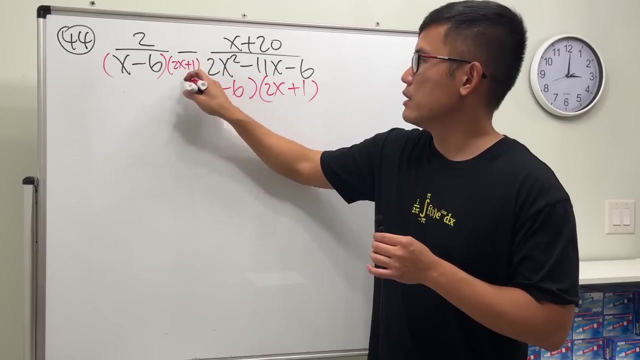 gives us 2x square, and this is negative 12x plus 1x. that does give us negative 11x, negative 6. good, so this time, though, we just need to come here for the first fraction and then multiply this by this, because that's what it needs. so 2x plus 1 on the bottom, and also 2x plus 1 on the bottom. 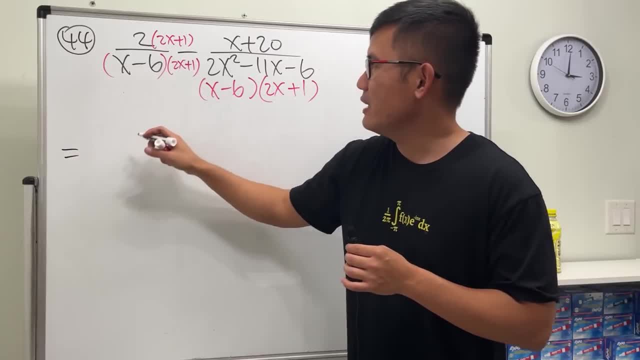 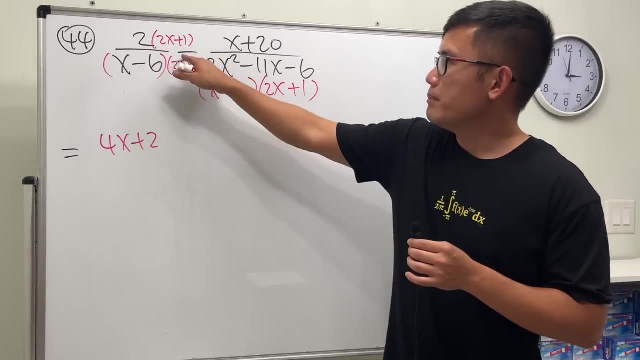 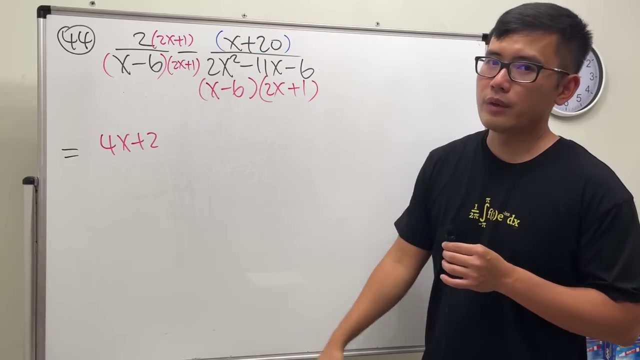 on the top. so we are looking at this is 4x plus 2. now be really careful. we are subtracting this fraction and technically deal with a invisible parentheses, like what i mentioned, it like two hours ago. so distribute the negative, we will get negative and then the. you know just. 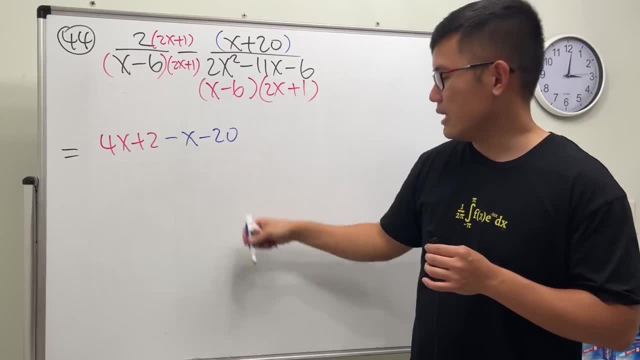 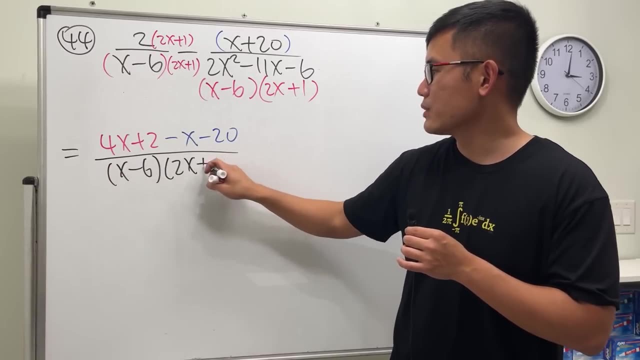 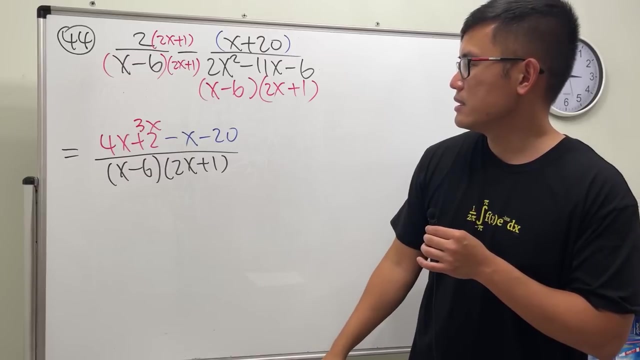 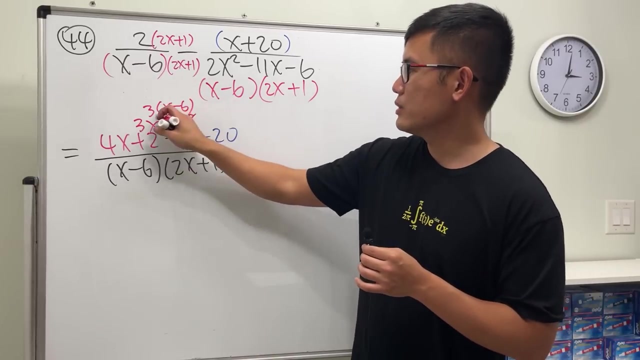 write it down like negative x and then minus 20, that's negative. and then you can do this: the denominator x minus 6, 2x plus 1, and now let's just fix the top, so this and that is 3x, and then this and that is minus 18, and then we can factor out 3 and then, better yet, we can cancel. 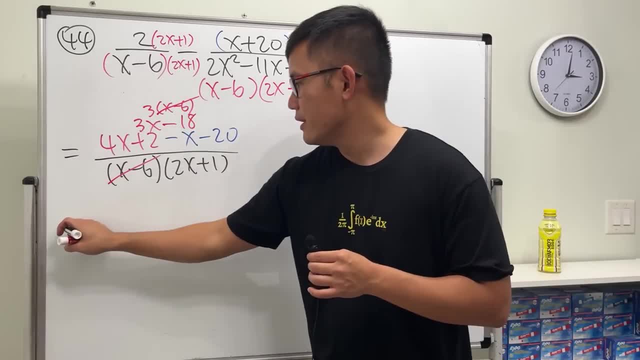 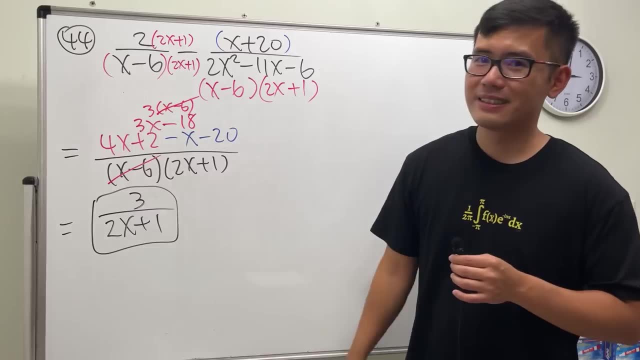 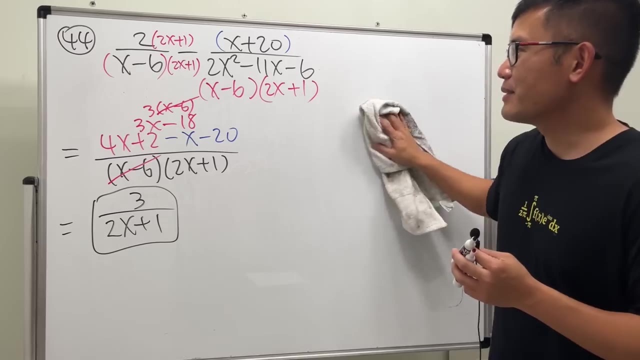 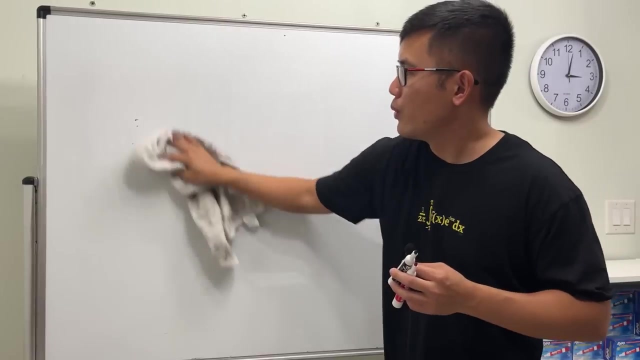 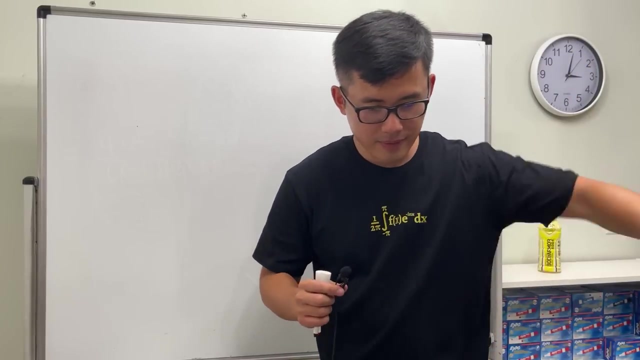 out the x minus 6.. so finally, guess what? we have one, two, three, three over two x plus one done. okay, i don't know why i think i just like to write it big. i don't know why i was hoping that i can finish this in like four hours. why did i think that? 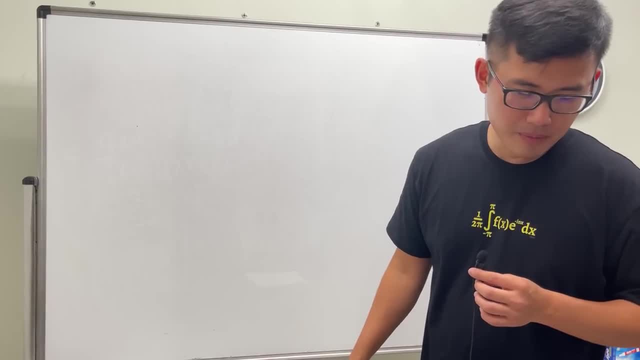 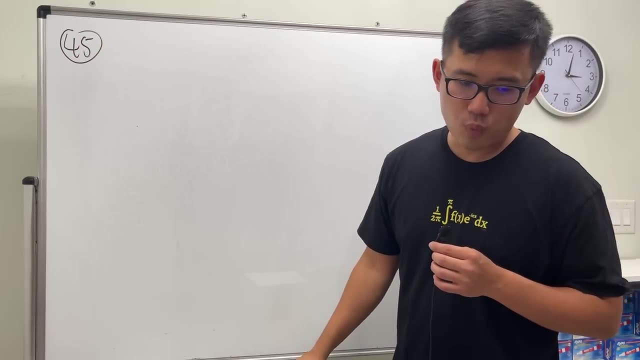 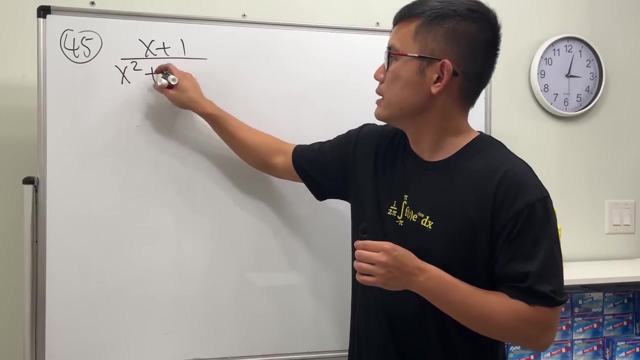 anyway, if you have the software i use, just remember to do the math. we have similar action. so we have x and y, and we have x squared plus x minus 20 over 4, and we have x squared plus x, and we have x squared plus x minus 20, and then Red and 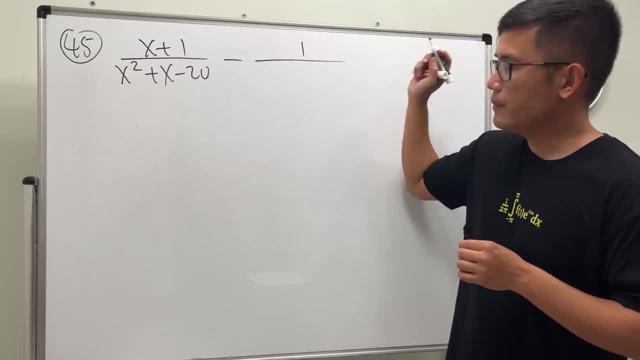 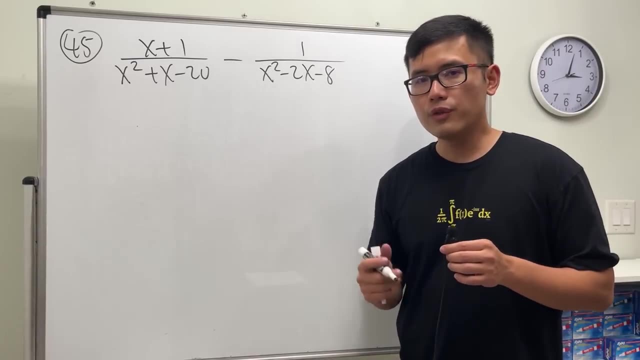 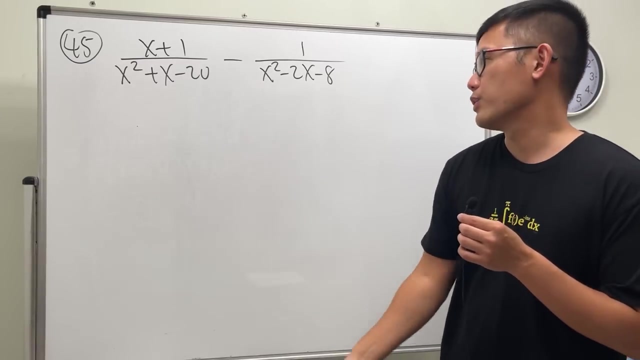 then minus one over, and here we have x squared minus 2x minus 8, right? so we're gonna look for the lowest common multiple for the denominator. so let's go ahead and factor things out. and because we don't know if they have any common factor or not, so right here, if we factor, we get. 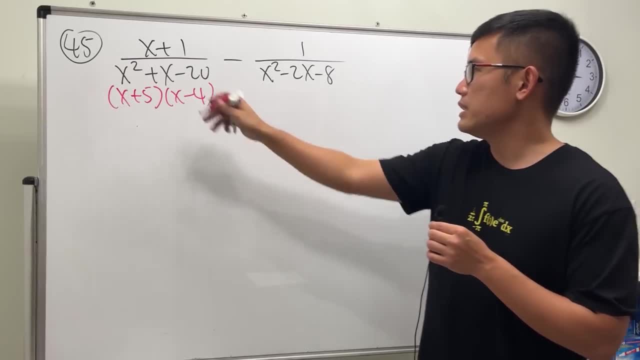 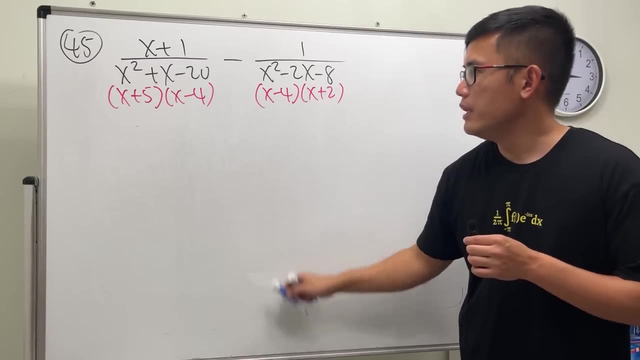 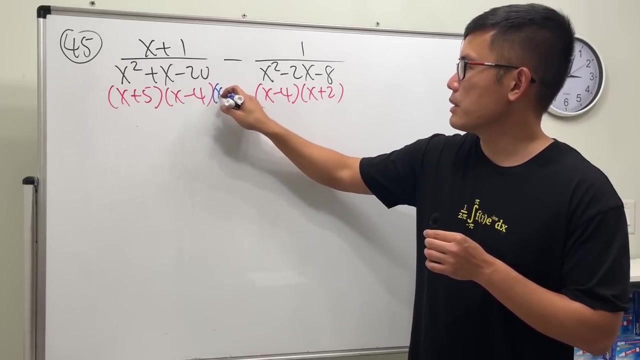 x plus 5 times x minus 4. yeah, and then for this we get x minus 4 times x plus 2. good, now the x plus 4 is in common. so for the first fraction, well, we need this, namely x plus 2, so we also come to the. 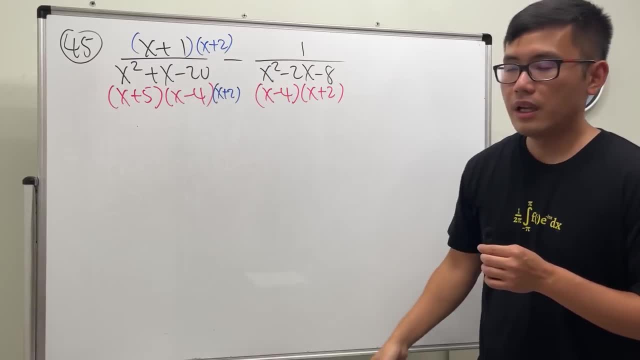 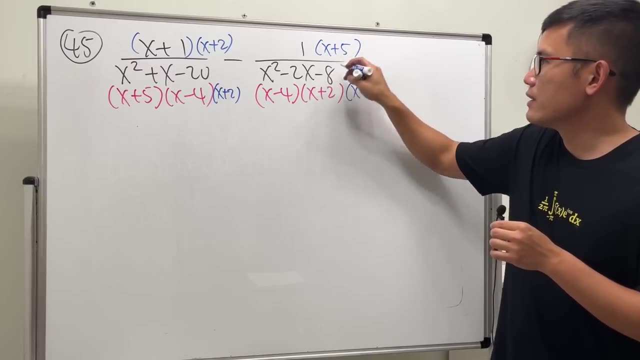 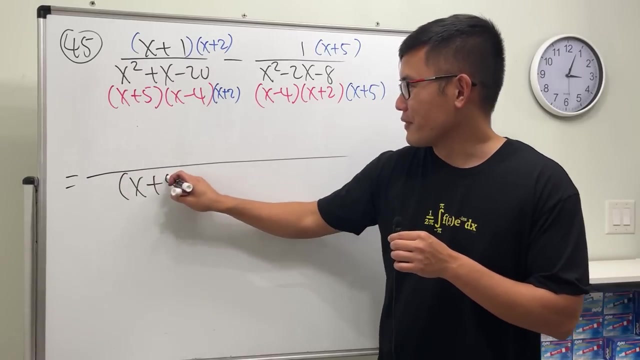 top and multiply x plus 2, and then for the second fraction we need the x plus 5. so let's multiply here x plus 5 and then x plus 5, all right, so we get x plus 5 times x minus 4 and then x plus 2. 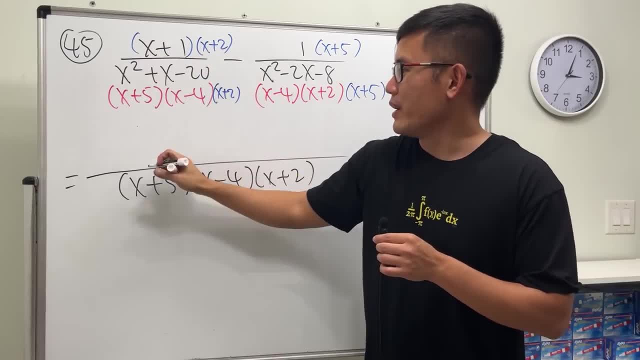 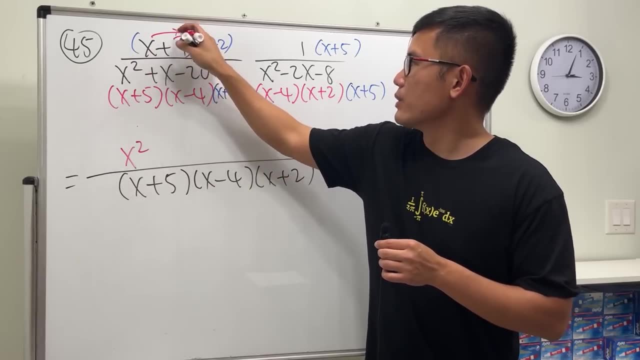 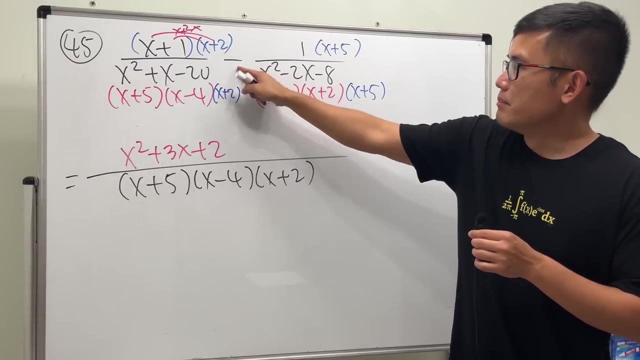 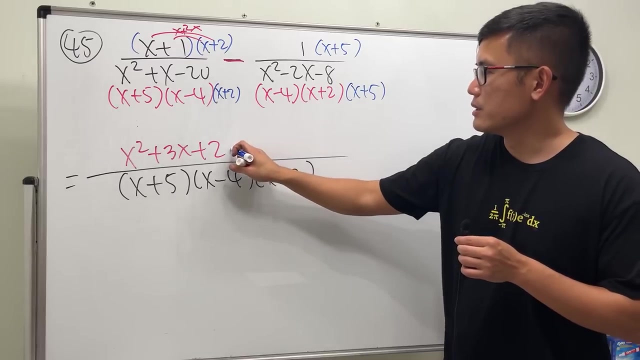 okay, multiply this out x square, and then this is 2x, and then another x, so all together is 3x, and then lastly, plus 2, yeah, and then this is the minus, and so it's minus. so we have a. let me just write it down like this to make it more clear: so it's a minus, and then the. 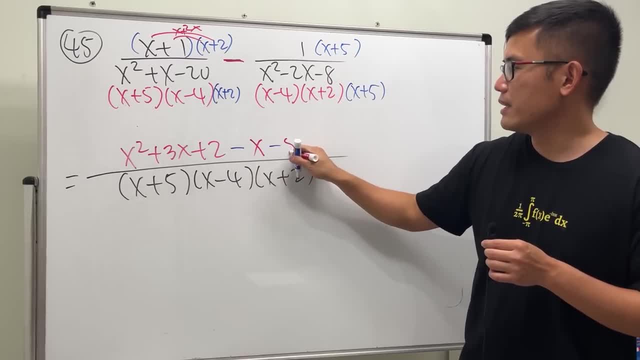 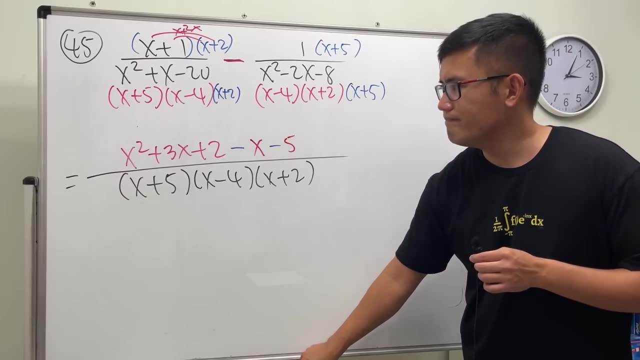 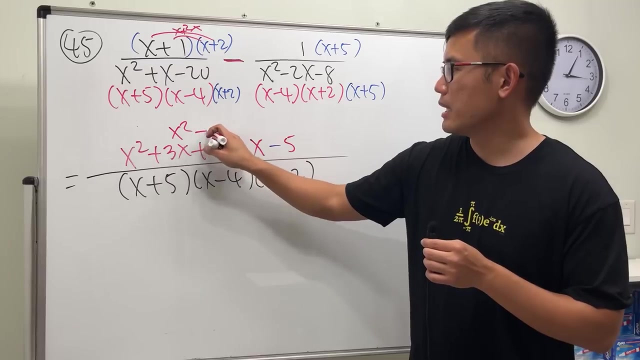 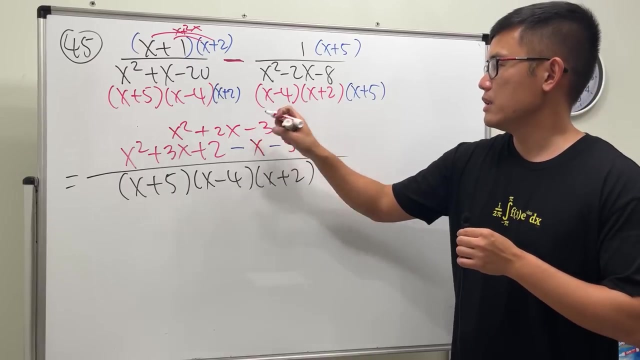 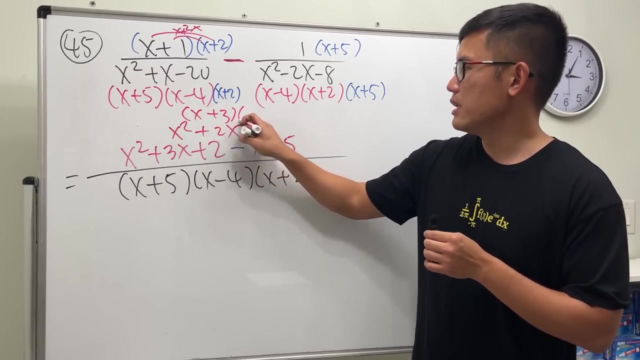 x and then minus 5. all right, so just like that. okay, so can we cancel out anything? okay, let's see, on the top we get x, square this, and that is plus 2x and then minus 3. yeah, and then if we factor we get x plus 3, x minus 1. unfortunately, we cannot factor anything. 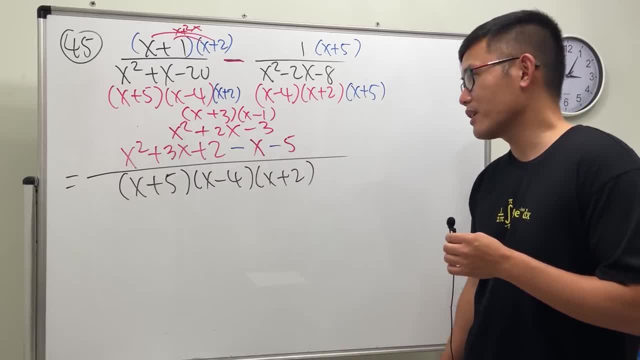 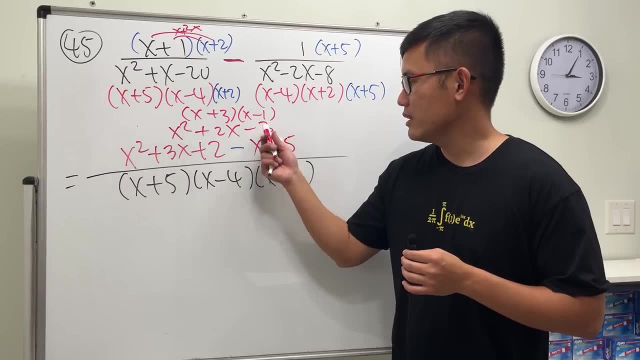 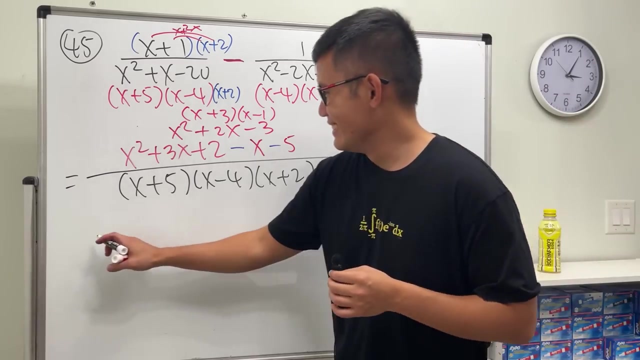 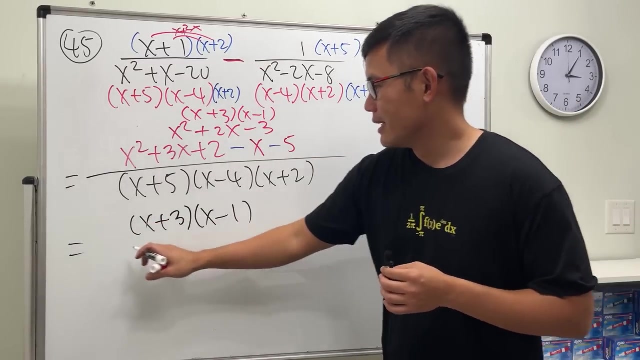 but do you guys notice? well, unfortunately, we cannot cancel anything, but do you guys notice what's so so cool about this? one, two, three, four, five, yeah, oh, i come up with this question. by the way, yeah, they came up with this question. and then, um, yeah, how did i come up? how was this? i started with the answer that i wanted and i worked backwards. 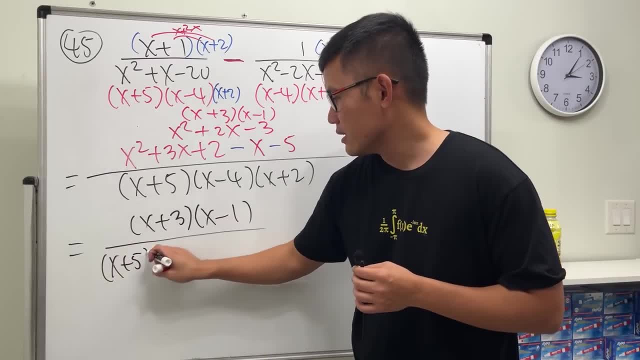 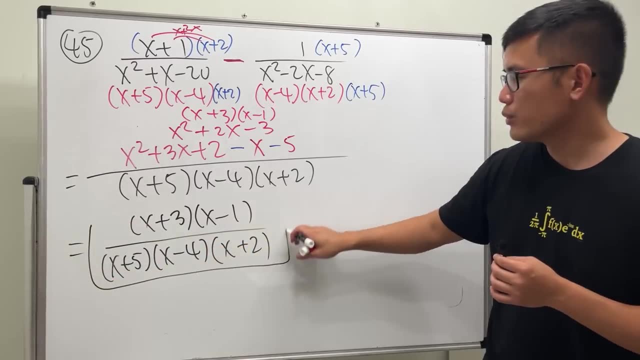 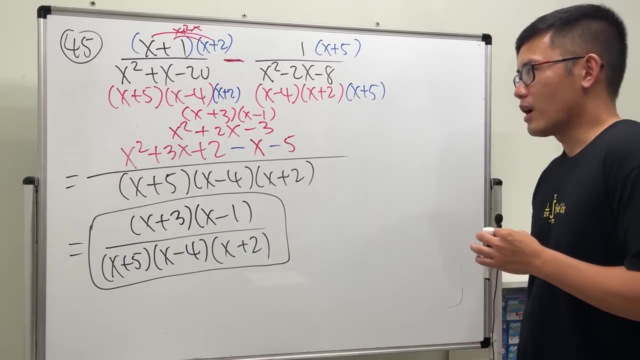 yeah, anyway, though, we'll just leave it like that. sometimes, if nothing can cancel, just leave it. yeah, and this one is pre-f. tamam, even though you are pre-calculated, even though you are pre-calculated, even though you are pre-calculated, then you can use this phone to make the graph for the rational function. 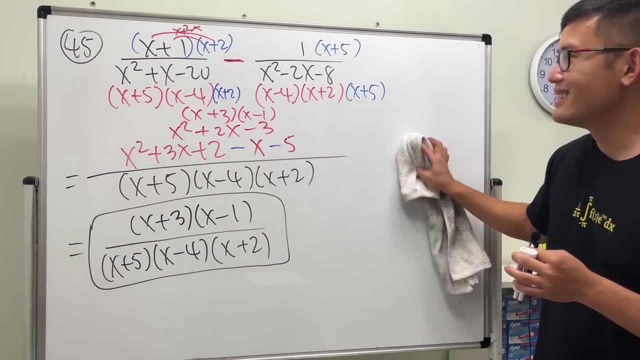 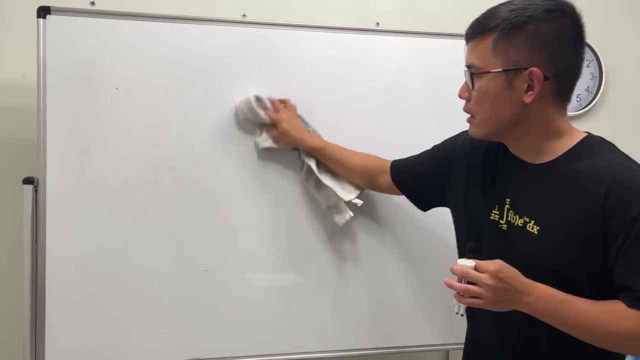 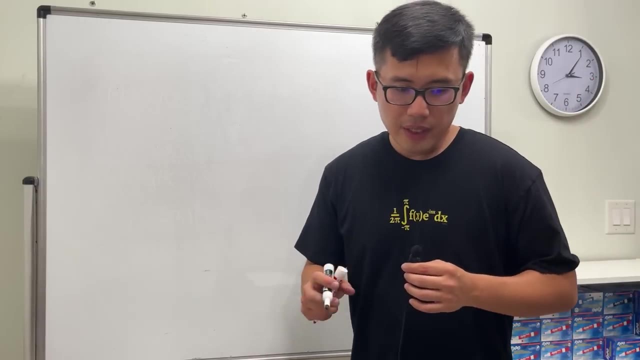 and all that, but anyway, this is number 45. okay, so just take the hanging one, take the number 46, just leave it. number 46. now you'll see the question right there. now you'll see the question right there. see, the question looks kind of weird. it's like why did i just cancel them out at the beginning? 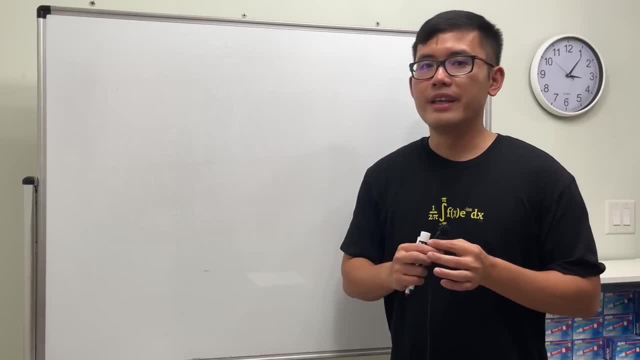 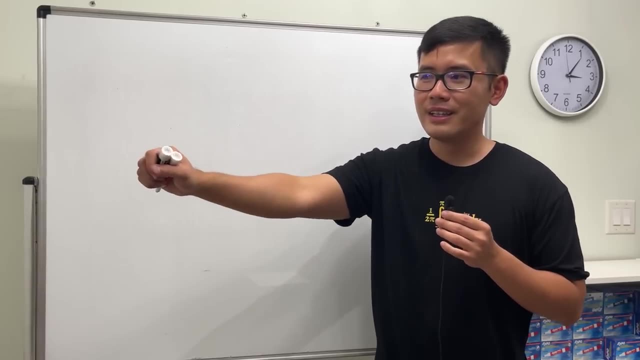 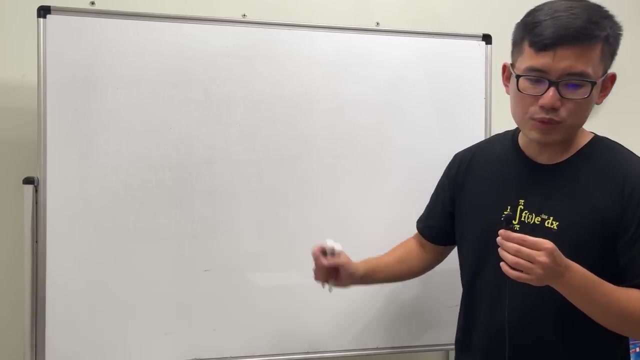 the reason is because these expressions they come from when we do the so-called derivative with product rule. sometimes you just have to write things down and then you get like a long expression and just have to be really observative. okay, this we can cancel, this we can combine that's. 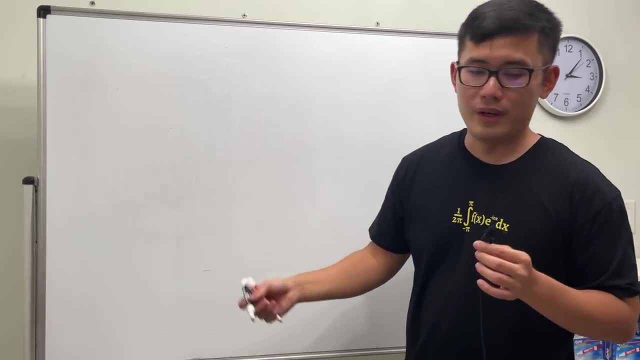 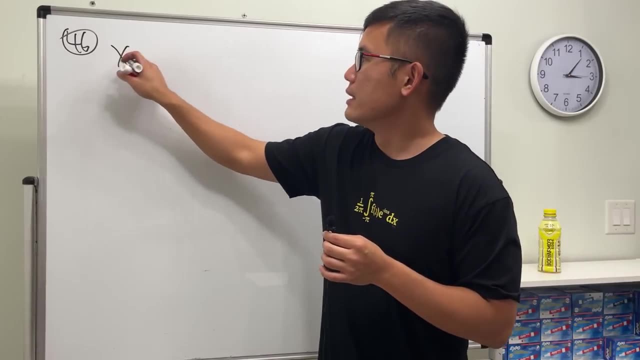 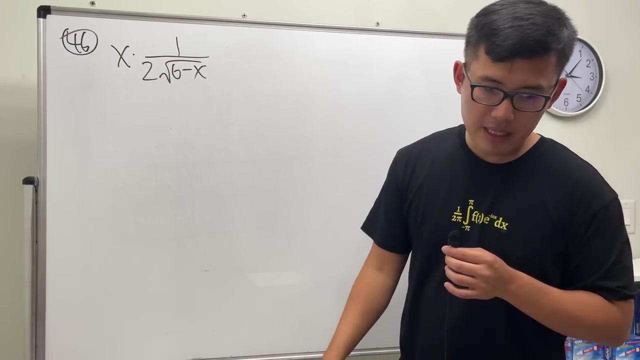 why so? i didn't make this up out of nowhere. that's what i'm trying to say. number 46: we have x times 1 over 2, square root of 6 minus x, and then times negative 2x. yeah, this is what i mean. 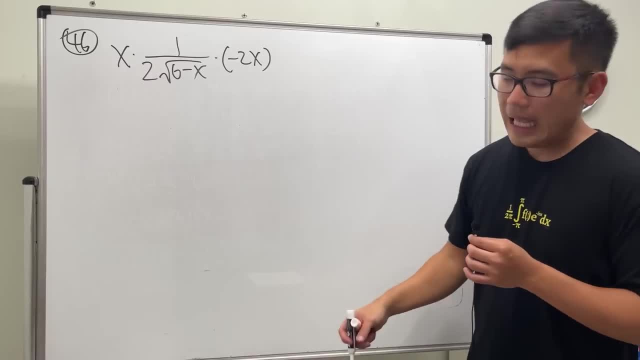 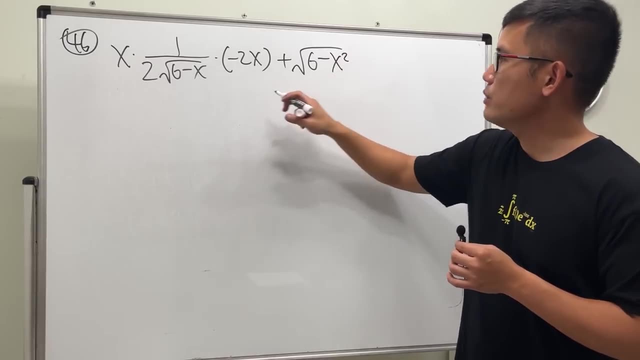 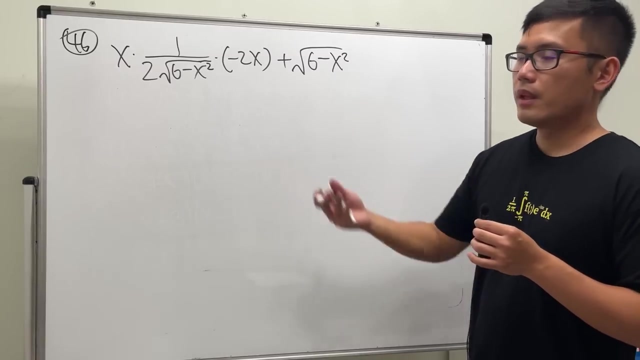 seriously, that's the expression. and then after that we have the plus square root of 6 minus x squared. oh sorry, this right here is supposed to be x squared. okay, so this is number 46. so let's see what we can do. first, if you look at this part, they are multiplying, of course. 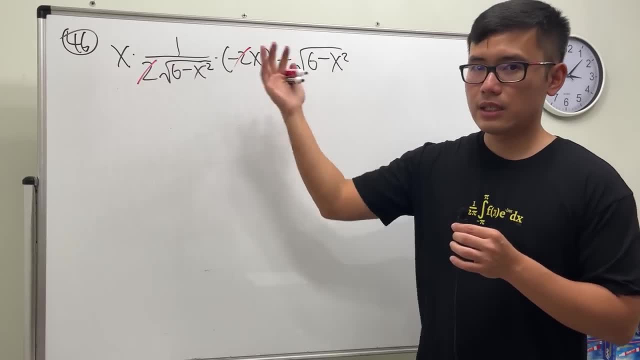 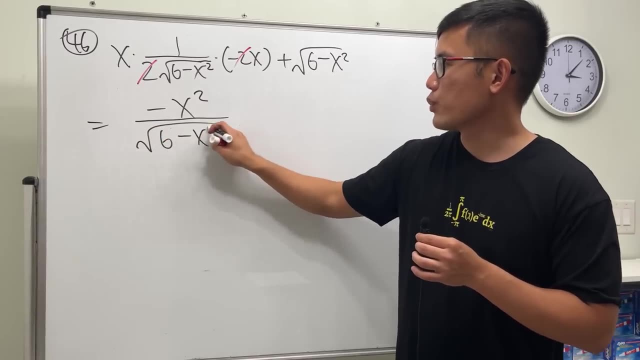 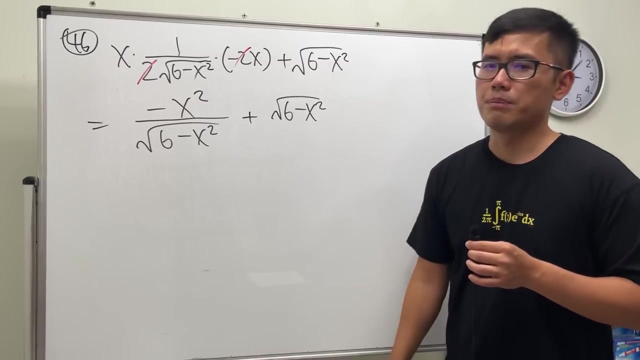 these two and that two can cancel x times negative x. that goes to the numerator. so we have negative x squared over square root of 6 minus x squared, and then for this one it's just square root of 6 minus x squared. how can we combine them? well, this is kind of the same over one, so let's just go ahead and multiply. 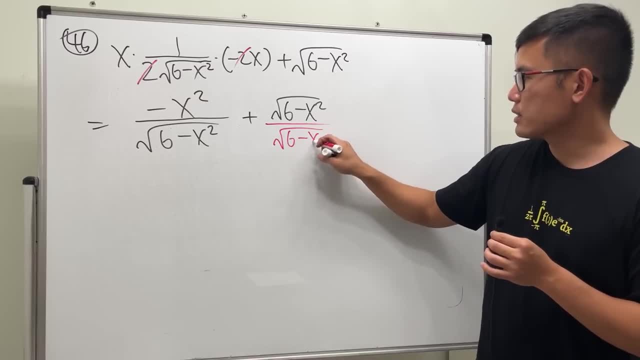 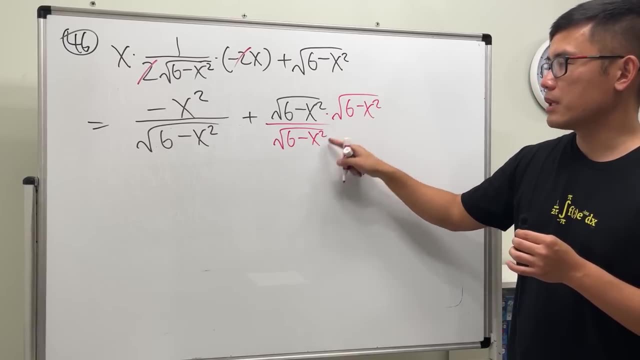 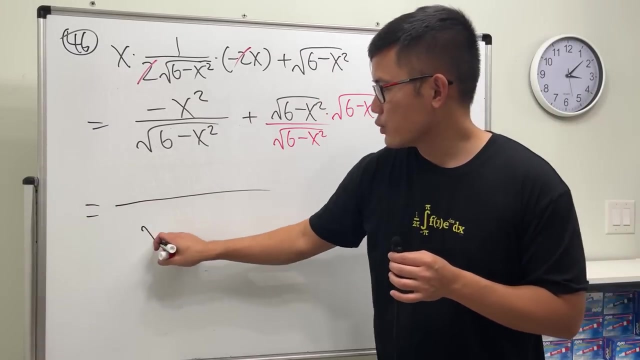 the denominator by square root of 6 minus x squared, and then yeah, so we can match with that and then do the same thing here. so multiply the top and bottom by what we need here- now they have the same denominator- and we will get what square root of 6 minus x squared. this is still negative. 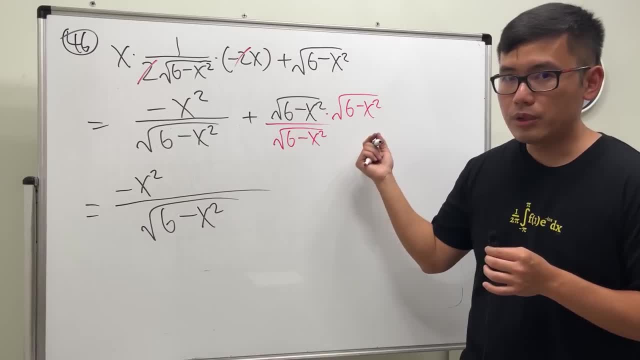 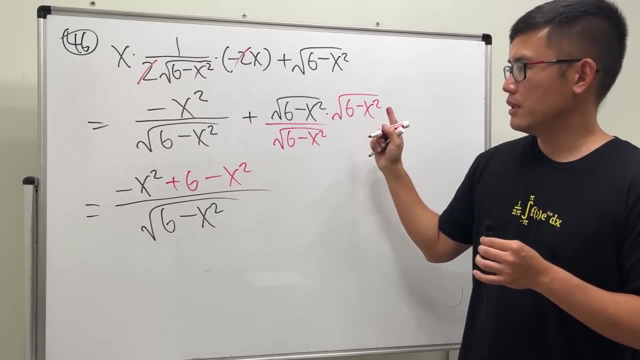 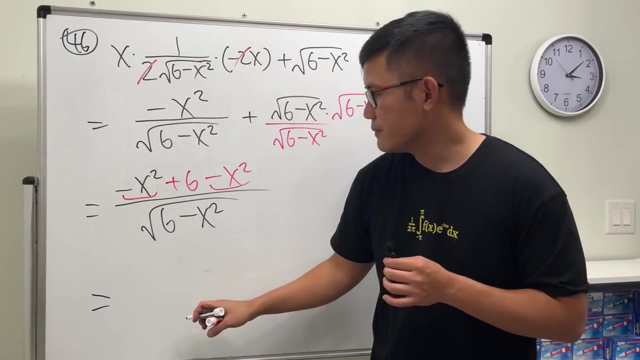 x squared. but then if you see this and that they multiply, you just get inside which is going to be plus 6 minus x squared. yeah, yeah. and then what can we do next? this and that can be combined, so we have. and now here's the thing: if the original expression we have, like minus x squared and x. 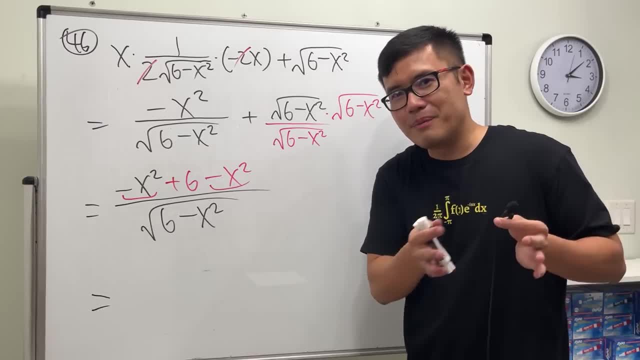 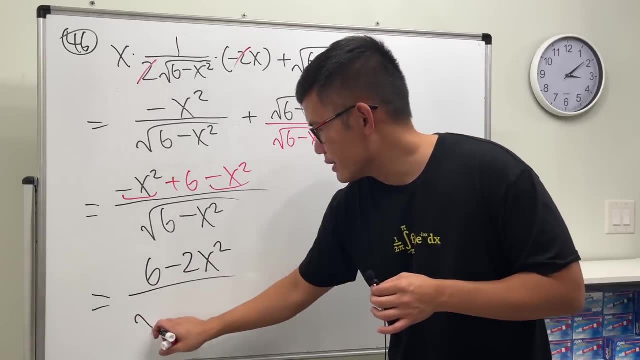 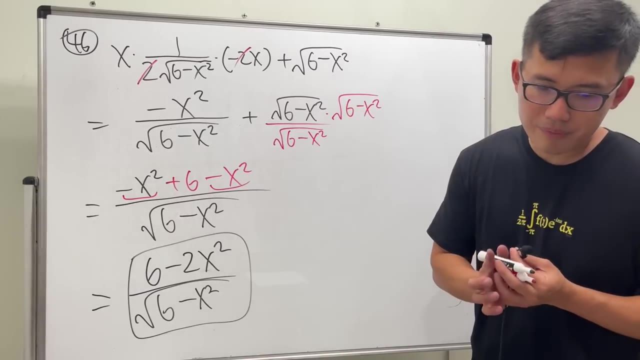 squared. at the end, i like to keep it the same order, so i'm going to write it as 6 minus 2 x squared over square root of 6 minus x squared. yeah, so i think this is how people usually like to write it as well, so that's the reason, and that's it, though. so even though we have the square, 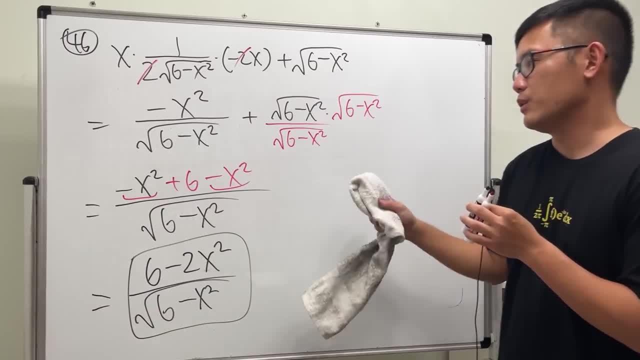 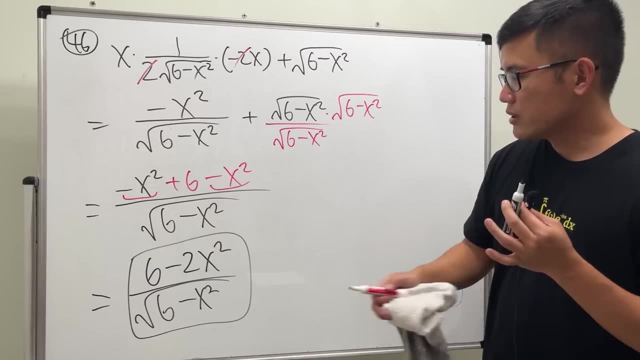 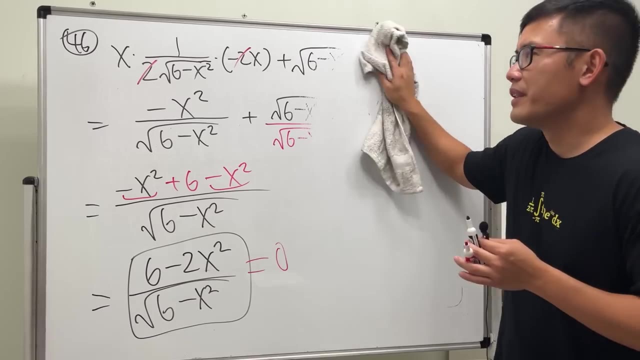 root expressions, we can still get a common denominator and we can still combine them together. and the reason that we want to combine this and that together is later on, we want to solve equation. we set this equal to zero and solve for x. yeah, but we are just focusing on how to do the simplification. that's why 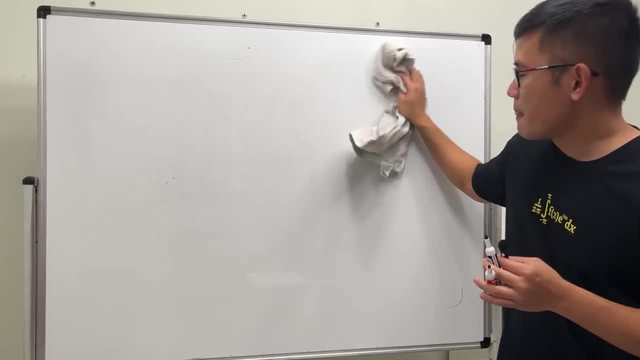 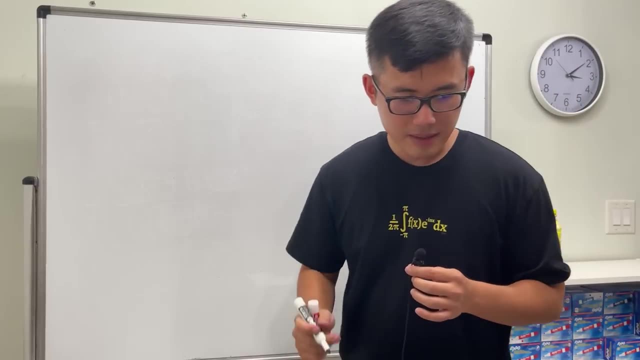 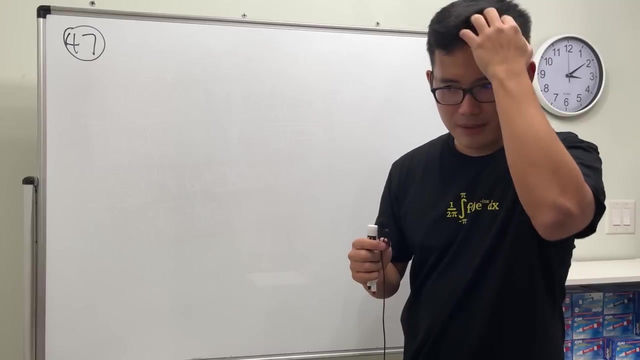 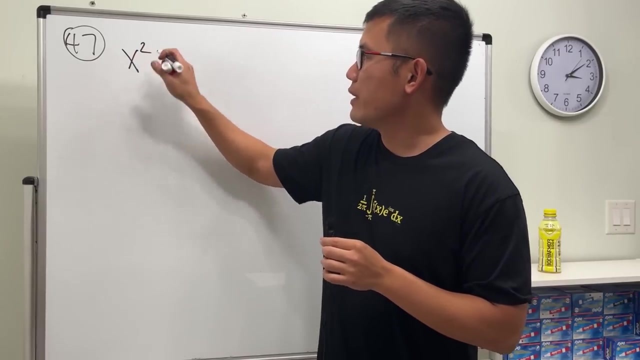 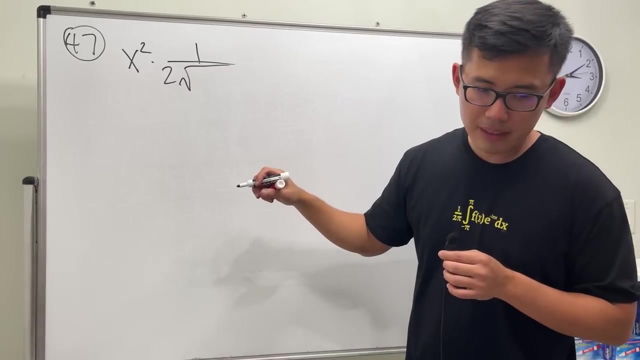 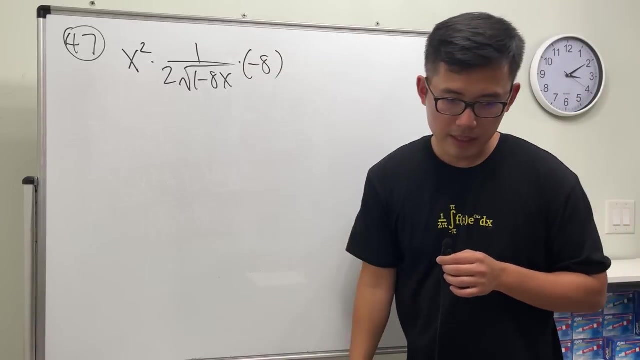 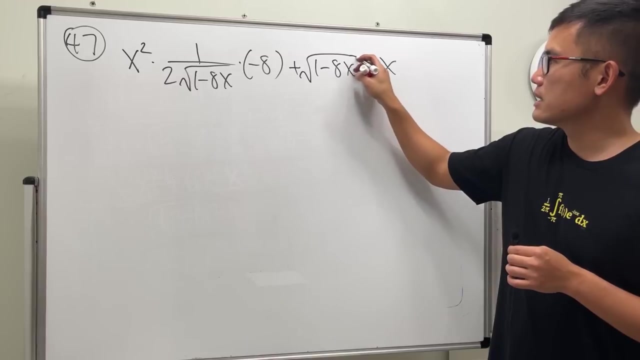 i'm not continuing anything else. number 47: does my hair look okay? all right anyway. number 47: we have x square and then, times 1 over 2, square root of 1 minus 8x times negative 8, and then plus square root of 1 minus 8x times 2x. yeah, so this is the question. 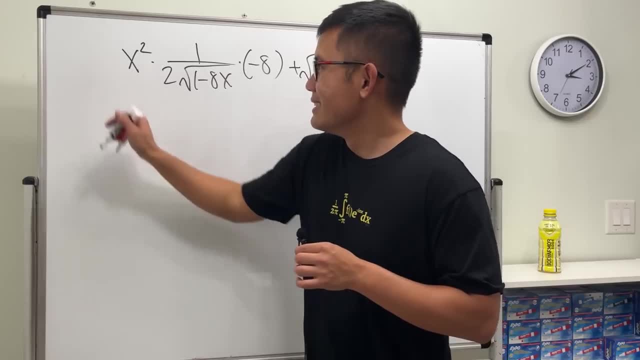 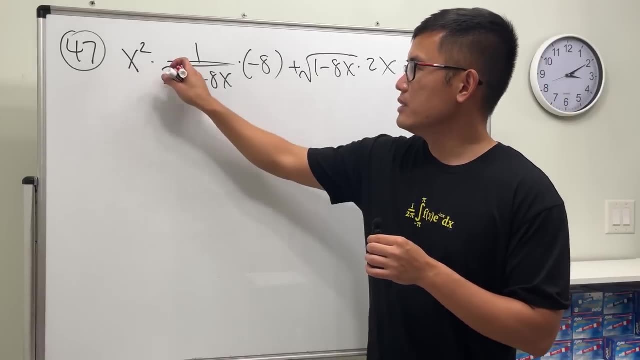 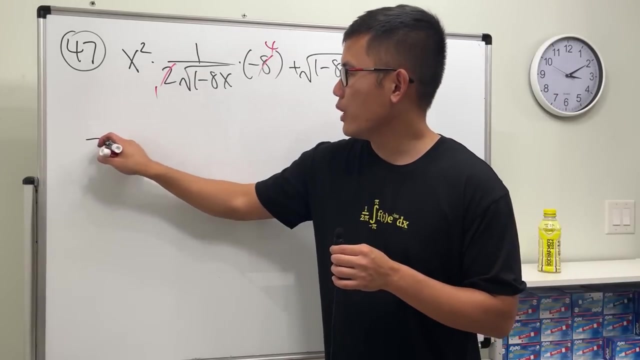 my handwriting is getting sloppy, huh, i'm sorry. 47 and then that. all right, let's just go ahead and simplify this one and then this 4. yeah, so we can reduce that. yeah, that's a follow. so the first part: we will have negative 4x squared. 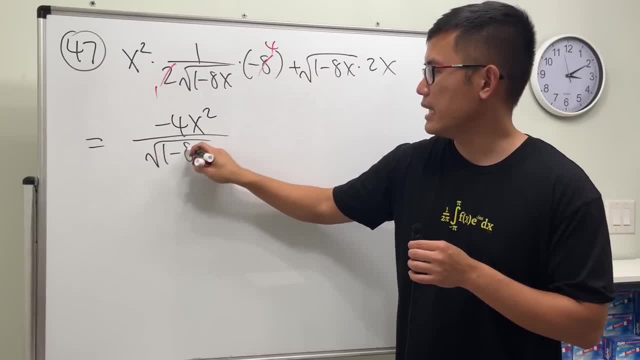 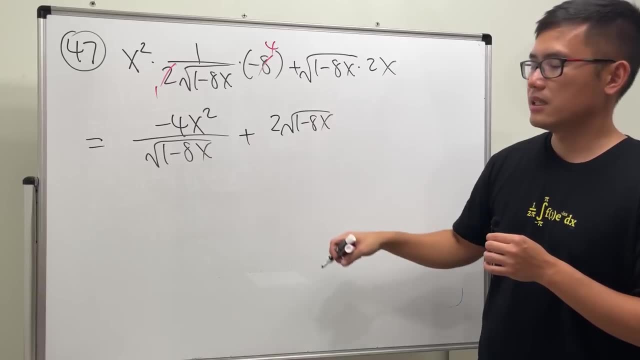 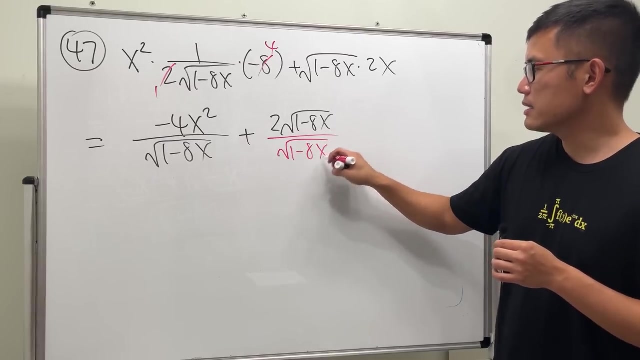 over this for the denominator, so square root of 1 minus 8x. and then for this one we just write this: 2, square root of 1 minus 8x, and we just need this denominator here. so let's multiply the bottom by square root of 1 minus 8x, and then let's also do the same on the top. 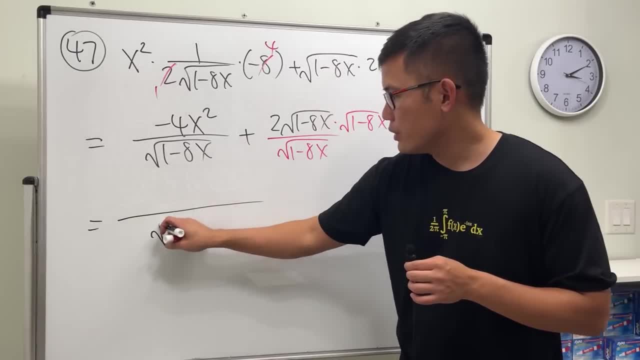 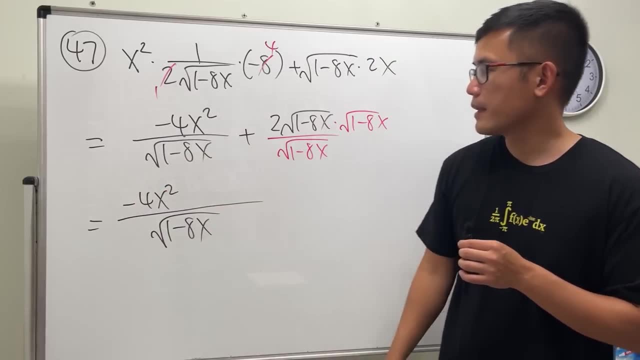 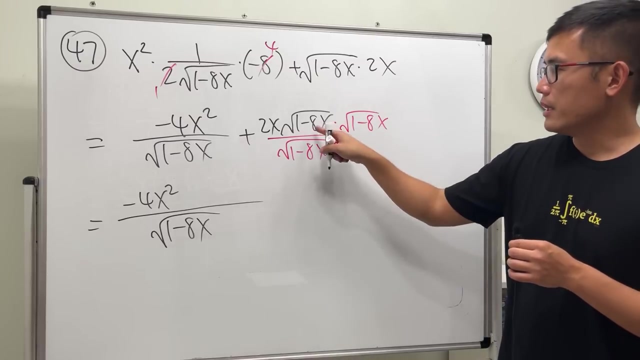 now we can put them together. this is just square root. we keep the same denominator, 1 minus 8x, and then this is negative 4x squared. this times that, sorry, it's 2x. sorry, okay, this time that's just 1 minus 8x. right, the square root doesn't matter anymore. 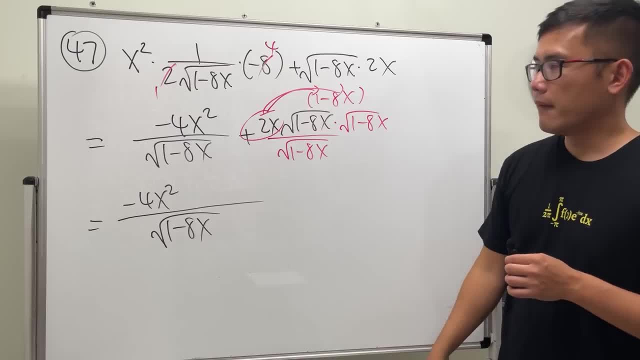 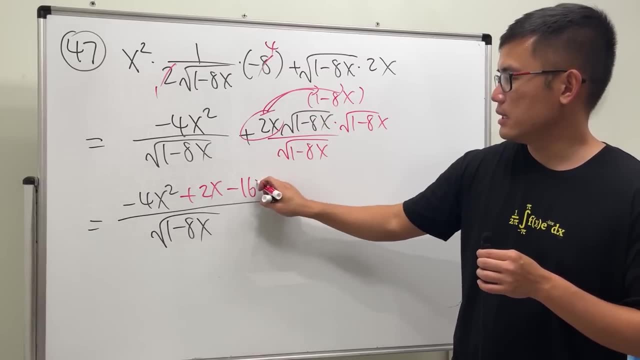 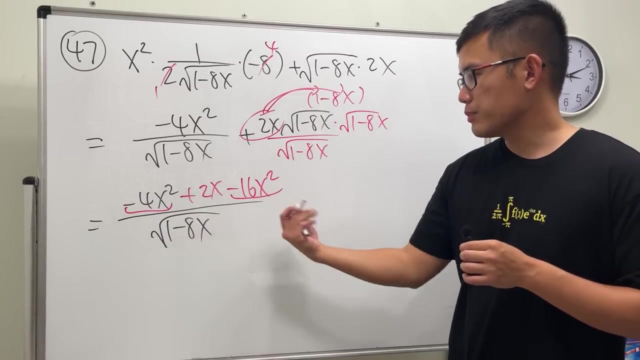 and it will take this, multiply in, so we get plus 2x and then minus 16 x squared, yeah, and then, finally, we'll just combine this and that together and let's just put the x squared at the end. so, ladies and gentlemen, we have 2x. 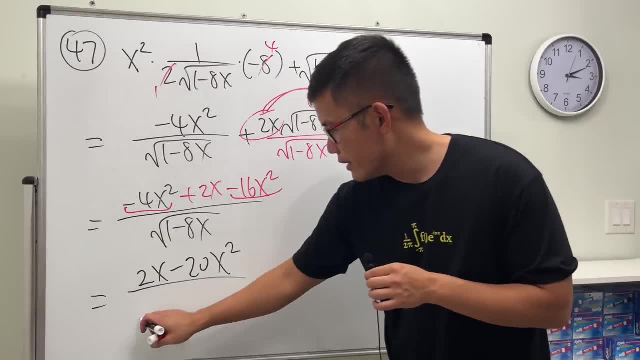 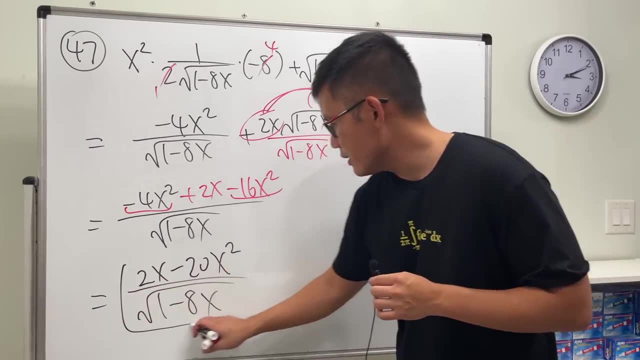 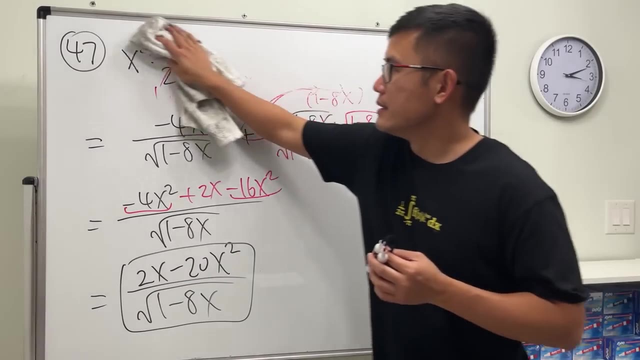 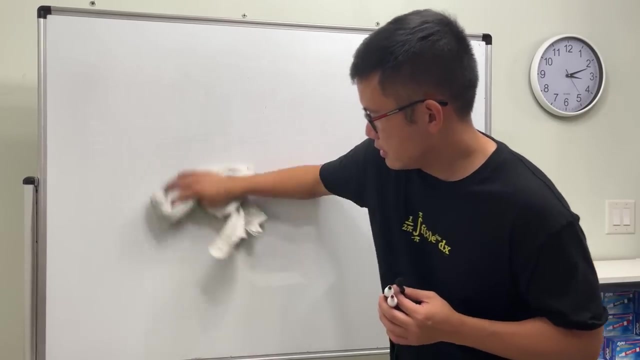 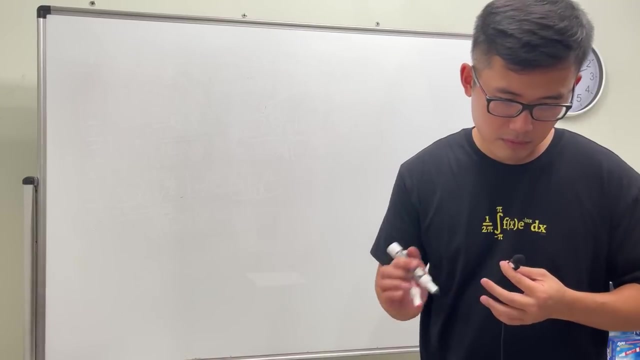 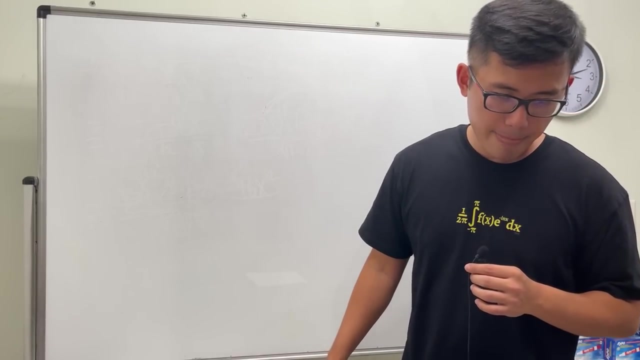 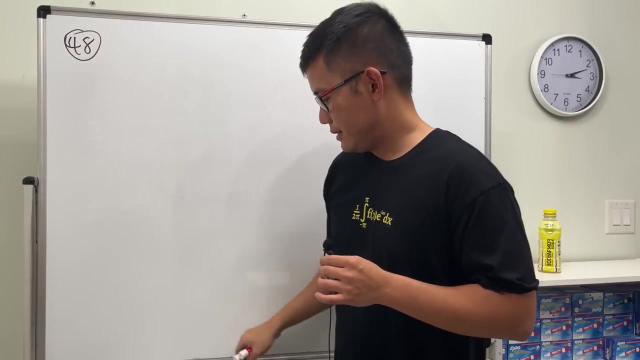 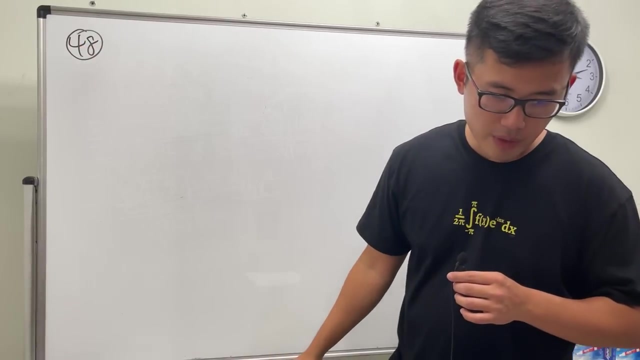 minus 20 x, square over square root of 1 minus x. yeah, pretty good, as I will say, and we are done all right, number 48. now the question may look like study. I don't know how this. let's just look at the question. I'm 48, so here we have 3 over 4 X to the 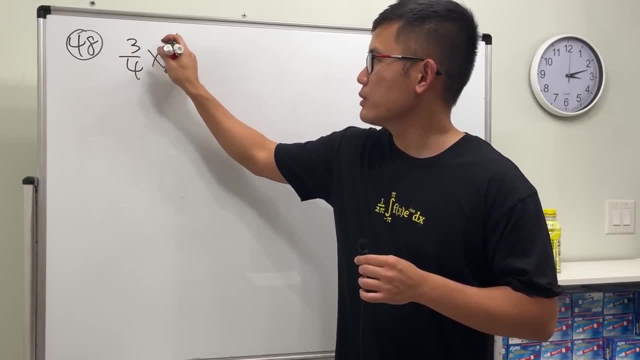 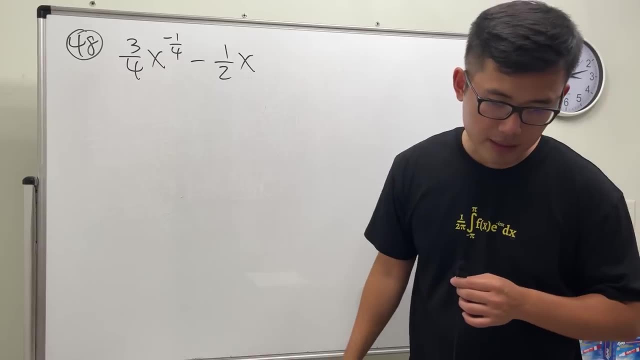 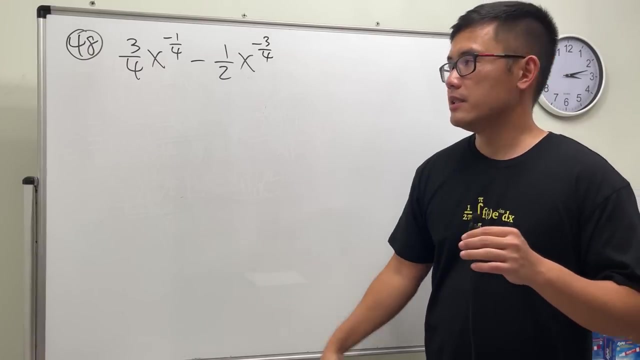 negative 1 over 4th power. so we have a negative exponent here, and then after that we have minus 1 over 2, and then this is X to the negative 3 over 4 power. first thing, first negative exponent. we can just bring it X, right. 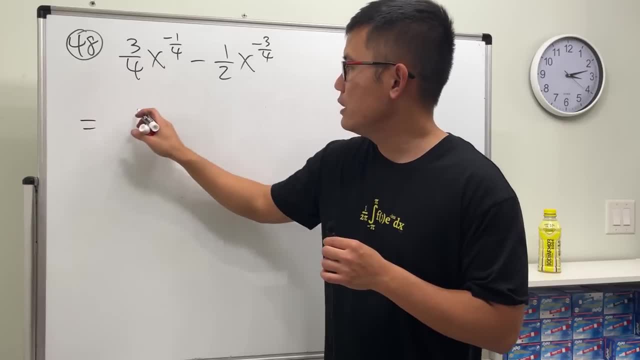 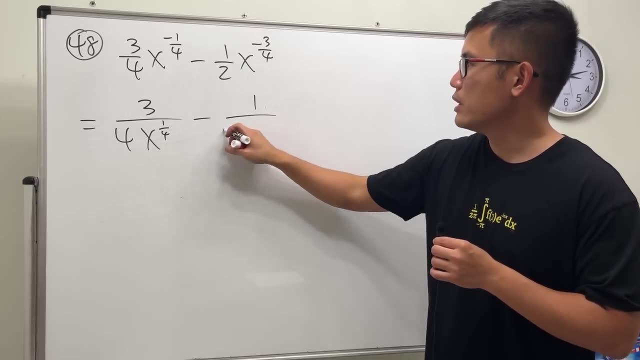 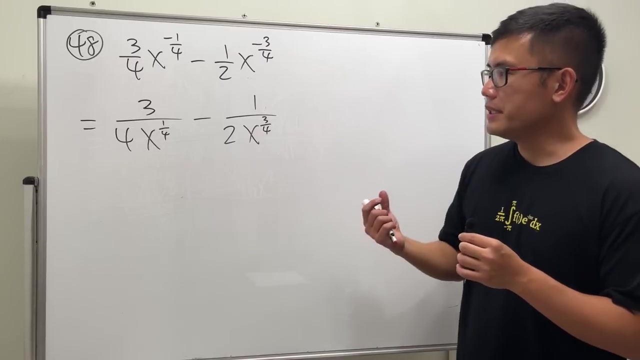 this term down to the denominator. so the first one is really 3 over 4, X to the 1 over 4 power. and then, minus the other one, 1 over 2. X to the positive is 3 over 4 power. right, so now, what exactly do we need? all well, firstly, let's. 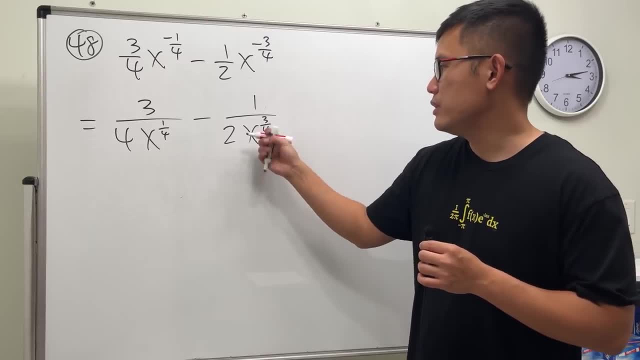 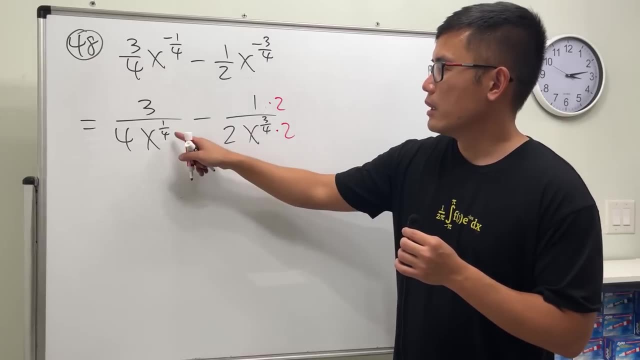 look at the number this is worth. this is 2. we need to right here. so multiply by 2, multiply by 2 so we can get a 4. now let's look at the X to the power. which one's bigger? it's 3 over 4, of course. so what do we? 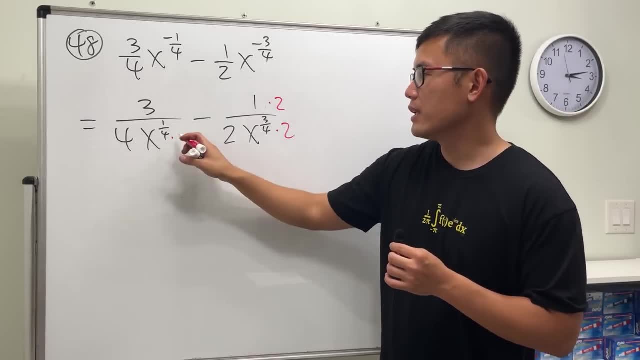 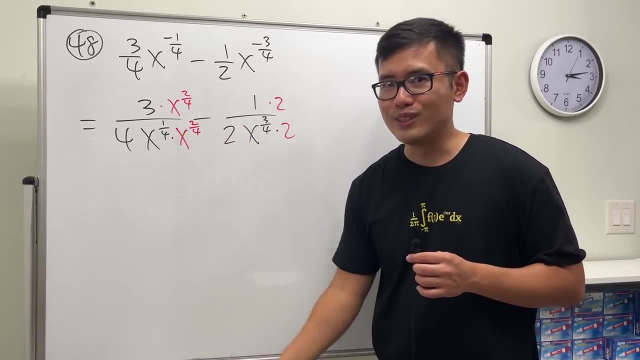 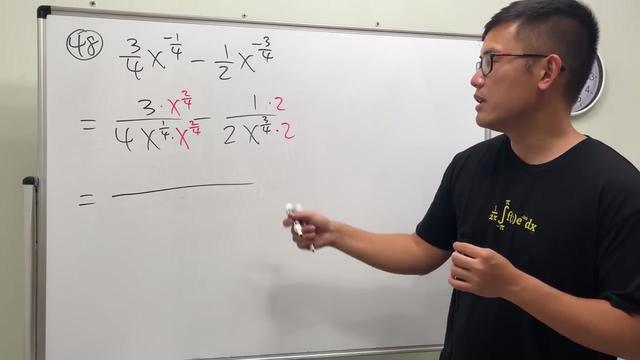 need. we need to have 2 over 4. so let's write yes, X to the 2 over 4 and then X x to the two over four. i know two over four is the same as one half, but let's do that later. but this way we can see that they will both have the same denominator, namely four, and then x. 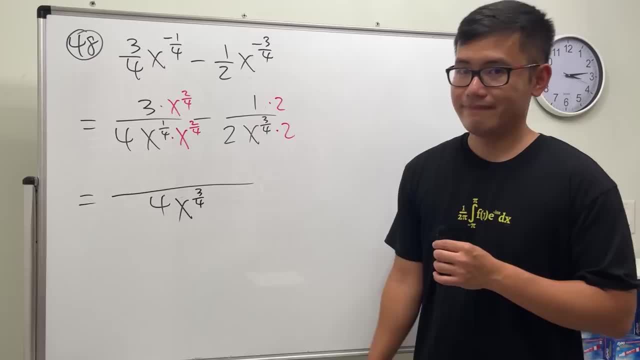 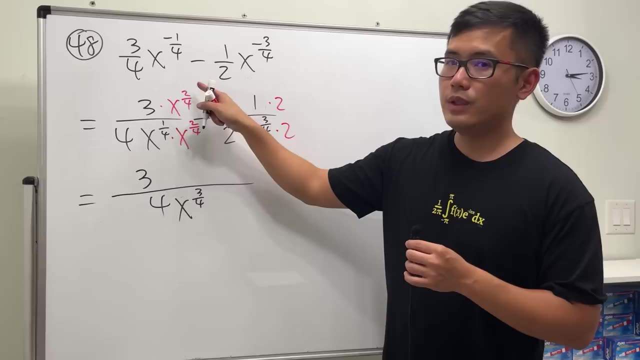 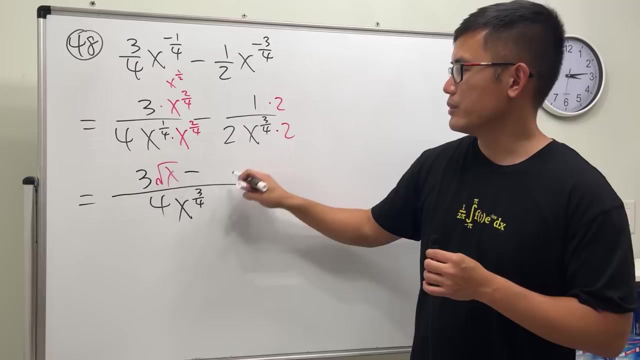 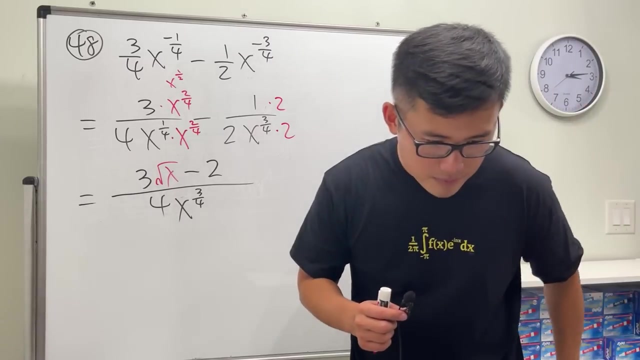 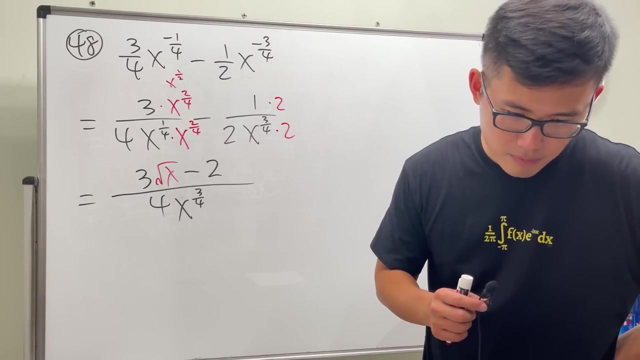 and then three over fourth power. all right, now, here we have three, and then this is just x to the one over two power, isn't it? namely square root of x and then minus two. yeah, so now it. yeah, well, i'm going to fix my answer key. this is a much better answer. 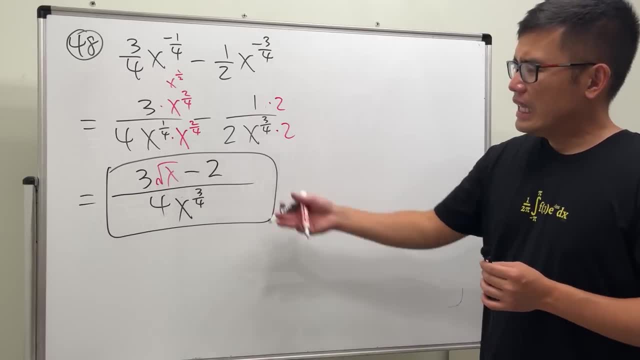 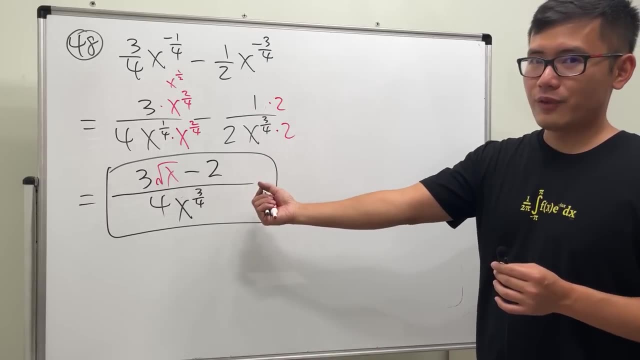 yeah, that's, that's it. that's it, that's it. yeah, you don't need to multiply the count you get. if you want, you'll leave that to you. okay, again, the reason that we combine the fractions is because we are going to set this to be zero and then so for x, so now we can just put the top to be. 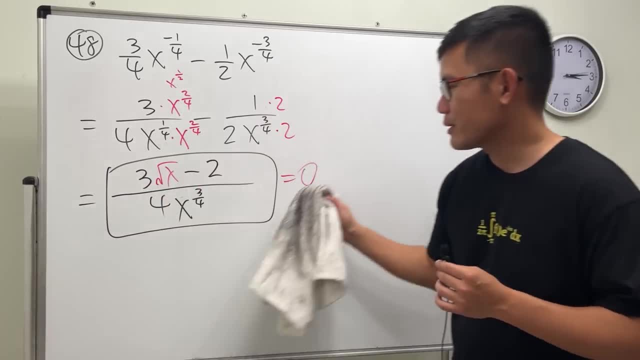 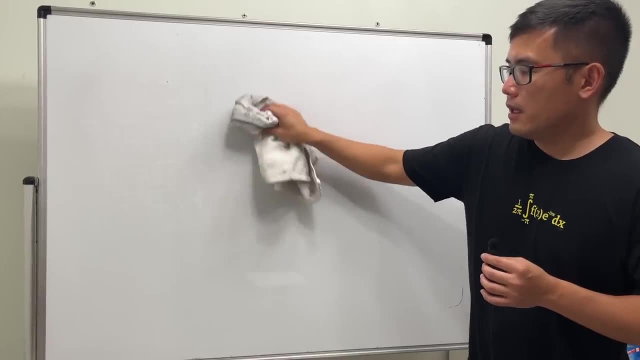 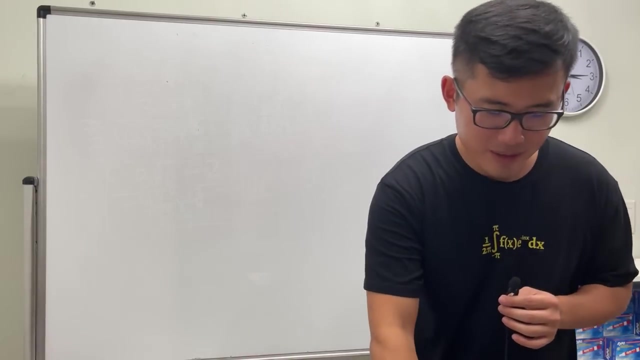 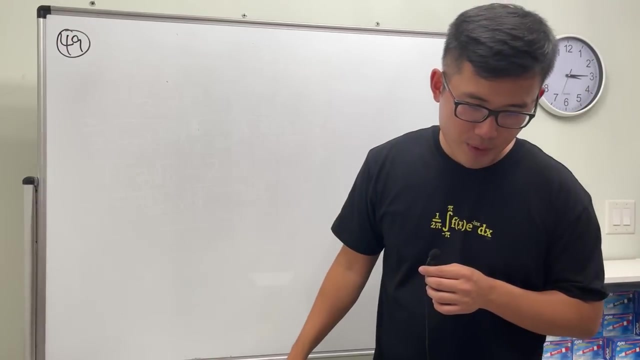 zero and we can go from there, yeah, but i'm not going to do that because, again, just we're just looking for the simplification and all those things it-and so we let's say 2009, number 49. a long expression is coming, so let's see number 49. we have x to the two-third power. 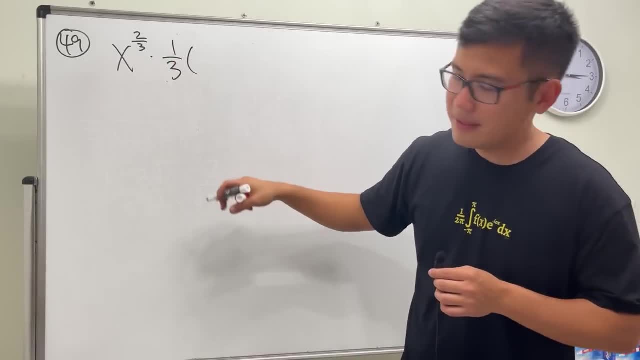 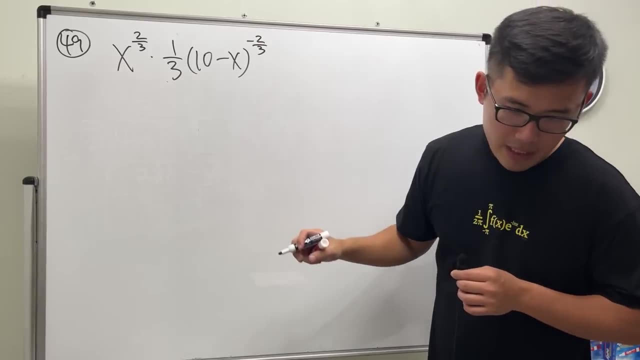 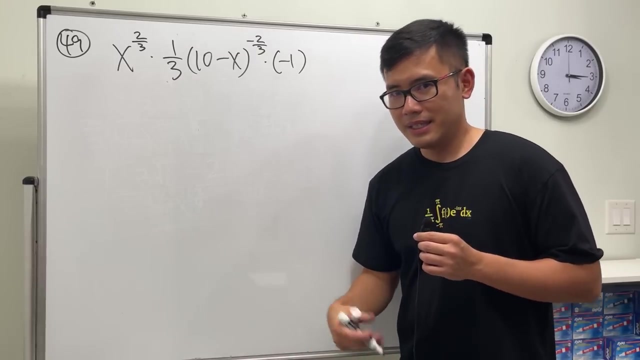 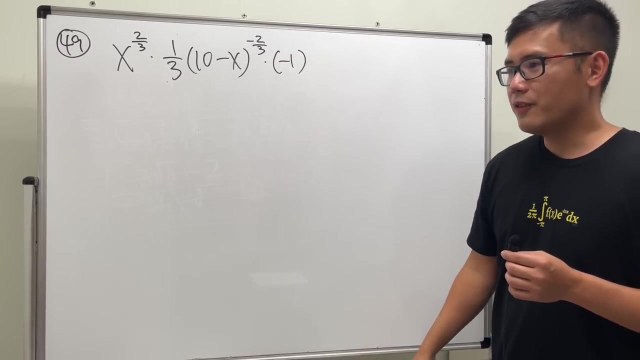 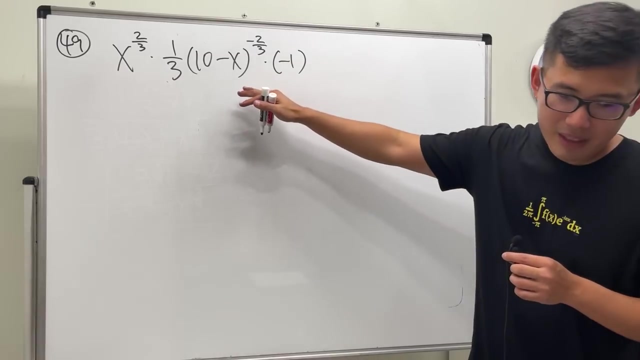 times one third, and then 10 minus x raise to the negative two-third power times, negative one. i didn't make this well, i did come with this question, but they came from different. they came from derivative by power. they come, they came from. they came from derivative by product rule and also the chain rule. but anyway though, and then after that we have: 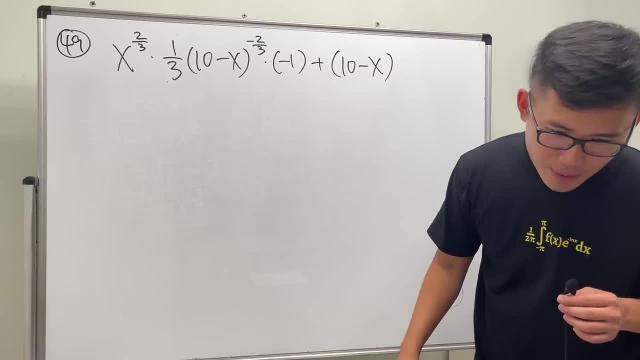 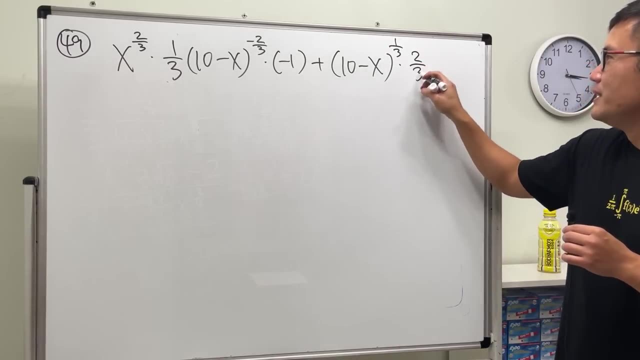 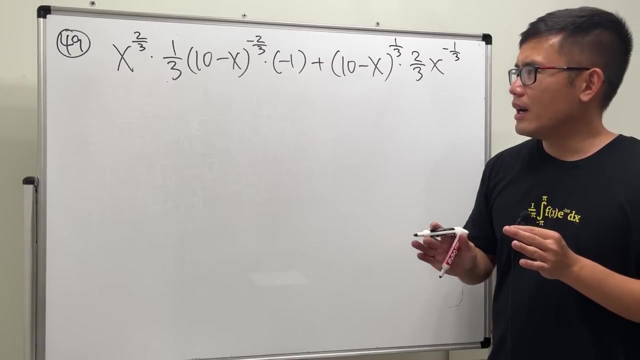 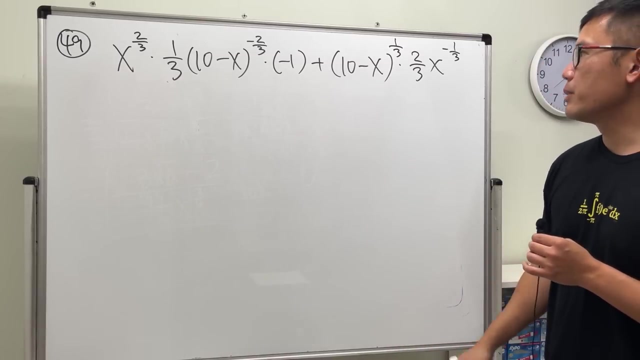 plus 10 minus x and raised to the one third power times two over three x to the negative one third power. yeah, so i would recommend you guys to do the following: so once you write this down right, we see negative exponents. let's just take care of that, and then let's just see. 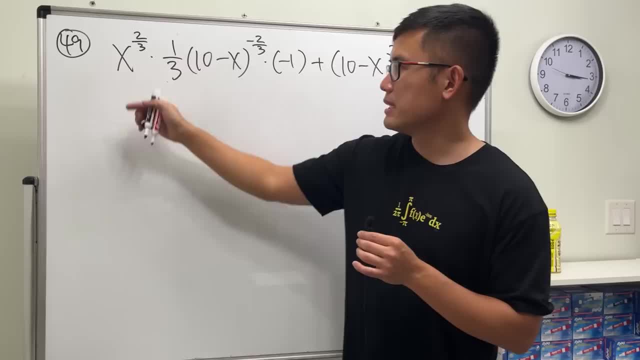 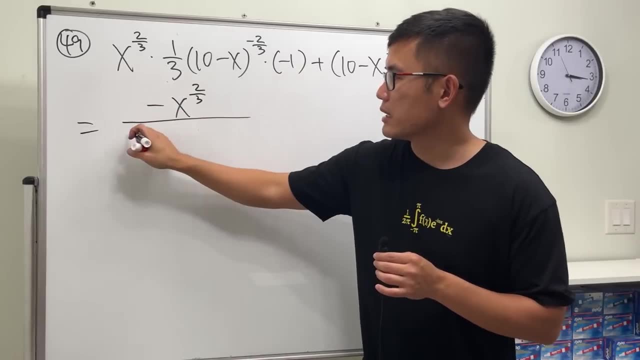 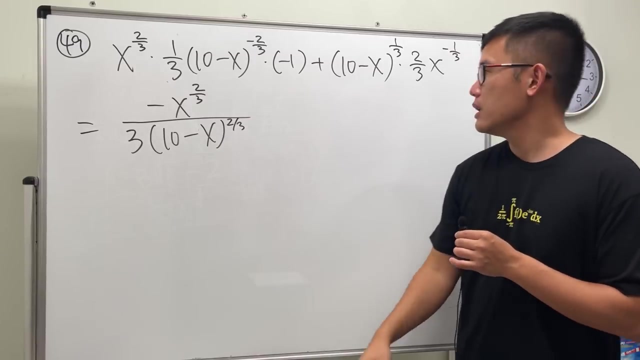 so this right here can go down to the denominator and we have a negative times that. so the first part is going to be negative: x to the two third power over three on the bottom. likewise 10 minus x to the positive two third power now. so that's the first part and for the second part we add: 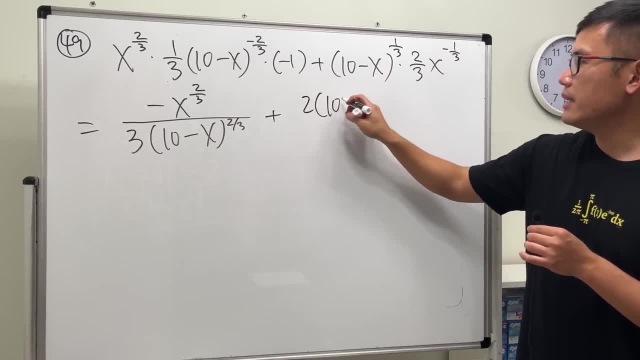 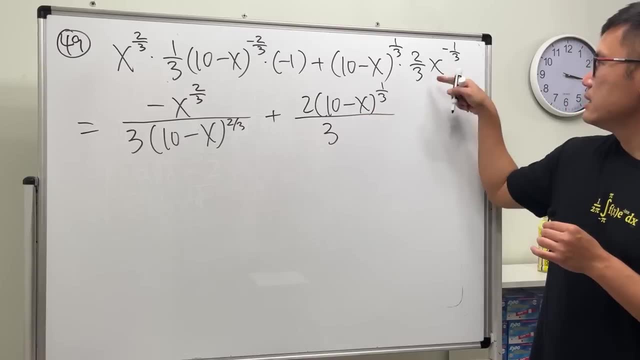 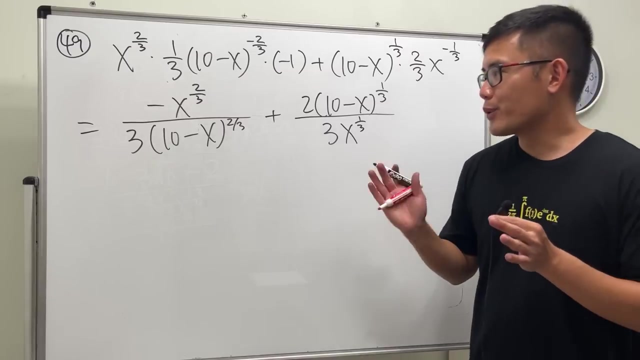 two on the top. well, two and that on the top, so two times 10 minus x to the one third power and the three on the bottom, and this is x to the positive one third power on the bottom. so that's what we have now. the question is, how do we combine them? huh, well, let's see. 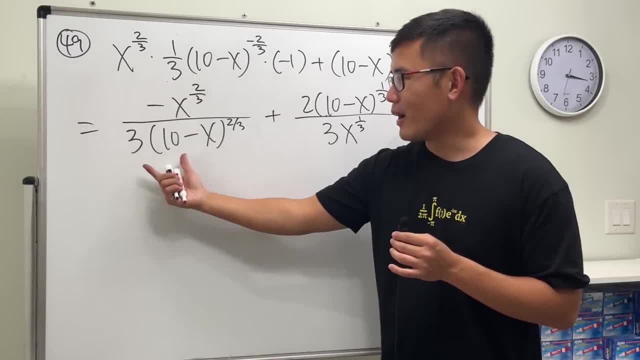 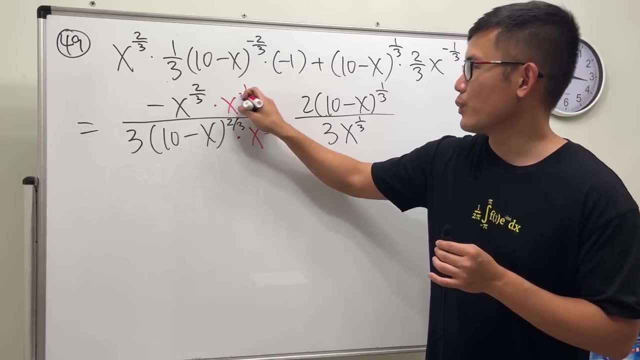 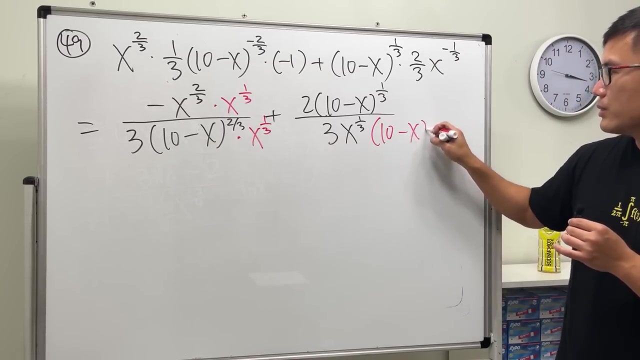 they both have three. that's good. this part does not have x to one third power, so we need that. so multiply by x to the one third and multiply by x to the one third. this part does not have that, so i'm going to multiply by 10 minus x to the two-third on the bottom, and then, of course, 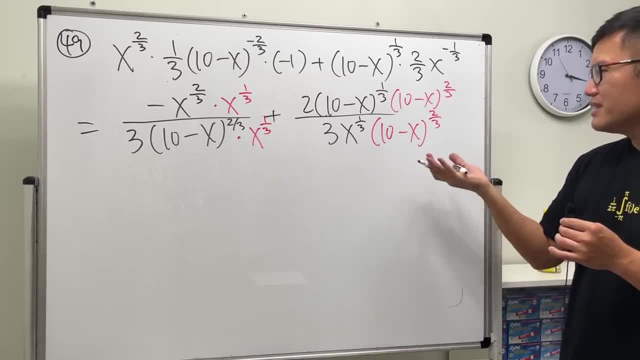 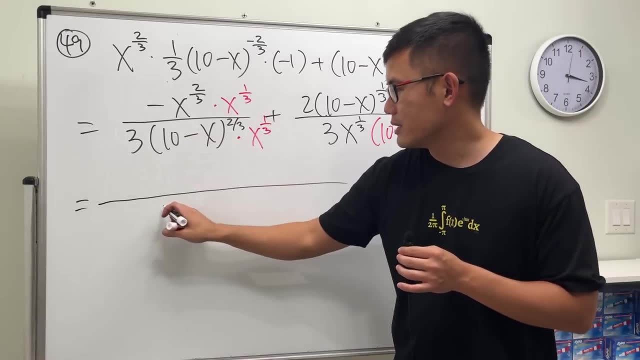 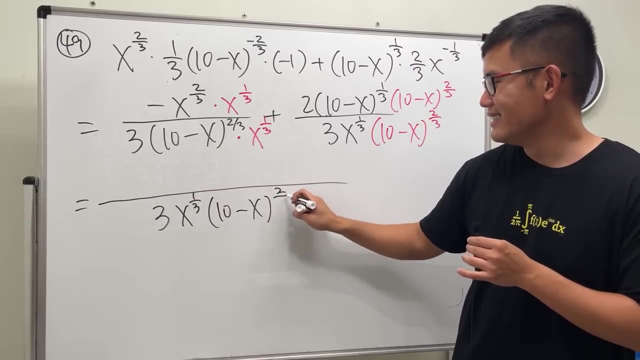 do the same on the top and you can see that it's actually working. working out really well, because after they have the same denominator, which is just three, and then x to the one-third and also 10 minus x to the two-third, okay, this is just what, two-third plus one-third. 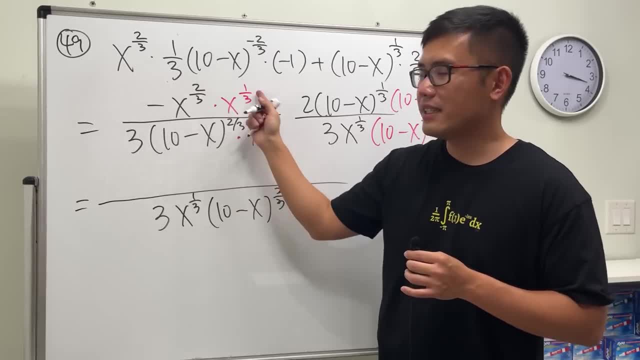 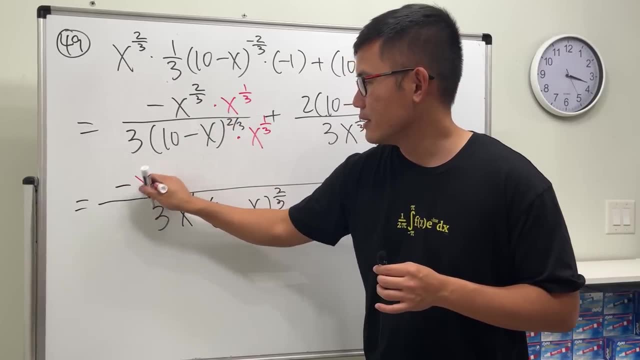 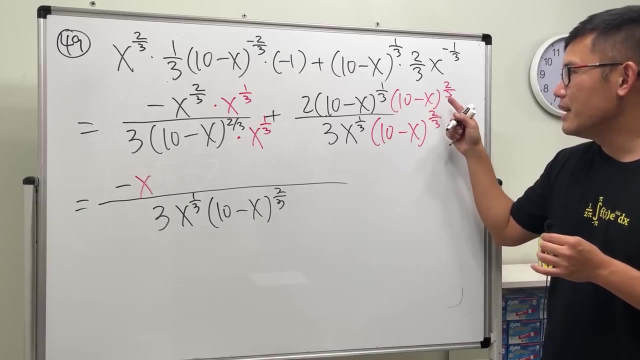 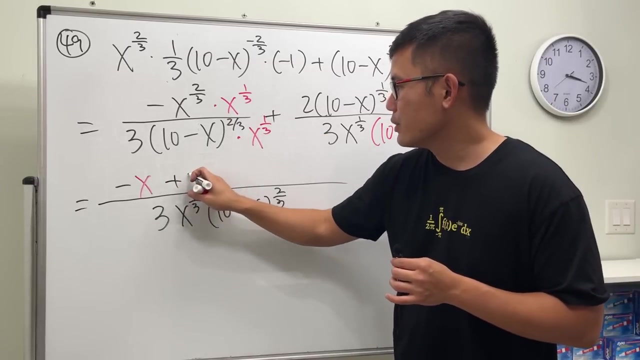 is just three-third, which is just one, right. we multiply them, we add the exponents, so it's just x, to the first power, namely negative x. so we have negative x, all right now. this times that one-third times, one-third power, and that power again, they add up to be just one. so it's just this. so right here, we just have to add two times. 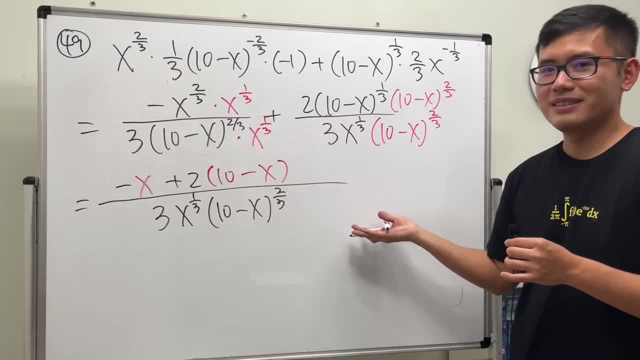 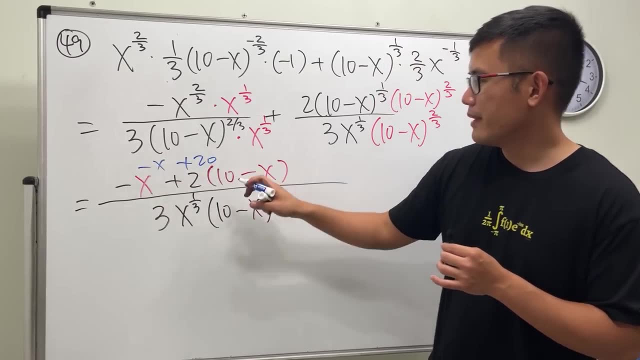 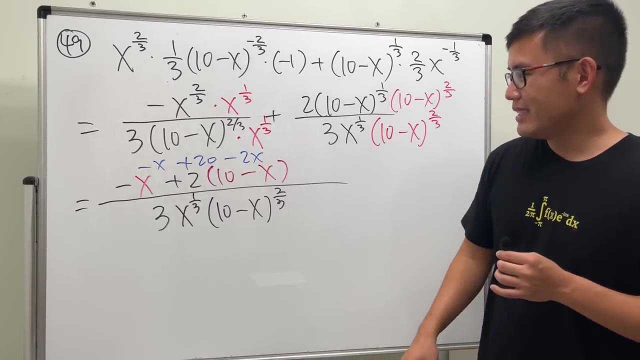 10 minus x. yeah, it works out so nicely, right, okay? and then let's see, this is just negative x, and then plus 20 and then minus 2x. that's about all. cannot really do anything else, so i will just write it down: 20 goes first, minus 3x. 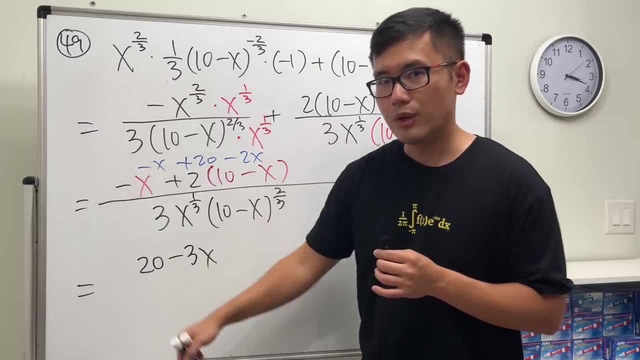 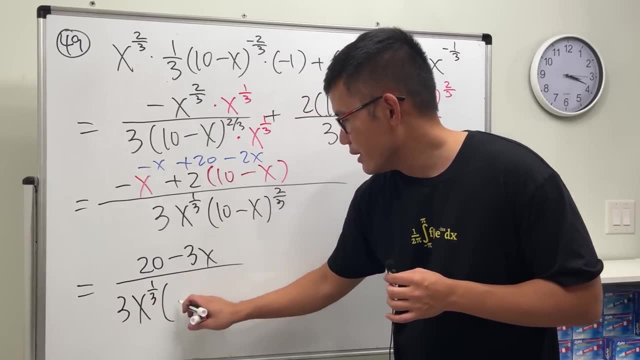 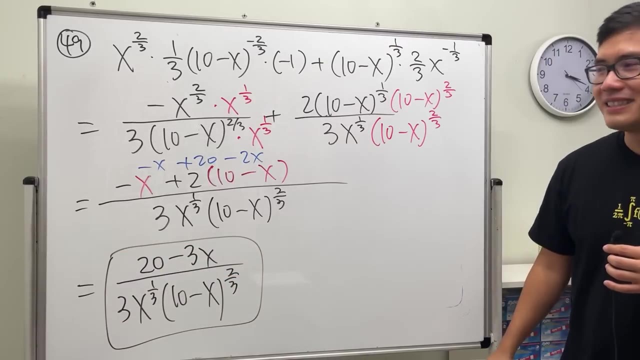 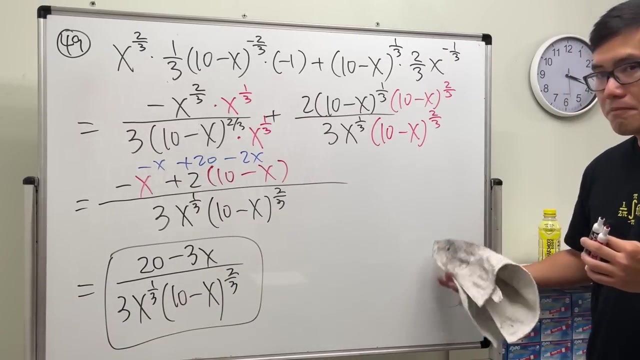 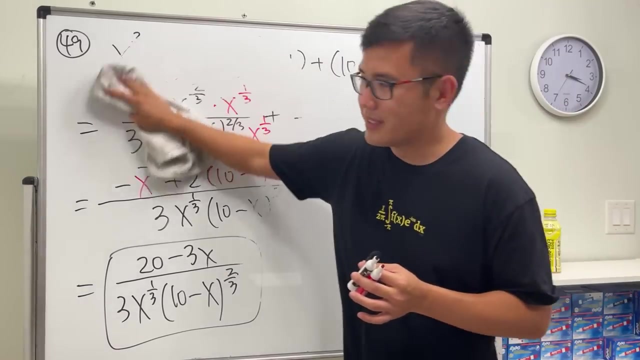 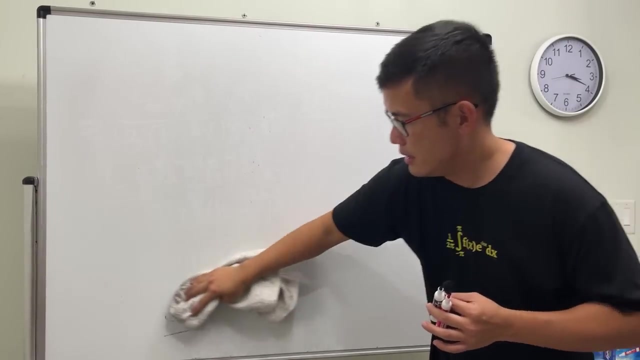 because originally you have the minus x at the end, right? so i also keep the x at the end. and then here we have the 3x to the one-third, 10 minus x to the two-thirds. yeah, i think it's pretty cool, yeah, okay, we have another one that's kind of similar to this. 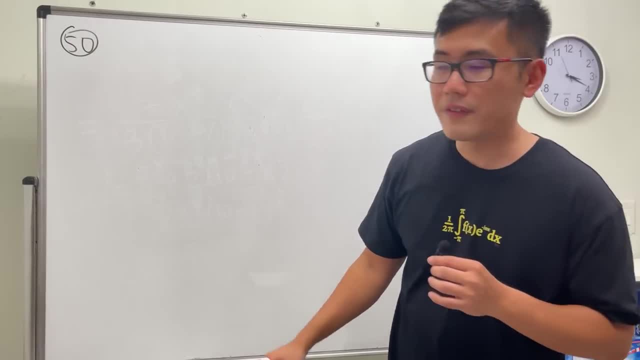 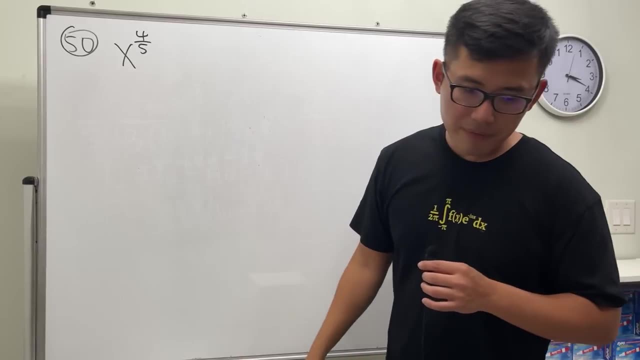 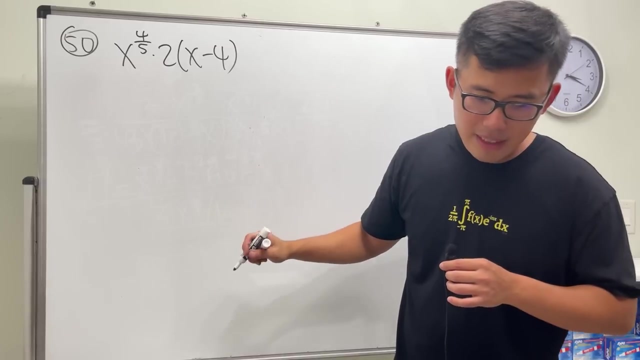 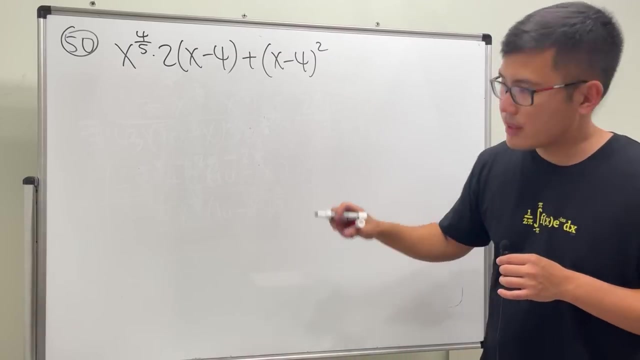 all right, number 50: here we have x to the 4 over 5, a, 4 over 5, and then times 2 parentheses, x minus 4, like this, and then after that we have plus parentheses, x minus 4, square, and then times 4 over 5, x to the negative, 1 over 5, power. 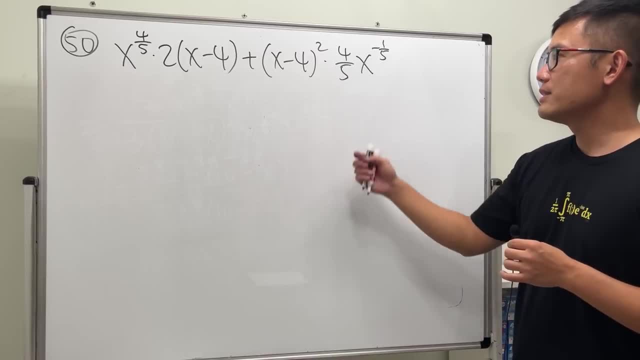 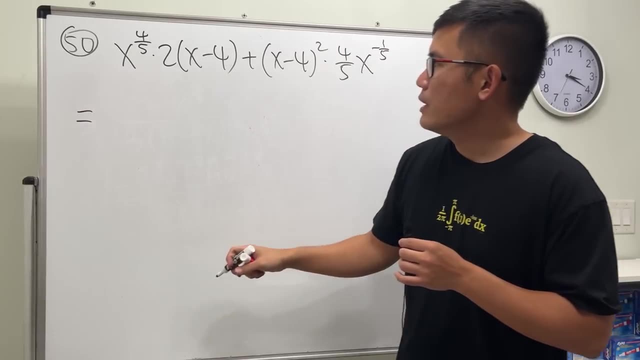 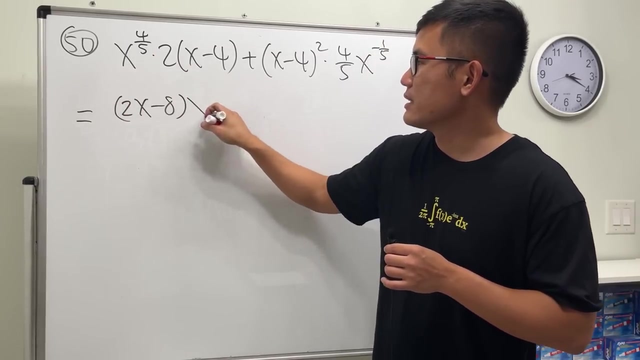 all right. so what exactly is going on? huh well, let's just go ahead and put this down to the bottom first, and then see you what we exactly we need. so right here. perhaps we can multiply this out, right? so this is 2x minus 8, and then we have the x. 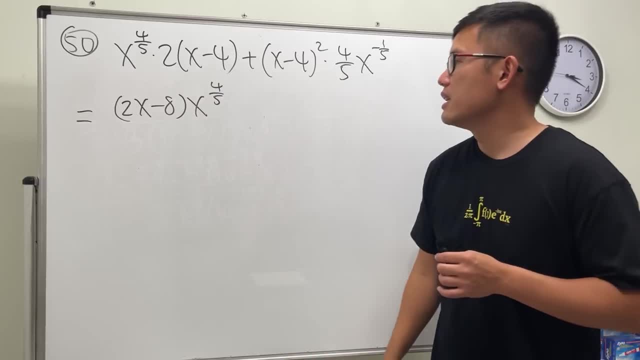 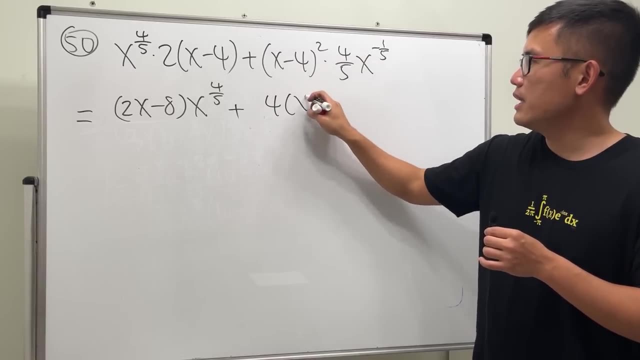 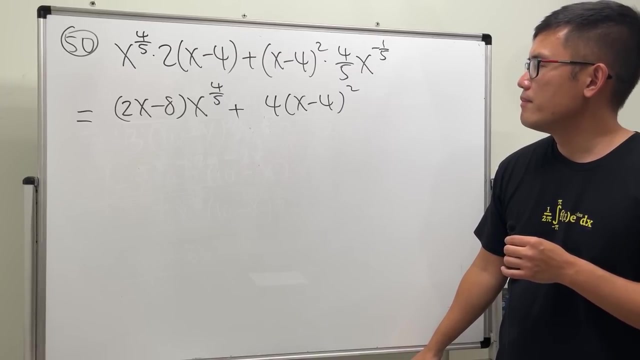 to the 4, 4, 5, so that that's that, and then i'm just going to write this four and that. so it's 4 parentheses x minus 4 square char 6. i'm thinking, if i want to factor here, if i want to factor, 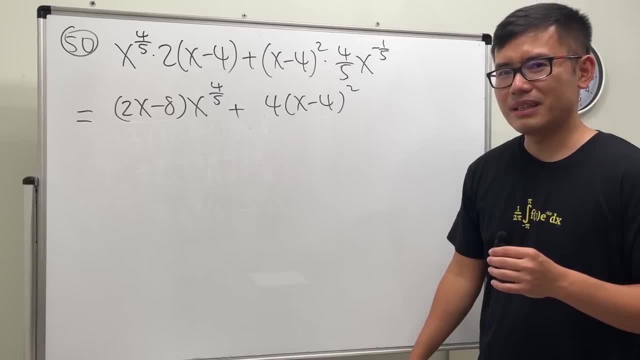 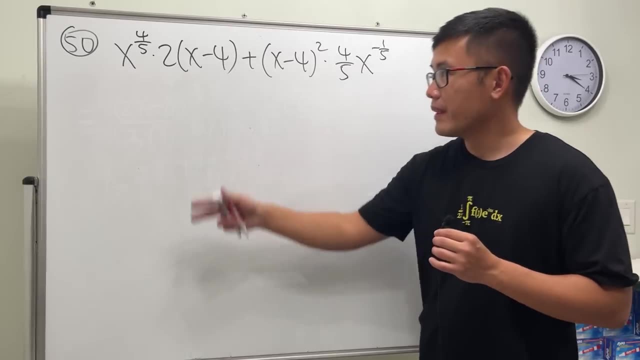 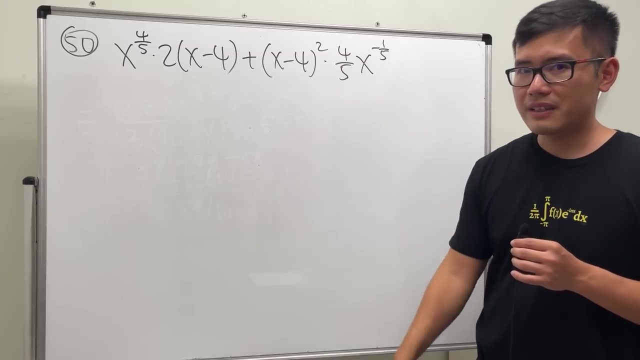 out the x minus 4. i think that's factor of the x minus 4. okay, let me show you. hold on, sorry. all right, so number 50.. notice that we have the x minus 4 here to the first power, likewise x minus 4 to the second power. we can factor it out. so let's go and do that first. so this and that. 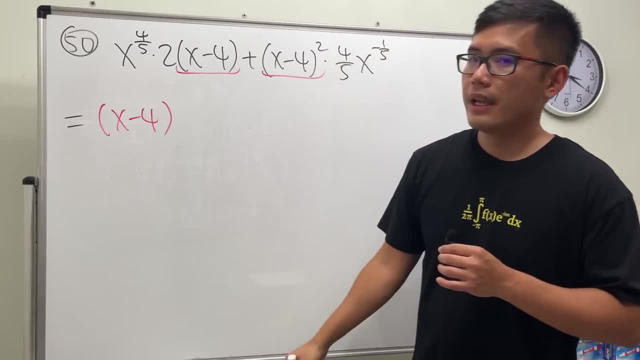 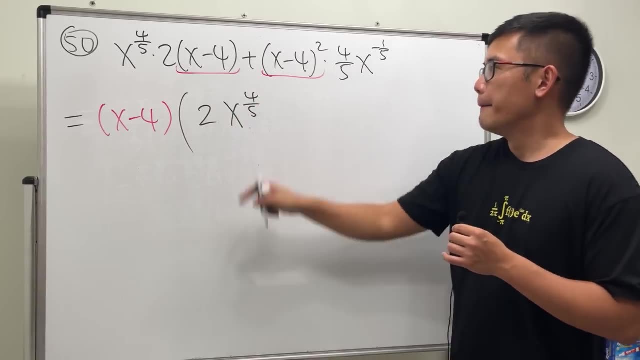 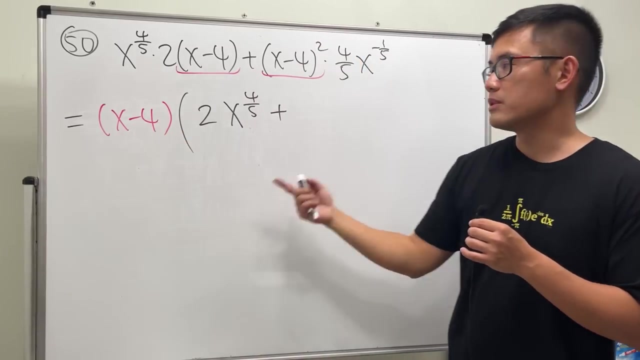 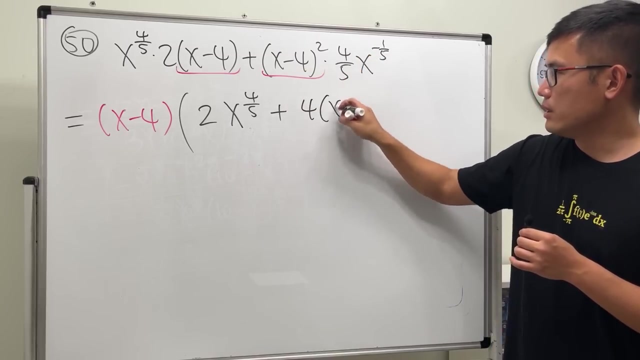 factor out an x minus 4, and then what we're going to get is 2 times that, so 2 x to the 4 over 5 plus now. this right here originally has two power. right now we took out one of them, so we have one more. so this right here is four and that, so four and then one more power. 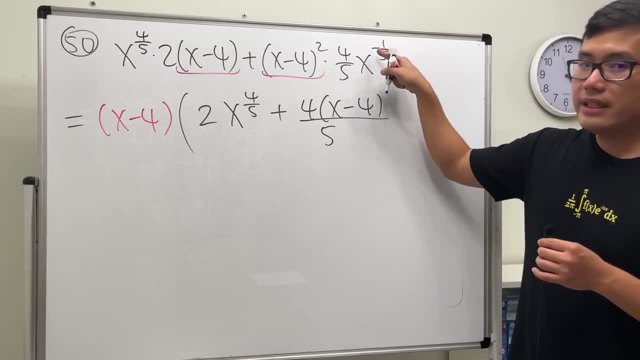 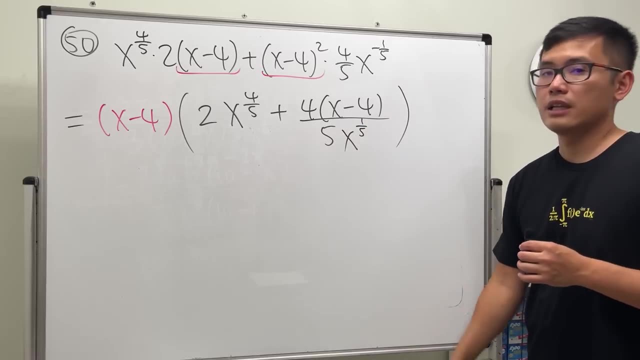 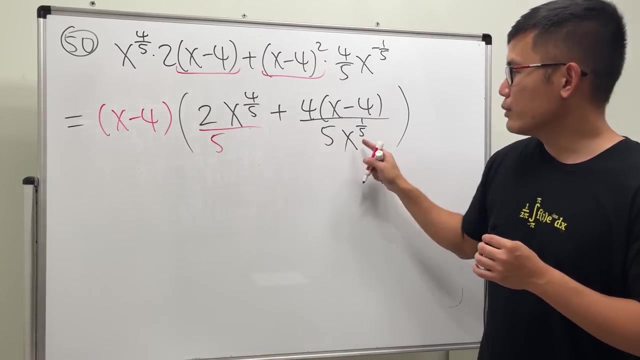 this is on the bottom, which is the five, and then negative one over fifth power. well, goes down here. so x to the one over five power. so, yeah, that's what we have, and now i'm just going to multiply this by five, and also x to the one over five power. 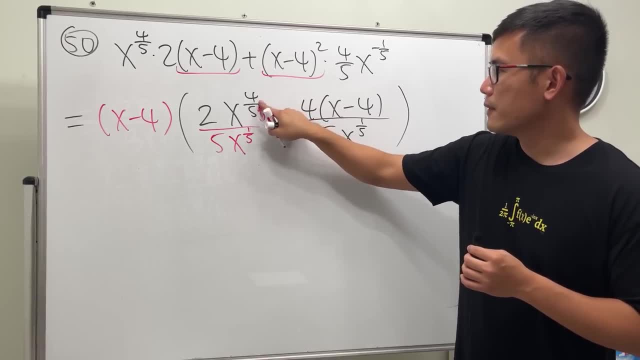 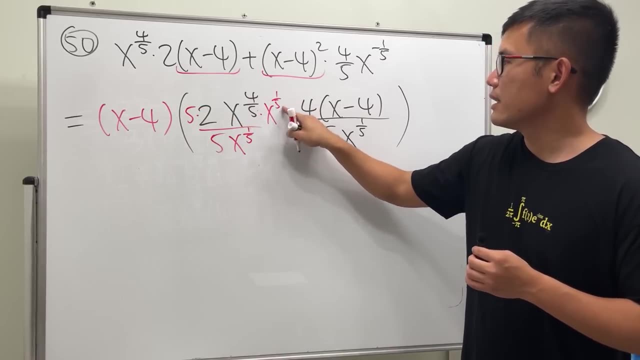 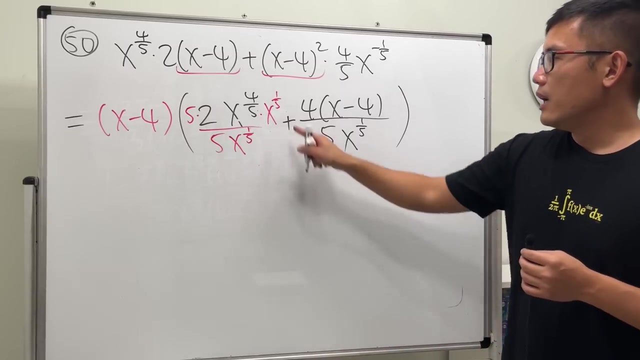 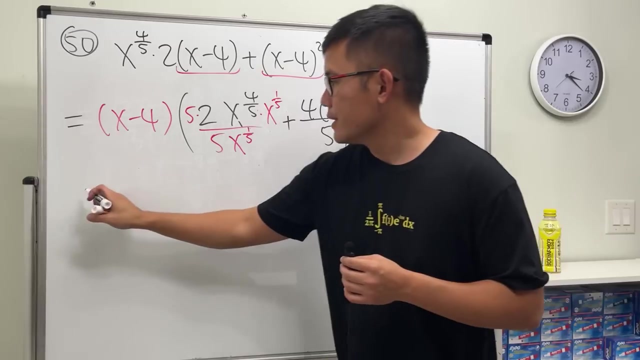 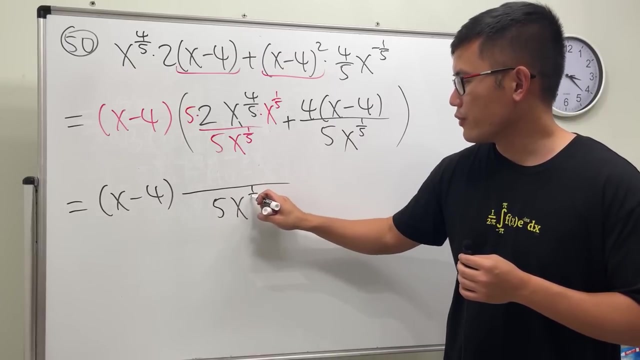 so multiply this by five, so it's meant to be like five right here, and then x to the one over five. yeah, and then the plus: okay, because this and that can be combined at five times two. okay, so x minus four times. the denominator here is five, x to the one over five power. 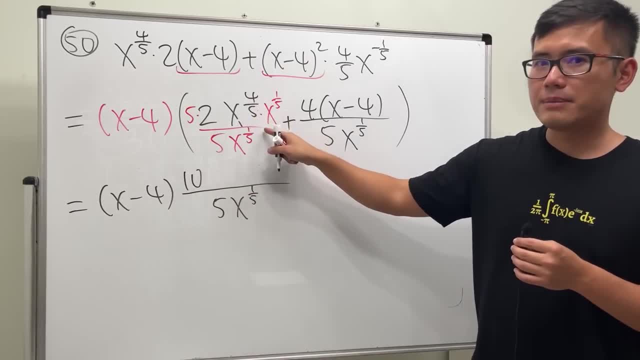 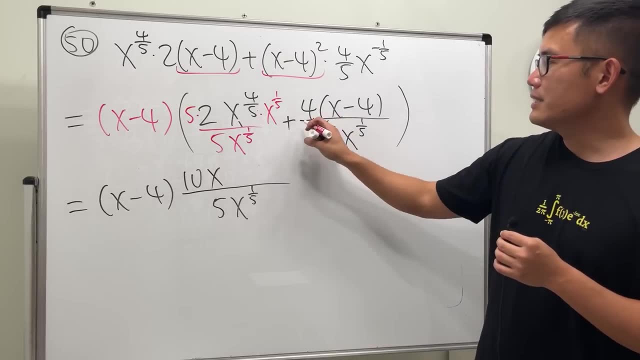 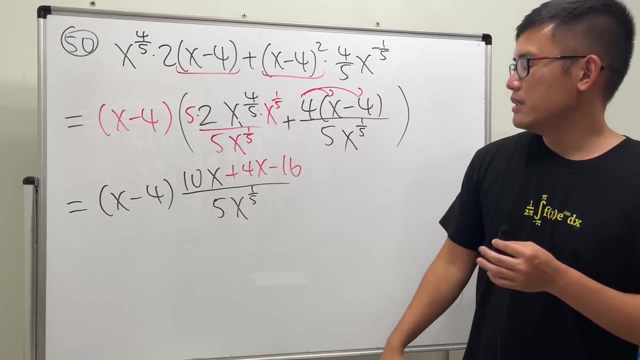 and this is ten. x to the four over five times x to the one over five is just x plus five over five, which is just x, so it's 10x, and then this guy just distribute, so we have plus 4x minus 16.. yeah, that's about all. 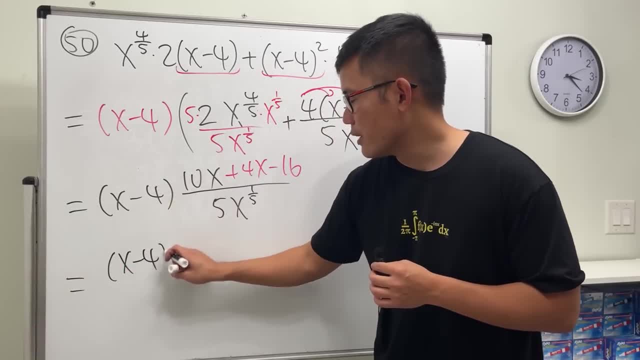 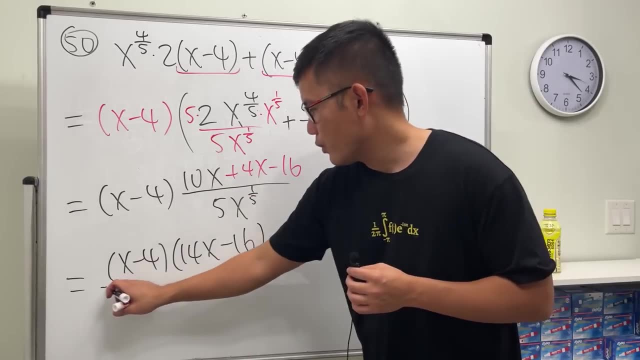 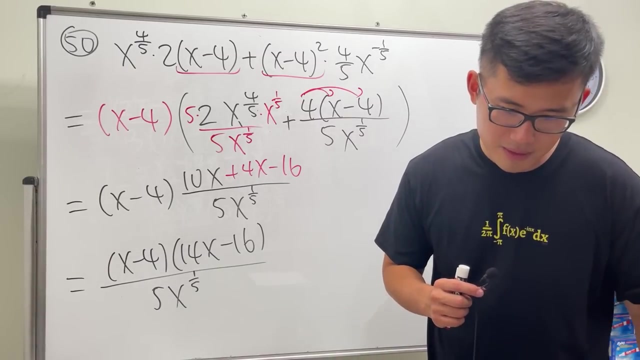 so here i'm going to leave it as x minus 4 and then combine this and that which is 14 x and then minus 16 over 5, x to the 1 over 5 and the f factor things out did. but my answer key right here: factor 2, because if i factor this in my struggle, 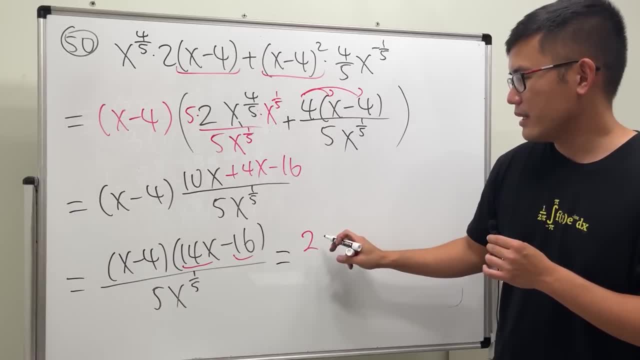 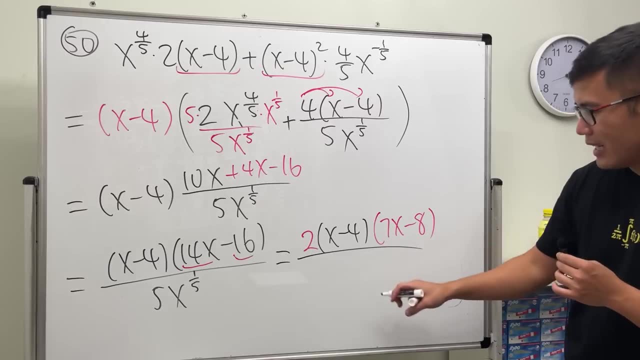 factor everything right. so i factor the order 2 and then x minus 4, and that becomes 7x minus 8 or over that denominator 5: x to the 1 over 5, 5x to the 1 over 5, 5x to the 1 over 5. 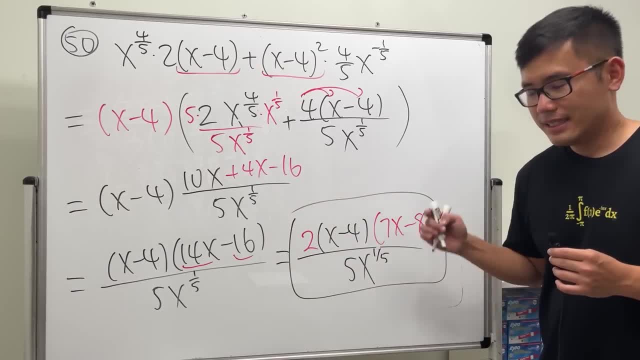 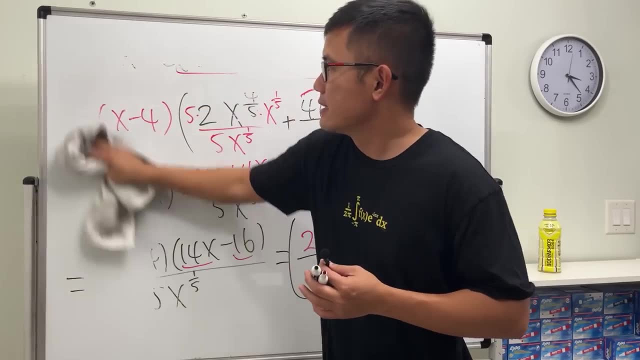 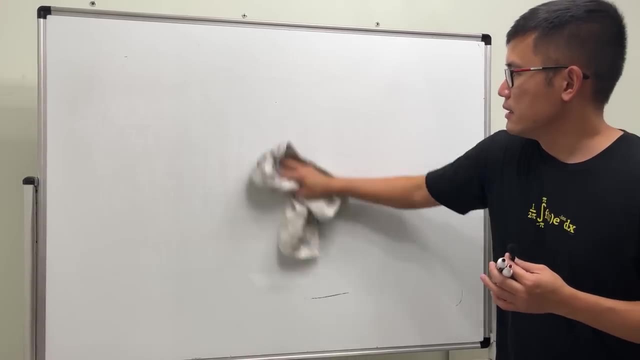 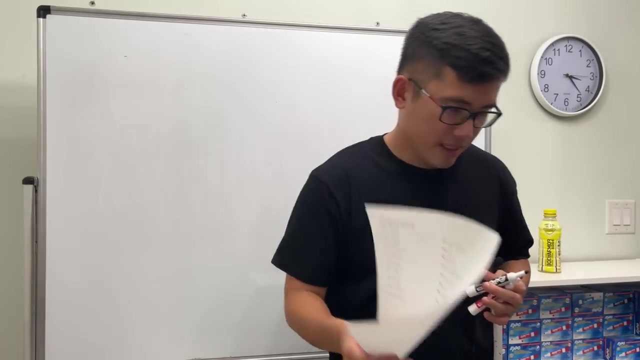 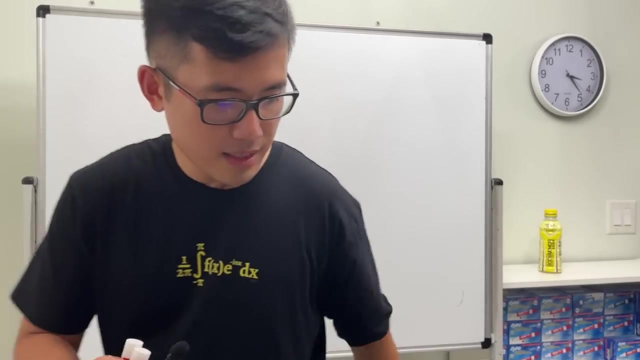 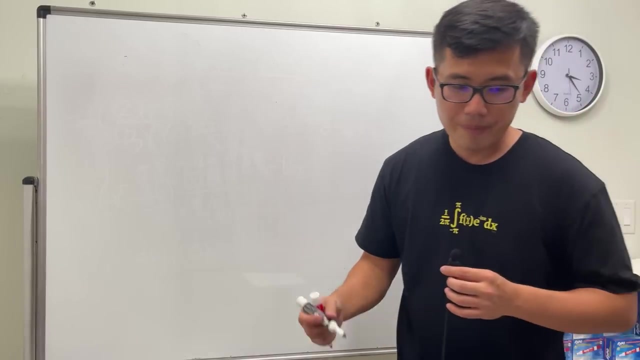 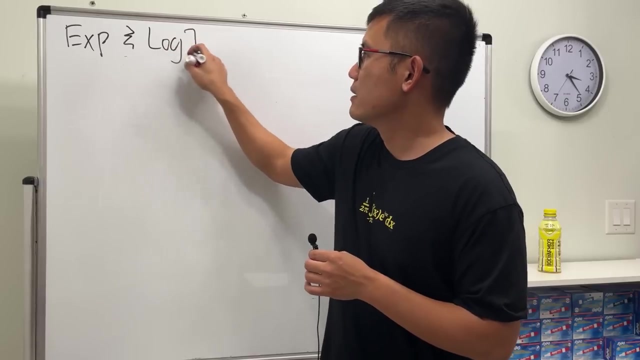 7x to the 1 over 5. yes, 50 degrees, Push it. wow, This sheet done. Take a look. Next one log and exponential. Not so bad, I would say All right. so exp and log right. 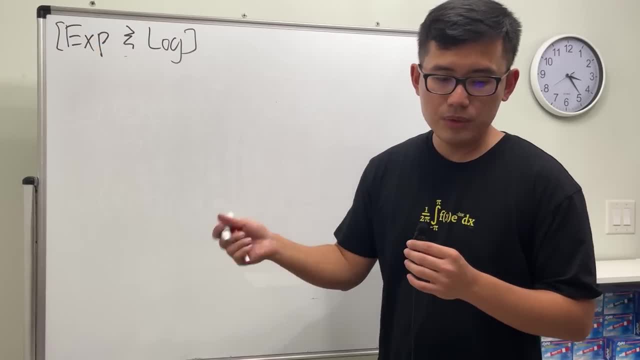 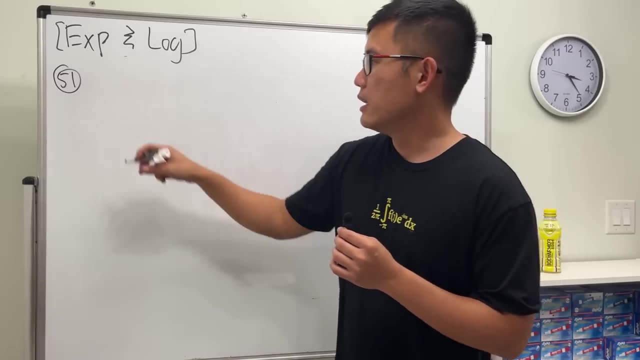 Logarithm and also exponential. Then in particular e to the 1 every power, So number 51.. We're just going to multiply things out And the expression is this: 2 times e to the x minus e to the negative x. 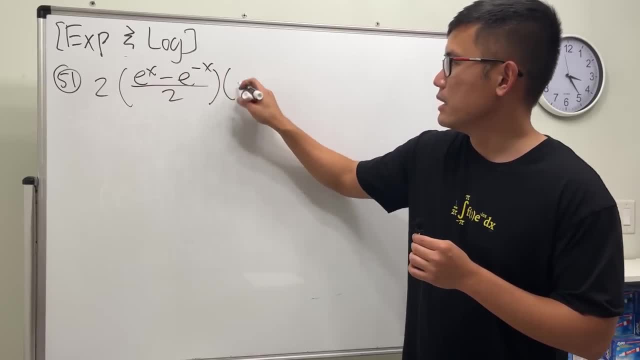 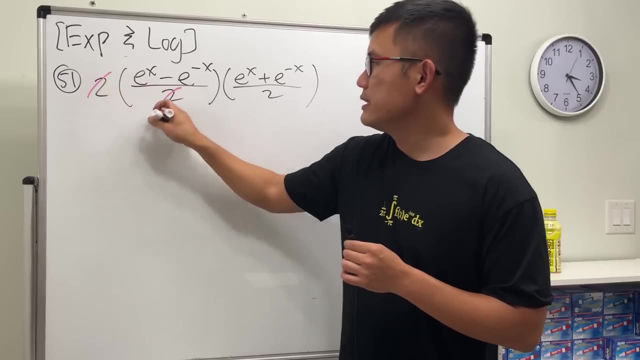 over 2.. Times e to the x plus, e to the negative, x over 2. First this and that cancel Good. And then we see that we have the 1 half right, So we can just keep it at the front like this. 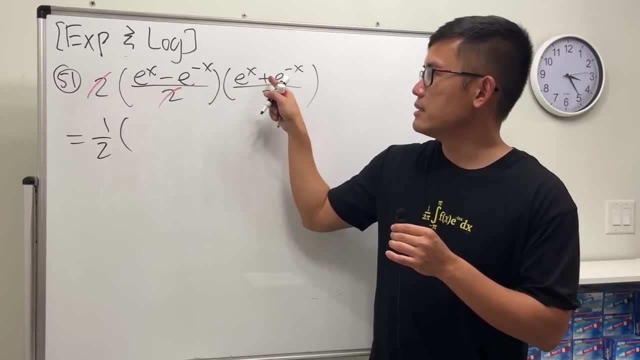 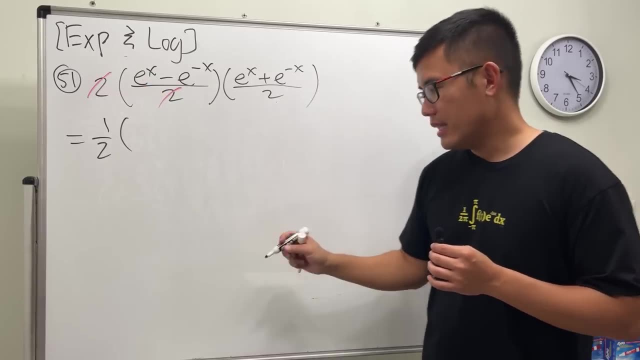 And now the beauty is that you see, this is minus and this is plus, So it's kind of like the count-you-can multiplication, huh. So we just have to square the first one. And now e to the x. if we square that, 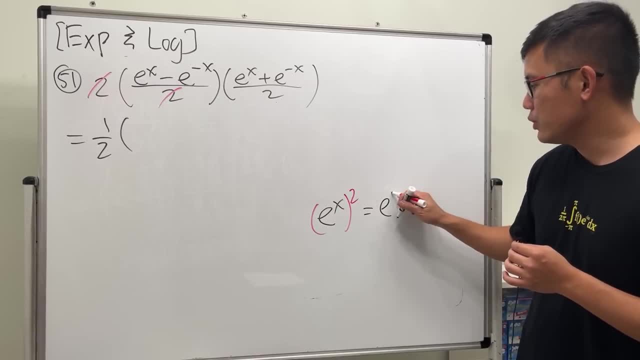 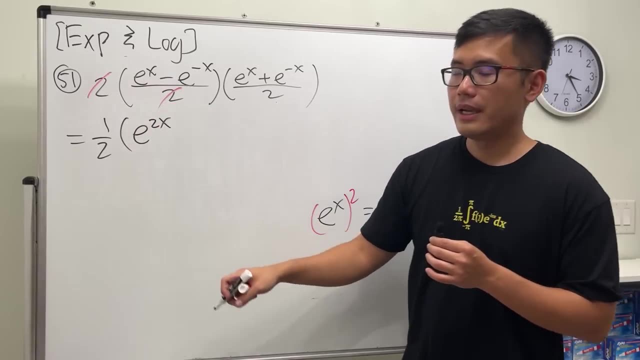 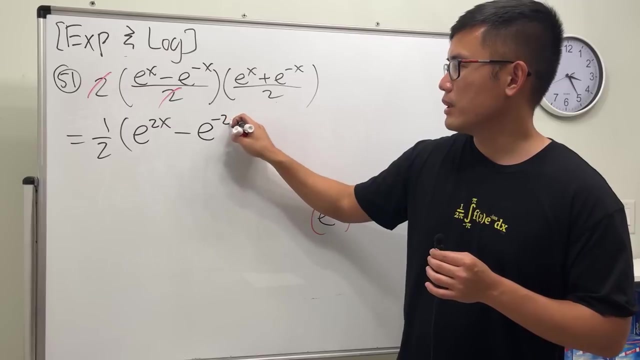 we just need to multiply the powers, It becomes e to the 2x. okay, So we will get e to the 2x And then minus square that. Again, you multiply negative x with 2. So it's e to the negative 2x. 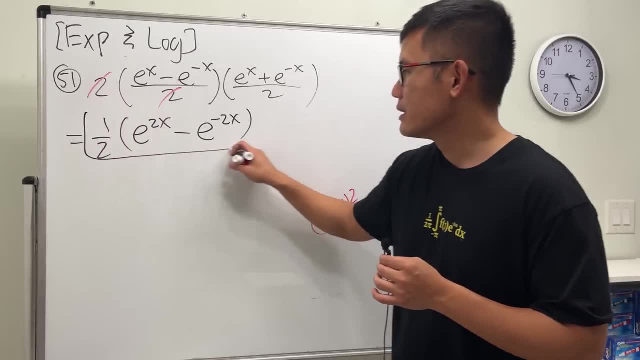 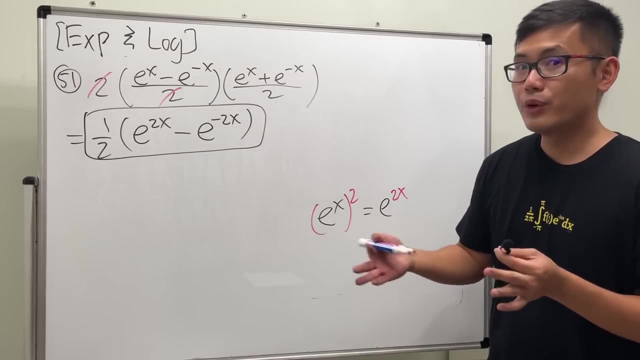 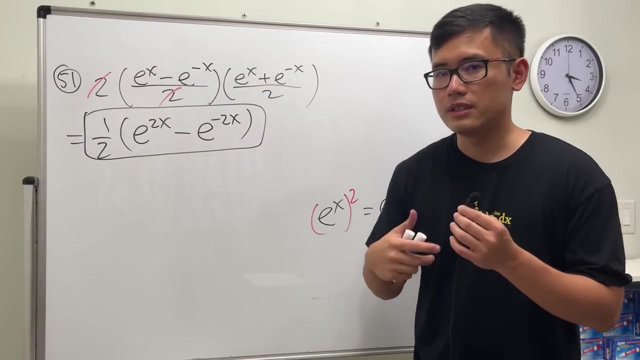 So it's like this And then, with all that, we are done. Okay, And here is a small preview to your calculus class, Because in fact, this expression, they actually represent some new functions. This one right here: 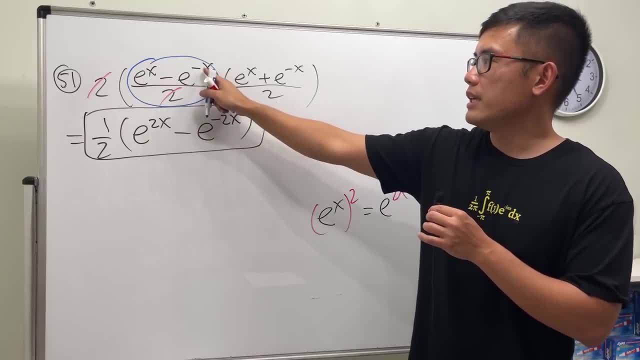 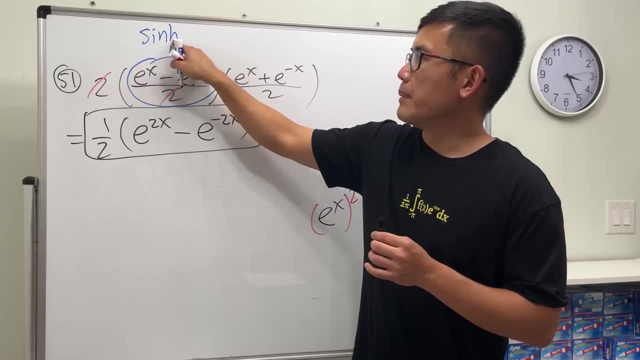 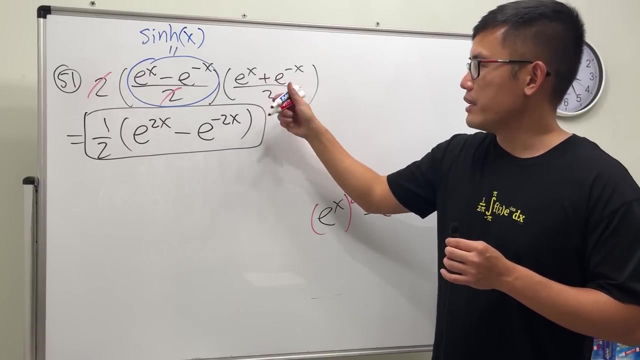 e to the x minus e to the negative x over 2, it's actually the so-called hyperbolic sine function, Hyperbolic sine function of x, And when we have the plus in between this, right here, it's called the. you guessed it. 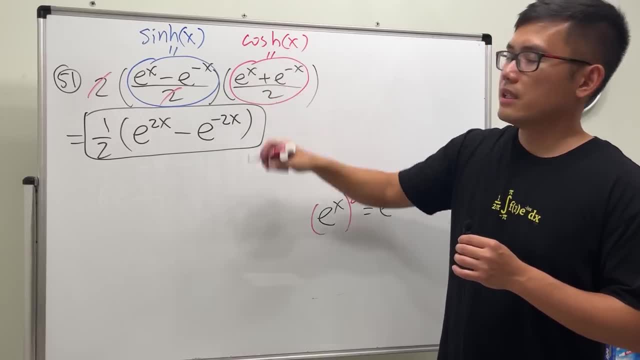 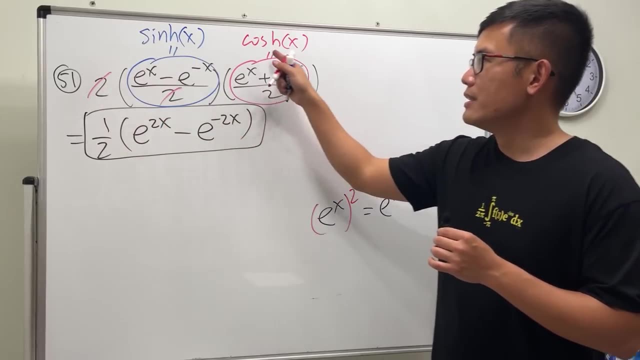 hyperbolic cosine function, Hyperbolic sine of x, And you can call this sinh and you can call this cosh. Yeah, And notice that if you have 2 times sinh and cosh, we end up with this. So what's this answer? 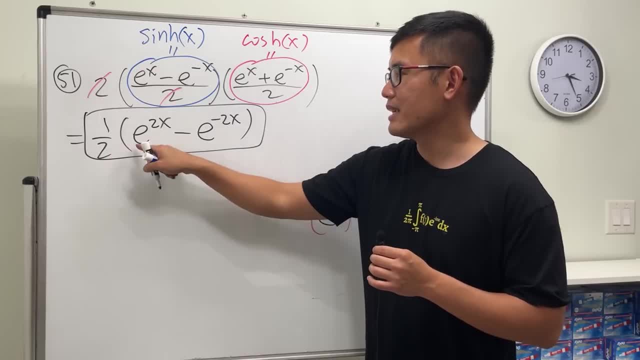 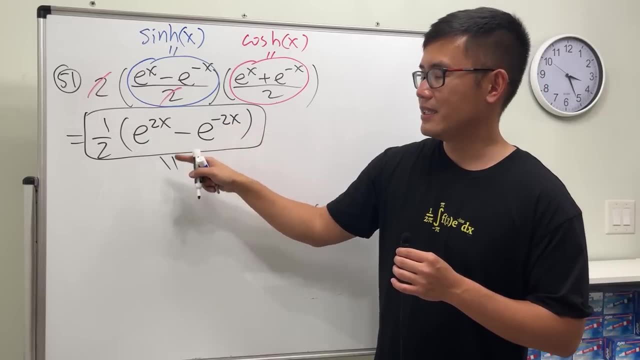 We have 1 half. Well, 1 half is like this: over 2, right, But you see the input here. we have 2x and then this is negative 2x, Yeah. So what do you think this is? 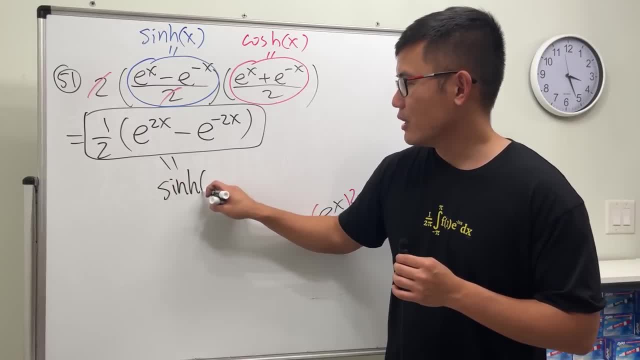 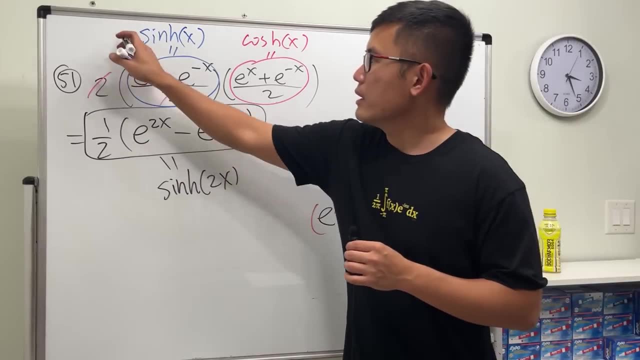 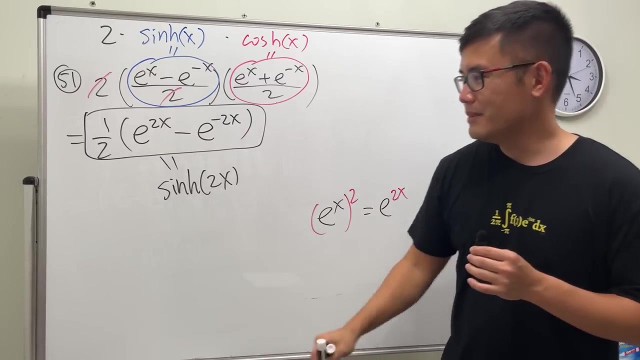 This is exactly sinh of 2x, with the 1 half, Because you can put that over 2, like that. So yes, 2 times sinh times cosh gives you sinh of 2x. This is very similar to what. 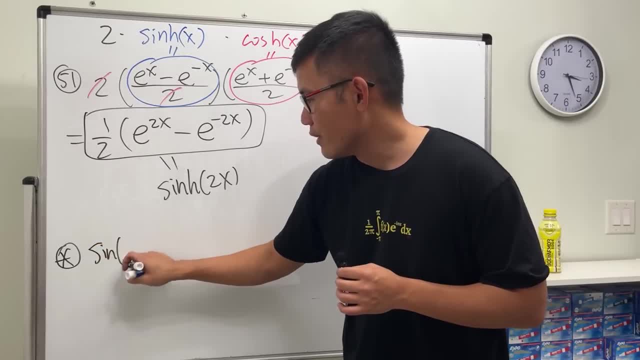 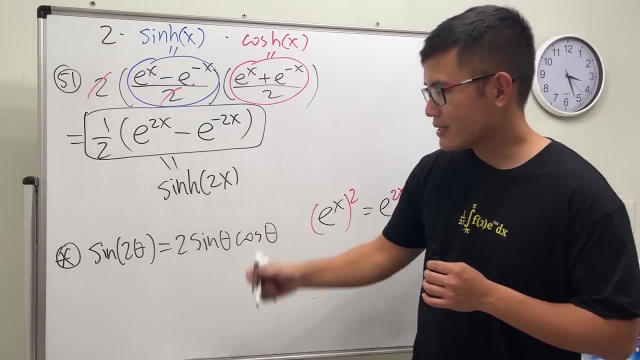 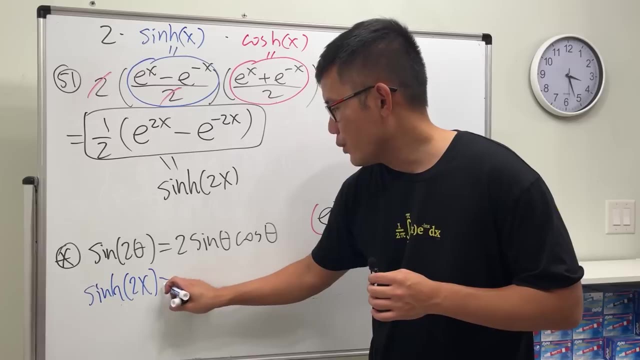 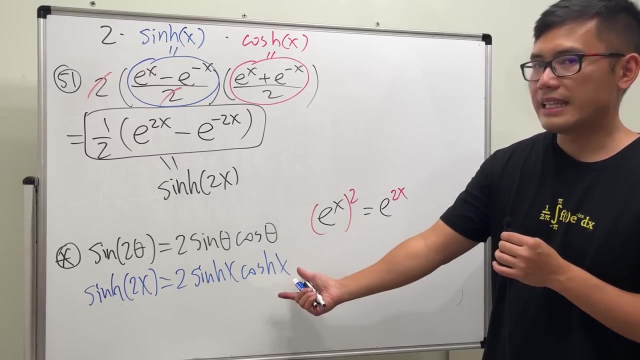 Your Google trick identity right: Sine of 2 theta equals 2 sine theta, cosine theta. Right now we are saying we have the sinh of 2x equals 2, sinh of x, cosh of x. Yeah, And to prove this identity, 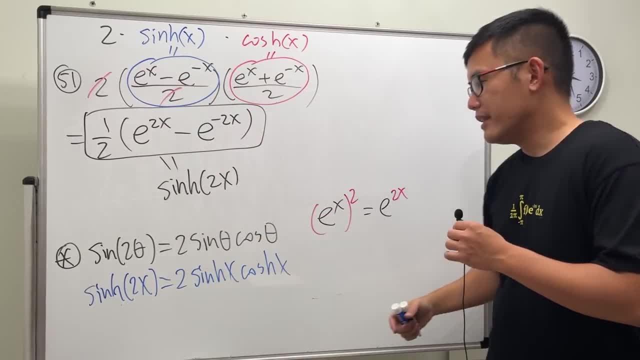 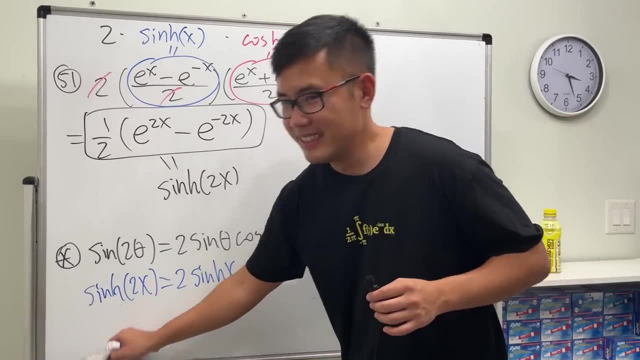 we just change them to the exponential version of them and then just multiply out, and then we got it. Yeah, So just like that. I'm sorry, I'm a little bit tired, But this is actually pretty cool stuff. So. 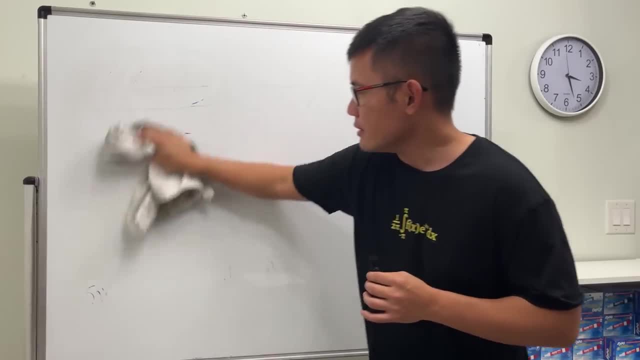 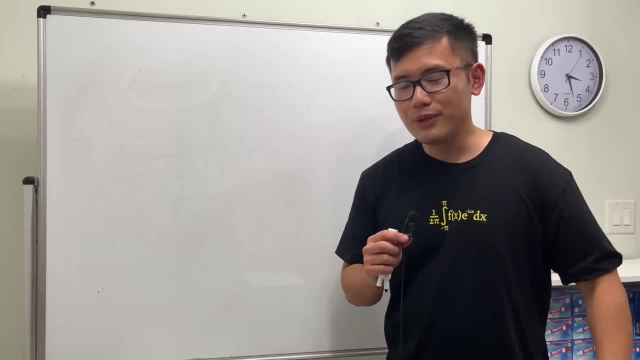 I just want to give you guys a quick preview. I also want to try. I will also try to. I would also like to try to finish the problems before I had to charge the phone. I don't know if my iPhone can go. 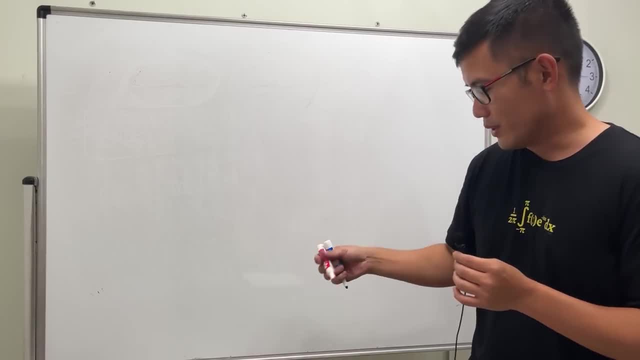 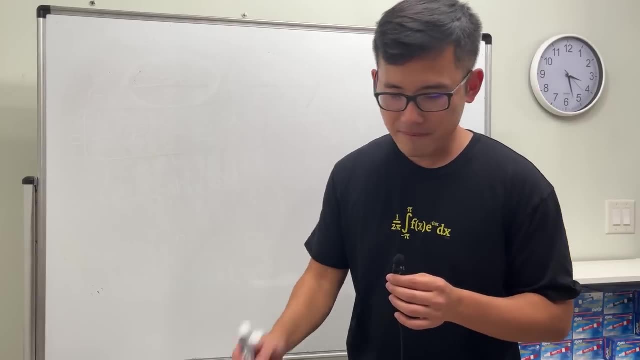 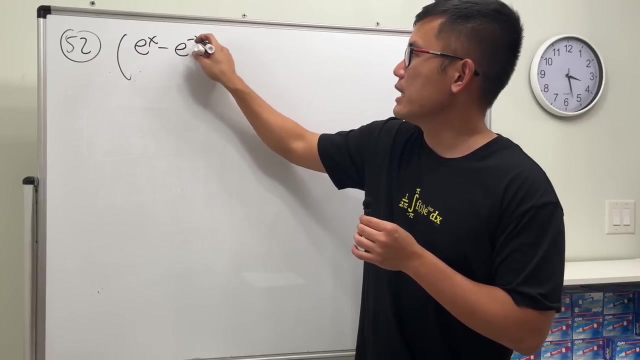 It was 100%. I don't know if it can go all the way. We will see Number 52.. Right, Right, Number 52.. Here we have e to the x minus, e to the negative, x over 2 square. 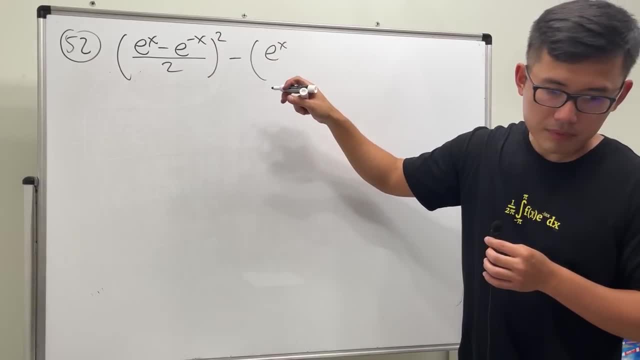 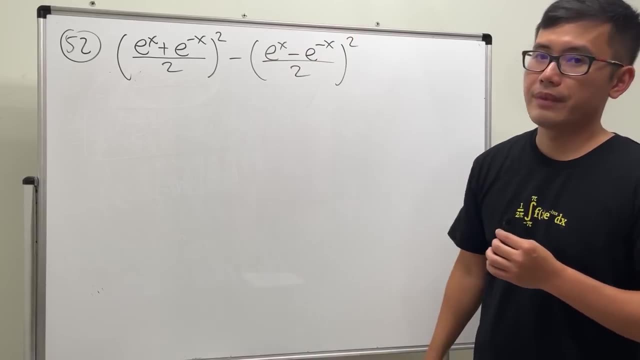 and then minus e to the x- Sorry, this right here should be a plus- And then minus e to the negative x over 2, and then square Right. So the question that's asking is this right here, which is cosh? 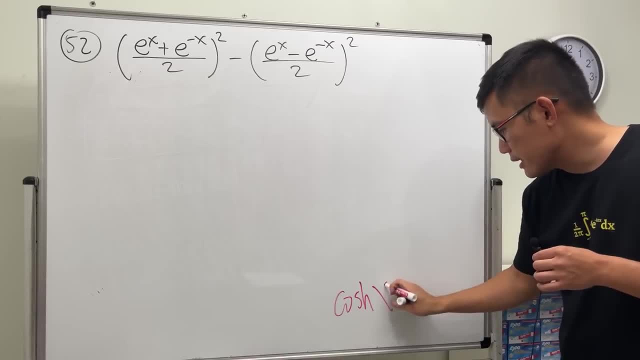 And the input here. you see the x and negative x, right. So the input here is x. And then we see that we have this quantity squared, So we have the square and we can put a 2 right here. 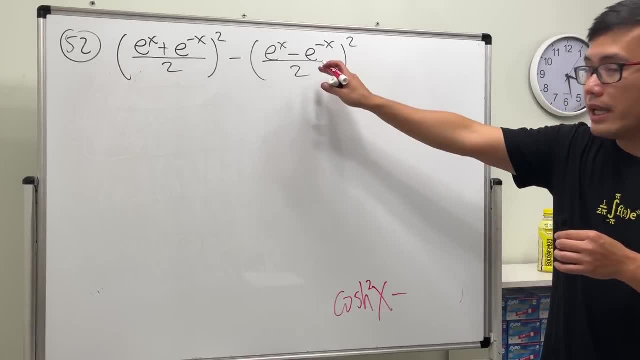 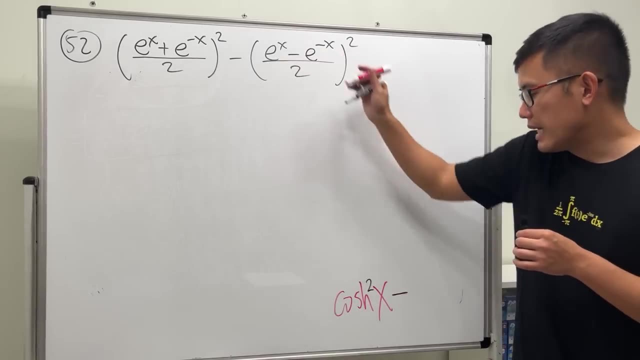 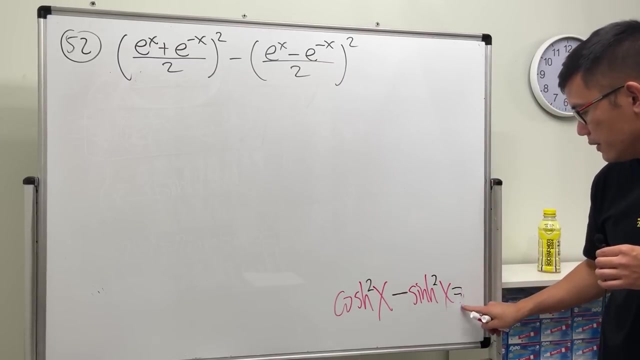 And then minus the other one is sinh. So we have the- Let's put it on this, It's cooler this way- 2, and then minus this inside is sinh of x squared. So we're trying to see what this will give us. 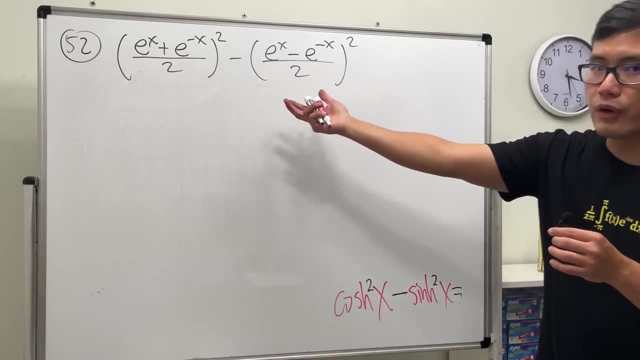 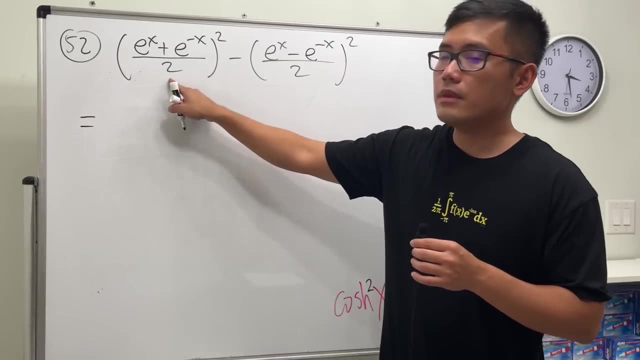 Well, all this right here, you don't have to know this in order to solve that, Because we just have to multiply it out and then simplify it. Okay, first thing. first, 2 squared on the bottom, Let's leave it 4.. 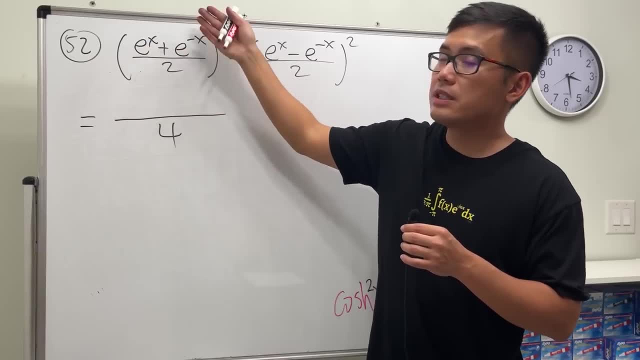 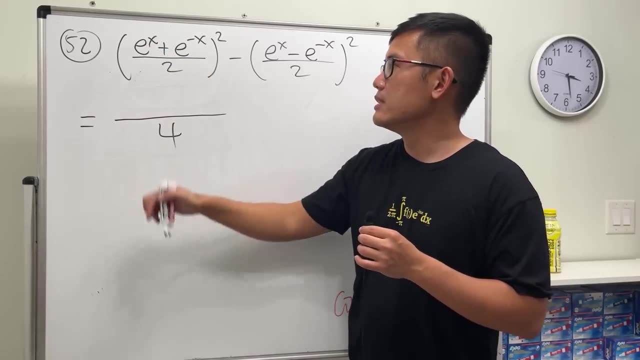 And then on the top where we see that we have a plus b squared, So just multiply out the binomial, right. So we take the first thing, square that, so we get e to the 2x Square. that just multiply the powers. 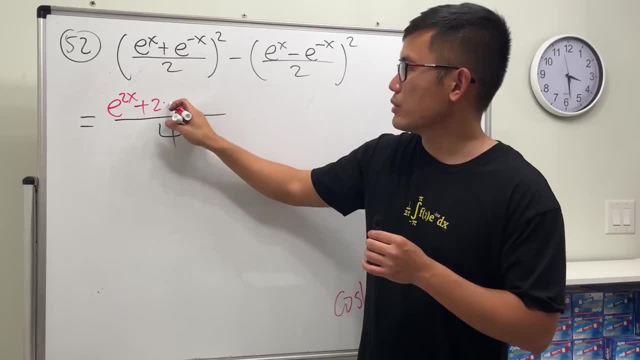 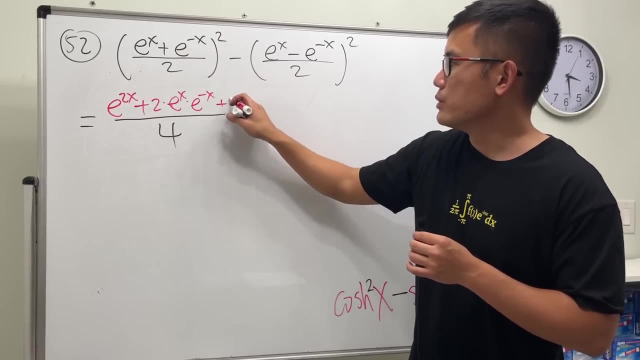 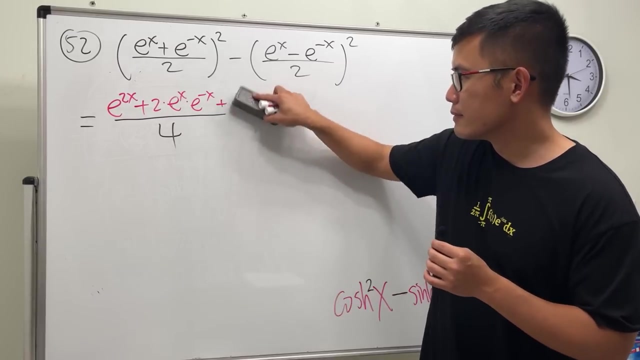 We add 2x, 2 times this and that, So 2 times e to the x And e to the negative x. Lastly, we add this thing squared, which is e to the negative, 2x, Then minus. 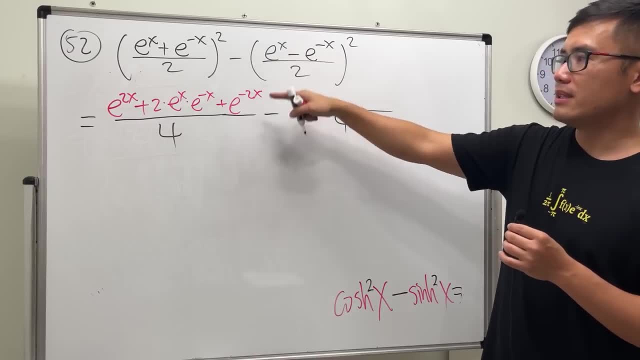 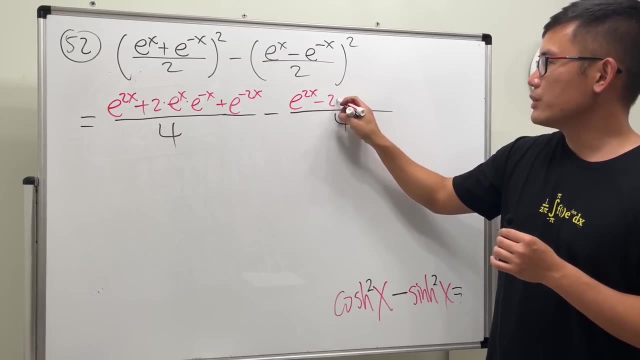 Same thing. Right here we have a 4. And then this is a minus, So we just change this to minus. So then the rest is the same. So we have. So we have e to the 2x minus 2 times e to the x times e to the negative x. 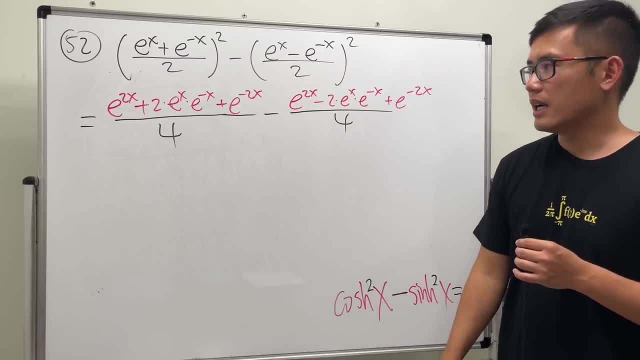 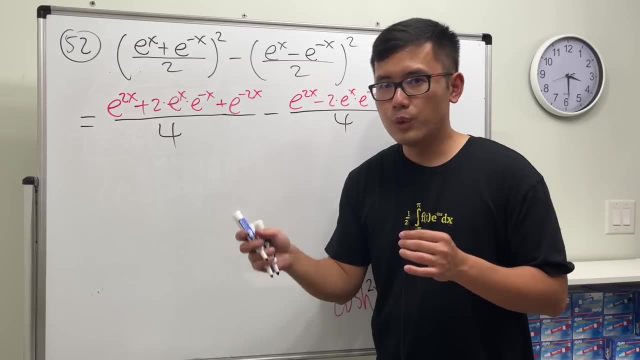 And then plus e to the negative 2x. Yeah, By the way, do you guys notice what this is? e to the x times e to the negative x. We add the exponent, It's just e- to the 0,, which is just 1.. 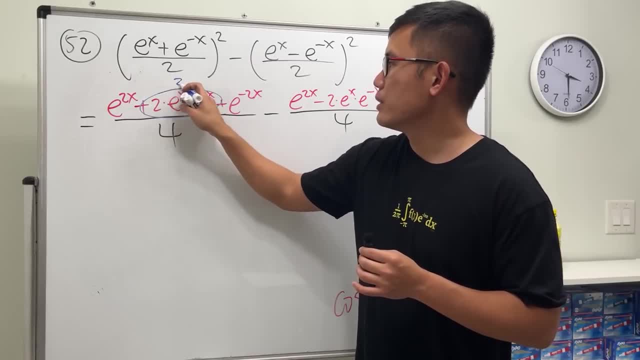 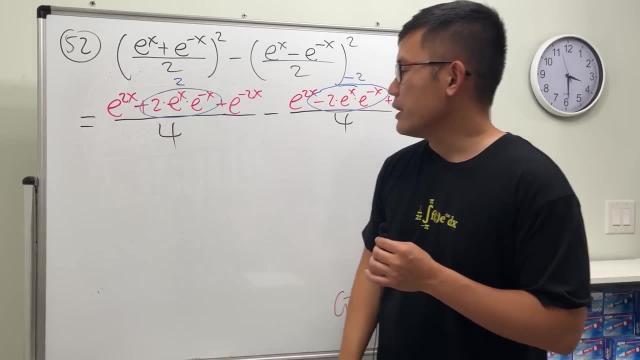 So in fact, this right here is just equal to 2. And this right here is equal to negative 2. Right, So yeah, Okay, And then right here we have minus. So I'm going to put them together and then just distribute the negative. 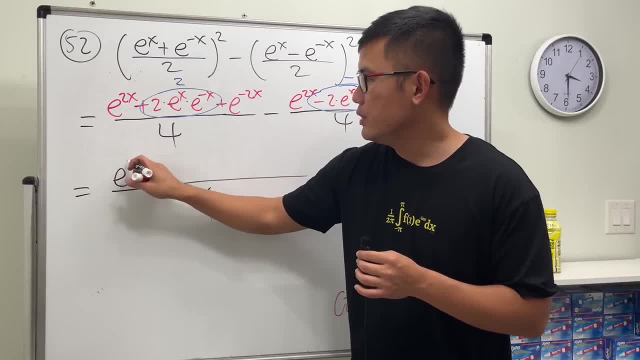 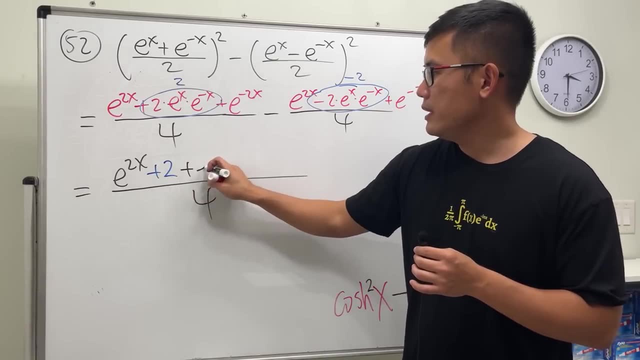 So together we have a 4. And then this is e to the 2x plus 2.. And then plus e to the negative 2x Distribute the negative, So we have negative e to the 2x. 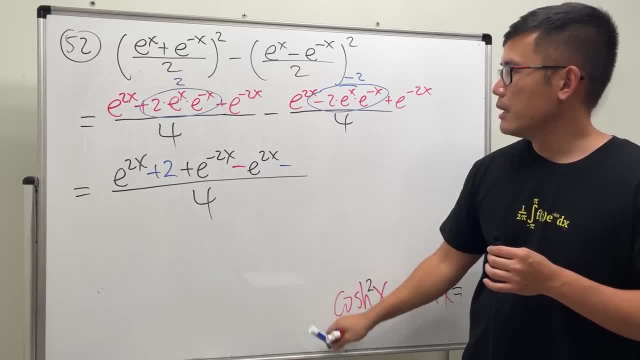 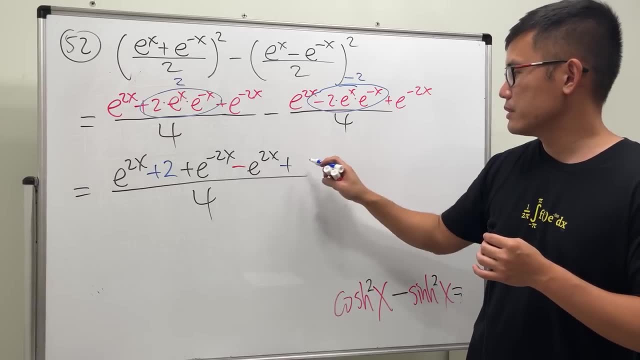 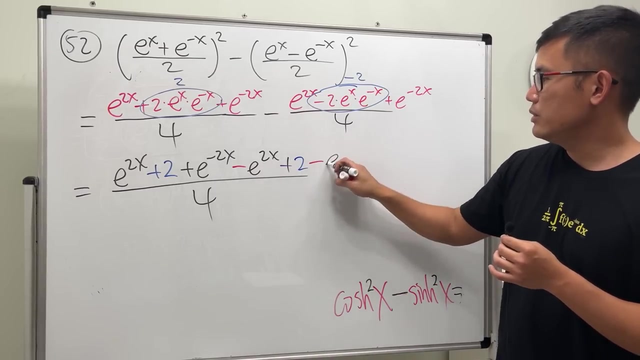 And then this is a minus, Right, But negative times, negative gives us a plus, And then We still have that 2.. And lastly, minus that which is e to the negative 2x. Okay, And now? what do we see? 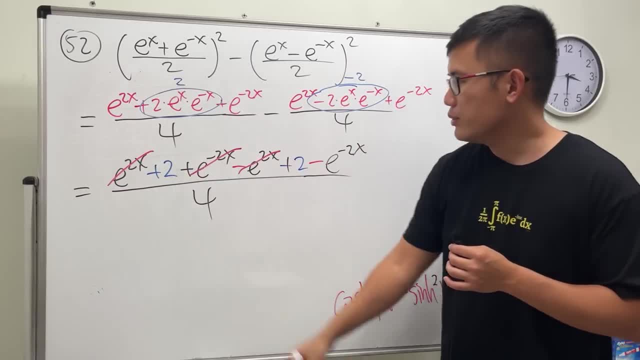 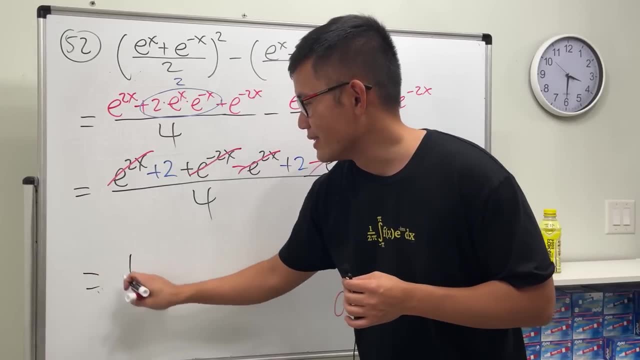 e to the 2x Cancel e to the negative 2x Cancel. It's that On the top we have 2 plus 2, which is 4. Over 4. So the answer is 1.. 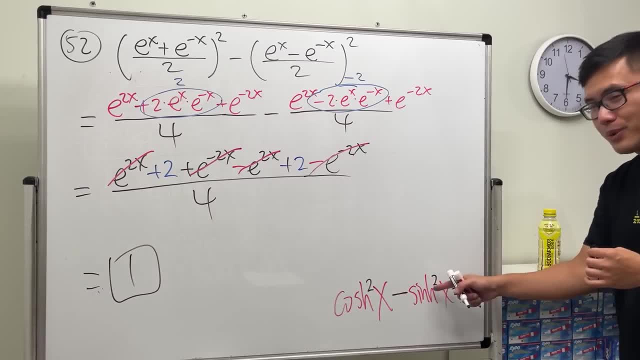 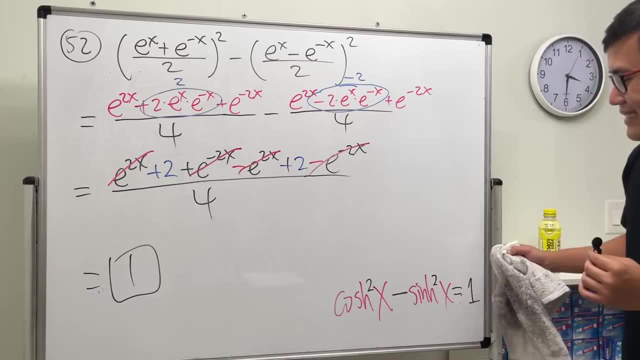 So this right here: Cos square x minus sin square x is actually just equal to 1.. This is one of the hyperbolic identity. Okay, It's very similar to cosine square plus sine square is equal to 1.. But this is a minus version. 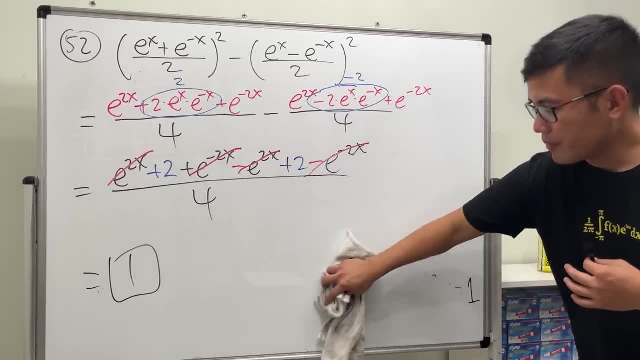 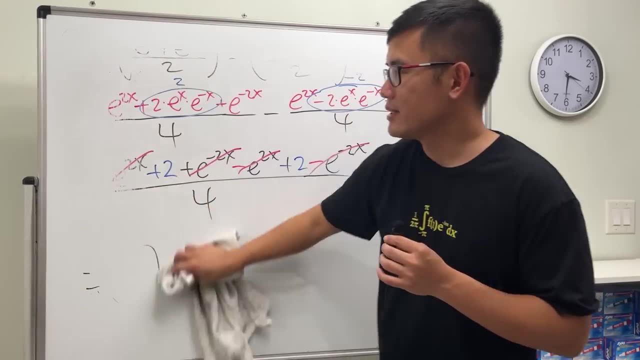 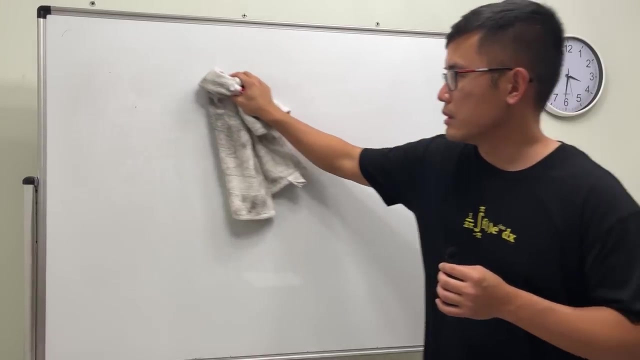 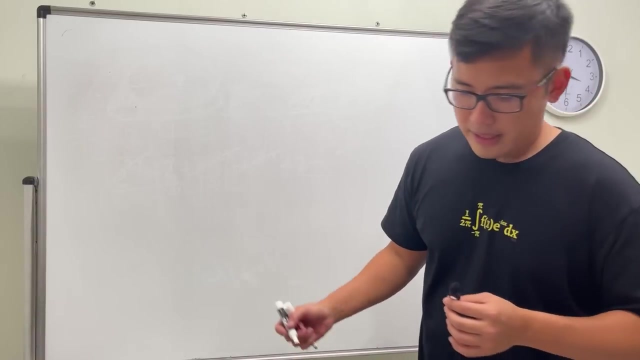 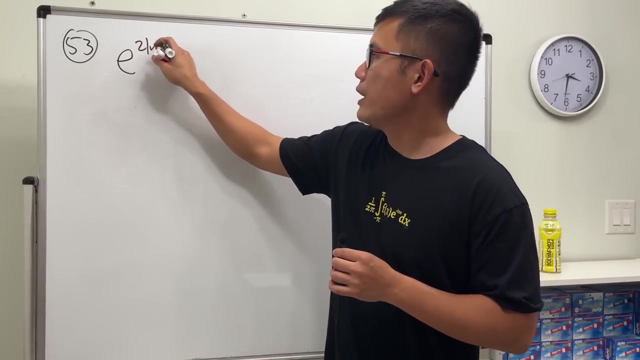 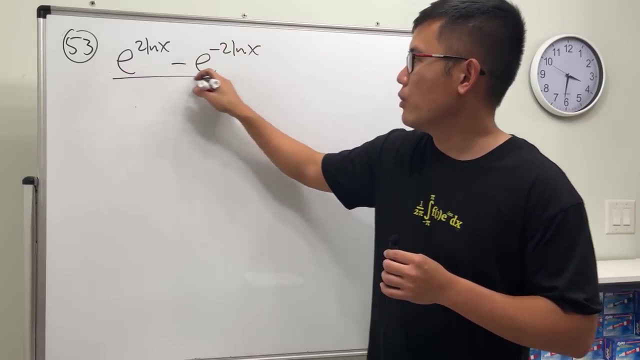 Yeah, And the reason for this is because this right here comes from hyperbolic instead of a circle. That's why, But again, it's just some preview. Alright, Number 53.. Okay, e to the 2 ln x minus. e to the negative: 2 ln x over 2.. 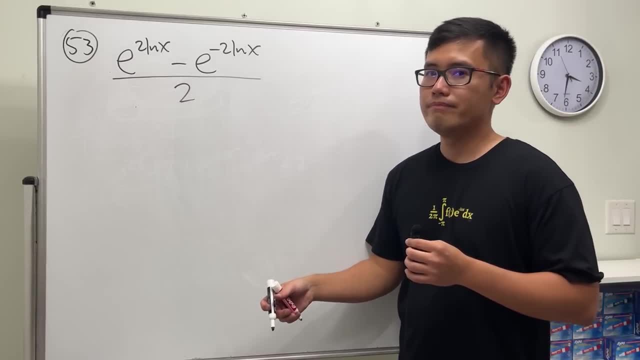 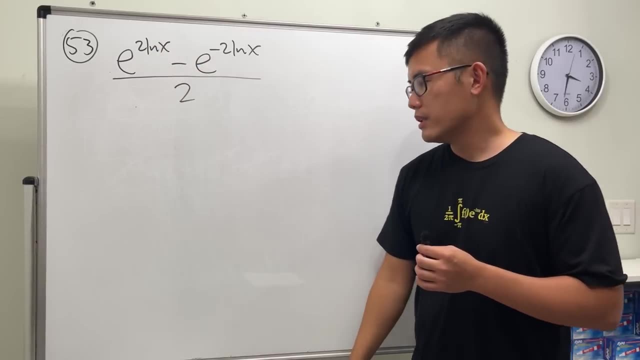 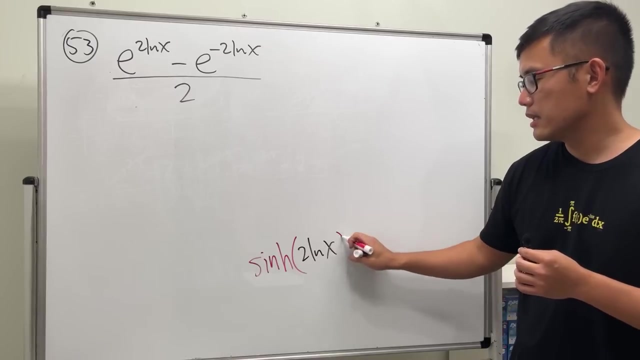 So this right here, Well, Well, the input is what? 2 ln x? and then it was a minus. So this question right here is asking hyperbolic sine of 2 ln x, right? But anyway, again, you don't have to know this, to simplify, 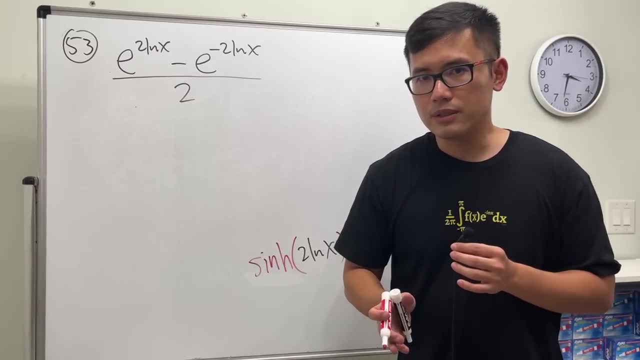 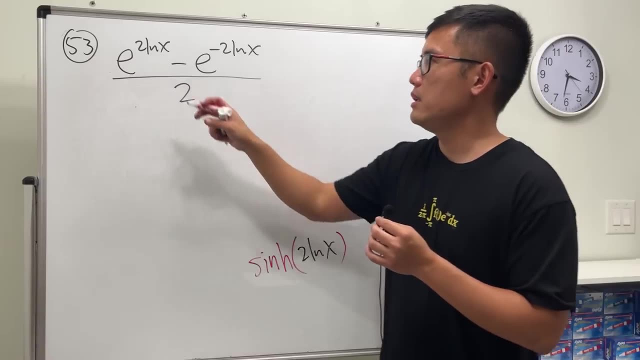 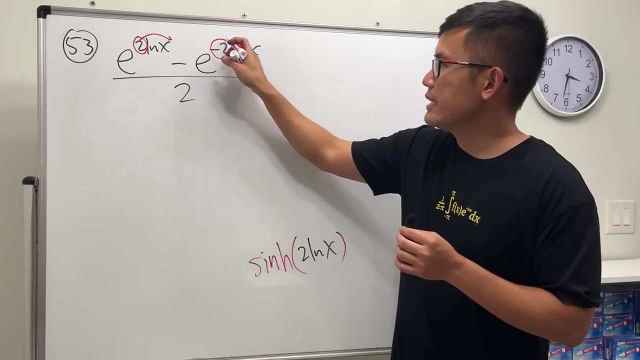 that Okay, e and ln, they can almost cancel it, because here we have two spotting us. But what do we do? Thanks to the log property, when we have 2 times ln, x, we can put a 2 right here, make that into an exponent. Likewise, we'll put a negative 2 right here into the. 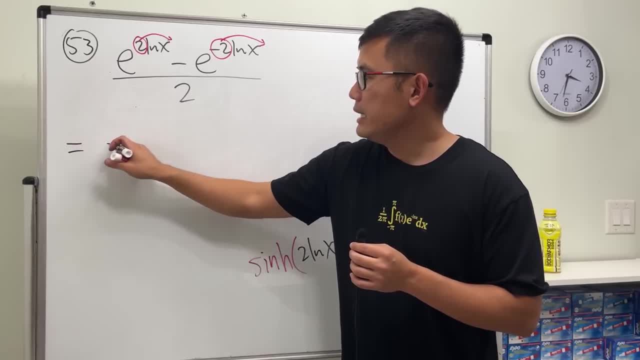 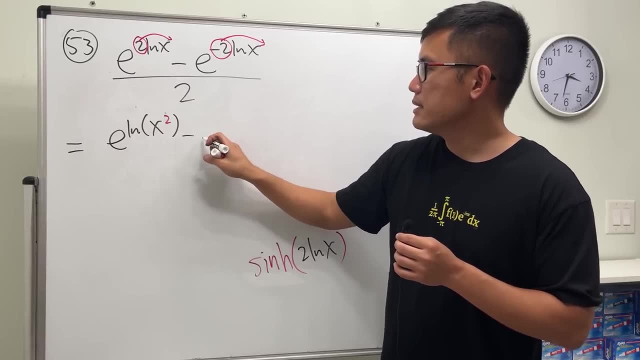 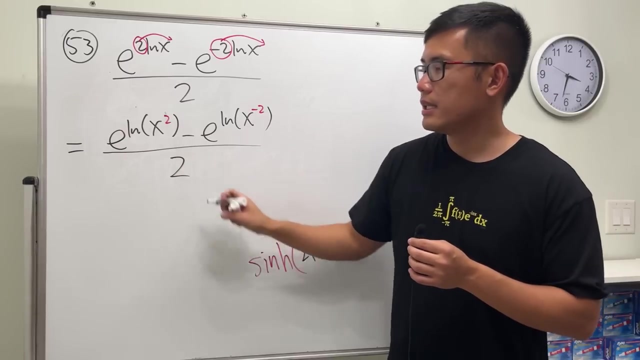 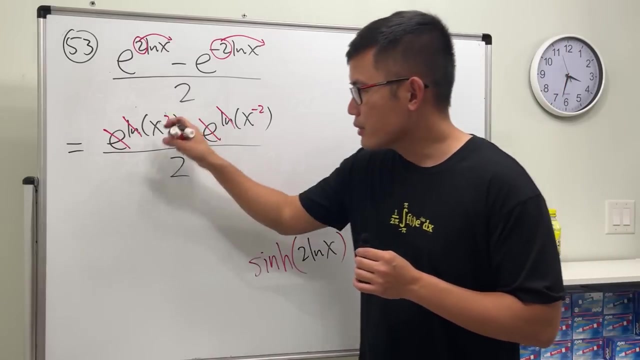 exponent. So we are going to get e to the ln of x squared, and then minus e to the ln of x, to the negative 2, or over 2.. And now we can cancel the e and also the ln, and then e and also the ln. Okay, So this: 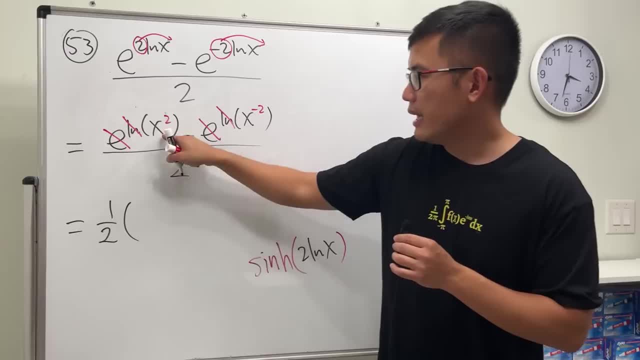 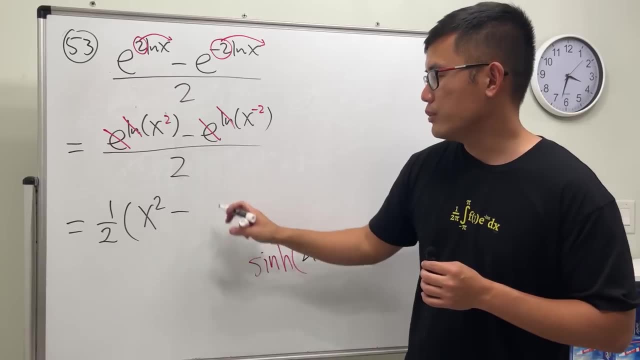 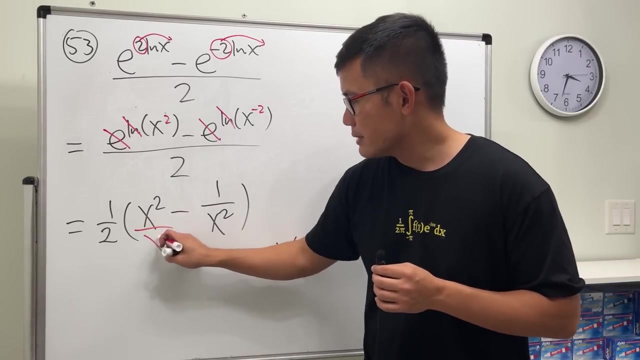 right here. let's just put on the one half like this right here, and this is just x squared plus- sorry, minus- x to the negative 2.. But x to the negative 2 is the same as 1 over x squared. And now what? We can combine them? We can multiply this by x squared and x squared. 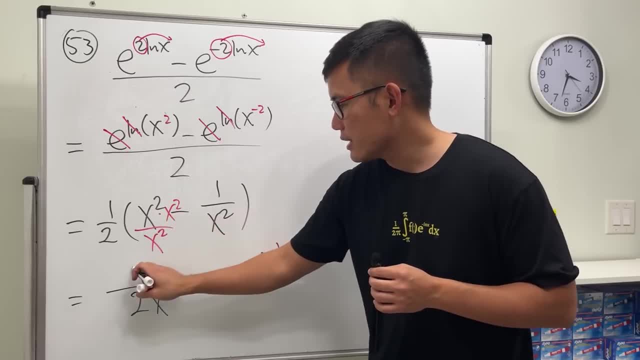 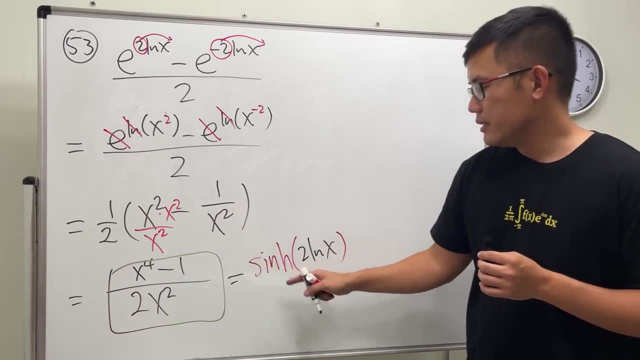 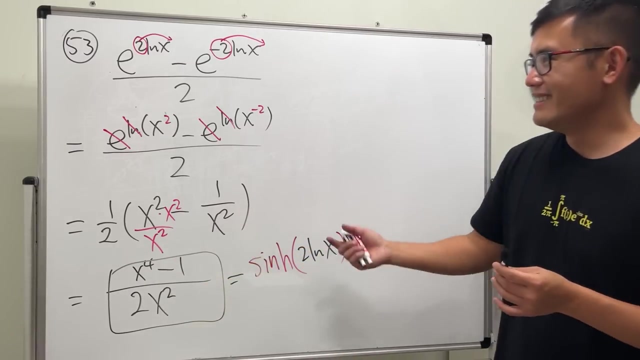 And then x squared on the bottom, And then this, and that is x to the fourth power, and then minus 1.. Yeah, so this right here. signature of 2 ln x. it actually is x to the fourth power minus 1 over 2, x to the second power. So, yeah, Okay, and then that's about it. 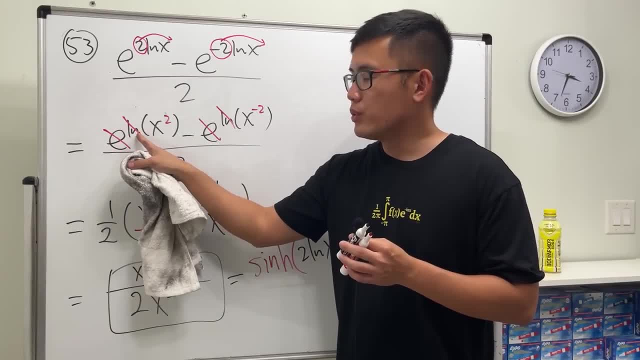 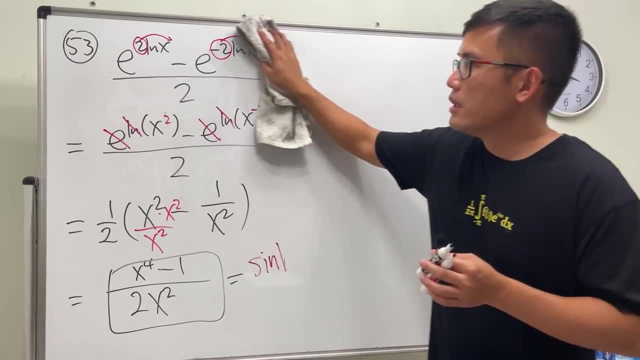 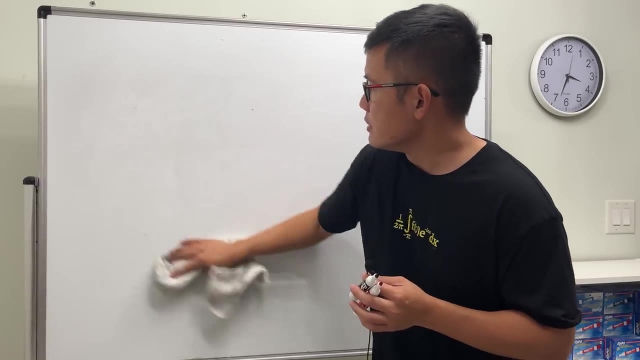 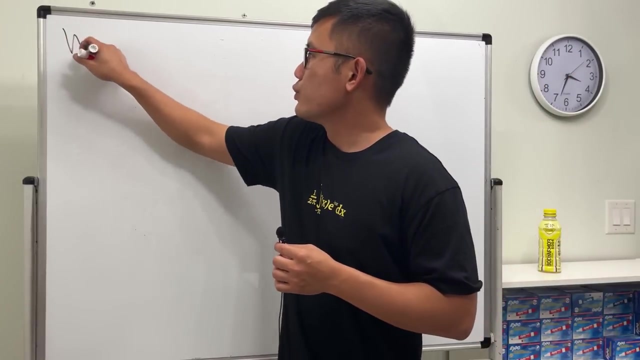 So keep in mind, though, right here, notice that e to the ln's power, they cancel, because they're just the inverse functions of each other. And for the next few questions, we are going to practice how to write some expressions with space e, So I'll just write this down. 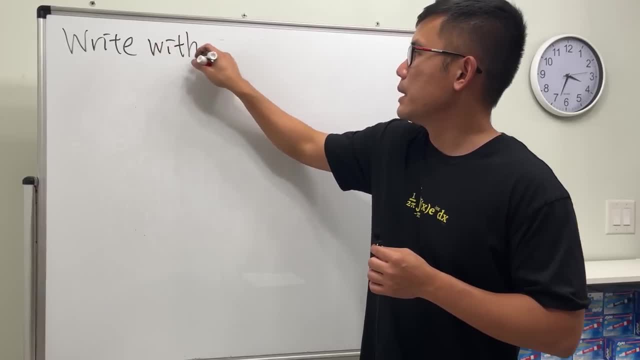 So the next few questions write the following: with e for the base, Okay, With space e. So the first one, which is e to the first power, And then the next one, which is e to the second power, And then the next one, next one, next one, And so this one, this one, next one, and. 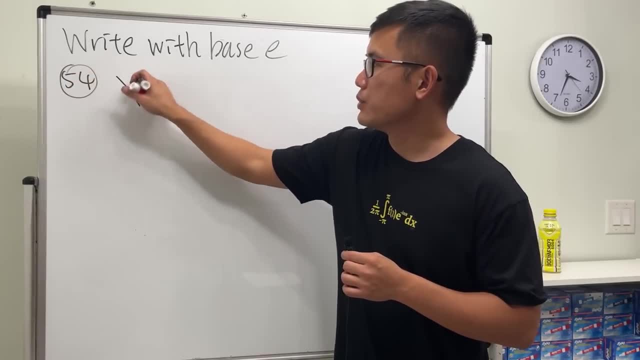 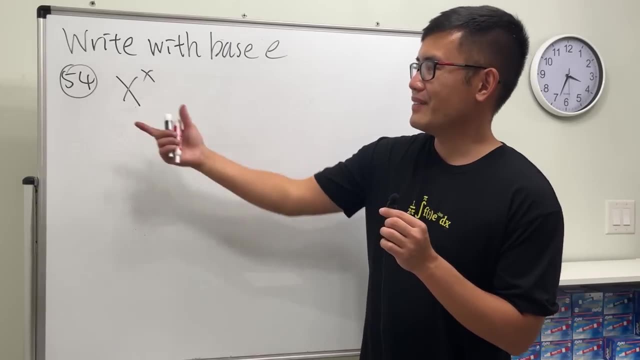 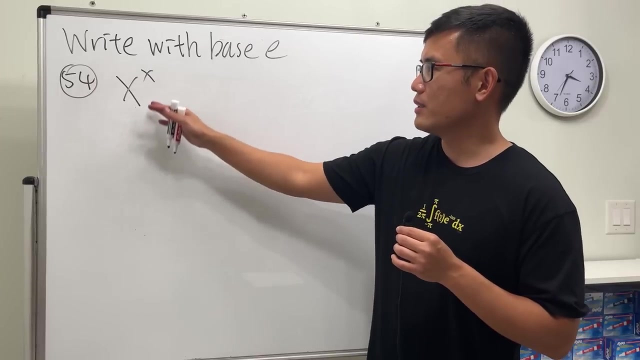 is number 54. i'm talking about x to the x power. it's pretty strange, huh? it's like the first time we see this. we have a variable for the base and then a power for the power. a variable for the base and also a variable for the power. we don't like that. we like to have base being e right. 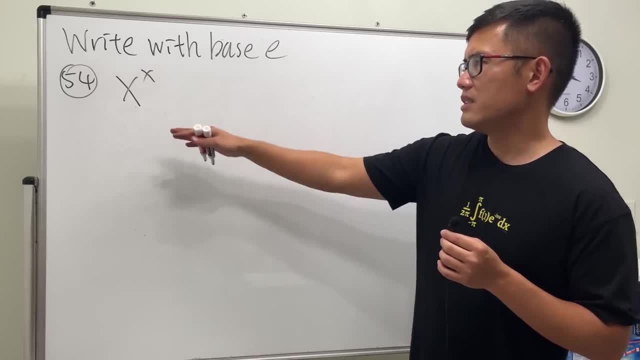 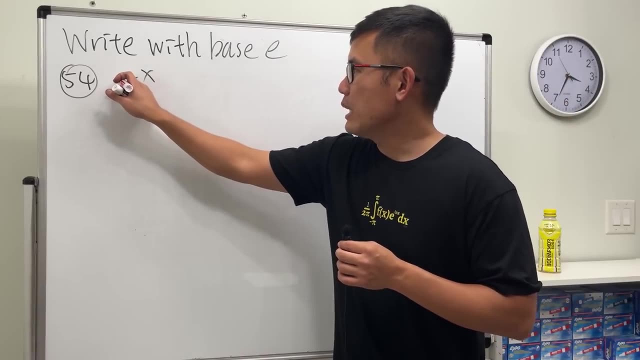 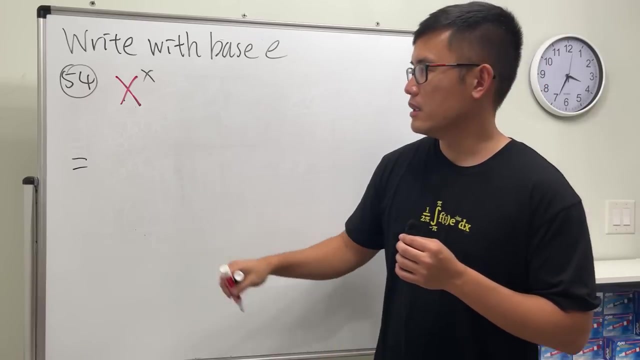 e for the base for exponential function is the best, and this is like a combination of like. let's just do it anyway. so we see that we have x here. that's not what we want. we want to have base e. so what can we do? that's what we did earlier. we are going to first write this as e, but then 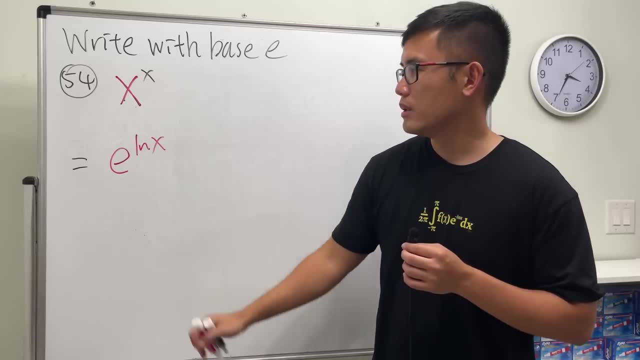 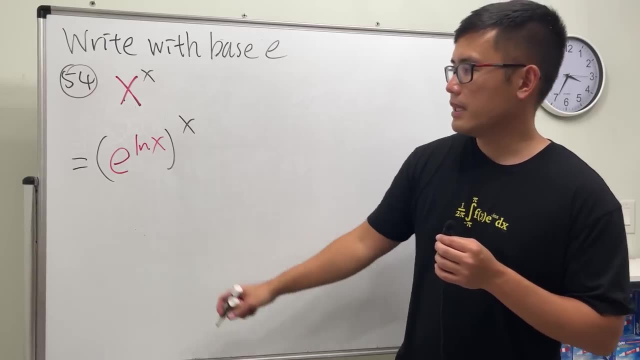 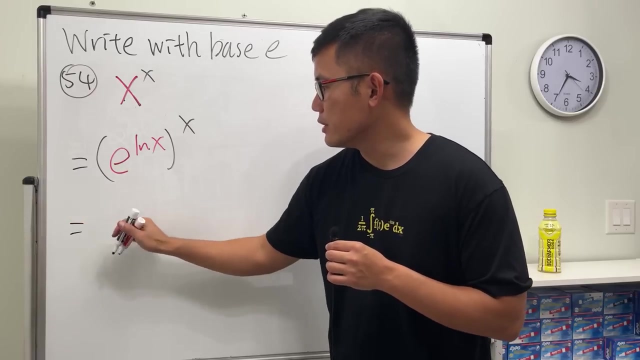 remember e and ln x cancel right, so we can write x as e to the ln x and then raise to the x power. but now we have e to this power and then to that power. so what can we do with the powers? multiple like them. so this right here is just e to the x times ln x power. 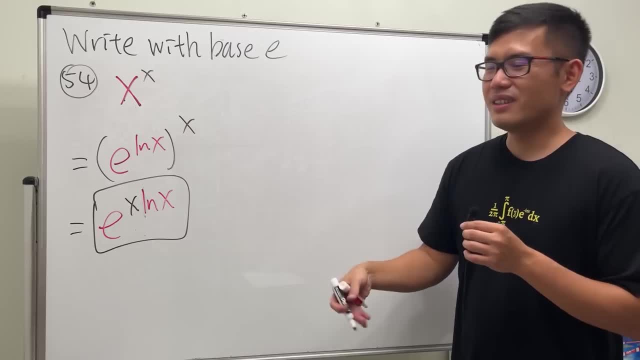 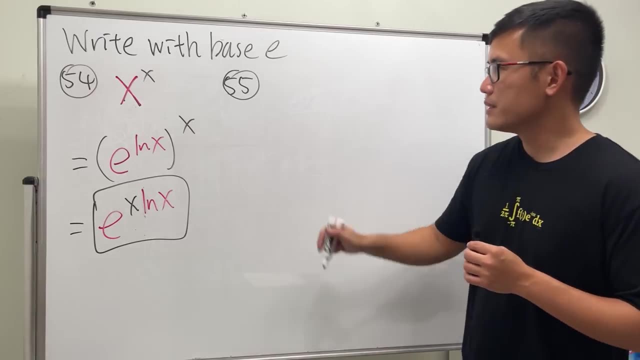 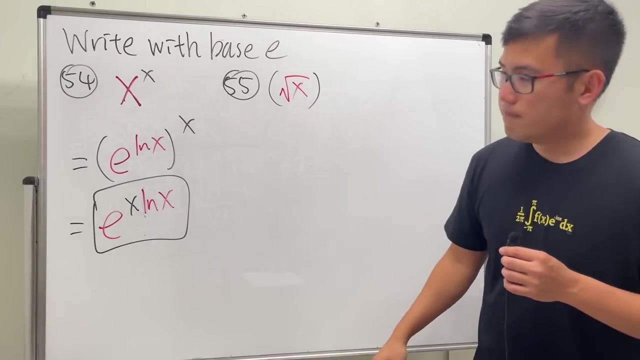 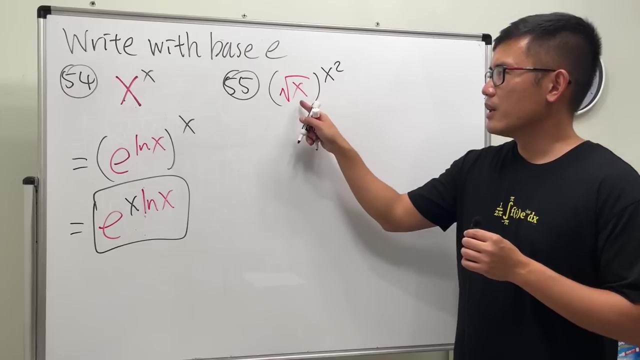 pretty crazy stuff, huh. so it's kind of like what we did earlier. right, just how to think backwards. okay, let's try another one number: 55 square root of x raised to the x square power. yeah, crazy, huh, but don't worry, what square root of x? let's write it down. let's write it down like: 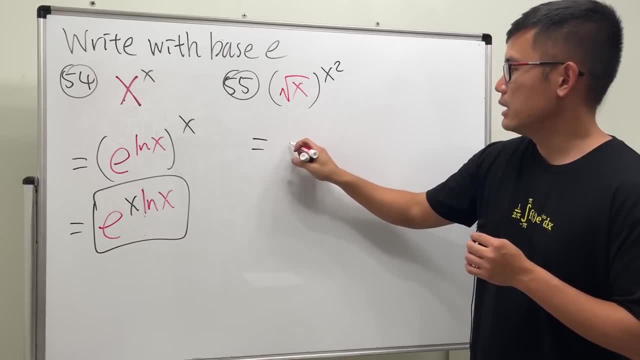 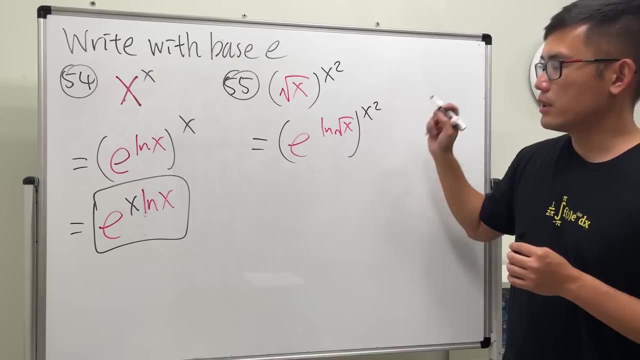 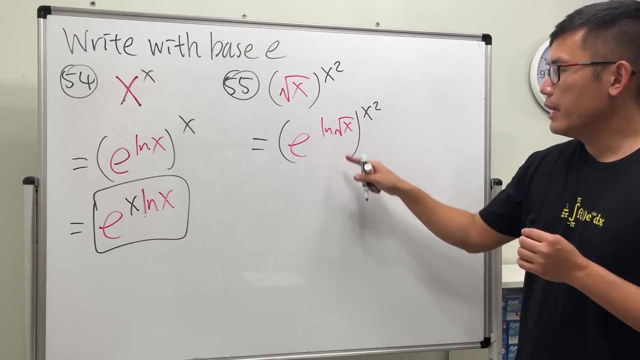 that first. so this, right here, we can put it as e to the ln of square root of x and then raised to the x square power. yeah, whatever this is, you just put inside the ln, because e and ln will cancel. and then we can of course multiply the powers. so this is e, and then we have the x square. 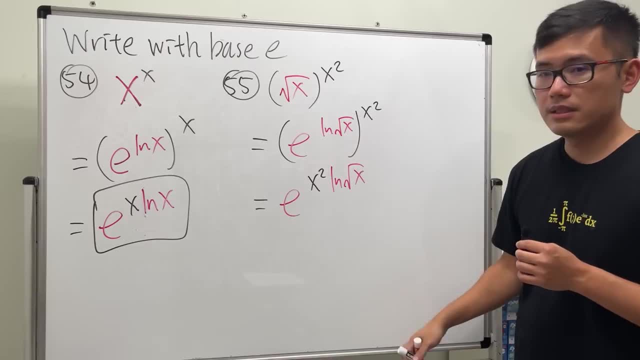 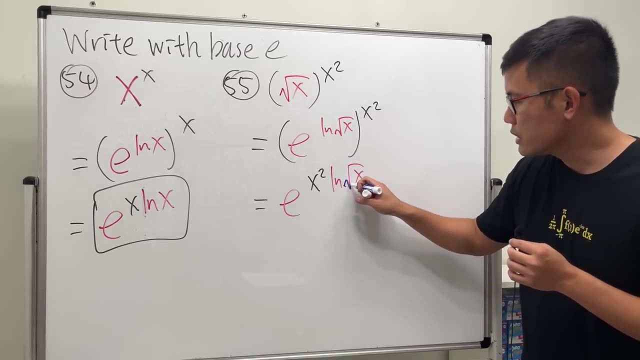 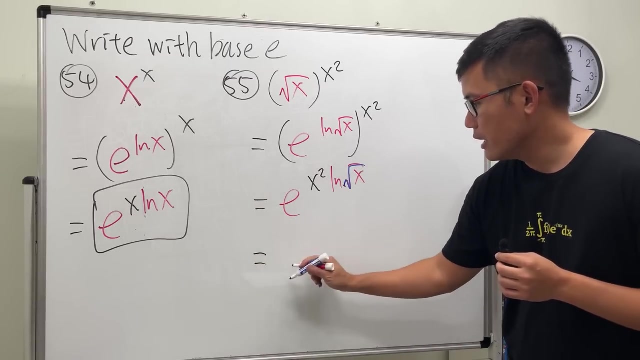 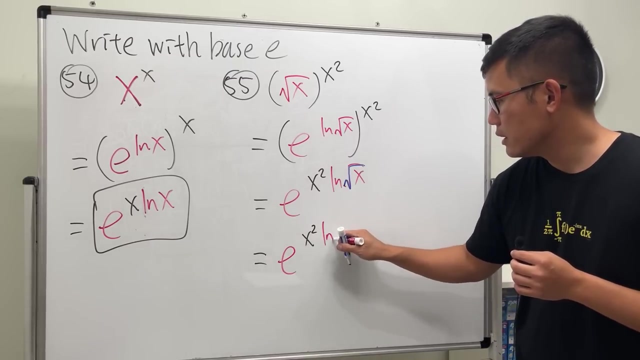 ln of square root of x like this. but in fact here we can actually continue a little bit more, because when we have the square root it's actually the same as one half power. so in fact i'm going to rewrite this as e, and then we have x squared and then we have ln of x to the. 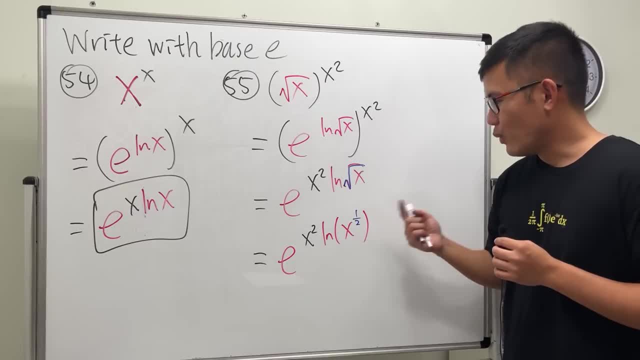 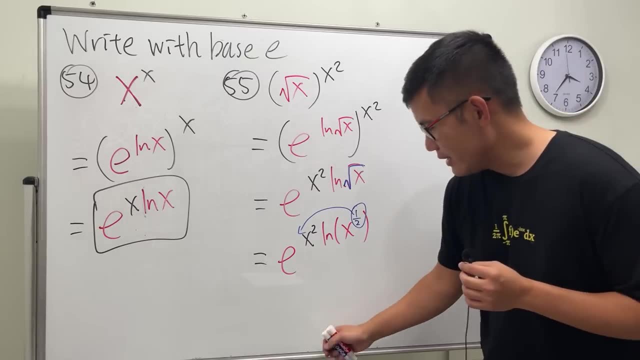 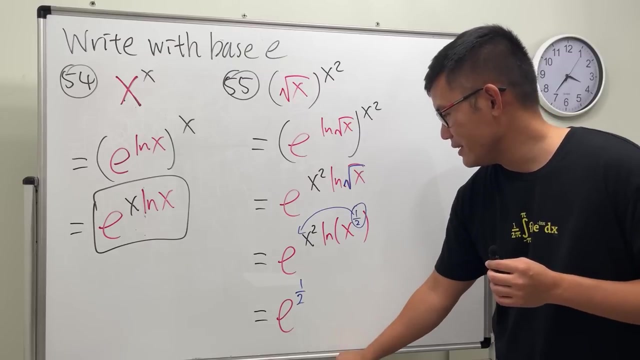 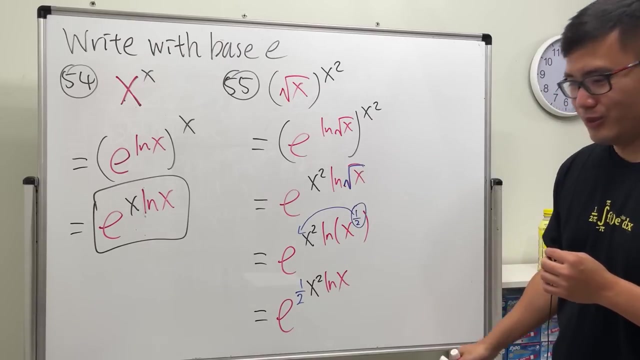 one half power like that. why, yes, we can put the one half to the front right, thanks to the log property. so, finally, i'm just going to present the answer for you guys as e and then one half, and then we have the x square and then ln x. yep, just like that, super, super cool. 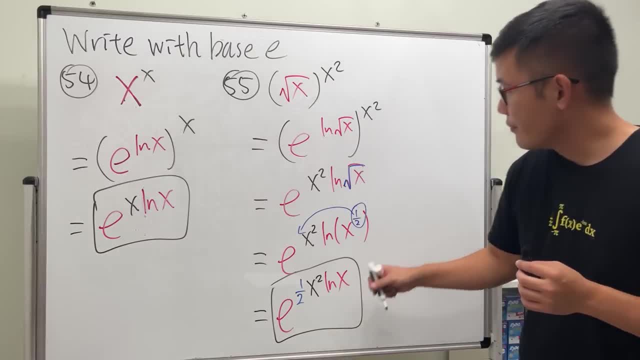 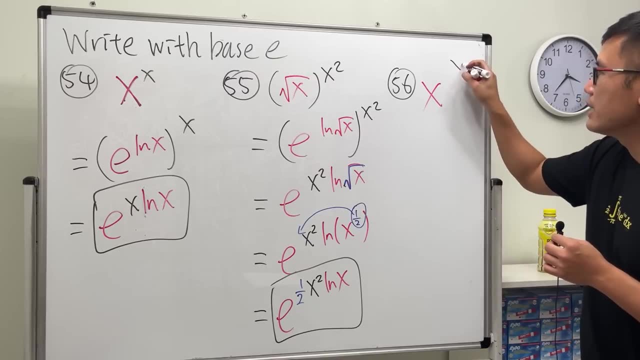 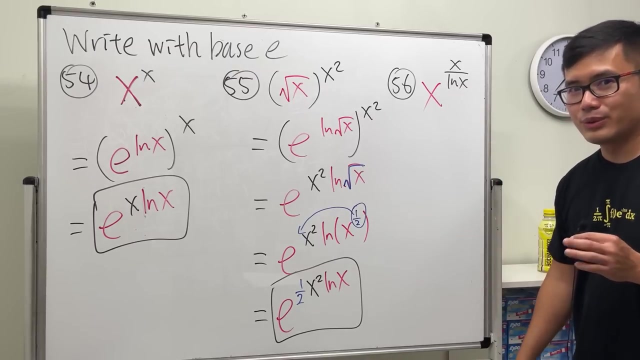 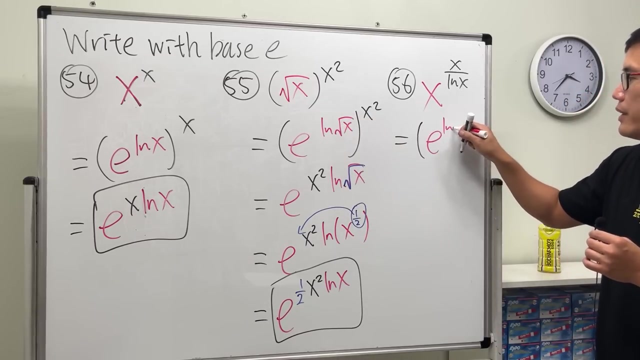 okay, and then we have one more, one more, number 56. i have x for the base and then the power is x over ln x power. you're not going to believe like how this simplifies too ready. let's go x again. let's do that right. so x is just e to the ln x power, but this time we raise that to the x over ln x power. 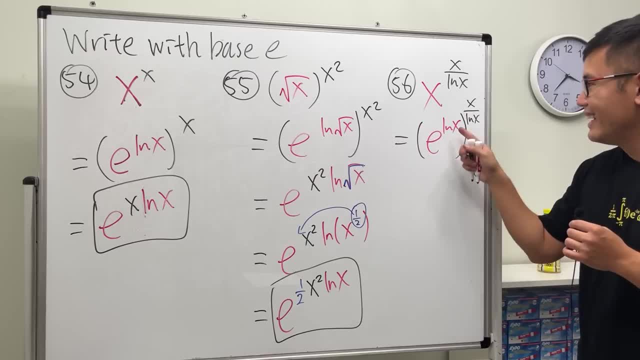 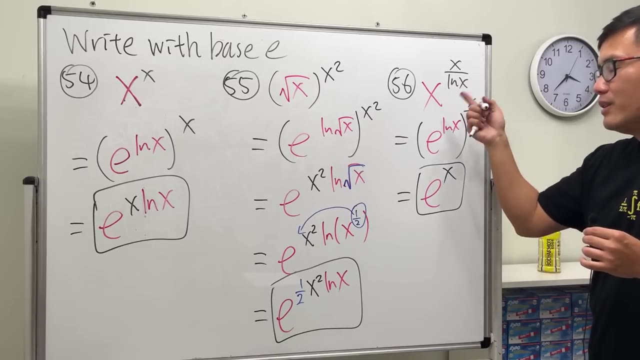 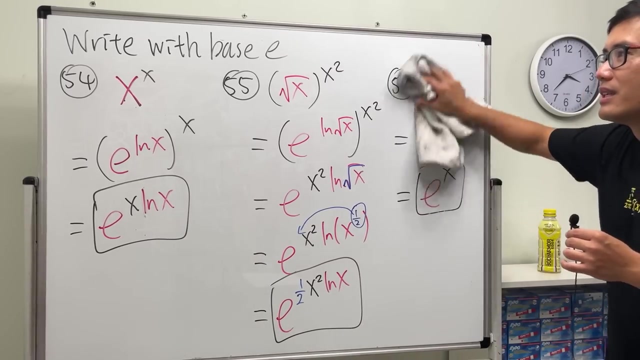 what would this two power do? we multiply along the x and this cancel. so in fact this right here is nice equal to e to the x power. yeah, so this can be like a very scary expression, but it's really just nicely: equal to e to the x, yeah. so just three quick examples that how you write like a crazy. 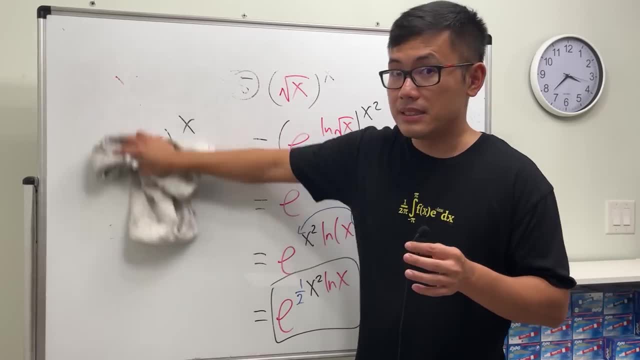 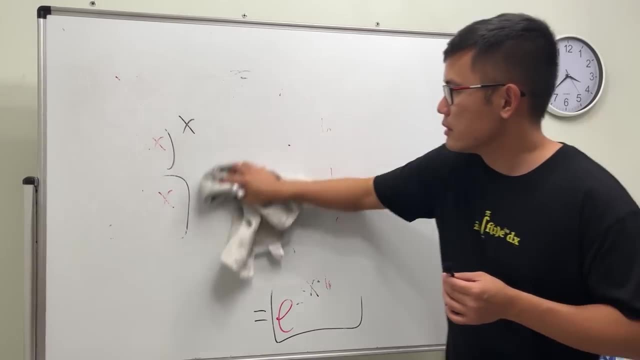 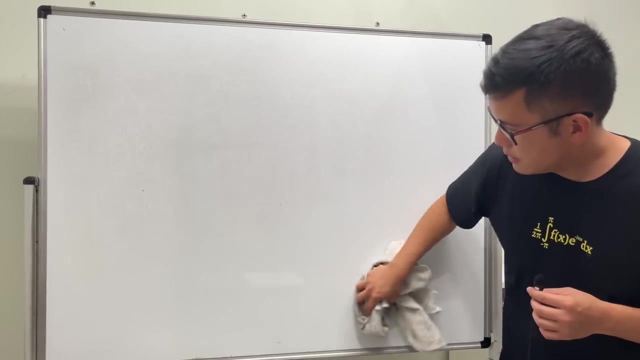 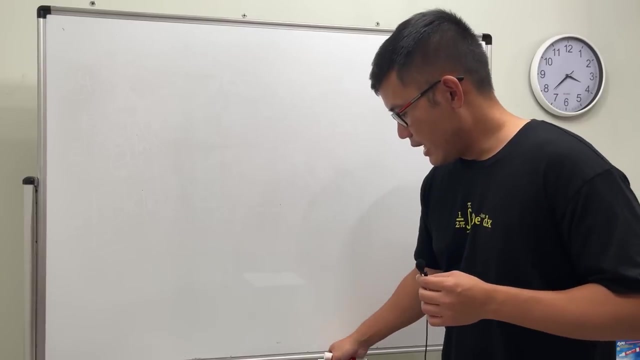 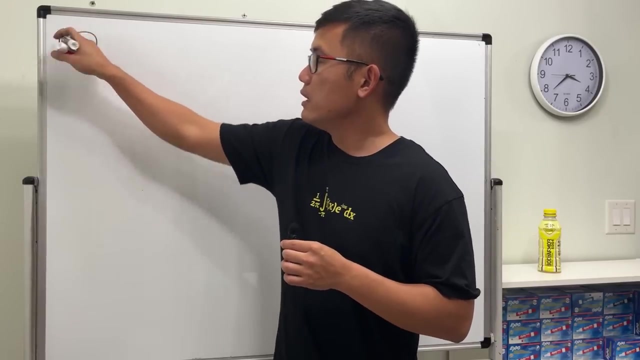 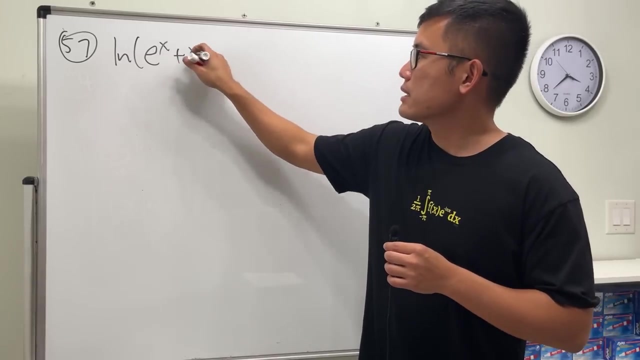 function right, you've got some power. but if the base is not e, then you do these kind of things to phase e. all right. now for the rest of this category we'll just practice some more logarithmic properties. so number 57: notice that we have ln of e to the x plus x, e to the x. 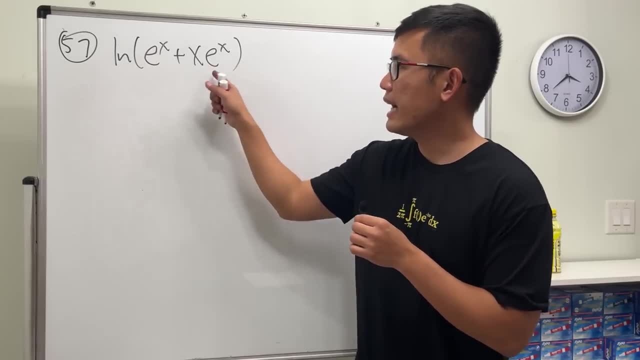 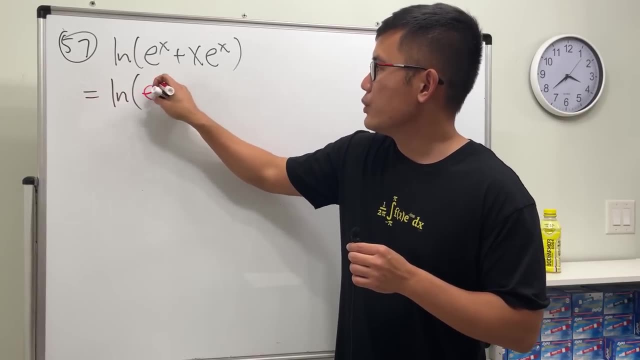 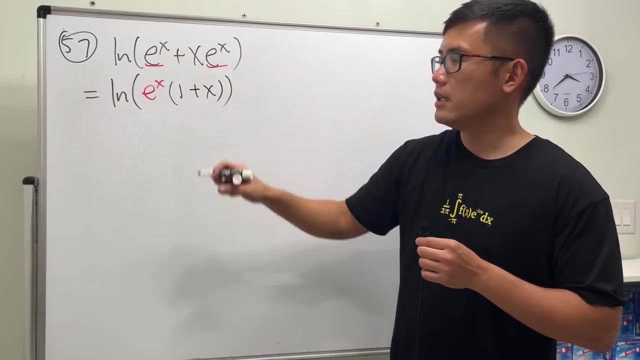 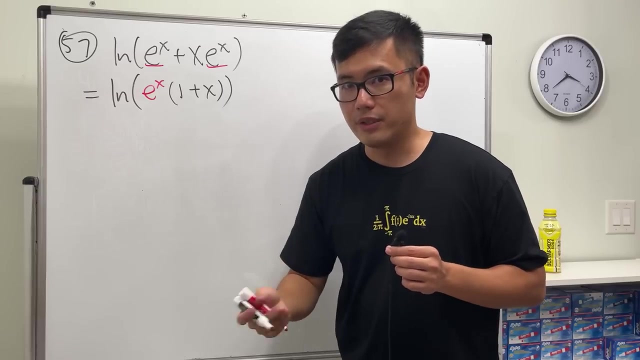 so what can we do in this case? if we look inside, both of them have e to the x. we can factor it out. so in fact, this right here becomes ln of e to the x right, and then the leftovers are 1 plus x, and the inside here is now a product of two things. ln of a product. it's a sum of the lns. 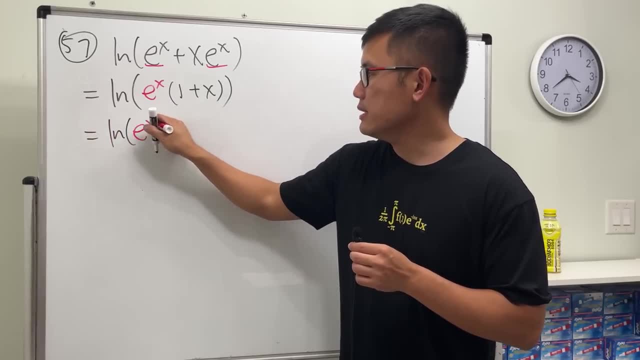 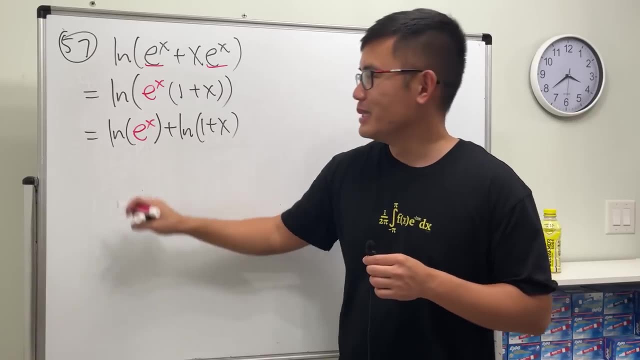 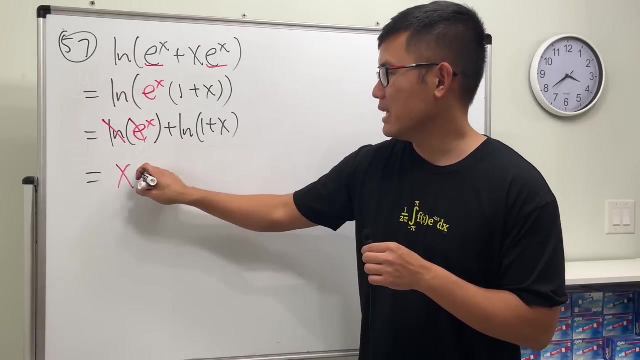 so we can write this as ln of the first thing, which is e, to the x, and then we add ln of the second thing, and what's the first one? yeah, ln and e can solve like that as well, because they are inverse of each other. so finally we get x plus. 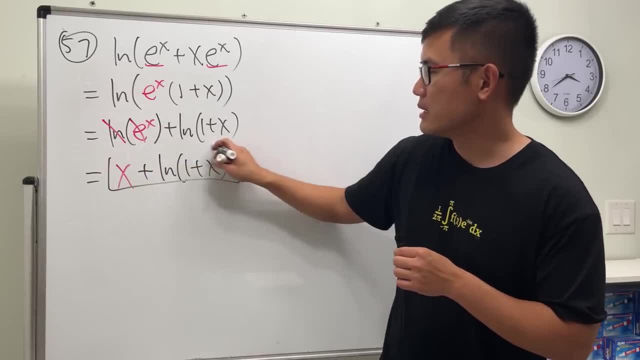 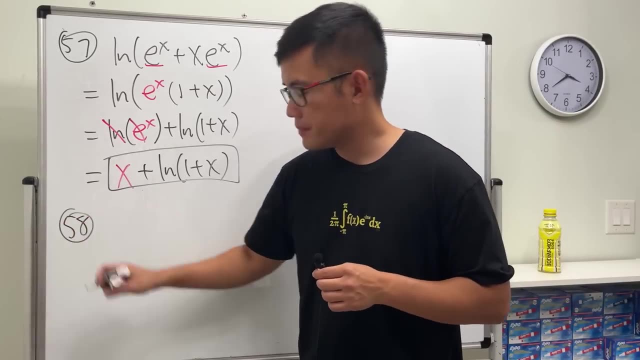 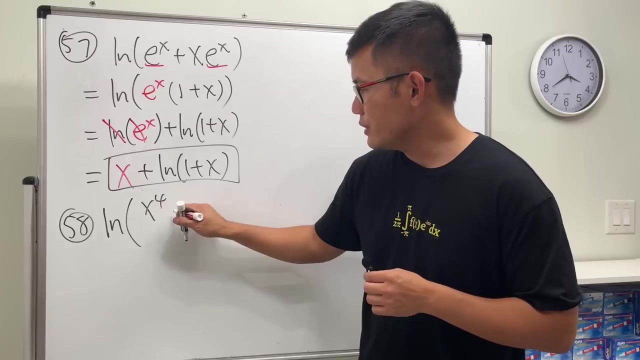 ln of 1 plus x. so that will be the simplification for this one. okay, i'm going to fill in number 58. here, number 58, we have a big expression, ln, of x to the fourth power, and we have the square root, x, square plus 1 over x plus 5.. 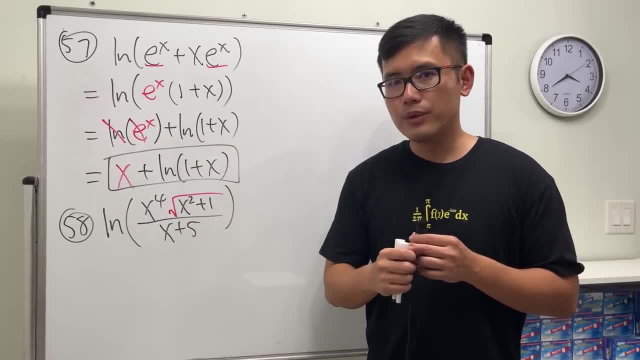 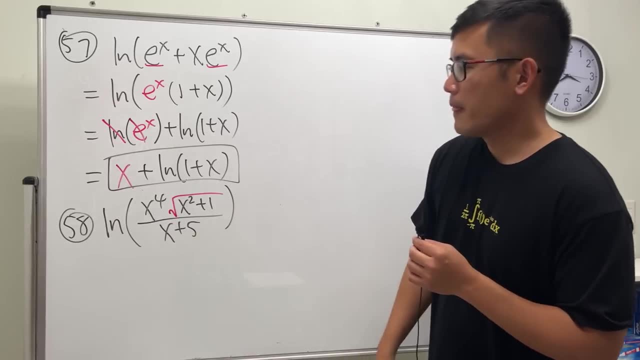 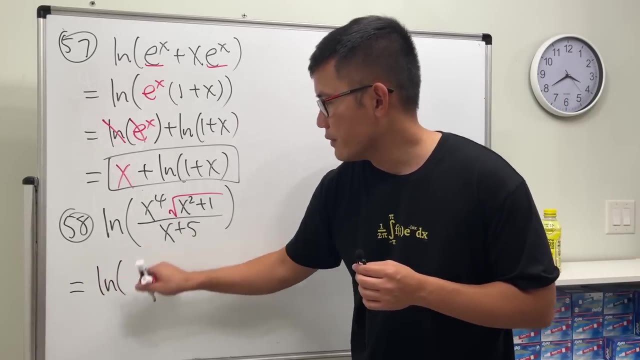 so similar to earlier. when we see product, we are going to break it apart as a sum, we are going to break it apart as a difference and we're going to do both of them at the same time. ready first one: we will have ln of this thing, which is x to the fourth power. 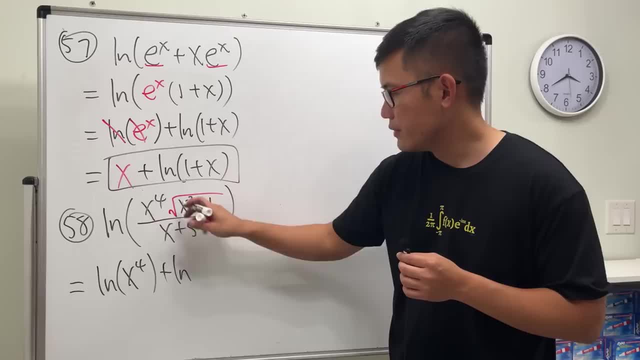 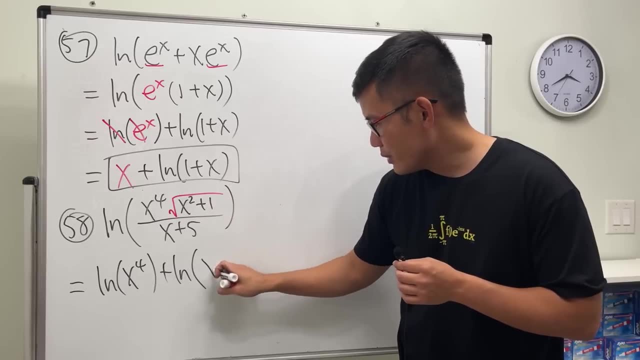 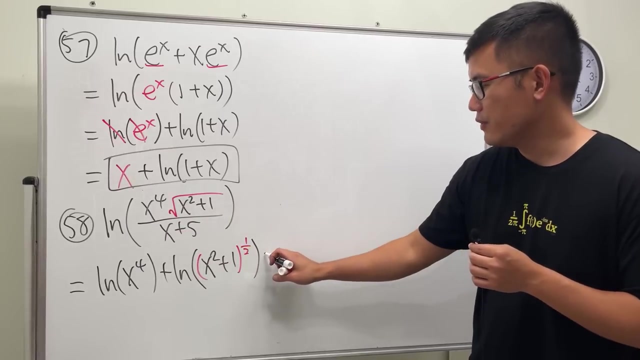 it was a product. so we add ln of this. i'm going to write the square root as a one half power, just like what we did earlier, huh. so i'm going to put down x squared plus 1 and then to the one half power, and then this right here is on the bottom. so it's a difference as minus ln of x plus 5.. 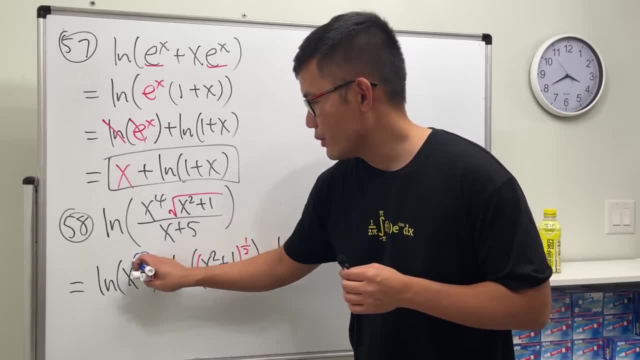 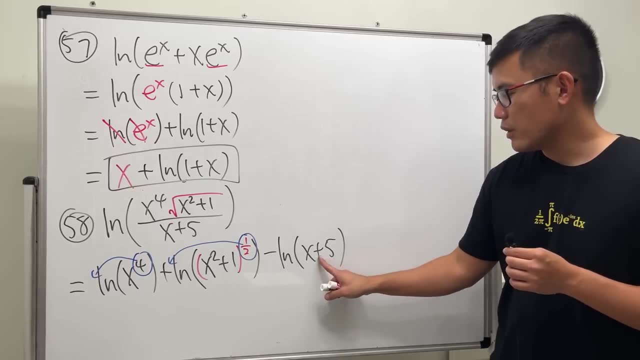 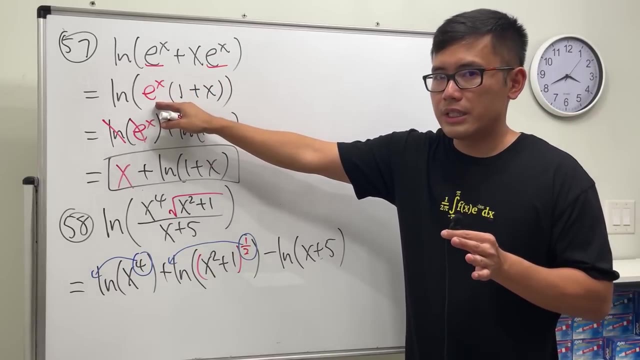 now we can put the power to the front, the power to the front, and then be really careful when you have a sum inside of the natural log. we cannot break them apart. earlier we were able to factor out the l. we were able to factor out e to the x, so it was a product. 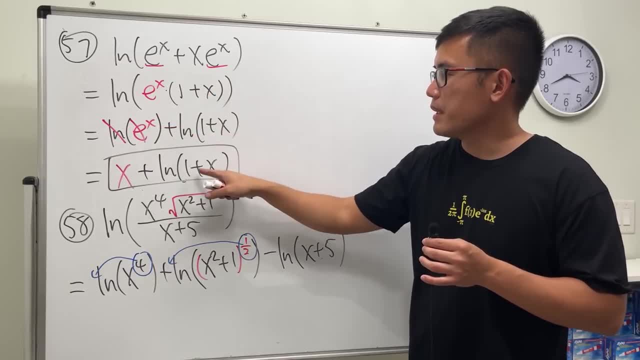 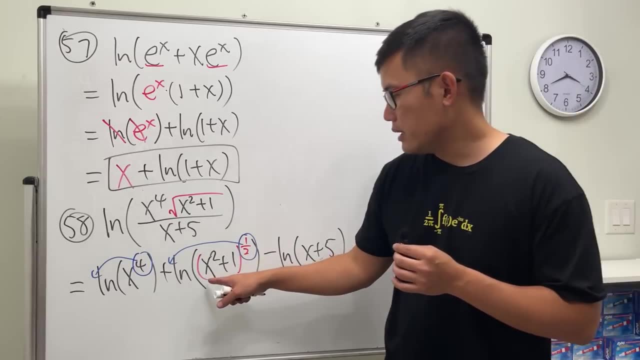 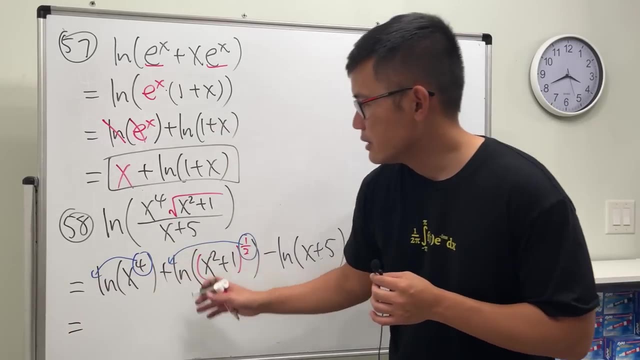 so we can break them apart. if it's a sum like ln of 1 plus x, we couldn't do a thing, so we leave it. so this one, we will have to leave it too, and likewise later on you will see, we just have to have one half at the front. that's the most we can do. anyway, though. this right here is the 4. 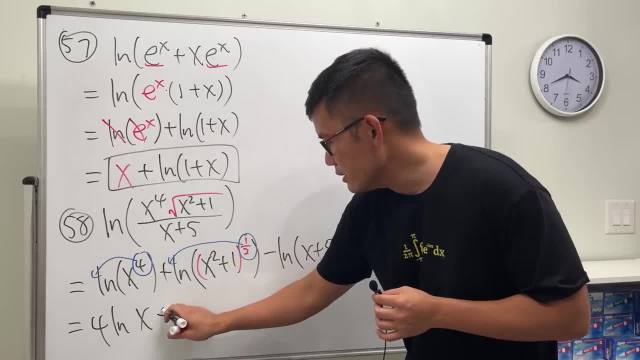 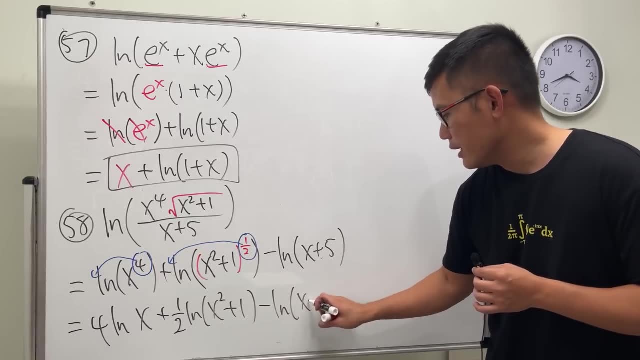 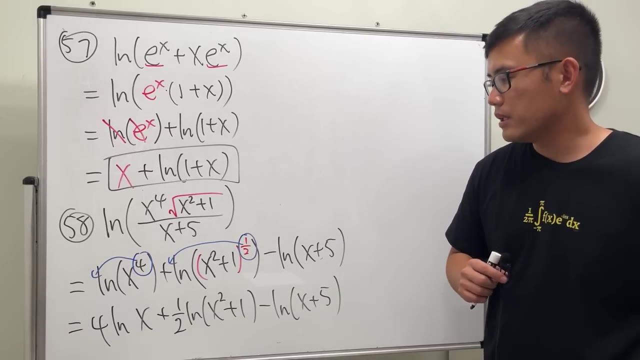 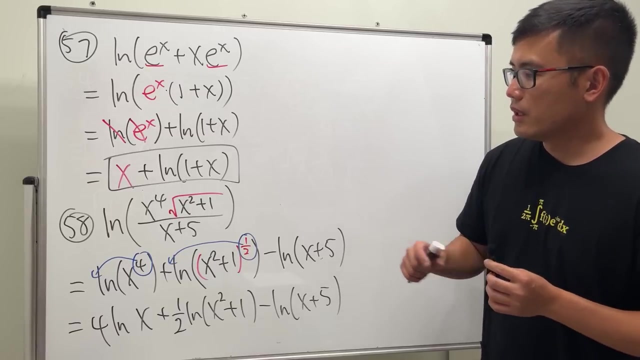 and then ln x and then one half at the front, ln x squared plus one, and then lastly, minus ln of x plus five. okay, and there's one little issue i want to address for this right here. if you take a look right here originally, can x be negative one. 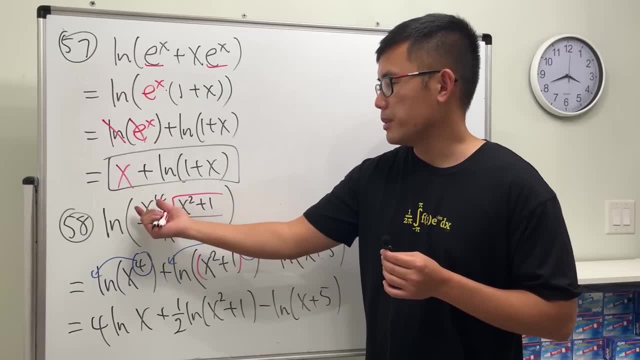 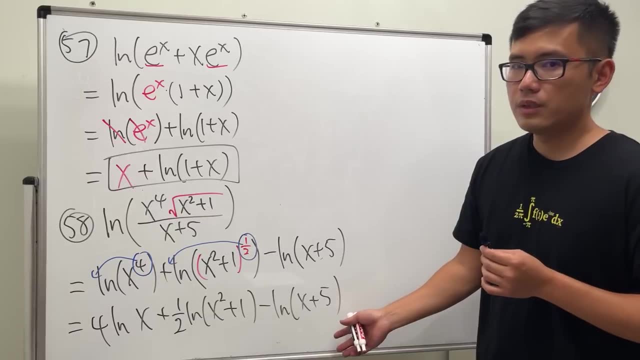 yes, because negative one put inside here, then that will be positive, that will be positive. negative one plus five. it's also okay. but if you look at this, can x be negative one? no, because we have one of negative one. we cannot have negative number itself with that one, right. 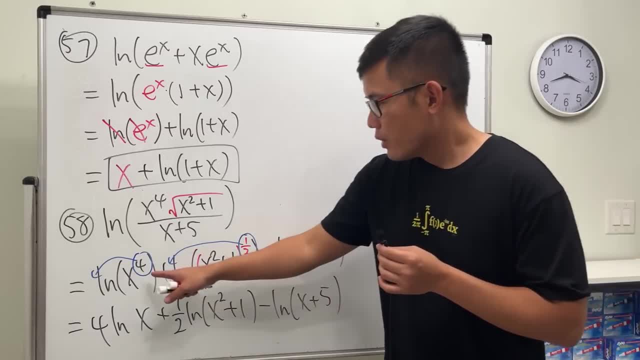 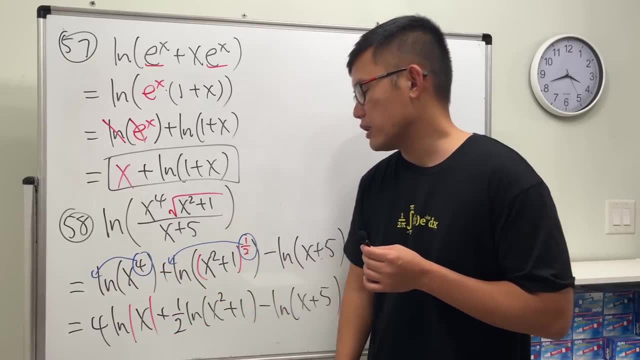 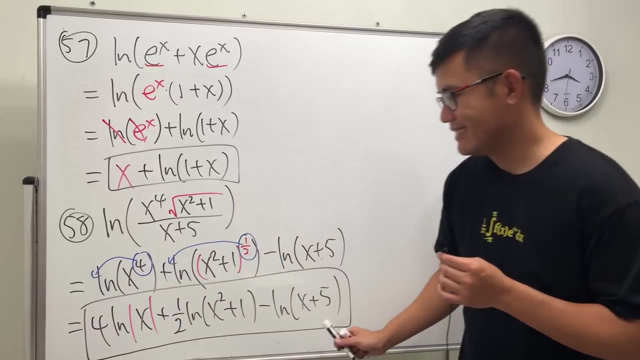 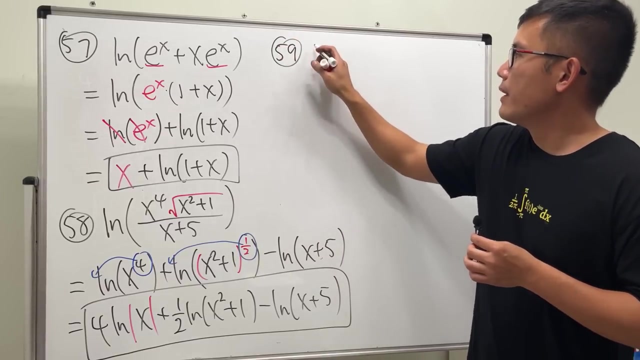 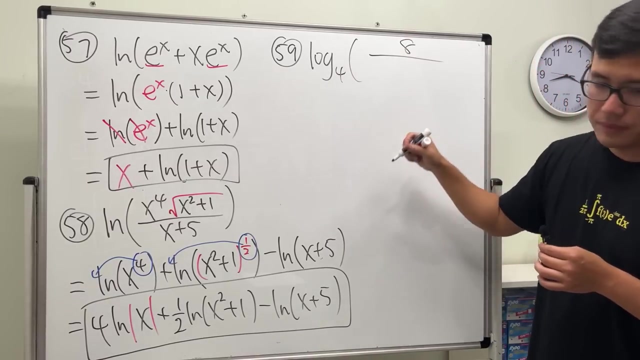 so something's wrong. here's the deal. we have an even power here. when we bring that to the front right here, to maintain the same domain, we will have to attach an absolute value. so that's a little thing, all right, done, okay. number 59: log base four eight over the fourth root. 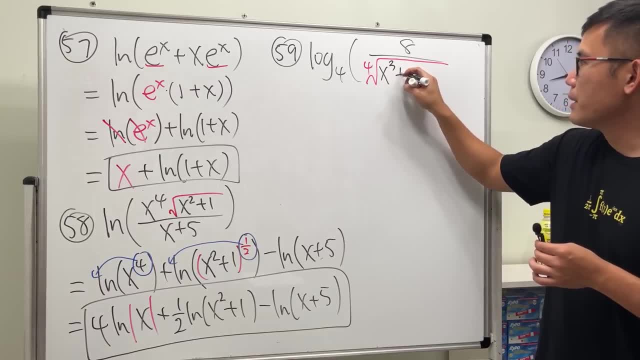 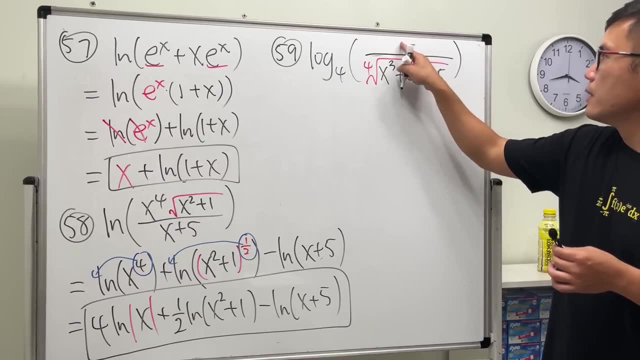 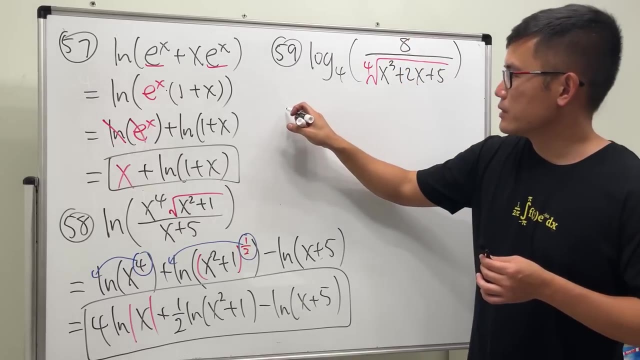 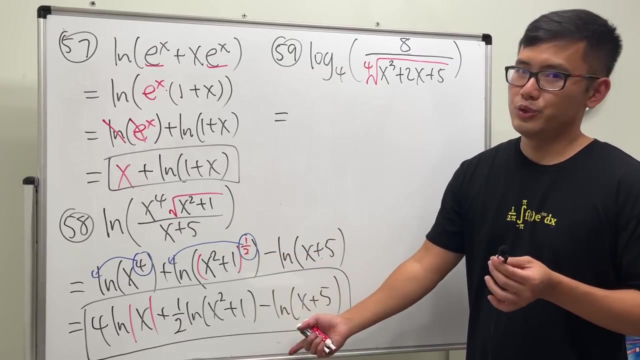 of x to the third power, plus 2x plus five. all right, so you see how earlier we took two steps. but if you want, can you go from here to here? sure, just be really careful, right, because you know you can break it apart and then bring the power to the front, right do. 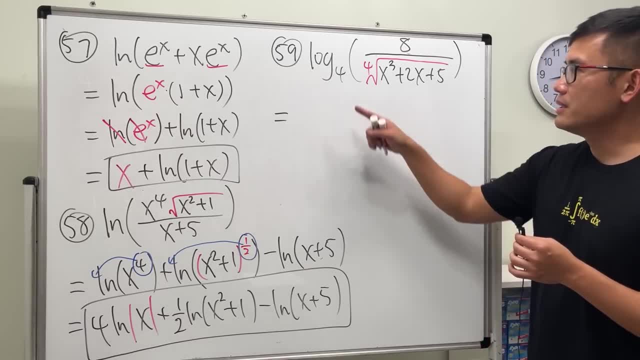 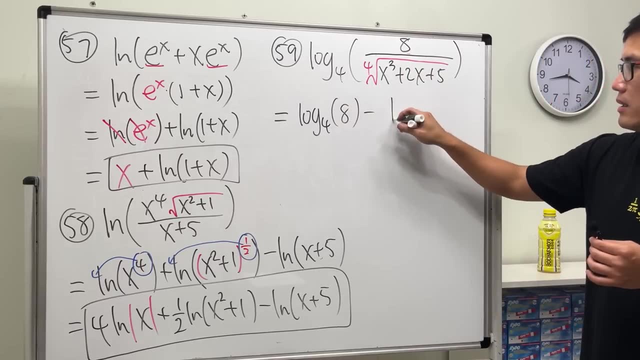 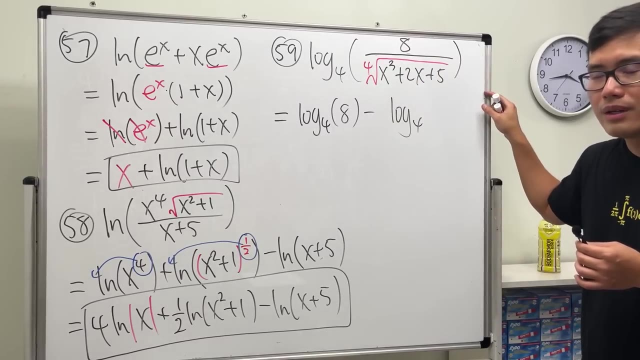 two things at a time. let's go ahead and do that right here. firstly, i'm going to have log base 4 of eight and then minus log base 4 of whatever this is. but we know this right here is the one over four power. the one over four can be. 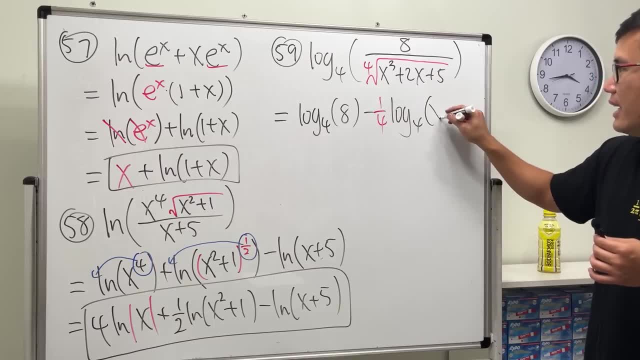 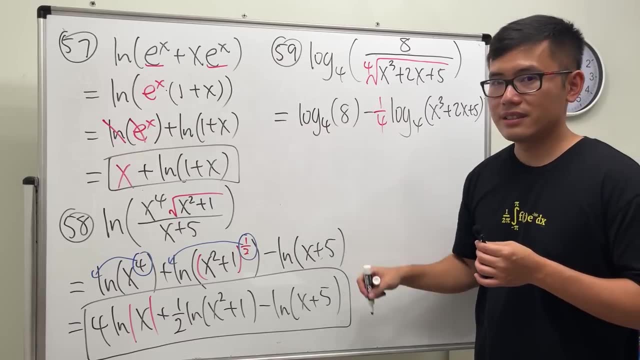 brought it to the front, and then we just have the inside x to the third power, plus 2x, plus 5, and now what exactly is log base 4 of 8? i'll show you guys a quick way to do this. that's why i come. 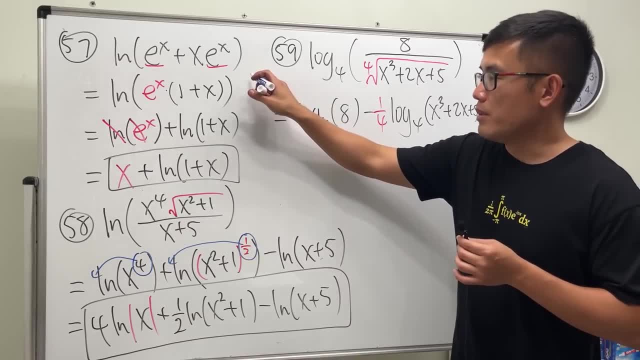 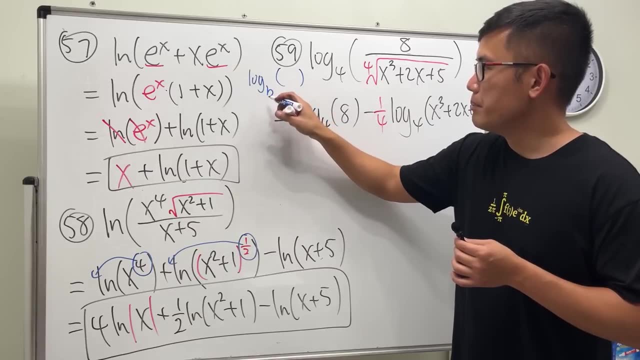 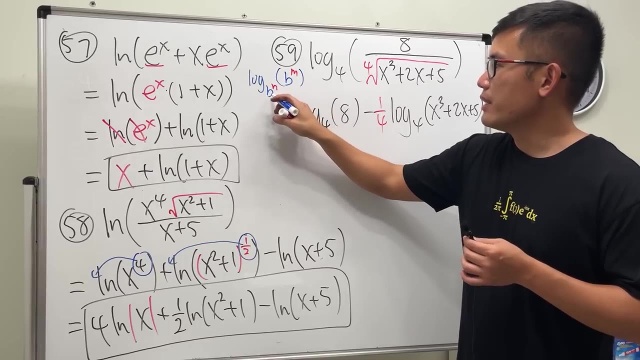 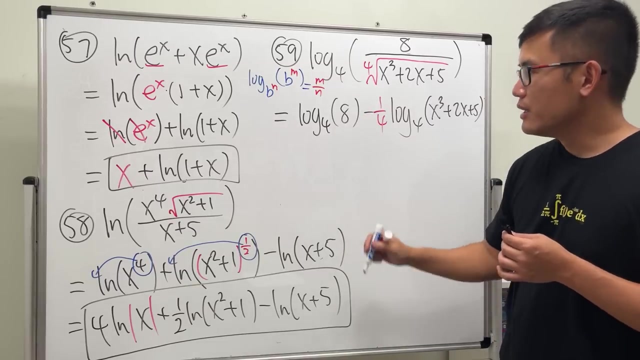 up with this question for you guys. the little formula that you can remember is when you have log, whatever base right here, if you can match b to sum n and then if this right here is b to sum m, okay, this right here is just equal to m over n, that's it. so if you look at 8, this right here. 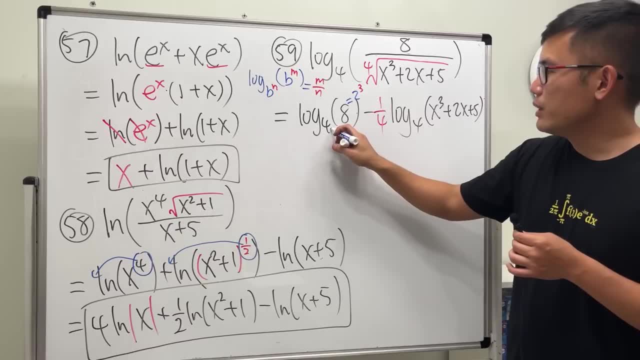 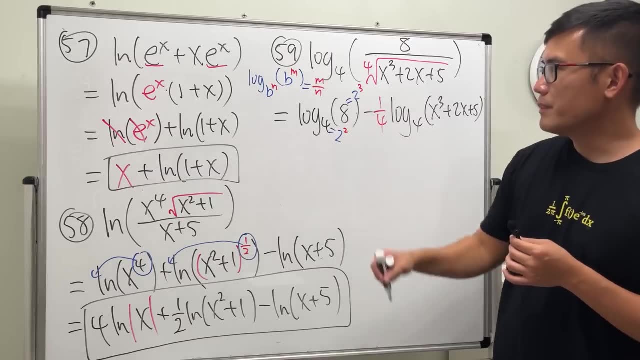 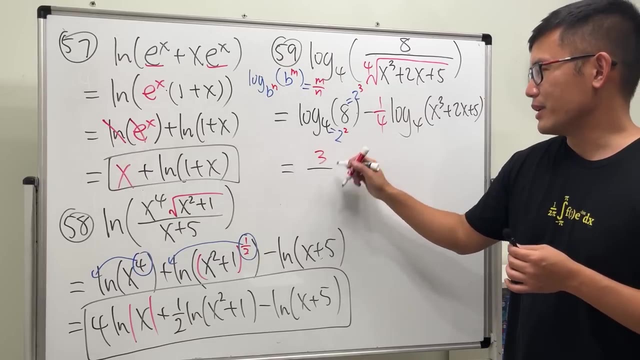 it's nicely equal to 2 to the third power, and if you look at 4, this right here is 2 to the second power. so it's just 3 over 2, right? so if you remember this, you can compute this in a very quick way. all right, i have another video on this right here. so 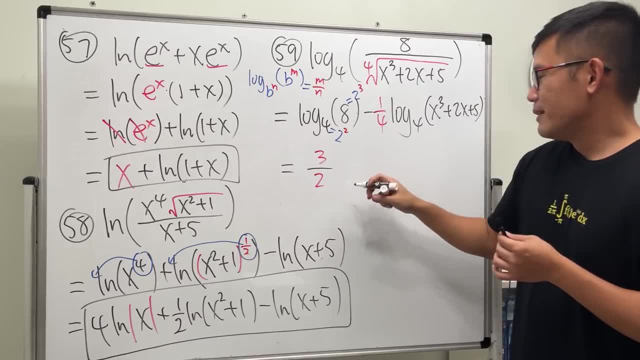 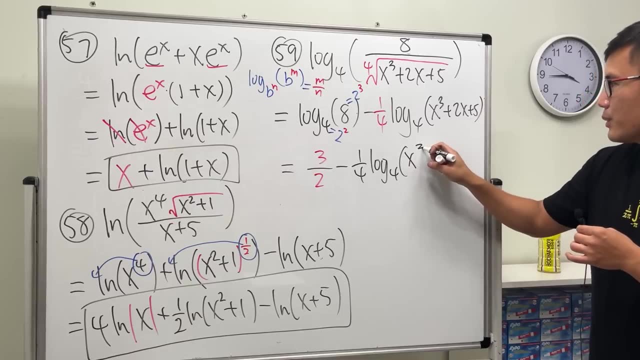 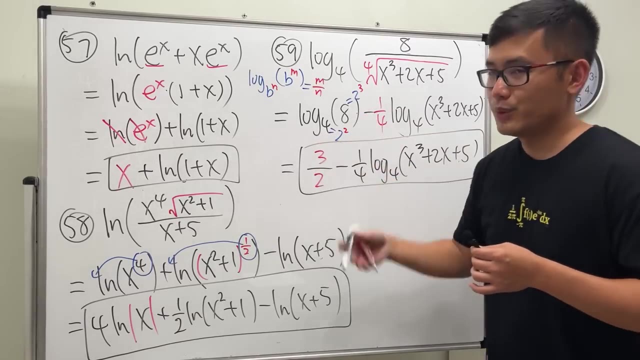 i will just link to you guys like the explanation. but yeah, that's all you have to remember for this, and then we cannot break it apart, so we'll just leave it all right. this is the best way to compute logarithm without using a calculator, so thanks. 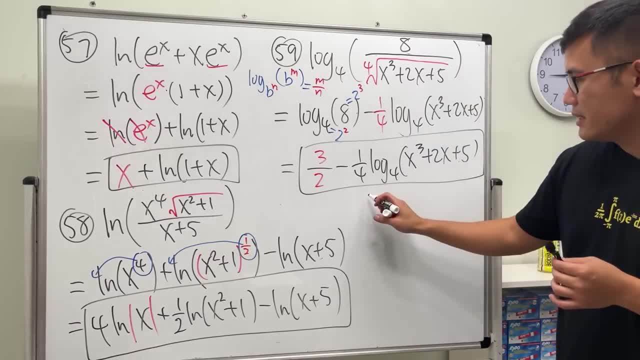 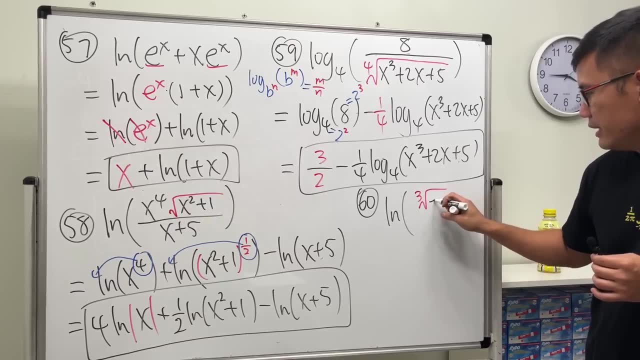 to the base and all that stuff. all right, number 60- i'm going to put it down right here: ln of the x over x squared plus 1 ready ln of this guy. but this is e to the x and then to the one third power ln and e cancel. so we have. 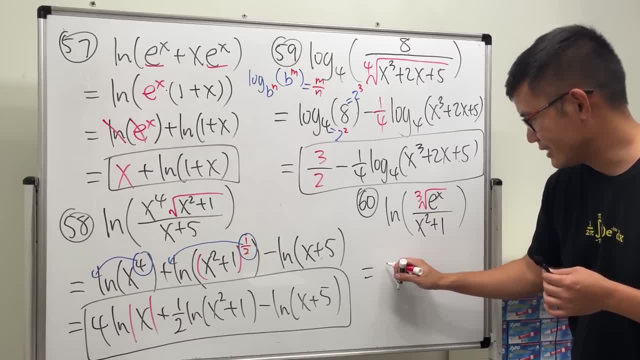 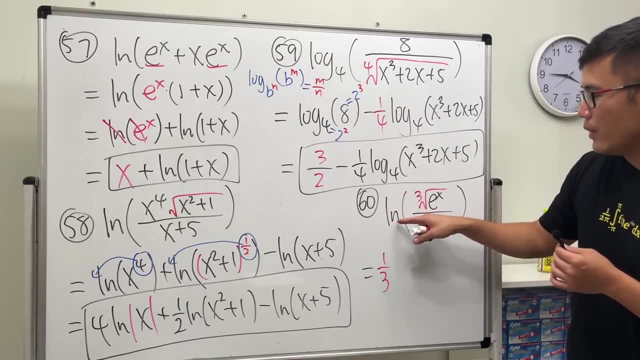 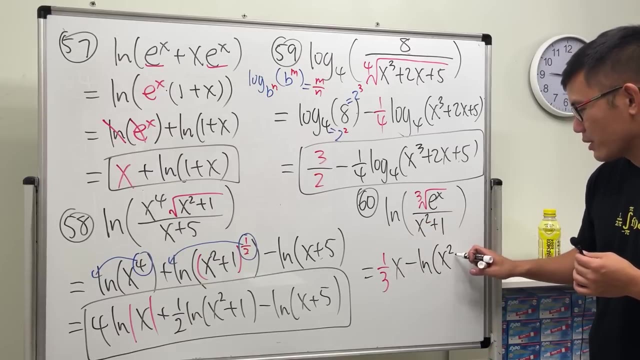 what? 1 over 3x? yes, so we actually just have 1 over 3. just think about 1 over 3. brought it to the front and then ln and e cancel, and we have the x okay, and then minus ln of that, which is x squared. 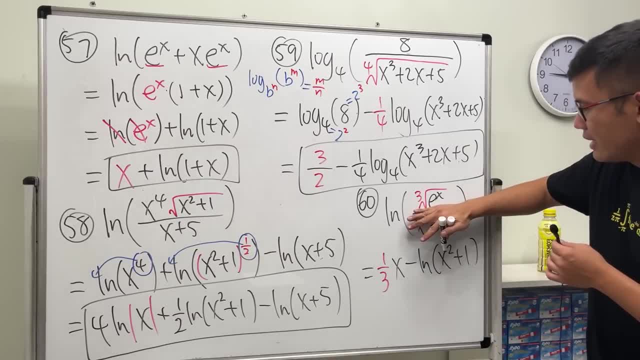 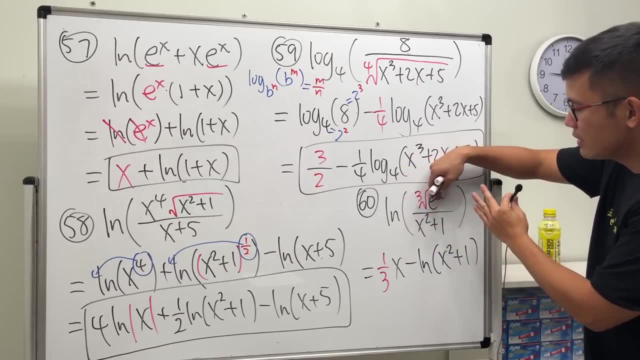 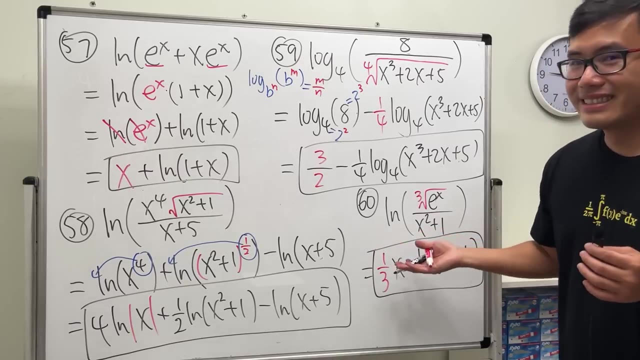 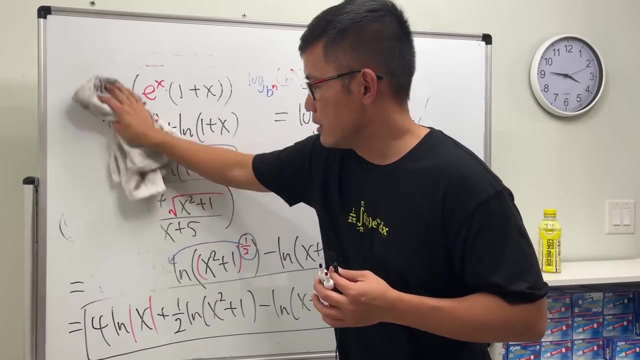 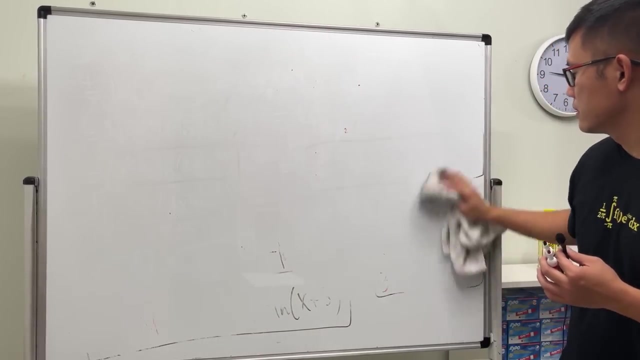 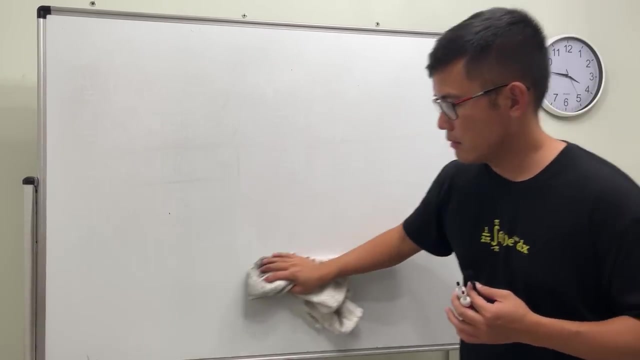 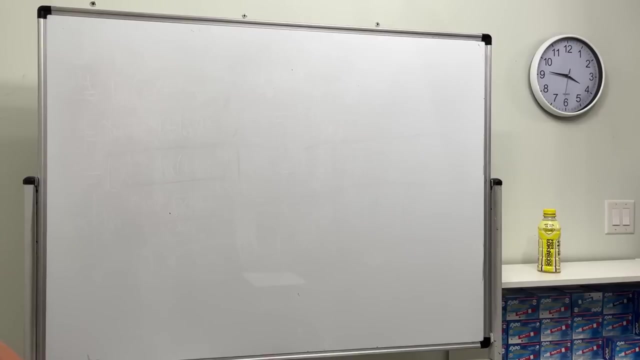 plus 1. okay. so again, look at e to the x and then to the one third power, one third to the front, so no more. and ln and e cancel. we have the x and then ln of the denominator, just like that. yeah, that's it okay. oh, 20 percent left. i will have to about. i will have to charge it soon. 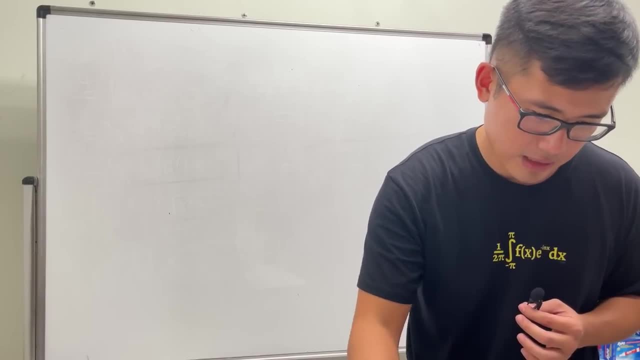 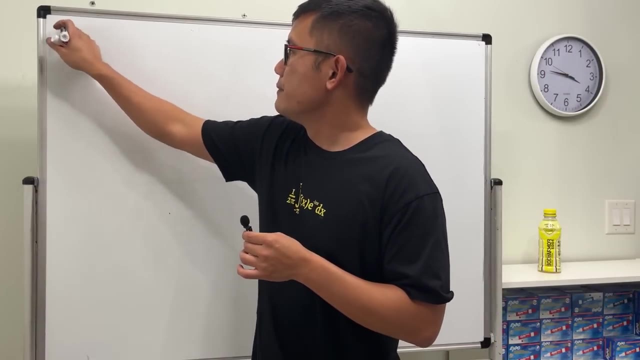 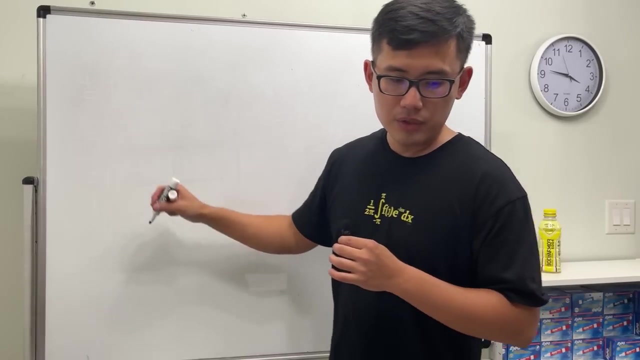 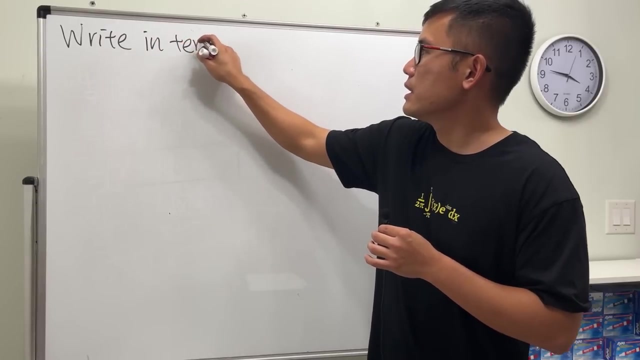 all right, number 61, number 61: we are going to write everything in terms of x to some power p. so i will just write this down: write the following in terms of x to some power. so if we have x to some power p, we are going to write everything in terms of x to some power p. 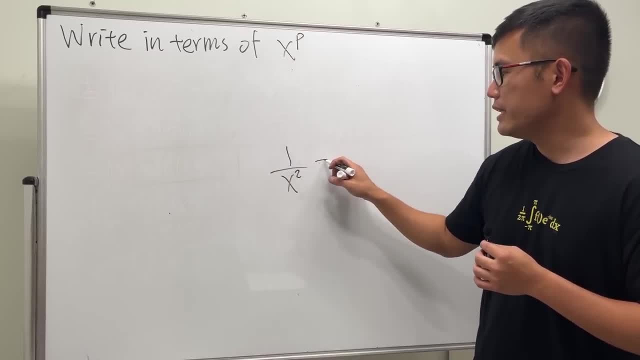 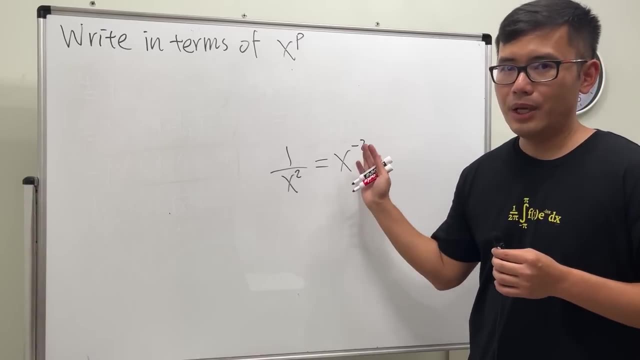 1 over x to the second power, then we will purposely write yes, x to the negative 2.. i know this is unusual, right, because usually we want to have this rather than that. but let me tell you calculus: if you want to use the so-called power rule, then we must have this form, so that's. 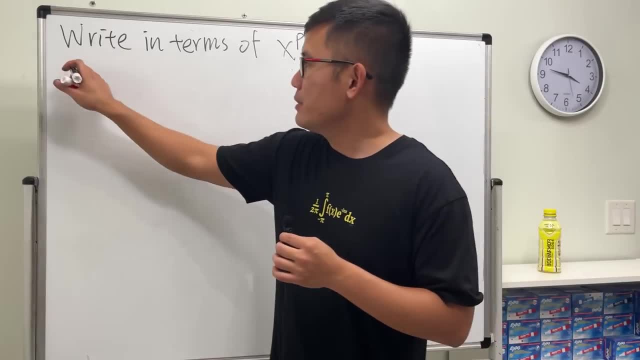 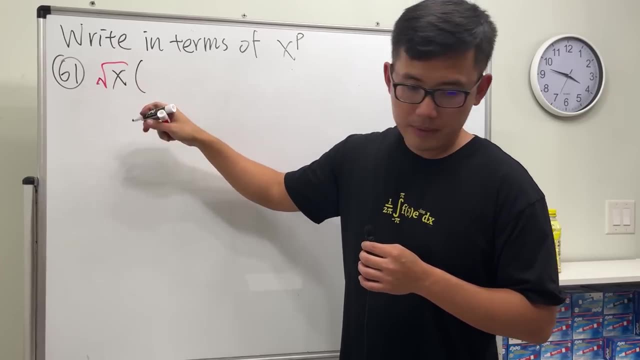 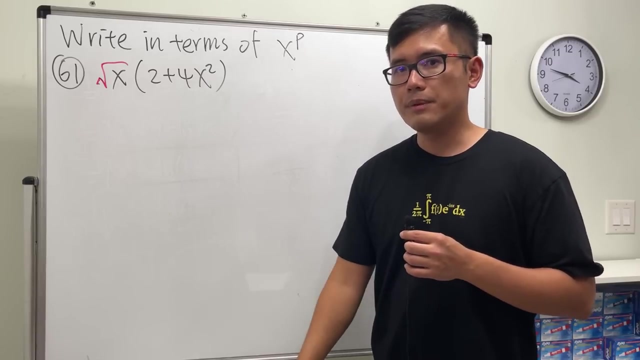 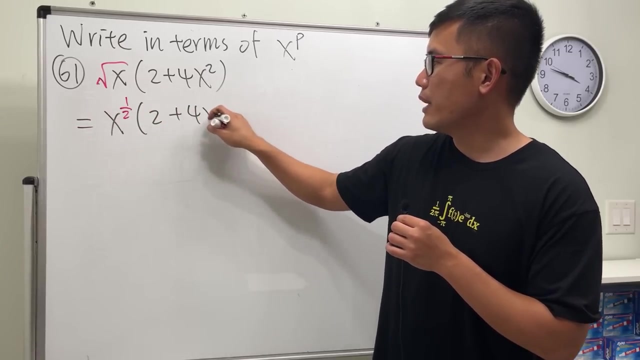 why so? let's see number 61. firstly, we have square root of x times 2 plus 4x squared. firstly, square root is the same as 1 half power, so we can look at this as x to the 1 half power times 2 plus 4x squared and then just distribute so we get 2x to the 1 half power. 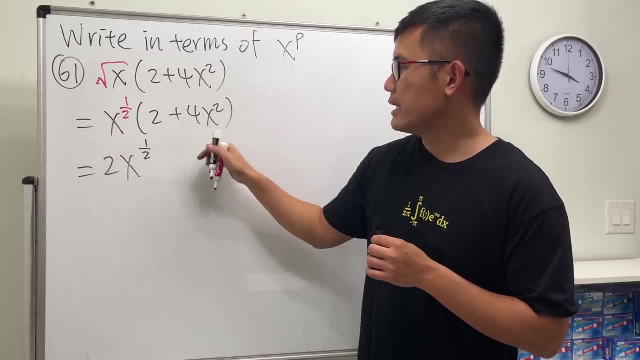 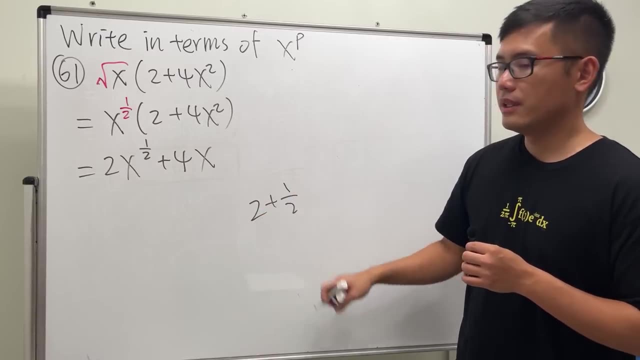 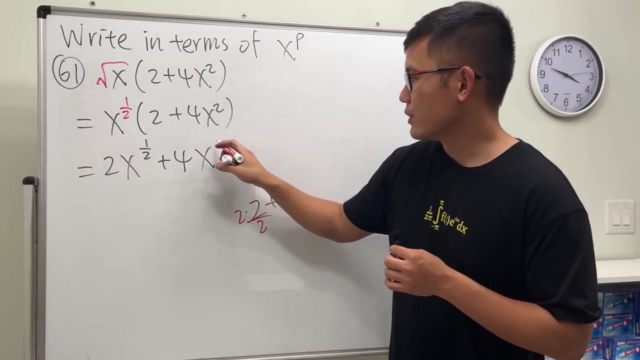 yeah, and then take this, times that. so we have plus 4x 2 plus 1 half, right, 2 plus 1 half, and then just get the common denominator all that stuff. so that's 4 plus 1 is 5. so let's put this down: 5, and then 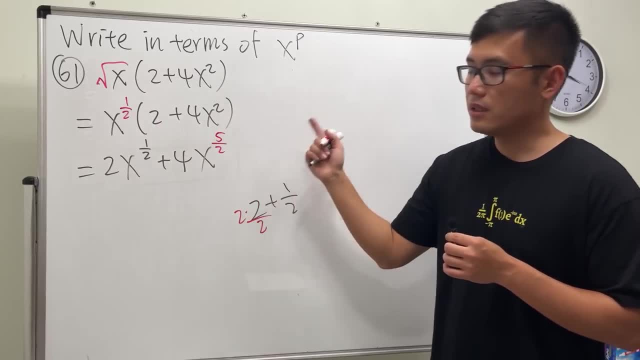 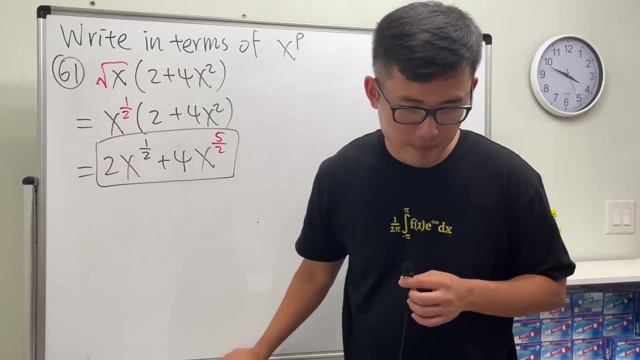 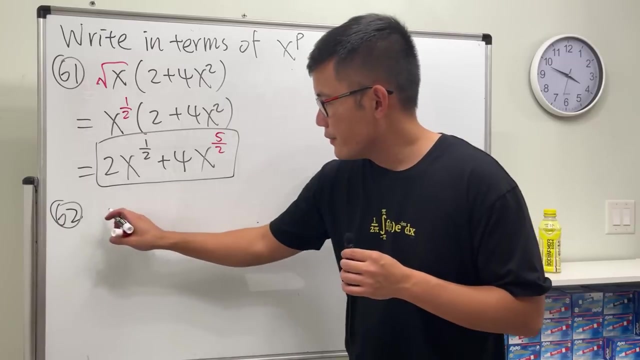 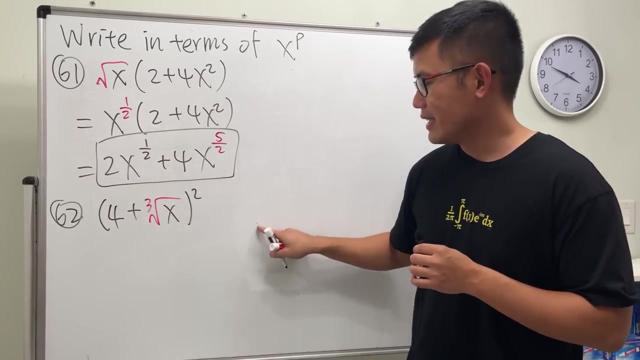 over 2. okay, so just add the exponents and that's it. that will do it. that will do it, okay. next one, number 62, we have 4 plus the cube of x, and then we square that. well, for this one i'm going to first write yes, 4 plus x to the 1. 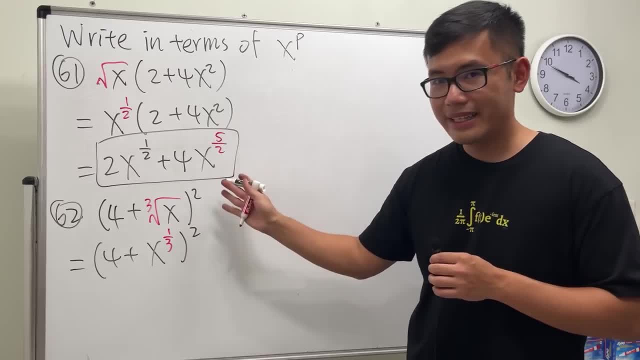 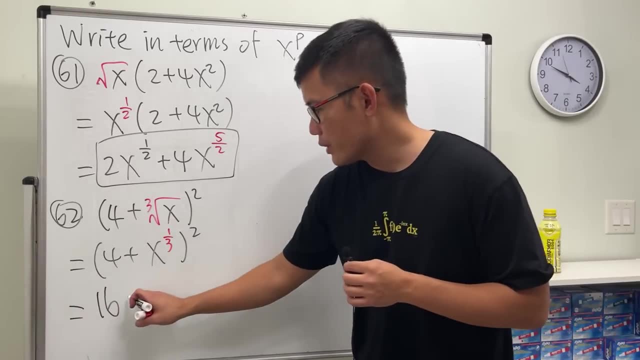 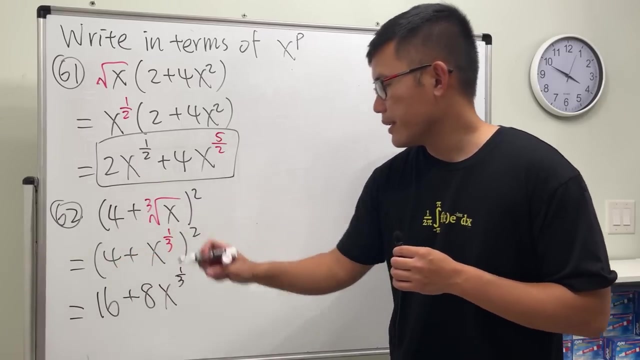 third power, but then we will have to square that and let's use the binomial formula, right? so i'm going to square this, which is going to give us 16.. next, we are going to add 2 times this and that, which is going to give us 8, and then keep this x to the 1 third power and, lastly, we add this square: 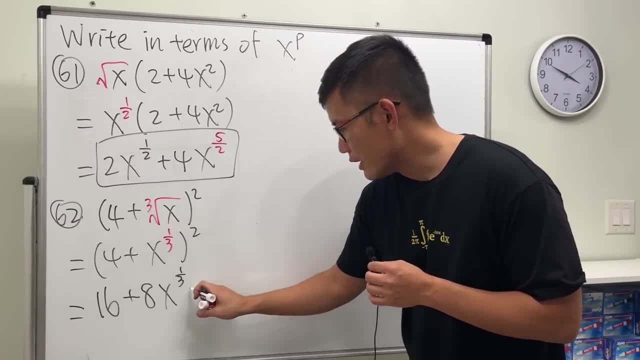 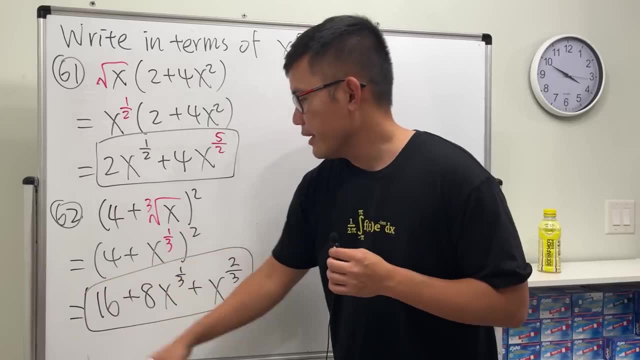 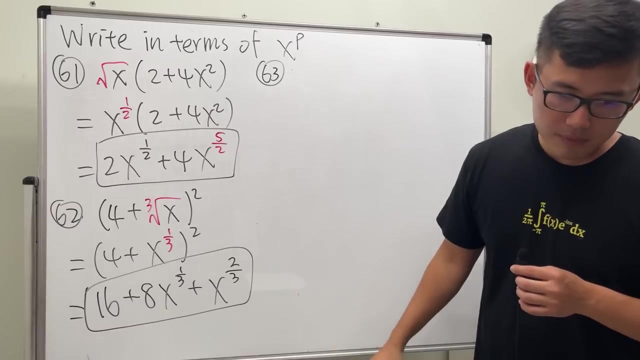 when we square this, we just multiply the exponent by 2, so we have plus x to the 2 over 3 power, just like that. then we're done. and then we can be happy and use the power rule, power rule, power rule. okay. 63, okay, this right, here is a little bit bigger multiplication. we have x squared. 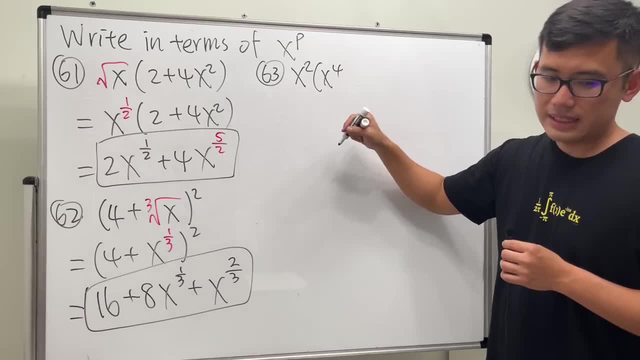 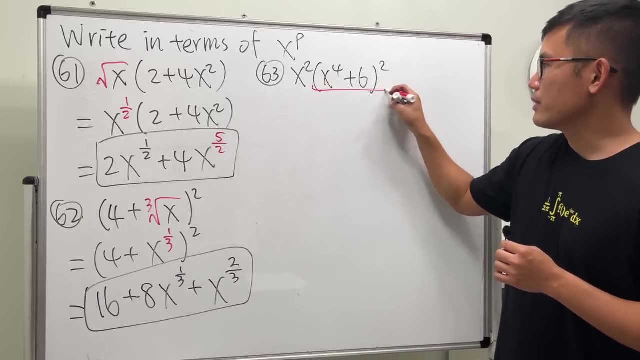 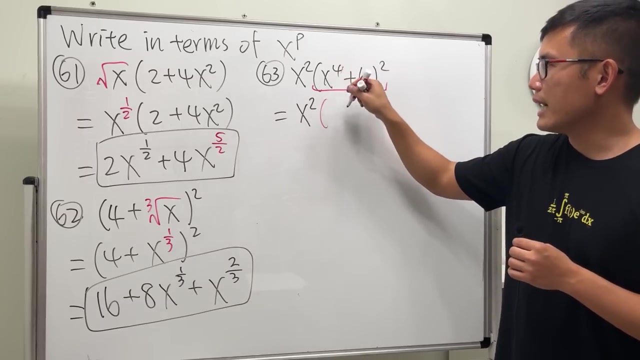 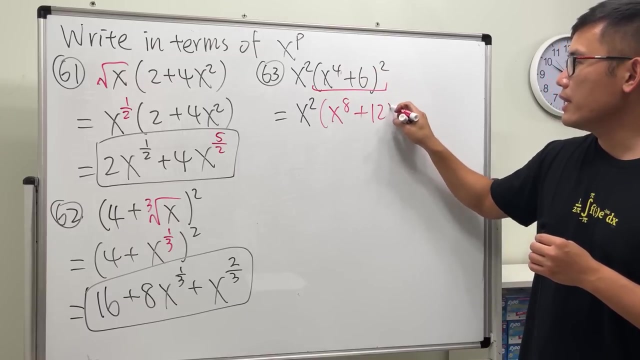 times x to the fourth, power plus six, and then square, or to vibration, do the exponent this one right here first. so here we have x, square, and then binomial, again right. so we have to square that. so multiply the power by 2, so we have x to the 8 plus 2 times this and that, which is 12, x to the 4, and then 6 square, which is 36. yeah, and then finally just distribute the x square. so we have x to the 10 plus 12x to the 3, therefore 16 plus 2 plus x squared twice. so in fact we have 2 x x squared. so we have x to the 8 plus 2x x squared, which is led the power. so here we add 6 and then больше applied this you can. you can see it work with your left hand. if you are versū ganzanx, remember going 0x christian at this point to round- then you're turning the volume, so you don't have any reason for the time, and so you have to cross so you can use. and then, finally, you can compute x to the plus 1 betweenosium, because so we have X. 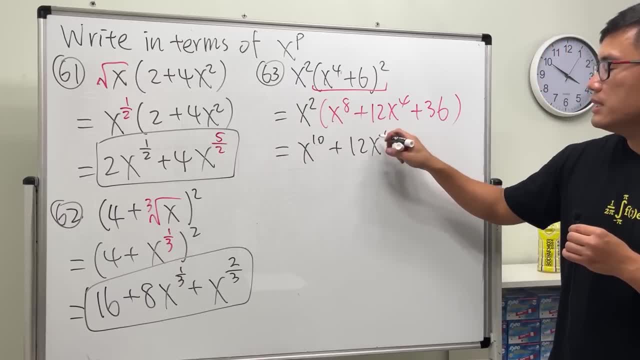 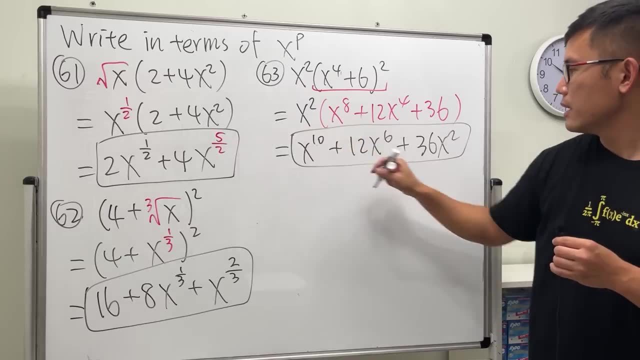 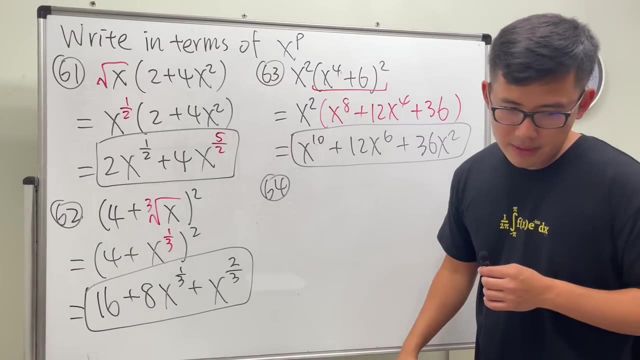 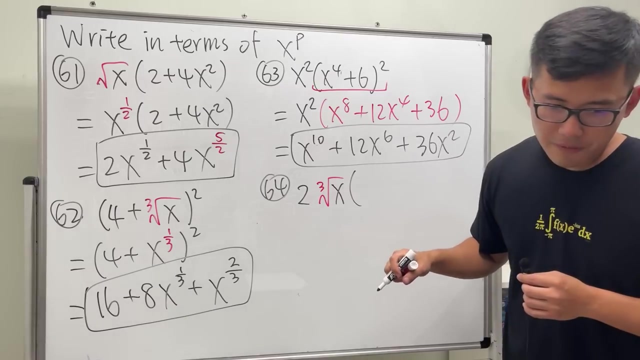 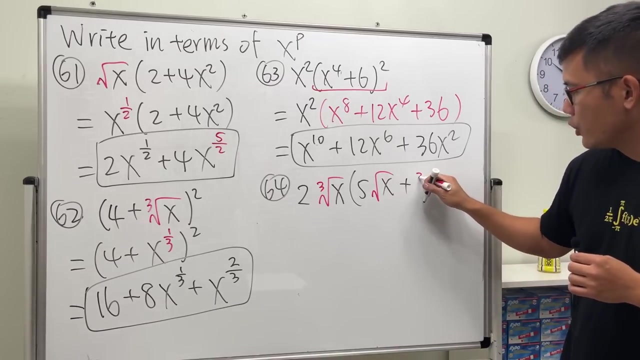 10 plus 12x to the 6th and then plus 36x squared, Done. Yeah, Alright, number 64.. We have 2 cube root of x times 5 square root of x And then plus the cube root of x squared. 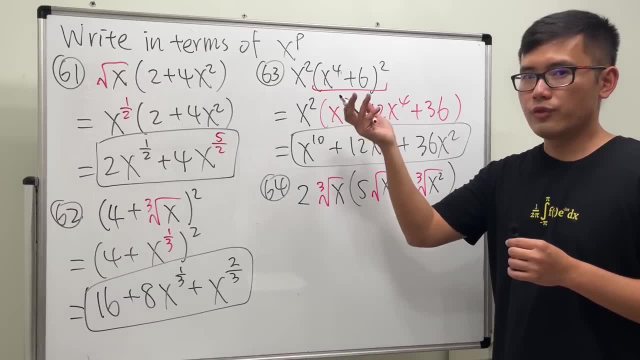 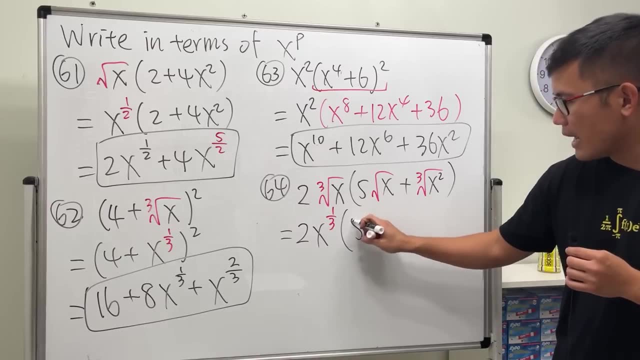 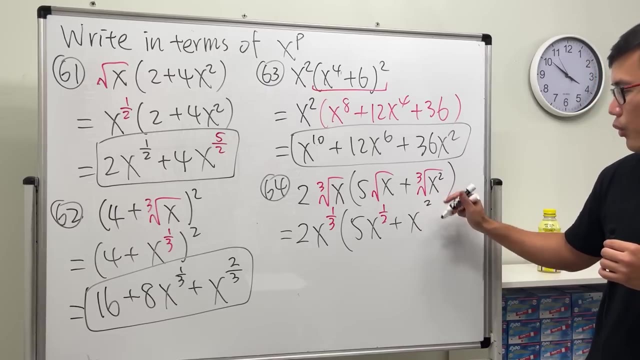 So the first thing is let's just change all the radical into fractional exponents. So this right here is 2x to the 1, 3rd power times 5.. This is x to the 1 half power, And then this is the same as x to the 2 over 3 power. 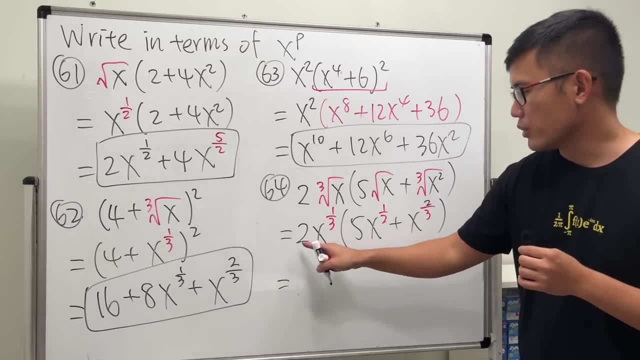 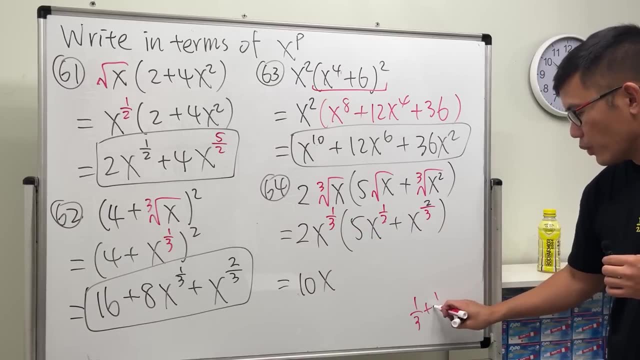 Okay, And then let's just multiply this in. So 2 times 5 is 10x. We will have to add the power. So just go ahead and do 1 3rd plus 1 half And I'll show you guys the TikTok way to do this. 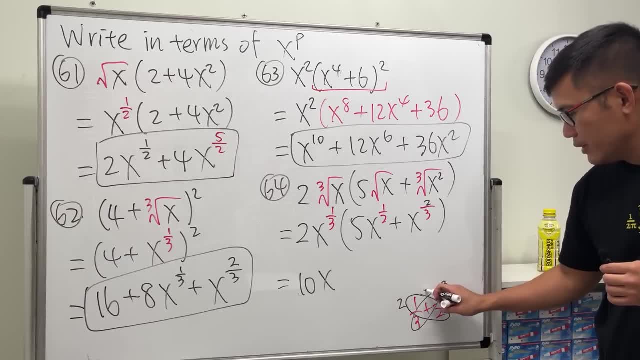 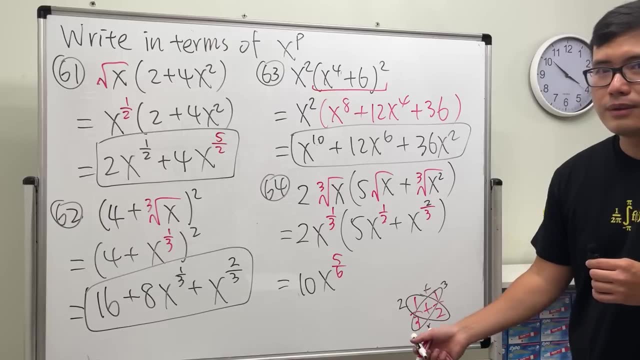 This times, this is 2.. This times, this is 3.. You add them and you multiply them, So you get 5 over 6.. Don't be too impressed. This is just adding fractions, Okay. And then next one, we add 2 times. that is just 2.. 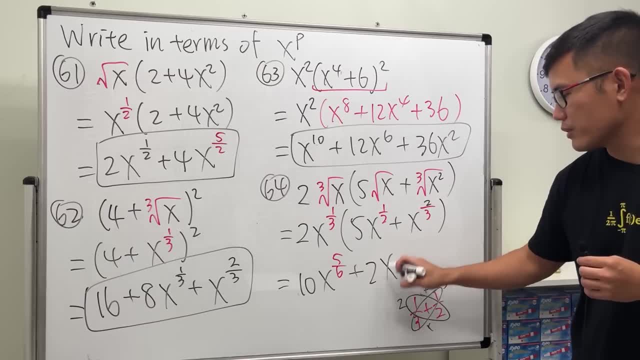 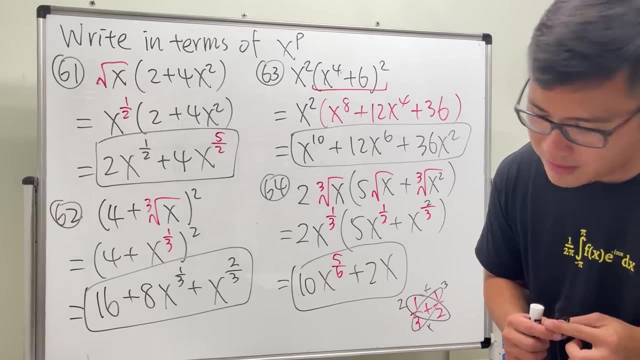 And then 1 3rd plus 2 3rd is just 3.. 3- 3rd, which is x to the 1st power. So this is it Okay, This is it So also. let me take a look at my answer key to see if I have my answer key being correct. 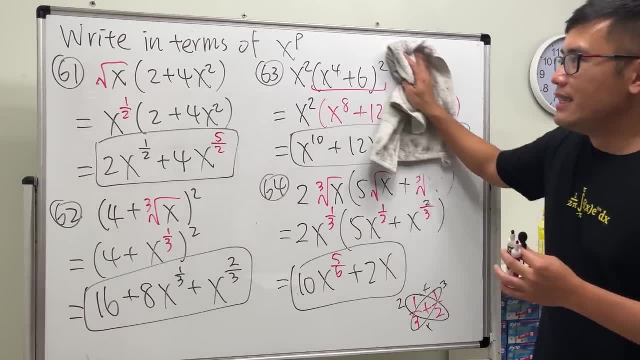 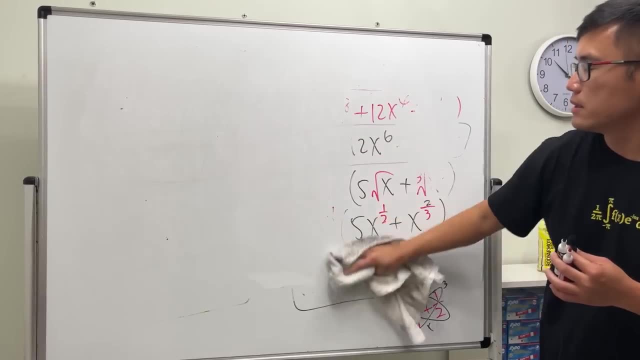 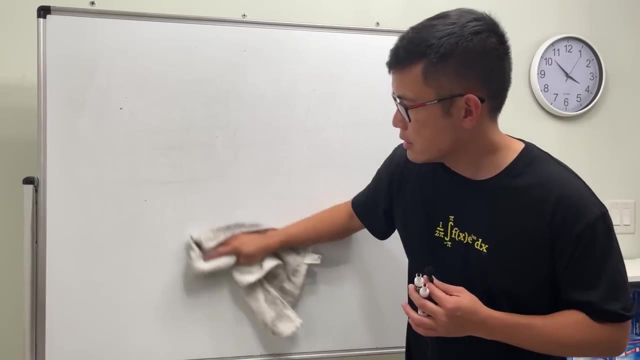 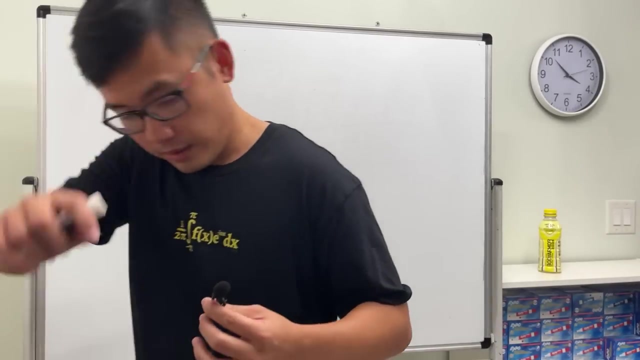 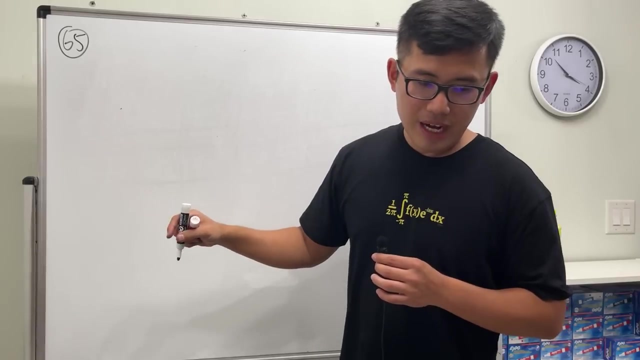 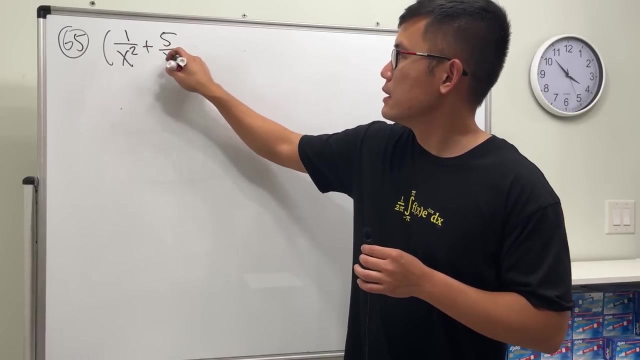 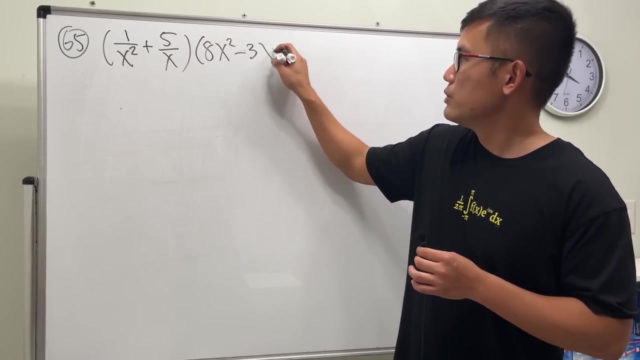 Very nice, All right. Next one: we have 65.. We have 1 over x squared Plus 5 over x, And then 8x squared Minus 3x. Well, we are going to take care of this. 2 power first. 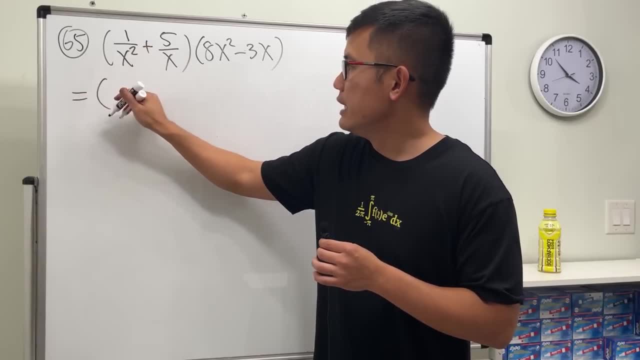 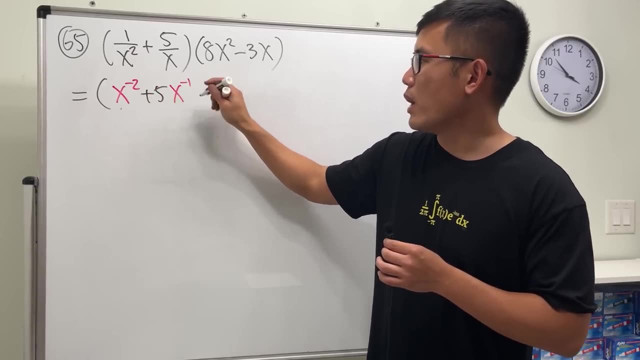 This right here becomes: I can write it as x to the negative 2. And then 5 over x. we can write that as plus 5, x to the negative 1.. And then this right here. let's just keep them as how they are. 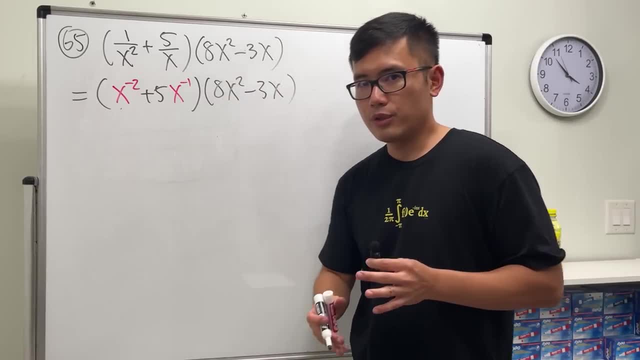 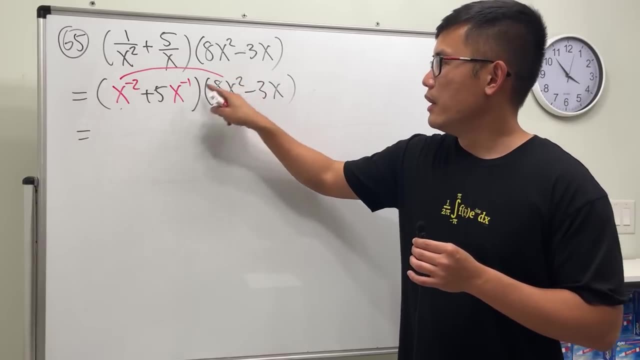 All right, Now we're just going to fold this out, right. So we take this, times that And remember we will have to add the exponent Negative. 2 plus 2 is 0, so the first one does not have x anymore, but we have the 8.. 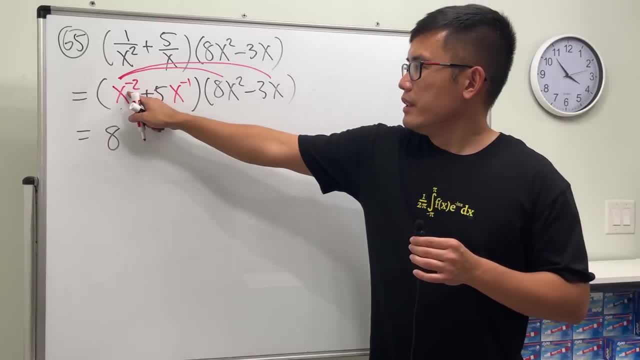 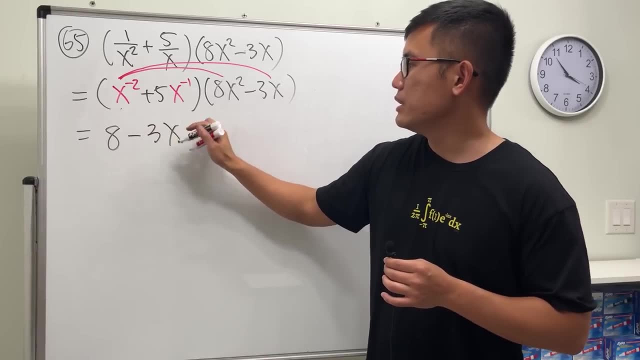 Next we take this times that Negative 2 plus 1, so it's x to the negative 1 power. So that will be negative 3, x to the negative 1.. Next we take this times that That's plus 40.. 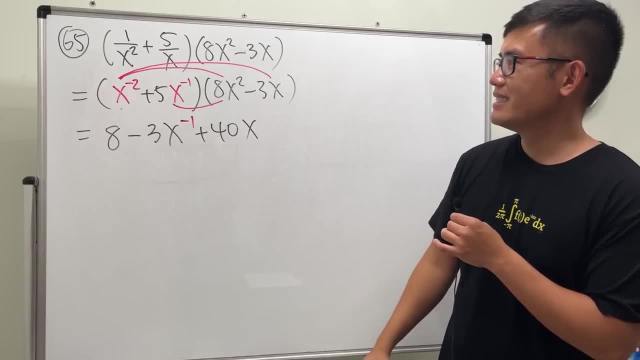 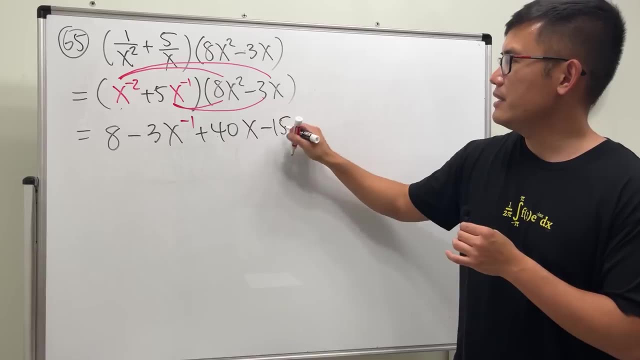 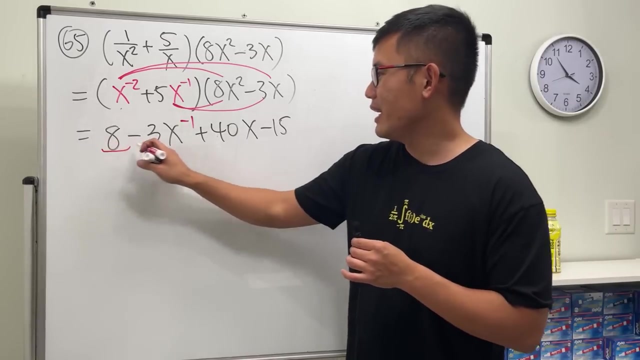 And then negative: 1 plus 2 is x to the 1st. Yeah, And lastly, this times that is minus 15 and no x, right? Negative 1 plus 1 is 0.. Yeah, And then, lastly, we just look at the 8 and also the minus 15.. 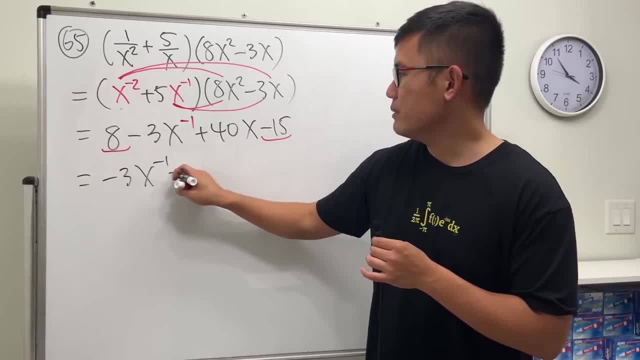 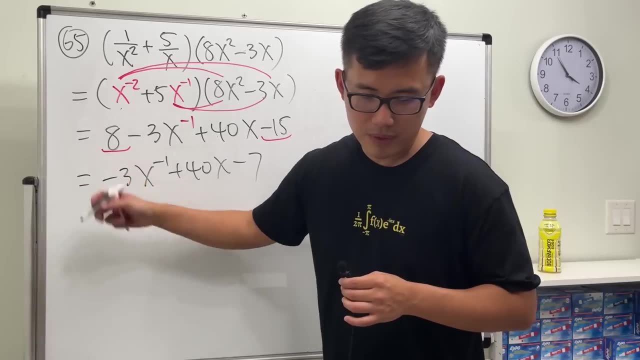 That should be minus 7.. So negative 3 x to the negative 1 plus 40 x and then minus 7.. That's what I have. Yeah, This is definitely okay. The water of this right here doesn't really quite matter. 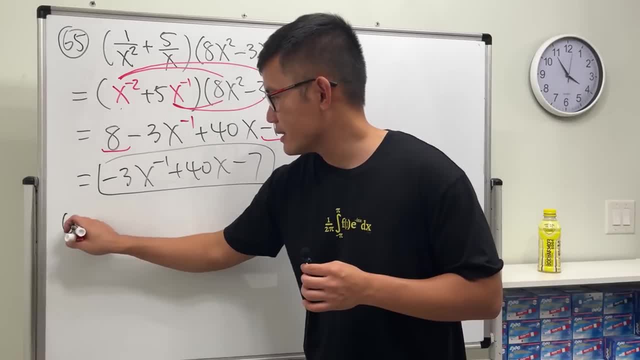 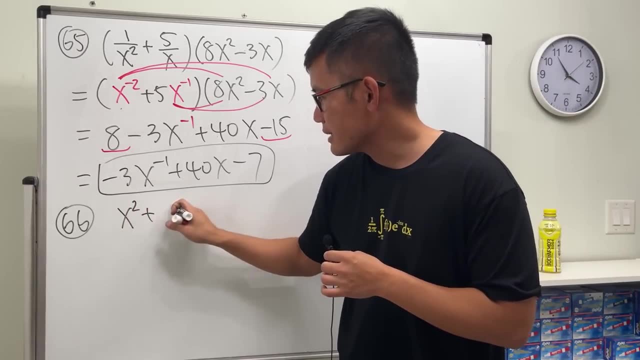 All right, Number 66.. Now we get to the fraction part. Here we have x squared plus 9 over x, No over 18, x to the 4th power. All right, So you have two ways to look at this. 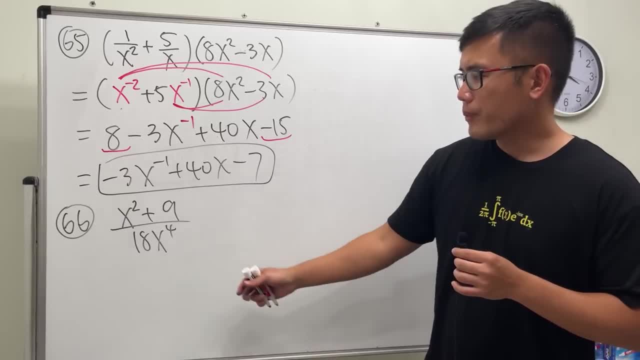 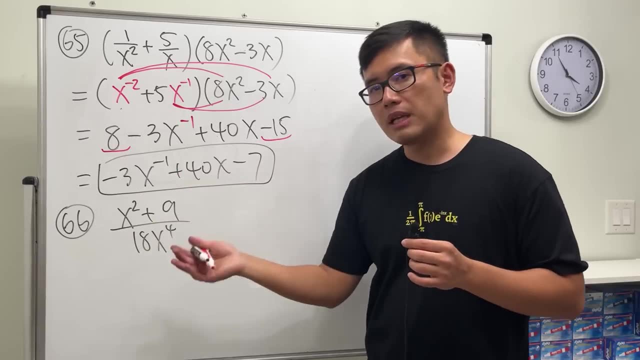 You can bring the x to the 4th power up and look at that as x to the negative 4 and then multiply it. That's fine. Or you can just split the fraction and then subtract the fraction. So you can just split the fraction and then subtract the fraction. 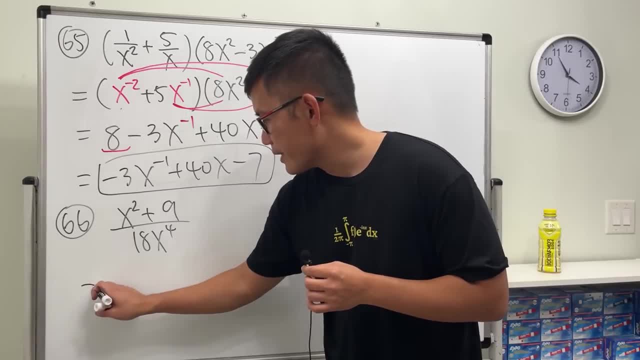 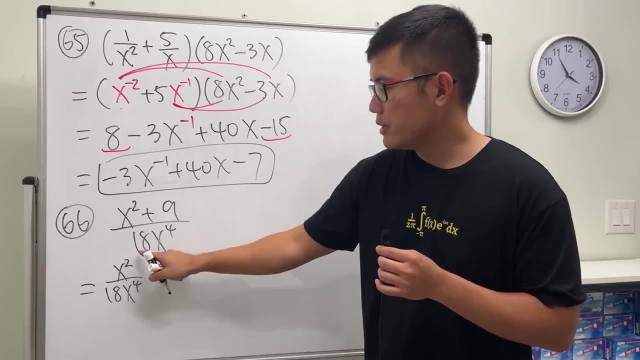 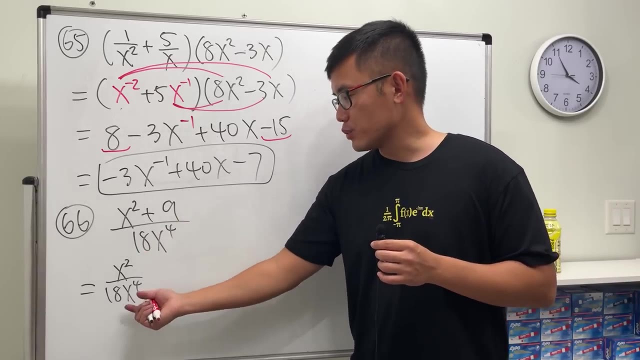 And then subtract the exponents. I will do the second way, This right here. I'll write it as x squared over 18 x to the 4th power. And we can do this because the denominator is just one term: 18 times x to the 4th power is just one term. 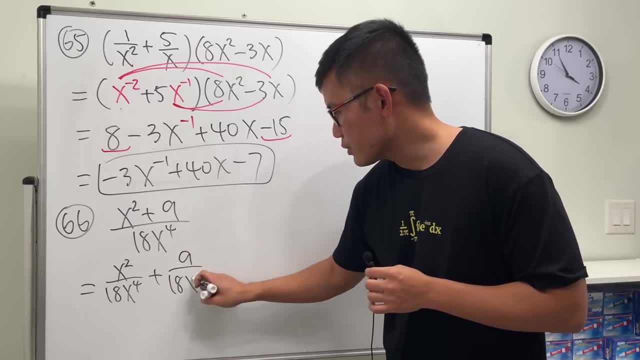 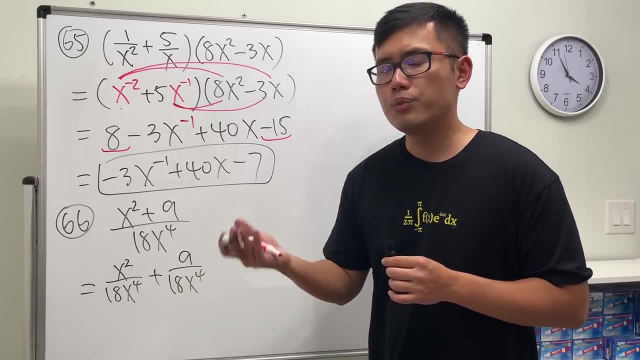 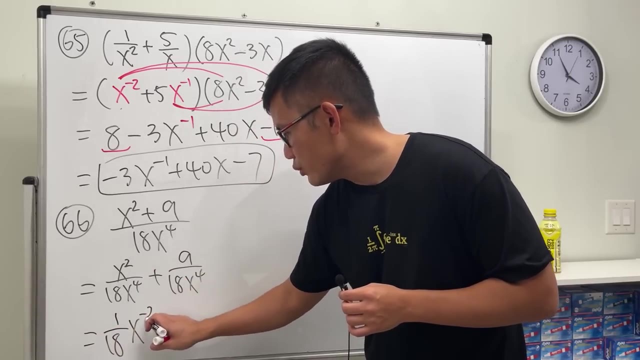 And then we add 9 over 18 x to the 4th power. Now simplify: 2 minus 4 is negative 2.. And that's a new power, All right. So right here I can write this as 1 over 18 x to the negative 2 power. 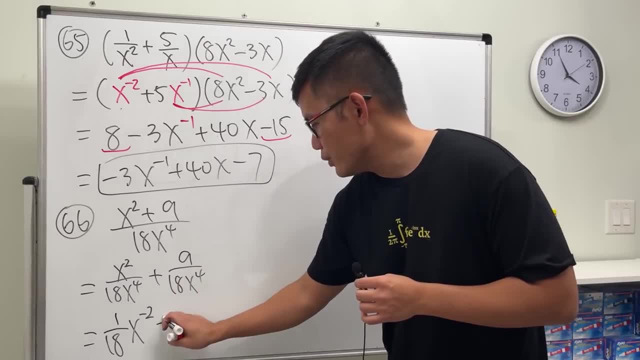 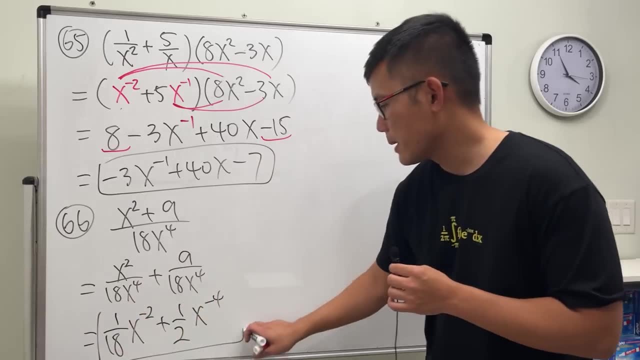 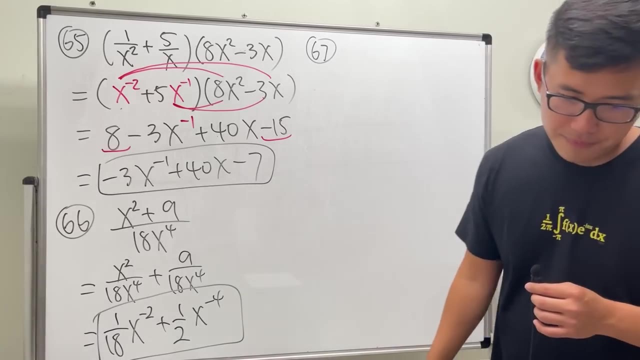 And then right here, 1 over 2, right, Let's reduce that the regular way. And then 1 over x to the 4th power, x to the negative 4.. Done Just like that: 67. 5x squared. 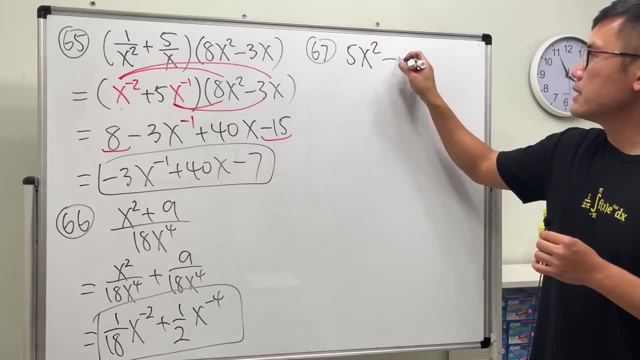 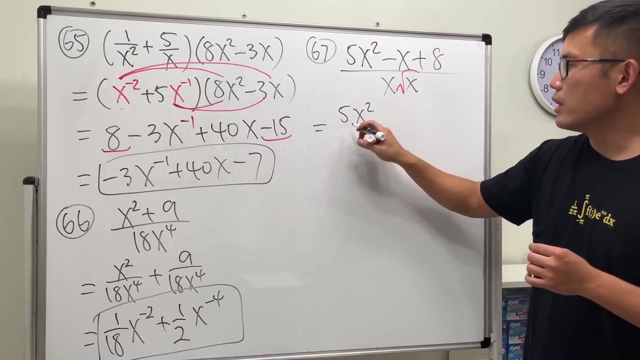 Minus x plus 8 over x squared root of x. Okay, So I'm going to split the fraction over there. So first we have 5x squared over. This is x to the 1st times, x to the 1 half, which is x to the 3 over 2 power. 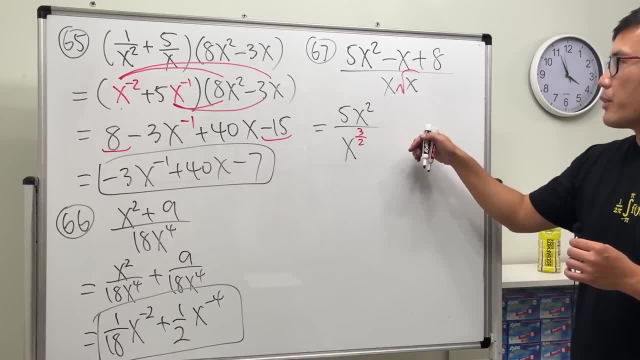 1 plus 1 half, 3 over 2.. And then do the same right here. In fact, I'm not going to write it, I'm just going to write it as x over x, And then this is square root of x. 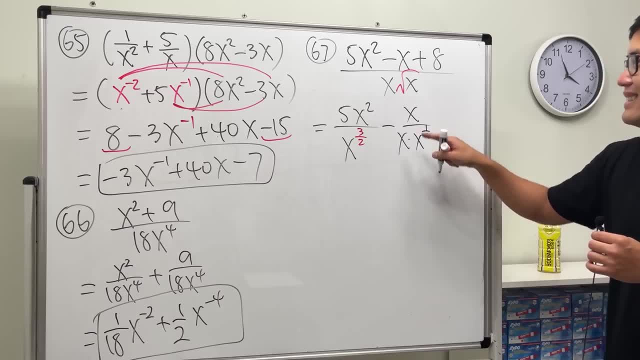 So x to the 1 half. Okay, I didn't combine it because I have x over that, So I can cancel that. And finally, for this one plus 8 over x to the 3 half. Perhaps I'll make the 1 half rare too. 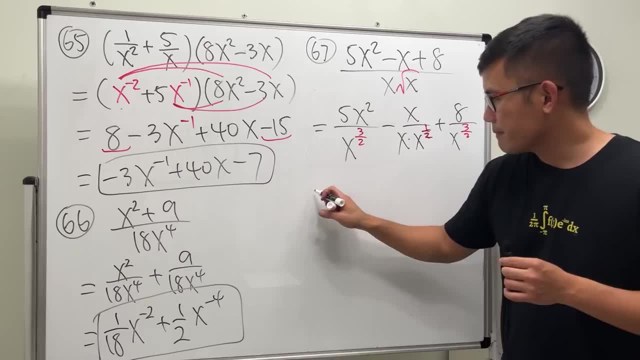 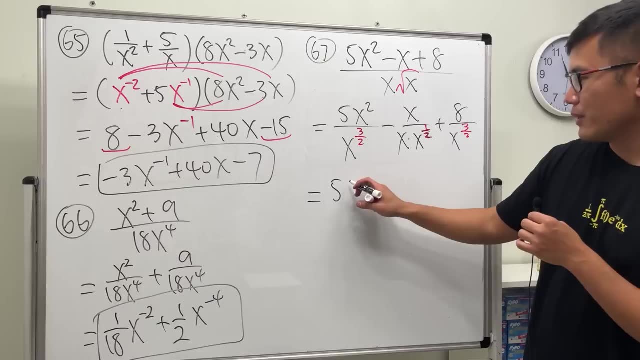 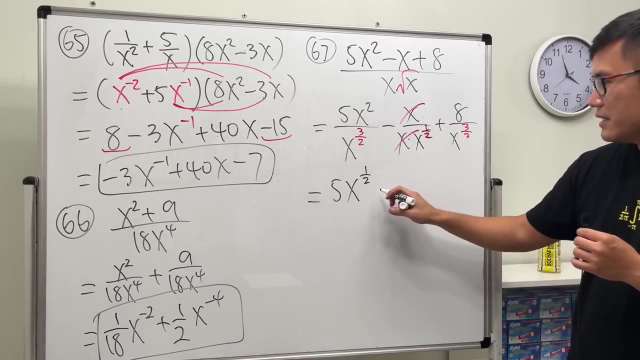 Okay, Anyway, So 5 is 5.. 2 minus 3 half is positive 1 half, So 5x to the 1 half. Next, this I can cancel. We have 1 half on the bottom, So that's the same as minus x to the negative 1 half. 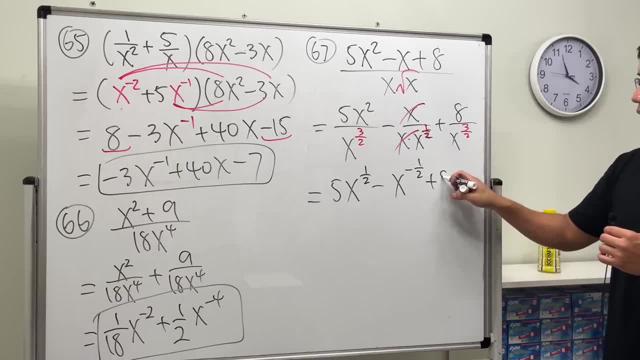 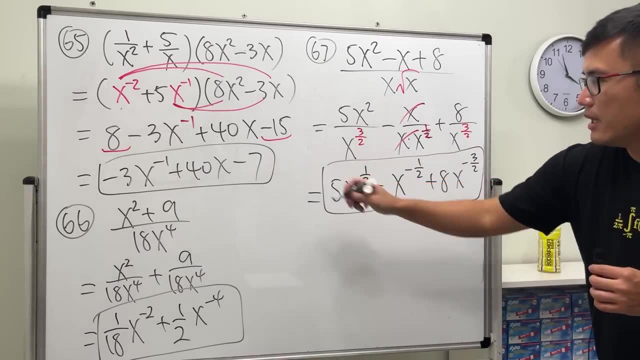 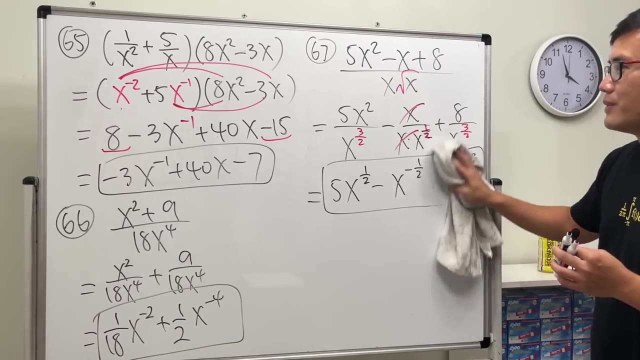 Lastly, just 8 over that, So we can say this is 8x to the negative 3 half, Just like that. Okay, I'm going to do 3 more and then I will take a drink. I'll take a sip of my drink over there. 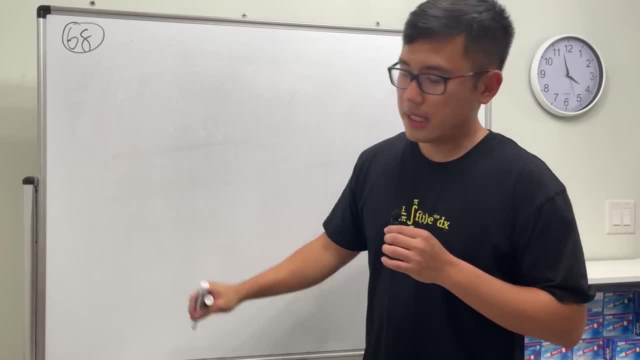 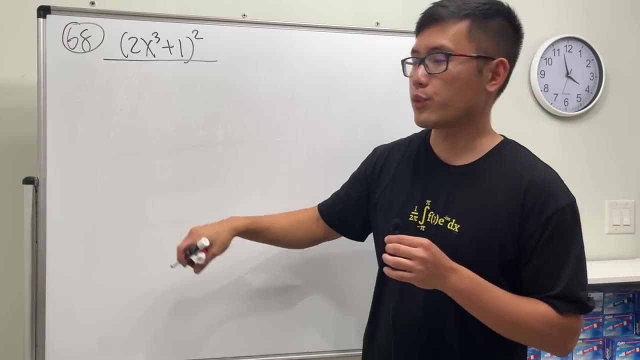 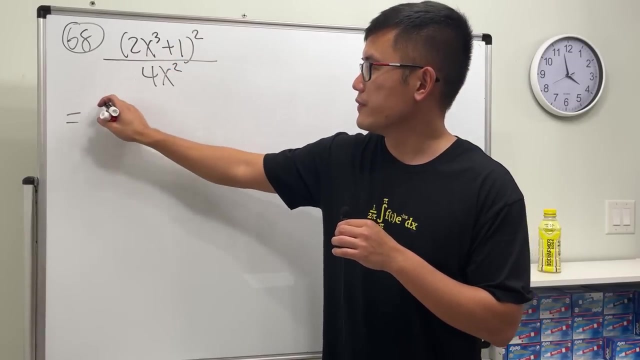 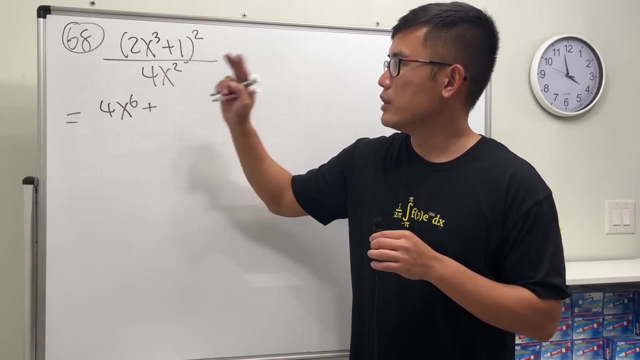 number 68. okay, 2x to the third power plus 1 square over 4x square. okay, open the top, so square the first one. so 2 square is 4 x to the third power square. you multiply the power by 2, so it's extra 6. we add 2 times this and that which is 4 x to the third power and lastly 1. 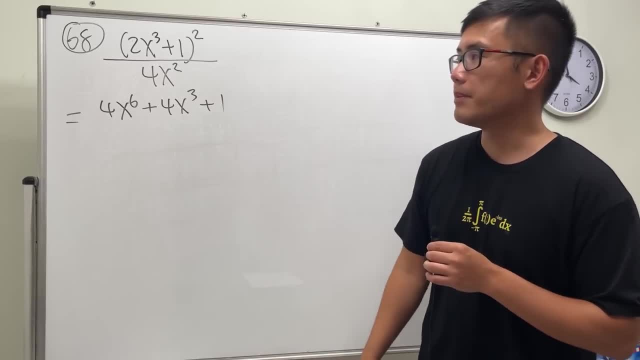 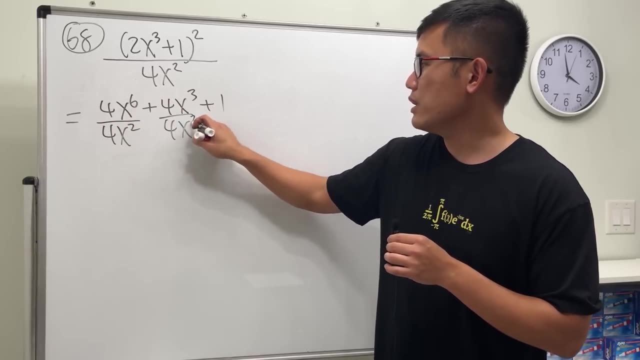 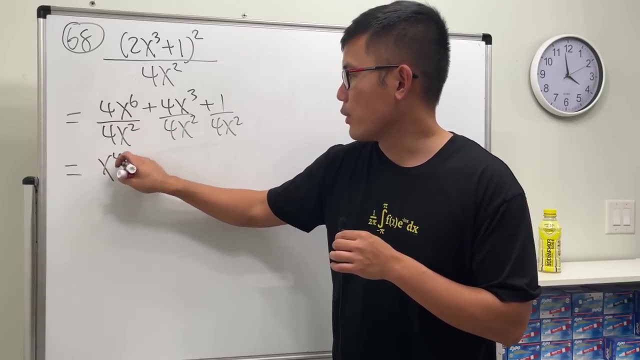 square, just plus 1. so that's the expansion for the top. and now for the bottom, we'll just go ahead. divide this by 4x square, divide this by 4x square and divide this by 4x square. so 4 and 4 cancel. the first one is x to the fourth power, next one: 4 and 4 also cancel. so we just have. 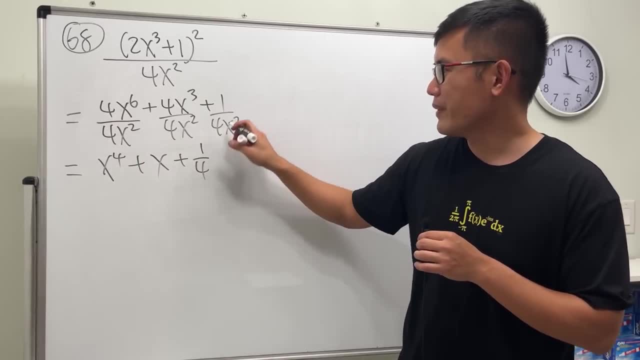 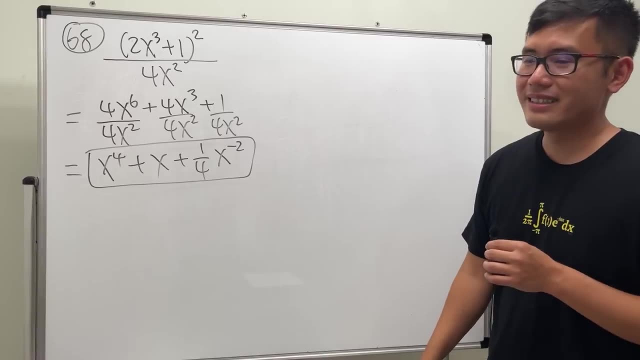 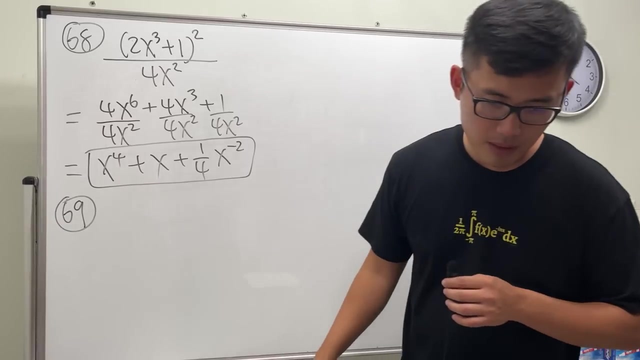 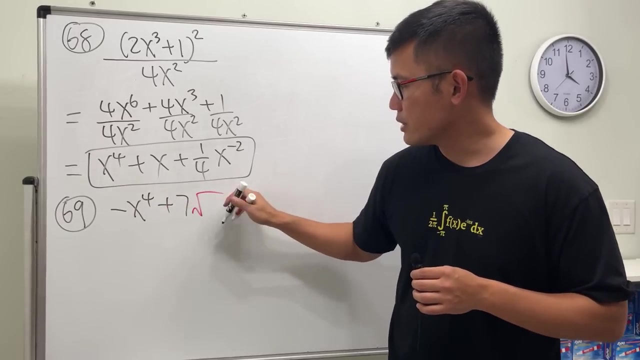 plus x and lastly, plus 1 over 4, and then we can write the x as x to the negative 2. so this right here will be the. you simplify the answer. yeah, all right, number 69. we have negative x to the fourth power plus 7 square root of x over. 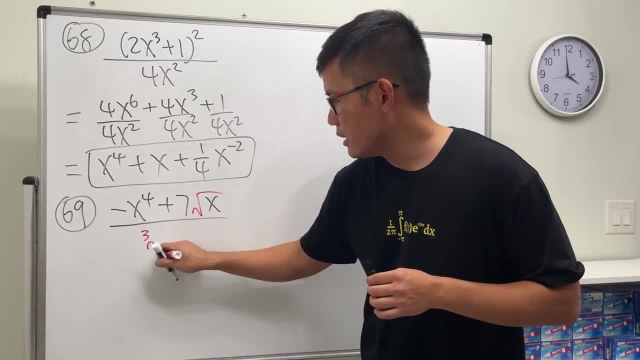 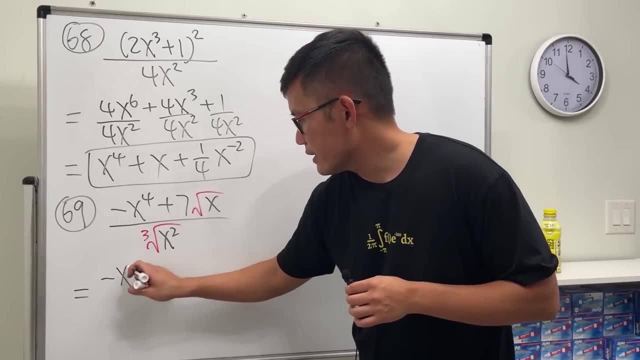 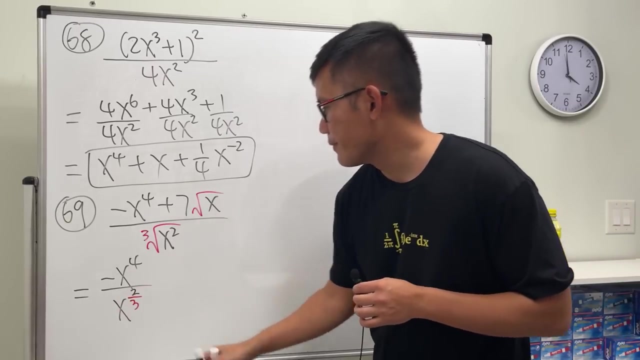 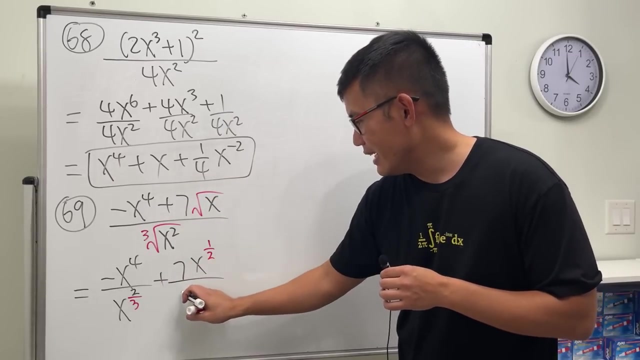 the cube root of x square. all right, this is negative x to the fourth power over. let's write this: this is negative x to the second power, plus 1, x to the second power, x and all the acredions, because obviously we've done minus 2, so the difference value of the BETA slope is negative 2 and that is. 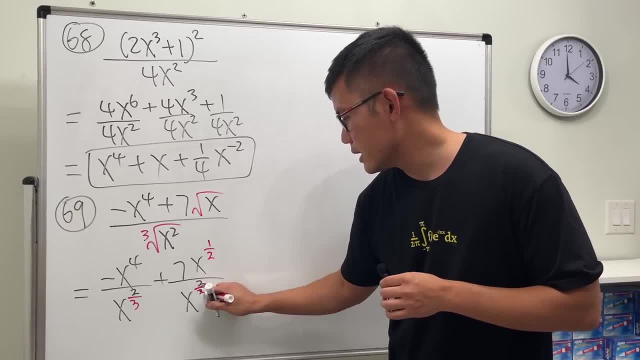 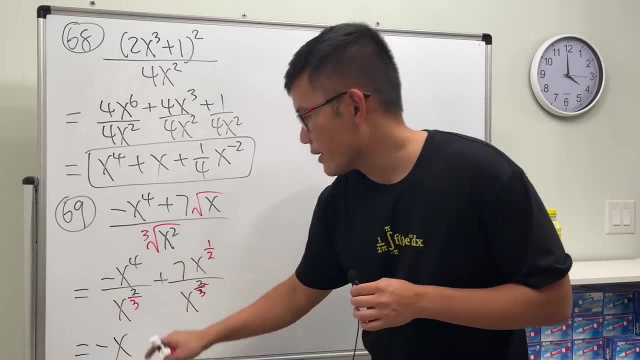 minus 2, 3. so it's negative. x to the second power minus 8 d, black fourth. okay, so this, i just need to write this in my COBRA process, and where exactly does it give me the okay? so minus 2 is negative. say what's negative. what's negative? alright, here we go. alright, so I just need to write this in my COBRA process to say what's negative. except we count these two, Subtract those one part 3 times and we can't solve this problem in class with more than 6x and all the other parts, and we have to add thisulty because we want to hold them together and we're gonna do some games and we can't solve the problem with some students. so what is negative? 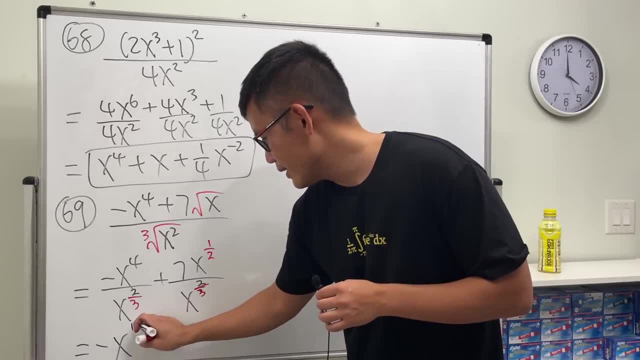 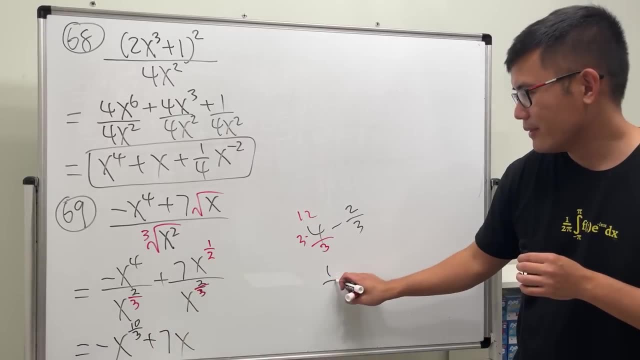 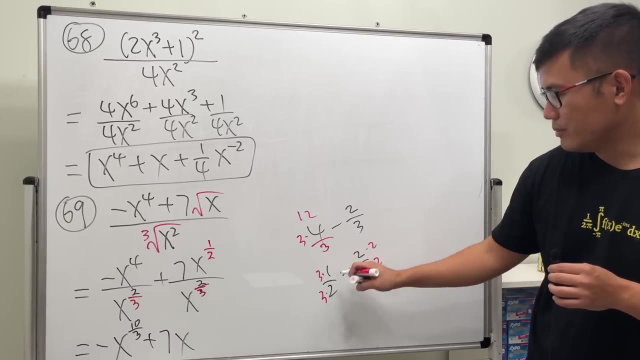 What does this mean? minus 2 is 10, so this is 10 over 3. next we add 7 by 1, half minus 2. 3rd. so we need to multiply this by 3, 3, 2 & 2, so 3 minus 4 is negative 1, so it's negative 1. 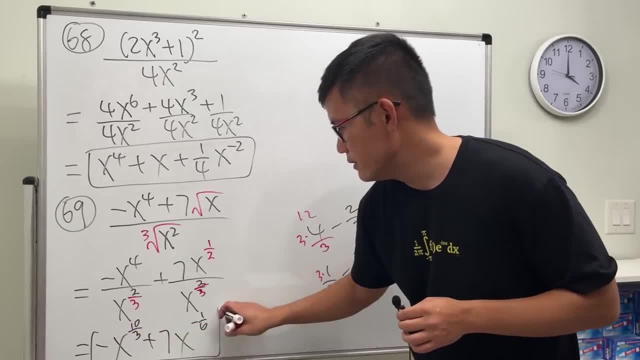 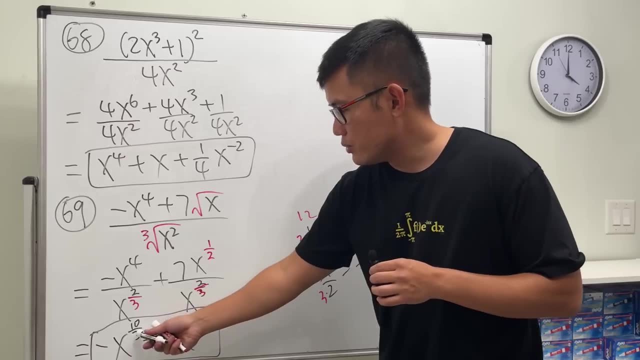 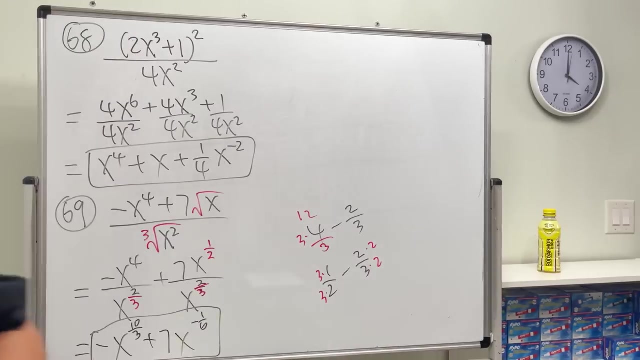 over 6. so let me just double check my answer key. yeah, so negative X to this 3 over 10 plus 7 X to a negative 1 over 6 power. yeah, and let me just check. maybe I need to. yep, I need to charge my phone now. 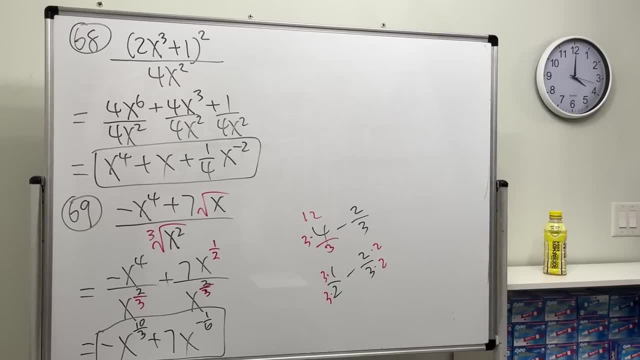 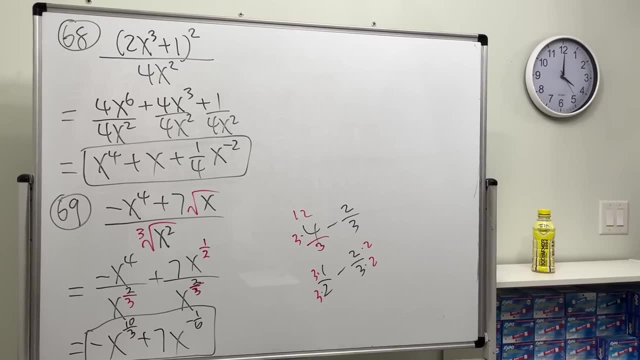 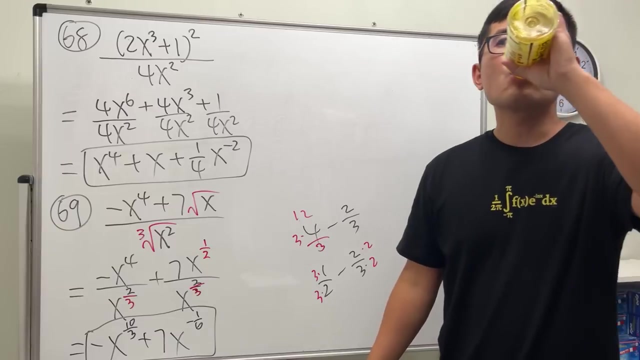 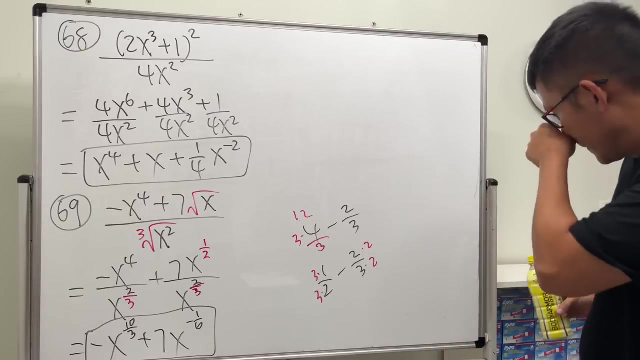 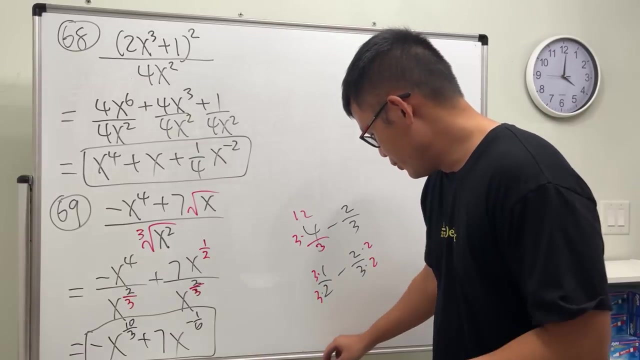 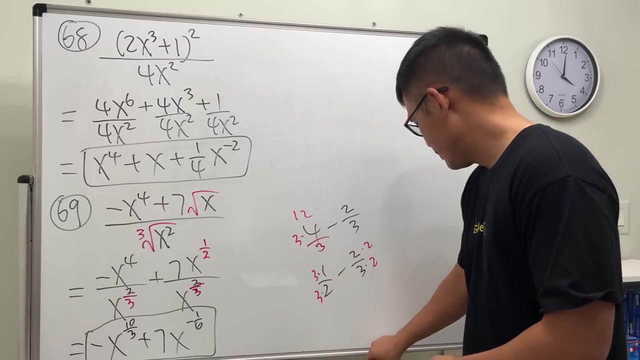 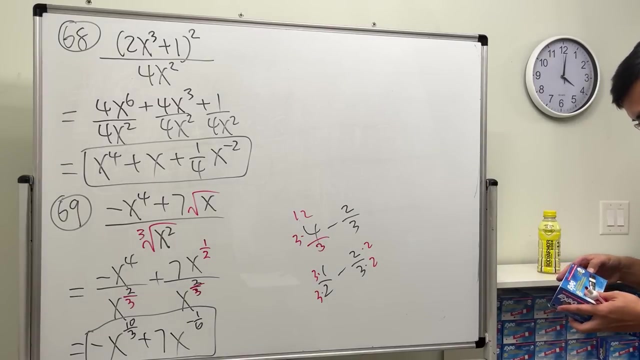 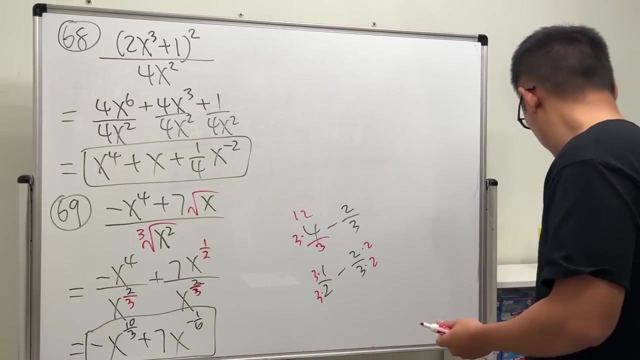 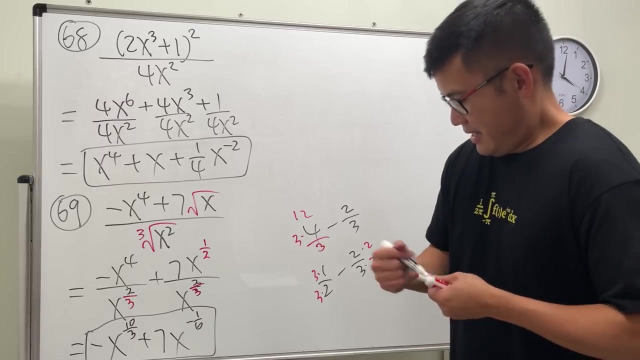 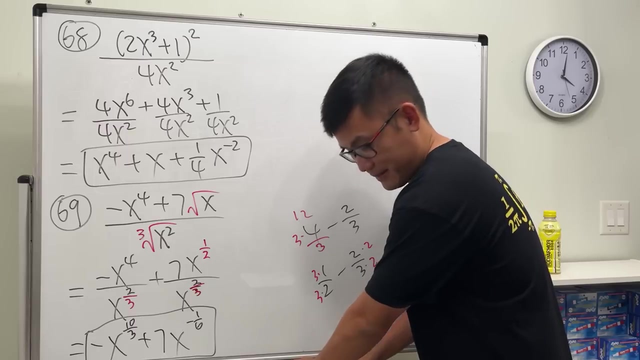 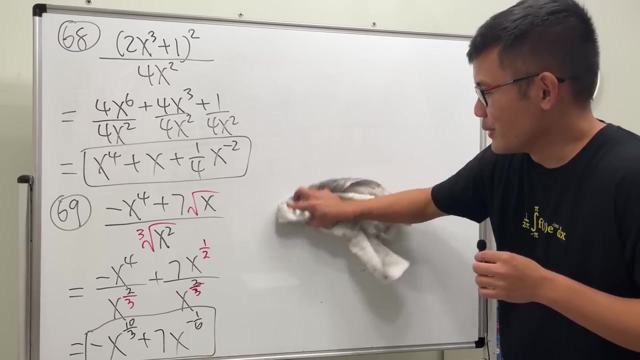 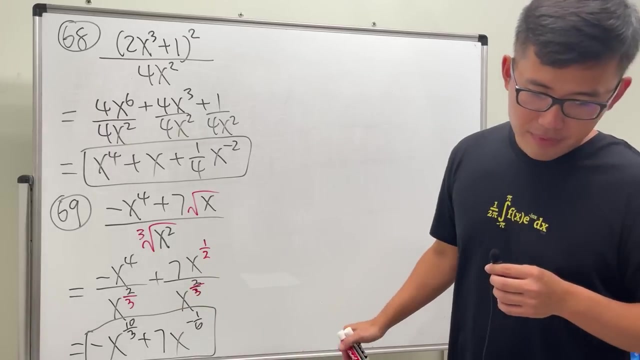 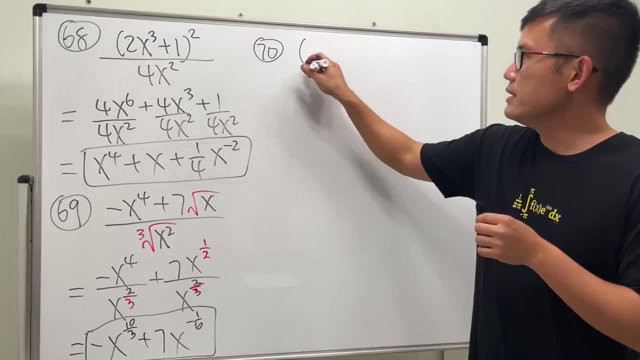 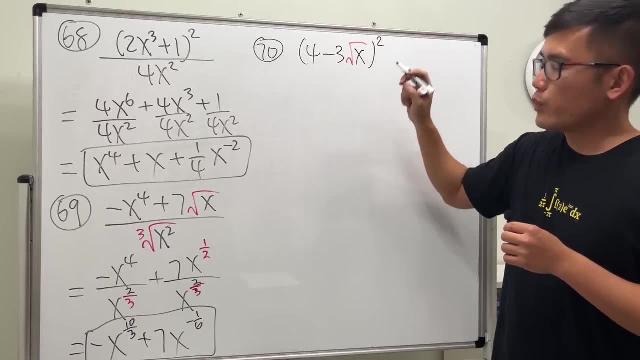 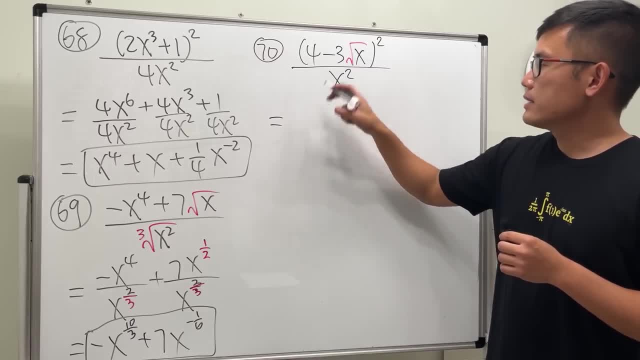 square root of X square over x square. alright, so let's go ahead and do the alright. so let's go ahead and do the alright. so let's go ahead and do the following: so expand the top right, so following. so expand the top right, so following. so expand the top right, so against binomial, so square the first one. 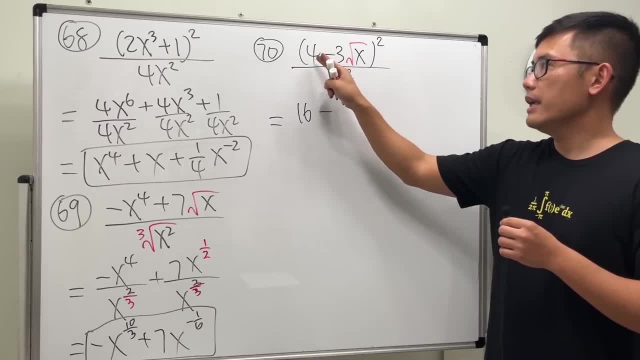 against binomial, so square the first one. against binomial, so square the first one. 16 minus 2 times 4 is 8 times 3. is 16 minus 2 times 4 is 8 times 3. is 8 times 3 is. 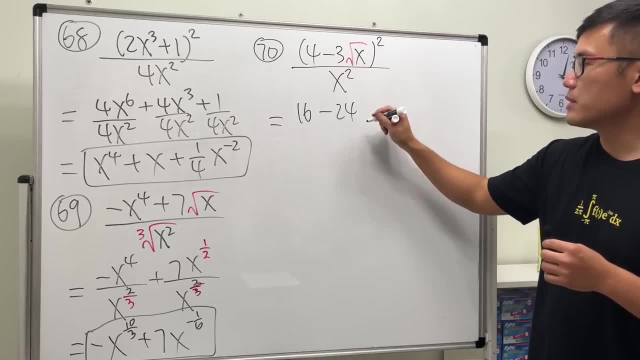 16 minus 2 times 4 is 8 times 3, is 16 minus 2 times 3 is 8 times 3 is 8 times 3 is 24, and then we have this term as 24, and then we have this term as: 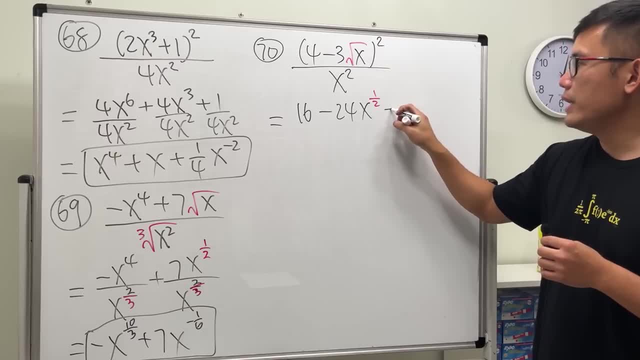 24, and then we have this term as well, which is X to the 1 half power, and well, which is X to the 1 half power, and well, which is X to the 1 half power, and lastly, we add this term square, so 3. 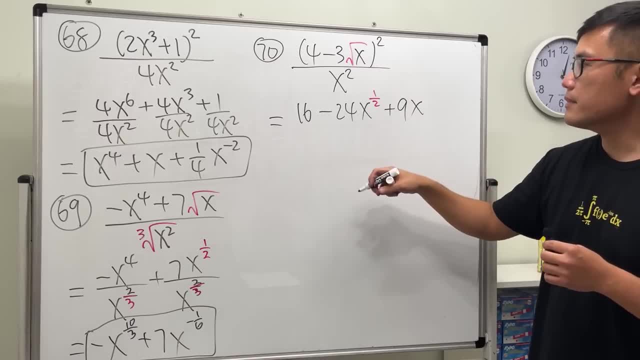 lastly, we add this term square, so 3. lastly, we add this term square, so 3. squares 9 square root square is just X. squares 9 square root square is just X. squares 9 square root square is just X. yeah, and then over X square, so it's over. 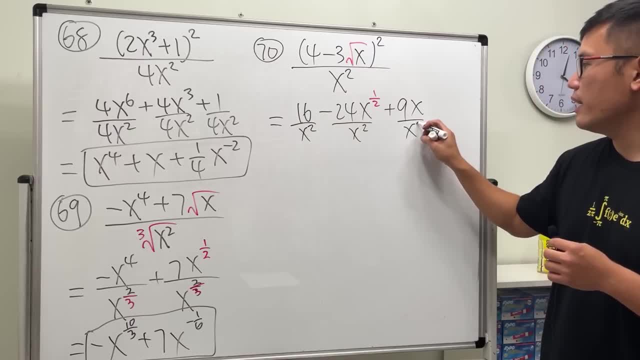 yeah, and then over X square. so it's over, yeah, and then over X square. so it's over X square here, over X square here and also X square here, over X square here and also X square here, over X square here and also over X square here. so the first one we 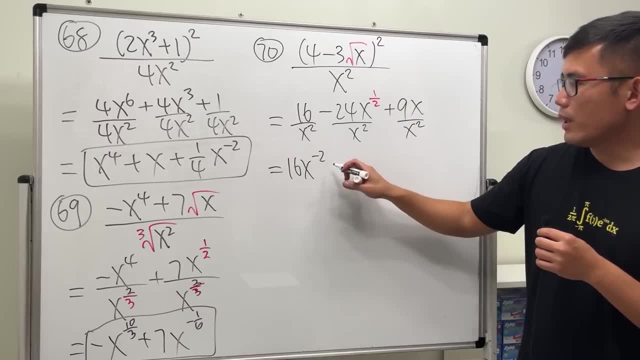 over X square here. so the first one we over X square here. so the first one. we can write this as 16 extra negative. 2 can write this as 16 extra negative. 2 can write this as 16 extra negative 2. next: 1 minus 24, 1 half minus 2 minus 4. next: 1 minus 24, 1 half minus 2 minus 4. next: 1 minus 24, 1 half minus 2 minus 4, over 4. pretty much so it's X to the over 4. pretty much so, it's X to the. 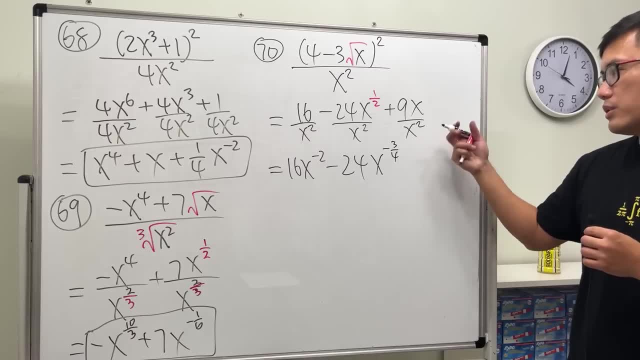 over 4, pretty much. so it's X to the negatives: 3 over 4, and this is 1 minus 2. negatives: 3 over 4, and this is 1 minus 2. negatives: 3 over 4, and this is 1 minus 2, just negative 1, so it's plus 9. X to the. 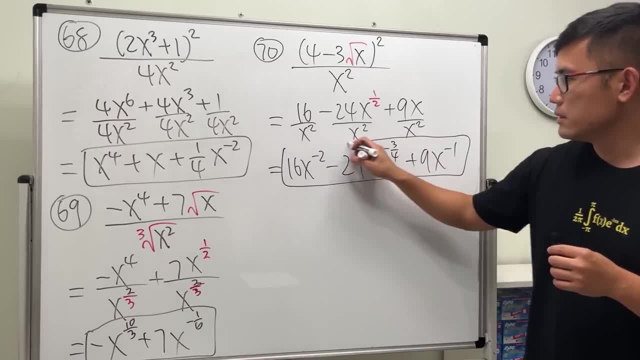 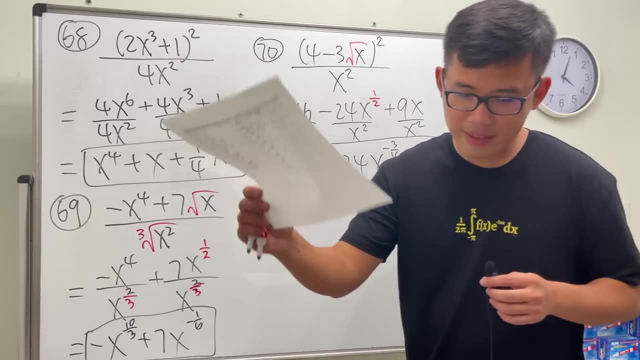 just negative 1, so it's plus 9 X to the just negative 1, so it's plus 9 X to the negative 1. yeah, we'd write in terms of negative 1. yeah, we'd write in terms of negative 1. yeah, we'd write in terms of X. cool, another sheet on okay. 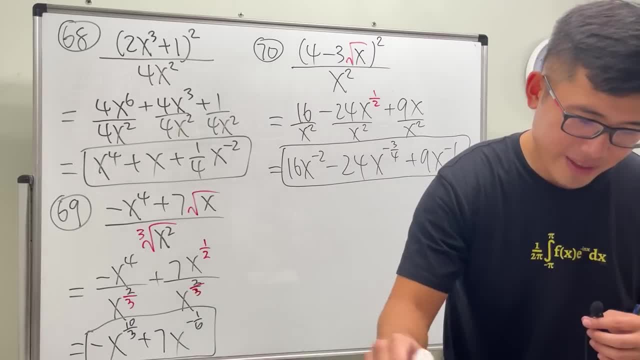 X cool. another sheet on okay. X cool. another sheet on okay. so another crazy one. okay, 30 more to go. so another crazy one. okay, 30 more to go. so another crazy one. okay, 30 more to go. I do not have question 101 this time. I. 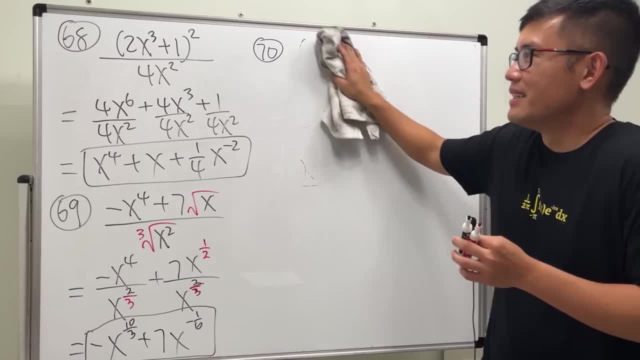 I do not have question 101 this time I. I do not have question 101 this time I because I have a perfect 10, exactly because I have a perfect 10, exactly because I have a perfect 10, exactly category, so I don't know what question. 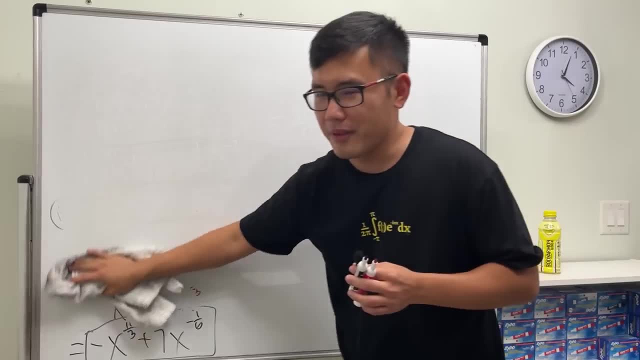 category, so I don't know what question category. so I don't know what question 101 should be. I don't know. maybe I'll 101 should be. I don't know, maybe I'll 101 should be. I don't know. maybe I'll come with something or maybe not. I have 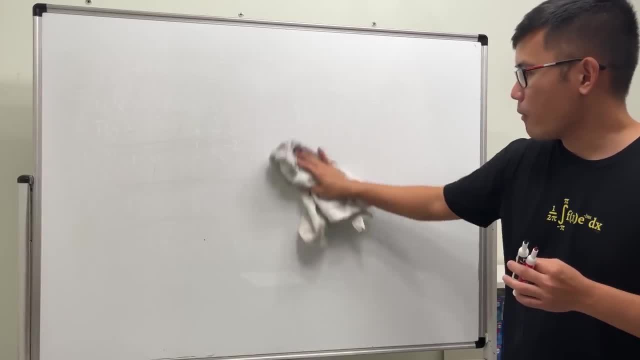 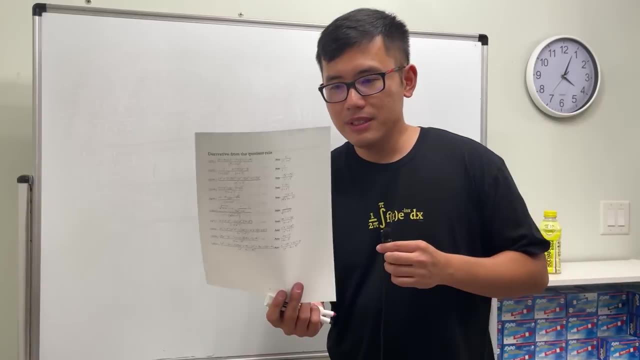 come with something, or maybe not. I have come with something, or maybe not. I have no idea. okay, no idea, okay, no idea, okay, you are going to see this kind of. you are going to see this kind of. you are going to see this kind of expressions from the quotient rule. so, 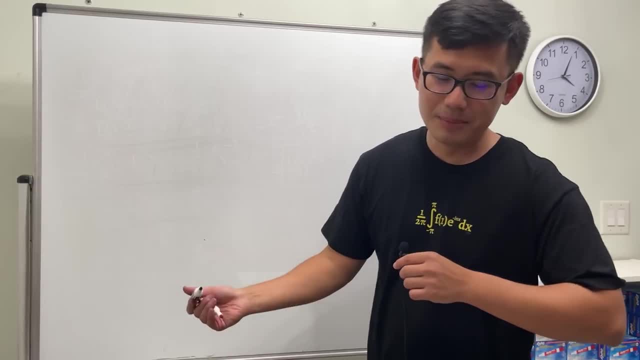 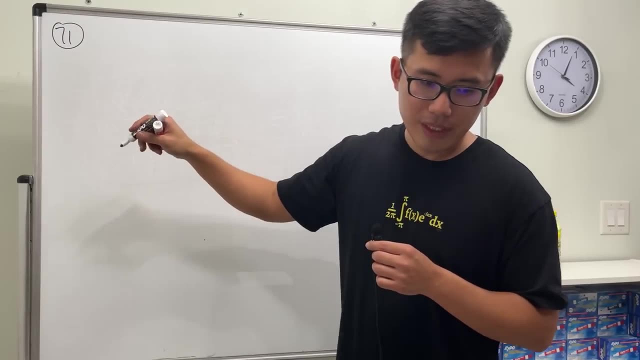 expressions from the quotient rule. so expressions from the quotient rule. so we're just going to do it simplify, we're just going to do it simplify, we're just going to do it simplify. hopefully the best. okay, number 71 we. hopefully the best. okay, number 71 we. 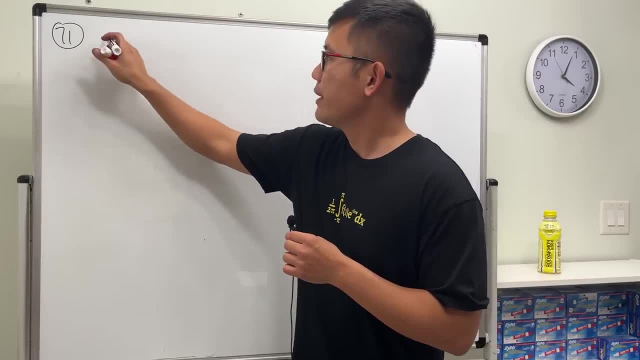 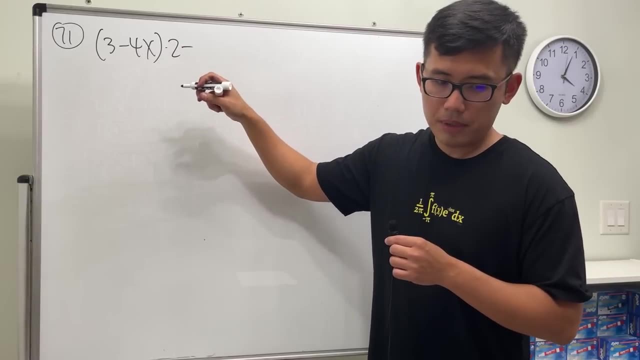 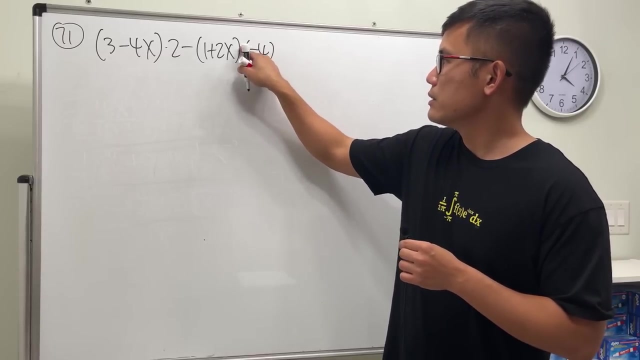 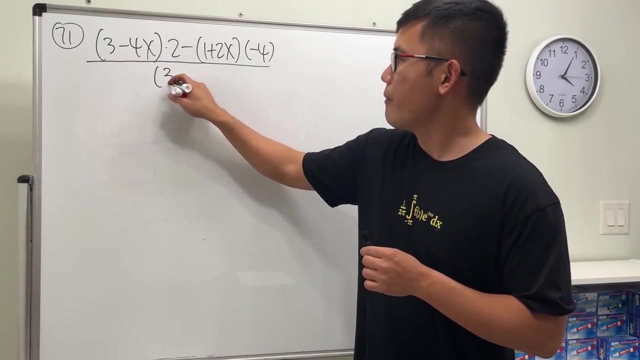 hopefully the best. okay, number 71: we have 3 minus 4 times 2 minus 1 plus 2x. have 3 minus 4 times 2 minus 1 plus 2x. have 3 minus 4 times 2 minus 1 plus 2x times negative 4 over 3 minus 4x. 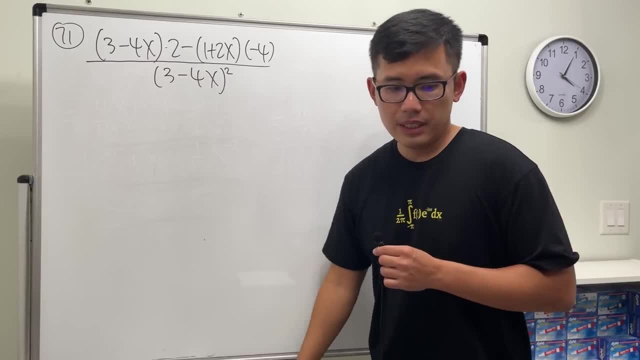 times negative: 4 over 3 minus 4x times negative: 4 over 3 minus 4x- square right. so yeah, this is actually from square right. so yeah, this is actually from square right. so yeah, this is actually from so-called the quotient rule. when we 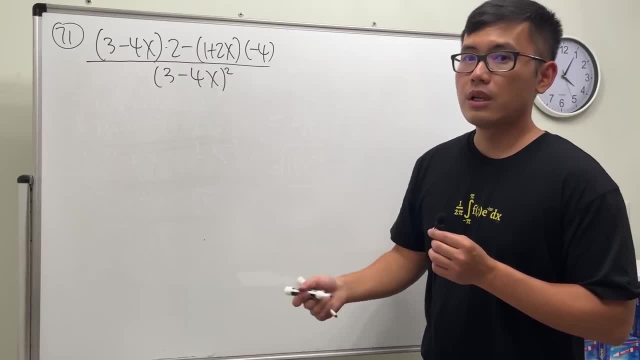 so-called the quotient rule, when we so-called the quotient rule, when we do the derivative, so we see this kind of do the derivative, so we see this kind of do the derivative. so we see this kind of crazy expression. what we do is just crazy expression. what we do is just 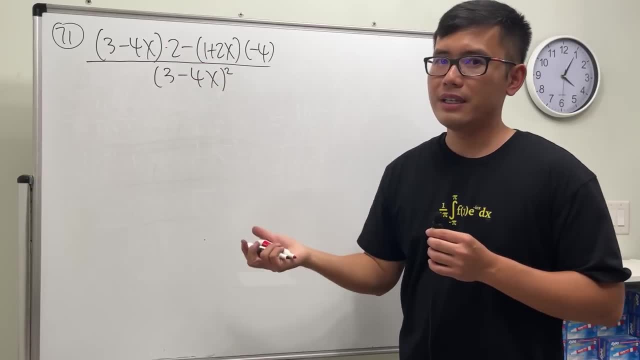 crazy expression. what we do is just like what we did before: look at the top. like what we did before, look at the top. like what we did before. look at the top, simplify it and then try to see if we simplify it and then try to see if we. 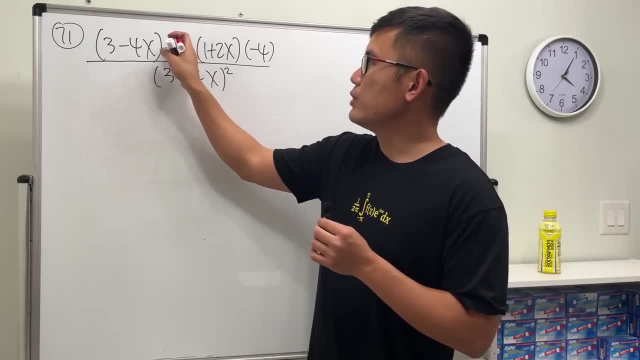 simplify it and then try to see if we can cancel anything at the end or not. so can cancel anything at the end, or not. so can cancel anything at the end, or not. so let's see, take the two distributed. let's see, take the two distributed. let's see, take the two distributed backwards, right, so we are going to get 6. 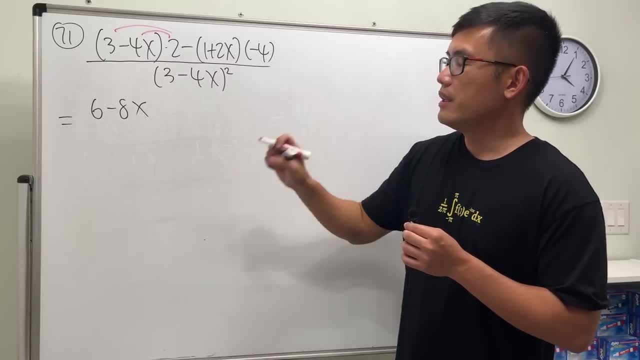 backwards right, so we are going to get 6 backwards right, so we are going to get 6 minus 8x. that's the best we can do now minus 8x. that's the best we can do now minus 8x. that's the best we can do now. negative and then negative. so make sure. 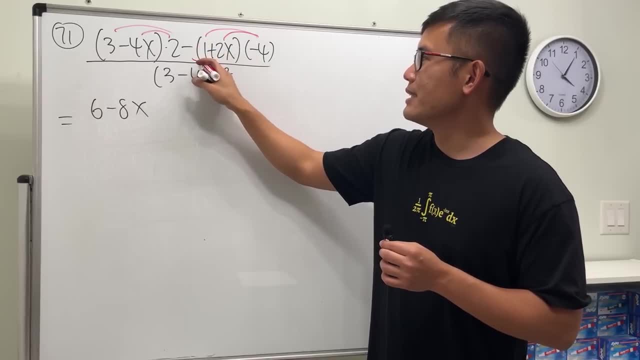 negative and then negative. so make sure negative and then negative. so make sure you distribute it and also make sure you you distribute it and also make sure you you distribute it and also make sure you distribute it. so it's positive: 4, just distribute it. so it's positive 4, just. 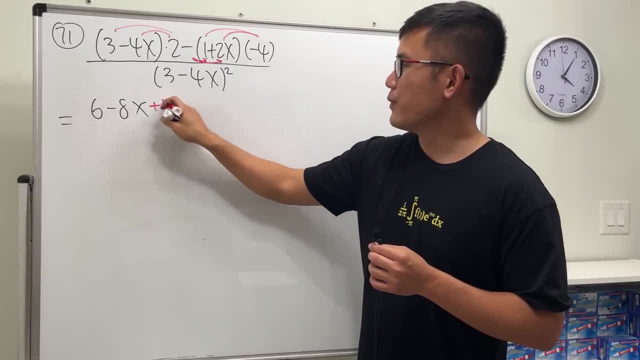 distribute it so it's positive 4 just signify positive 4 times this, which is signify positive 4 times this, which is signify positive 4 times this, which is plus 4, plus 4, plus 4 positive 4 times that, which is plus 8x. 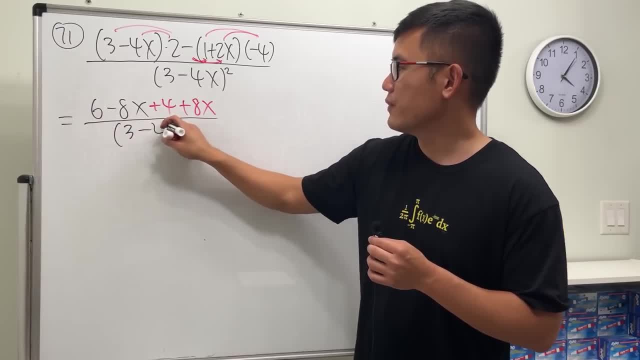 positive 4 times that which is plus 8x. positive 4 times that which is plus 8x. over the denominator which is 3 minus 4x. over the denominator which is 3 minus 4x. over the denominator which is 3 minus 4x square. 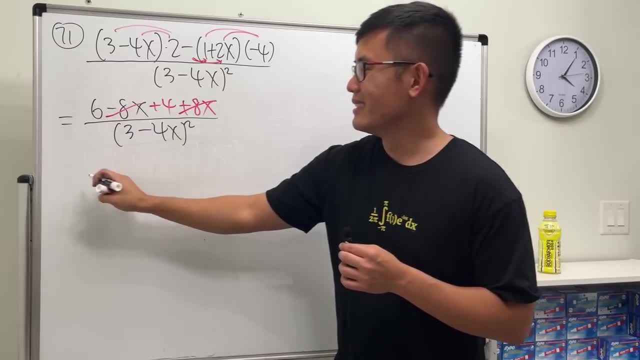 square square: 8x minus x bye-bye, and then 8x minus x bye-bye, and then 8x minus x bye-bye, and then together, together, together, 6 and 4 is 10 over this guy which is 6, and 4 is 10 over this guy, which is. 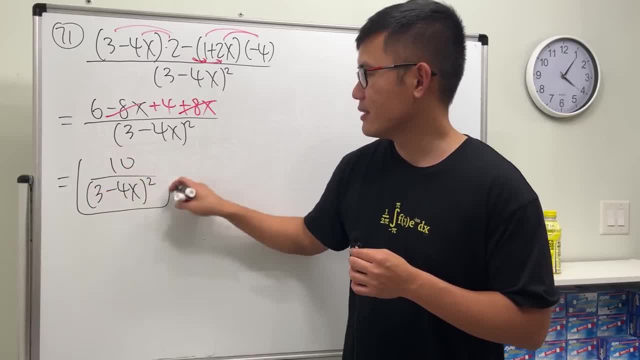 6 and 4 is 10 over this guy, which is 3 minus 4x and then square, and then we 3 minus 4x and then square, and then we 3 minus 4x and then square, and then we are done. 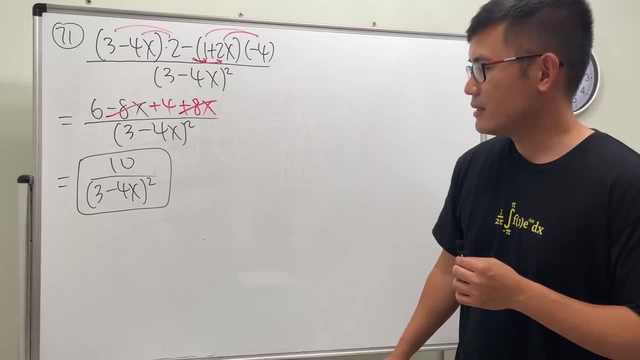 are done, are done, cool, cool, cool. now the next one, now the next one, now the next one. i'm going to, i'm going to, i'm going to just come here and write it, so number 72. just come here and write it, so number 72. 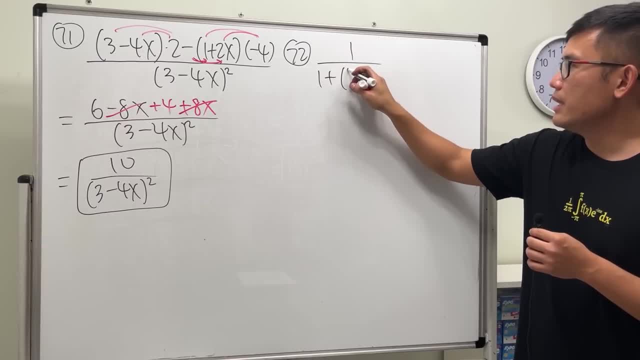 just come here and write it. so number 72: we have 1 over 1 plus parentheses x plus. we have 1 over 1 plus parentheses x plus. we have 1 over 1 plus parentheses x plus 1, 1, 1, so x minus 1. 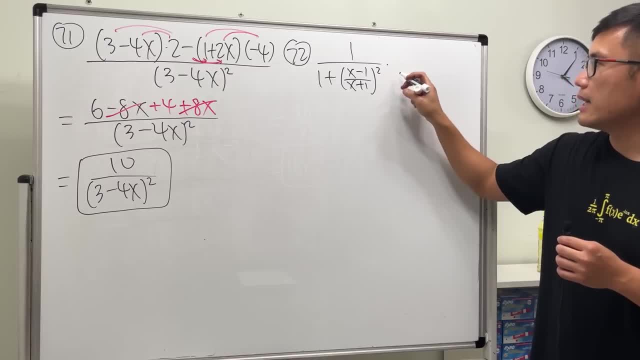 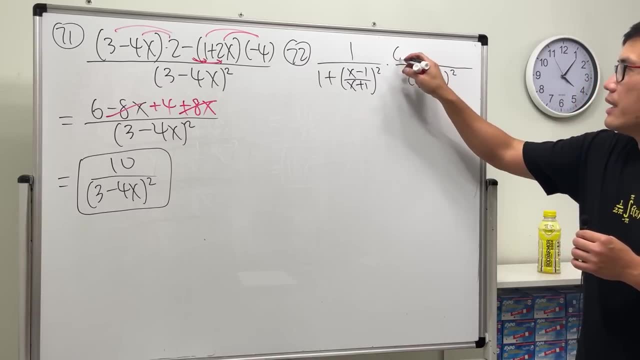 over x plus 1 over x plus 1 over x plus 1 square times, square times, square times. this right here, this right here, this right here, we have, we have. we have x plus 1 square and then x. x plus 1 square and then x. 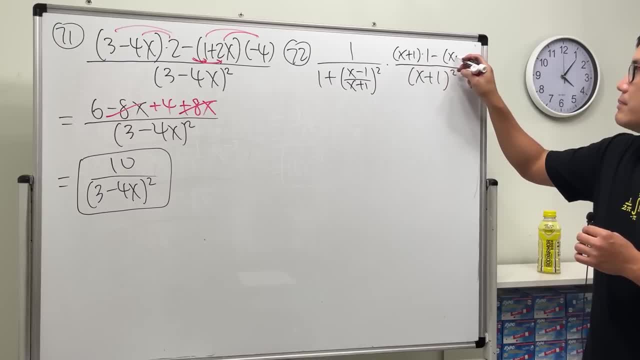 x plus 1 square, and then x plus 1 times 1 minus plus 1 times 1 minus plus 1 times 1 minus. x minus 1 times 1- crazy stuff, but don't. x minus 1 times 1- crazy stuff, but don't. 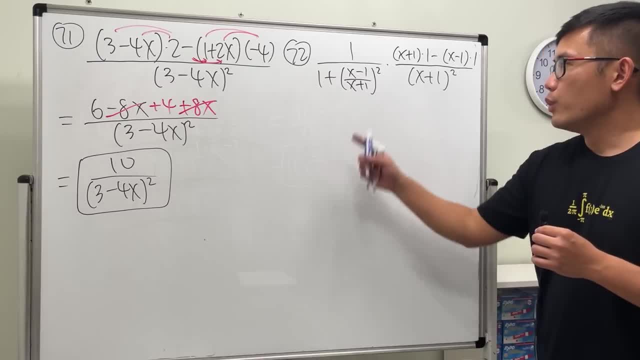 x minus 1 times 1 crazy stuff. but don't worry, i cut you, worry, i cut you, worry. i cut you. firstly, we have this fraction times the firstly. we have this fraction times the firstly. we have this fraction times the other. so technically, there's the. 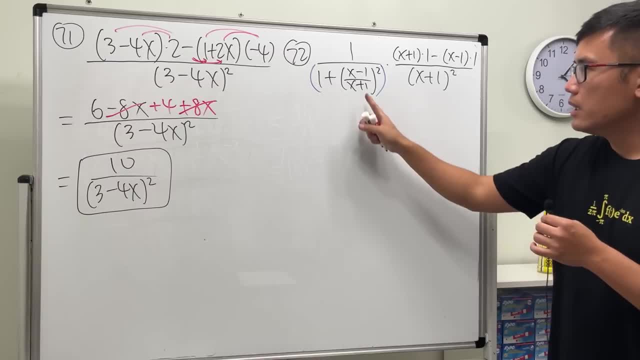 other, so technically. there's the other, so technically. there's the invisible parentheses on the bottom. invisible parentheses on the bottom, invisible parentheses on the bottom. and then notice, and then notice, and then notice. this right here, right x minus 1 over x. this right here, right x minus 1 over x. 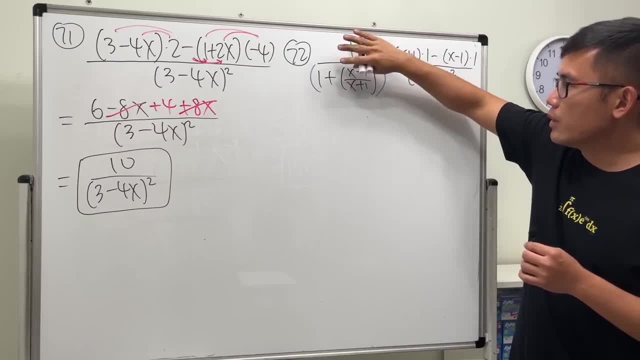 this right here. right: x minus 1 over x plus 1 squared plus 1 squared plus 1 squared. we can look at the top being squared and we can look at the top being squared and we can look at the top being squared and also the bottom being squared. 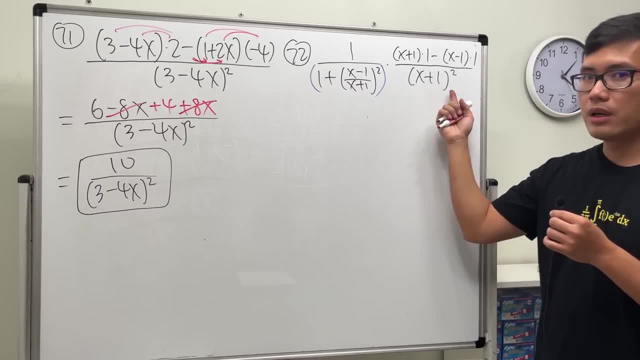 also the bottom being squared, also the bottom being squared, and we are lucky because this right here is, and we are lucky because this right here is, and we are lucky because this right here is: x plus 1 square. x plus 1 square. x plus 1 square. what we can do is just go ahead and take. 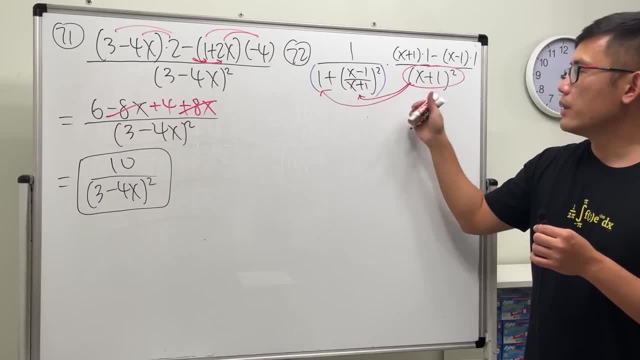 what we can do is just go ahead and take. what we can do is just go ahead and take this, distribute this, distribute this, distribute right. take the whole thing, distribute right. take the whole thing, distribute right. take the whole thing distribute, because that way, what we are going to 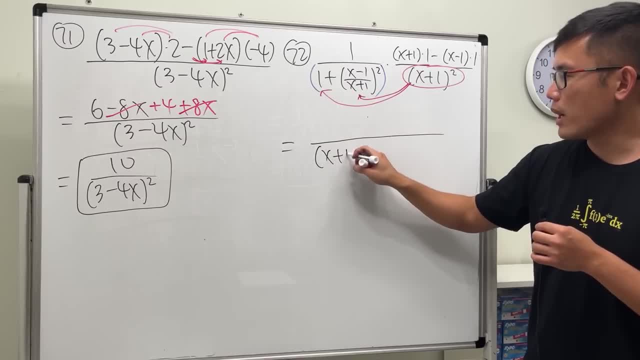 because that way what we are going to, because that way what we are going to get, is this times, that which is just x get, is this times, that which is just x get, is this times that which is just x plus one square. and when we take this: 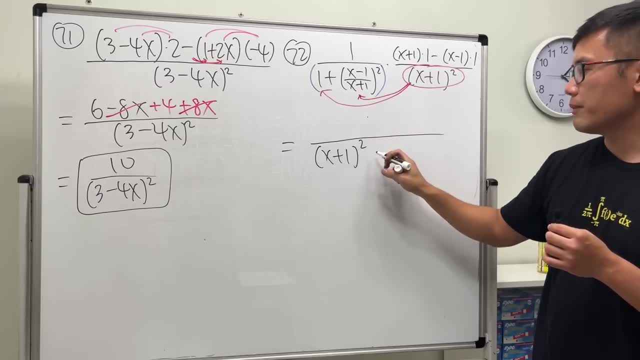 plus one square, and when we take this plus one square, and when we take this, times that the denominator, and that will times that the denominator, and that will times that the denominator, and that will cancel. so we just have plus cancel. so we just have plus cancel. so we just have plus x minus one square. okay. 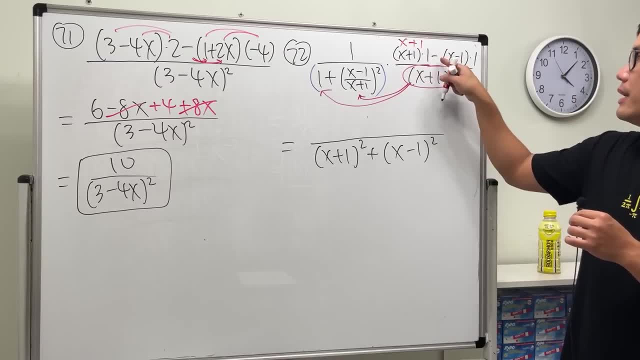 x minus one square- okay. x minus one square- okay, on the top. let's see this is just x on the top. let's see this is just x on the top. let's see this is just x plus one and then minus x plus one and then minus x. 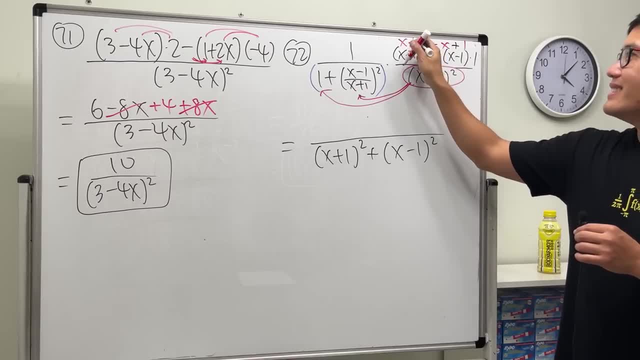 plus one and then minus x, and then plus one, and then plus one and then plus one. so of course this and that just cancel. so so of course this and that just cancel. so so of course this and that just cancel. so one plus one is two. one plus one is two. 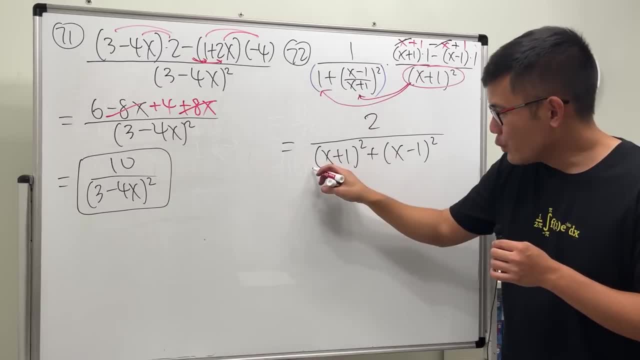 one plus one is two times one is two times one is two times one is two. and then, right here, let's multiply this. and then, right here, let's multiply this. and then, right here, let's multiply this out. we get x squared out. we get x squared. 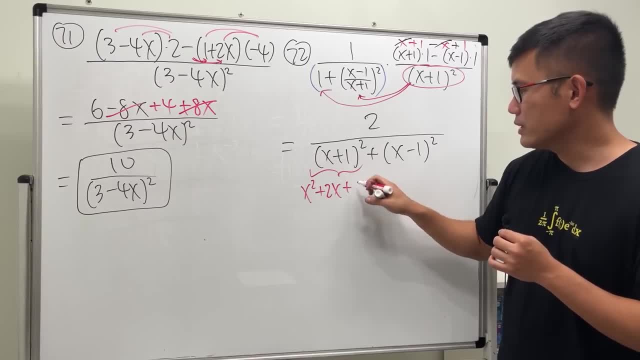 out. we get x squared plus two times this and that which is 2x plus two times this, and that which is 2x plus two times this and that which is 2x, and then plus one square, and then plus one square, and then plus one square, and then, for this version is: 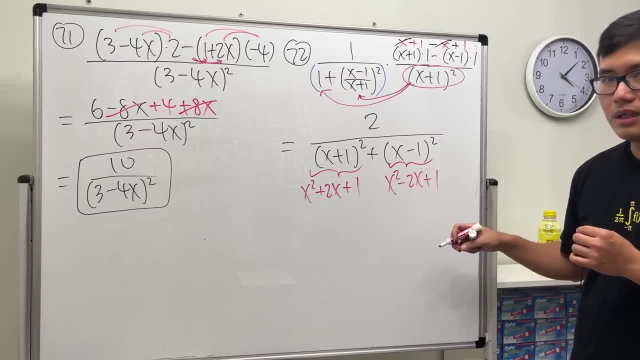 and then for this version is: and then for this version is: x squared minus 2x and then plus one. x squared minus 2x and then plus one. x squared minus 2x and then plus one. we're adding this and that together. but we're adding this and that together, but 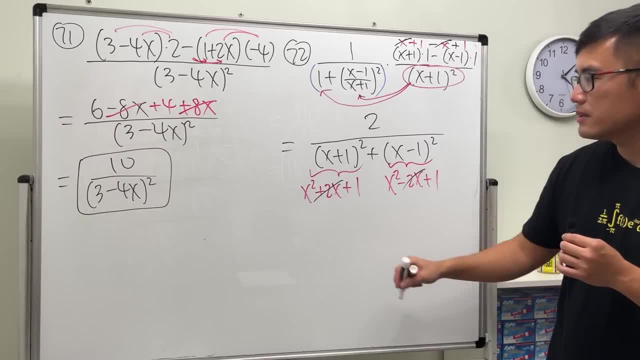 we're adding this and that together, but we see that. we see that. we see that 2x and negative 2x, they will be gone. 2x and negative 2x, they will be gone. 2x and negative 2x, they will be gone. finally, we have two on the top over. 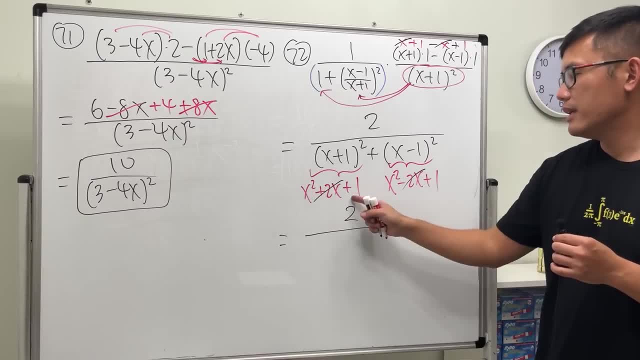 finally, we have two on the top over. finally, we have two on the top over: this and that which is this and that which is this and that which is 2x squared and then 2x squared, and then 2x squared and then two, so we can factor out the two and then. 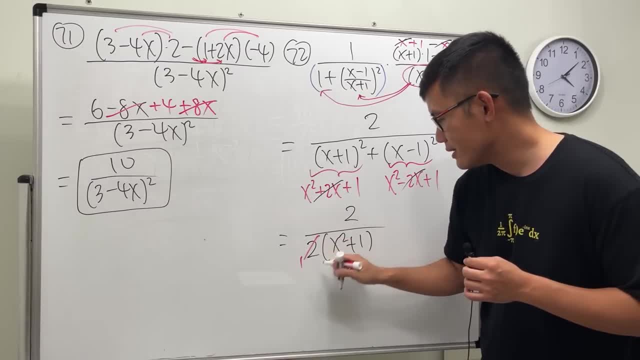 two, so we can factor out the two, and then two, so we can factor out the two, and then x squared plus one, x squared plus one, x squared plus one, and then reduce, and then reduce, and then reduce, so finally we get one over x squared. so finally, we get one over x squared. 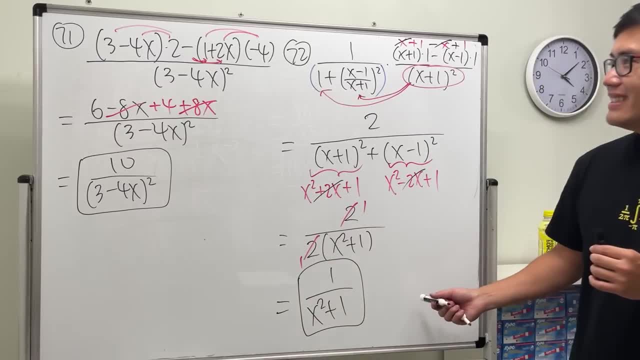 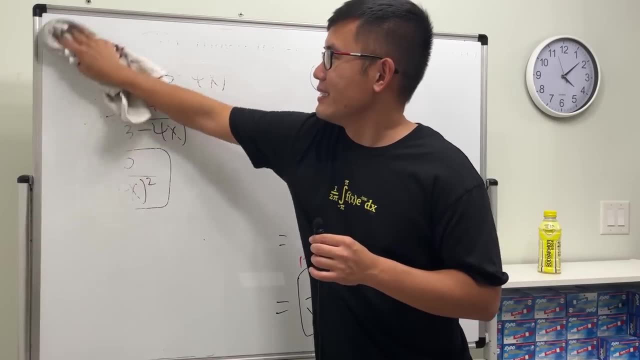 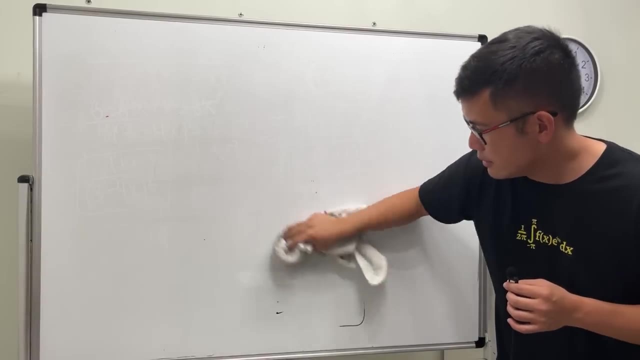 so finally we get one over x squared plus one plus one, plus one, done, done, done, okay, okay, okay. so some of these kind of questions they can, so some of these kind of questions they can, so some of these kind of questions they can actually simplify really really well. 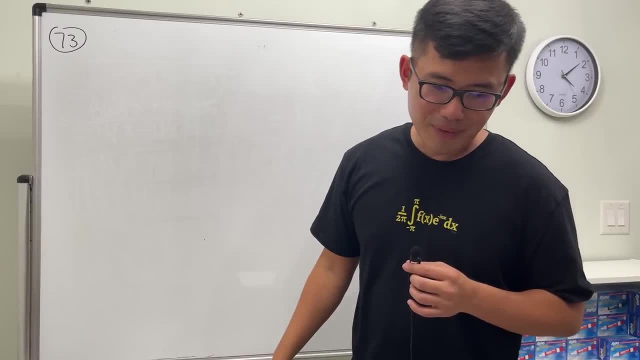 okay, okay, okay, okay. number, number, number, number number, so. so some of these kind of questions they can actually simplify really really well. so some of these kind of questions they can actually simplify really really well. number 73: we have the following: so on: we have x to. 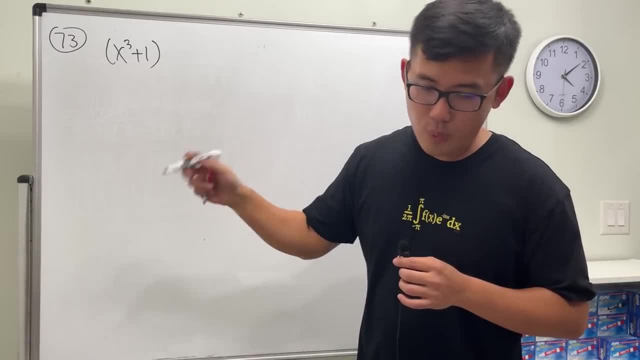 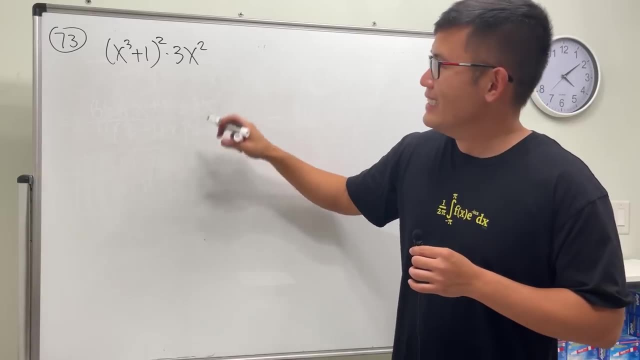 number 73. we have the following, so on. we have x to number 73. we have the following, so on: we have x to the third power plus 1 square times 3x. the third power plus 1 square times 3x. the third power plus 1 square times 3x square. and then minus x to the third. 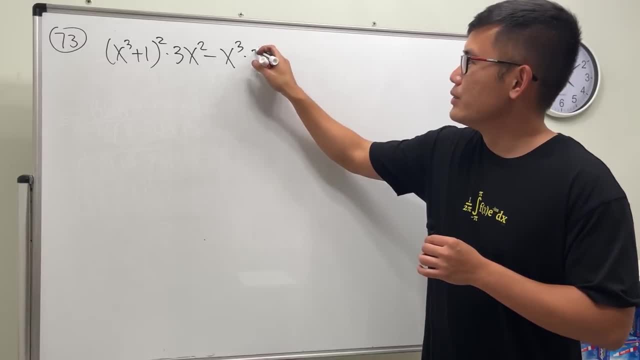 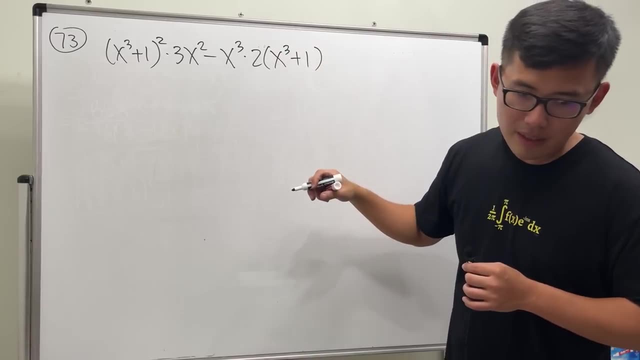 square and then minus x to the third square, and then minus x to the third power. times 2 times x to the third power. power. times 2 times x to the third power. power. times 2 times x to the third power plus 1 and then times 3x. 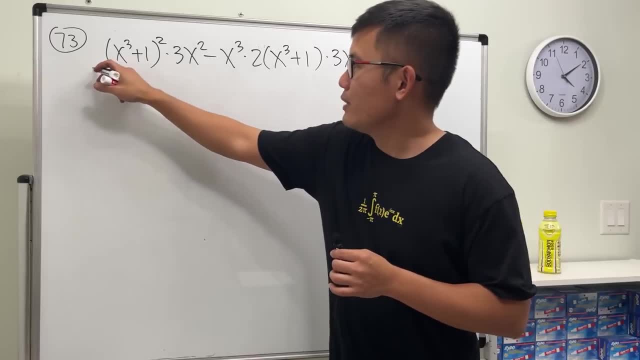 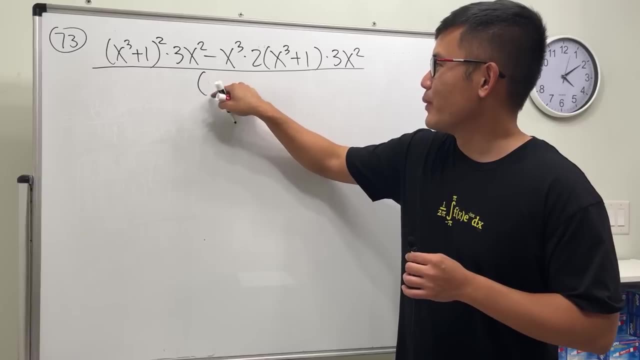 plus 1, and then times 3x plus 1, and then times 3x, square, square, square everybody over. x to the third power, x to the third power, x to the third power plus one, and then to the fourth power: okay, plus one. and then to the fourth power: okay. 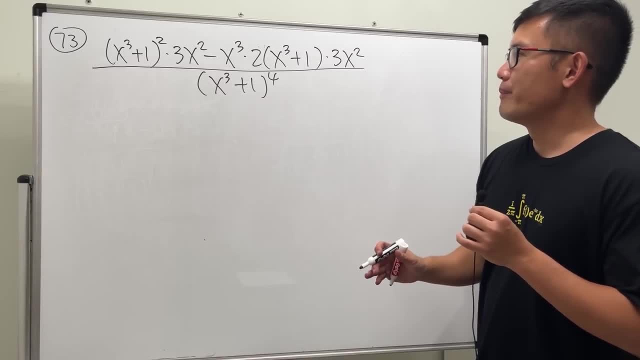 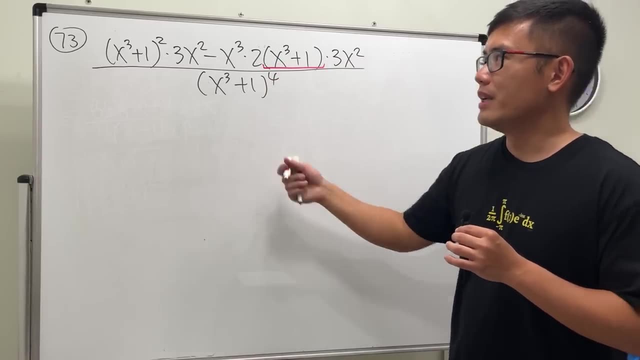 plus one. and then to the fourth power. okay, number 73, number 73, number 73, hmm, hmm, hmm, before we multiply anything, before we multiply anything, before we multiply anything, notice that here we have notice that, here we have notice that here we have x- to the third power plus one, and this: 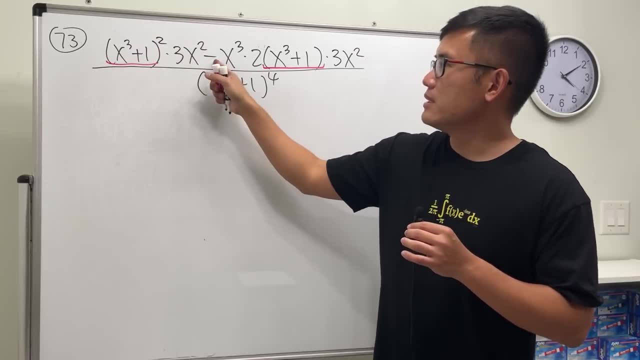 x to the third power plus one, and this x to the third power plus one. and this right here has a second power. so right here has a second power. so right here has a second power. so this is one term right because it's. this is one term right because it's. 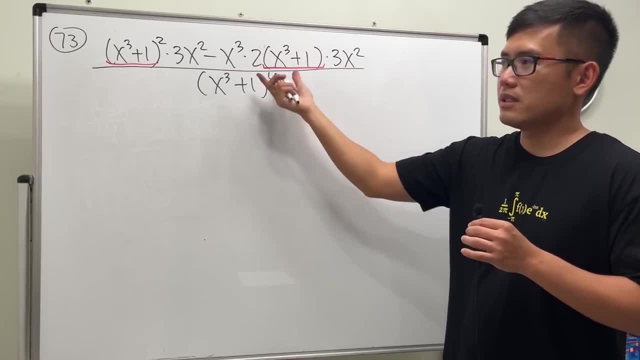 this is one term right, because it's separate by this, separate by this, separate by this subtraction, and this is another because subtraction and this is another because subtraction and this is another because that's just multiplying it. that's just multiplying it, that's just multiplying it, so we can actually factor that out. so 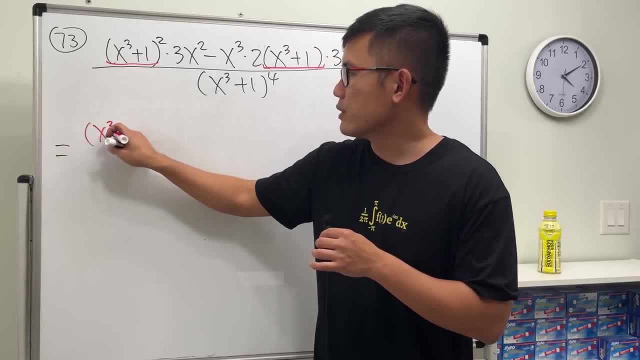 so we can actually factor that out. so, so we can actually factor that out. so let's see this right here: if we factor- let's see this right here- if we factor- let's see this right here- if we factor it out, we will get x plus 3 power plus. 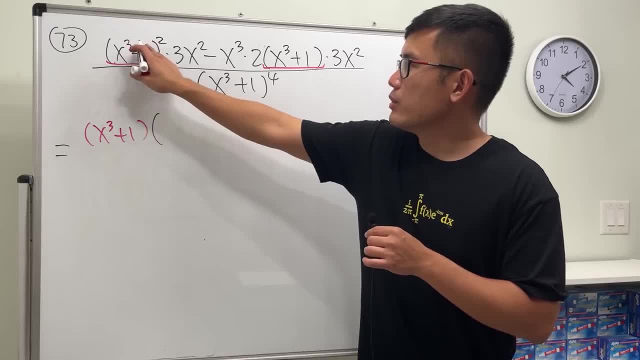 it out. we will get x plus 3 power plus it out. we will get x plus 3 power plus one all the way at the front, and then one all the way at the front, and then one all the way at the front, and then this is going to be okay, we can write. 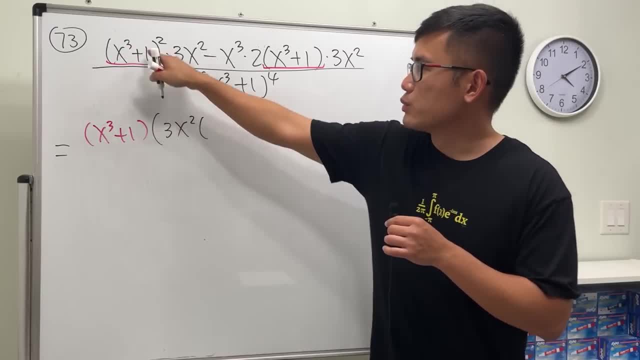 this is going to be okay. we can write. this is going to be okay. we can write this down first. so this down first. so this down first. so 3x squared times one more of this right. 3x squared times one more of this right. 3x squared times one more of this right. so just x to the third power plus one. 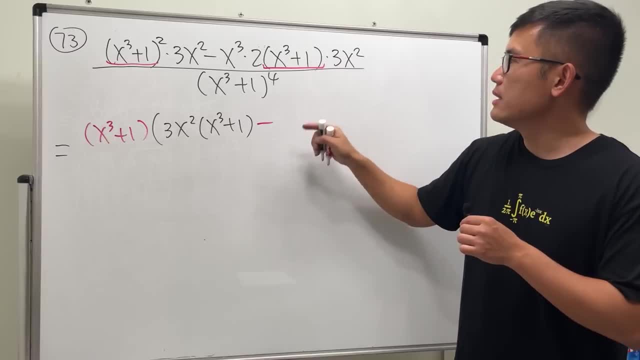 so just x to the third power plus one. so just x to the third power plus one. minus, minus, minus. put this down, minus. put this down minus. put this down: minus. 3 times 2 is 6 and the x squared times 3 times 2 is 6 and the x squared times. 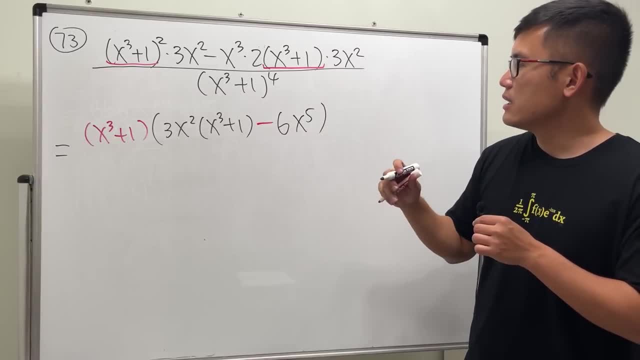 3 times 2 is 6 and the x squared times. that is x to the fifth power, that is x to the fifth power, that is x to the fifth power. yes and over, yes and over, yes and over this denominator, which is x to the third. 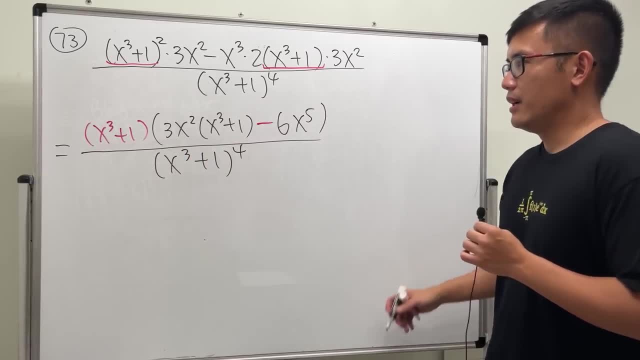 this denominator which is x to the third, this denominator which is x to the third, power plus one to the fourth power. power plus one to the fourth power. power plus one to the fourth power. okay, okay, okay. one thing we can cancel this out with. one thing we can cancel this out with. 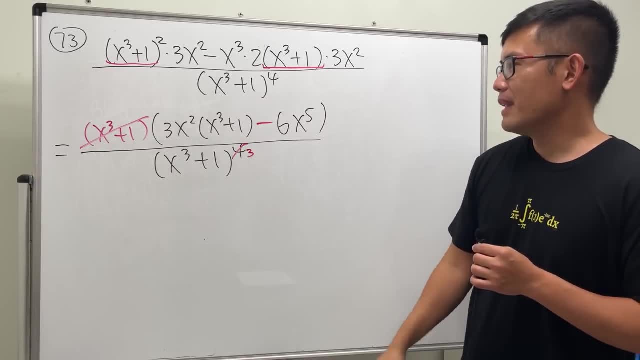 one thing: we can cancel this out with one of them. right, so the power becomes one of them. right, so the power becomes one of them. right, so the power becomes three, three, three. now we just have to work this out. if now, we just have to work this out. if 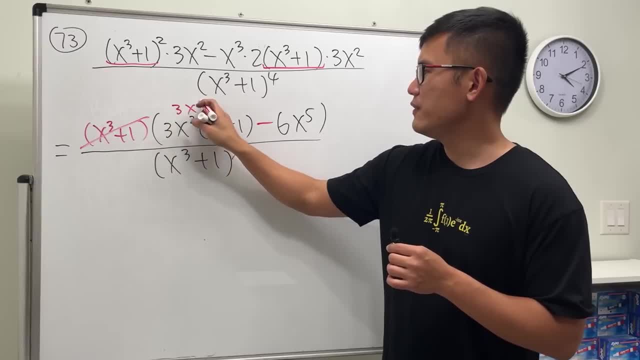 now we just have to work this out: if we multiply this, how we get, we multiply this, how we get, we multiply this, how we get 3x to the fifth power, and then plus 3x to the fifth power, and then plus 3x to the fifth power, and then plus 3x- squared. 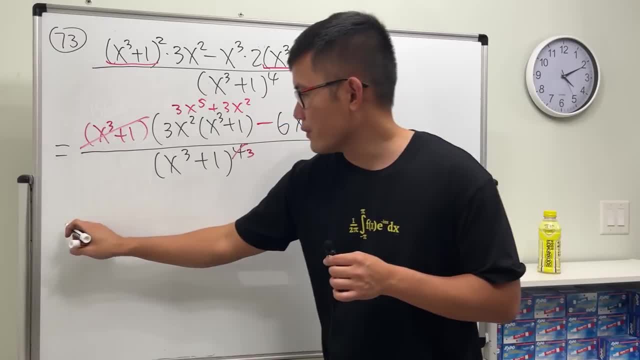 3x squared, 3x squared, and this and that can be combined. so we and this and that can be combined. so we and this and that can be combined. so we will, so, finally, will, so, finally will. so, finally, 3 minus 6, which is negative, 3 x to. 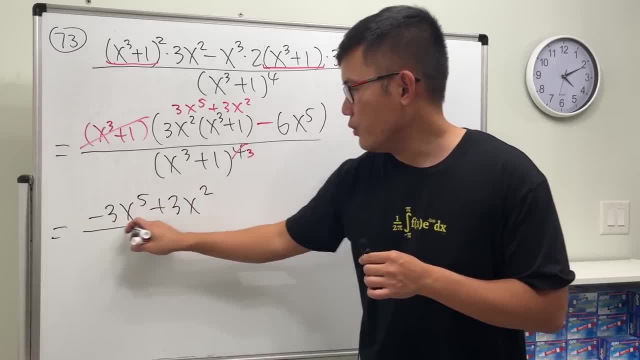 3 minus 6, which is negative. 3 x to 3 minus 6, which is negative. 3 x to the fifth power plus 3x squared. the fifth power plus 3x squared. the fifth power plus 3x squared, or over that which is x to the third. 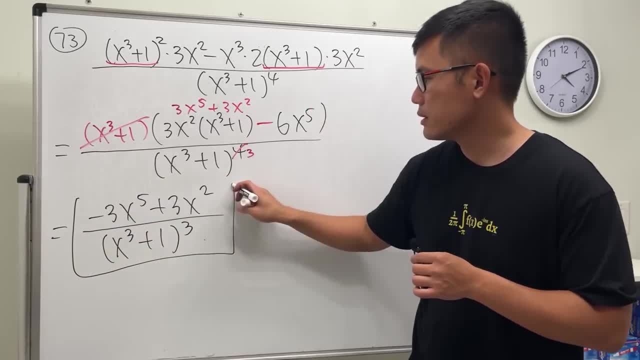 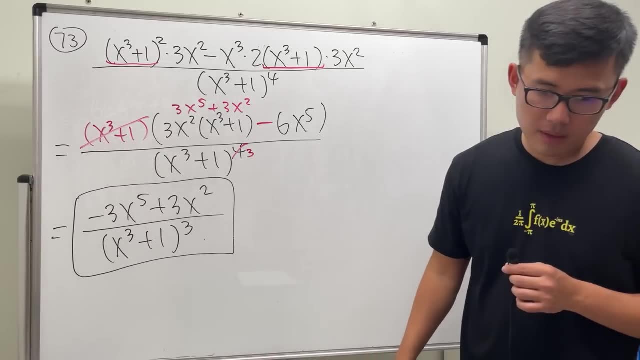 or over that which is x to the third, or over that which is x to the third power plus one, and then to the third power plus one, and then to the third power plus one and then to the third power. done, yeah, and then here is the trouble again i. 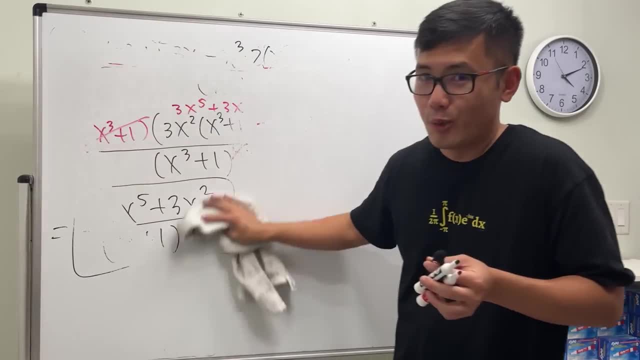 yeah. and then here is the trouble again. i, yeah, and then here is the trouble again: i will have to erase the board like every will have to erase the board like every will have to erase the board like every single time, single time, single time, because the question is so big. and then 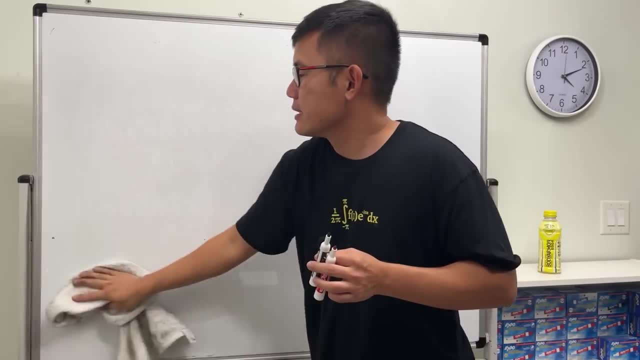 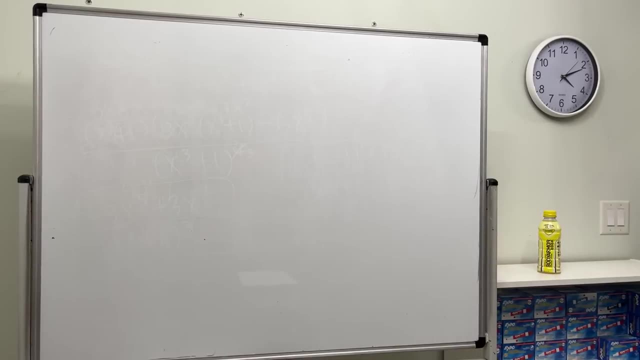 because the question is so big, and then, because the question is so big, and then, yeah, it will take the whole board to. yeah, it will take the whole board to. yeah, it will take the whole board to fit in the equation. okay, just let me make sure that. 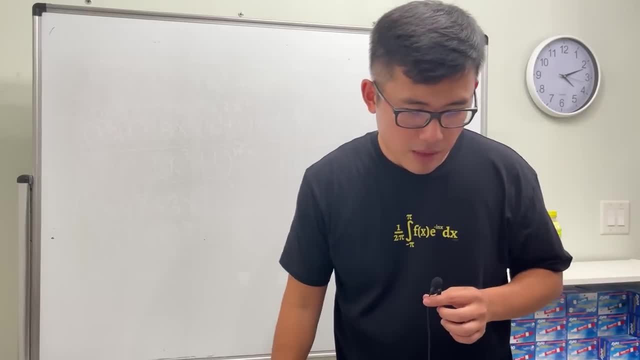 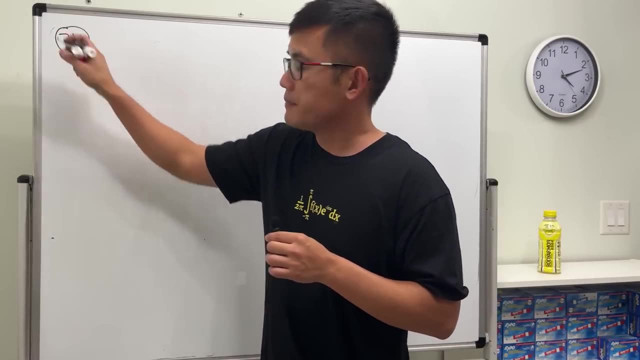 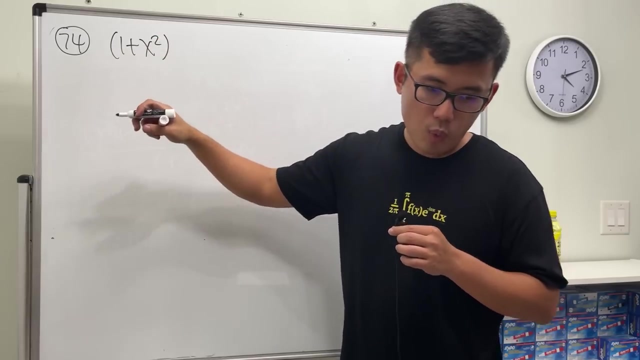 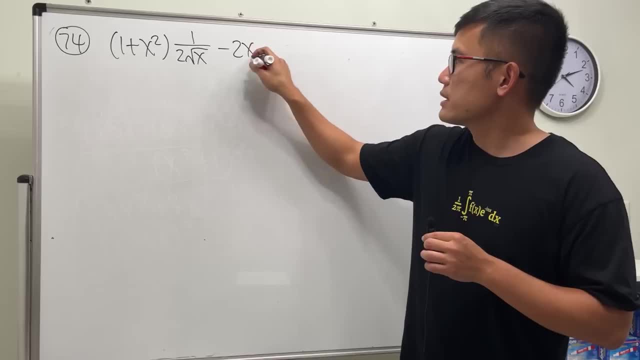 times 1 over 2x. 1 over 2 square root of x times 1 over 2x. 1 over 2 square root of x and then minus, and then minus, and then minus. 2x square root of x over 2x square root of x over. 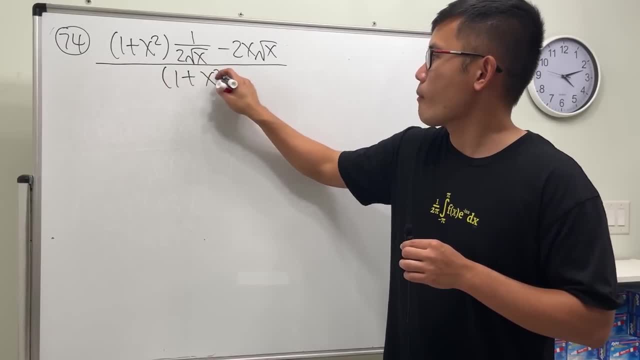 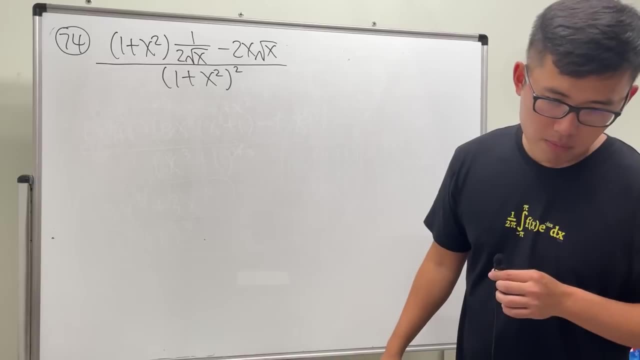 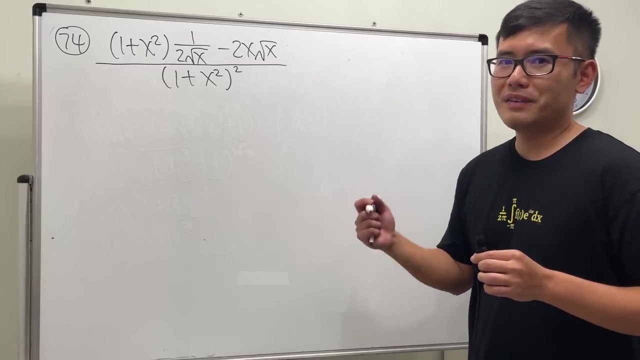 2x square root of x, over 1 plus x square square. 1 plus x square square. okay. so 1 plus x square square. okay. so 1 plus x square square. okay. so how can we simplify this? how can we simplify this? how can we simplify this? well, we have a complex fraction, so we have: 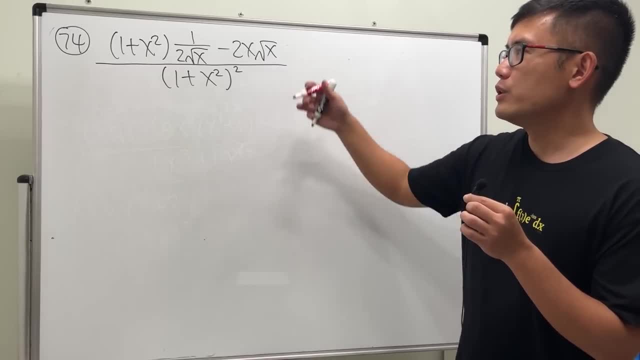 well, we have a complex fraction, so we have. well, we have a complex fraction, so we have to remember what we did before. right to remember what we did before. right to remember what we did before, right. if we have a complex fraction, we're just. if we have a complex fraction, we're just. 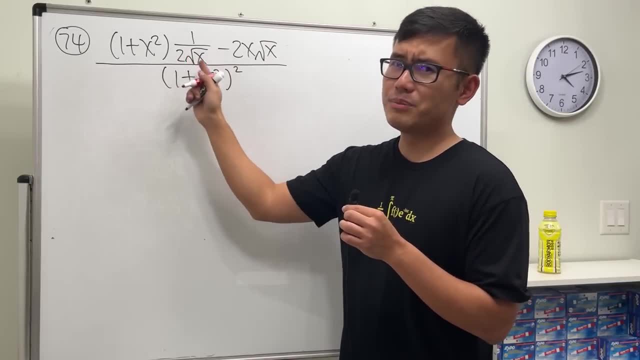 if we have a complex fraction, we're just going to multiply the top and bottom. by going to multiply the top and bottom, by going to multiply the top and bottom by the common denominator the small one. so the common denominator the small one, so the common denominator the small one. so just this. so let's go ahead and multiply. 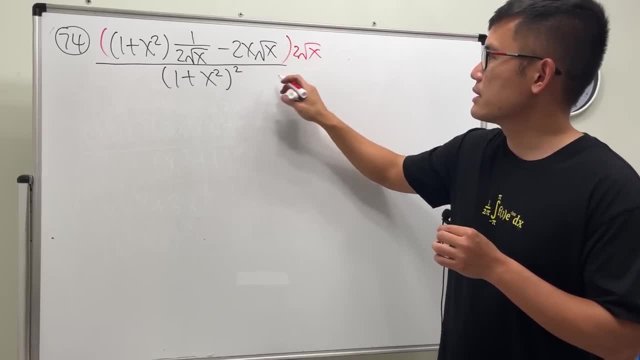 just this. so let's go ahead and multiply just this. so let's go ahead and multiply the bottom and the top by the bottom and the top, by the bottom and the top, by 2 square root of x, 2 square root of x, 2 square root of x. okay, let's see what we get. take this times. 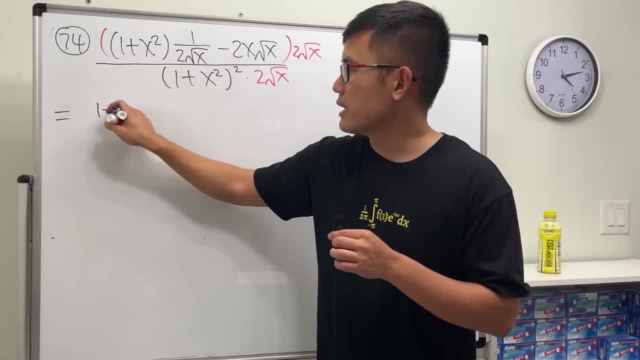 okay, let's see what we get. take this times: okay, let's see what we get. take this times: the first term, the first term, the first term: they cancel. so we just have 1 plus x. they cancel. so we just have 1 plus x. they cancel. so we just have 1 plus x square. 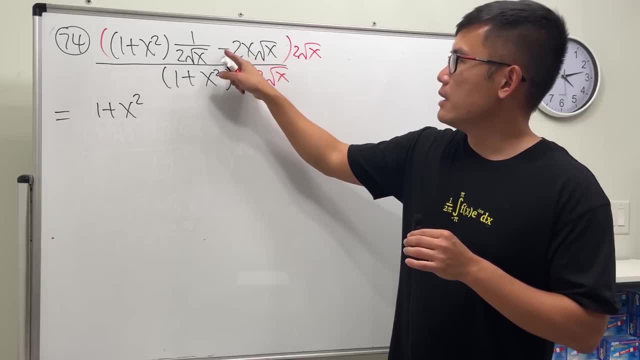 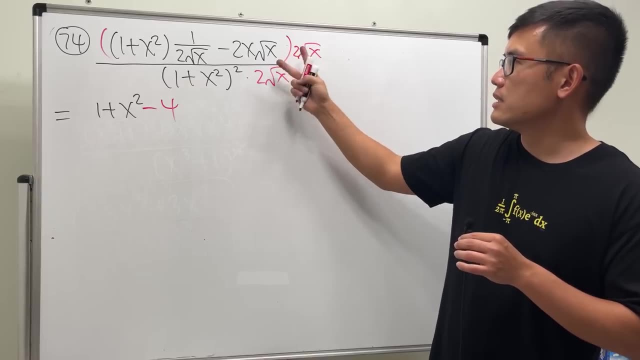 square, square. nothing else, nothing else, nothing else. next we take this times, that next we take this times that. next we take this times that minus minus minus 2 times 2 is 4. 2 times 2 is 4. 2 times 2 is 4. square root of x times square root of x. 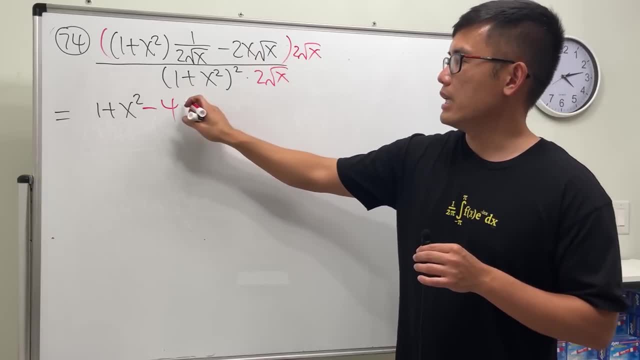 square root of x times square root of x. square root of x times square root of x. this is just x. this is just x. this is just x times one more. so it's x square. yeah, times one more. so it's x square, yeah, times one more. so it's x square. yeah, it's x. 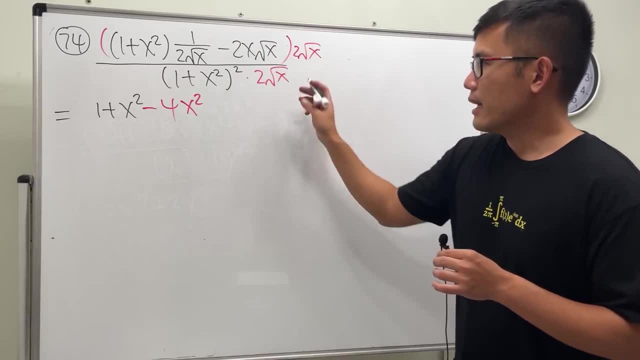 it's x, it's x. one more so x squared. one more so x squared. one more so x squared. and then on the bottom we'll just keep, and then on the bottom we'll just keep, and then on the bottom we'll just keep it as that. so that is 2 square root of x. 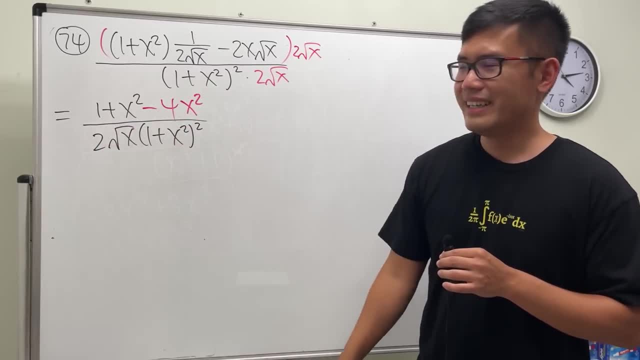 it as that: so that is 2 square root of x. it as that: so: that is 2 square root of x times 1 plus x square, and then square times 1 plus x square, and then square times 1 plus x square and then square. and of course, right here we can combine: 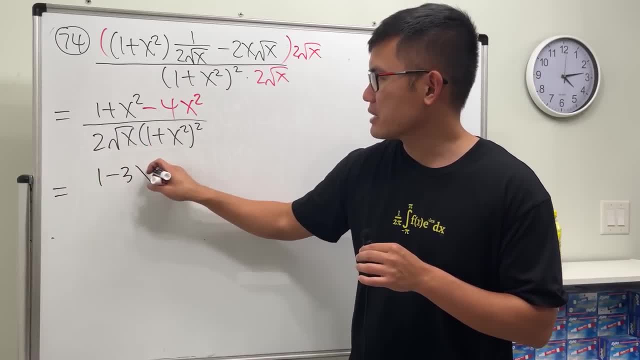 and of course, right here we can combine. and of course, right here we can combine like terms. so this is 1 minus 3 like terms. so this is 1 minus 3 like terms. so this is 1 minus 3 x square over 2, square root of x times 1. 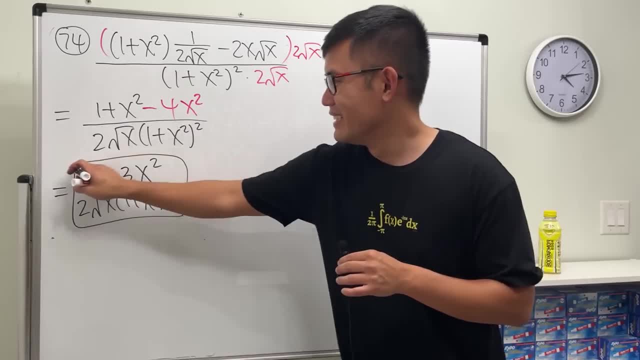 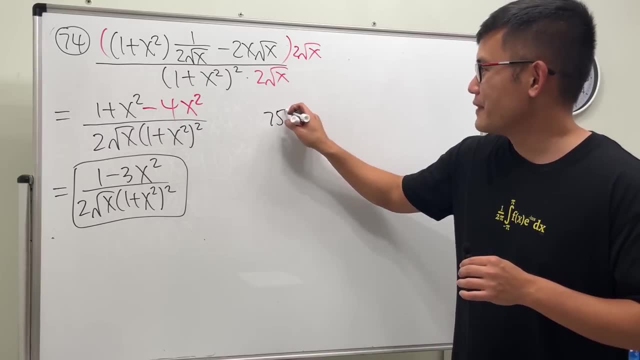 x square over 2, square root of x times 1. x square over 2, square root of x times 1 plus x square, and then square plus x, square, and then square plus x, square, and then square. yay, done, yay, done, yay, done. uh, let me fitting number 75 here should: 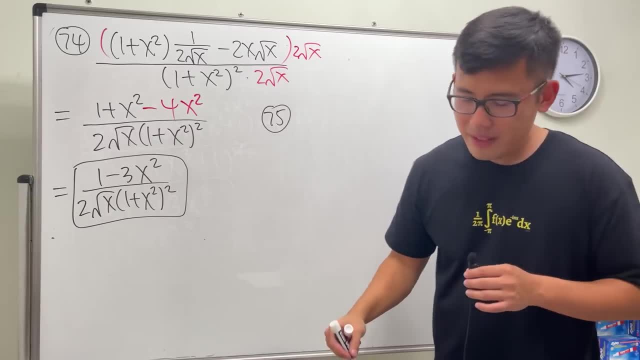 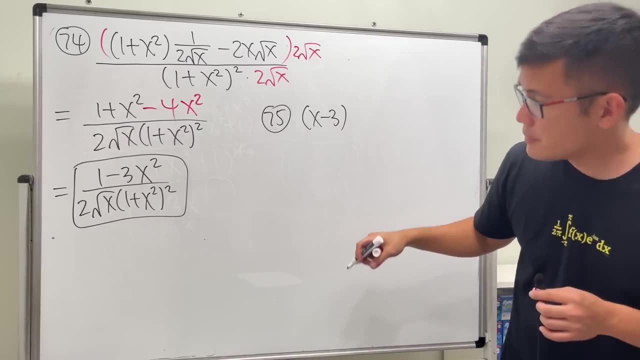 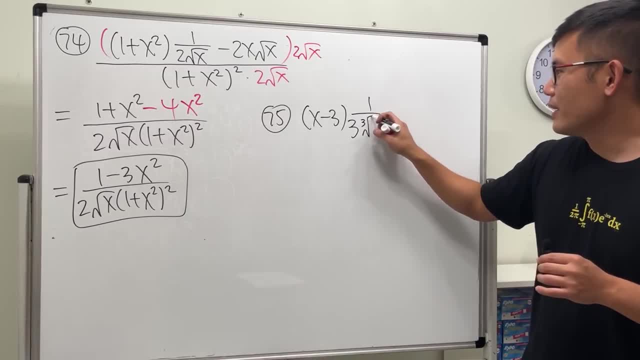 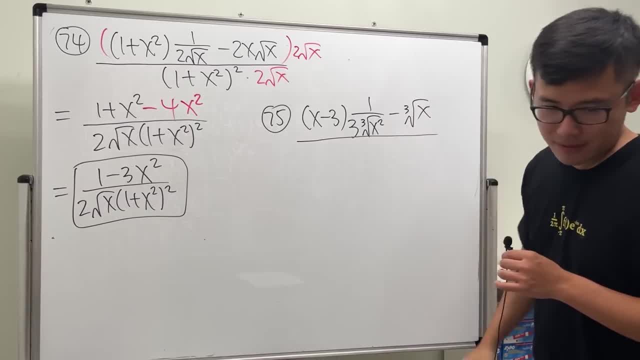 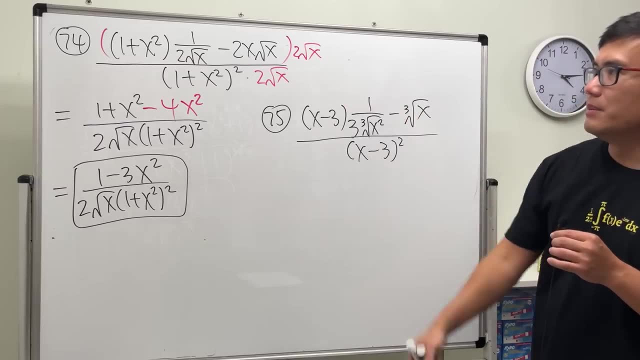 yeah and then minus. yeah and then minus. the cube root of x, the cube root of x, the cube root of x, over over over x minus three square. all right, so very similar. let's just go all right. so very similar. let's just go. all right, so very similar. let's just go ahead and get to work. 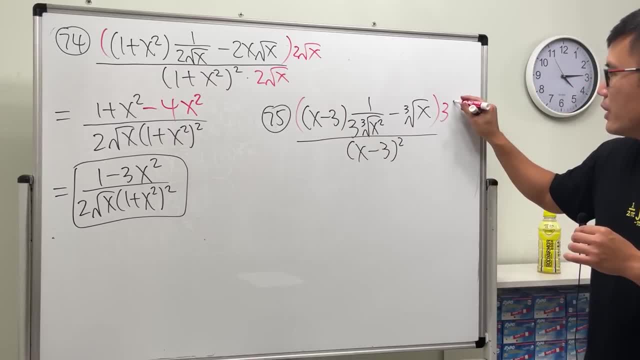 ahead and get to work, ahead and get to work. multiply the top and bottom by this. so multiply the top and bottom by this. so multiply the top and bottom by this, so three cube root of x square, so three. three cube root of x square, so three, three cube root of x square. 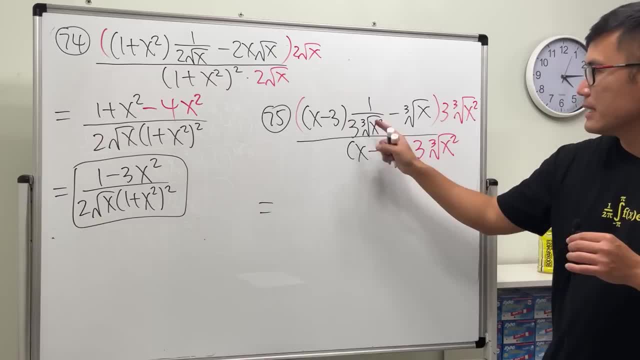 three cube root of x square, so three cube root of x square. three cube root of x square, so three cube root of x square. okay, okay, okay, take that times that they cancel. so we take that times that they cancel. so we take that times that they cancel. so we just have x minus three first. 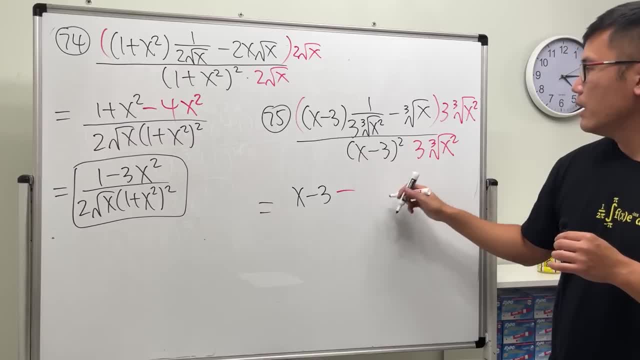 just have x minus three first. just have x minus three, first then minus. all right, this is just a regular three. all right, this is just a regular three. all right, this is just a regular three. but cube root of x times cube root of x. but cube root of x times cube root of x. 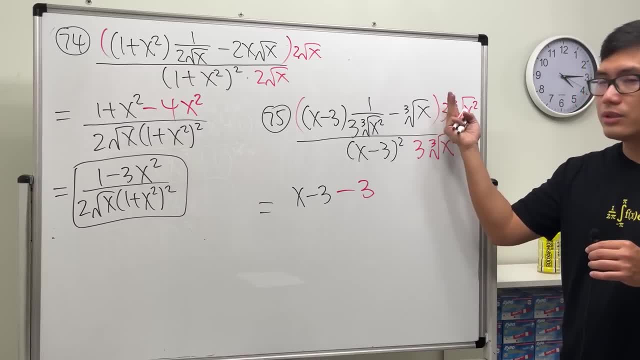 but cube root of x times cube root of x. square, it's just x. yeah, because you add square, it's just x. yeah, because you add square, it's just x. yeah, because you add that powers inside just third power x, that powers inside just third power x. 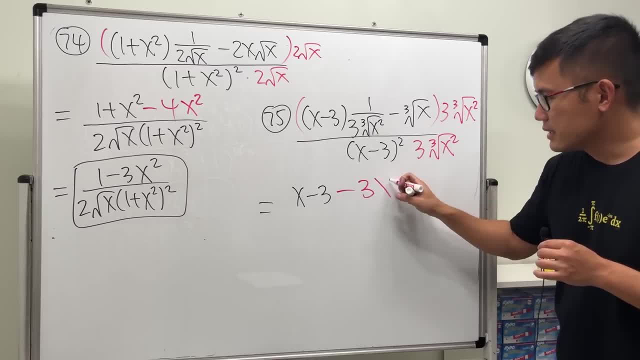 that powers inside just third power- x plus third power inside, plus third power inside, plus third power inside of the cube root, such as x- okay, and of the cube root such as x- okay, and of the cube root such as x- okay, and then on the bottom, we'll just leave it. 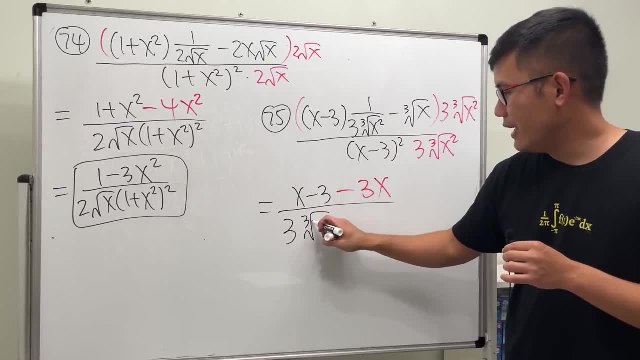 then on the bottom we'll just leave it, then on the bottom we'll just leave it. so three, so three, so three. cube root of x. square times x minus cube root of x. square times x minus cube root of x. square times x minus three. three, three square. and then of course this and that. 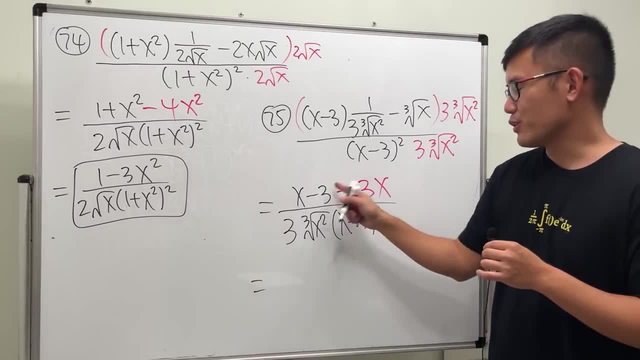 square, and then of course this and that square, and then of course this and that: cancel them out, cancel them out, cancel them out. and because x comes first here, so i will, and because x comes first here, so i will, and because x comes first here, so i will also write that down first. so negative. 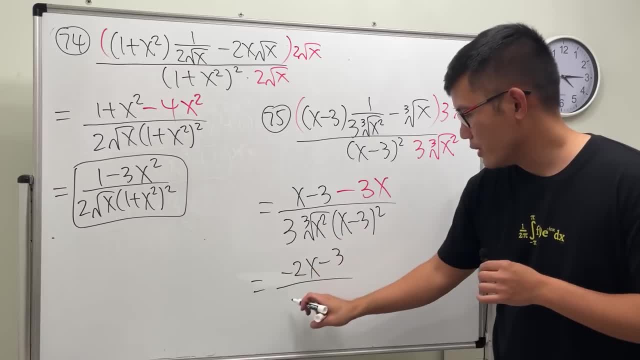 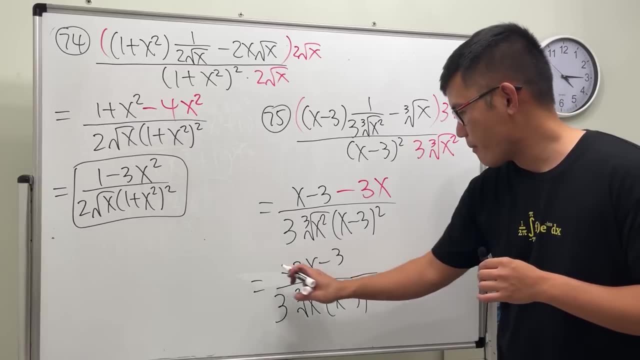 also write that down first. so negative. also write that down first. so negative. two x two x. two x minus three. over minus three, over minus three over three, three, three. cube root of x. square times x minus three. cube root of x. square times x minus three. cube root of x. square times x minus three and then square. 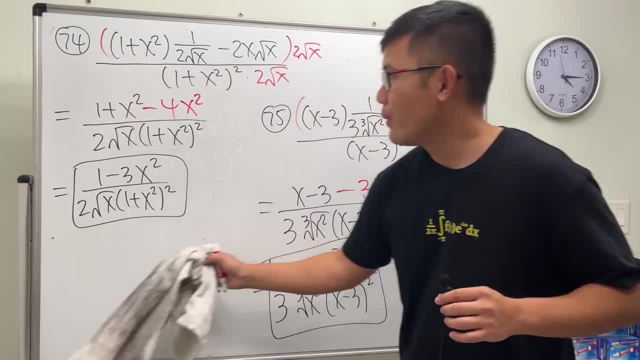 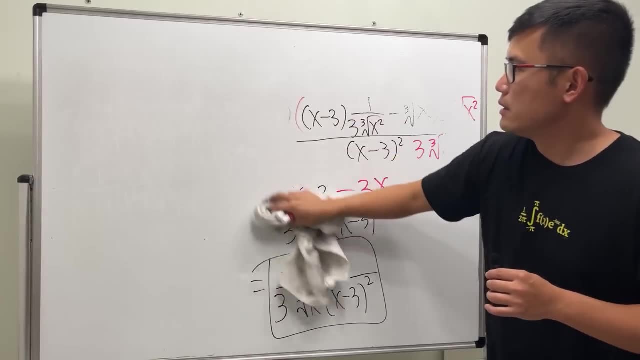 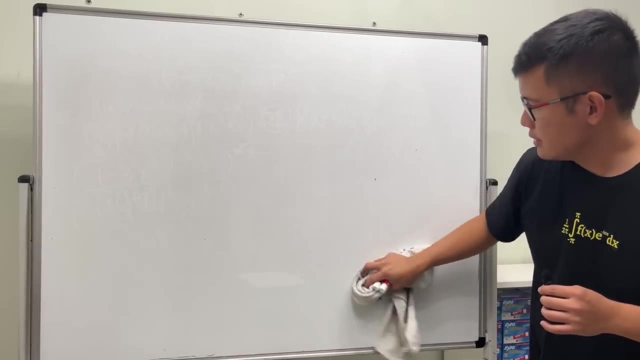 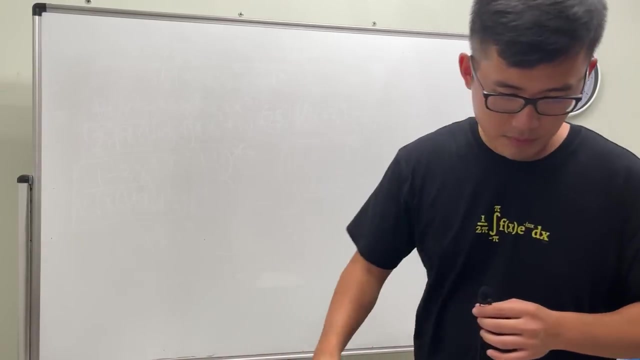 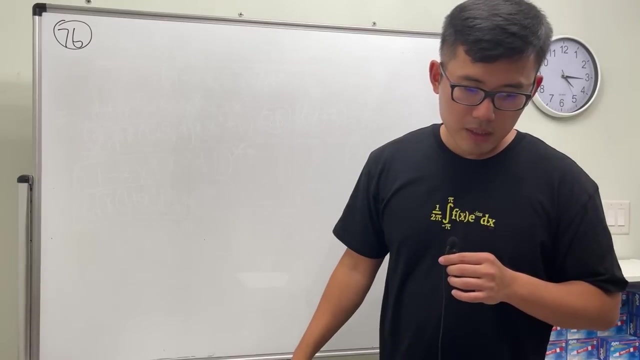 just like that, like that: 76. okay, we have square root of 76. okay, we have square root of 76. okay, we have square root of one minus. so square root: one plus x, one minus. so square root: one plus x, one minus. so square root: one plus x square. 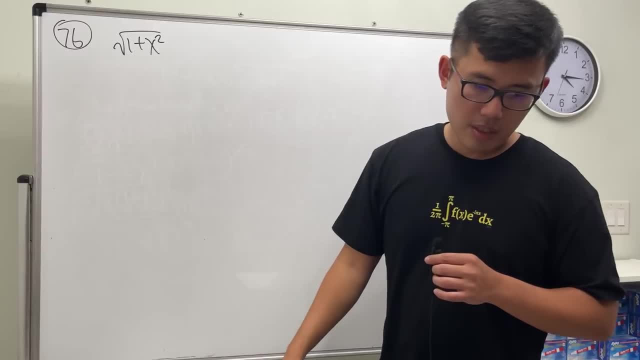 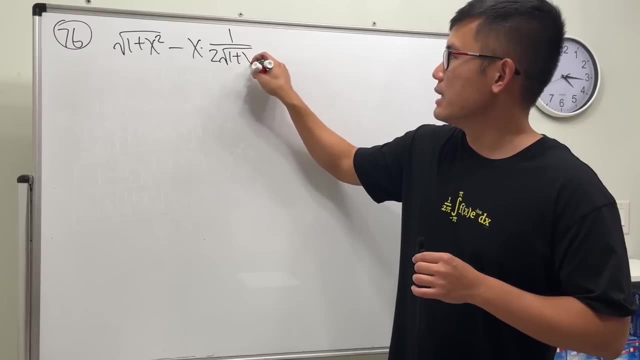 square square square root of one plus x. square square root of one plus x. square square root of one plus x. square minus x, minus x, minus x times one over two. square root of one times one over two. square root of one times one over two. square root of one plus. 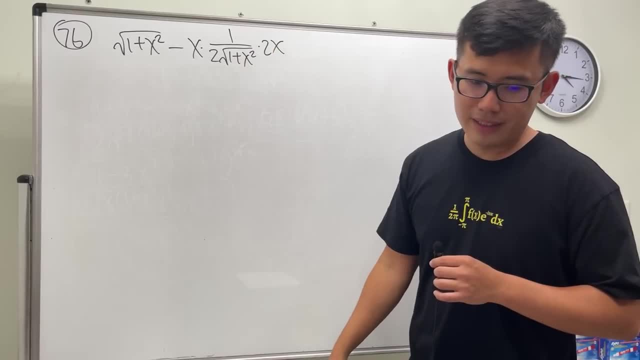 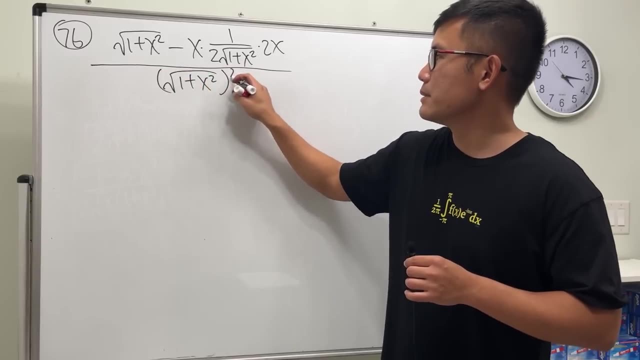 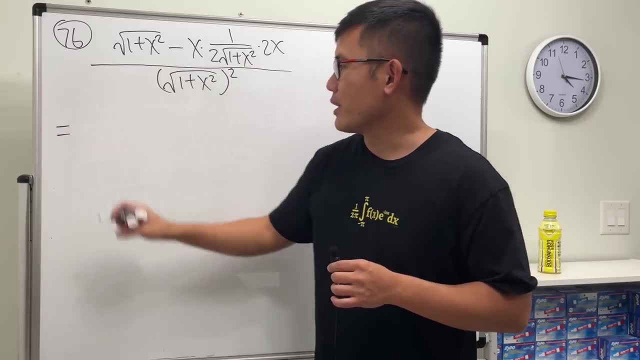 but then we square that, but then we square that. so that's good, right out, okay, let's see. so that's good, right out, okay, let's see. so that's good, right out, okay, let's see what's going on. what's going on, what's going on. firstly, you should notice this right: 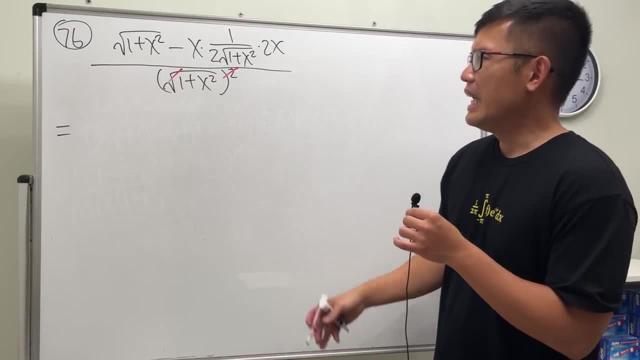 firstly, you should notice this right. firstly, you should notice this right away, away, away, square, and also the square root square, and also the square root square, and also the square root: cancelled, yeah, cancelled, yeah, cancelled, yeah. and then again we have okay, two and two, and then again we have okay, two and two. 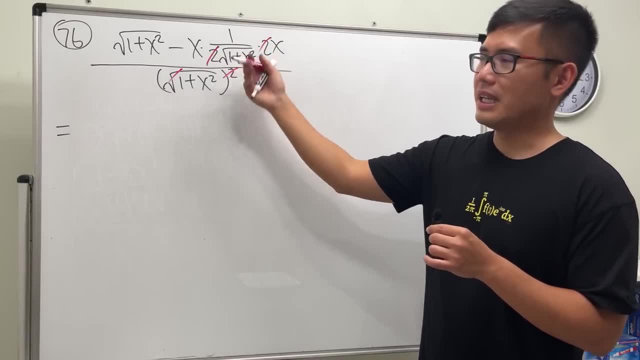 and then again we have, okay, two and two cancel, that's good, but we have this cancel, that's good, but we have this cancel, that's good. but we have this little denominator. so let's multiply the little denominator. so let's multiply the little denominator. so let's multiply the top and bottom by. 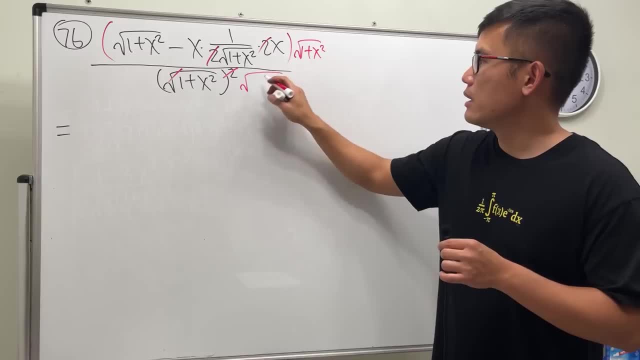 top and bottom. by top and bottom by square root of one plus x squared. square root of one plus x squared. square root of one plus x squared plus x squared okay. plus x squared okay. plus x squared okay. so what exactly do we have this times? so what exactly do we have this times? 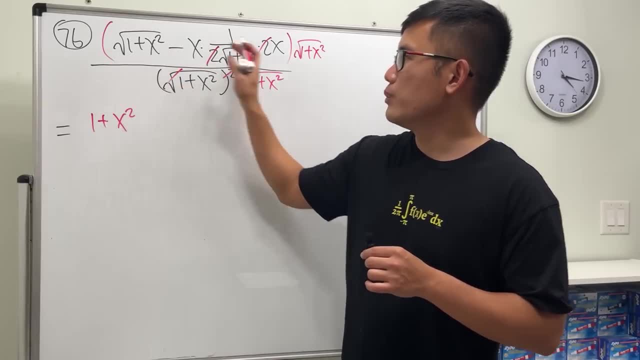 so what exactly do we have this times? that is just, that is just. that is just one plus x squared right- no more square one plus x squared right- no more square one plus x squared right. no more square root, root, root. this times that they cancel. but we have a. 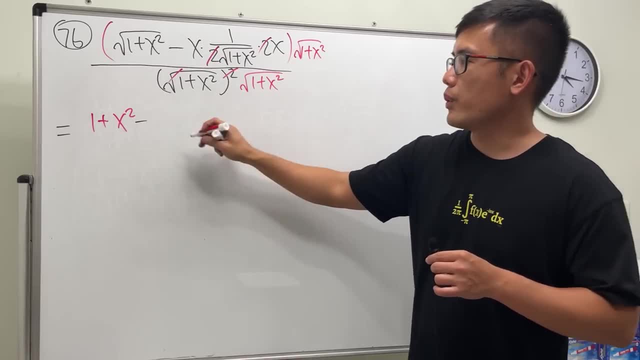 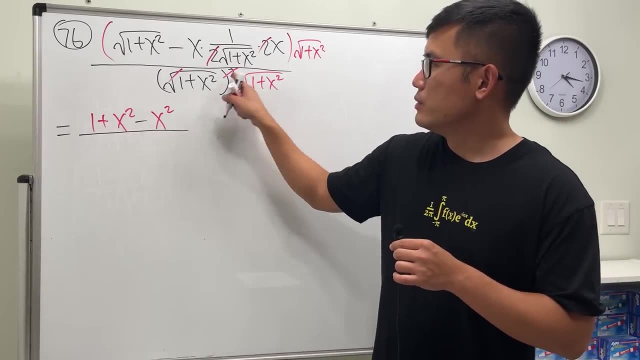 this times that they cancel. but we have a this times that they cancel. but we have a: minus x times x is x squared minus x times x is x squared minus x times x is x squared right, right, right, good, and then good, and then good, and then here, the earlier they canceled it. 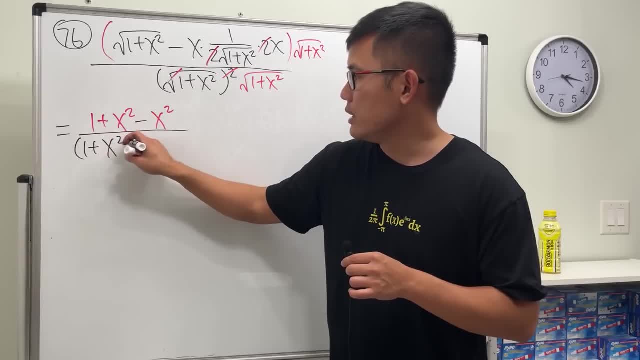 here. the earlier they canceled it here, the earlier they canceled it already. so we have already, so we have already. so we have parentheses, one plus x to the parentheses, one plus x to the parentheses, one plus x to the second power, and then we have the second power, and then we have the. 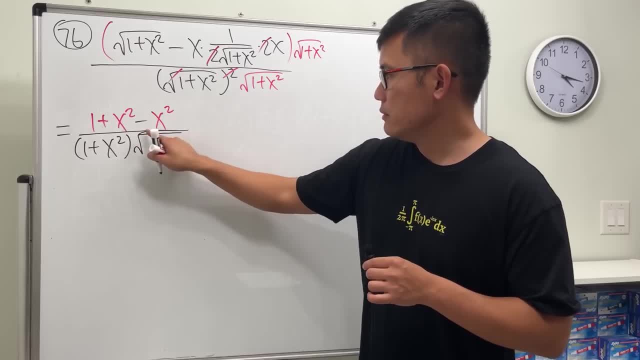 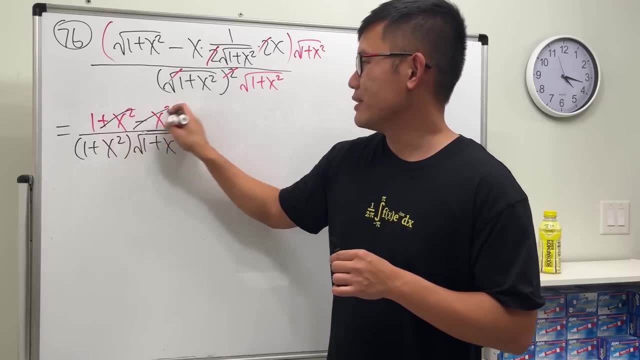 second power. and then we have the square root, so square root of, so, square root of, so, square root of one plus x squared. one plus x squared. one plus x squared on the top, on the top, on the top, this and that cancel out, so it looks that. 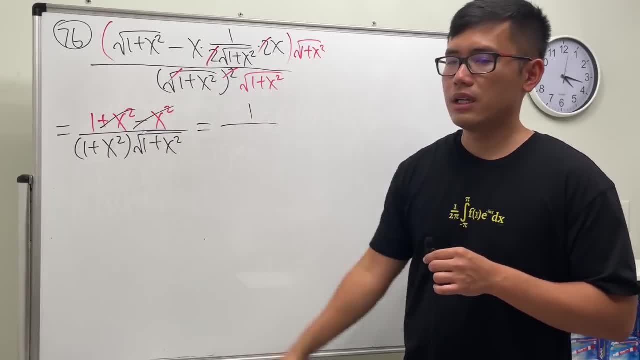 this and that cancel out. so it looks that this and that cancel out, so it looks that we just have, we just have, we just have one over one over one over that right, that right, that right. but notice the inside: this is one plus x. but notice the inside, this is one plus x. 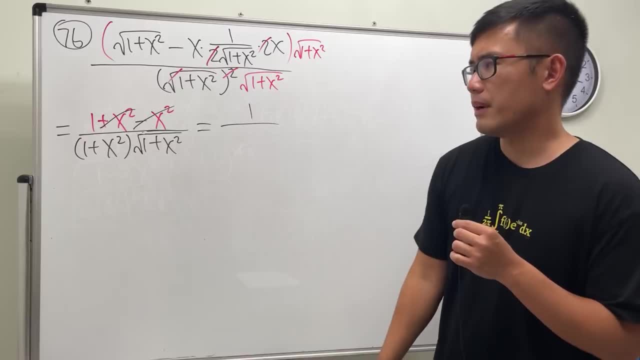 but notice the inside. this is one plus x square, and this is also one plus x square, and this is also one plus x square, and this is also one plus x square. so in fact, we can combine the square. so, in fact, we can combine the square. so, in fact, we can combine the powers. 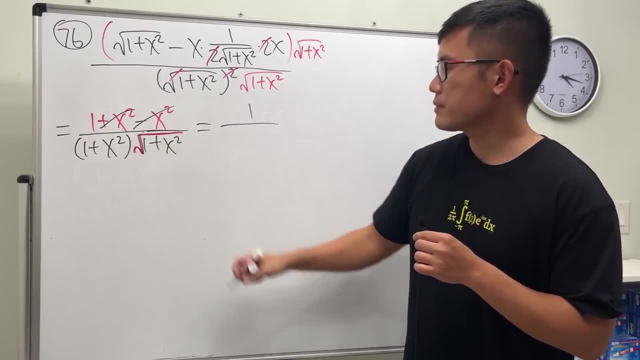 powers, powers. this right here is the same as one half. this right here is the same as one half. this right here is the same as one half. power, power, power. so let's go ahead and write it down. so let's go ahead and write it down. so let's go ahead and write it down like this: this is: 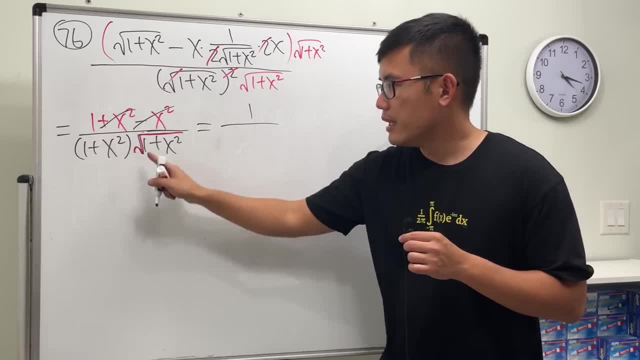 like this: this is like this. this is okay. let's do this in our head. okay, let's do this in our head. okay, let's do this in our head. this is the same as one half power. this, this is the same as one half power. this, this is the same as one half power. this is the first power. so one plus one half. 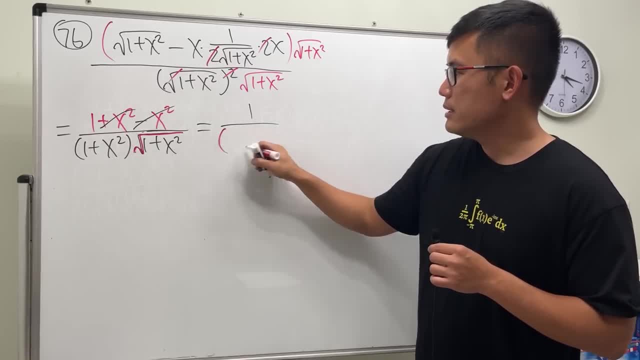 is the first power. so one plus one half is the first power. so one plus one half, three half. so we can write this as three half. so we can write this as three half. so we can write this as parentheses to the parentheses to the parentheses to the three half power with one plus x. 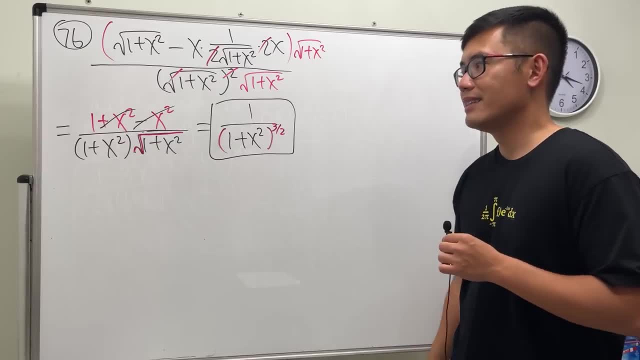 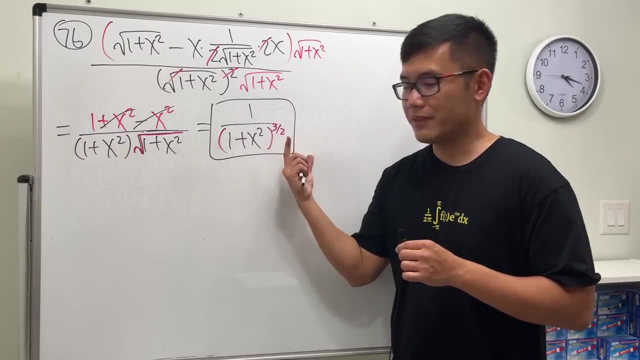 three half power with one plus x. three half power with one plus x- squared side, squared side, squared side. yeah, yeah, yeah, okay. one half power, okay, one half power, okay, one half power and the first power and the first power and the first power. add the powers, we get three half and we 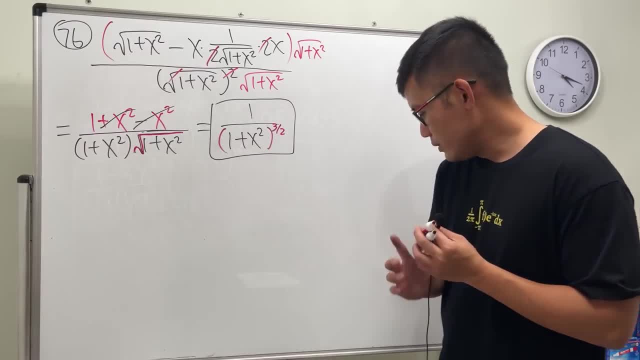 and the first power, add the powers, we get three half. and we and the first power, add the powers, we get three half. and we can just leave it like that, can just leave it like that, can just leave it like that. and if you want to rewrite this in, 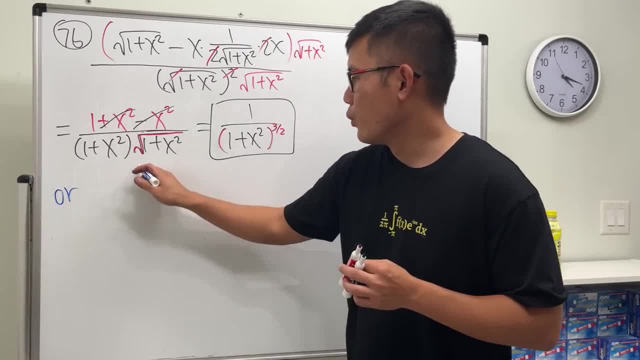 and if you want to rewrite this in, and if you want to rewrite this in different ways, you can also write this different ways. you can also write this different ways. you can also write this as one over, as one, over as one over the half power becomes a square root. 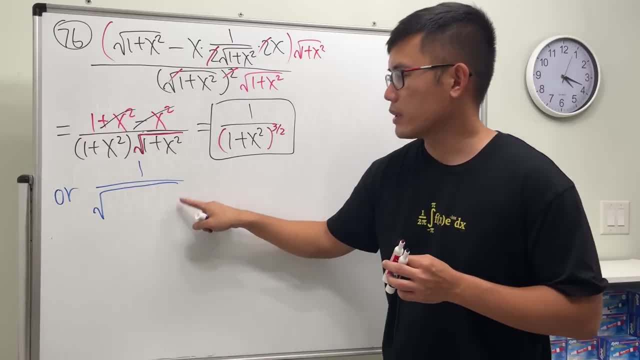 the half power becomes a square root, the half power becomes a square root, and then, and then, and then, the third power. you can put the third, the third power. you can put the third, the third power. you can put the third power on the outside or inside, usually. 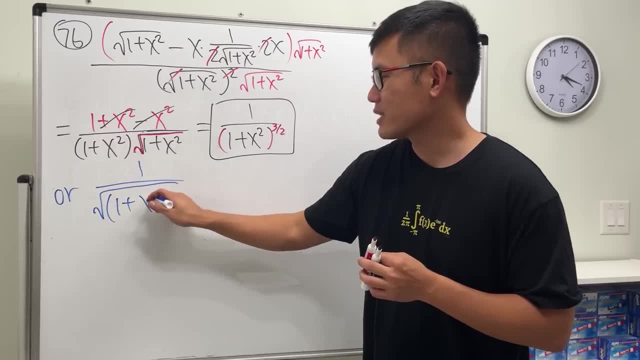 power on the outside or inside. usually power on the outside or inside. usually inside might look better. so just put it inside might look better, so just put it inside might look better. so just put it. one plus x square and then third power. one plus x square and then third power. 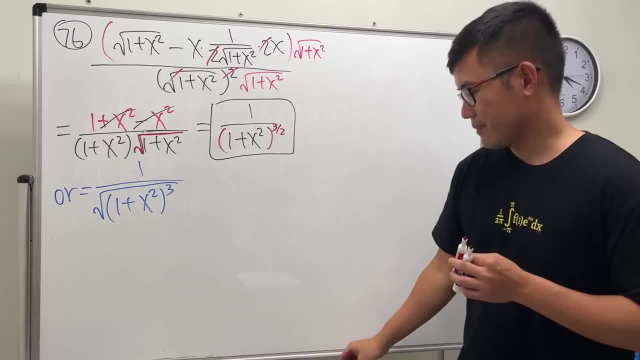 one plus x square, and then third power. so so, so, this or that okay, this or that okay, this or that okay, well, better. yet you can also look at two- well better. yet you can also look at two- well better yet, you can also look at: two plus one is three, and then the square. 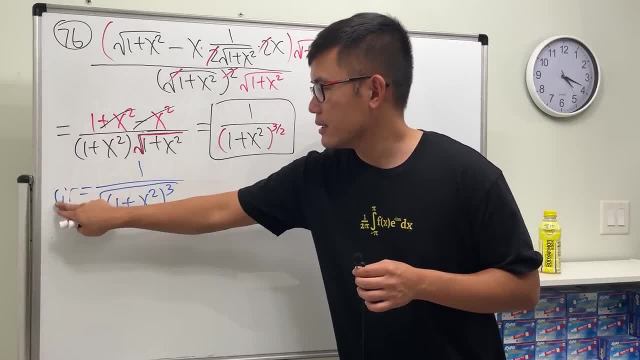 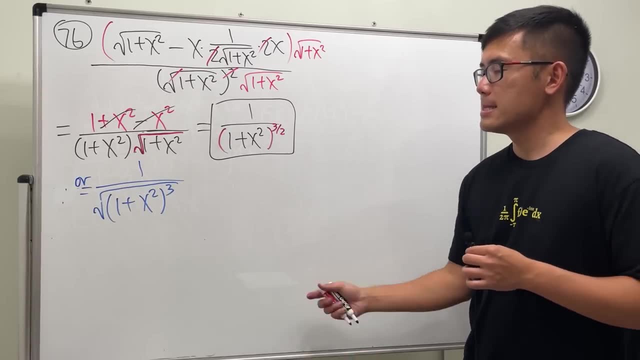 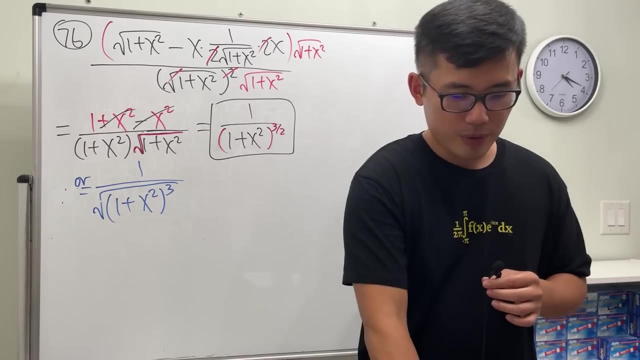 plus one is three, and then the square plus one is three, and then the square root is root is root is the half power. so yeah, okay, number 77 to 80. okay, number 77 to 80. okay, number 77 to 80. the question gets even bigger and bigger. 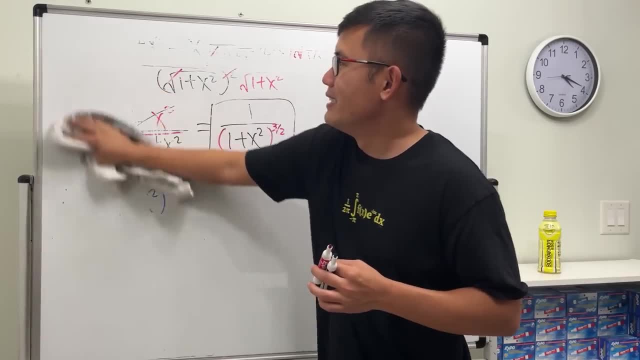 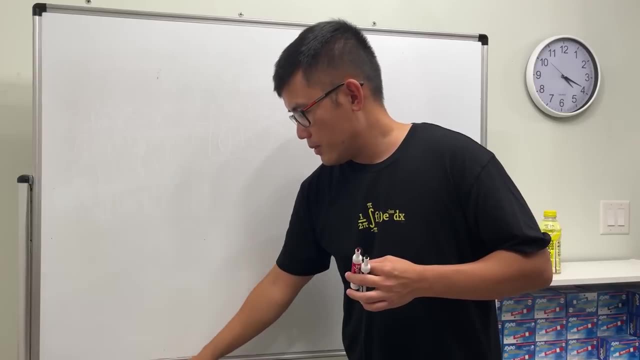 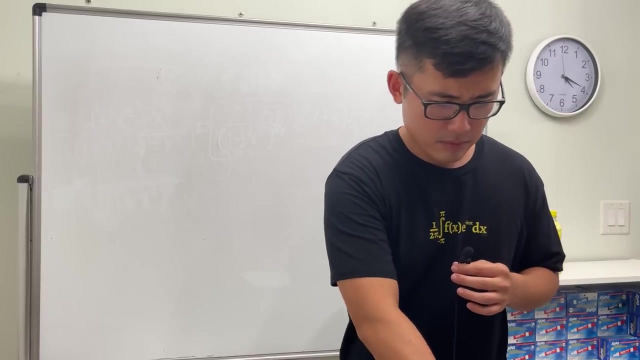 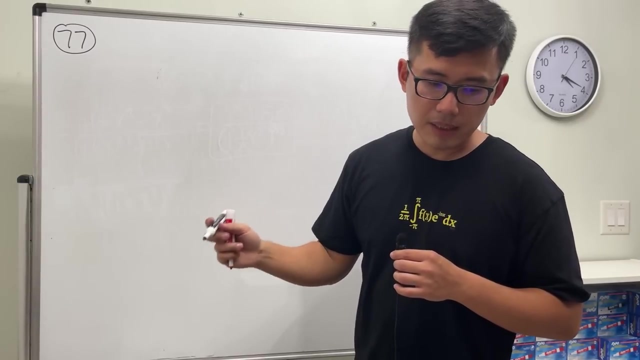 the question gets even bigger and bigger. the question gets even bigger and bigger. so i will have to erase this. so i will have to erase this, so i will have to erase this again. all right, number 77. we have x plus e to. all right, number 77, we have x plus e to. 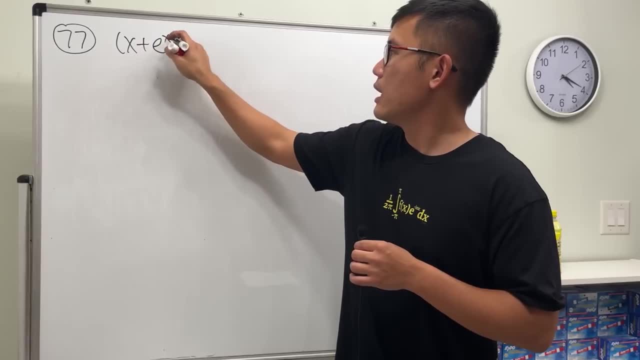 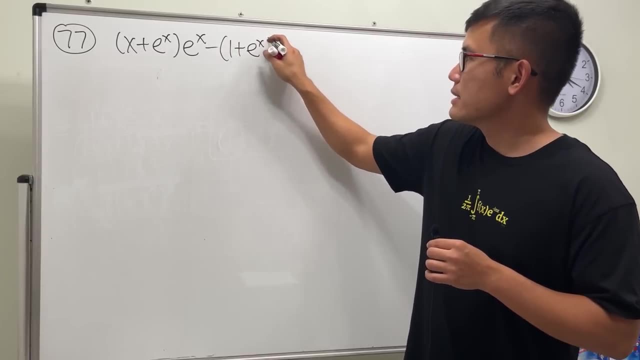 all right, number 77: we have x plus e to the x, the x, the x times e to the x and then minus times e to the x and then minus times e to the x and then minus 1 plus e to the x times 1 plus e to. 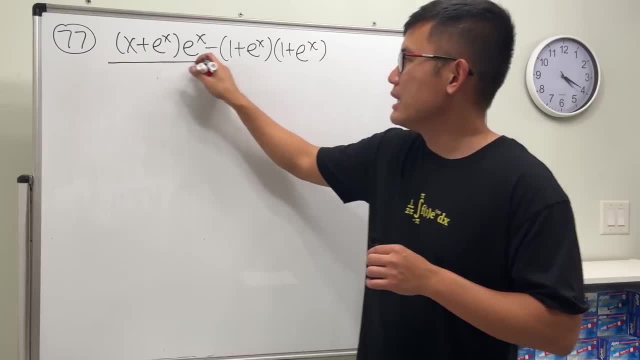 1 plus e to the x, times 1 plus e to the x, 1 plus e to the x, times 1 plus e to the x, times 1 plus e to the x, 1 plus e to the x, times 1 plus e to the x, and then all divided by: 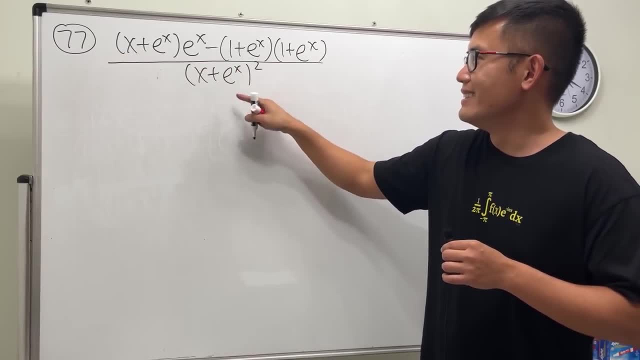 and then all divided by, and then all divided by x plus e to the x, and then square: x plus e to the x, and then square x plus e to the x, and then square. okay, let's just go ahead and get to work. okay, let's just go ahead and get to work. 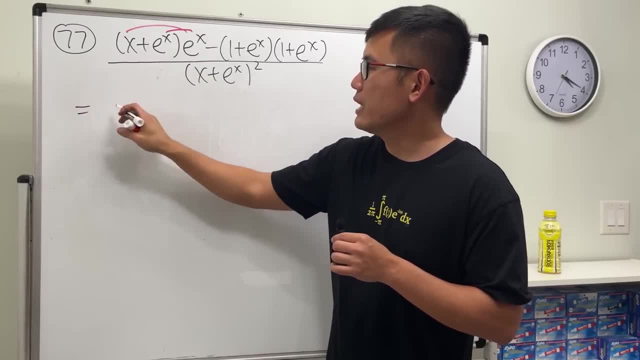 okay, let's just go ahead and get to work. so take this, distribute it backwards. so take this, distribute it backwards. so take this, distribute it backwards. all right, so we get x, e to the x. all right, so we get x, e to the x, and then e to the x times e to the x. 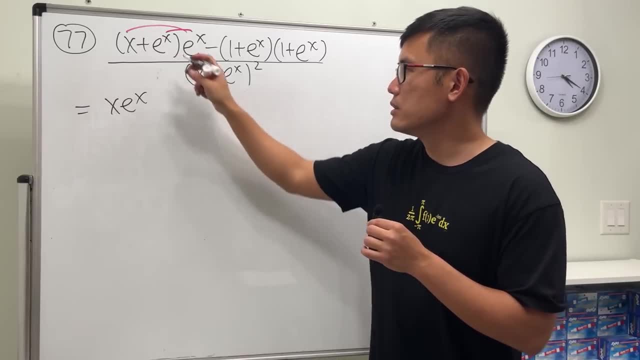 and then e to the x times e to the x, and then e to the x times e to the x. we just add the powers together. we just add the powers together. we just add the powers together. x plus x is just 2x, so together we get. 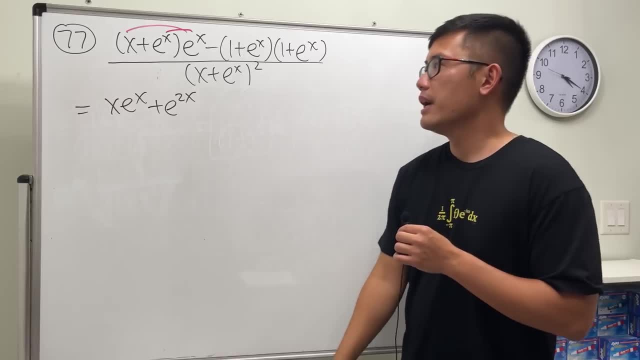 x plus x is just 2x, so together we get x plus x is just 2x, so together we get plus e to the 2x plus e to the 2x plus e to the 2x done for that part, and then we are going. 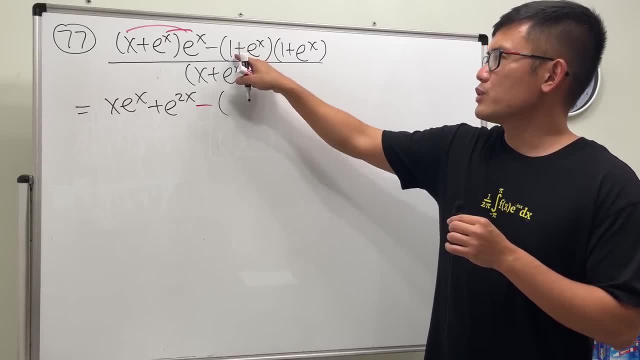 done for that part, and then we are going done for that part, and then we are going to to to subtract. now this is just 1 plus subtract. now this is just 1 plus subtract. now this is just 1 plus e to the x square right, so we can just. 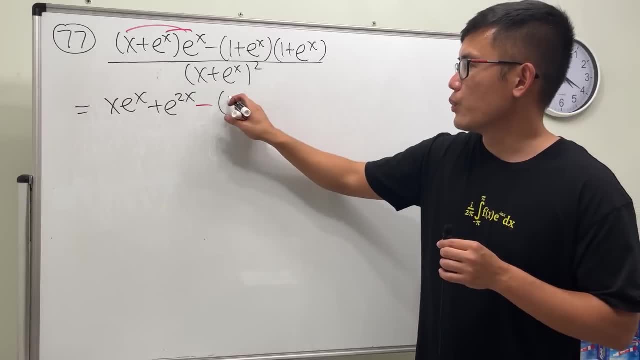 e to the x square right, so we can just e to the x square right, so we can just go ahead and go ahead, and go ahead. and binomial expansion, that, so just one. binomial expansion, that, so just one. binomial expansion, that, so just one, and then plus. 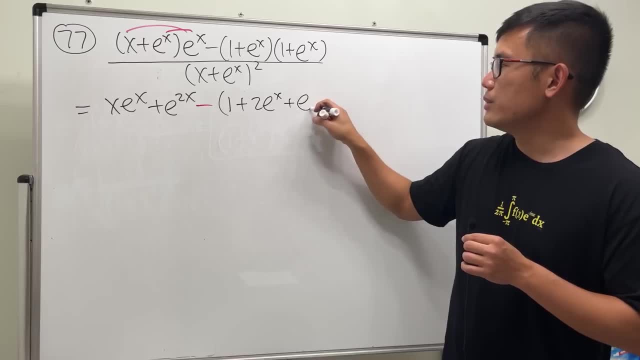 and then plus, and then plus two e to the x, and then plus e to the two e to the x, and then plus e to the two e to the x, and then plus e to the 2x, 2x, 2x, okay, and that's about all. 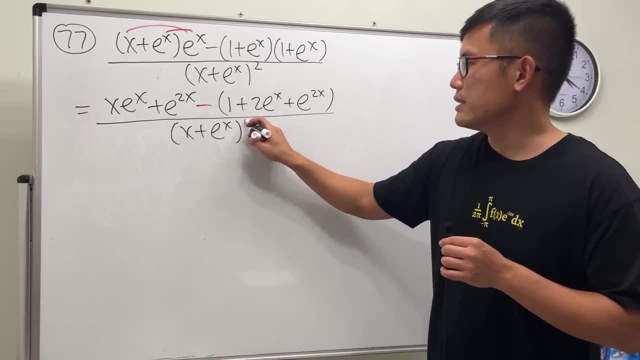 okay, and that's about all. okay, and that's about all. now, over now, over now over: x plus e to the x, and then square, x plus e to the x, and then square x plus e to the x and then square. and notice that right here we can just 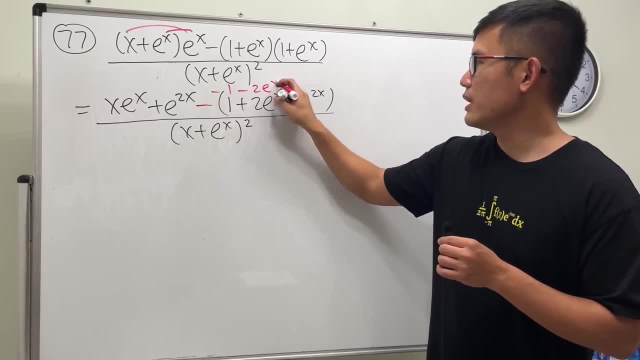 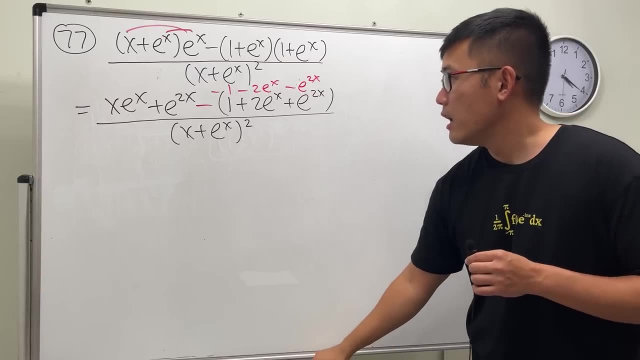 and notice that right here we can just and notice that, right here we can just. okay, so this is minus one minus two e. okay, so this is minus one minus two e. okay, so this is minus one minus two e to the x and then minus e to the 2x. 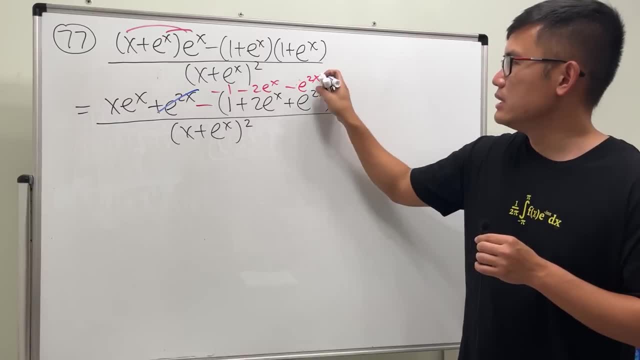 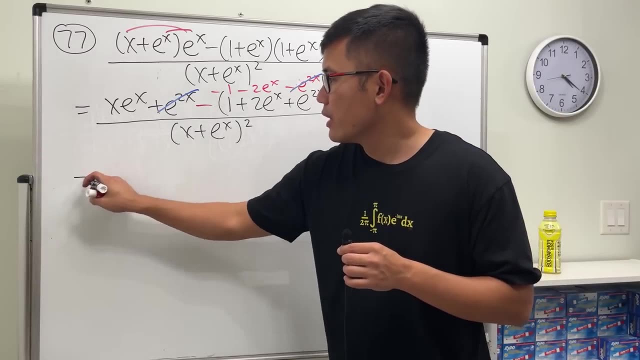 we can cancel out e to the 2x with that. that's the most we can do. so that's the most we can do. so that's the most we can do. so here we have x e to the x minus. here we have x? e to the x minus. 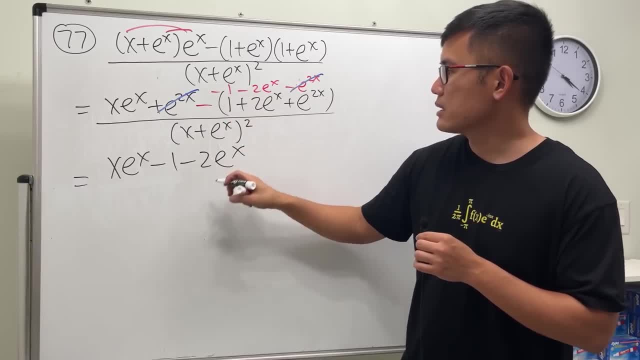 here we have x e to the x, minus one minus one minus one minus two e to the x. two e to the x, two e to the x. everybody over everybody, over everybody over x plus e to the x. x plus e to the x plus e to the x. 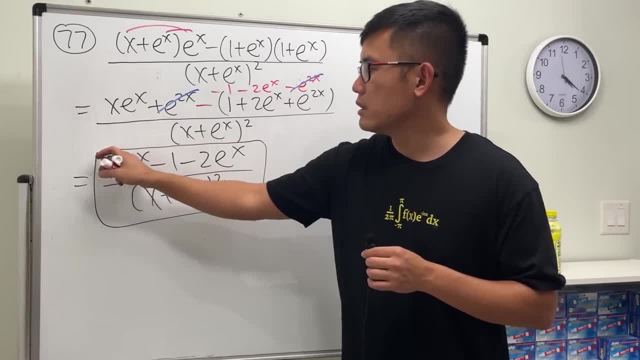 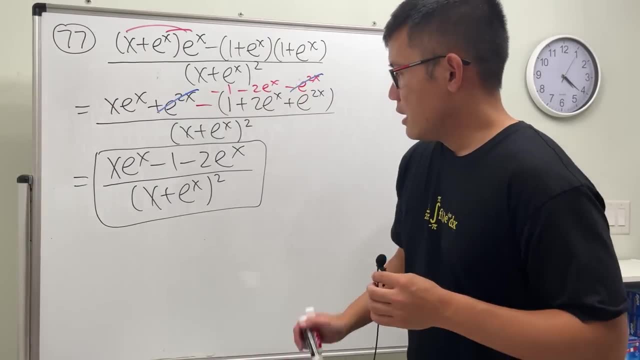 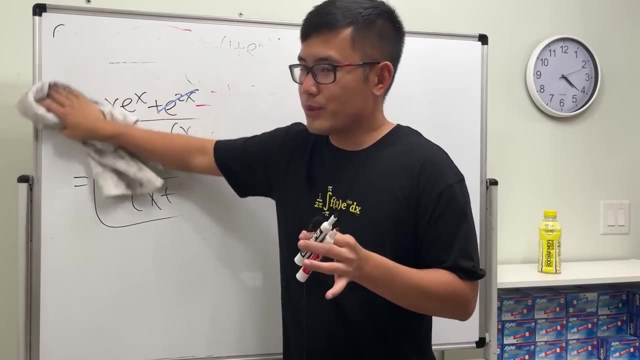 x plus e to the x plus e to the x, and then square, just like that. okay, because earlier the phone was at 10, because earlier the phone was at 10, because earlier the phone was at 10. right, i want to make sure that. right, i want to make sure that. 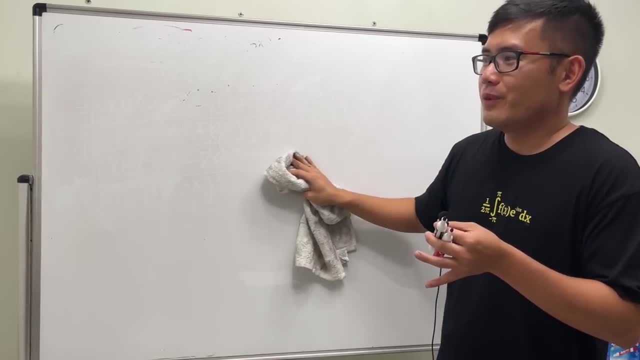 right, i want to make sure that the charge actually works and of course i the charge actually works and of course i the charge actually works and of course i wouldn't want to stop the video, wouldn't want to stop the video, wouldn't want to stop the video. so 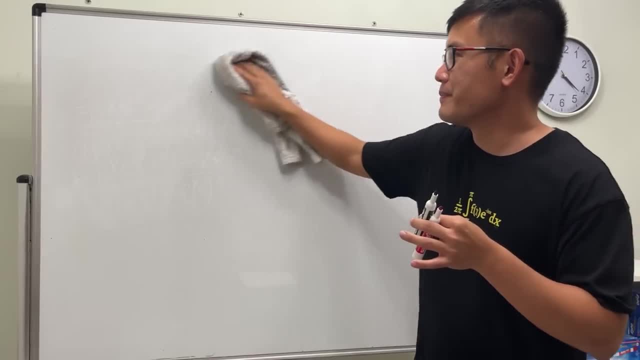 so so and then you know if i have a microphone, and then you know if i have a microphone and then you know if i have a microphone attached to the attached to the iPhone. I had to buy a different connector, So the connector I don't think the best. 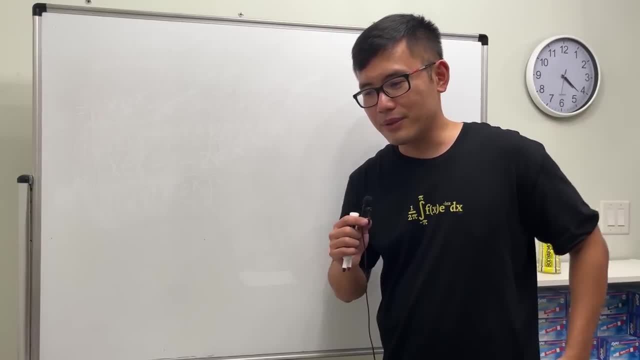 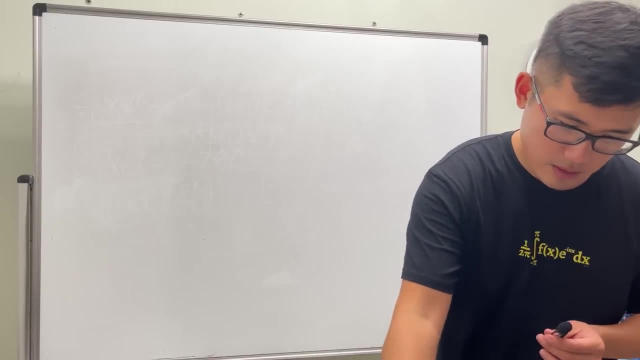 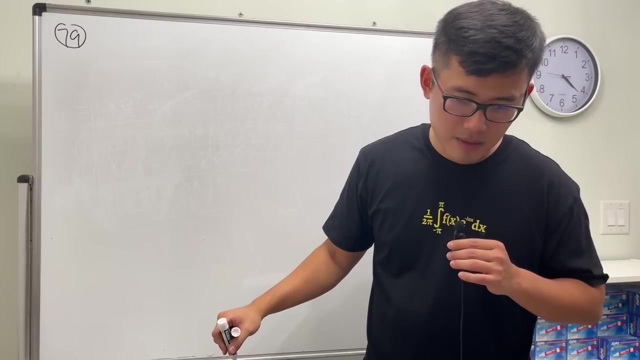 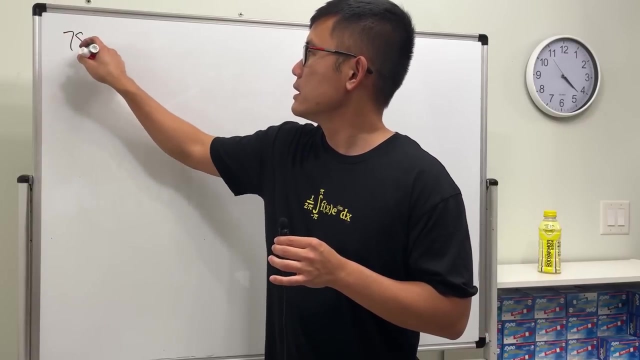 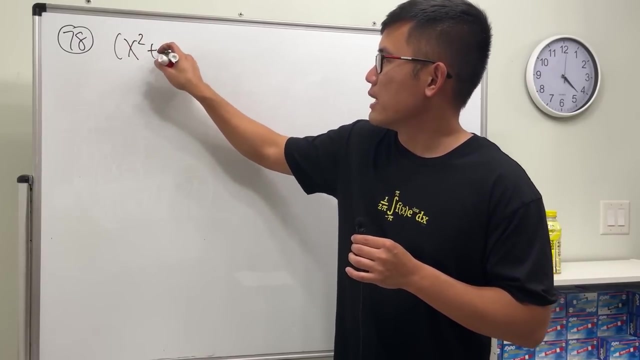 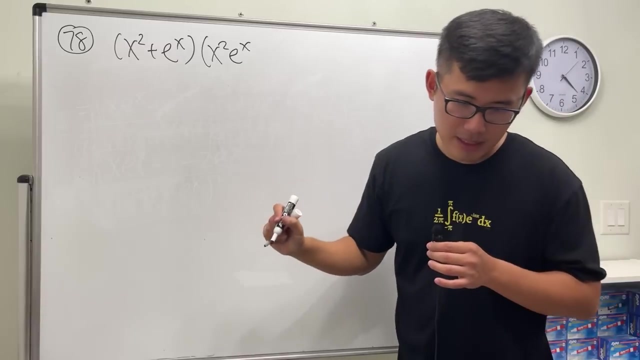 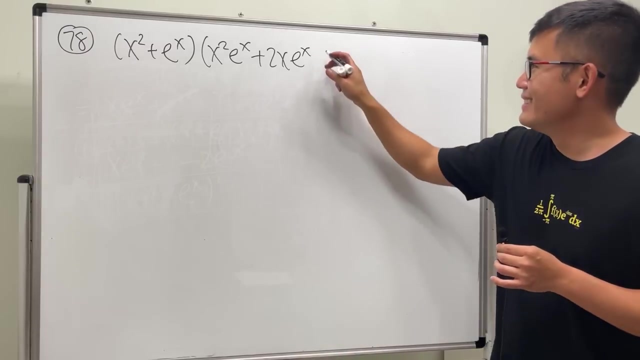 Yeah, a connector with the charger and also the microphone. Yeah, No, I didn't do 78, Oh Ready. X square plus e to the X times. X square e to the X plus 2x e to the X Minus. x square e to the X times. 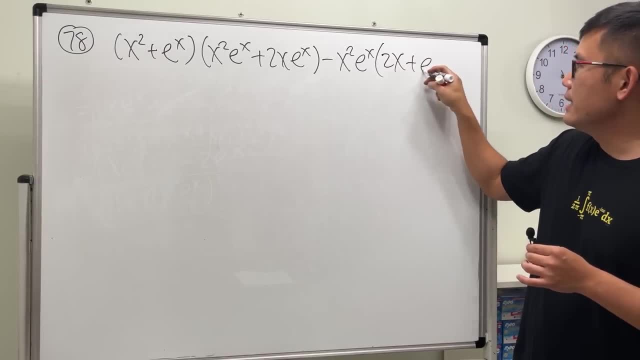 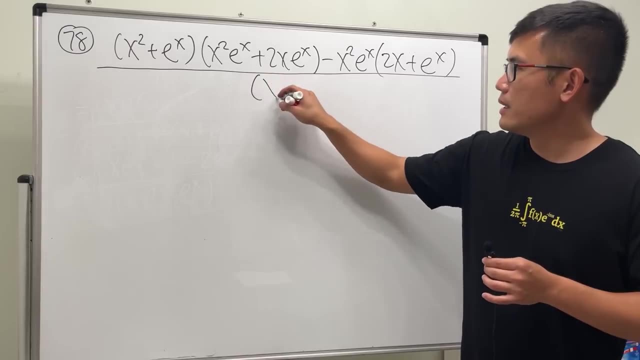 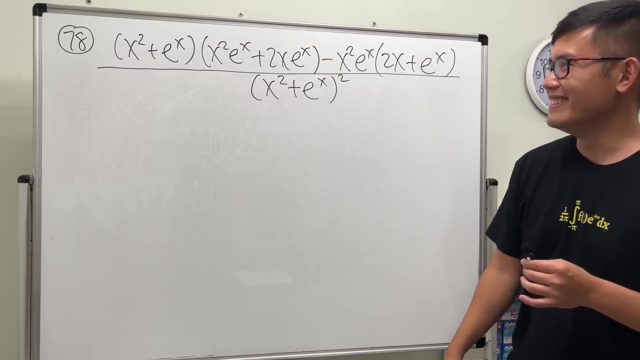 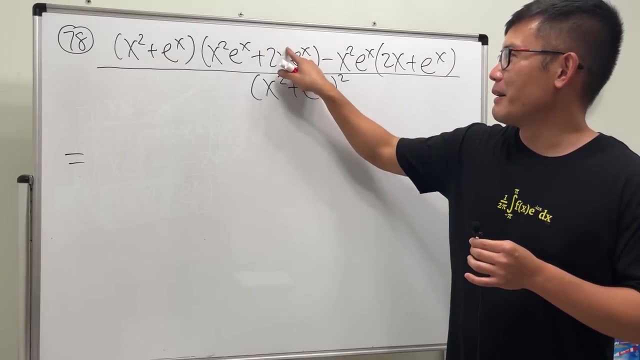 2x e to the X, no 2x plus e to the X, all over X square Plus e to the X and square. Wow, When I was typing out these questions they didn't look that long, but once I have to write them down on the board. 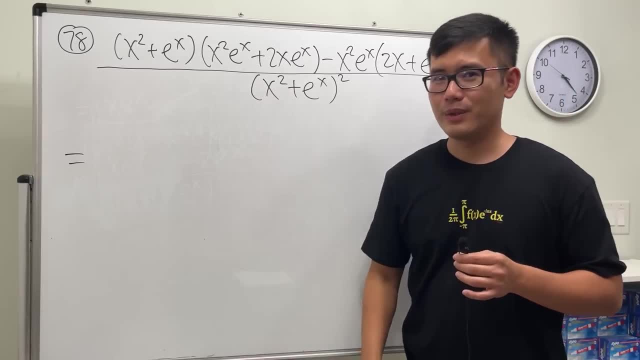 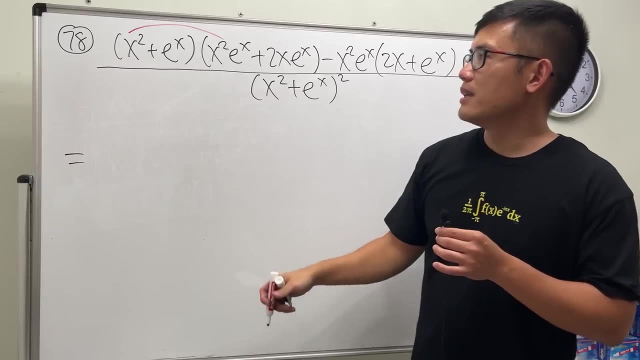 Oh, my goodness, That's okay, we can do it. Here we go. This is the binomial times, a binomial right. So let's go ahead, multiply and technically I should not say binomial, binomial loosely speaking. Well, technically speaking is a. 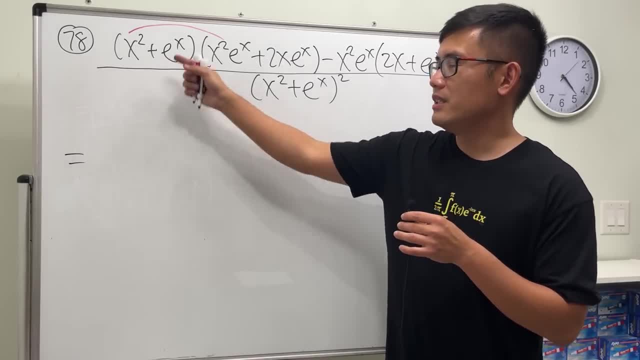 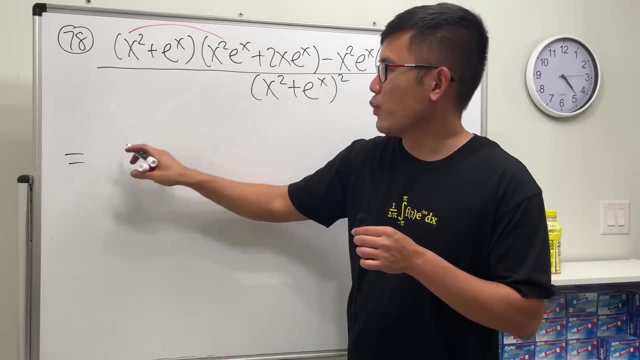 Polynomial has two terms. but this is not polynomial when we have e to the X. So anyway, I'll just say two terms times two terms, So we'll just forward. All right. So take this times that we get X to the fourth power, e to the X. 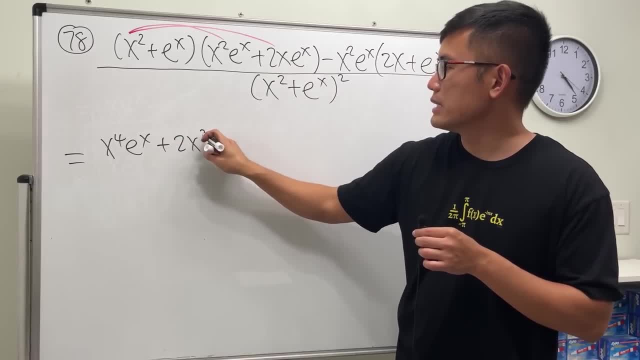 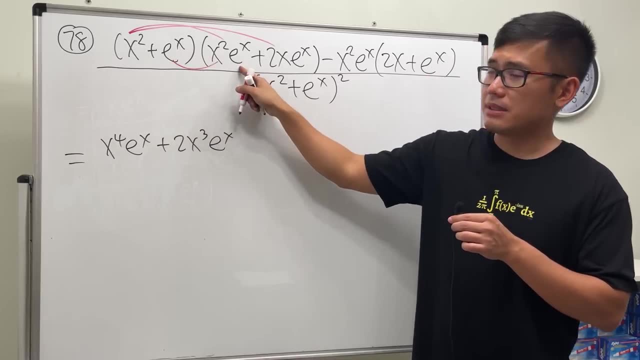 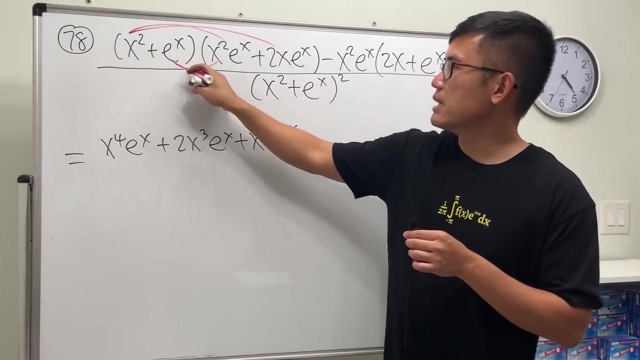 Next to this: times that we get plus 2x to the third power And then e to the X, Yeah, and then take this times that, e to the X, times that you add the powers and then the x squared, just leave it So: e to the 2x here. and lastly, this times that, so we have plus 2x, e to the 2x. 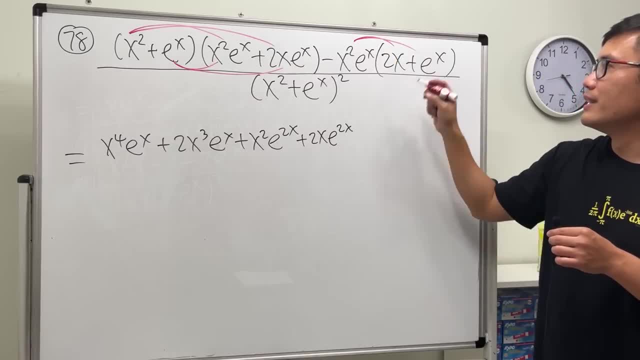 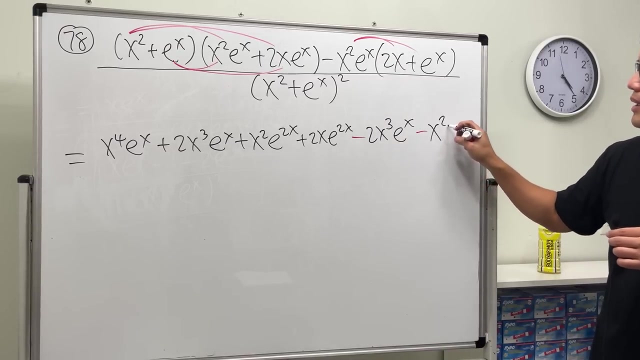 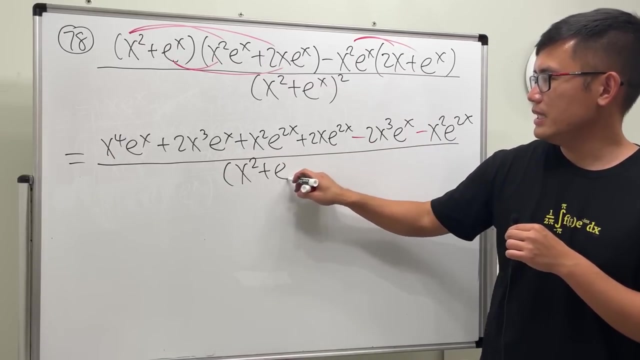 Okay, and then we'll take this distribute hood so we get minus 2 E, the 2x to the third power and an e to the X and then Minus X, where e to the 2x all over, X square, plus e to the X and then square. 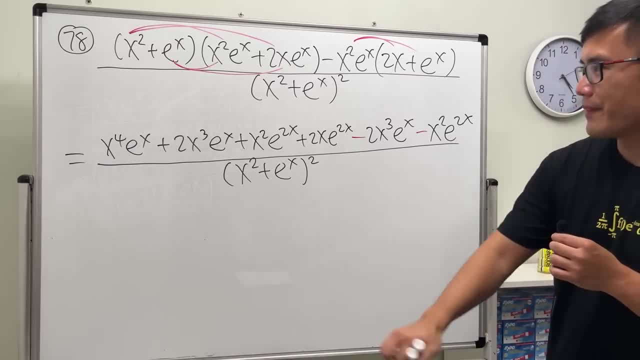 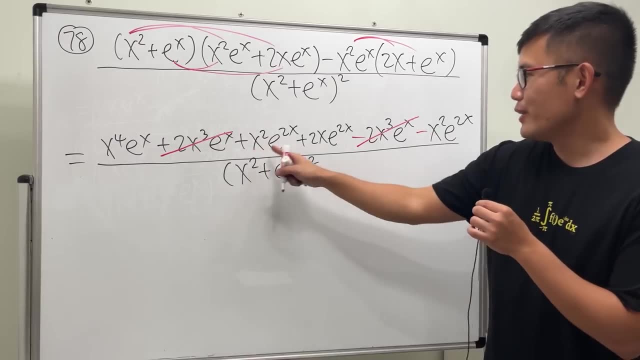 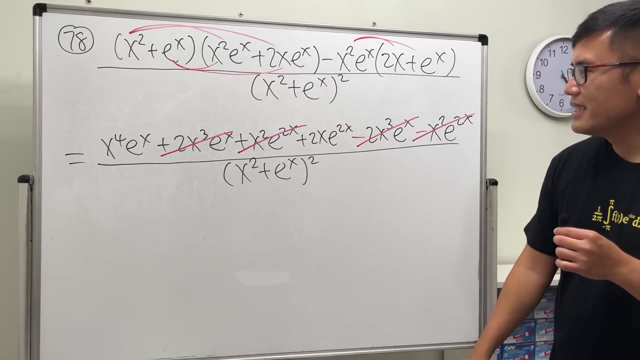 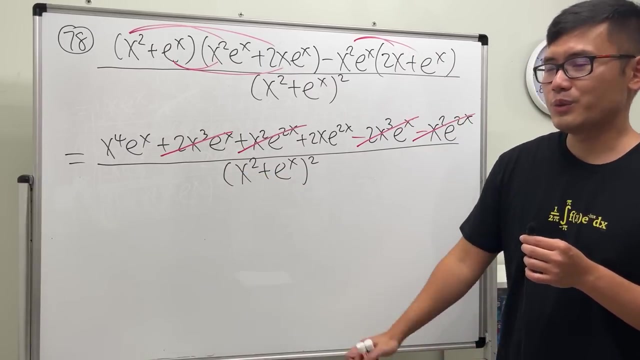 Okay, let's see now: 2 X to the third power, e to the X. this and that cancel X square e to the 2x: they also cancel. Yeah, that's about all, and we have this and that. can we factor stuff up? Yeah, but it does not really do us any good, so we can just leave it. 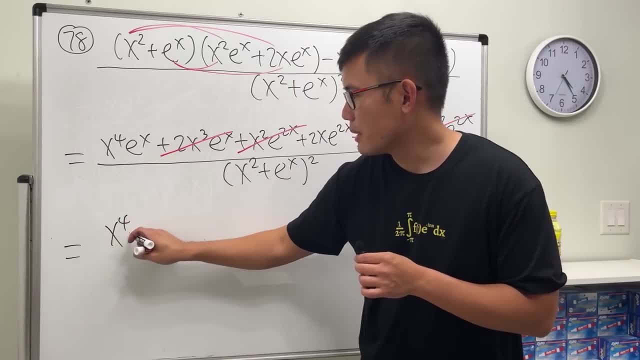 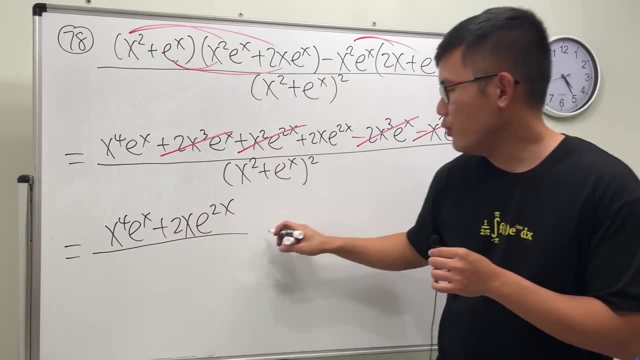 So the final result? we can write it as X to the fourth power, e to the X, and then plus 2 X, e to the 2x- Everybody over this guy- which is X square, plus e to the X, and then square, And here's the final result. 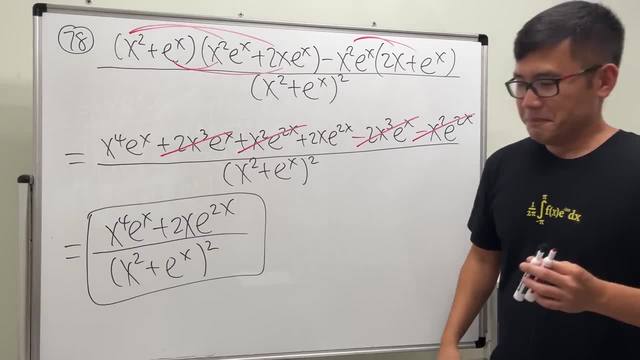 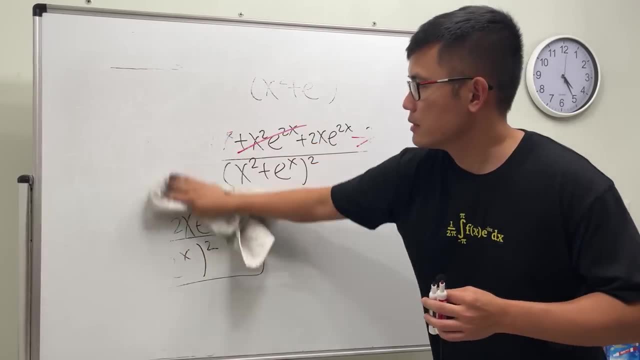 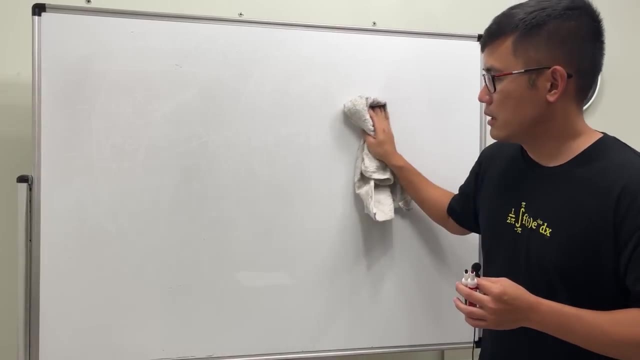 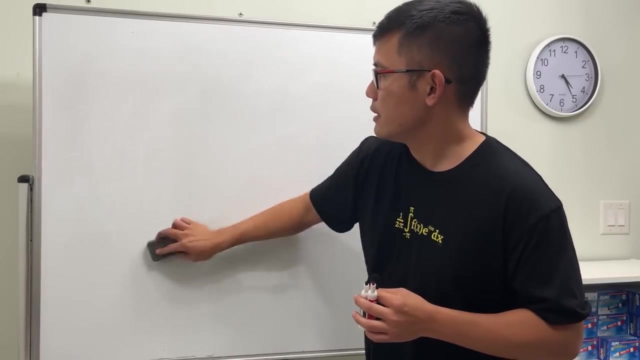 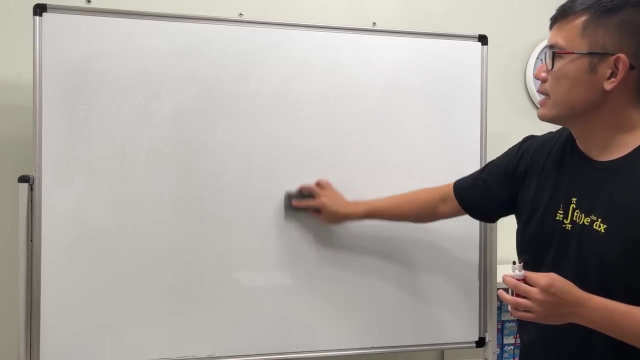 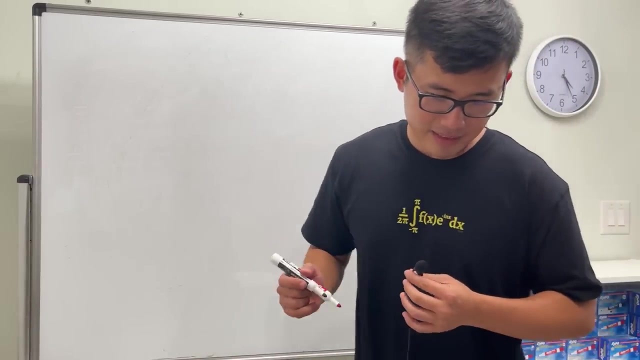 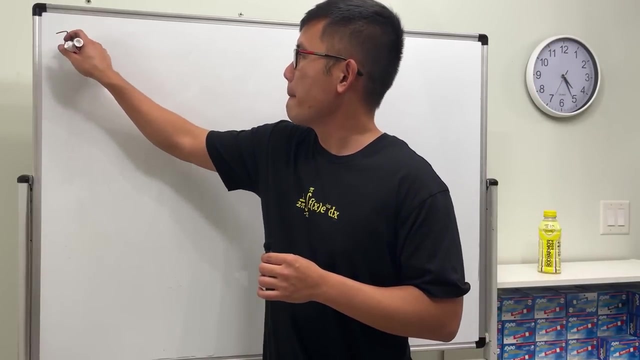 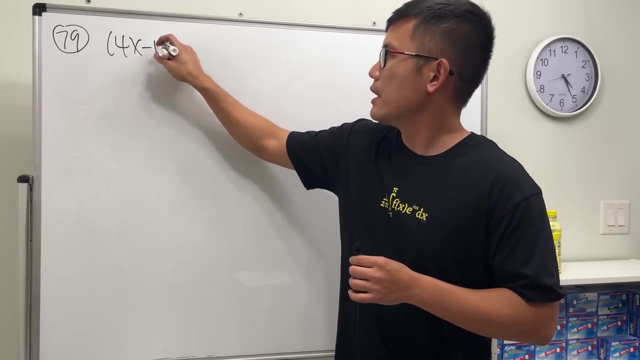 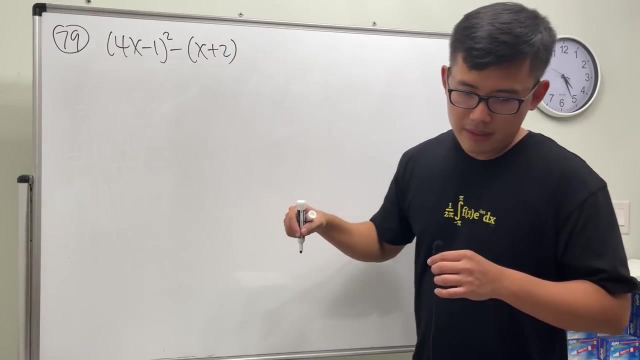 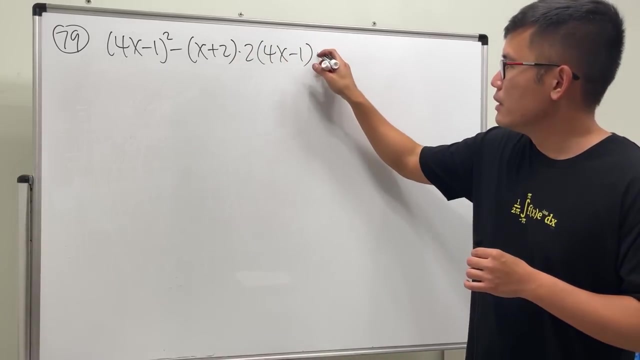 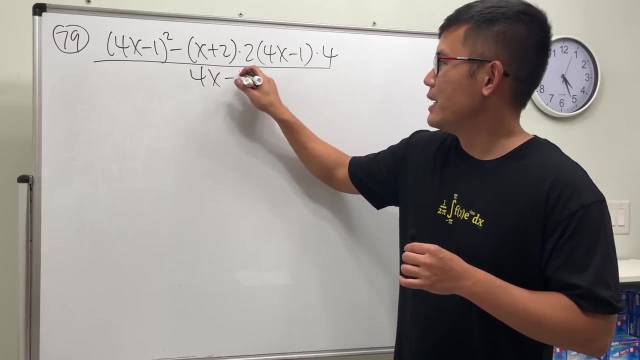 Now you make a decision. Three, Oh Alright, number 79: 4x minus 1, square minus x plus 2, times 2, 4x minus 1 and then times 4. all over 4x minus 1 to the 4th power. 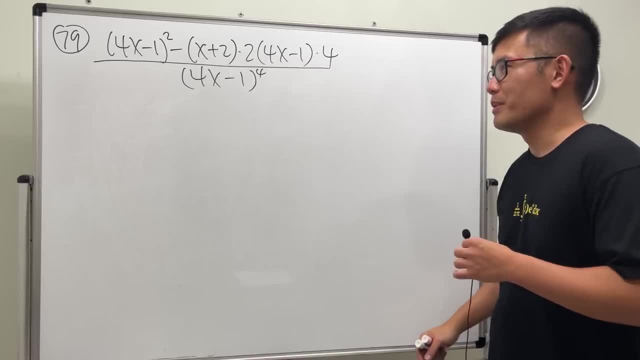 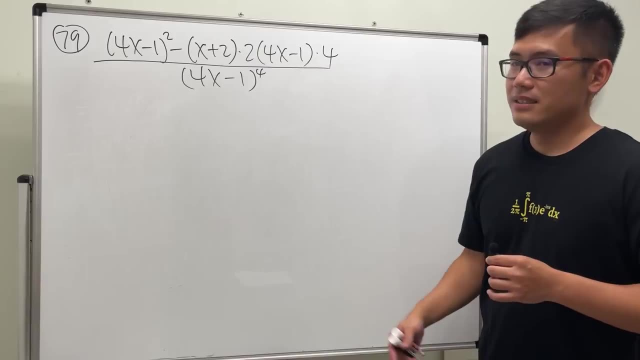 Technically it should be square square Comment down below, if you know what I mean by that. But anyway, though, if you can tell me where did this question come from, that would be pretty cool too. But anyway, now to simplify it. 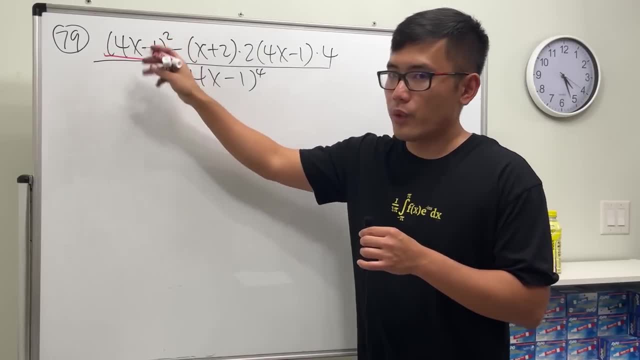 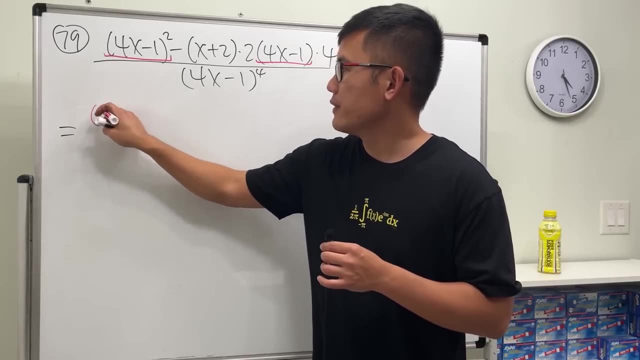 notice how here we have 4x minus 1 square and here we have 4x minus 1.. So take advantage of that. Let's factor it out first. So here we have 4x minus 1.. Okay, and this one. 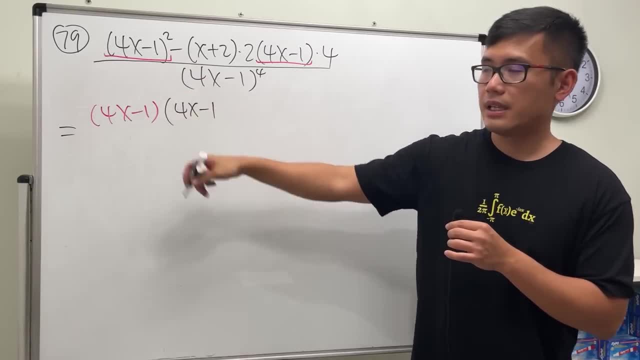 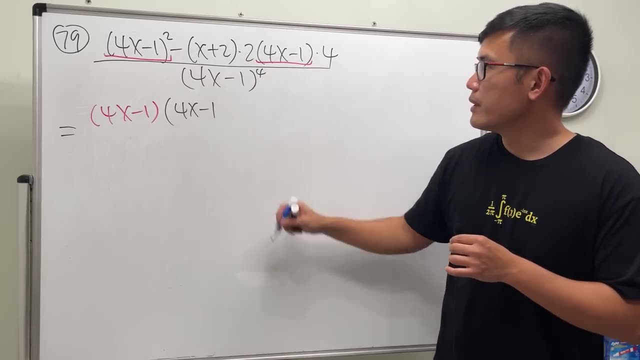 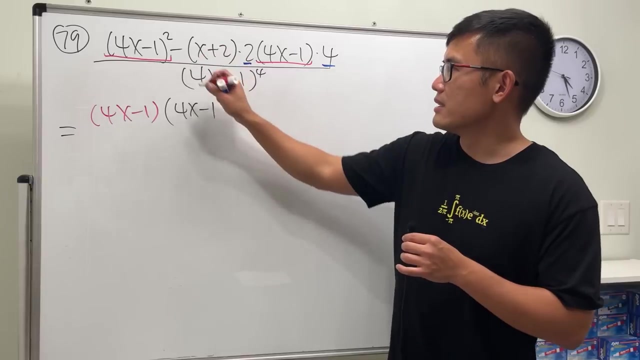 here will be 4x minus 1 left, And then what do we have left then? This is 8.. So I'm going to actually use blue. This is 8.. Okay, So perhaps I will just leave it like this. 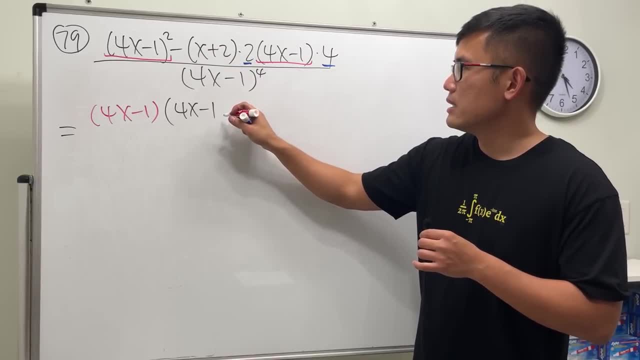 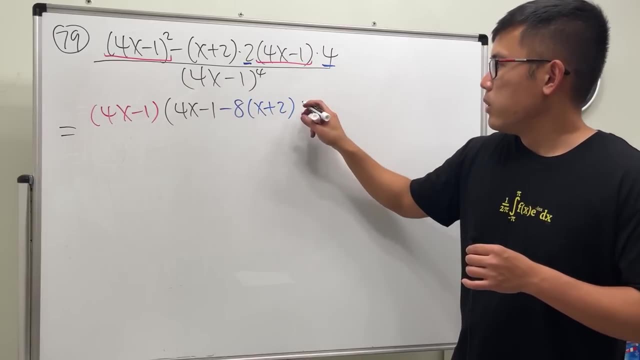 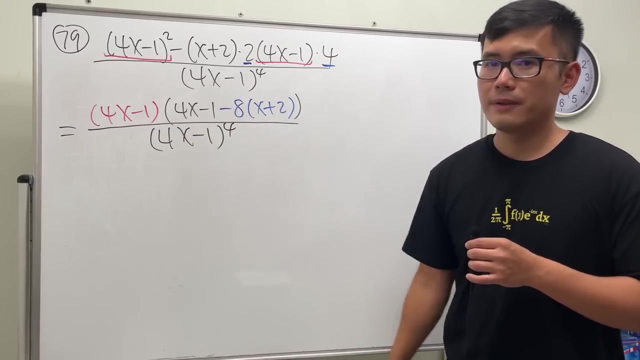 So we have the minus. Let's keep it like this: Minus 8 and then x plus 2.. Yeah, Okay, Over. this is 4x minus 1 to the 4th power, Then we can cancel, right. 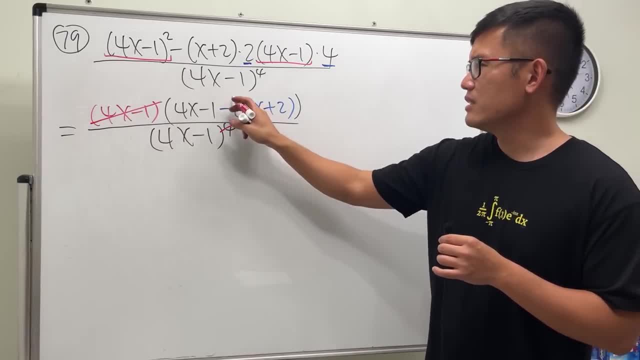 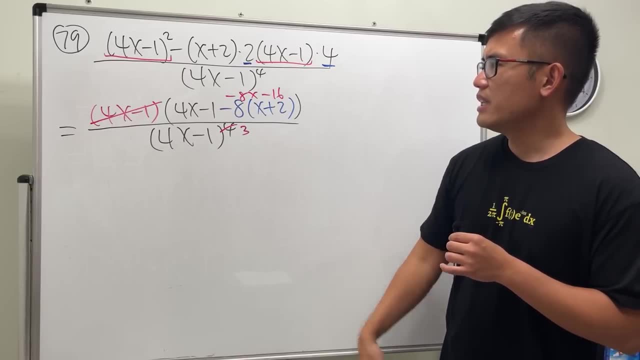 one of them out. That's good, And now we can just fix the inside. So this is negative 8x minus 16.. Yeah, and just combine it, That's all. So finally, 4x minus 8x is negative 4x. 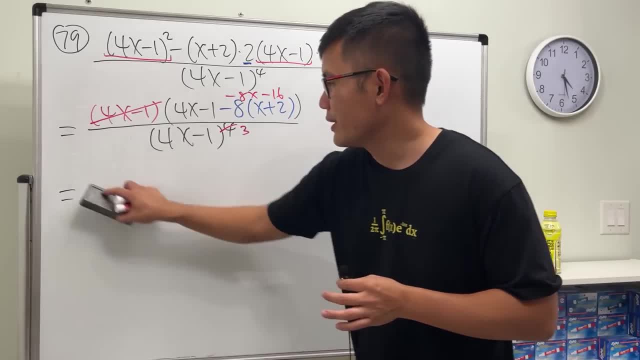 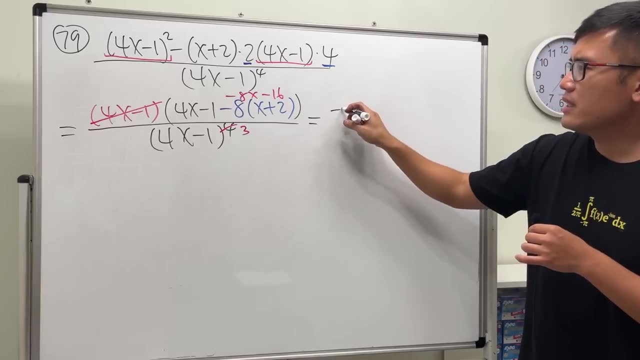 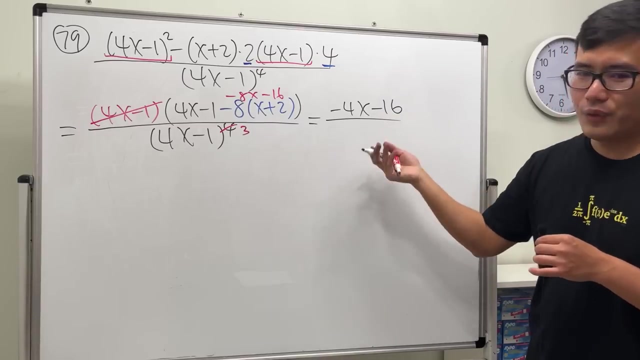 Can I? I think I'm just going to write down the answer right here so I can use the button to do the next one. So this right here equals this, and that is negative 4x and then minus 16.. Okay, Can you find out the negative 4?? Yeah, 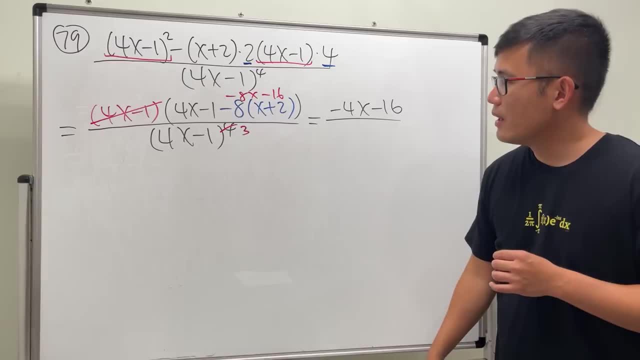 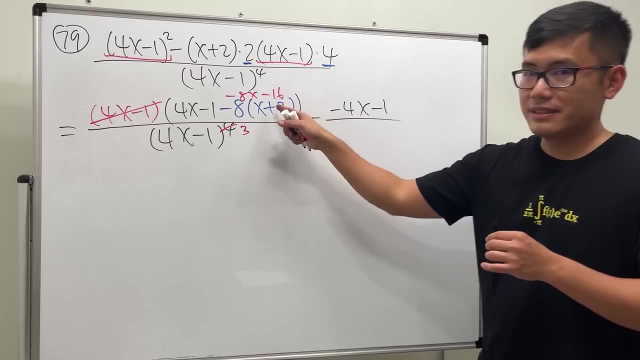 But it doesn't really matter. No, it's not. No, no, no, no, no, no. Negative 1 minus 16.. So it's minus 17.. And then not for the answer: 4x minus 1 to the 3rd power. 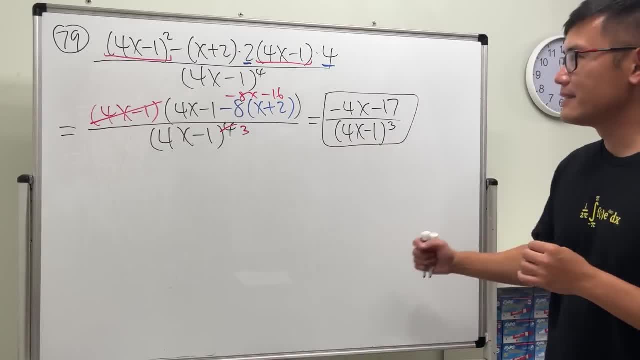 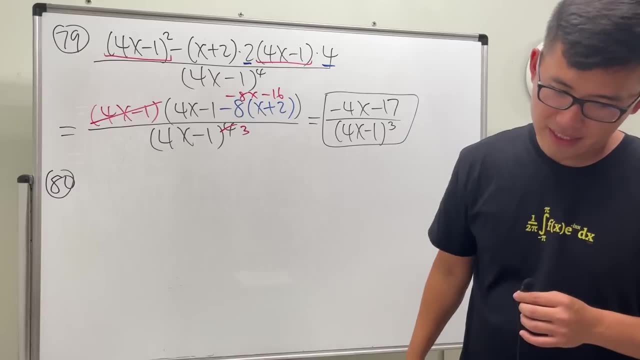 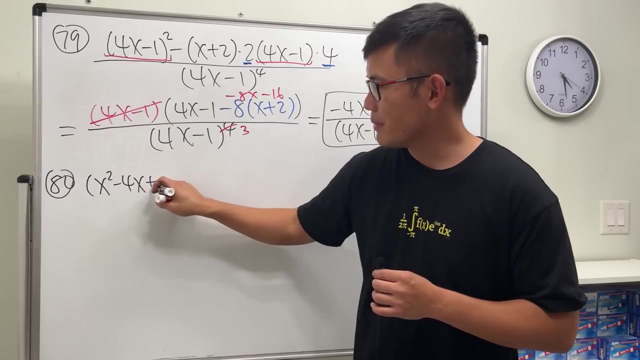 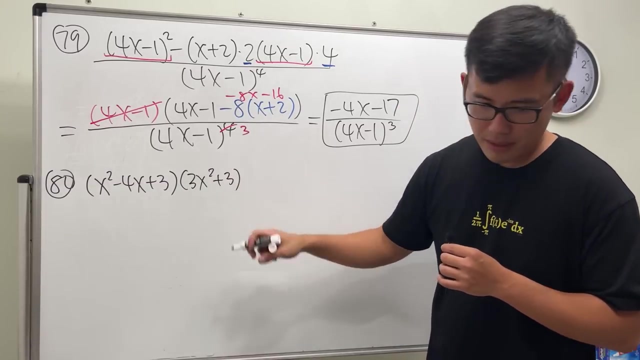 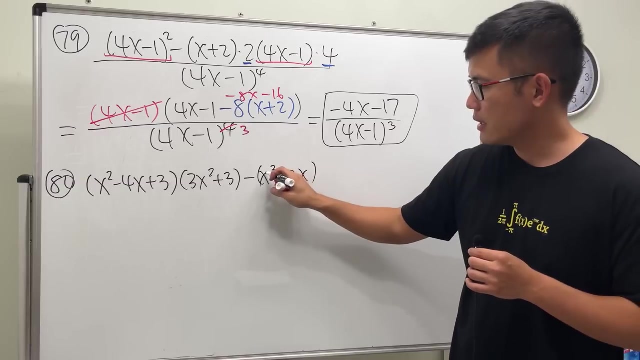 Done, Yeah, 80.. You'll see this one, Okay, ready, Ready, Okay. x squared minus 4x plus 3 times 3x squared plus 3 minus x to the 3rd power plus 3x times. 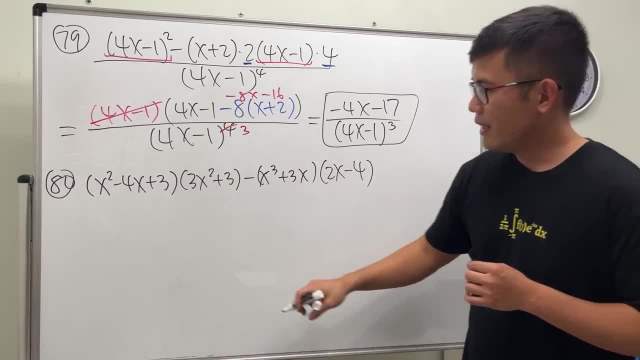 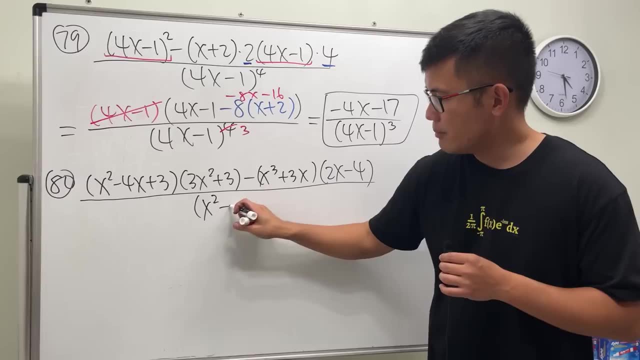 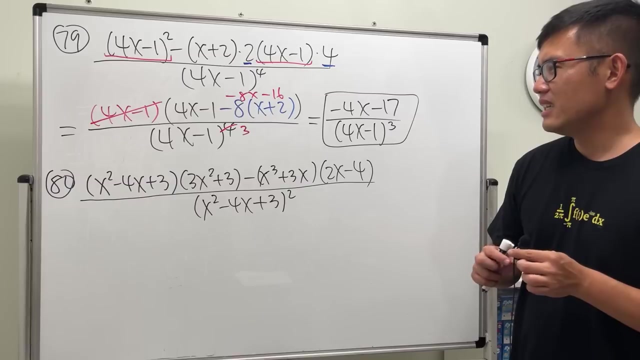 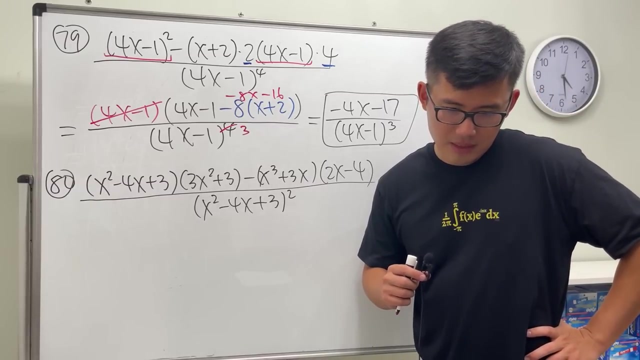 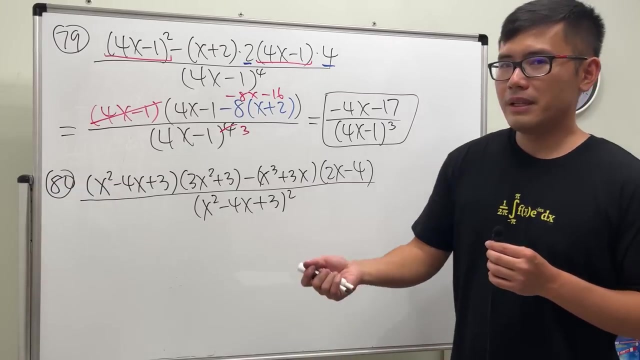 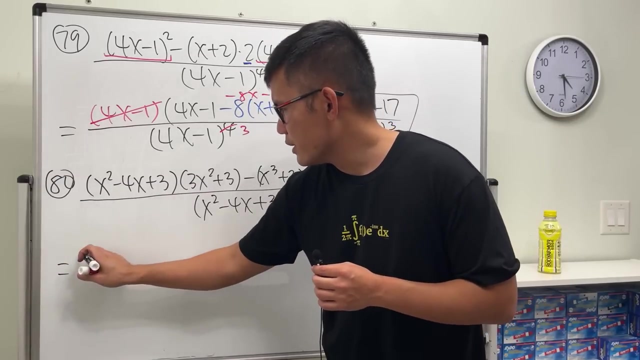 2x minus 4.. Everybody over x plus 3x square minus 4x plus 3 square. oh my god, can we factor anything though? yeah, we cannot factor anything, so we just have to deal with it, multiply the out and combine terms and then hope for the best. yeah, so here we go, this times that we get 3x to the. 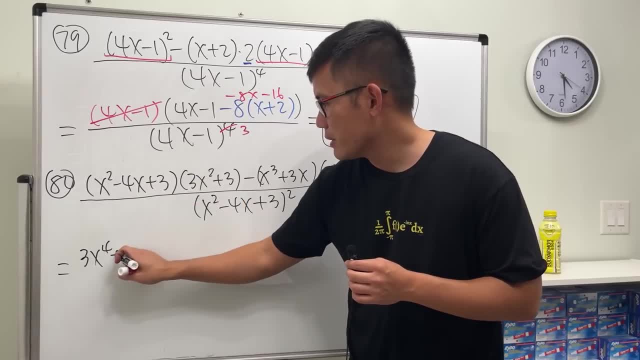 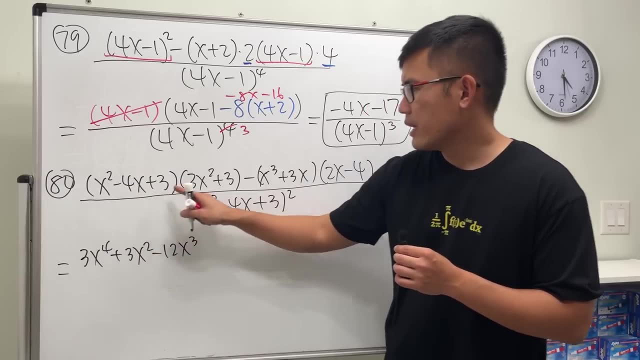 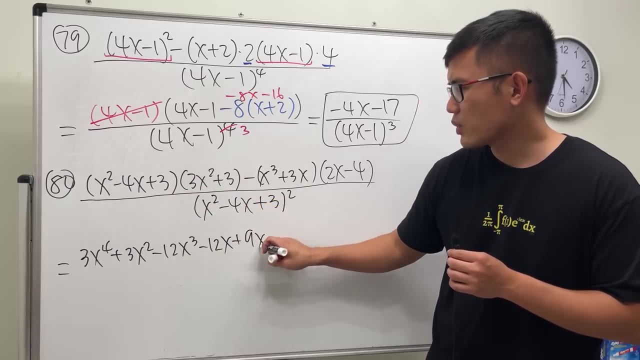 fourth power: this times that we get plus 3x square. next move to this times that which is negative 12x to the third power, and then this times that is negative 12x, and then this times that is plus 9x square, and then this times that is plus 9. okay, 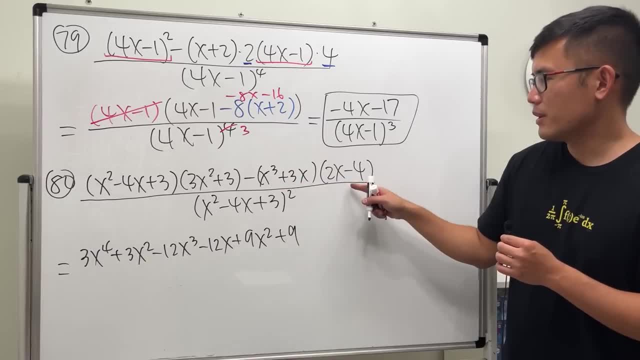 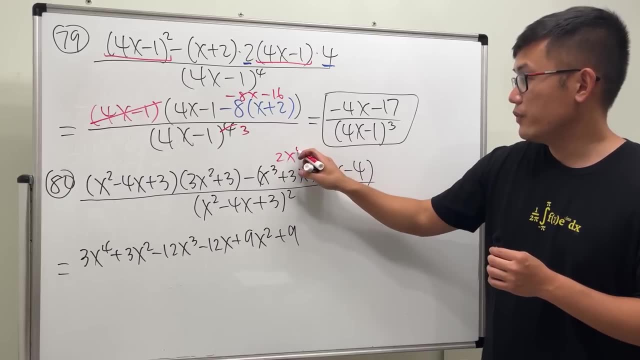 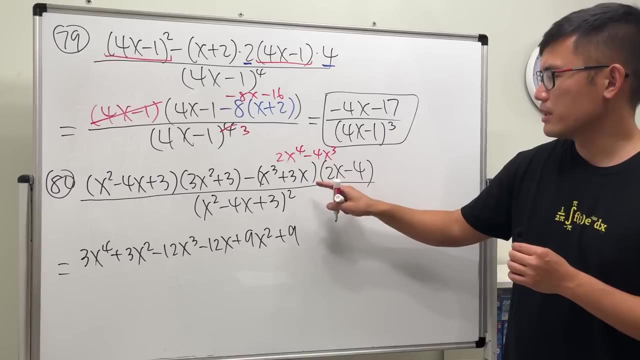 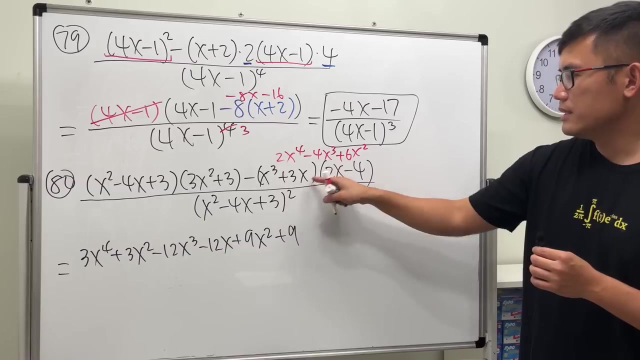 and for this one I'm just going to multiply out right here first and then distribute negative. so if you look at this times that is 2x to the fourth power and then this times that is negative 4x to the third power and then this times that is plus 6x square, this times that is minus 12x, and then I'm. 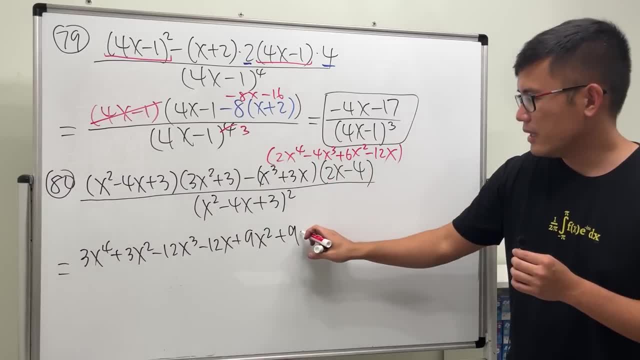 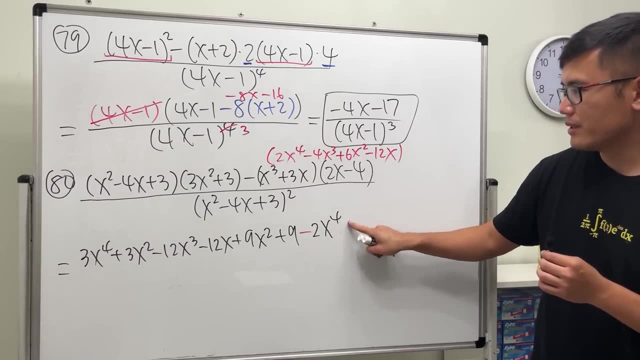 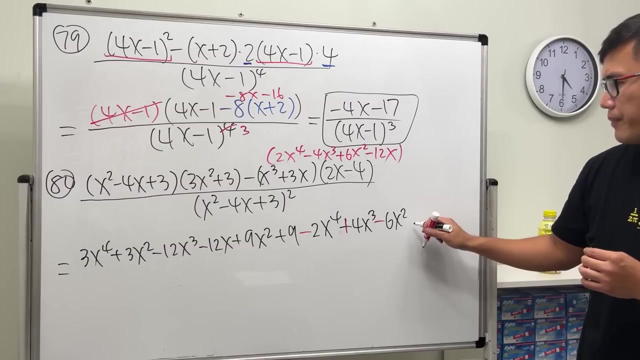 going to distribute a negative, so I will get negative 2x to the fourth power plus- oh, I like to do this. let me show you negative times negative anyway. and then 4x to the third power and then becomes negative 6x square, and then negative times negative, and then we have the 12x square, 12x. wow, all over. 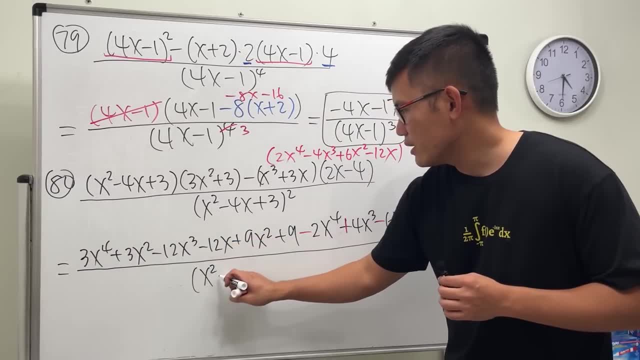 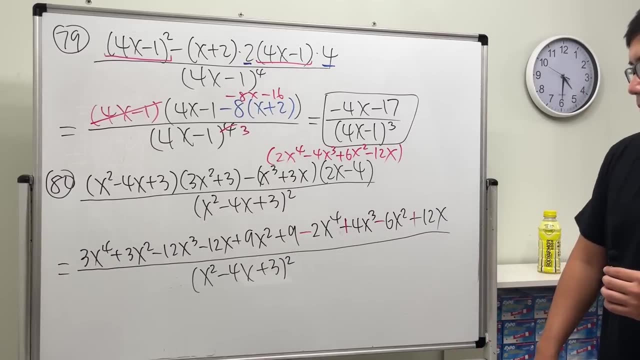 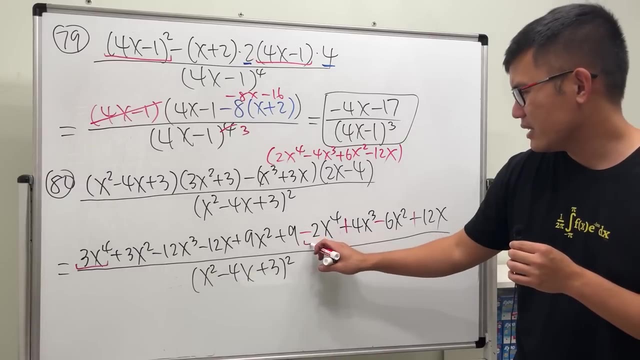 this guy x square minus 4x plus 3 and then square: all right, let's see what we can do with it. so let's look at all the x to the fourth power term. we have 3x to the fourth power and then minus 2x to the. 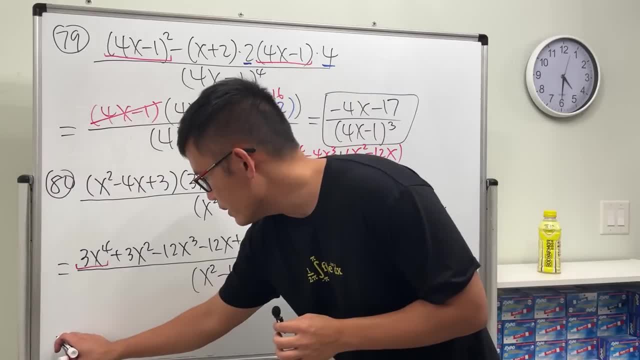 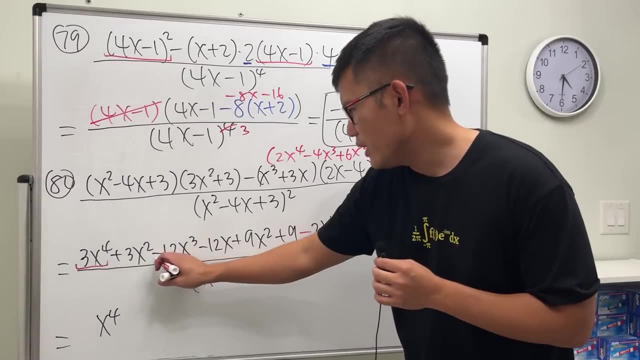 fourth power. so that's just 1x to the fourth power. so x to the fourth power, all right. next let's look for the x to the third power term. here we have minus 12x to the third power, plus 4x to the third power, so that's minus 8. 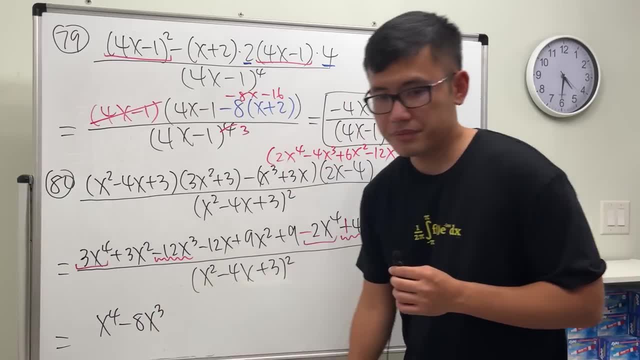 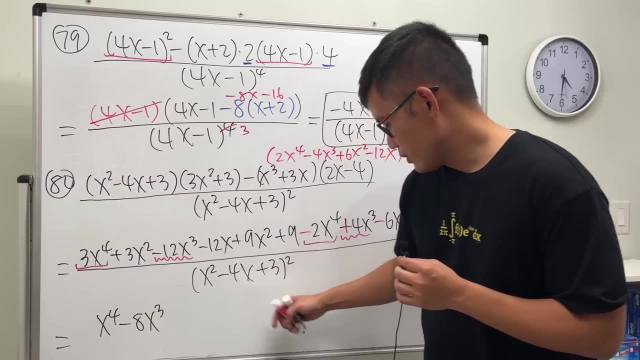 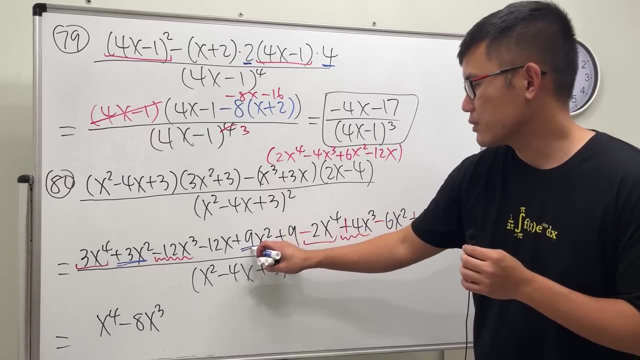 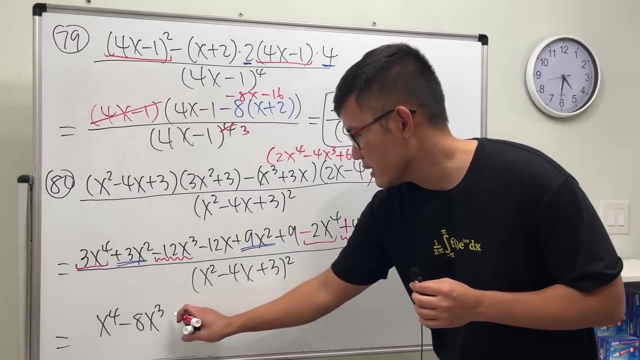 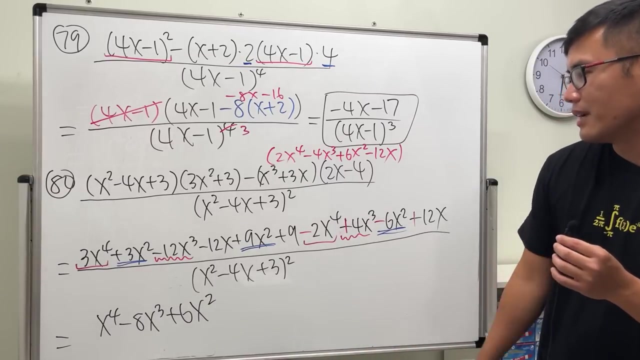 minus 8 x to the third power, all right. and then next one x squared terms. let's see, oh it's blue. 3x to the second power plus 9 x to the second power is 12. 12 minus 6 is positive 6. so this right here, plus 6x squared, all right. and then, oh, we can have. 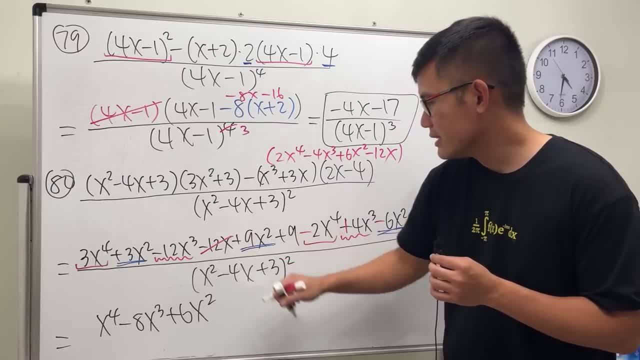 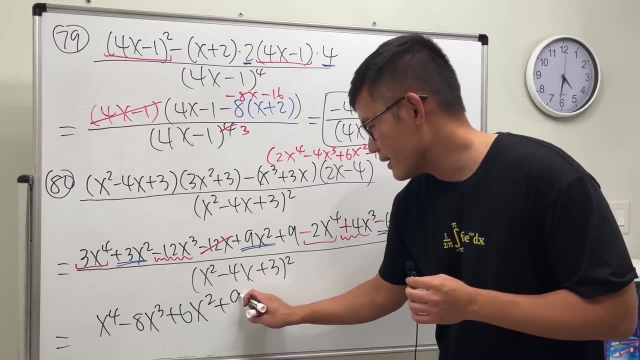 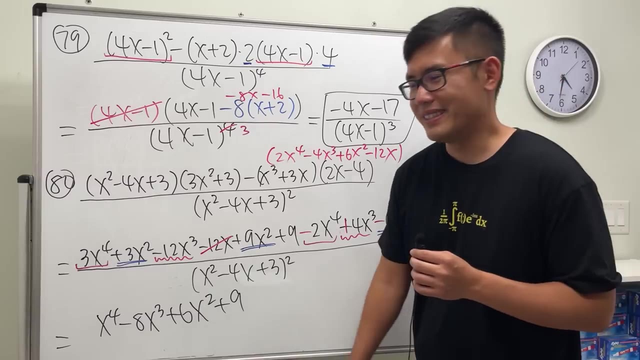 something canceled. this is negative 12x, positive 12x and this something get canceled it. and then this is plus 9, so just put a plus 9, okay. so that's pretty much a simplification for the numerator. can we possibly factor this? I have no idea, that's not even. 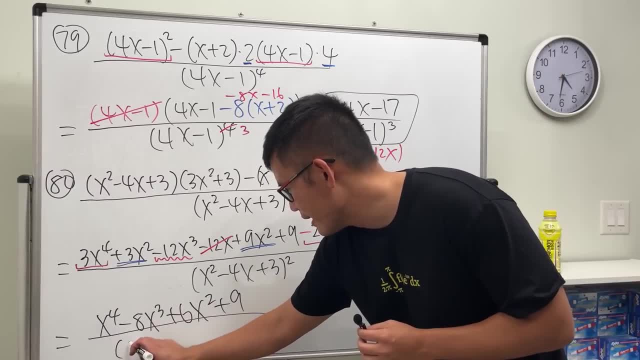 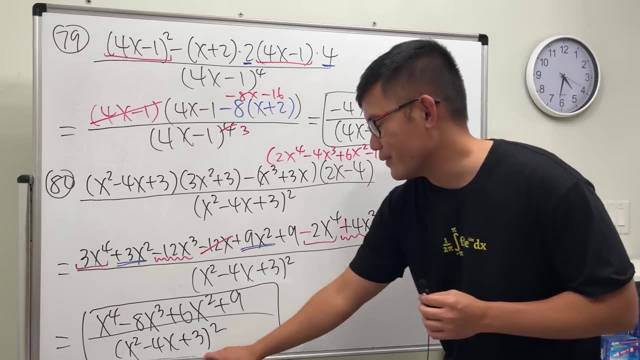 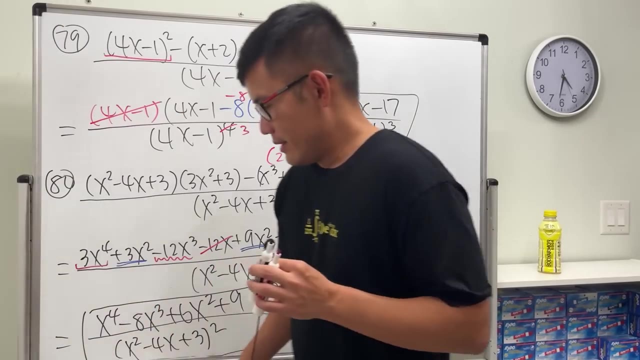 bothered with it. let's just look at this and then over x squared minus 4x plus 3 squared, and then call it for the day for that question. okay, all right, so let me just take a look. yay, I hope the audio is okay, but anyway, this is number 80. yeah. 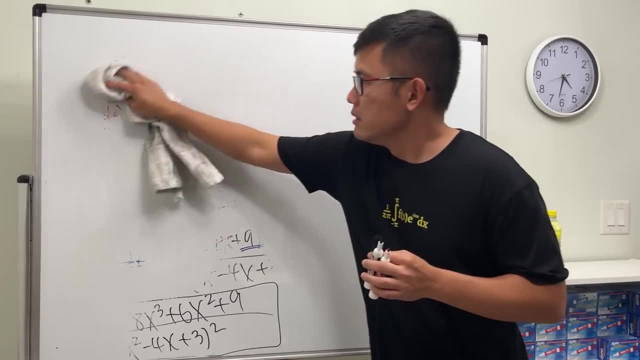 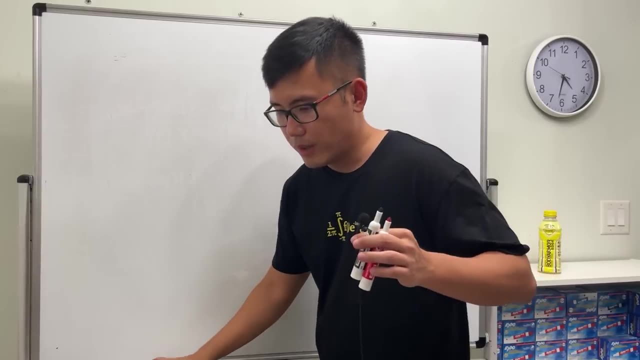 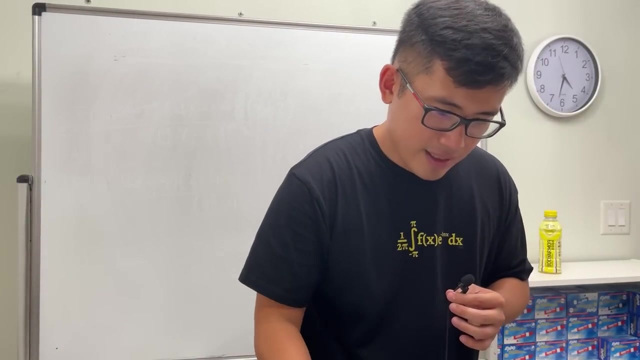 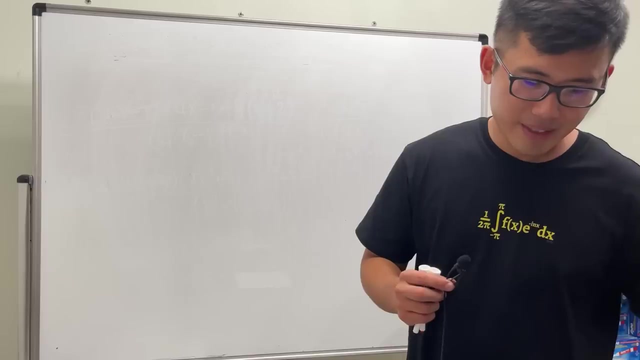 just fine, I want to Bad friends. I definitely have their agreement. let's just take a look. let's go come on wait. how nearly hours has this beam- it's 1st наконец tested- three hours of. okay, it's not so bad, I like it very late. anyway, wait, how many hours has this been? it's only 3, 1, 3, 8 hours and four. okay, it's not so bad like it's very late. anyway, S nova theseStoriesders. Okay, next we'll continue when I come up with anotherINDO. 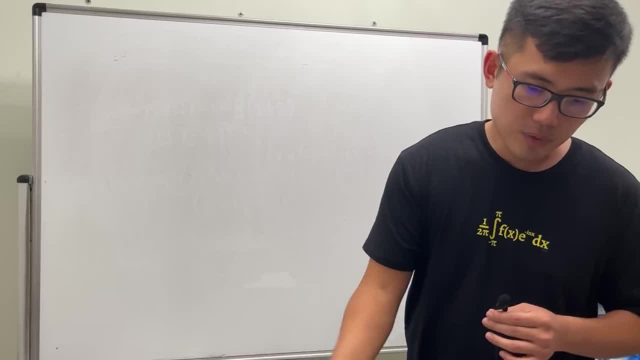 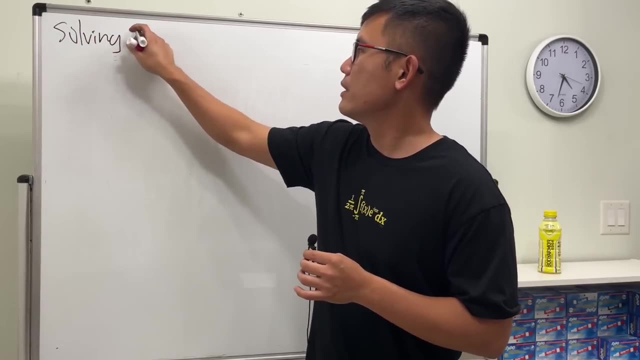 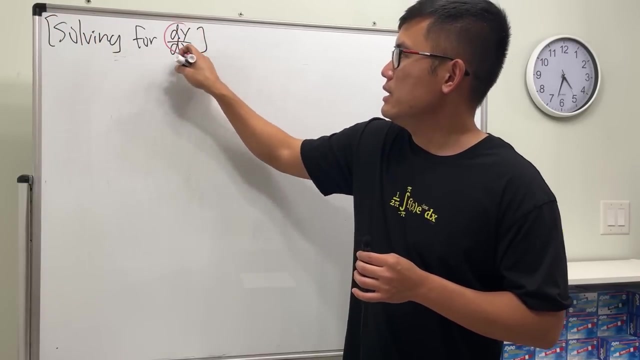 okay next, but I should also play it again, just so that we didn't miss the speed of it. solve equations: right, but this one is like solving for dy dx. it's like: let me just write down. so i want to tell you guys that this right here that we're using this is actually like a variable. 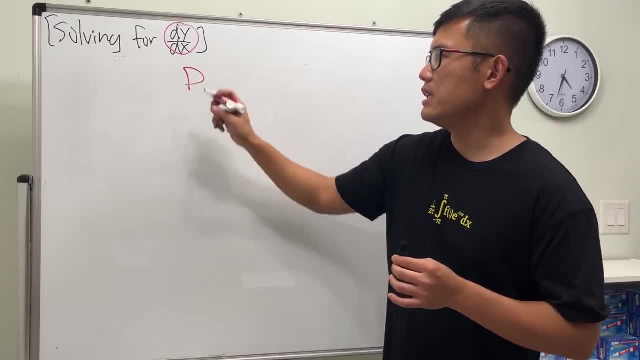 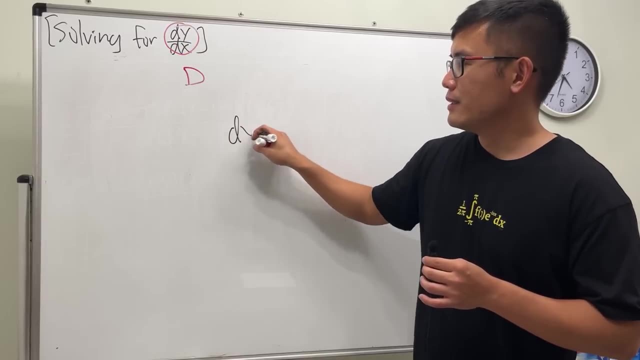 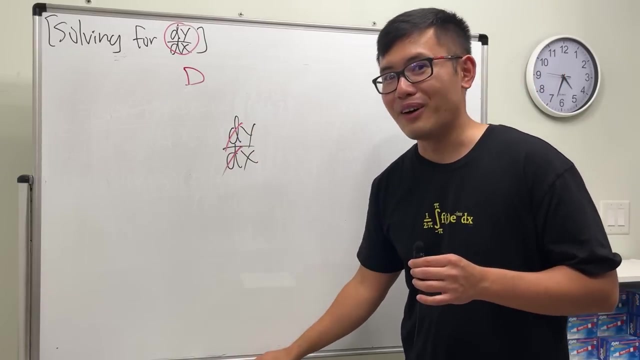 itself. okay, you can look at this as like capital d right for like derivative that kind of thing. do not cancel the d and d right, dy dx. do not cancel this out and out. don't do that the whole thing. right, there is a notation itself, okay, and the goal is to isolate that. 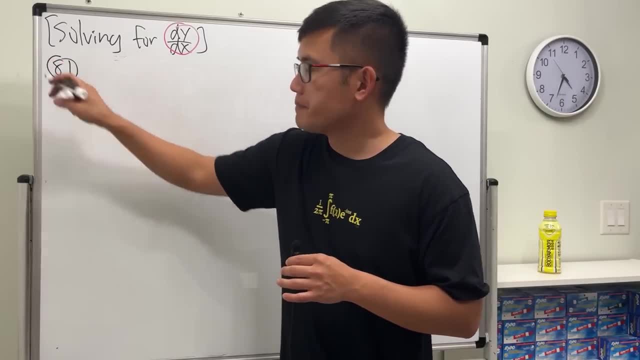 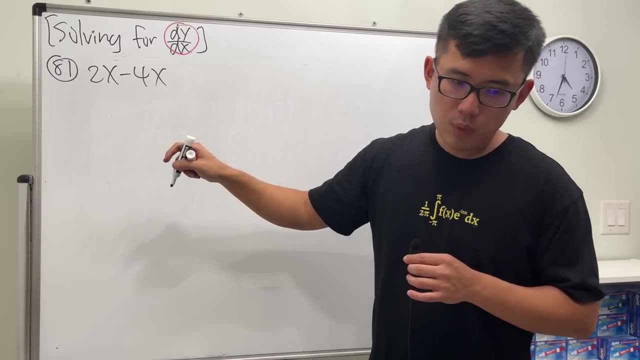 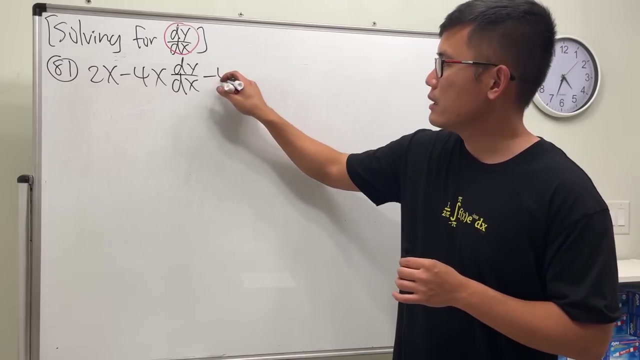 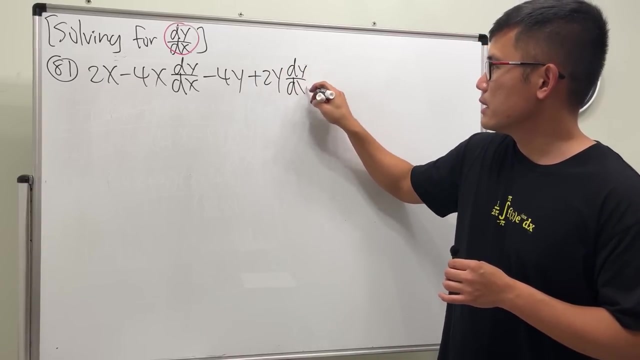 and let's see number 81. so firstly we have this root of 2x minus 4x, and then dy dx minus 4y, plus 4y plus 2y, and then dy dx equals 0. so this is the so-called implicit differentiation. 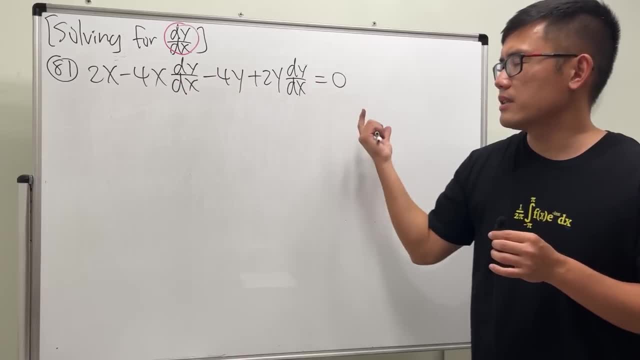 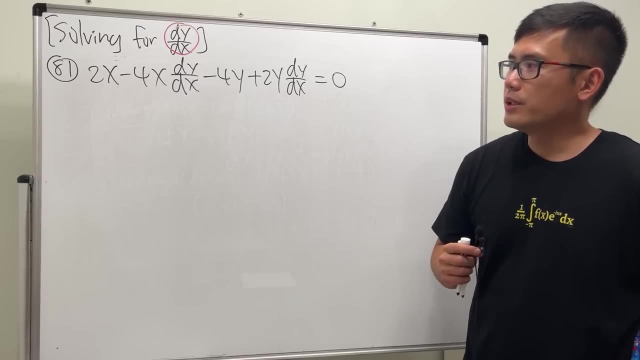 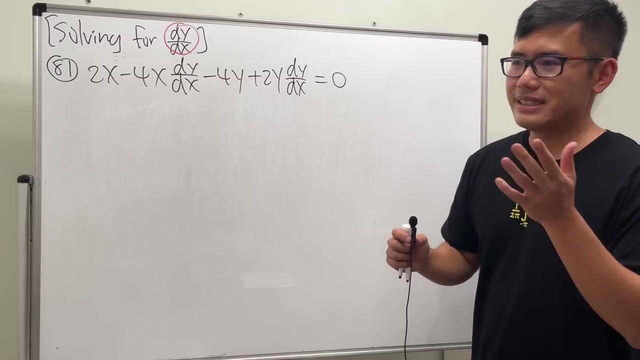 and again i am using the dy dx notation. this is the whole thing and our goal is to just isolate that for this kind of questions. you will see that the expression is like very, very scary and if you, you, you, just keep track everything, it's not so bad. let me show you guys how i like to do it. 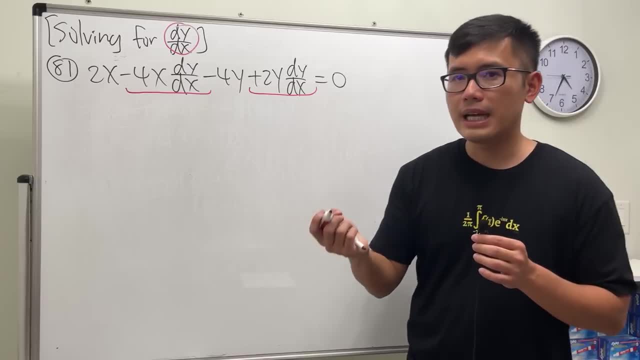 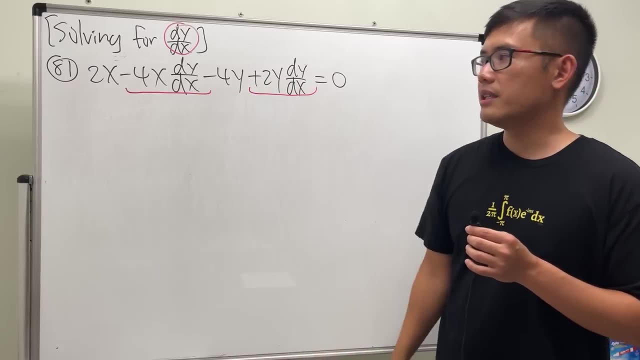 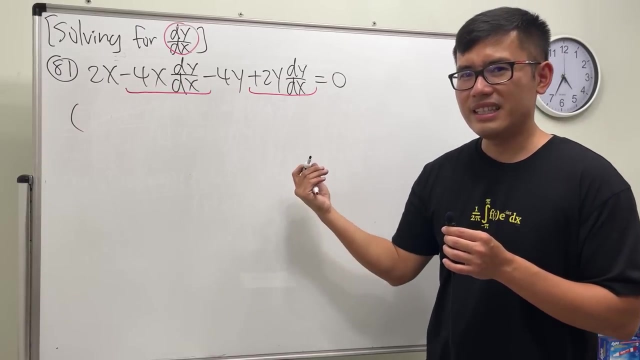 firstly, let's just look at the terms as dy dx and then keep it on one side. so i will keep them on the left hand side because they have dy dx and i'm going to factor it. i'm going to just put down parentheses and i'm going to put down the dy dx at the end of the parentheses. 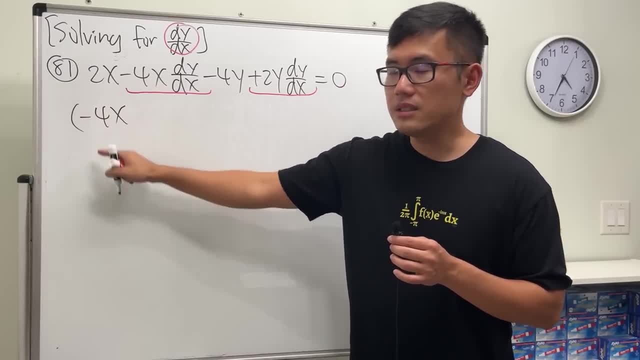 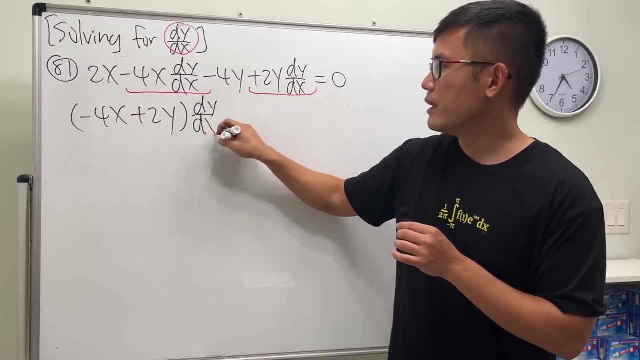 so you see this right here will be the negative 4x. i'll leave it like this. and then plus two. why plus two? why just like that? and then we will have the just like that, and then we will have the just like that, and then we will have the dydx at the end. 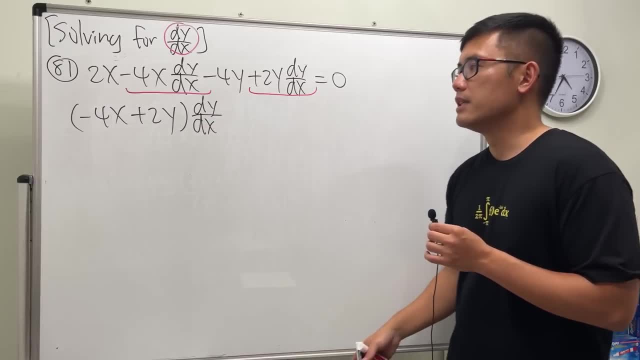 dydx at the end. dydx at the end. and the reason i had to have the dytx at and the reason i had to have the dytx at the end, and the reason i had to have the dytx at the end and the reason i had to have the dytx at the end, it's because, if you put that at the front, 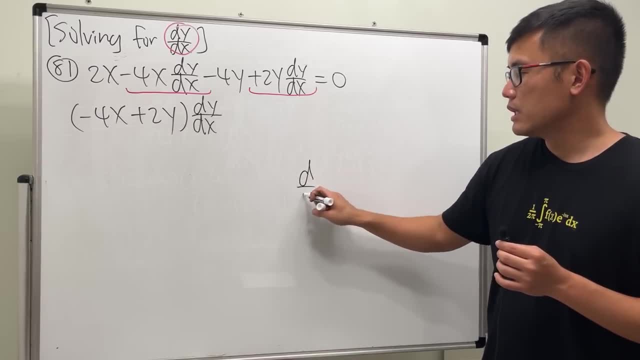 it's because if you put that at the front, it's because if you put that at the front, it might look like a different notation. because it might look like a different notation, because it might look like a different notation, because this means the so-called. you take the derivative. 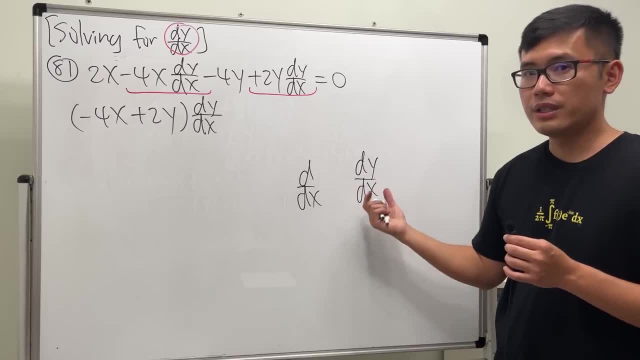 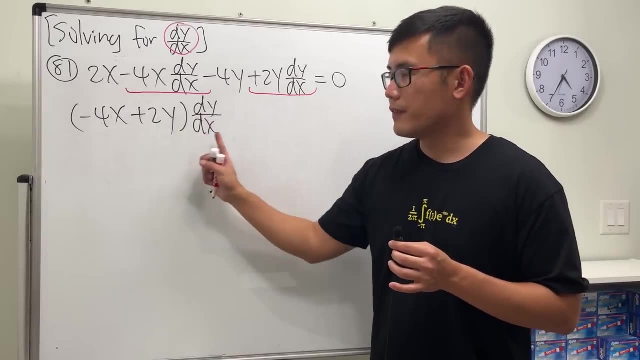 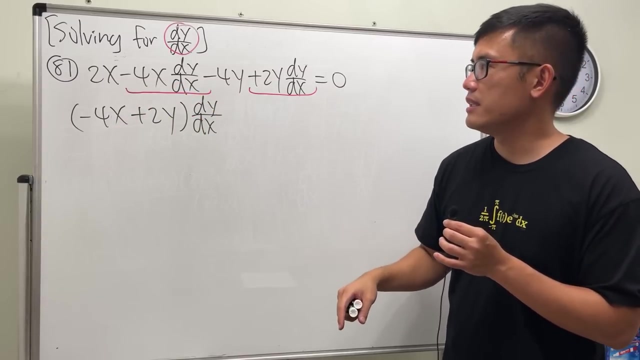 this means the so-called. you take the derivative, and this is the derivative, meaning the result. already they are very different things, so that's just that. but for now, again, just treat this as a variable and let's focus on how to isolate that. so we took this and that out, and then we have the dy dx at the end and we are going to 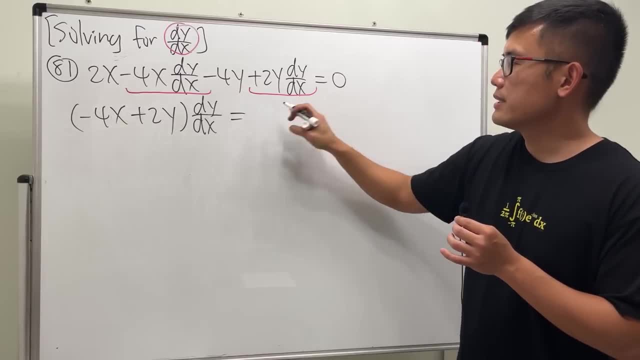 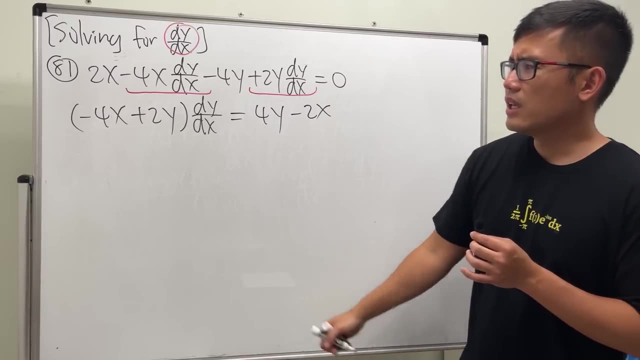 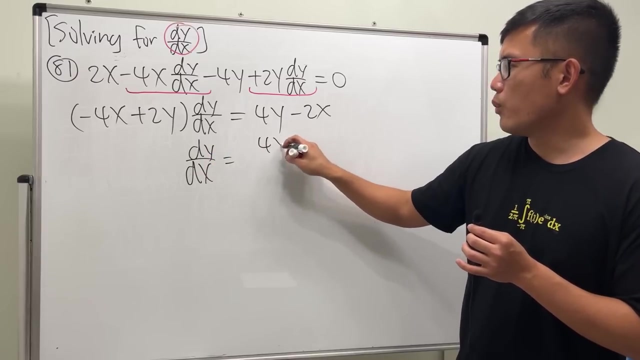 move this and that to the other side. so move this to the other side, we get past the 4y. and then move this to the other side. we get minus 2x, yeah, and then you see that we can now just divide this on both sides, right? so that's pretty much it. dy dx equals 4y minus 2x over. let me write down the 2y. 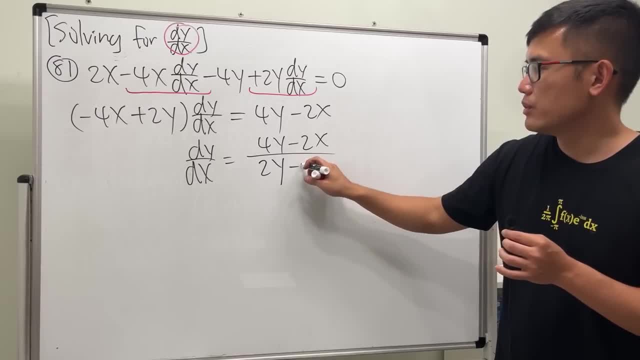 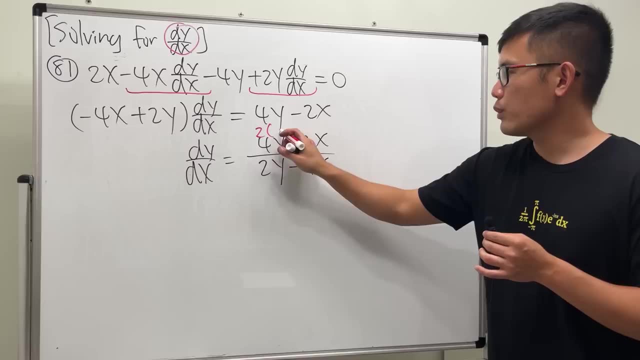 first and then minus 4x. yeah, can we reduce? yes, we can factor out two, and that will give us 2y minus x. and then, right here, we can factor out 2, and that's y minus 2x and this 2 and that will cancel. so we just have 2y minus x over y. 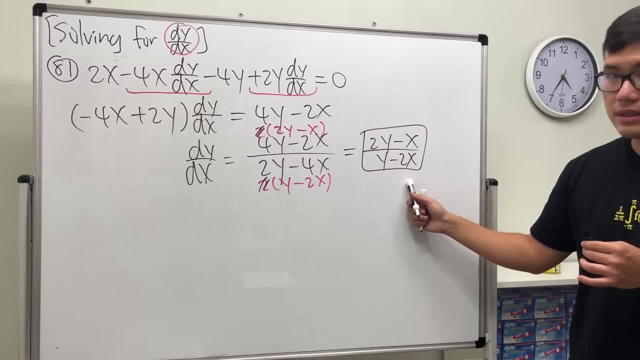 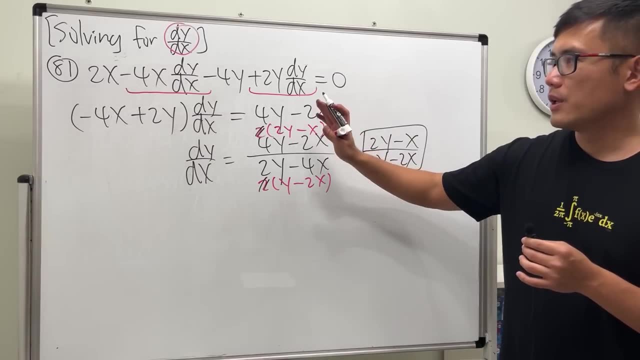 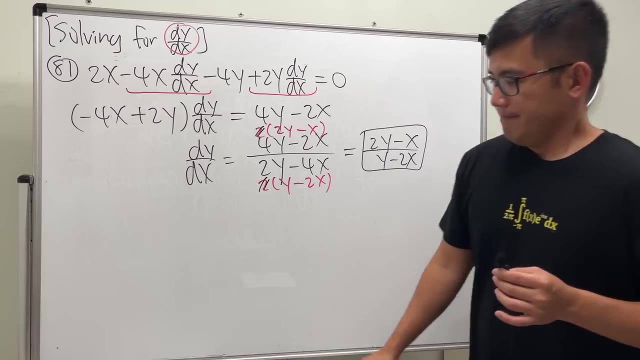 minus 2x done right. so you will see, this is actually really not so bad. it takes about like two lines usually. uh, depending if you have like big fractions or not, you just notice all those lines are so big. so that's why we're going to kind of 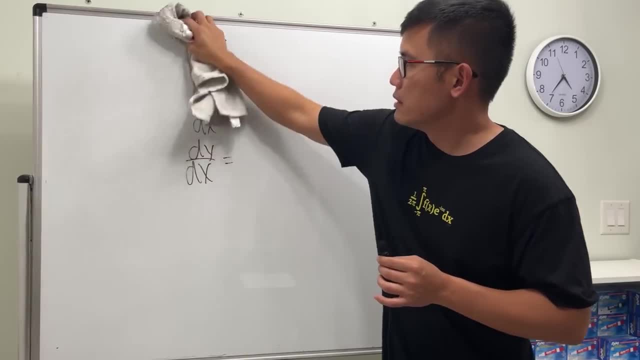 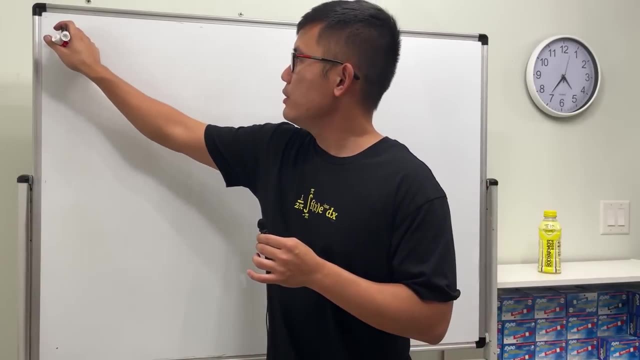 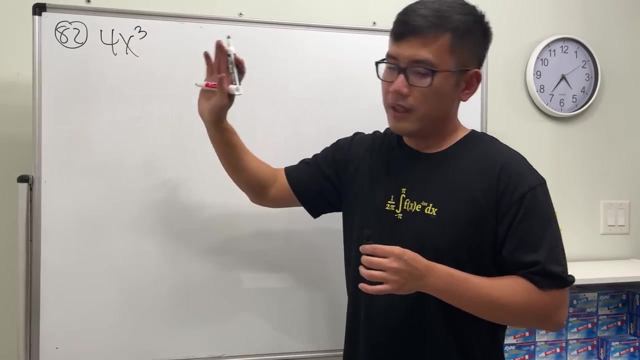 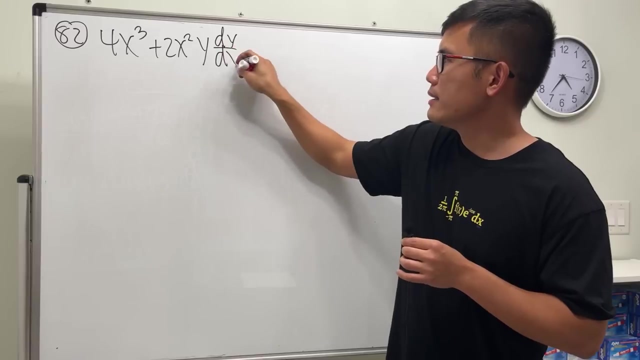 do a little bit of a math test over here. if you notice that my right number 82. all right, it takes like i'm just going to write it down. i'm not going to talk too much. 4x plus 3, power plus 2x squared y, dy, dx. 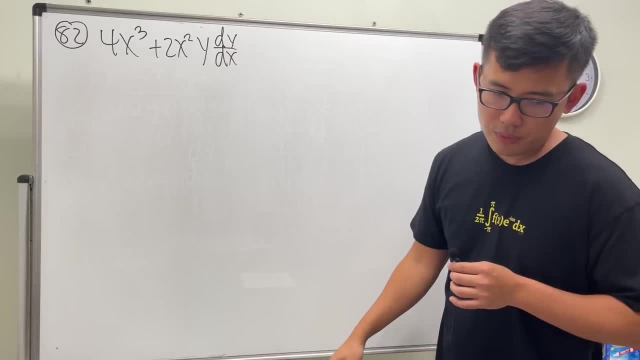 all right, number 82: all right, it takes like. i'm just going to write it down, i'm not going to talk too much. four x plus three. power plus two x square y dy dx x plus two x square y dy dx Plus 2xy square. 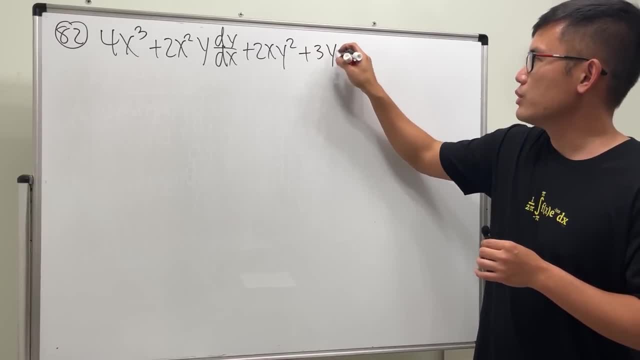 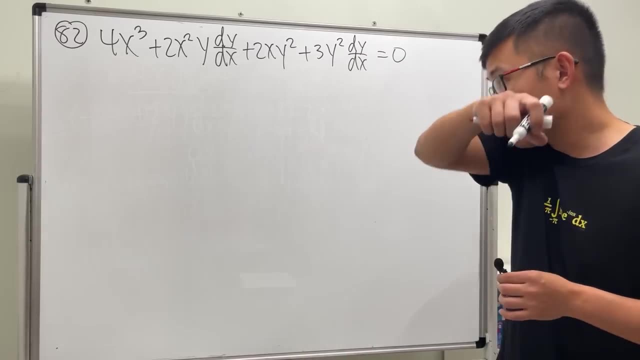 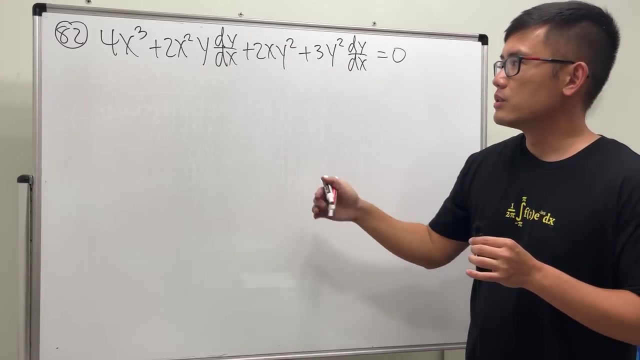 Plus 3x plus 3y square Divided x and that's equal to 0. Alright, so once you have this expression again, do what we did earlier: this turn and that turn. they have the dy dx right, So let's just go ahead. We write down: 2x, square y. 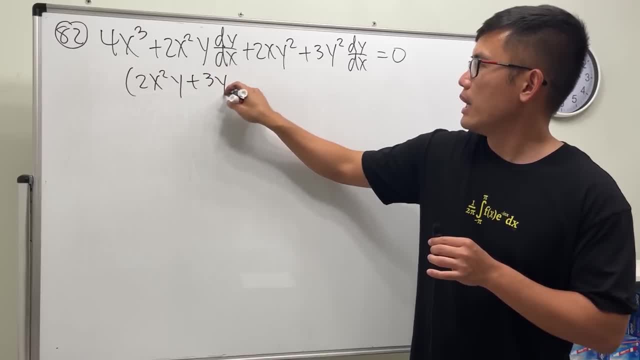 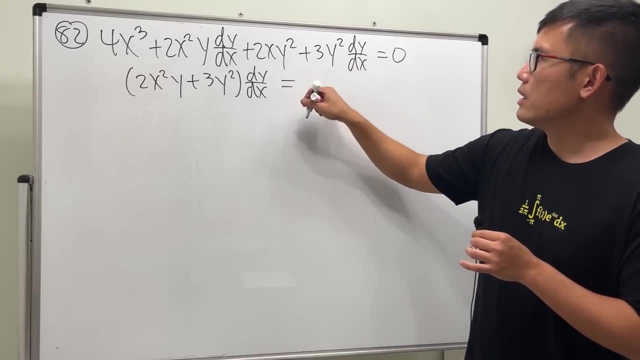 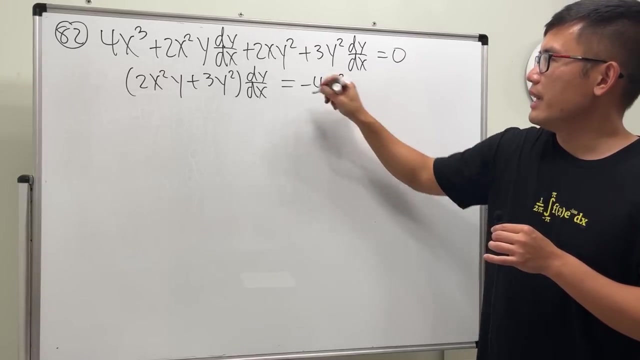 plus 3y square, and then we have the dy dx and then let's see We will move this and not to the other side. So perhaps let's put this: first: That's all negative 4x to the third power and then minus 2x y square and at the end just divide this on both sides. 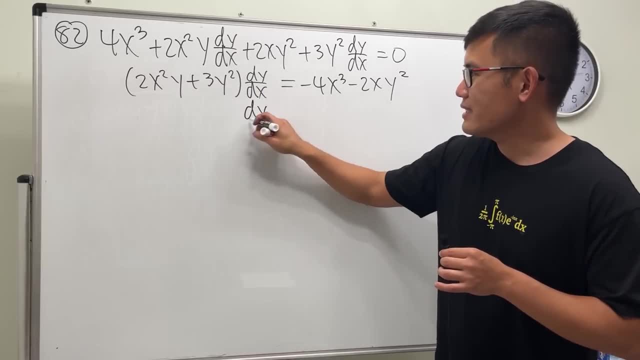 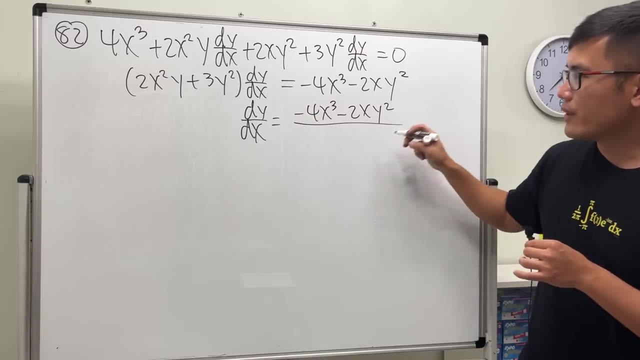 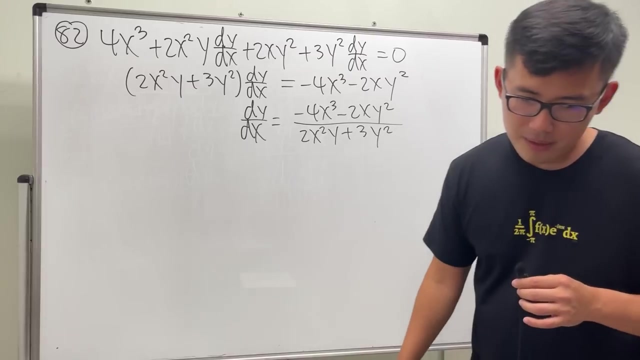 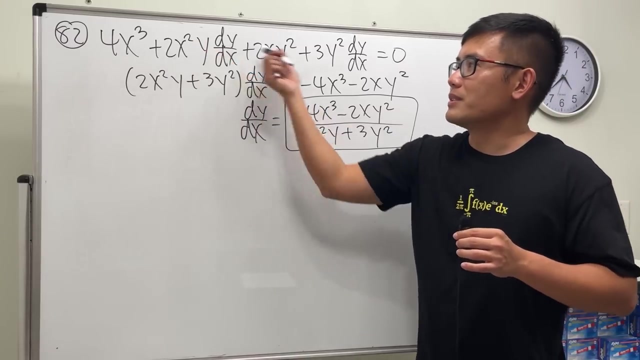 That's it. Yeah, so dy dx equals negative 4x power minus 2x y square over 2x square y plus 3y square. Yeah, just like that. Yeah, and I would like to tell you, For doing this kind of things, the hard part is come with this expression when you are actually doing the calculus. 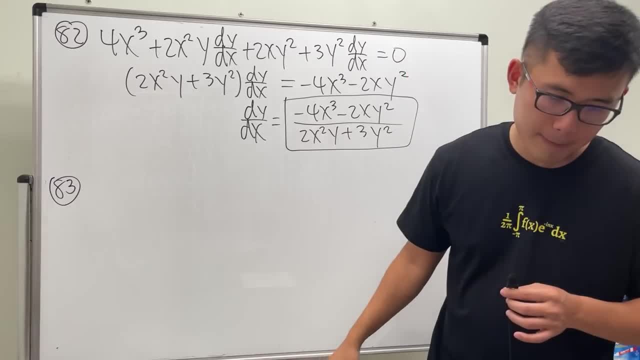 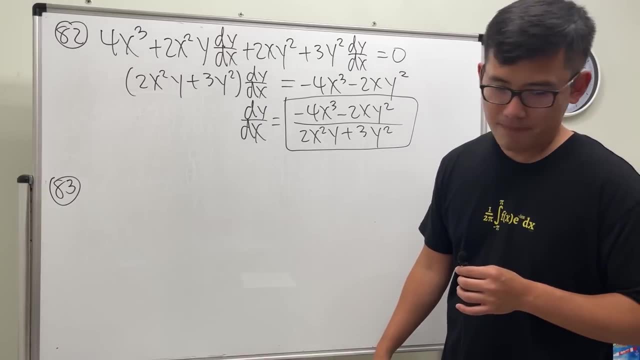 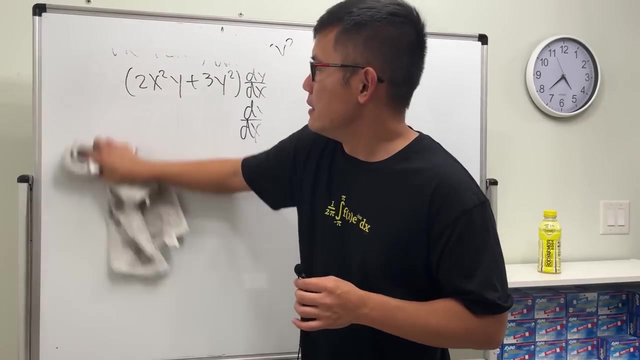 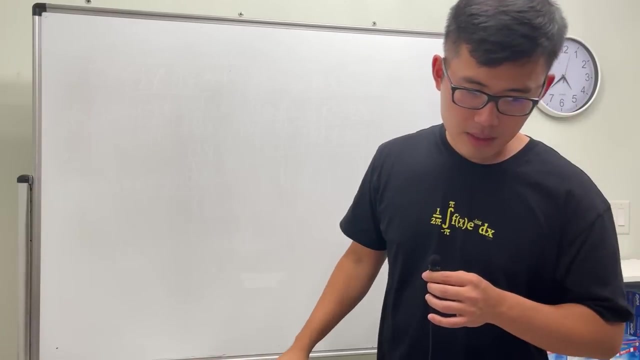 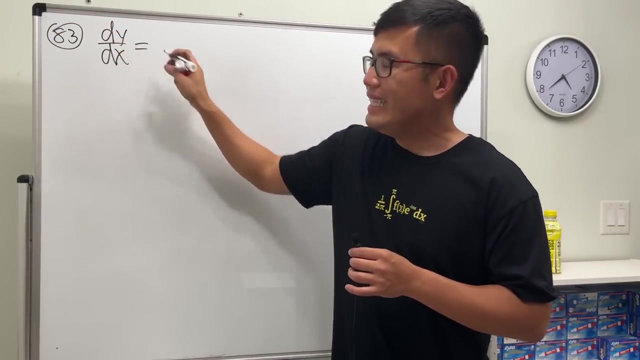 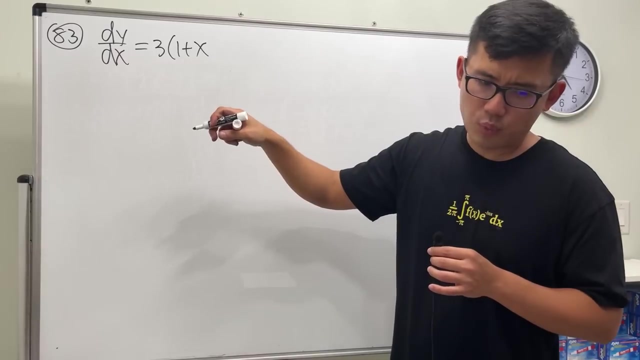 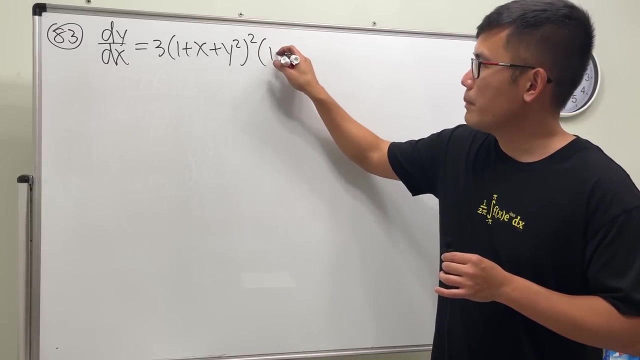 Yeah, All right. next one, a little bit more challenging. challenging enough that I think I should erase the board Right, number 83. We have dy dx here and that's equal to 3 times 1 plus x plus y, squared and Square, and then times 1 plus 2y dy dx. 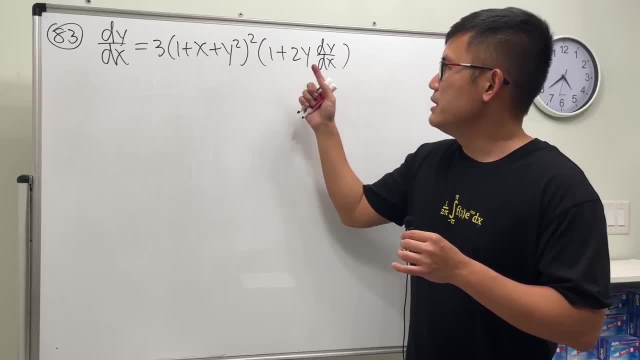 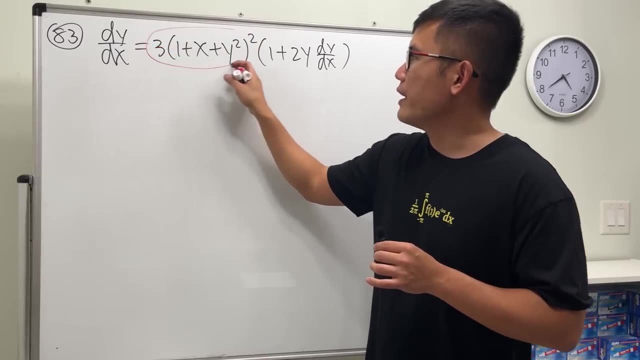 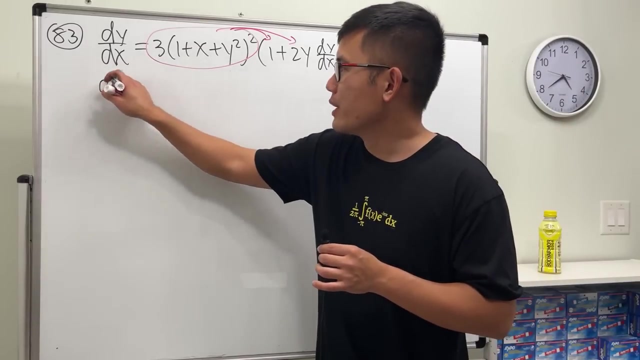 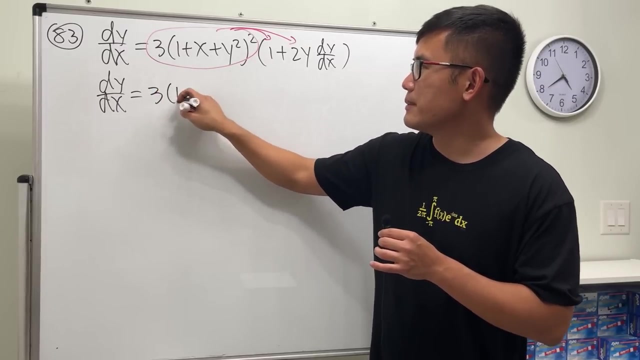 Yeah. So here's the thing. You see, we have this thing times. then here We have a ty dx. All we will have to do first is take this whole thing, distribute Right, so let's do that. so hey, we will get dy dx equals. so this whole thing multiplied by one. just leave it three times one. 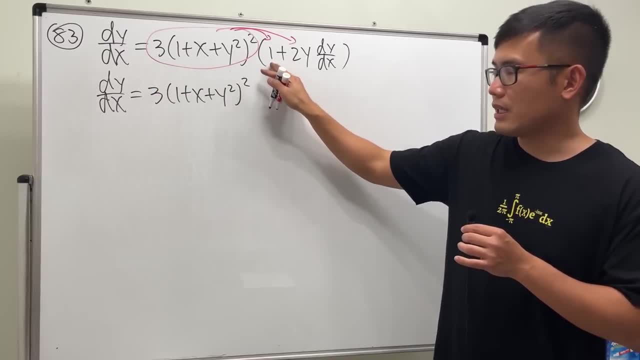 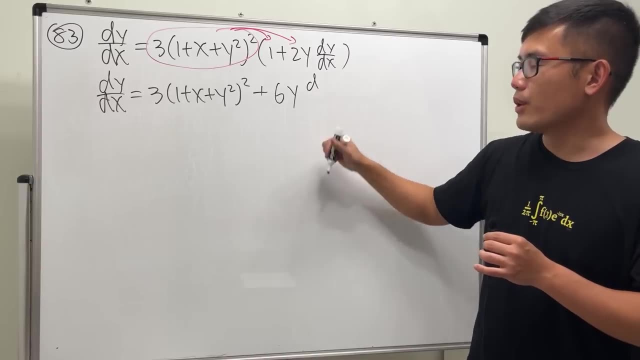 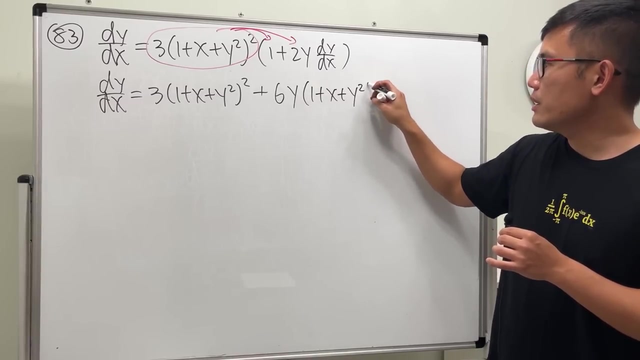 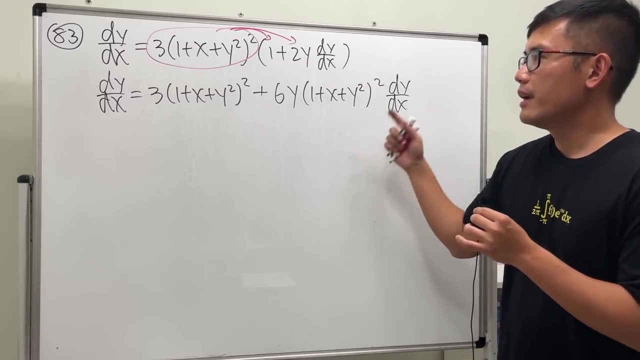 plus x plus y square square, done plus three times two, so we have six and then the y and then dy dx. no, sorry, and how old, i think. one plus x plus y square square and then dy dx. okay, now we have dy dx here and then dy dx over there, and this is technically like the one dy dx. 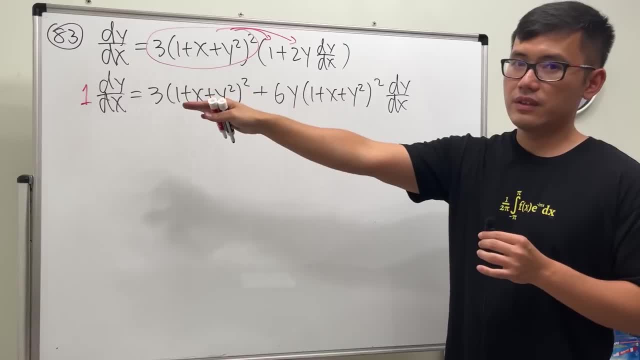 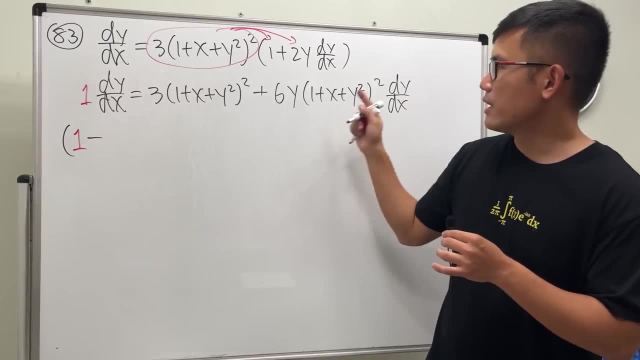 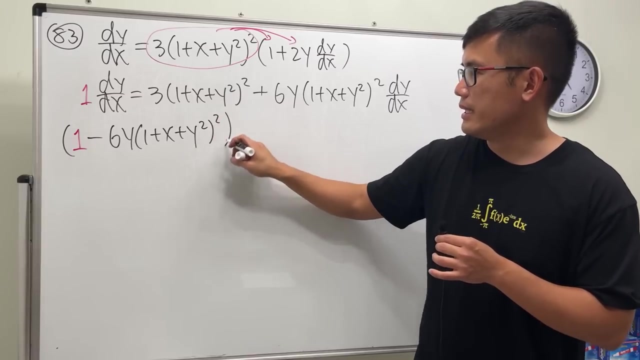 we will move this to the other side and that will be negative, and then we'll factor out the dy dx, so it will look like one right here, and then minus this term, which is six y, and then one plus x plus y, square, square, and then factor out the dy dx at the end. 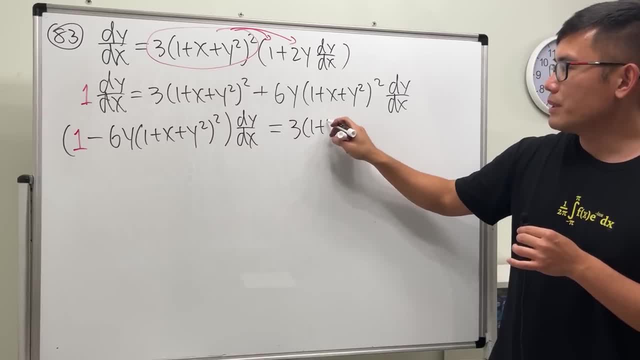 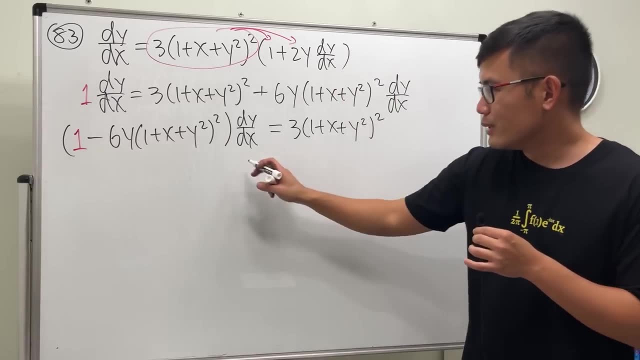 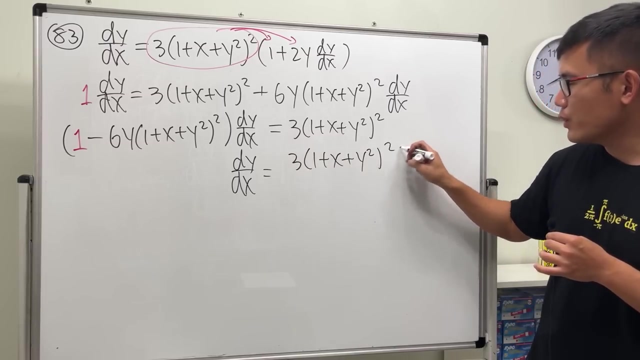 and that's equal to that guy, which is three times one plus x plus y square and then square, and then finally we can just divide this on both sides, that's all. so dy dx equals three times one plus x plus y square, and then square all over one minus six, y times one plus 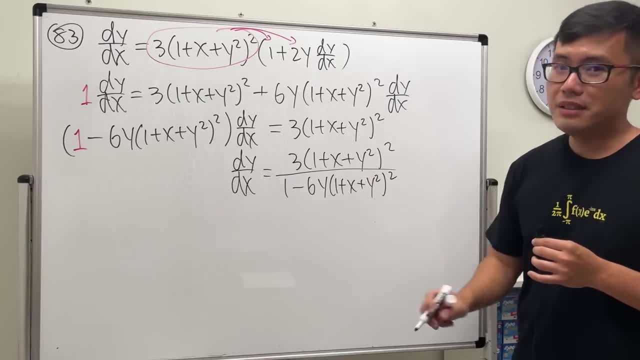 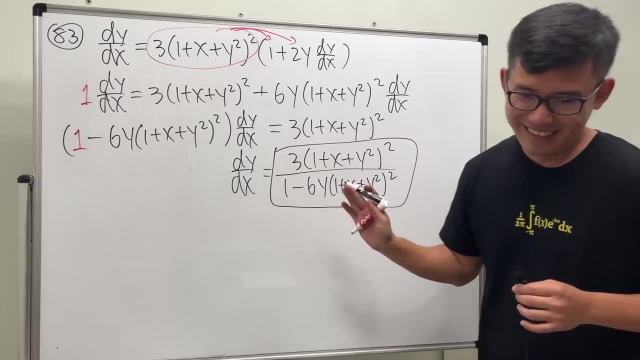 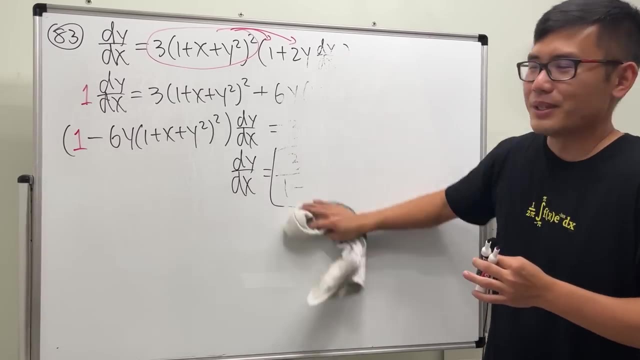 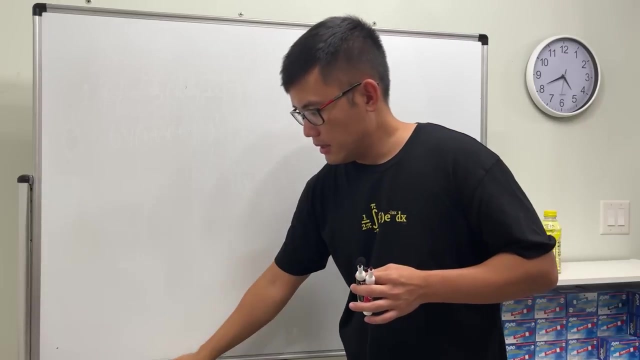 x plus y, square and then square. should we expand this? no, don't do that, don't. it's not healthy. don't, just leave it like that. just do it like that. like, please don't, don't, don't. i'm going to erase this right away, all right. number 84: 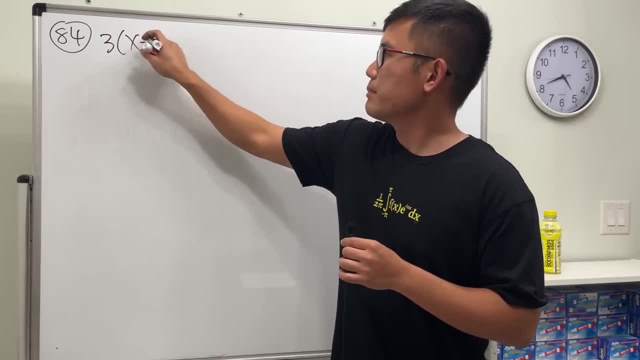 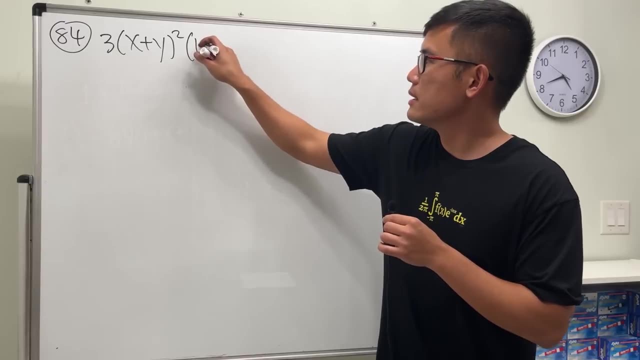 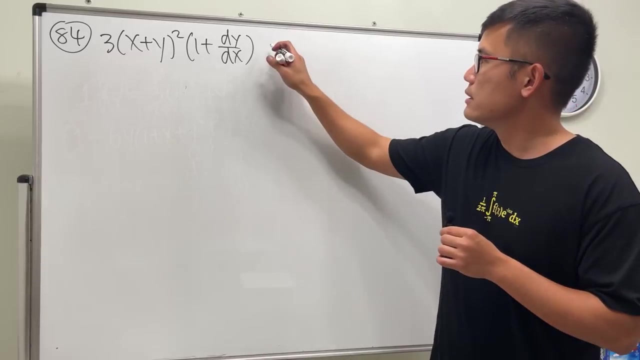 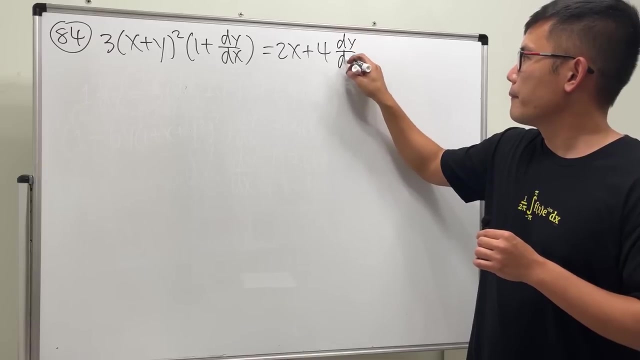 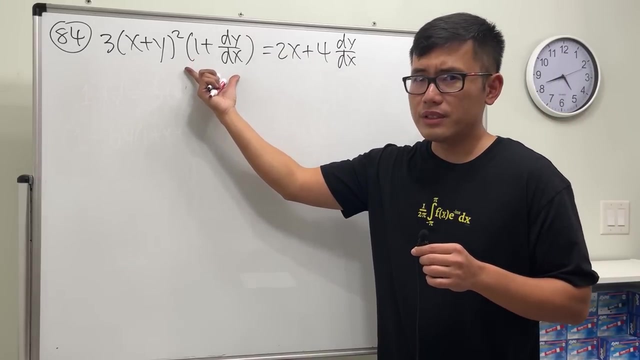 three times the parentheses: x plus y square, and then we have one plus dy dx and that's equal to 2x plus 4 dy dx. yeah. so how do we do it, this dy dx? yeah, so inside of this parentheses, and we have this in front. 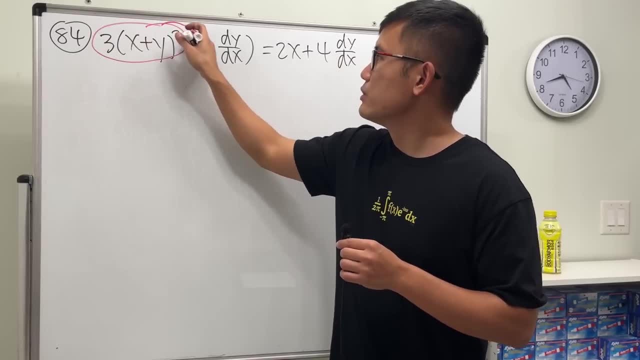 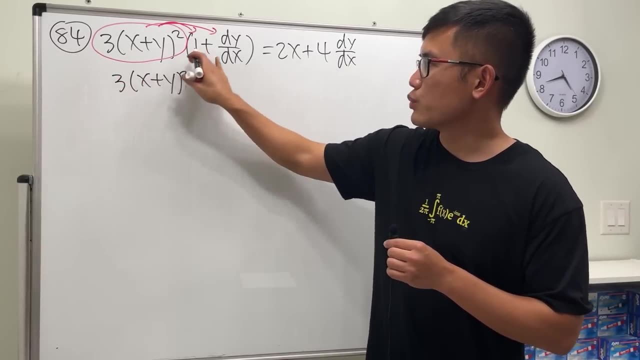 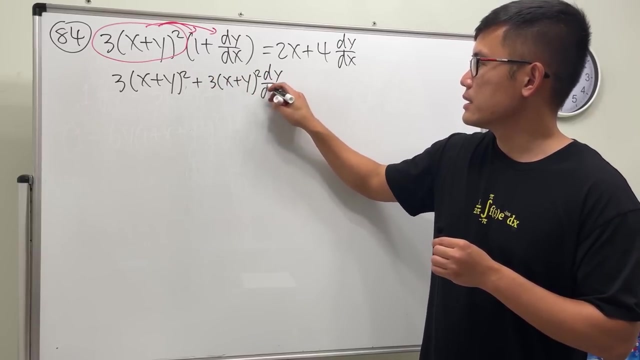 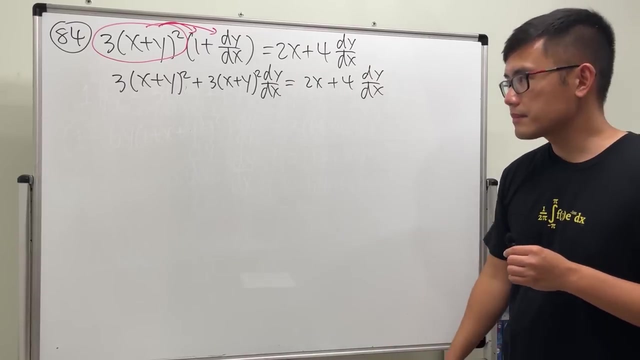 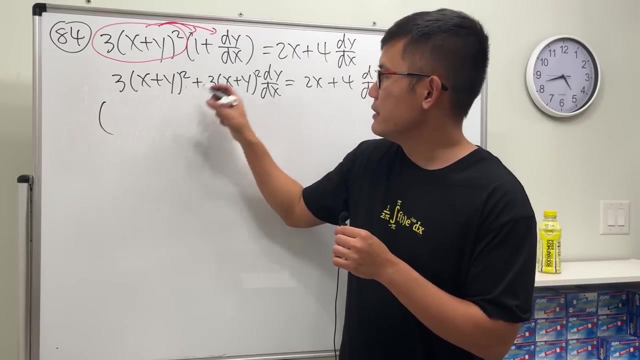 so we'll take this thing, distribute, distribute. yeah, so we get 3 times as plus y2 times one, just this plus three times x, plus y square dydx, and then that's equal to 2x plus 4 dy d x. now i'm just going to move this to the other side: factor out the dy dx, so we have this, which is three times x times y square, and thenó. 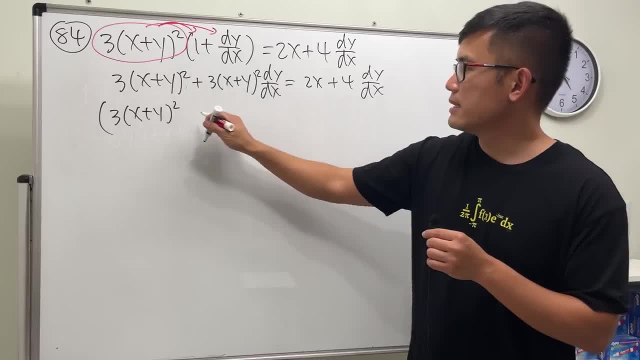 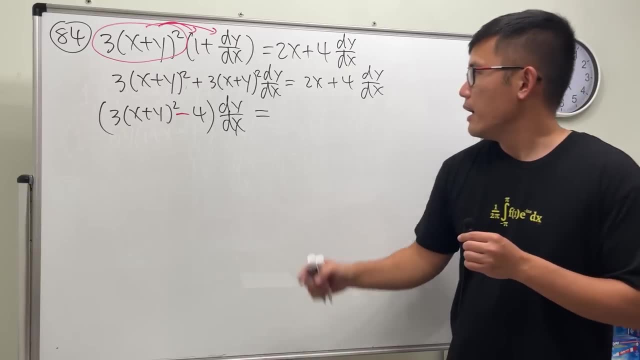 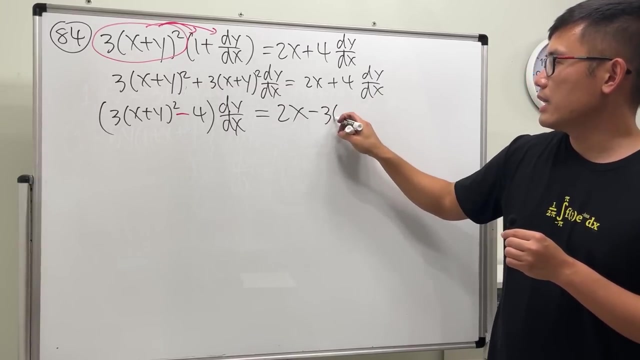 x plus y square and then minus the 4 and then they have the dy dx term that's equal to the 2x is still here, but we will move this to here because it didn't have the dy dx. so minus 3 times x plus y square and then finally just divide this on both sides, so we have dy dx. 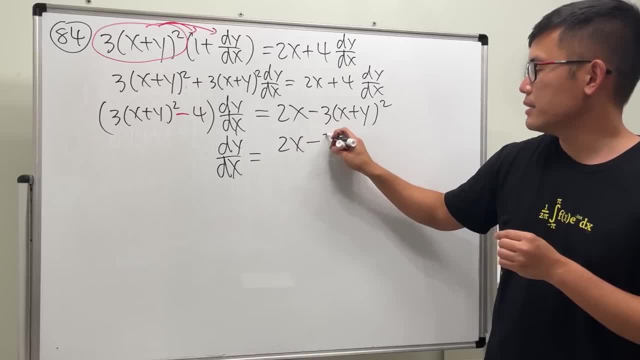 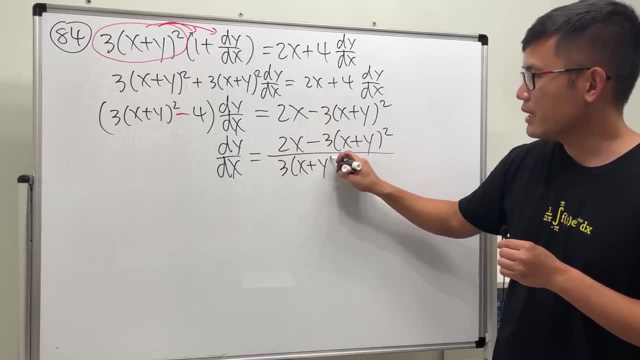 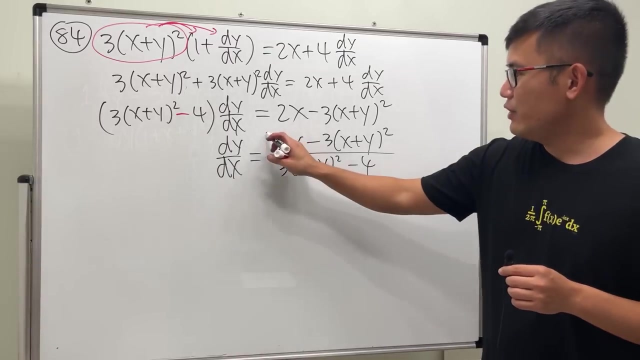 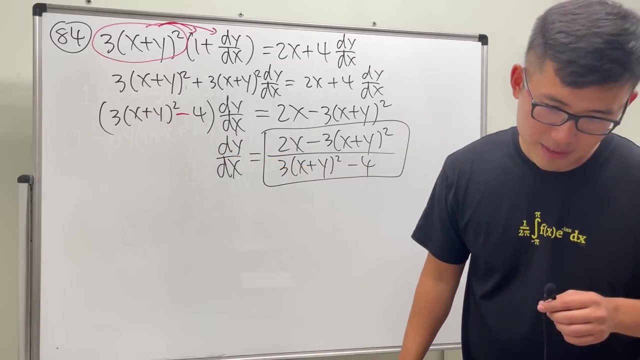 equals 2x minus 3 times x plus y square over, that is, 3 times x plus y square, and then minus 4. so we expand this. no, don't do that, just leave it like that. everybody will be happy. seriously, all right, yeah, okay, so far, so good. huh, and now let's take a look at. 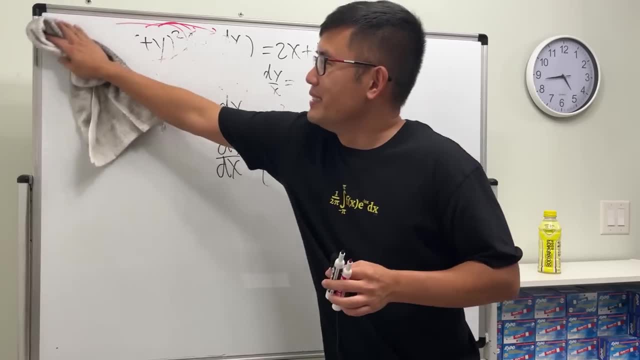 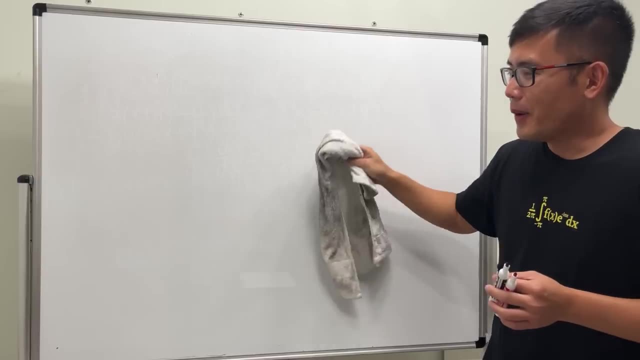 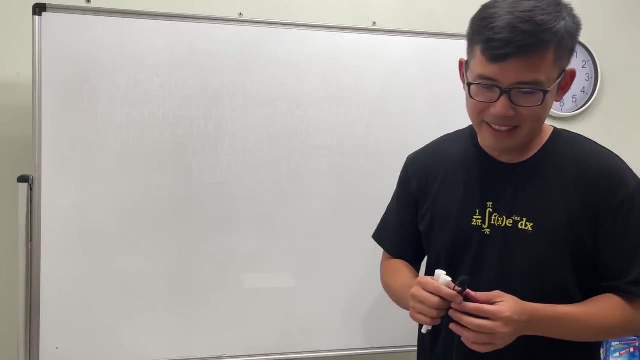 something else. some more crazier examples. crazy enough that i have to erase the board. i just realized this right here is very tiring because i have to erase the board almost every single time, even though the questions are not that hard. but it's like tiring. 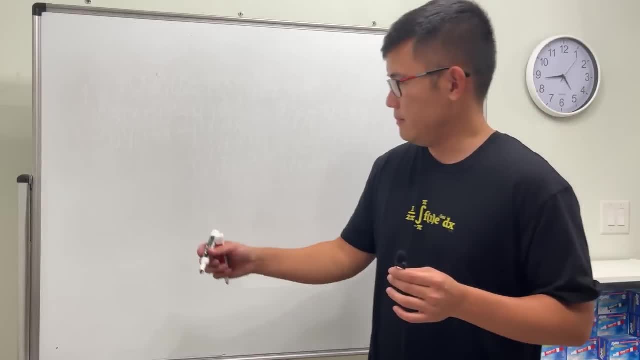 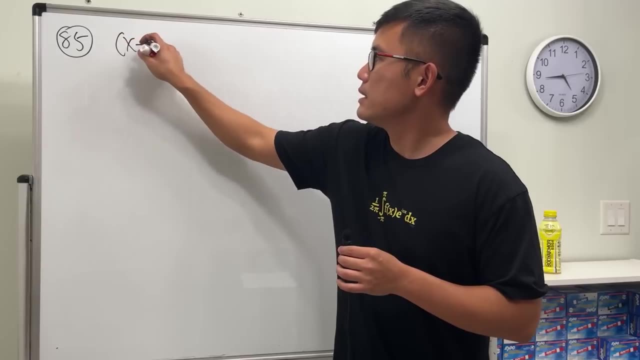 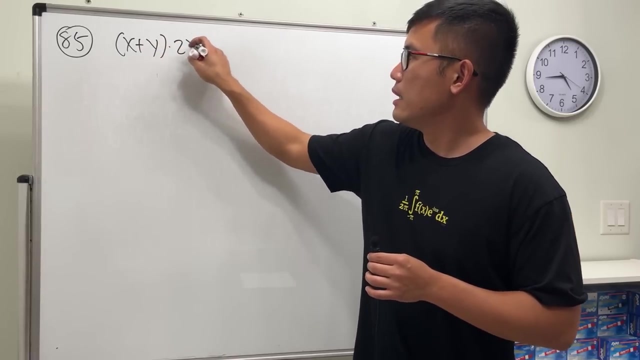 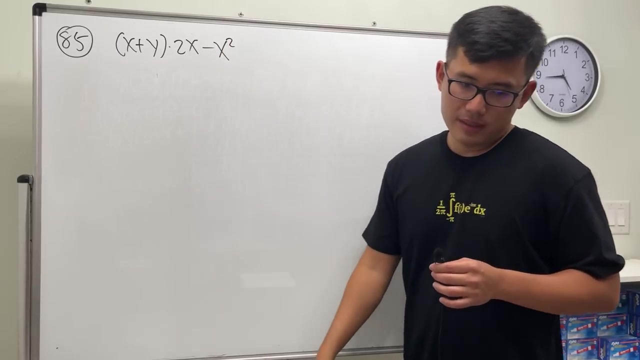 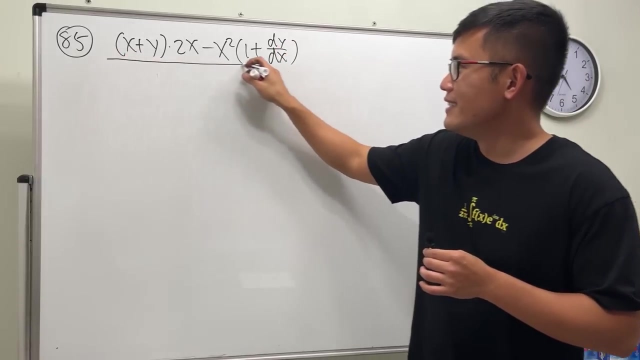 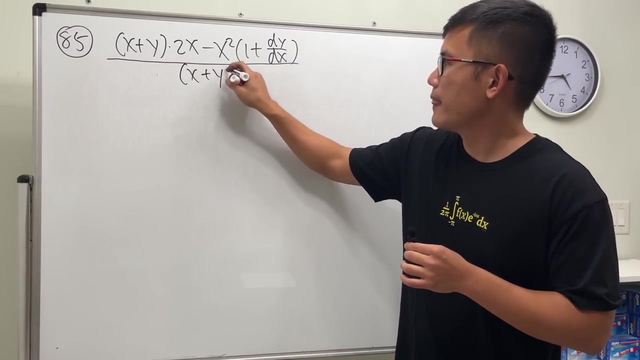 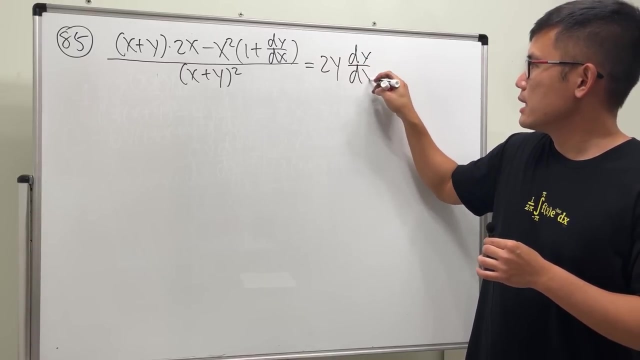 okay, i will not complain anymore. let's check this out. 85, all right. x plus y times 2x, x plus y times 2x minus x square times 1 plus dy dx everybody over x plus y square zu Hunter sounding. are you in from the? 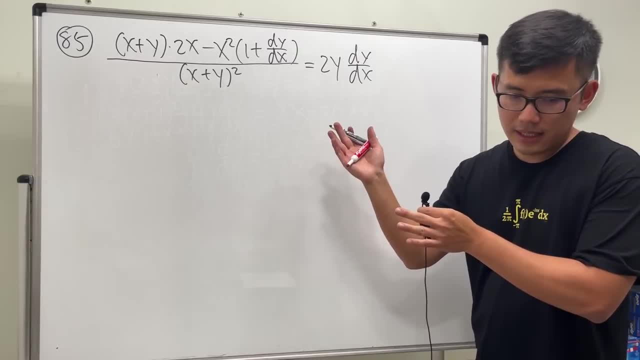 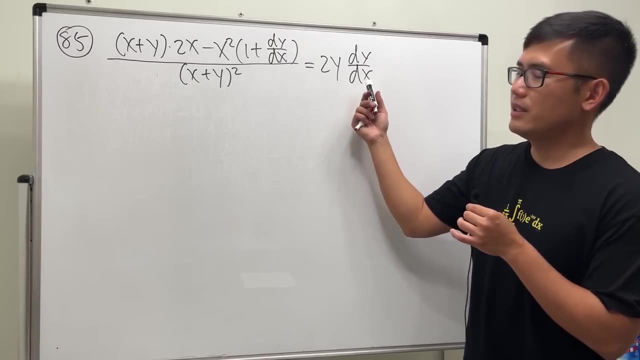 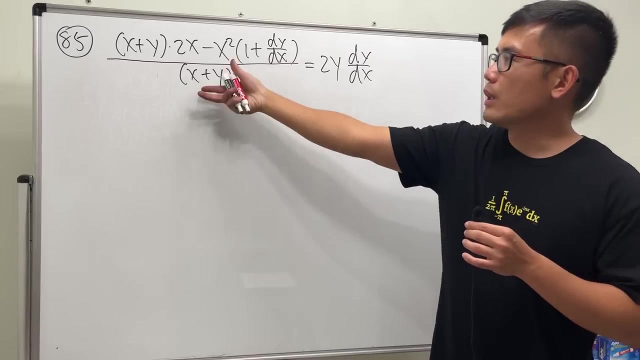 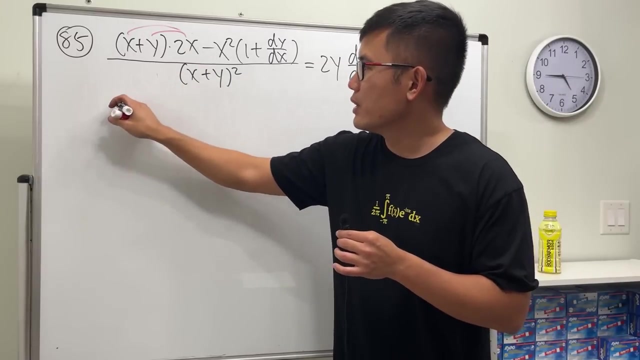 written dimension into this n space. so this, let me calculate and say y times 2x is nothing, because using the overweight vector table, because the over here equals 2y, dy, dx, let's just distribute this guy and it's no power. so it's okay. so here we get 2x, square, yeah, and 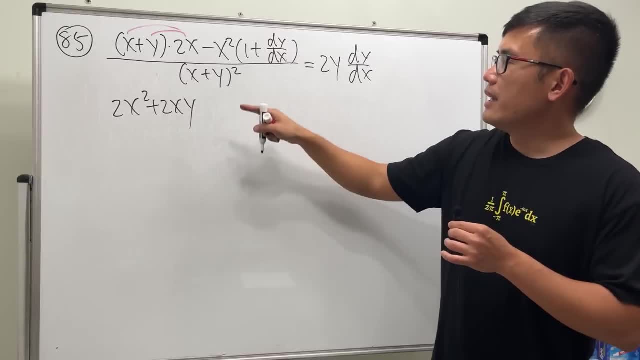 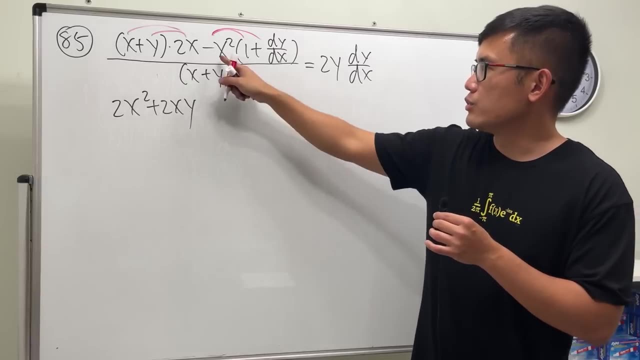 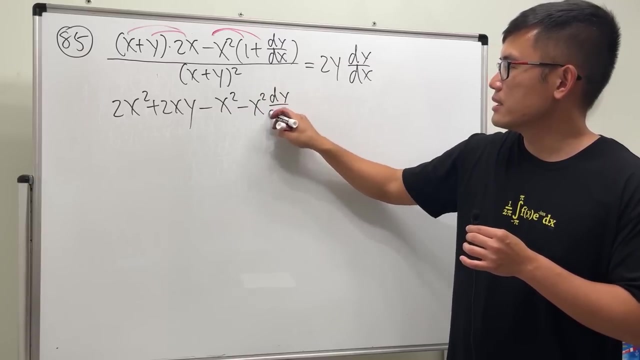 then plus 2xy, okay, and then i will also distribute this. yeah, because i have to make sure they have separate terms, right. so distribute. so this right here will be negative x square and then minus x square, dy dx. yeah, make sure we are ready. just say earlier, when we have stuff inside in front. 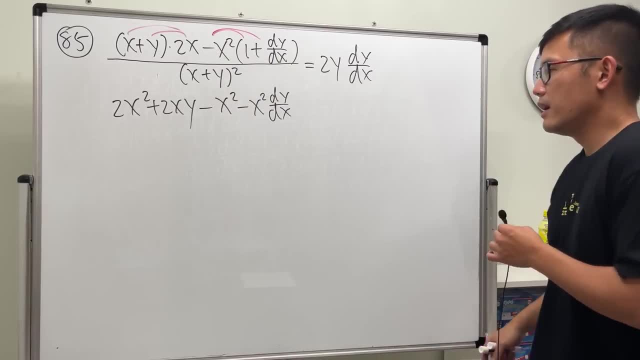 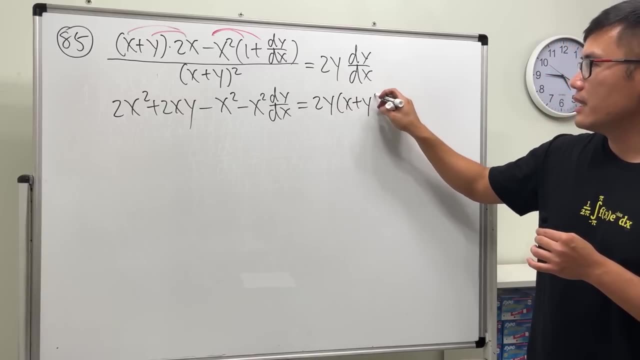 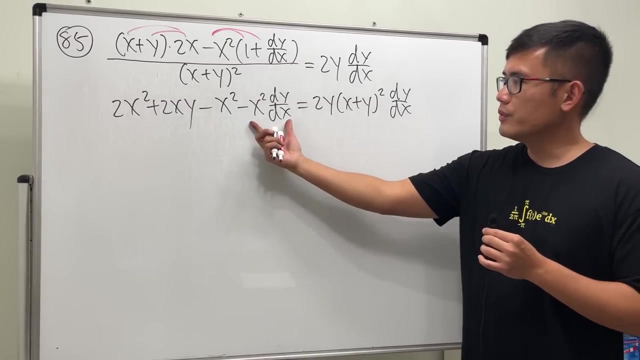 of the parentheses. you get the dx inside. we have to distribute: yeah, so far, so good, and then we'll put this right here. so this is 2y x plus y square, and then you y dx, and for this one in particular, i'm going to move this to the right-hand side so that i can keep all 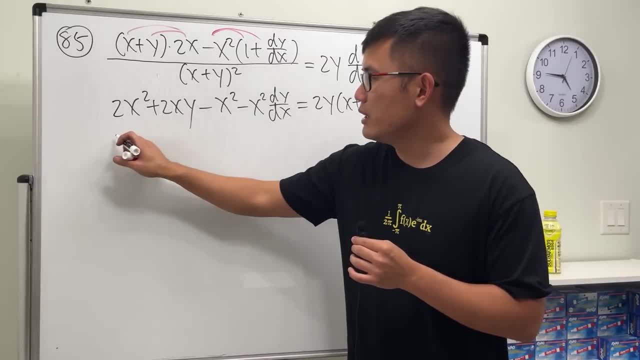 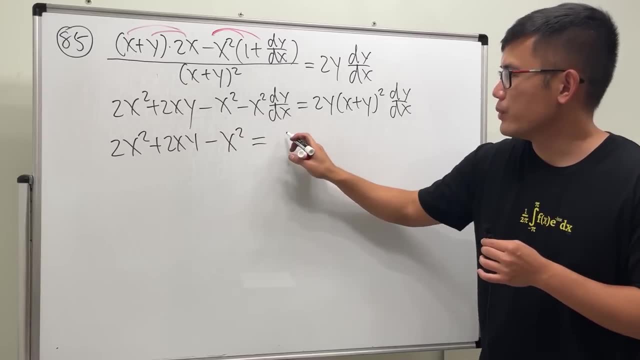 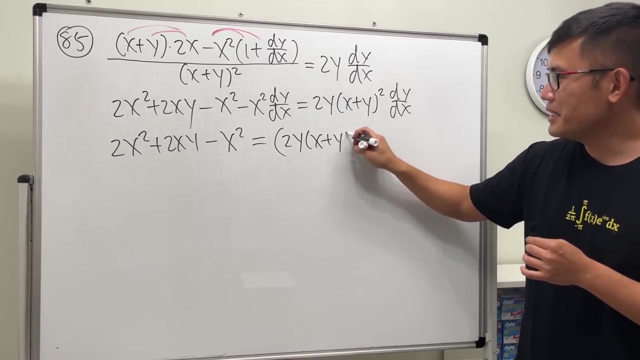 this positive. okay, so right here, i'm just going to leave this: 2x square plus 2xy minus x square, and then that's equal to this. this, this is still here on the right hand side. so 2y times x plus y square. bring this to the other side, becomes a plus, and then we have x. 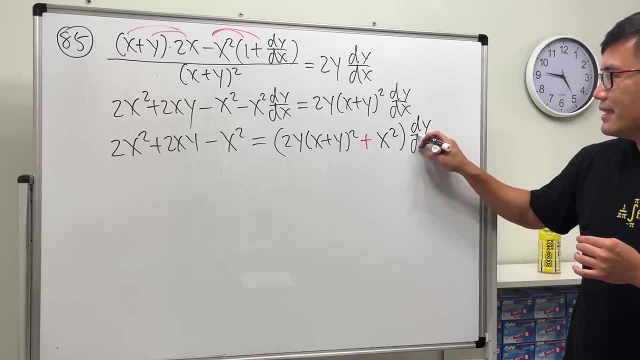 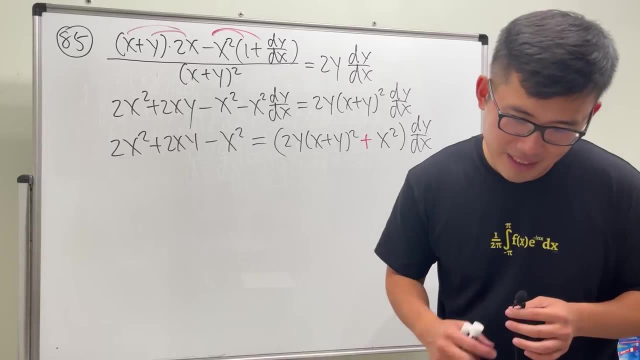 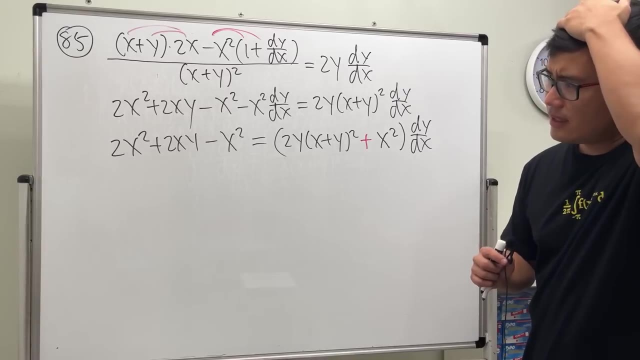 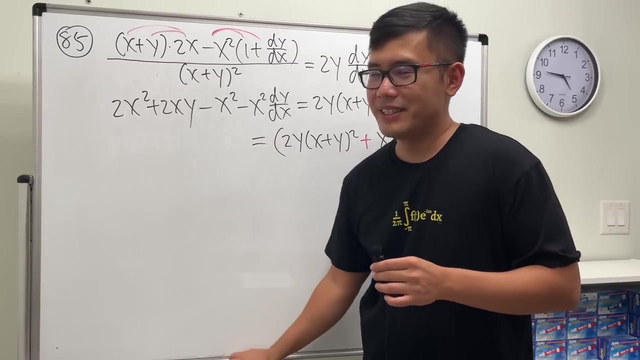 square like so and then dy dx. so we expand this. I'm going to leave that to you. the idea expanded. no, I did not spend that. no, I did not spend that. and oh, notice, I forgot this thing that we can do. check this out: 2x square minus x. 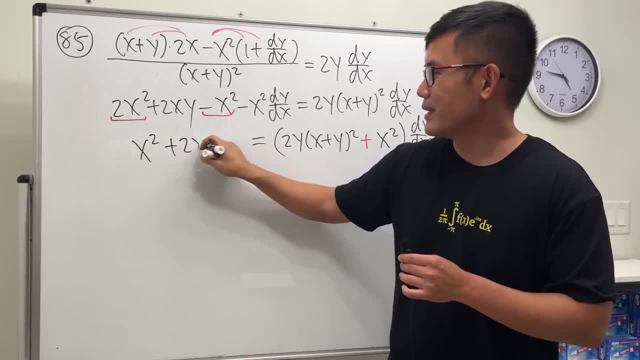 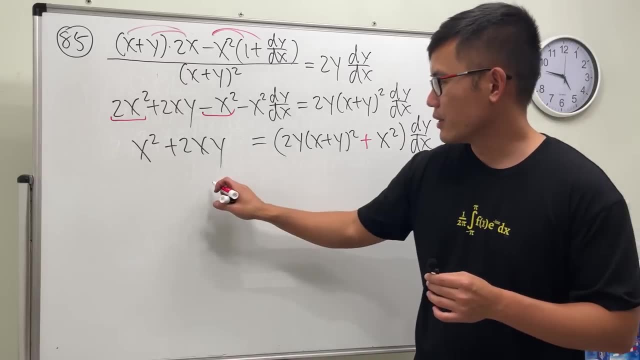 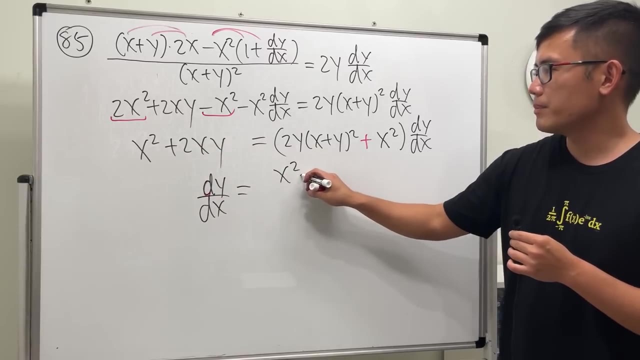 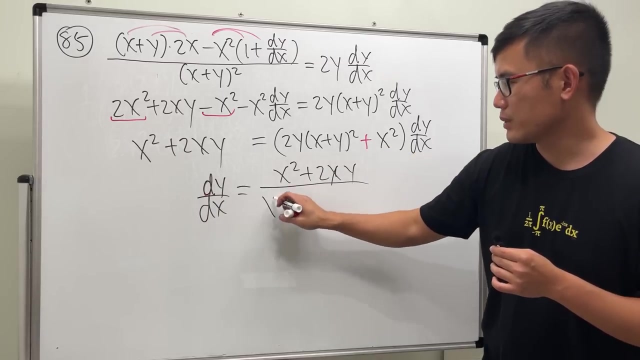 we can just say x square and then put 2x y. yeah, now, let's just divide. so, ladies and gentlemen, divide the x equals this thing, which is x square plus 2x y over. perhaps I'll write this down first, because that will line up with the x square. yeah, so this? 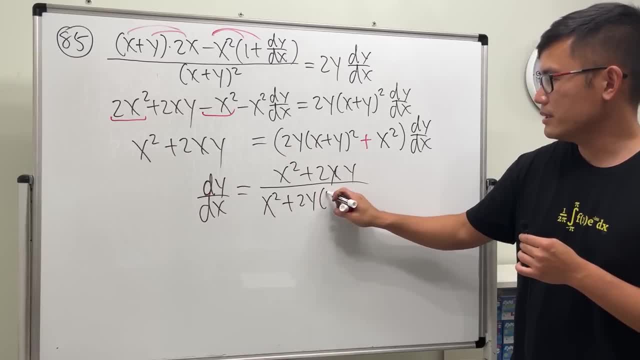 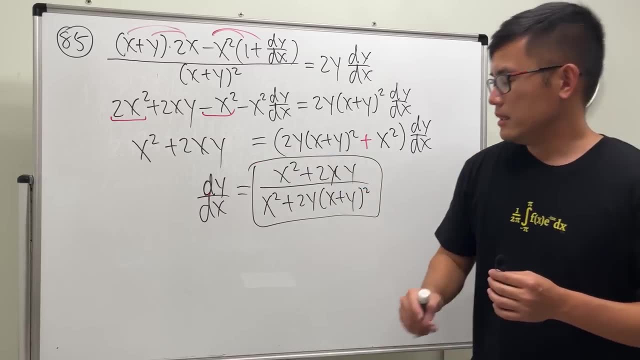 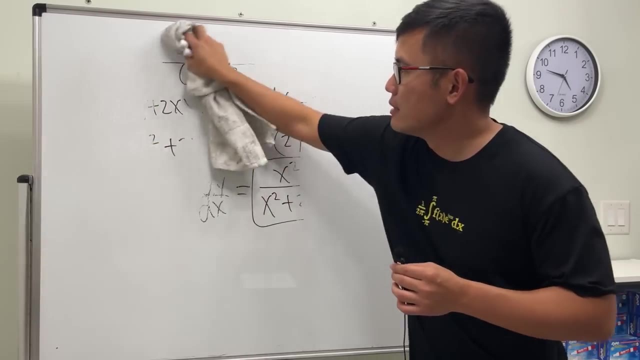 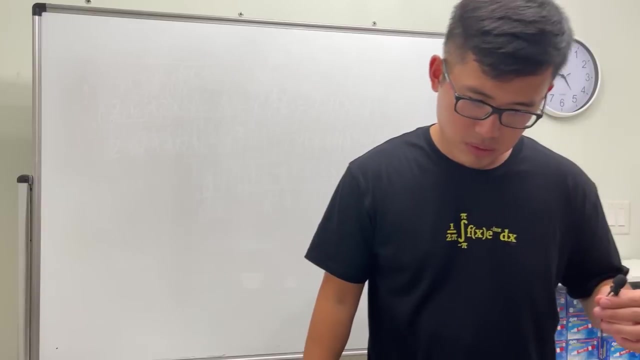 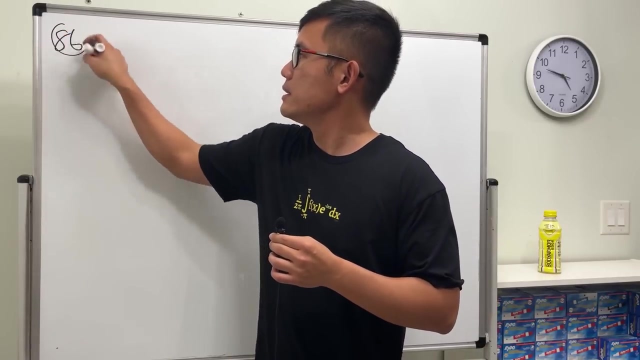 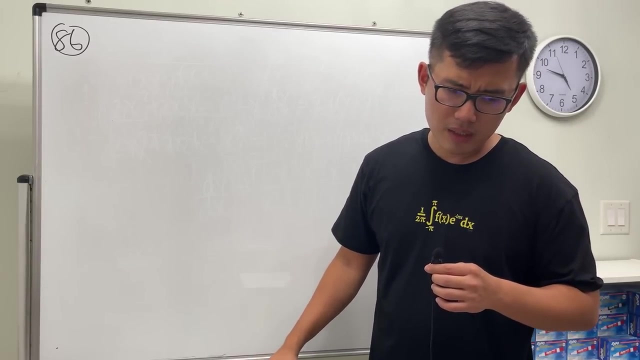 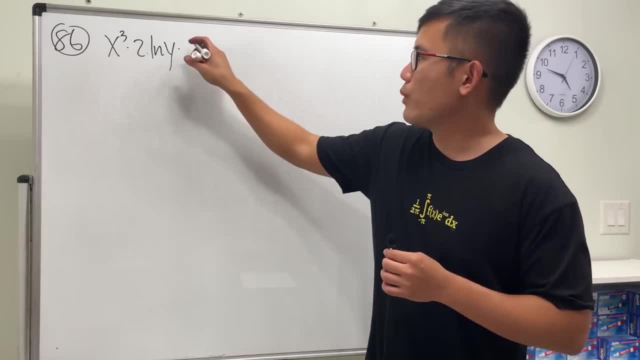 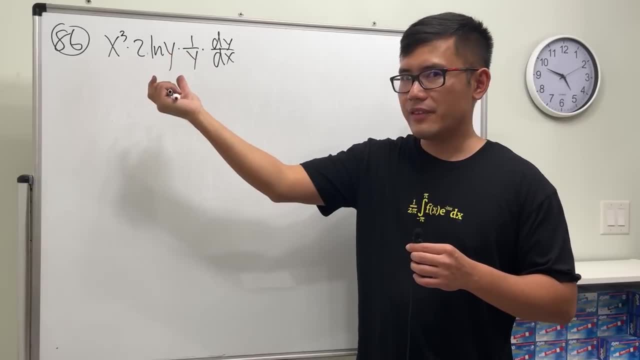 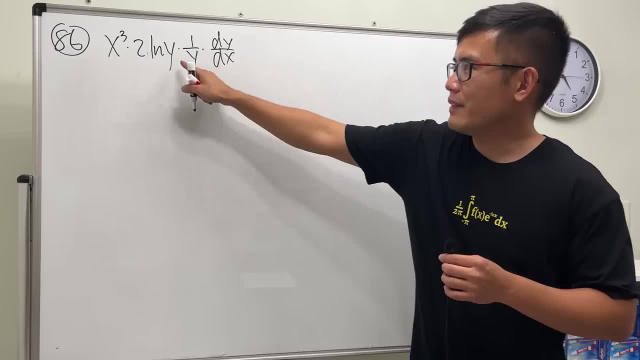 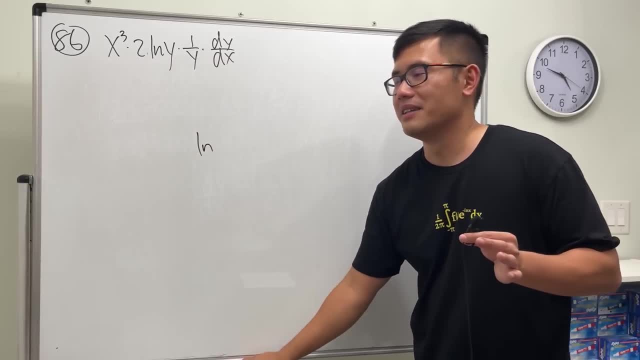 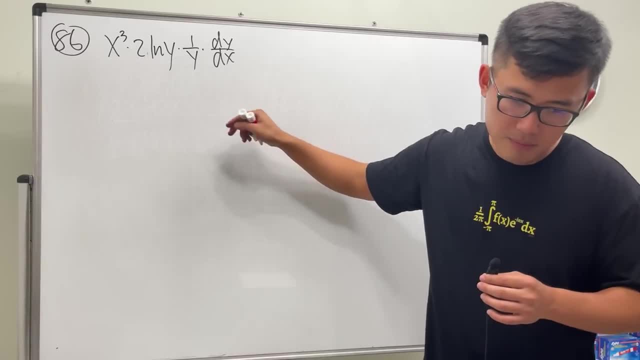 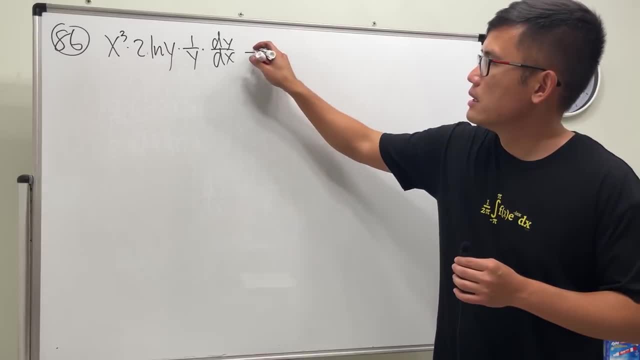 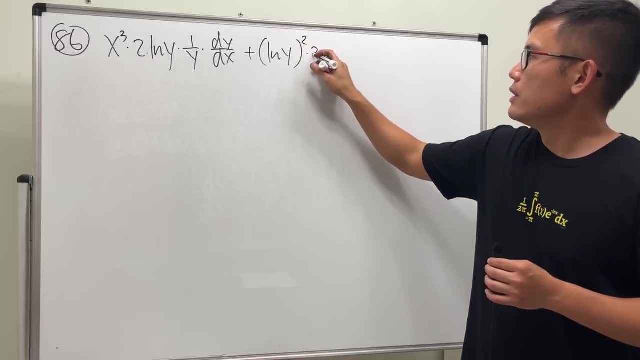 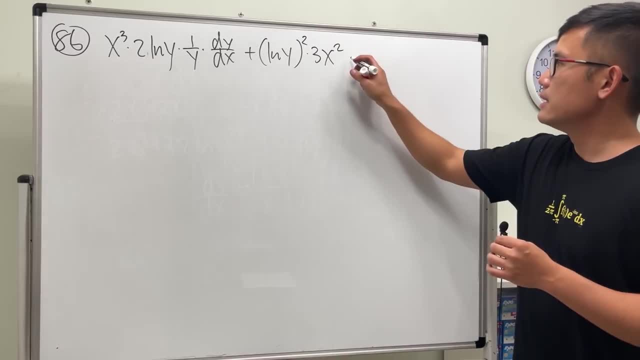 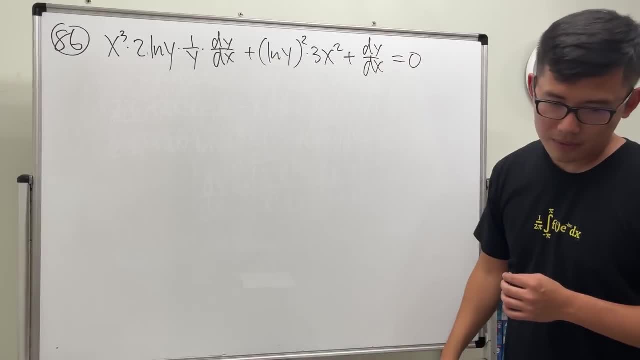 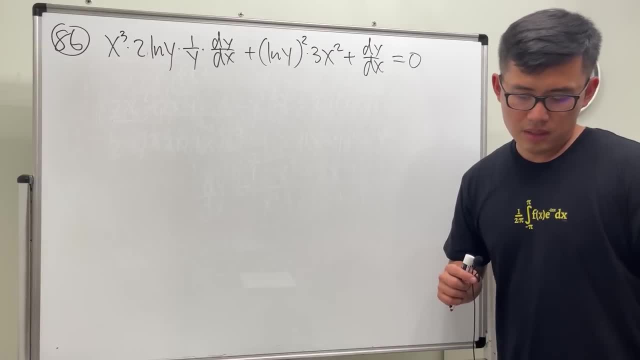 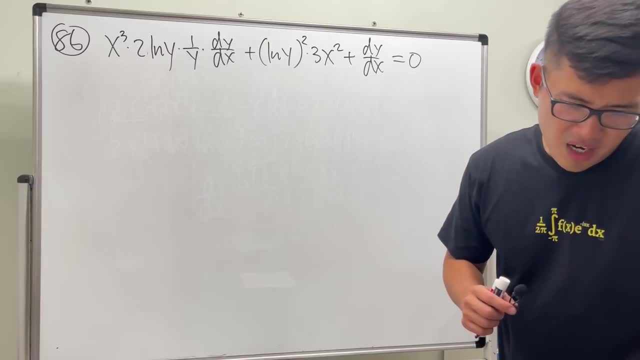 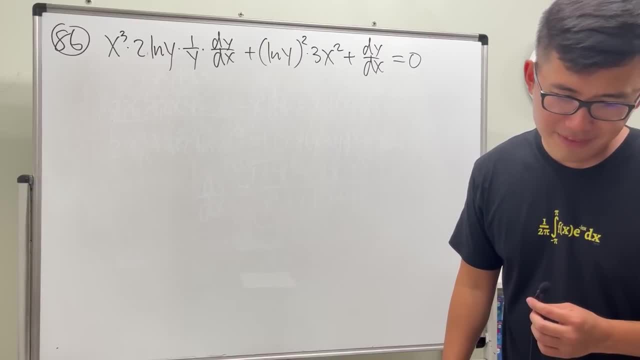 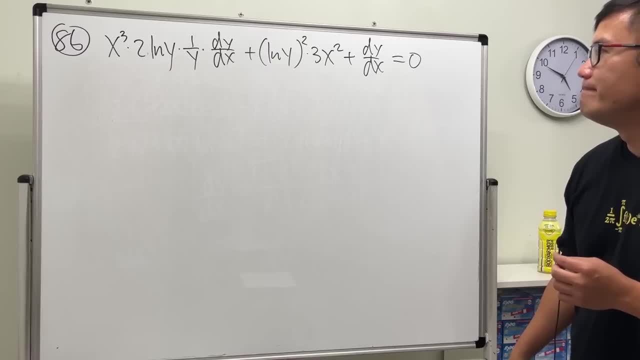 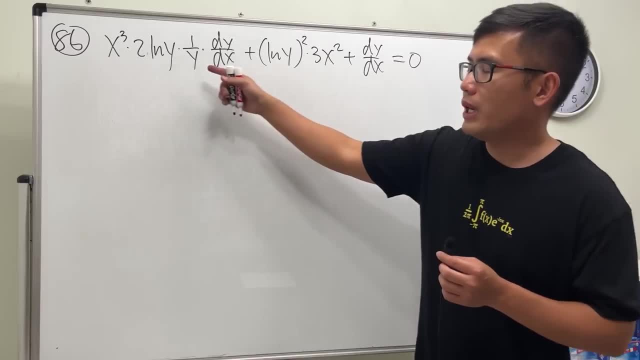 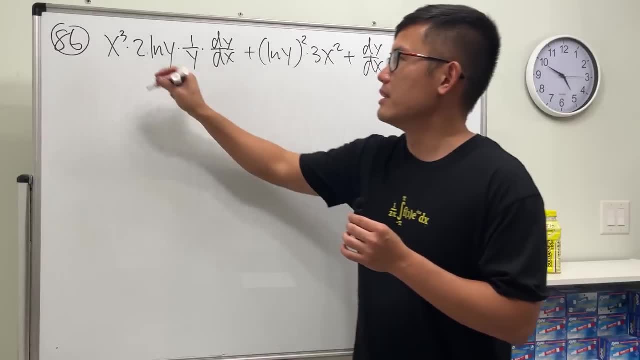 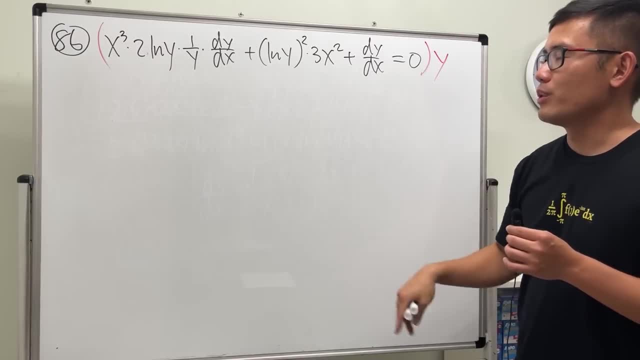 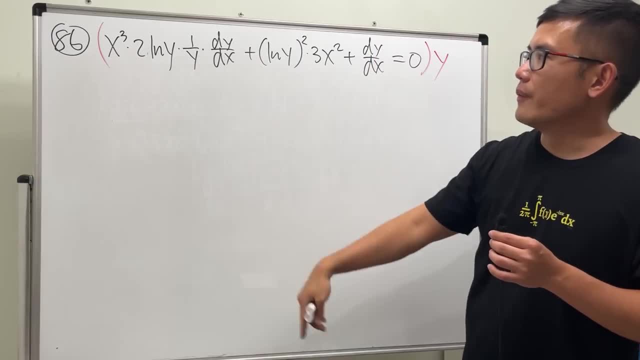 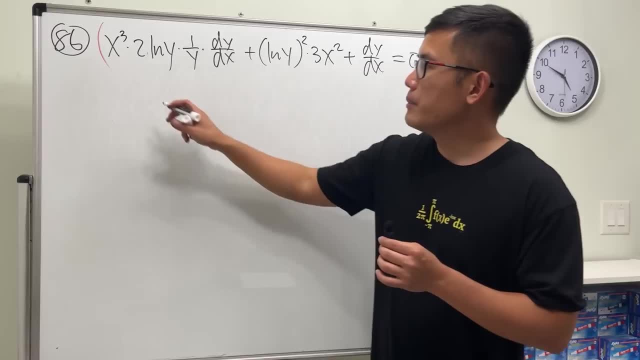 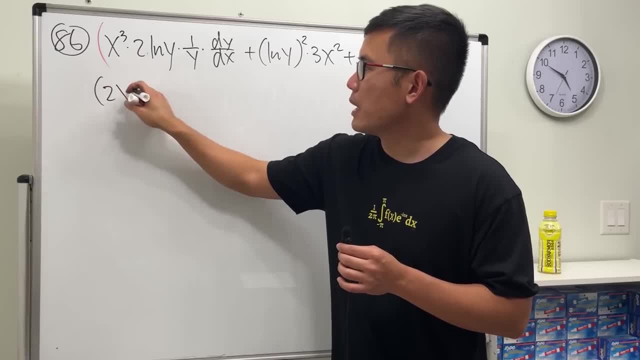 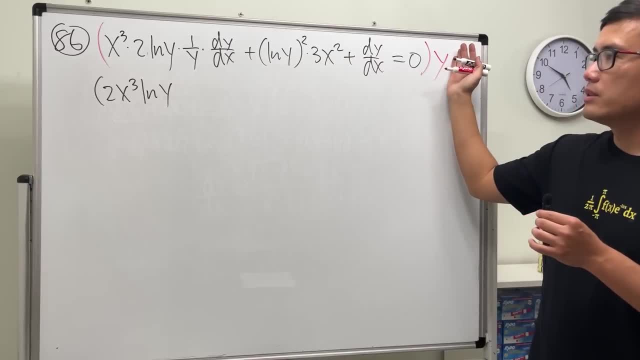 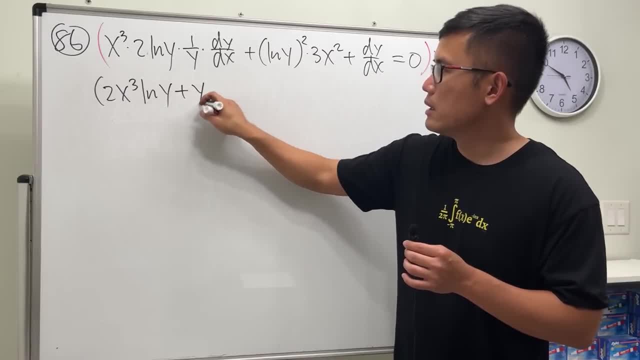 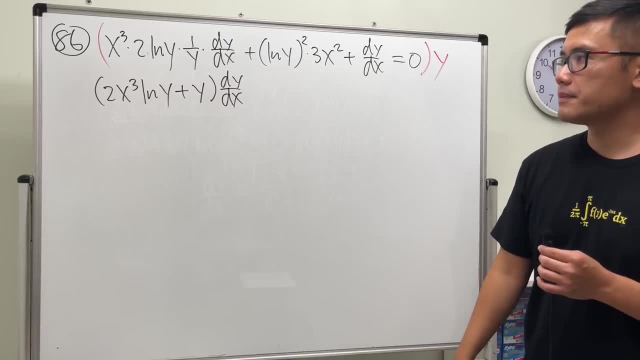 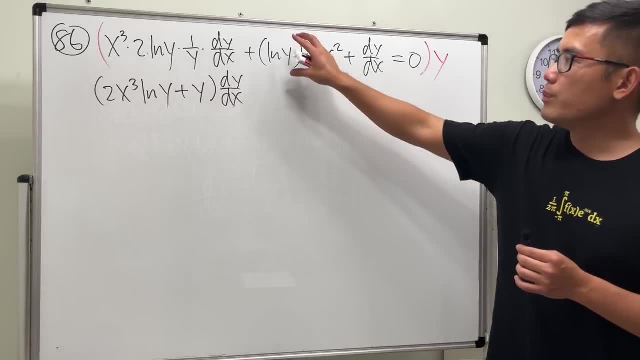 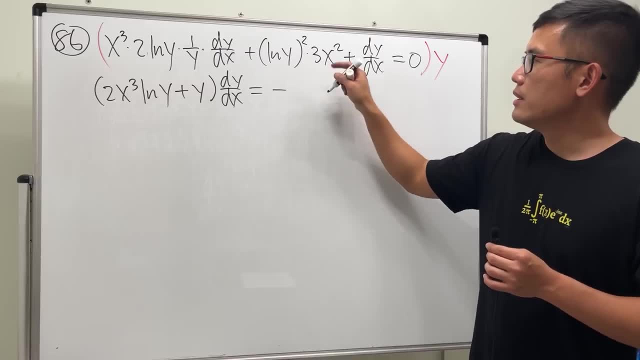 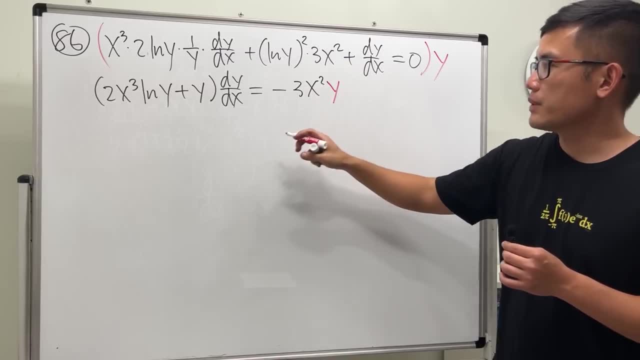 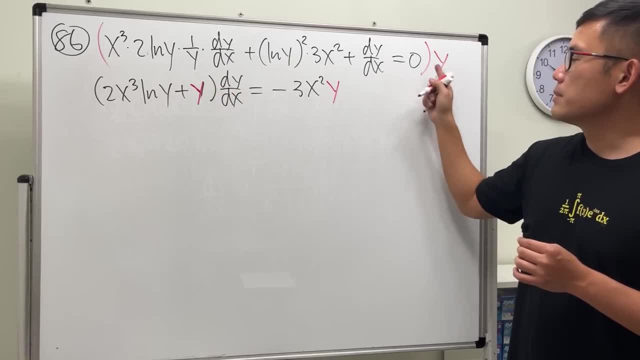 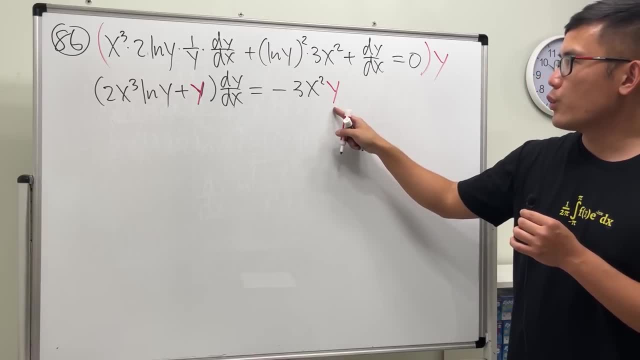 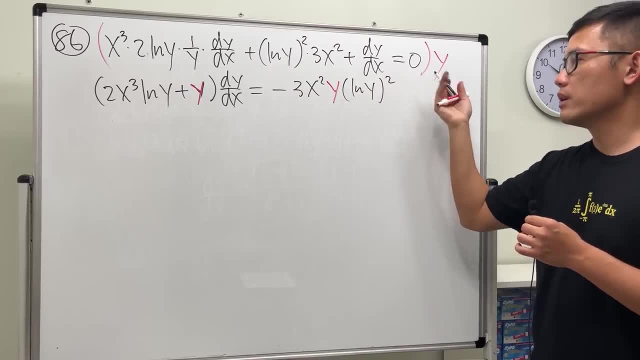 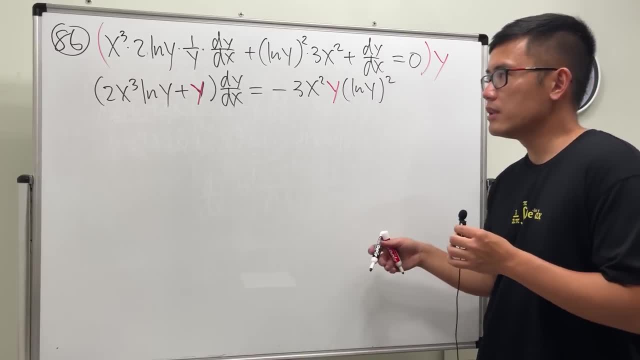 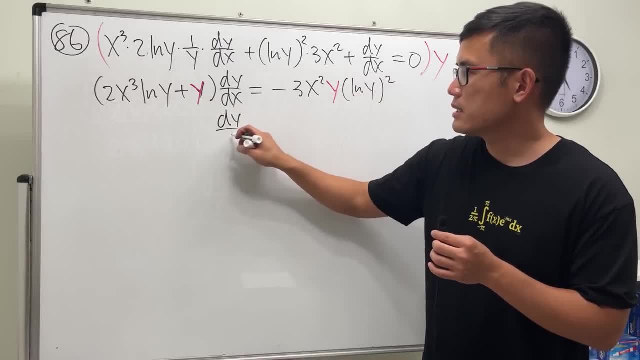 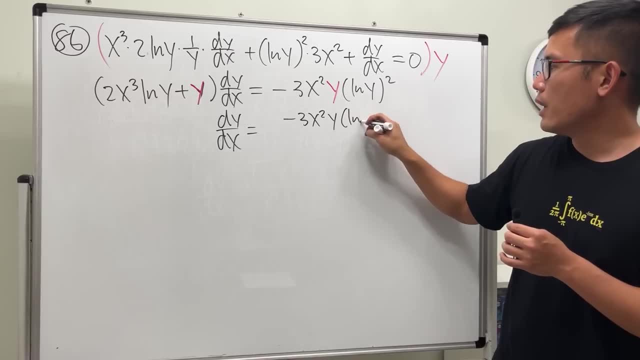 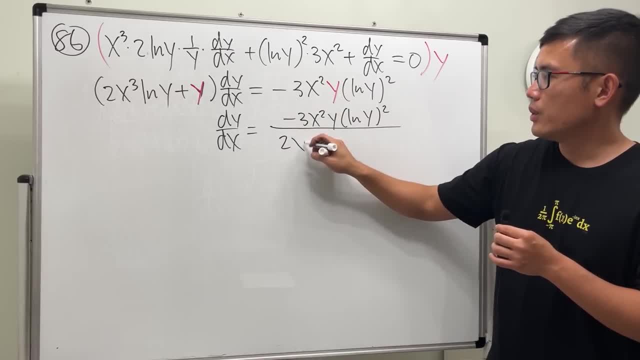 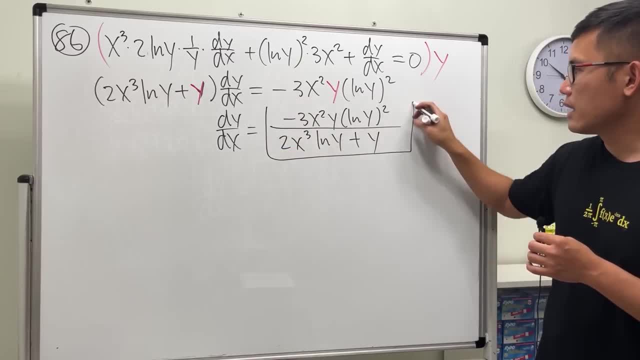 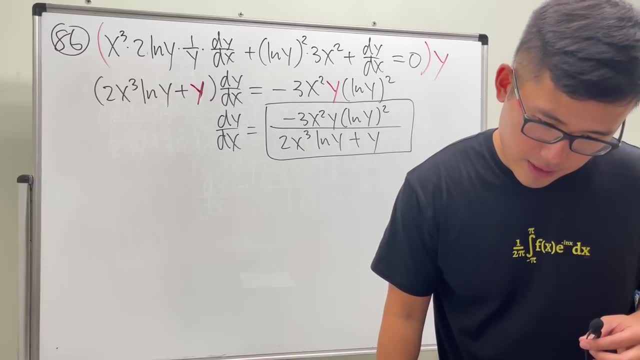 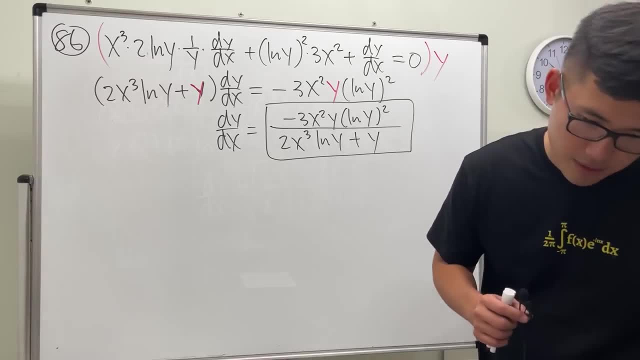 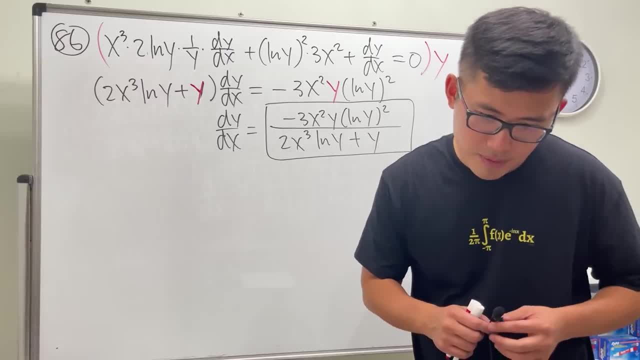 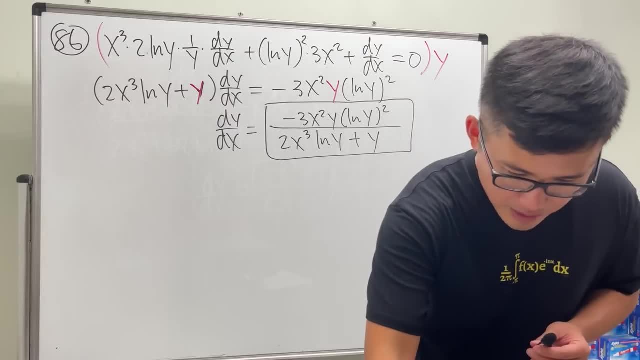 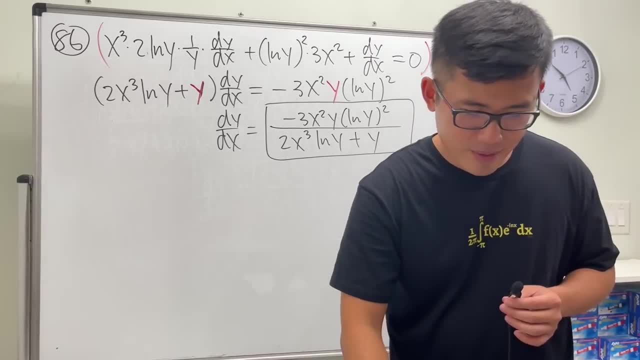 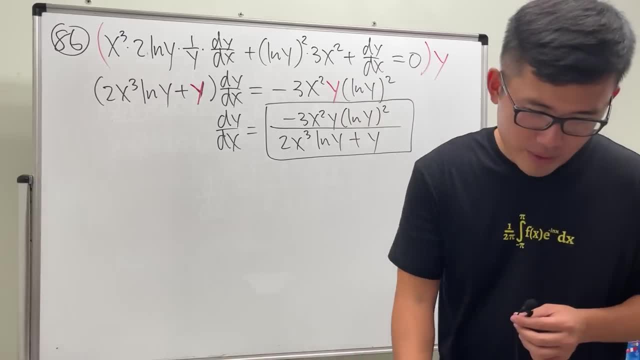 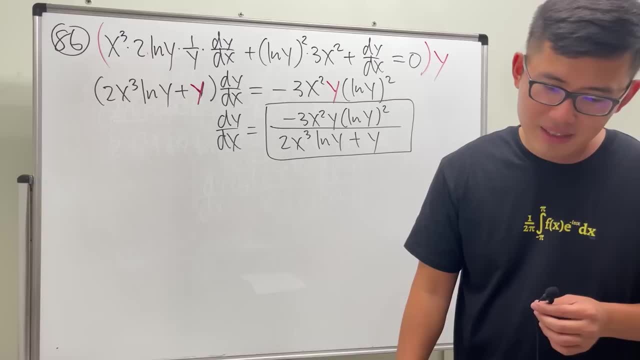 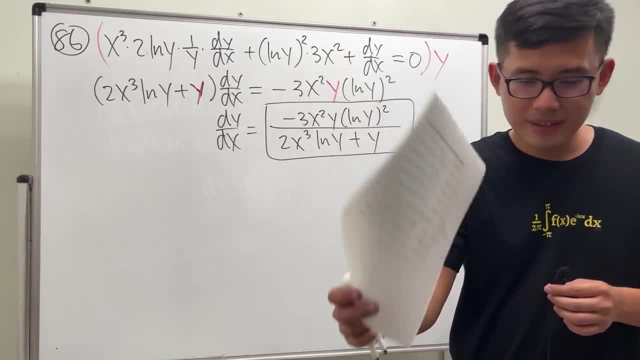 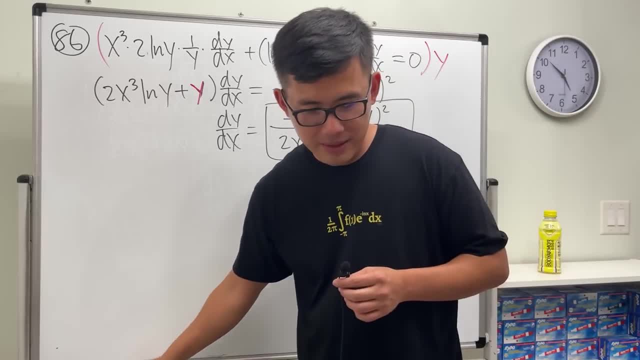 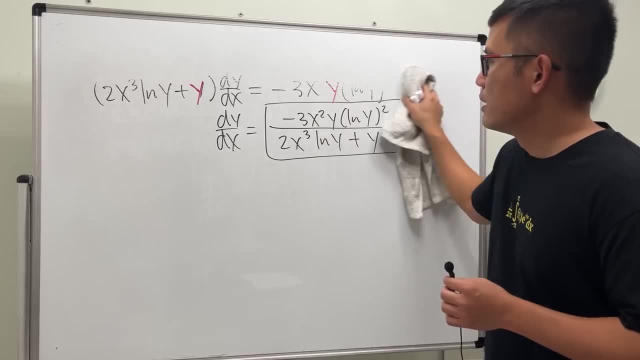 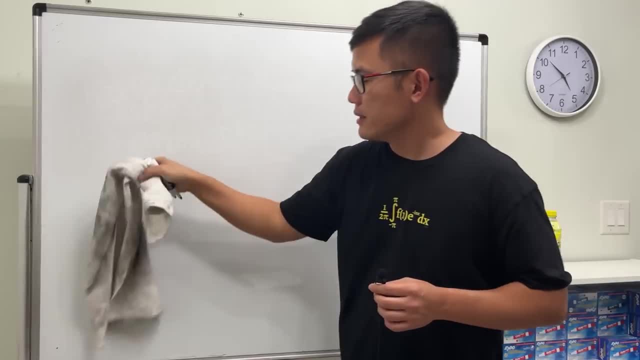 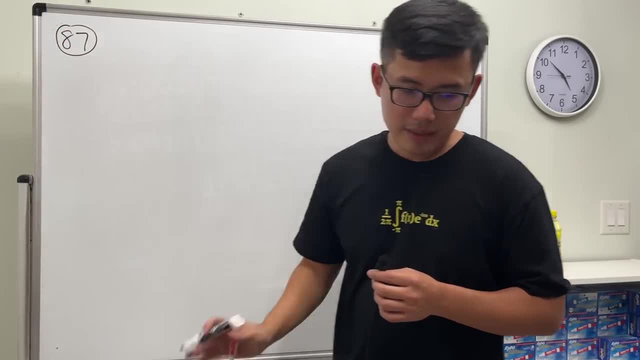 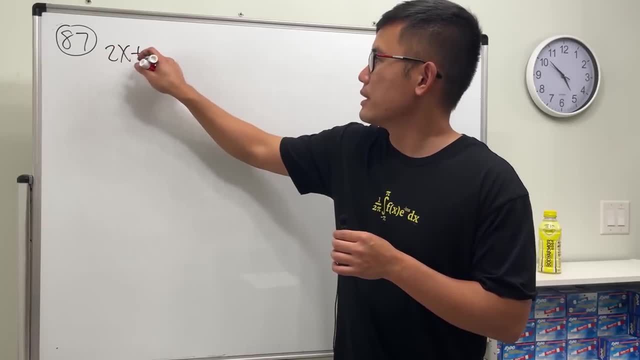 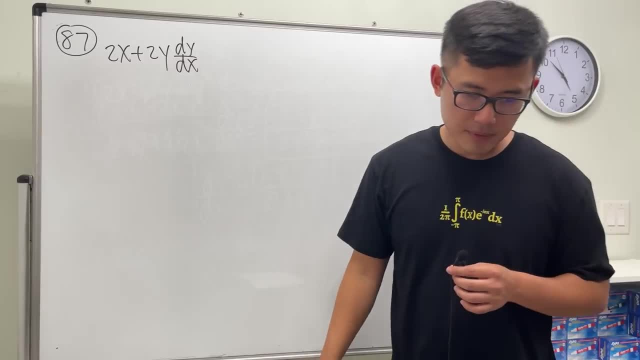 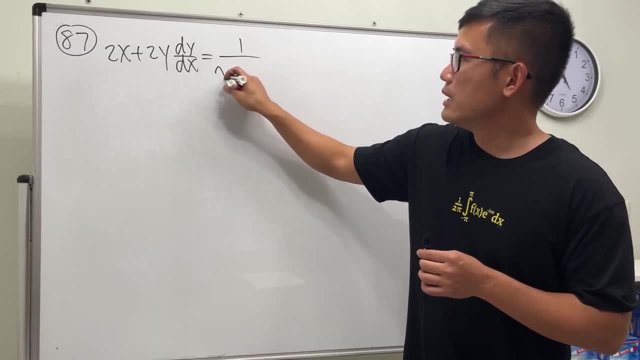 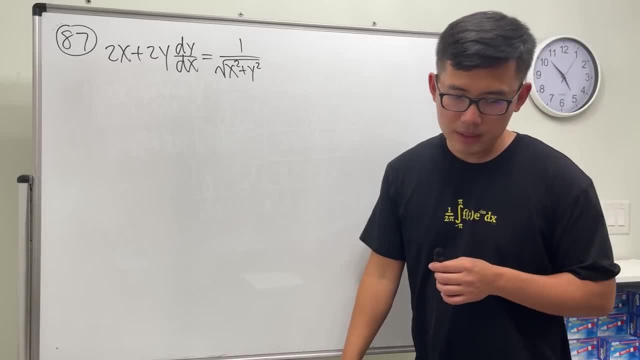 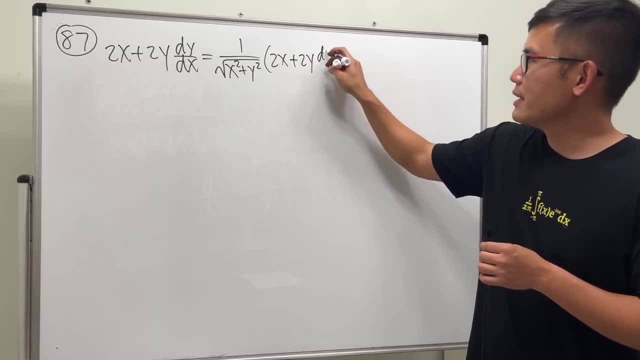 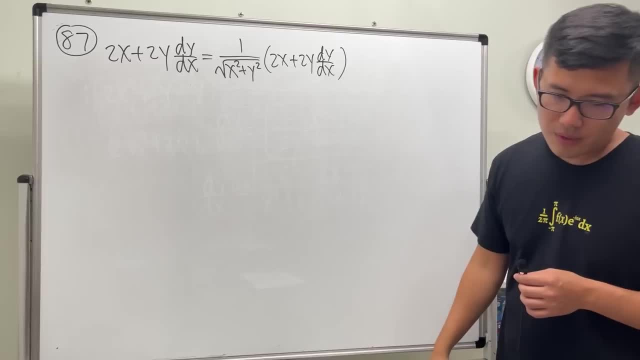 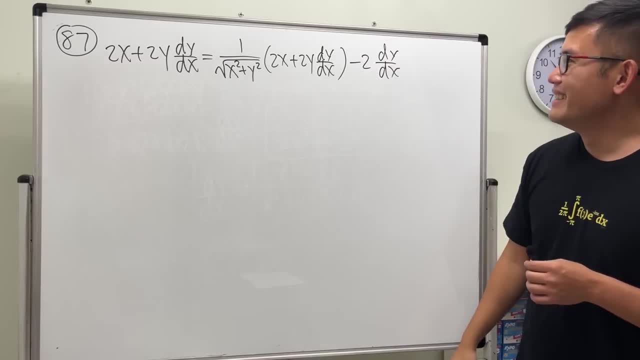 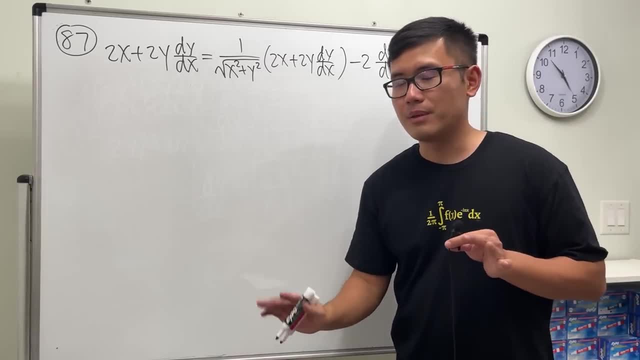 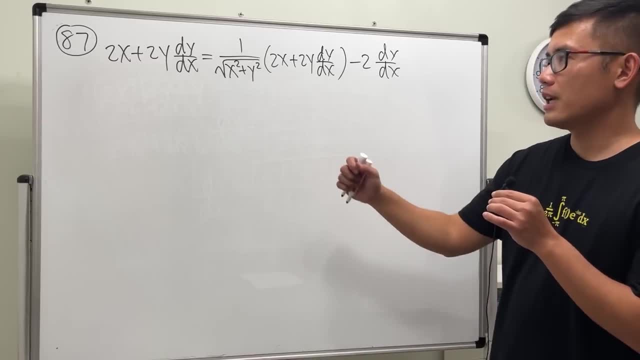 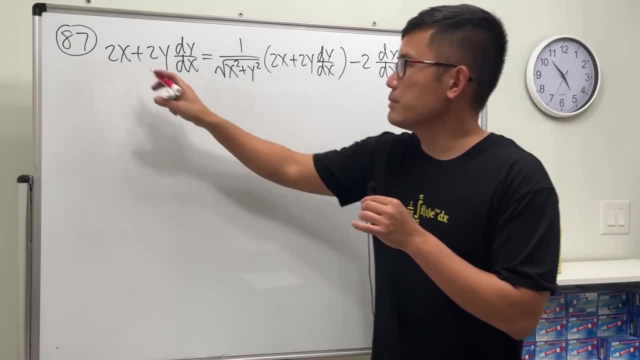 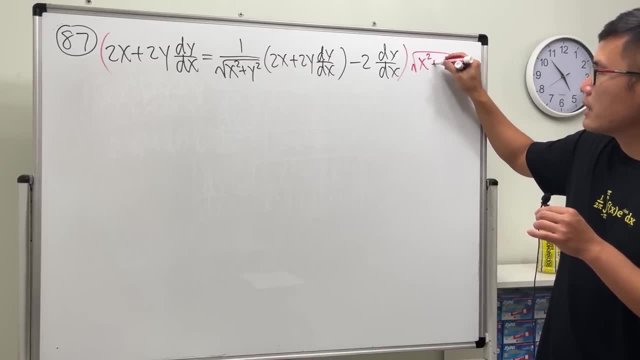 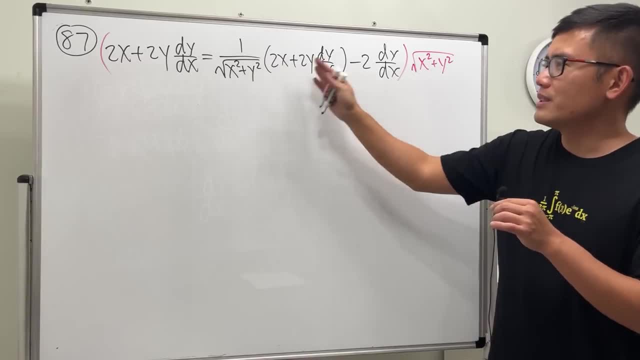 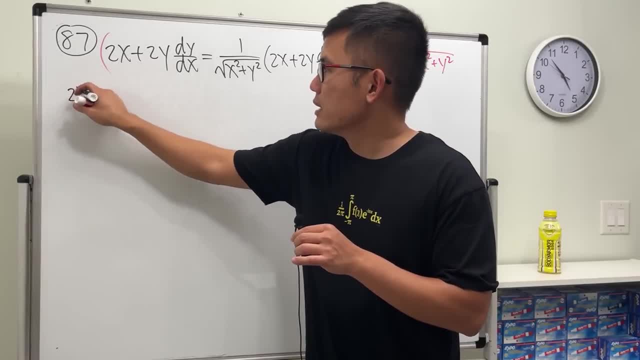 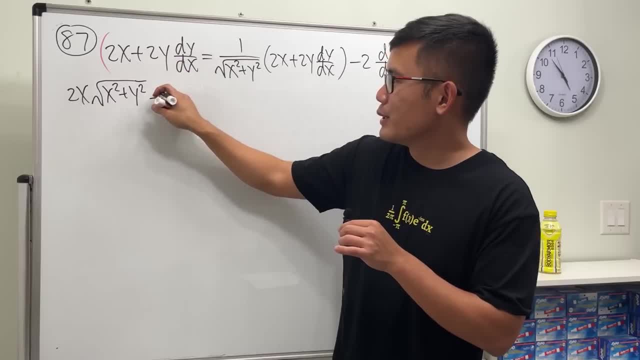 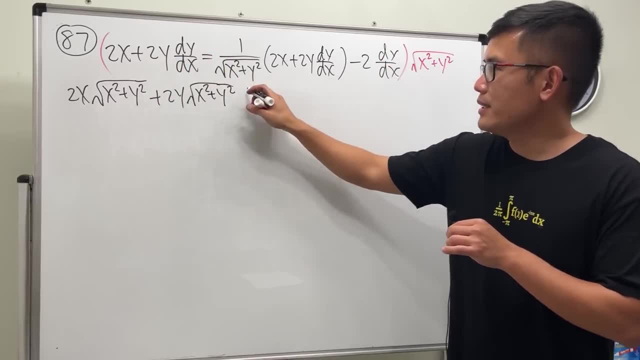 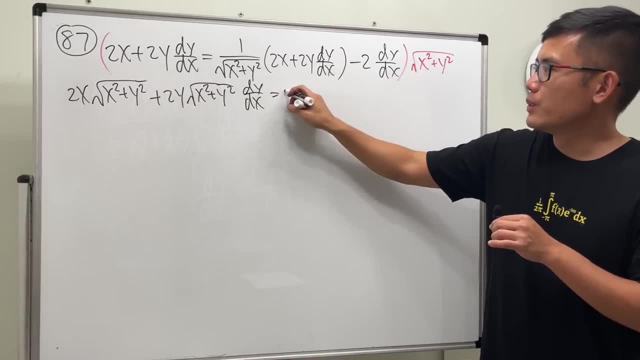 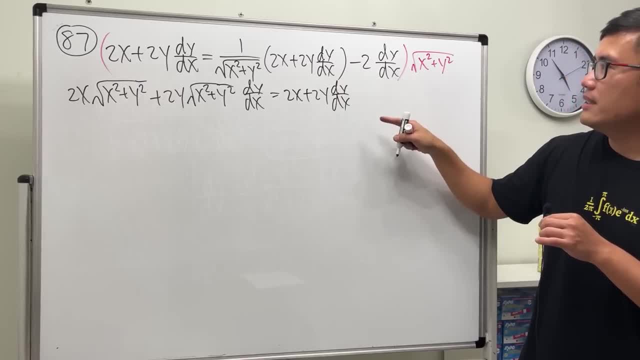 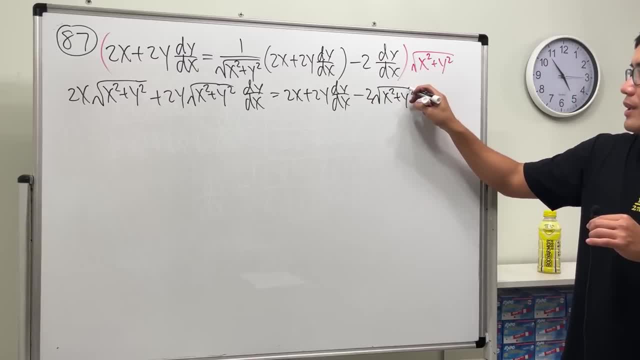 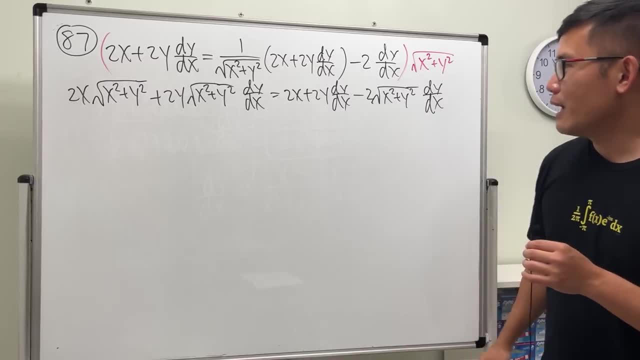 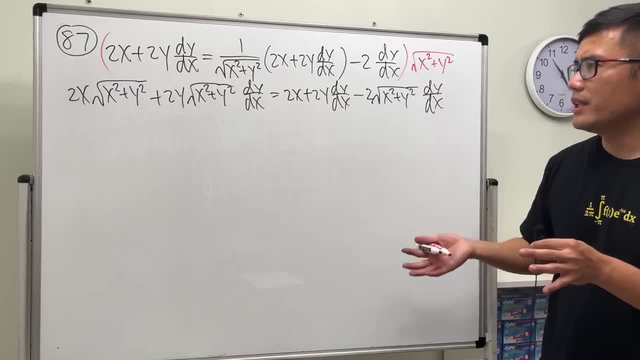 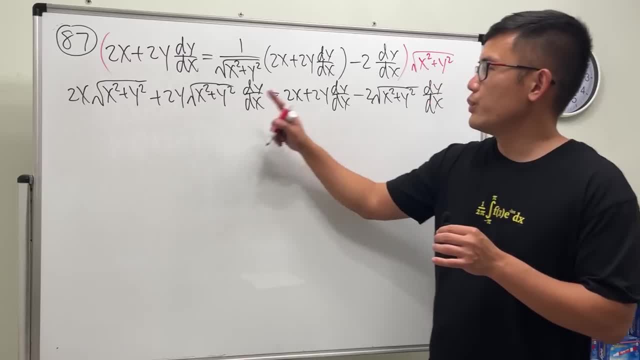 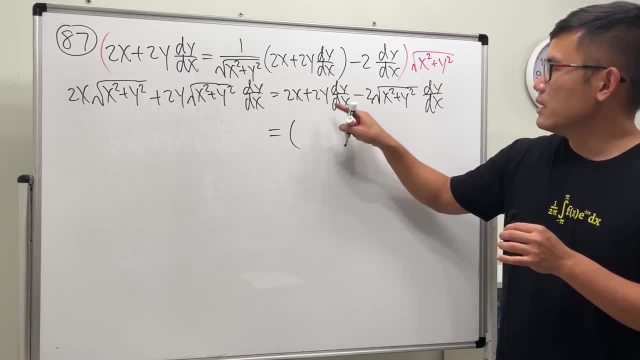 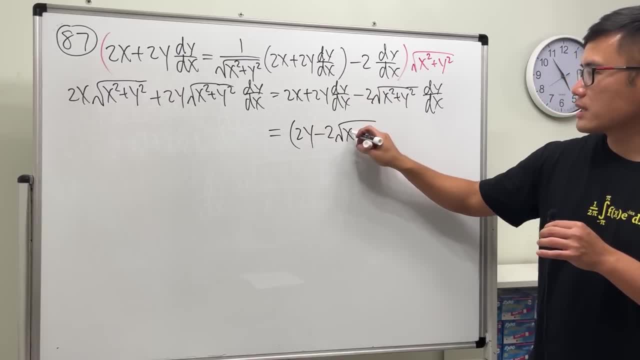 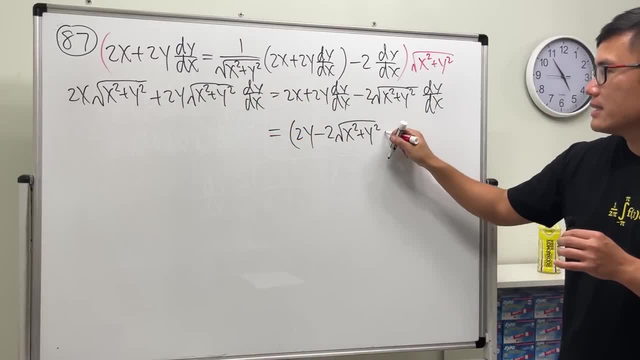 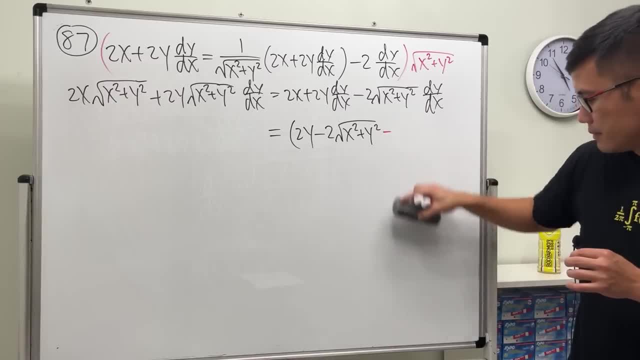 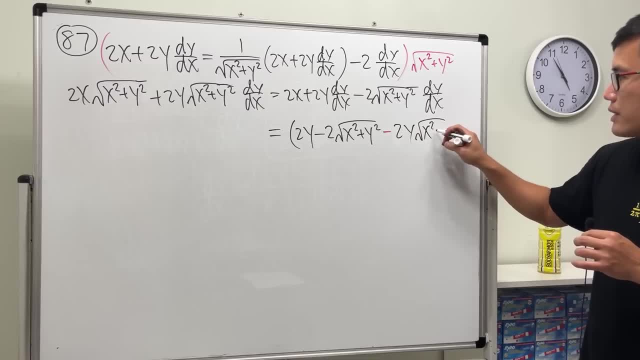 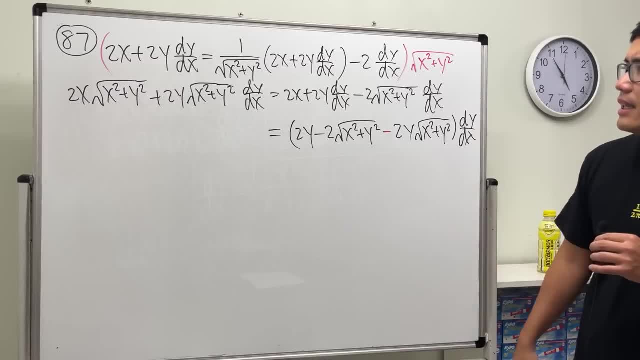 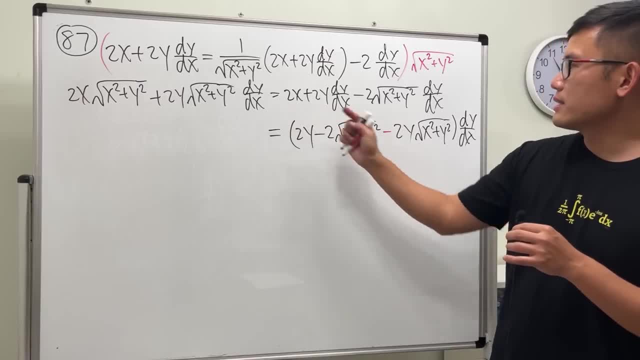 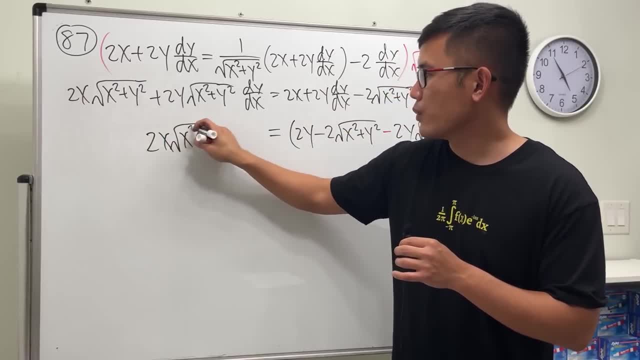 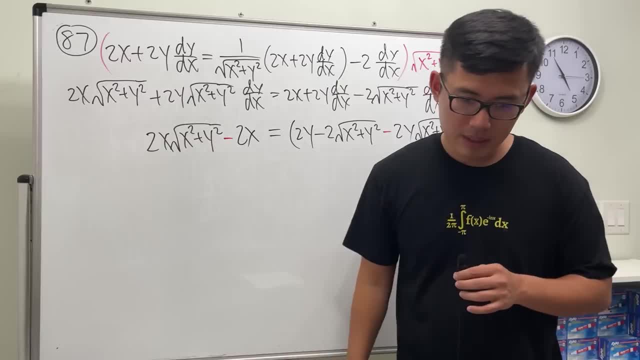 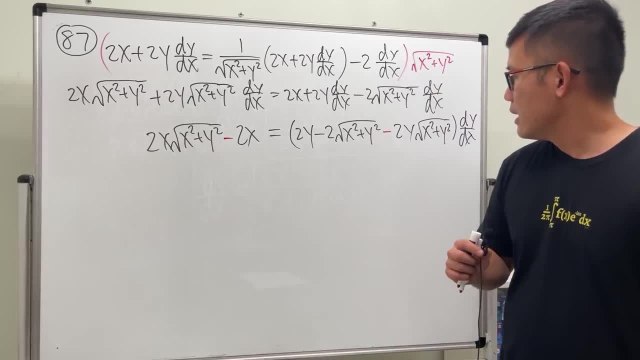 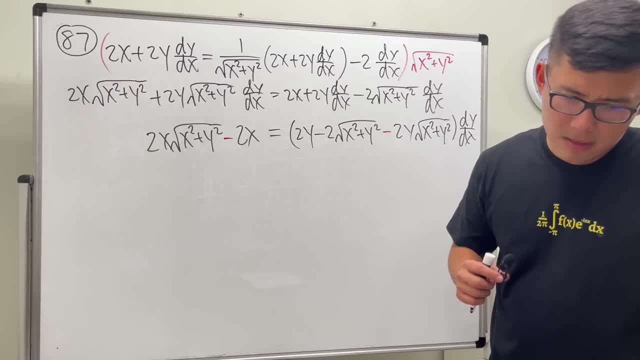 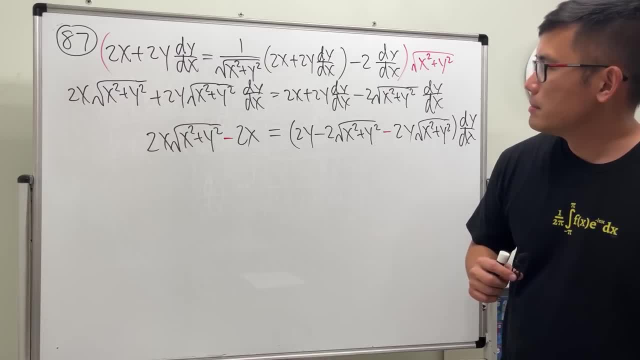 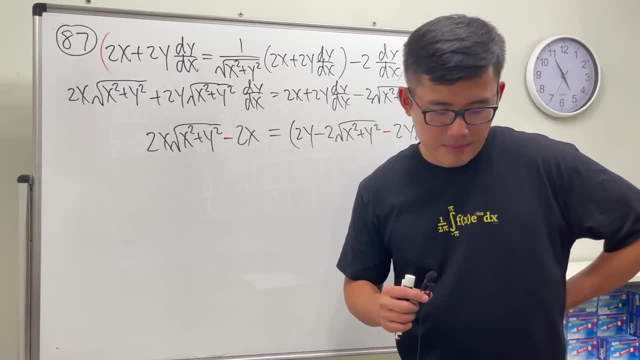 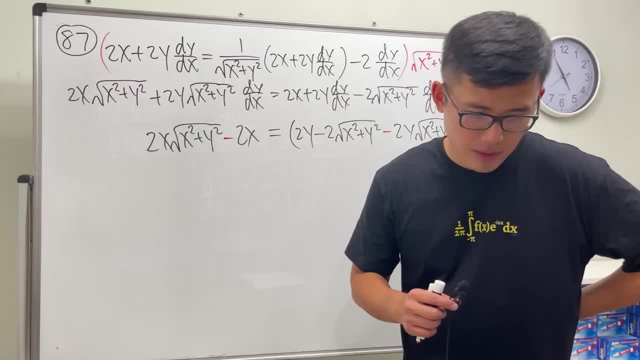 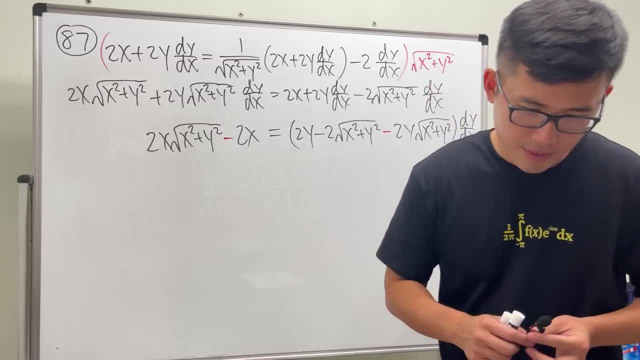 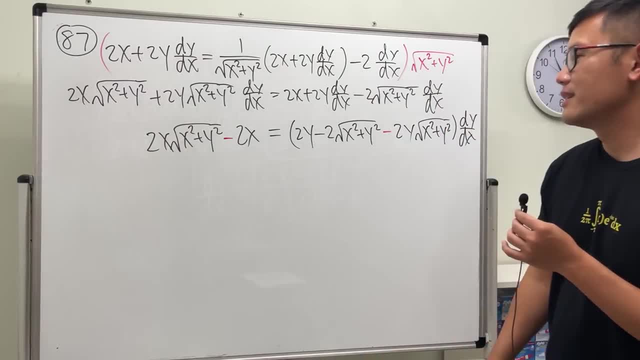 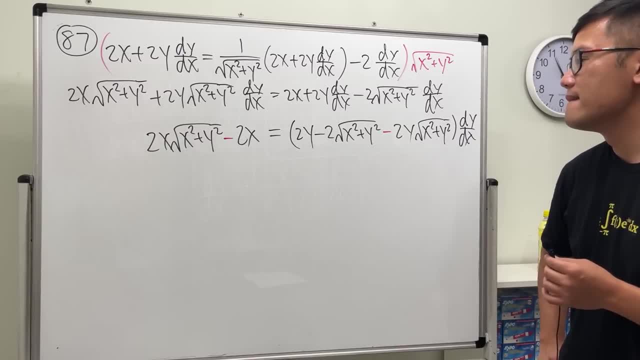 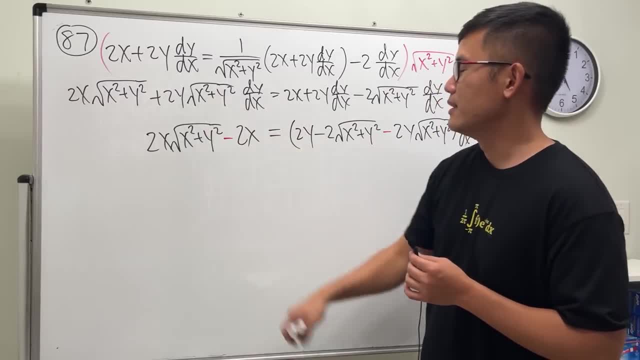 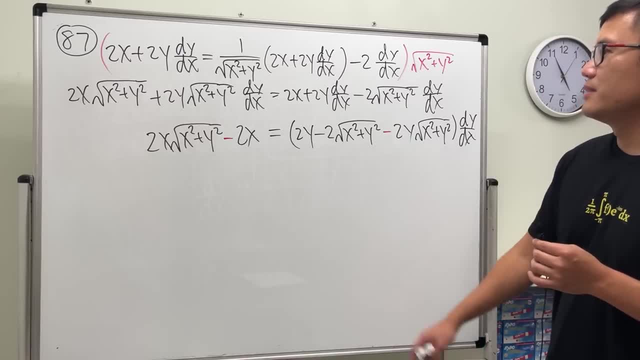 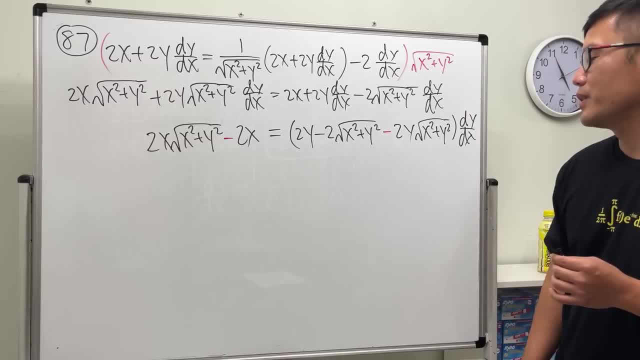 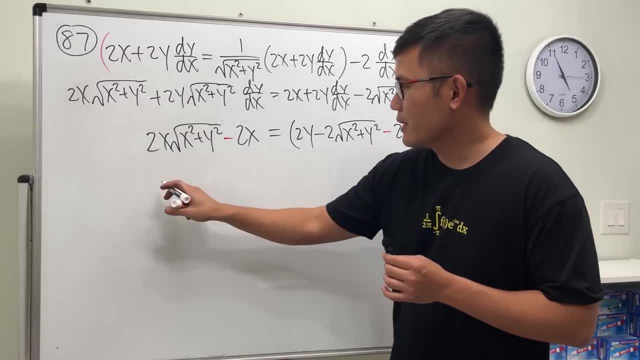 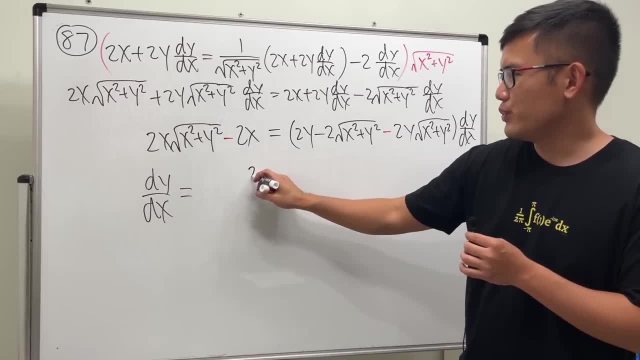 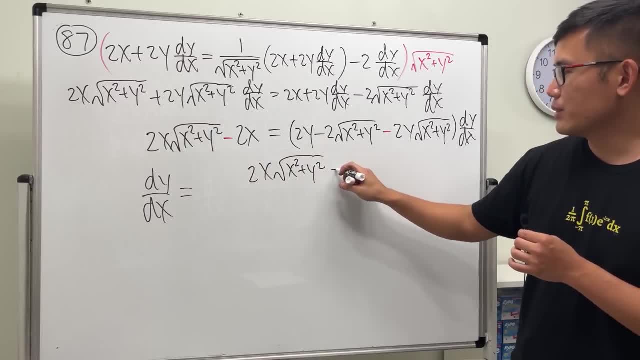 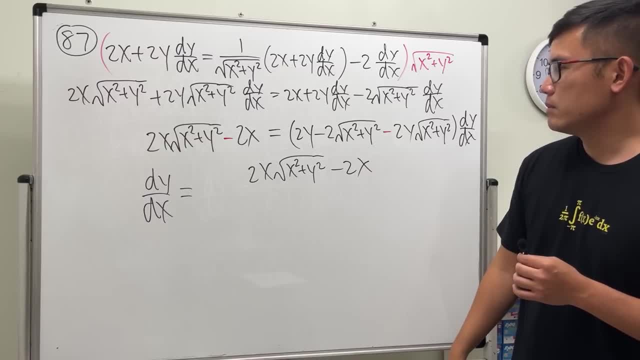 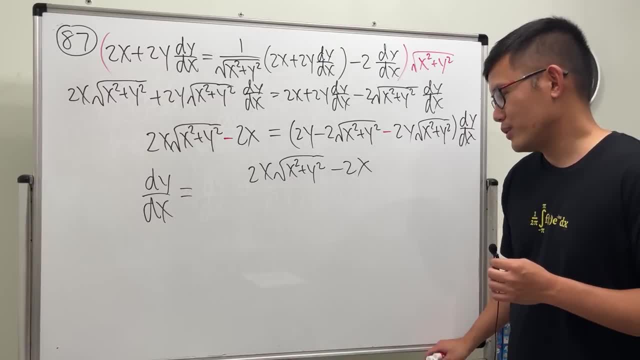 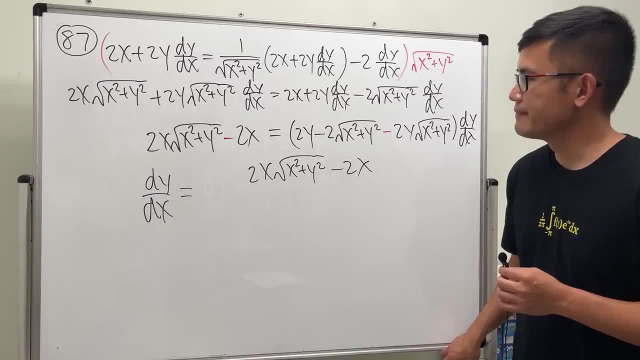 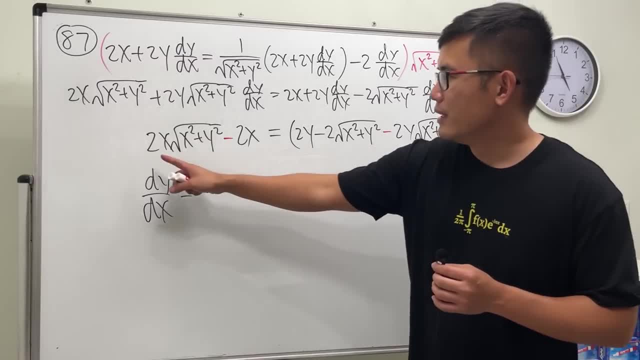 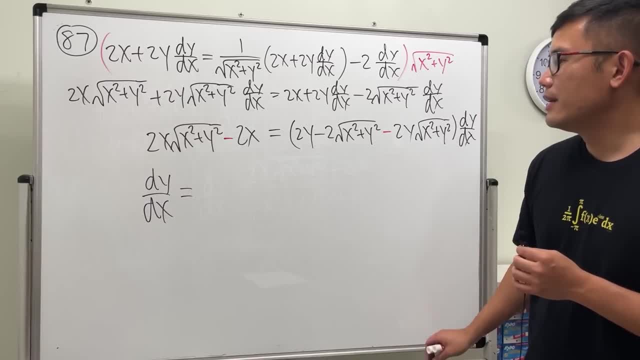 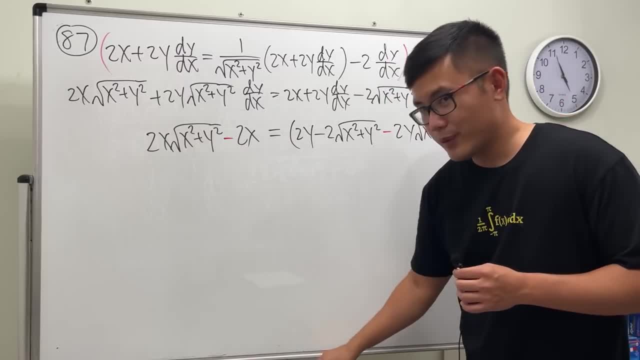 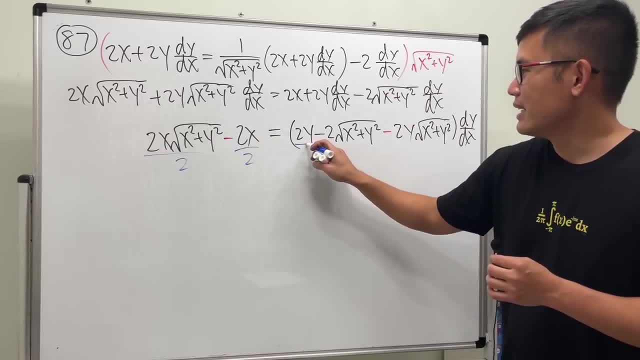 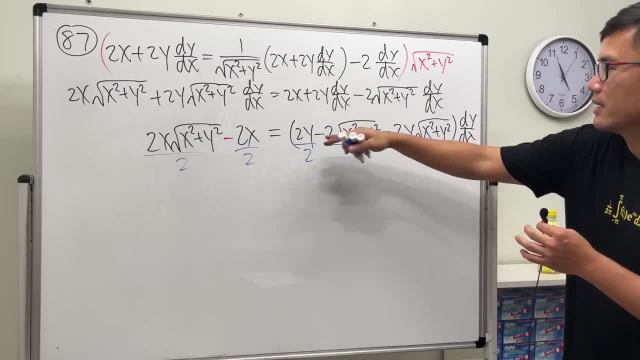 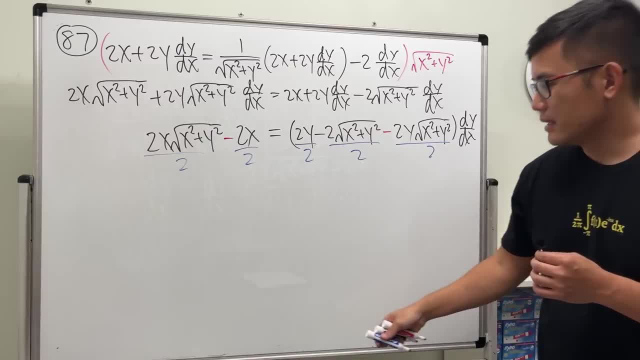 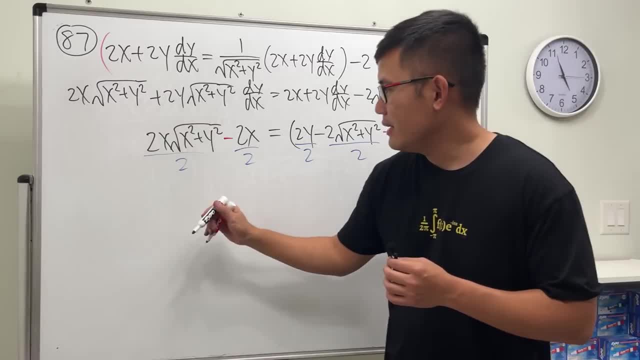 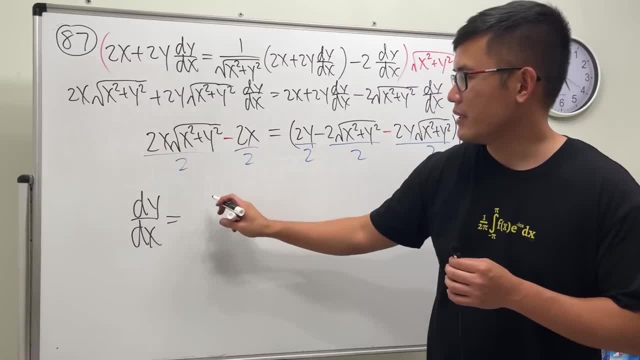 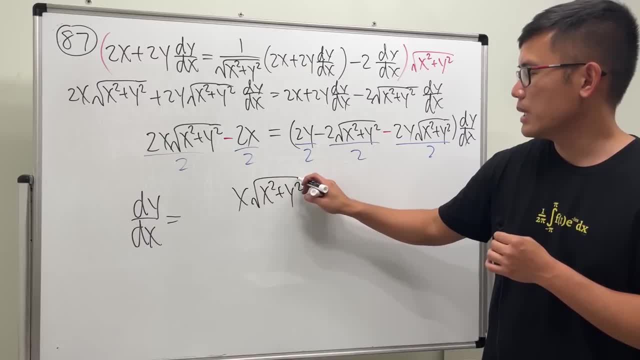 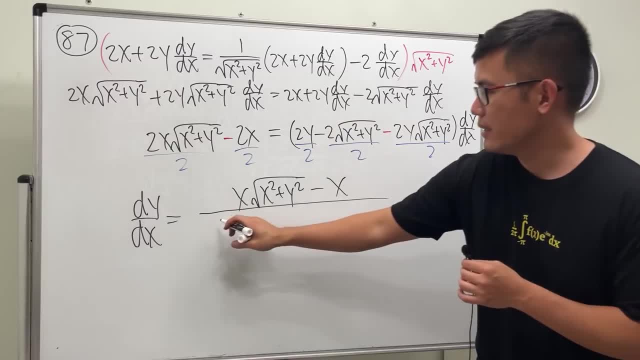 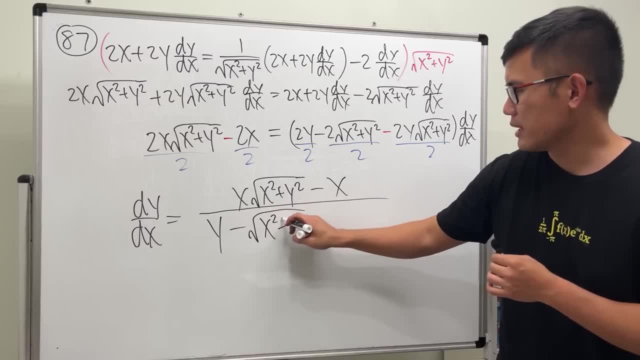 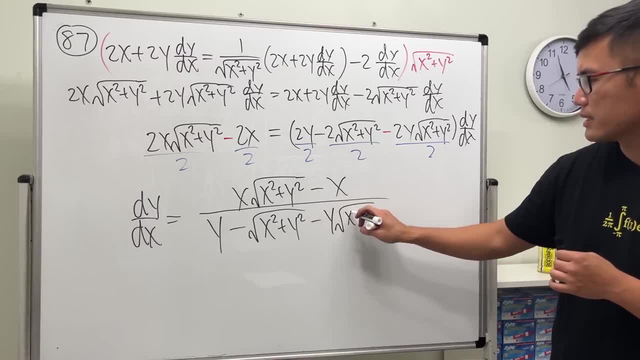 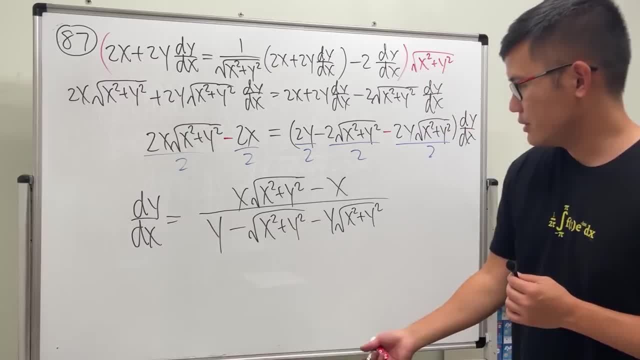 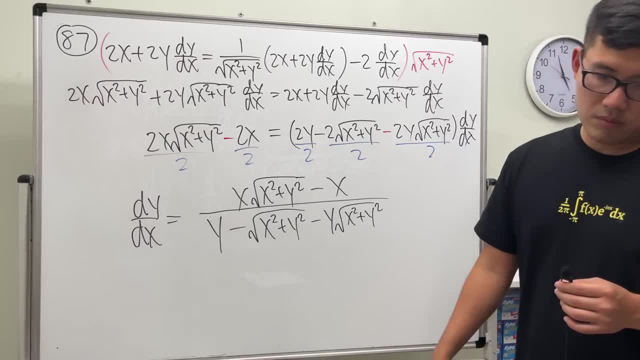 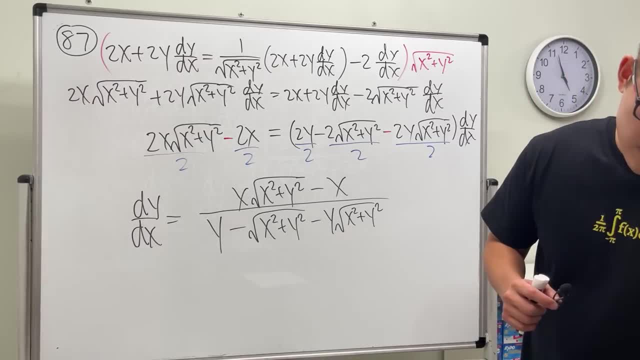 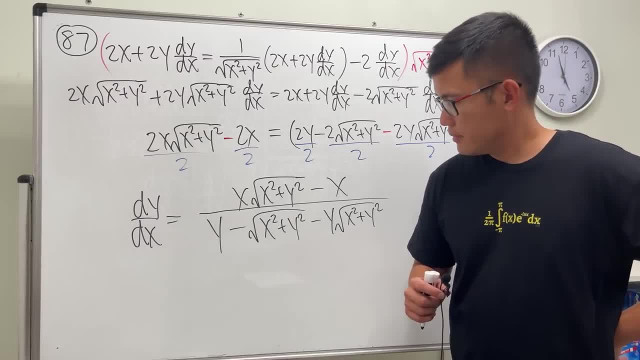 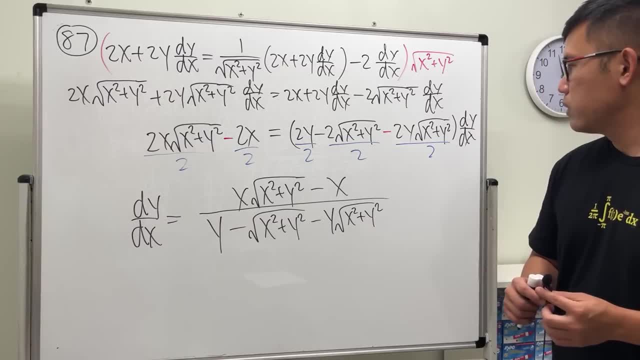 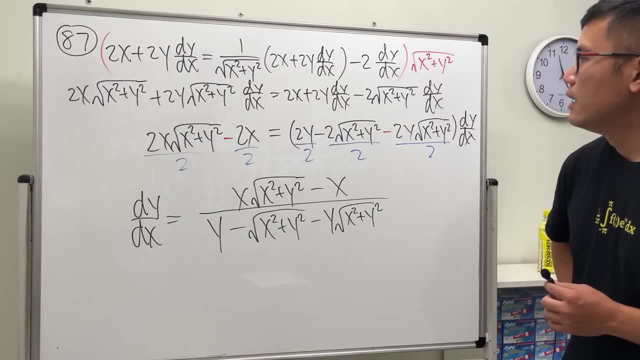 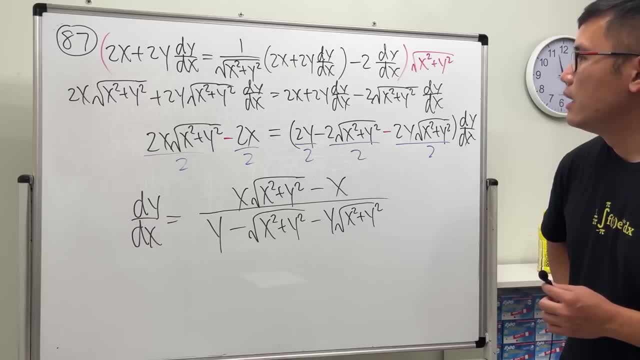 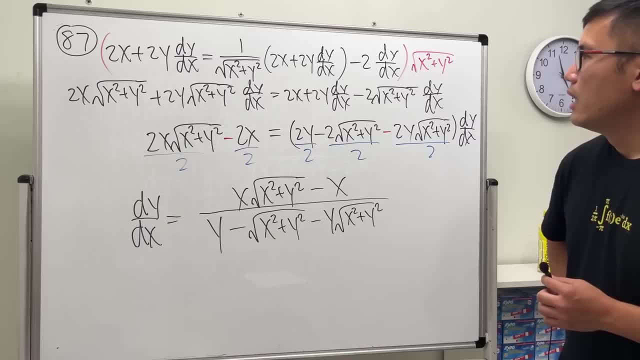 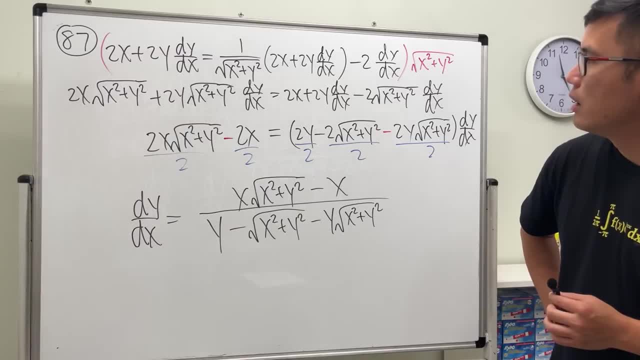 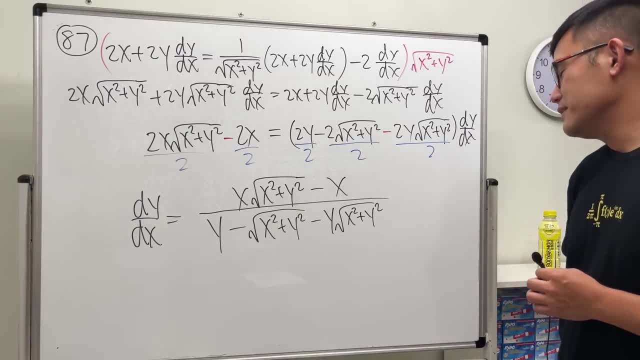 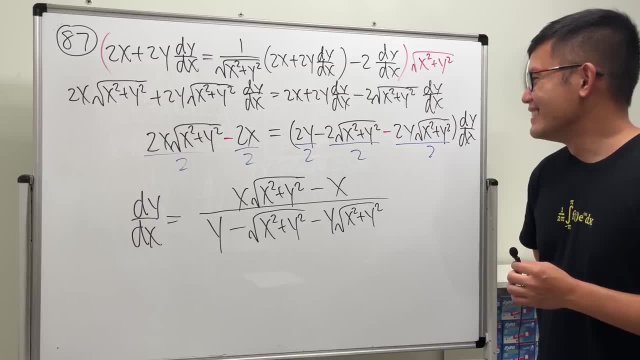 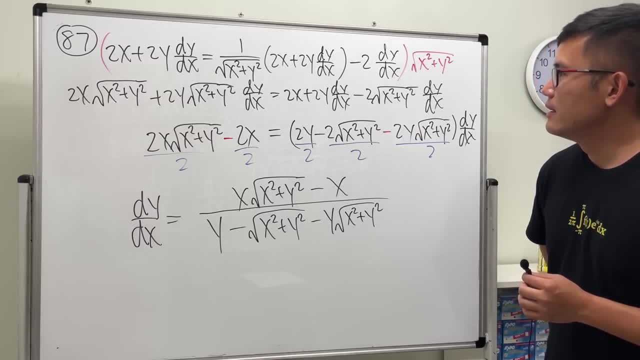 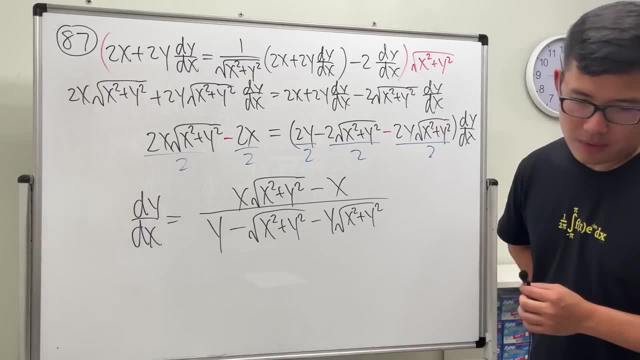 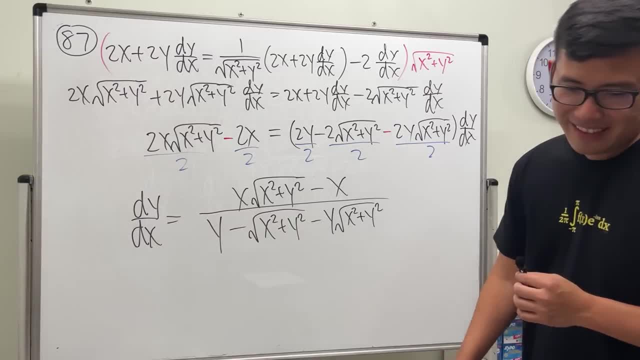 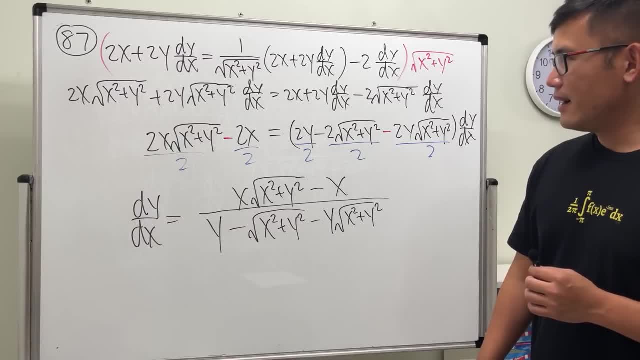 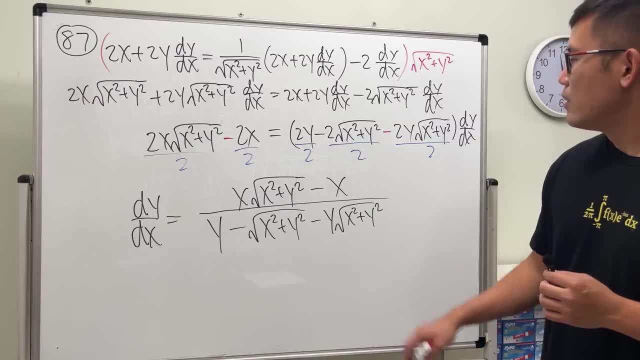 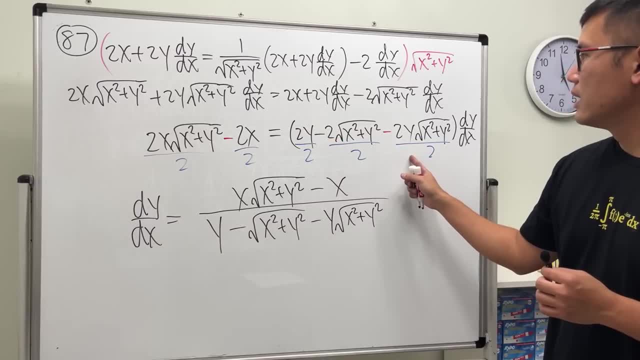 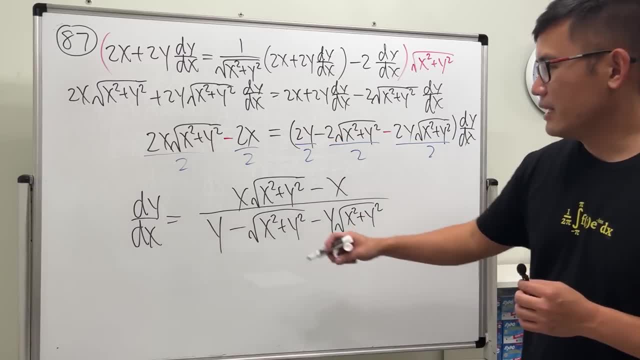 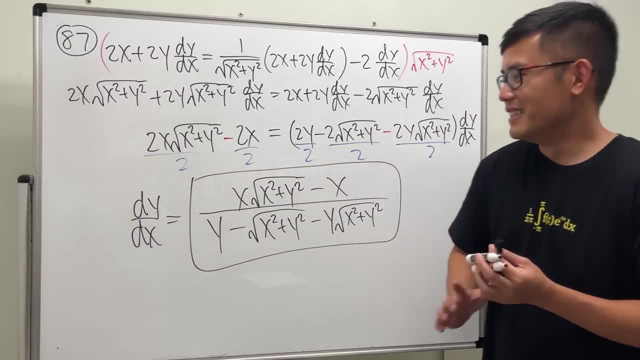 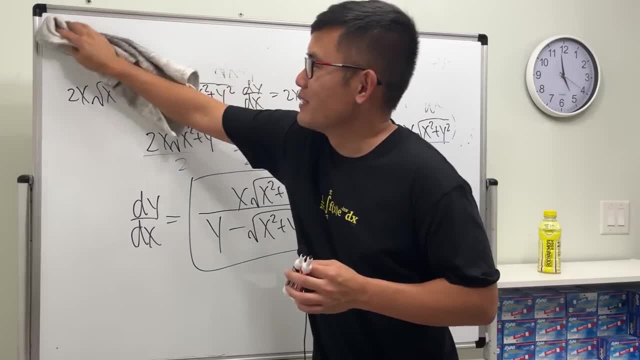 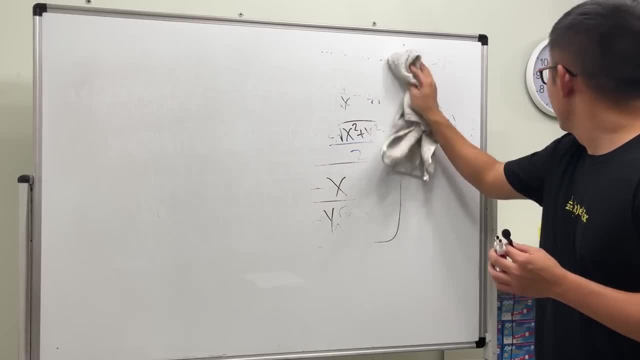 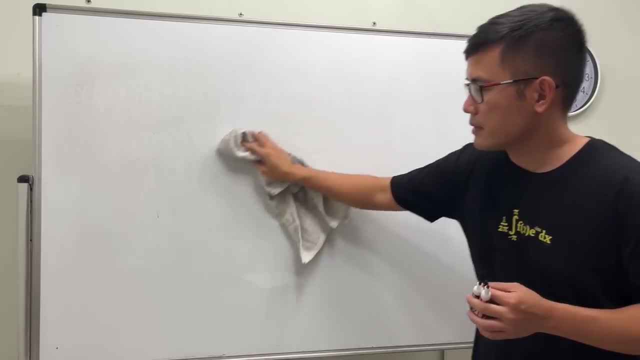 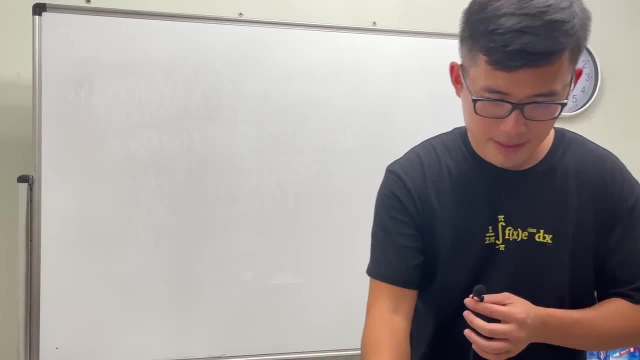 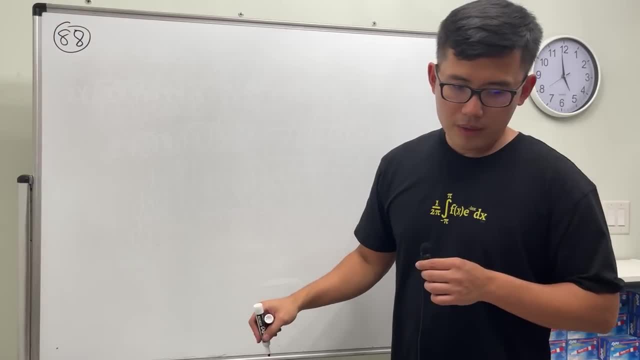 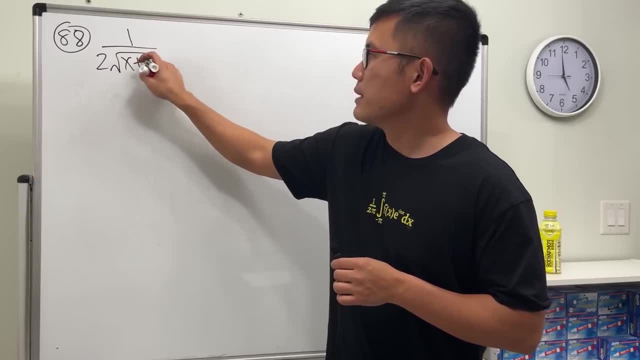 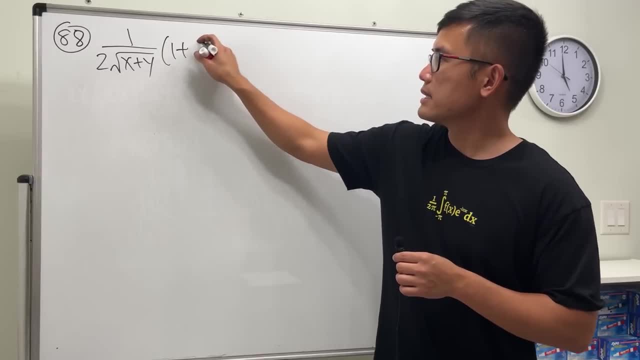 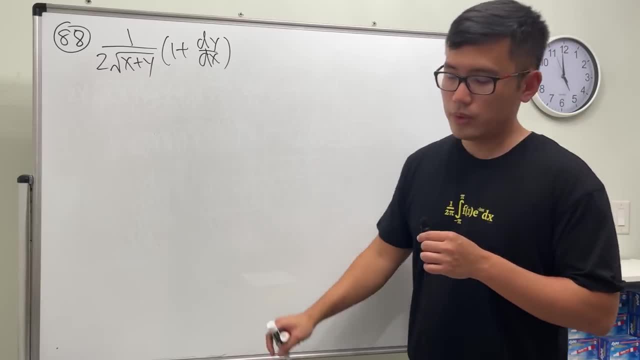 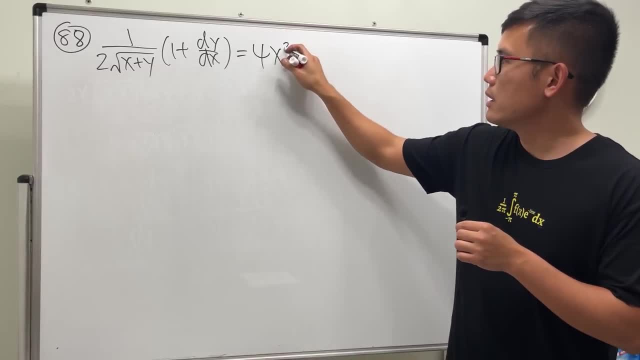 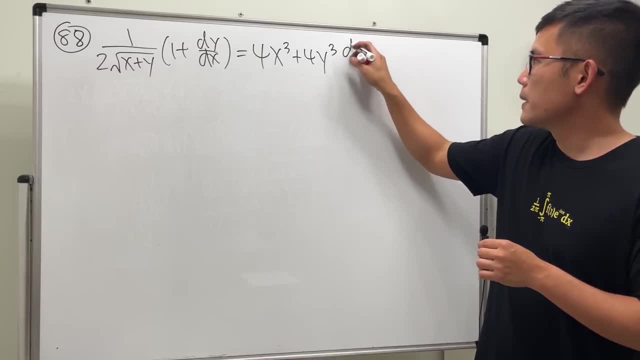 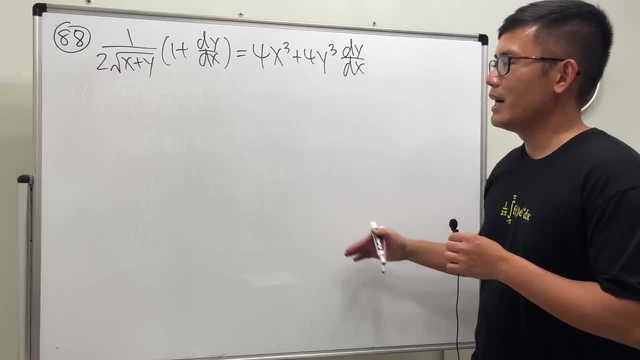 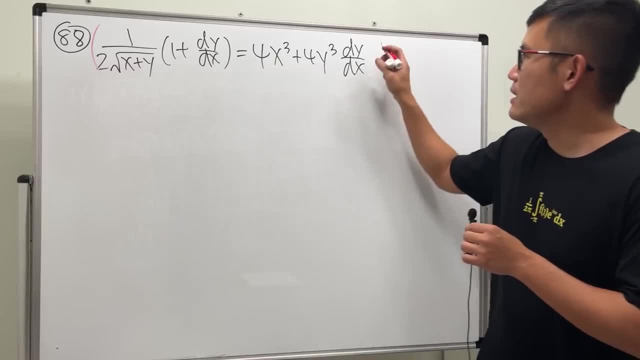 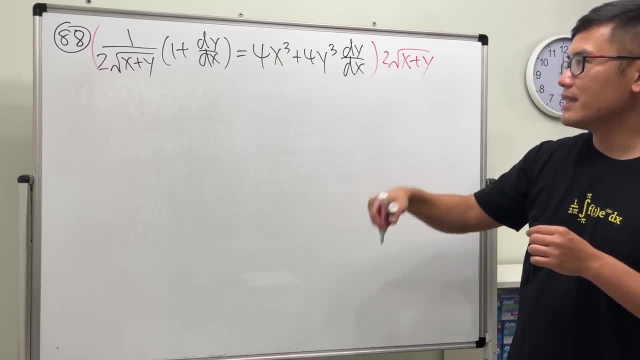 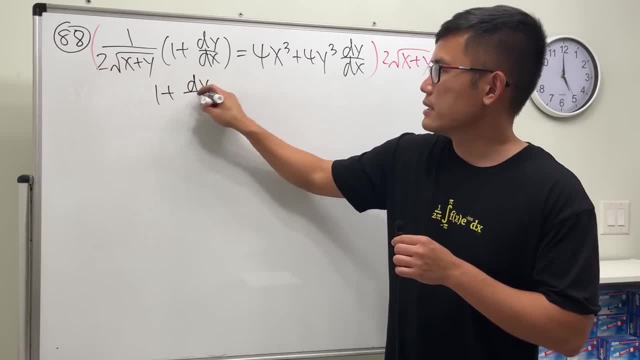 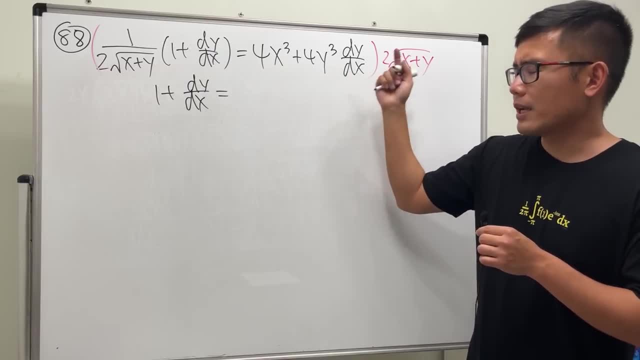 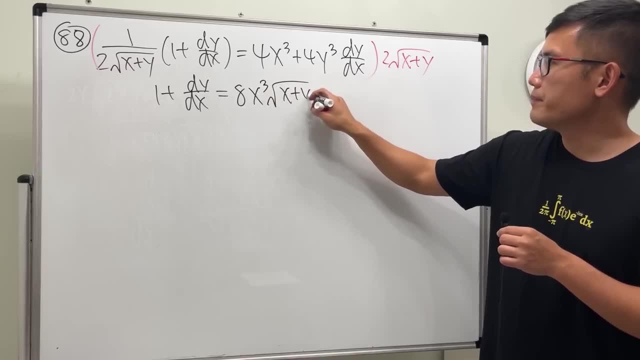 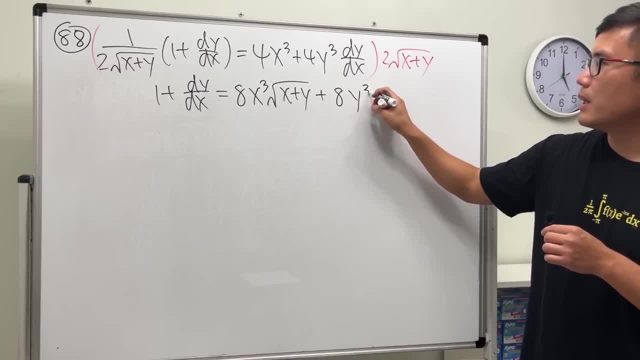 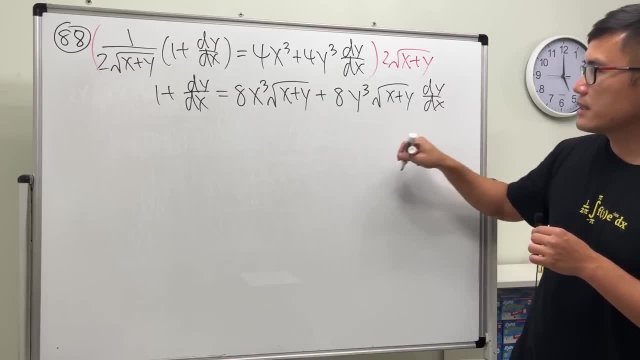 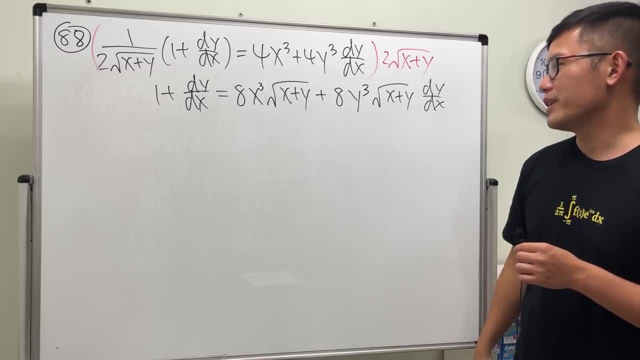 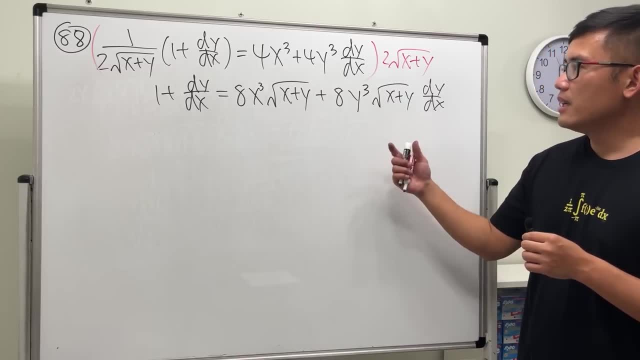 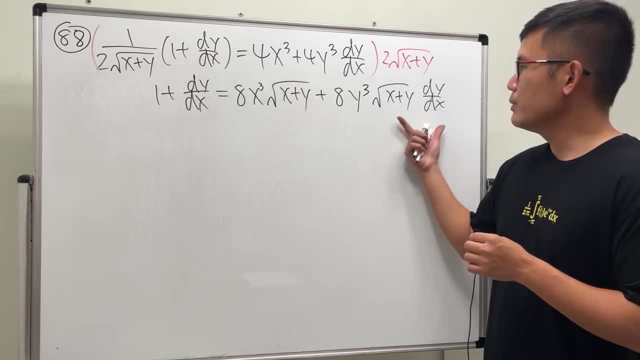 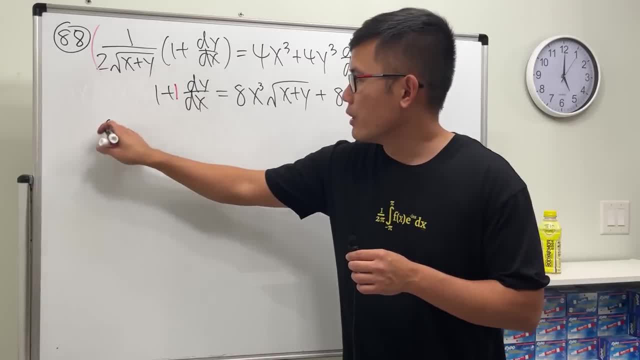 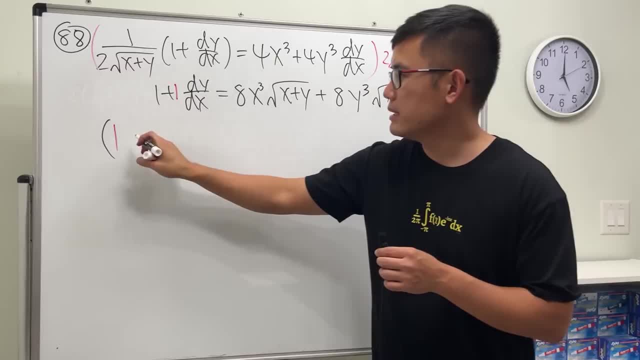 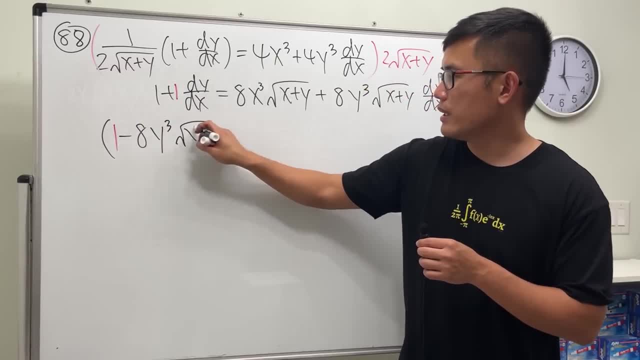 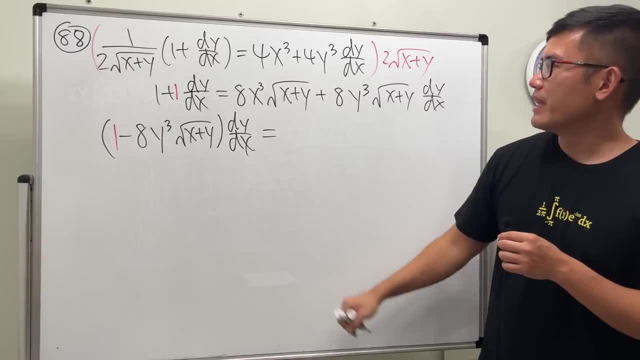 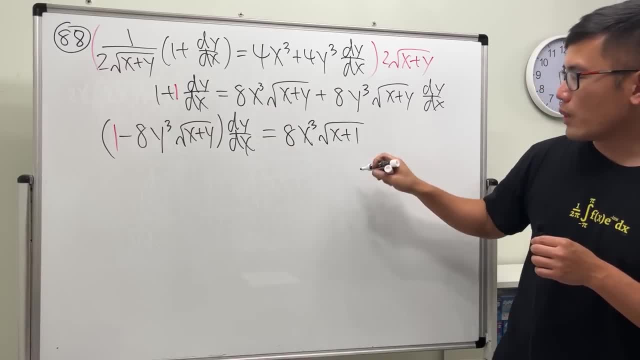 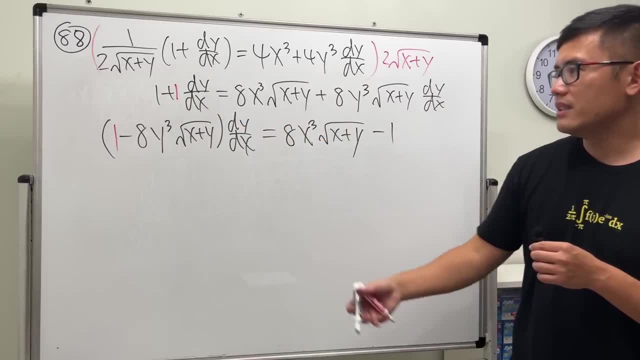 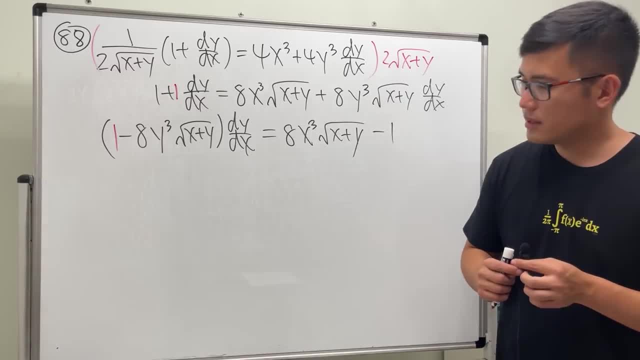 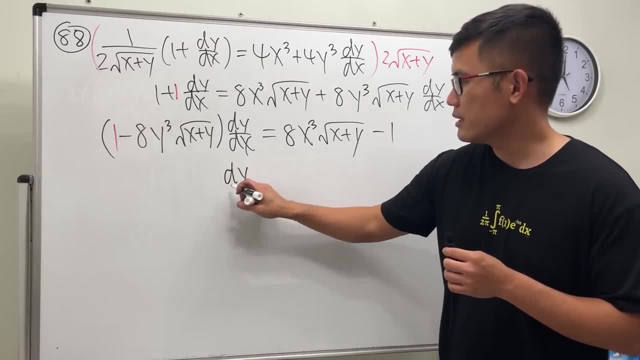 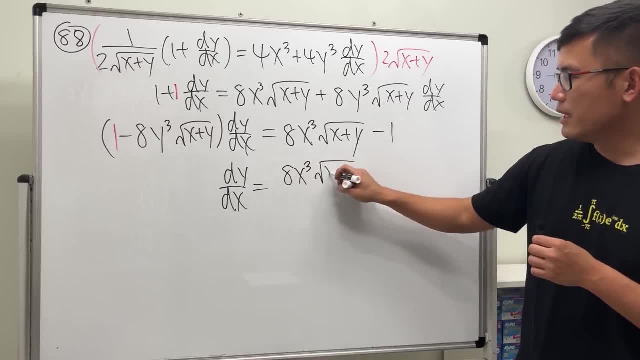 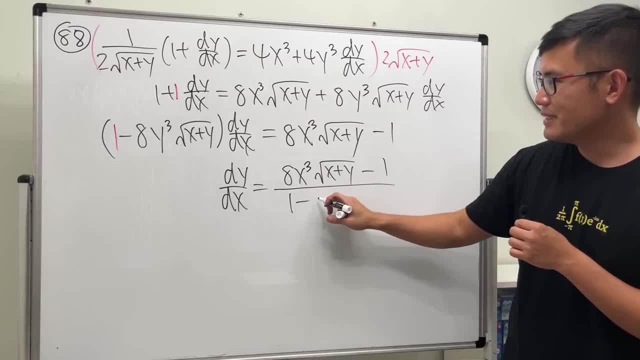 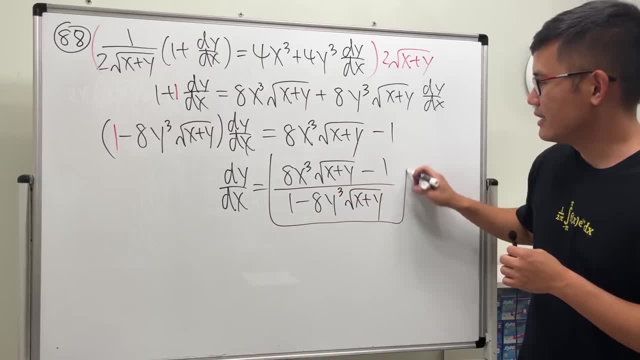 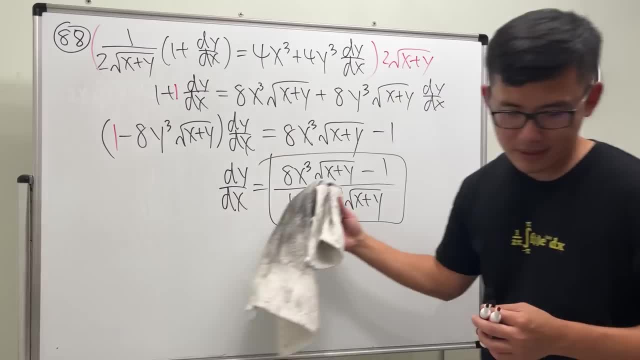 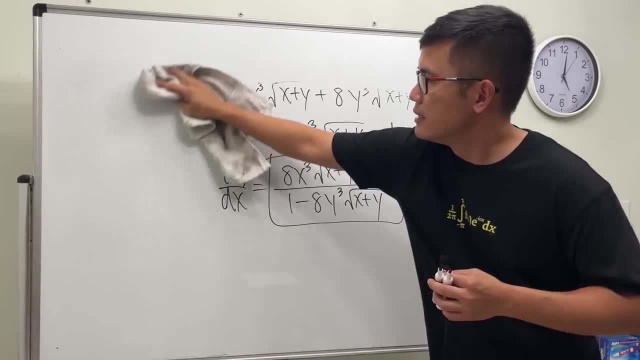 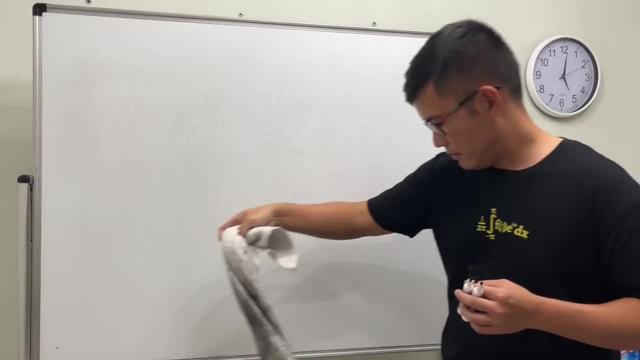 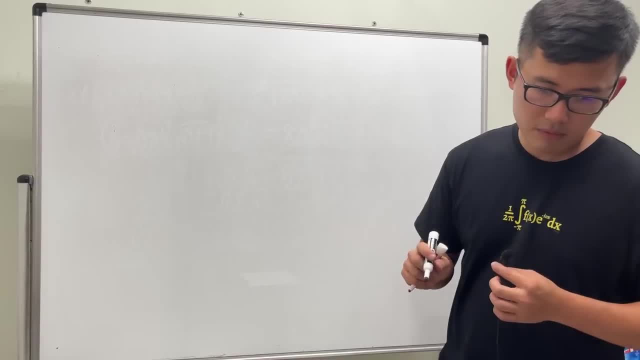 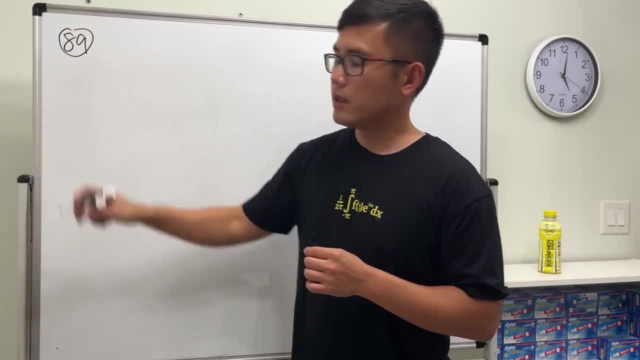 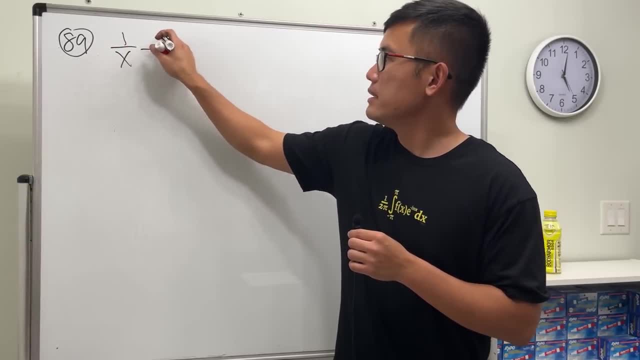 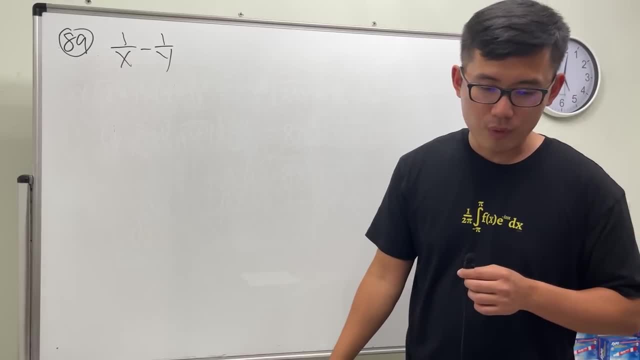 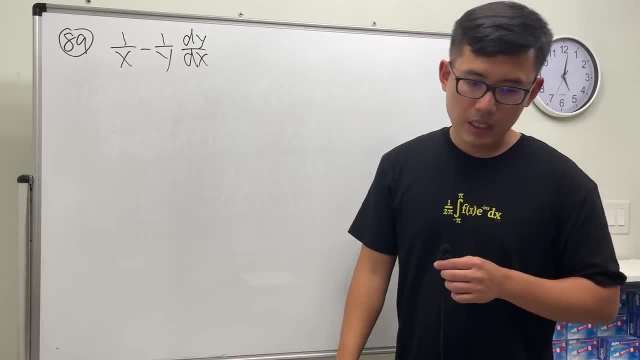 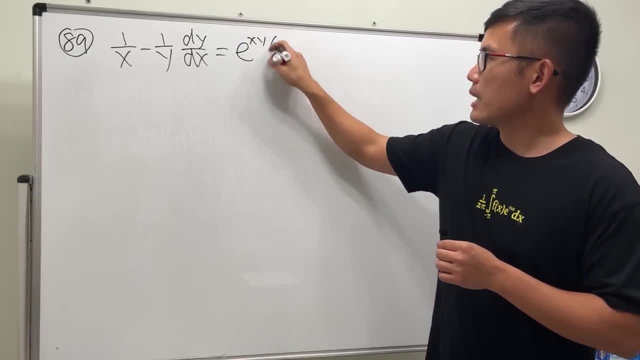 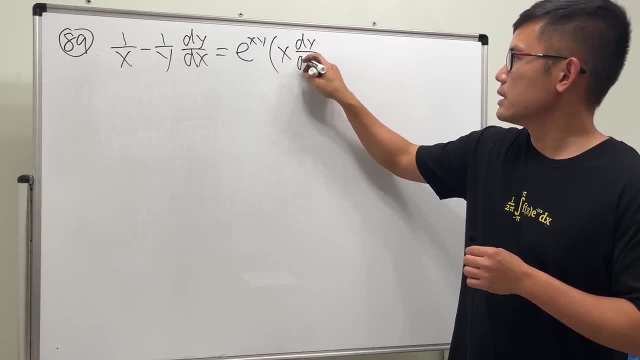 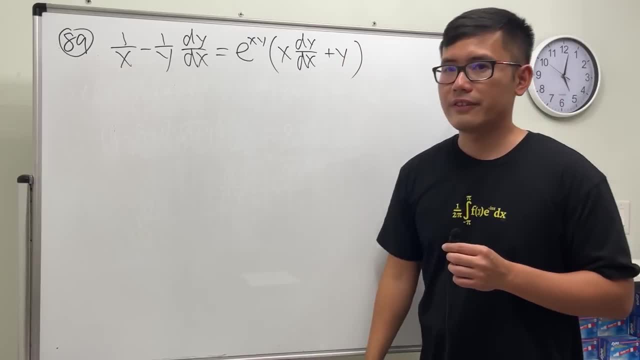 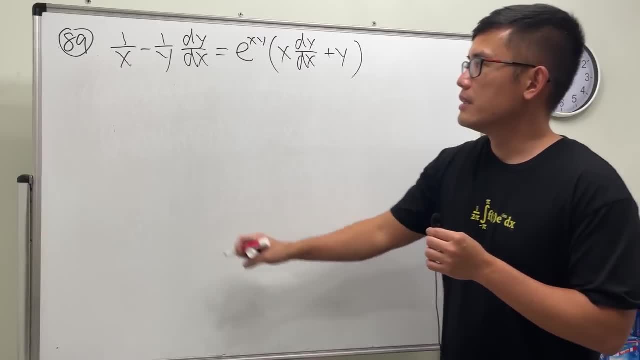 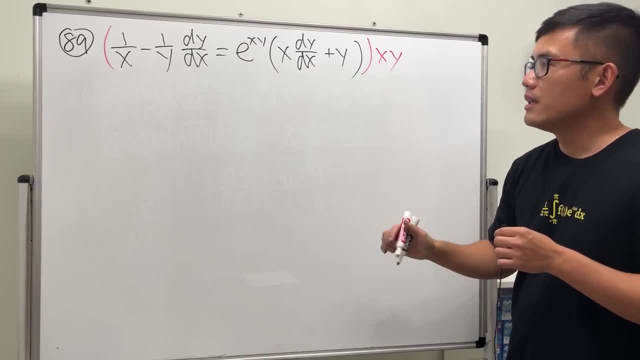 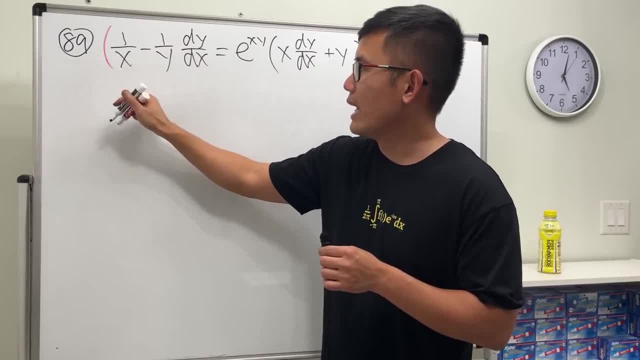 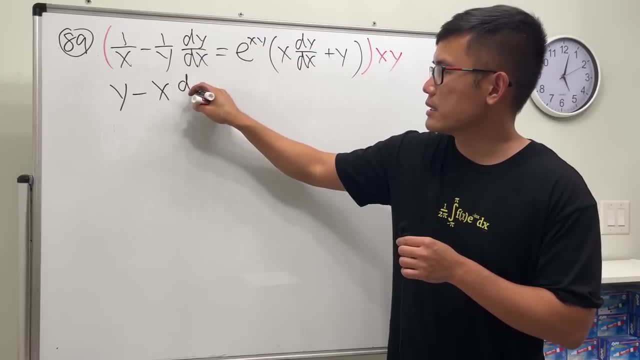 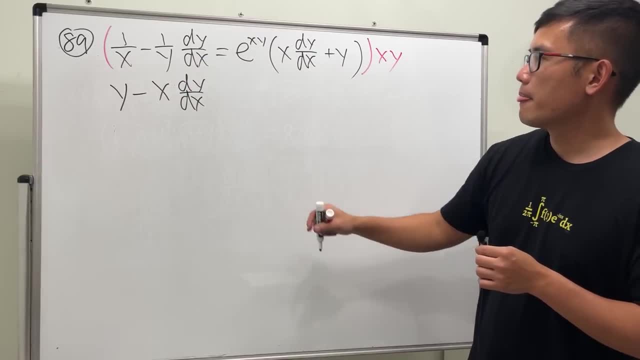 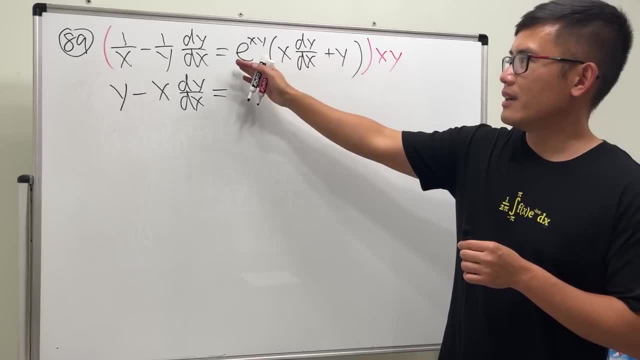 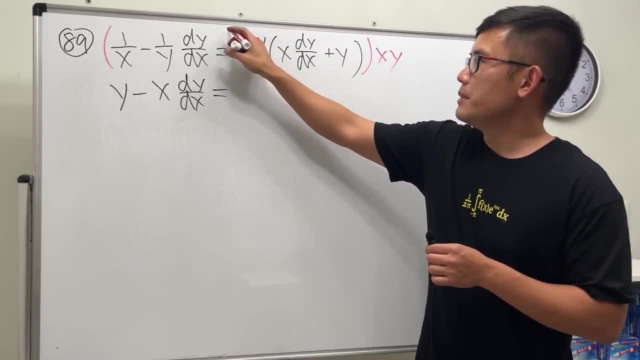 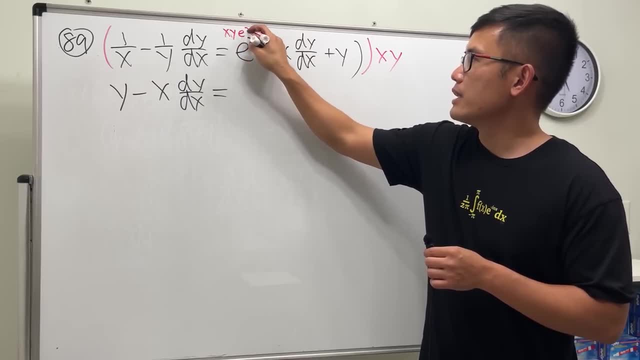 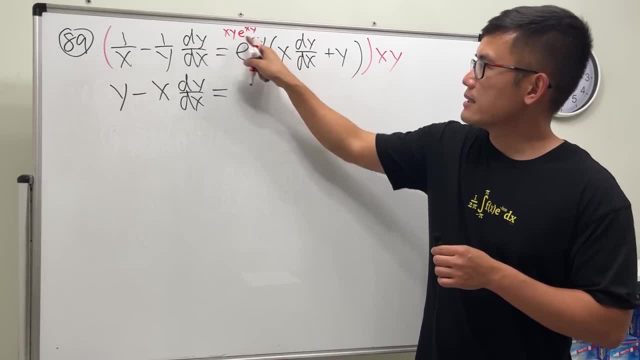 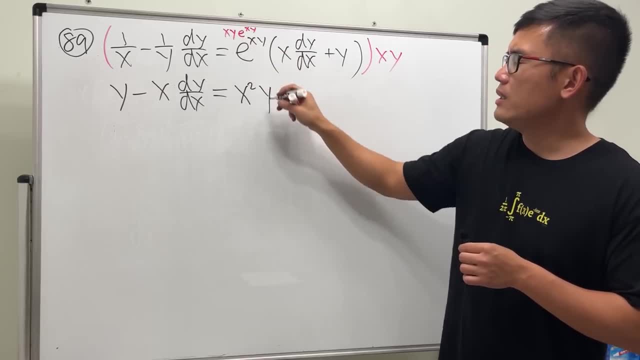 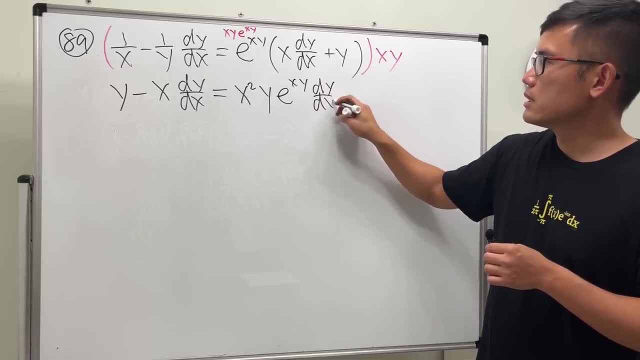 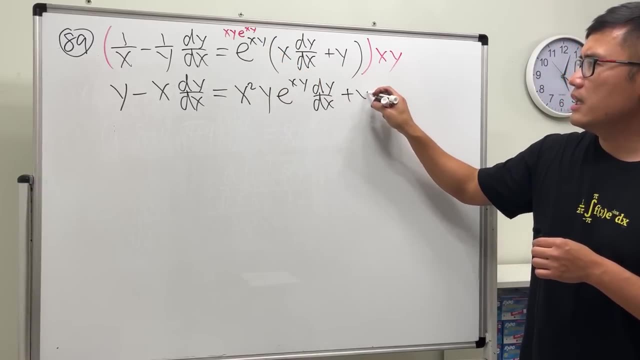 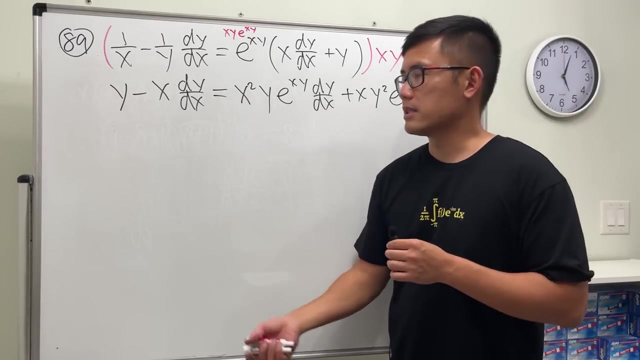 x to the third power times, 2l and y. x to the third power times, 2l and y. and so take this, multiply by that, we get this, and then next we take this times that, so plus x and the y square, e to the x- y. yeah, okay, to keep things positive, i'm going to move this to the 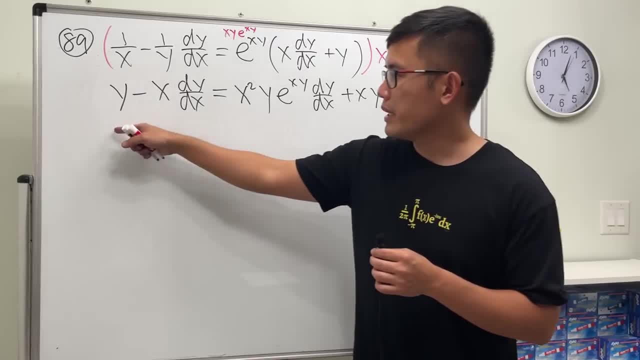 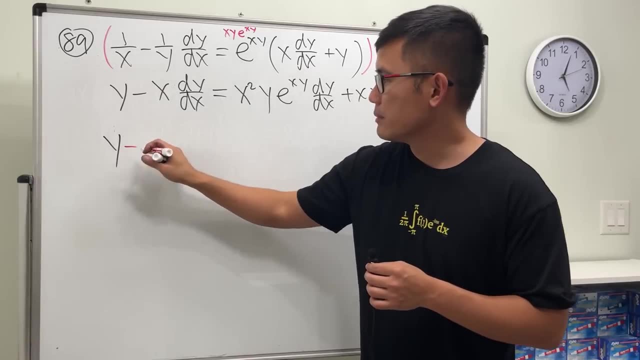 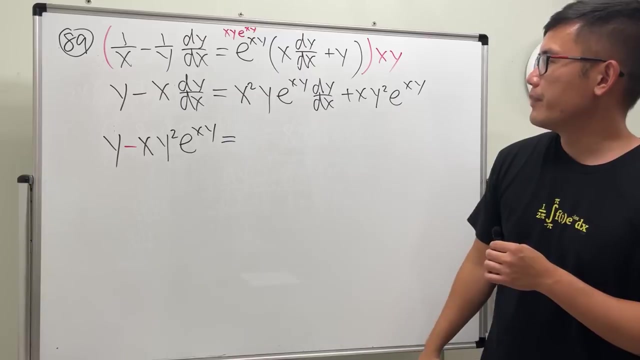 other side and then move this to the other side. so we have this y here. this doesn't have the x, this does not have the dy dx. put it to the other side, so it becomes a minus x y square e to the x y. that's equal to okay, so leave this, which is x square y e to the x y plus. 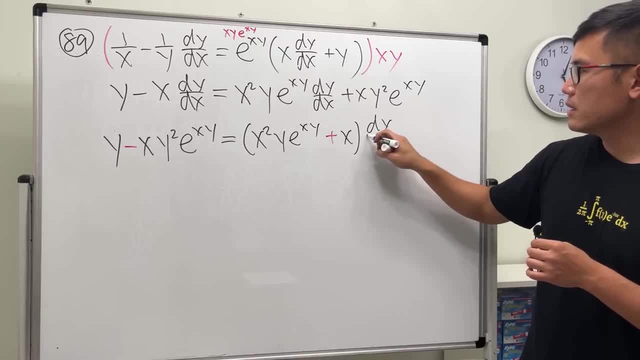 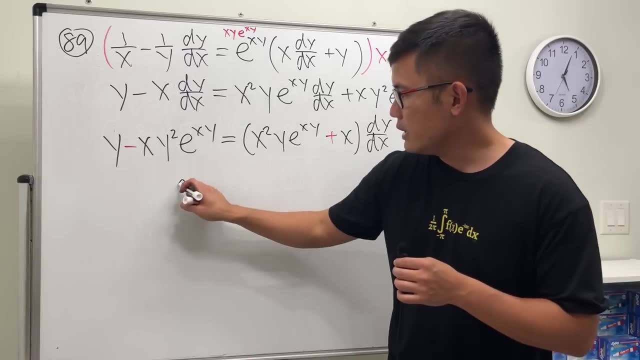 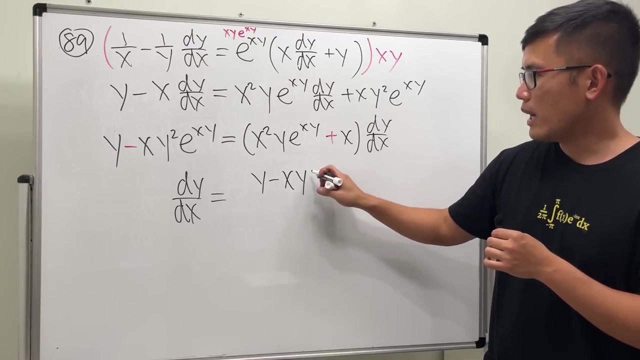 x and then dy dx. that's pretty much how to do this kind of questions. and then, lastly, just divide this on both sides. so we have dy dx, equals over there. we have y minus x, y, square e to the x, y over this right here, and because the water of addition doesn't matter, 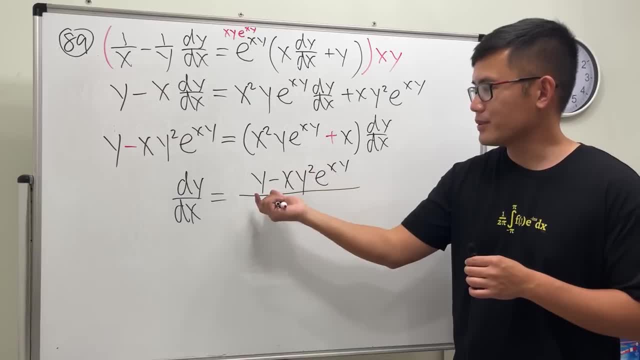 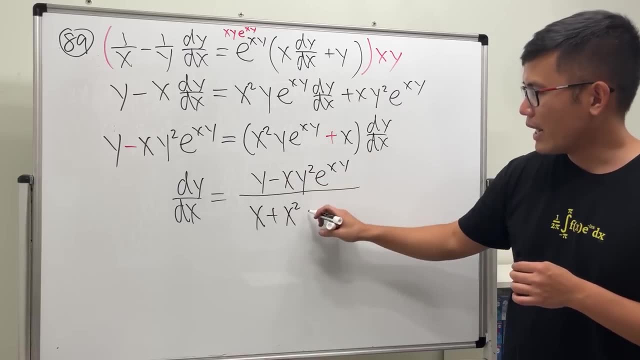 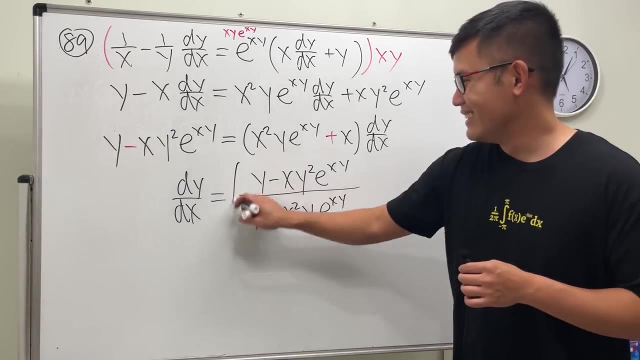 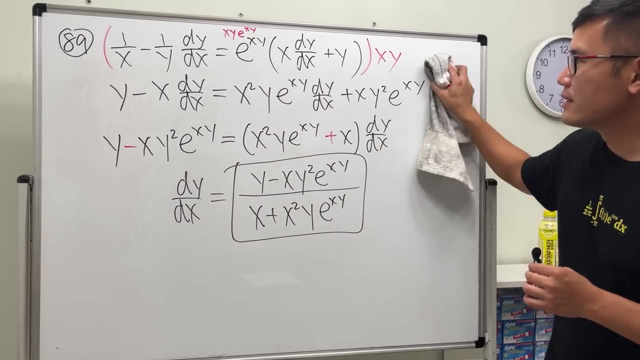 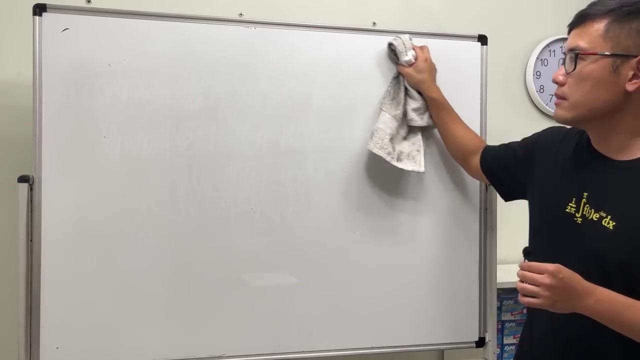 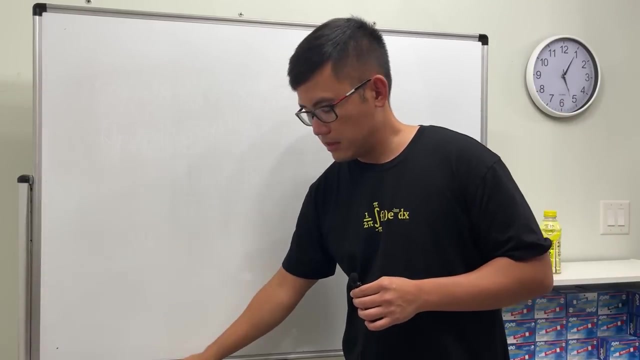 and i like to have the single term that goes first. right, so it's x. so let's put the x first plus x square y, and then e to the x y. yeah, that's how i have on my answer key as well, just like that. all right, one more with the differentiation one. one. one more with the dy dx business. 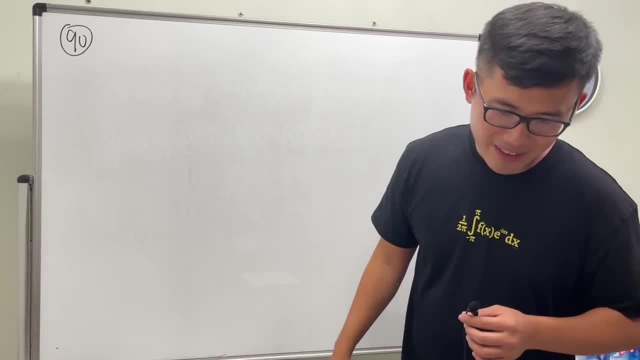 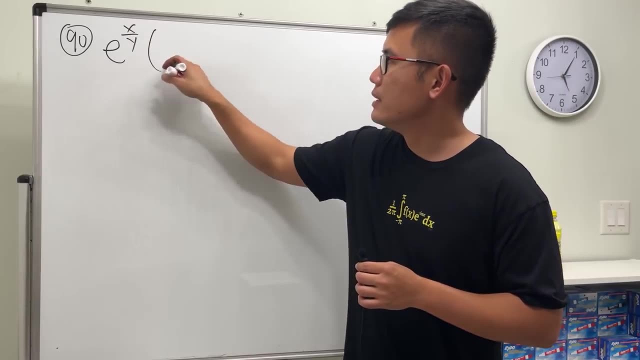 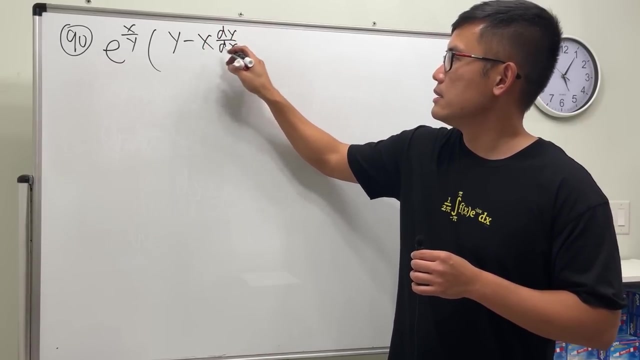 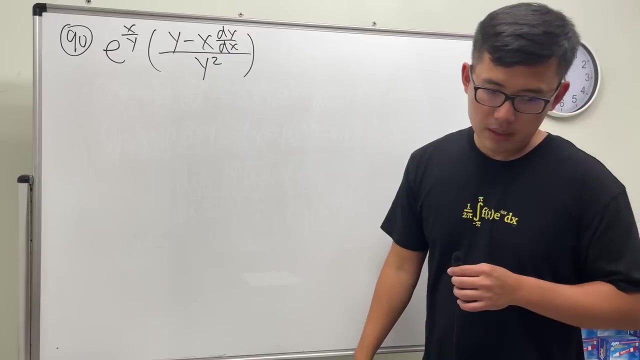 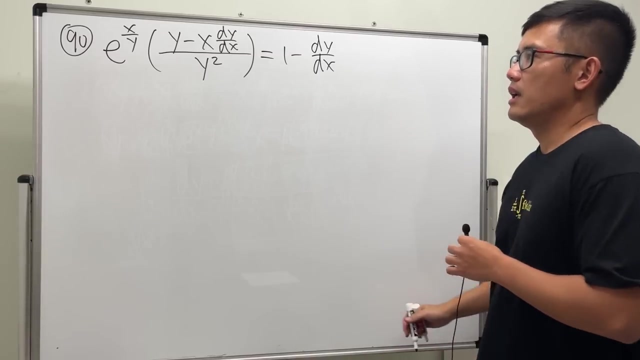 number 90. okay, e to the x, y, e to the x, over y times, y minus x. divide the x over y square and this is equal to 1 minus dy dx. okay, first thing. first, this equation has the y square on the bottom right, so let's. 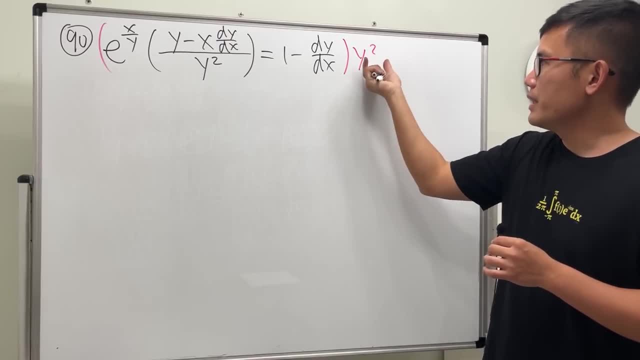 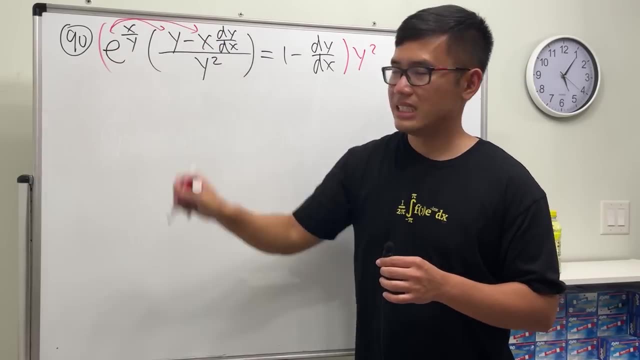 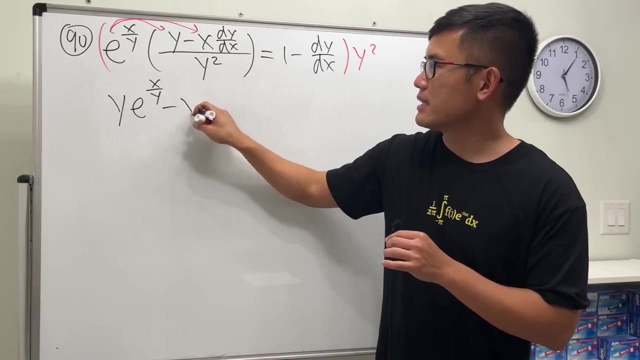 multiply everybody by y square. so when we take this, times that they cancel. but in the meantime let's also distribute this inside. yeah, so first we get y e to the x over y's power and then minus x e to the x over y's power, and 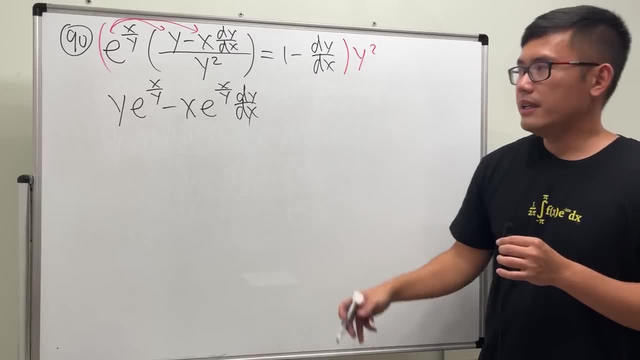 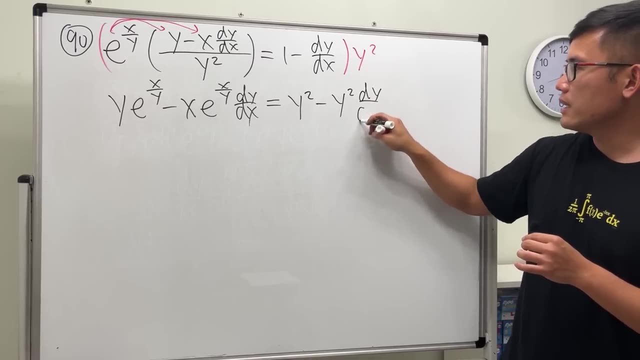 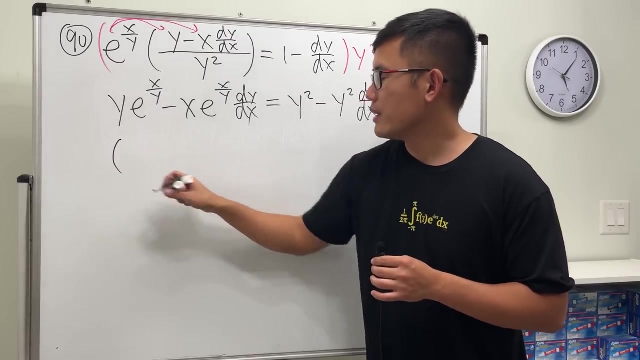 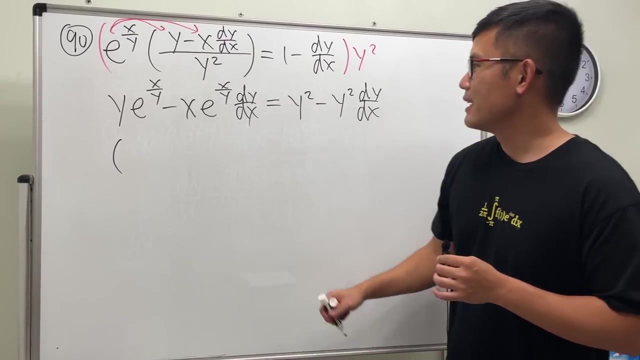 then the dy dx and then take this times down. we get y square. take this times down with minus y square, dy dx. now i'm going to move this to the other side. so this was negative moving to hold on hold that, move it. yeah, let's move this to the other side. 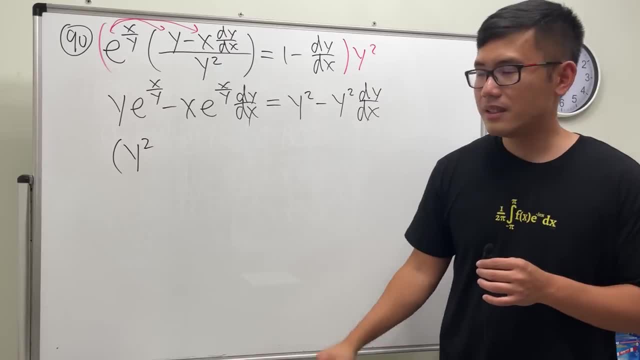 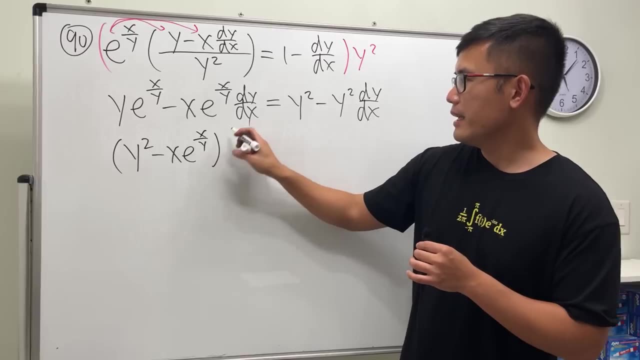 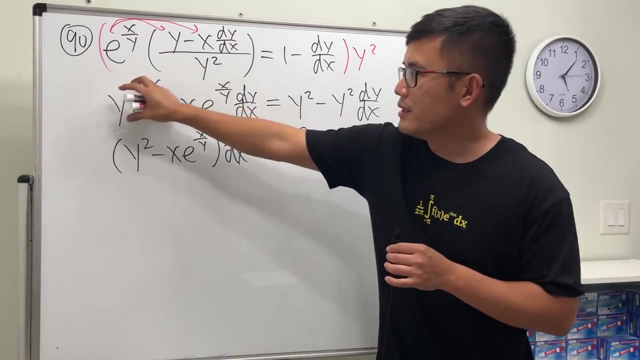 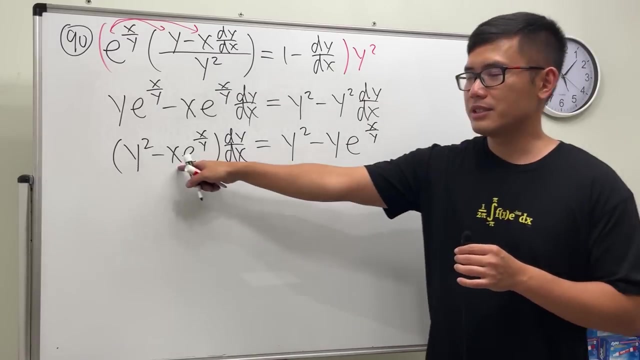 so we'll have y square being positive here, and then this right here states inside right: minus e, minus x, e to the x over y, and then dy dx and that's equal to this. right here is the y square, but bring this to a here, so we have minus y, e to the x over y, all right, and lastly, let's just divide. divide that. 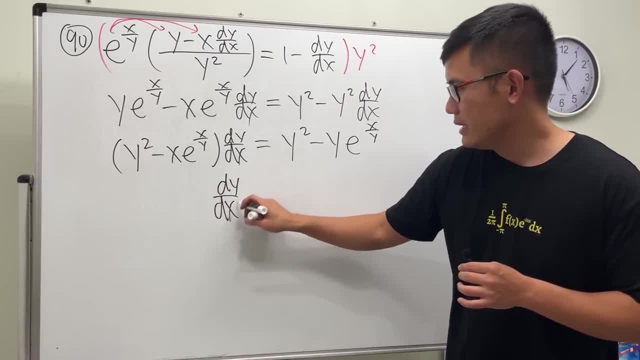 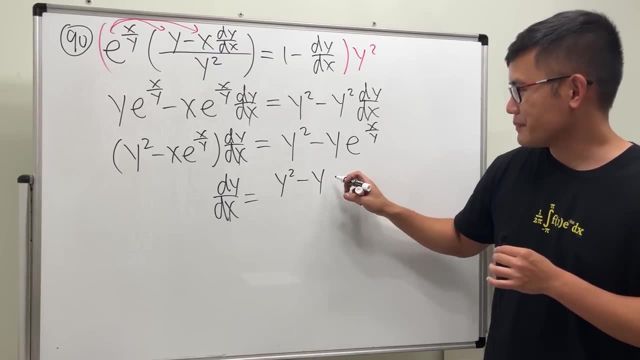 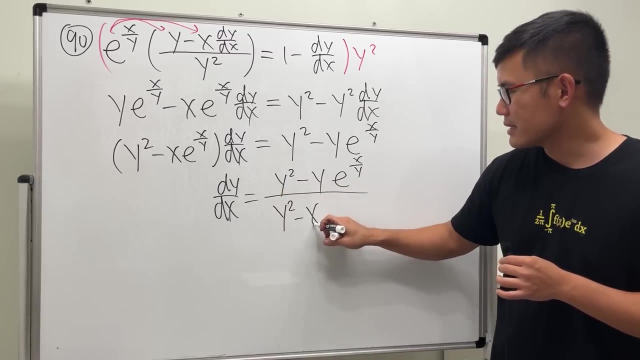 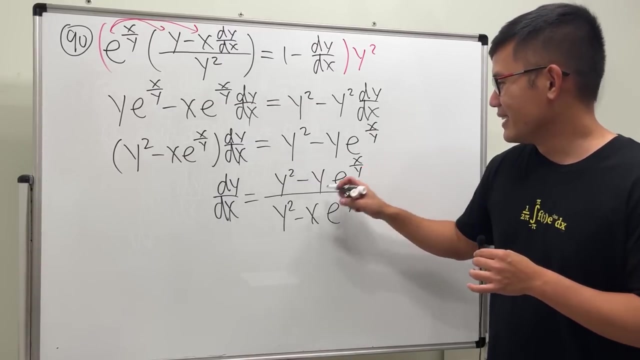 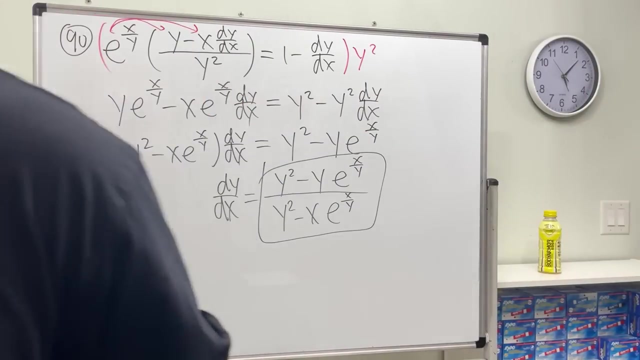 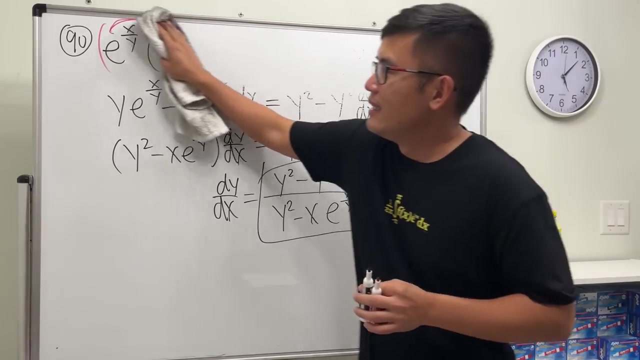 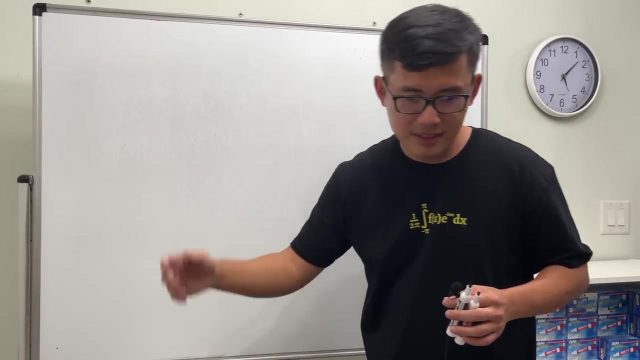 and we'll be done so. dy dx equals y- y square minus y e to the x over y over y square minus x e to the x over y. okay, okay, okay, it's. it's only four hours and 17 minutes, but like 5 am. why am i doing this to myself? huh. 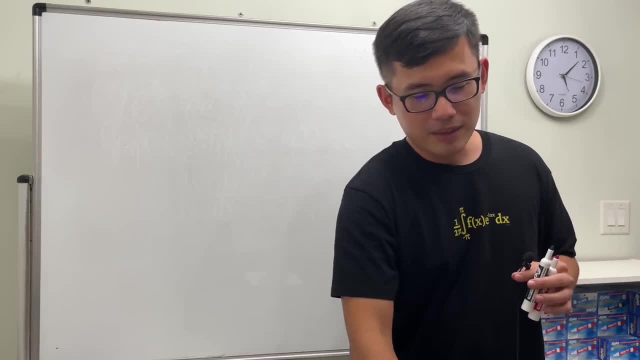 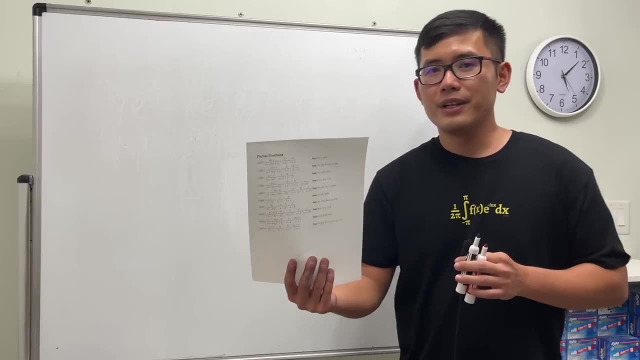 okay, partial fractions. some of you guys may have done it in pre-cal, some of you guys have not. doesn't matter though, but let me tell you: if you're only taking calc one, this right here- you don't have to worry about it too much, but if you are taking cal 2, then 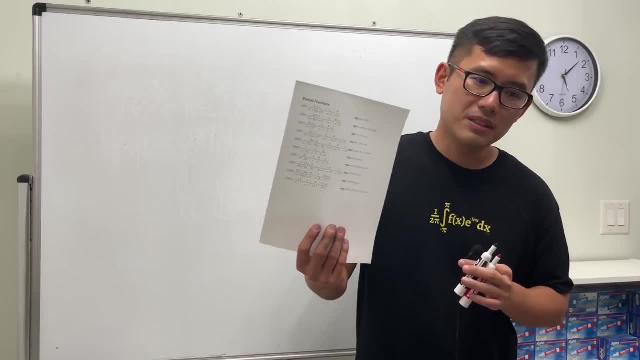 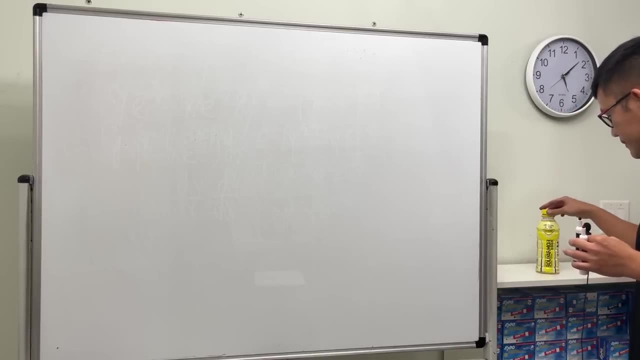 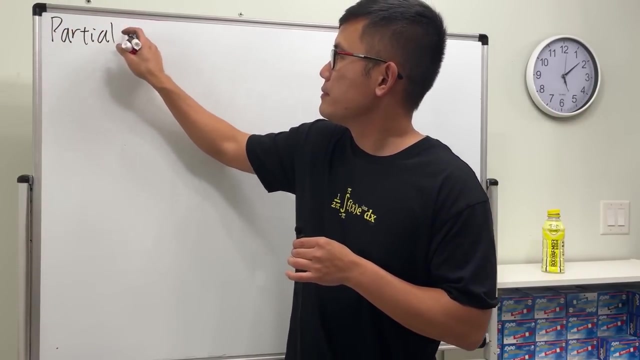 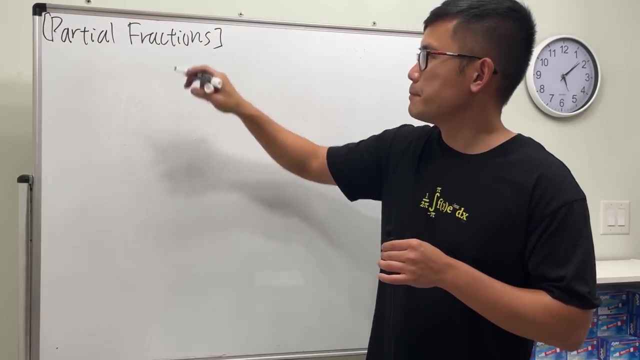 make sure you come back here and see how we solve for the a, b, c, d, for partial fractions. okay, so this is what you're going to see now. i'm going to take cm here. this is the. this is good, all right. this is good, all right. 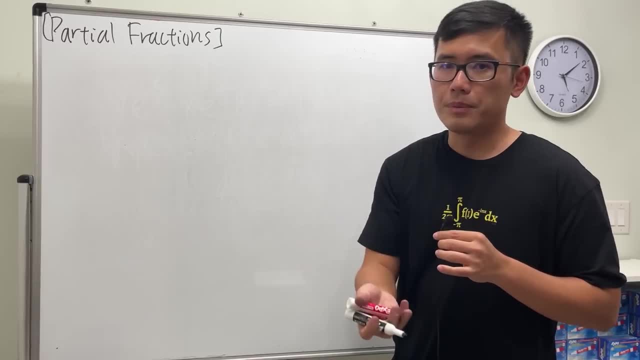 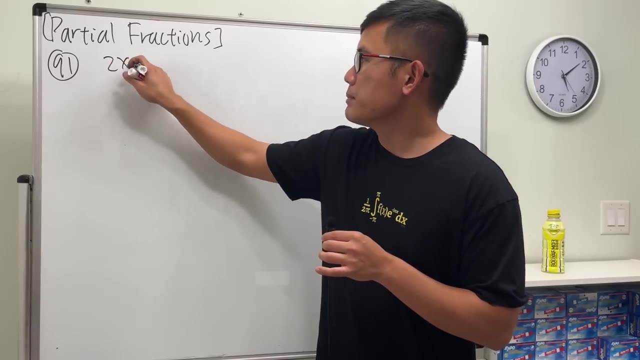 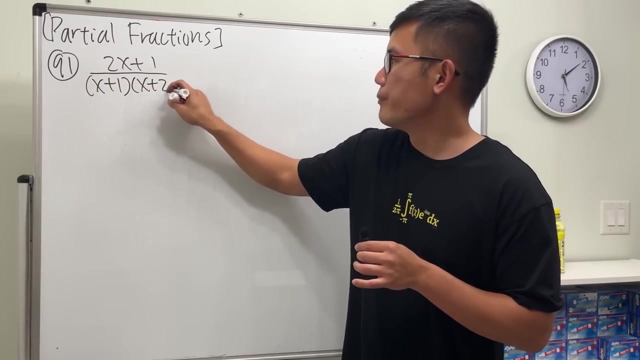 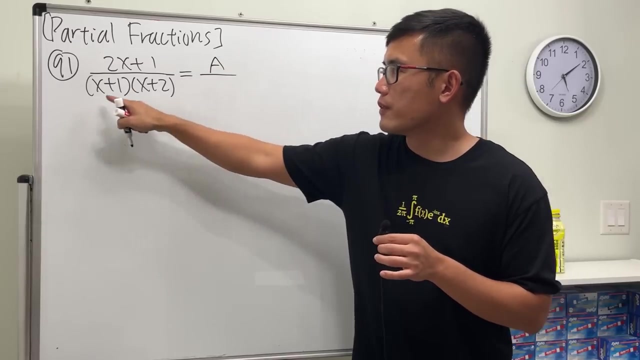 how to how we can break a big fraction into a smaller pieces, into smaller pieces. take a look at number 91. if we look at 2x plus 1 over x plus 1 times x plus 2.. i'm just going to tell you that we can break this apart as some number a over the first denominator, x plus 1 plus. 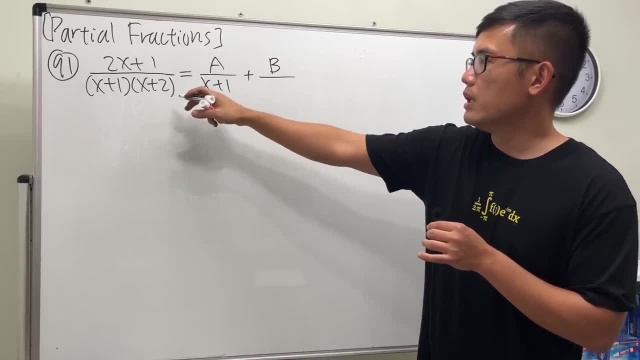 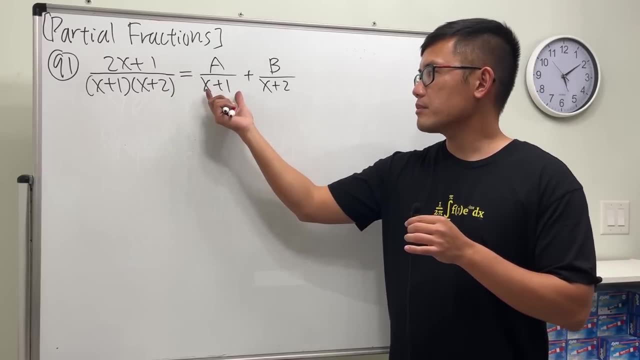 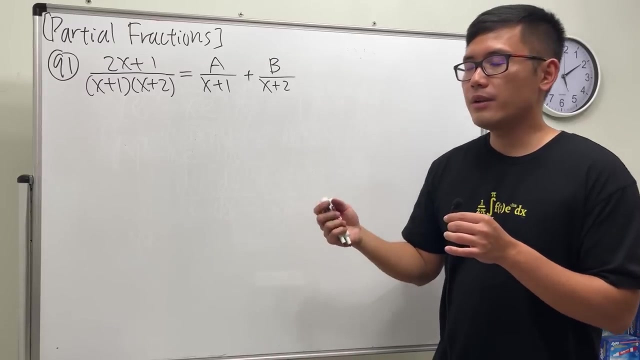 some other number- we call it capital b- over the other denominator, which is x plus 2.. and if you think about it, it should make sense, because when we have these two little fractions, when we add them, of course, we'll get this for the denominator and we just have to find out the correct number a. 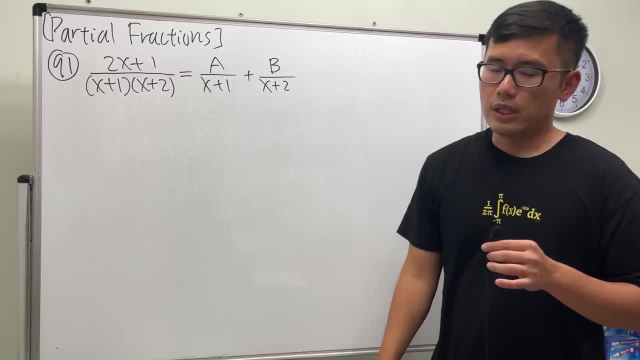 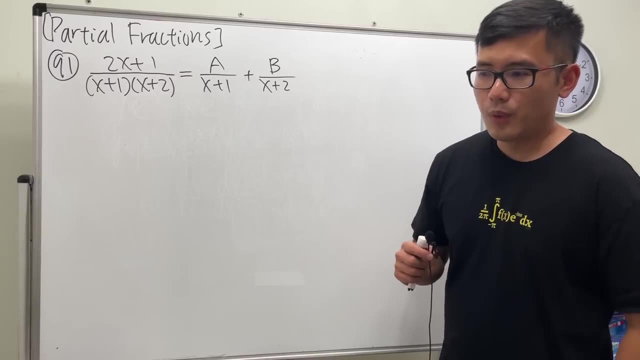 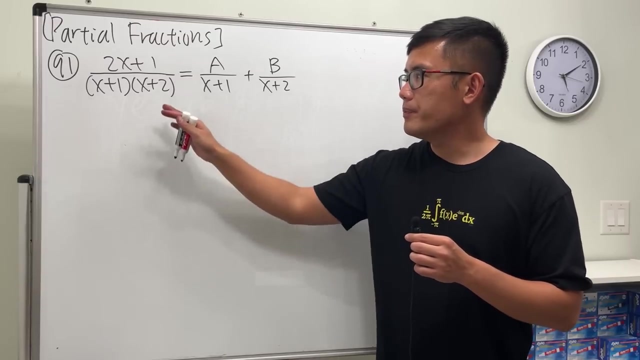 and b, so that we can end up with 2x plus 1, right, just like what we did earlier for the lcm and also how we did for the lowest common denominator, and then combine the fractions. but right now we're just doing this backwards. i'm not going to go over like how we break it down in details. i have another video for that. 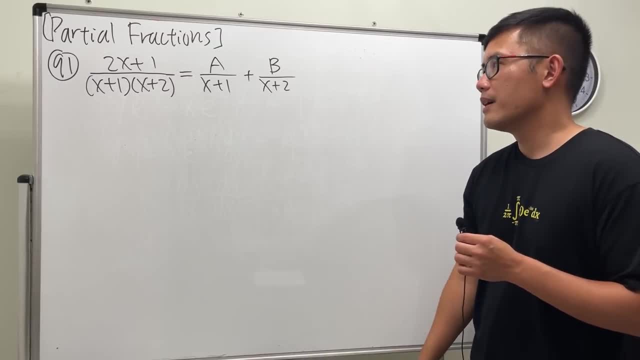 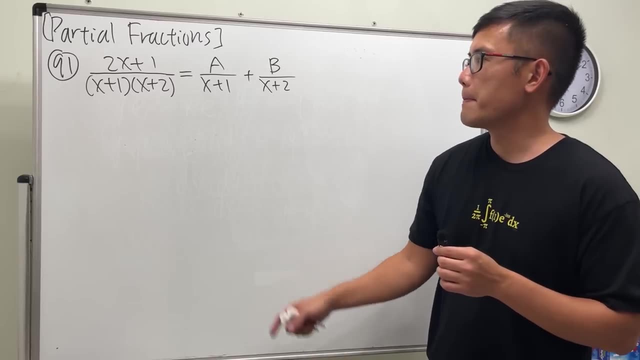 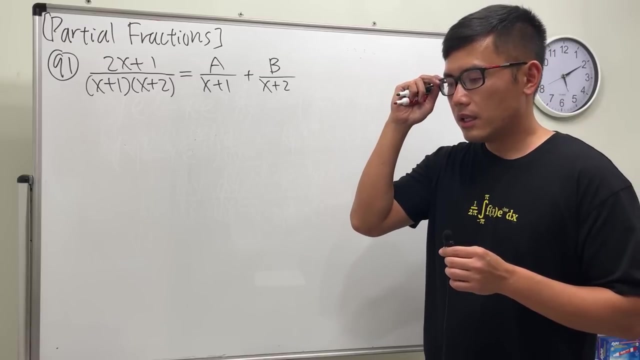 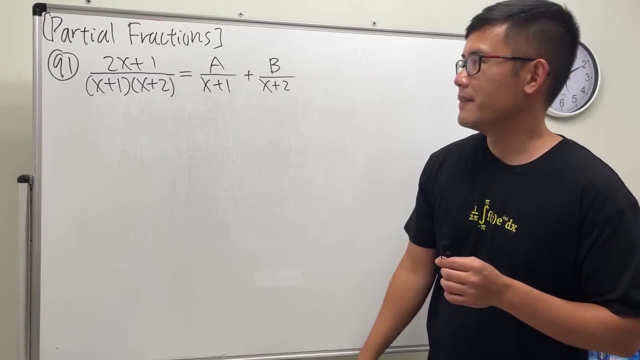 but this, we're just going to be solving equations. here we go number 91, this right here. it's an easy case. i'll tell you a and b can be very easily done, right. i'm going to tell you guys how well. of course, obviously, let's do it if you want to. i'm going 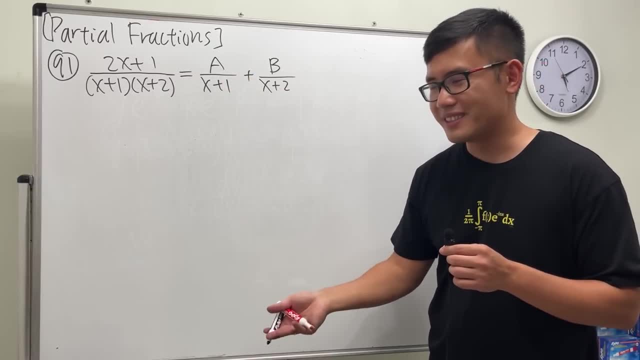 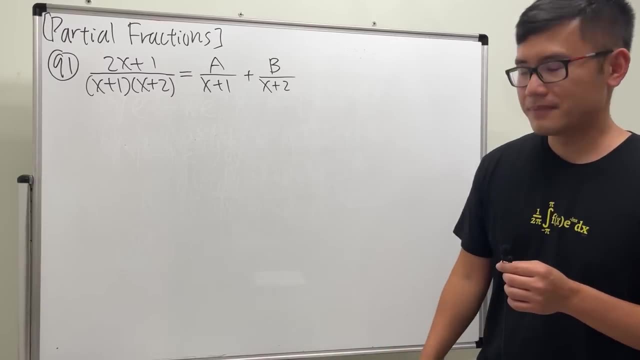 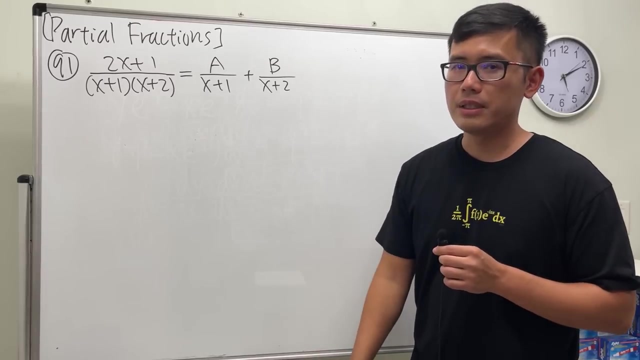 to show you guys a short way, but i'm going to give you guys the proof of the short way first, and then i'll give you guys a short way. let's do it. just 10 more questions i want to solve for a. a has x plus 1 for the denominator. you know what we have: an equation. 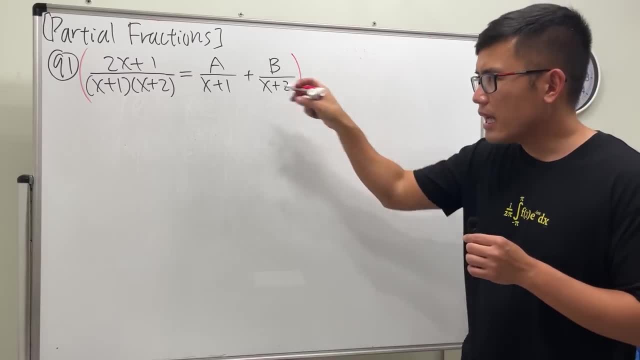 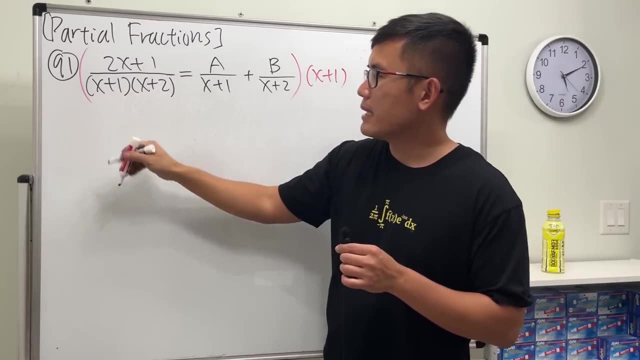 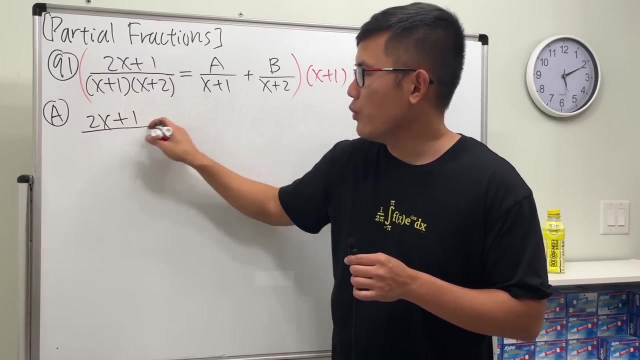 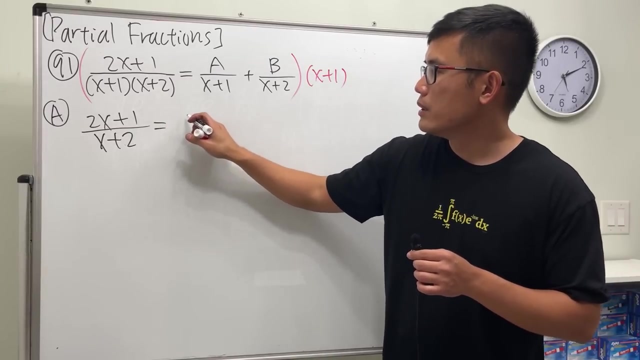 let's just go ahead and multiply this by that denominator, namely x plus 1, just that. just that you'll see why. when we take this, multiply by that, you get 2x. by the way, this is for a, okay for a. we give 2x plus 1 over this, and that will cancel. so we just have x plus 2.. and then this is equal to a. 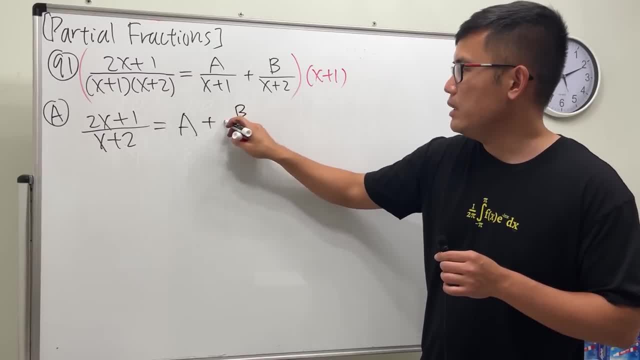 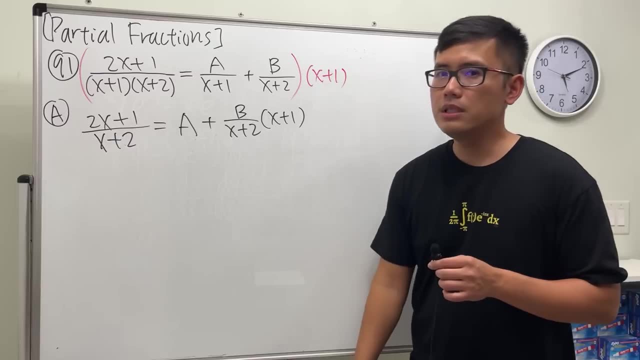 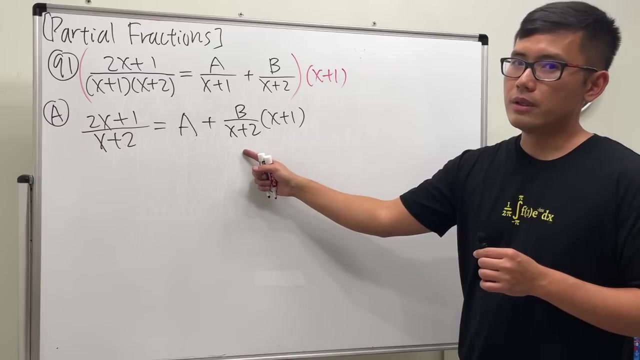 they cancel already and then plus b over x plus 2 times x plus 1.. and you see a is pretty much alone. right, doesn't have the denominator anymore, but b does. however, not only b has the denominator, but b also has the x plus 1.. if we 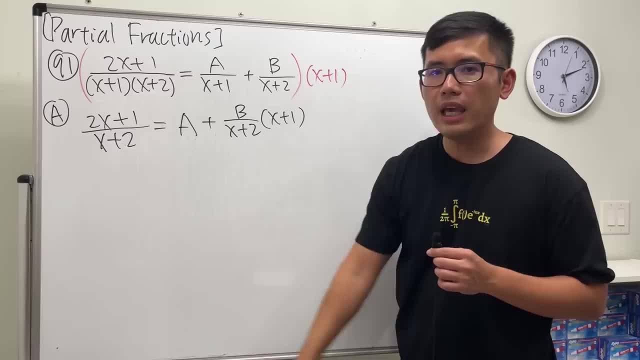 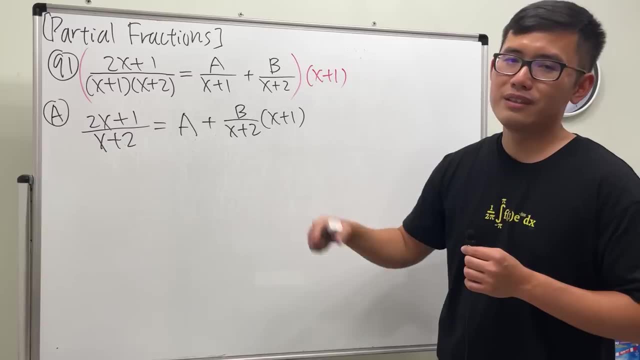 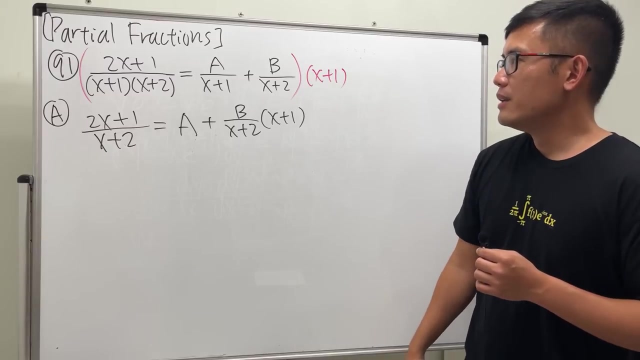 can somehow get rid of this term, then we can get a, but how, though? well, how can we make this turn 0? x has to be. what negative 1? see, if we put negative 1 here, this will be 0, so this one will be sure. yeah, so what we are going to. 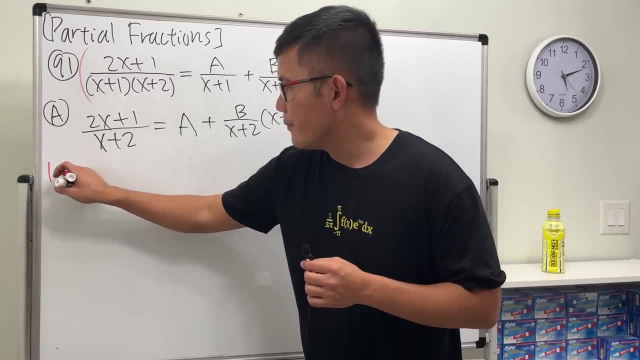 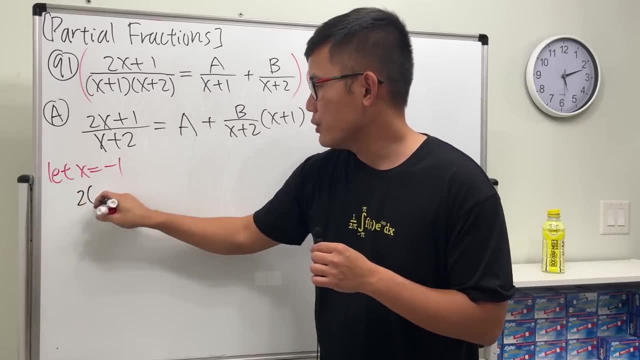 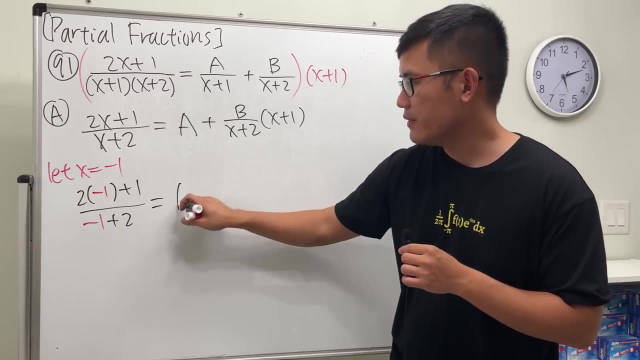 do is we are going to let x equals negative 1 and just plug into all the x's, so we are going to get 2 times negative 1 plus 1 over negative 1 plus 2, and this is going to give us the a value. 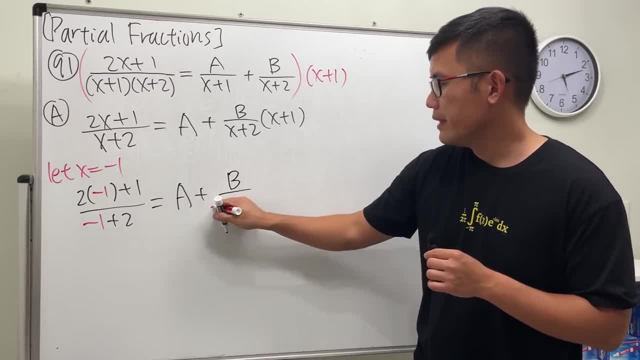 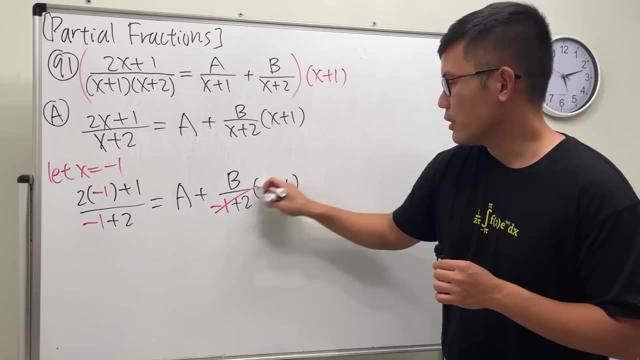 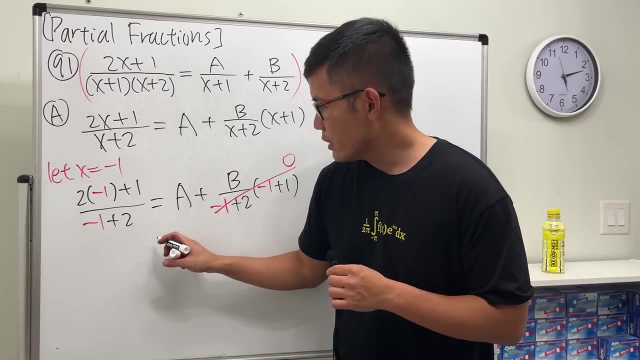 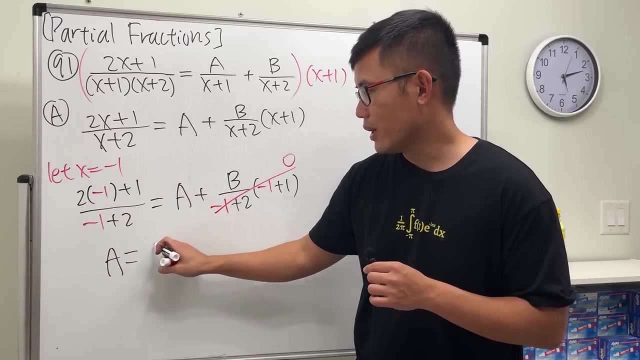 i will show you this plus b over negative 1 plus 2 times negative 1 plus 1.. this is just equal to 0.. yeah, no more. so, as you can see, a is just equal to that. so a is equal to what? negative 2 plus 1 is negative 1 over. 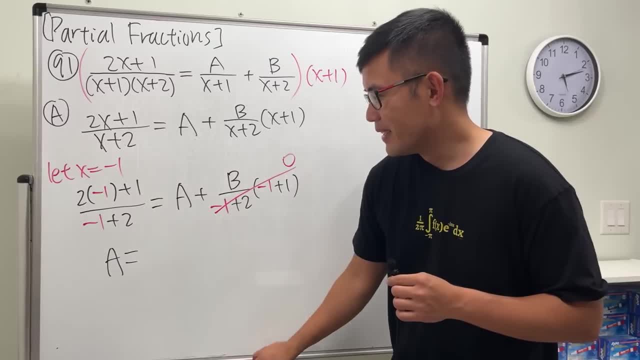 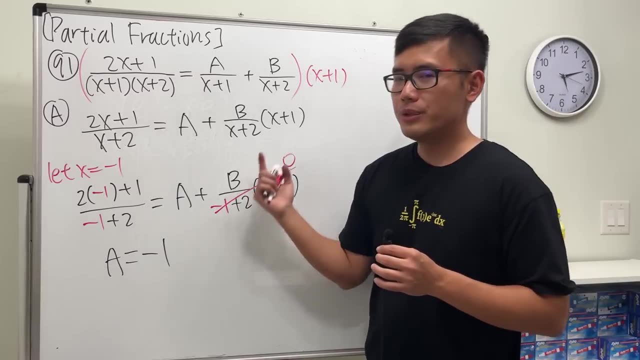 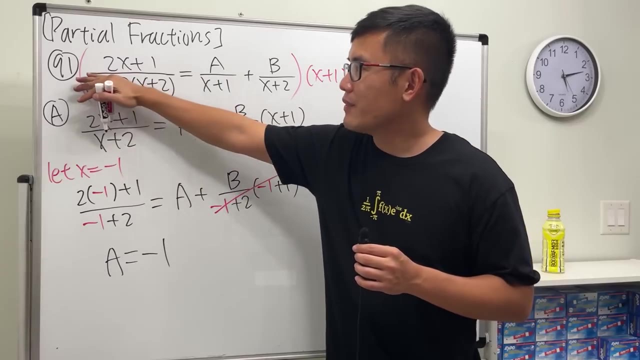 1.. so just negative 1. a is just equal to negative 1. done, yeah, and in fact you are going to notice we don't have to go through this every single time, because we can actually just look at this and then just do the so-called cover-up: just cover up the same denominator and then plug in x equal to negative. 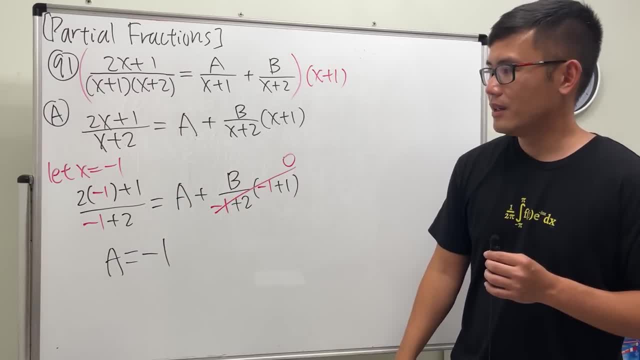 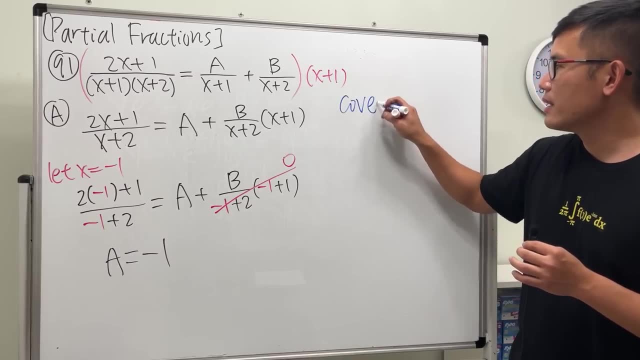 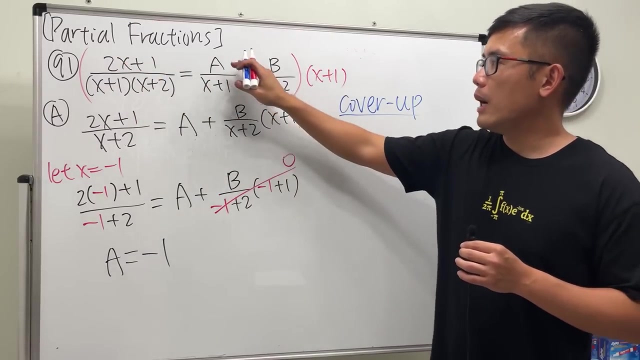 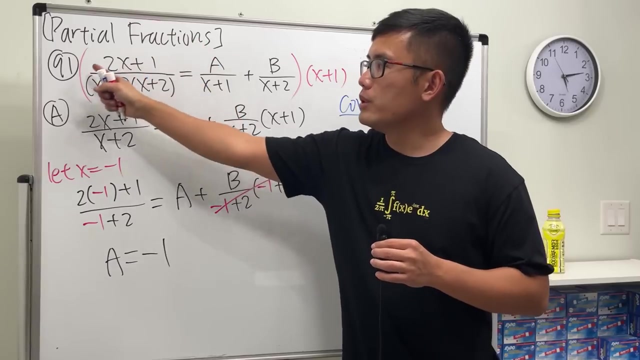 1 for here and here. you see, this is what we have. this is what i mean. i'll do this one in blue. this is the so-called cover-up method. okay, look at this equation. i want to solve a. a has x plus 1 for the denominator. we go back to the original. we cover up the same denominator. 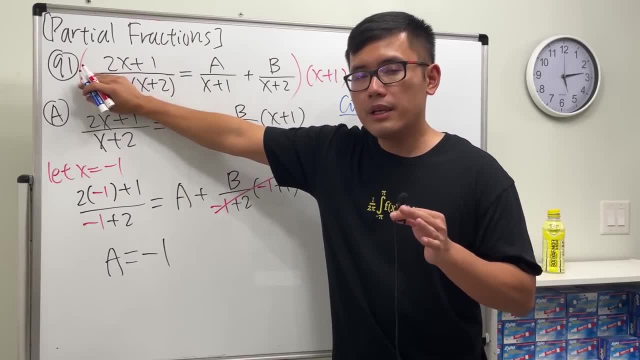 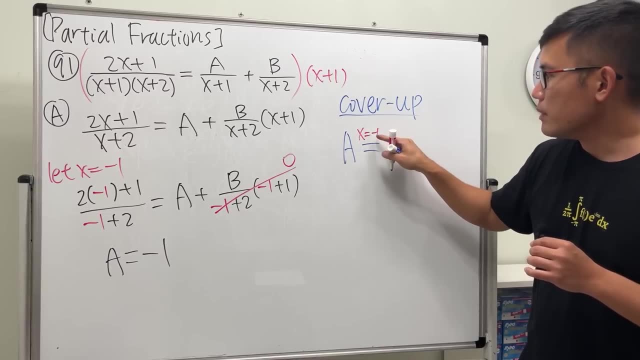 but we have to ask ourselves how can we make x plus 1 equal to 0? x has to be negative 1, so x has to be negative 1, and we put this in here and here. so we just write it down: 2 times negative 1, so this: 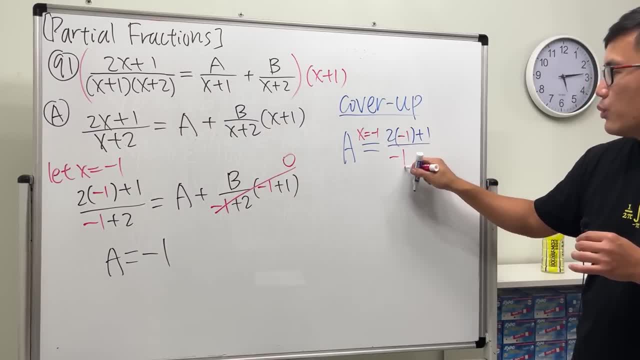 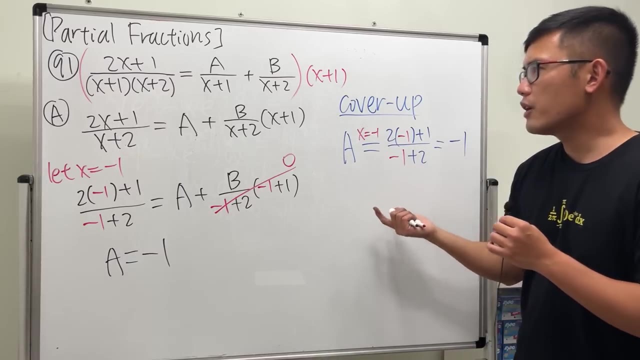 2 times negative: 1 plus 1 over negative 1 plus 2.. That's going to be negative 1.. And then we are done. This is the reason why it works. This is the reason why it works, And let's practice the cover-up for B. 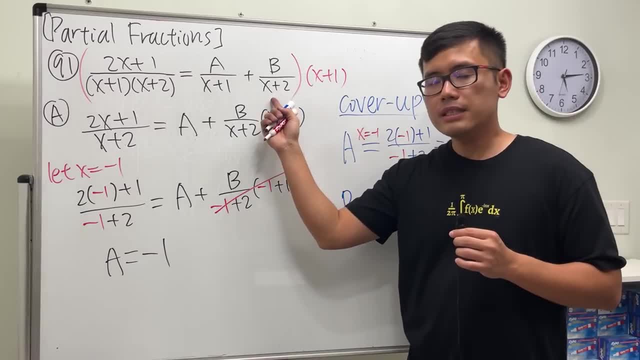 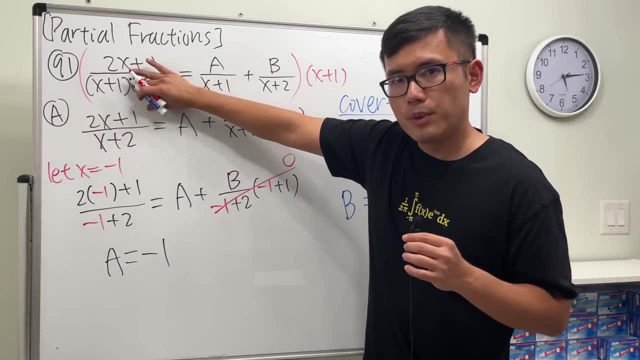 For B? well, it has x plus 2 for the denominator. So we go back to the original cover, the same denominator, But x plus 2 equals 0. x has to be 1. Negative 2. So I'm going to put in negative 2 here. 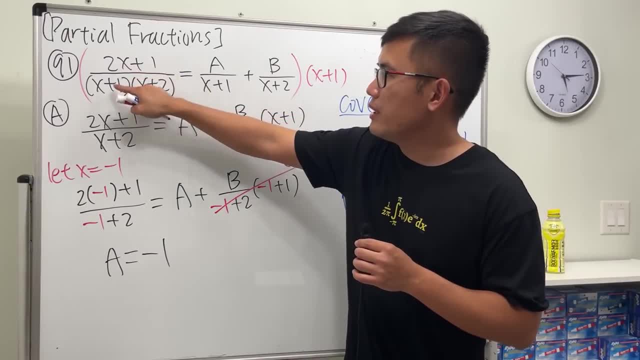 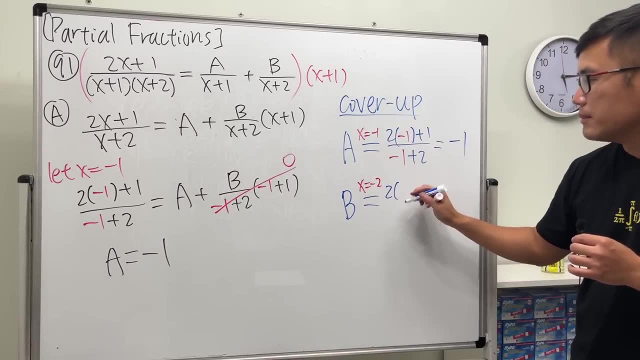 And then I will plug in negative 2 into here and here of the remaining x's. So we are going to get 2 times negative, 2 plus 1, over negative 2 plus 1.. Now check this out: This is negative. 4 plus 1 is negative 3.. 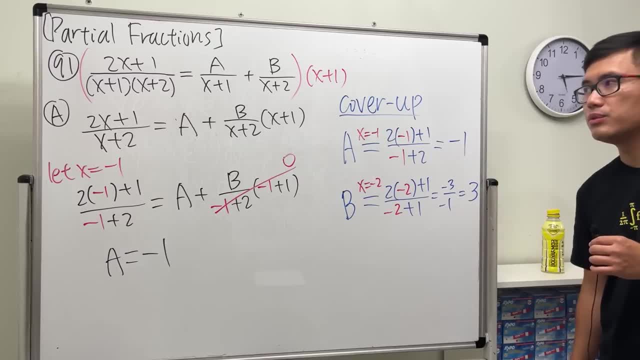 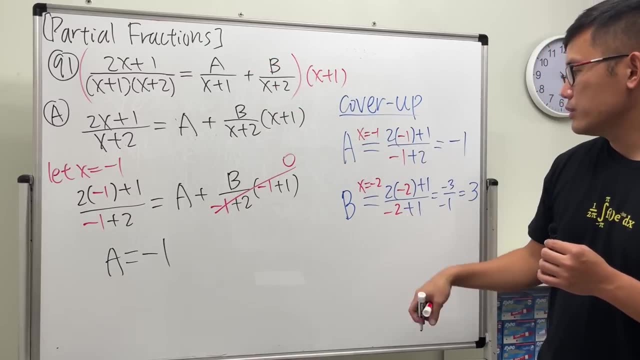 Over negative 1.. Altogether, we get positive 3.. So we are done. And that's exactly what we are trying to do. We are trying to figure out what a and b's are. So right here I'll just tell you: a equals negative 1, b equals 3.. 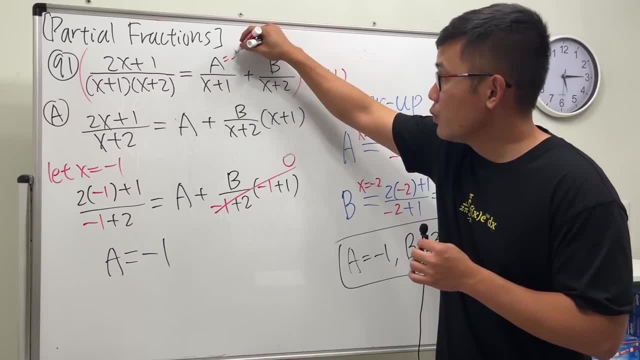 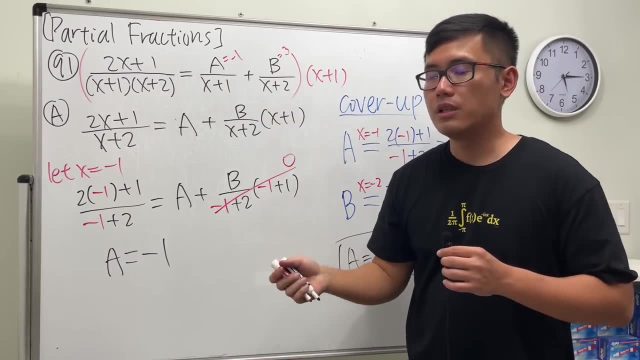 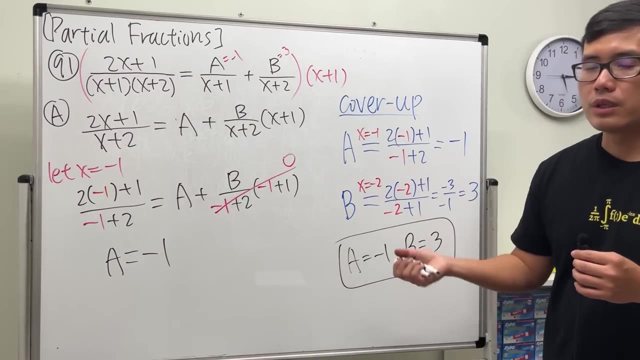 So we can come back here and say: this is negative, 1 and b is equal to 3. And if you combine these fractions like the way I showed you earlier, you will get that Guaranteed, All right. So this is why the cover-up works. 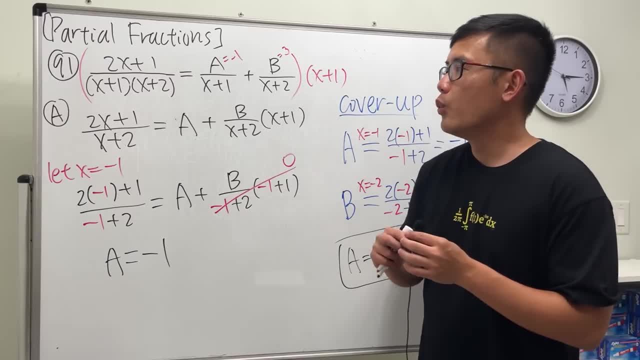 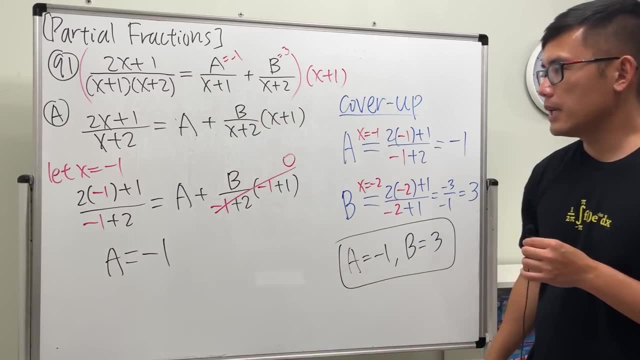 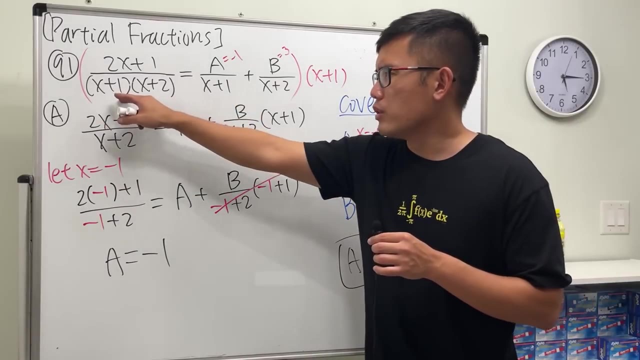 And let me tell you, the cover-up works nicely when we have linear denominator, meaning x to the first power, Yeah, Yeah. And then another thing is that you have to make sure that the denominator is the same as the original fraction. All right, 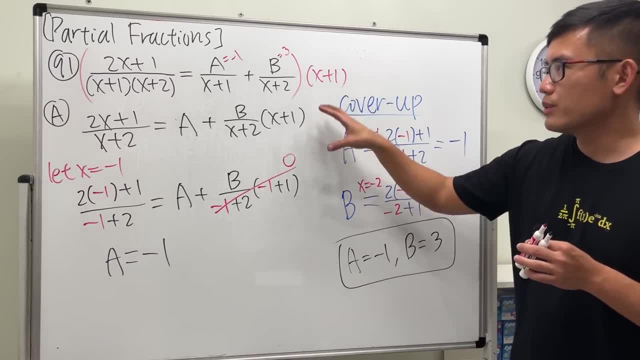 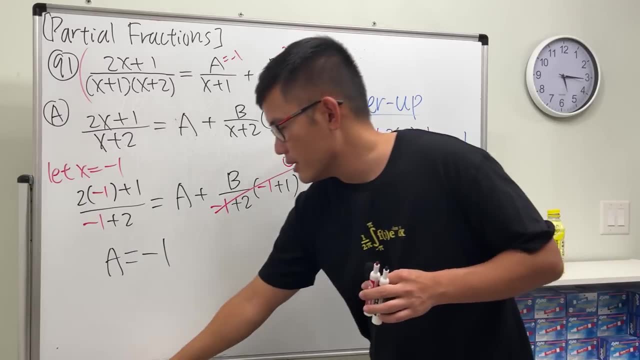 Yeah. So I think this is clear. If you want to go through b, Just multiply out everybody by x plus 2. And then work it out like that. Okay, But I'm not just going to show you guys the cover-up, because there are also other cases. 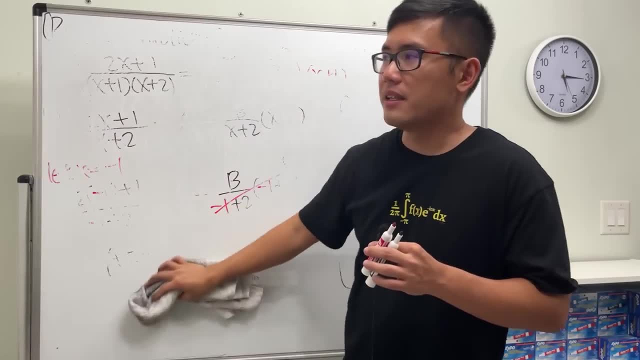 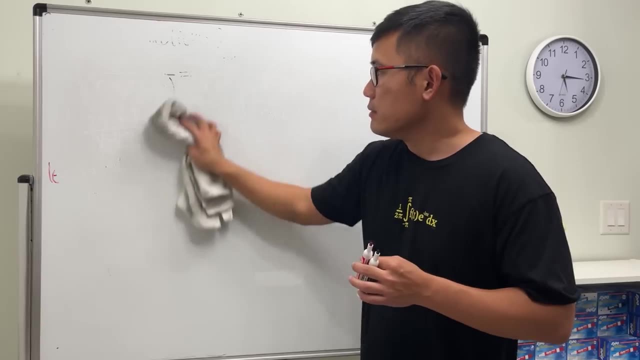 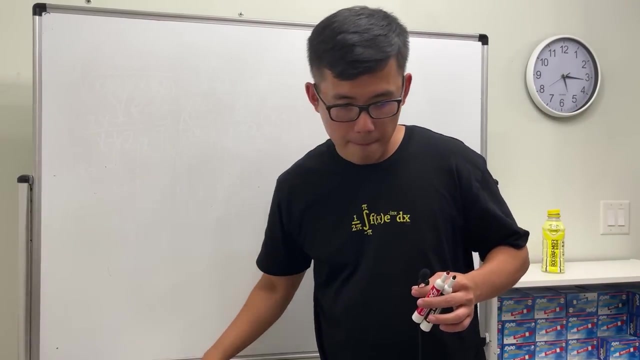 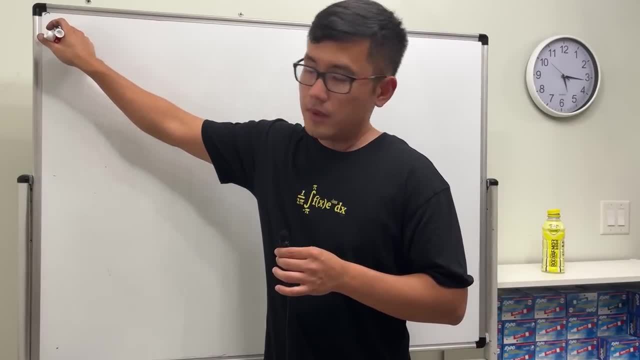 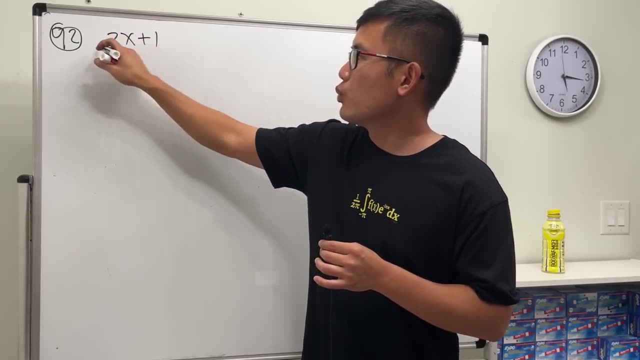 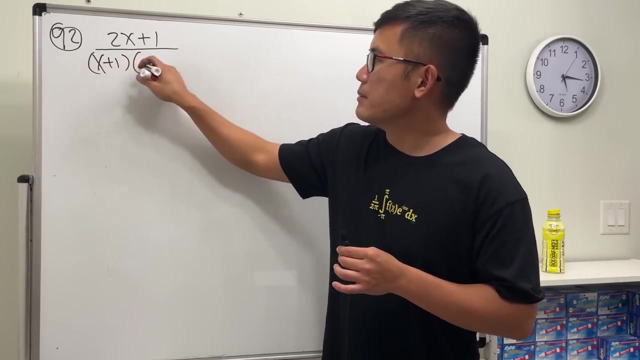 Next one, 92. Notice this one. We still have the same numerator: 2x plus 1.. But the denominator. I changed it a little bit. Earlier it was x plus 1 times x plus 2.. Right, But this time instead of just the first power. 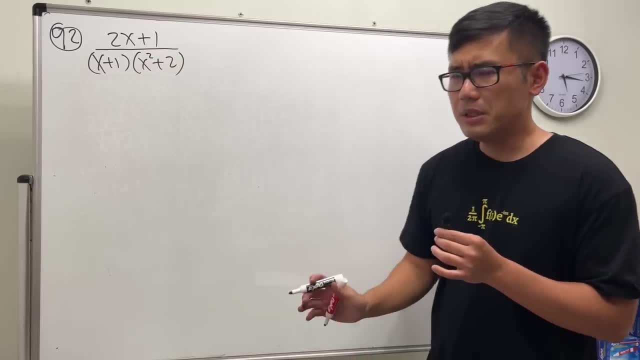 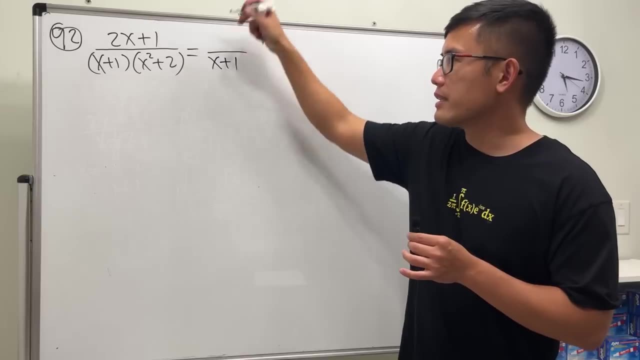 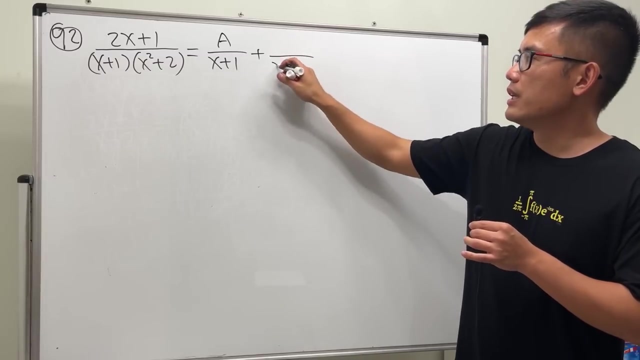 first power. we have the second power and you will see. the breakdown is the following. i will tell you, we still have this for the first fraction, right: x plus one on the top- we don't know what the number is, such as a- and then the second fraction. we have this for the denominator, which is x squared plus. 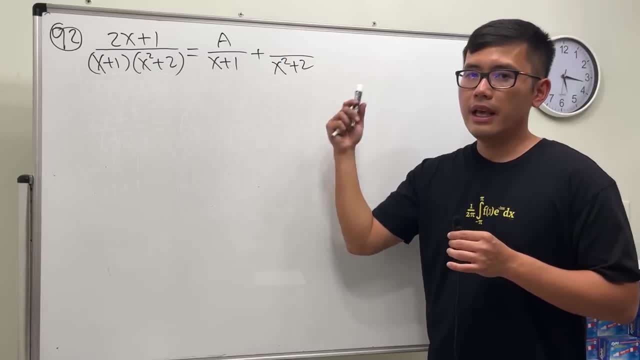 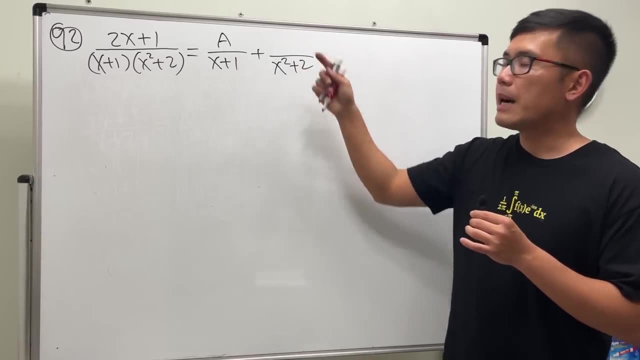 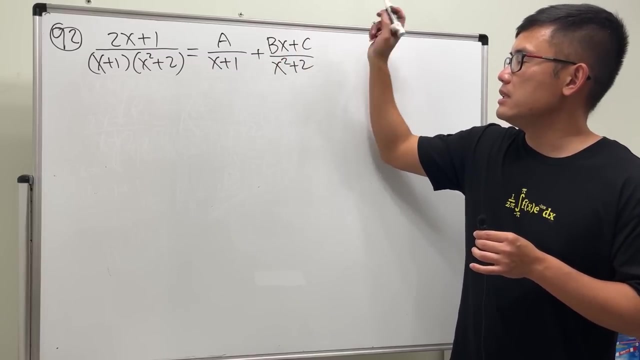 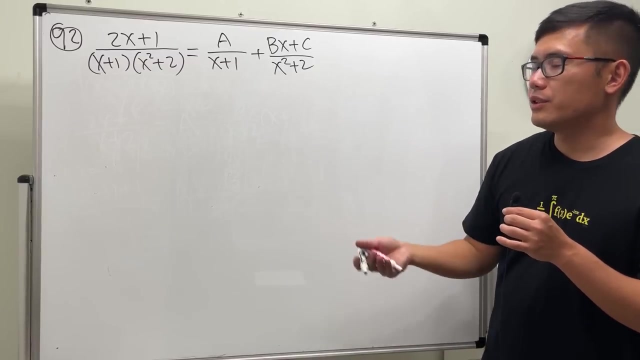 two. but notice we cannot factor x squared plus two with real numbers. so if this is the irreducible quadratic, the top will be set up as a linear meaning. we have bx to the first power plus c. so this is quite different than what we had earlier and for more explanation you can check. 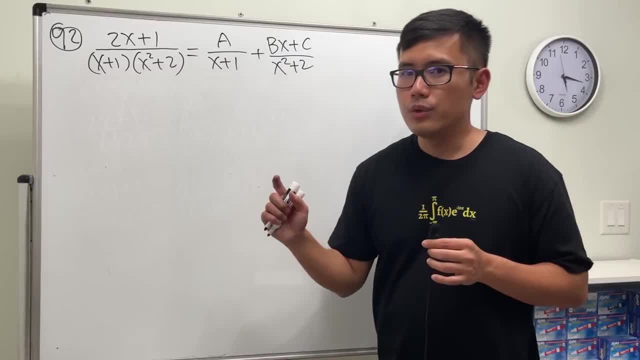 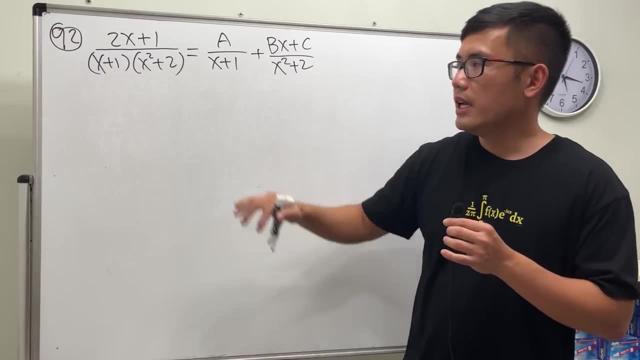 out my other video for it. now we can do a cover-up for one of the letters, and that is a, because this and that have the same denominator and we can cover this up and make it equal to zero. so for a we can do a cover-up for the first power and we have bx to the first power plus c, and that is. 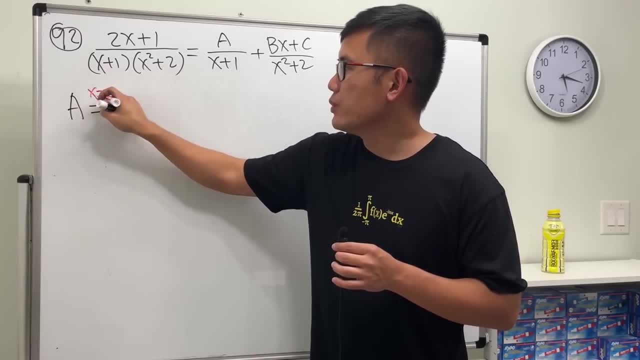 a, because this and that have the same denominator and we can cover this up and make it equal to zero. This is just going to be when x is equal to negative 1, like what we did earlier. We copy this up, so just put the negative 1 into here and here. 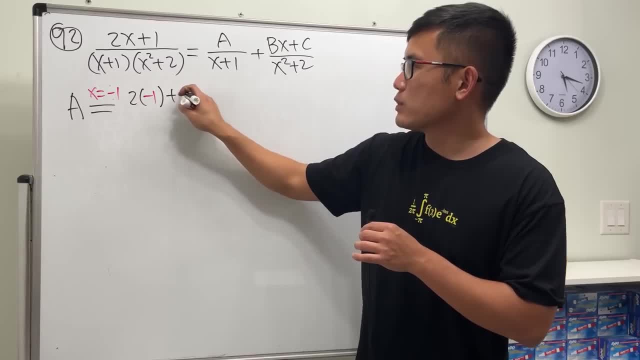 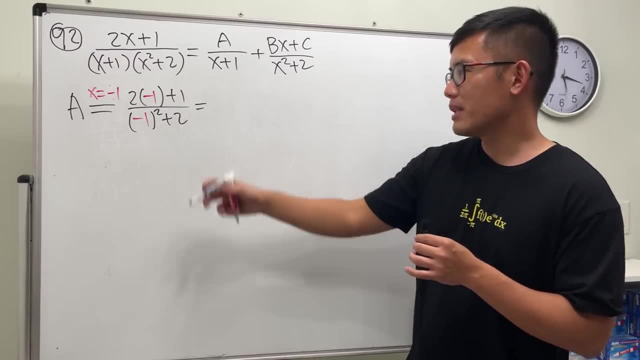 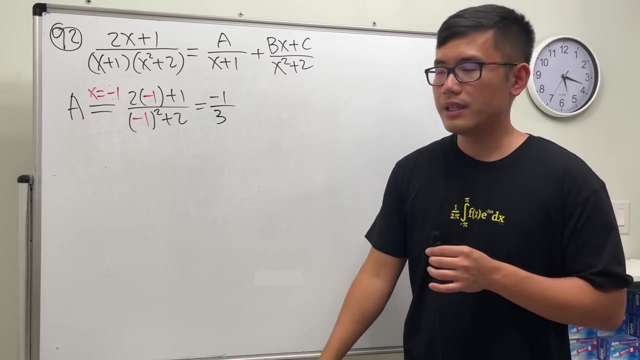 So we get 2 times negative: 1 plus 1 over negative, 1 squared plus 2.. That's negative. 2 plus 1 is negative, 1 over this is 1 plus 2 is 3.. So a is equal to negative 1. third, 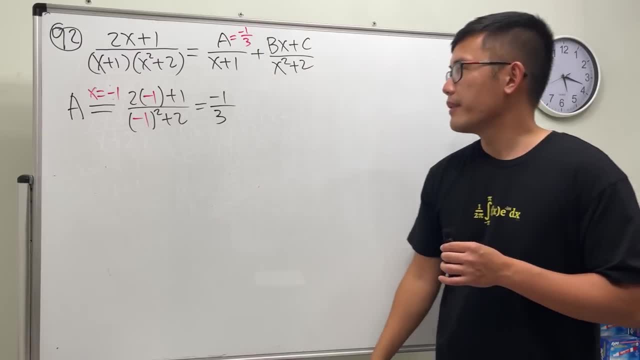 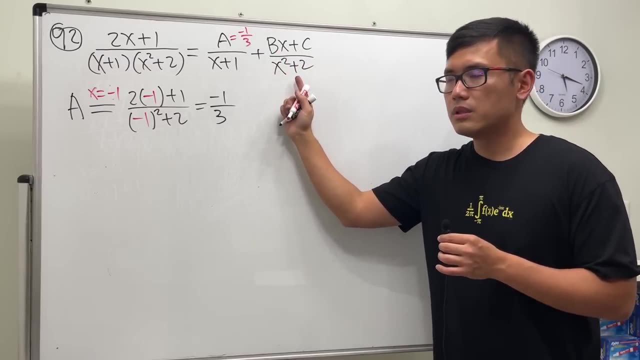 So we are good for that. But now the problem is that you see we have bx plus c on the top of the x squared plus 2. If we copy this up, what are we solving? b or c. That's the problem, right? 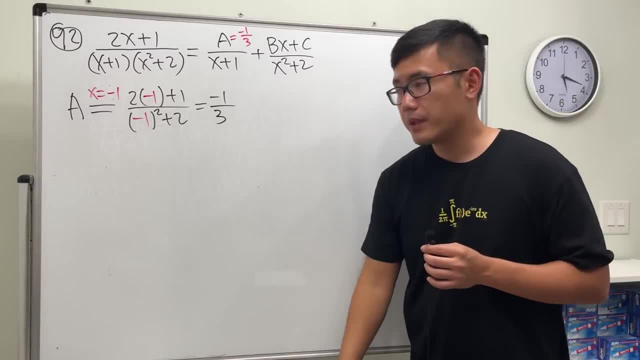 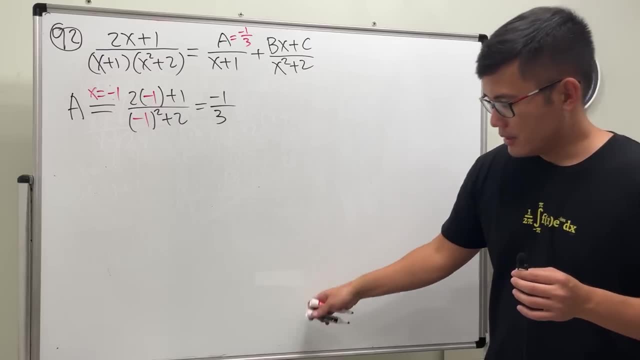 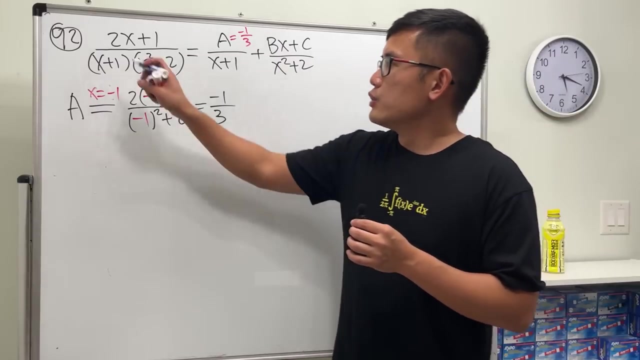 So the cover does not really work for b or c. So what we do here is the traditional way. I think the traditional way is the way that students can follow along much better, Especially the first time when we're doing this Traditional way. 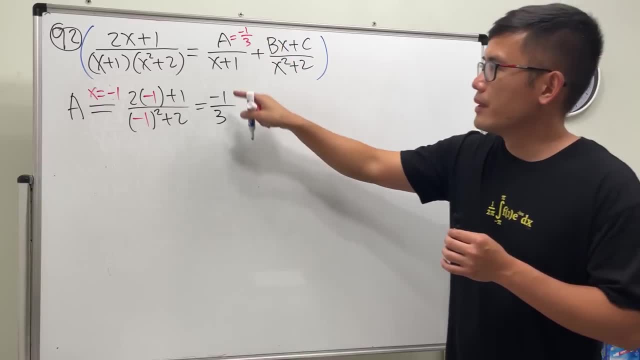 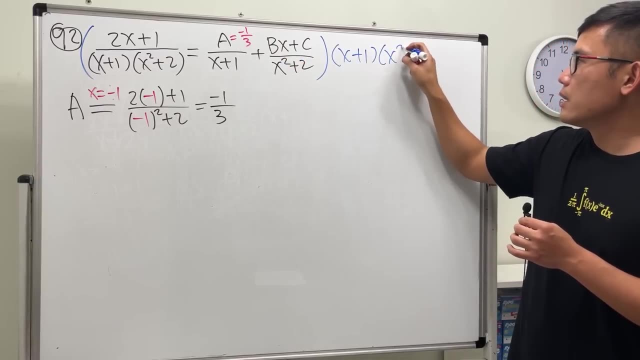 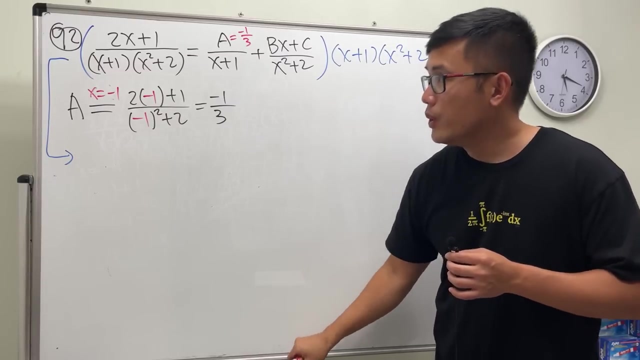 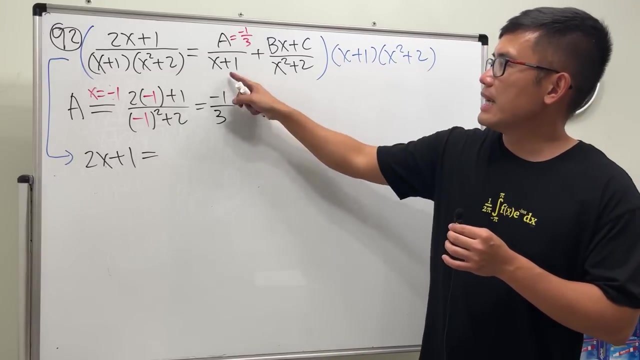 Multiply everybody by the whole denominator This and that, Just this and that, The whole common denominator Right, Right, So that we will see the left-hand side is 2x plus 1.. And then the right-hand side. Take this times that the x plus 1 cancels. 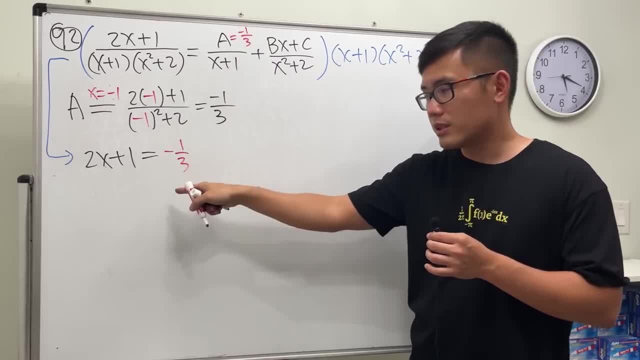 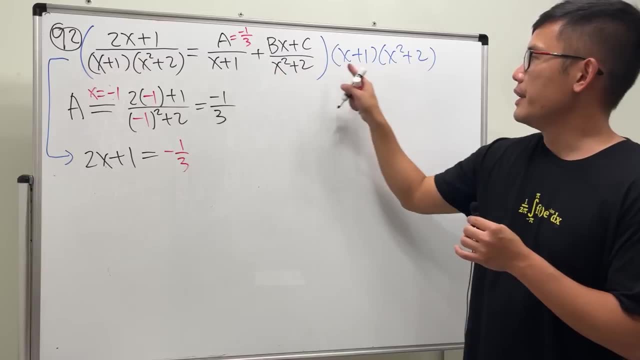 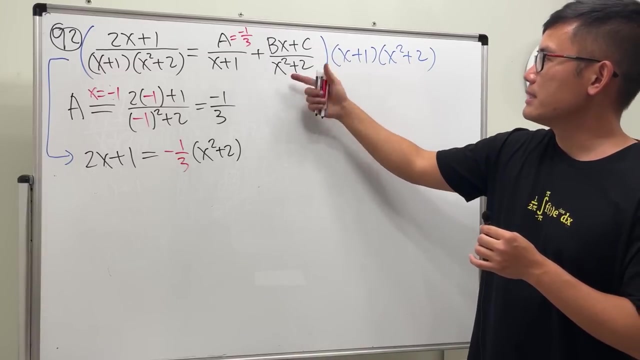 So we have the negative 1 third. We know the a already, so definitely use the cover-up whenever we can. So negative 1 third. They cancelled it, But we still have to multiply by x squared plus 2.. Next we take this times that: 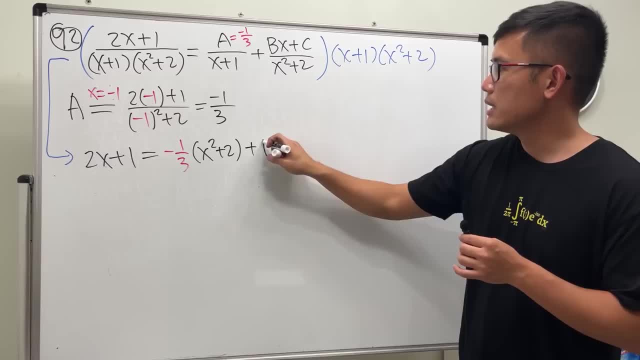 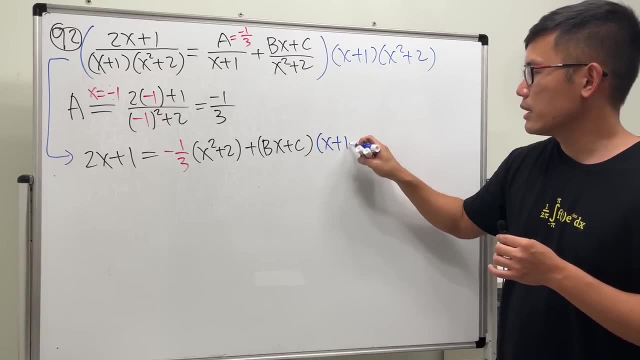 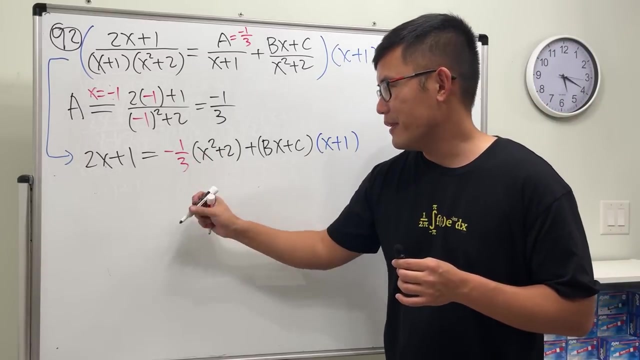 x squared plus 2, cancel, But we still have the plus bx plus c times This, This, which is x plus 1.. Okay, And then right here, we're just going to work out the right-hand side. So same thing. 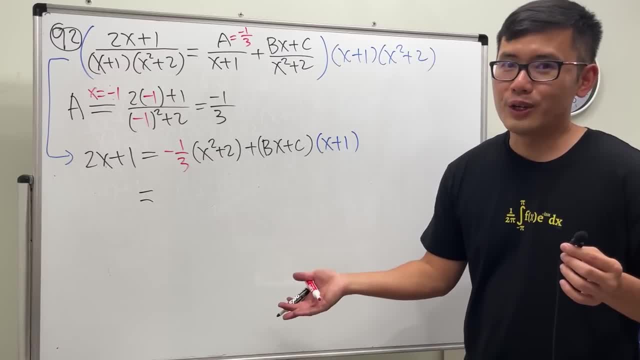 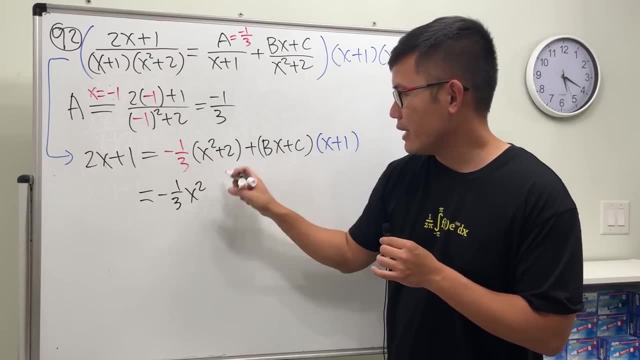 Distribute. and then I told you, this is the algebra drill, Just algebra, algebra, algebra. Whew, Alright, so this is negative 1 third x squared, and then minus 2 third. And for this, right here, just multiply this out. 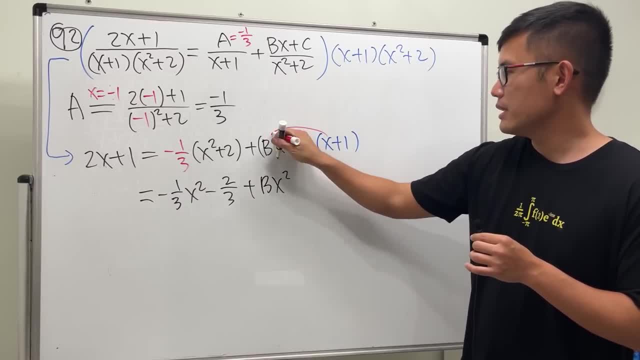 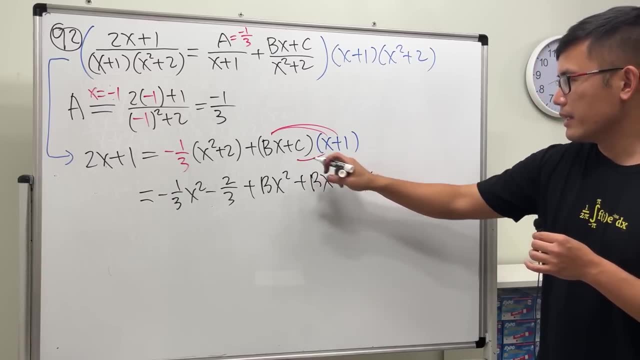 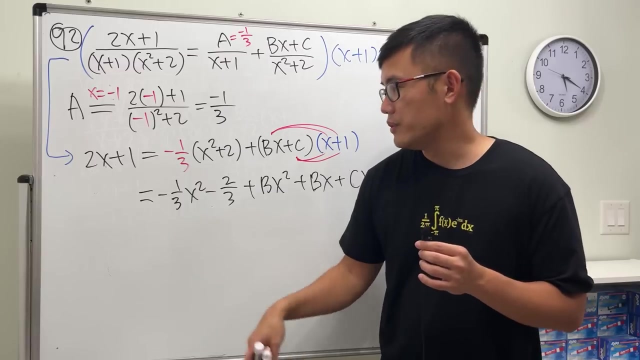 This is plus bx squared, And then, And then plus bx, and then plus cx, And then, lastly, we have the plus c, And then next step is we collect the coefficients. Notice this and that they both have the x squared term, right. 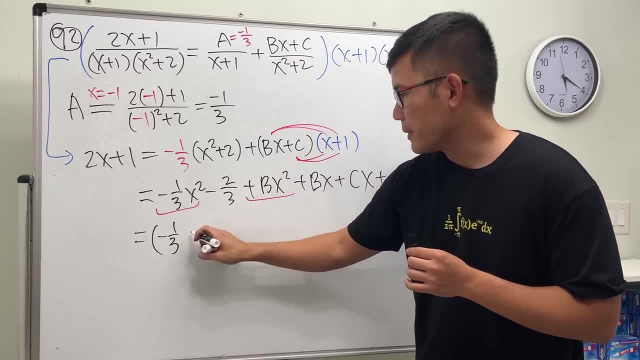 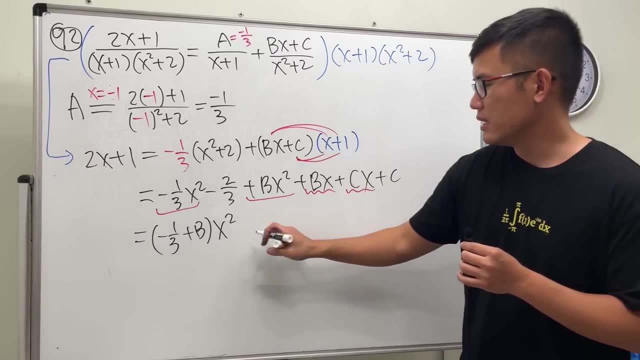 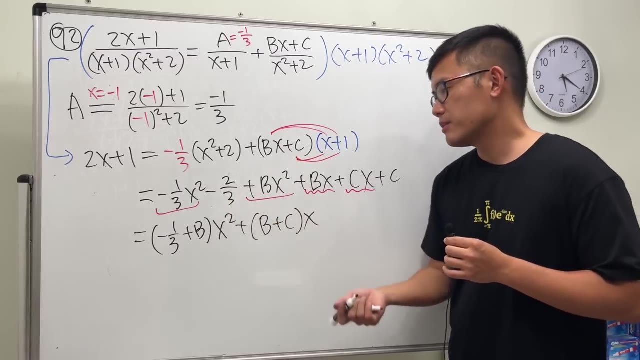 So we can put down negative 1 third plus b and then x squared. Next we have bx and cx, So we can say plus b plus c and x And lastly they are the terms with no x. So we can just say plus c minus 2 third. 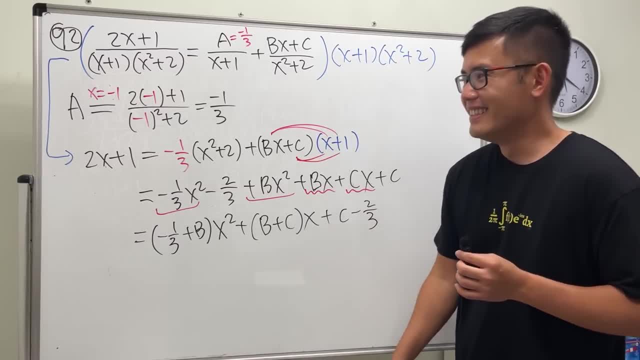 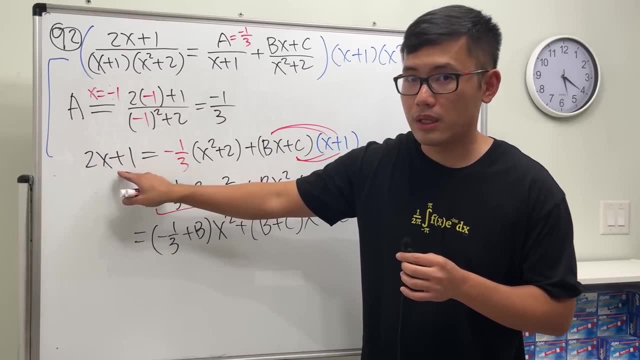 Now we're going to play a game called mix and match. Take a look at the left-hand side. Originally we just have 2x plus 1.. We do not have x squared, yeah, So technically that's 0x squared. 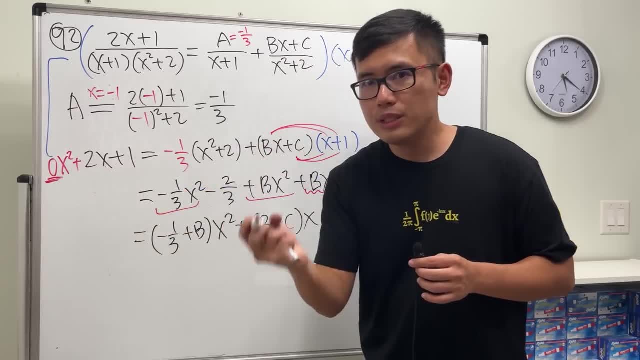 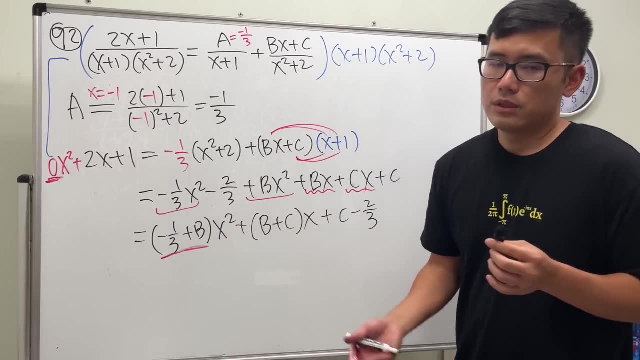 But you see, on the left-hand side we have 0 for the coefficient of x squared, But on the right-hand side we have this for the coefficient of x squared. So what does that mean? That means this must be equal to 0.. 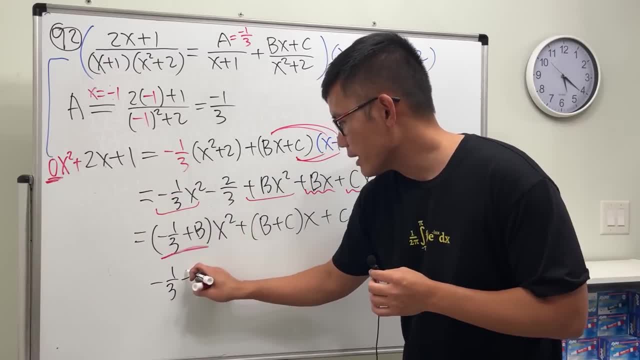 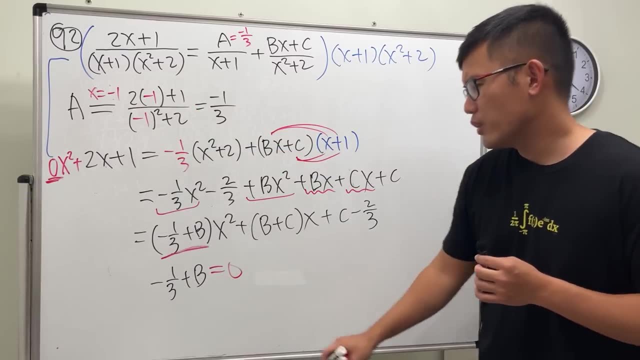 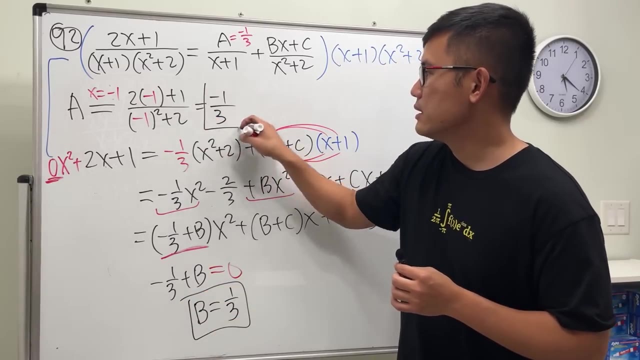 So right here, we must have negative 1 third plus b, It has to be equal to 0. Match the coefficient. Once we set this condition, we can solve for b. b is simply just 1 third. So a is this, b is that. 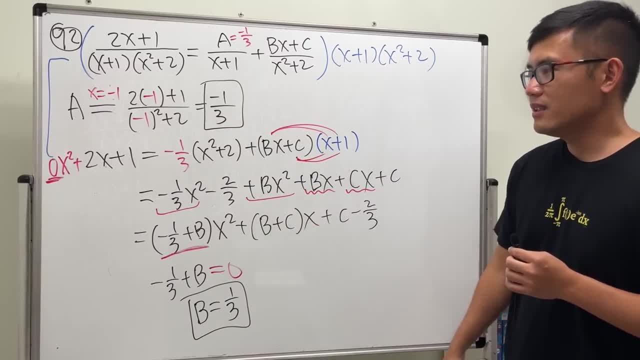 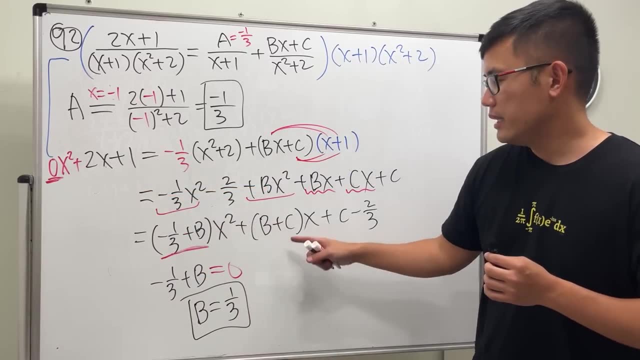 How about c? Well, it depends on how you like it. You can set up this to be 2.. We know b already. You can put it here, And then you can say: 1 third plus c has to be 2.. 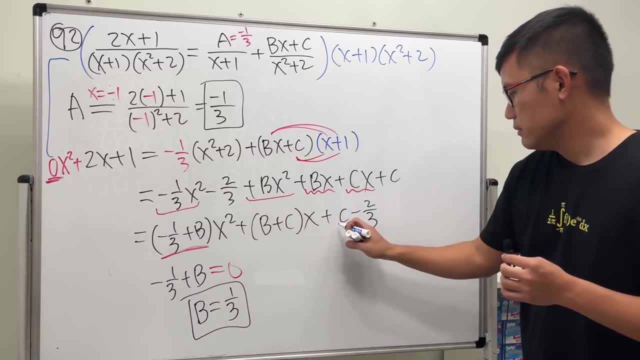 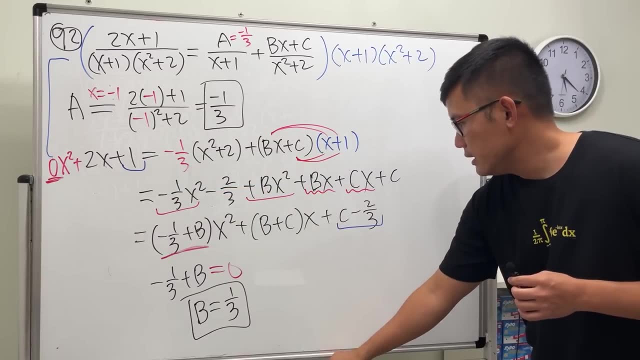 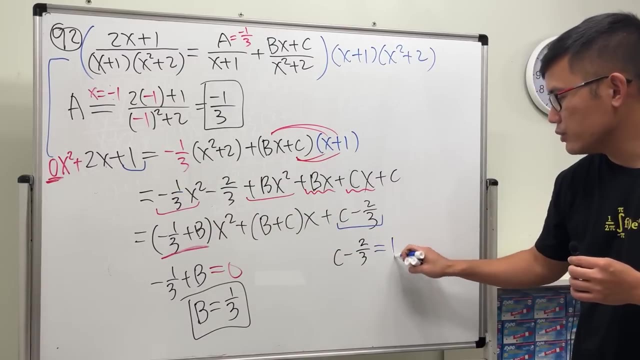 Or we can also use the last term, Constant term here, Constant term here. So this means c minus 2 third has to be equal to the constant term on the left-hand side, which is 1.. And if we have this, just add the 2 third on both sides. 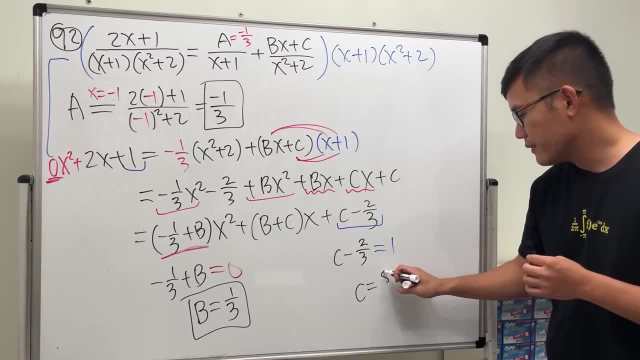 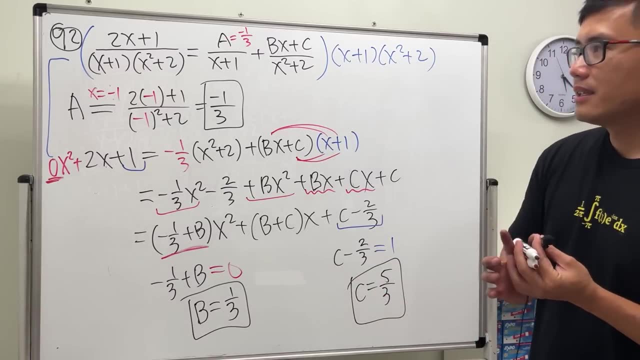 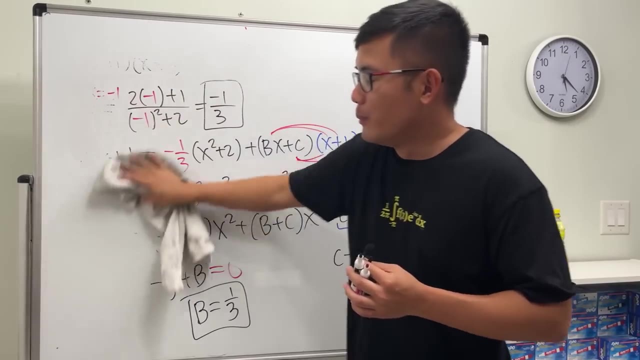 So c equals 1 plus 2. third is 5 over 3.. Yeah, So that's it. Yeah, that's it. I thought the algebra told you, The more comfortable you are with algebra, the better time you will have in calculus. 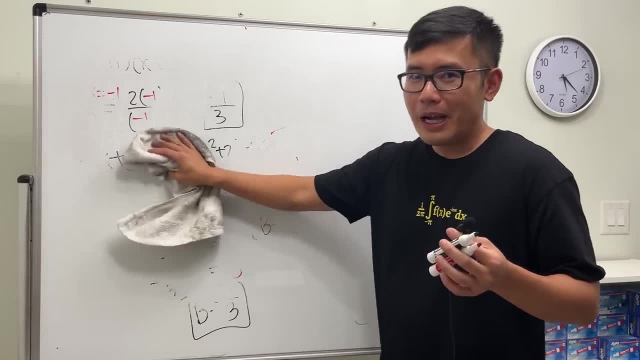 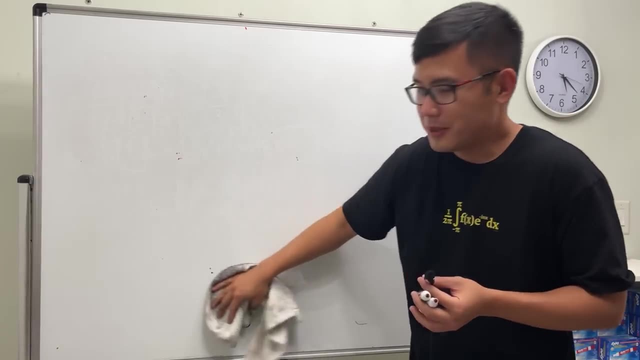 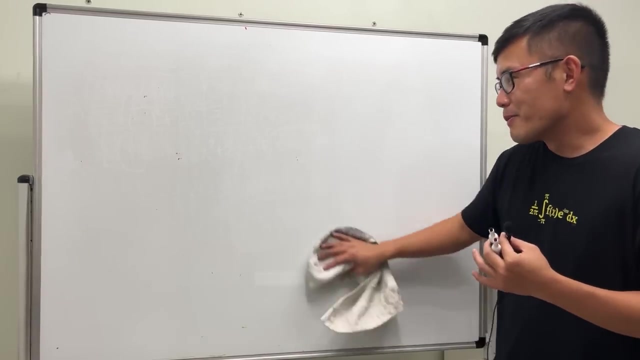 I know some of these are super long, But you know I'm doing this with you guys. Maybe you don't need to listen to all my explanations because they are just algebra right, But hopefully this video can inspire you to actually just practice your algebra skill and then pay more attention to your algebra. 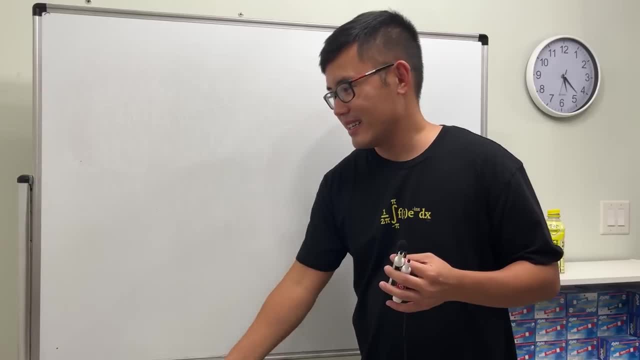 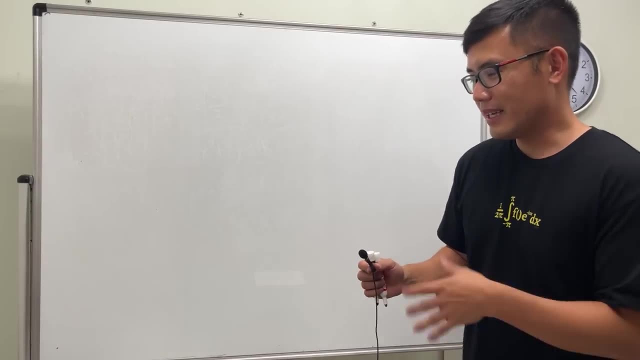 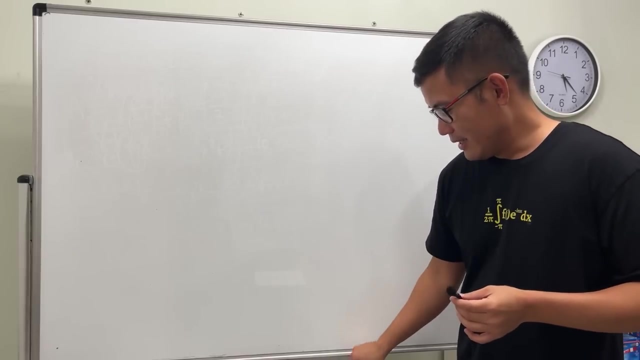 And Yeah, Just like a little encouragement for you guys. That's my goal. Hopefully this right here is not teaching you guys anything new. It's just like telling you guys that you should practice this, this, that, And it's just a lot of work. 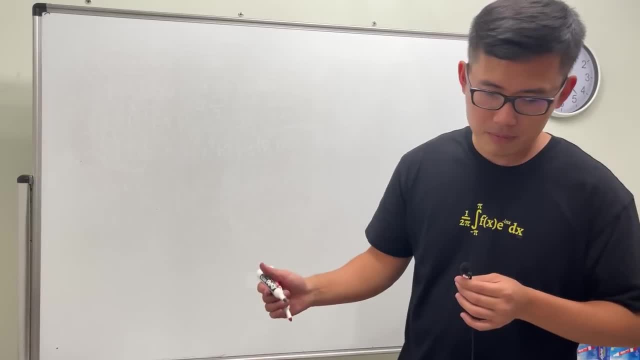 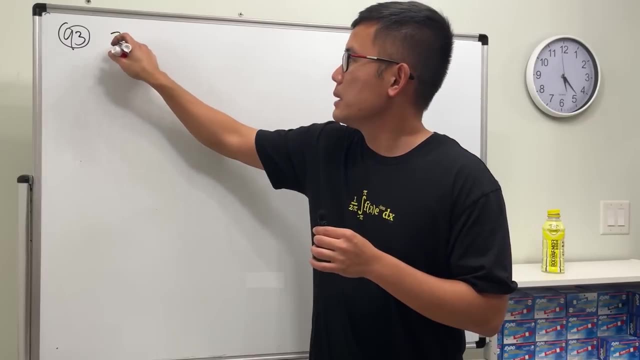 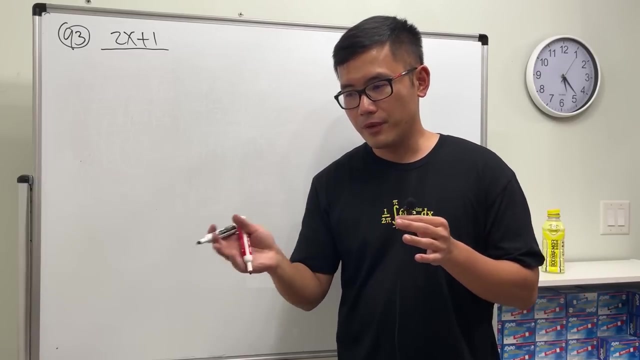 I know. Okay. next one, Number 93.. We have 2x plus 1.. Again, same numerator, Because I have that video talking about how to break down the fraction. that's why I'm using the same exact numbers. 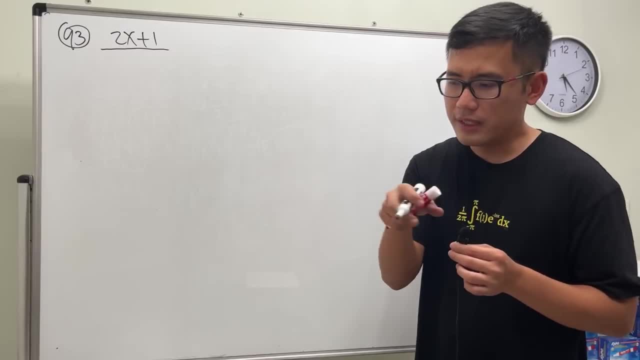 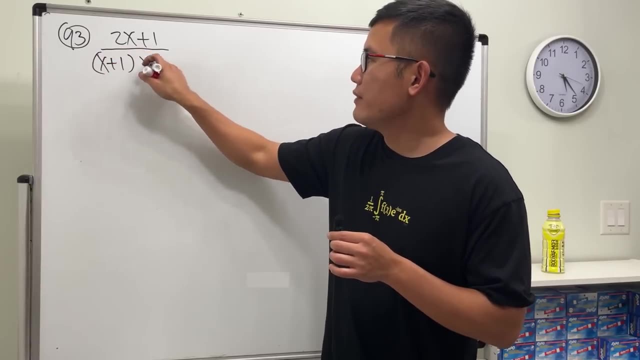 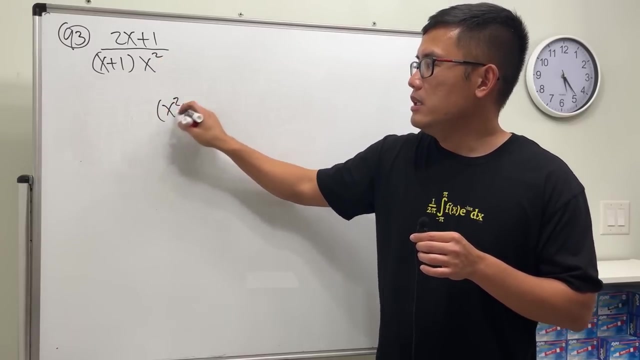 And then it's just how you pay attention to the denominator. By the way, first we still have x plus 1. But here we have x squared. Notice this is x squared, unlike x squared plus 2.. Earlier, this factor was not factorable. 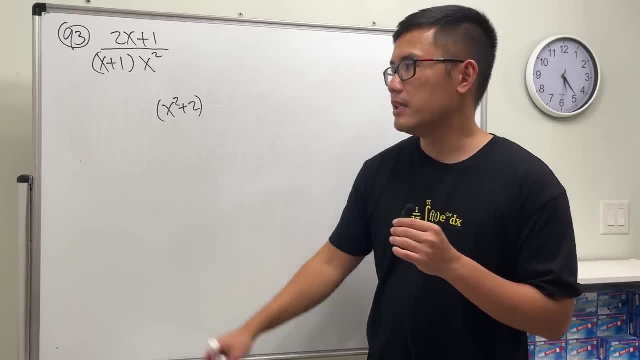 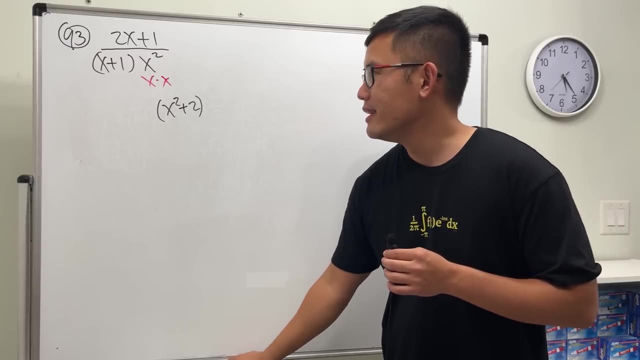 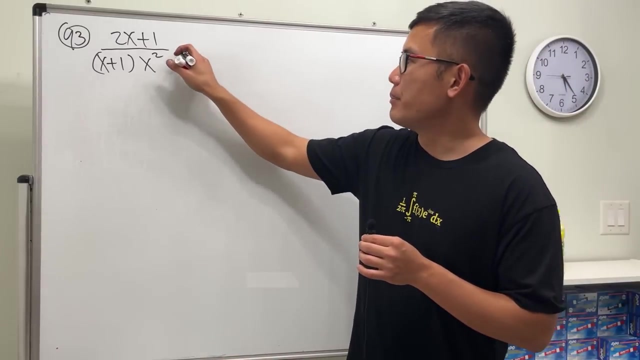 But this right here is Because technically x squared is the same as x times x, Meaning just x Multiply yourself twice. It's kind of factorable. It's called a repeated factor. Okay, But I will tell you we can break this apart as. 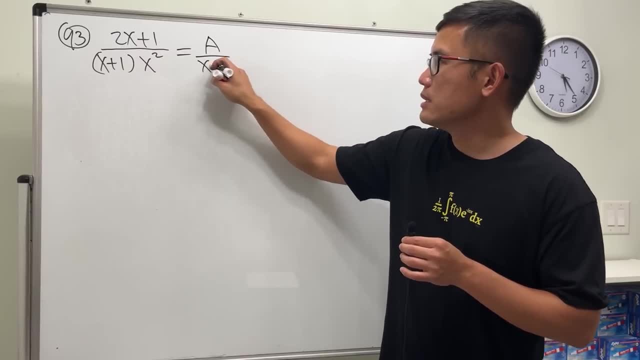 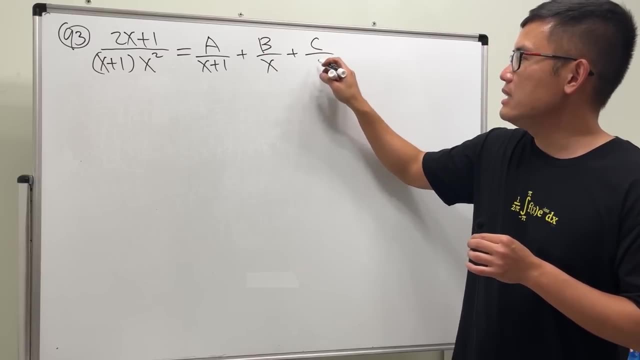 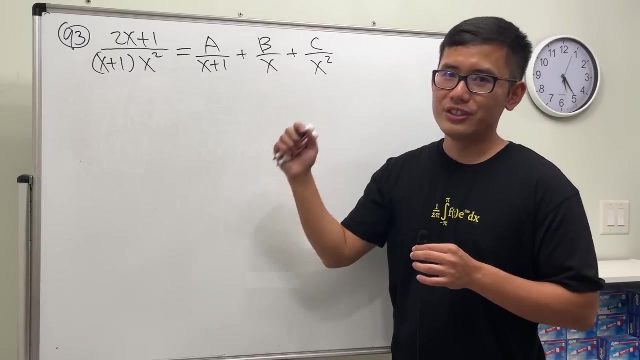 some number a over x plus 1.. And then plus some number b over just x, And then some other number c over x, squared. You might be wondering how did we end up with this right here, right? Well, you can check out my other video to see how we break down the partial fractions. 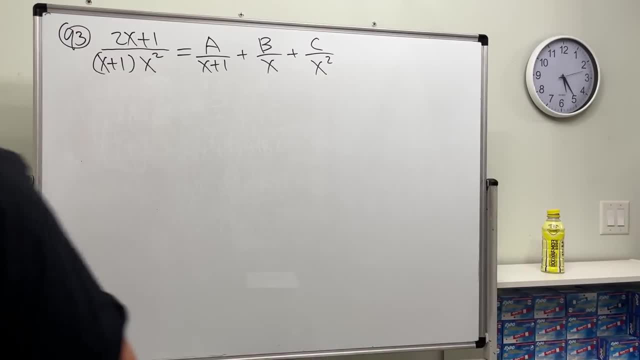 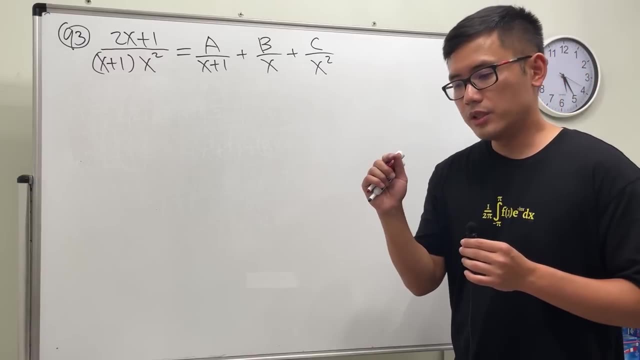 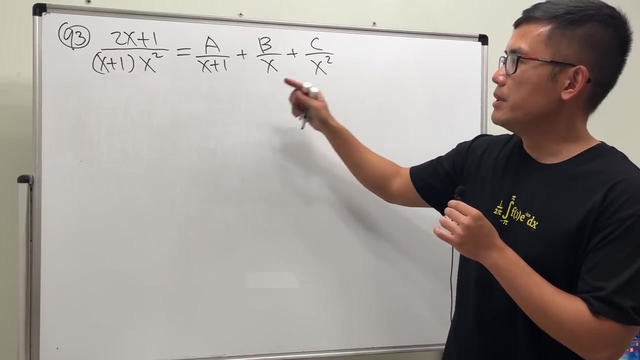 Hold on, let me just take a look at the Good- All right Good news for you guys. We can solve, for We can use cover-up for two letters. They are a and c Because this denominator happens from the original. 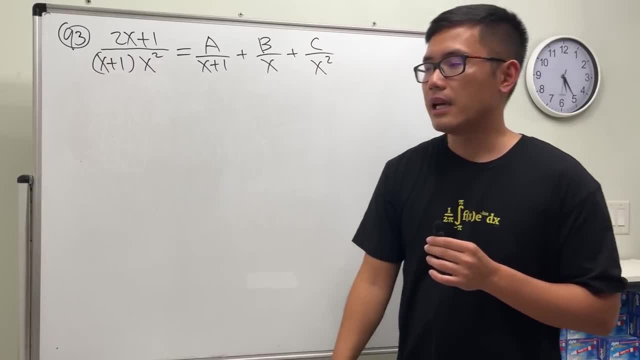 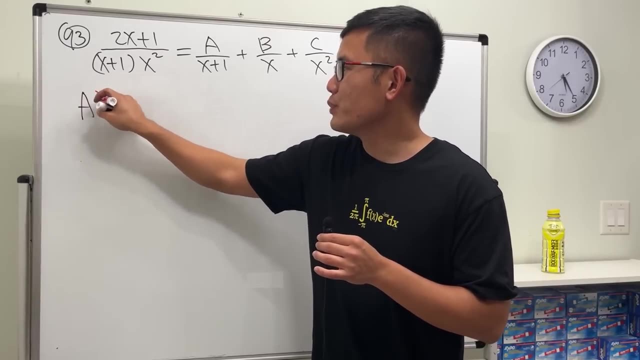 And we have the same thing right here. Yeah, So whenever we can use the cover-up, go ahead and use it. a will be. You guessed it. x will be equal to negative 1. Put it here. Put it here. 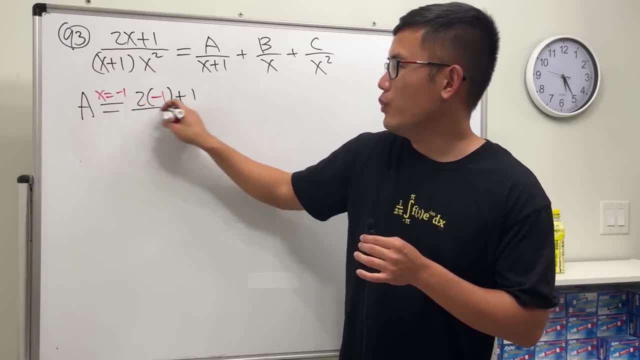 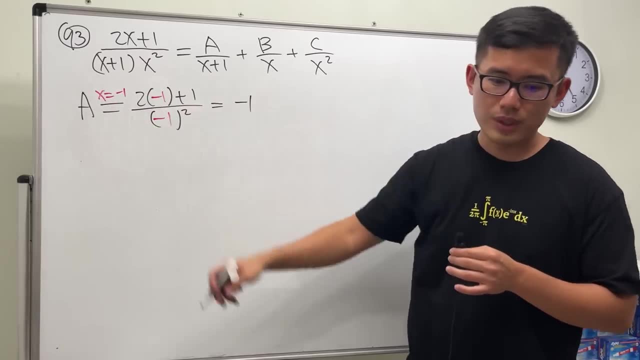 So we have 2 times negative, 1 plus 1 over negative 1 squared, That's negative. 2 plus 1 is negative, 1 over 1.. Just negative 1.. Yeah, And then let's also do the c here. 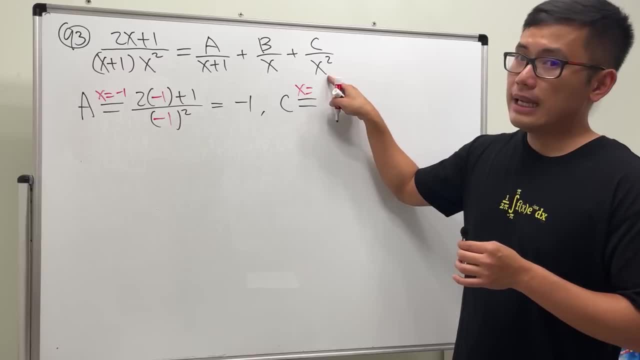 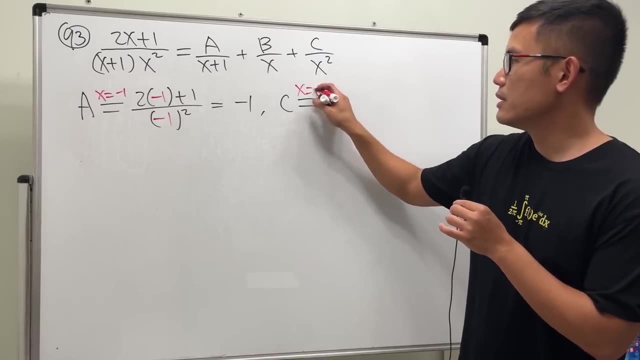 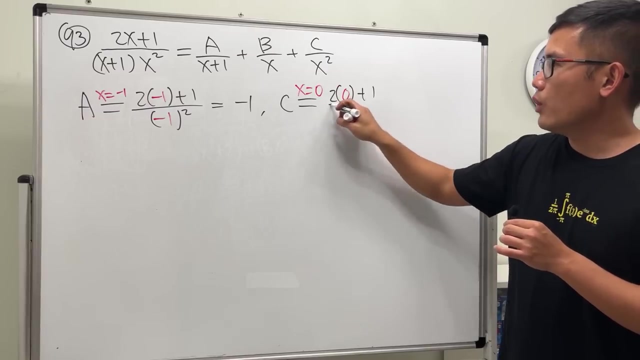 c equals. This has x squared. I come here, I cover this. How can we make x squared equal to 0? x has to be 0. Yeah, And we put 0 here and here. So we have 2 times 0 plus 1 over 0 plus 1.. 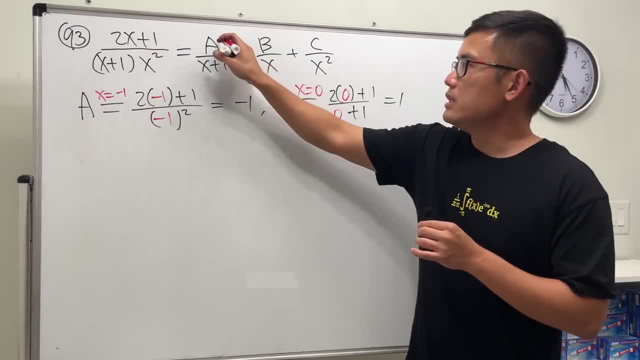 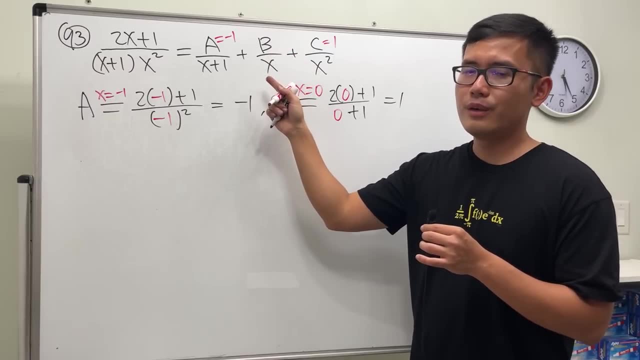 And that's just equal to 1.. All right, So we see a is equal to negative 1 and c is equal to 1.. And you might be wondering how come we cannot do cover-up for b. Well, this is only x to the first power. 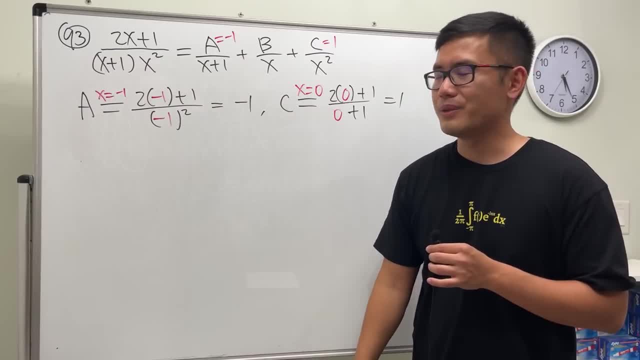 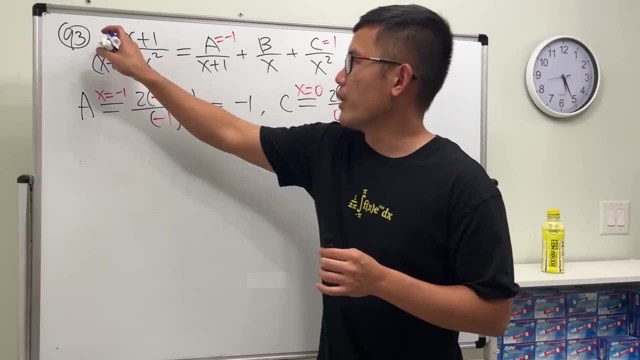 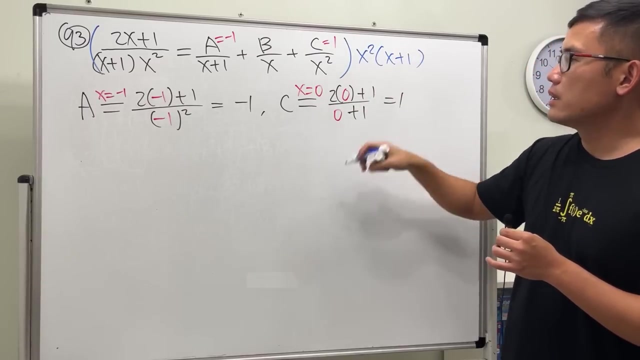 If we use 0 here, We used it already. No, No, we cannot do cover-up for b, So let's do it the traditional way. Let's multiply everybody by the denominator x, squared x plus 1.. So on the left-hand side. 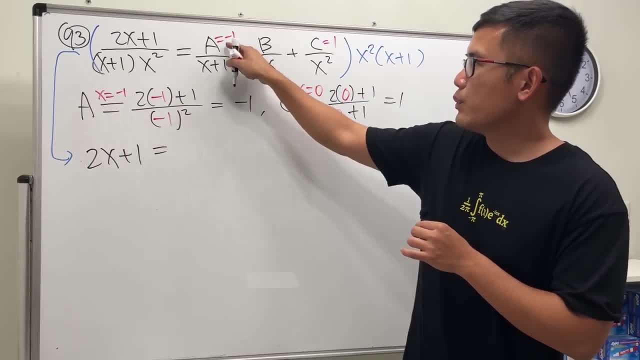 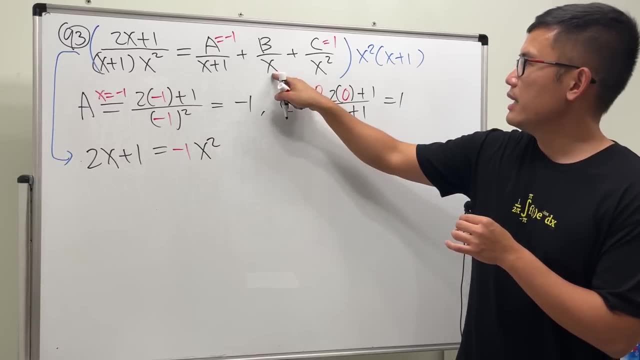 we get 2x plus 1.. On the right-hand side we have the negative: 1. This and that cancel, And then we multiply by x squared, And then next x and x, just cancel. one of them, right. And then the b. we still don't know. 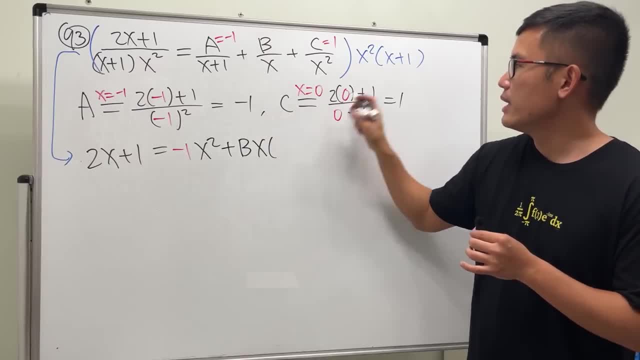 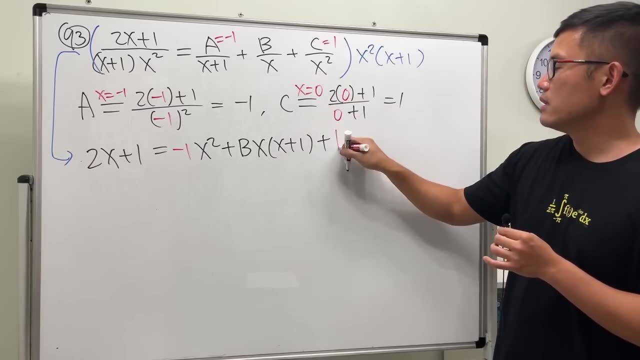 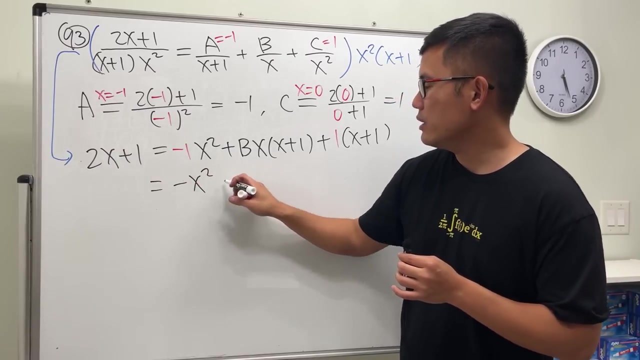 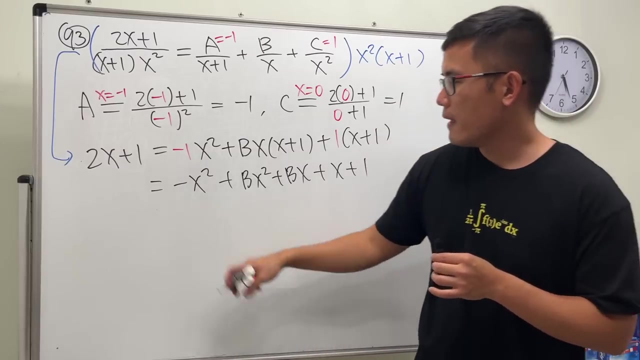 So plus bx, And then one more term which is x plus 1.. Then this and that cancel c is 1.. So we just have that And then work out the right-hand side. So this is negative: x squared plus bx, squared plus bx, and then plus x plus 1.. 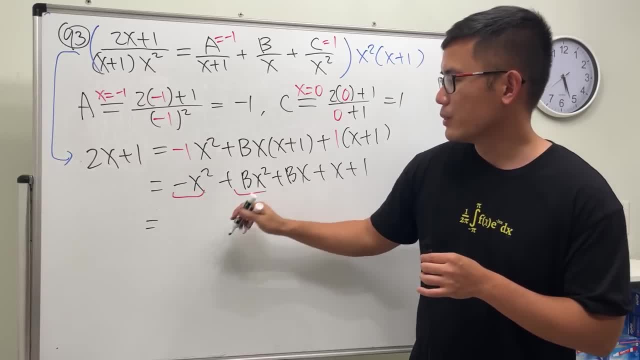 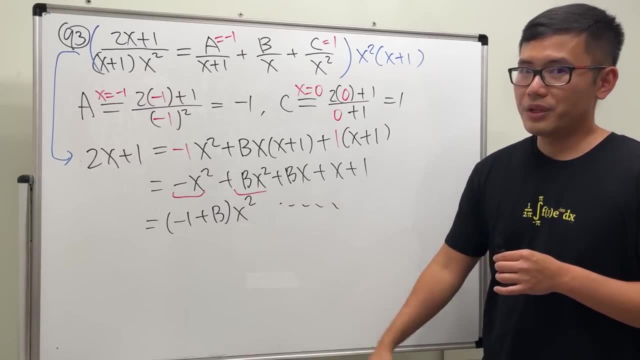 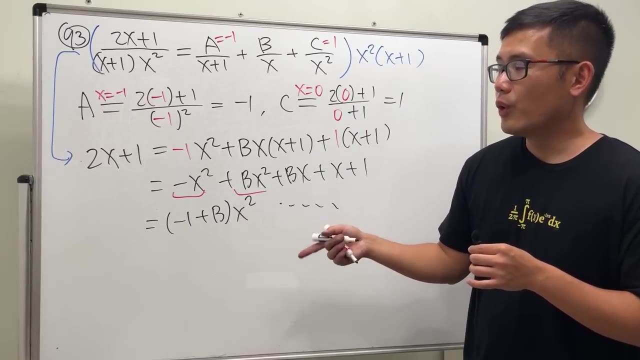 Here you see that we can combine this and that, which is just negative 1 plus bx squared, And we don't need to care about the rest, Because when we have this right here, when we have this right here again, the left-hand side is 0x squared. 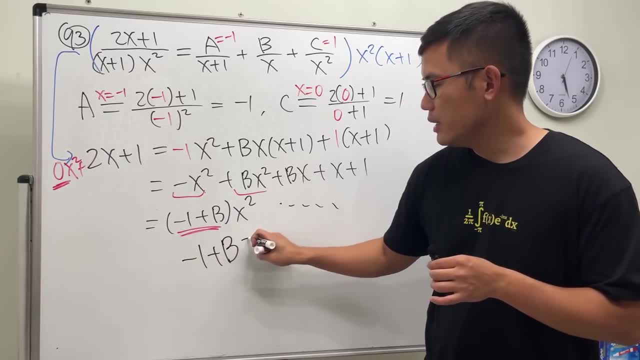 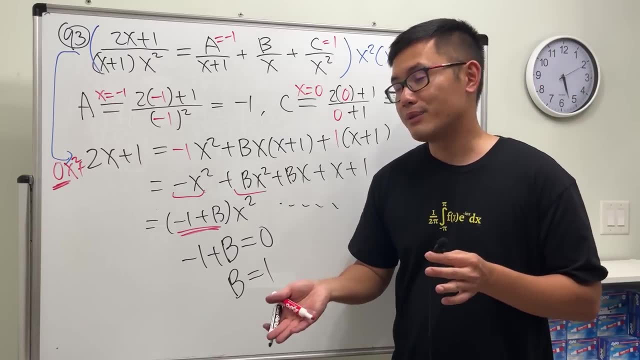 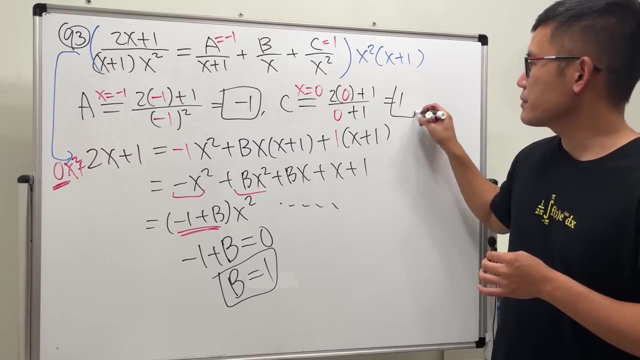 So we must have negative 1 plus b equal to 0, meaning b has to be equal to 1.. Once we have this, we are done. We don't have to continue with the rest. So a is negative 1.. b and c happen to be 1 in this case. 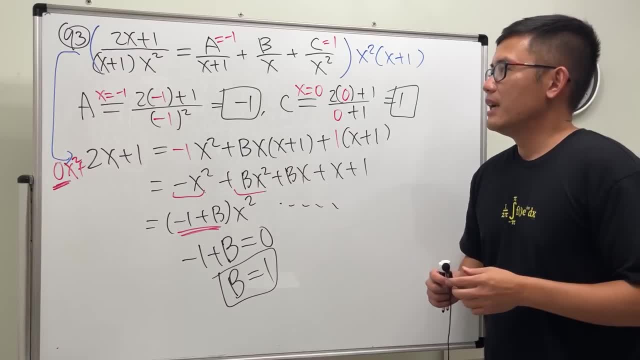 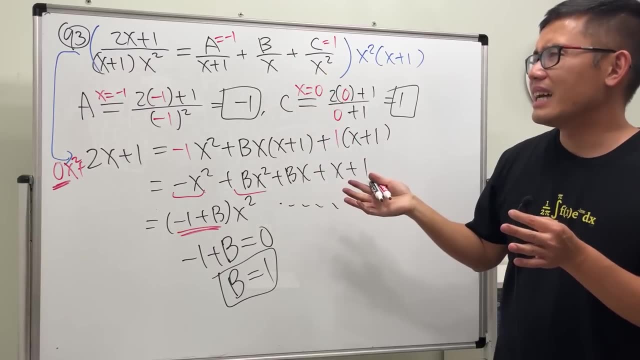 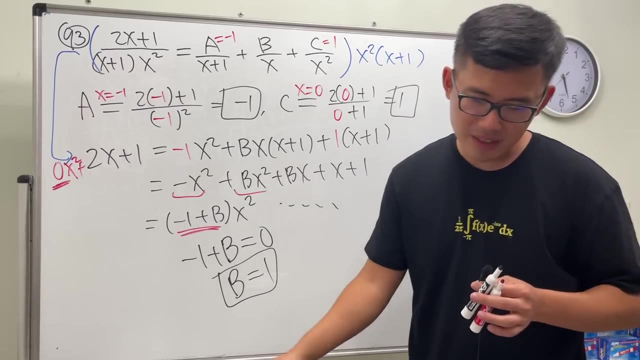 Yeah, it just happened to be the same number, But we cannot do cover-up for b. We couldn't do cover-up for b, Even though it seems like, yeah, just a coincidence for that. Just a coincidence for that. You'll see the next one. 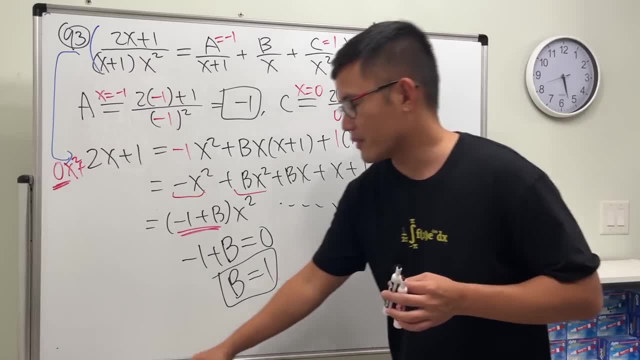 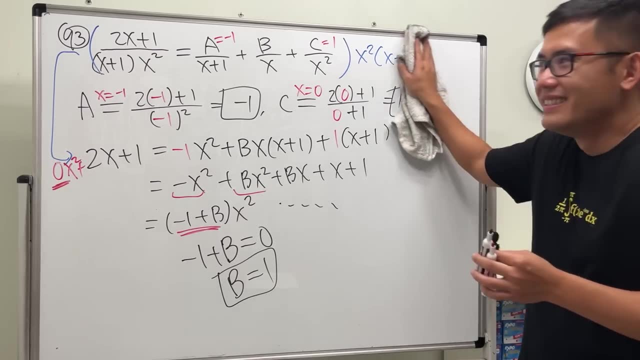 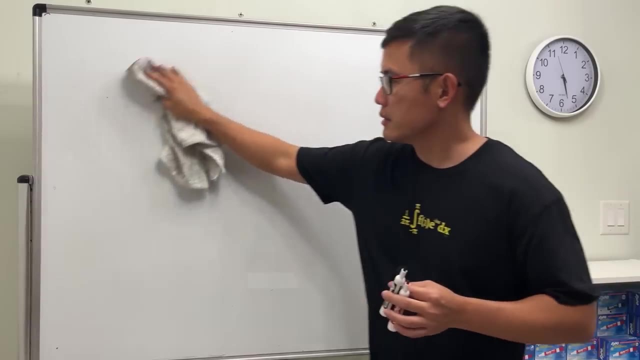 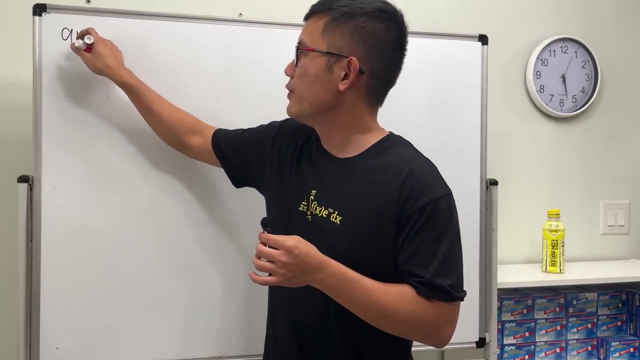 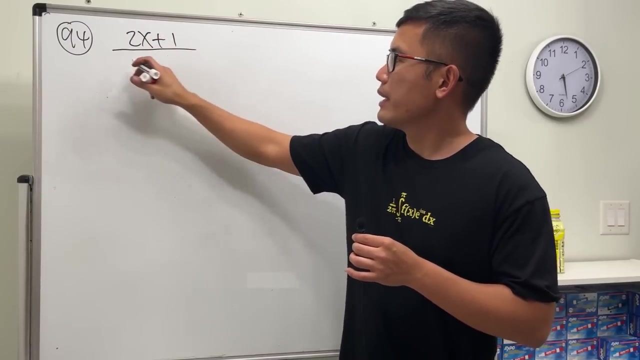 It's very similar And then we cannot do cover-up. It's tiring 5.30.. All right, Number 94.. We have again 2x plus 1 over here. we have x plus 1 again. 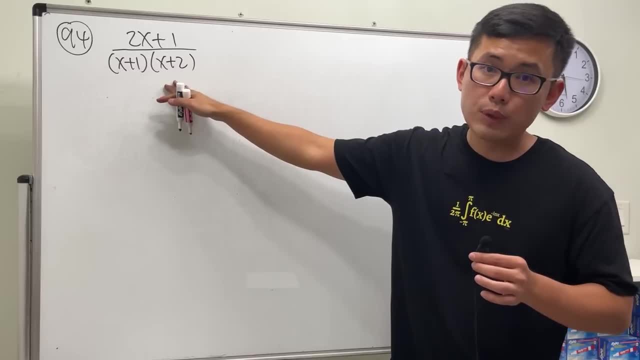 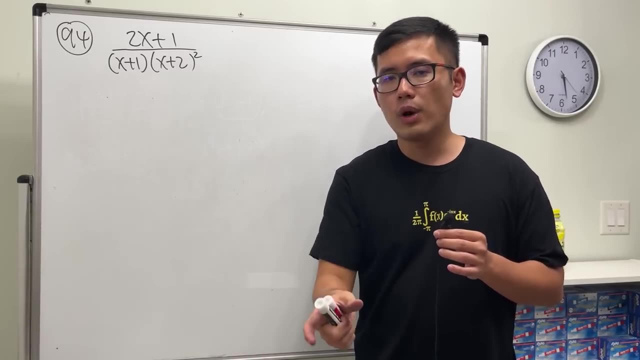 And then, instead of x plus 2, because this is actually equation 91, right now we have the second power. So this right here means x plus 2 happened twice. If it's happening twice, then we will have to build up the power. 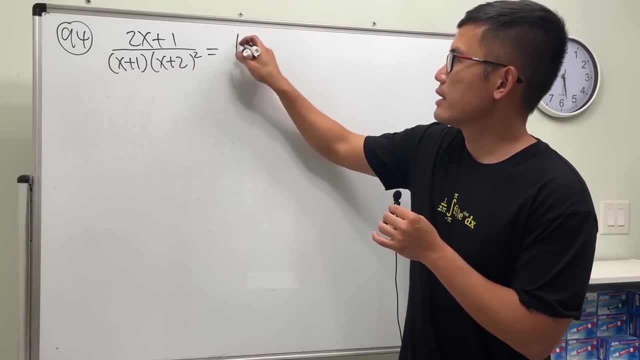 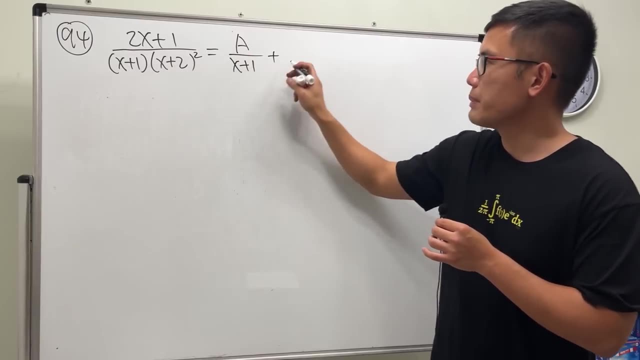 when we set up the partial fraction, So it looks like sum number a over the first denominator, which is x plus 1. And then build up the power starting from this to the first power, So x plus 2.. And then go up one more time. 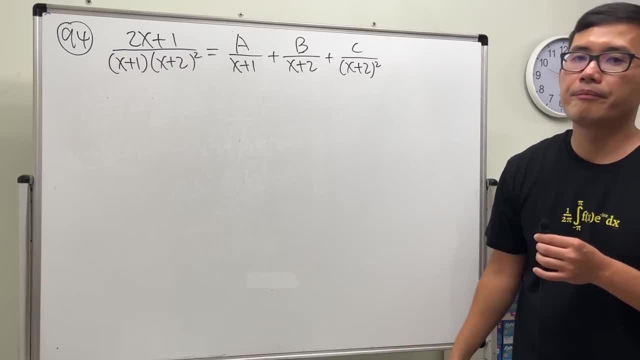 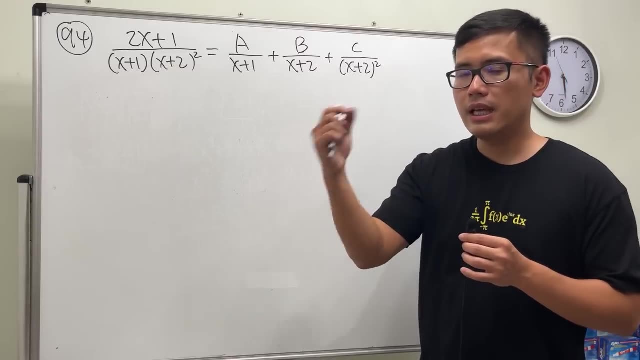 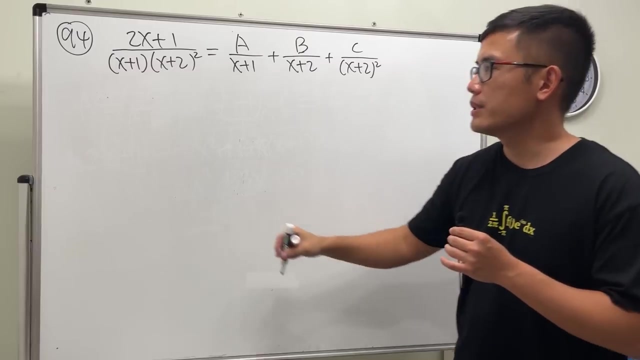 x plus 2 square and then c. Yeah, Okay. So you see, this is similar to what we had earlier. Right, We built up the power. earlier was x and x square. We can use cover-up for a and c. Let's go ahead and do it. 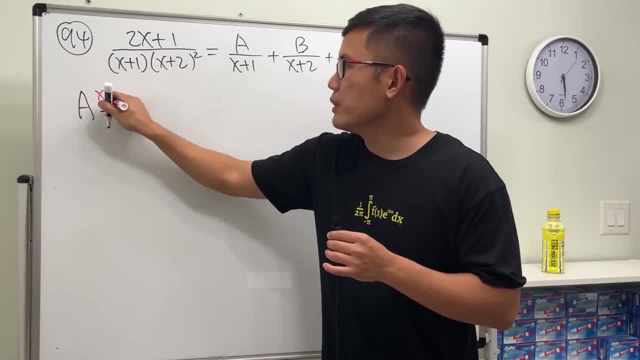 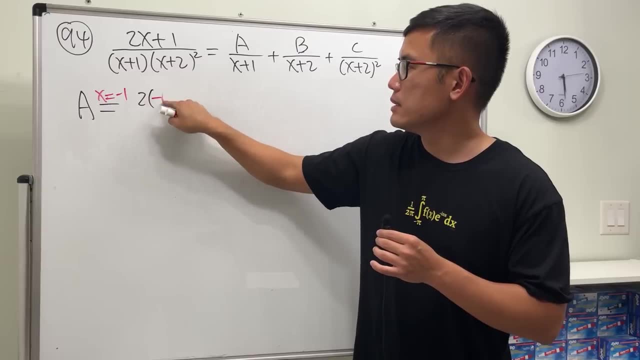 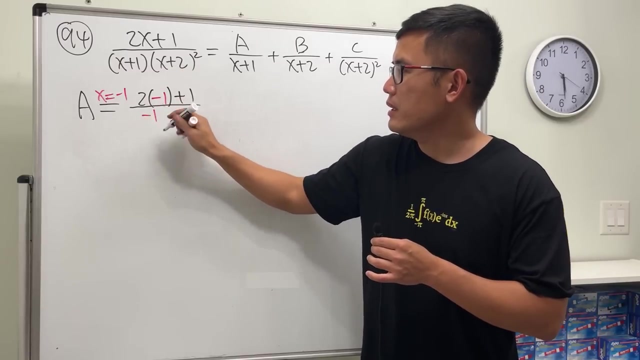 a will be when x equals negative 1.. Put it here. Put it here, So we have 2 times negative 1 plus 1 over. put negative 1 here plus 2 and then square, That's negative 2 plus 1.. 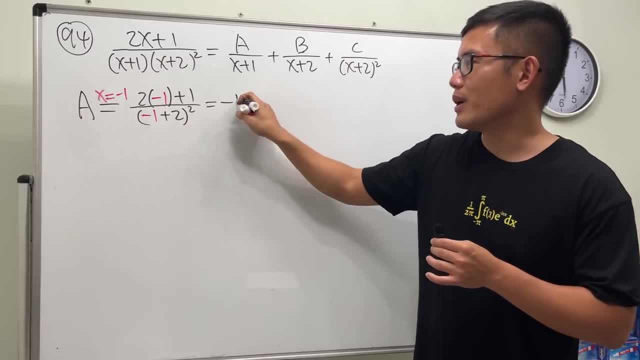 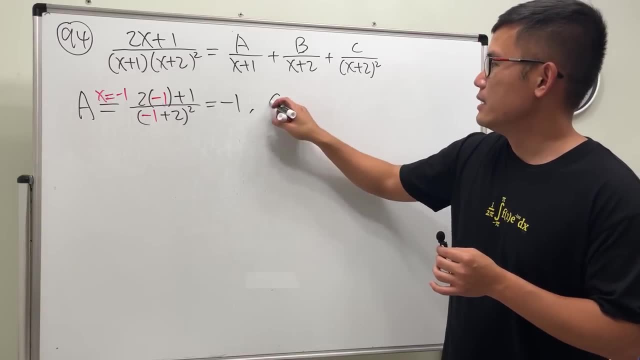 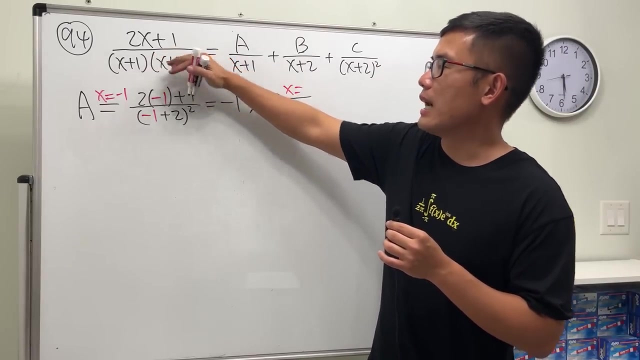 Negative. 1 on the bottom is 1.. So it's negative 1.. a is negative 1.. Okay, And then c equals when x equals negative 2.. Right, Come here. Cover up the whole denominator: c is equal to negative 2.. 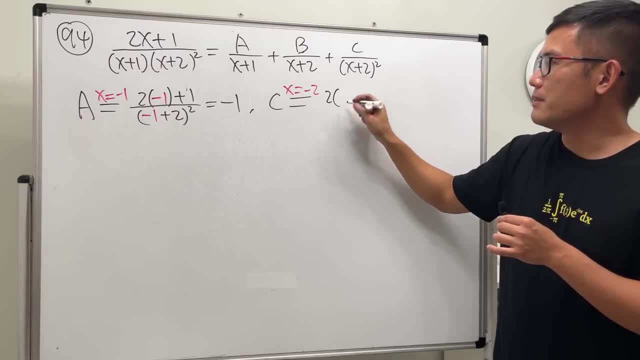 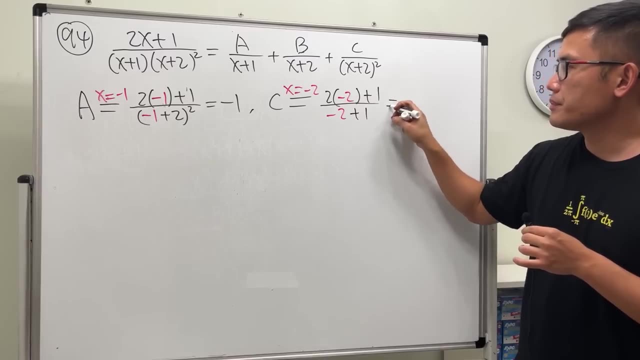 Cover this up, but you put the negative 2 here and here. So we have 2 times negative, 2 plus 1 over negative, 2 plus 1.. That's negative 4 plus 1 is negative, 3 over negative 1.. 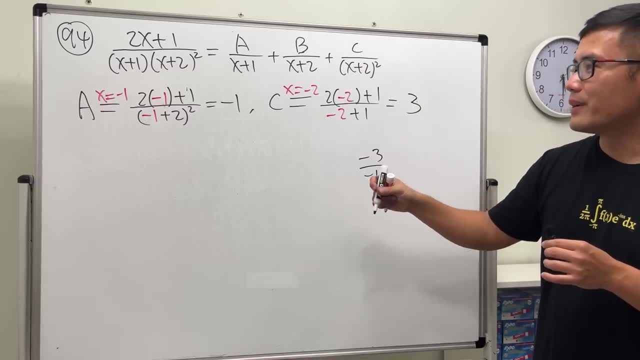 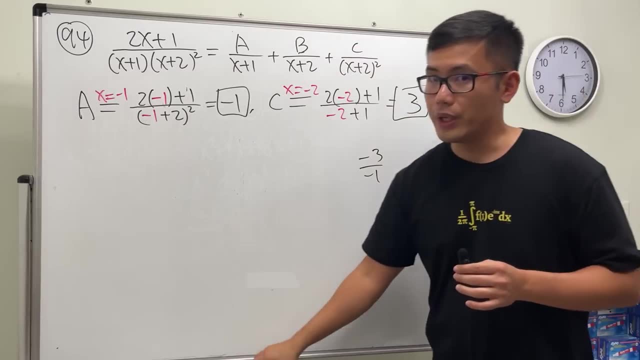 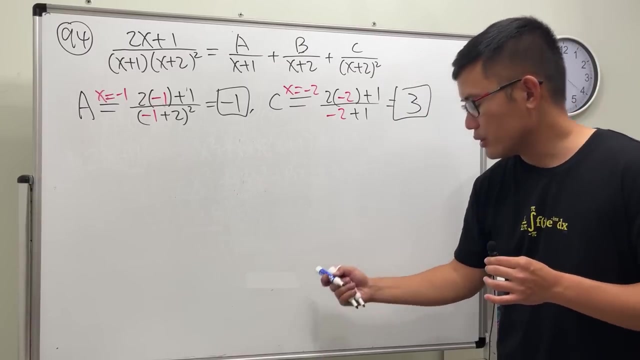 So c is equal to 3.. So we got our a and c already. Now to find b, we cannot use cover-up and it's not the same number as 3.. Okay, No, So let's just go ahead and do the traditional way. 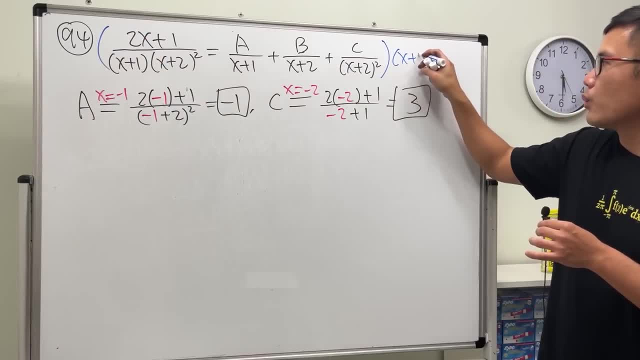 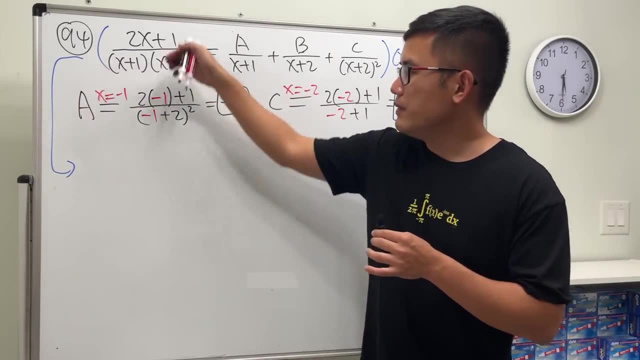 Multiply everybody by x plus 1 times x plus 2 square. Okay, Let's see what this is going to give us. Define side, we still have 2x plus 1.. This times that the x plus 1 cancel. 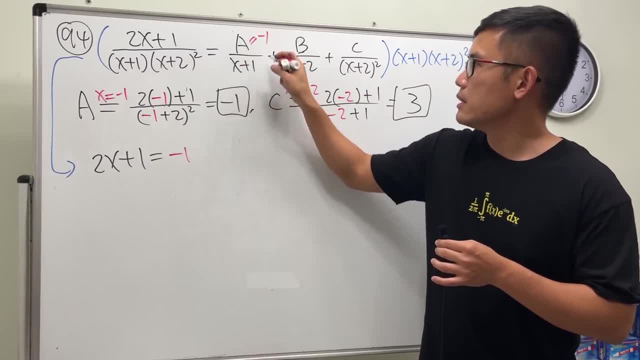 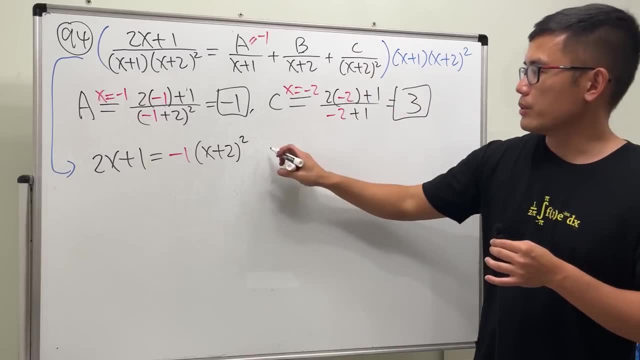 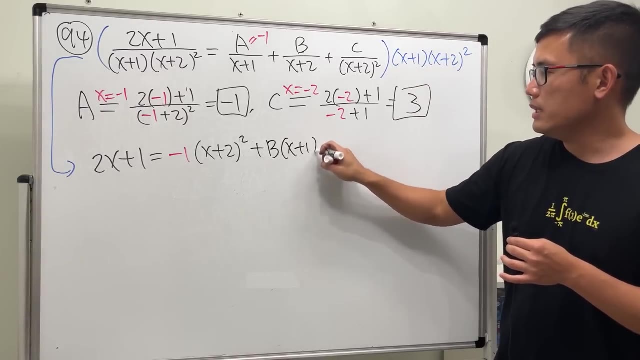 a is negative 1.. So negative 1 times this, which is x plus 2 square b. we don't know. so keep it x plus 2, cancel one of them, but we have this term, which is x plus 1 and then x plus 2.. 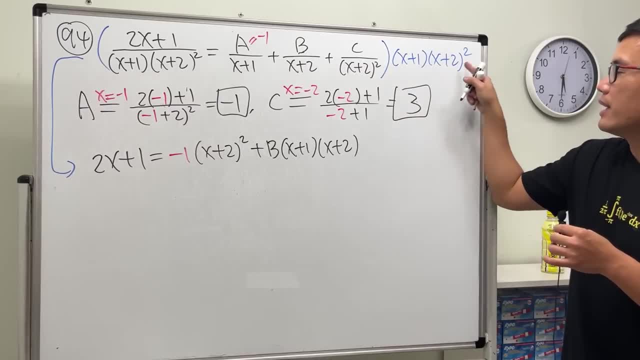 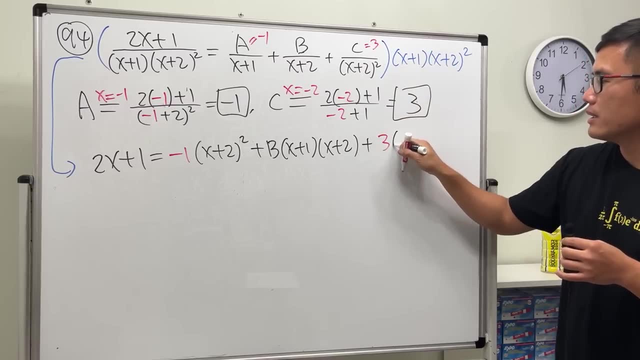 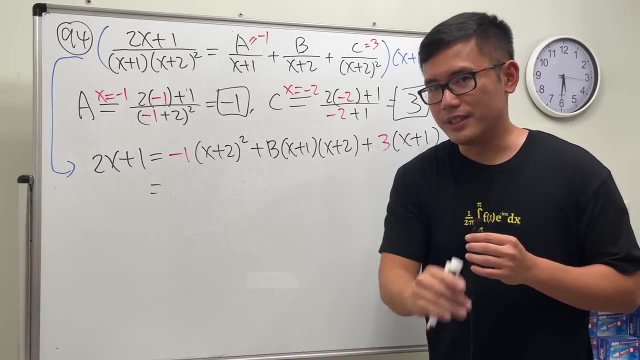 And then x plus 2 square cancel. So we have c, but c is 3.. So we'll just say plus 3 times x plus 1. And work out the right-hand side. So let's do this in our head. 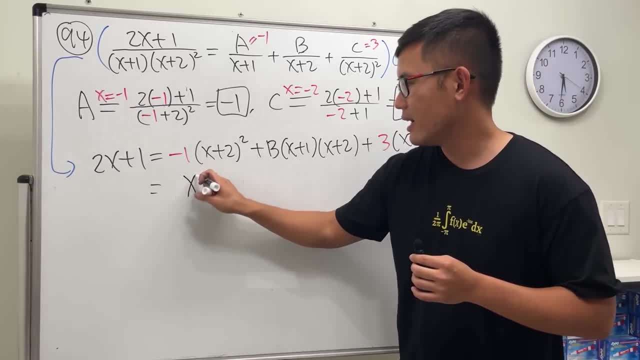 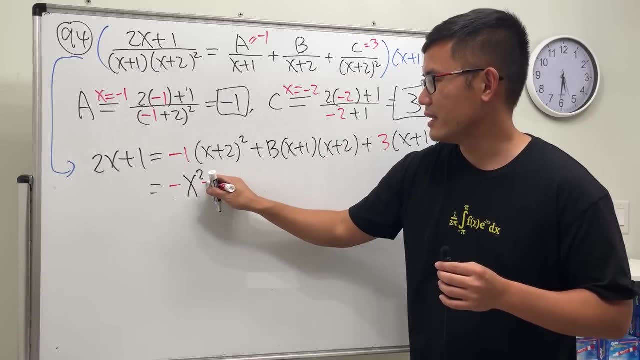 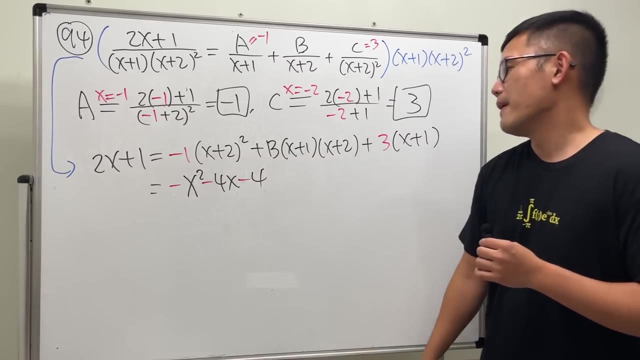 Open this, we get x square, But negative, Plus 2 times this and that which is 4x, But negative. Lastly, plus 4 square, but you change that to negative. Okay, All right. Next x times x is x square. 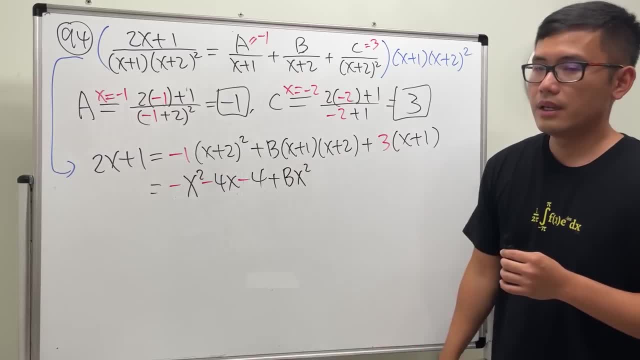 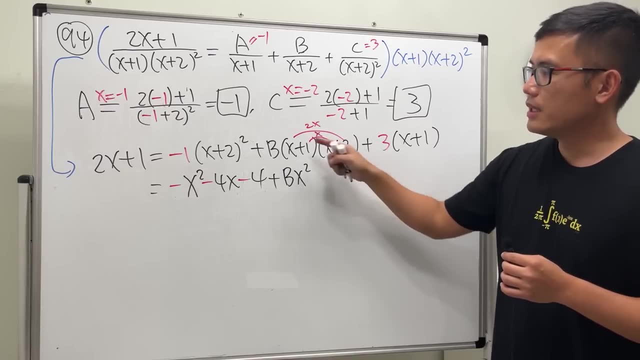 but we have the b, So bx square. Next, This times this is 2x And this times this is x, All together with 3x, 3 times b, so plus 3bx, And then, lastly, 1 times 2 is 2,. 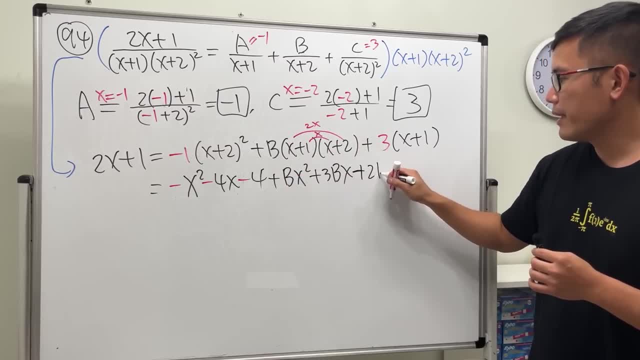 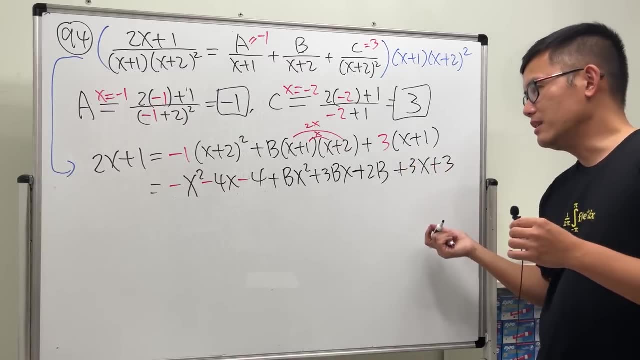 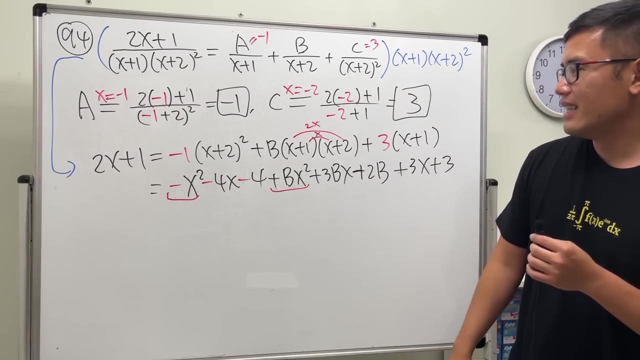 but times b, so plus 2b, And in fact you don't need the last one, but might as well 3x plus 3.. And the reason is because, just earlier, in fact, we just care about this. 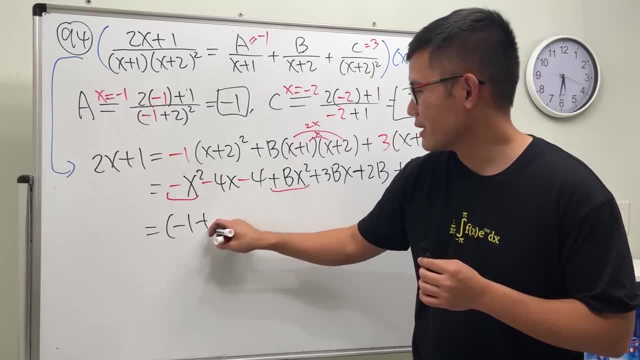 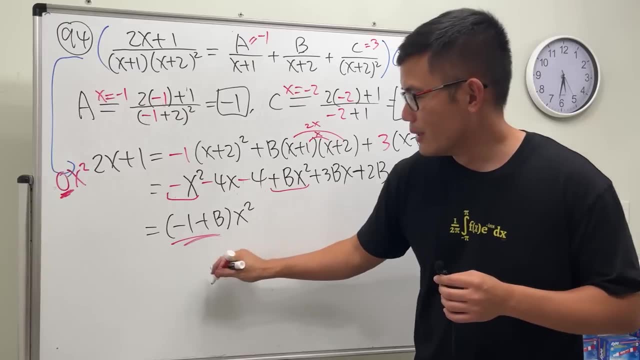 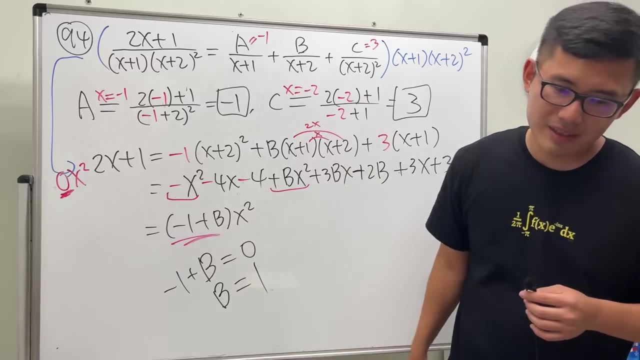 Yeah, Okay. So we get negative 1 plus b times x square And again 0x square 0. So b negative 1 plus b equal to 0.. b is equal to positive 1.. Yeah, This middle term is not always positive 1.. 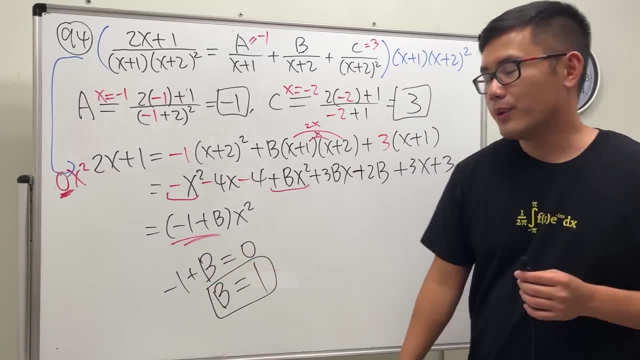 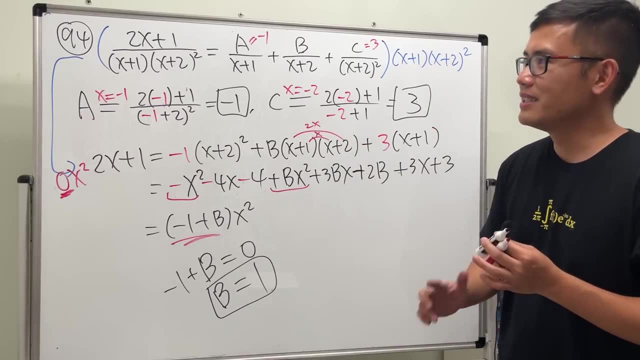 Okay, But I just want to tell you, But I do want to show you, that b and c, they are not always equal either. So this is how you, how to just set it and work it out. That was number 94.. 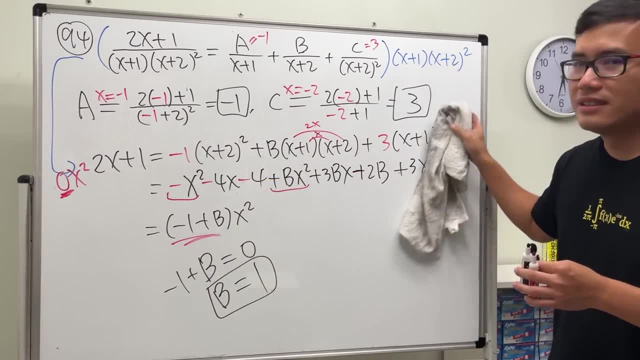 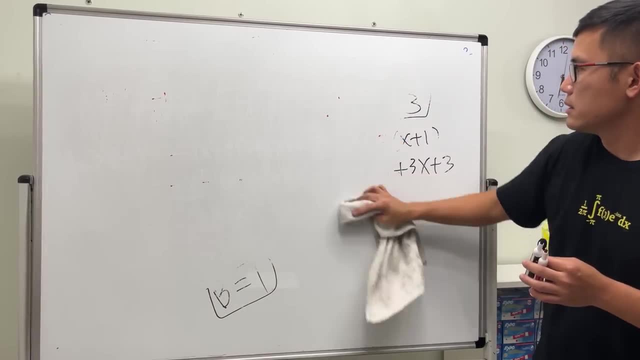 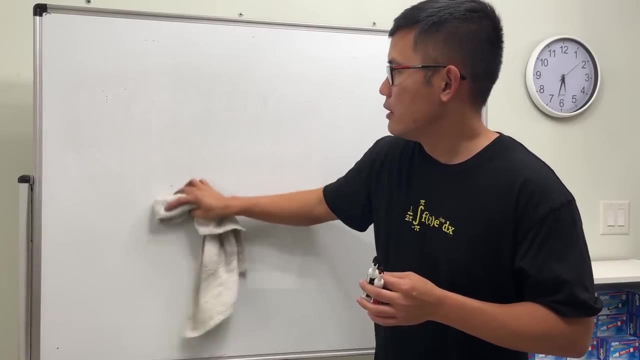 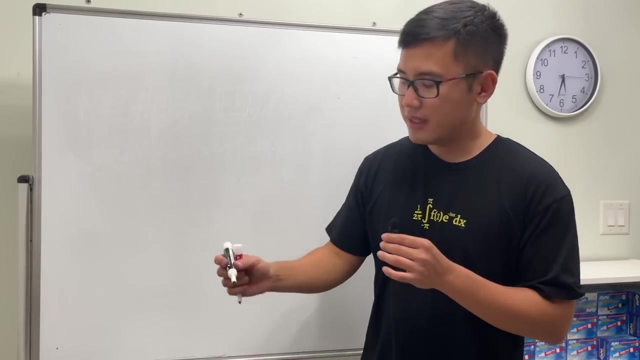 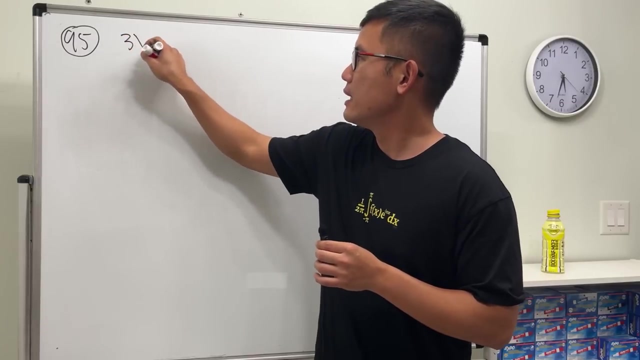 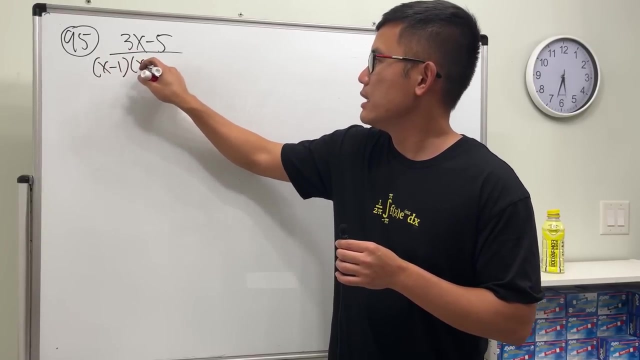 And then let me tell you we are going to move on to like some other numbers rather than these. All right, Number 95. Here we have 3x minus 5 over x minus 1, x minus 3, and minus with one more. 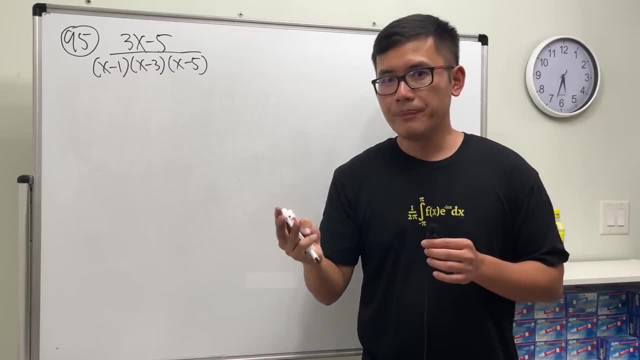 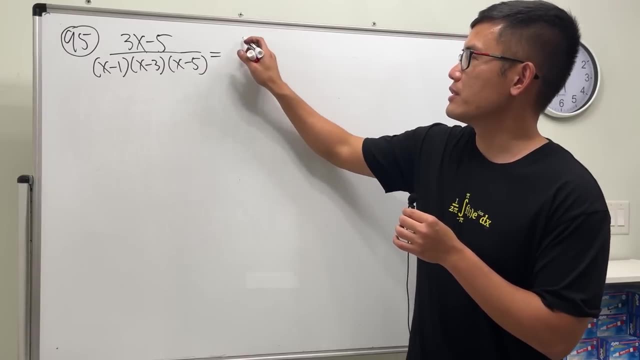 x minus 5.. And you see we have three distinct meaning, different right, Three distinct linear factor. When we break it apart, we get three little fractions. So each one we have, you know x minus 1, and the next one will be. 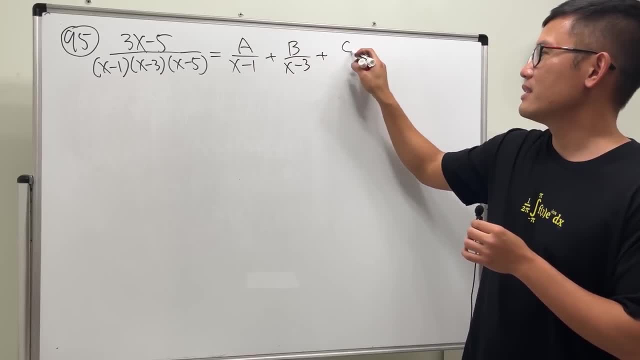 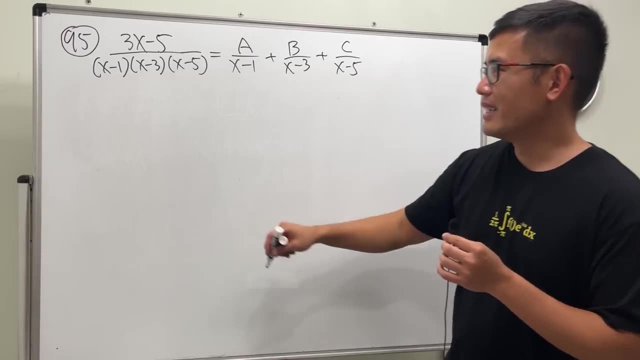 each one. we have there their own denominator: Non-repeated, Yeah. So just like this, And the good news is that we can use Carver for all three, So let's go ahead and make that happen. a equals: it has x minus 1.. 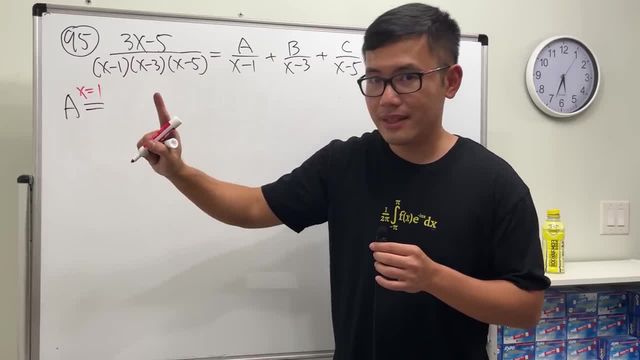 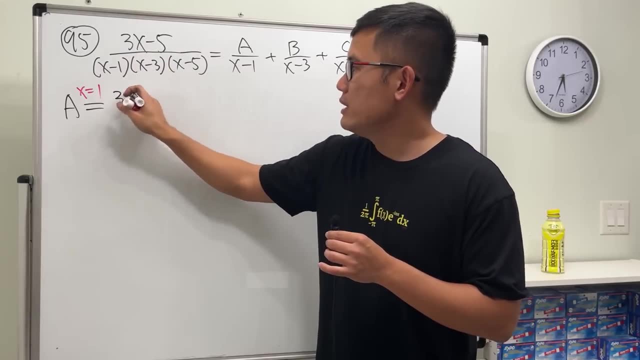 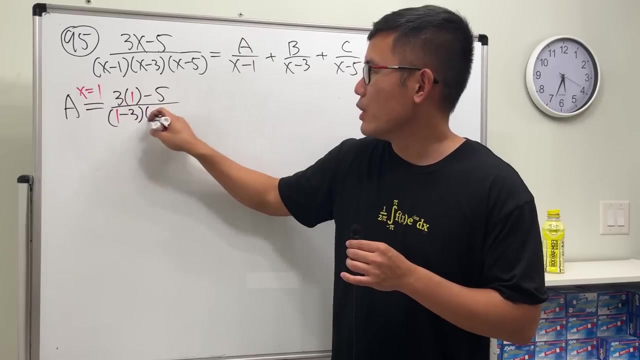 Carver this. So this time a is equal to 1. That x equal to 1.. Put it here, put it here and put it here, So we get 1 minus 5 over 1 minus 3 times 1 minus 5.. 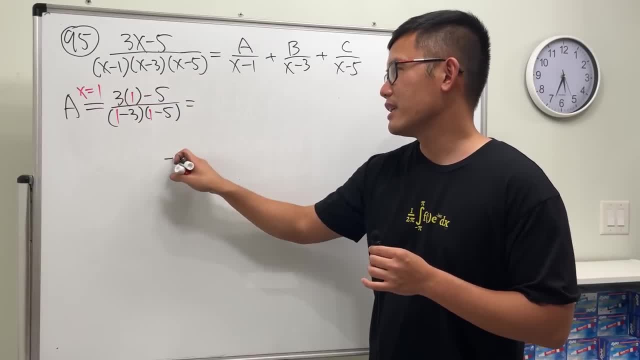 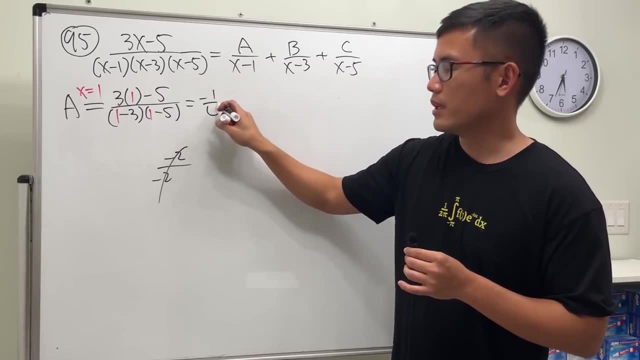 Okay, That's 3 minus 5, is negative 2 over, that's also negative 2, so they cancel. And then that's negative 4 on the bottom, so negative 1 over 4.. Yeah, I got you right. 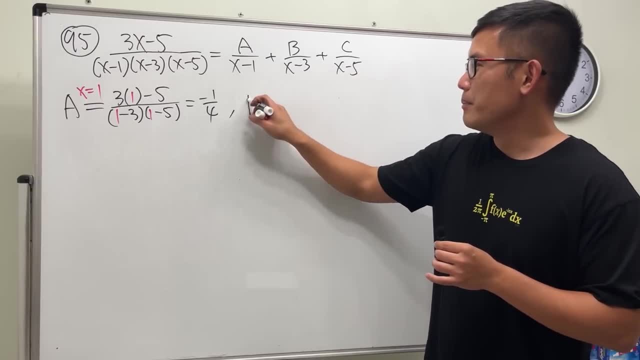 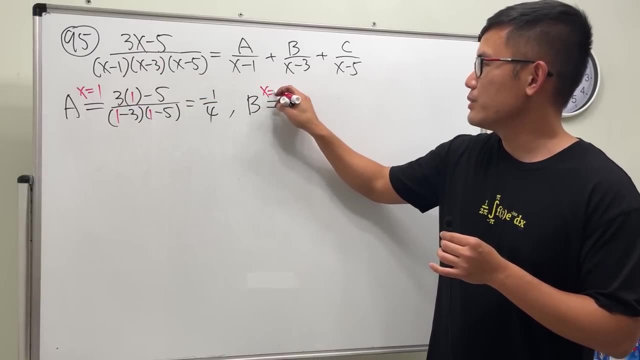 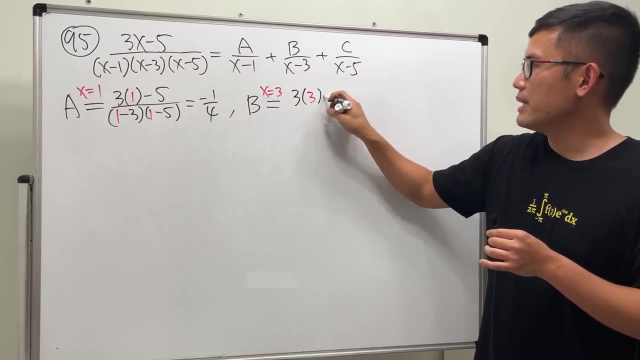 I'm looking at my answer key. Okay. Next b is well Carver. of this denominator, x has to be 3.. So x is equal to 3.. Put it here, put it here. put it here. So we have 3 times 3 minus 5. 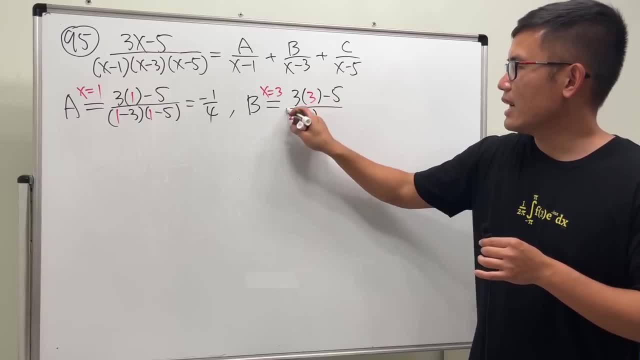 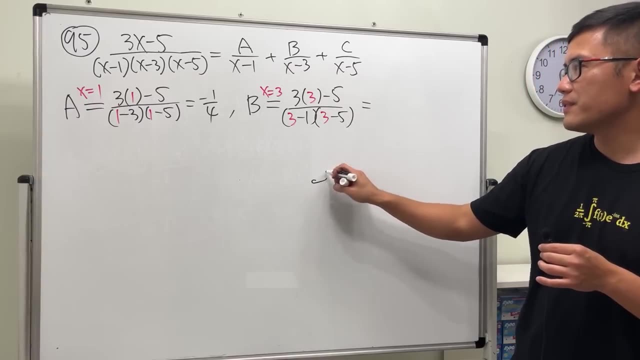 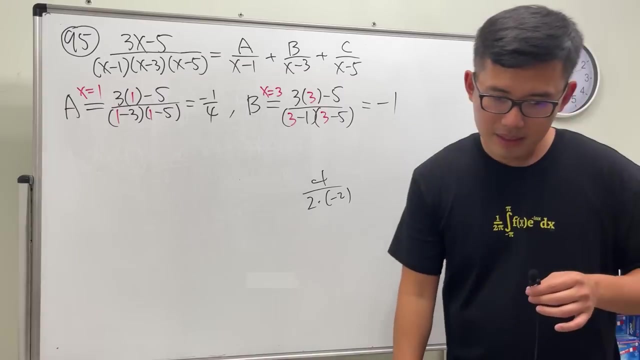 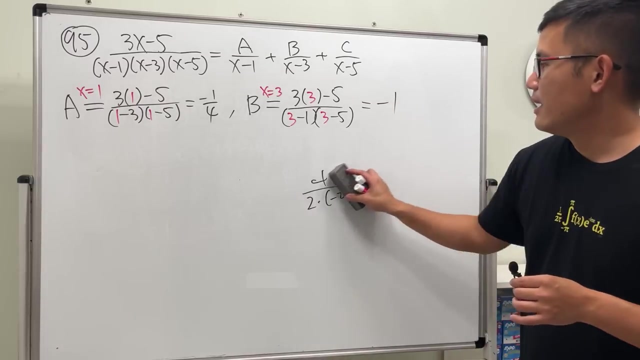 over 3 minus 1 times 3 minus 5.. Okay, That's, 9 minus 5 is 4 over 2 times negative, 2. So altogether it's negative: 1. Yes, Yes, Okay. And lastly, 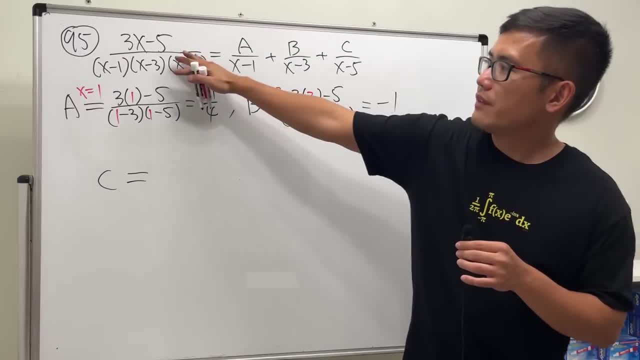 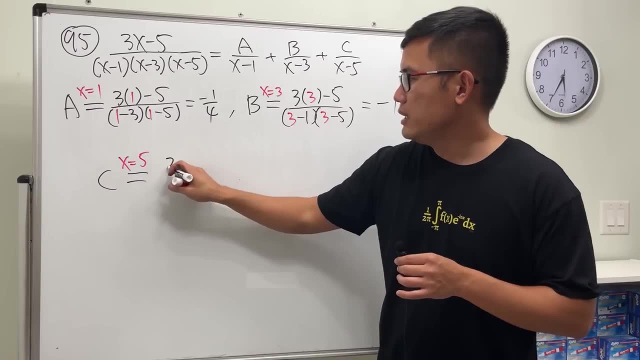 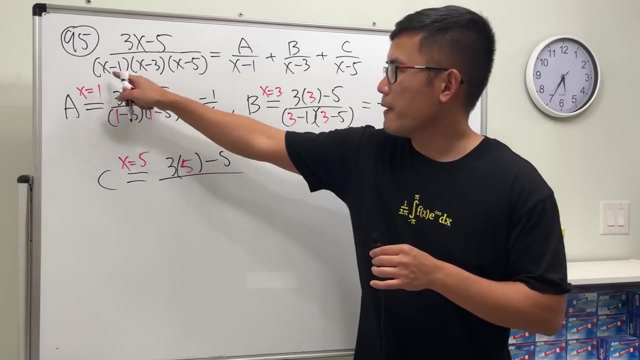 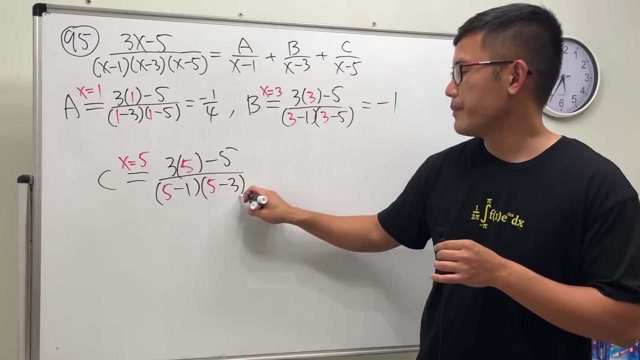 c is equal to Carver, this x has to be 5.. So 3 times 5 minus 5 over 5, 5 in here, right? So it's 5 minus 1 times 5 minus 3.. 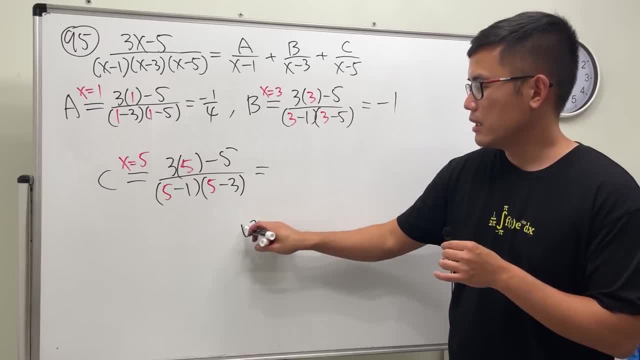 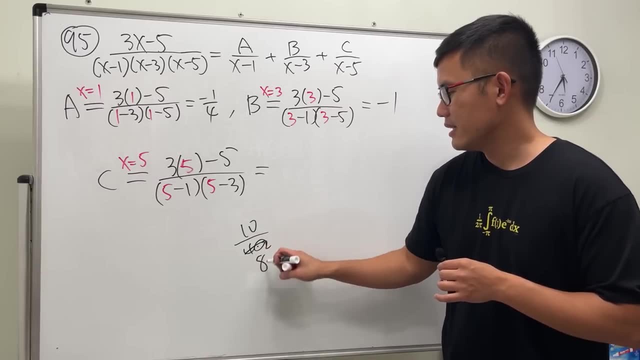 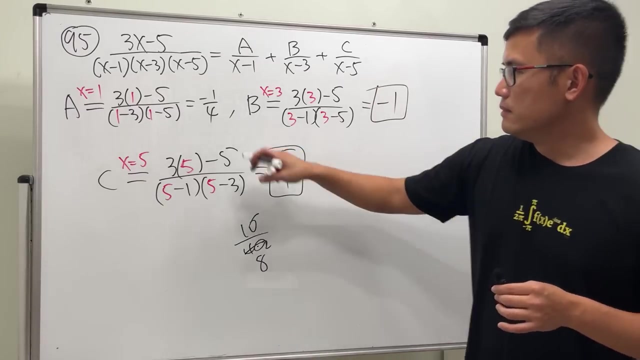 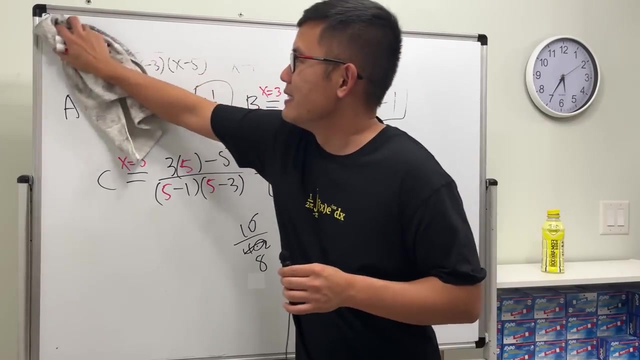 So that's 15 minus 5 is 10 over 4 times 2. Why is this so hard? This is 8. Reduce is 5 over 4.. Yay, So done Just like that. Yes, Okay. 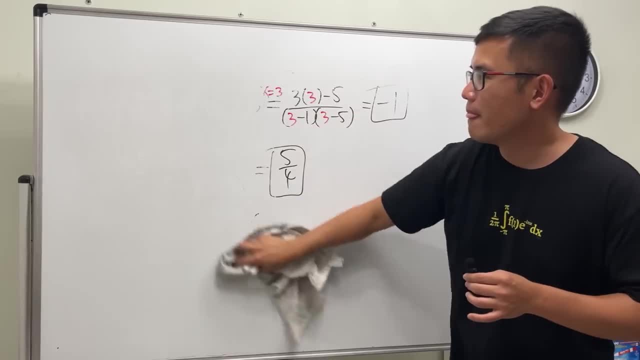 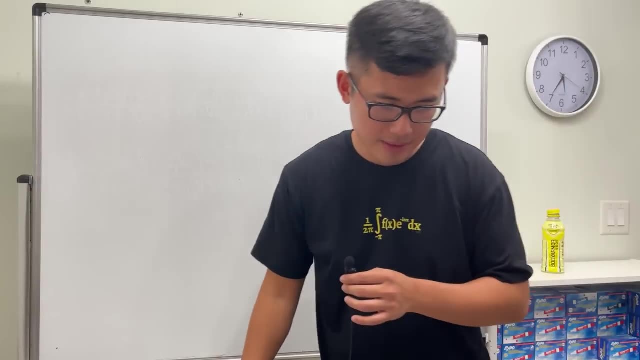 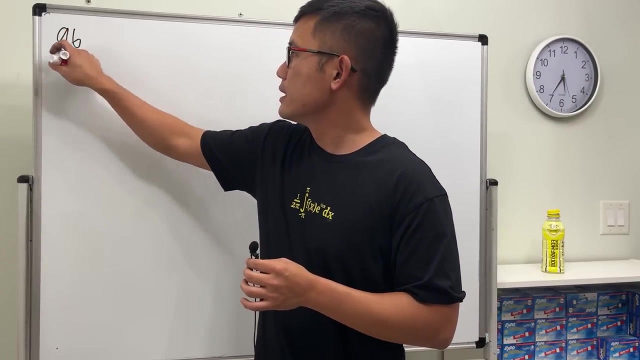 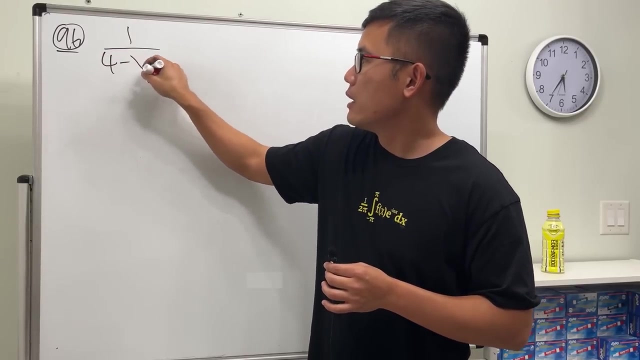 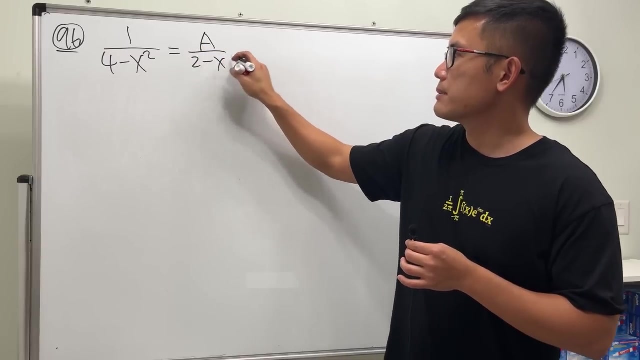 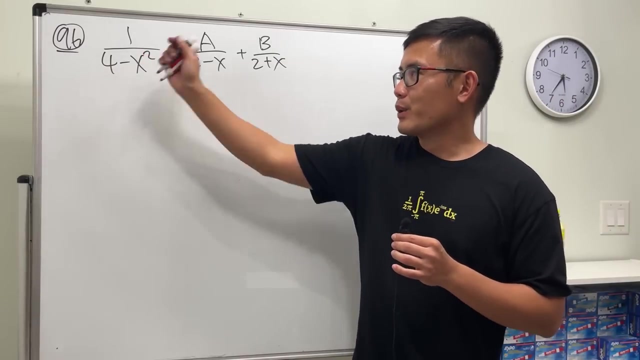 Couple more questions, Seriously 96.. We have 1 over 4 minus x, squared All right. And then this is equal to a over 2 minus x plus b over 2 plus x. For this one, notice that the original denominator was not factored in. 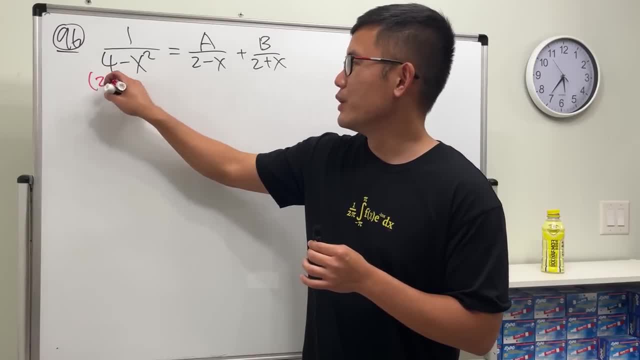 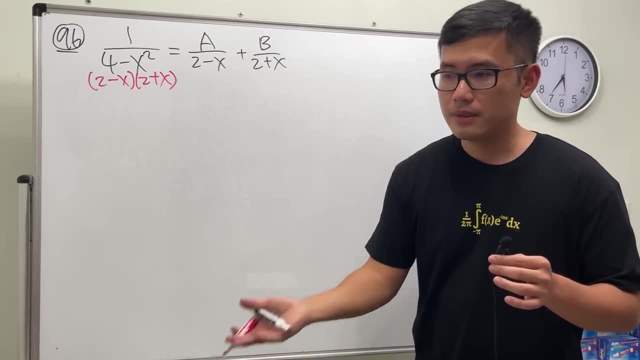 But we can factor it ourselves, right. So in fact, factoring this, we get 2 minus x times 2 plus x, And then we do have this and that, And you know it, We can do Carver up for both of them. 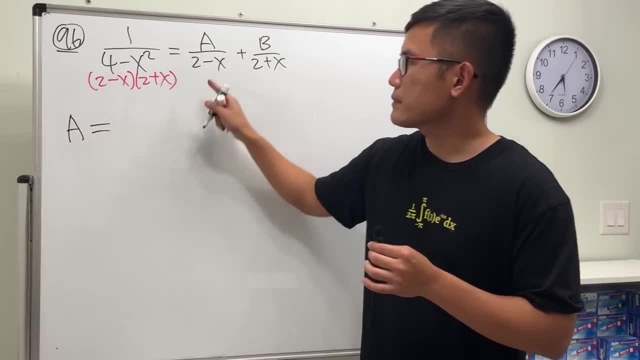 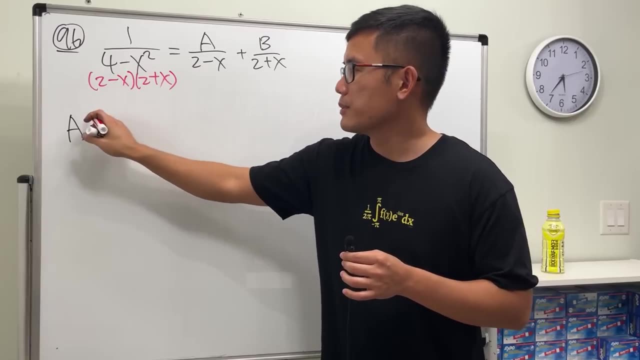 Awesome, a equals Carver, the same denominator. So we put the denominator: x has to be 2, right, 2 minus 2 is 0. So x has to be 2. And we put the 2 here, So we have 1 over 2 plus 2.. 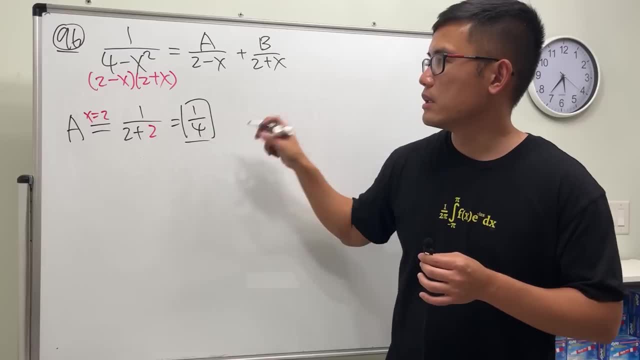 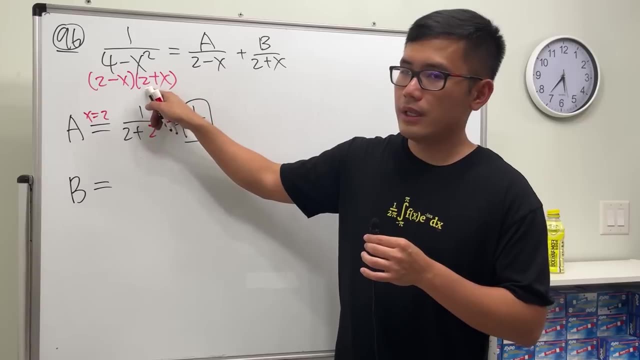 So a is equal to 1 over 4. Done, And then b equals Carver this up. So x has to be negative, 2. So x has to be negative, 2. We put it here: We have 1 over 2. 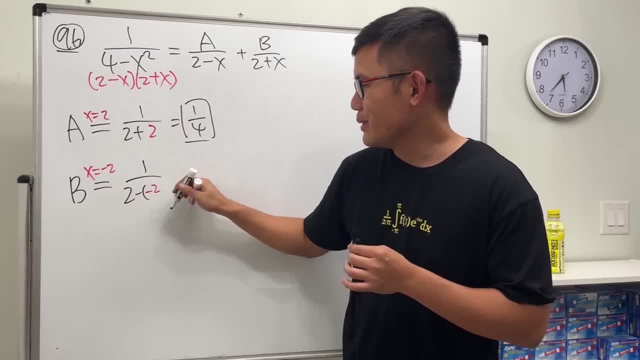 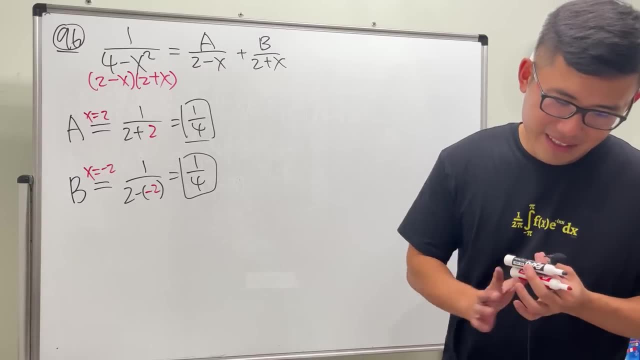 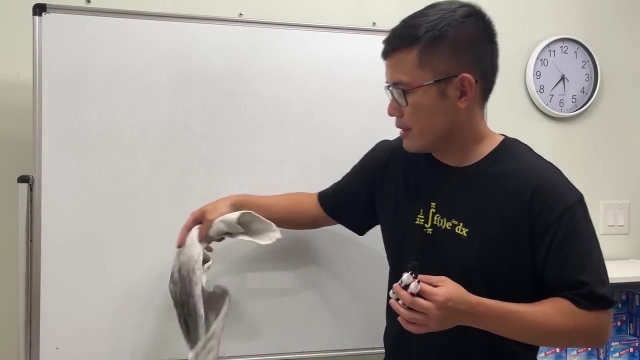 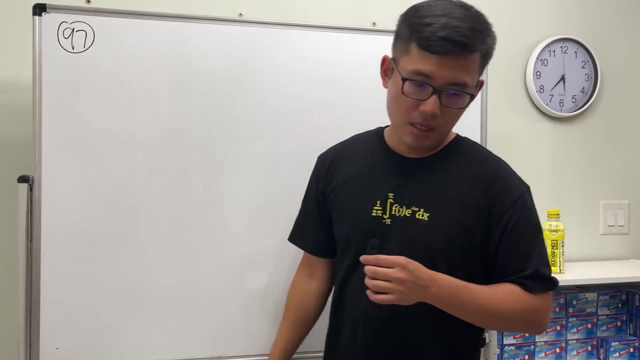 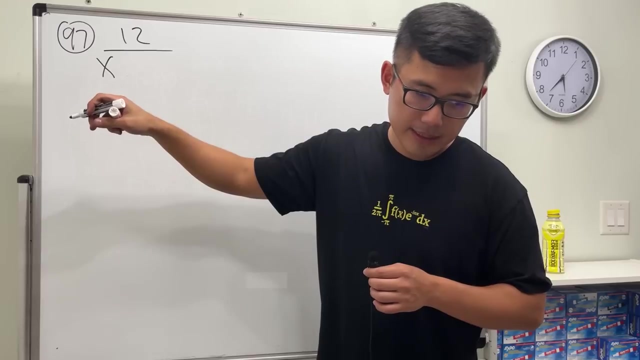 minus x is negative 2. And that's 1 over 4.. Again, Done, Yeah, that's a nice one, Okay. Okay, Number 97.. First, we have 12 over x to the third power minus 3x squared. 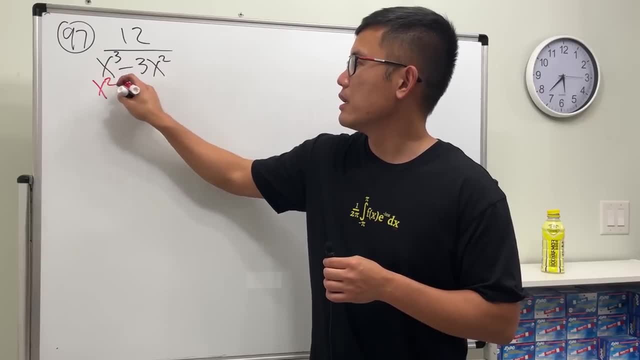 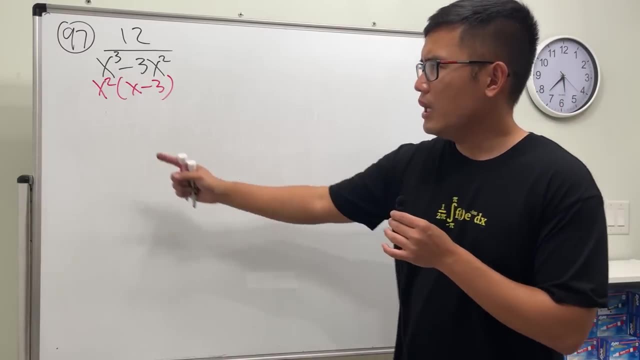 Let's see, Let's factor it. We can factor out x squared And then we get x minus 3.. Yeah, So that is what we have, And you see we have x squared here. So just think about what we did earlier. 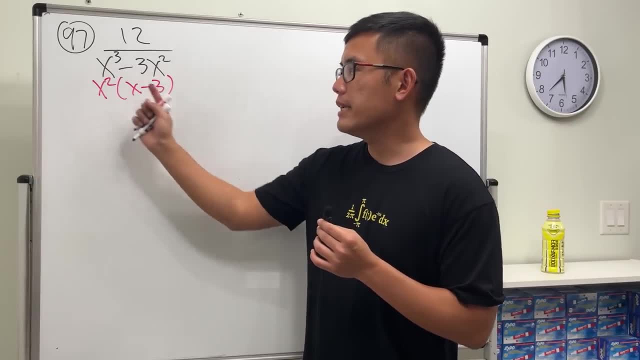 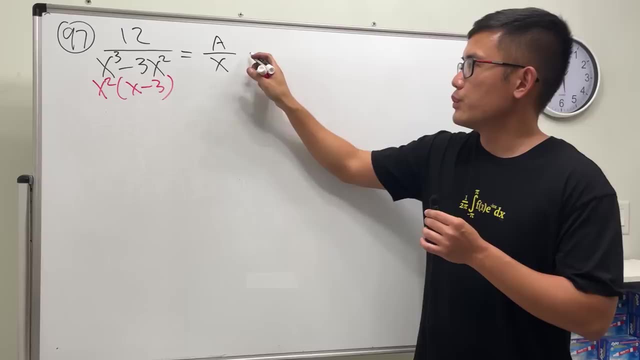 When we want to break it apart, we will have to build out the power, because x squared means x times x. So the first thing we will have is some number over x. Next we will have: you know, go to x squared, Yeah. 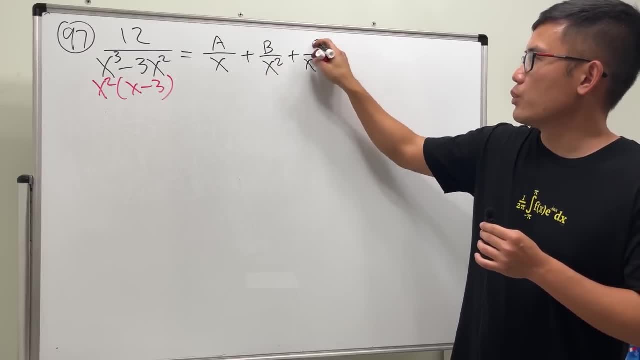 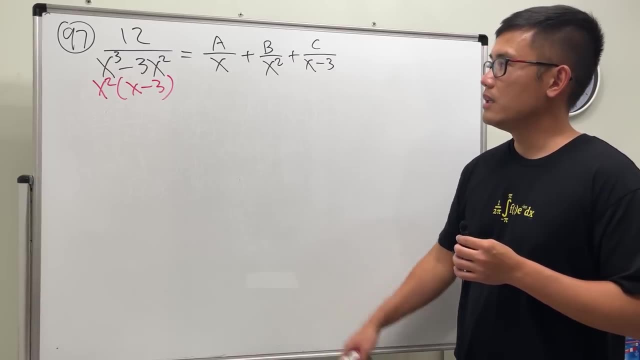 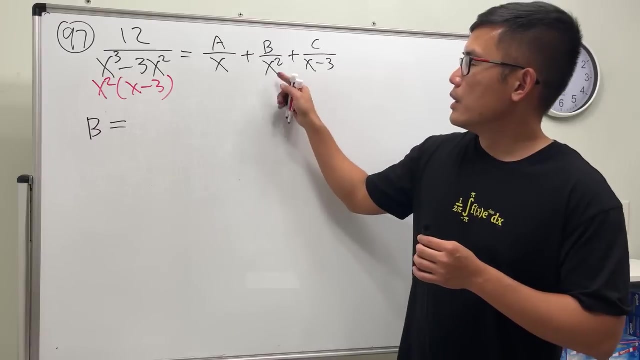 And then next we have that, So in this particular order. Okay, All right, We can do algebra for two letters. What are they? b and c? So let's go ahead and make that happen. b equals well, copy this. 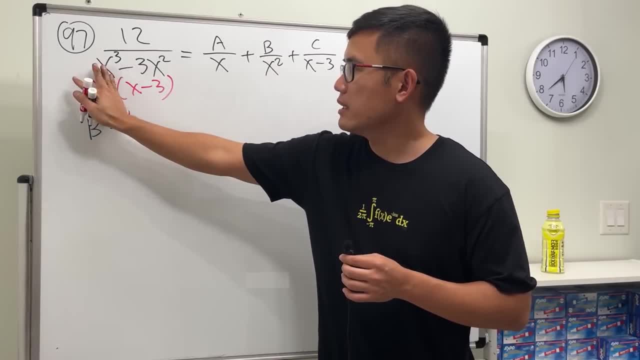 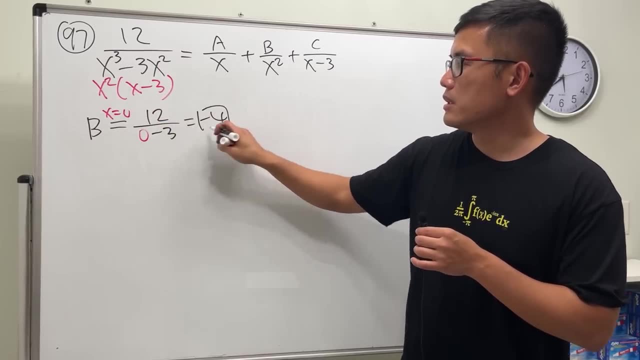 x has to be 0. All right, Copy this: x has to be 0. So we are going to get 12 over 0 minus 3, which is negative 4. So b is negative 4. c equals. 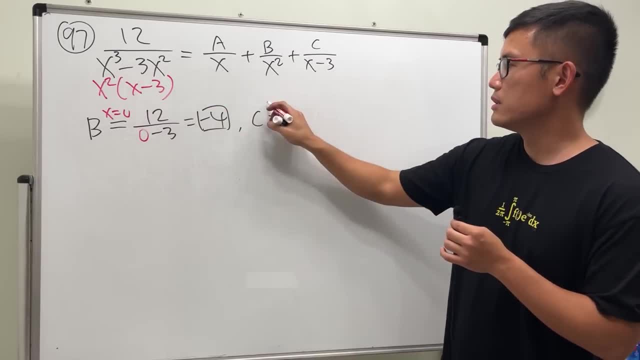 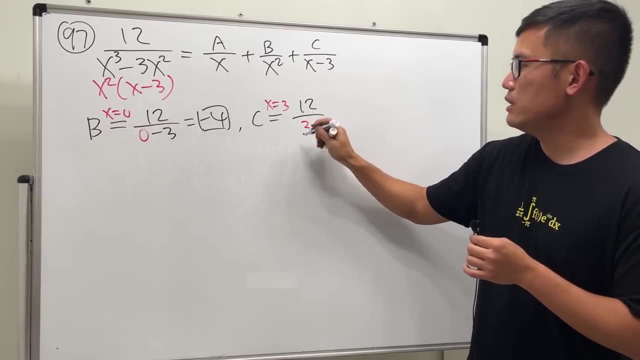 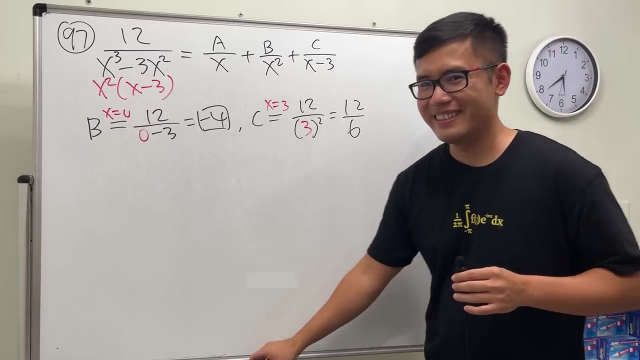 copy this: x has to be 3.. So x is equal to 3. And we put it here. So we get 12 over 3 squared. This 12 over 6 is 2.. Just kidding, Just kidding, Just kidding. 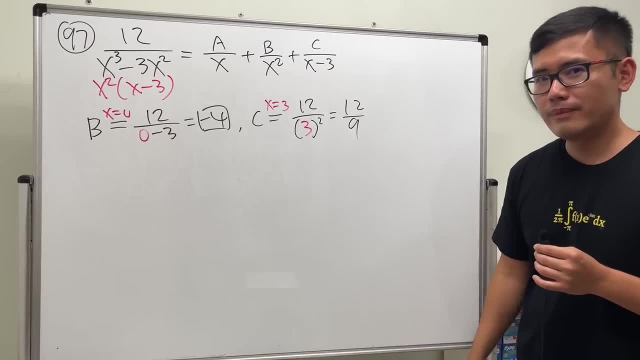 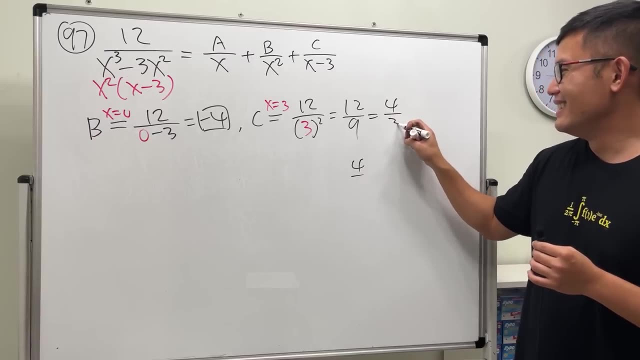 9.. 12 over 9 is what I forgot. 4 over 3.. Yeah, All right. So so far so good. And um, of course, this is not it yet, because we still have stuff for a. 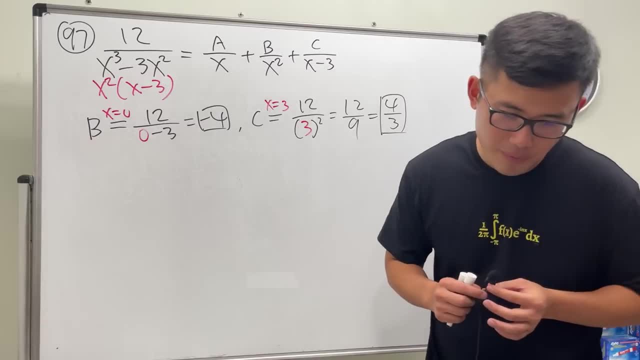 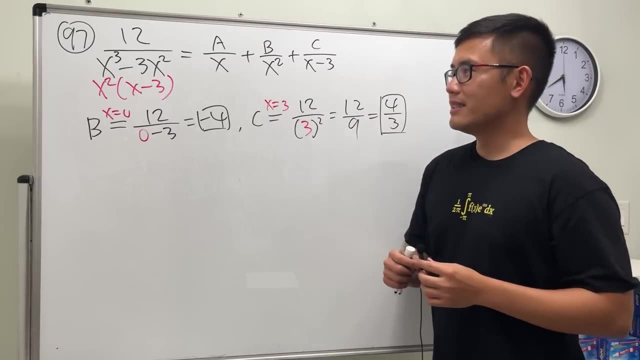 right. So you know the deal. we cannot do: cover up for a, So let's go ahead and make that happen. So so far, so good, And um, of course, we have x squared over a. 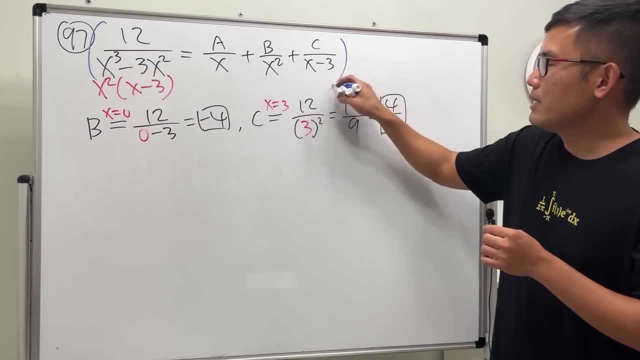 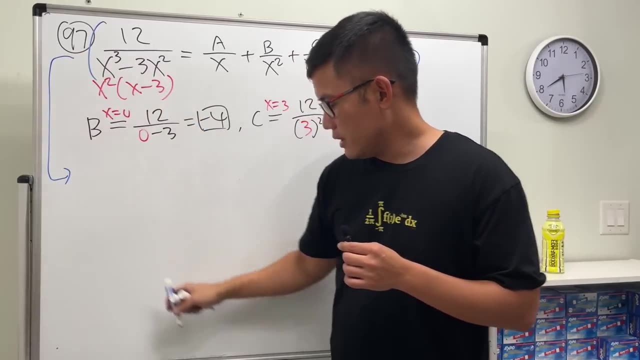 So let's just go ahead. do the traditional way: Multiply everybody by the denominator, which is just x squared times x minus 3.. And then let's see what this will give us. On the left-hand side, we just have 12.. 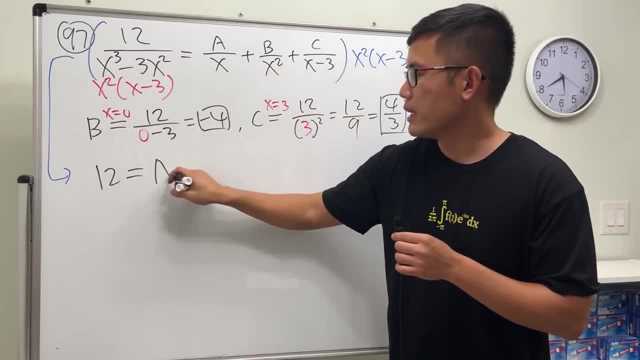 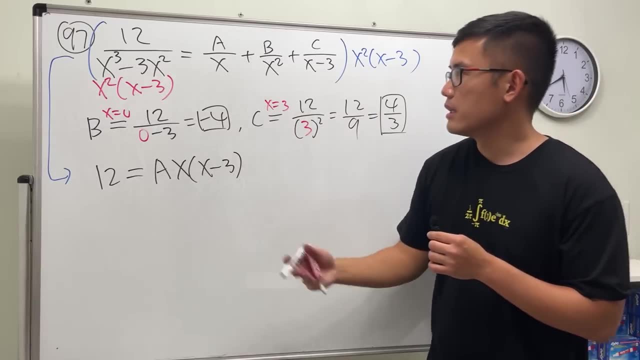 And that's equal to a. we don't know x, and one of them will cancel, So we have another x, and then x minus 3.. Continue: x will cancel, b is negative 4.. So we have negative 4,. 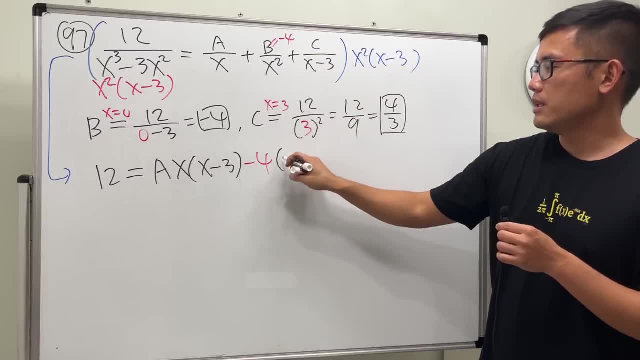 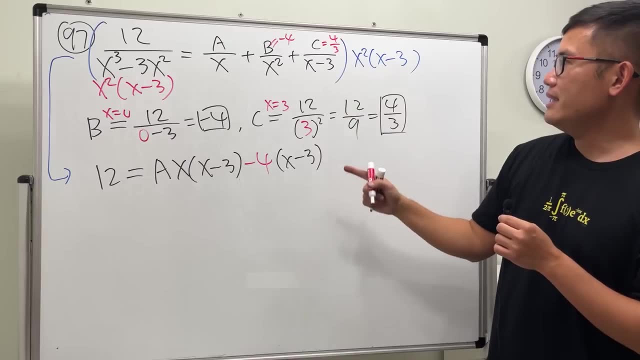 times x minus 3.. Then c is 3,, uh 4 over 3.. And this and that cancel, So we just have plus 4, over 3, x squared. So that's what we have. 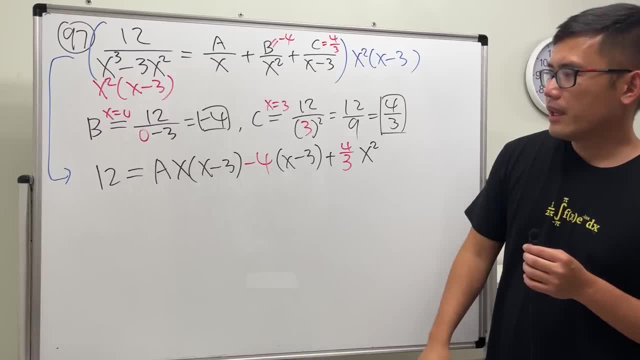 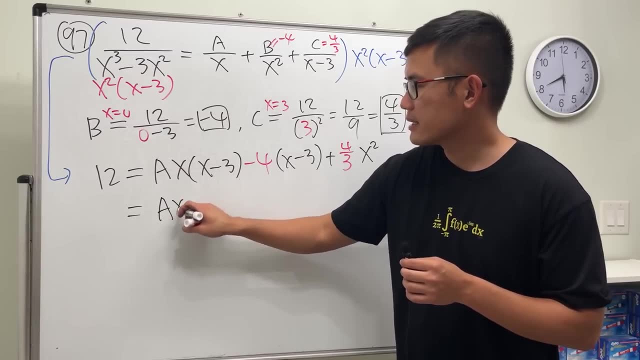 And now let's see: If we multiply this out, we get a x squared, Right. So if we multiply this out, we get a right, a x squared. And let me tell you, it doesn't matter. 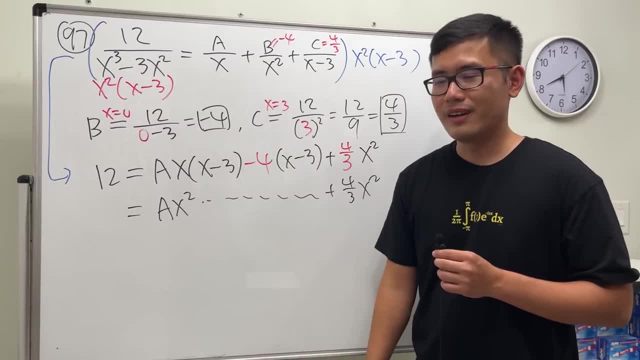 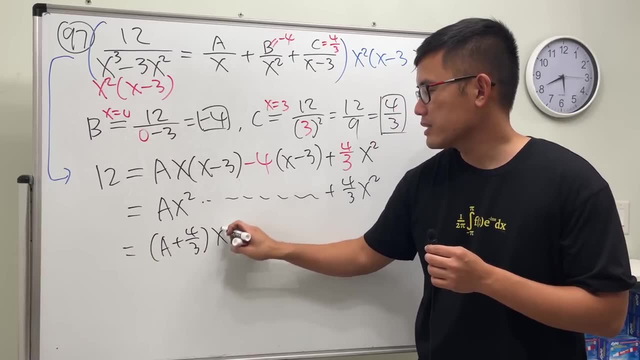 And then plus 4 over 3, x squared, Because none of them will give us x squared, And then, in fact, if you look at it, we must have a plus 4 over 3, x squared. 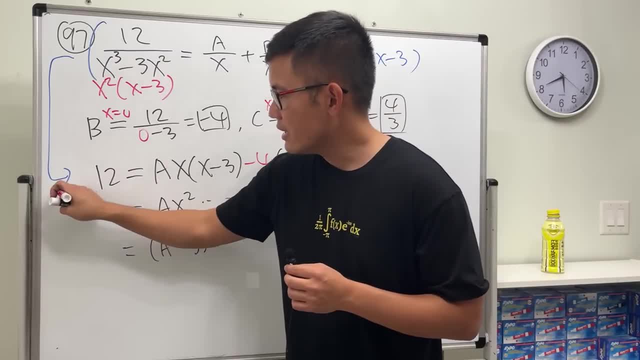 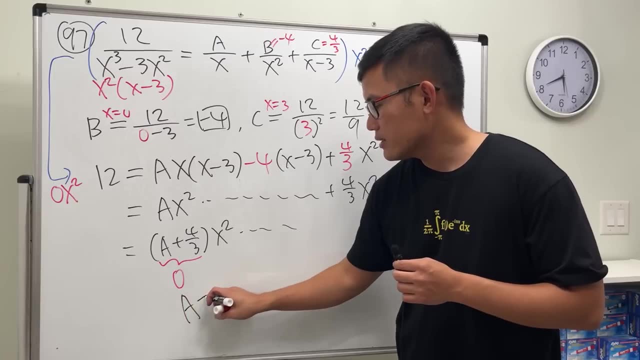 So what does that mean? The left-hand side: again it was 0, x squared Right. So that means this right here has to be 0. Meaning that a negative 4 over 3. Done. 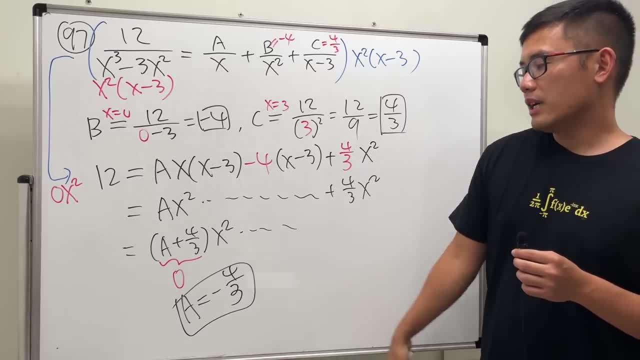 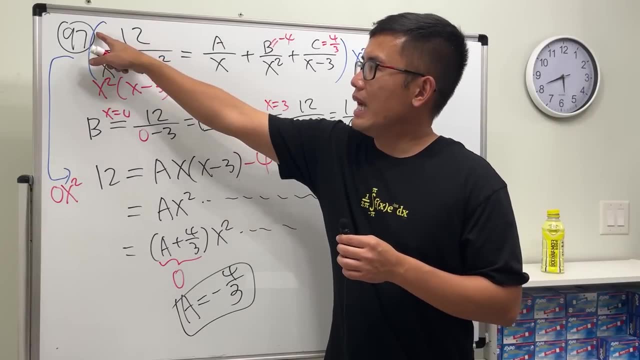 Now all the time it's like the opposite of a. Now all the time it's the opposite of c. though Imagine if this right here, we have x squared plus 12. Then it would be 1x squared. 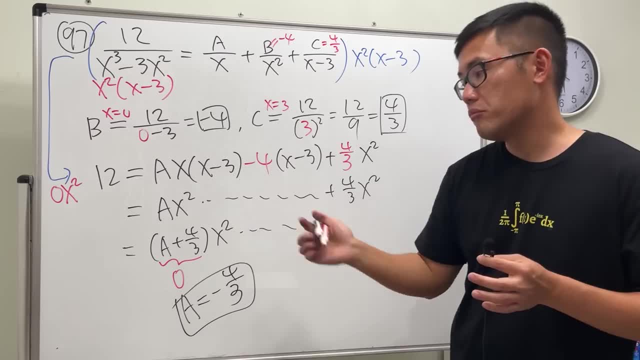 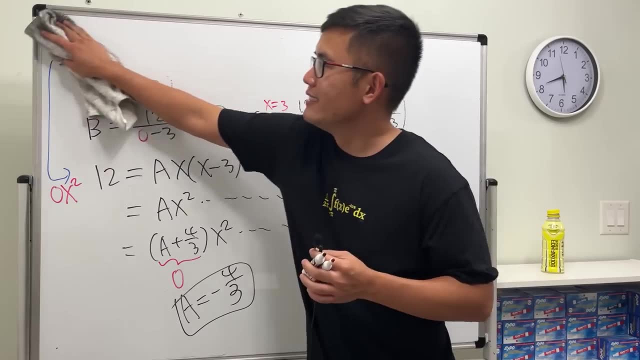 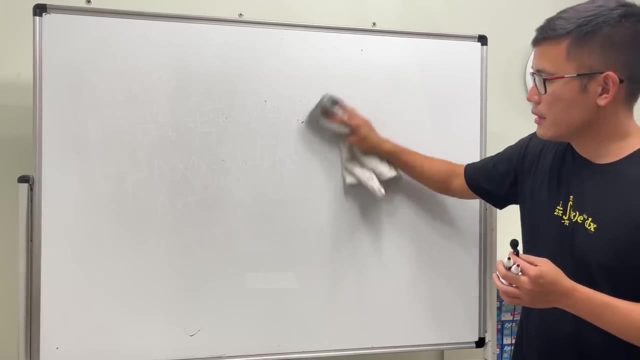 Then we would have to set this to be 1.. Yeah, So just saying: Well, we're done. a b c. a b b c, u, x, c, z d. 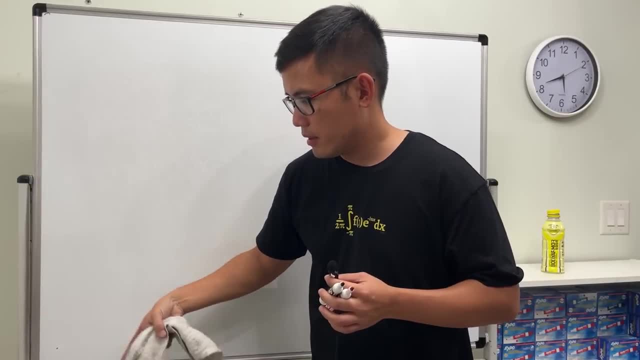 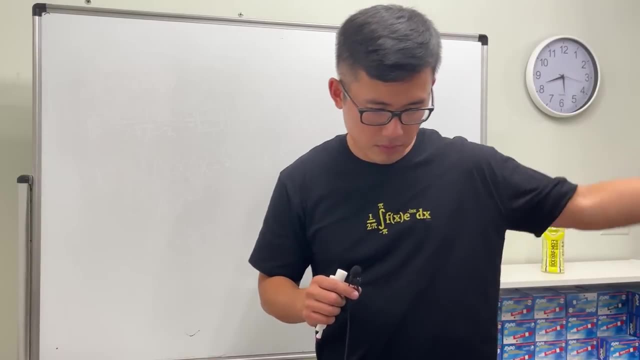 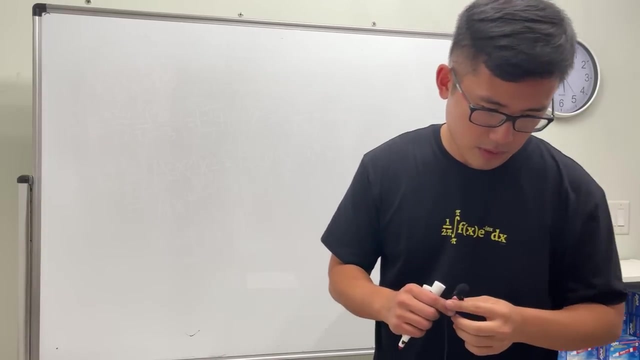 a, y, d so So. So again, we have to get this to be 6 over 3, c, z, c, c, z, v, z g, z z n n. 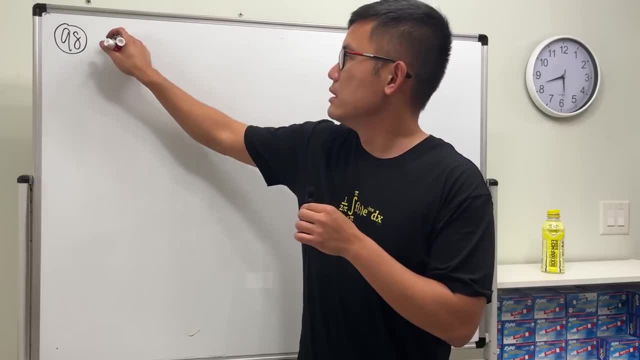 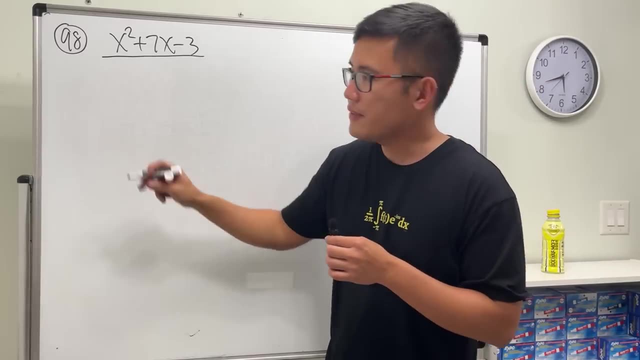 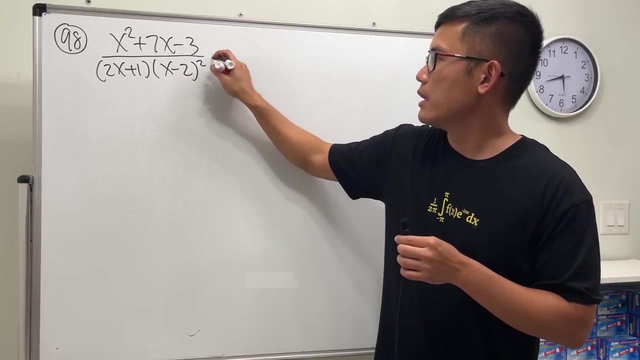 8, number 98, we have x squared plus 7x minus 3.. So now you see, like a numerator I give you more stuff And on the bottom we have 2x plus 1 times x minus 2, squared Right. So again, this means x. 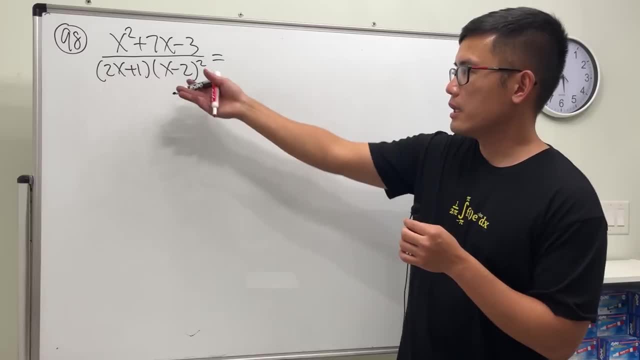 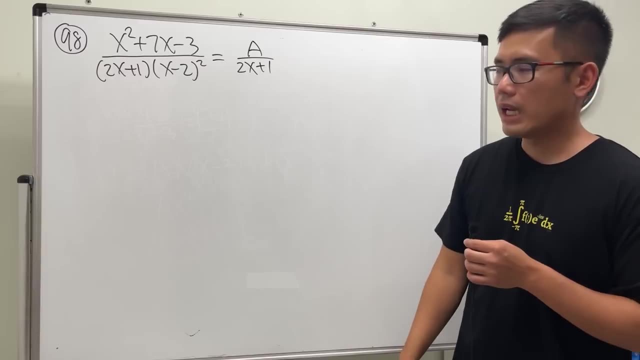 minus 2 times x minus 2.. So we had to build out the power, And the first term is the first denominator is 2x plus 1.. So this is what we have, And then build out the power. So we have plus x. 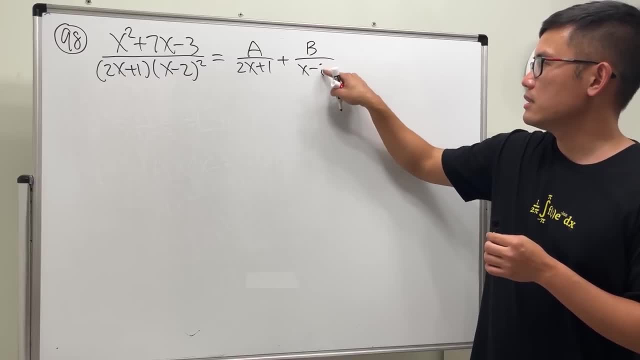 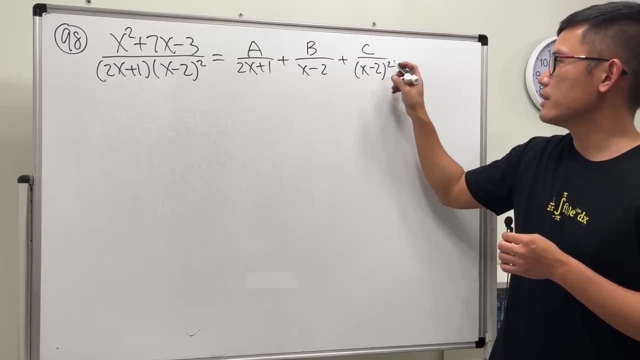 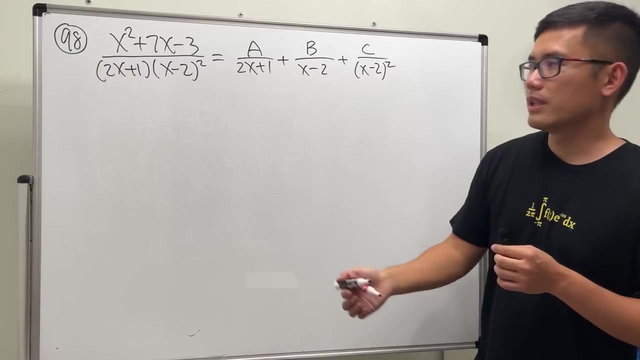 minus 2 to the first power And the top is just a constant And then another constant over x minus 2 squared. Okay, Cover up two people right, A and C. So let's make that happen. A equals cover this. 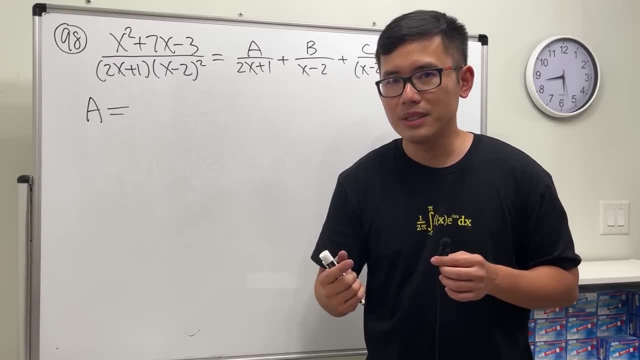 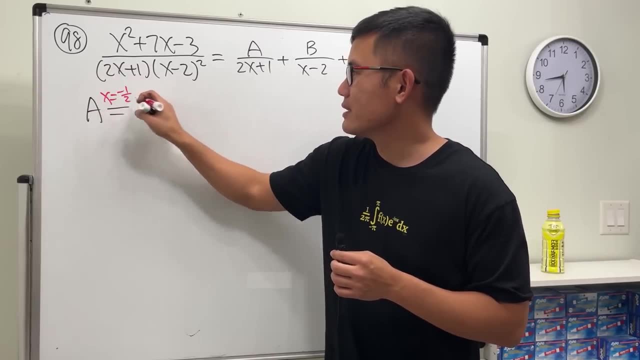 up: 2x plus 1.. A equals 0.. A has to be x, has to be negative 1 half. Yeah, this is a fraction 1.. Oh my goodness, But we can handle it right, Hopefully. I don't know Why do I have to do this to myself? Anyway. 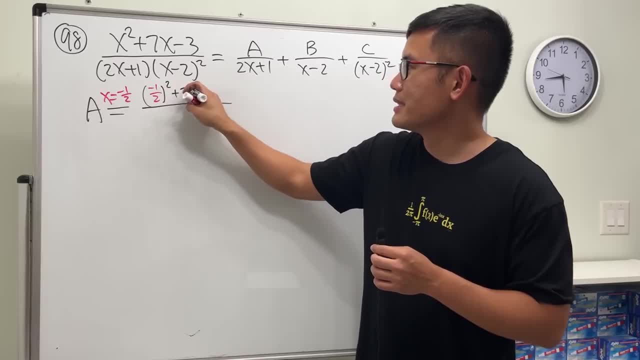 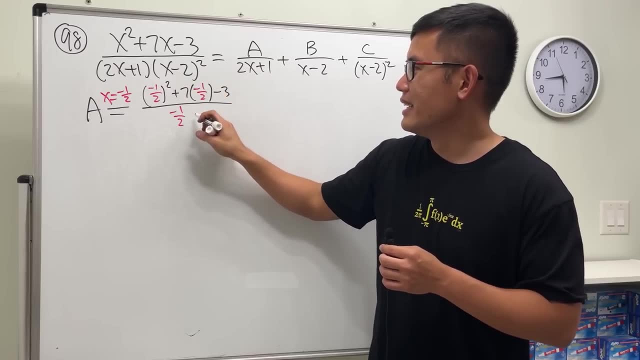 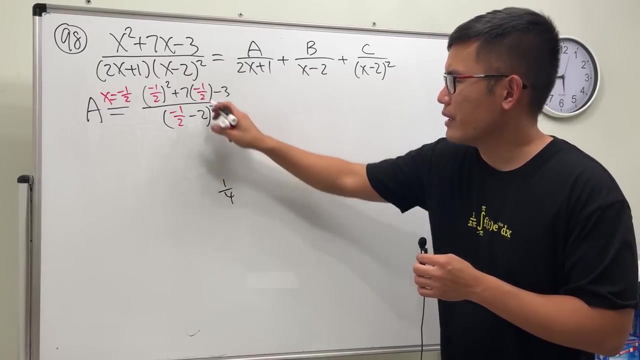 Negative 1 half squared plus 7 times negative 1 half, And then minus 3.. And then put the negative 1 half here, And then minus 2.. Okay, I do this to myself, Anyway. Over there is 1 over 4.. And then this is minus 7 over 2.. And then 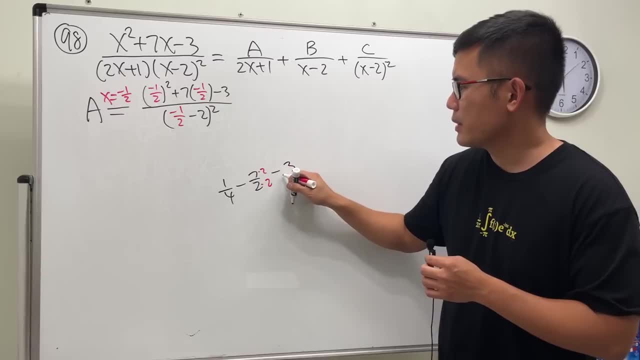 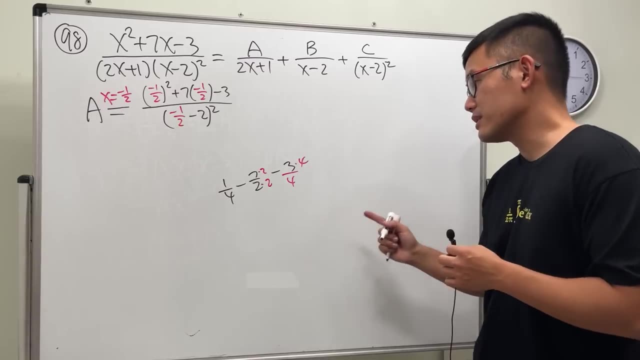 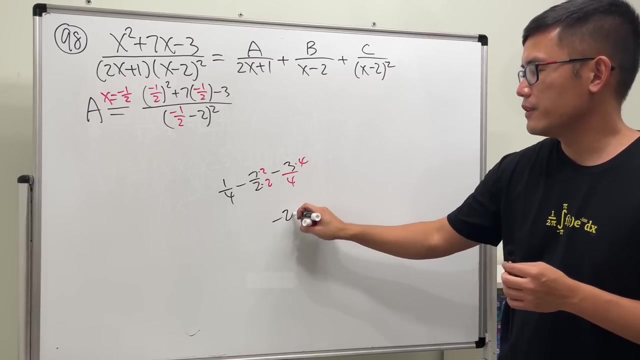 minus 3.. So multiply by 2, multiply by 2, multiply by 4, multiply by 4.. 1 minus 13.. 1 minus 14 is 13. Negative, 13.. And then minus 12 is minus 25 over 4.. Okay, So that's the numerator. And on the 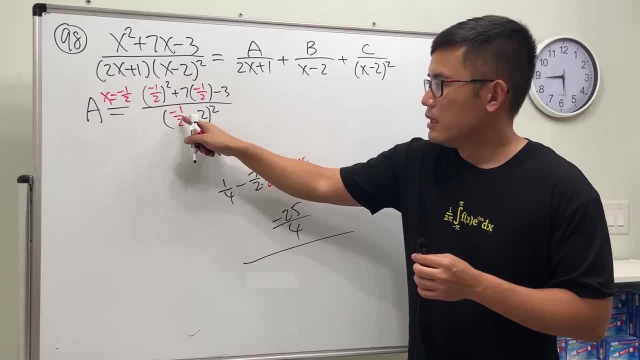 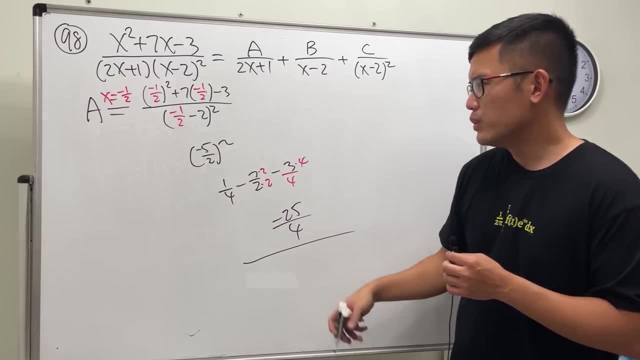 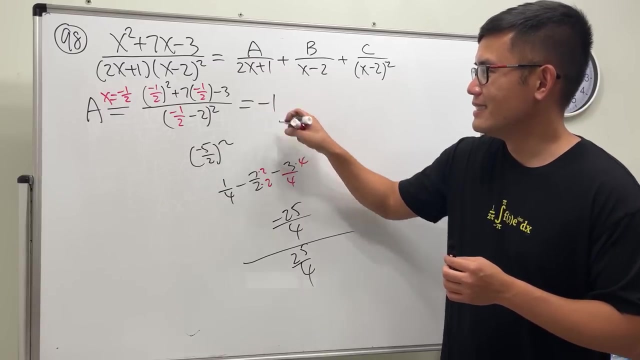 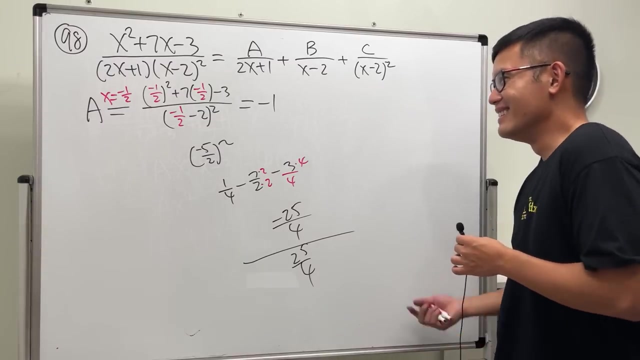 bottom. This is negative, 2 over 2.. So we have 5 over 2 negative and square of that, Which we get 25 over 4.. You're killing me? So a is equal to negative 1.. Yeah, That's correct according to my answer key. But yeah, So just compute it. Fractions and. 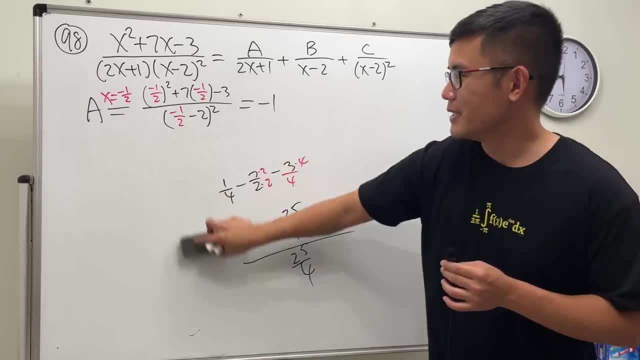 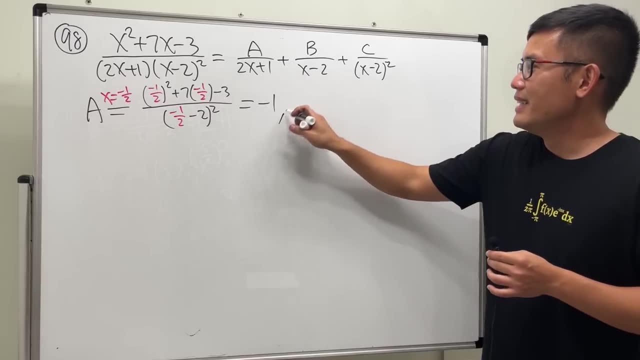 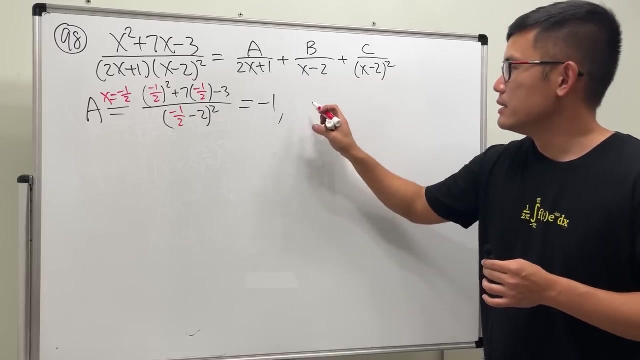 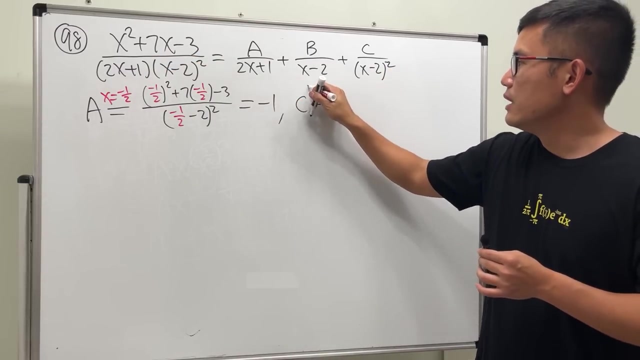 and then the bottom. just get the common denominator and all that stuff. we'll use a calculator. if you can use a calculator, just go for it anyway. b equals- no, cannot do it for b. c equals cup. okay, cover this up. x has to be two. yeah, so x has to be two. put it here, put it here, put it here. so. 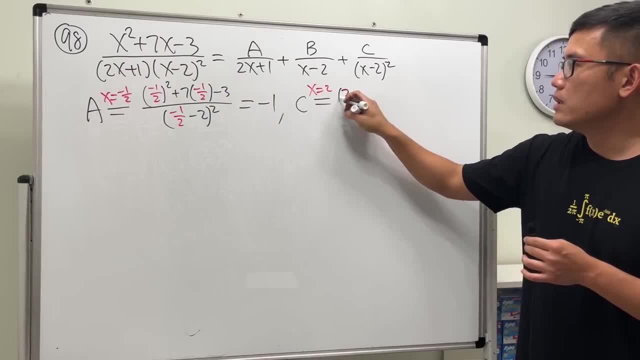 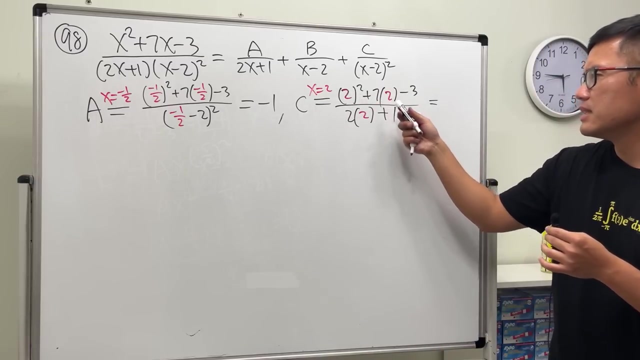 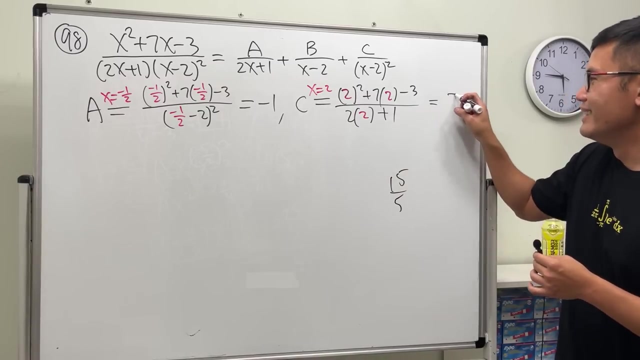 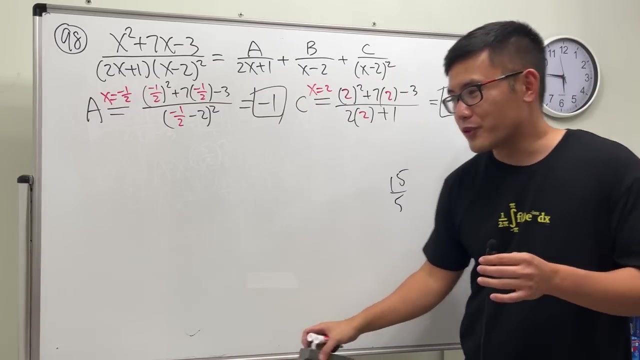 we get two square plus seven times two and then minus three over two times two plus one. okay, four plus fourteen is eighteen minus three is fifteen over five, three. yeah, nice numbers you usually hold to cover when we do partial fractions. when i set other questions i'll try to make it like nice numbers because 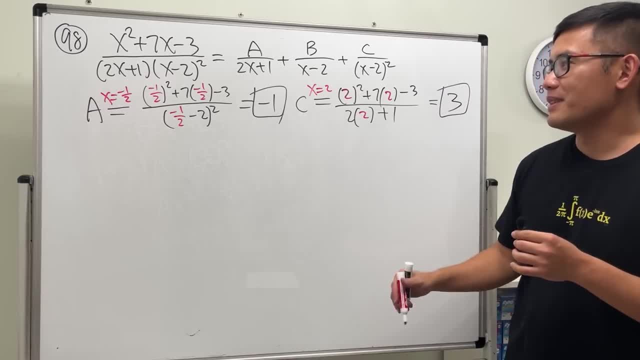 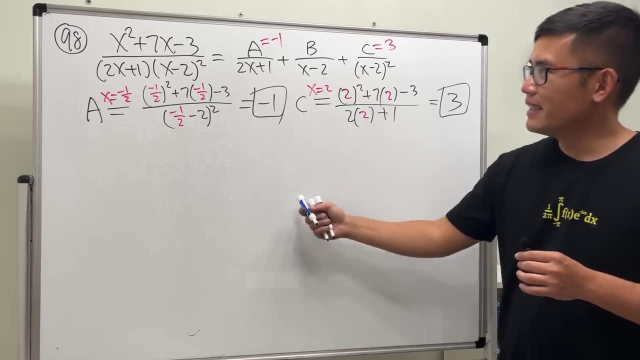 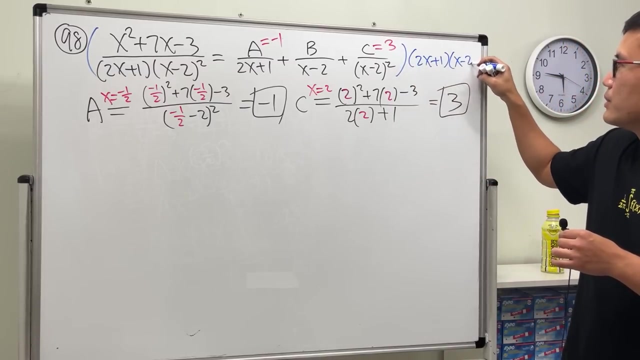 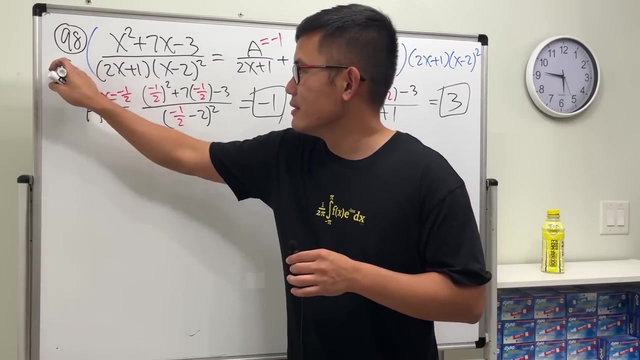 otherwise that people go crazy, including myself. but anyway, a is negative one and c is equal to three. for b, let's multiply everybody by 2x plus 1 x minus 2 square on the left hand side. oh, i forgot to draw my blue arrow, so 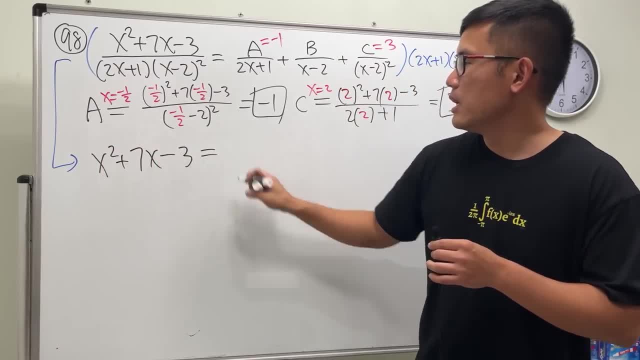 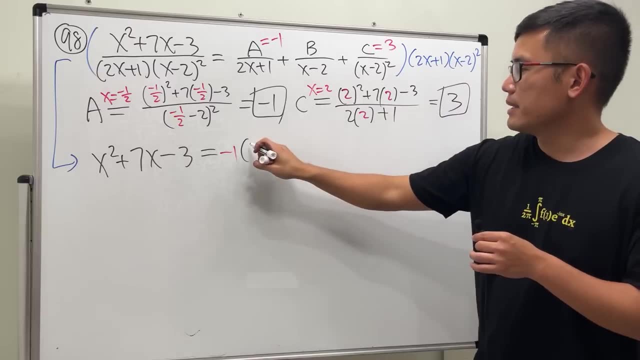 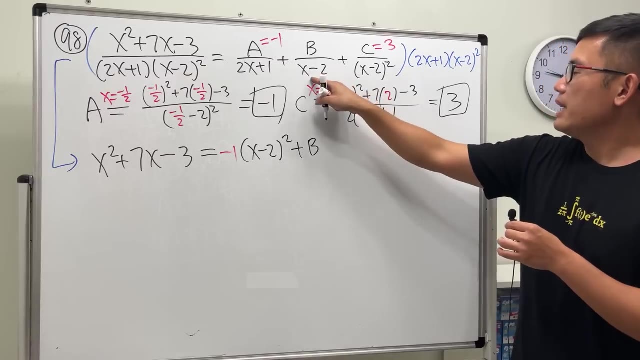 x squared plus 7x minus 3.. okay, this and that cancels. so we have negative 1 times x minus 2 square, and then b, we don't know. so put on plus b x minus 2, cancel one of them and we have this and that right. so 2x plus 1 x minus 2.. 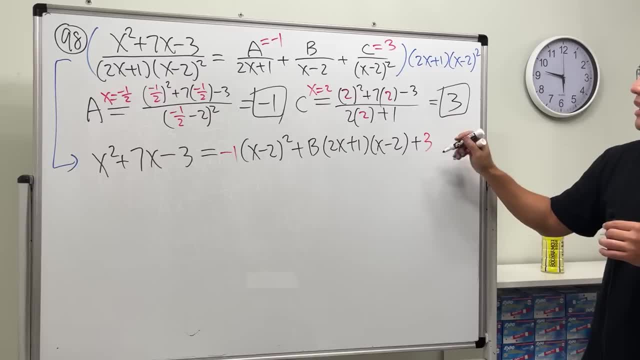 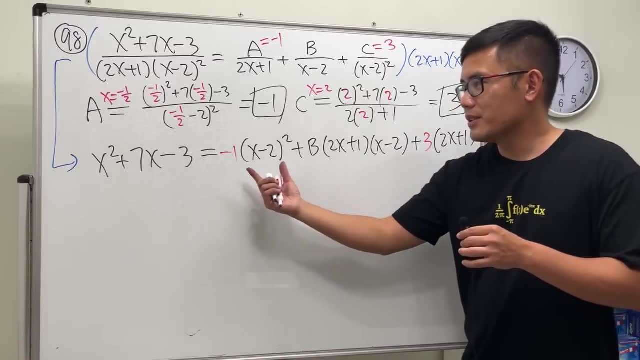 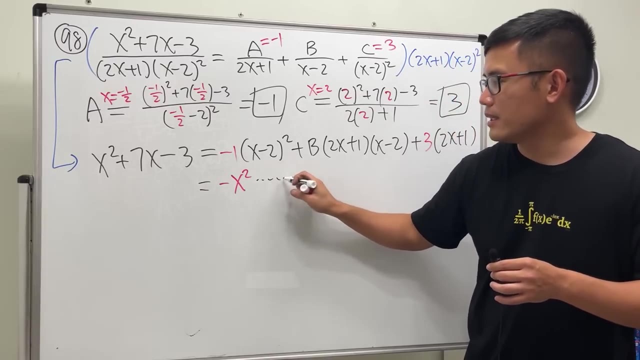 lastly, this and that cancel, so we have plus 3 and then 2x plus 1.. okay, you know the deal right here. let's just care about the x squared term. we get negative 1 x squared, so and then don't worry about it. this and that. 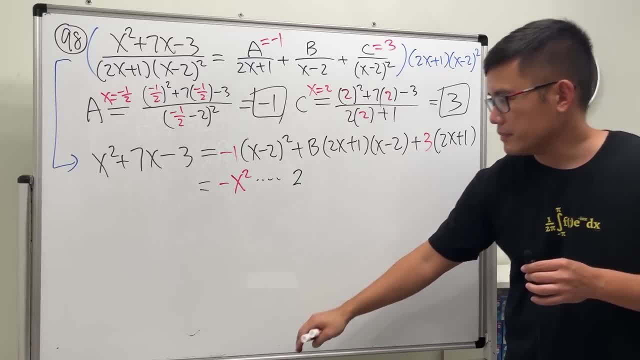 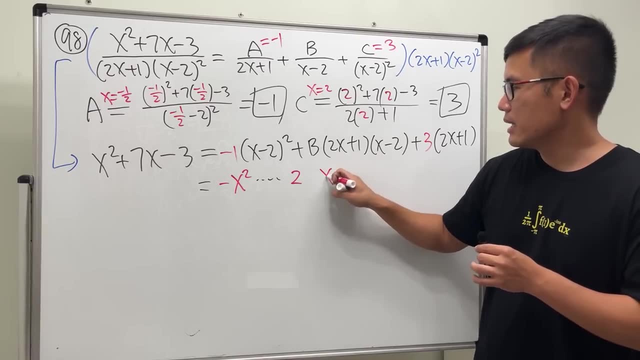 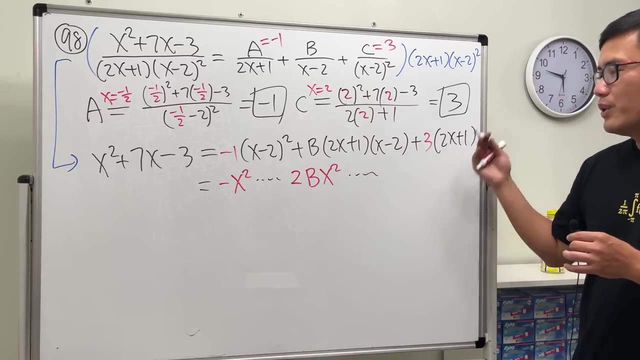 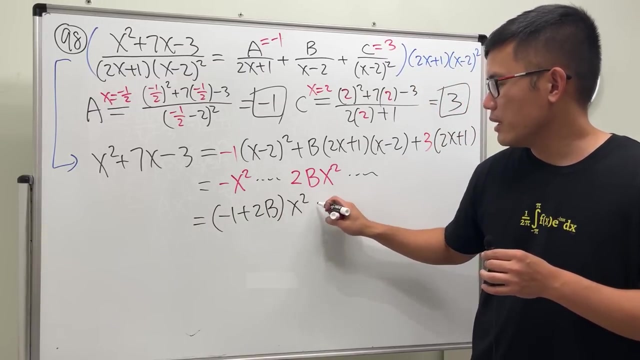 give us two. let's do this: two x squared, yeah, 2x squared, that's the only x squared term. but multiply by b: yeah, and then we don't have any other x squared term. so you see, we must have negative 1 plus 2b x squared. 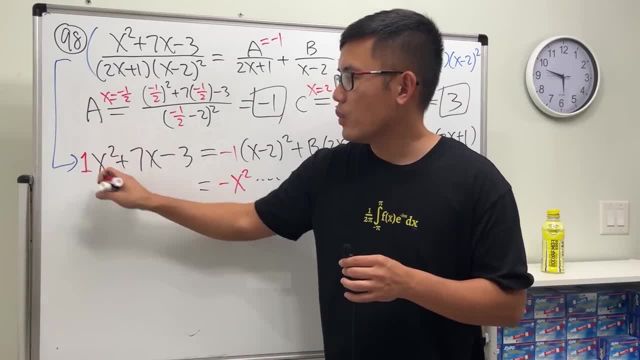 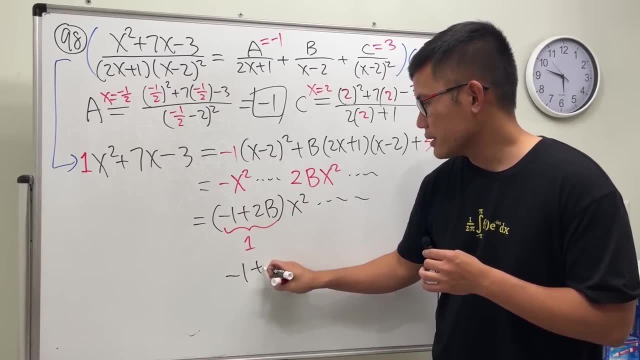 but this time, though, on the left hand side, this is a 1- 1x squared. so that means this right here has to be 1.. so negative 1 plus 2b equals 1.. so that means this right here has to be 1.. so negative 1 plus 2b equals 1.. 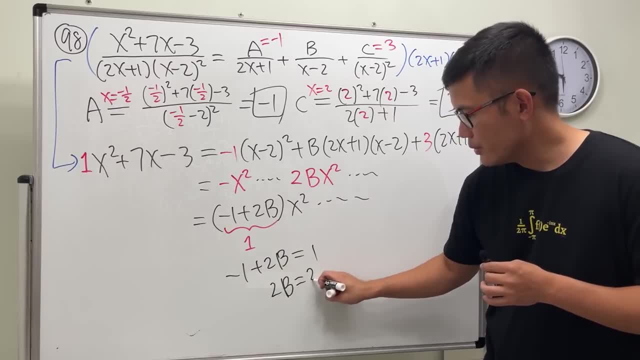 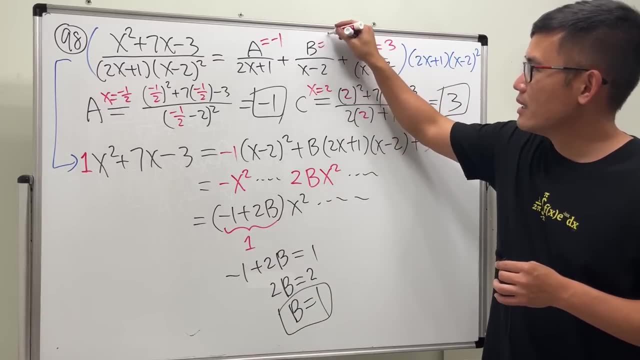 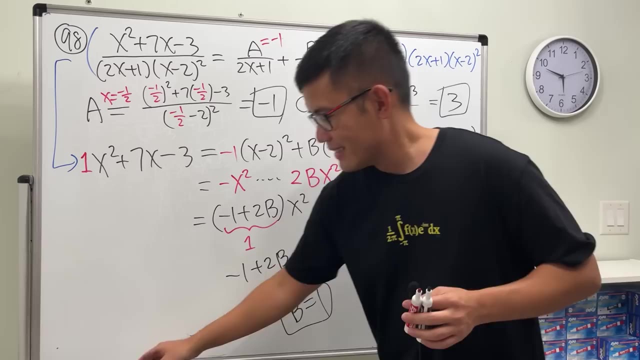 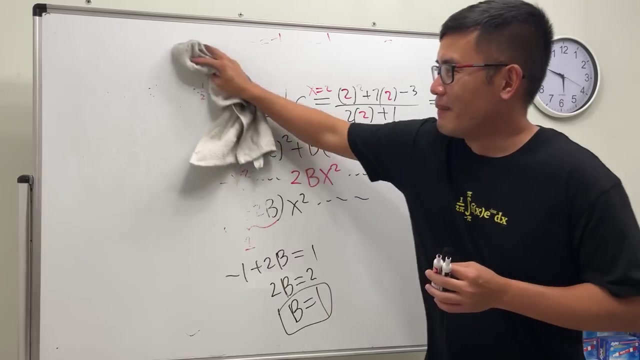 move this to b equal to. b equals 1.. okay, b equals 1.. done, yeah, this is more like workout, both for the mind and also for the hands, and because i've erased all this stuff, let me see if i can finish this one. 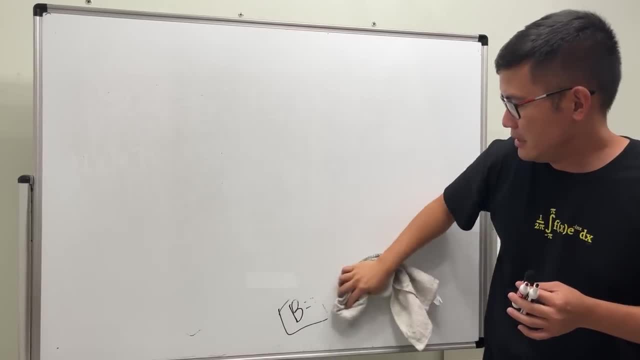 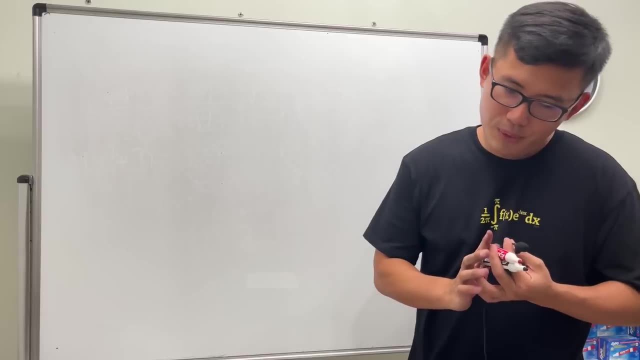 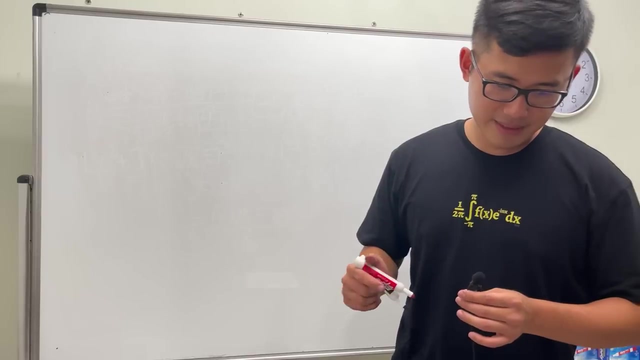 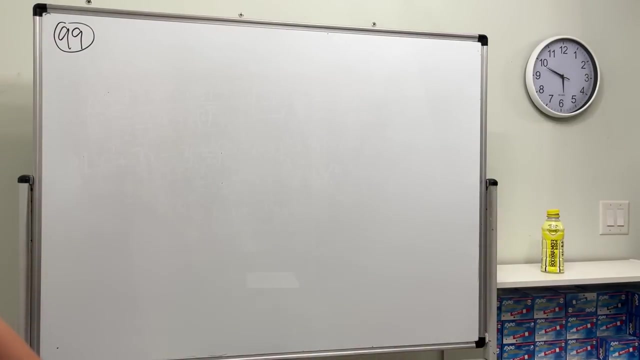 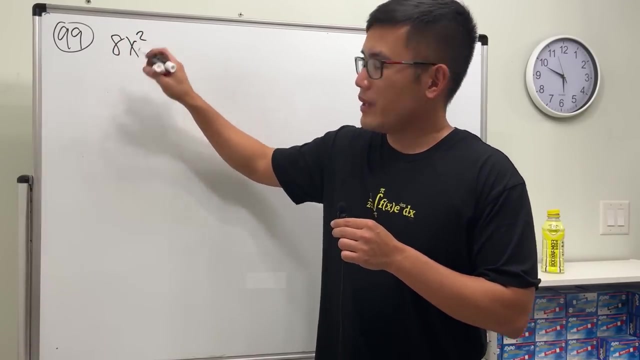 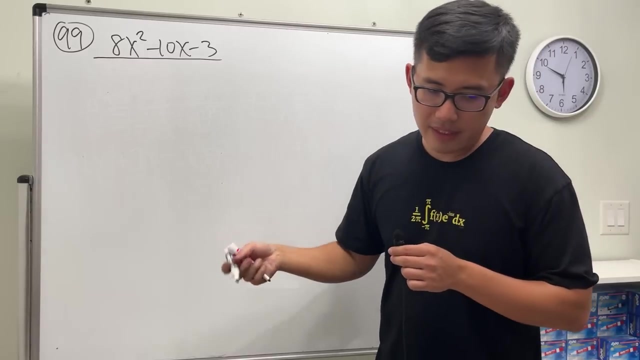 by six. Two more questions, two more questions. Wow, number 99.. Okay, five hours, Number 99,. we have 8x squared minus 10x minus 3 over. we have x minus 4 times x squared plus. 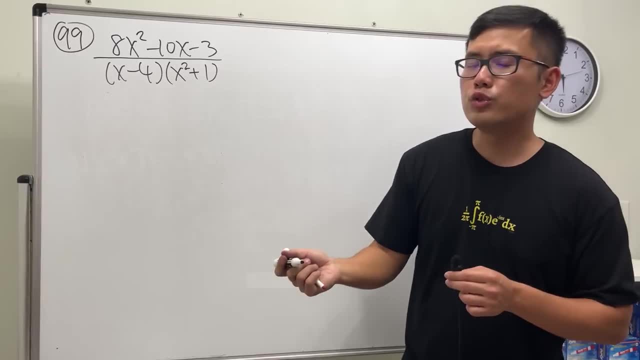 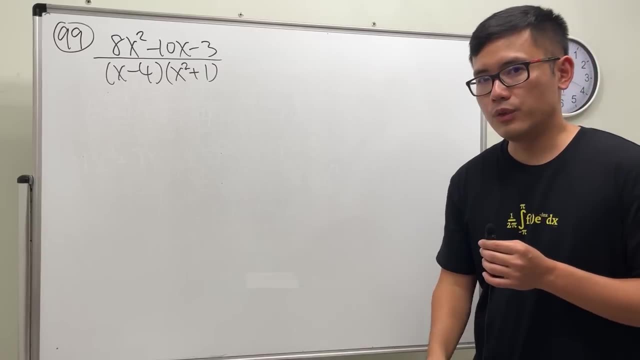 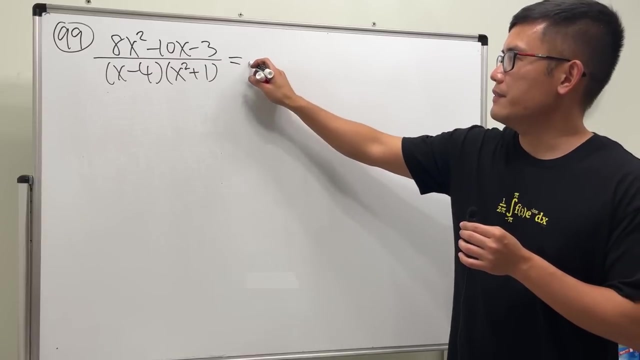 One. Notice this right here: it's an irreducible quadratic with real numbers, right? We cannot factor x squared plus one with zero numbers. It's factorable if you do plus i, minus i, but let's not do that. Anyway, this is linear. so we will have x minus 4 and then some number. 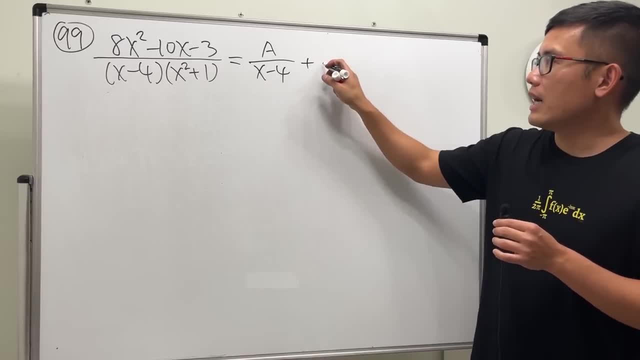 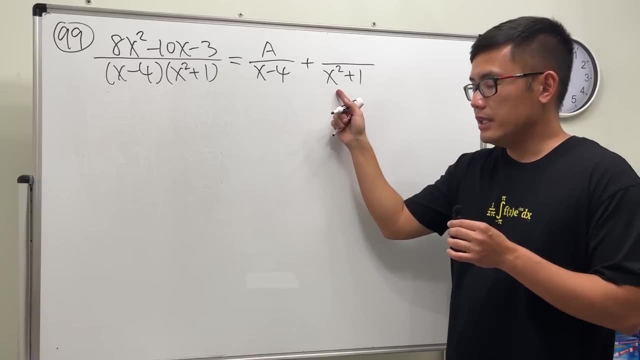 a on the top. And then for this right here, we will just have this right here: x squared plus one, but the top is a quadratic, it's a linear. This is an irreducible quadratic, so the top will be a linear. So we have bx plus c. 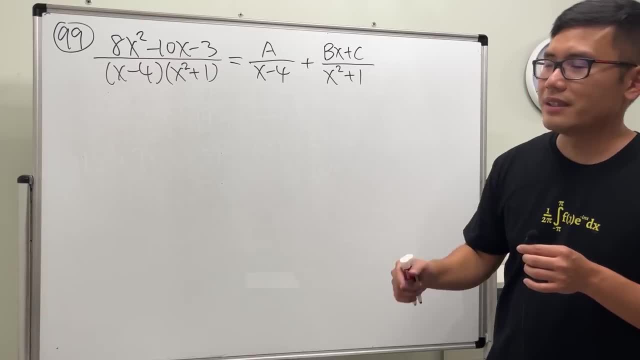 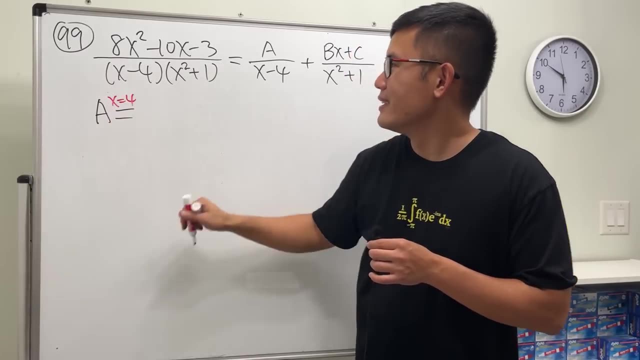 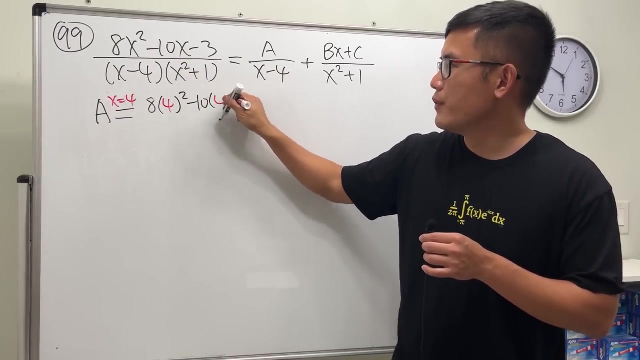 Now we can only do cover up for one letter, which is a, so let's just take advantage of that. x has to be four. yeah, So we are looking at eight times four, squared minus 10 times four, and then minus three over. put four in here, so we have four. 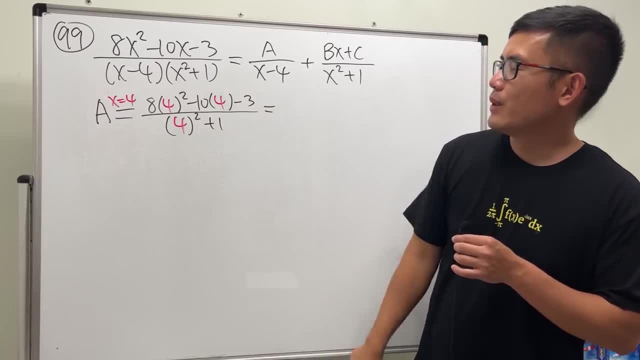 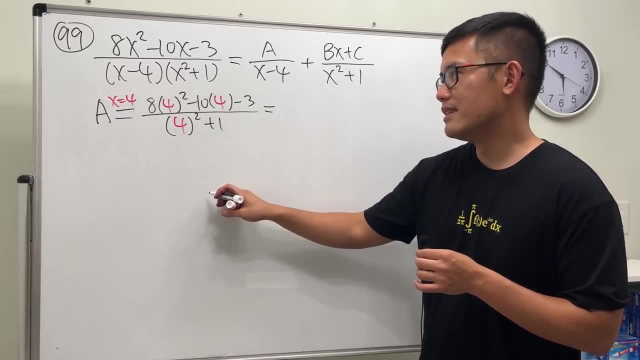 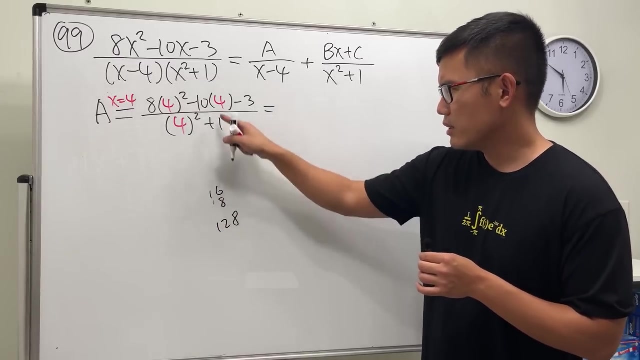 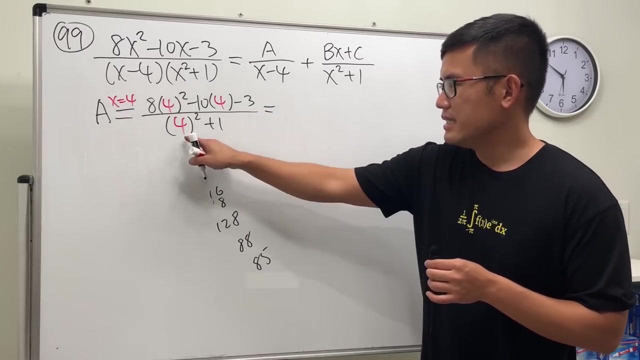 Four squared plus one, Wow, This is 16, times eight, 128.. Yeah, and then minus 40,, so it's uh 88. And then minus three is 85. This is 17. So we give five. 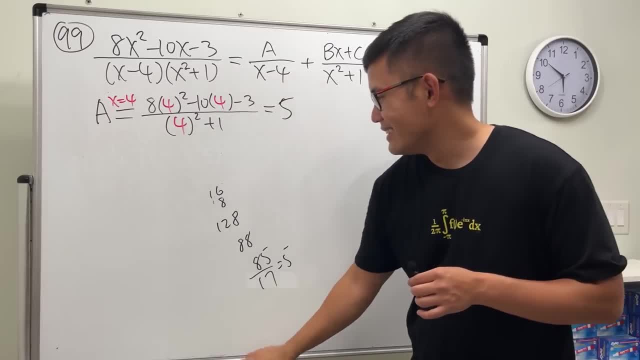 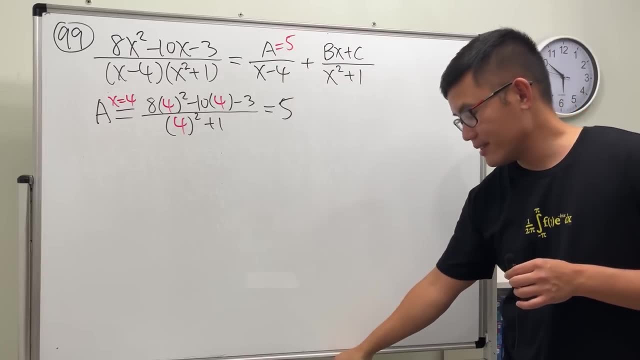 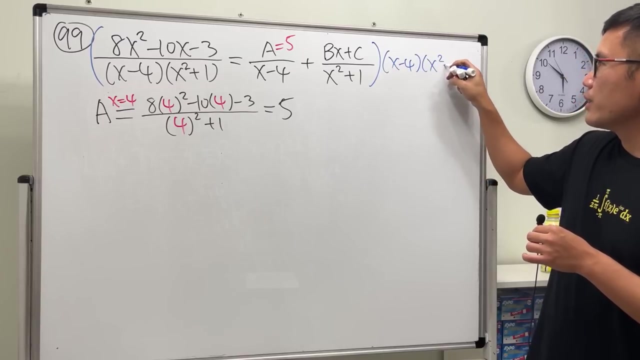 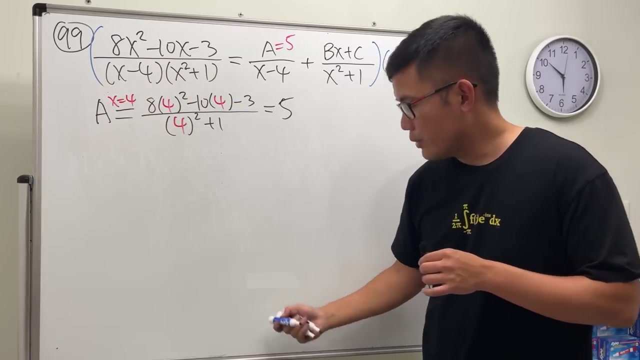 All right, So this right here it's equal to 5. all right, B and C, traditional way. let's just go ahead, do it: X minus 4, X squared plus 1, so take this times that we will have. well, blue arrow, so we have. 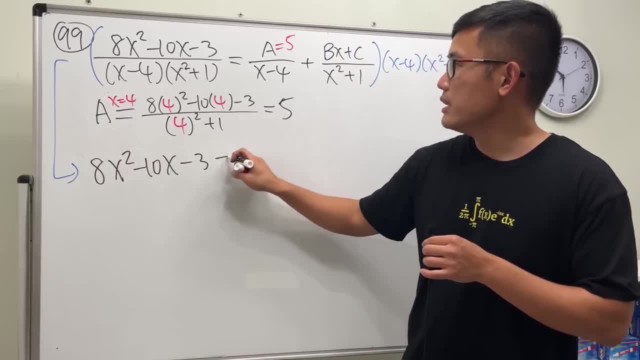 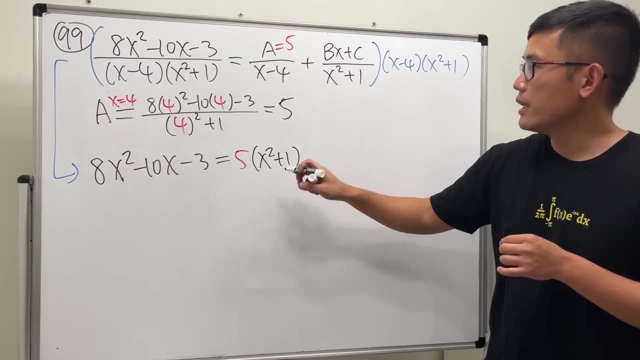 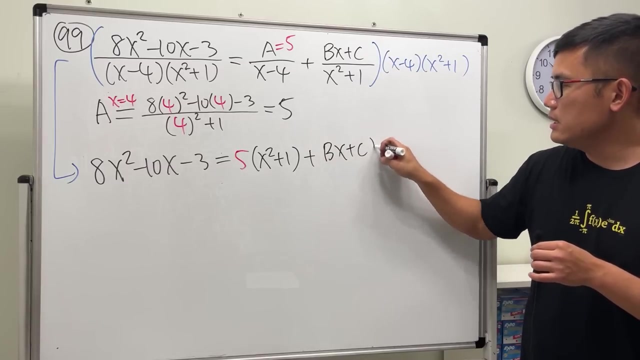 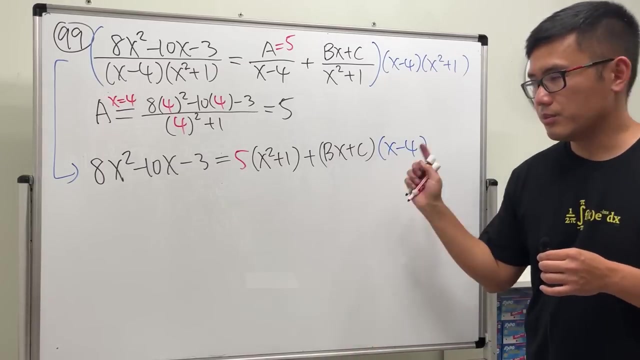 8x squared minus 10x minus 3, this is equal to 5. this and that cancel. but we have that x squared plus 1 and the next we will have this and that cancel. so this times that. so plus B, X plus C, with X minus 4, yeah, and then just multiply so. 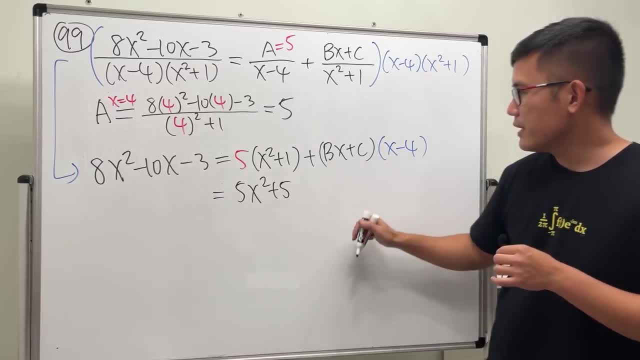 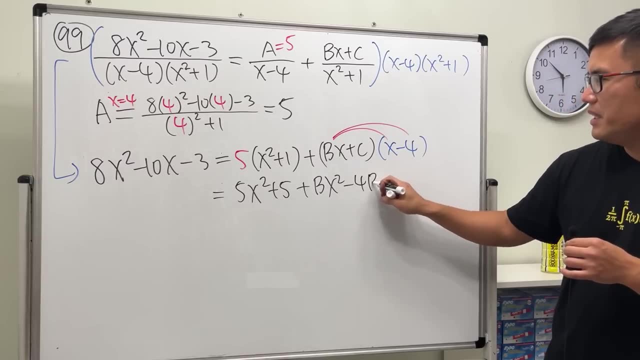 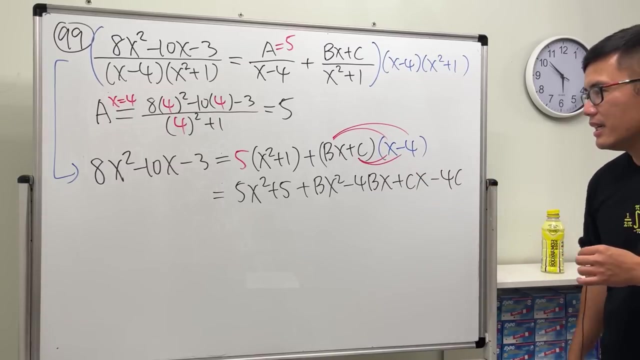 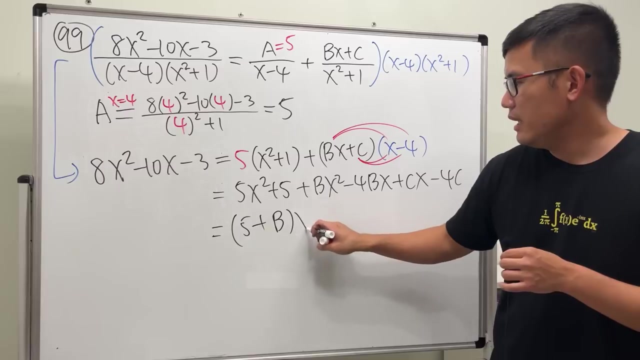 this right. here is 5x squared plus 5. this times, this is plus B, X squared. this times, this is minus 4 B, X, and then plus C, X, and then, lastly, minus 4, C. now let's look at 5 plus B. right, that's the x squared term. 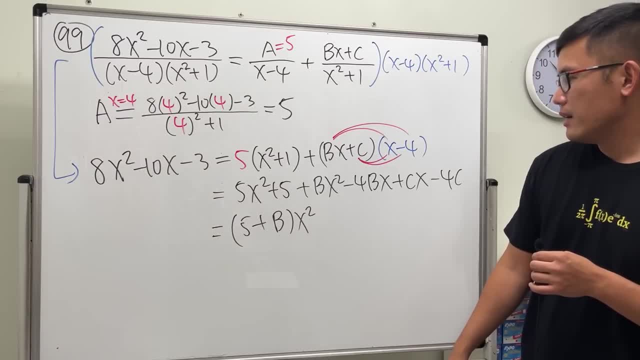 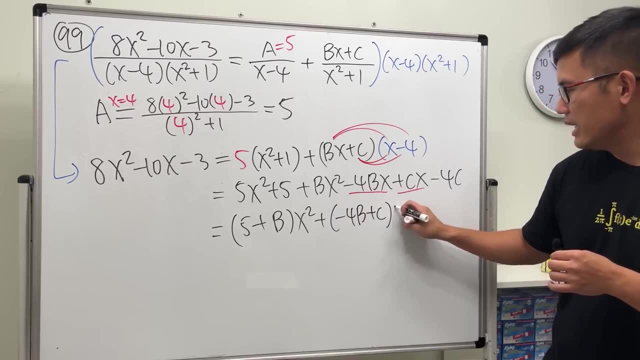 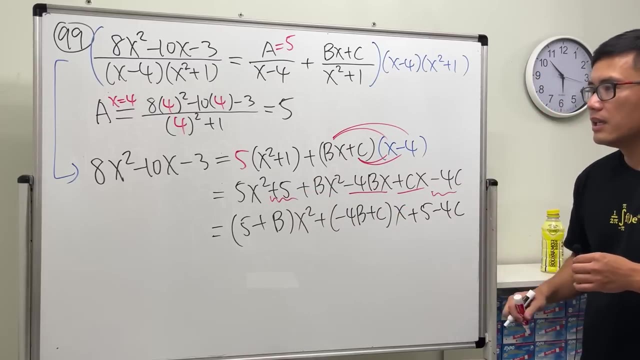 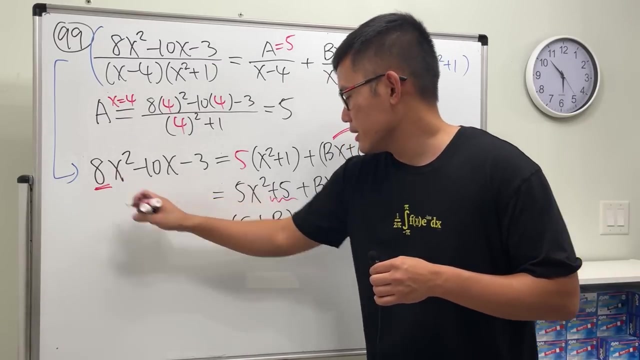 and then let's do this, this, and that is plus negative, 4, B plus C, X, and lastly we have the 5 minus 4 C. so plus 5 minus 4 C. all right, this right here: 5 plus B, X, squared it must be equal to 8. so B has to be 5. 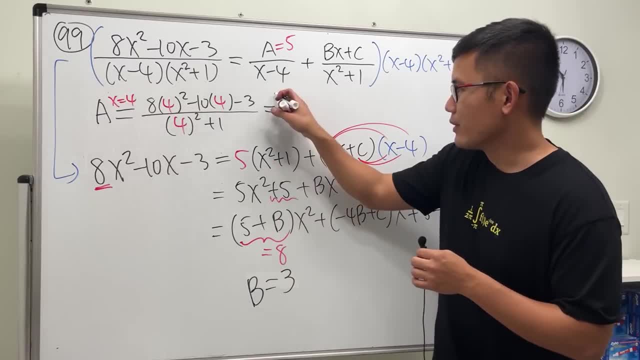 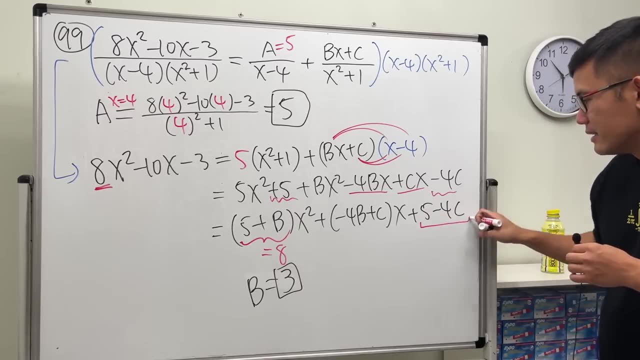 plus 3 is 8, so B has to be 3. yay, so A is 5, B is 3. and then let's just this right here: this has to be the same as negative 3, so negative 4. C has to be equal to move this to the other side, so negative 8, so C has to be. 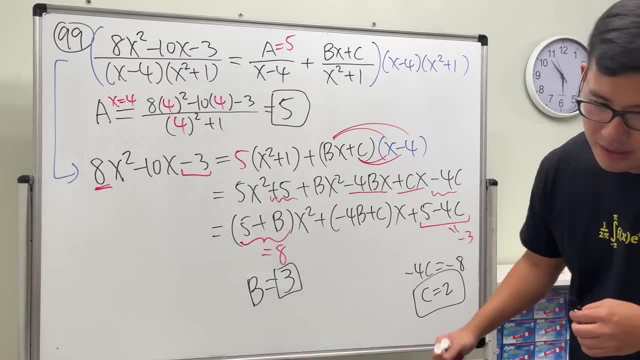 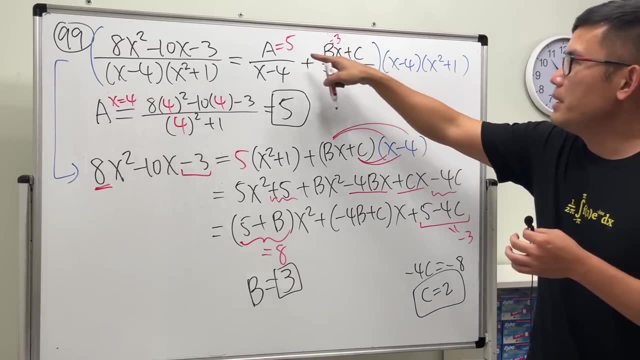 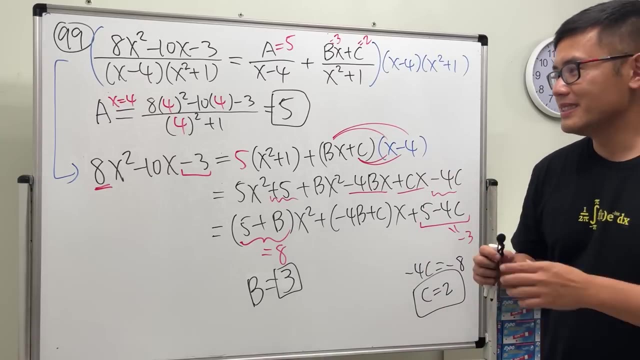 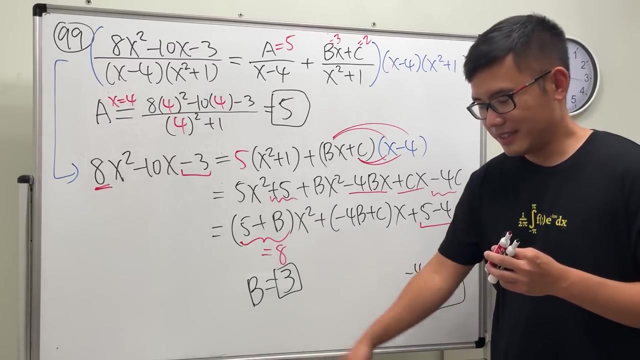 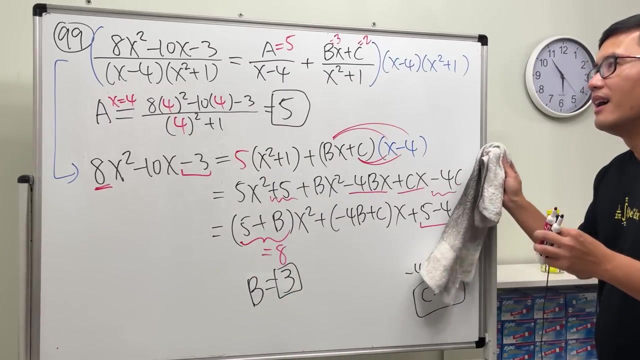 2. yay, so this time we see that B is 5, C is 3 and then. so B is 5, B is 3 and then CS2. yeah, they are all different numbers. it's not like opposite of each other or not, but 99, take a look. okay, ladies and gentlemen. question number 100. 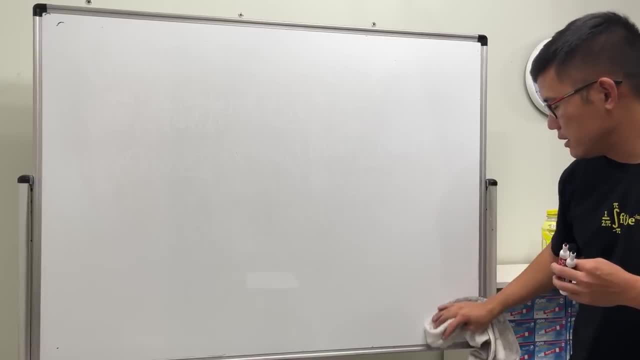 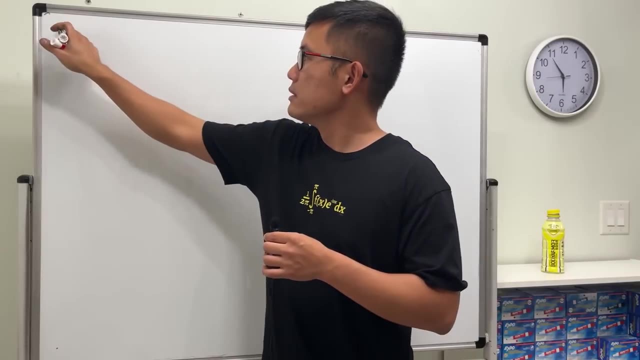 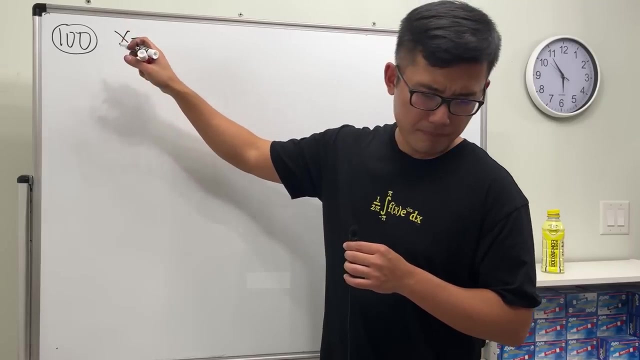 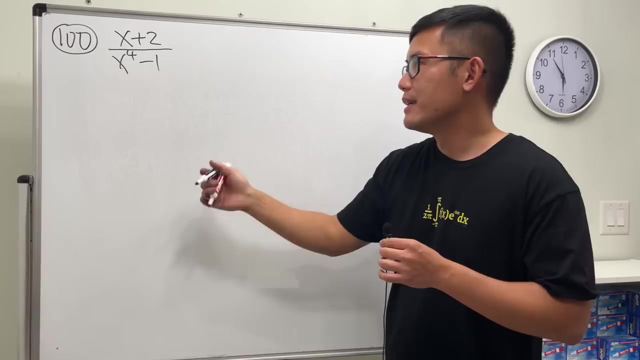 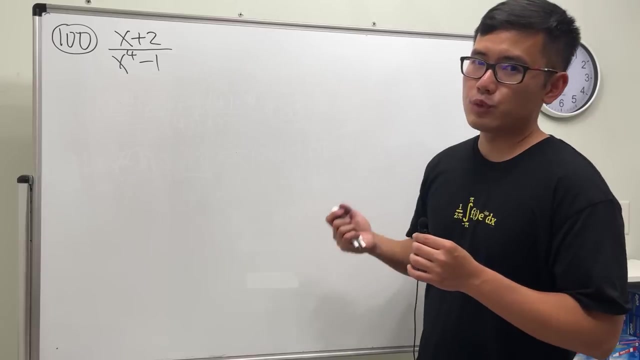 question number 100. here we have X plus 2 over X to the fourth power, minus 1, and then if we factor this, we can x squared minus 1 times x squared plus 1. right, but x squared minus 1 can be factored here again. so if you look at: 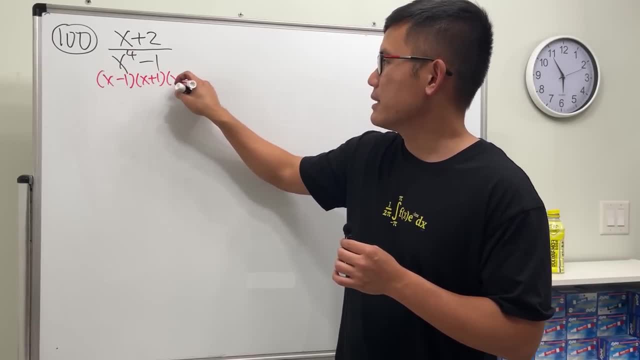 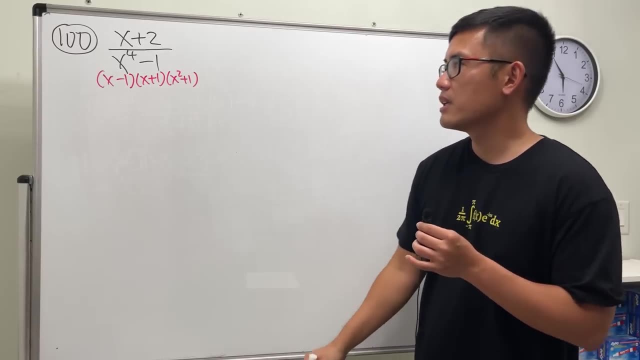 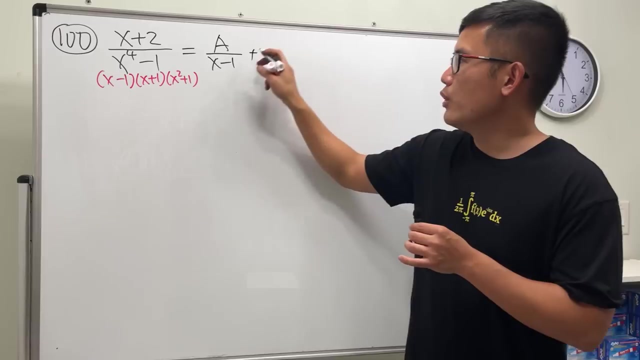 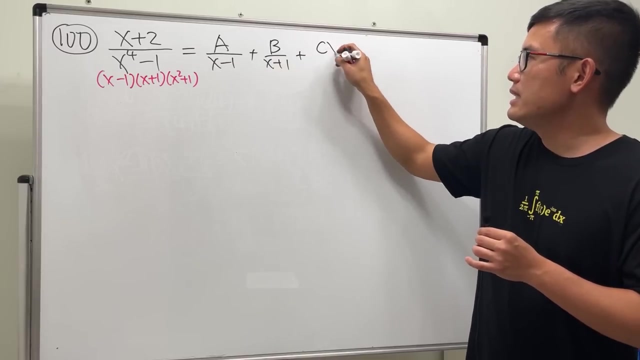 this: it's actually x minus 1 times x plus 1 times x squared plus 1, so we have three factors and the last one is an irreducible quadratic. so the setup is some number a over this denominator and then some number B over that denominator and then a linear term over this denominator, so C, X plus D over. 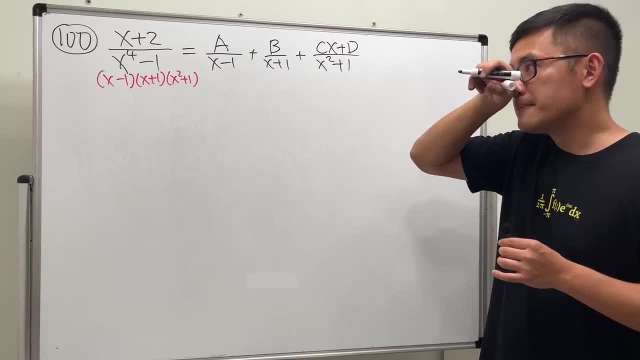 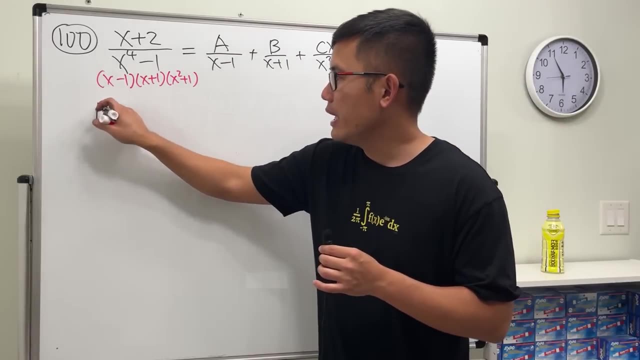 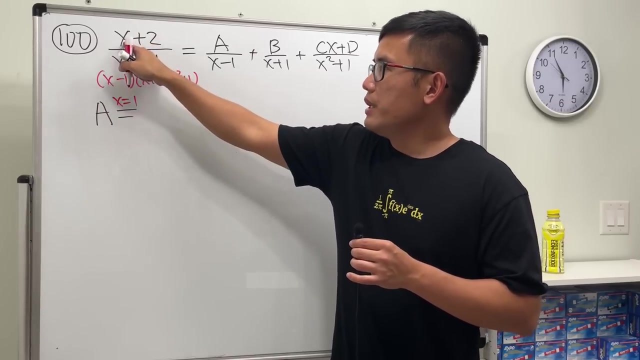 x squared plus 1. yeah, all right. good news: car for a, car for B. get to work for that, right. so a equals same denominator. cover this up. X has to be 1, put it here, put it here, put here, so we have 1 plus 2. 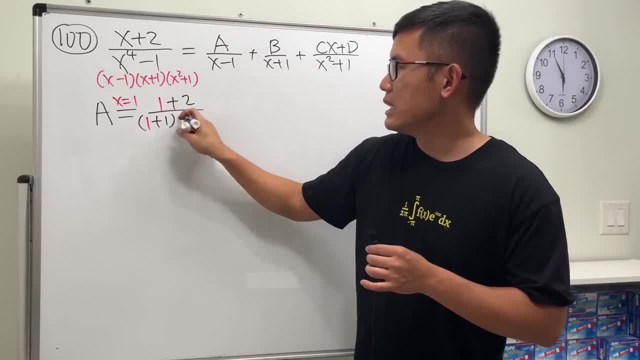 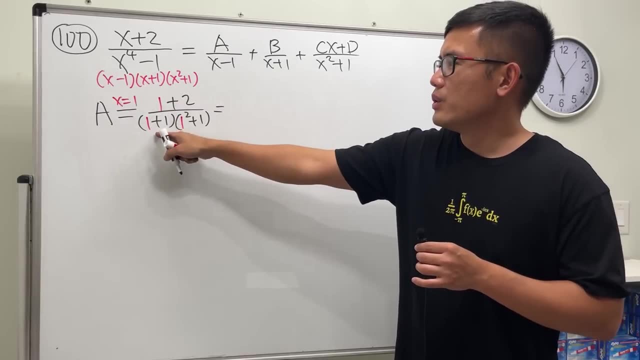 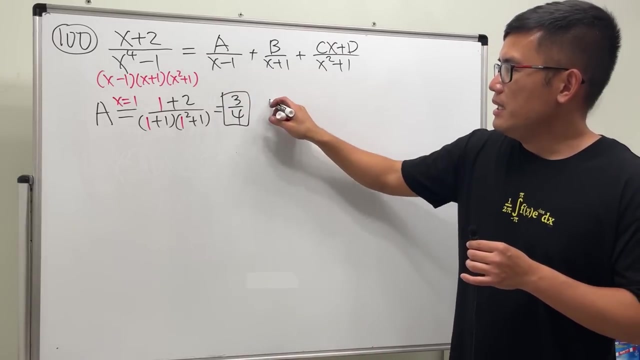 over 1 plus 1. 1 square plus 1, Okay, so that's 3.. 2 times 2 is 4, so it's 3 over 4.. That's A, And then B equals x has to be negative 1.. 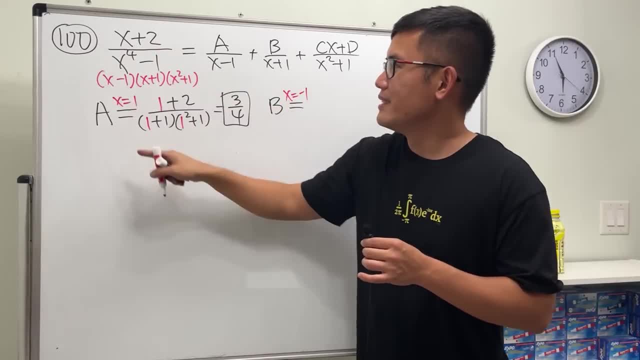 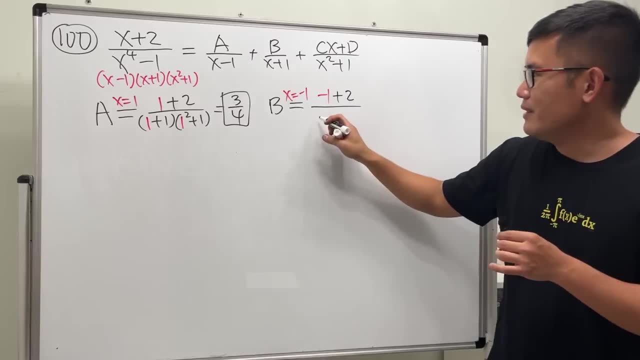 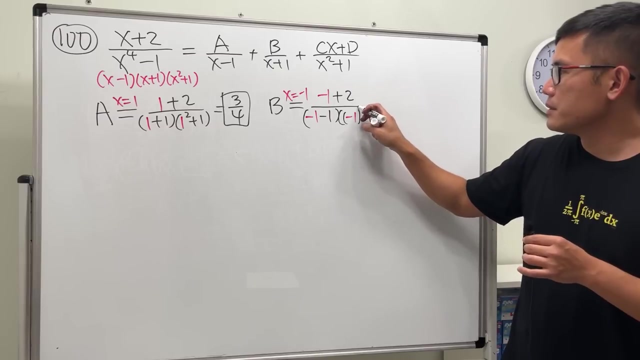 So x equals negative 1.. Put it here, Put it here, put it here. So we have negative 1 plus 2 over negative 1 here, minus 1 times negative 1 squared plus 1.. Okay, so on the top is 1 over. this is negative 2,. 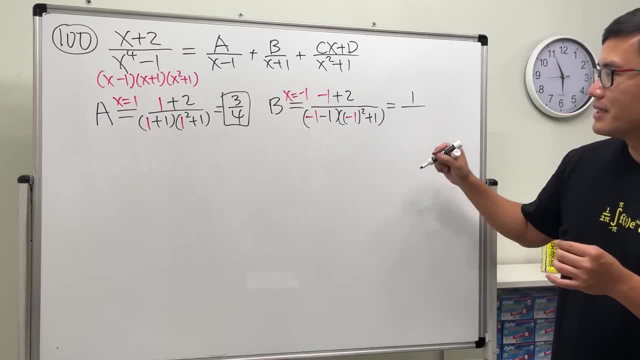 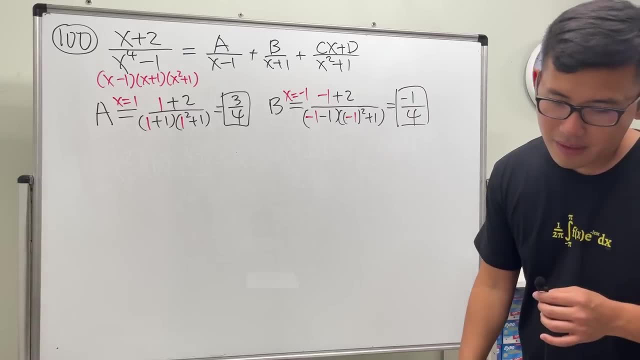 times 2.. So it's 4 by negative. So B is equal to negative 1 over 4.. Yay, I got it right. Okay, and now the moment that we have been waiting for: right C and D. 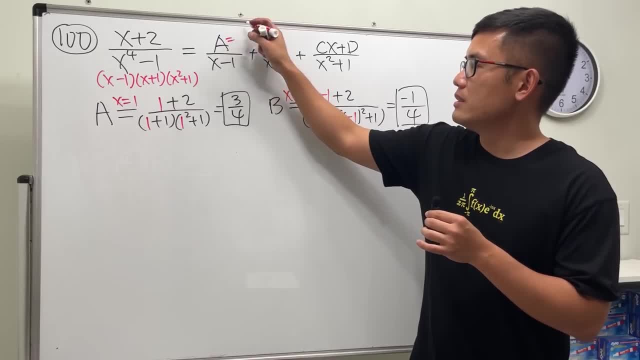 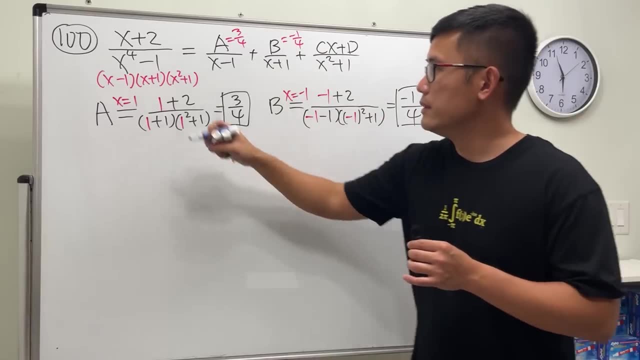 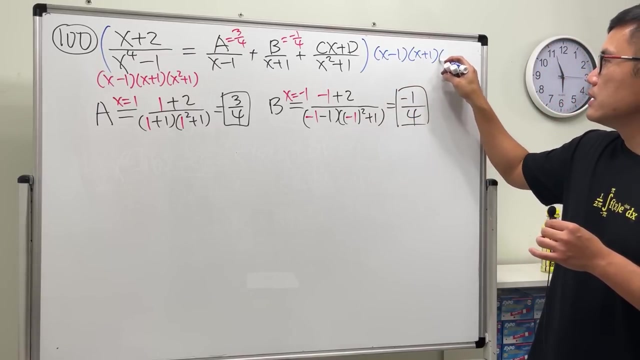 Yes, we have to just do the traditional way. huh, So this is 3 over 4, and B is equal to negative 1 over 4.. All right, So x minus 1, x plus 1,, x squared plus 1.. 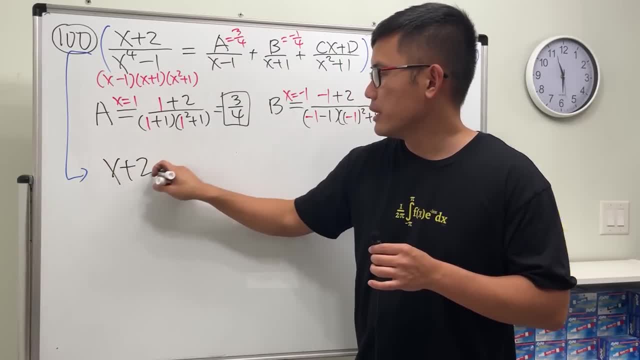 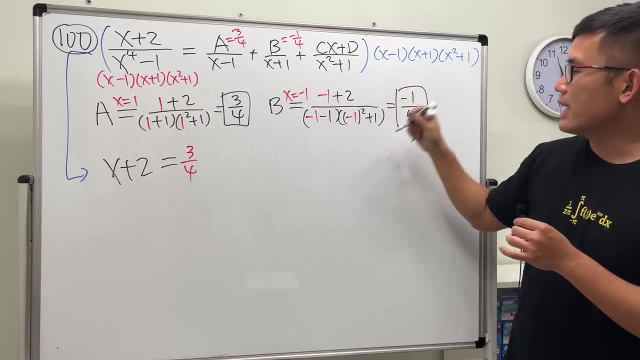 All right, so here we have x squared plus 1.. All right, so here we have x squared plus 1. And this is equal to: here we have 3 over 4.. This and that cancel. so we have this and that. 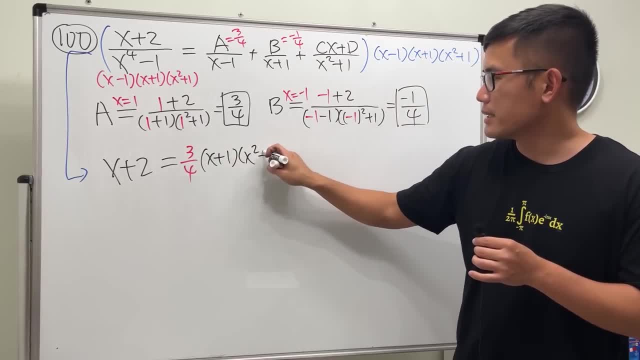 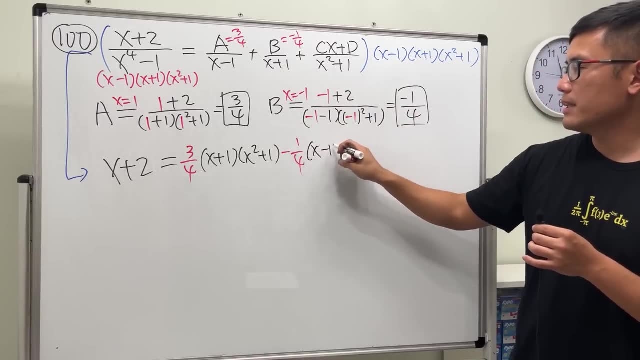 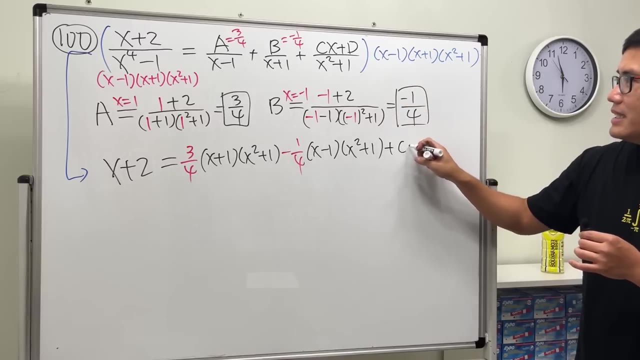 So it's x plus 1 times x squared plus 1.. Next we have B, which is negative, 1 over 4.. This and that cancel. so we have x minus 1, x squared plus 1.. And lastly, this and that cancel, we have plus Cx plus D. 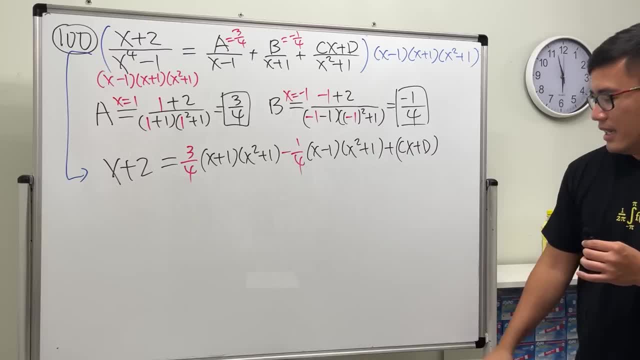 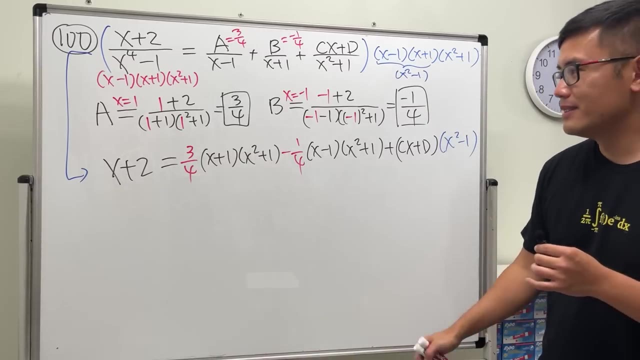 times this two together is x squared minus 1.. So I'll just multiply by x squared minus 1.. Huh, Okay, Just do the algebra right. Okay? So let's multiply this and then distribute the 3 over 4.. 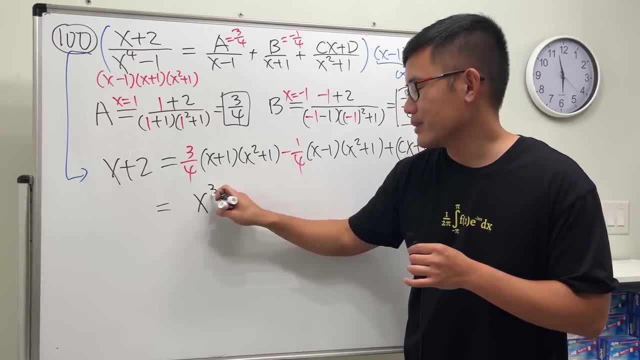 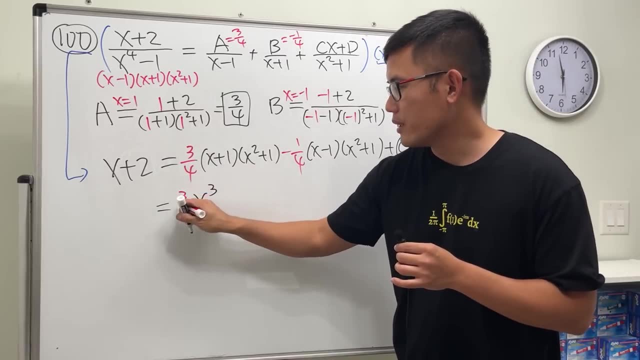 So here we get x to the. oh, this is hard. Let's see This times that is x plus 3 power. Okay, but multiply by 3 over 4. next, I'll take this times that, which is just X, but then. 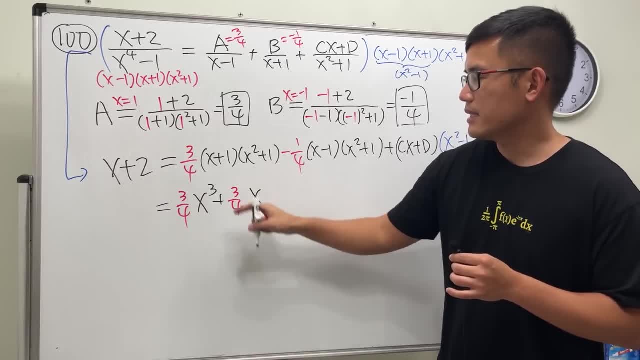 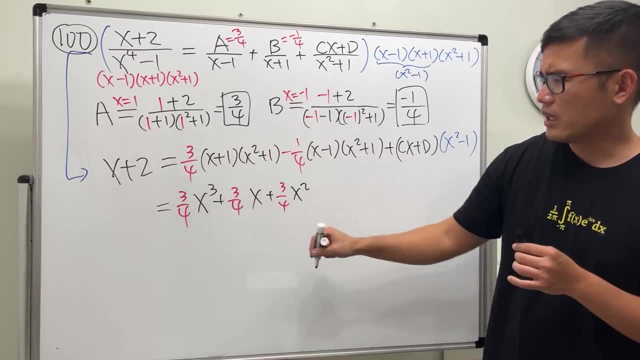 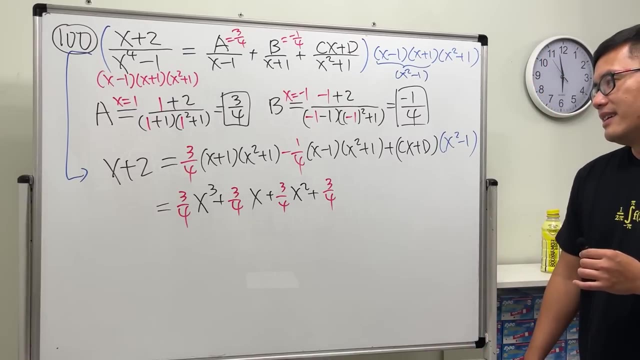 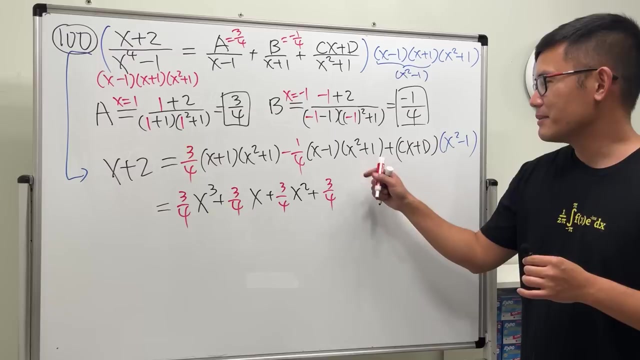 I will multiply by 3 over 4. next, I'll do this times that which is plus X square, but I will multiply by 3 over 4. and lastly, 1 times 1, I will have that 3 over 4. okay, all right, let's do this. so this times, this is X to the third power. 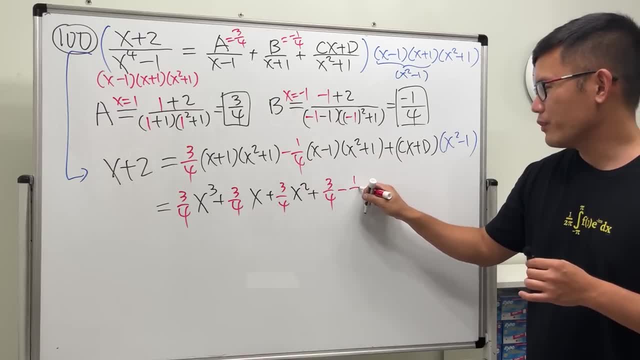 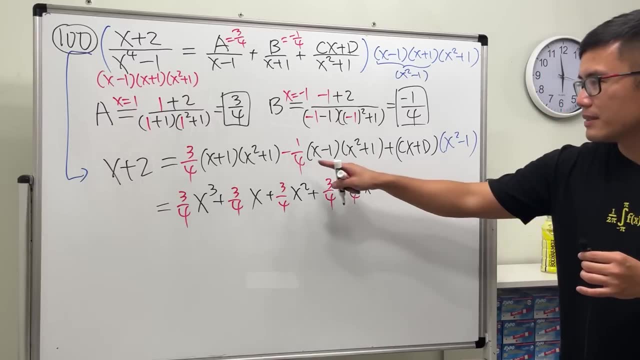 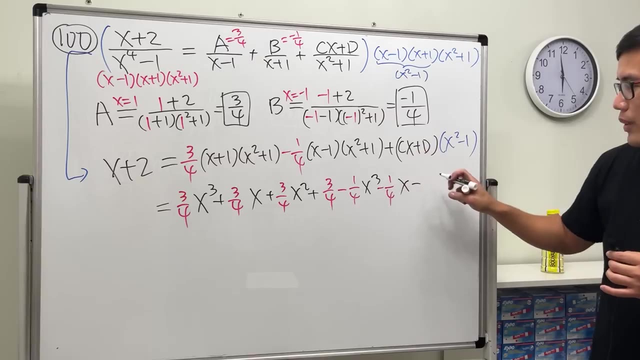 distribute the negative, so we have minus 1 over 4. X to the third power: this times this is X, but multiply by negative: 1 over 4. and then, this times, this is negative X square, but multiply by this, which becomes positive 1 over 4. and lastly, this is negative but multiply by. 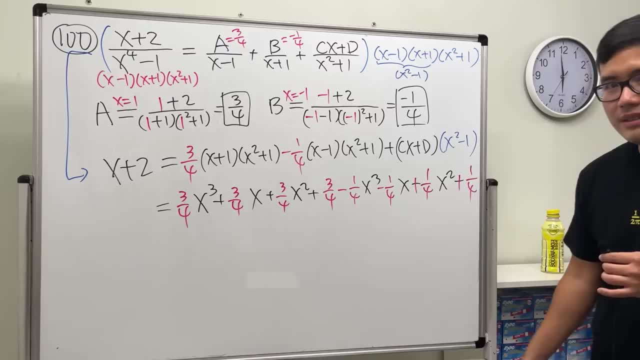 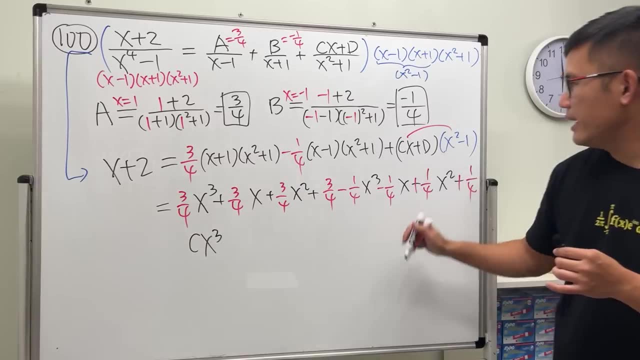 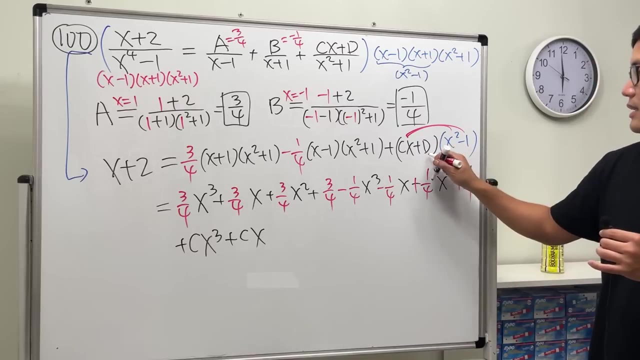 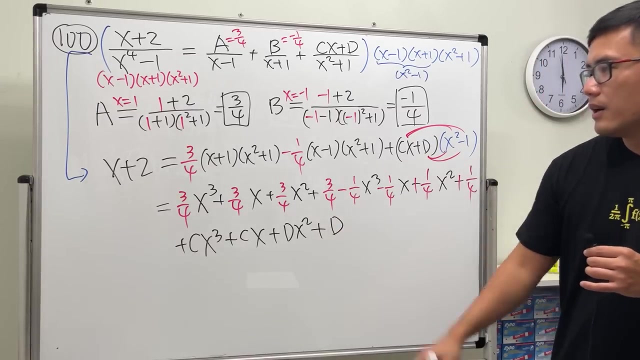 that becomes positive, 1 over 4. okay, and then multiply this out, so CX to the third power. then this times this is CX and then DX square, lastly D. all right, let's see that, see that. see, show me the X to a third power. okay, what this, this and that okay. 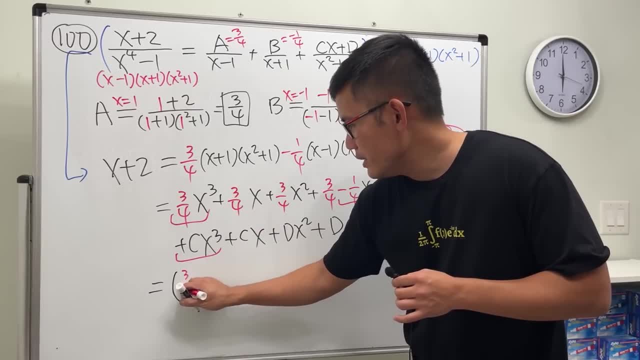 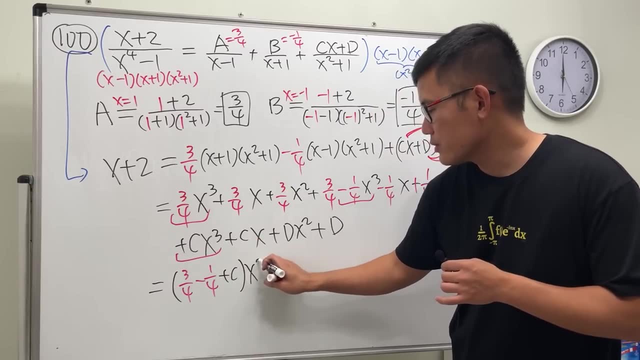 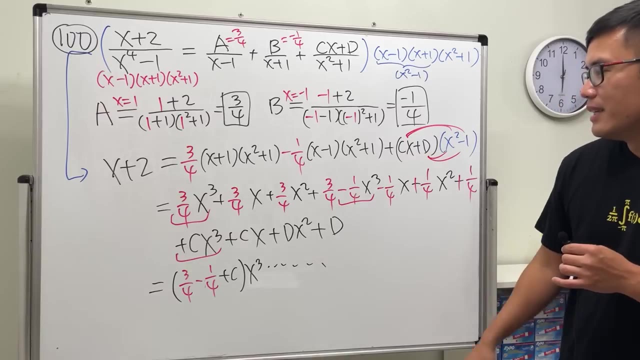 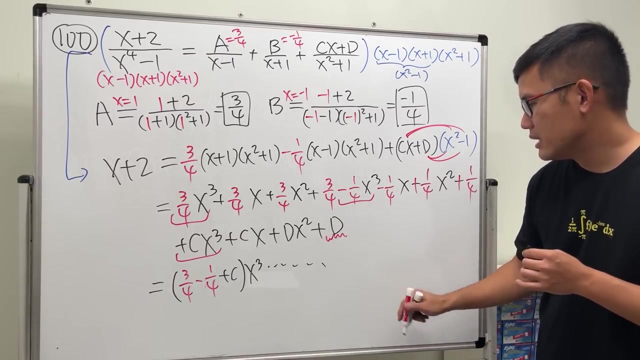 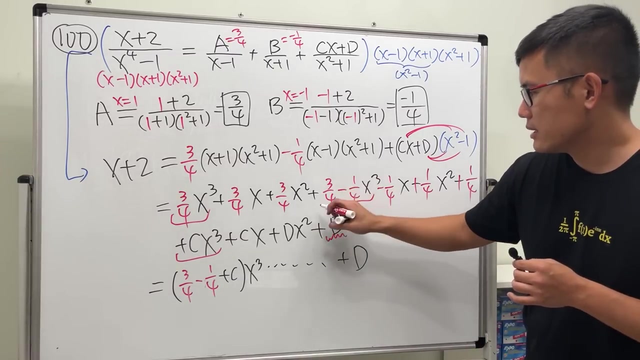 so we see that we have three over 4, minus 1 over 4, and then plus C, extra third power. so thanks to this we can figure out what C is and then, because we can use a unit, we can use the last number. we have D, right, it has no X, and then this has no X, plus 3 over 4, and 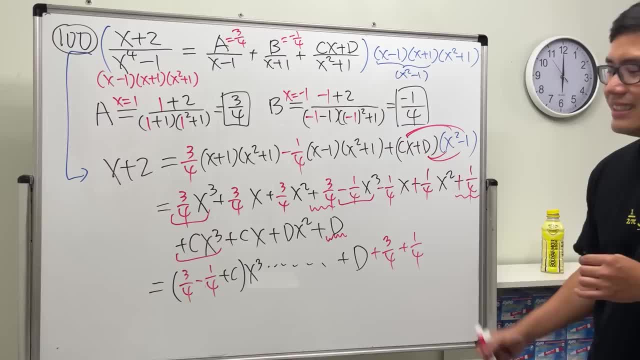 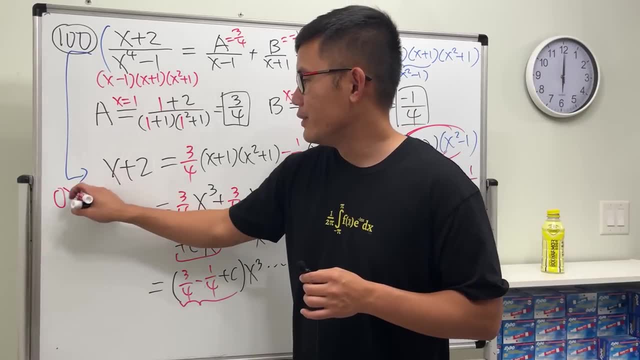 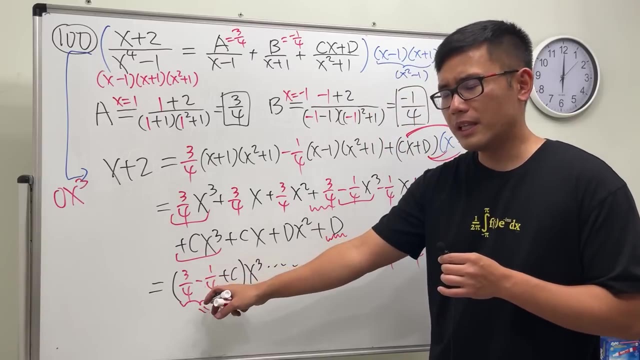 plus 1 over 4. yes, no X. alright, so let's figure out what this is. this is X to third power term, and here we have no X plus third power. so this right here should be equal to 0. so this and that 3 over 4 minus 1 over 4, 2 over 4, which is 1 half plus C, equals 0 C. 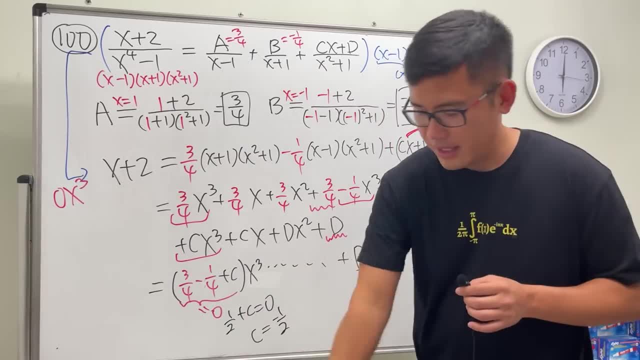 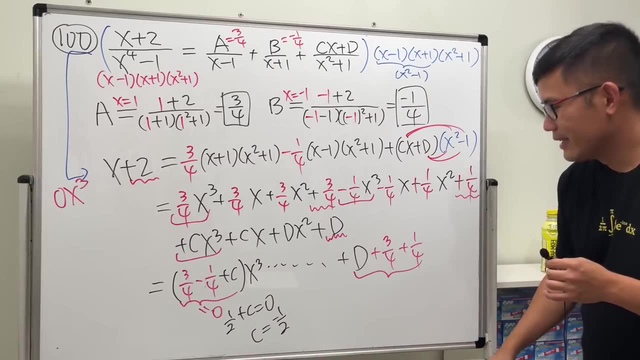 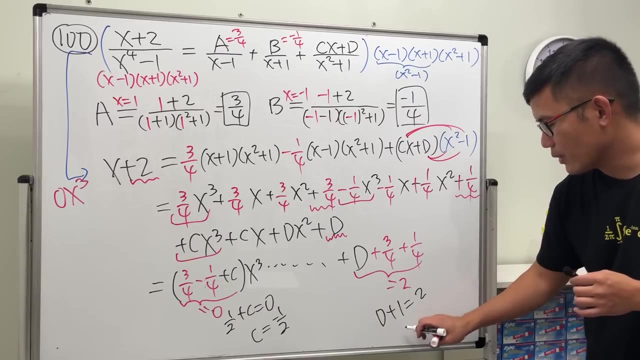 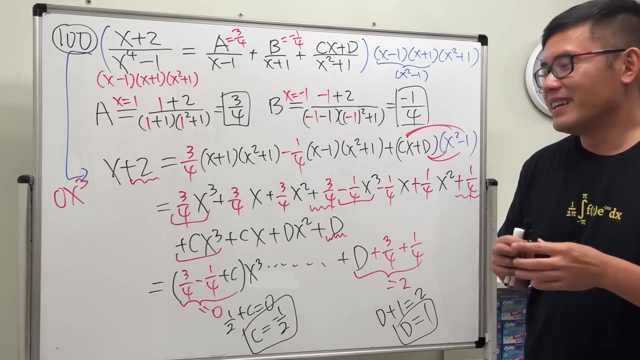 equals negative 1 half. yay, and then this right here, it's this term, yeah, so it should be equal to 2 and that's 1. so D plus 1 equals 2, so D equals 1, C is negative 1 half and D is equal to 1. done 100 questions, just algebra, yeah. 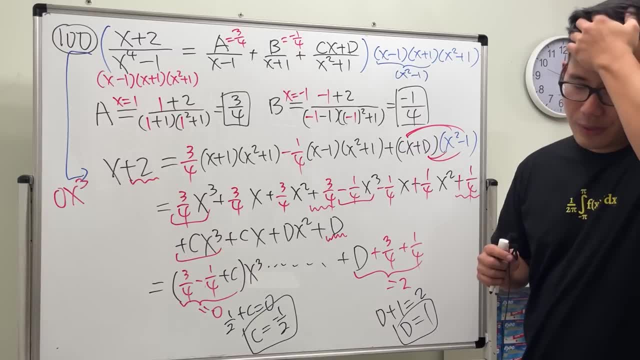 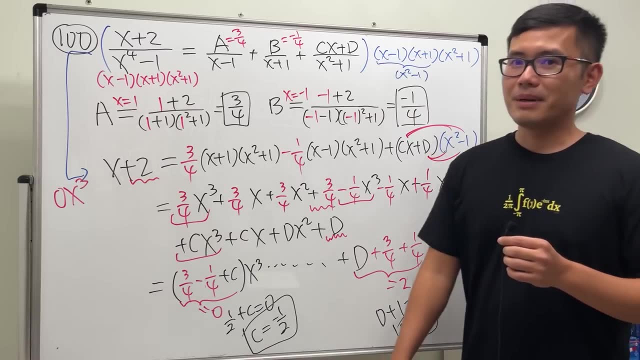 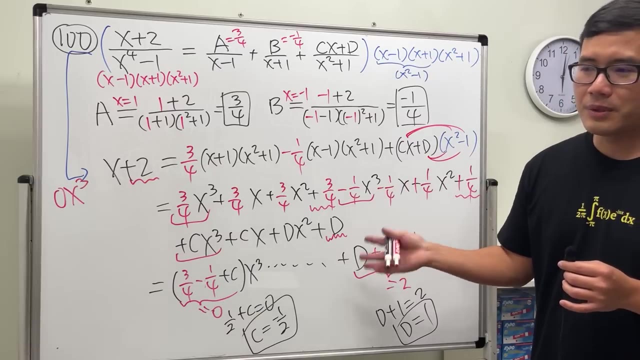 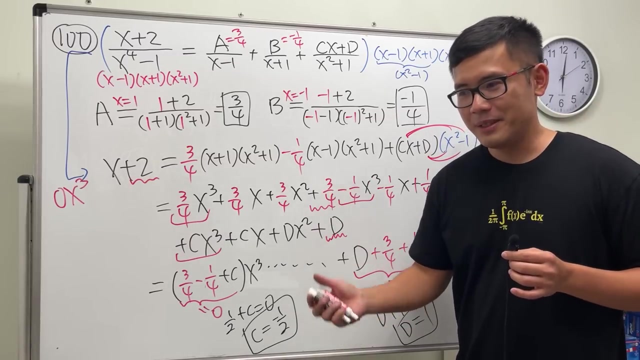 what the algebra, what I cannot say all algebra that you're seeing, calculus, because there are a lot more seriously. yeah, but it's a matter of you if you want to practice or not, and the better you are with algebra, the more comfortable are. the more comfortable you are with algebra, you will have a better time in. 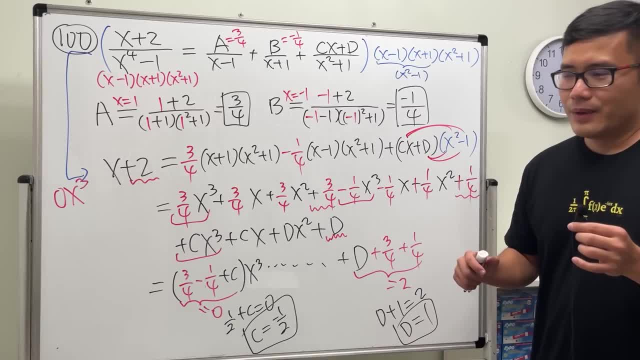 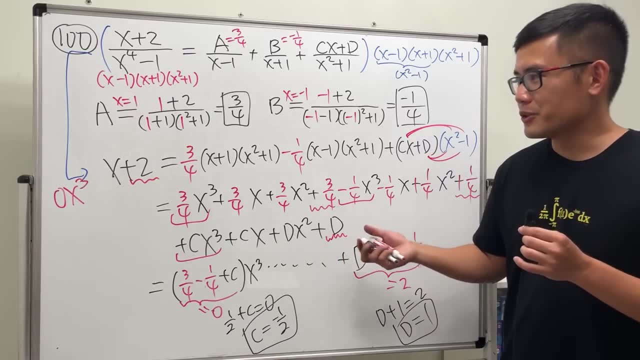 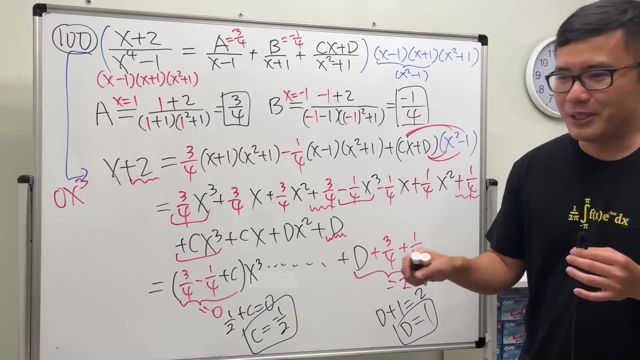 calculus. because, well, first I will tell you, sometimes when you learn calculus, concepts are already but you also struggle with the algebra. that will be impossible. algebra should be your second nature. when you do the computation, okay, and then if you have algebra done, then you can really enjoy your. 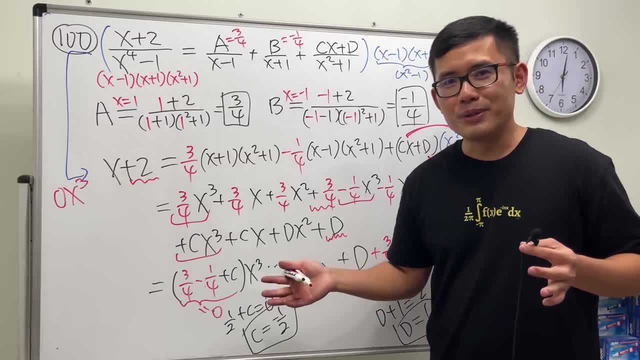 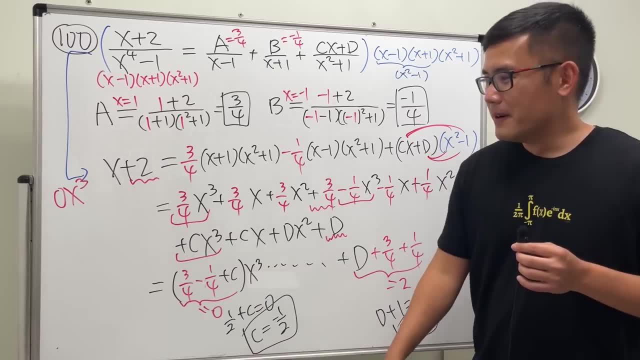 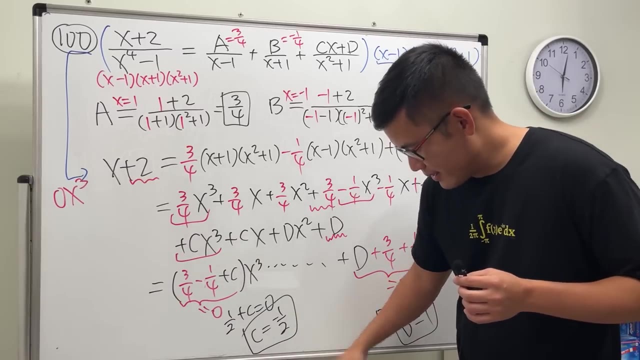 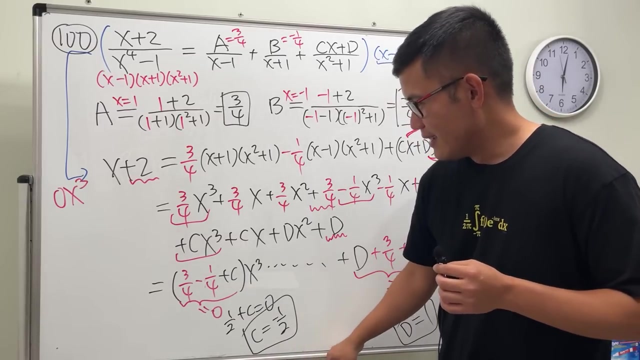 learning calculus and I know what happened to the trick. right, I'm going to come with something else for you guys for trick, but right now, 100 question. I know as a tradition I should do 101, right? so am I going to do 101? yeah, let's. 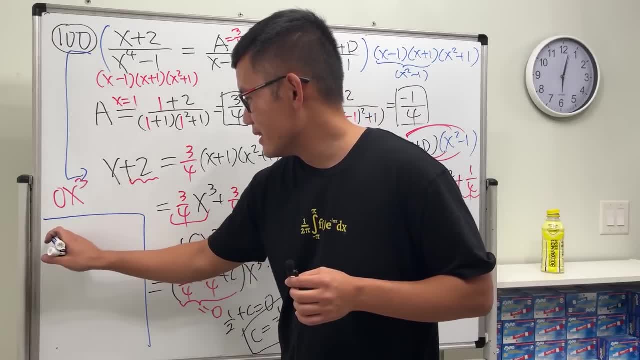 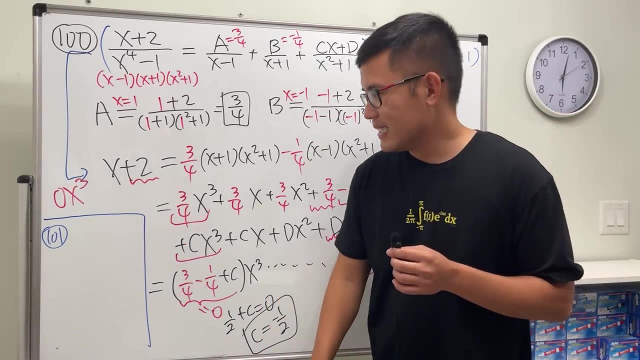 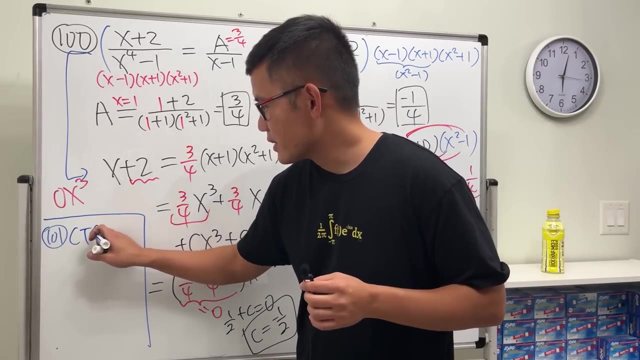 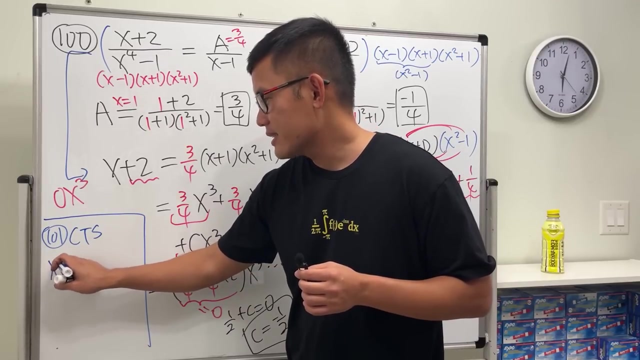 let's do 101. what exactly am I going to do for 101? I really didn't prepare. I definitely didn't prepare. that's, that's complete square. how's that? how would you complete the square CTS? let's just do small example. how would you complete a square for solving this equation? X square no. 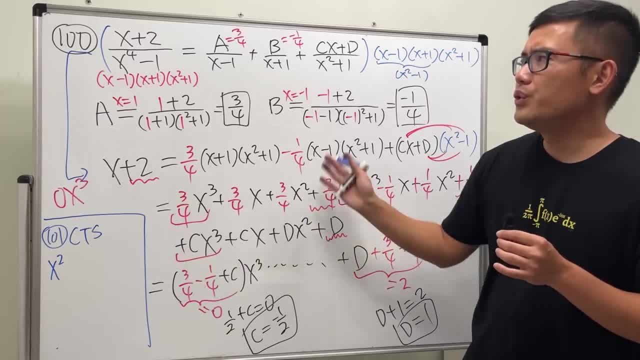 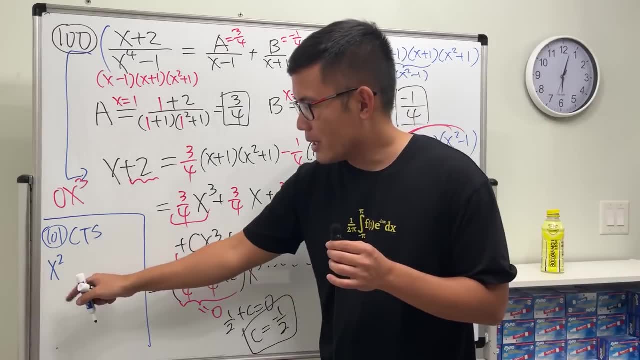 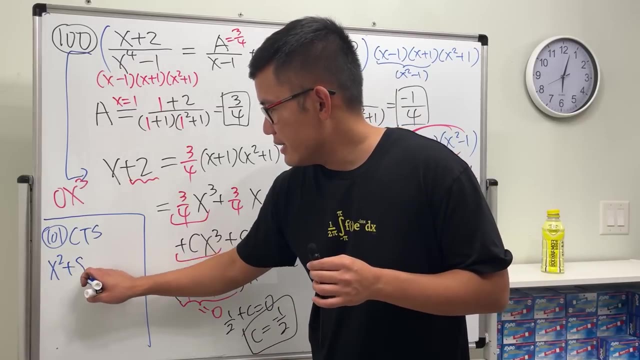 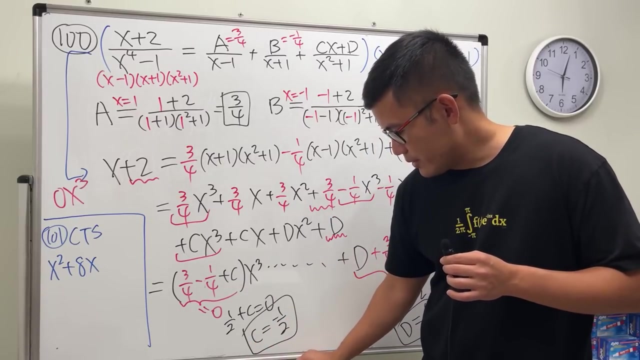 that's just complete a square, because when you do what's that called partial fractions, sometimes you may have to complete a right. how would you complete a square for this X square plus 8x? yeah, well, first I'll tell you. we have to make sure the coefficient of x grace 1 in this one. 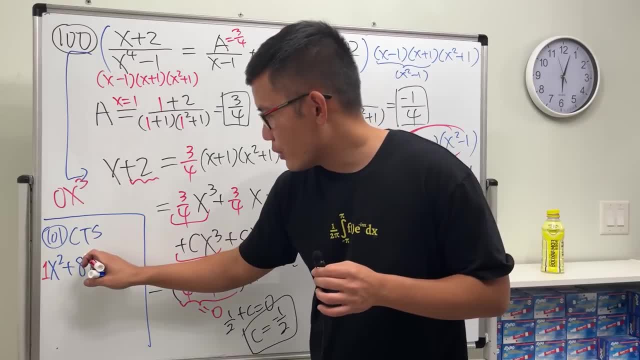 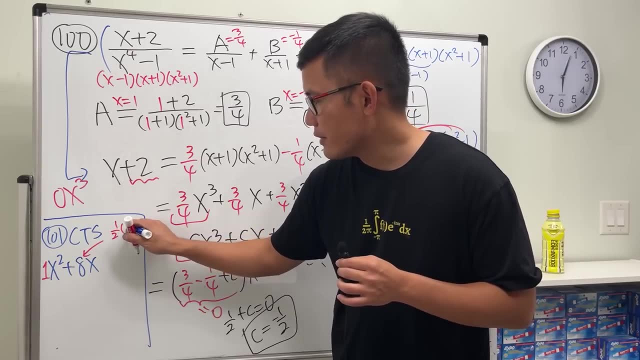 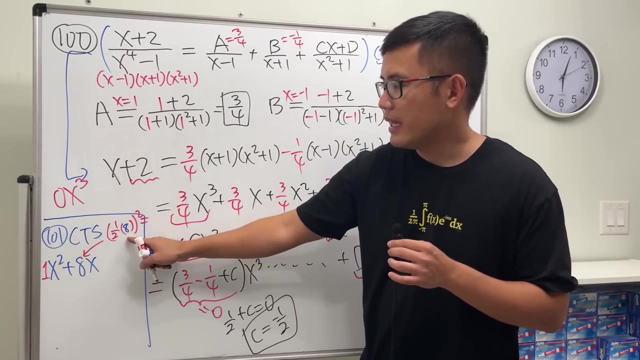 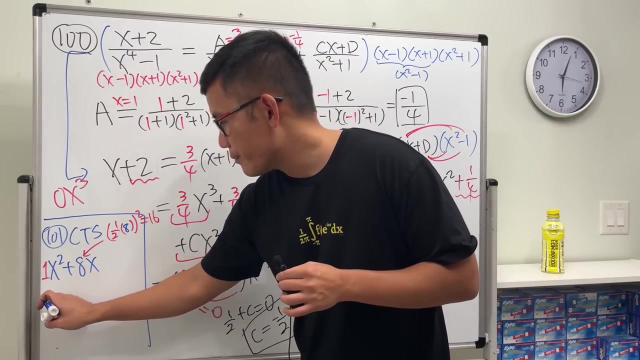 good, then you do the following: look at the coefficient of X, which you will have 8. then what we do is we take half of that which is half of 8, and then we square it. I call this the magic number. half of 8 is 4, 4 squared is 16.. so if we have this this right here, we are going to write it as x. 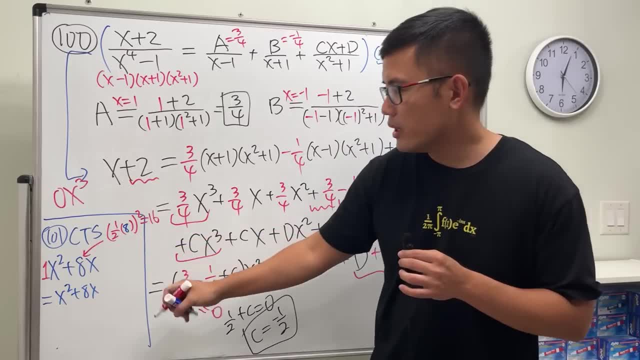 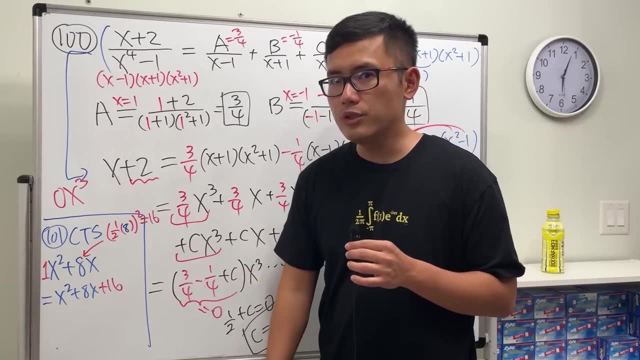 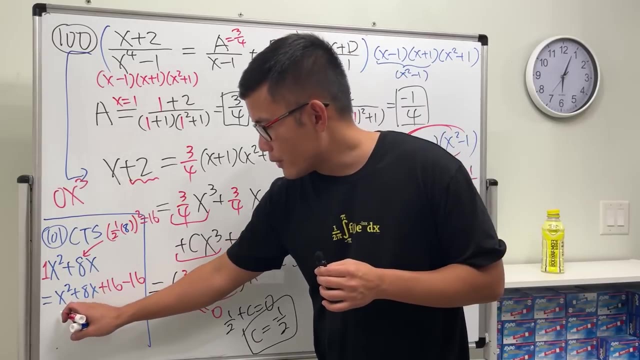 squared plus 8x, and then we can complete the square by adding the 16.. but this isn't going to change the whole thing. this is not the same as the original anymore. right, don't worry, just go to minus 16 after that, and then the magic number is so powerful, so magical, because the first three 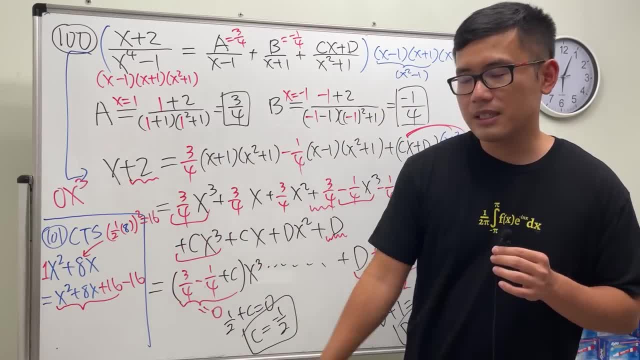 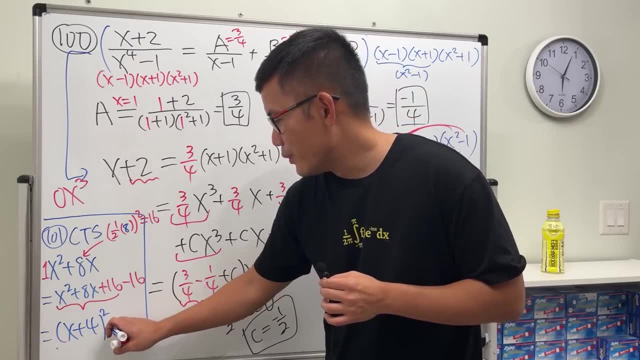 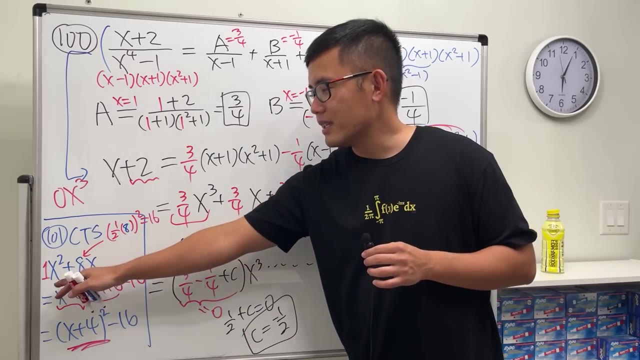 term is the popular square: x plus 4 times x plus 4.. so we get x plus 4 square and then, right here you see that we have that minus 16.. so this, right here, is a perfect square. that's how you complete the square when you have a quadratic term, and we've just focused on this too. yeah, and this is: 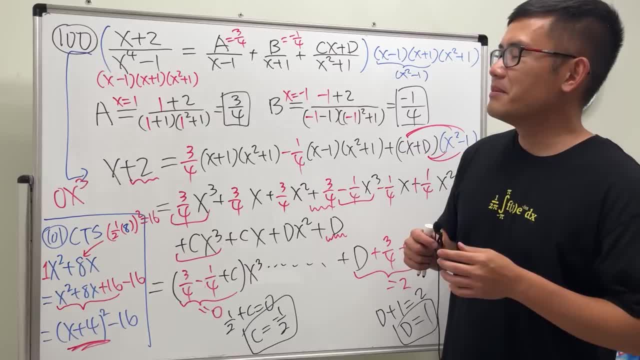 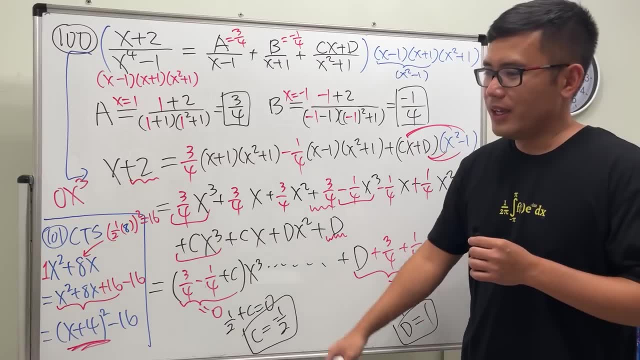 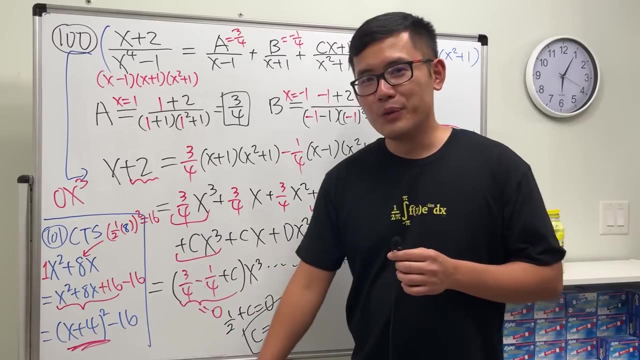 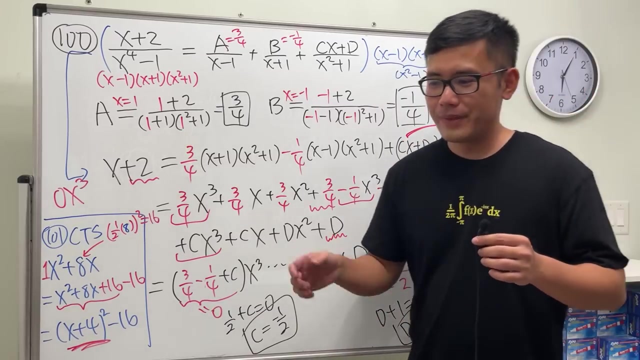 useful when you want to solve, like quadratic equation, or sometimes if you want to do integral width, uh, this kind of weird things. then you complete a square. your life will be happier. there we have it. 101 algebra equation. all right, so hopefully you guys can find this video helpful if you're taking. if you're taking.